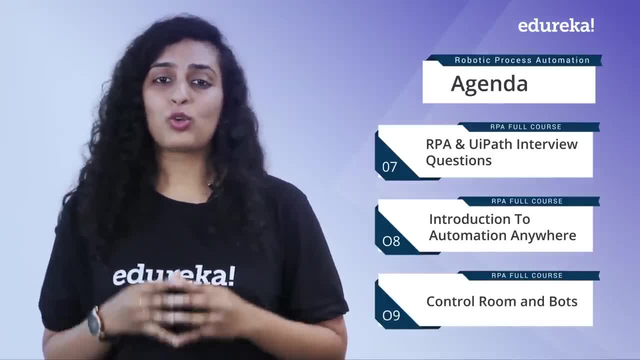 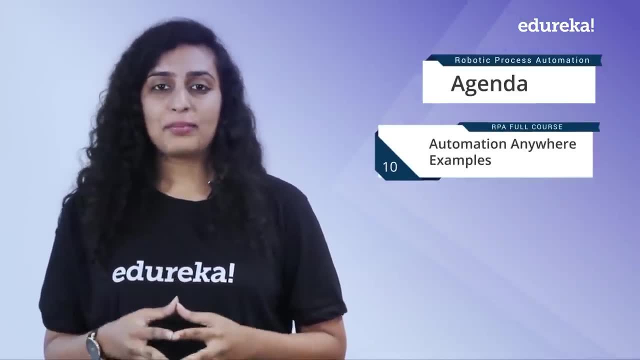 we'll talk about control room and bots, where we'll understand the different control room components and the different bots offered by Automation Anywhere. Once that is done, we'll talk about the different Automation Anywhere examples and then we'll have an interview questions section on Automation Anywhere. 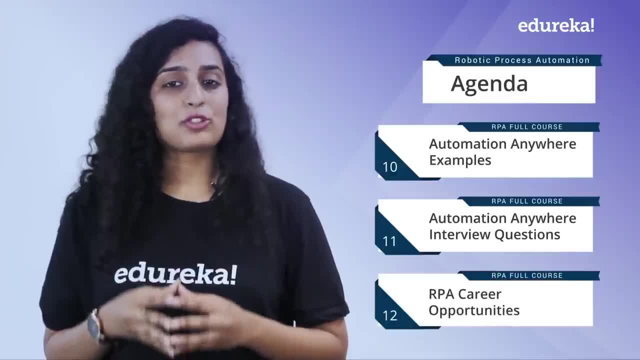 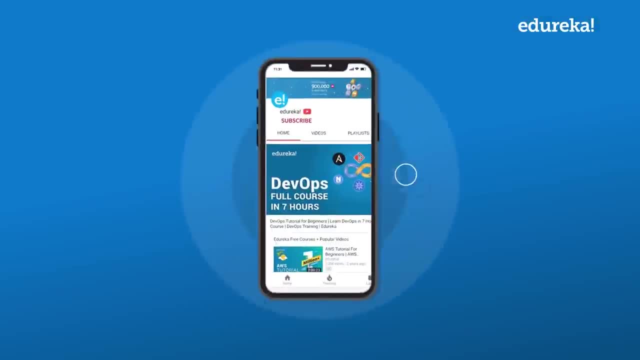 Finally, we'll end our session with a discussion on RPA developer's roles and responsibilities. With this, I've come to an end to my agenda. Now, before we move forward, I would like to request all of you to subscribe to our Edureka. 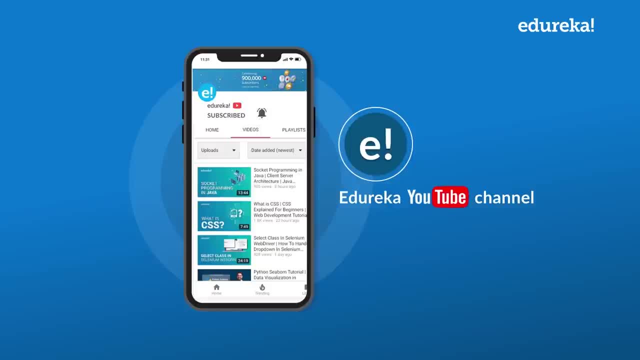 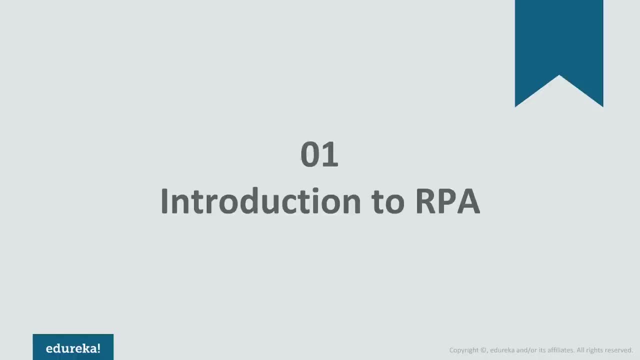 YouTube channel to get daily notified on the top trending technologies. On that note, let's get started. Hey guys, this is Hemant from Edureka. Welcome to this session on what is Robotic Process Automation. Now, as you guys know, RPA is quite a buzzword in the industry right now, and most 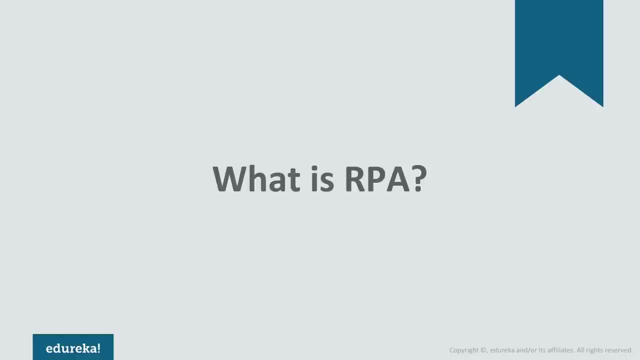 of you must have heard about RPA by now, right? And for those of you who are still new to the topic, guys, don't worry, I'll be discussing all about RPA in this session and by the end of the session, I guarantee you that you'll be able to create your first automation project. 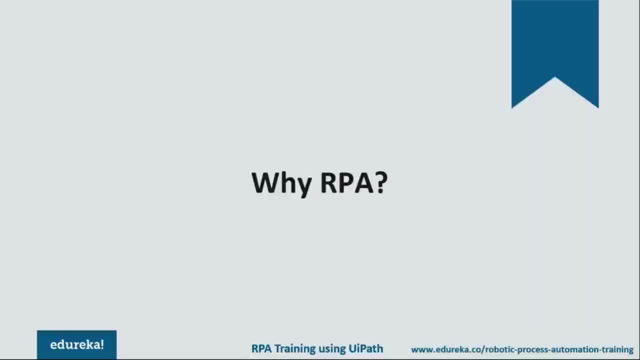 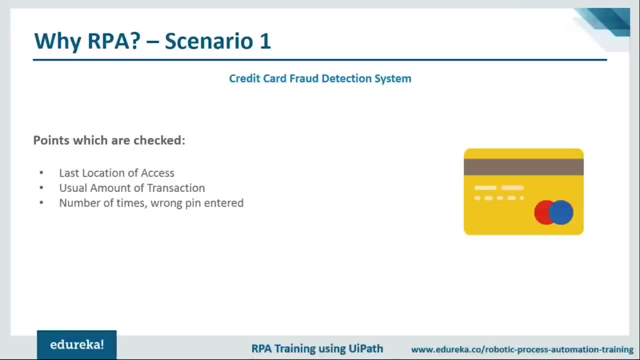 in any of the RPA tools. Let's move on to the first topic of today's discussion. The second topic is: why do we need RPA? So why RPA? So let's explain this using an example. As you know, every bank has this system that 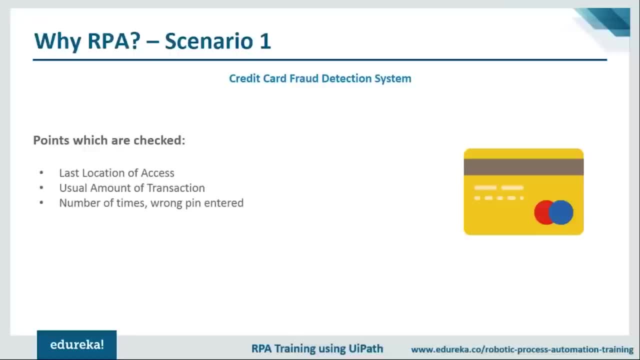 is called a fraud detection system. So let's take the example of credit card fraud detection system. Now. any transaction that is coming in it is judged on the basis of rules that you have designed. So let's consider these rules to be something like this: 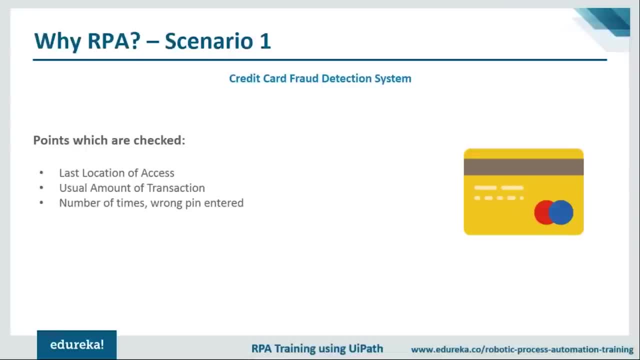 So, for example, the last location of access of your credit card is far away from the base, from the axis which is showing on the screen right now or which is being showing in the transaction right now. So it becomes suspicious. Second, the usual amount of transaction. 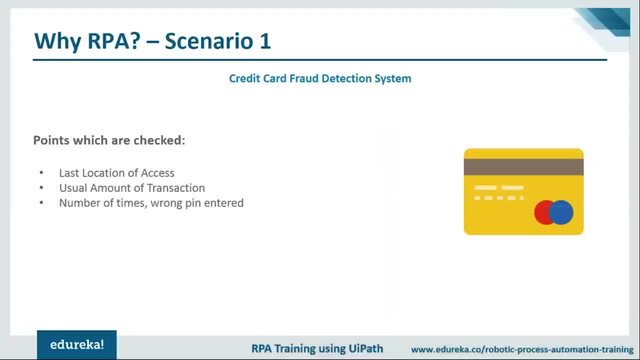 that maybe in a month you transact around 20 to 30,000 of cash from your credit card, but suddenly you made a transaction of 500,000, right, So that is a huge number. that also becomes suspicious. And the third rule could be that the number of trials 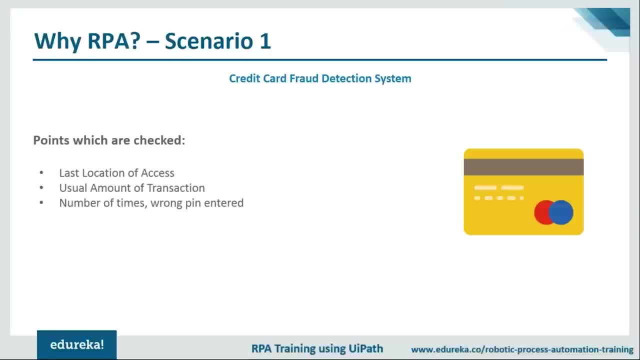 or the number of times you entered a wrong PIN right. So this could be that someone got hold of a credit card and he's trying to get money out of a credit card, but he's not able to get your PIN right, So this could also be a suspicious transaction, right? 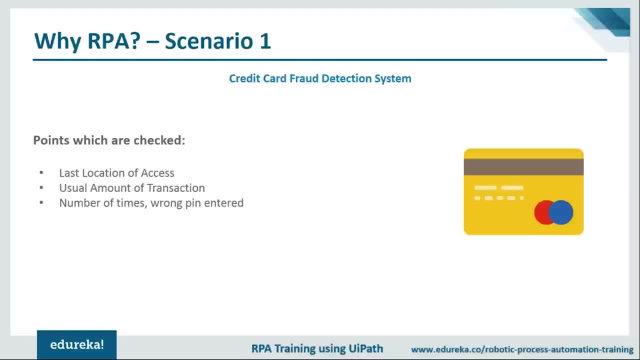 So if you were to judge a transaction based on these rules, one way of doing it is through the human workforce. So this human workforce was actually being used like 10,, 15 or 20 years back, when there was no automation system or no automation tool which was invented right. 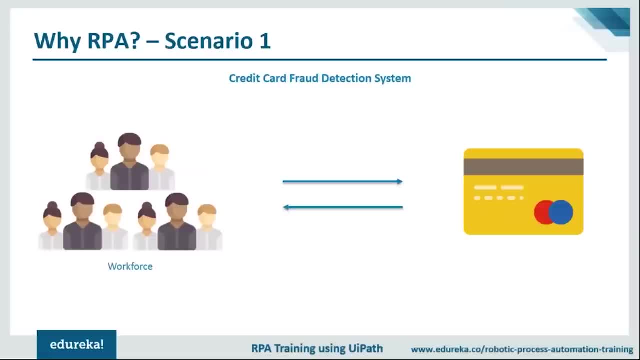 So there were a lot of people whose sole purpose was to investigate each and every transaction And authorize that transaction based on those rules. all right, But as and when automation came in now, 95% of those transactions are automated and the rest 5% of those transactions. 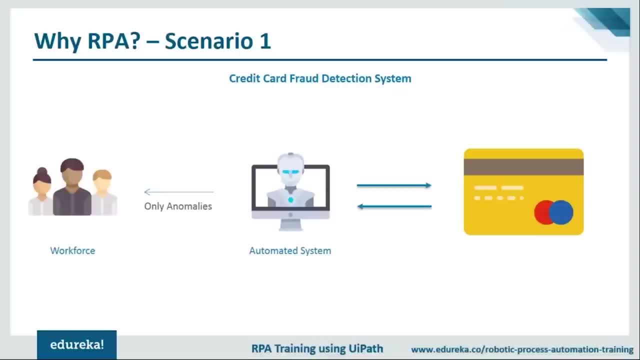 are just flagged as an anomaly. Now, why are they an anomaly? Anomaly are basically the transactions which cannot be judged by the automation system. Now, you cannot program your code to judge everything right. You cannot program your code to see the world. 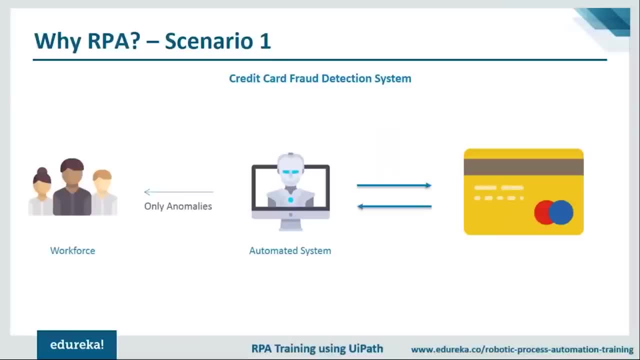 Right. So there are always some loopholes and there are always some situations that the computer cannot judge, and that's where you need human intelligence. So this is where you will be needing your expertise and you'll be judging whether this particular transaction is fraudulent or not. all right, 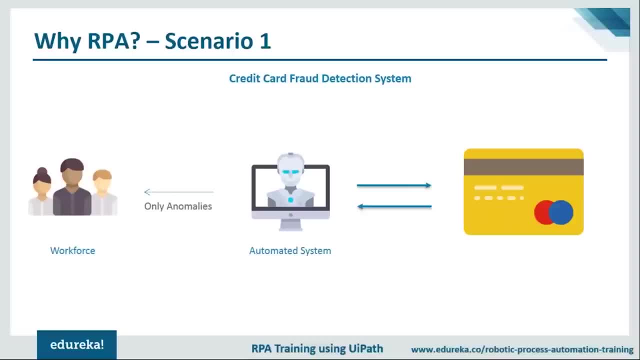 So this basically clears it out. when people ask me- it's quite often asked question- that will RPA replace the human workforce? So, guys, that is not entirely true. right, It may reduce the workforce That is already existing on a project. 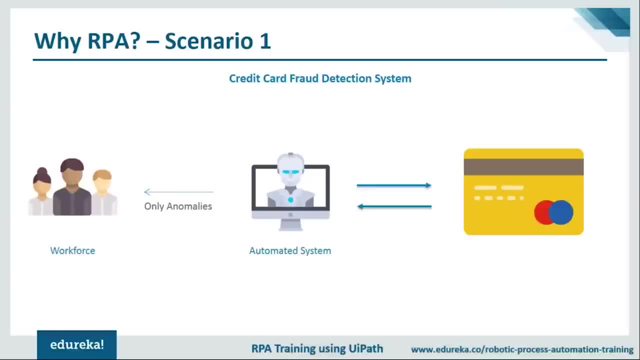 but it will never be able to replace the human workforce which is already working, Because in every department you need that human touch, because the basic difference between a machine and a human is that machines are good in following the things that we tell them. all right, 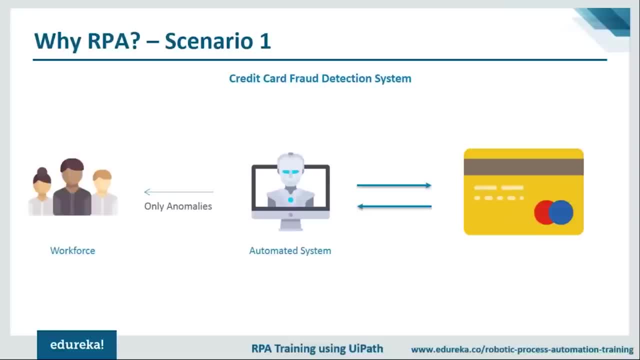 But humans are capable of thinking out of the box. They're able to think of something new, which machines are not right. So there will always be vacancies for humans to work inside a department, all right. So let's take another example. 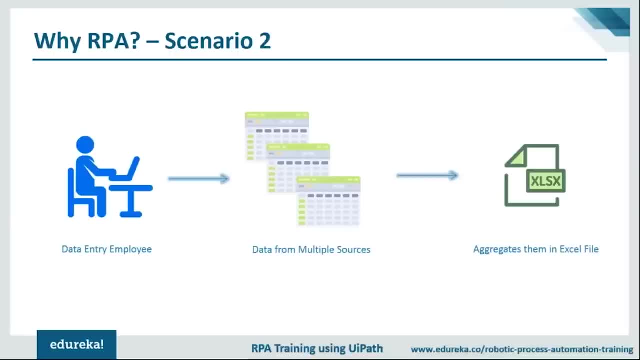 Let's take the example of a data entry employee. So the typical job of a data entry employee is to take data from multiple sources and aggregate them inside one file, right? So basically, this employee would follow the same steps each and every day for each and every iteration, right? 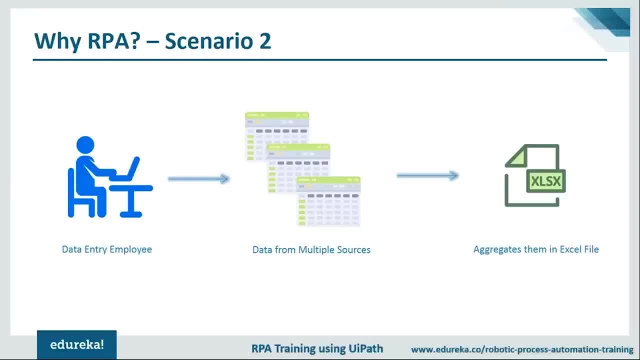 And then save it inside one file. So he's doing the same steps every day and then getting his job done. What if we can do that? What if we can tell our computer to do those same tasks and get the same job done? right? 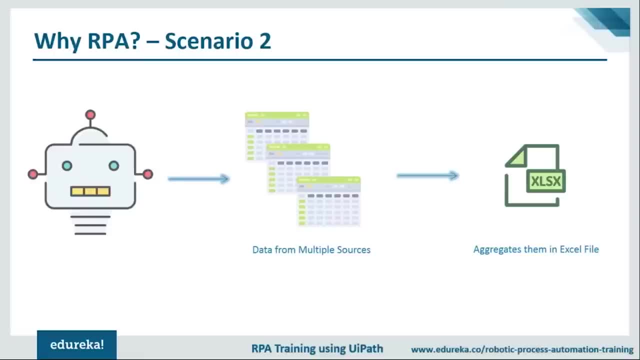 So this guy will then automate the task. So this: we are basically automating the task by making use of a robot or a machine or an RPA tool, And now our tasks become more fast and they become more robust, they are more accurate, et cetera. right, 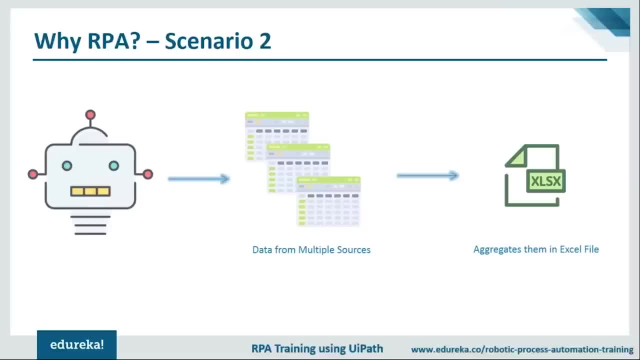 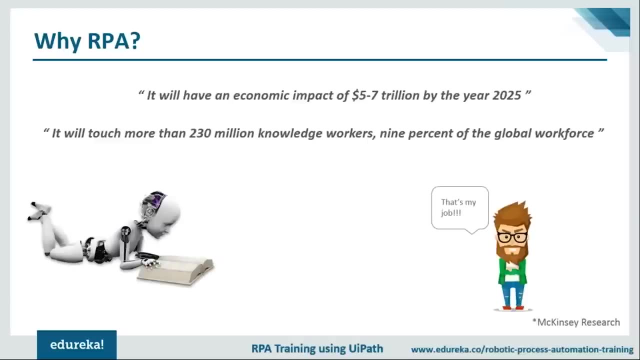 So in some situations, automation becomes a boon, and in some situations, it could be actually a threat to your job. all right, So let me give you some facts. So, according to McKinsey, by the year 2025, there'll be an impact of five to seven trillion dollars. 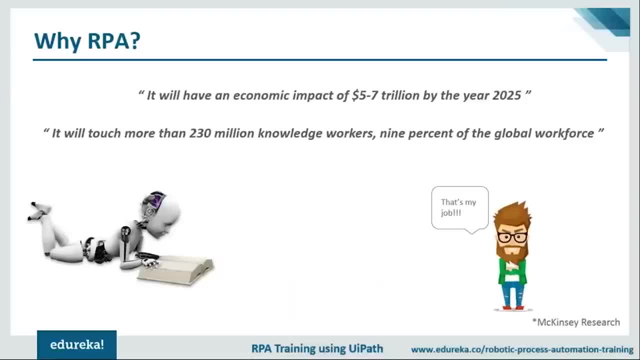 Right, five to seven trillion dollars is a huge amount of money, guys. It also says it will touch more than 230 million knowledge workers. all right, So don't get scared with this line, because it says it will touch the jobs of 230 million workers. 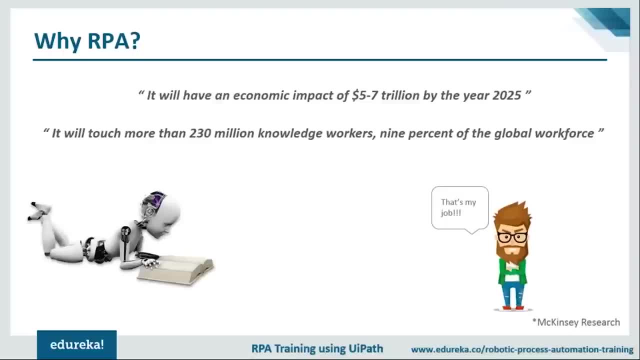 So what that basically means is that whatever tasks that you are doing today, maybe you'll not be able to do them tomorrow, Tomorrow you might be doing a different job or a different set of tasks will be expected from your job, right? So this is what you mean by there'll be a touching. 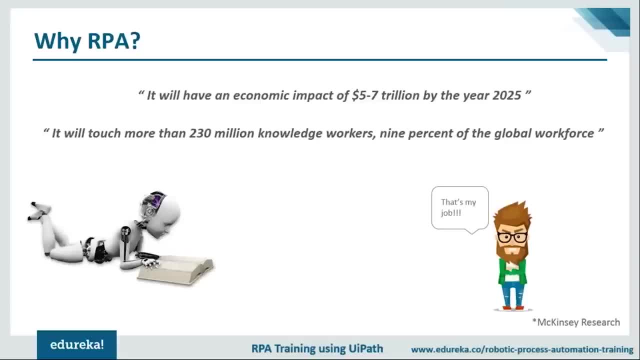 more than 230 million knowledge workers. So that is basically nine percent of the global working population, right, So don't be scared with the fact, guys, but it is always good to know about all the new technologies which are coming in the world. 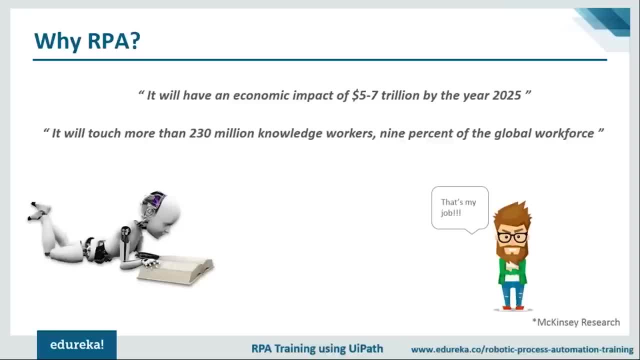 And, obviously, if you're best at what you do, nobody can replace you. all right. Having said that, let's move on and understand why RPA is. let's move on and understand why RPA is. let's move on and understand why RPA is. 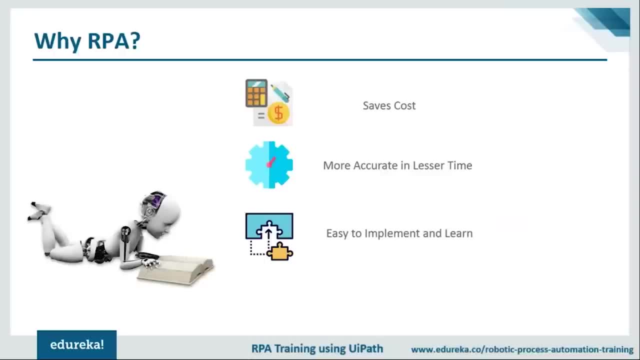 RPA is relevant from a company's perspective, all right. So if I'm a CEO of the company and I have to think about implementing RPA in my company, what are the things that I'll consider? So, first of all, if I'm using RPA, 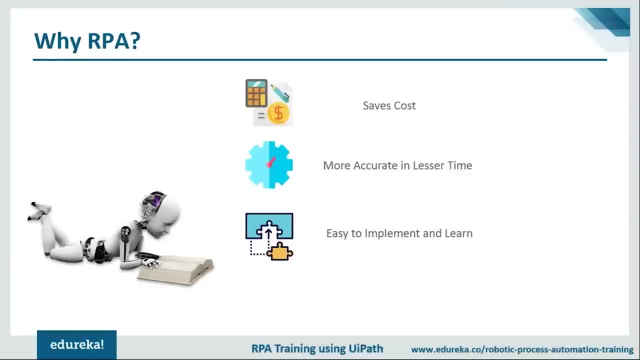 it saves a lot of cost because I'm downsizing my workforce with a drastic number, right, So I'll not be paying salary to a lot of employees now and also I'm getting my work done very fast, right. So it saves cost and, like I said, 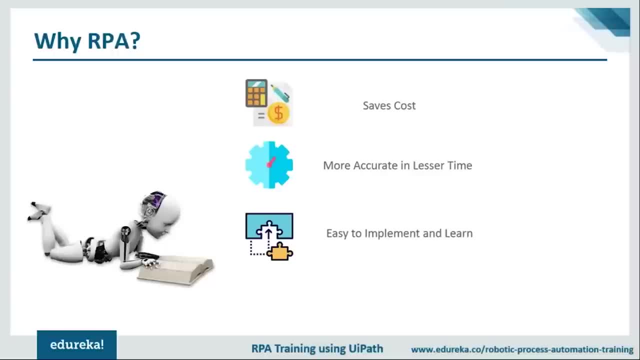 it is more accurate in lesser time, because machines, they do not commit mistakes, guys. They never get tired, they never commit any error, and hence they are very accurate. and that too, they do each and every task in the least time possible. all right. 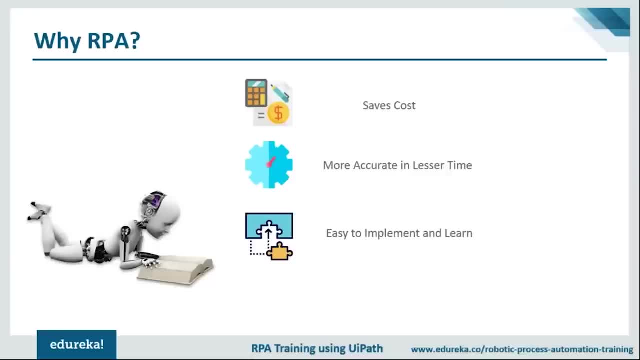 The third point is it is easy to implement and learn. This is probably the most important point: right To do any task, you can write a code right. So what's the point of writing thousands lines of code for a very small task? 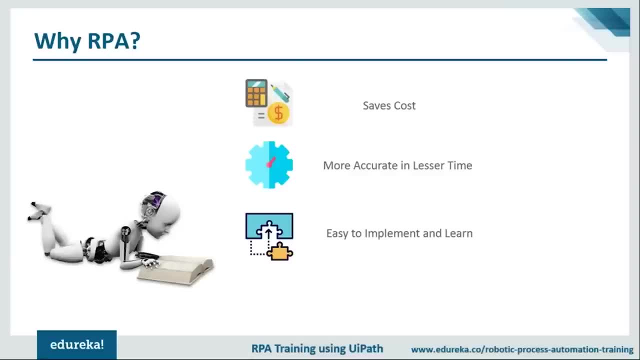 It's better to do the task on your own rather than writing thousands lines of code in it, But that's the best part about RPA. Whatever demo I showed you in the beginning of the session, it is all done using DAG and DROP and it hardly takes five minutes to configure it. 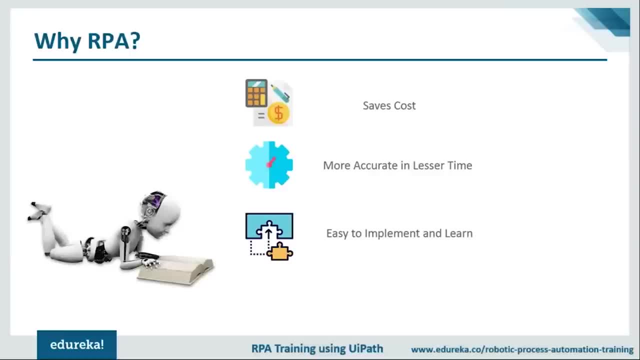 And if you don't believe me, hang on till the end of the session and I'll show you how you can do that demo. all right, So with this, guys, we have understood why did we need RPA, and let's move on to the part. 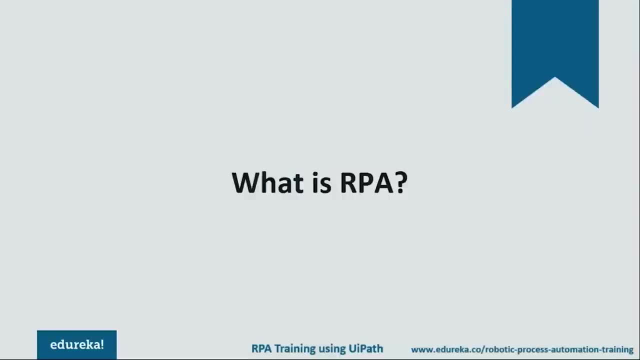 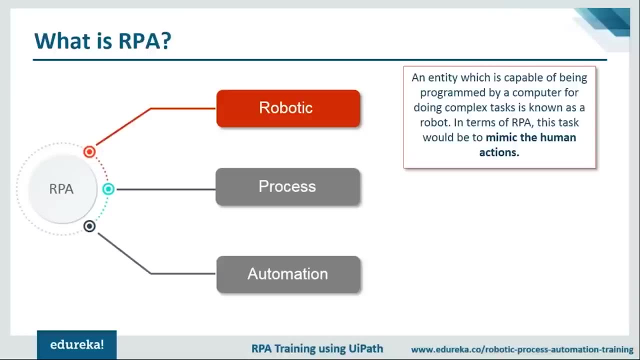 where we'll understand what RPA exactly is. All right, so what is RPA? So RPA, as you might have guessed, it's an acronym for robotic process automation, right? So let's understand the three terms one by one. 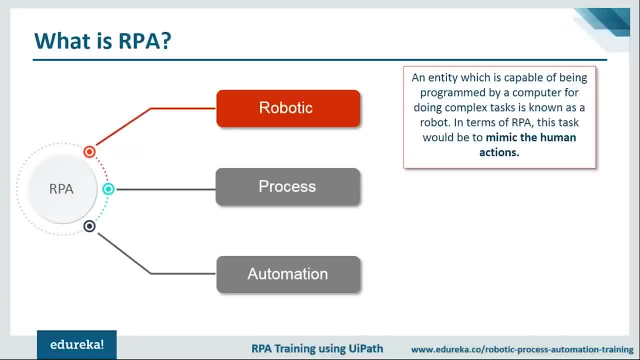 So what is robotic? Robotic is basically an entity which can be programmed to mimic human actions. So any entity which can mimic human actions on being programmed is called robotic. Then comes process, so a sequence of steps which lead to a meaningful activity. 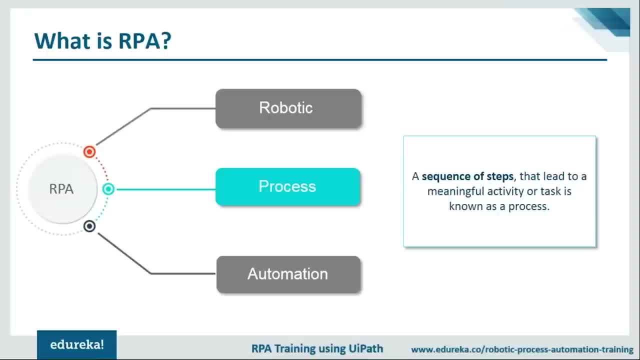 For example, you make tea right. So to making tea, the first step would be to pour some water, let it boil, then put some tea leaves, let it boil, and then to pour some milk in it. Right, your tea is ready. 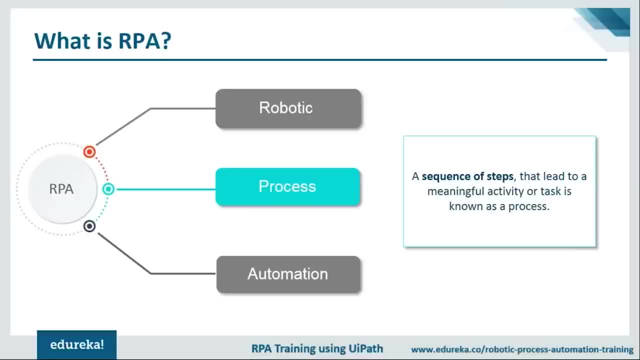 So you did three steps and with the help of these three steps, your tea is ready, right, So this becomes a process of making tea. Then comes the type: automation. So what is automation? Automation basically means when a task happened automatically without human intervention. all right. 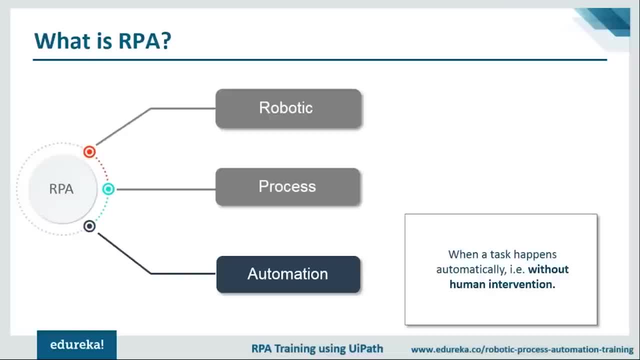 So whenever a task happens without any human intervention, it becomes automation. Now, if you take the words robotic process automation, robotic means mimicking human actions to do a process without human intervention. This is the meaning of RPA. this is what it basically means. 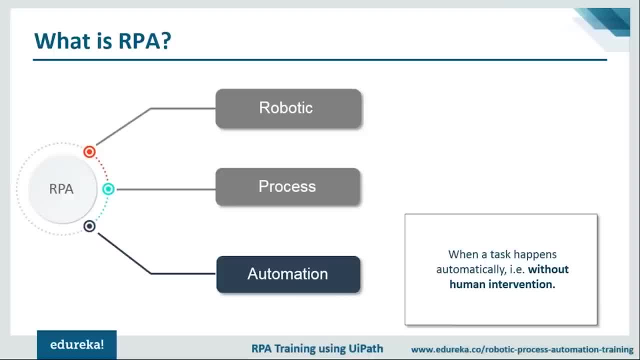 This is the definition of RPA, all right. So now that we have understood the definition of RPA and we have understood why do we need RPA- we saw how RPA can work. let's go on and understand the different tools using which we can actually implement the RPA technology. 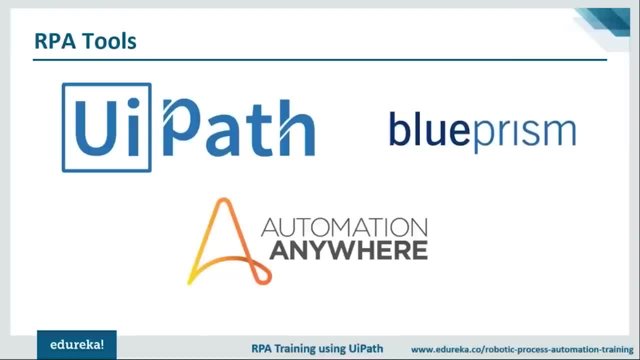 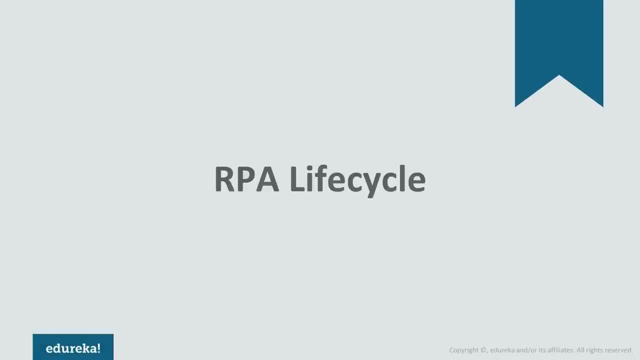 All right. as of now, there are three tools which are at the top of the ladder, which are UiPath, Blue Prism and Automation Anywhere. These are the three best tools in the RPA world. So now that you know what exactly robotic process automation is, 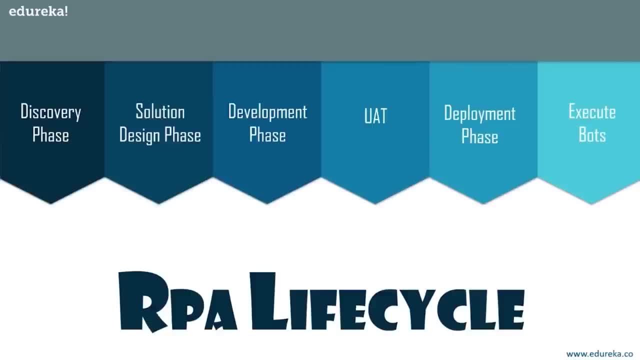 let's get into RPA lifecycle. So RPA lifecycle has mainly five stages and an additional stage that is to execute the bot. So the starting stage is the discovery phase, then we have the solution design phase, then we have the development phase. 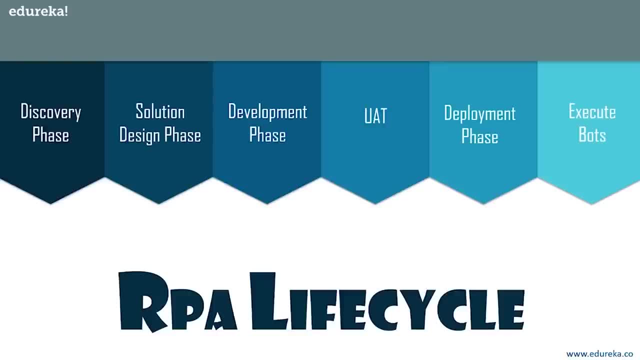 then the testing phase, that is, the user acceptance test, then the deployment phase and finally, the bots are executed. So, guys, these are the various phases of RPA lifecycle. Don't worry, We'll be discussing about each one of them in depth, one by one. 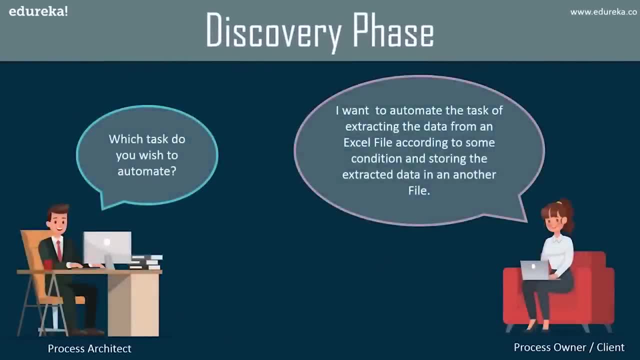 So let's start with the first phase, that is, the discovery phase. So the discovery phase is the phase, basically, where you look, the requirements are analyzed. For example, let's take a scenario where we want to automate the task of, you know, extracting the data from a specific Excel file. 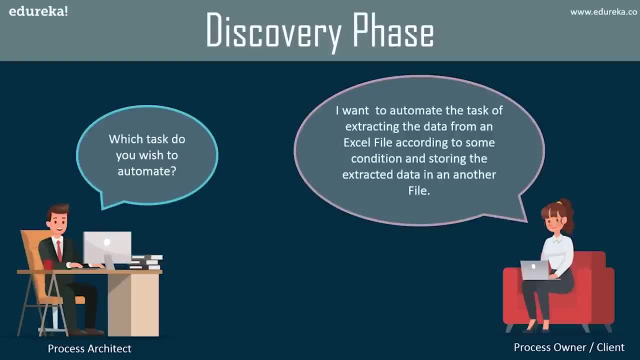 according to some condition, and then the extracted data must be stored in another Excel file. So that is basically our client requirement. Now the client goes and gives us a requirement for the process architect. So process architect is basically the person who interacts with the clients. 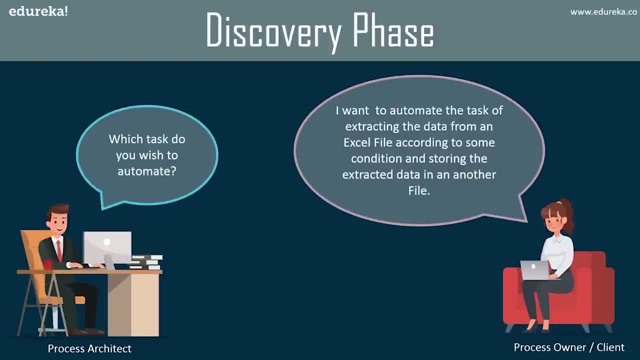 and ask for the requirements of the clients. So we're here, as I just mentioned before, that we're going to consider a scenario of how to extract a data from an Excel file according to some condition and then store the extracted data into another Excel file. 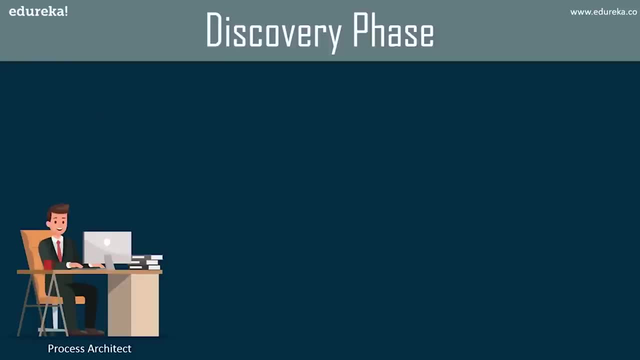 So now what happens in the discovery phase is that the first step is to analyze the client requirements. So the process architect sits with a steam and analyzes the client requirements. Once the client requirements are analyzed, then the process Architect decides whether the process can be automated or not. 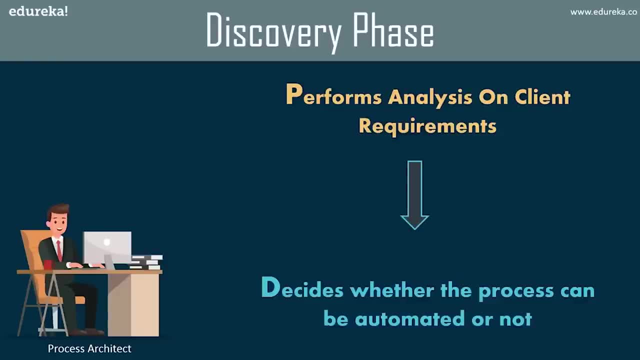 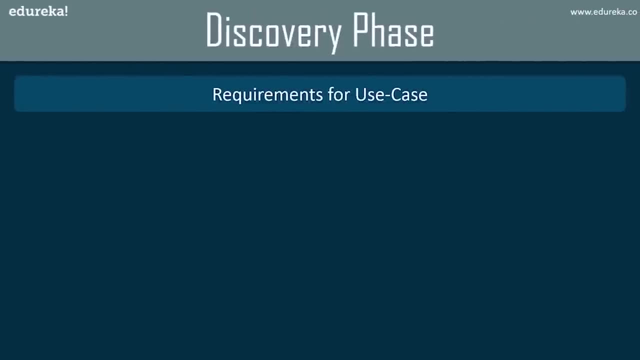 Let me tell you guys, not every process can be automated. There are few dependency issues. you know where some processes can be automated and when some cannot be. well, the scenario that I've considered definitely can be automated. So all the requirements for our use case are basically a system. 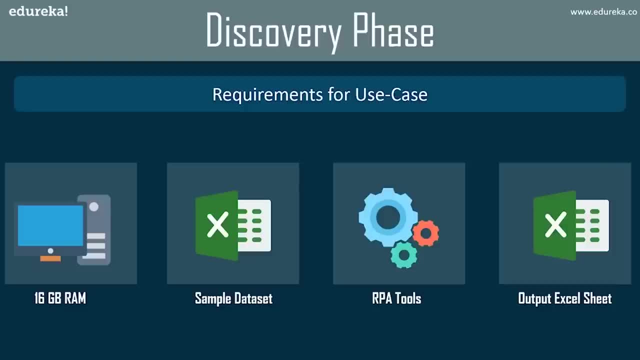 with a 16 GB RAM- basically a good memory system. Then we have a sample data set from which the data has to be extracted. after the sample data set, We have an output sheet where we're going to store the extracted data And finally, 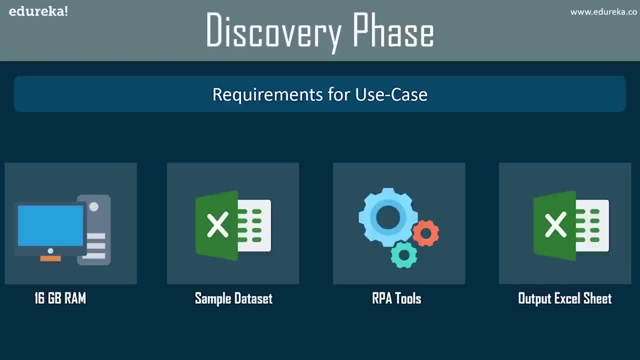 we have a tool to automate the task. So basically, these are the requirements for our use case. So, according to your task, or maybe according to your clients requirement, you will have a specific set of requirements for specific tasks to be automated. Now, once all the requirements are analyzed, 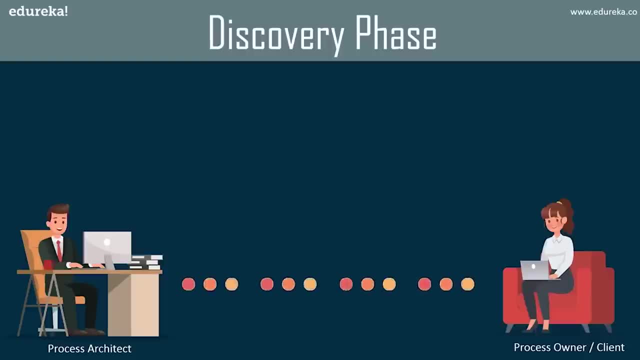 obviously there comes a scenario where you have to decide: you know where the process can be automated or not. So, for example, let's consider, if the process cannot be automated, then the process architect just directly informs the client that you know the process cannot be automated. 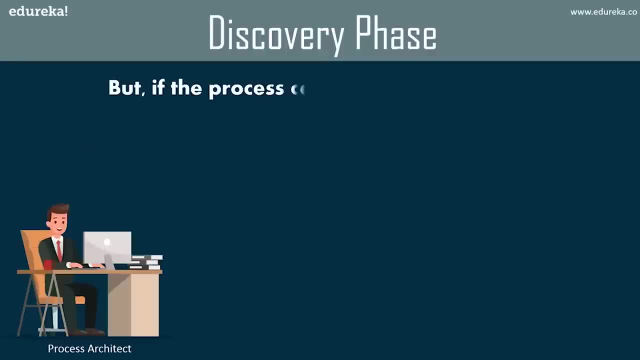 and then obviously lets down to reason. but yes, if the process can be automated, then the next step is that you know the complexity is measured. So when I talk about complexity I mean that basically all the dependency issues are checked, and then all the network issues, RAM issues, dependency issues, 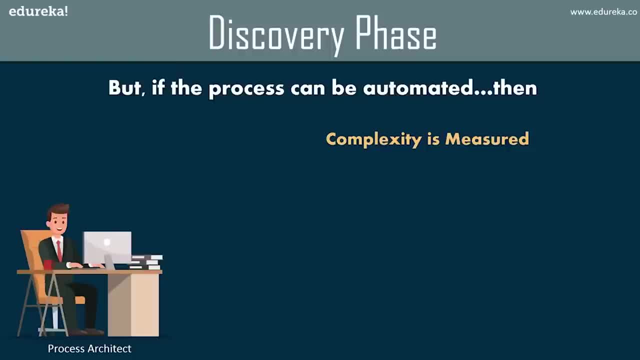 Maybe you can understand by the fact that if you automate a specific task, how much can the users use that task, and so on? right. So that's how the complexity is measured And finally, the benefits provided by the automation are also taken into account. 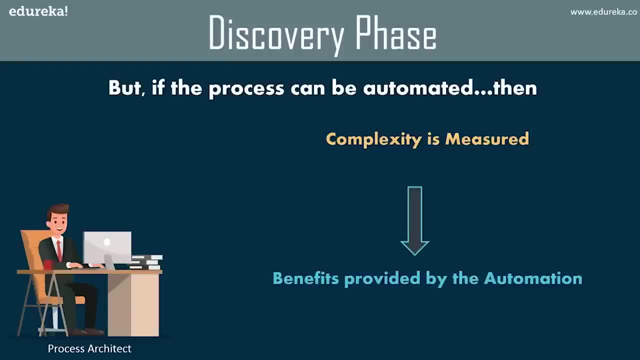 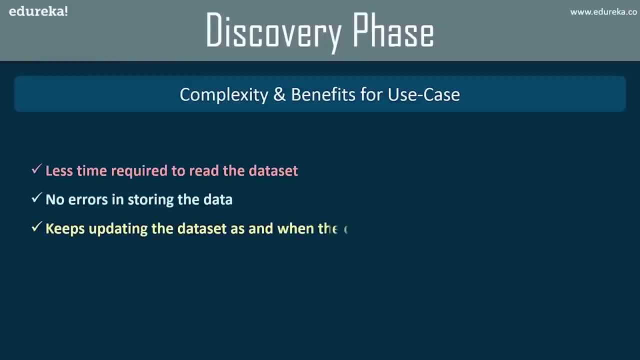 So obviously when you're doing some action you need results back, So that's what is measured at the last step of this particular phase. So benefits for our use case could be that you know less time will be required to read the data set. 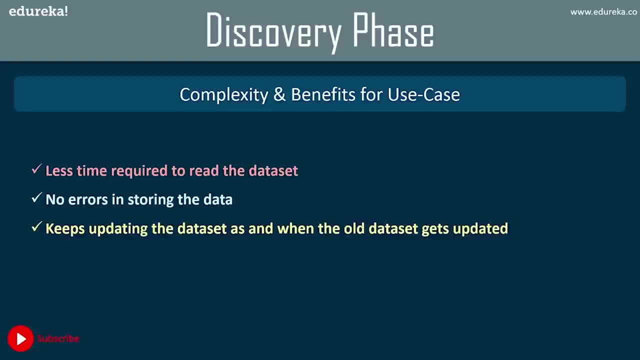 So, for example, if you consider a employee sitting and reading each tuple of the sample data set and check the condition, So if the condition satisfies, he has to manually store all the data into the output data set. now, obviously this would be time-taking right. 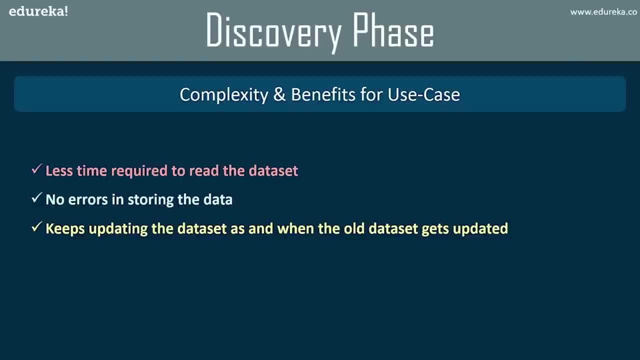 So if you just automate the stars- and less time would be required, obviously no errors would be there in storing The data set. and finally, even if our sample data set gets updated automatically, our output sheet also gets updated. So that's how, basically, you can decide. 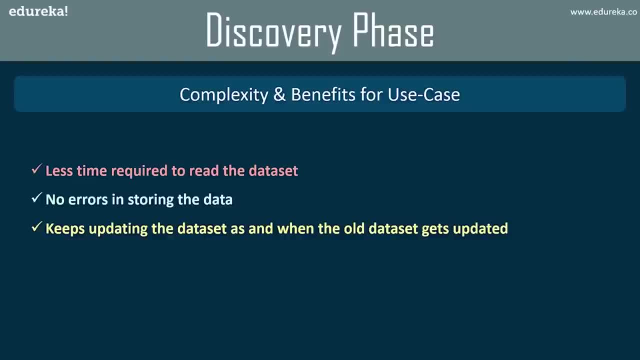 on what are the complexity and benefits of your automation. So if I have to just summarize Discovery Phase for you, then what happens is that the process architect communicates with the client and takes the requirements of the client. after that, The client's requirements are analyzed. 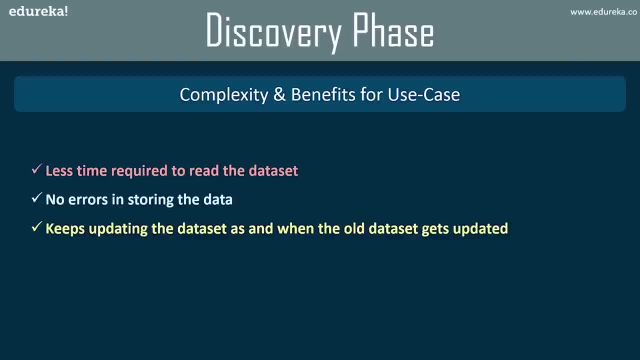 and then it is decided whether the process can be automated or not. once if it is decided that the process can be automated, The complexity of the process is analyzed and also the benefits of the automation are taken into account. So, guys, this was an end to the Discovery Phase. 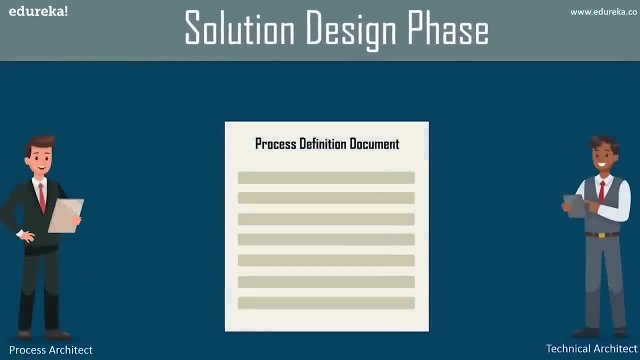 Now let's move forward with the next phase, that is, the solution design phase. So in the solution design phase, what happens is that the solution for your automation is designed, So the process architect sits down with the technical architect and both of them make the process definition document. 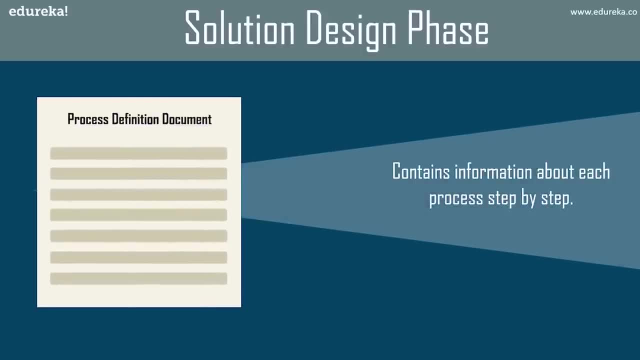 Now the process definition document is a document which contains information about each and every step of the process in depth. So basically, once the process definition document is designed, the next step that comes into picture is basically deciding the budget, the number of people working on the project, time to be spent. 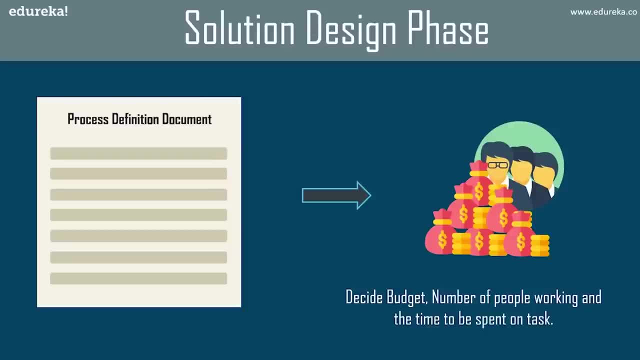 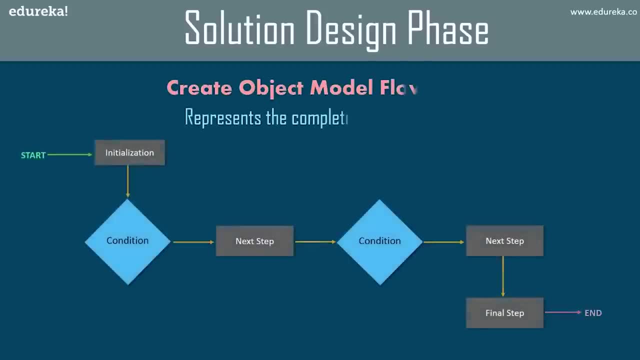 on the project, what will be the production environment, and so on. So all these requirements are basically analyzed, and once this is also analyzed, the next main step that comes into picture in this particular step is the designing of the object model flow chart. So, basically, the object model flow chart represents the complete flow. 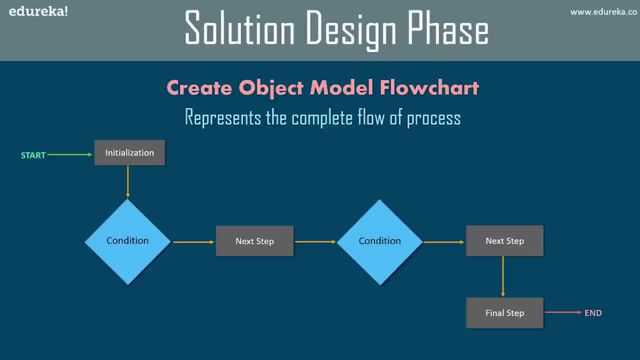 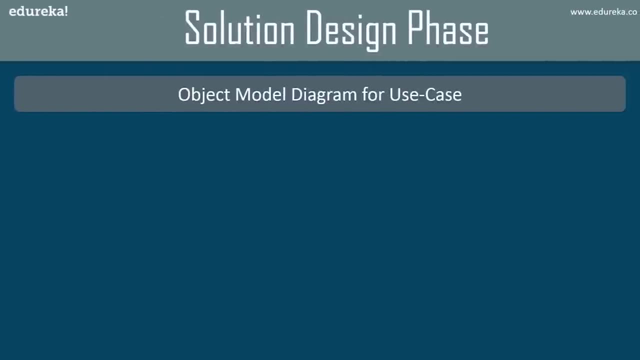 of the process. So anybody in the further steps developing the bot can refer to this particular diagram and then finally create the board. Now the object model diagram for the use case that I considered would be as you can see on your screen, So we would start the project by mentioning the part. 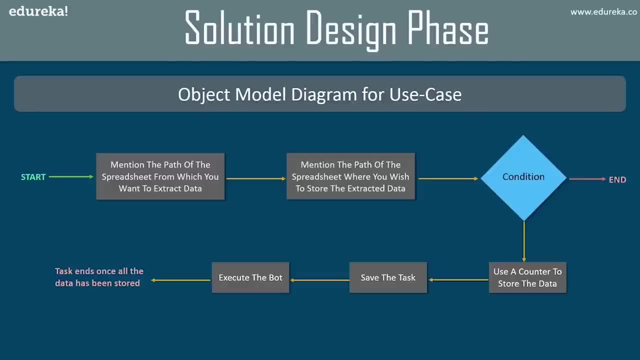 of the spreadsheet from where we want to extract the data, That is basically from the sample data set, and then we would also mention the part of the spreadsheet where you wish to store the extracted data after. that will mention this condition. Basically, let's say, you know if we have a sales column. 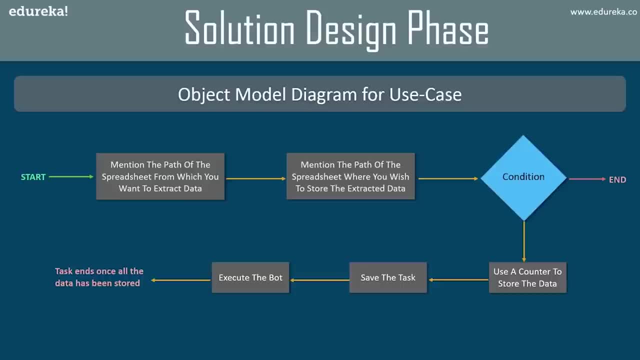 then if sales is greater than 2.5 lakhs, then we want all the data from that particular road to be stored into our output data set, So that particular condition will be mentioned, and after that we'll use a counter variable to basically initialize a loop such that you know. 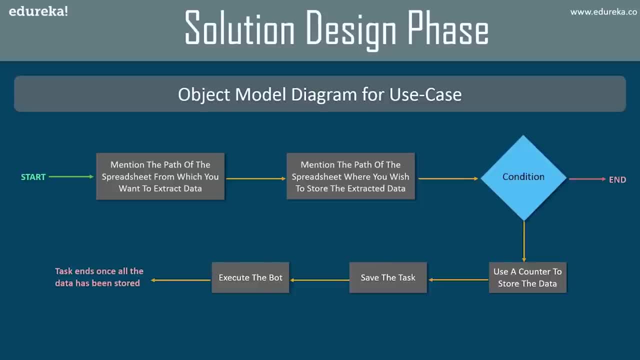 for every time the condition is satisfied, that particular row values would be stored into the output data set and then the counter increases, by which I mean that you know the next row will be analyzed. after that, the task would be saved and we will execute the board now. 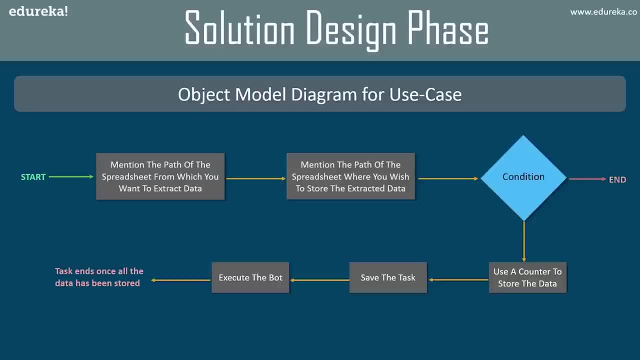 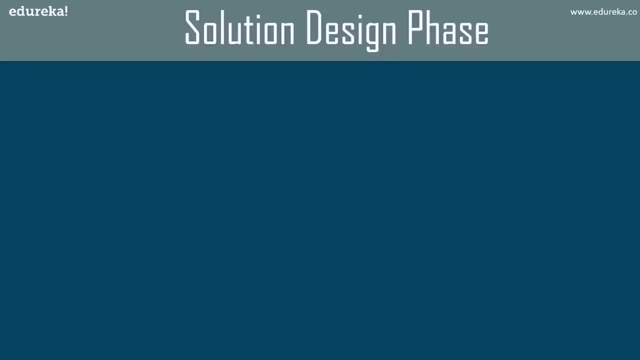 We have the condition does not satisfy, then the task ends then and there, right. So that's how you can basically design an object model flow chart. guys, Now, once the object model flow chart is designed, the next step that you have to decide in this particular phase is the RPA tools. 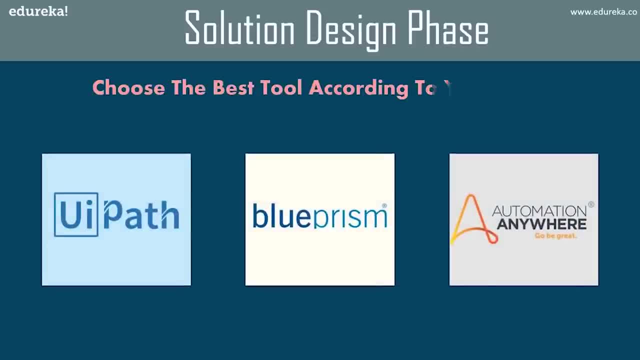 on which you want to automate your task. Now there are enormous amount of tools in the RPA industry, but the top three tools in the RPA market are uipath, blue prism and automation anywhere. So these three tools will basically help you cater your needs. 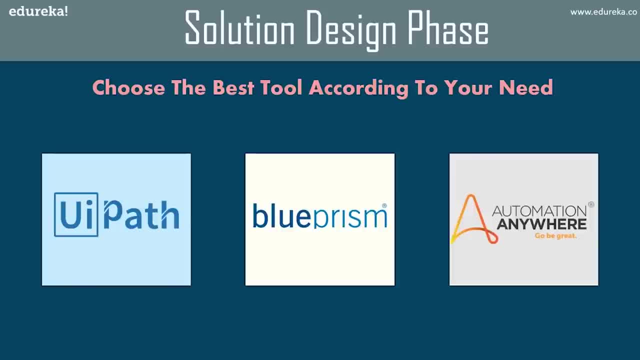 to your client requirements. So it's completely your call on which tool that you wish to choose. So, if I have to summarize the solution design phase for you guys, after the discovery phase, where it is decided that you know the process will be automated, what happens is the first step. 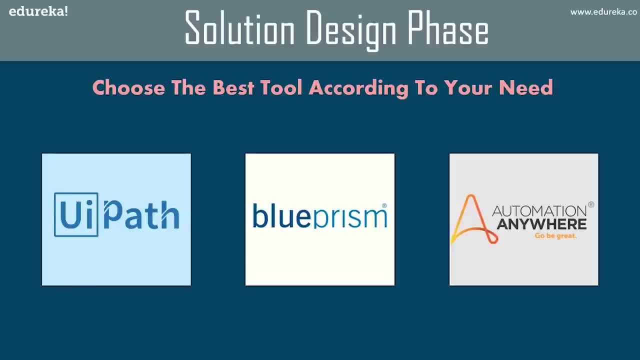 that you have to do is basically create a process definition document wherein you mentioned all the information about the process step-by-step. after that, What do you have to do is you have to decide the other requirements, like the budget, the number of people and the time to be spent on the process. once that is done, 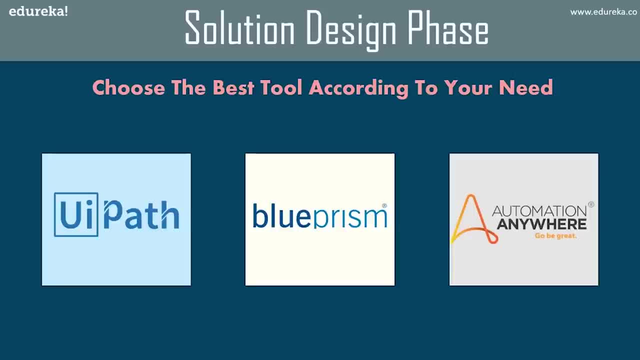 You have to create an object model flow chart which basically shows the workflow of the project or basically you can understand that you know- it shows the flow of the process for the automation to be developed And finally you have to choose an RPA tool. 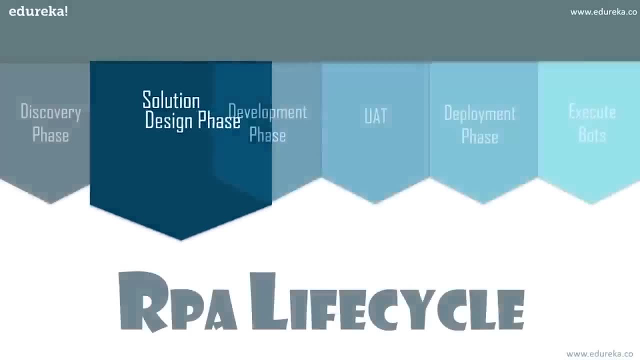 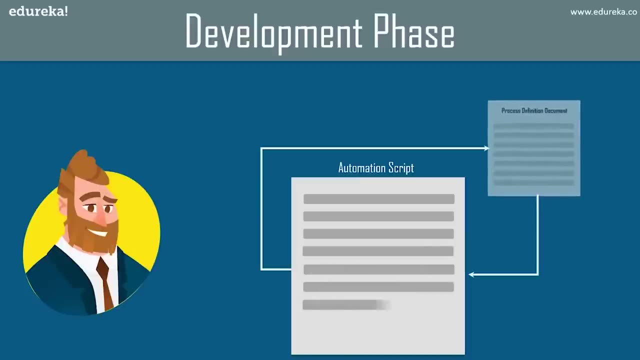 upon which you'll automate your task. So that was about the solution design phase, guys. Now let's move forward with our next phase, that is the development phase. now, the development phase is the phase, basically, where you know the automation is developed. So the automation developer basically refers: 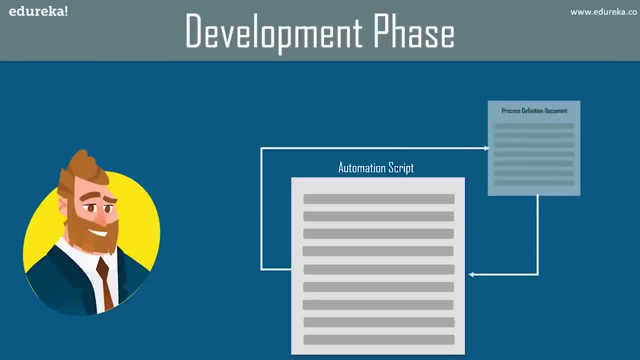 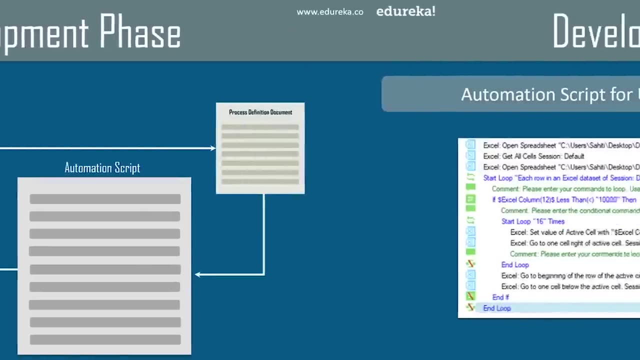 to the process definition document and starts creating the automation script. or you can understand that you know the workflow of the automation, So that's how the automation developer comes into picture. So for our use case, our automation script would be as you can see on my screen. 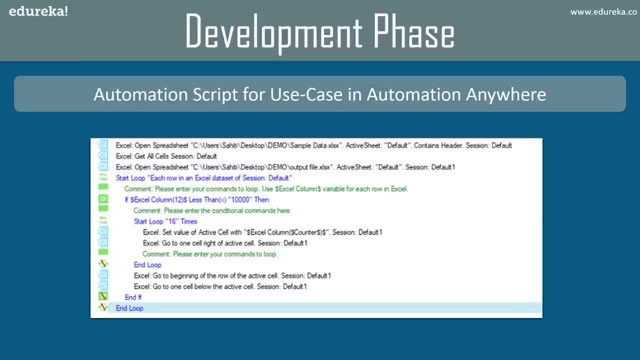 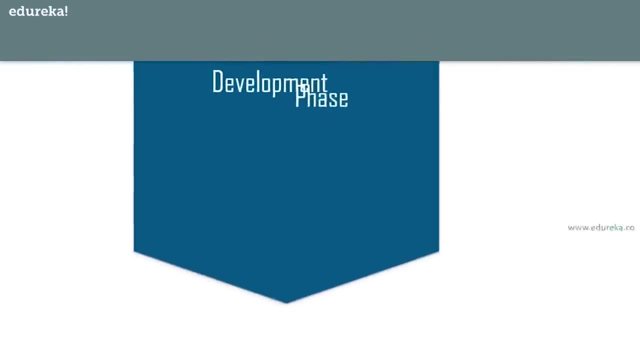 and I've chosen automation Anywhere. but this is how, guys, the automation script looks. basically, you just have to create a workflow using the different activities or commands in the chosen RPA tool. So, guys, with this we come to an end of the development phase. 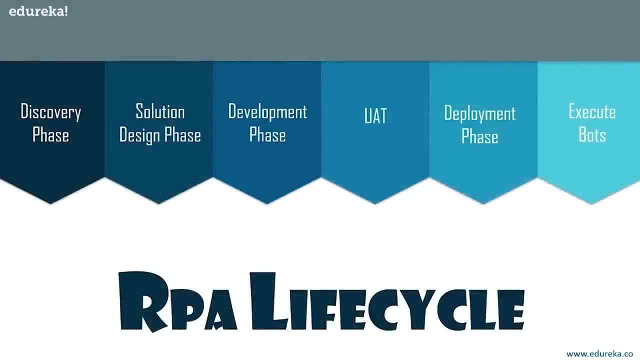 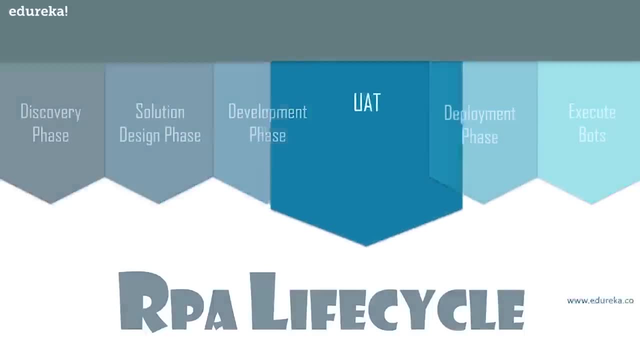 So development phase was quite simple, guys. Basically, it is this phase where you know the automation is actually developed or you can see the bot is developed. Now, once the bot is developed, the next phase that comes into picture is the UAT phase, that is, the testing phase. 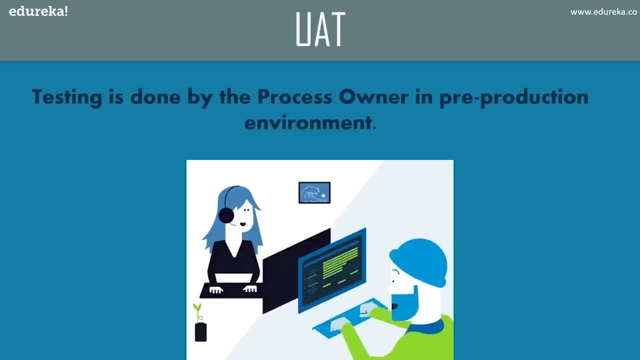 So the testing is basically done by the process owner in the pre-production environment to check whether the developed bot is working or not. So, basically, the bot is deployed to check how the users would use that bot and if there are any errors which still have to be rectified right. 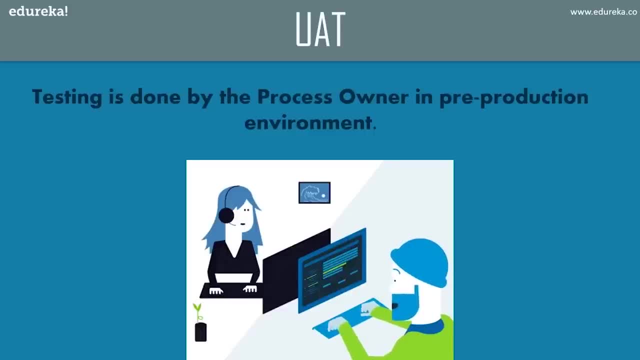 So the UAT phase is quite simple, like in any other software testing lifecycle, or you can say the SDLC lifecycle, the testing phase, how we test a simple software. the same applies over here: that testing is done for the developed bot in the pre-production environment. 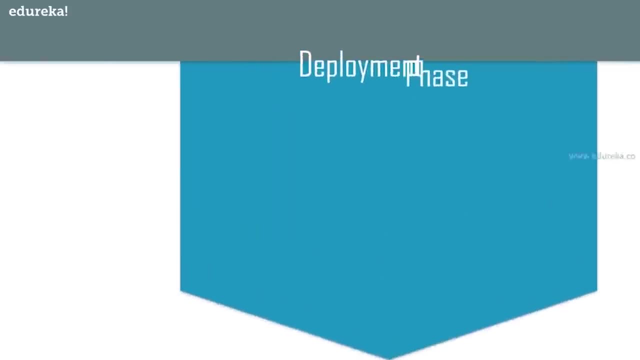 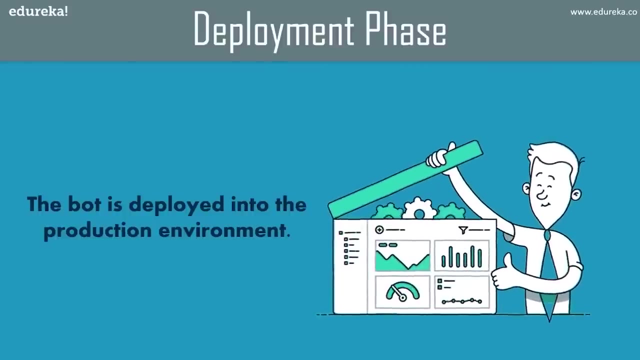 So, guys, that was about the UAT phase. Now let's move forward with the final phase, that is, the deployment phase. Now, the deployment phase is the phase where, basically, the bot is deployed into the production environment. So once the bot is developed and then it is tested into the pre-production environment, 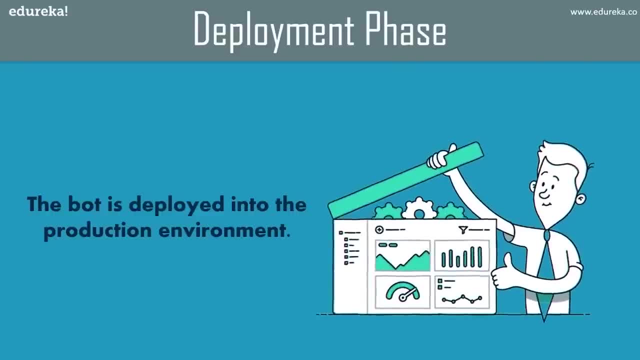 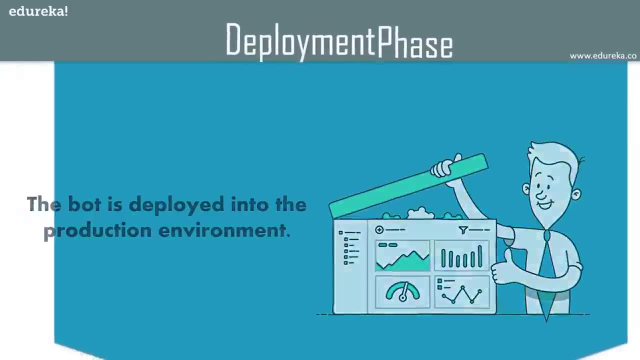 and once it passes that test, the next phase that comes is basically the deployment phase. So basically, the bot is deployed into the production environment and the users can use that port. Now, once the bot is deployed, the final phase, or you can say the additional phase- 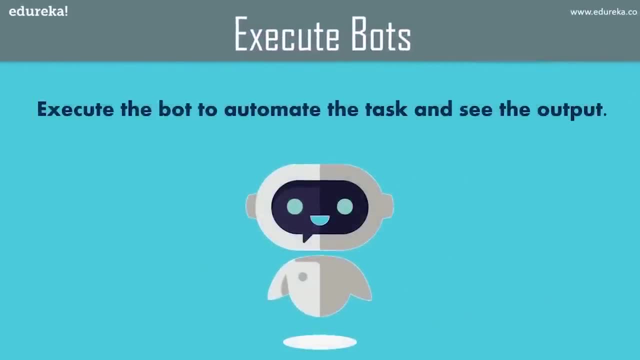 to this particular RPA lifecycle is executing the board. So once the users have access to the board, which is deployed into the production environment, the users can just run or execute the boss to generate meaningful result. So in our scenario, what I considered was this particular sample data set. 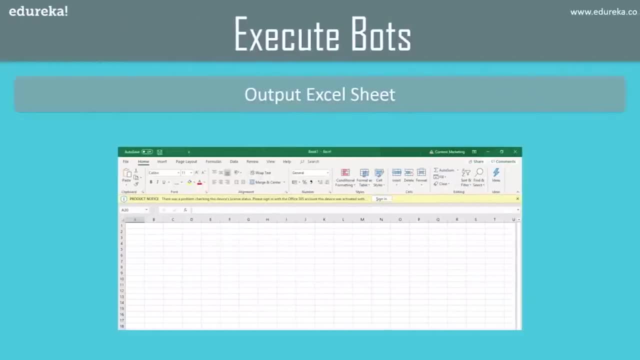 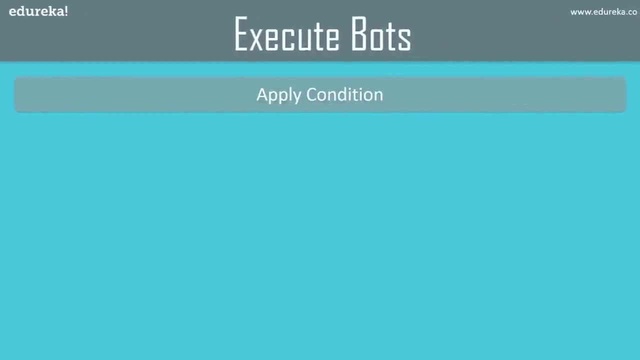 having n number of rows and columns. This was the output Excel sheet, which is basically a sample blank Excel sheet. Now, the condition that I wanted to apply was on the sales column, which was present in the sample data set. So if the sales was greater than 2.5 lakhs, 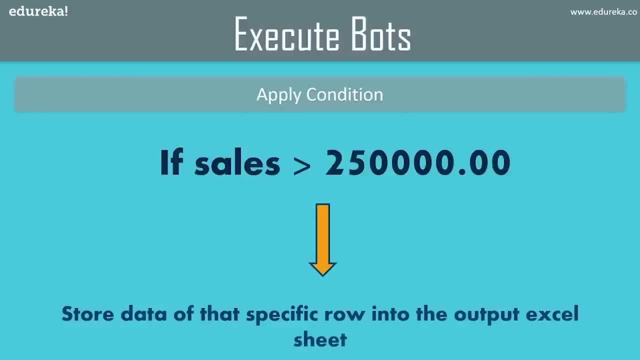 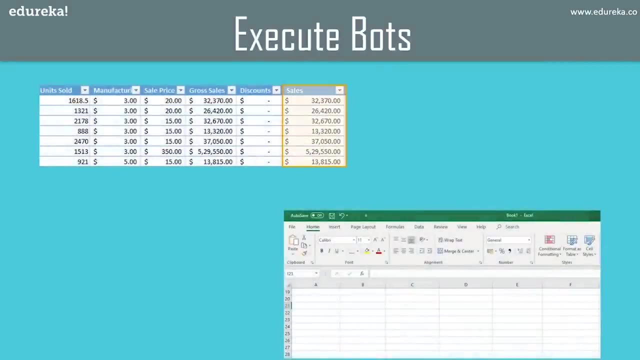 what I wanted was to store the data of that particular specific row into the output Excel sheet. So when I execute the bot, what happens is that first the sales column gets highlighted from where we want to extract the data, After that all the values which have the value greater. 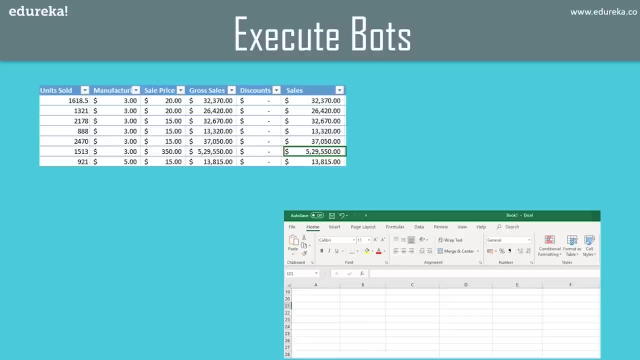 than 2.5 lakhs will be taken into account. So, if you consider the sample data set that I chose over here, only one row has the value greater than 2.5 lakhs, So that particular row values would be stored into the output data set, right? 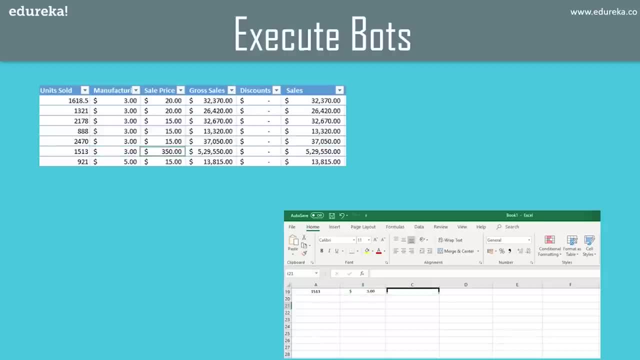 So all the rows, all the values from units sold, manufacturing, sales, price, cross sale, discounts and sales will be stored, one by one, into the output data set. as you can see, that's happening. So, guys, this was just a single row example that I showed you over here. 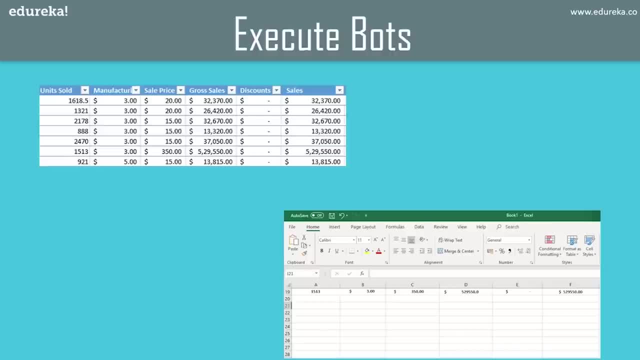 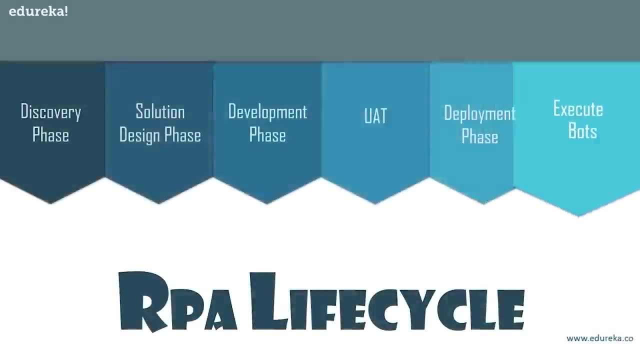 You can take a complex data set and then you can create the same automation script and you will understand that. you know all the data is being stored into the Excel data set. So with this, guys, we come to an end of the RPA life cycle. 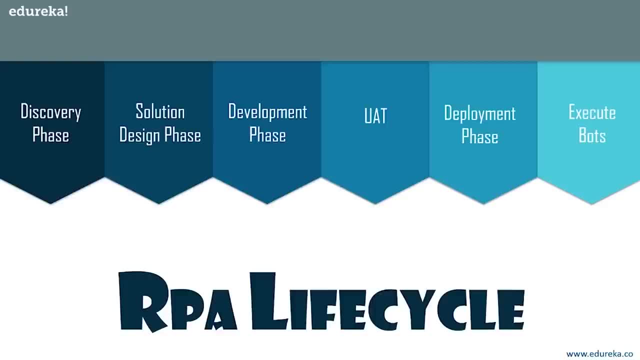 So if, after just give you an overview of the complete RPA life cycle, then you basically start a project where you first analyze the requirements and check whether the process is eligible to be automated or not. If yes, then you move forward, If no, then you inform the client that you know. 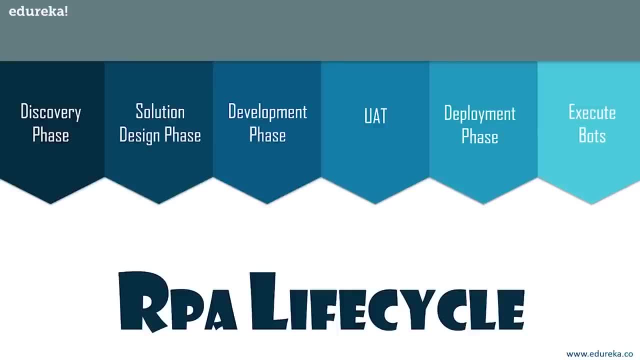 the process cannot be automated. So if the process can be automated, then you measure the complexity of the project and then analyze the benefits of the automation. So until this all the steps would be considered as a discovery phase. after that you move forward with the solution design phase. 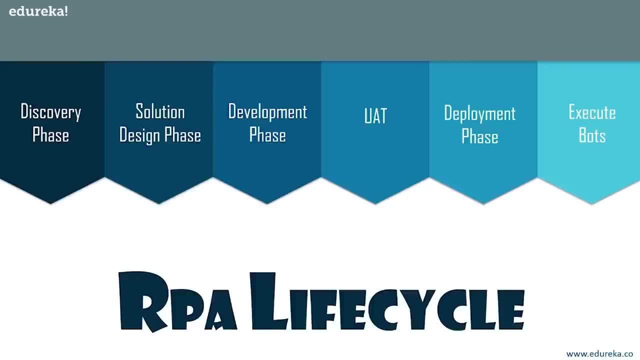 where you create a process definition document which will contain information about all the processes step-by-step, basically into depth. after that, you decide upon the budget, the number of people to be working on the project and other factors such as time to be spent on the project. after that, you create an object-mounted flow chart. 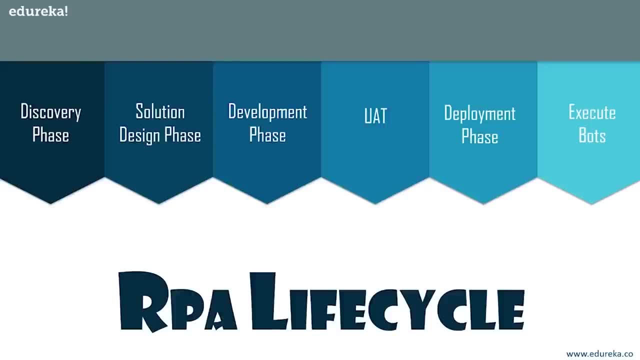 which basically shows the flow of the process, and then finally choose an RPA tool upon which you wish to automate the task. So these steps will be considered as the solution design phase. after that, the life cycle moves on to the development phase, where you develop an automation script referring to the process definition document. 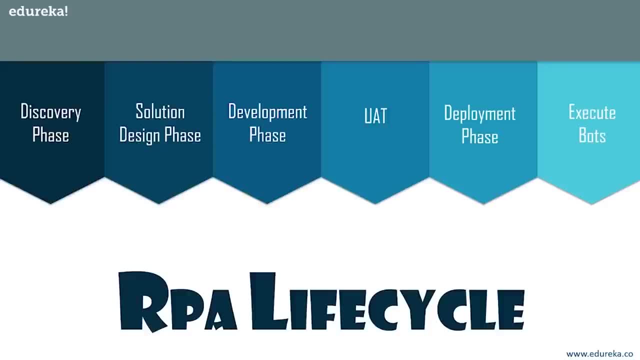 and finally move to the testing phase, where you test the developed automation or basically where you test the developed bot in the pre-production environment. Now, if there are any errors, or so maybe any additions that are found to be added, then the board goes back to the development phase. 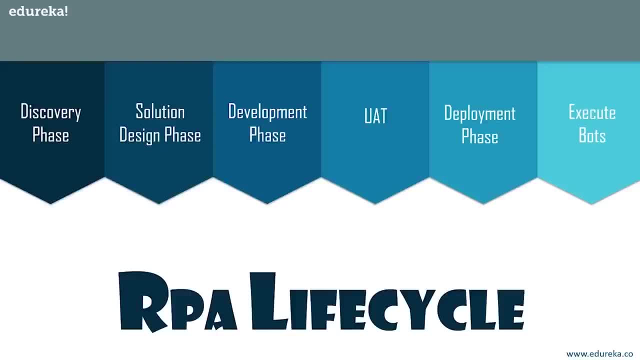 where the development team sits and works out to find the solution of the problem and again pushes the board to the testing phase and then, once in the testing phase, if the board is approved, into the pre-production environment, it is then deployed into the production environment. that is basically a deployment phase. 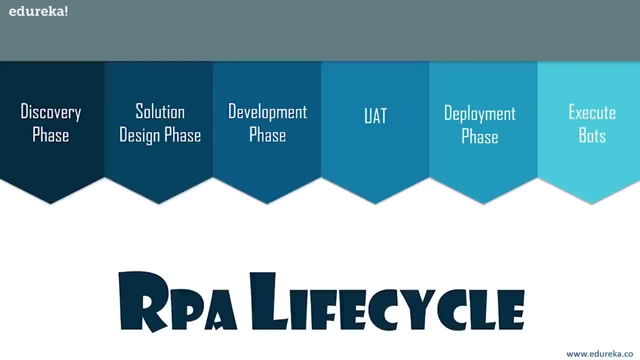 Now, even after deploying the board into the production environment, if there are any errors found into the board, then the board goes back into the development and the testing phase and again the board is deployed into the deployment phase and finally you execute the bots to generate meaningful results. 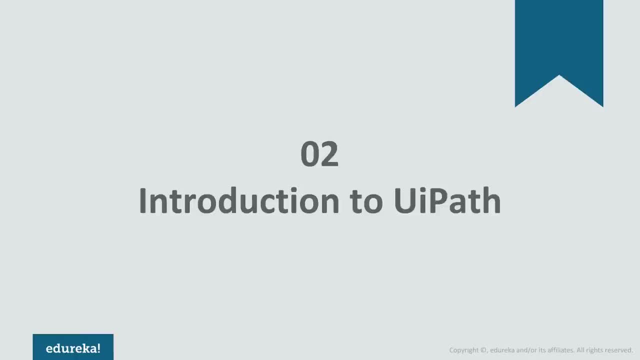 that is to see the output. Let's get started with UiPath Studio. So UiPath Studio is basically a dashboard through which you can automate various kinds of tasks. Now, this dashboard has various options that I will talk about later in the session, and all these options can be used to you know. 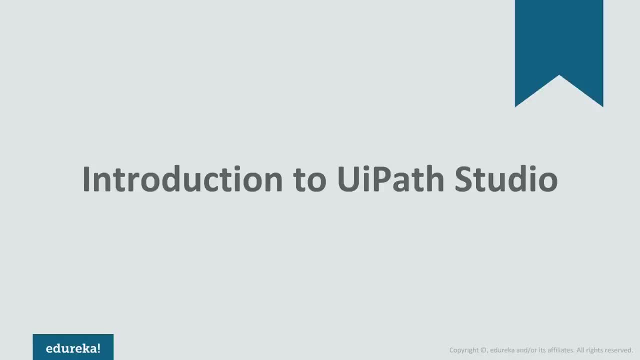 integrate various platforms and then automate different kinds of tasks, either it be like Excel, PDF, or maybe you want to automate tasks on an application, or maybe if you want to scrape data, then you can do all kinds of actions like that. So before I move forward, 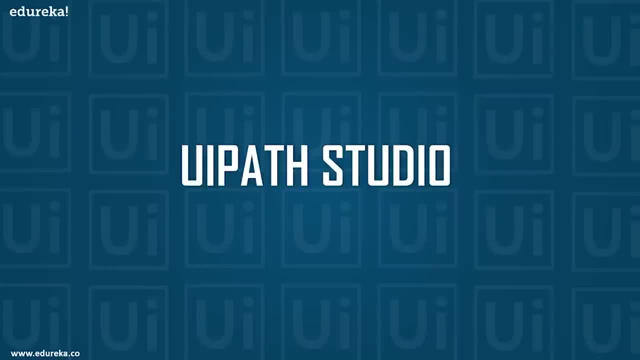 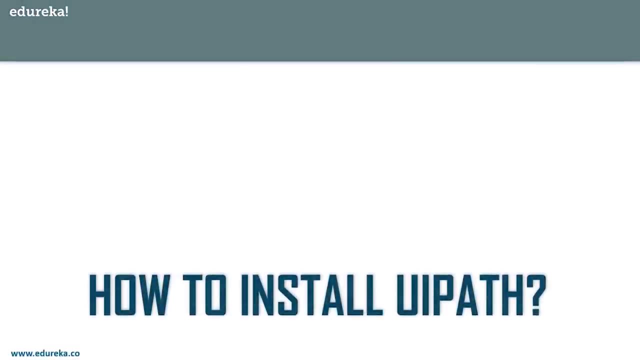 and show you how the UiPath Studio looks and how you can get started with automating tasks. Let me just tell you the steps to install UiPath. So the steps to install UiPath are as you can see on my screen. Initially you'll have to go to the official website. 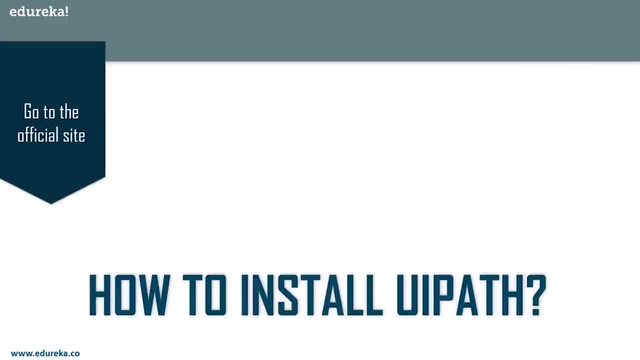 to download either the Enterprise Edition or the Community Edition. Now UiPath offers both these editions. the Community Edition is the pre-edition where a user can download that particular edition, practice what he wants And then, once he thinks he gets an hands-on experience on the tool, then you can go forward. 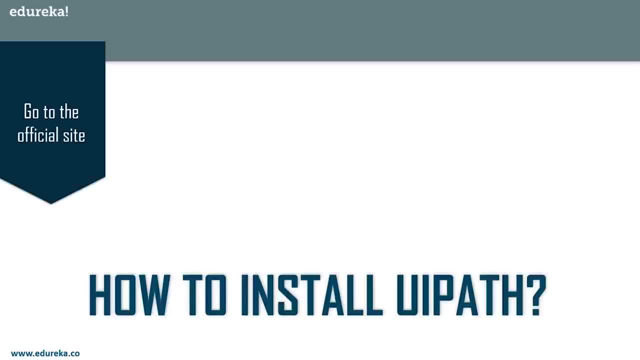 and download the Enterprise Edition to use it at an enterprise level. right after that, What you have to do is, once you choose which edition that you want to go for, you have to fill in your details, like you know: name, email ID, phone number and so on. 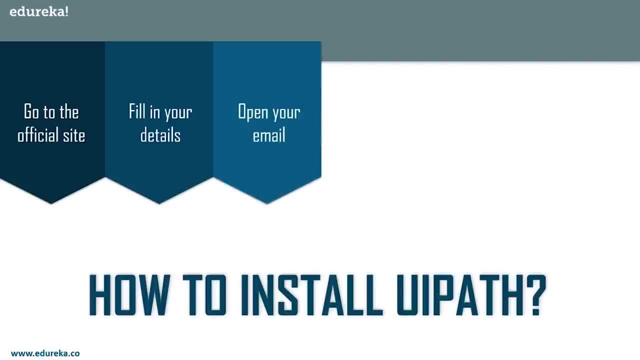 and after that you have to open your registered mail. Now you have to open your registered mail because you know you'll get a mail saying that you know, thank you for installing UiPath Studio. So let me just open that and show you once. so this is the mail. 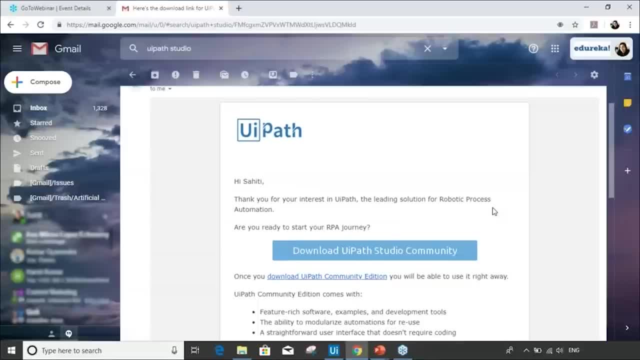 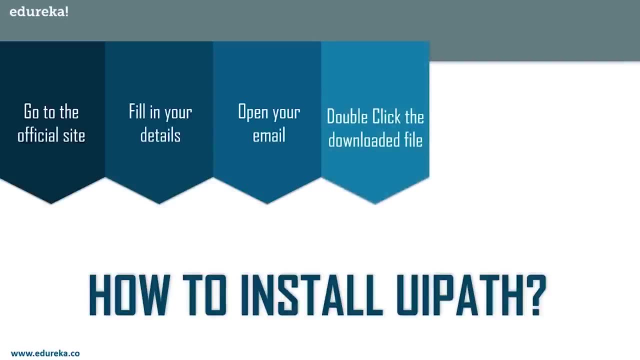 that I had got for that. you know you can download the link. So basically in your mail you get your download link to download the Community Edition. after that you can just go forward and click on the download link. Once you click on the download link. 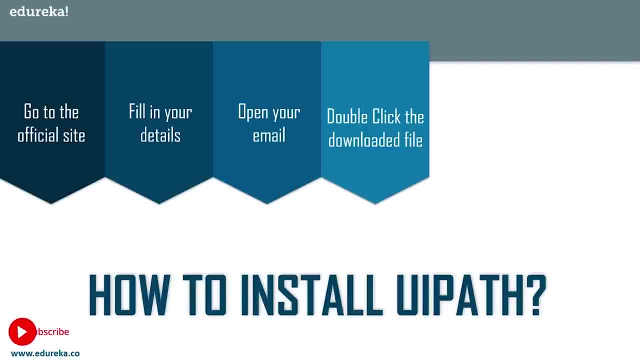 you'll observe that you know UiPath is getting downloaded. So once you think that in it is downloaded, what you have to do is you have to double click on the downloaded file and the setup will initialize. So once the setup initializes, you'll see a dialog box. 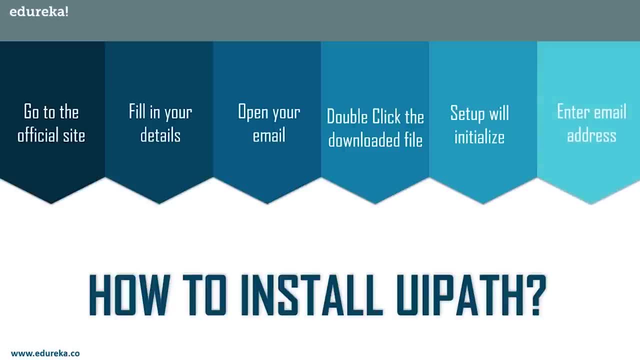 which will pop up. So over there you'll have to mention your email address. that is, your registered email address, and then you're good to go. So once all these steps are done, you will see that you know you have installed UiPath Studio, right. 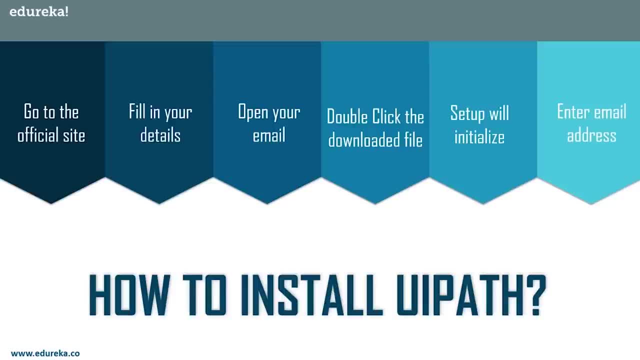 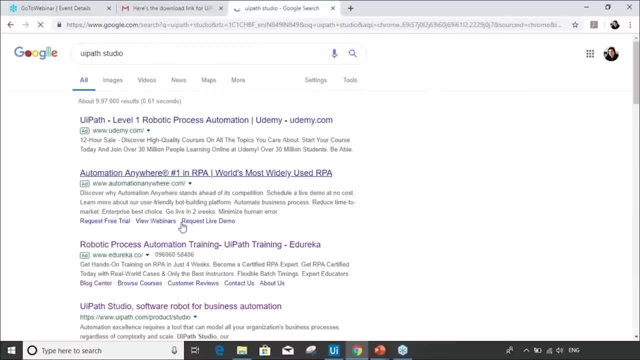 So before I move forward and show you how UiPath Studio looks, Let me just go to the official website and show you from where you can start installing UiPath. So let me just search for it. Right, so we are. this is basically the UiPath official website. 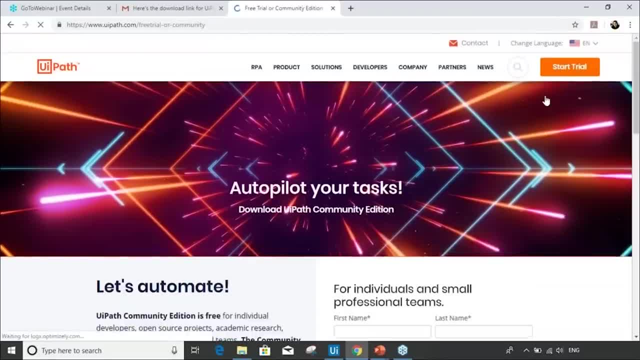 on which you have to go. So we are. what you have to do is you have to click on the start trial button and then you'll get two options, That is, the Enterprise Edition and the Community Edition. So if you have to choose Community Edition, 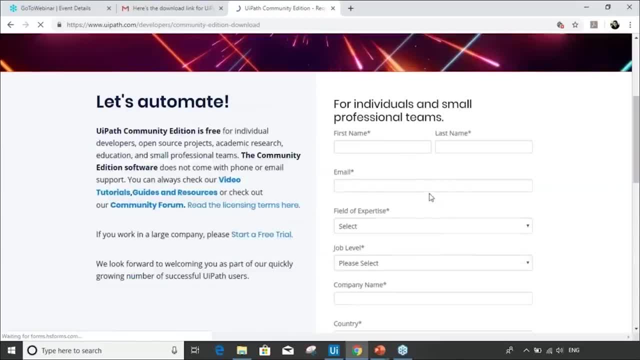 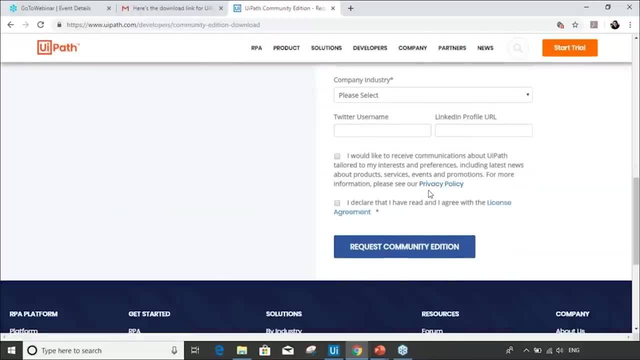 just click on Community Edition and then what you'll do is you'll mention your details like in a first name, last name, email and so on. right now, once all this is done and then you accept the license agreements, You just have to click on request Community Edition. 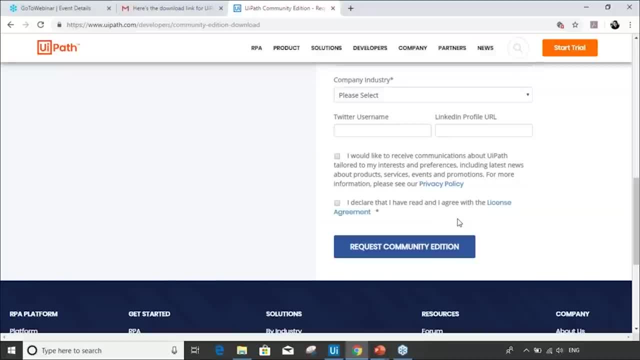 and then you'll get the mail that I showed you before. So once you get that mail, you'll have to follow the next steps, right? So I hope the installation part is clear Now, once UiPath Studio is installed into your system. 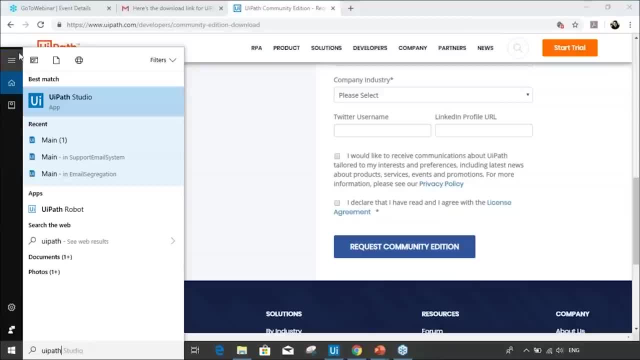 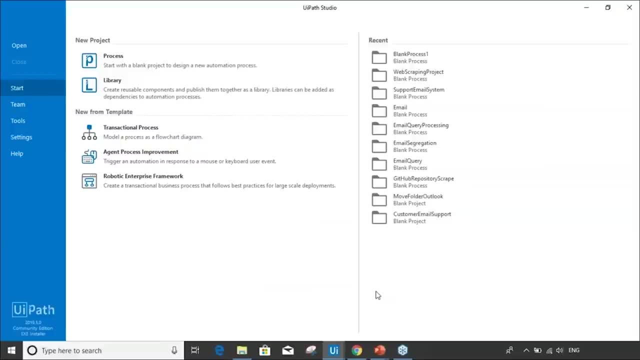 Let me just open and show you how that looks, right? So I'll search for UiPath Studio over here. So let's wait for it to open. So, as you can see on my screen, my UiPath Studio dashboard has opened. So now in the session, what I'll do is that you know. 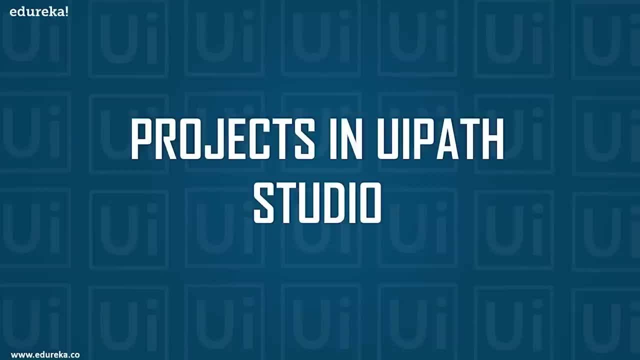 I'll first discuss the projects in UiPath Studio. So there are basically various kinds of projects that you can create in UiPath Studio. So let's discuss each one of them one by one, and then I'll show you in UiPath Studio how you can create a project. 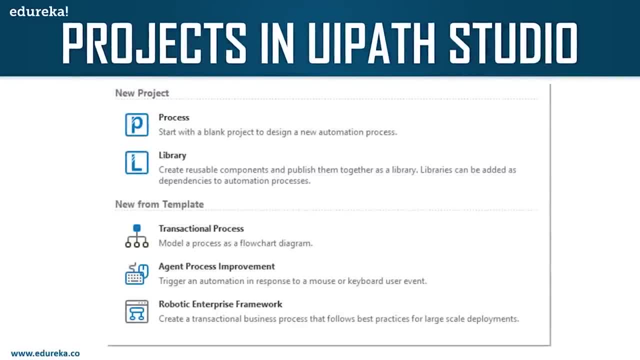 So mainly there are five kinds of projects that you can create in UiPath Studio. That is the process library, transactional process, agent, process improvement and robotic Enterprise framework. So starting with process. so process is basically used when you want to create a blank project or maybe you want to design a blank project inside. 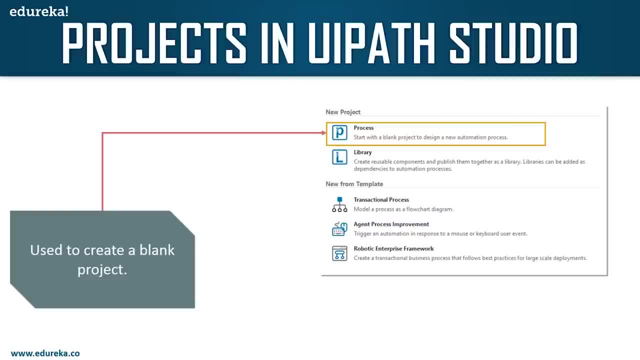 which you wish to add, the automation workflow process. So that is when process is used. So whenever you want to create a blank project, remember that you know you have to use the process. type of project. moving forward, We have the next type of project, that is, library. 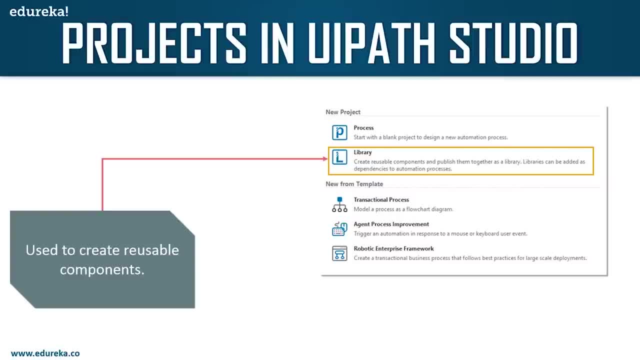 So library is basically used to create reusable components and then publish them together as a library. So what you can do is that you know, maybe you're working in an enterprise and then maybe you will have to use a specific amount of components again and again. 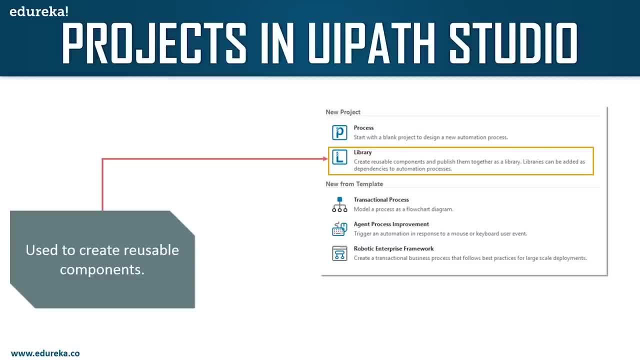 for every kind of automation workflow that you wish to work on, right. So what you can do is that you know you can create those reusable components, publish them together as a library and then everybody can use it again in their automation workflows. So, irrespective of the fact that you know, 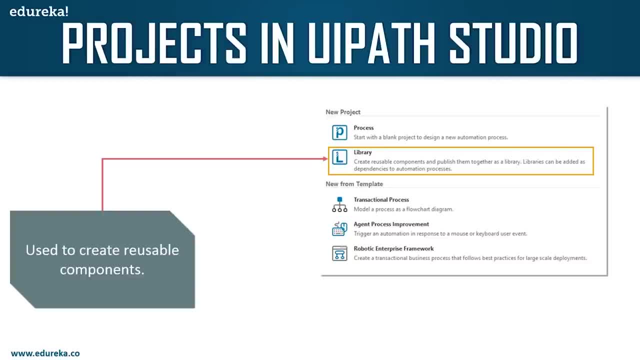 which automation workflow they are creating. they can use those particular reusable components in their workflows, right? So libraries can be also added as dependencies to automation process. So that was about libraries, guys. Now let's move forward with the next type of project, that is, transactional process. 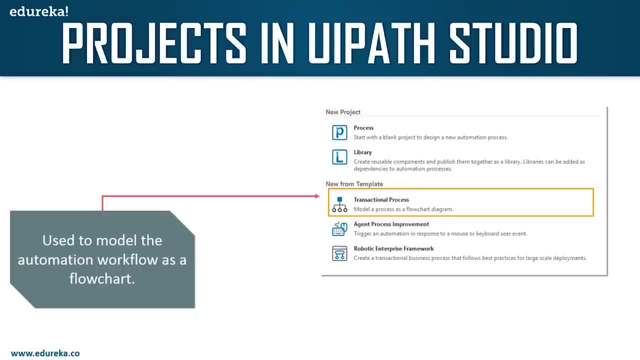 So transactional process, as the name suggests, is basically used to model a process as a flow chart diagram. So whenever you want to model the automation workflow as a flow chart diagram, you can definitely start by using the transactional process. So what will happen is that when you use this kind of process, 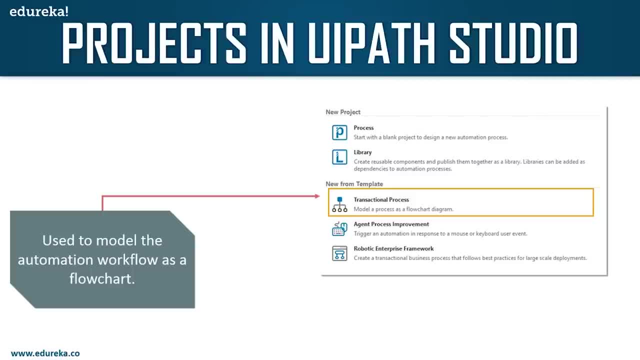 you'll have a clear workflow or maybe a complete object diagram of how your process is working and in which step what is happening. right? So it may happen that you know when you are using uipad. you may want to automate complex stars, right? 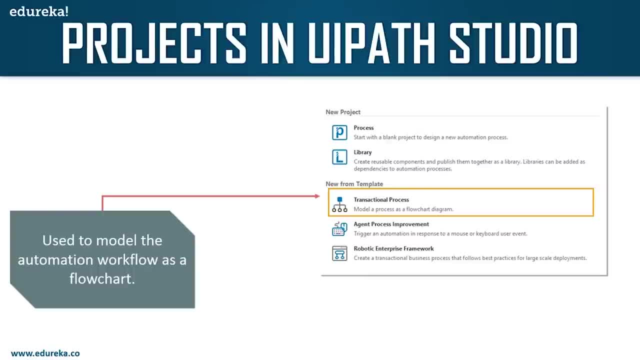 So in such kind of scenarios you can use this transactional process. next, Let's move forward with the next type of project, that is, agent process improvement. The agent process improvement project is basically used when you want to trigger an automation in response to a mouse or a keyboard user event. 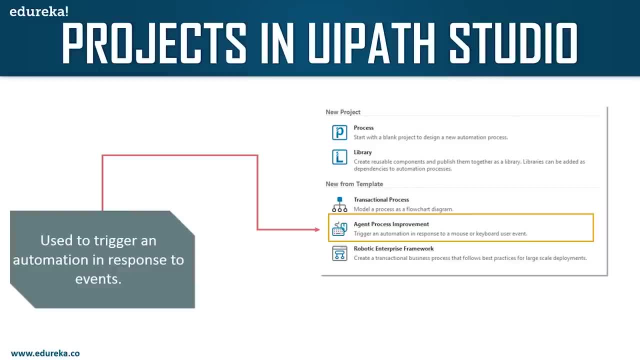 So, whenever you think that a user may have a mouse or a keyboard event and then you want to trigger an automation, Then you basically use this kind of process, that is, the agent process improvement and finally, moving forward with the last type of project, that is, the robotic Enterprise Framework. 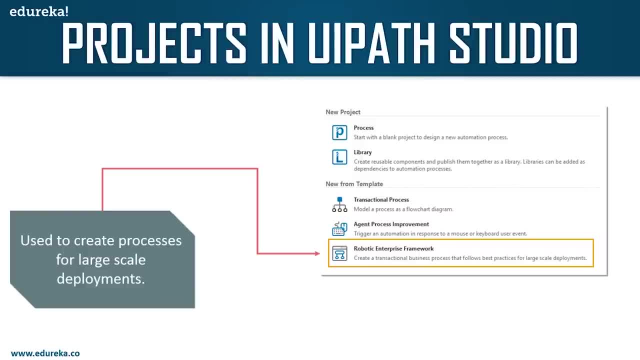 So the robotic Enterprise Framework is basically used to create transactional business processes that follow the best practices for the large-scale deployment. So whenever you think that you know you're working in an enterprise maybe, and then you have to make sure that the large-scale deployment 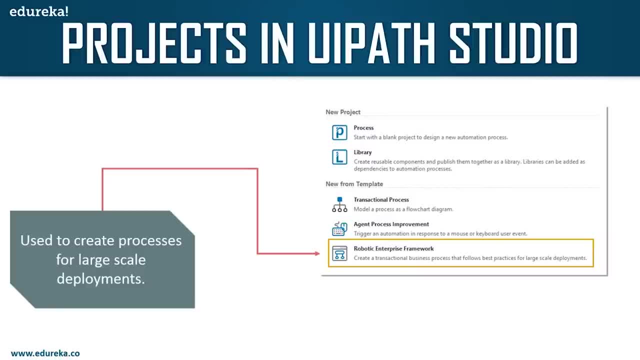 then you can definitely use this robotic Enterprise Framework kind of projects. So, guys, these were the different kinds of projects in uipad studio, that is, process library, transactional process, agent, process improvement and robotic Enterprise Framework. So let's move back to my uipad studio. 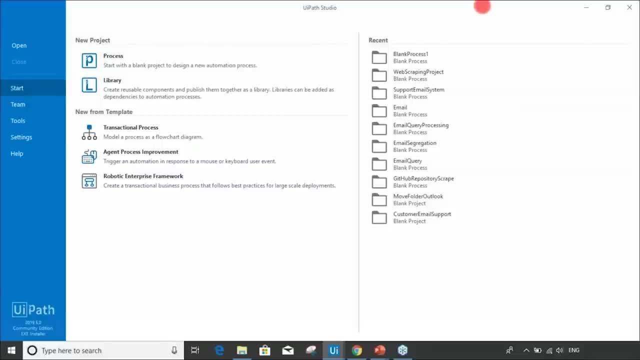 and let me just show you how you can create projects. So the first thing that you see when you open uipad studio is basically different kinds of projects that you can create on the left hand side and the projects that are already created, or maybe the most recent one on the right hand side. 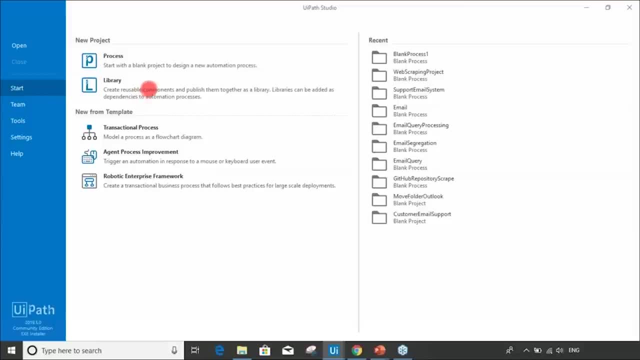 of your studio. So over here, as I discussed before, we have five kind of projects and on my right hand side I have various projects that I had created before. Now to create a project, what you have to do is you have to just double click on any of the options. 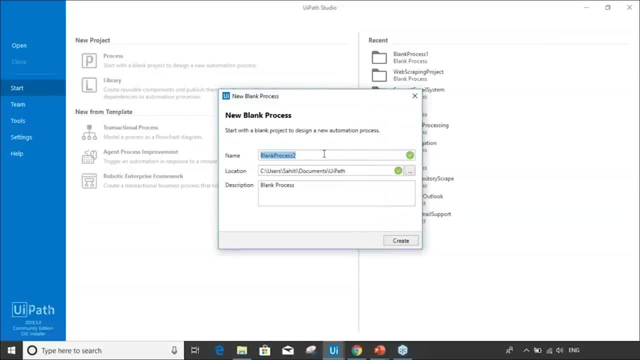 So let's say I want to create a blank process, right, So I'll double click over here. and then let's say we mentioned the name of the blank process. So let's say I mentioned sample, and then let the location be the same and description be, let's say, sample project. 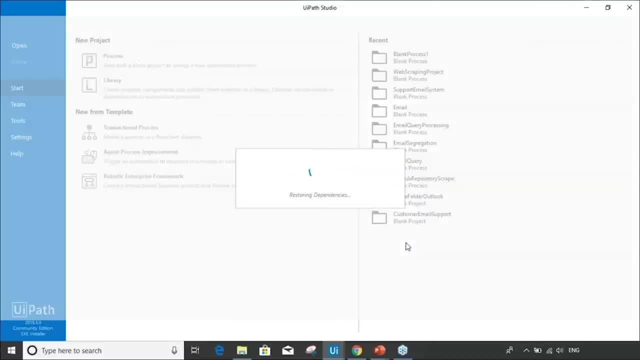 and then I'll click on create. now, Once you click on create, you'll see that you know, automatically a project is getting created with the name sample, right? So let's just wait for that to happen. So, as you can see on my screen, guys, a project is created. 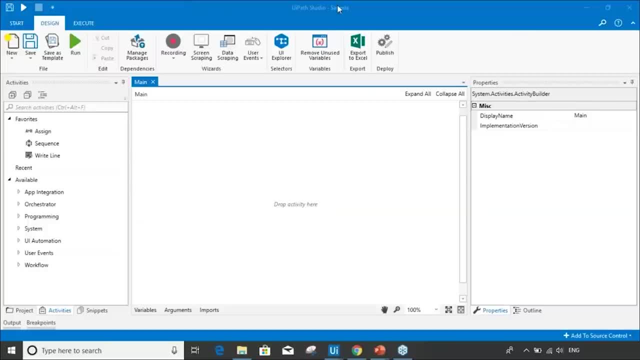 with the name samples. So this is basically you: how you can create a blank process or any kind of project that you wish to now over here. when you open your project you will clearly see that you know you have various kinds of options in the UiPath studio dashboard. 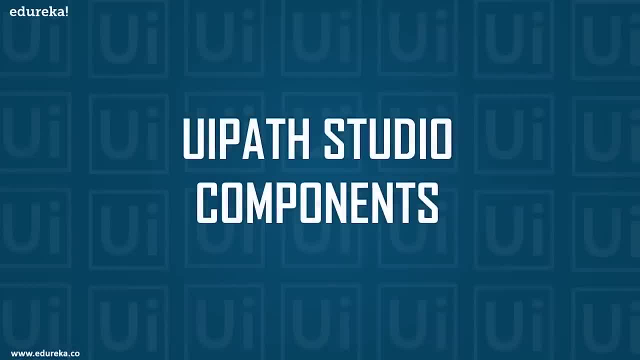 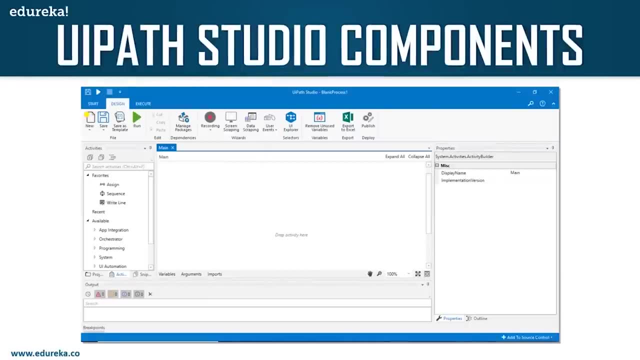 So next in this session on UiPath studio, I'm going to discuss the various components of UiPath studio. So starting with the main components, There are mainly four components that you need to understand about. that is, the ribbon pane, activity pane, output pane and the properties pane. 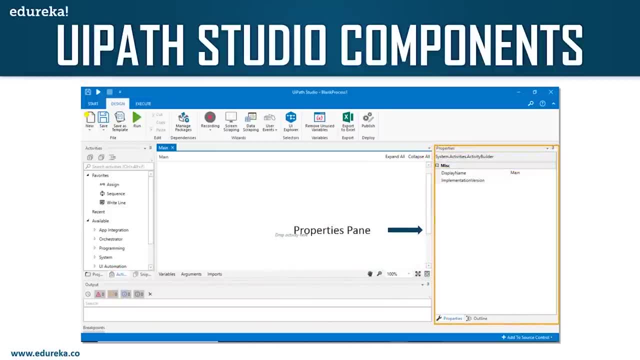 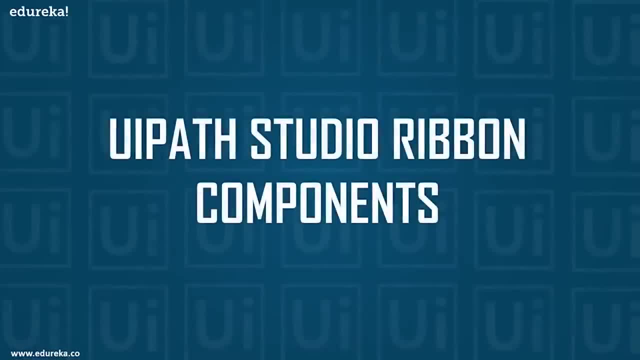 So these are mainly the four panes that you need to understand about in the UiPath studio. So, don't worry, We'll be discussing each one of them one by one. So we'll start with the ribbon pane components. So in the ribbon pane components, 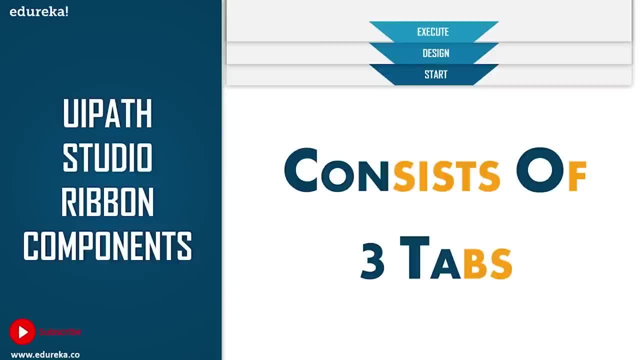 there are many three tabs, if you observe so over here. that's the start, design and execute. all these three tabs have their own options, So we'll discuss each of these tab one by one so that we get a good understanding about the various options in UiPath. 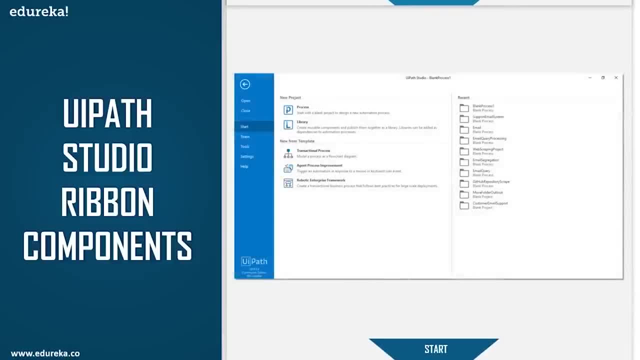 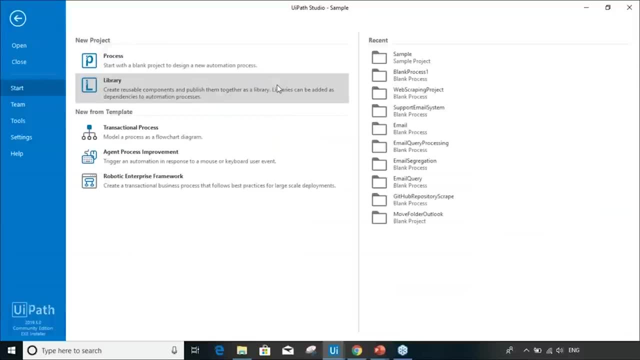 So, starting with the start tab, when you click on the start tab you'll be redirected to the screen where you have various options to create projects and your recent projects. So if I just click and show you, you'll clearly see that you know you'll be redirected to this particular screen. 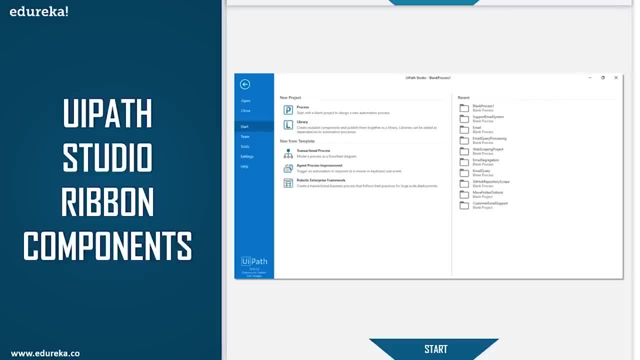 So that was about the start tab. So start tab is basically to redirect you to the starting point where you can either create a new automation workflow or maybe, if you wish to open a recent project, then you can do that right. So that was about the start. now moving on to the design tab. 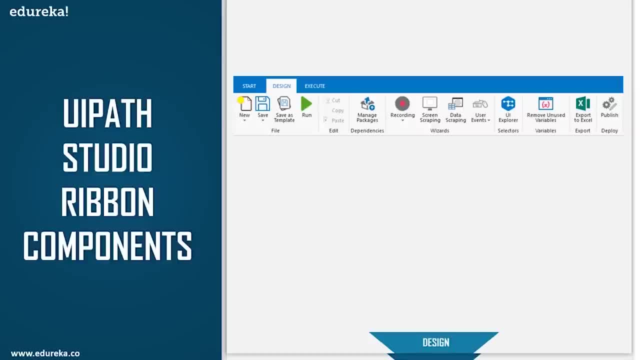 So the design tab has various options, as you can see on my screen, like in a file: edit, dependencies, wizards and so on. So we'll discuss each one of them. So starting with file. So the file tab in the design section is basically used to either create, save and execute the project files. 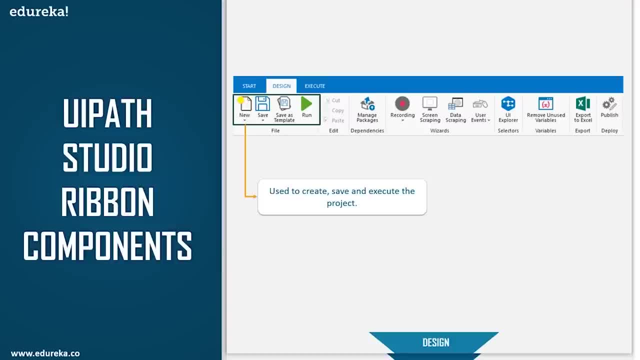 So basically, you can use to you know, create a new main XML file and then either save the existing file, or maybe you can save the file as a template and then also execute your project. Moving on to the edit option, The edit option is basically used to cut copy paste. 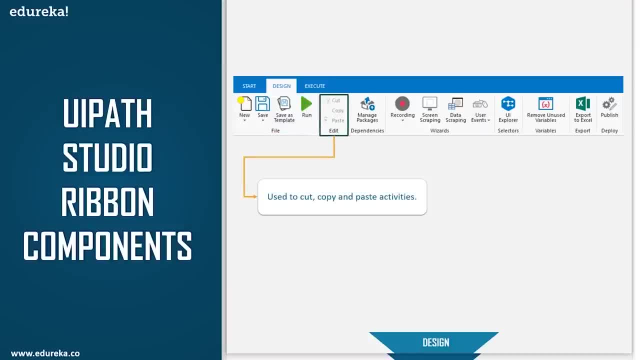 the activities in your automation workflow. So whenever you drag and drop few activities in your automation workflow and maybe you just want to cut some activity, copy it and then paste it somewhere else, and you can definitely do that by using this particular option. The next option that we have is manage packages. 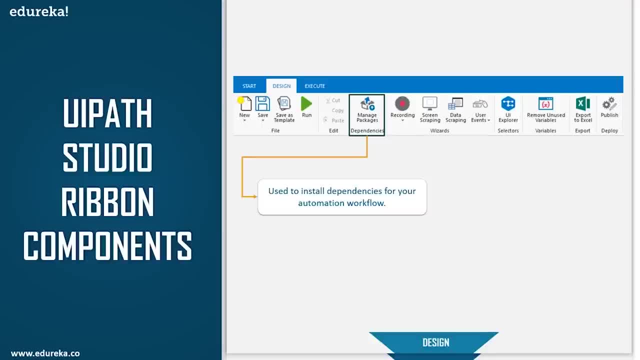 So the manage packages option is basically used to install various packages required for your automation workflow. So, don't worry, I'll show you how that can be done. moving forward, We have the results tab, which have various options for recording. So the recording option is basically used to record actions. 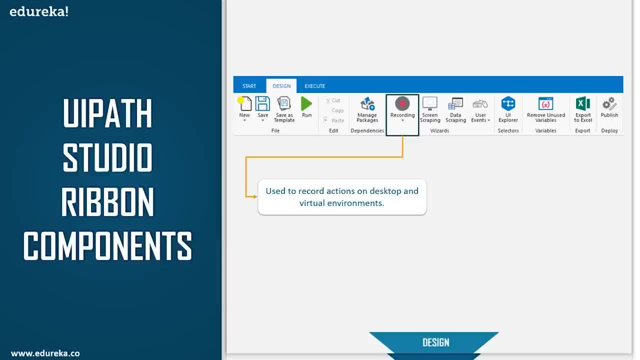 on either the desktop environments or on the virtual environment. Maybe if you just want to record few actions and then if you wish to store that particular recorded actions into your automation workflow, then you can use this option of recording. moving forward, We have the screen scraping and the data scraping wizard. 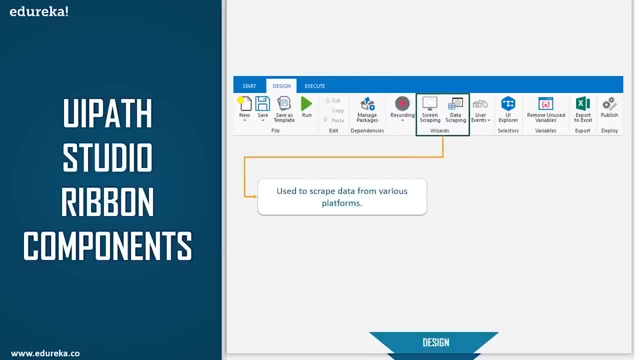 So, as the name suggests, the screen scraping and the data scraping wizards are basically used to scrape data from various platforms, either Whether it be a web page or maybe an excel file, to any kind of application. now, to scrape data, these results mainly use the OCR Technologies. 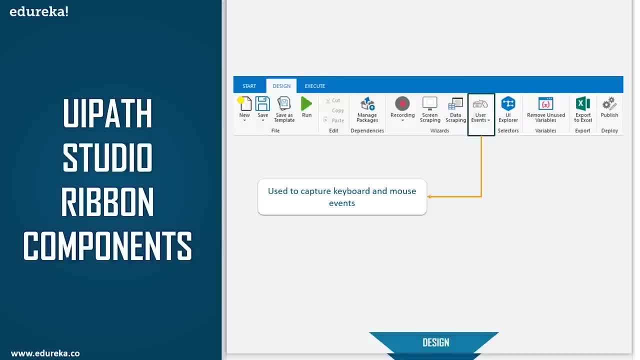 after that in the Wizards tab, We also have the user events. Now these user events are basically used to capture keyboard and mouse events. So whenever you have a user clicking something, or maybe just you know clicking on enter or space bar or maybe tab or any kind of keyboard event that happens, 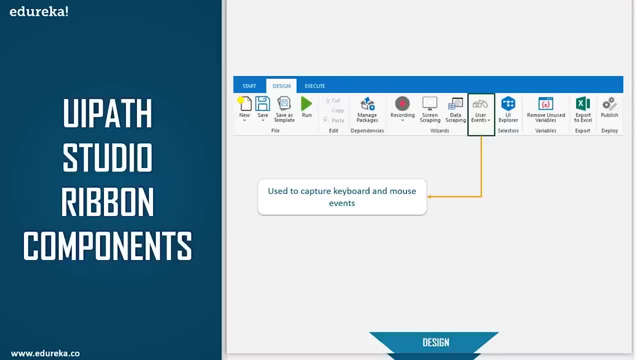 or user event. you can use this particular option to capture that particular event. after that We have the selectors tab. So the selectors tab has the UI Explorer. So that is basically used to. you know, play around with the selectors and then validate them. 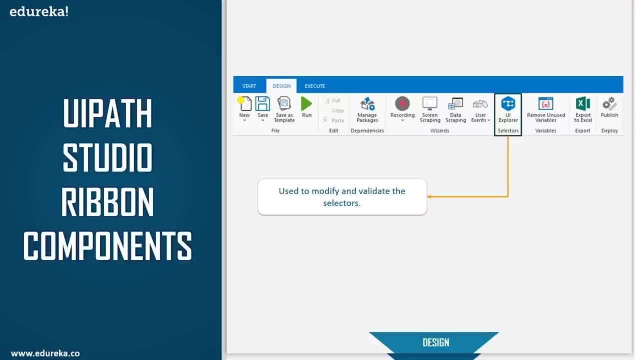 So, for example, if you perform some action on any web page and then automatically few selectors will be stored into your automation workflow, right now you can click on this UI Explorer and then you can make sure what kind of selectors that you wish to choose after that. 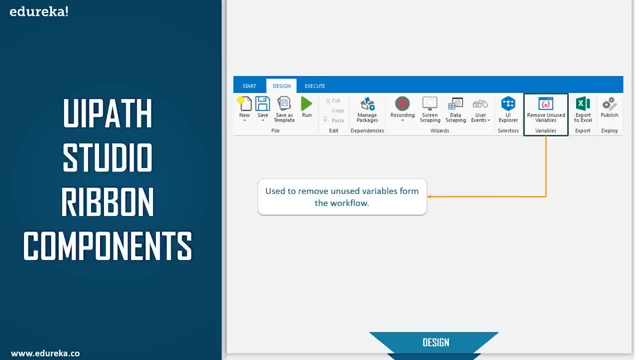 We have the next section, that is, variables. So in the variable section we have remove unused variables. now, in an automation It may happen that you might create more number of variables than you require, right, You can just remove all the unused variables to just avoid any kind of confusion after that. 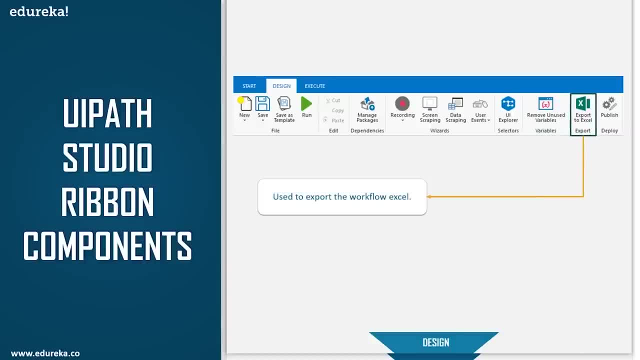 We have the export option. The export option is basically used to export the workflow to Excel. So whenever you want to export your data, or maybe workflow, to Excel, you can definitely do that. And finally, coming to the deploy section, which has the publish options, 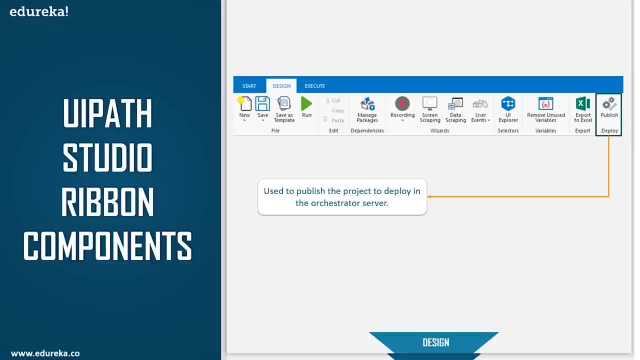 So the publish option is basically used to publish to project to deploy it in the orchestrator server. So when it is deployed into the orchestrator server then that particular project can be implemented on thousands of computers or thousands of pieces, either to automate the front office. 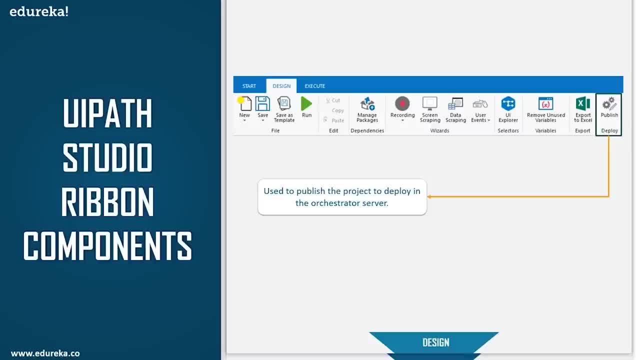 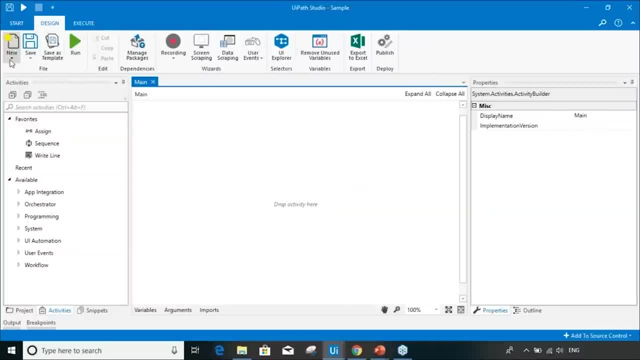 processes or to automate the back office processes. So let me just shift back to my uipath studio and just show you the different tab. So, guys, this is the design section which has these options that I just discussed. So if you click on new, you can clearly see that you know. 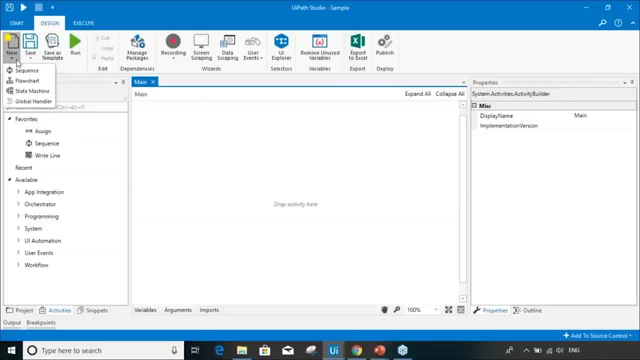 you get various options, like you know: sequence, flowchart, state machine and global handler. So sequence is basically to add a new sequence, flowchart is to create a new flowchart, state machine is to create a state machine kind of process, and so on. After that we have saved, we can either save all the files. 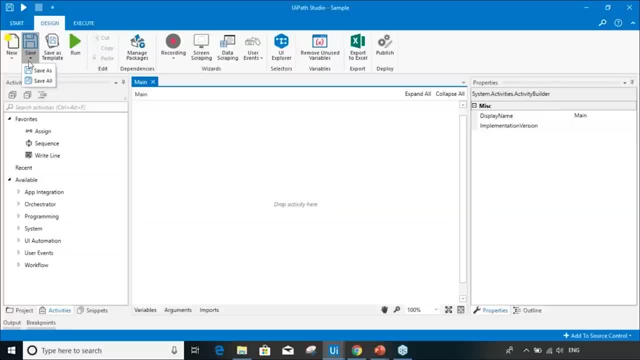 that we have open, or we can just save a specific file with a specific name. Now, in the save as template option, we can basically save a project as a template and then execute it. now as I was talking about the manage packages option, So let me just open this and show you so in the manage packages. 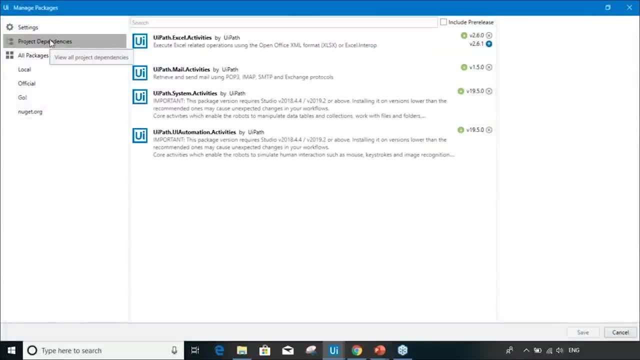 options. when you click on it you'll clearly see that you know. first option is project dependencies. So over here you have all the project dependencies that are used for this particular project. Now maybe it may happen that you know you want to install more dependencies, right? 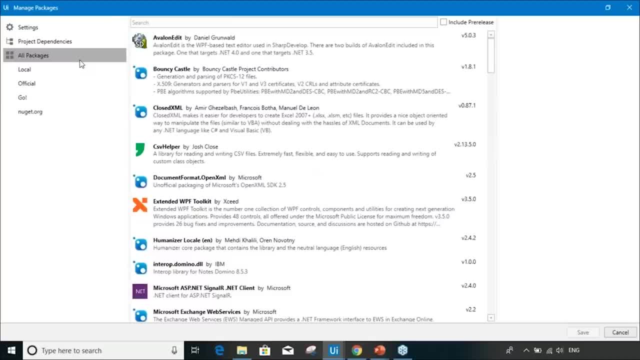 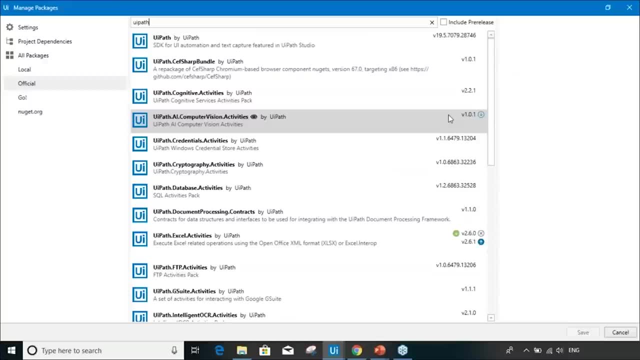 So for that what you can do is you can either go to all packages where you have n number of dependencies which can be installed, or you can go to official, which have all the official packages. So we have. I just search for UiPath. you can clearly see. 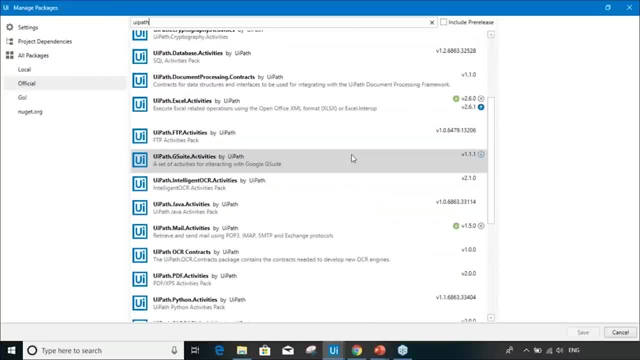 that you know it has so many activities, so you can just install them based on how you want to do So. for example, let's say I want to install the FTP activity, So I'll just click on this arrow and then click on save. 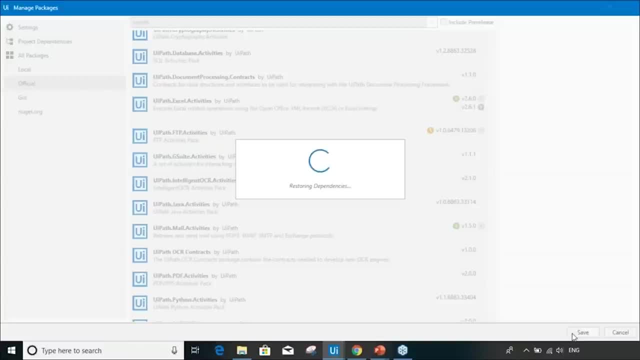 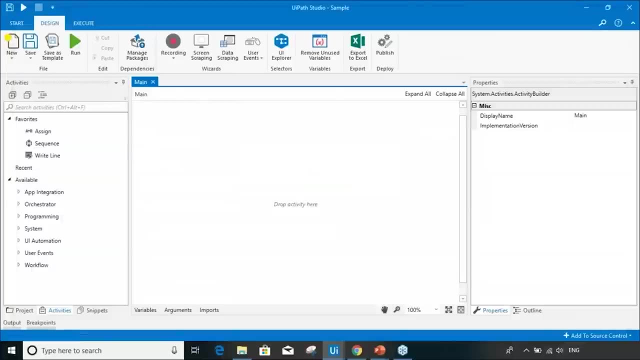 and then you'll see that you know all the dependencies are getting installed and then all are getting restored right. So let's just wait for that to happen. So once it is installed, you can clearly see that. you know you've been redirected to your dashboard. 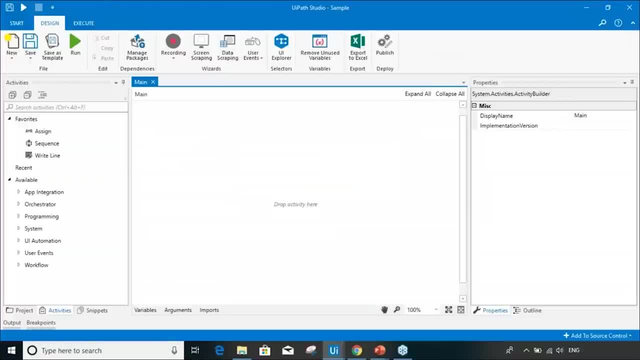 So that's how basically you can use manage packages option to install various kinds of packages. The recording option has various options, like basic desktop, web image and native Citrix. So all these recording options can be used to record ways kind of actions, either on the desktop environments or on web. 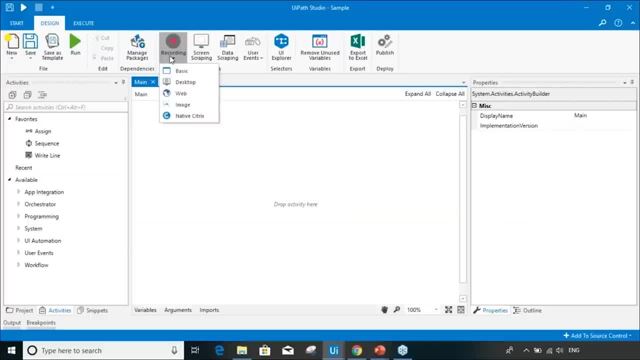 or maybe on an application or maybe on a virtual environment or on the Citrix environment. So if you can use basic to record PC actions, desktop is again used to record, you know, actions happening on an application on the desktop or maybe the user of the mouse, events the web is used. 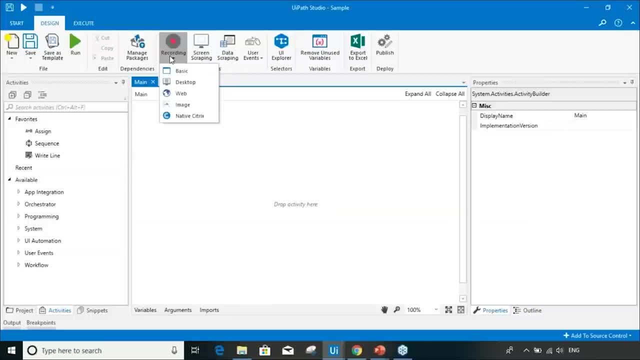 to record actions on the websites, The images used to record actions on basically the virtual environment and similarly, the native Citrix option is used to record actions on Citrix environments. So that's how you can use the recording option. coming to screen scraping and data scraping, 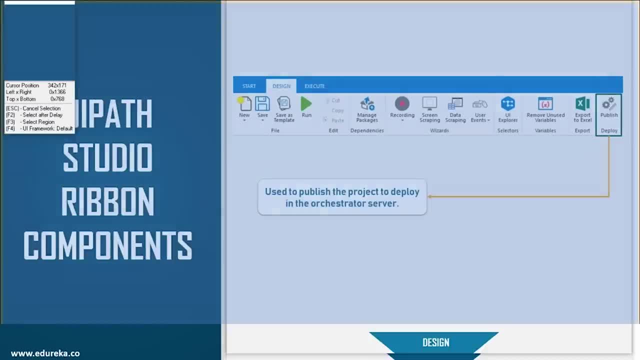 So if you click on the screen scraping option, you'll see that you know the screen will get scraped. So whatever screen that you wish to get scraped, you can just click over that. You can just drag and click over here and then you'll be redirected to this particular option. 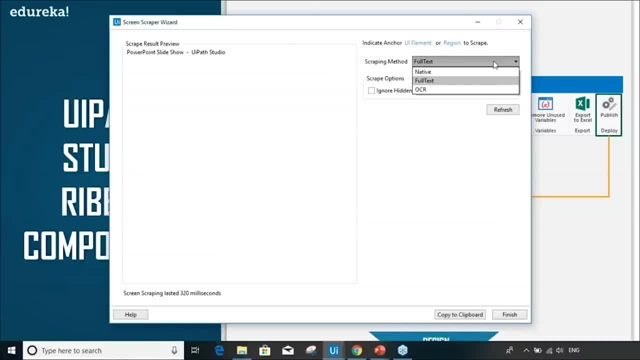 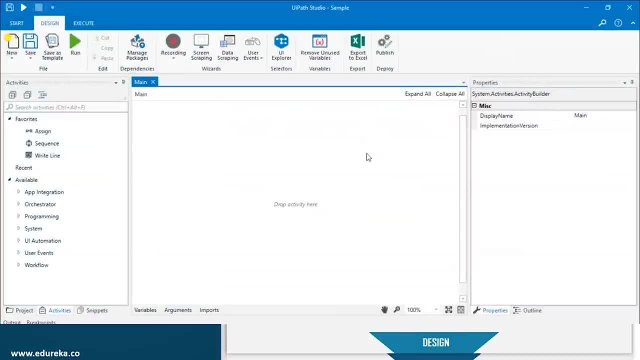 where you know you can just choose whatever scraping method that you want- either full text native or OCR- and then click on finish right. So I'm just going to close this part because I don't want to save it. So, since over there I was talking about full text native- 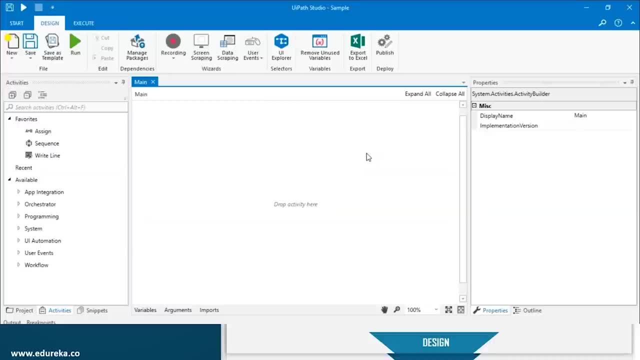 or OCR. what I meant by that is full text- will only basically extract all the text present in the area that you mentioned. the OCR will also extract text from basically the images present in that particular area, and native is to extract data from the Citrix environment. 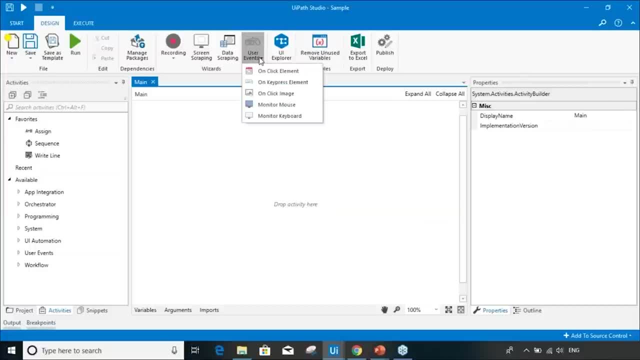 So that was about screen scraping. So, coming to user events, you can just use this option of user events either on on click element on key press element on click image monitor mouse or monitor keyboard. So that was about user event. guys, moving forward, We have UI Explorer, as I told you before it plays. 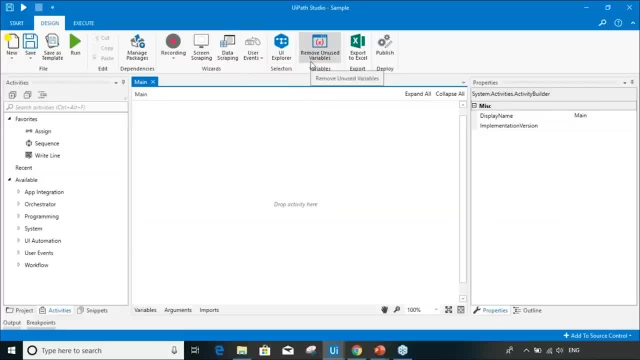 around with selectors comes saying goes with variables. variables are used to remove unused variables. This is used to export workflow to the Excel file and this used to publish. So that was about the design tab, guys. Now let's talk about the third tab of the ribbon pane. 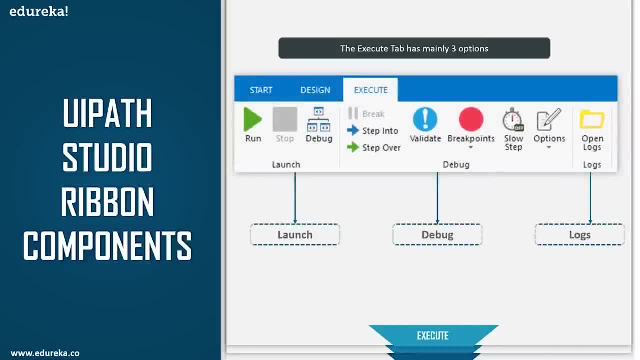 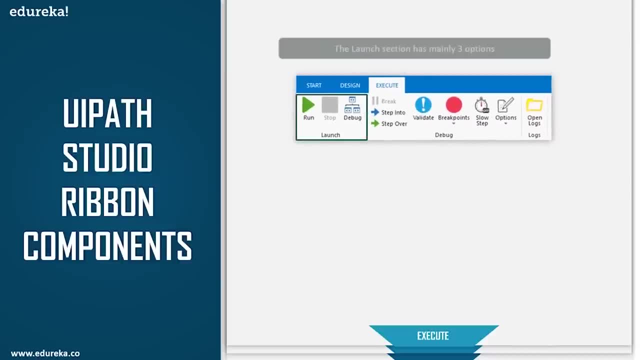 that is the execute tab. So the execute tab has many three options: that is the launch option, debug option and the logs option. So talking about the launch option first, the launch option basically has again three options: that is, to run, stop and debug. So the run option is basically used to execute your project. 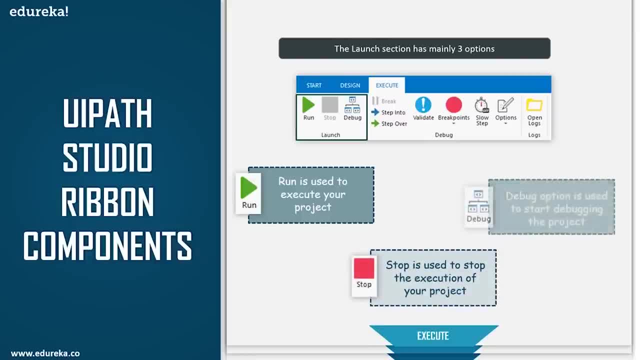 The stop option is used to stop the execution of your project and the debug option is used to start debugging the project. So there's a difference between run and debugging your project. What happens in run is that you know, you just execute it and then finally, you come to know. 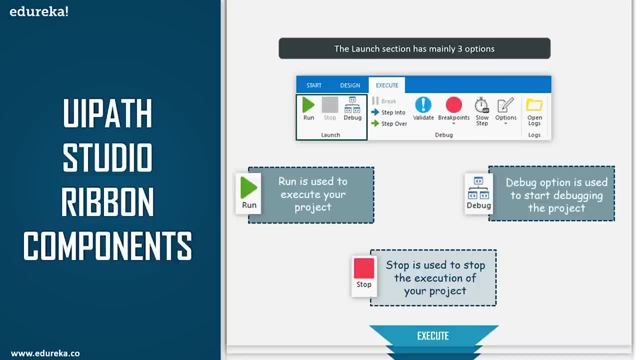 whether there's an error or not. So if there's an error, the execution stops midway and sees that you know, XYZ is the error. But if you choose the debug option, what happens is that each, every step is executed, So the debug option will basically take more time. 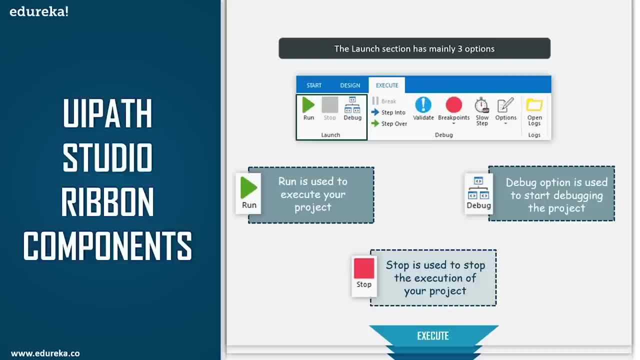 for execution than the run option. So that was about the launch section, guys. Let's move forward to the next section, that is, the debug section. So the debug section basically has five options, that is, the step into step over, validate, breakpoint, slow tap and options talking about step into step over. 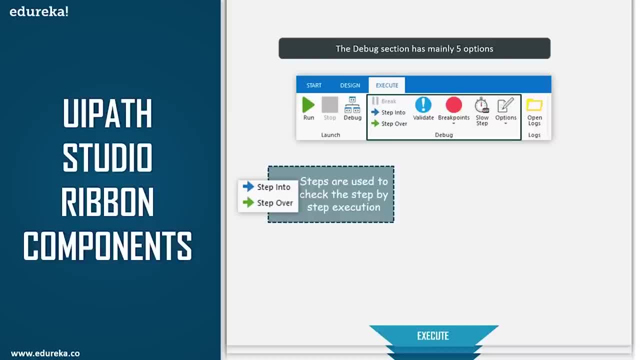 So the steps are used to check the step-by-step execution. For example, let's say you know we have a complicated workflow and then you want to check the step-by-step execution to understand where it is going wrong. Then you can use this particular option. apart from this, 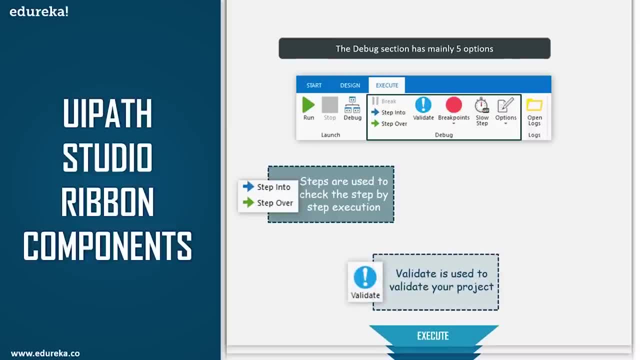 We also have the validate option, So the validate option is basically used to validate your project. after the validate option, We have the breakpoints, So the breakpoints are basically used to define a breakpoint while debugging the project. So maybe you want to define a breakpoint. 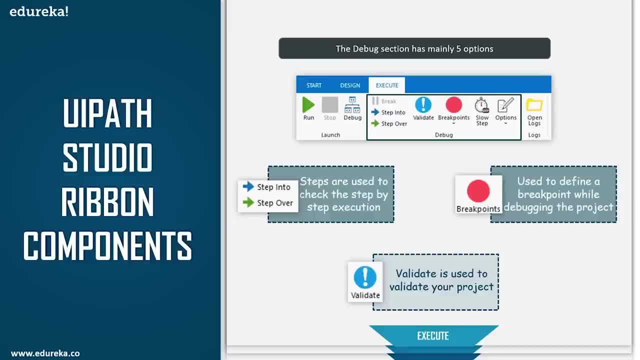 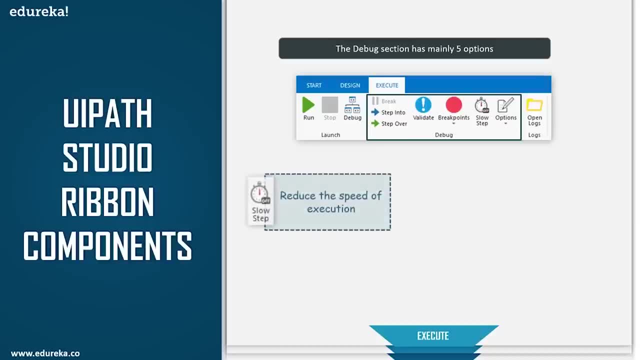 so that you understand: you want to stop your execution right there and then maybe you wish to check something, or maybe, if you wish to change something, you can definitely do that by using breakpoints. after that We have the slow step option, So the slow step option is basically used. 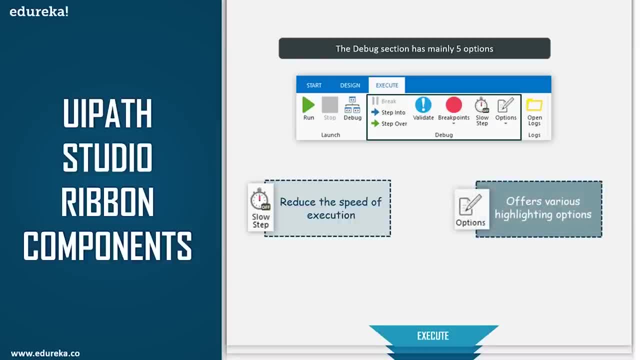 to reduce the speed of execution. And finally, we have options. So options basically offers various kinds of options to highlight a few tasks. So that was about the debug Section, guys. now let's move forward and see the final section, that is, logs. 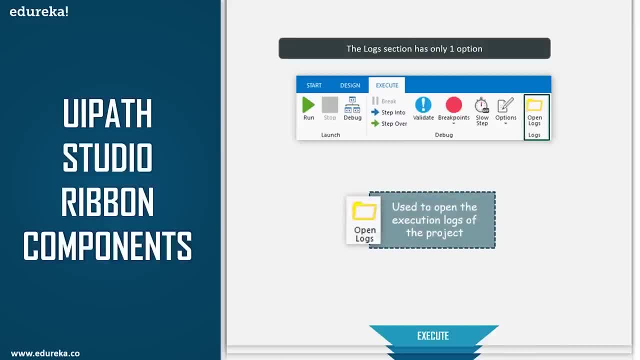 So the logs basically have only one option, that is, you know, the open logs option. So the open logs option are used to open the execution logs of the project, right? So basically, if you have any error then you can also go back and check in the log. 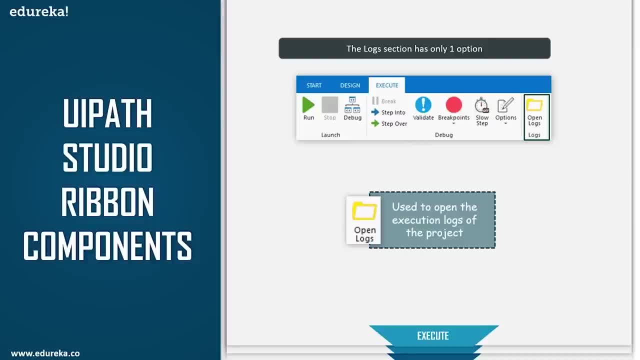 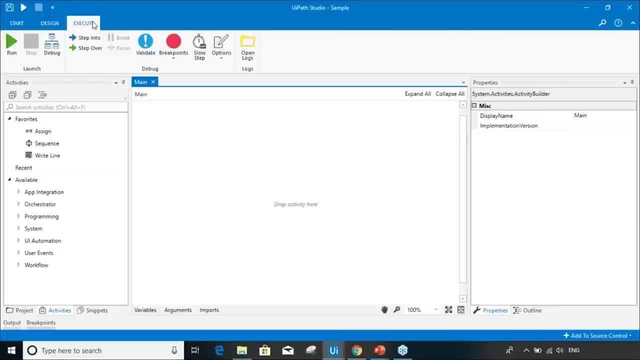 where you're facing the errors. So now let me just shift back to my uipath studio and show you these options. So, as you can see on my screen, these are the ways options, that is, the launch, debug and logs. Now, apart from that, if you wish to know more, 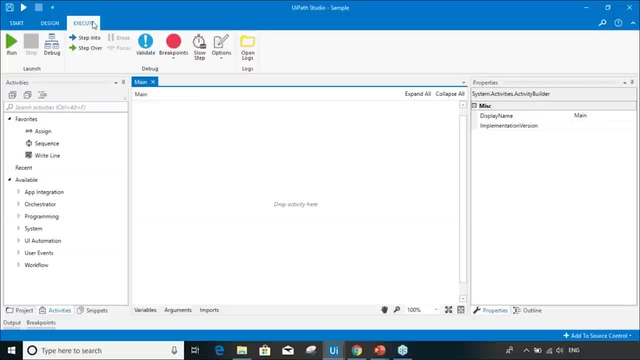 about how you can use this options, then you can refer to my session on error handling in uipath, where I've talked in detail of how you can use various activities and these options to debug your project. So that was about the ribbon tab guys. 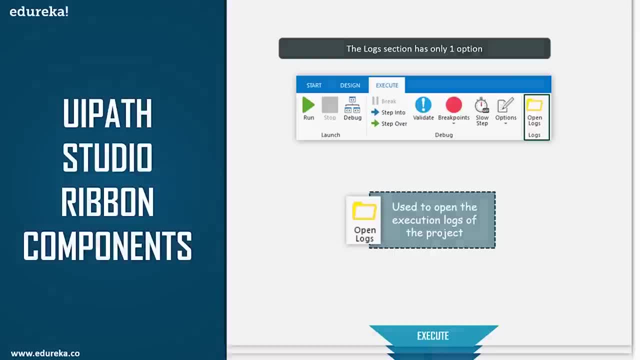 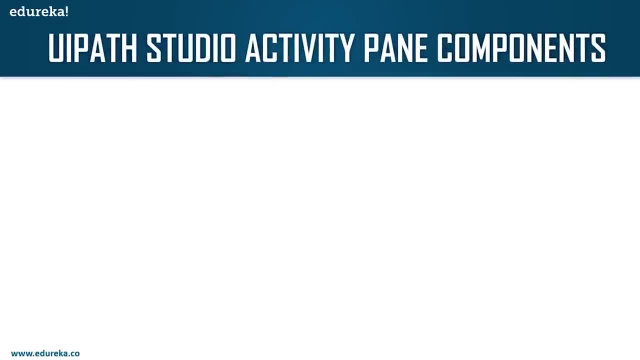 So with this we come to an end, to the components of ribbon tab. Now let's move forward and discuss the next pane, that is the activity pane. So the activity pane also has various components. So that is mainly app, integration, orchestrator, programming system. 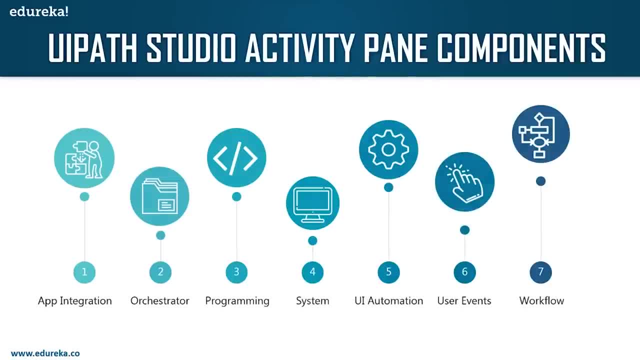 UI automation, user events, workflow. So all these seven components are present in the activity pane. now, before I move forward and talk about these options, Let me just tell you that activity paint is one of the main paints of the uipath studio. that is because it has all the activities. 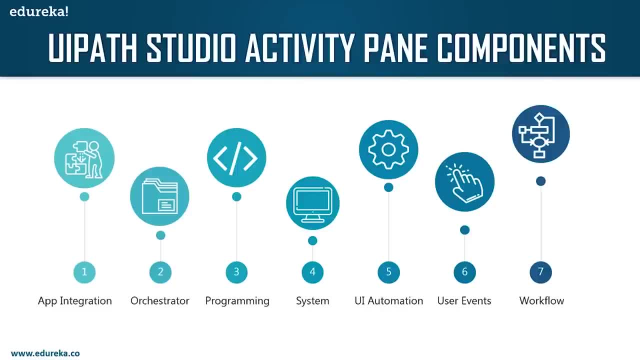 that are required to automate a workflow. So in uipath studio you don't have to write anything or you don't have to sit and code anything. You just have to drag and drop activities to perform any kind of task. So for example: 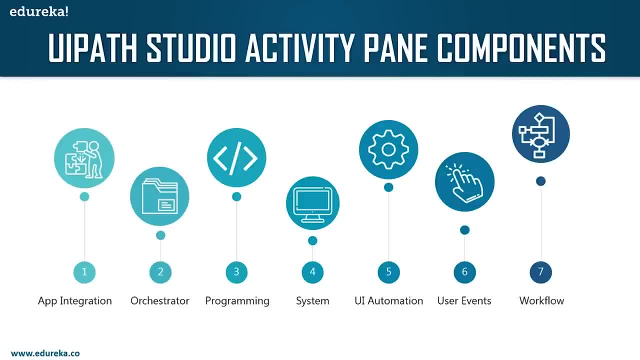 let's say, you want to play around with the for loop, right? So you want to run a loop, So, and that is a for loop that you wish to, so you don't have to sit and program it, You can just drag and drop the for loop activity. 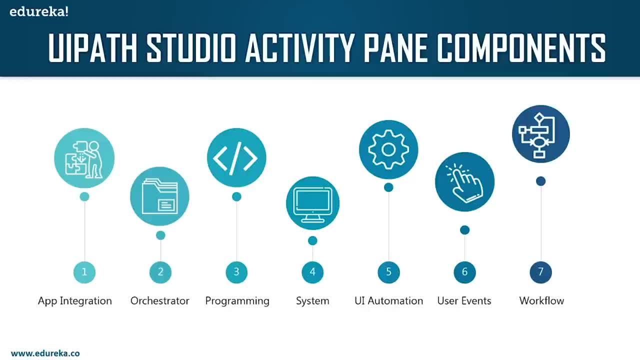 from the activity pane and then you're good to go right. So the components that you can see on my screen are basically the headlines of Wales activities present in the uipath studio. So let me just shift back to my uipath studio and show you. 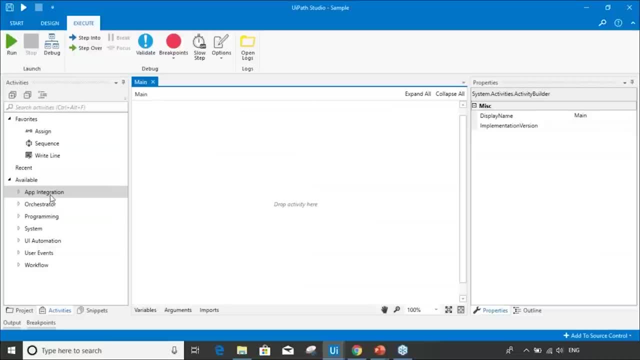 so, as you can see on my screen, these are the components that are present, that is, app integration, orchestrator, programming system, UI automation, user events and workflow. So if I just click on app integration, you have various options to integrate apps, like you know: CSV, Excel, FTP, mail and so on. after that, 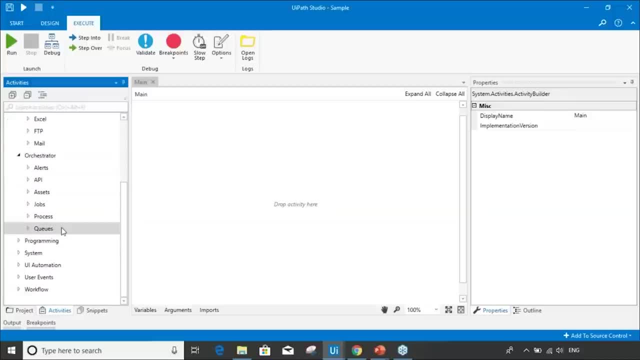 in the orchestrator part, we have various options like alerts, API assets, job processes and queues. So basically these options will again have various activities beneath them after that, coming to programming, So the programming option will basically have collection, data table, debug, execute, generic values and string. 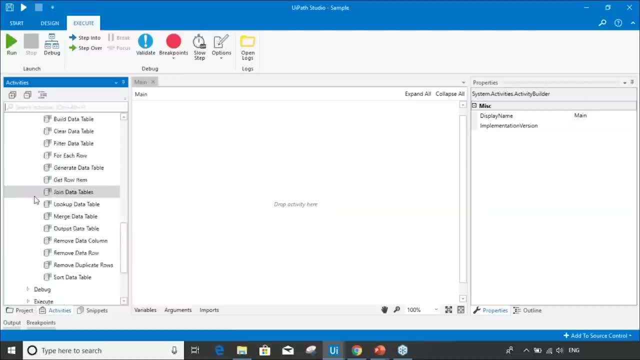 So we are. you can either create a data table or, you know, add a row, delete a row. Maybe you can add a collection, delete a collection and the debug something, and so on. in the system option You have various options for like application clipboard dialogue. 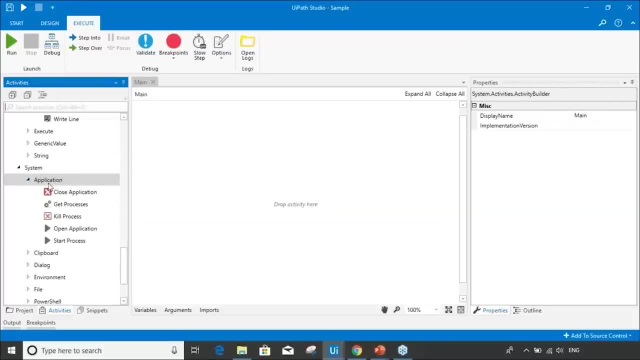 environment, file, partial and VB scripts and the application. you have closed application, open application and so on. So, basically, activity pain is really simple, guys. It has various options for different kinds of activities. Now, coming to UI automation, You have various options like browser element image, OCR text. 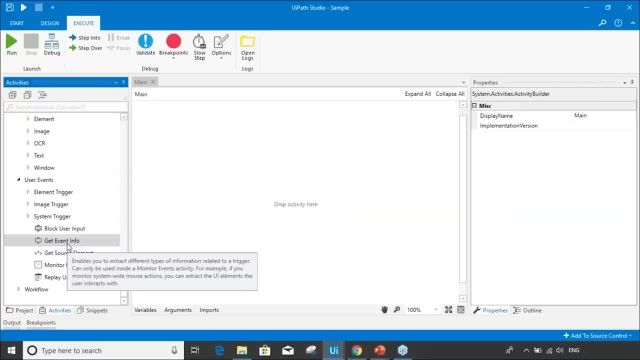 window. coming to user events: to user events has various options like element trigger, image triggers, system trigger and so on. and coming to workflow, The workflow has various options, like in a flow chart, checkpoint, control, error handling and so on. So basically, these are ways, options that you have an activity. 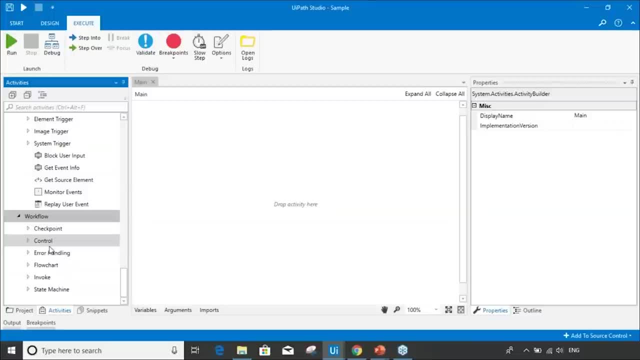 pain and beneath them. also, there are ways, activities present, so you can drag and drop any activity based on whatever your need is. For example, let's say I want to drag and drop a flow chart. I can just drag and drop it into my screen. 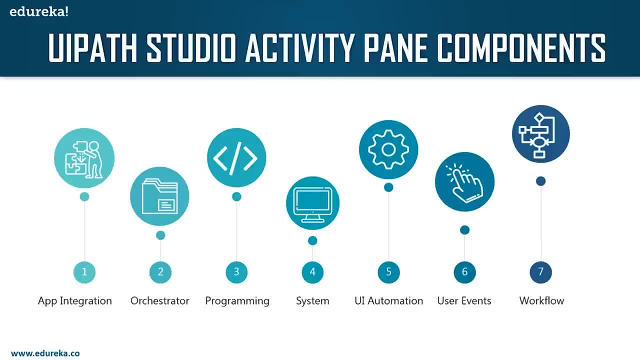 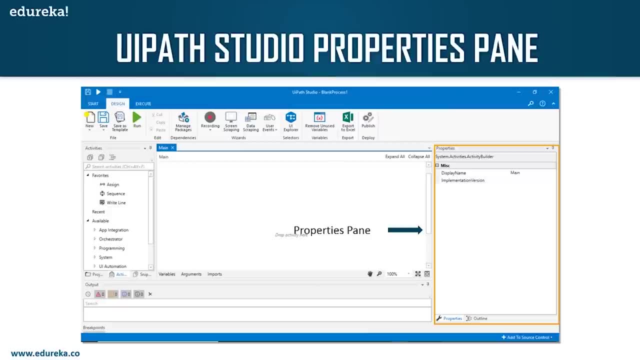 and then I can start using it. So that was about the activity pain, guys. Now let's move on with the next pain, That is the property speed. So every activity will have its own properties, right? For example, let's say in the flow chart activity. 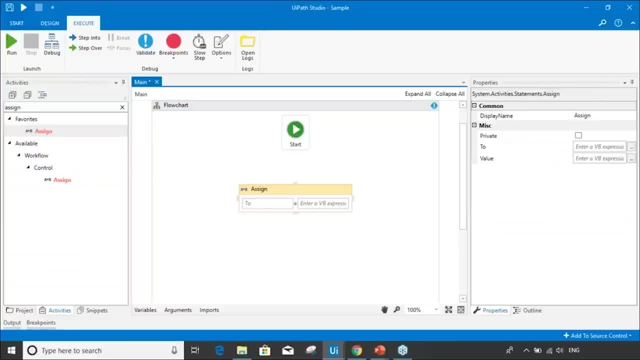 if I search for an assign activity and then drag and drop it over here now, this particular assign activity will have its own properties, that is, the two section and the value section, and the flow chart itself will also have its own properties. right So to configure properties of each. 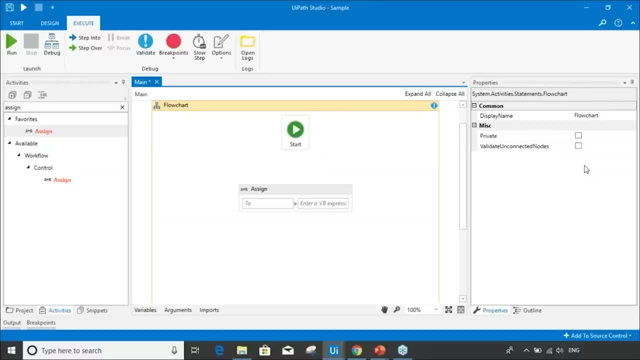 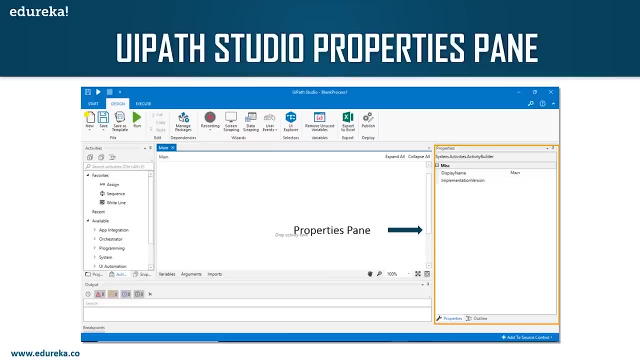 and every activity separately and then make sure that you know there's a coordination between all the activities in the automation workflow. We can use this property section. So that was about the property section, guys. Now let's move forward with the final pain of this dashboard. 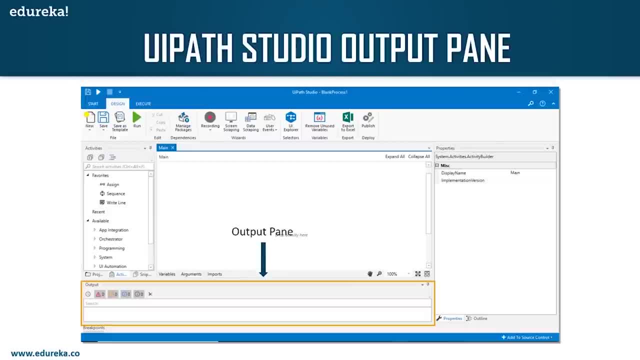 That is the output pain. So the output pain, as the name suggests, is basically used to view the output of your automation workflow. So once you execute your project, what you'll see? that you know the sample project has started executing. and once you see that in it has executed, you see a final message. 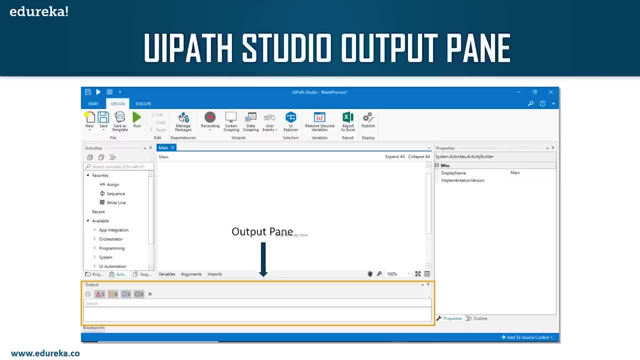 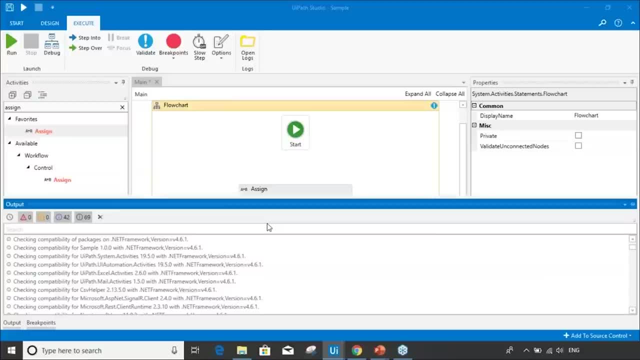 saying that you know sample project has been executed. right, So basically that's how you can use the output pain. Now, the output pain also shows the compatibility of various packages, maybe project dependencies, also shows where are the breakpoints and so on. right, So that was about output pain, guys. 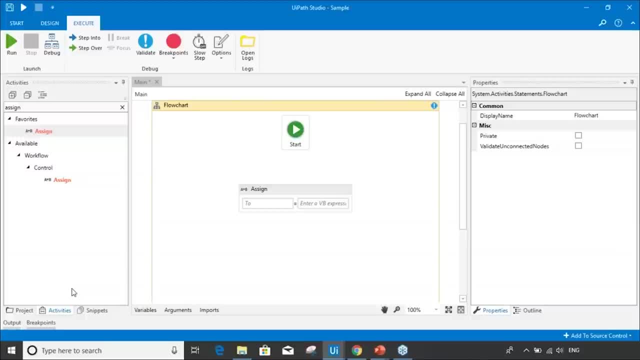 So the output pain is basically used to just view the output of your automation workflow. So, guys, that was about the different paints in uipath studio. I hope you know. you've understand what are the different paints in uipath studio. So let me just show you how you can drag. 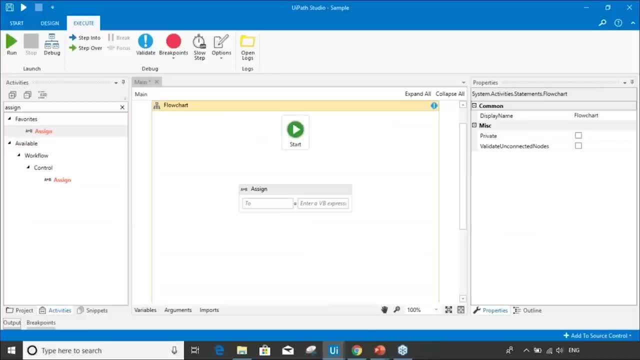 and drop activities in the uipath studio and how you can use them, so that you understand and get started with uipath right. So let's say you know we want to find out whether a number is even or odd, So what will be the condition for it? 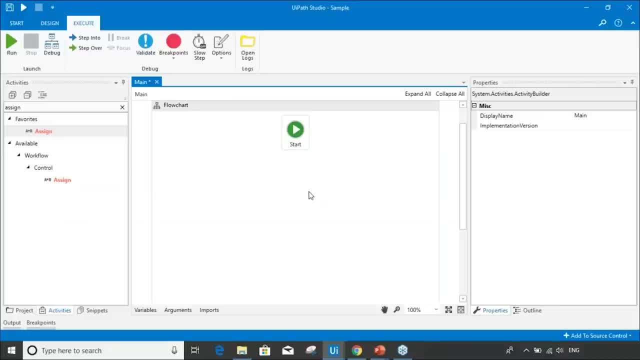 So first what we'll do is basically we'll get the numbers to be entered. Let's say you know the first number is 596.. We know that's even. so let's just prove that you know it's even and the second number will put in two. 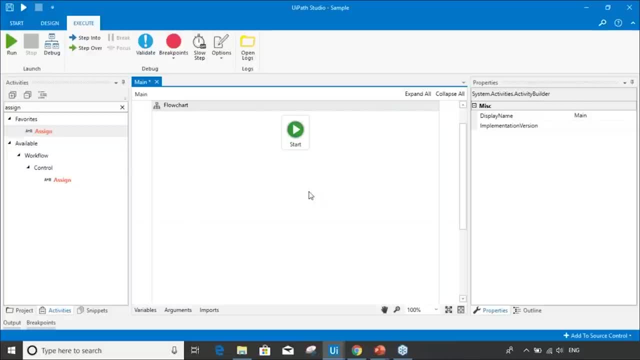 Now, what we'll do is that we'll divide first number by second number. if the remainder is zero, then that means it's an even number, But if the remainder is one, then that means it's an odd number, right? So let's just do the same. 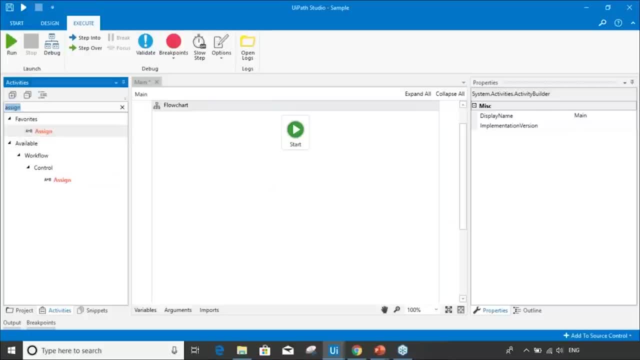 So I'll just use the flow chart that was initially there. Now, what I'll do is that you know I'll drag a sequence. So sequence is basically to put in all the automation steps into one flow, right? So I can just either rename the sequence also. 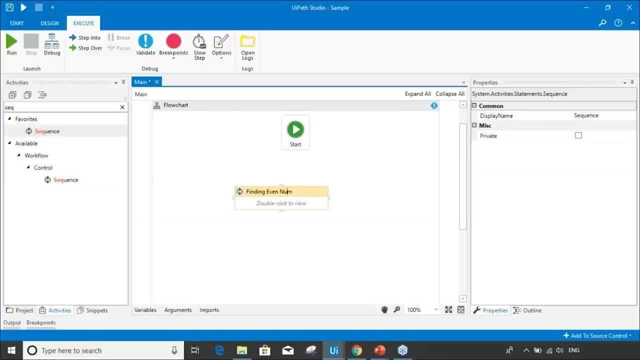 Let's say, you know, finding even number. After that, what I'll do is I'll double click over here and then I'll start dragging and dropping the activities. Now, initially, what I said was that you know I wanted to input a number, right. 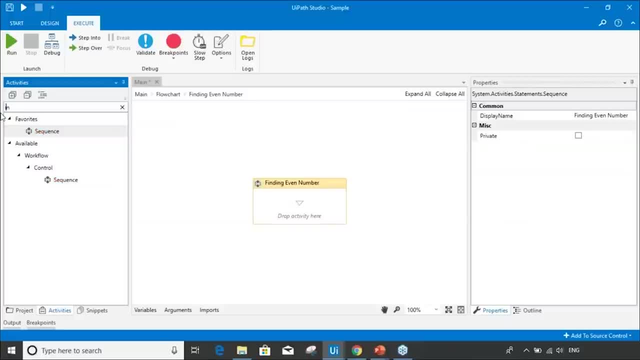 So to input a number you'll have to ask the user for the number right. So for that you'll drag and drop the input dialog option and then you'll mention the title. So let's say you know first number And that's in the label. 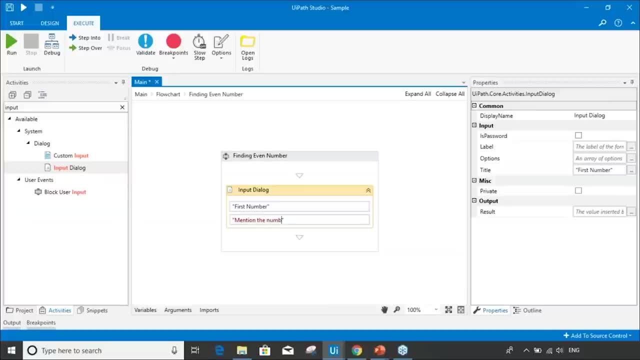 I'll mention the number. Now, what I'll do is I'll store the output of this particular input dialog in a variable. So for that I'll create a variable. So to create a variable, what I have to do is I can either right-click over here: 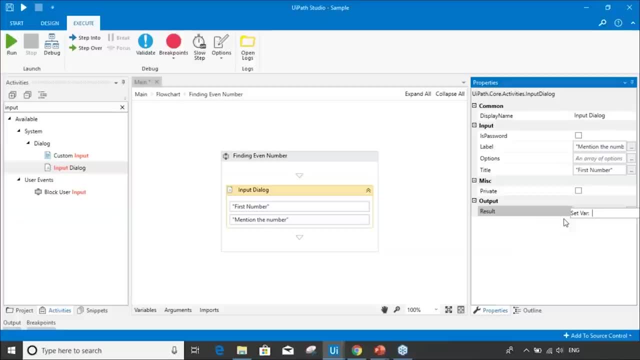 and choose the option of create variable, or I can either use the keyboard shortcut control K and then mention the variables name. So let's say I mentioned the variables name to be number one Now. after that I'll again drag and drop an input dialog. 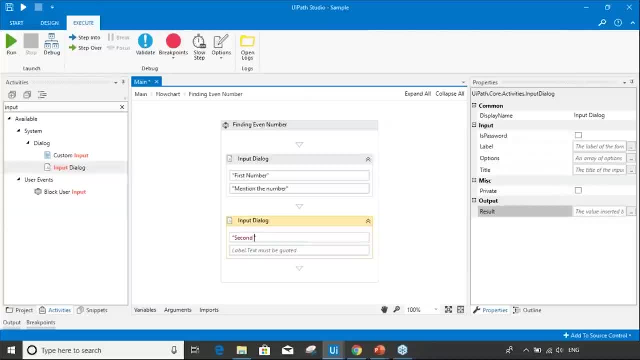 and let's say we mentioned the title to be second number. And let's say we mentioned the text label to be again mentioned, the number Right. So over here again I'll create a variable. So for that I'm pressing on control K. 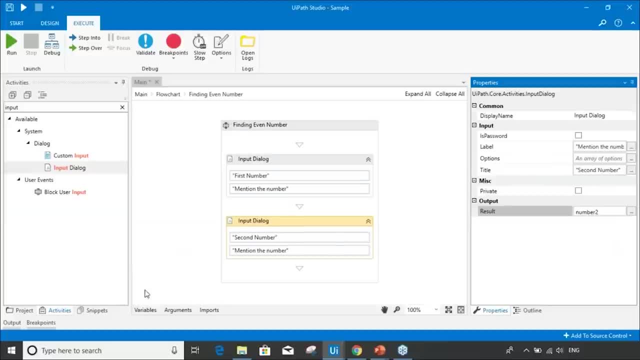 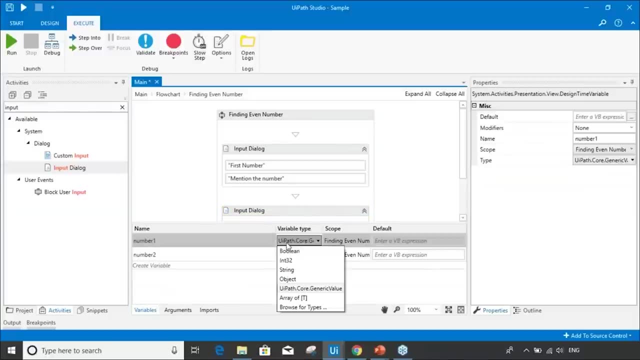 and then I'll mention the variable name, Let's say number two. right, You can just check your variables in the variable Spain. So, as you can see, my variable type is generic, So I'll just change that to end. So when you click over here, 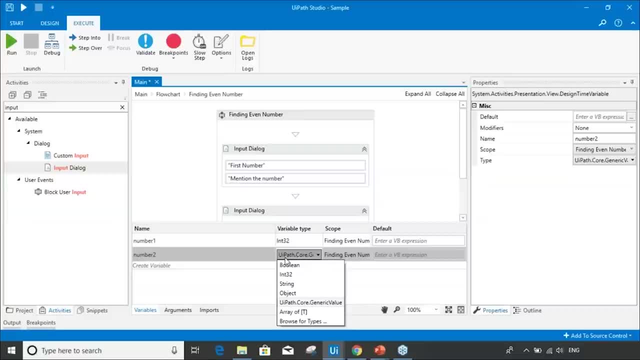 you'll see the most popular used variable types over here. I've got various options, But yes, I'm clicking on end because my number is of integer type. right after that, What I'll do is I'll drag and drop an, if else loop. 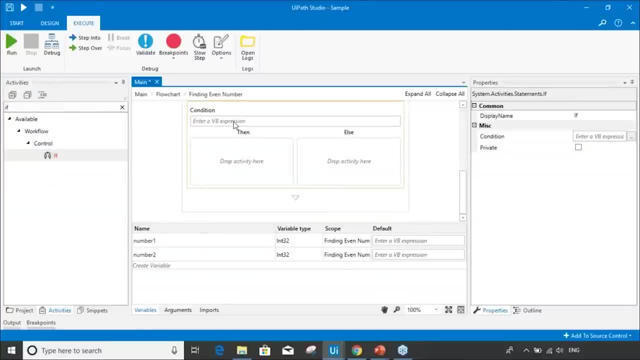 So I'll search for if I can drop it over here, and then what I'll do is I'll mention the condition. So let's say I mentioned number one, mod number two equal to zero. So what I'm doing is that you know, if number one divided by number two gives a reminder zero, 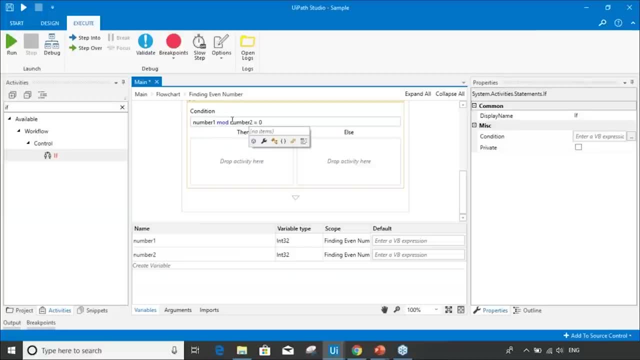 then we'll say that you know it's an even number. else will display that you know it's an odd number. right now, Once you mentioned the condition, let's say: you know we want to just display the output. So for that, what I'll do is I'll search for a message box. 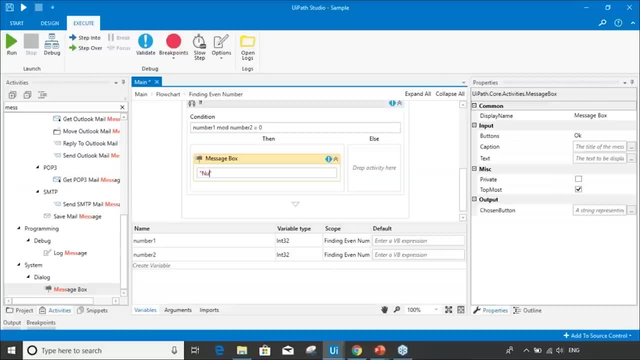 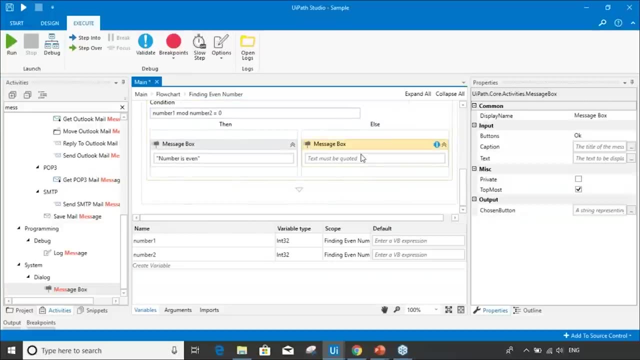 Drag and drop it over here. And let's say I mentioned the text, number is even. and let's say, you know, if it is not even, then we want to display the message. number is all. It's odd. So I'll just mention: number is odd. 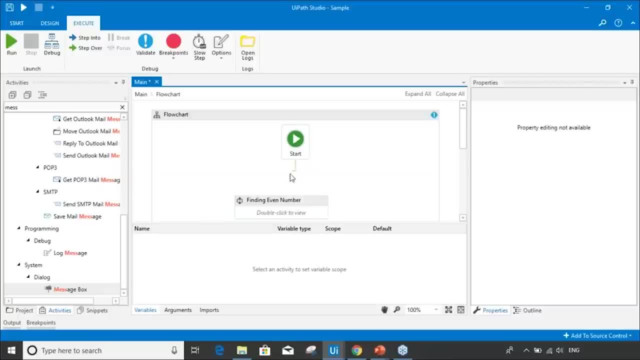 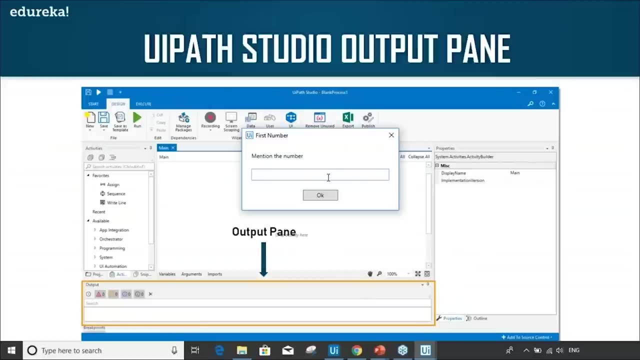 So now I'll go back to my flow chart and then what I'll do is I'll connect the starting point of the flow chart to the sequence and then I'll just execute this particular project. So let's say, now we mentioned the first number to be 596. 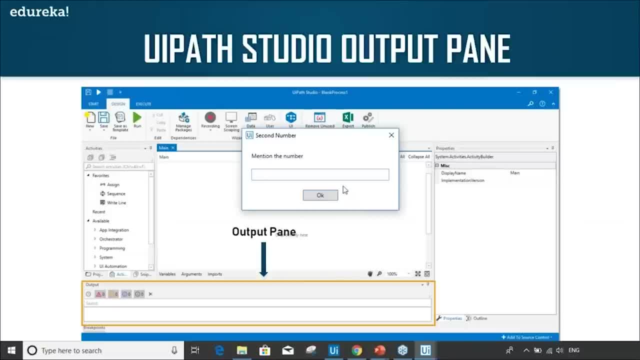 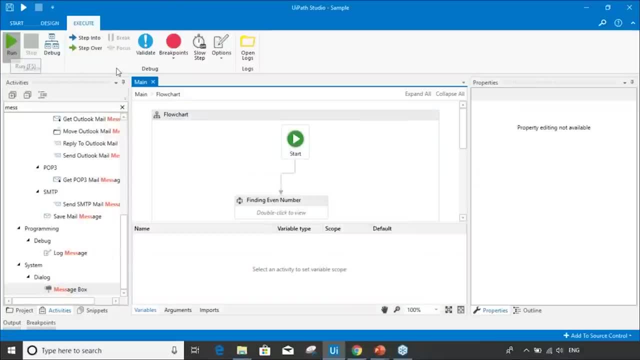 So we'll just click on OK after that and we'll mention the second number. Let's say to click on OK, and then we'll see the message. that number is even now. Similarly, if you just want to execute again, let's say: you know. 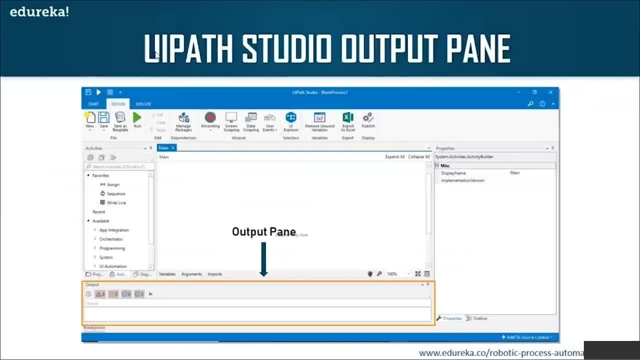 we want to enter an odd number. So let's just do the same. So let's check for odd number. Let's say I mentioned 679, click on OK, and then I'll mention to click on OK again, and then you'll see that you know. 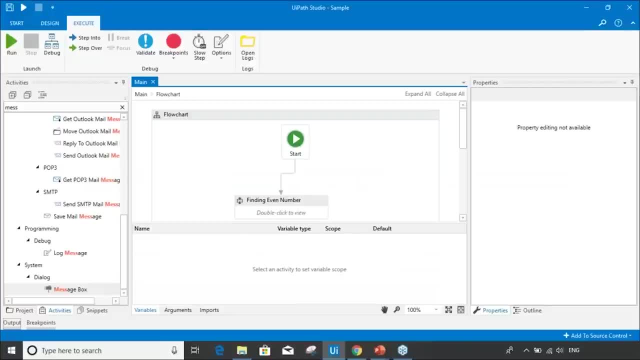 the number is odd. So, guys, that's how basically you can use uipath studio. So instead of run over here, you can also have clicked on debug and then you would see step-by-step execution. So this was a simple project on uipath studio. 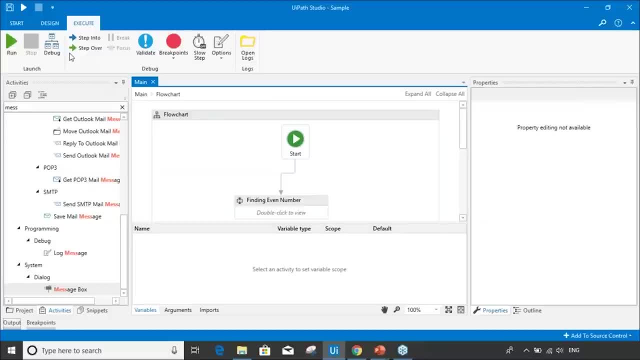 This was just an introductory session of how you can use your iPad studio or how you can get started with uipath studio. Now, before I end this session on uipath studio, let me just go back to the documents of my system, and then I'll show you something interesting over there. 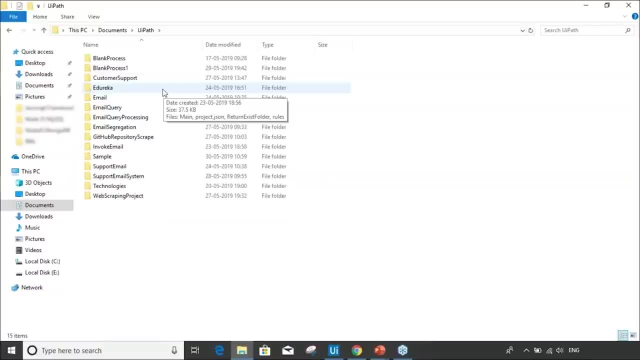 So if you go to the documents of your system, you'll have a folder known as uipath. So in the folder of uipath you'll see various project files. So these are all the projects that I have created till date. 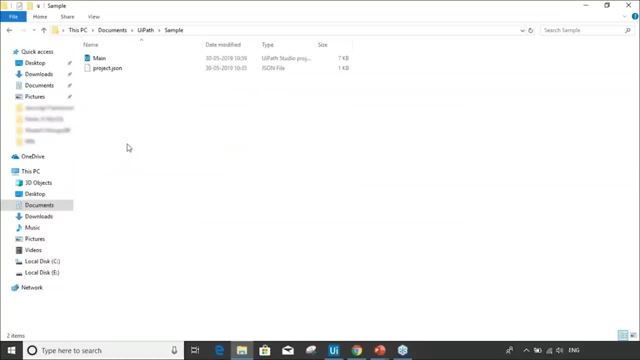 Now, for example, let's say we go to the sample project that we just created. You'll see mainly two files in that: that is the main file and the project or JSON file. The main file is basically your uipath automation workflow and the project dot Jason file contains all the information. 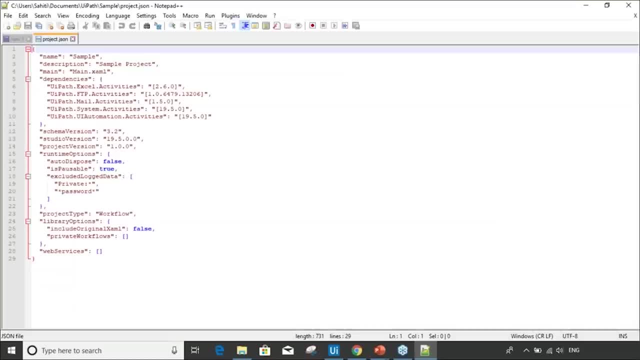 about your project. So if I just open it with my notepad plus first, you'll see that. you know, it has the name, the description, the main- that is basically what is the name of the main file- and then the dependencies also. So it has all the version names, the dependency files. 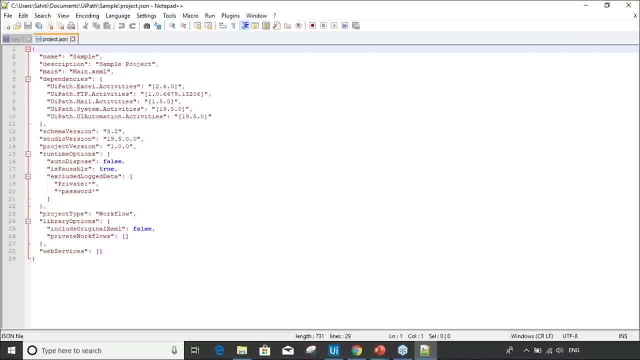 the name of your project and all other related information right. So any day if you wish to just understand the configuration of your projects that you created for uipath studio, then you can go back to your project or Jason file and understand what are the dependencies present. 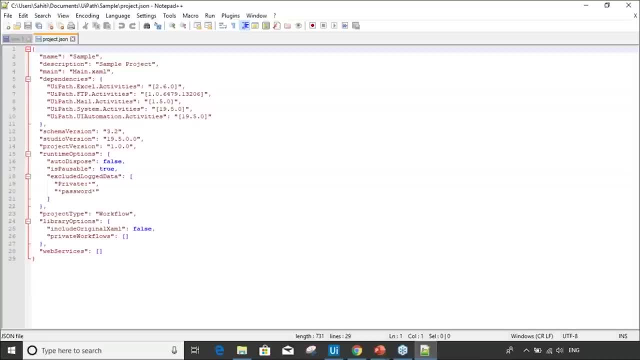 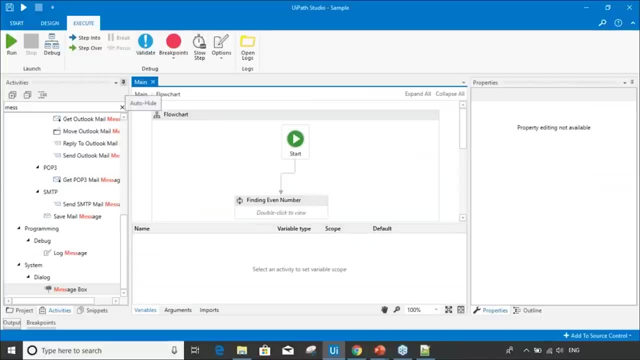 for your project, What is the name and maybe what is the version and so on. So, guys, that was about uipath studio. now uipath also has various other components, like you know: ui robot and uipath orchestrator. now talking. 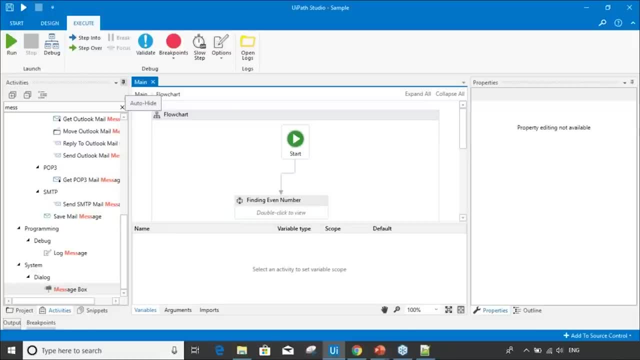 about the connection between all these three components. The basic connection is that whatever automation workflow you create in uipath studio is executed by the ui robot and then, once you execute it, you can deploy that particular automation workflow and publish that project in the orchestrator server. 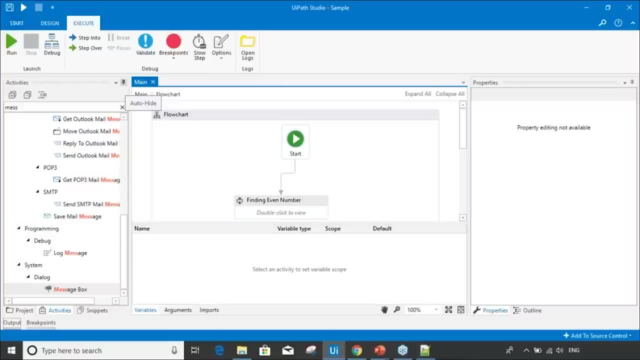 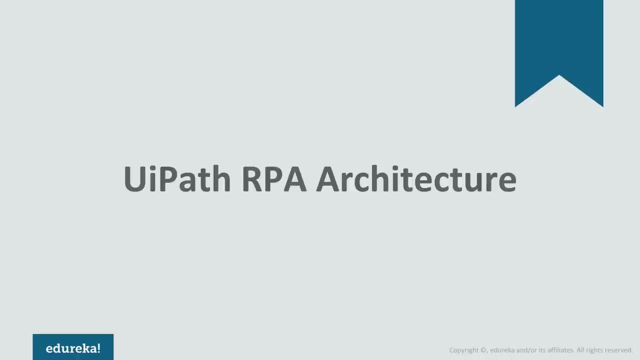 so that, through orchestrator server, hundreds of PCs can automate either the front office processes or the back office processes. So let's get started with uipath architecture. before I start with uipath architecture, I'm going to first cover a few important components. 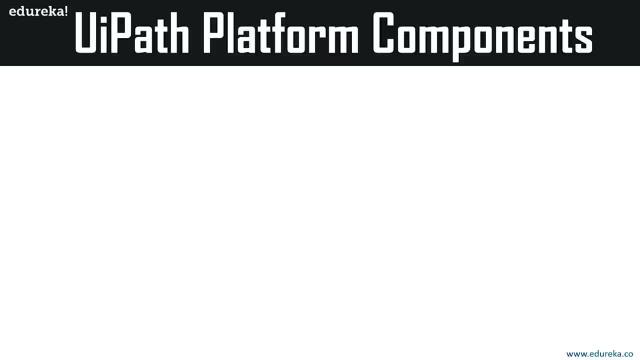 of uipath platform so that you understand the architecture in a really simple way. So, starting with uipath platform component, there are mainly three platform components that you need to understand about. that is, the uipath studio, uipath robot and uipath orchestrator. 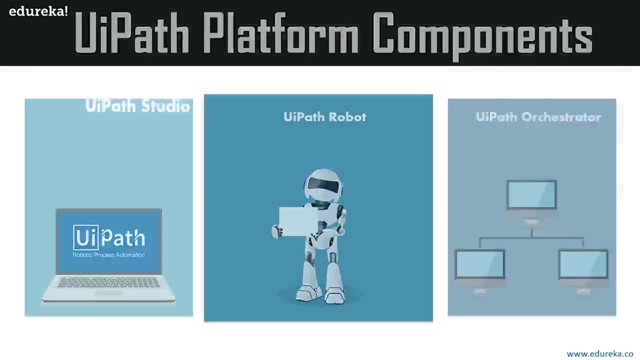 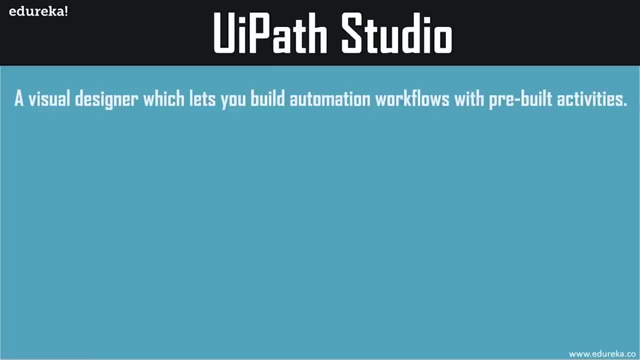 So we'll be looking at to each one of them one by one. So let's start with uipath studio first. So uipath studio is a visual designer which lets you build automation workflows with pre-built activities. It's basically a GUI dashboard with the help. 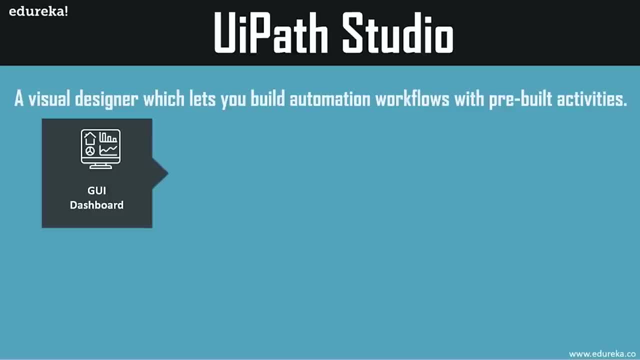 of which you can automate tasks, or maybe you can design the automation workflow with the help of the pre-built activities. It has various complexity levels through which you can build different kinds of project. So those could be the process library, transactional process, agent, process improvement. 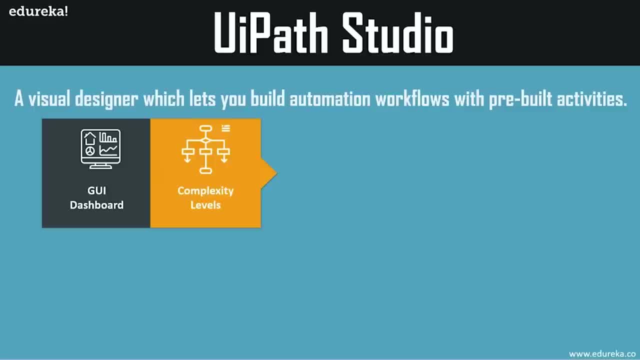 and robotic Enterprise framework. talking about process process is basically a blank project which is used to design the new automation process. The library is used to create reusable components and publish them together as a library. The transactional process is to model a process as a flow chart diagram. 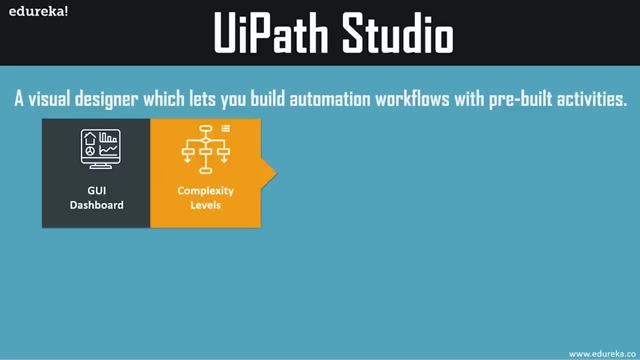 The agent process improvement is basically used when you want to trigger an automation in response to a mouse or a keyboard event. and finally, talking about the robotic Enterprise framework, This basically creates a transactional business process that follows the best practices for the large-scale deployments. 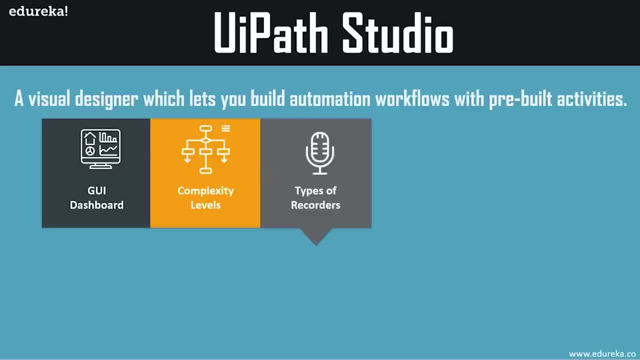 Apart from this, uipath studio also offers different types of recorders, such as the desktop, the web, the Citrix and so on. So all these kinds of recorders can be used to record various actions on various platforms. after that, It also offers logging and exception handling features. 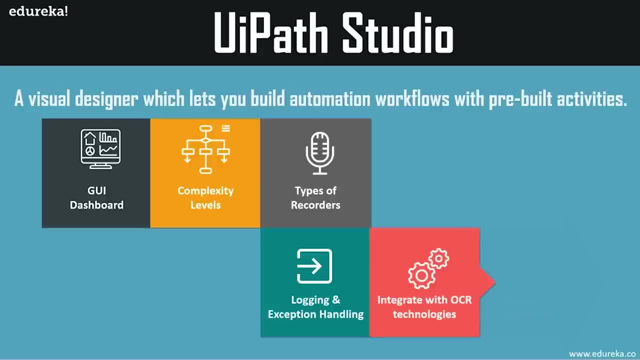 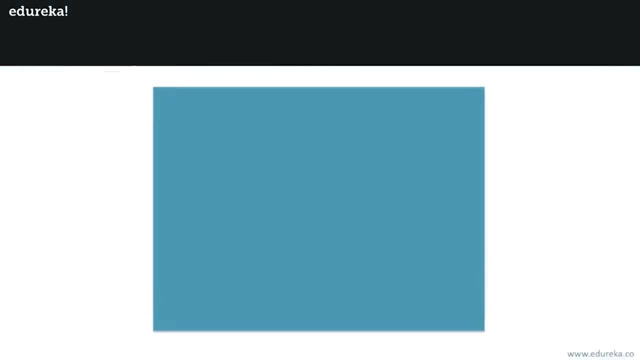 and integrates with various OCR technologies to capture text or maybe to capture images, and also creates reusable components. So, guys, these were about the various features about uipath studio, So let's move forward with the next platform component, that is, the uipath robot. 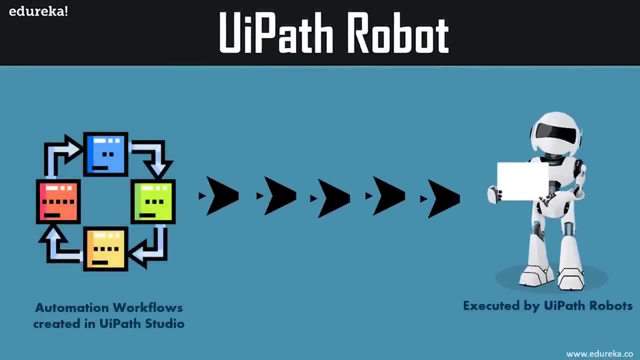 So uipath robot is basically the platform component which executes the created automation workflows in uipath studio. So the automation workflows which are created in uipath studio are basically executed by the uipath robots. They mainly have only one functionality, that is, to execute the automation workflow. 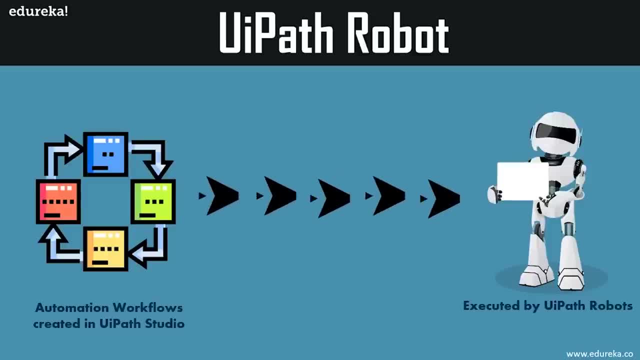 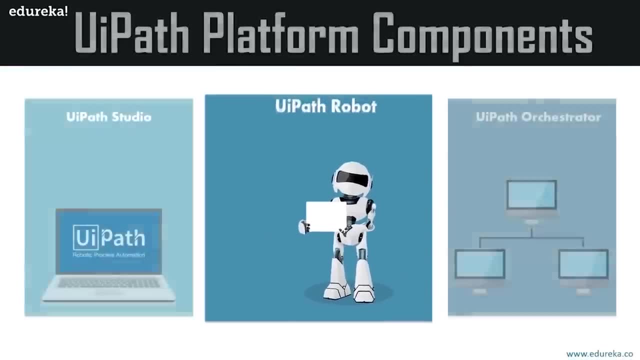 Now you can either have a single uipath robot or you can have multiple uipath robots based on the kind of task that you're using or based on the kind of addition that you have. So this was about the uipath robot, guys. 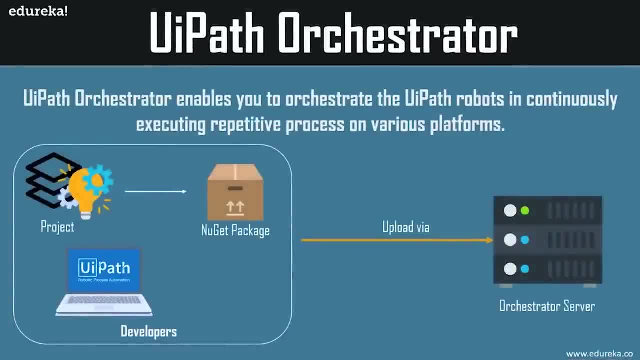 Now let's move forward with the third component, that is, the uipath orchestrator. So uipath orchestrator basically enables you to orchestrate the uipath robots in a continuously executing repetitive process on various platforms. So when I say continuously executing repetitive process, 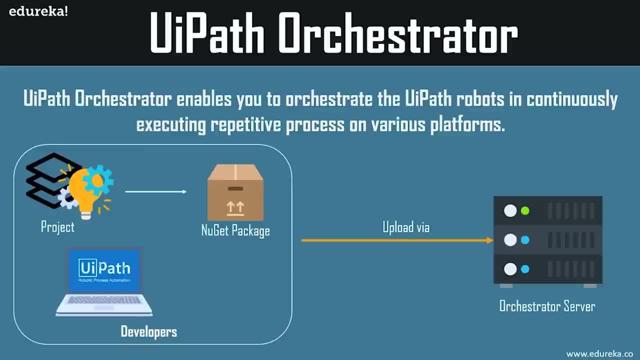 on various platforms. what I mean? that you know you can create a project in your uipath studio, publish it into the orchestrator server And once you publish into the orchestrator server you'll assign it to a robot and maybe a specific robot can basically automatically execute. 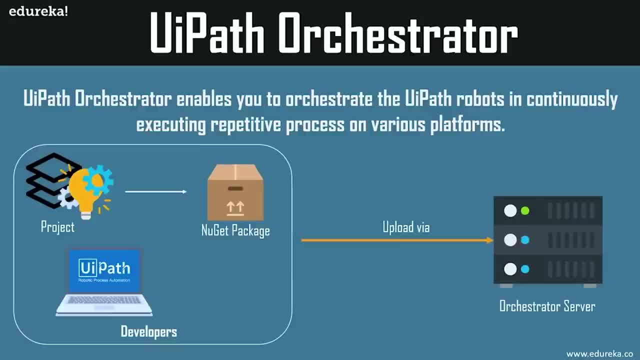 and monitor that particular process in various back-office or front-office processes. So let's understand the same. So, for example, let's consider that you know you have a developer who has developed a specific task or maybe a specific automation workflow in the uipath studio. 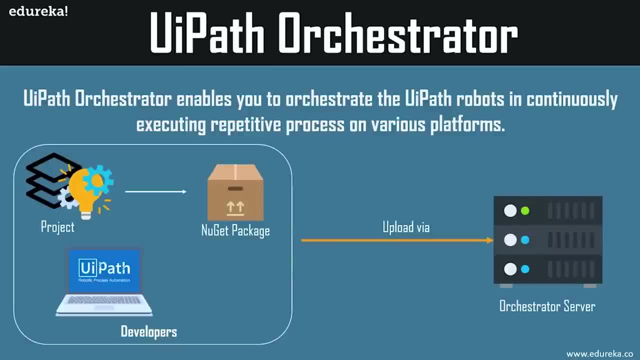 Now what happens is that that particular task is published as a project and then a NuGet package is created. So what is NuGet package? So when I say NuGet package, the NuGet package is basically a free and an open-source package manager designed. 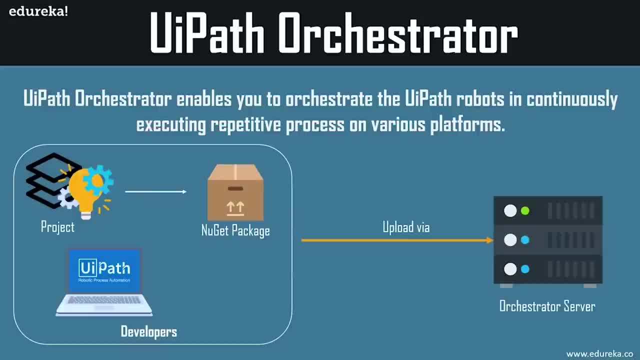 for the Microsoft platform development. So this can be either used from the command line and can be automated with scripts, and it supports multiple programming languages, but is mainly also used for NET framework packages. And let me also tell you that uipath's underlining framework is completely based. 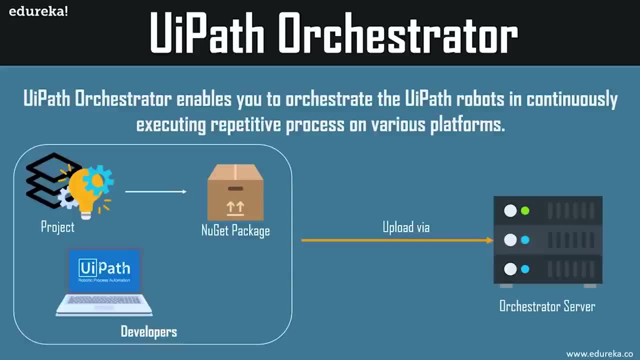 on NET. So basically, that's how the NuGet package comes into picture, and then the project is uploaded via the orchestrator server. So when I say orchestrator server, what happens is that once the project is published from the uipath studio, 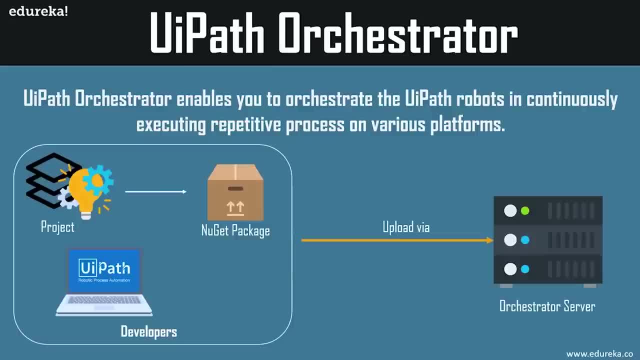 the project can be searched in the orchestrator server and then a process is created. Once the process is created, what happens is that you assign the process to a specific robot and then a job is created to execute the task, or basically execute the process on various systems. 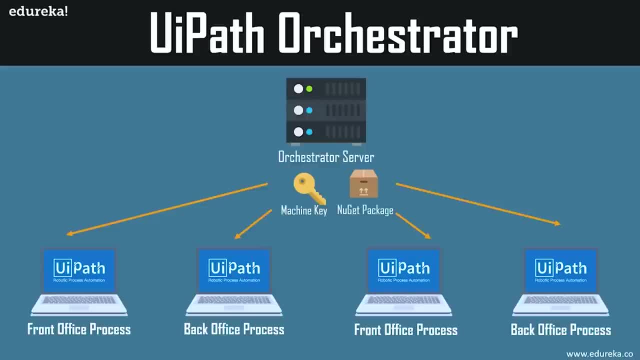 So that's what is happening. So every orchestrator server has a machine key and a NuGet package, and then what happens is that every robot is given a specific user, or, you can say, a specific system ID in which a specific process has to be executed. right, 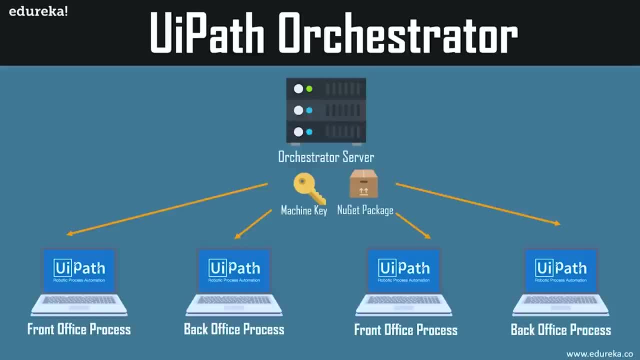 So, if you consider the back-office processes, the robot automatically executes and monitors the back-office processes. But if you consider the front office processes, what happens is that the orchestrator server only monitors the specific process. But yes, a user has to sit and execute the process. 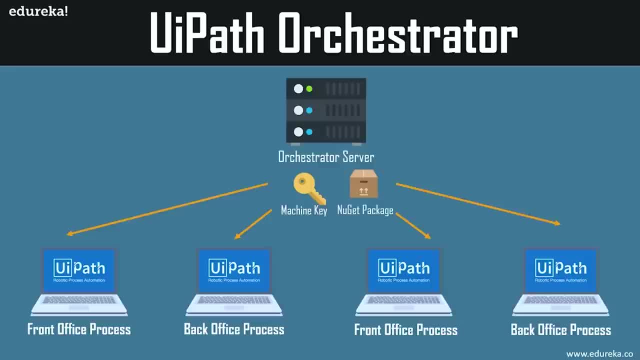 So that's the difference, guys. in front office processes, The user has to sit and execute the process and the orchestrator server only monitors the process. But when it comes to the back-office processes, the orchestrator executes and monitors the processes. So that's how, guys, the orchestrator works. 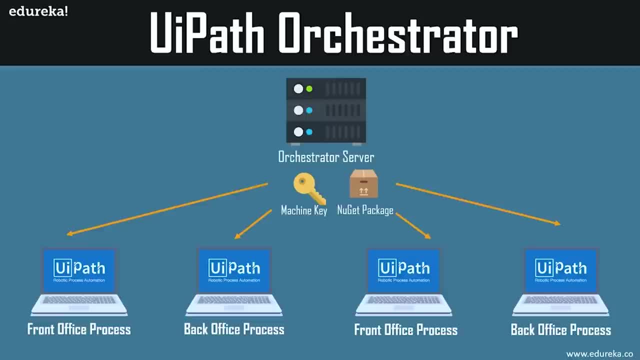 It's really simple to understand. So if you just want to understand in depth how to create an environment and give the machine ID and then give a proper key, execute a task, create a process and then job and finally use that robot to perform a task, 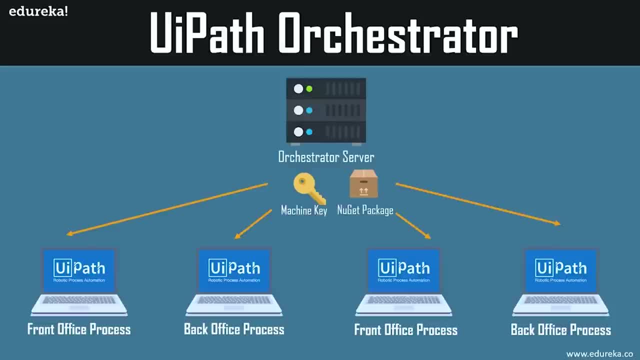 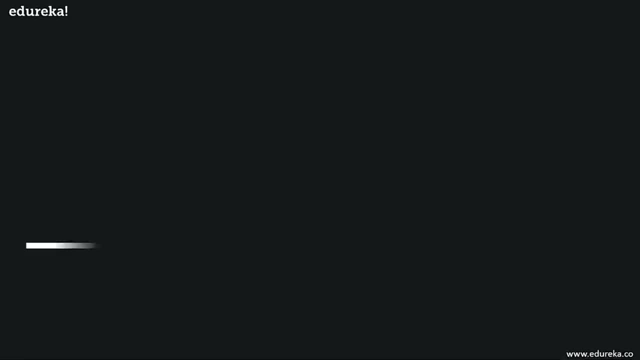 So that's how guys orchestrator works. So these were the various components of UiPath platform, that is, UiPath studio, robot and orchestrator. now moving forward with the final topic for today's session, that is UiPath architecture. But let me tell you guys, whatever I was talking till now was also a part. 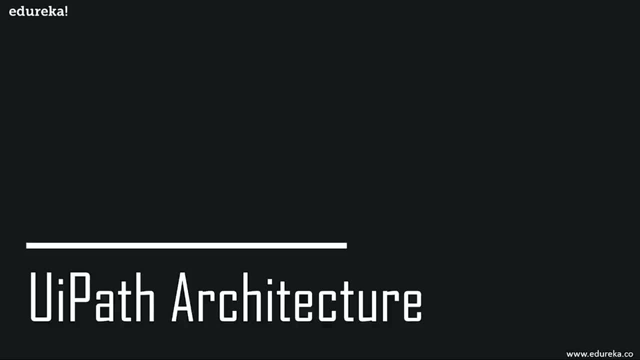 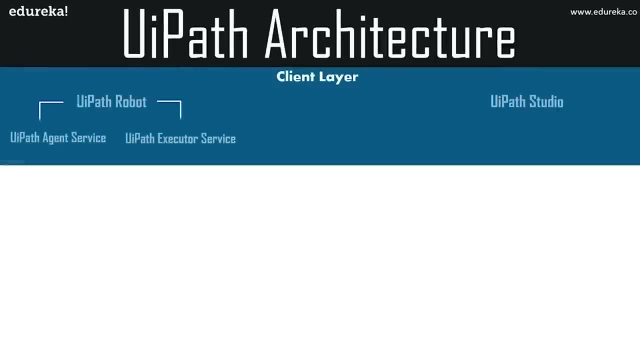 of the UiPath architecture. I just spoke as different, different platform components. Now I'll show you how these three components come together and work for you to execute a specific task. So, as you can see on my screen, this is basically how the architecture is divided. 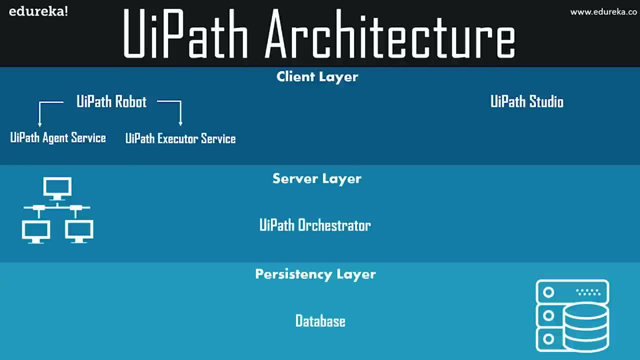 So there are mainly three layers: the client layer, the server layer and the persistency layer. the client layer is basically the layer where the developers sit and then, you know, create automation workflows. So over there obviously we have the UiPath robot and the studio. the studio is basically a place. 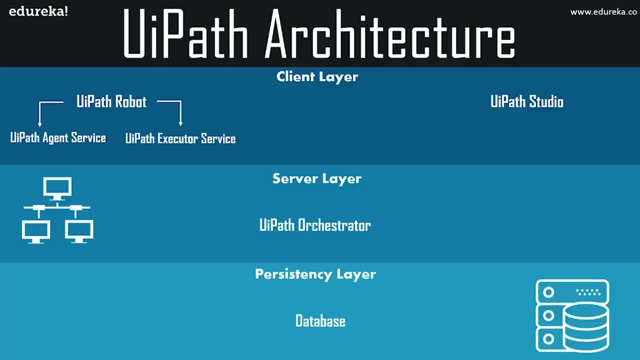 where you create automation workflows, as I just spoke before, and the robot executes those created automation workflows. Now the UiPath agent service is basically the single point of contact for all the executors through which the messages are logged into the orchestrator service, which processes them further. 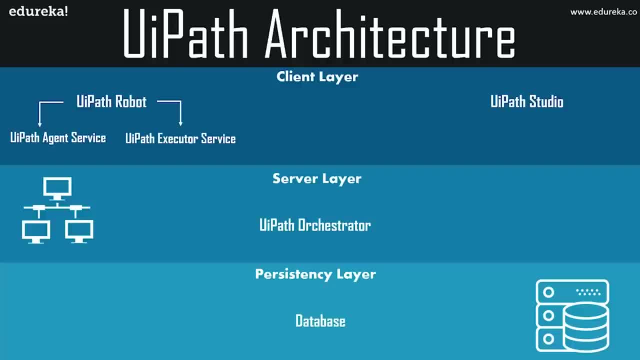 to the sequel server of the sequel database and coming to the executor service, the executor service is basically used by the robots to execute the task. So these are the two main components that you have to understand about the UiPath robot. next, moving forward, We have the server layer. 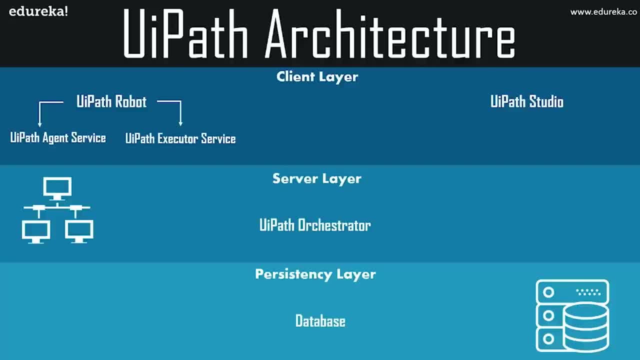 So the server layer basically has the UiPath orchestrator which takes care about the monitoring, the deployment, the configuration, the queue management, the logging of the task or you can consider the logging of the automation workflows. So you can consider that you know the orchestrator is the main place. 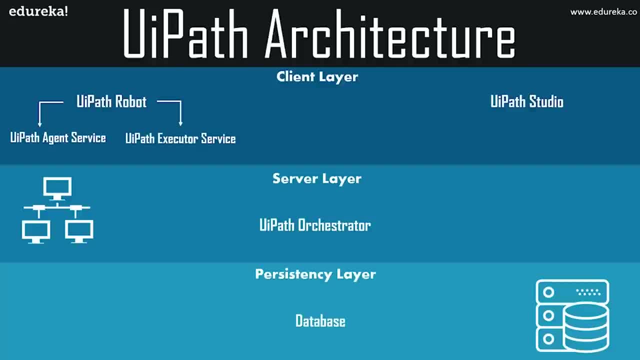 where everything is taken into control, and then the client layer is the place where you actually create the automation workflows. coming to the third layer, that is the persistency layer, So the persistency layer is basically the layer where we have the database in this particular layer. 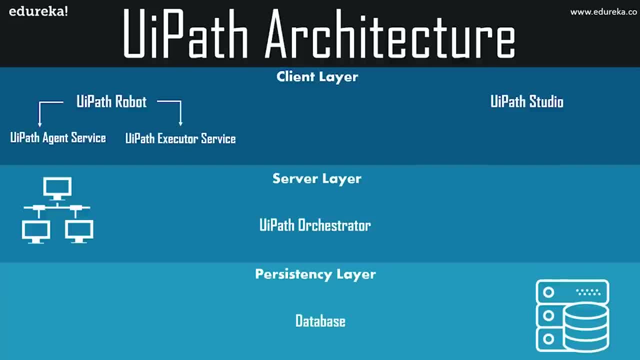 We have various kind of information, like you know: the robots configuration, maybe the robot groups, which robots are single robots working for a specific task, or maybe a specific user. then there's information about assigned processes: which process is assigned to which robot and then which environment. 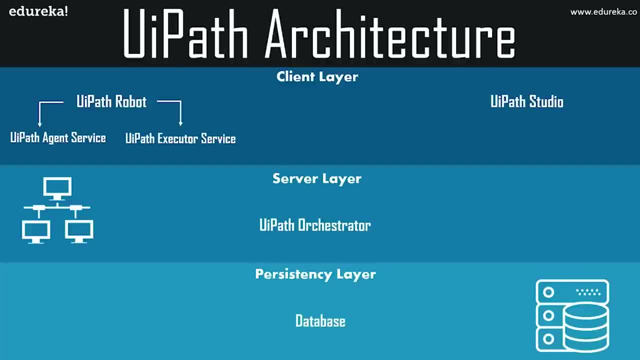 is used for it. Then we also have information about queues and queues items. So that was about the architecture guys. So if you just have to understand UiPath architecture, then mainly you have to get a good understanding on the main platform components of UiPath. 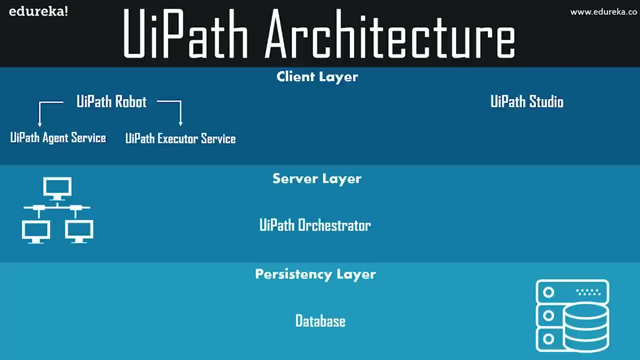 that is UiPath studio robot and orchestrator. after that You just have to understand that. you know they work on three layers, that is, the client layer, server layer and the persistency layer. So the client layer has the robot and the studio where basically the automation workflows are created. 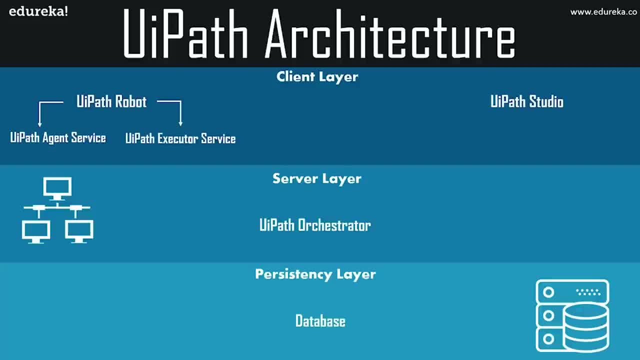 and then the robot executes them. The server layer has the orchestrator layer, where the orchestrator works and orchestrates your UiPath report. So over there you have ways of the factors, like you know: monitoring, deployment, configuration, queue management and logging, and finally coming to the persistency layer. 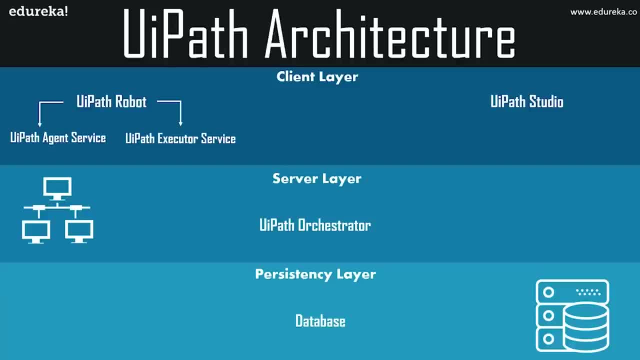 The persistency layer is the layer where we have a database. So over there we have various kinds of information, like you know: the report configuration, the report groups, and then we have also information about the assigned processes: which processes are assigned to which robots, what environment. 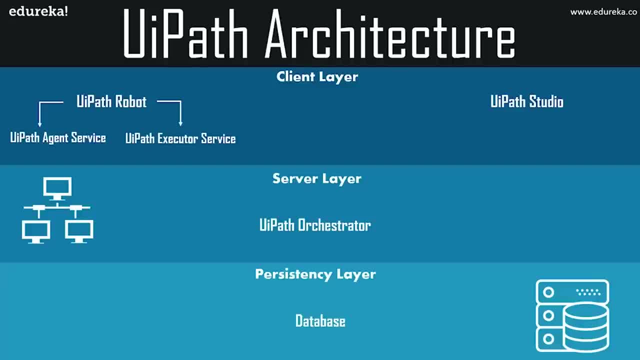 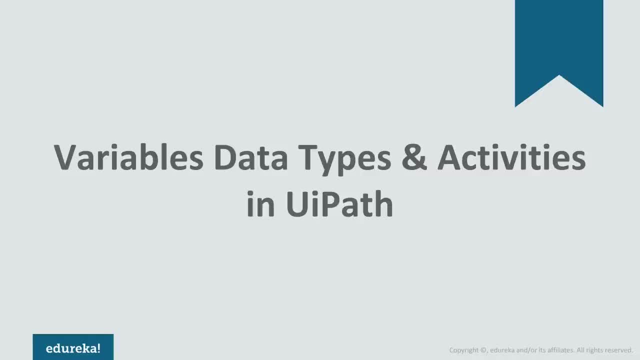 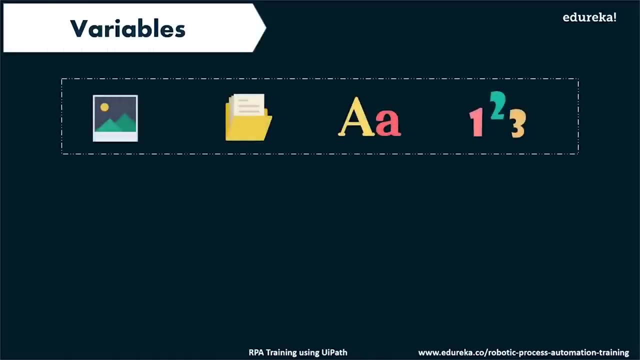 and so on, and then the information about queues, and then what are the items in the queues. So, guys, this was about the UiPath RPA architecture. So we'll start today's session by understanding variables first. So variables in UiPath are very much similar to the variables. 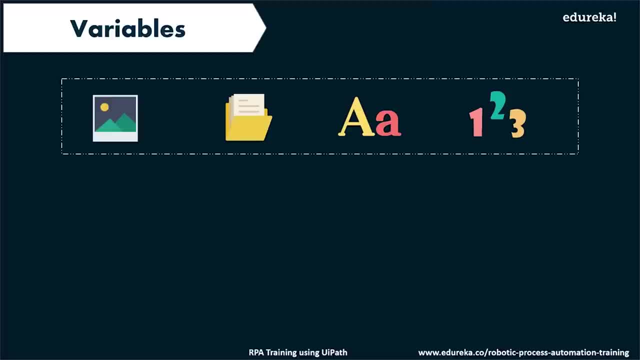 in any other programming languages or you know the mathematical field. So if you just observe an equation, like you know, y is equal to 3x plus 5, right? So you'll observe that you know x and y are basically variables in mathematical. 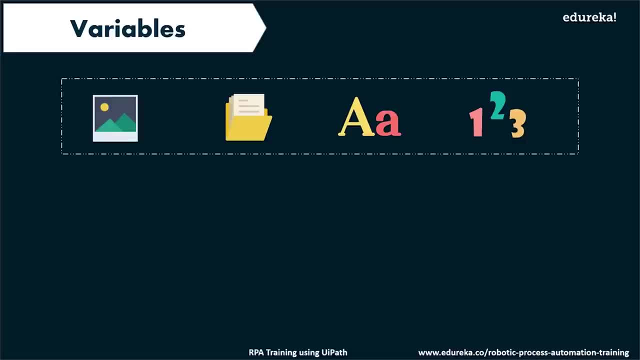 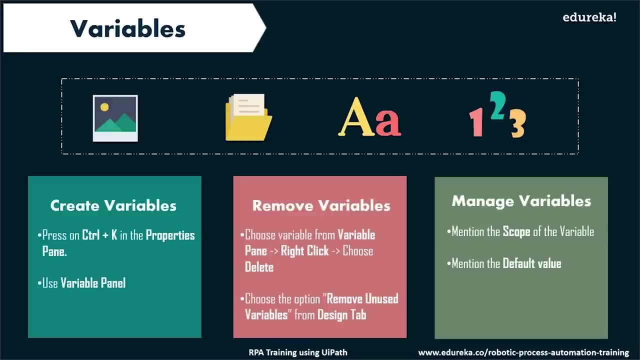 Right. So whenever x changes, you obviously know that y changes, right? So, guys, that's how variables work in UiPath also. So, basically, in UiPath you can use variables to store the files, folders, alphabets, numbers and any kind of values that you want down. 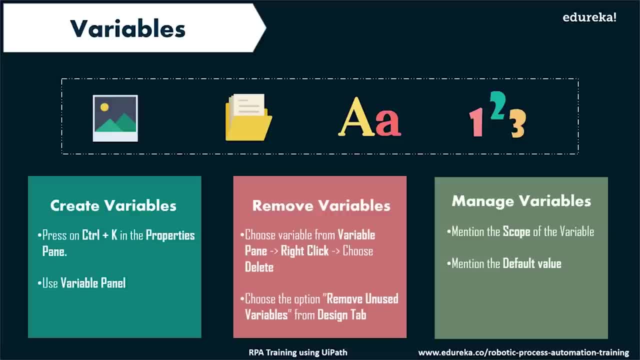 like in any other programming languages, even in UiPath, you can create variables, you can remove variables and you can definitely manage variables. So to create variables, that are basically two options. that is, you can either go to the properties pane of a particular activity, press on control. 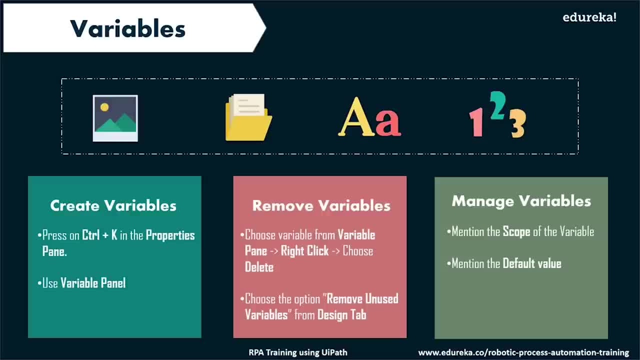 key in the output section and then set a name for your variable, or you can directly use the variable panel. So don't worry, I'll show you how that's done, But before that let me just tell you how you can remove variables and manage variables. 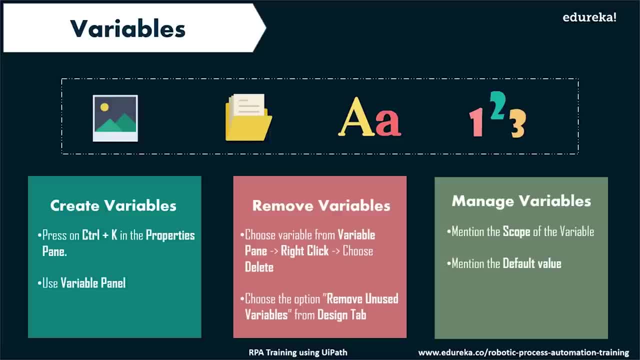 So to remove variables, what you can simply do is you can go to the variable pane again, right click over there, choose the delete option, or you can use the ribbon tab and over there you'll see an option of you know: remove unused variables, right? So whatever unused variables are present in your sequence, 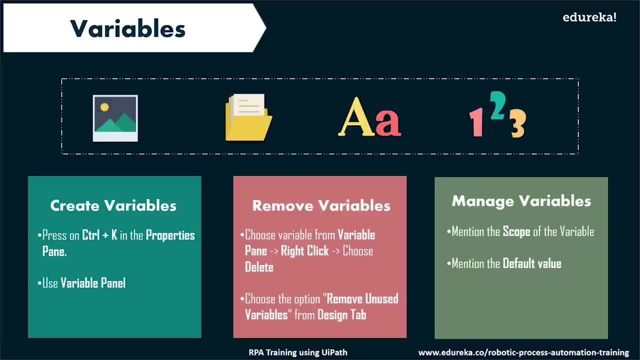 or are present in your file will be removed when you click on that particular option. And when I say manage variables, by manage variables I mean that you know you have to decide the scope of the variable, and you can also mention a default value for your variable. 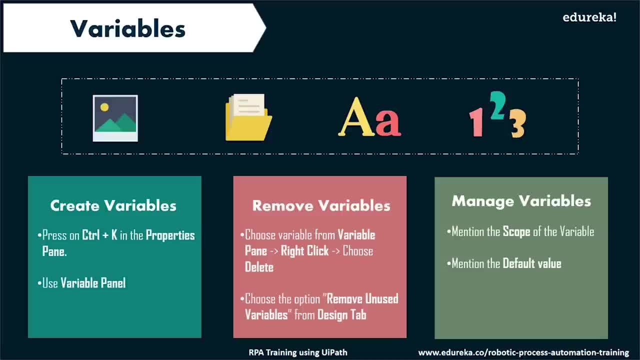 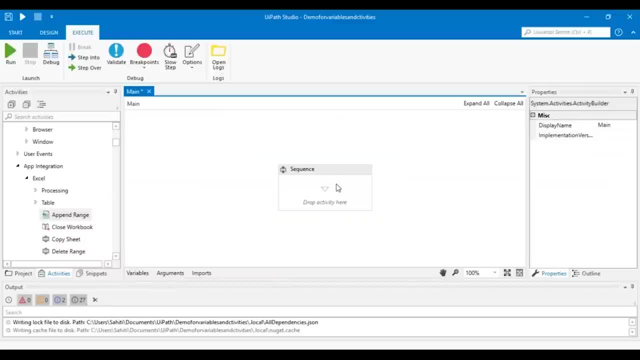 So that's completely your call, how you want to define the scope of the variable and if you want to mention the default value or not. So let me just show you how that's done. first, I'll just remove this particular activity right. So now, if you just want to create a variable for this particular sequence, 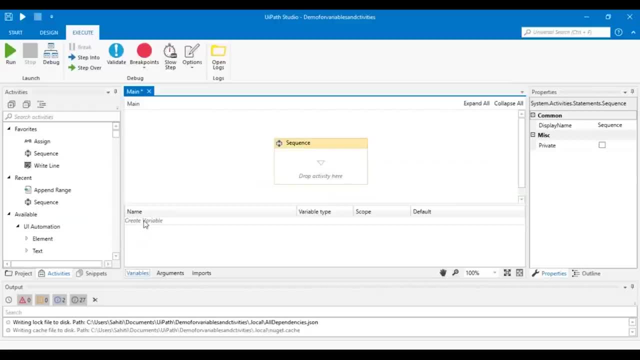 what you can simply do is you can click on this variable pane and then over here, if you click, you can just mention the name of the variable, Let's say sample, and then you can mention the variable type. So it could be either a boolean variable, 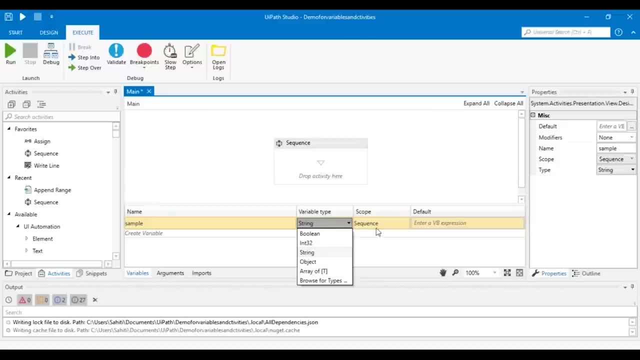 int, string, object, array of t variables and so on. right Now, the scope of this particular variable would be sequence and the default value, Let's say it's ABC, right? So I've just defined a variable for this particular sequence. 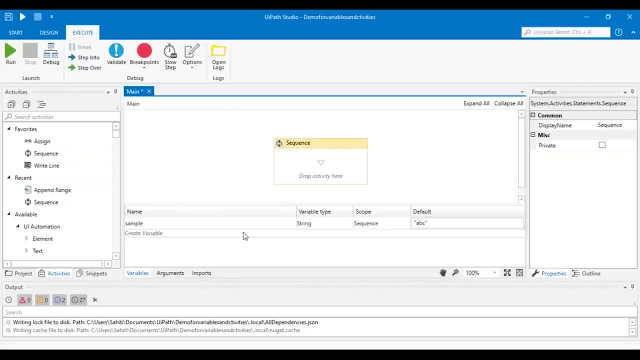 So when I click on this particular sequence, you'll see that you know there's a variable created for this particular sequence. Now, if you just want to see the other option, let's just drag and drop a message box activity And then what you can do is in this particular activity. 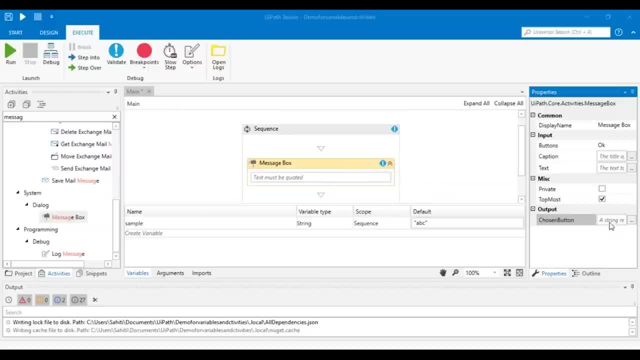 what you can simply do is you can go to the message box activity, You can go to the properties pane of this activity, Then you go to the output section and press on ctrl K and let's say ABC, right, So you'll see that you know. 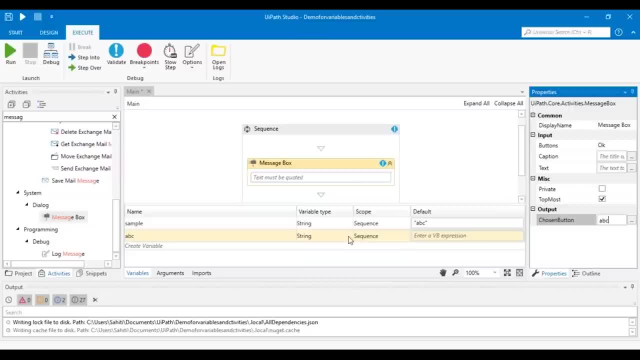 ABC variable has been created automatically, of the string type and it has the scope of sequence and there's no default value mentioned Now. one more thing that I would like to tell you about variables is that you know when you change a variable over here. 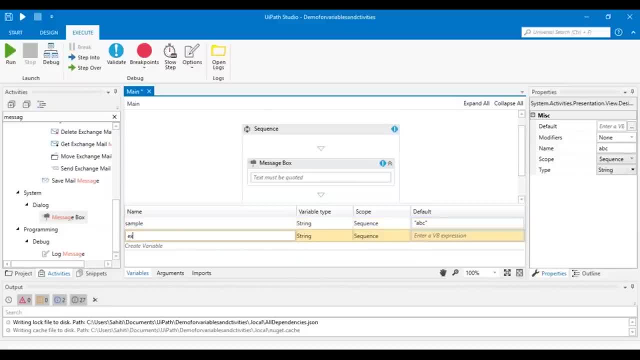 it will get changed everywhere else. that variable is mentioned, right? So let's say I mentioned it to be example, right? So I've changed ABC to be example. So if I click on this particular activity of message box, you clearly see that 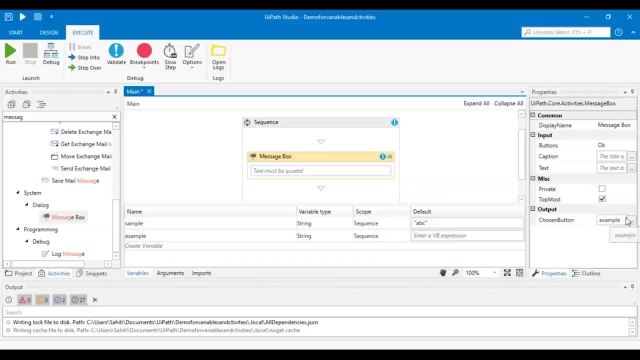 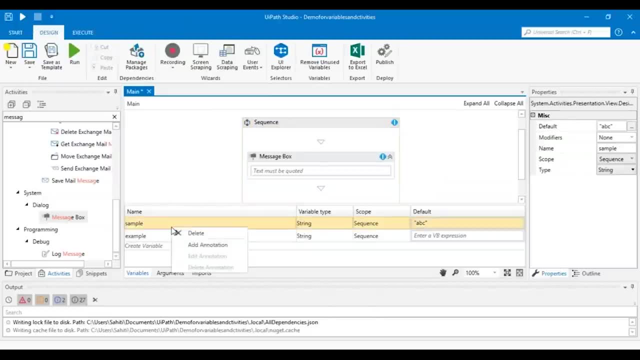 you know, the variable name has changed from ABC to example. So, guys, that was all about variables. Now, if you just want to remove the variable, what you can simply do is you can either go to the variable pane, right click over here and then choose the delete option. 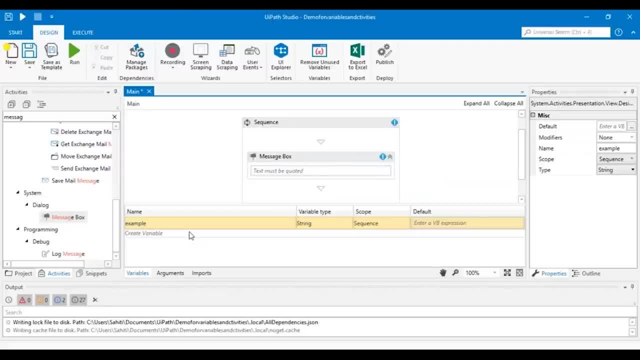 So if you choose a delete option, you can clearly see that you know that particular variable has just vanished, right. That means it's just removed Right Now. as I said, there's another option for removing variables that is mainly used to. 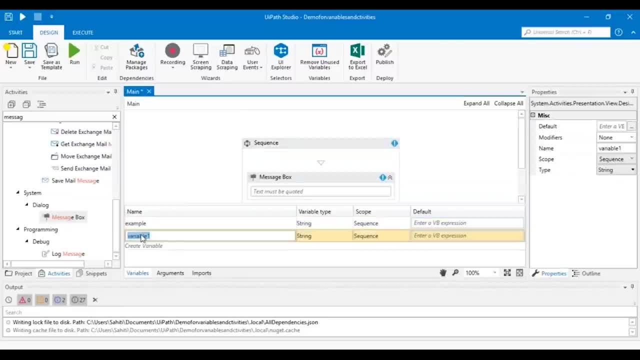 you know, remove the unused variables. So, to remove any unused variables, let me just create a new variable, that is sample 2, right Now, what I'll do is I'll click on this option of remove unused variables. So when I click on this option of remove unused variables, 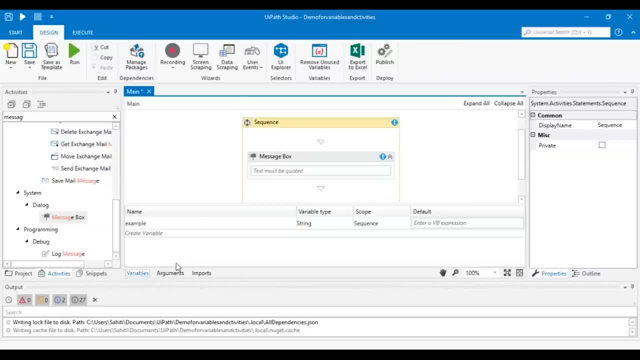 you'll clearly see that. you know the sample 2 variable has got removed, right? That's because we have not used that variable. So that's how you can remove the unused variables. Now, coming to the third point, where I was talking about managing variables. 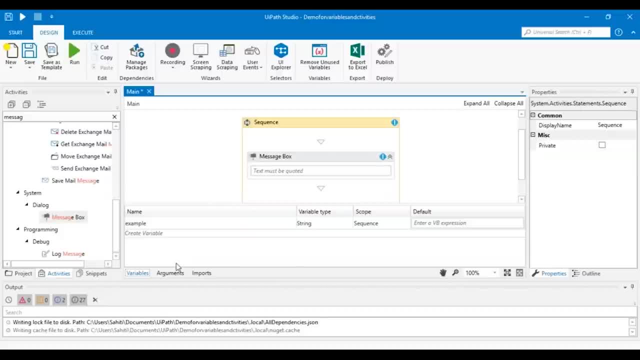 so when I say managing variables, you have to define the scope of the variable, And if you want to define a default value for that variable, then you can very well define a default value for it. So, for example, when I talk about scope, 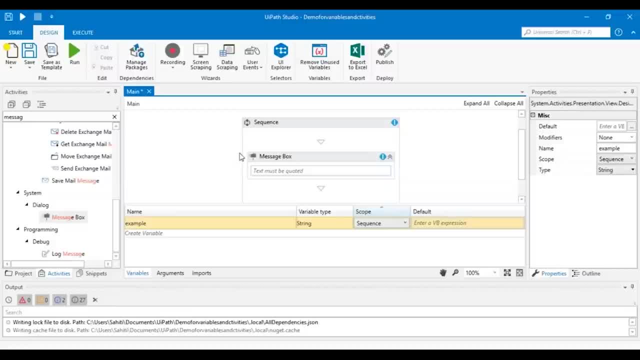 the scope option at present is just for sequence, But yes, if I had any other particular value, like you know, if you had a flow chart inside this right, So I'll just put a flow chart, I'll just search for a flow chart. 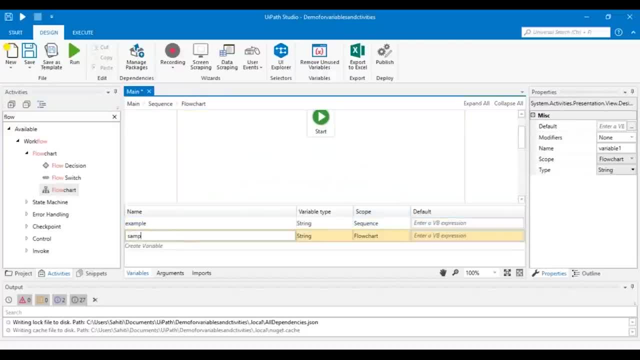 right. And then let's say I had created a variable of sample. right Now, over here I can define the scope: whether the variable has to be just used for the sequence that was created before, or it has to be just used for the flow chart. 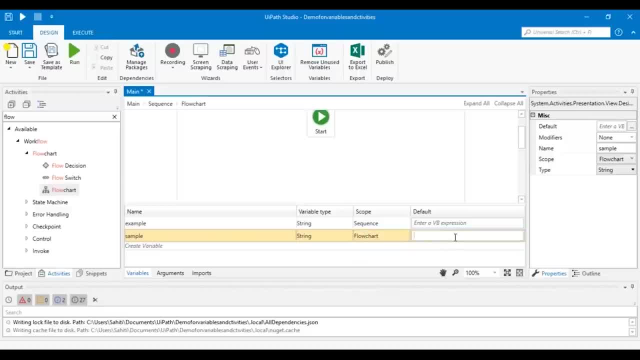 right. So that's how I can choose over here. and coming to the default value, You can definitely mention default value in double quotes. So if it's a spring value, then you can definitely mention the default value in double quotes. coming to the array values, 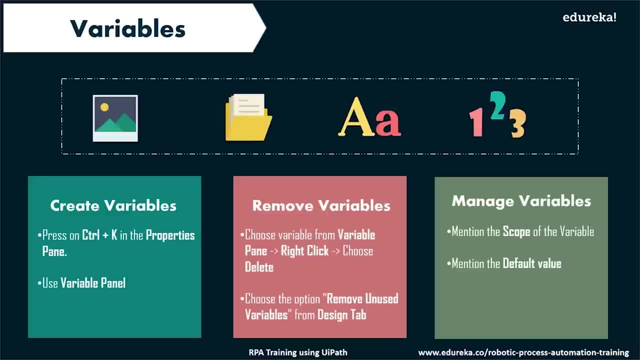 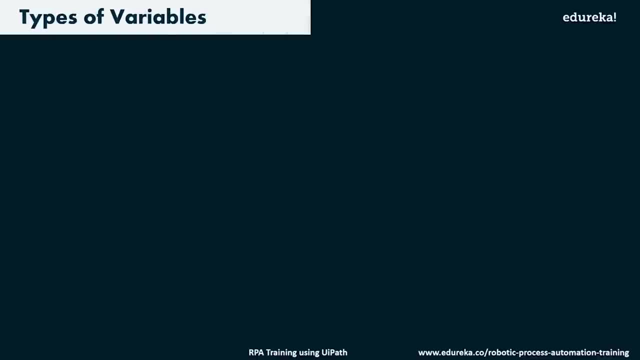 You can store them in brackets and so on. right, So that's how, guys, you can, you know, create variables, remove variables and manage variables. Now let's talk about the different variables, That is, basically the different types of variables that UiPath offers. 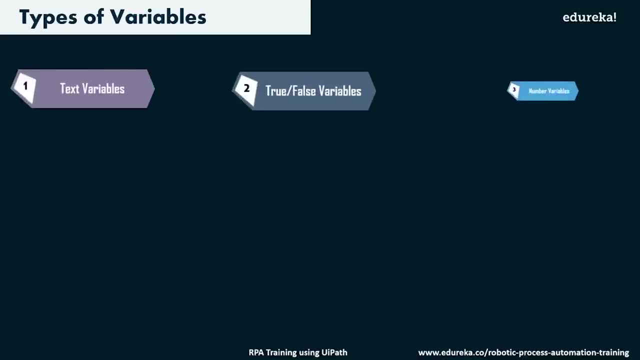 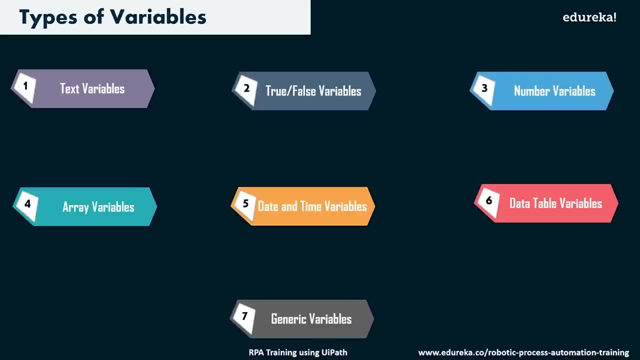 So UiPath basically offers the text variables, the true and false variables, the number variables, array variables, data time variables, data table variables and generic variables. So the text variables are basically used to store the spring values, or you can say the textual values. 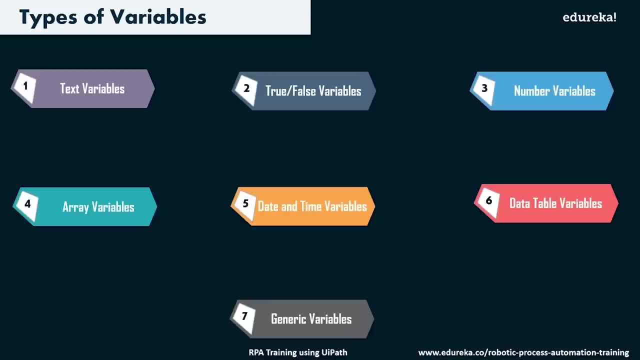 The true and false variables are basically the Boolean type variables which define. you know, if it's true then do an action and if it's false then do another action. The number variables are basically the integer type variables. The array variables store array of any type. 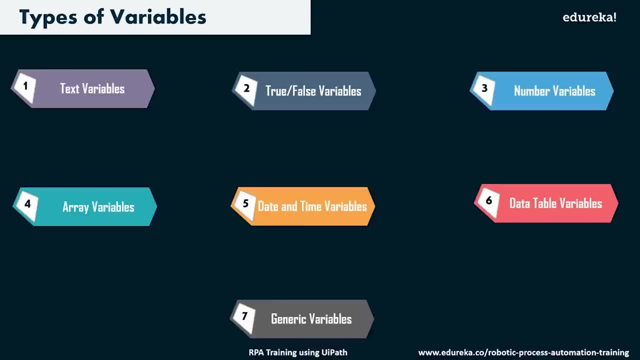 So basically you can have an array of string values or array of integer values and so on. Date and time variables store the date and time. The data table variables basically store the values in form of a table. So, for example, if you extract data from a website, 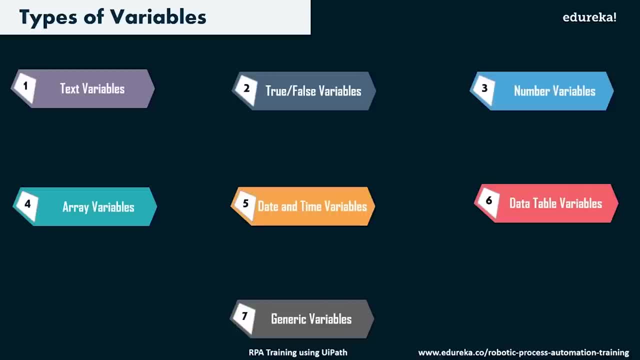 then you see that you know all the data is being stored in a data table variable. That's because you know the data scraped from a website is being stored in a data table variable and then you can store it in any other file by using that particular variable. 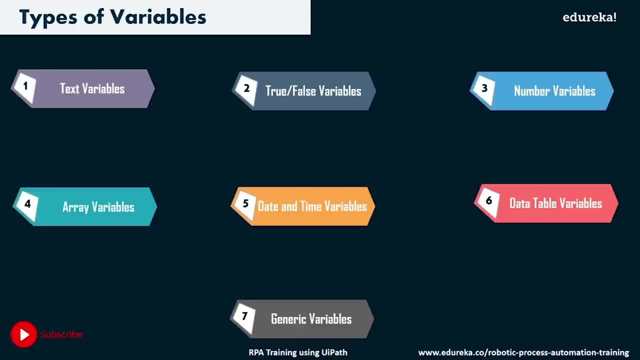 Coming to the generic variables. So when I say generic variables, so you can define an email variable, you can define a body variable, like where you want to identify the body of an email, or you know if you want to identify a database, or if you want to identify a mail message, and so on. 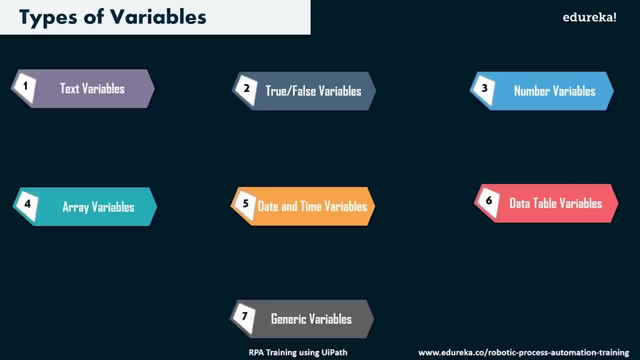 right, So those were the various types of variables, guys. So now let's just look into short demos of, you know, text variables and the number variable, so that you understand how these variables work and then how you can use these variables. So let me just shift back to my UiPath Studio. 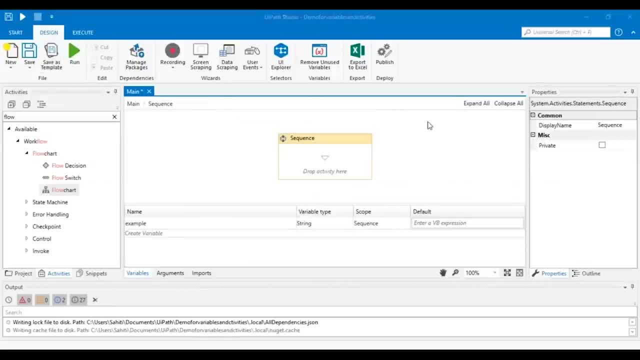 And now what I'll do is I'll basically delete everything from here. So now what I'll do is I'll create a variable for displaying your name, right. So to do that, what I'll first do is I'll drag an input dialog. 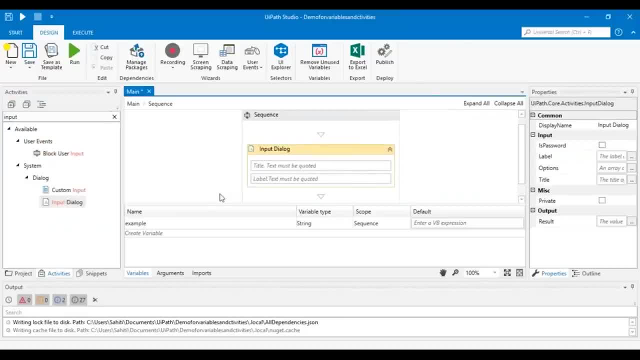 Into the sequence. So when I drag an input dialog into the sequence you mainly have to mention the title and the label. so you can mention you know title, like what's your name, And then in the label you can say: mention your name. 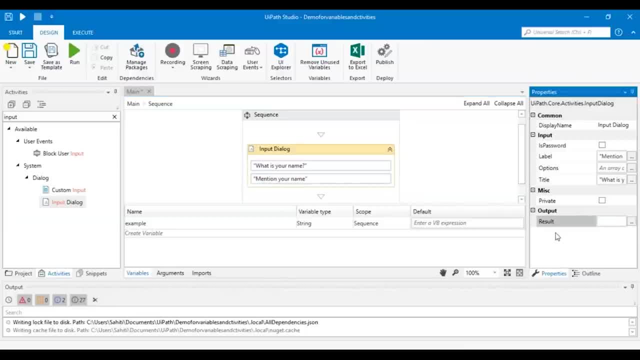 Now what you can do is in the output section of this particular activity, you can press on control K, mention a variable. Let's say you know name. right, You'll see that you know the name variable has been created. Now what you can do is you can change this variable type to spring. 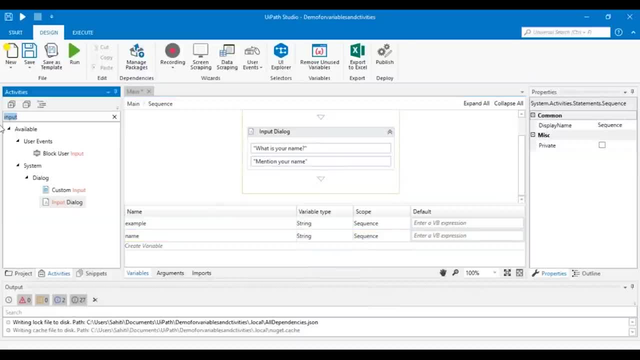 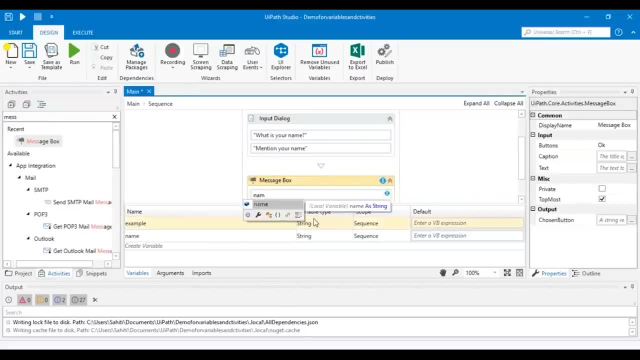 right. And then what we can do is, you know, we can just display this value, right. So to do that, what you can do is you can just search for a message box, drag and drop it over here and mention name. 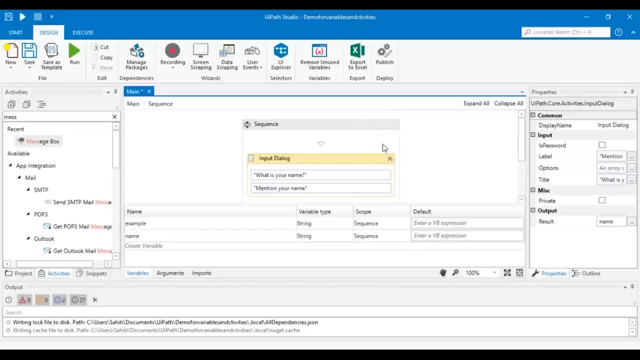 right. So what have I done over here? What I've done is I've dragged an input dialog, you know, which will basically mention my name, So I'll take the output, So whatever name that I mentioned into the input dialog, that value would be stored in the variable name. 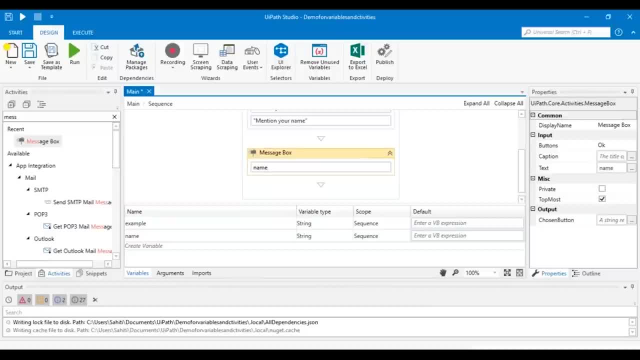 After that, that value will be displayed in a message box. So now to display in a message box. I've used that variable again, right? So now what I'll do is I'll just execute this particular execution. All right, so you can see that. 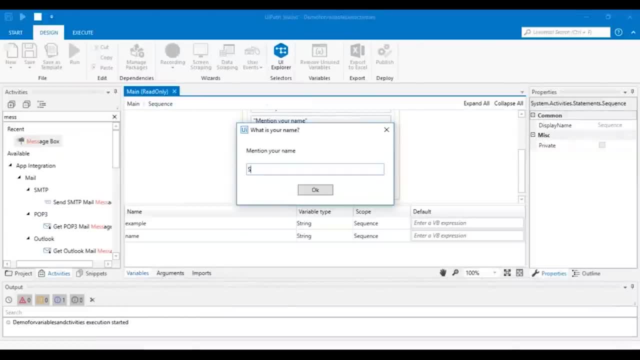 you know you've got an input dialog to mention your name. So let's say I mentioned my name and then I'll click on Okay in the message box. you'll see that you know, society has got printed right. So that's how you can use the text variable, guys. 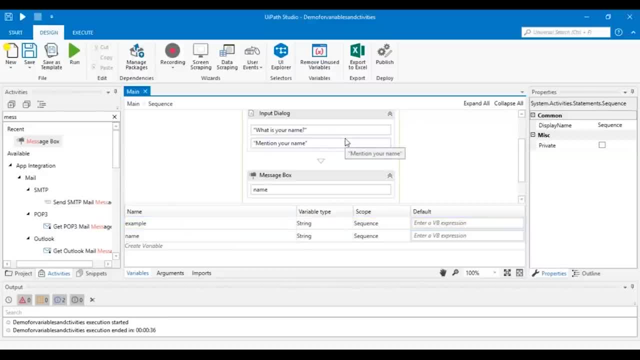 It was really simple. You just had to use the string value- That is basically the name- and then assign it to variable type string, and then you can just use that particular variable to display the output again. Now, similarly, let's do the same for the number variables. 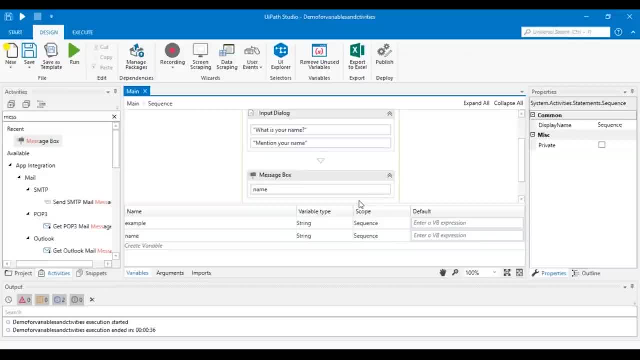 So to use the number variables, let's say: you know we want to find out our present age right Now. to do that, what you can do is in the input dialog you can ask you know the birth year to the user. 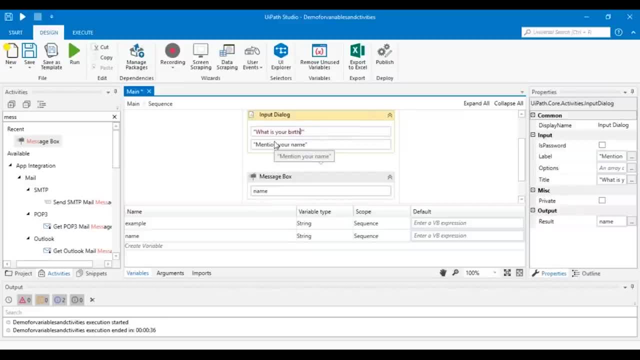 So let's say, you know we can mention over here What is your birth year, And over here I'll mention: mention your birth year. Now, what I'll do is in the output section I'll just change this particular variable. 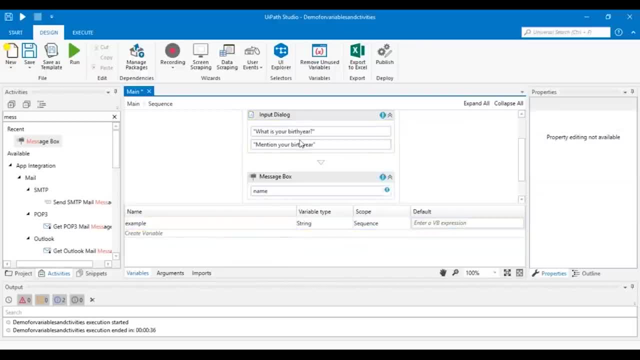 So to change this particular variable, either I can choose the option of deleting the variable or I can just use, you know, remove the particular variable from over here. So what I'll say is I'll just remove this particular variable, and now what I'll do is I'll press on control K again over. 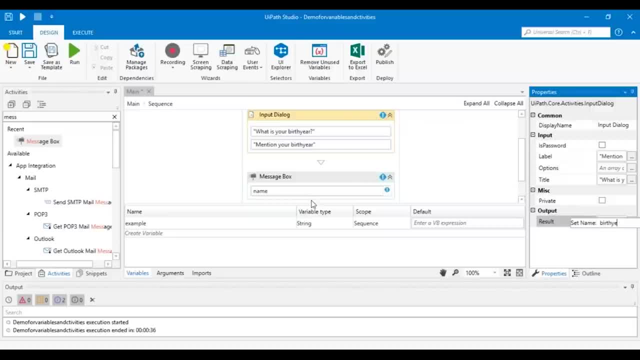 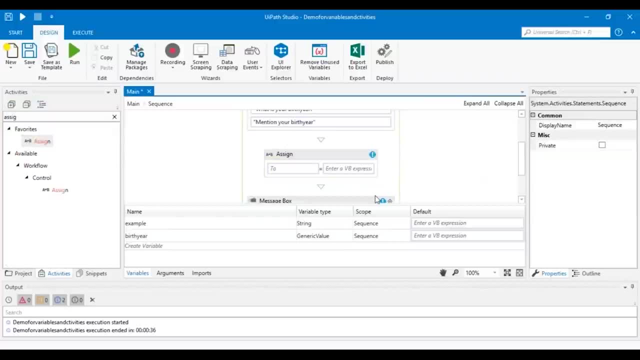 here and then I'll create a new variable. Let's say, you know birth year right Now. what I'll do is I'll use the assign activity over here. What I'll do is I'll subtract the birth year from the present. 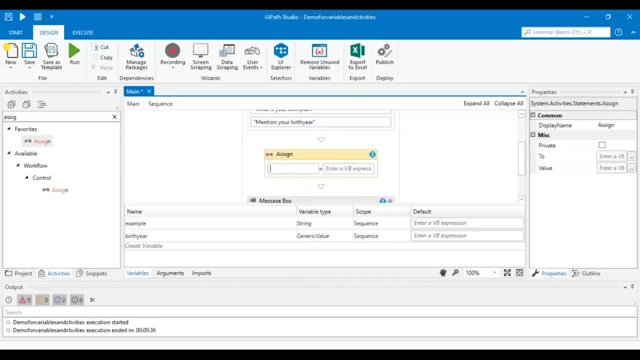 year and then assign it to a new variable, right? So to do that, what I'll do is I'll create a new variable. Let's say, you know, I create a variable to be present age of n-type, So your birth year can also be of n-type. 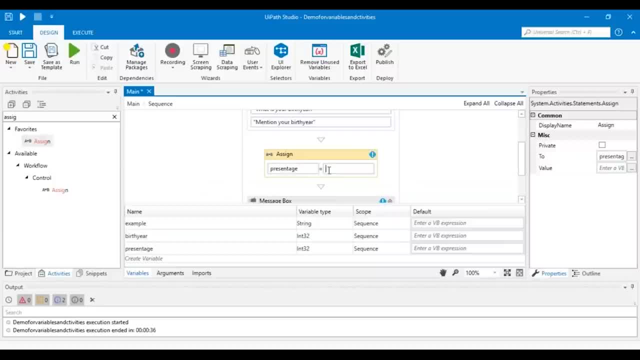 right. So I'll just mention present age over here And what I'll do is I'll subtract 2019 and birth year. So basically, what I'm doing is I'm subtracting birth year from 2019.. And in the message box, 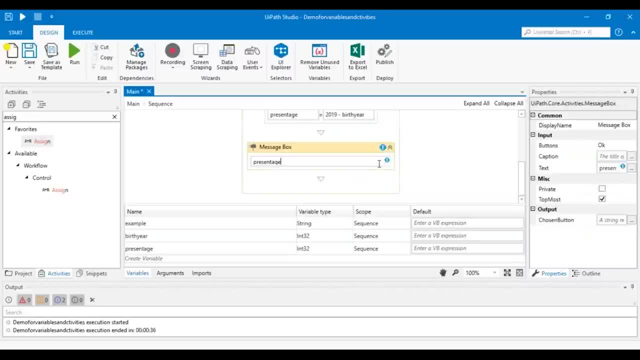 what I'll do is I'll print present age. All right, when you just type in present age, you would see an exclamation in the message box, right? So that's because of you know the message box when it wants to print an output. 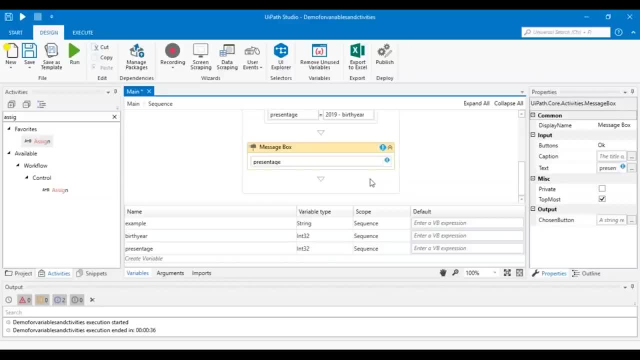 it has to be converted to a string. So when you want to convert the int variable to a string variable, what you can simply do is you just have to type type in to string and you can see that you know if any int variable can be converted to a string variable. 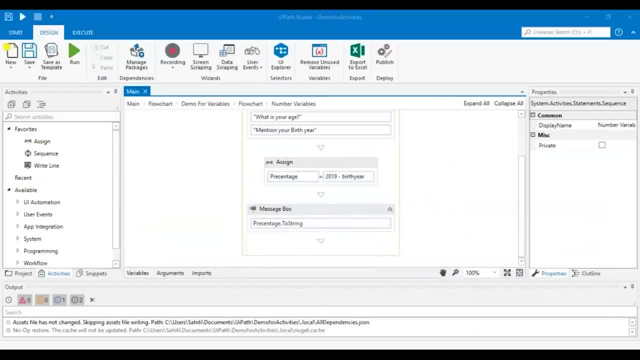 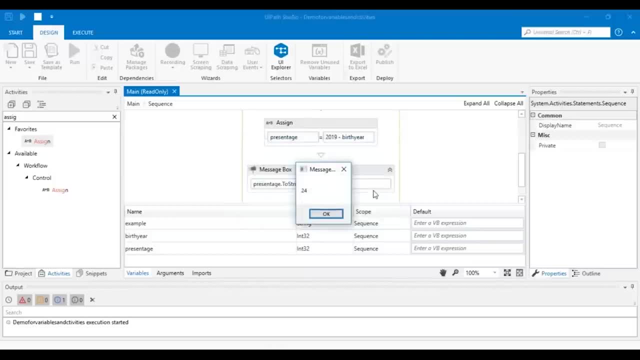 just to print the output right. So now I'll just execute this execution again. All right, So over here let's mention our birth year, suppose 1995.. So on a rough calculation you can see that you know. 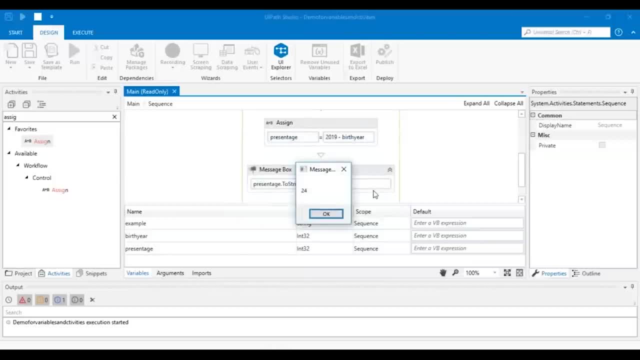 2019-1995 is basically 24 years. So in the message box you would see an output of you know, 24, right? So, similarly, if you want to you know, just print a sentence that you know. 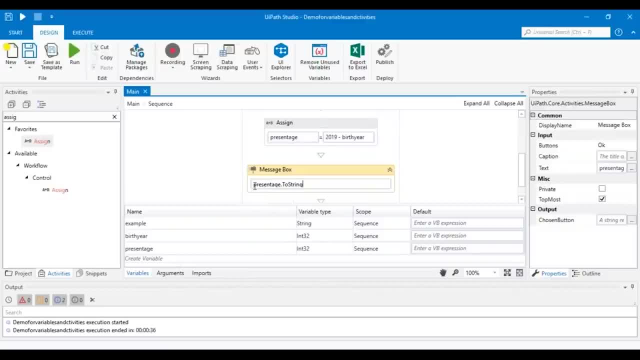 the present age of person X is 24.. What you can do is you can type that sentence out. So for that you'll mention double quotes and you'll mention the sentence that is present age of, let's say, person X is, and then you'll put plus sign over here. 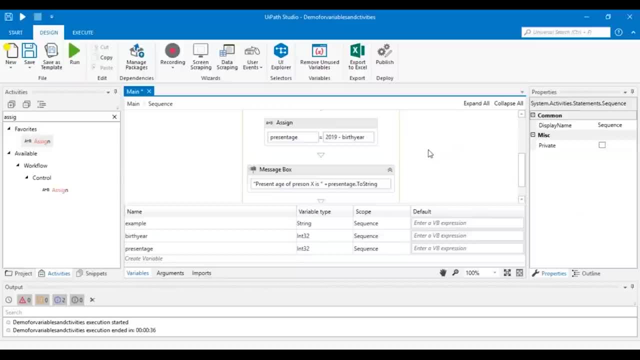 So what will basically happen is the output you would see is the present age of person. X is 2019 minus the birth year that you mentioned, right? So I'll just execute this project again. Let's just mention our birth year again. So let's say I mentioned 1997,. 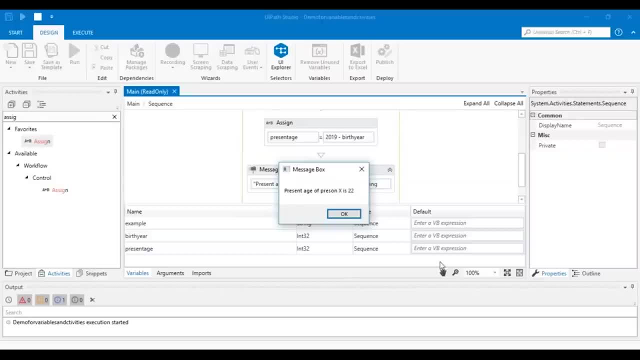 right, I'll click on. Okay, you'll see that you know present age of person X is 22.. So, guys, that's how you know you can integrate text with the variable, so that you know you get a better output. 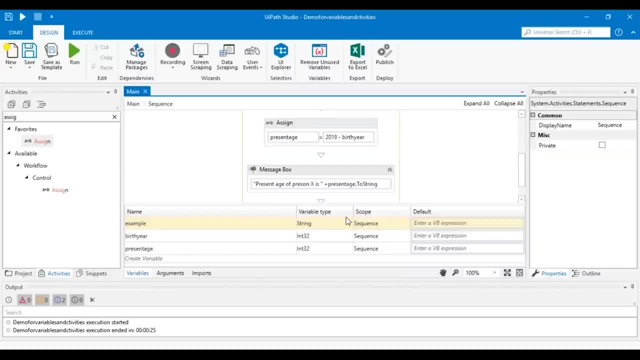 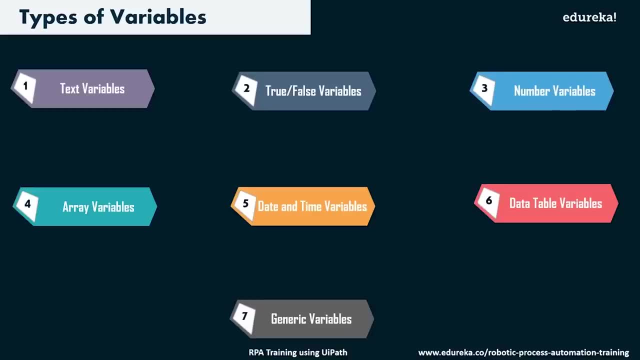 So, guys, these are really basics that you need to understand before you start actually automating tasks with UiPath, so that you clearly see the output right. So, guys, that was all about the different types of variables in UiPath. Now let's move on to our next topic. 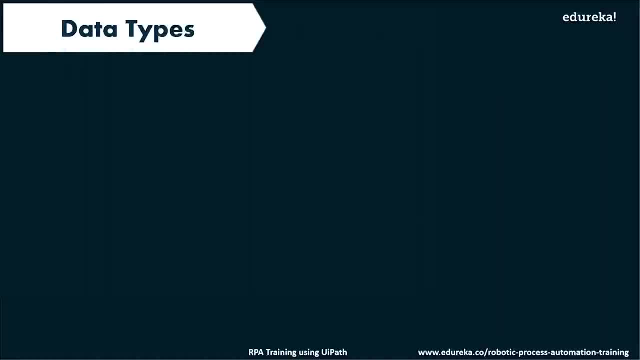 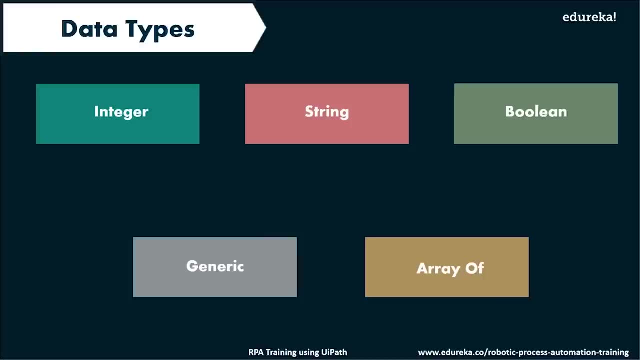 That is the data types. So basically, there are mainly five types of data types in UiPath, That is, the integer, string, Boolean, generic and array of data types. So, as you can see, whenever I created a variable, you would see that. 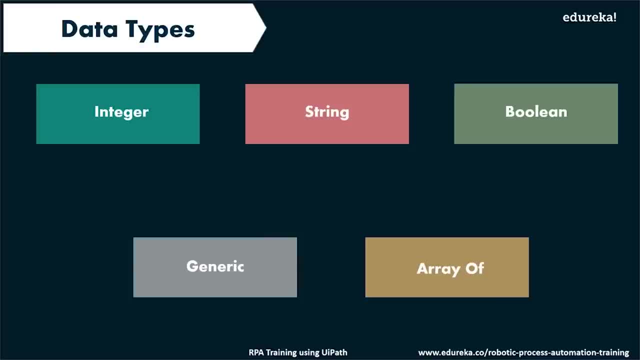 you know, in the variable type we got an basic option of, you know, integer, spring, Boolean, generic and array of. So let's just explore these one by one. So for that I'll shift back to my UiPath studio. 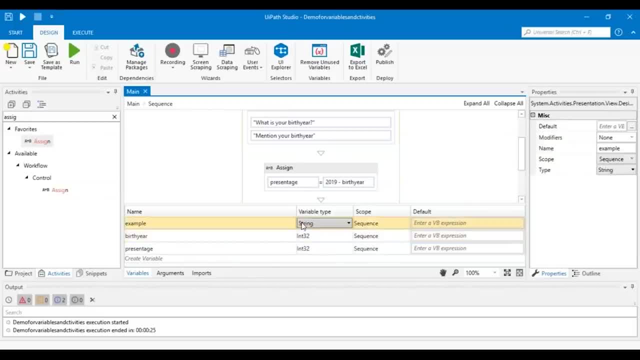 All right. So let's just say, you know I choose this particular variable Now in the variable type, when I click over here, you can see that you know you have an int type, string type, object, array of T and Boolean. 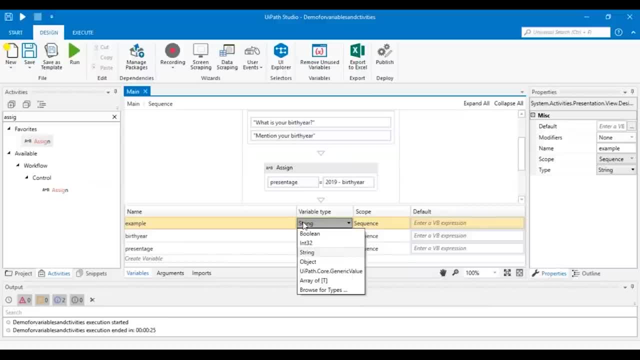 right. So basically, int is basically an integer. Basically all the int values can be stored in this particular data type. The string is basically for the text values. The Boolean is basically for you know, true or false, that is, one or zero. 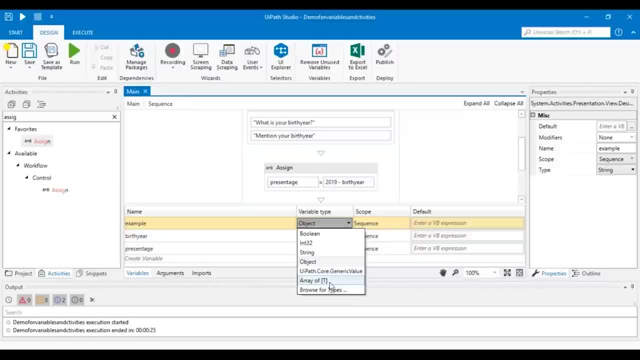 The object is basically to store the object values. Array of T is basically used to store array of any integers. So suppose if I say array of T, then over here for T I'll get various options of you know int Boolean. 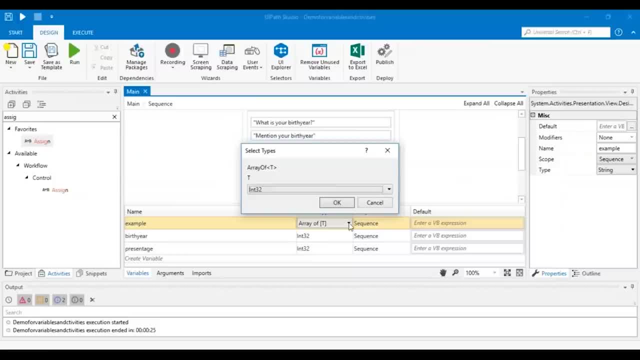 string again, For example, if I want to choose mail merge or something. so what I can simply do is I can just go for browse for type, and then I can search for mail merge, and then I can click on OK right. And once I click on OK, 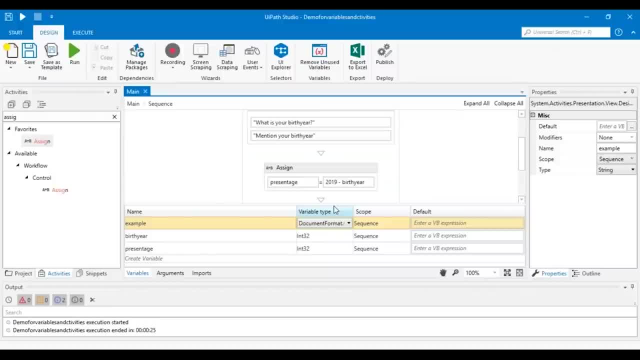 you can again click on OK. So basically, this particular variable, that is, the example variable, will have an array of T, that is, array of mail merges. right, It would basically be an array of many mail merges. Now, that was about data types, guys. 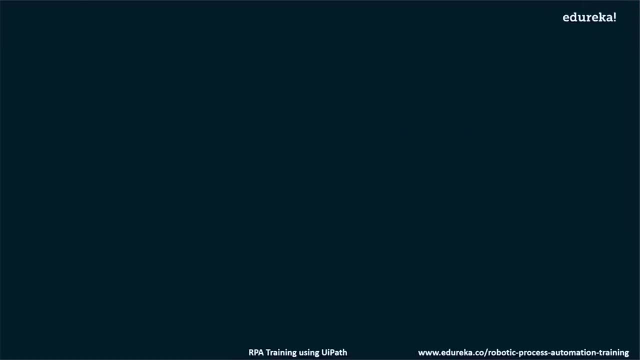 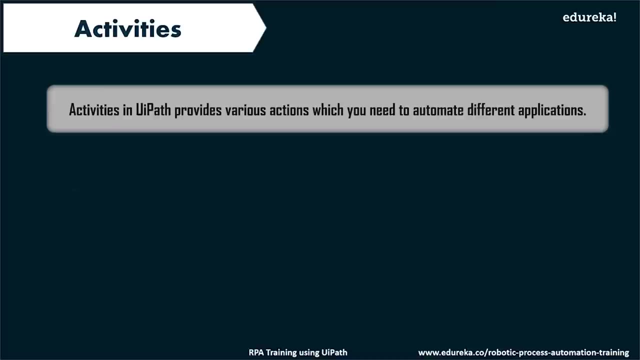 Now moving on to the next main topic for today's session, that is basically activities. Now, since I've already given you examples of you know how to use variables and how to use UiPath. you must have already understood what activities are. 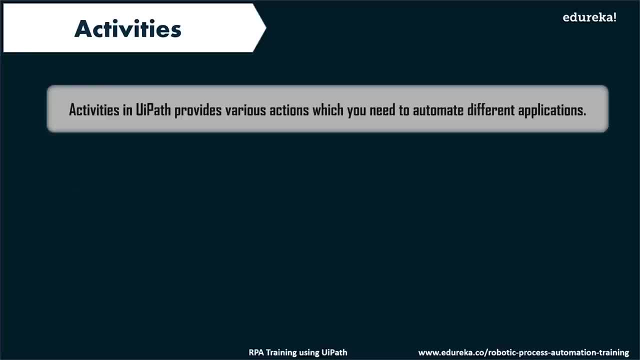 right. So basically, activities in UiPath provide various actions which we need to automate different applications. So basically, when I wanted to just display the output, you saw that. you know I use the message box activity to display the output. 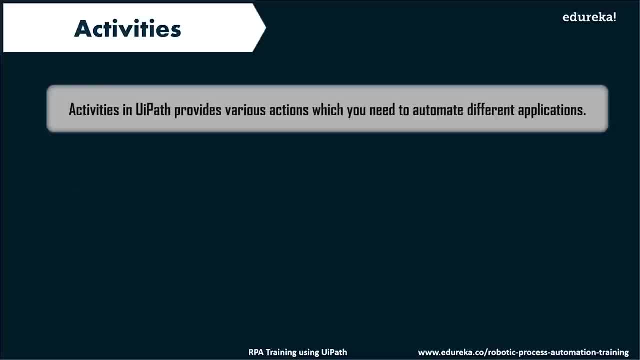 right. Similar to that, I use an assign activity to assign a particular value to a particular variable. So, guys, similar to this, we have various kinds of activities, but in this session I'll be mainly focusing on top eight activities that you should. 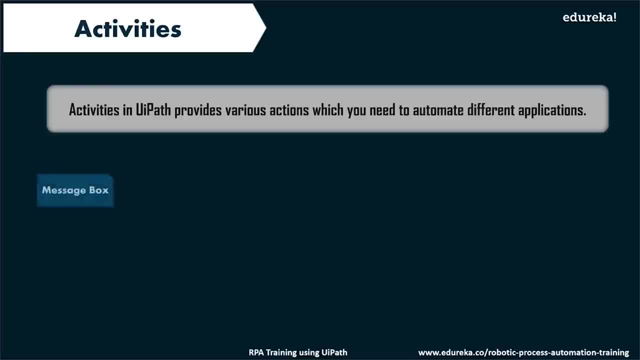 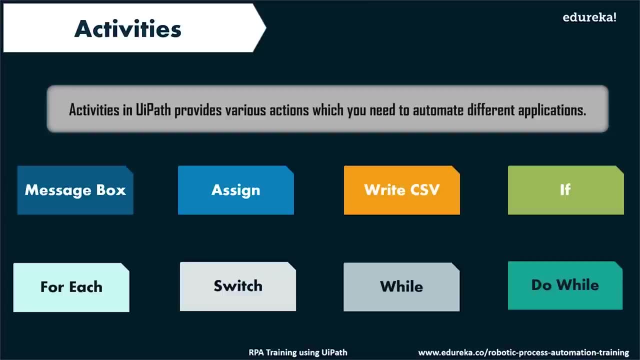 know about in UiPath. So those are mainly the message box: assign, write, csv, if for each activity switch while and do while loops. So basically I'm talking about these activities because, guys, you know, these activity concepts are similar to the programming knowledge. 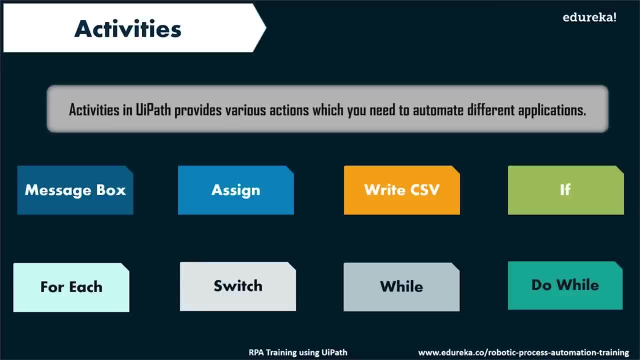 that we have. Whenever we code for something, we would always see that. you know we want to display the output. We would assign few values to a particular variable, We would write the output or, you know, we would just print the output. 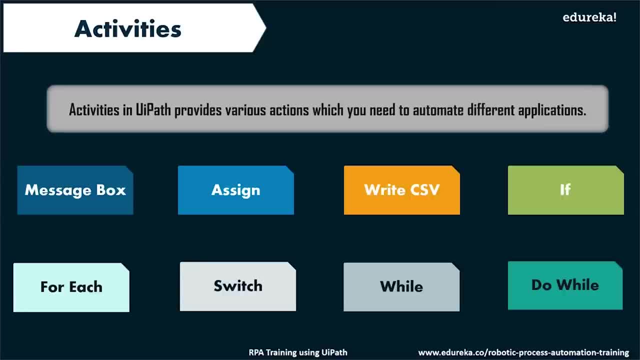 We would use the if loops, the for loop, the switch while and do while loop. So that's the reason I've picked up these activities to discuss. So we'll be discussing about each one of them one by one, and then I'll show you short demos on how to use these particular 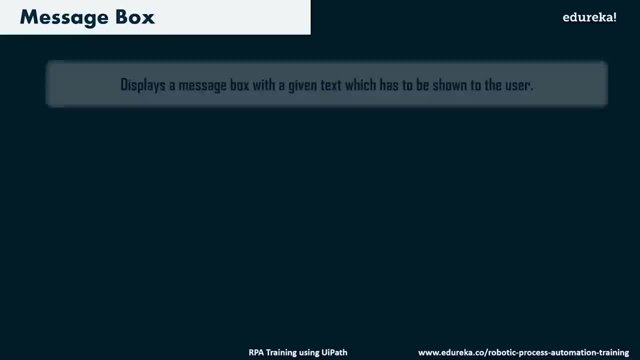 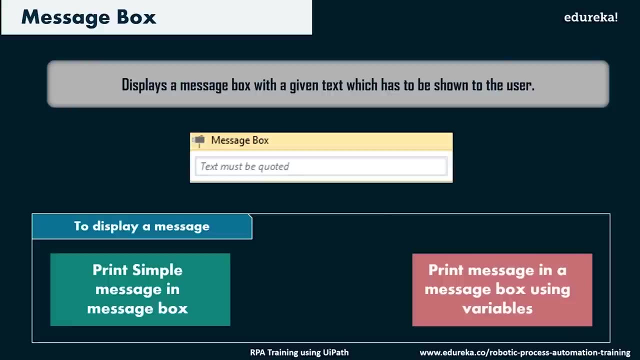 activities. So let's start with the first activity, That is, the message box. So, as you might have already known by now, message box is basically used to display a given text which has to be shown to the user. So basically whenever you want to display an output to the user, 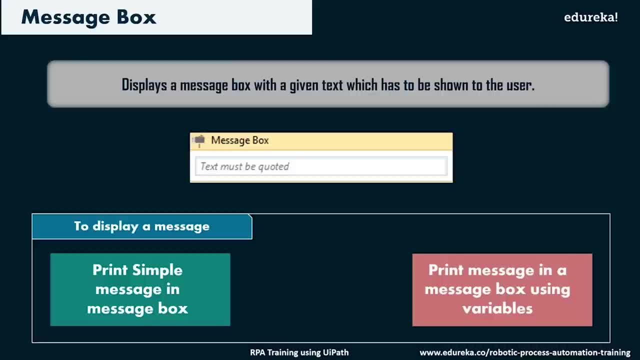 you can use a message box. So now what I'll do is I'll just show you how to print a simple message in a message box that I've already shown you, but I'm just going to show it to you again, and then we'll use a simple variable to display an output in. 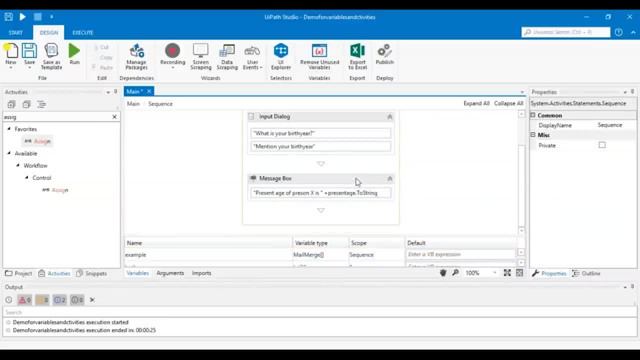 the message box. So what I'll do is I'll just remove this particular assign activity and then I'll just change this particular line to the birth year of person X. So we are. you can clearly see that. you know I am going to use this particular variable of birth year. 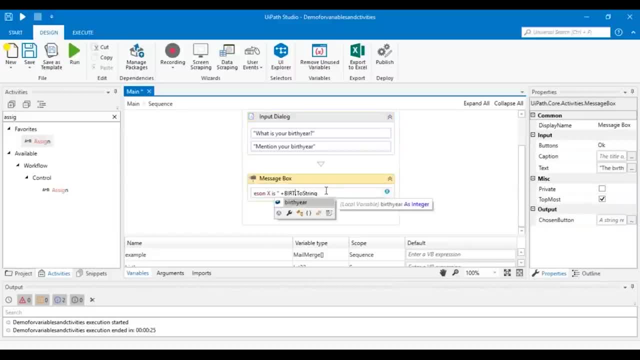 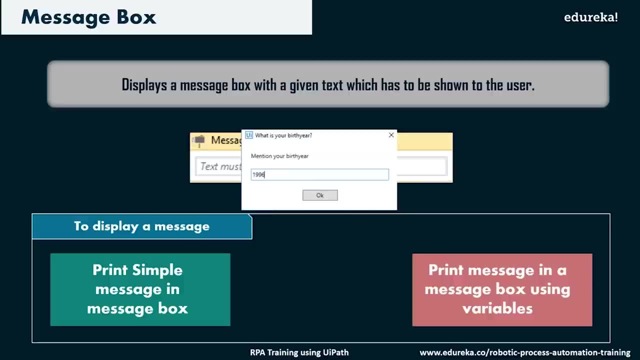 So I'll just change this present age variable to birth year, Right? So now what I'll do is I'll execute this execution again. So let's say, you know I mentioned 1996, right? So when I click on, 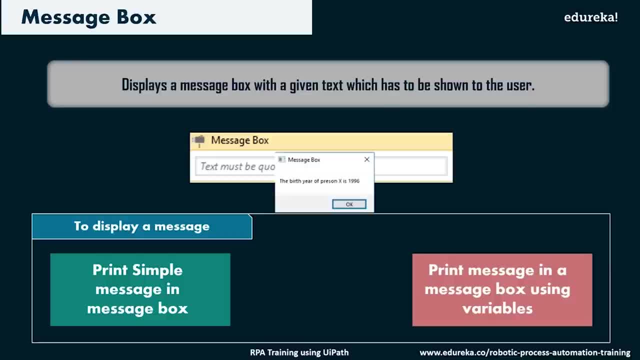 okay, you'll see that, you know you. in the display box, that is basically in the message box, You'll see the output to be the birth year of person. X is 1996.. Right, So we are. what I've done is I've basically done two things, that is. 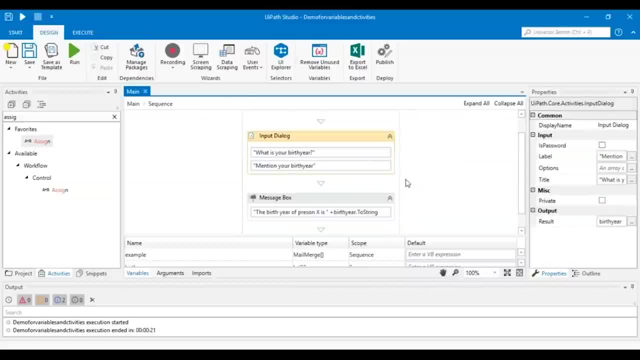 basically, I've used the variable to display a message in the message box And apart from that, I've also used a particular sentence in the message box directly. Right, So you can use a particular sentence directly or particular value in the message box directly to just show the output. 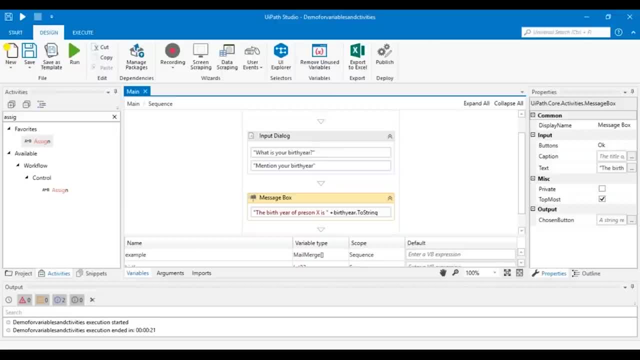 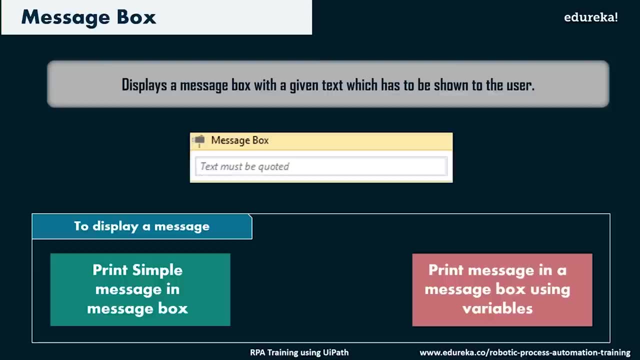 or you know, just display the value to the user, or you can also use a pre-created variable which is already used in some other activity to just, you know, combine it with message box and display the output Right. So, guys, that was all about the message box activity. 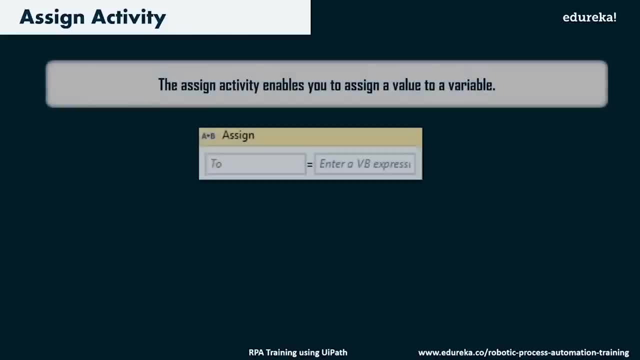 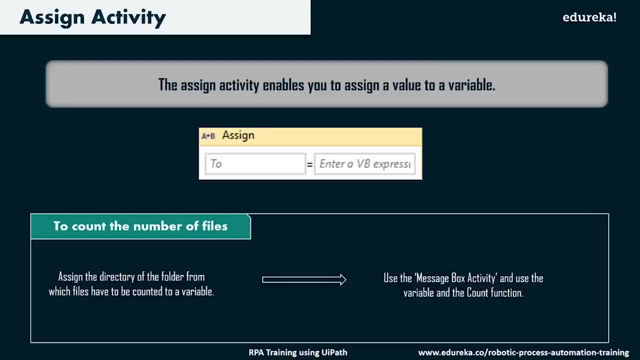 Now let's move forward to the next activity, that is, the assign activity. So the assign activity is basically used to assign a value to a variable. So whenever you want to assign any value to a particular variable, you can use this particular activity. 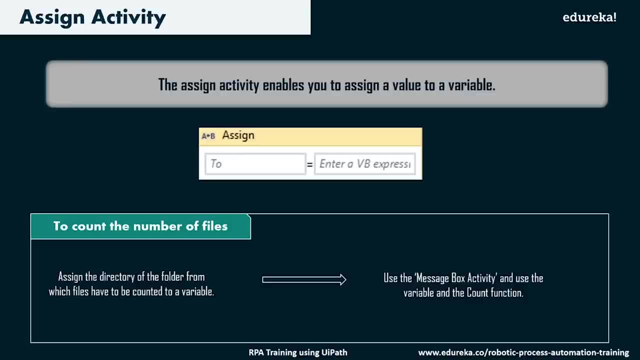 I've already shown you how this works, but let me just show you again. So what I'm going to do is I'm going to count the number of files in a folder and then we'll display the output that you know so many files are present in that particular folder. 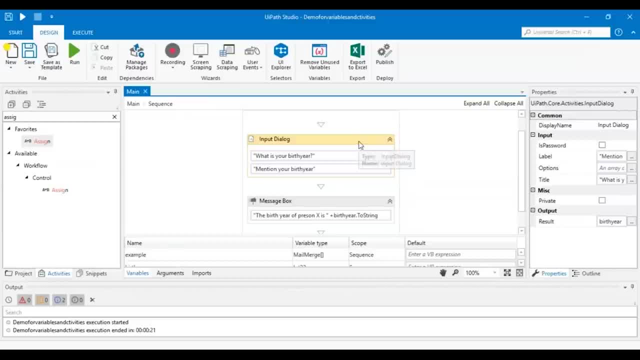 Now to do that. what I'll do is I'll just use this particular sequence and then I'll just remove this input dialog. Now I'll drag and assign activity and over here what we'll do is we'll assign the number of files in a particular folder. 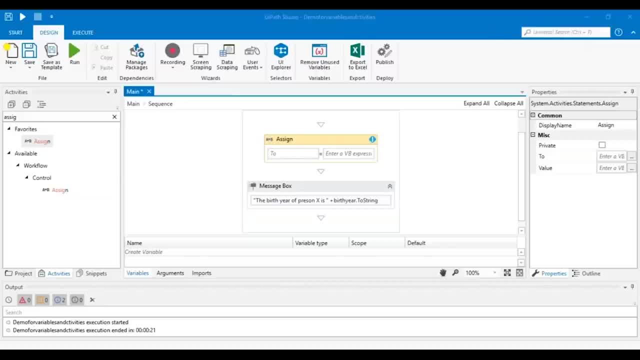 to a variable right. So let's just create the variables first. So to do that, what I'll simply do is I'll just go over here in the variable panel, mention number of files and let it to be of n-type right. 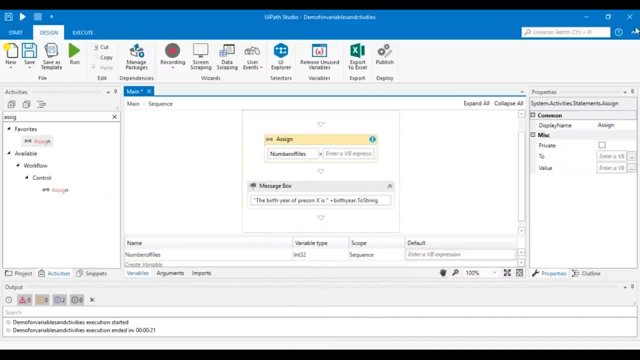 Now what I'll do is I'll just mention number of files. So now what I'll do is I'll assign this number of files to the directory. So for that what I'll do is I'll use the get files function. So for that you have to mention directory dot get files. 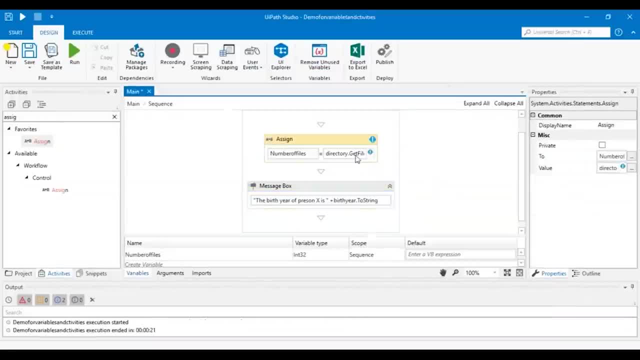 And then in the brackets you can mention source path. So over here, what I'll do is I'll mention the variable of source path And then, before I just conclude this particular execution, I'll just create a variable for source path And in the default value, 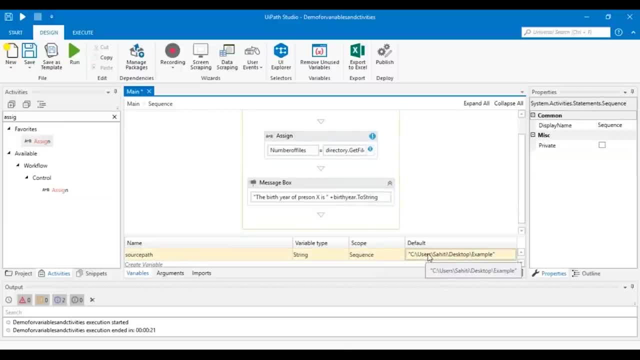 I'll mention the path of the source file, right? So I've mentioned the directory of that particular folder over here in the default value. Now, if you observe over here in the assign activity, you'll see that in there is an exclamation mark. 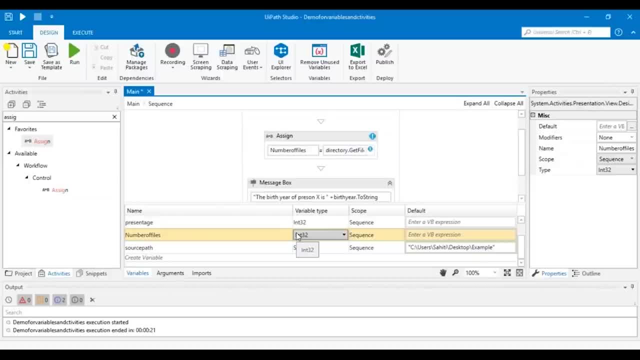 right Over here. what you can do is you have to change the variable type. So I'm sorry, it was not int, It should be array of string, right? So basically, we are getting all the files from a source path where the 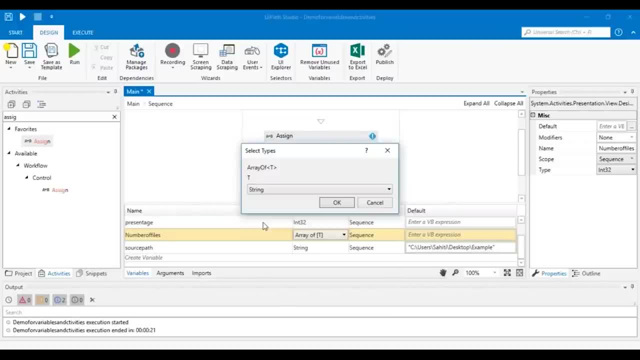 source path is basically a string, right? So what I'll do is I'll just mention string over here. So when you change over here, you'll clearly see that you know. the exclamation mark is gone right now in the message box. 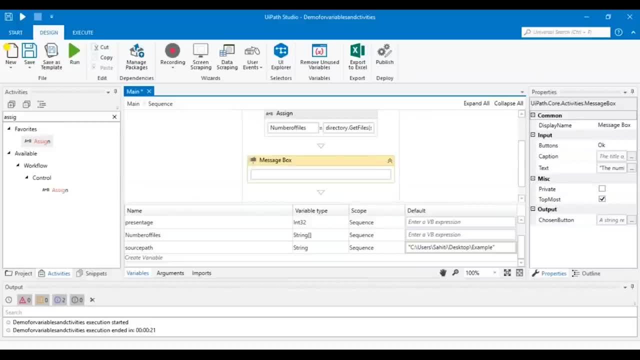 What I'll do is I'll mention a sentence where you know the number of files in the particular folder are so on. So basically the count would be mentioned over here. So over here I'll just mention the sentence in a double quote saying the: 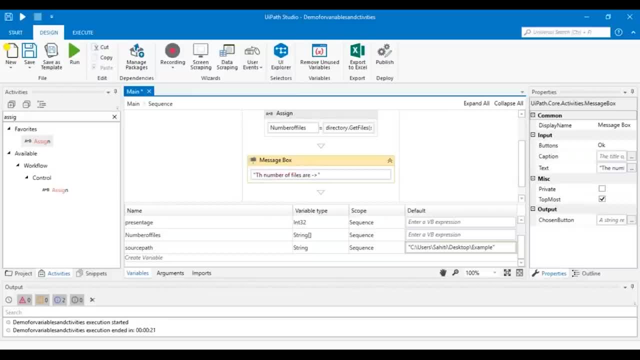 number of files are, and then I'll use plus. I'll mention the variable, that is, number of files. I'll convert into count, So basically it would count the number of files and then we'll convert the complete value to string. right? So that's how you can do it. 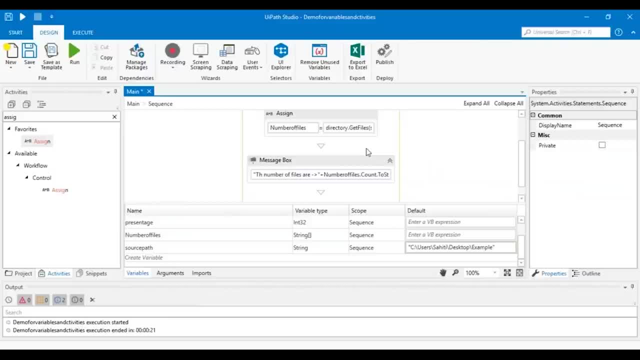 So basically, what I'm doing is I've assigned the source path to a particular variable and then I'm using the get files function to get all the files from that particular source path and then assigning that particular value to a particular variable, and then I'm just displaying the output in a message. 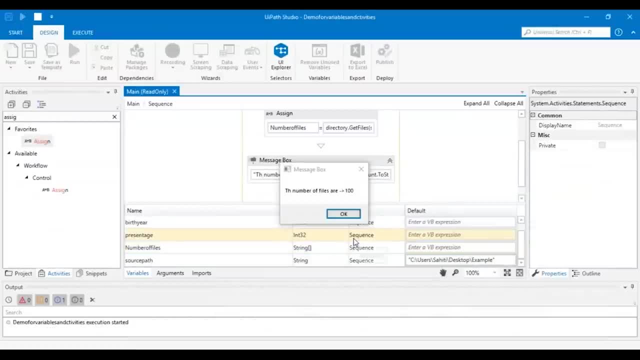 box, right? So I'll just execute this particular execution. All right, so you can clearly see that we've got an output that you know. the number of files are basically hundred, right? So, guys, that's how you can use the assign activity. 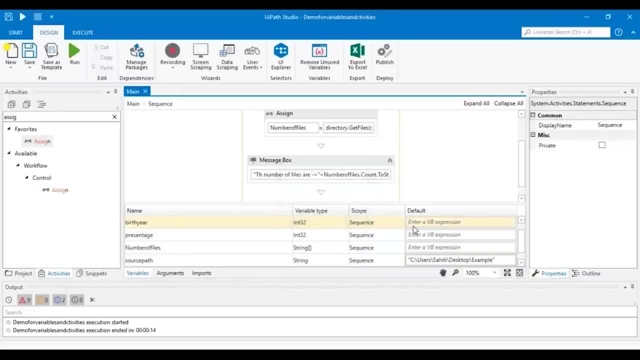 You can use this assign activity to assign a particular value to a variable, So that value could be any kind of value, like you know: integer value, string value, an area of values, and so on. So that's your call, basically. now moving on to the next type. 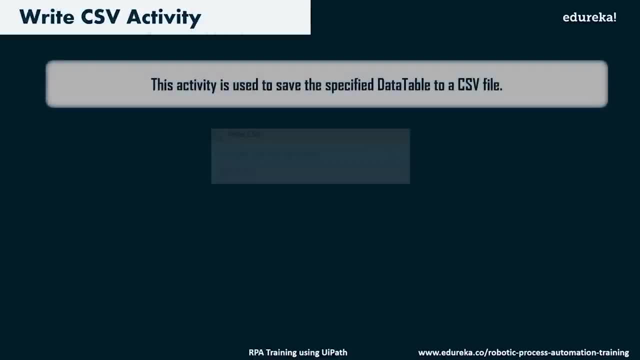 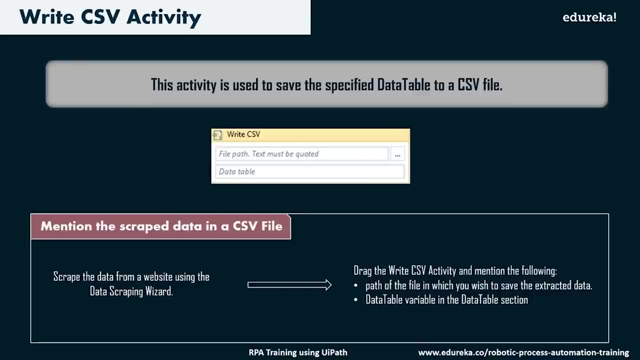 of activity. That is basically the right CSV activity. The right CSV activity is basically used to specify a data table in a CSV file. So basically, whenever you want to specify a data table in a CSV file, then you can use the right CSV activity. 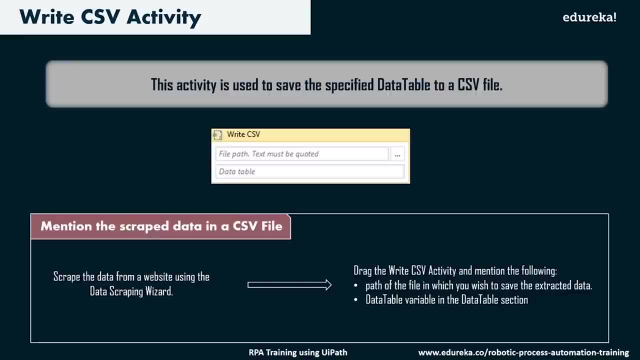 So now let me just show you how to use this particular activity. So for that, what I'll do is I'll just scrape the data from a website and then I'll store it in a CSV file, right? So let me just shift back. 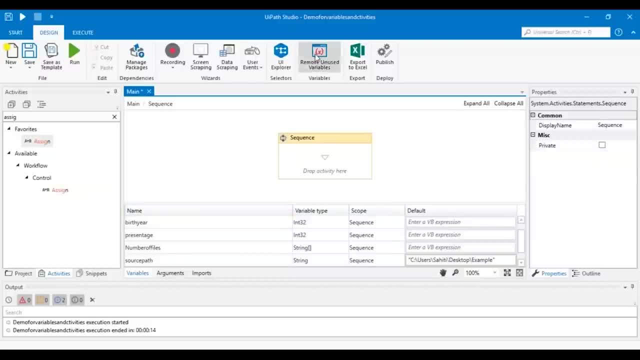 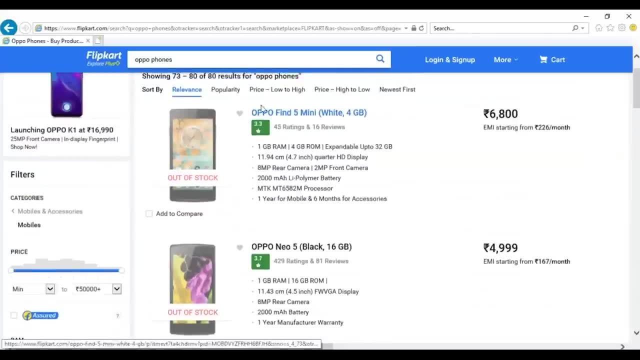 Now what I'll do over here is I'll just remove all these activities and all the variables. Right now, what I'll do is I'll just open in the Internet Explorer a website, and then what I'll do is I'll scrape this website, Right. 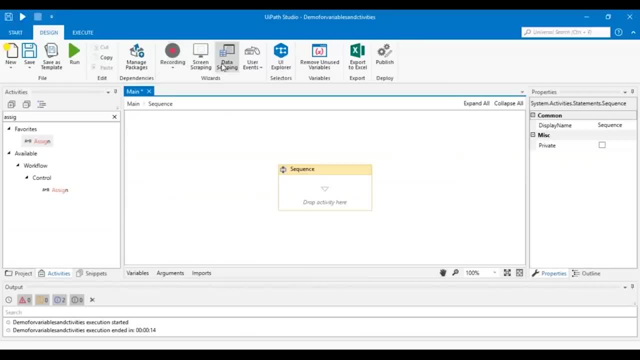 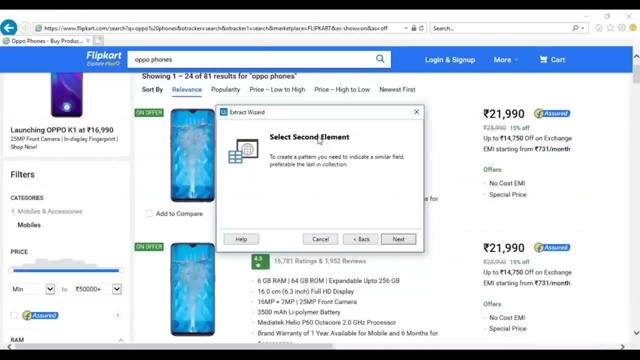 So I'll just open this particular website Now. what I'll do is I'll go to the data scraping option. I'll choose the elements, So I'll click on next and mention this element, then after choose the second element to create a pattern. 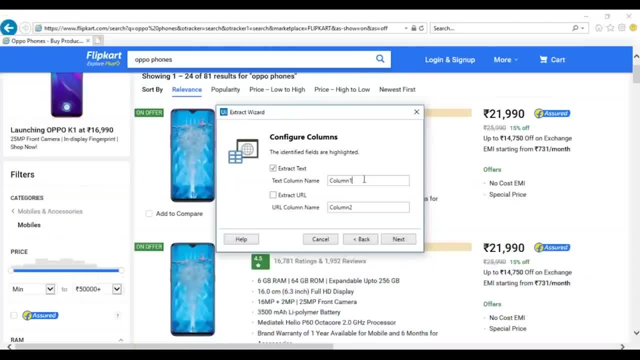 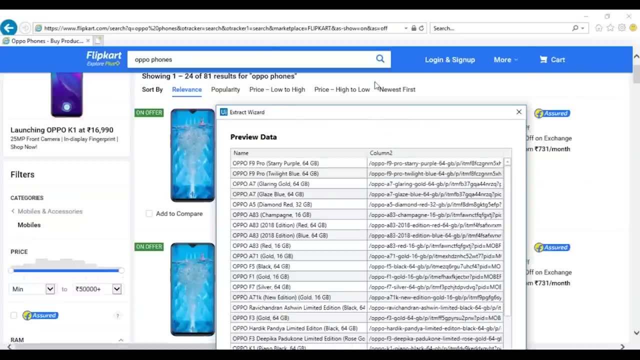 I'll again click on the second element to basically create a pattern. and then let's say: you know, we mentioned the column name to be name and we also want to extract the URL Similarly. I'll click on next and then you can see that. 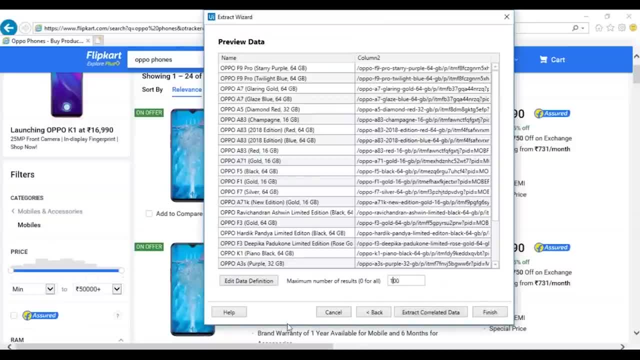 you know so much data will be extracted, Right? So let's say you know the maximum number of records are basically 500.. So basically we can see that you know whatever data has been there in the following pages also will. 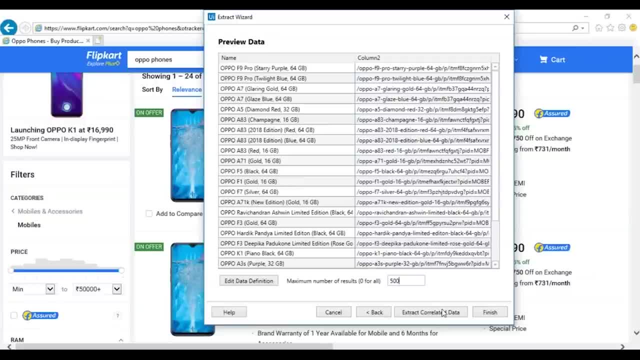 be extracted. So I'll show you how that's happening. But before that, what you can do is we can also extract correlated data. So for that let's say you know we want to extract price, I'll just choose over here. 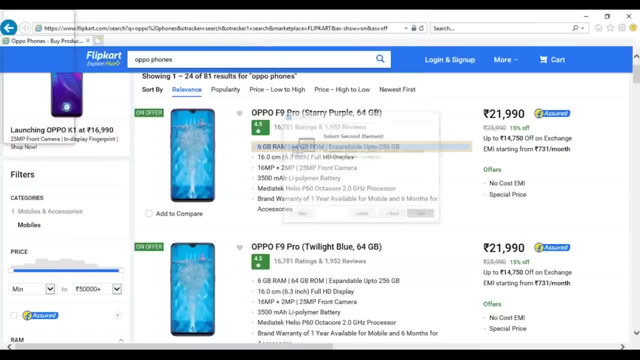 I'll just click over here and then I'll click on next to basically, you know, create a pattern again. So I'll click on next and I'll choose the second element. So I'll just mention this column name and click on next. 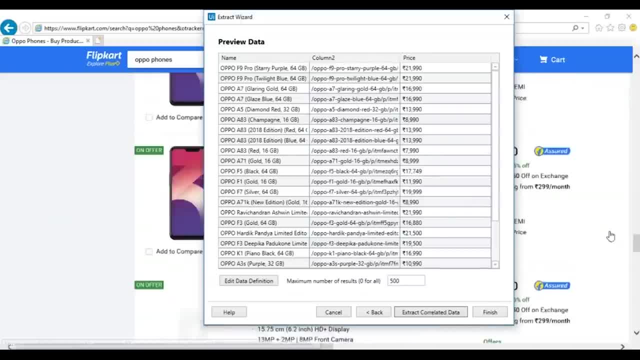 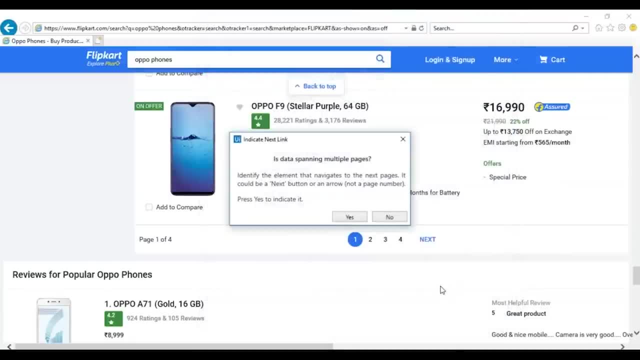 You'll see that in a price has been extracted. Now I'll just click on finish on this particular wizard to basically finish The Acting part. So I'll just click on finish and then you'll see an option of you know if you want to span the data across multiple pages. 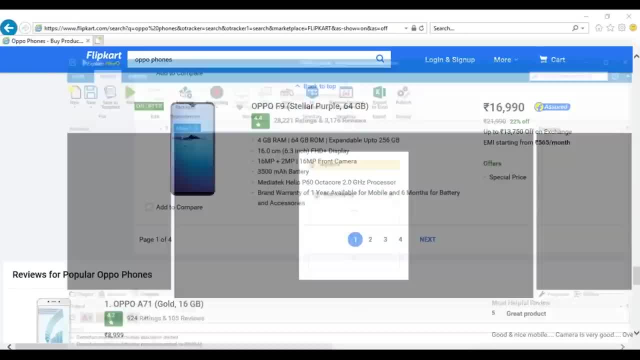 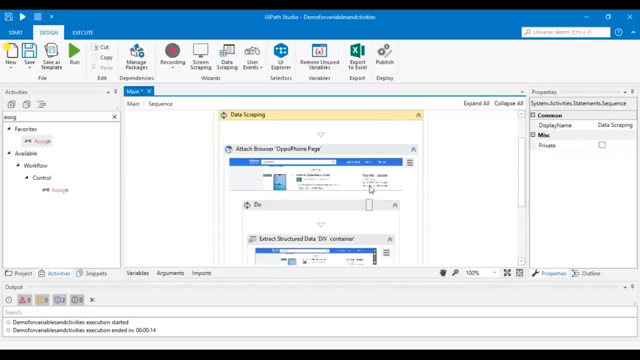 So what I'll do is I'll click on yes to indicate so. I'll choose this option of next and you'll see that you know my data scraping wizard is ready right now. in the data scraping wizard You'll clearly see that your browser has been attached and 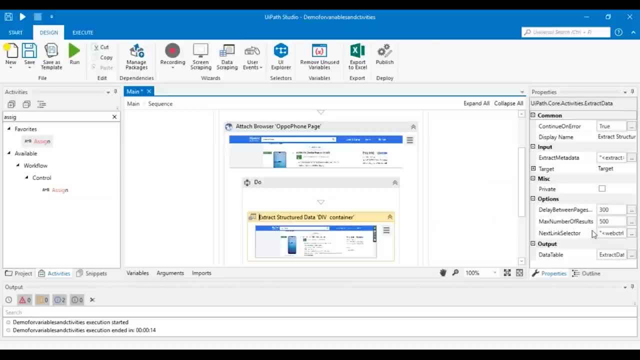 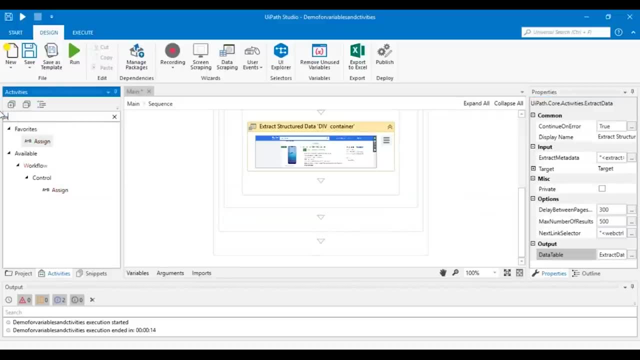 then what data has to be extracted will be stored in this particular variable, That is the data table variable right now. if you want to store the extracted data into a CSV file, then you have to use the right CSV activity. So for that I'll just drag and drop it over here. 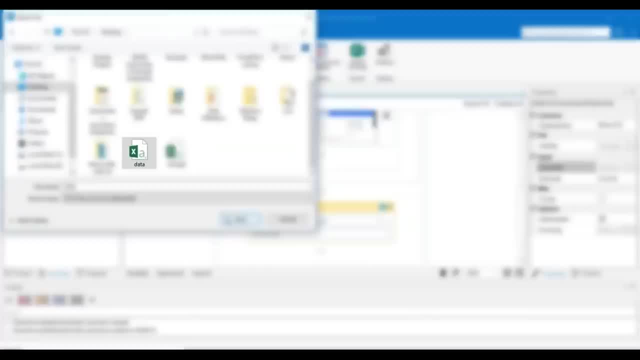 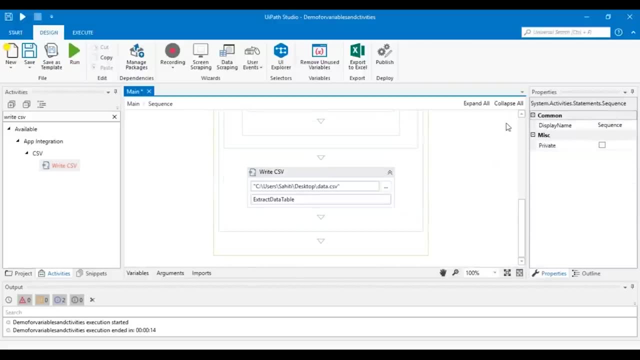 And then I'll mention the file path. So I'll browse for types and let's say, you know I mentioned data right, and in the data table option I'll mention the extract data table, right. So that's how you can use this particular activity, guys. 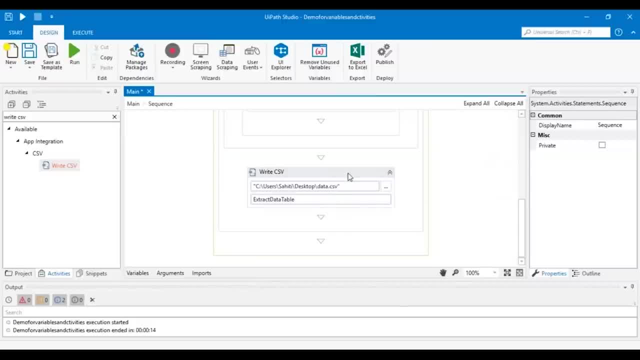 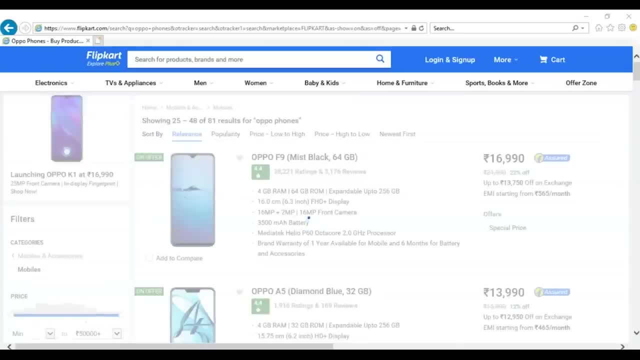 You have to just mention the path of the CSV file and then you have to mention the data table variable. So let's just click on run and let's wait for the execution to happen. So, as you can see on the screen, your data is getting scraped. 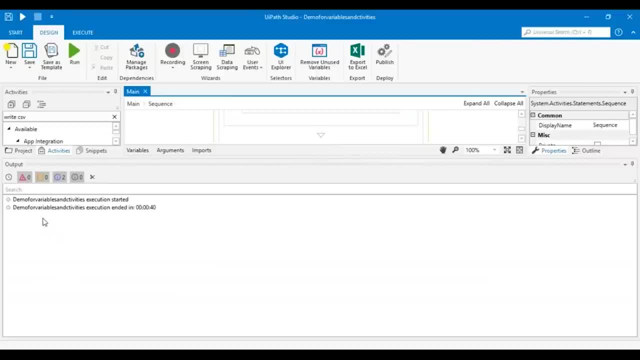 from the multiple pages right. So in the output pane you can clearly see that you know the execution has ended. That means our data must have got stored in the data CSV file. So let's just open that particular file and see. 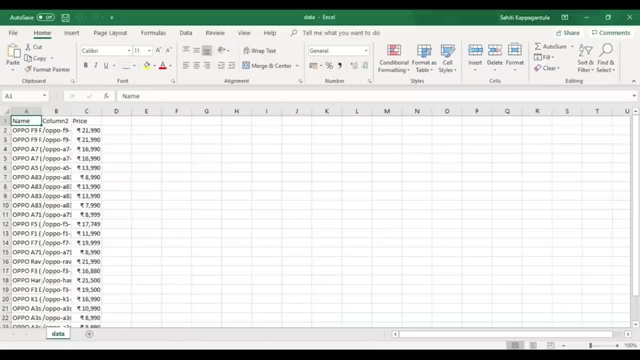 So, as you can see on my screen, you can clearly see that you know the name, the column and the price have got extracted and they're stored in this particular file, right? So basically, guys, that's how you can use the right CSV activity. 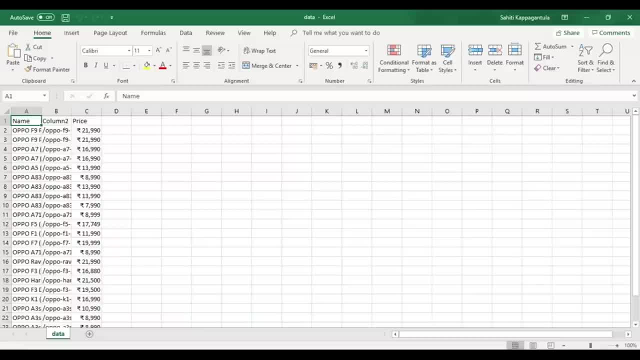 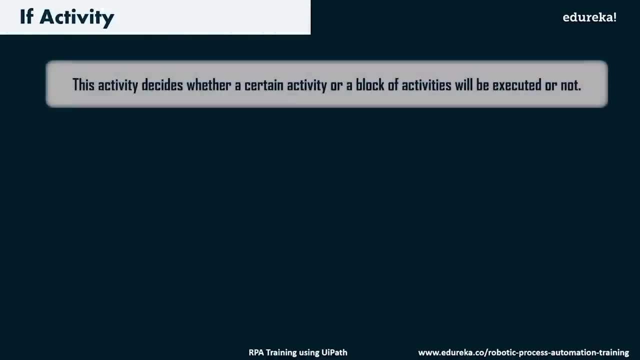 So whatever data you scrape or you know, whatever value that is stored in a data table variable can be stored by using the right CSV activity. Now moving forward to the next activity, that is, the if activity. now, if activity, like in any other programming language. 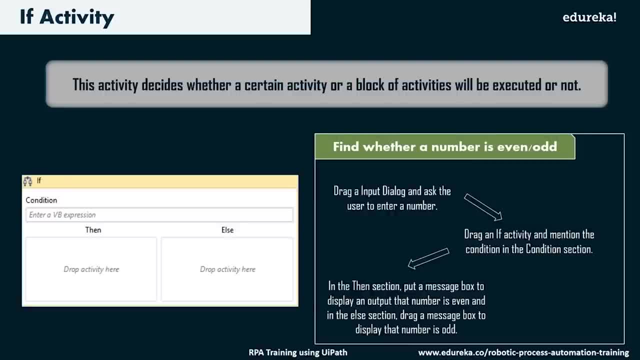 basically decides whether a certain activity block or a block of activities will be executed or not. So you must be knowing about the if-else condition right. So if the condition holds true, then a set of activities or you know the set of tasks would be done. if the condition holds false, 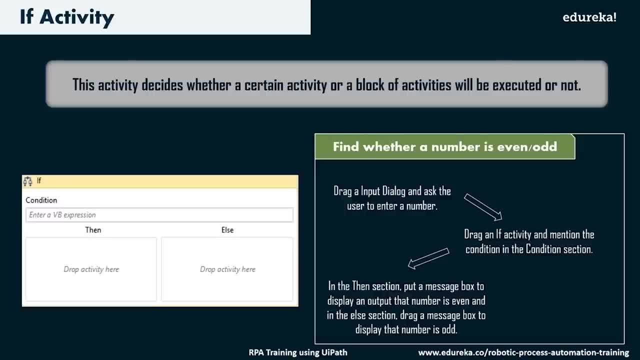 then a set of something else would be done, right? So that's what happens in UiPath Also, We have an if activity in which basically we have to mention the condition and then we have to basically mention the activities that has to be performed. whether you know. 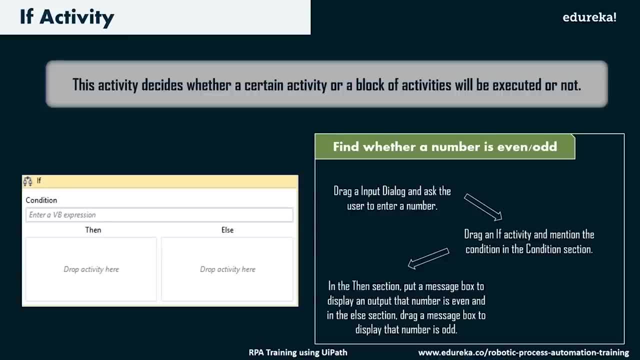 when the condition holds true and when the condition doesn't hold true, right. So now, what I'm going to do is I'm going to find out whether the number is even or odd. So, for that, what I'm going to do is I'm going to drag an input. 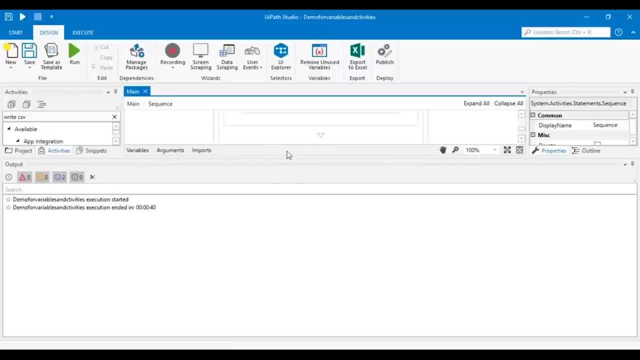 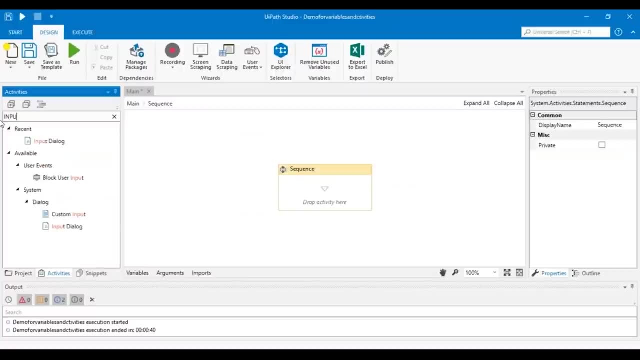 dialog first. So let me just shift back and then let me just drag this down. I'll remove this part and now what I'll do is I'll drag an input dialog right over here, I'll say what is the number And let's say: mention your number. 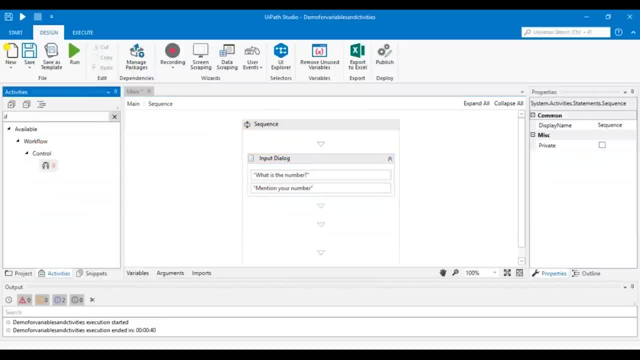 Right and over here will drag an if activity underneath that number. And when you drag an if activity you can clearly see that you know we have a condition block and then an else block. that basically means when the condition holds true, the then block would be. 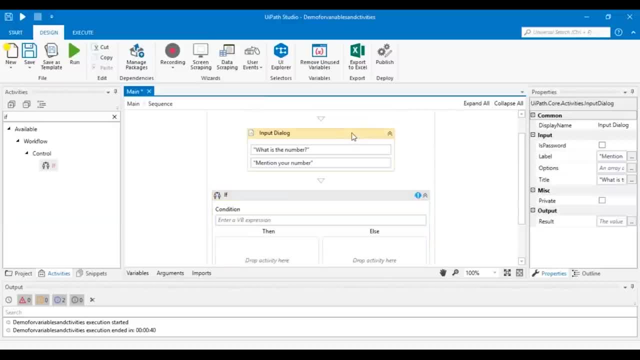 executed, else the else block would be executed, right? So, but before that, in the input dialog, let's create a variable and let's say number. So, basically, whatever number that we give as an input would be stored in this particular variable, right? 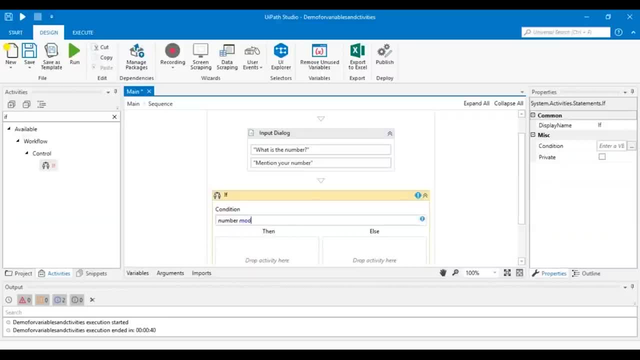 Now we'll use the condition. that is basically number mod 2 equal to 0,, right? So when a number is divided by 2, and if it gets a value of 0, that is basically a reminder- is 0, that means. 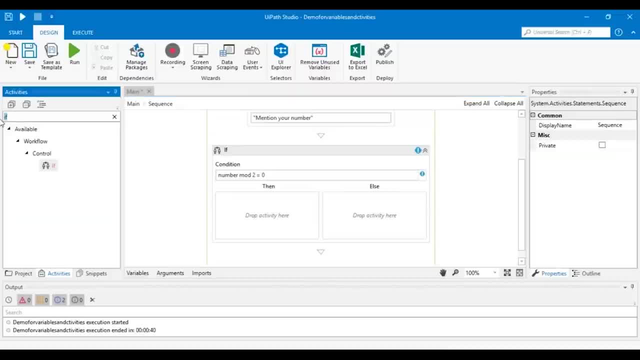 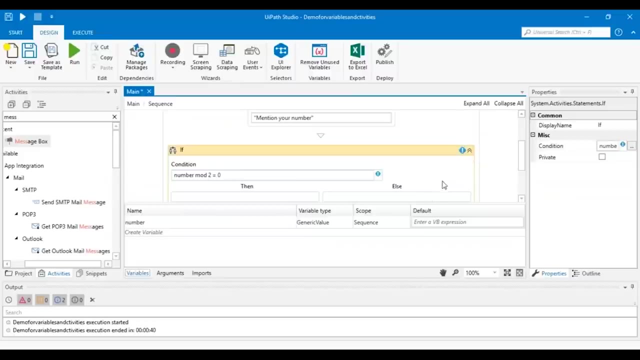 you know the number is even, else the number is odd right. So for that will display a message box in the then condition which says number is even and in the else block will say number is odd Right now in the variable type. 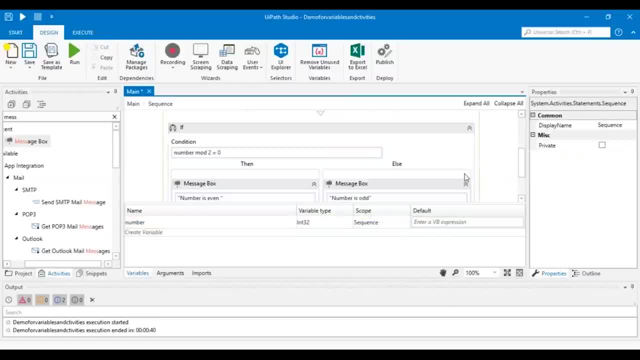 Let me just change this to end first, right? So when I change the variable type to end, you'll see that. you know, the exclamation mark is gone right Now. what I'll do is I'll just execute this particular sequence. 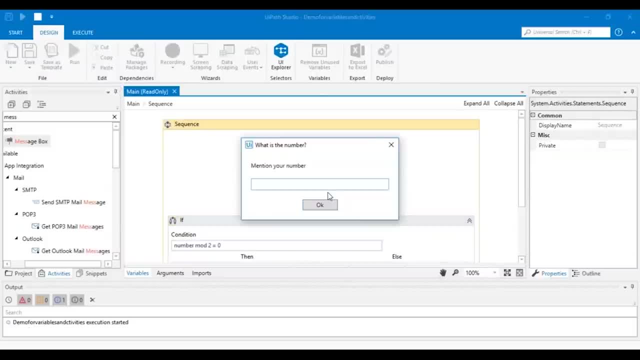 So let's just execute this particular sequence. So let's say I mentioned 456.. I'll click on OK and you'll see the output that you know. the number is even right. So because 456 is even now, similarly, let's execute it again and let's put an odd number and see if. 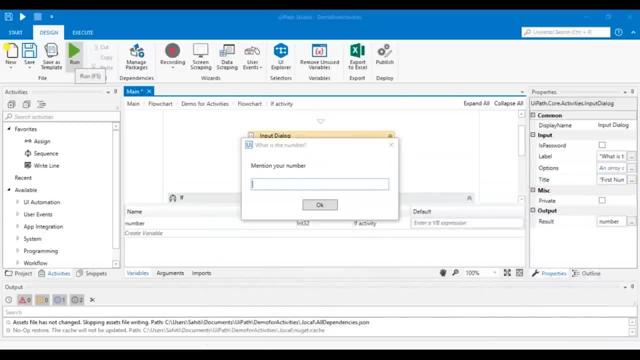 you know the condition: prints or not. That is basically if the output prints the number is or not. So let's say 987, right? So I'll just type in 987 and you can see the output that you know. the number is odd. 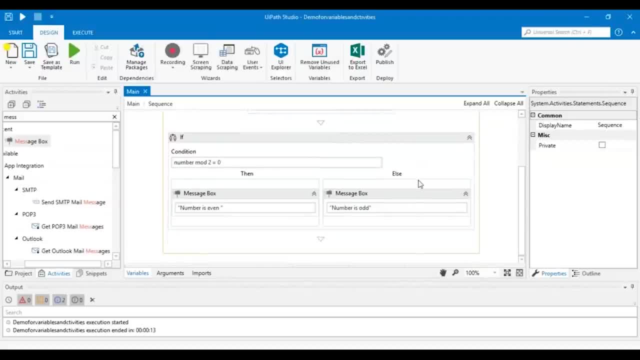 right. So, guys, that's how you know the if condition works. So, basically, it completely works on a condition that whether, if your condition holds true, then the then block would execute and else the else block would execute. Now, over here, I've just mentioned a single activity, guys else, 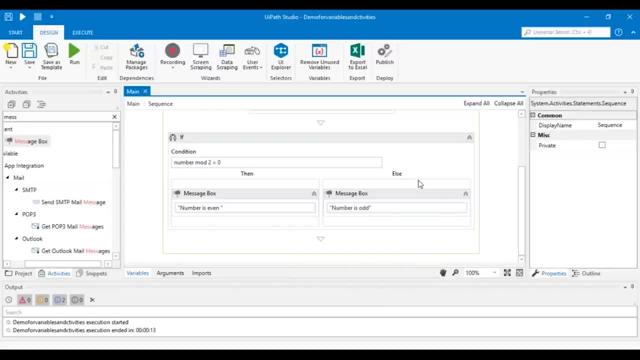 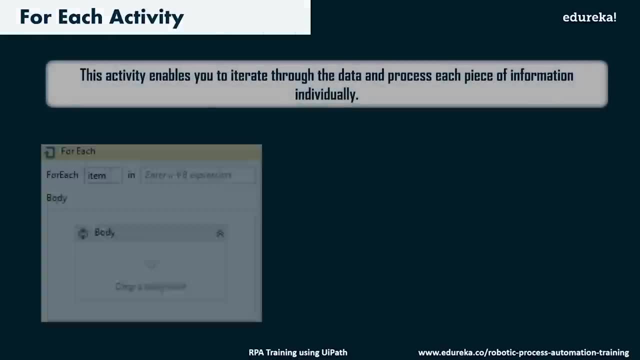 You can also mention a flow chart under which you can have n number of activities, right? So, guys, that was all about the if activity. Now let's move forward to the next activity, That is, the. for each activity There's a. for each activity is very much similar to the fall. 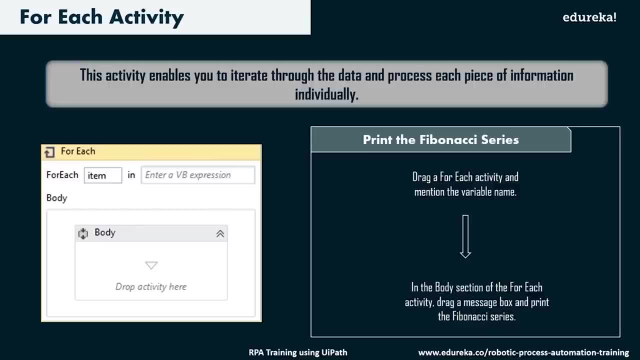 loop in our programming world. So the for each activity basically enables You to iterate through the data and process each piece of information individually, right, Whenever you want to iterate through the data, then you can use the for each activity. So when you drag the for each activity, 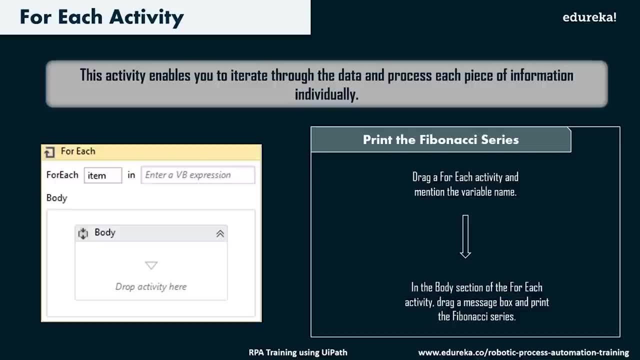 you would see in the blog that you know for each item in a variable expression, right? So you basically have to mention the expression over there. That is basically a variable, and then for each item in that particular variable expression, a set of activities would be. 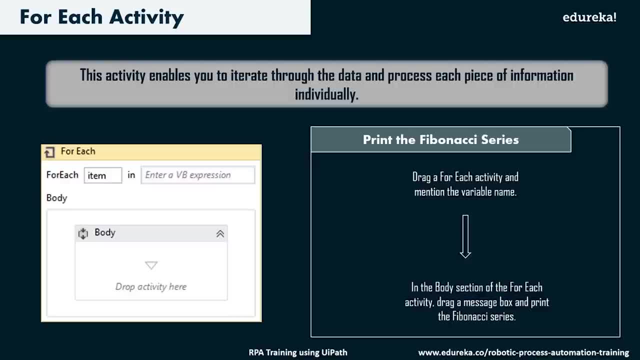 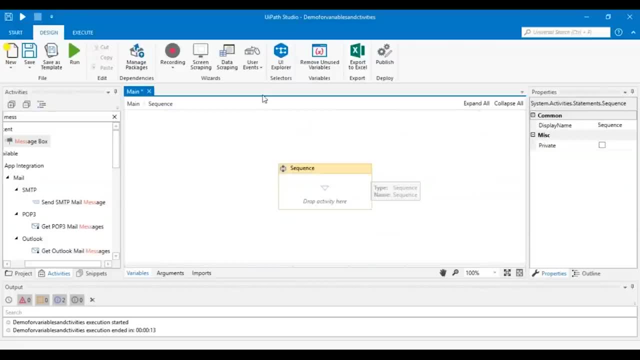 executed, that would be mentioned in the body section, right? So for now, I'm going to show you how to print the Fibonacci series. So for that, what I'm going to do is I'm going to drag the for each activity. So for that. 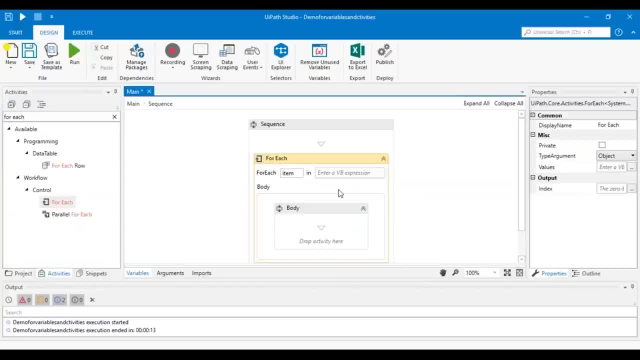 let me just remove all these and search for for each activity. Now, what I have to mention over here is that you have to mention a variable expression. So let's say FB series, right, So that's what I have to create. So let's say: 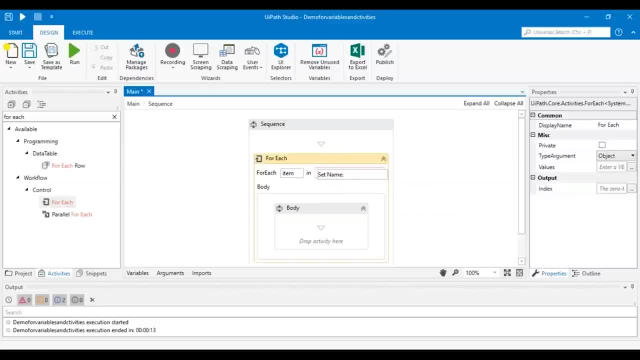 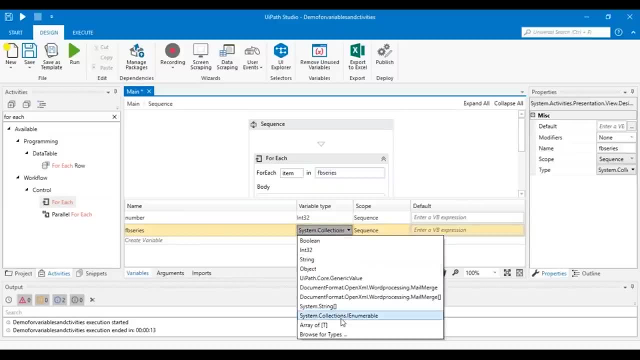 you know I mentioned a variable to be FB series, So I can press on control K over here. mention FB series. go to the variable panel right. So in this variable type I'll mention array of T and it has to be of integer variable. 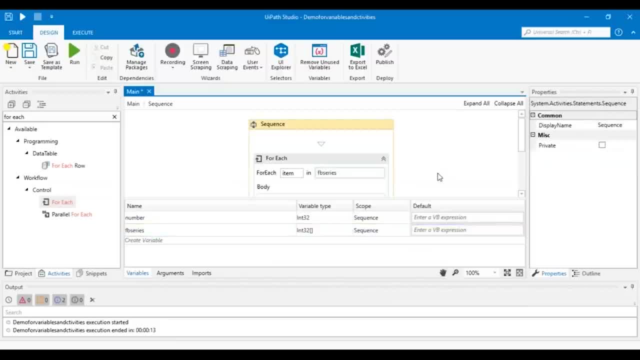 It's right. So I'll click on OK. So you'll see that you know this will be an array of integer variables and over here I can mention the default values. So I'll mention the Fibonacci series. So let's say I'll mention till 89,. 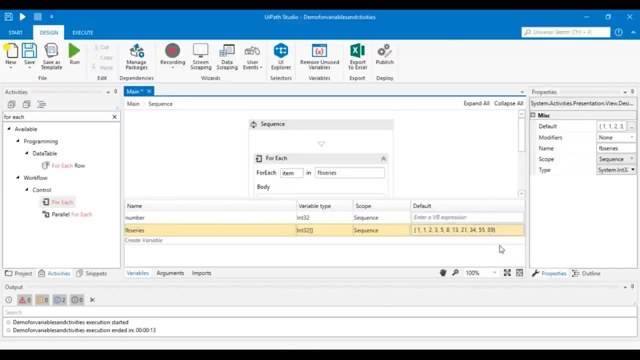 right. So, as you can see, I have mentioned the Fibonacci series till 89.. So now to print the Fibonacci series, I'll just put a message box which would say that you know, the number in the Fibonacci series is so much. 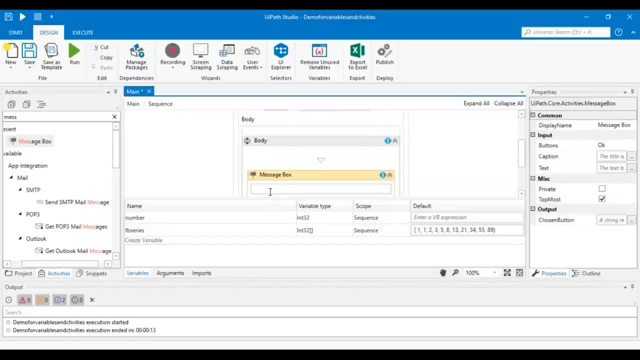 So for that, what I'll do is I'll search for a message box, I'll drag and drop it over here and in double quotes I'll mention the number present in the Fibonacci series is, and then I'll put a plus sign and mention the FB series sequence. 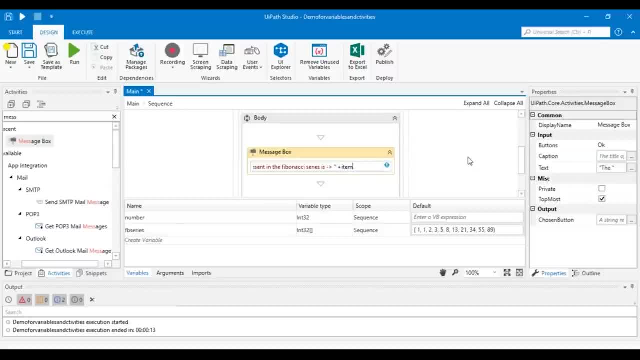 That is FB series. I'll mention item to string right. So according to whatever you've mentioned in the default value for your variable in FB series, that is still 89, your message box would continuously display the output of you know. 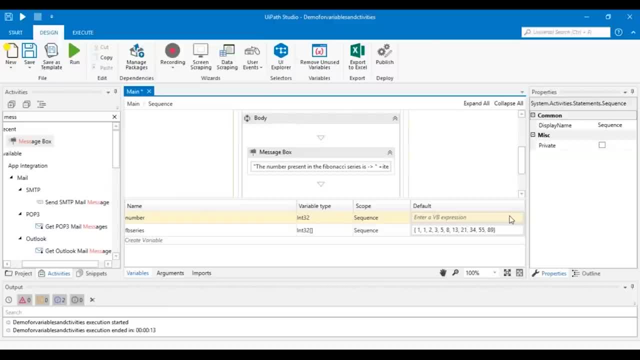 every item. So it would first display the output for one, then one again, then two, three, five, eight and so on. So since you know it would take time, I'll just remove from 13.. So let's just keep it till eight over here. 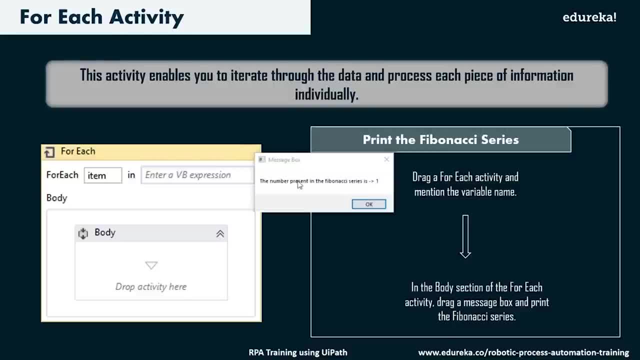 Now let's just execute this particular execution. You'll see an output that you know the number present in the Fibonacci series is one. If I click on okay, you'll see again an output that it's again one, then two. 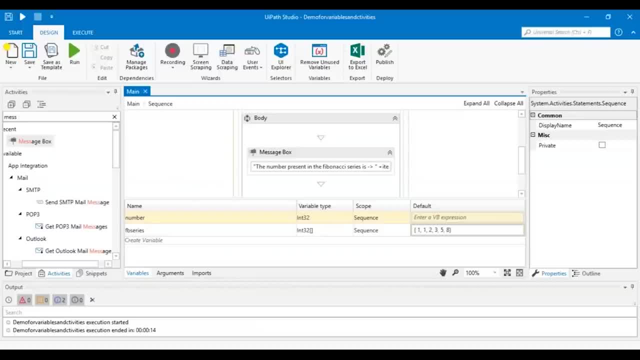 then three, five, eight, and then, when I click on okay, finally, you would see that you know you'll be redirected to your dashboard, right? So, guys, that's how you can use the for each activity, So for each item. 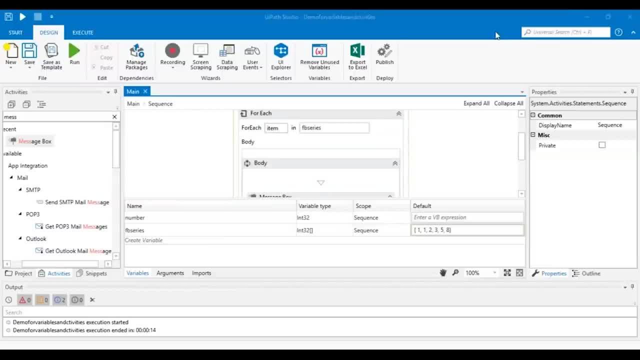 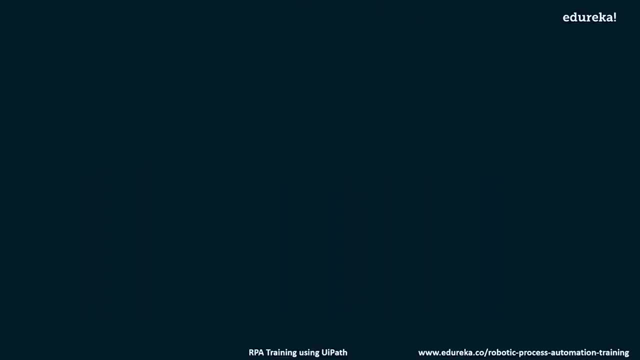 in a variable expression, you would see that your loop is getting executed again and again, right? So that was about for each activity, guys. Now let's move forward to the next activity, That is the while activity. So, basically, this activity enables you to execute a specific 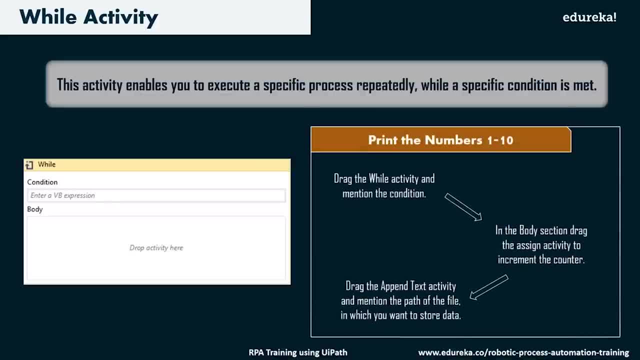 process repeatedly while a specific condition is met, right? So basically, while a condition is met, you will see that you know something is getting executed repeatedly, right? So basically that something could be a single activity or a block of activity. So that's completely on what kind of automation that you're. 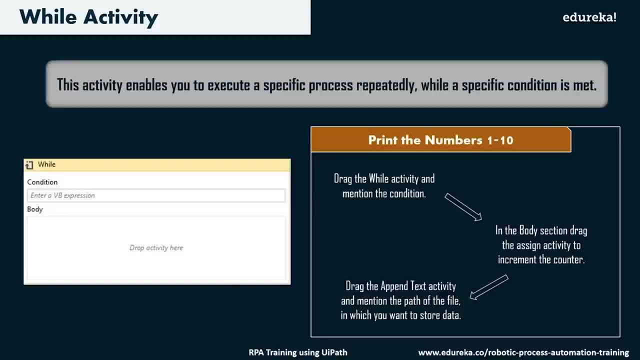 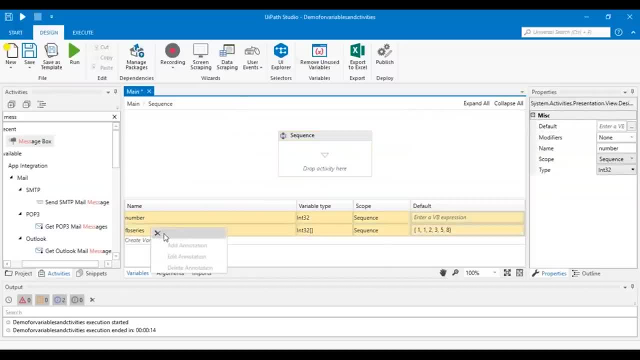 performing. But for our scenario, what I'm going to do is I'm going to print the numbers from 1 to 10.. So let's just do that. So I'll just remove this. for each activity, I'll remove all the variables so that there's no confusion. 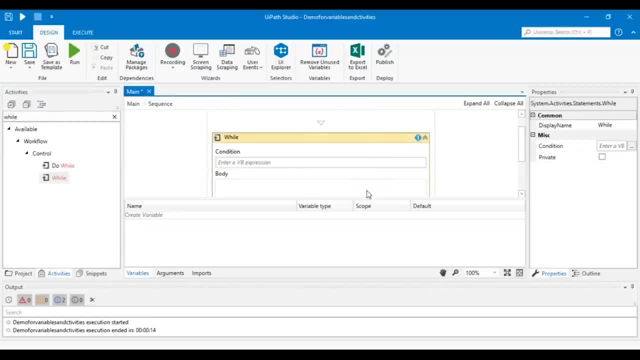 And now I'll search for a while loop. So, as you can see, I've just dragged the while activity. Now we are have to mention the condition, but before that I have to create a variable for it, right, So I'll just press on control K. 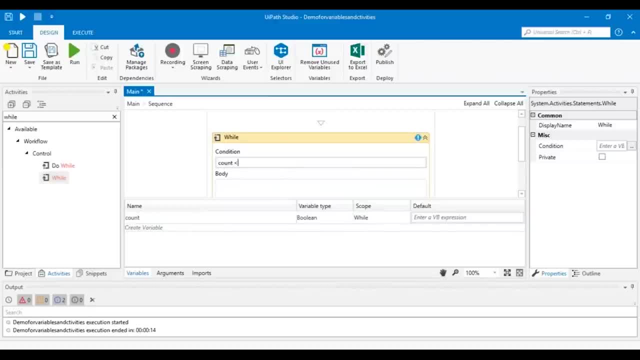 Let's say, you know I create a variable count. So basically count should be less than 10.. So my condition is that you know, I want to print the variables to 1 to 10.. So until the count is less than 10,. 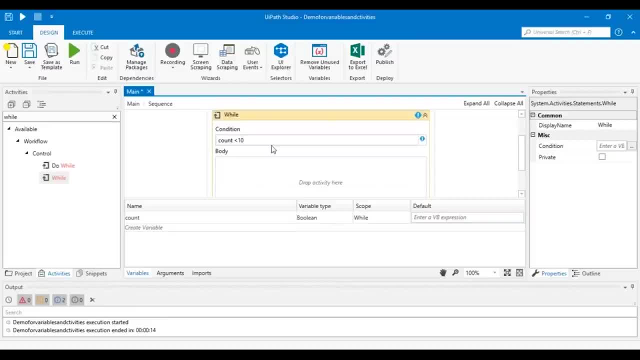 so basically 10 would be considered. So until the condition approves, you would see that you know this set of activities would be executed. So in the body section I'll just drag and assign activity to increment the counter. So what I'll do is I'll assign count is equal to count plus. 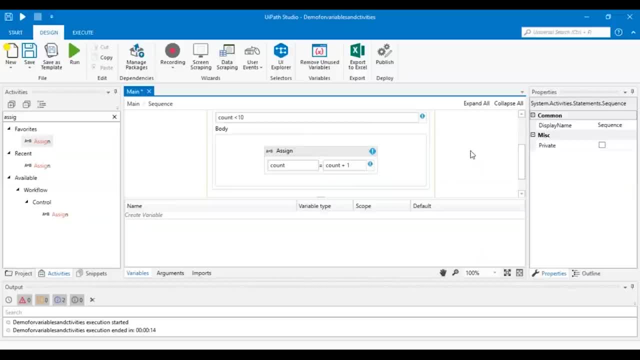 1.. So, since we want to print the output of you know, the number is 1, the number is 2, basically, the count is 1, the count is 2, and so on till 10.. I'm using this particular activity. 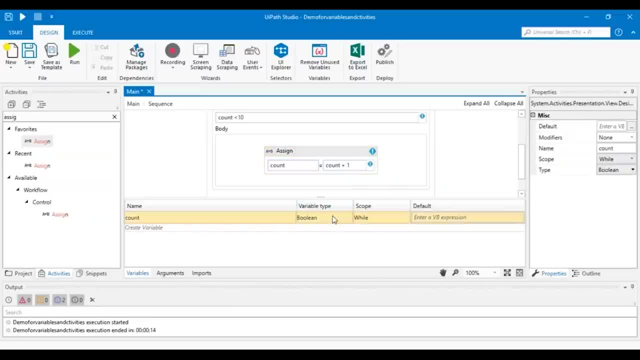 Now observed over here is that you know I've got an exclamation mark. That's because you know our variable type is boolean, So I'll just change it to end and you'll see that you know your exclamation mark is gone. 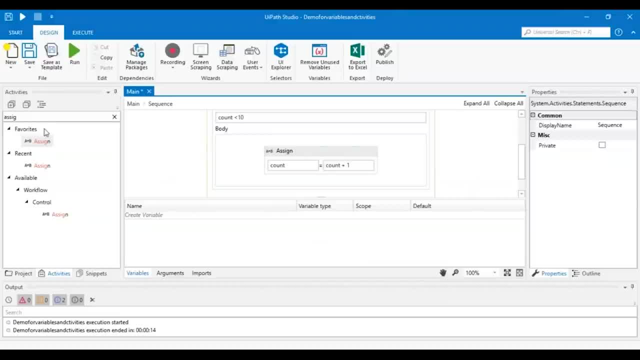 So now, before I move forward with this session, I just forgot to tell you that you know, the manage packages section is really important in this particular studio. So what basically happens is that you know, when you install UiPath, it's not necessary that all the packages would be pre-installed. 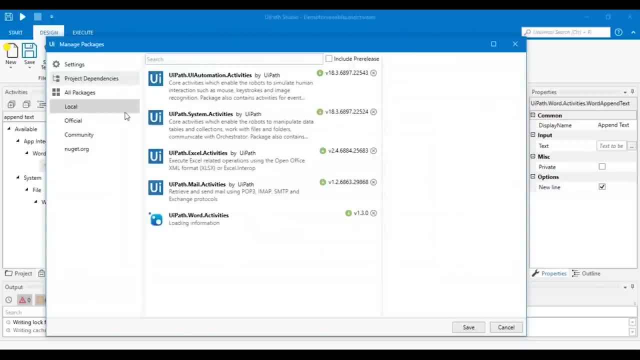 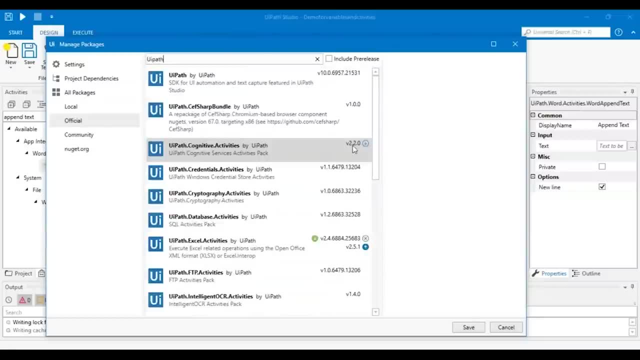 right. So, for example, if you go to the manage packages section, you'll see the option of you know the official packages and when you search for the official packages and when you search for UiPath, you'll clearly, clearly see that. 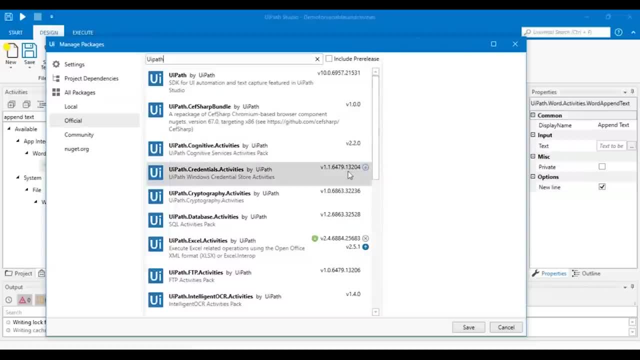 you know, some of them are not installed in my system and all. So basically, if I'm working with, like you know, the databases or emails and all, then I have to install the packages to get the activities related to them right. 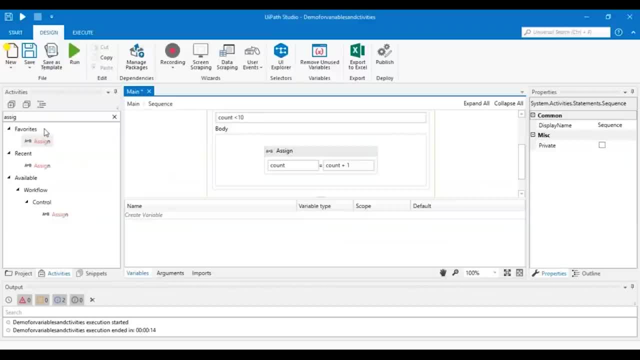 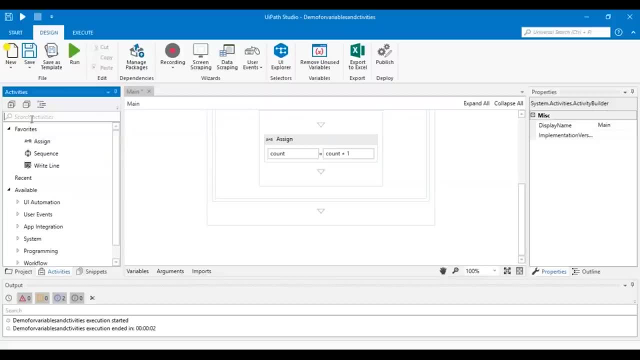 So remember installing the packages for your required actions. So I'll just close this window. And now, once we've used the assign activity, we want to mention the output in a particular file. So for that, what we can do is we can use the append line activity. 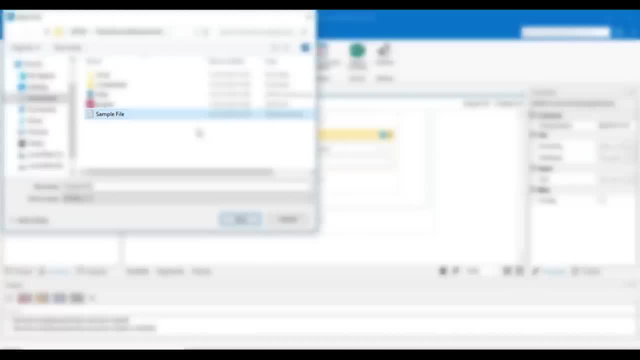 And then we can mention the file path. So I'll just open over here. Let's say: you know I, I create new text document and mention sample files, right? So I'll mention this, I'll click on save And then over here. 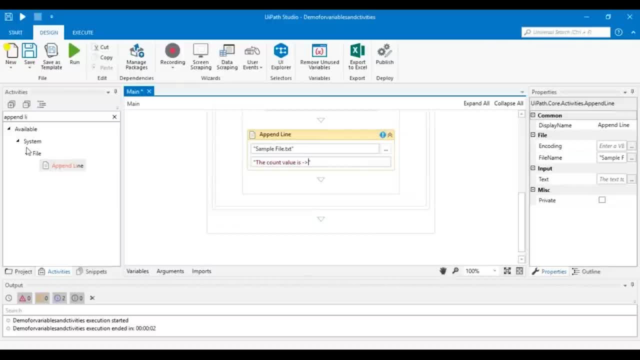 I'll mention the text to be: the count value is, and it has to be plus count to string. right Now. once this is done, let's just click on run So you can see that the execution has ended. So we'll just open that particular file. 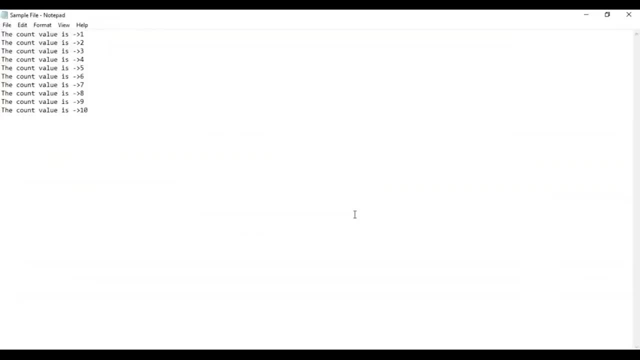 All right. So when I open this particular file, you can see the output that you know: the count values: One, two, three, four till 10, right, So, guys, that's how the while loop works Now. 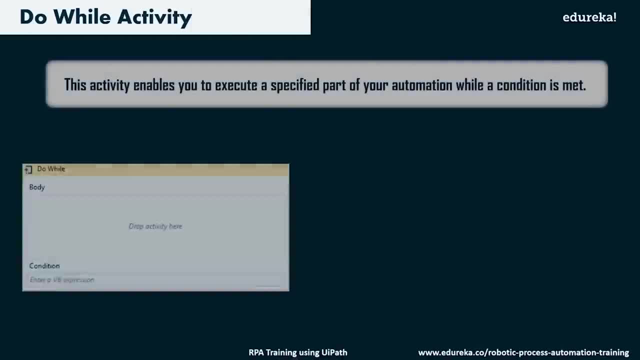 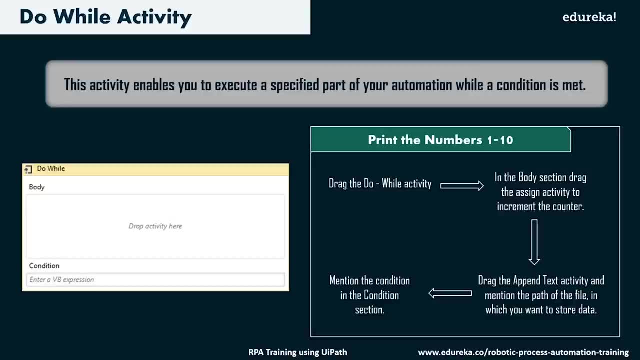 let's move forward to the next activity, That is, the do while activity. So this activity basically enables you to execute a specified part of your automation while a condition is met right. So basically, what's the difference between while and do while? is that so? 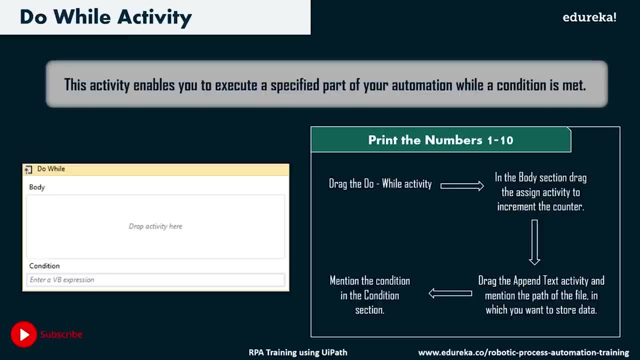 in the while activity, the condition is first checked and then the set of activities will be executed. and it's the reverse in the do while activity, first activities will get executed in the do while activity and then the condition will be executed. We check right. 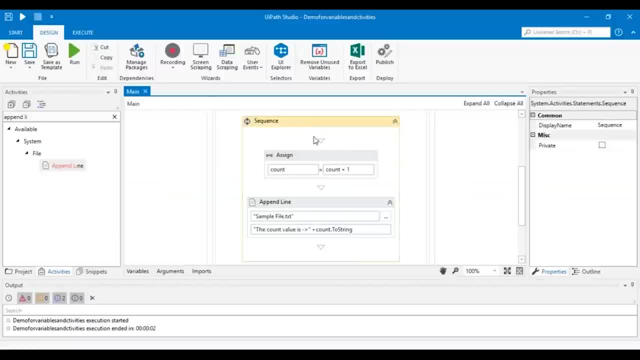 So for that, what I'll do is I'll just show you the automation again. So let's just remove this part of while activity. Let's drag a do while activity Now. Now we hear, what I'll do is I'll again use the append line. 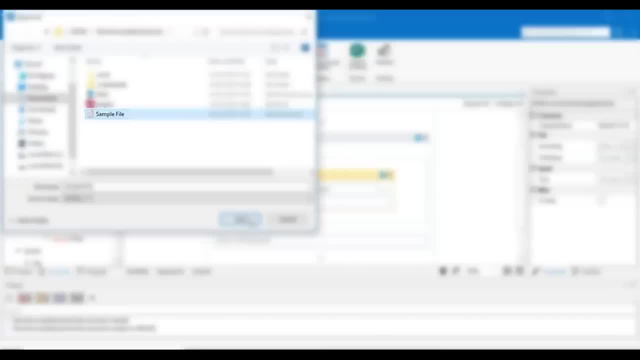 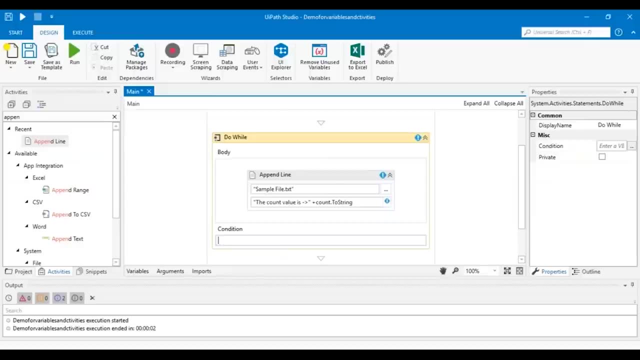 activity. I'll mention the file path. So let's say I mentioned this, the same file again, and in the text I mentioned the count values to be count to spring. Now we are. what I'll do is I'll again create a variable of count right, and then I'll change the variable type to be end. 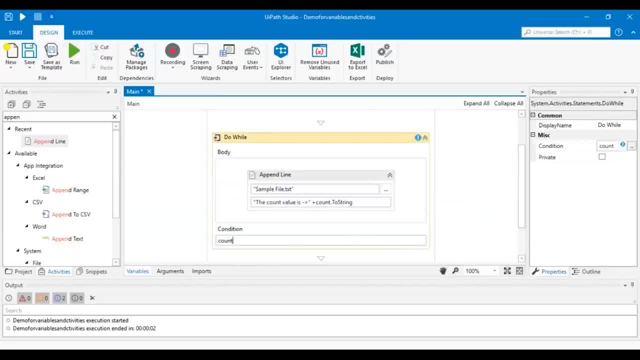 Right. So on the condition part, I forgot to mention less than 10.. So I'll just mention less than 10 and you'll see that you know you're good to go. So, basically, in the do while activity, what I've done is I mentioned what task has to be done and 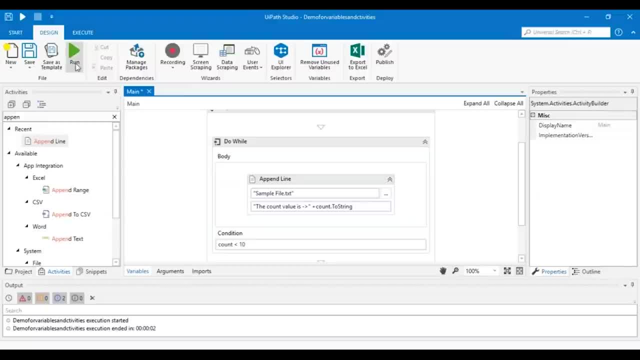 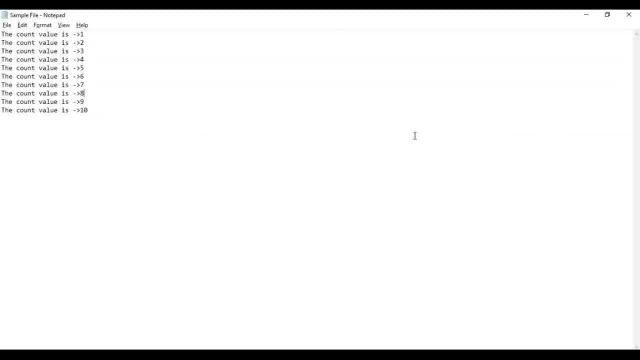 then the condition would be checked right. So I'll just execute this particular execution. All right, so you can see that you know it. execution has started, All right. So once the file gets executed you will see an output that you know. 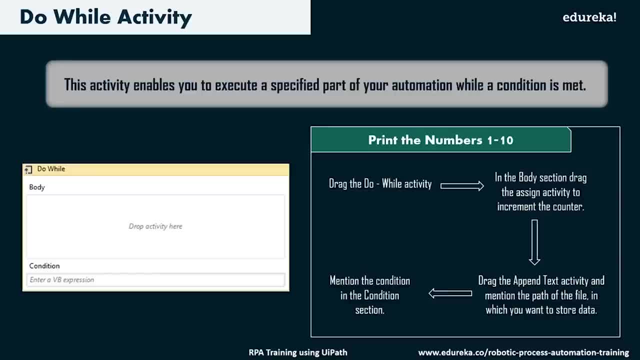 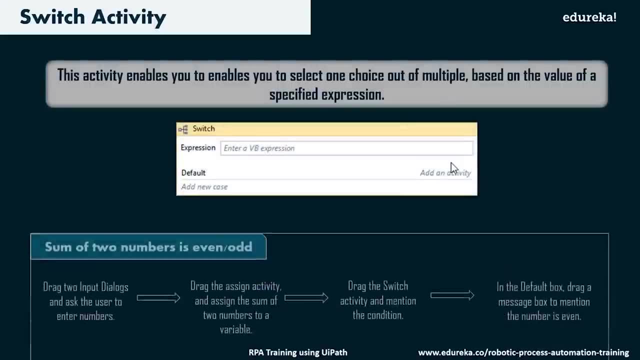 the count values 1, 2, 3, 4 to 10, right. So, guys, that's how the do while activity works. Now let's move forward with the next activity, that is, the switch activity. So the switch activity basically enable you to select one choice. 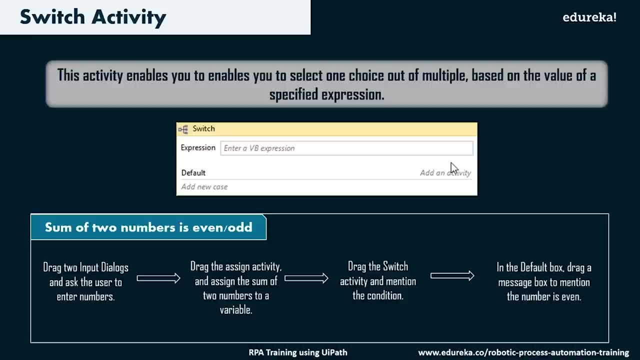 out of the multiple choice based on the value of the specified expression, right? So whenever you want to choose one choice out of the multiple choices present, you can use the switch activity. So, for that, what we're going to do is we're going to see a. 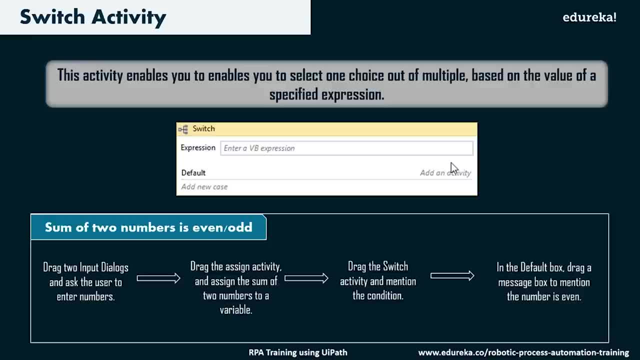 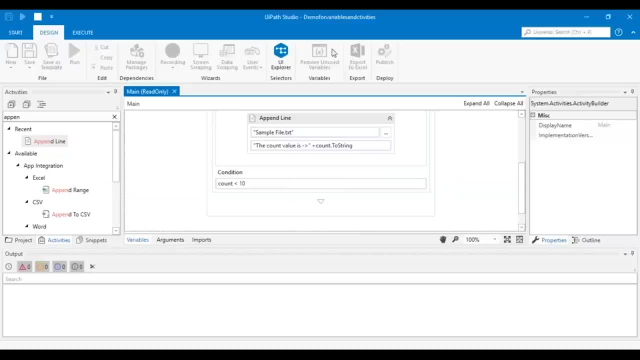 simple automation. you know where we're going to add two values and then what we'll see is whether the particular sum of those two values is an even number or an odd number, right? So for that, what I'll do is I'll just remove this particular activity. 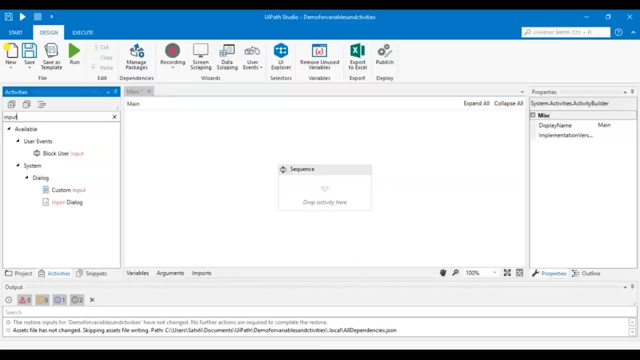 So I'll just remove the do while activity and then first I'll add the input dialog. So in the input dialog I'll mention what is the first number and the label and mention mentioned the first number. So in the output section of this particular input dialog 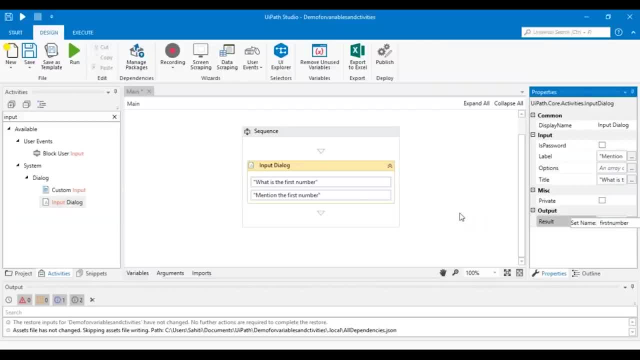 I'll mention first number. So that's basically. I'm creating a variable of first number. Now, Similarly, I'll add an input dialog and then I'll mention the second numbers. that is, what is the second number And in the label section. 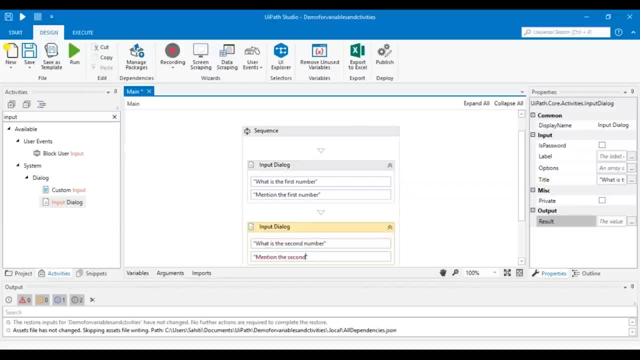 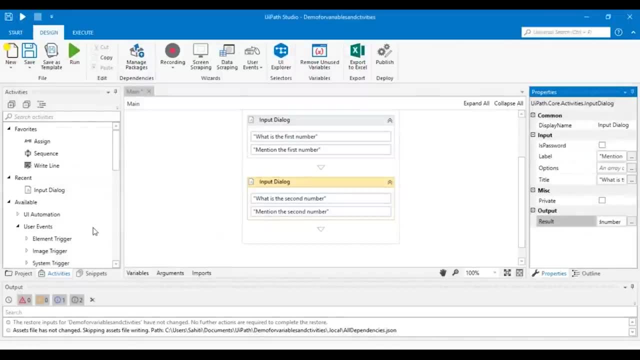 I'll again mention, mention the second number. Now what I'll do is, in the output section of this particular input dialog, I'll create a variable for second number. right now, What I'll do is I'll add these two numbers, right? So basically I'll drag and assign activity. 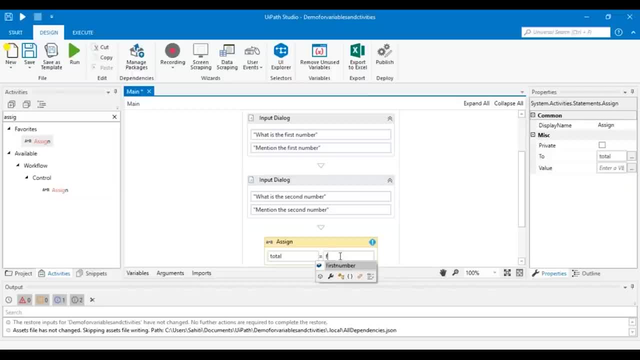 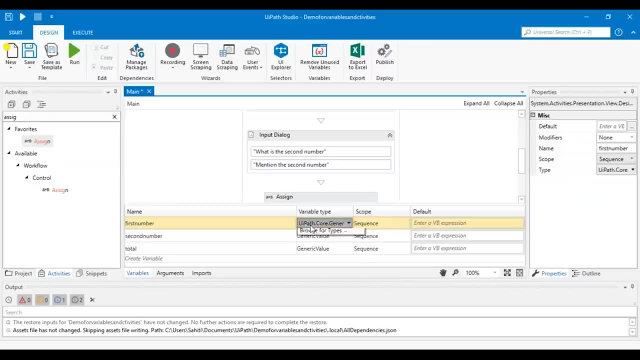 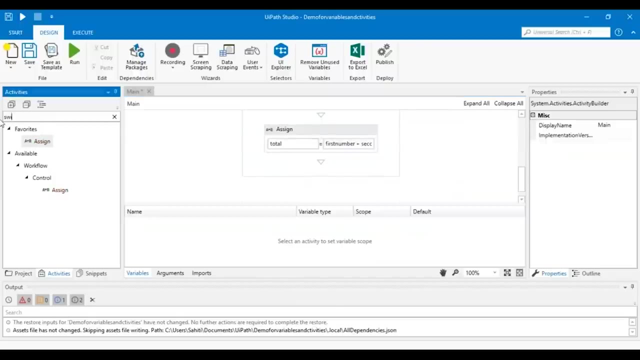 I'll create a variable total and over here I'll add first number plus second number. Right now in the variable panel I'm just going to change all these variable types to end. So I'll just change this variable types to end. And now what I'll do is I'll drag a switch activity. 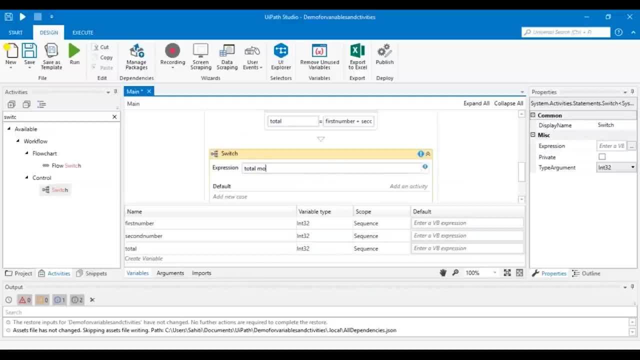 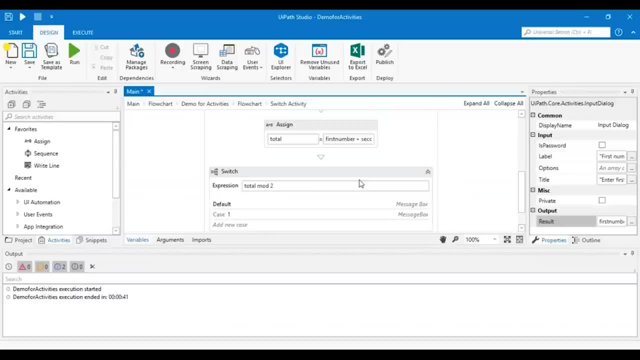 Now in the switch activity, what I'll mention is total mod 2 equal to 0.. Now, after you mentioned this over here, what do you simply have to do is, in the default section, you have to drag and drop a message box and then over here. 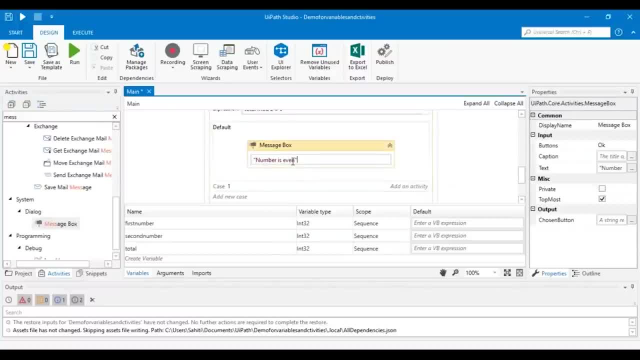 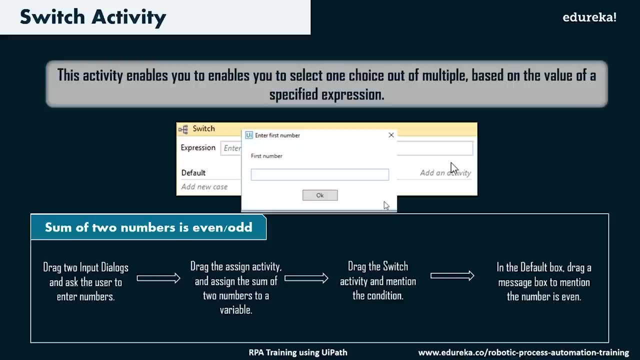 you have to mention the number is even else. you know the number is odd, right? So that's what I've mentioned Over here. Now what I'll do is I'll just execute this particular execution. So let's enter the first number. 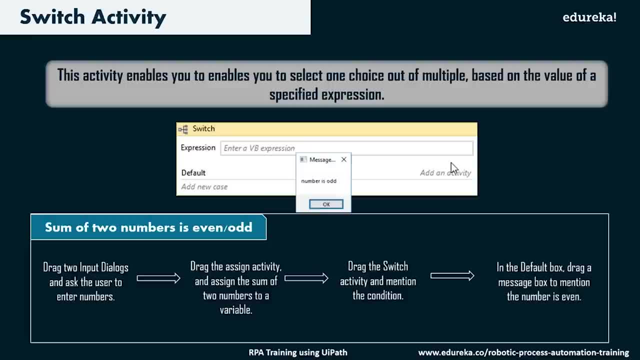 That's 23.. Let's enter the second number, That's 12.. So we should get an output that you know the number is odd. So I've displayed an output that you know the number is odd. Similarly, if I execute it again, 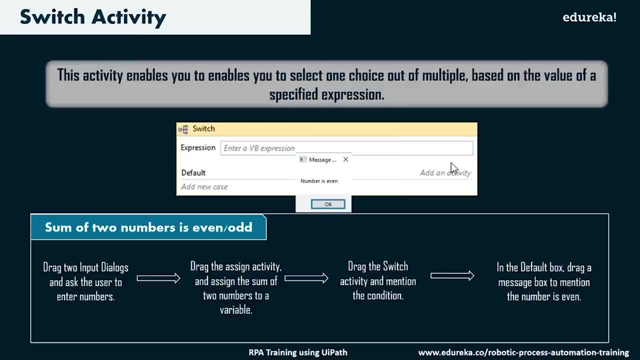 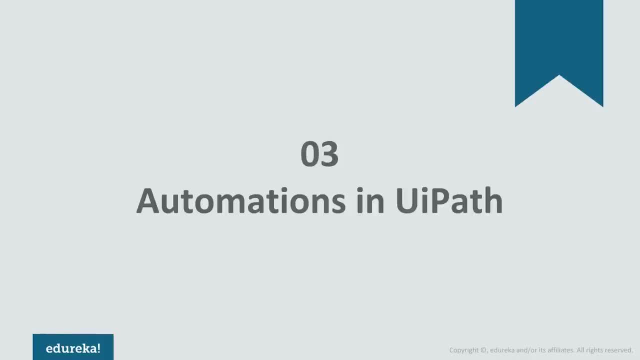 let's display the first number to be 12, second number to be 24.. So we would get an output that you know the number is even right. So, guys, that's how you can use the switch activity. Why do we need Excel automation? 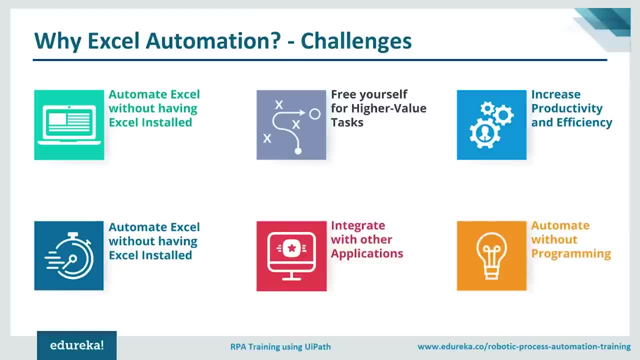 Well as all of us know that Excel is perhaps the all-time champion in storing, organizing and manipulating the data. Excel is easy to use and is also highly popular, but it is not always user-friendly and at times it can prove to be very time-consuming and hard to integrate with other applications. 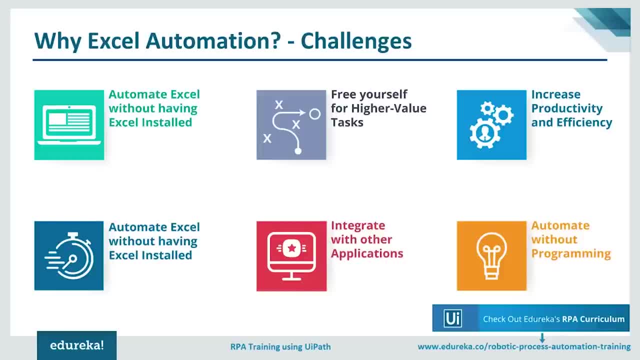 So, in today's environment, where everything is multi-application focus, with data constantly being transferred between applications, migrating and integrating data into platforms can therefore become troublesome. right So to perform large number of tasks with good accuracy and speed, and also to integrate with other applications to provide 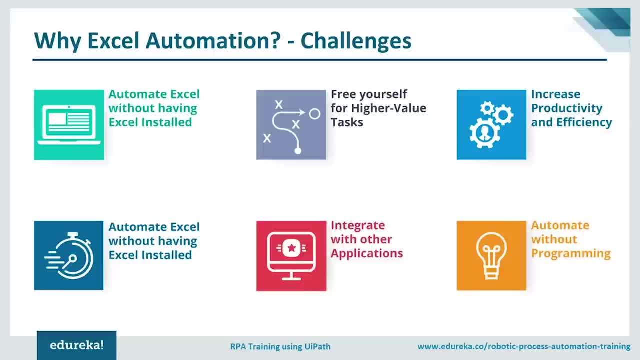 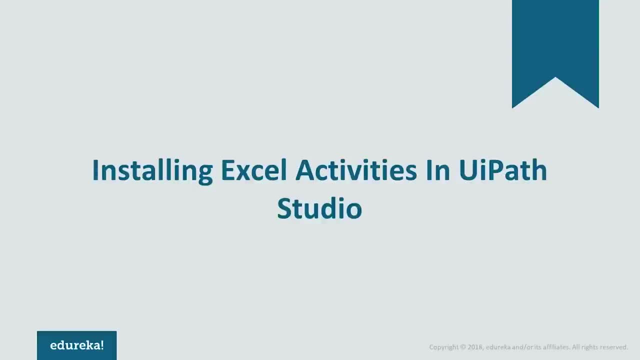 high productivity efficiency, Excel had to be automated. So, guys, these were the reasons why Excel automation came into first place. Now, how do we implement this Excel automation? Well, that is really simple. You just have to implement it by using a tool. 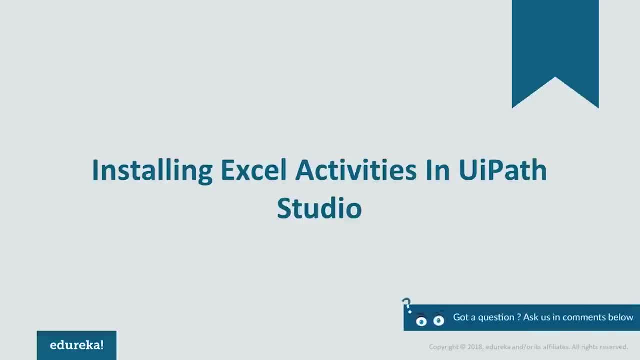 Right, So here we'll be using the UiPath tool to automate Excel activities. So I'm assuming that all of you are well versed with the UiPath interface and workflow passing variables between actions, right? So these concepts will help you out throughout this tutorial. 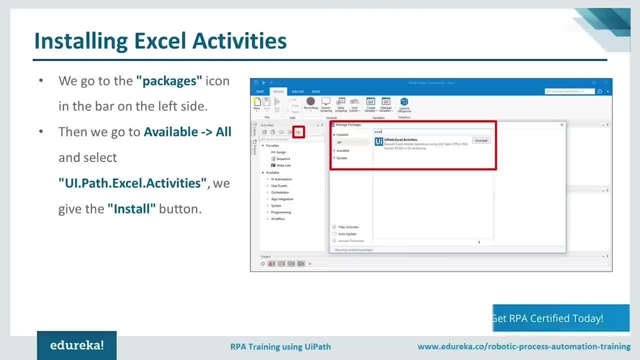 So now let's get started. So, as I told you before that, we'll be using the UiPath tool to automate activities related to Excel, But before that you have to install the Excel activities in UiPath Studio. So for that, let me show you how you can do that. 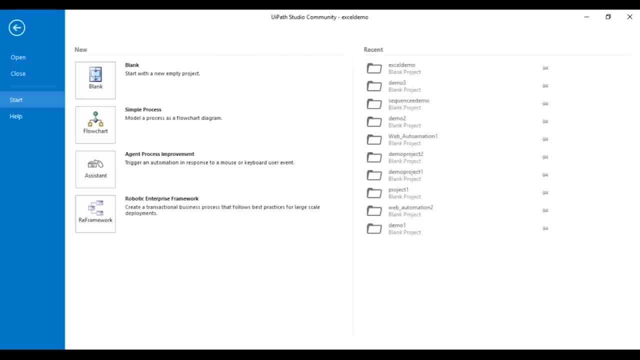 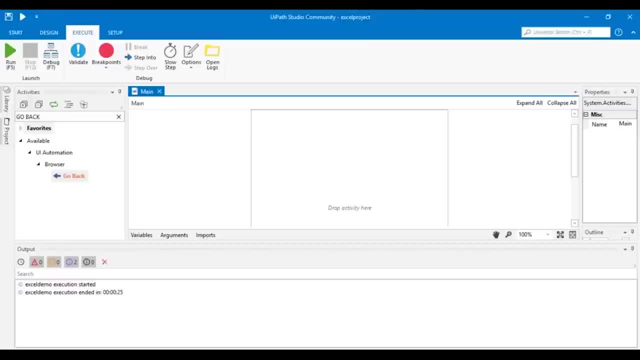 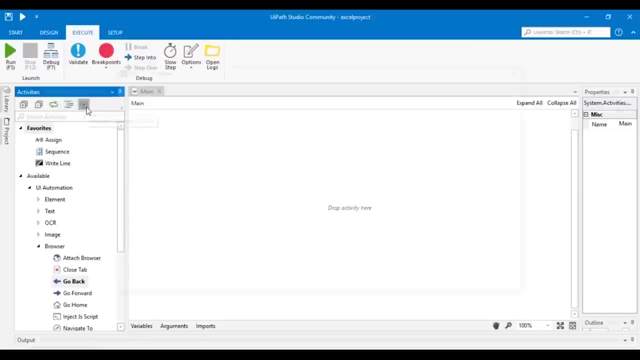 All right. So let me just open my UiPath tool and let me show you how that happens. So for that, let me just open this blank project. So when you open your UiPath Studio, you can go to this manage packages option. 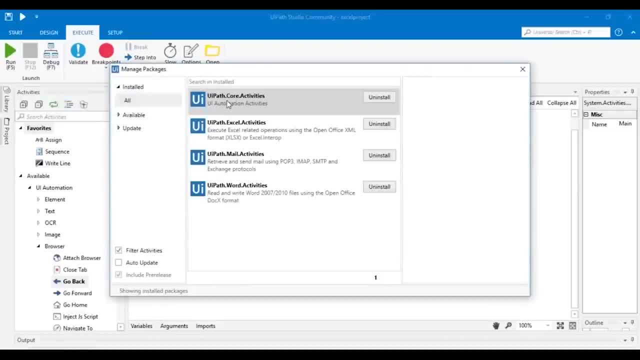 All right. So when you click on this, this is where you can check if your Excel activities or any other such activities- for, like the word activities, the mail activities- are installed or not. So in my system you can already see that the Excel activities are installed. 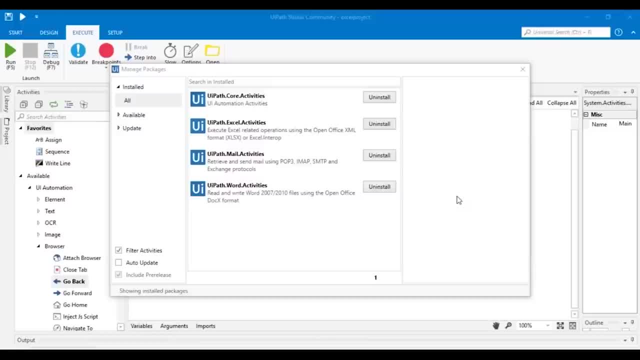 All right, just in case, if Excel activities are not installed on your system, you just have to search in the search bar for Excel activities and click on the install radio button. All right, so that would automatically install all the packages related to the Excel. 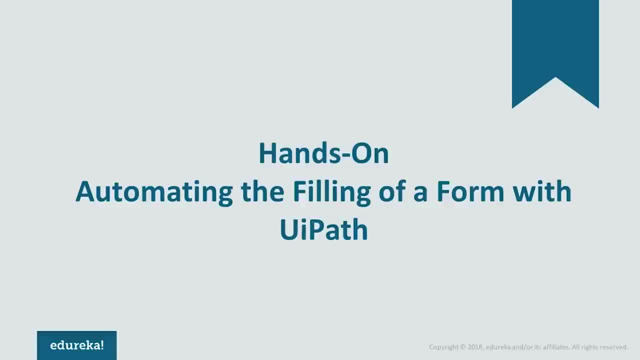 activities. Now let me just close this, Okay. So now that you know how to install the Excel activities and you know the reason why you should automate the Excel activities, Let's move on to a hands-on, Where we'll be creating an automation to fill a form with UiPath. 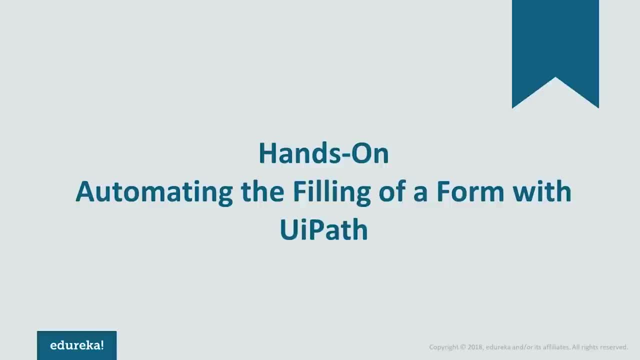 All right. So what this automation is going to do is that we're going to have a set of details stored already in a CSV file and then we'll create a Google form. So when you run this automated task, all the details are fetched from the CSV file and Google form fills. 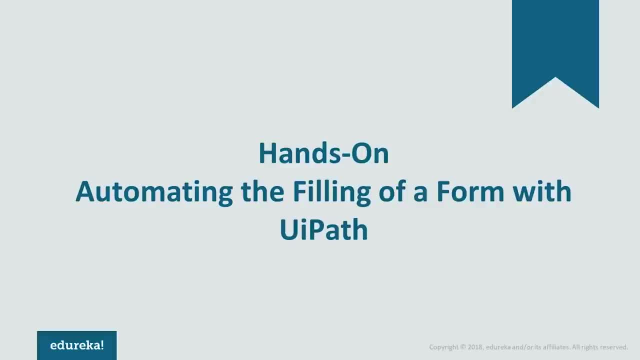 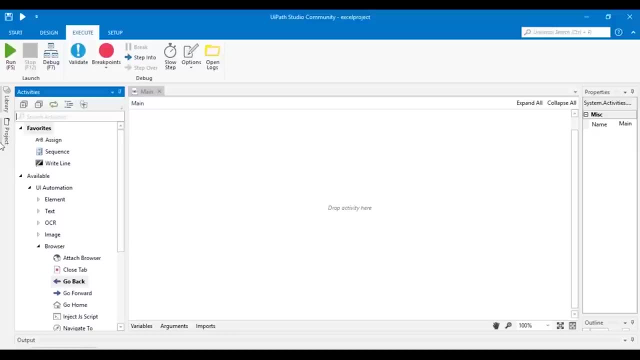 automatically. So now let's continue with our demo. So, to understand this, let's go back to our UiPath tool. All right, So let me just go back to my UiPath tool. So we already Have a blank project created here. 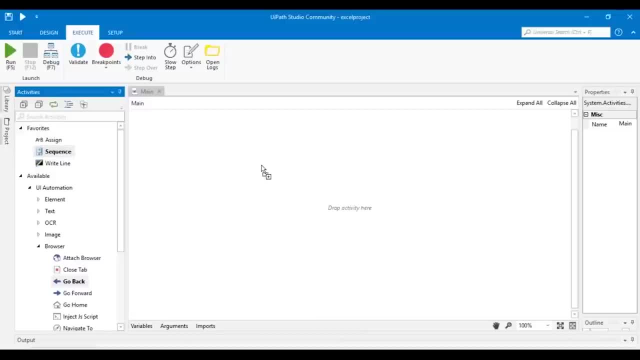 So now let's just drag and drop a sequence in the workspace, All right? So, basically, sequence is a place where all your activities are performed. So, since we're dealing with the Google form here, let's first create a Google form, All right? 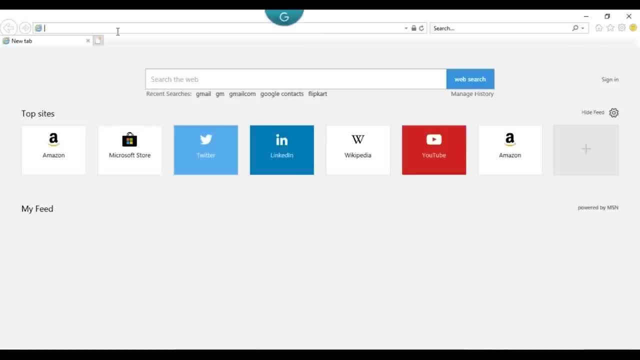 So for that let's go back to a browser. So now let's just create a Google form here. So for that let's just type in Google for Google forms, Go to Google forms and then let's create a blank Google form. 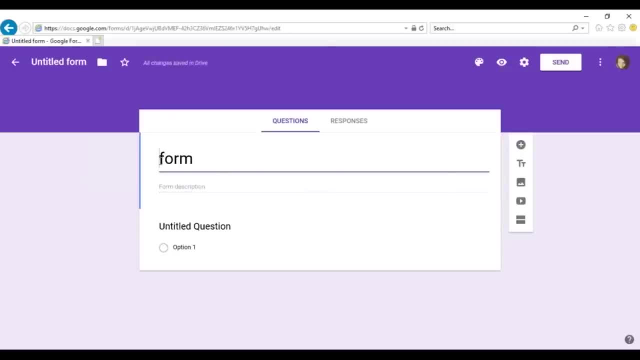 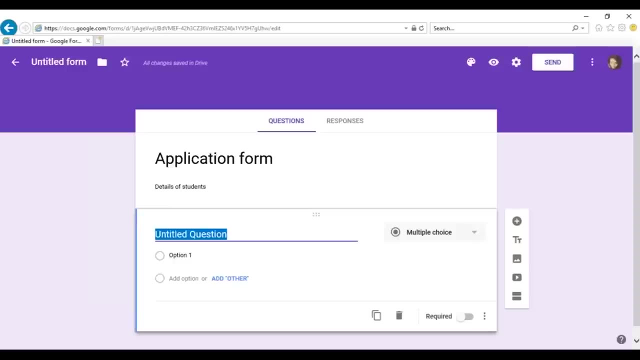 All right. So let's just say we create an application form, So let's just type in the name as application form and the form description as details of students, right? And then let's start adding questions. So let the first question be the name. 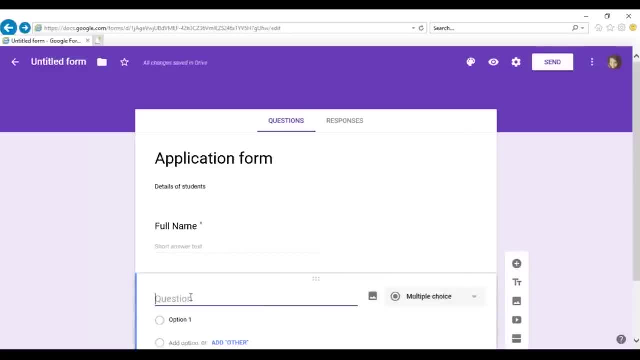 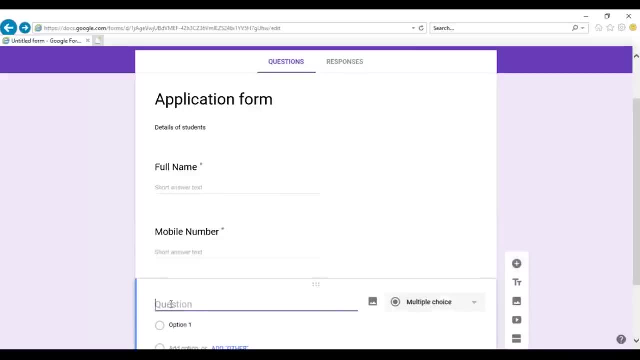 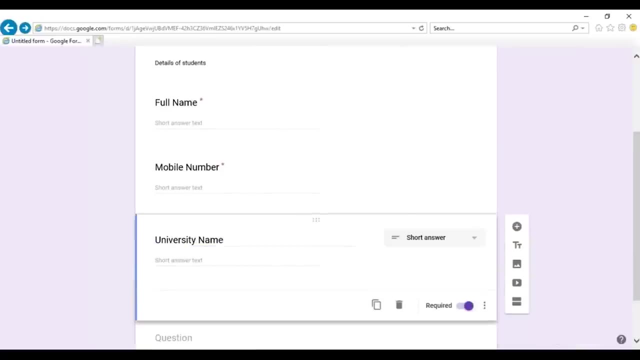 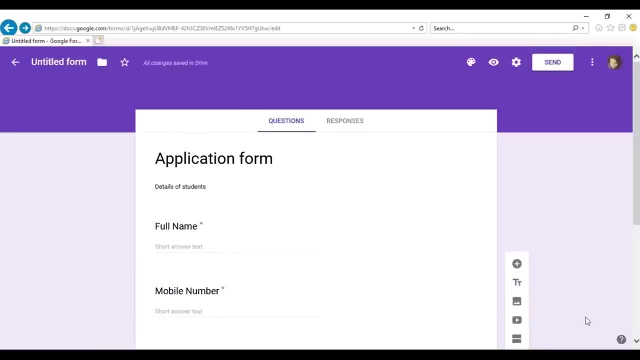 All right, The second question be mobile number. Let's add one more question, Which could be University name, And finally the email ID. So, guys, this is a simple form. Well, you can customize your form as you want. Now, 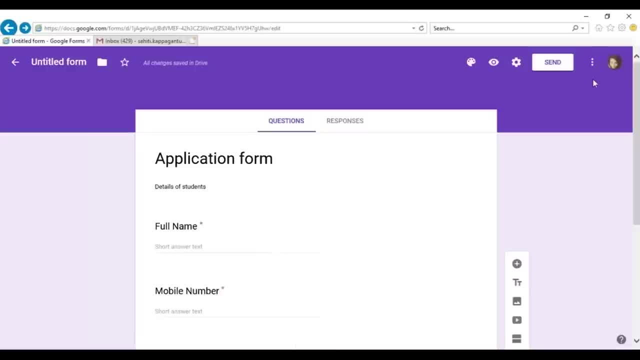 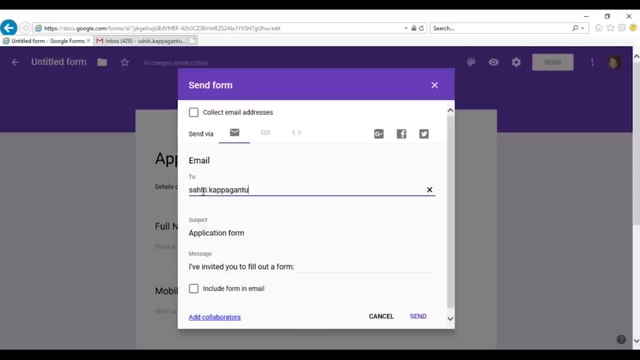 let me just send this Google form to anybody, right? So let me just send this Google form to myself. So let's just type in my mail ID, All right, and click on send. Once I click on send, let me just open my mail ID. 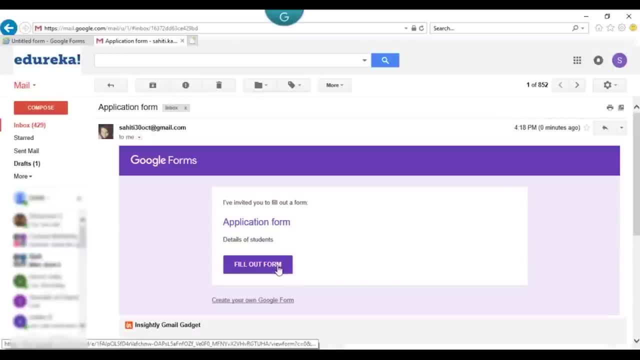 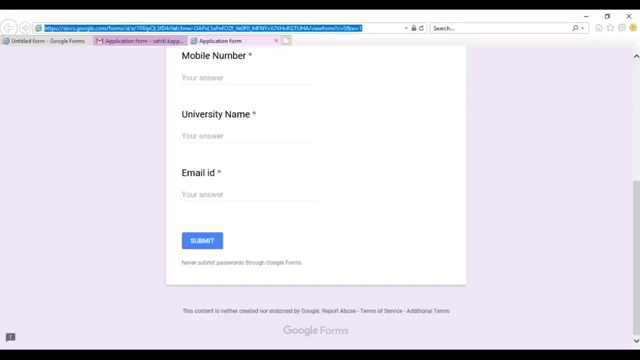 And then you can see that I've got an application form right. So let me just open this application form. So the link over here has to be included in your sequence. So let's go back to our uipath tool. Let's search for an activity named open browser. 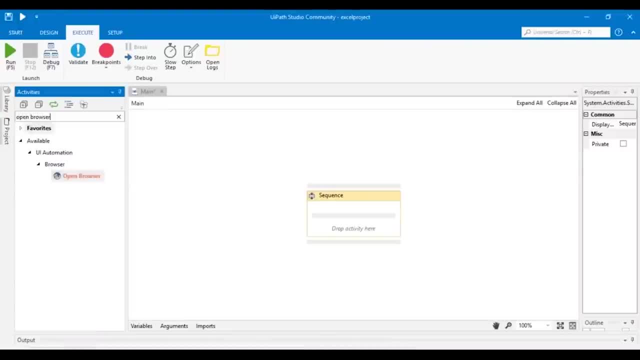 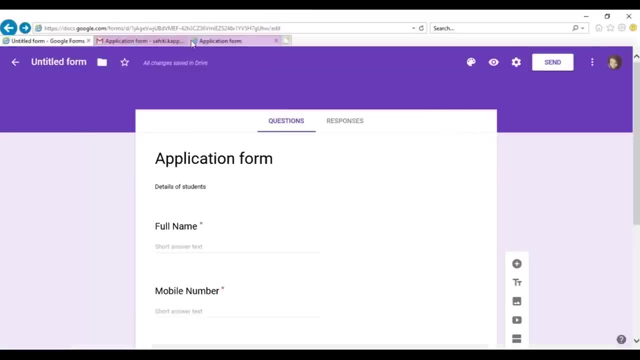 So let's search for open browser and then drag and drop it here. Once this is done, in the URL over here you have to specify the Google forms link, right? So let's go back to a form. copy it. Let's come back to the uipath tool. 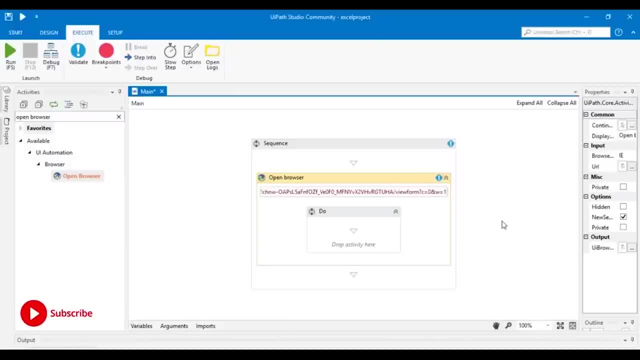 open double quotations and then paste it over here. All right, Now, after you're done with this, in the do section of your open browser, you have to include a type into to identify the questions of the application form. All right, So for that. 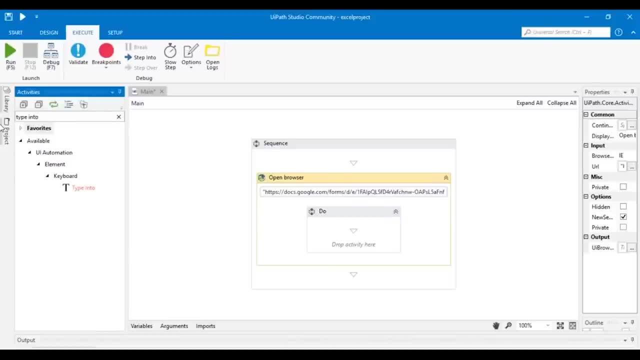 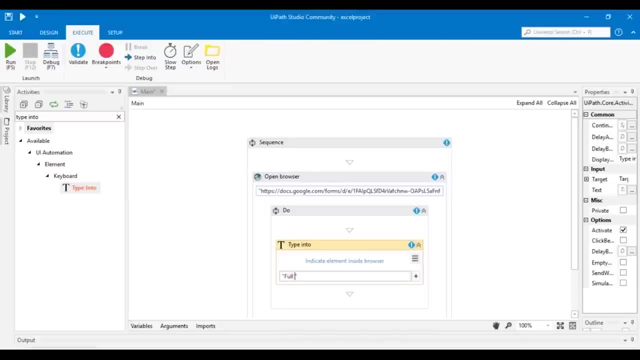 let's just search in the activity pane for type into and then drag and drop it here. All right, So if the first question is about full name, so let's just type in the text That's full name And to indicate the element in the browser. 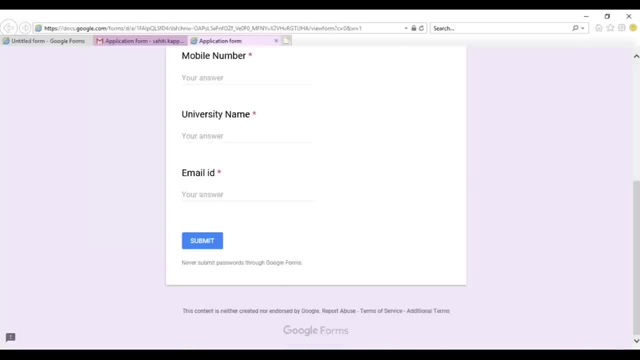 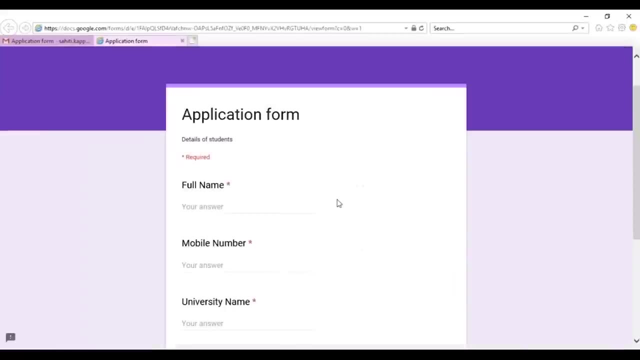 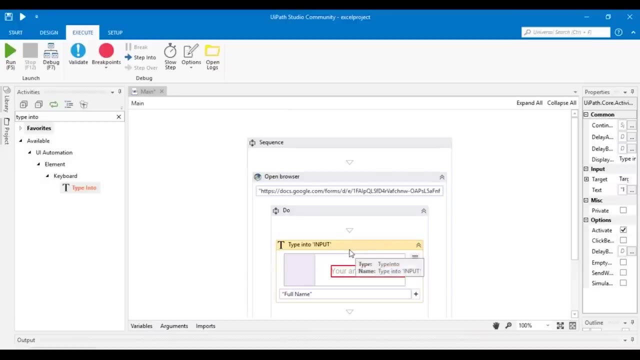 you have to first open that application form, right? So let me just open that application form, Go back to the uipath tool, click on this indicate element browser and then choose this field, right? So I've chosen this field. So, basically, this is the field that it identifies your answer. 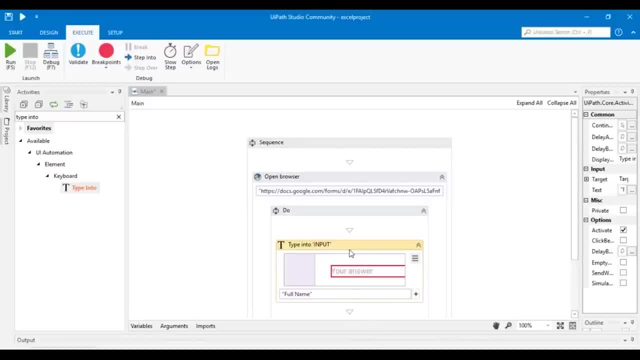 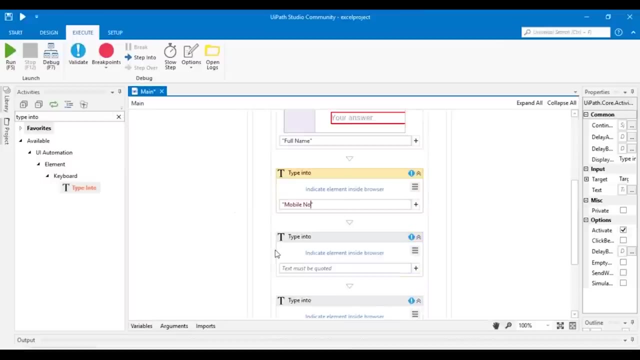 right. So when the first question is about full name, your answer would be feeded here automatically. Similarly, we have to do the same, But the next three inputs also right. So let's just drag three type into here And then include the text: mobile number, University name. 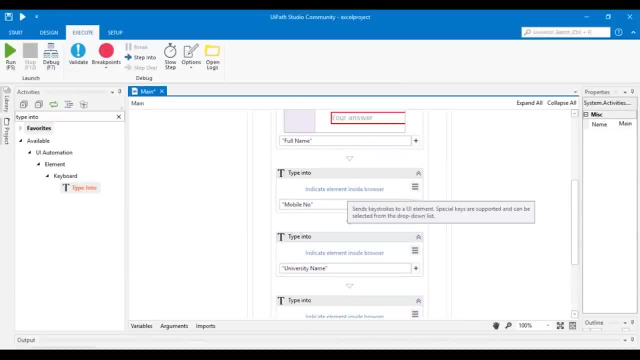 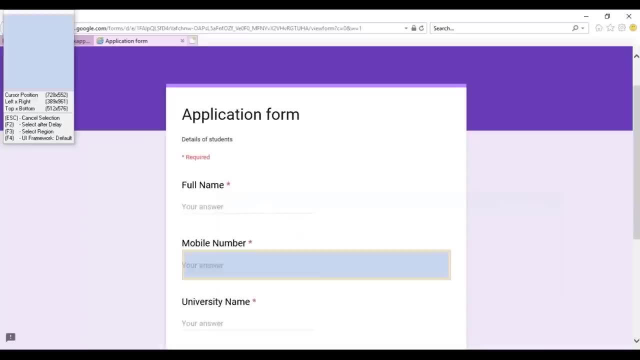 And then email ID. So let me indicate the element inside the browser for mobile number. So let's just open that and let me choose over here. Similarly, let me do it for the University name and also the email ID, right? So let me just open. 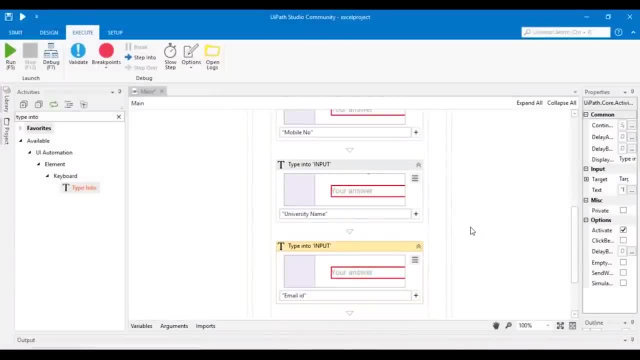 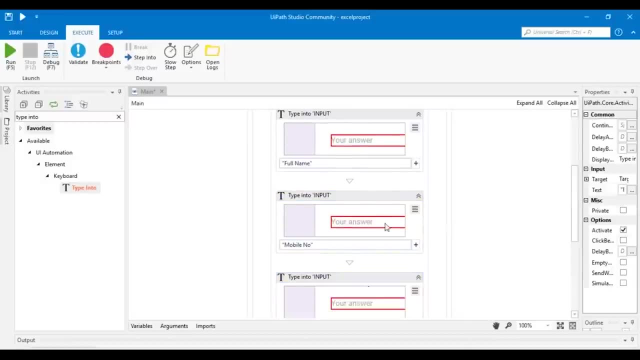 That All right. So, guys, this was the basic step to input all the fields. But here let's put some test information to check whether it's working or not. All right, So I'll remove this full name and include a name here. 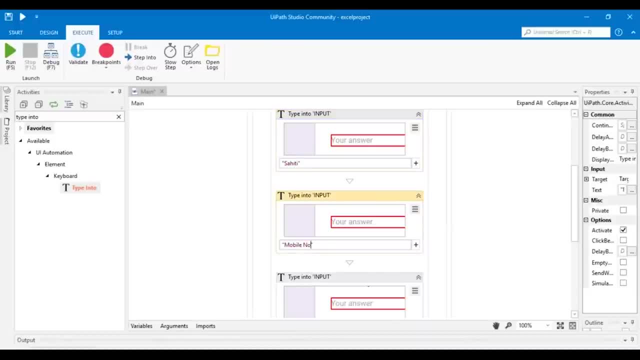 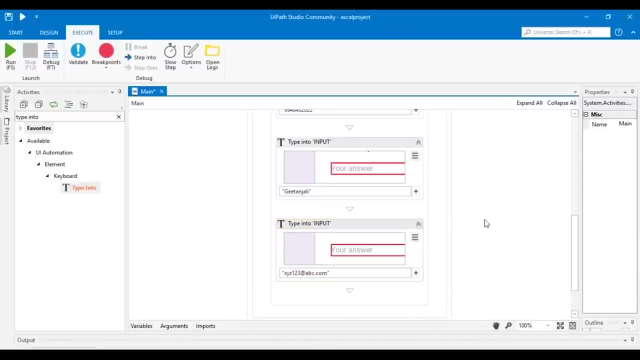 Let's say, I put a name- sahiti- With mobile number And let me again also include the email ID, right? So let me just do it, Huh, All right. So now let's just check if it's working or not. 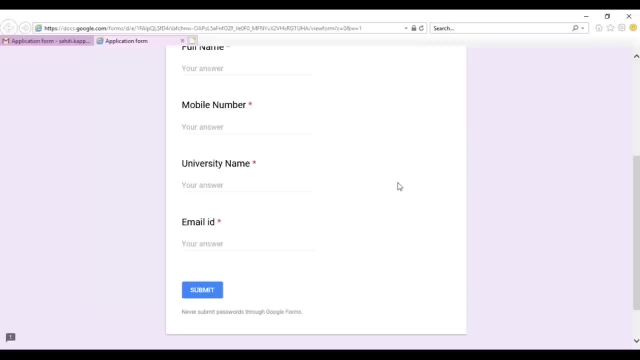 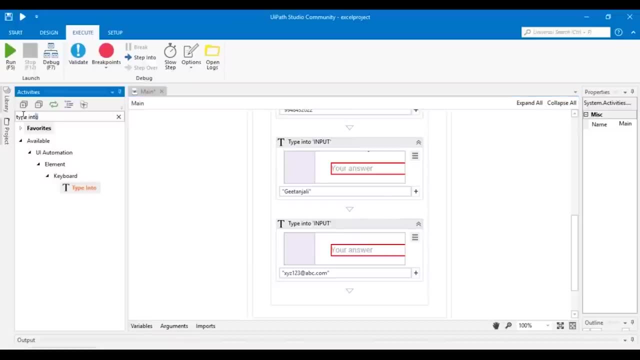 So when you open this form you can see that after you fill in all the details you click onto the submit button right. So we have to automate that moment also. So for that in the activity paint we're going to search for a click activity. 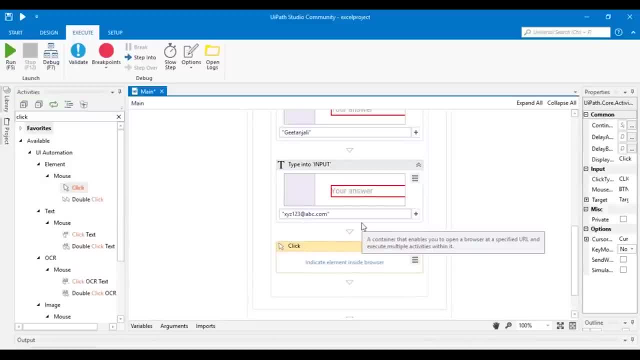 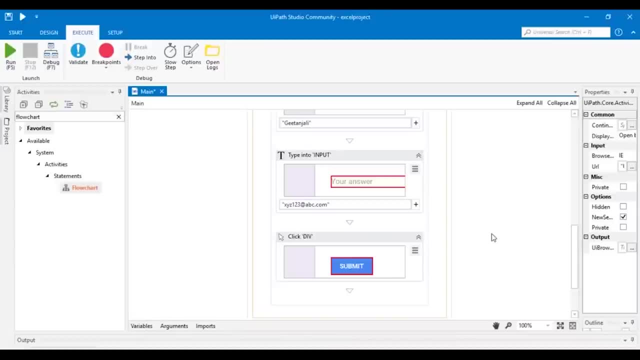 So let me just drag and drop the click activity here and then indicate the element inside browser right. So let's just click here and then do that. So now, once you've automated your click button also, there could be some times that because of your network issues, 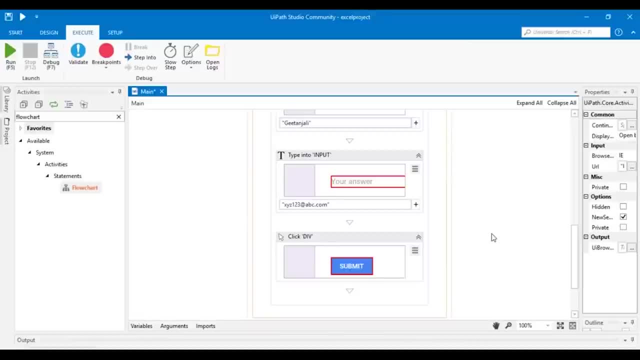 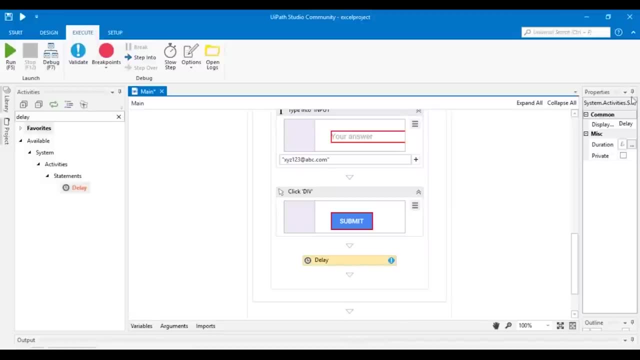 the page may not be loaded immediately, right? So for that we're going to add a delay activity. So let's search in a delay activity and then let me just drag and drop it. here in the properties panel of the delay activity, Let's add: for how many seconds do we want the delay? 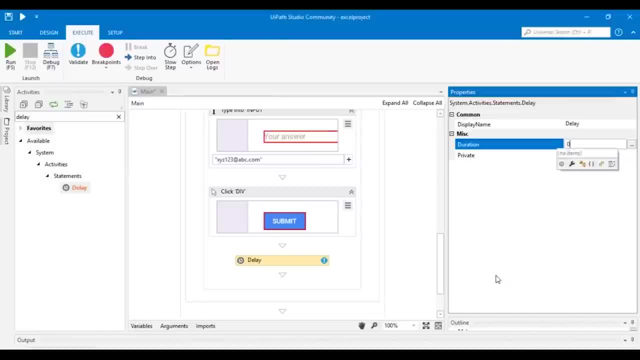 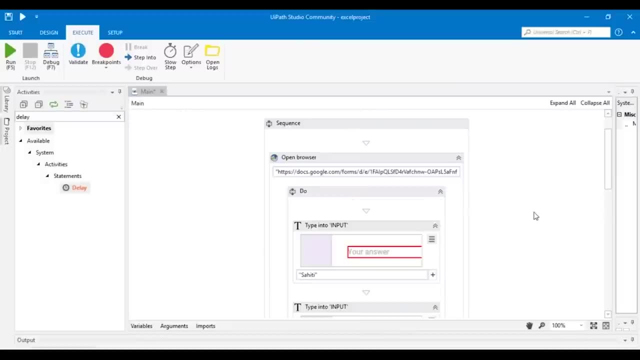 So let's say, if I want the delay for three seconds, I'll add in this format: All right, So this would basically add a delay of three seconds. So if you observe here, this complete sequence is only working for a single input. 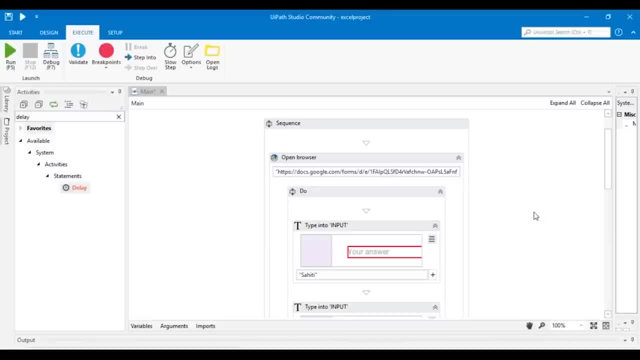 Now, if you want to add more and more records, then we have to press on to the go back button right, So we'll choose a go back activity from the activities pane and then drag and drop it here. So now let's just run this program and see what's happening. 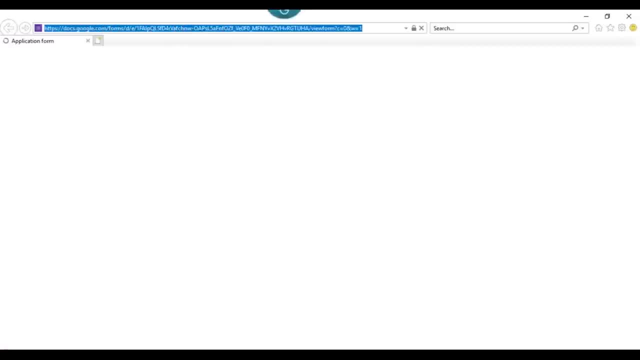 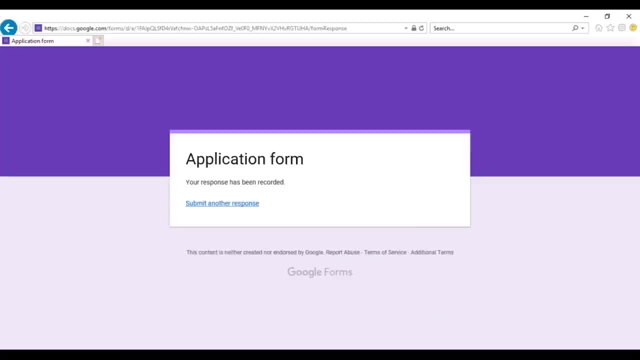 What's going to happen is the Google form will start filling by itself by the input we have given, right? So we have given this input and it's filling by itself. after that It's clicking On the Submit button and it's going back now. 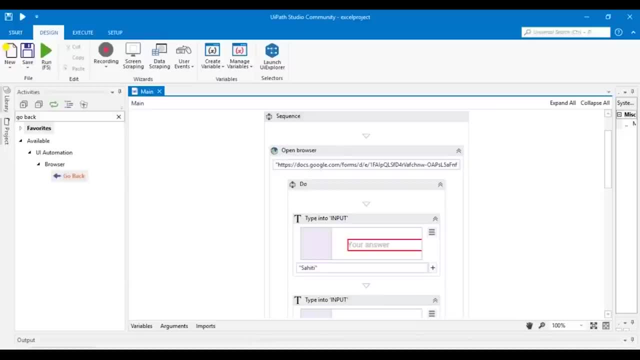 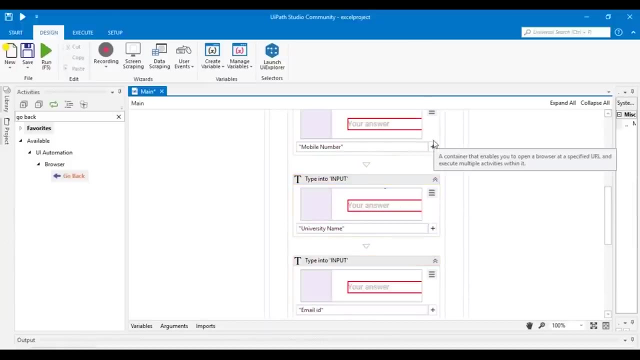 This was for one input. What if we want to do it for many more records and we wanted to fetch the data from a CSV file? So for that, let's just change the text here first, Now to read the data from a CSV file and to repeat this actions. 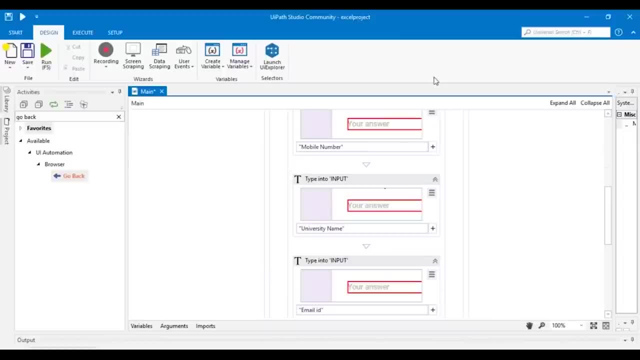 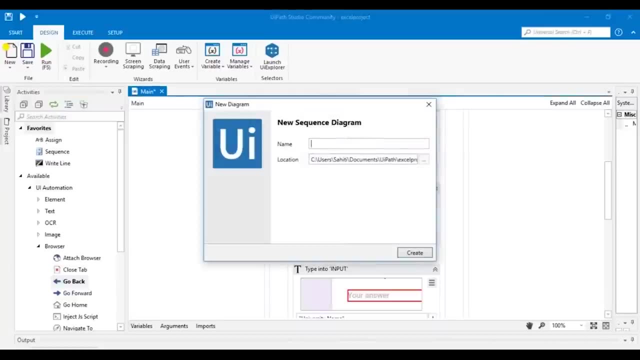 again and again we have to create a flow chart. So for that let's first create a sequence again. So let's just close this and then go to a new sequence and let's just say we name it as Excel demo and then let's click. 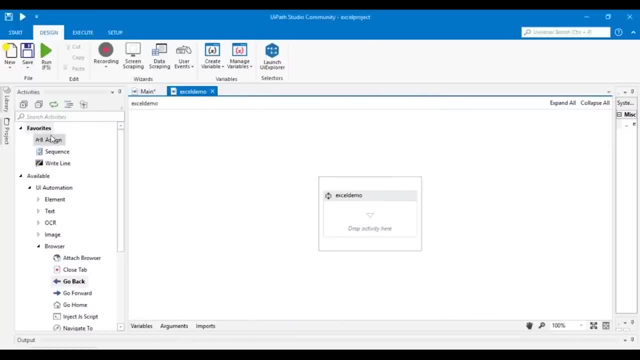 on create. In this you have to add a flow chart, right? So let's search for a flow chart now and then let's drag and drop it here. Once you drag and drop a flow chart, let's add a sequence here, right? 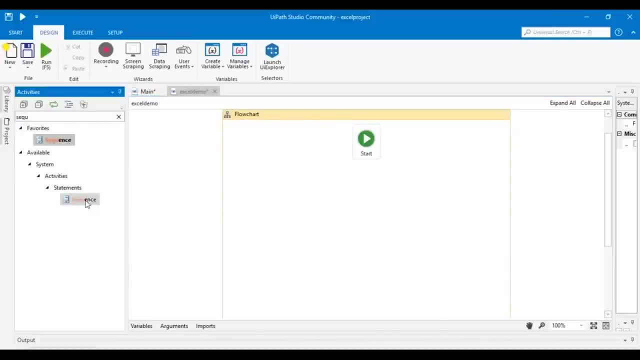 So let's just search for a sequence and then let's add it here. Now open the sequence and then copy all The activities in this particular sequence and paste it there. So let's just copy all the activities from here and then let's paste it here. 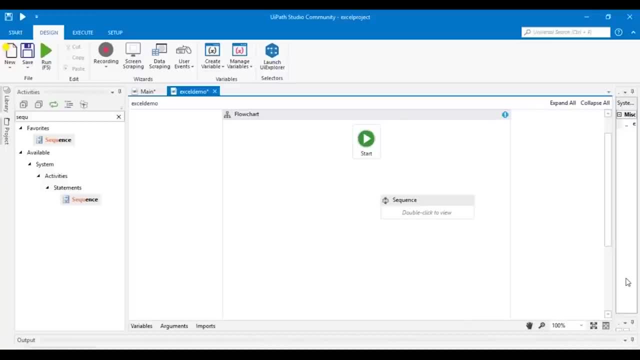 So now you have copied all the actions inside this particular sequence to add them into the flow chart. So now what we want to do is we want the Google form to fetch the data from a CSV file. So let me just show you a CSV file where I've stored the 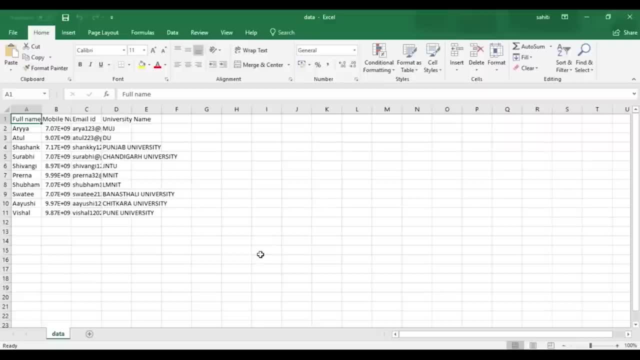 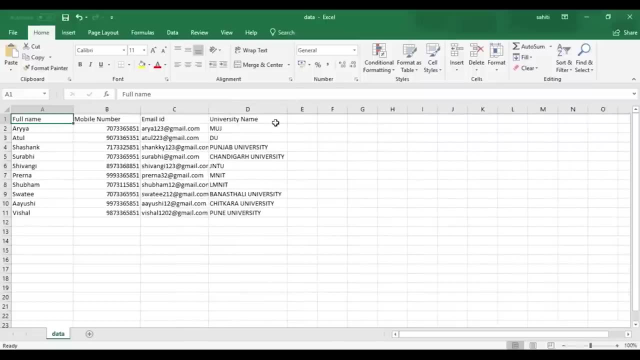 data, right? So let me just open that CSV file. All right, you can see that I've put in the details for full name, mobile number, email ID and University name, right? So let's just see now how the Google form fetches the data. 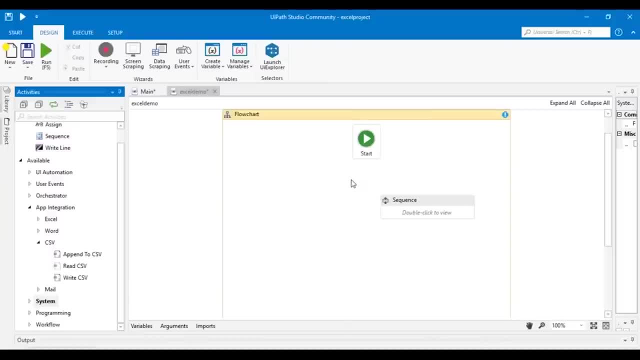 from this file and fills it over there, right? So let's go back to the UiPath tool and let's search for an activity known as read CSV, which would help us reading all the data in a CSV file. All right, so let's just search for read CSV activity and then let's 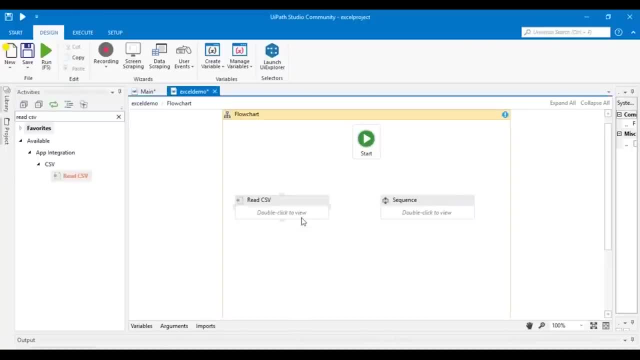 drag and drop it here. So once you drag and drop this activity, just click over here to open this activity. All right, So in the file path option you have to mention the file From which it is going to fetch the data. 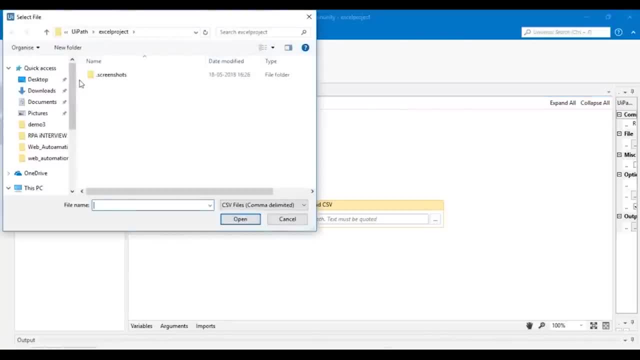 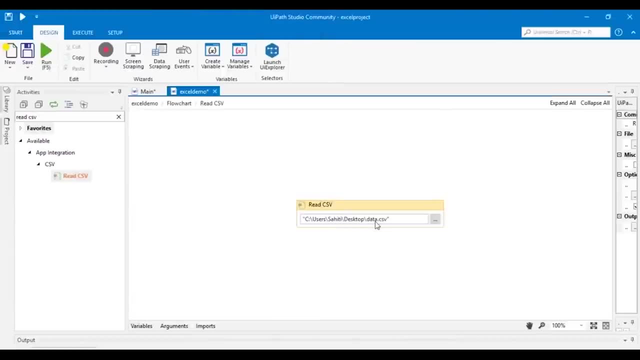 right, So let's just so. let's just click on this tree dots. go to desktop, choose the data CSV file and click on open. this would automatically include a file path. All right, Now our CSV file must have an output format of data table in. 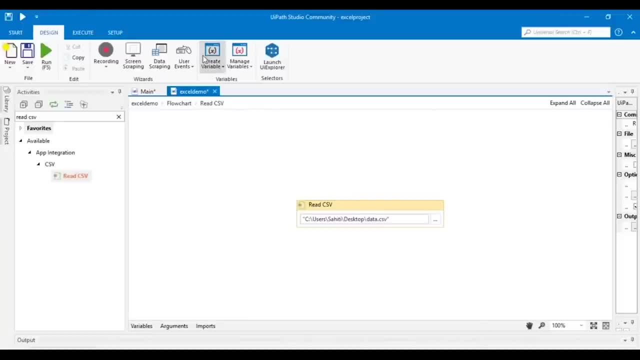 order to be processed. So for that we're going to create a variable. So let's just click on create variable, go to table and choose the table name. Let's say I choose the table name as data table and then click on Okay. 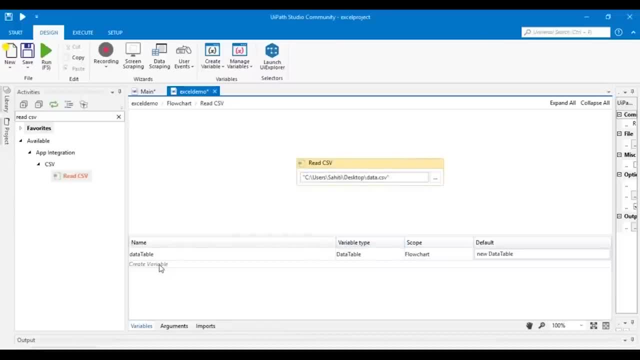 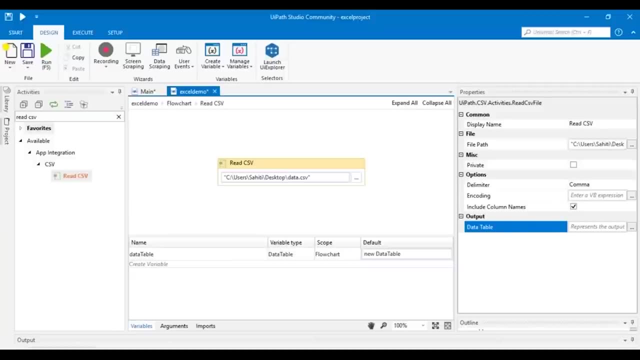 once this is done, in the variable section you can see that the variable data table is created. All right. So now in the property section you have to mention the data table variable in the output field. All right, So let's just mention the data table variable. 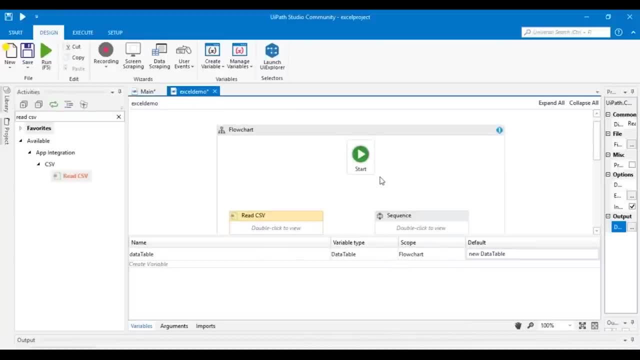 Now let's go back to a main sequence and see what's happening. So we know that the start node has to be connected to the read CSV activity, since the data has to be fetched from here, right? So let's right click on the read CSV activity and choose set. 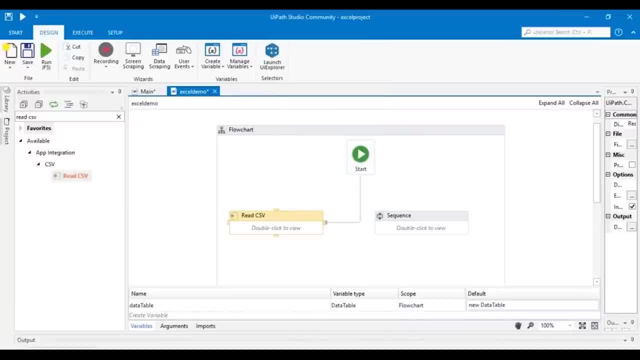 as Start node. All right, So let's just summarize what's happening till now. right? We selected a start note from where all the data would be fetched. We mentioned the file path from which all the data should be fetched, and then it would be connected, and then we created a. 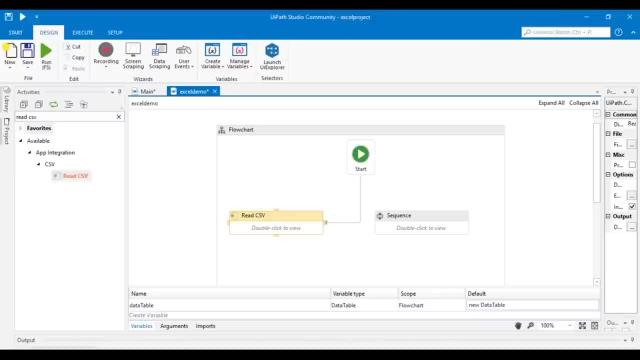 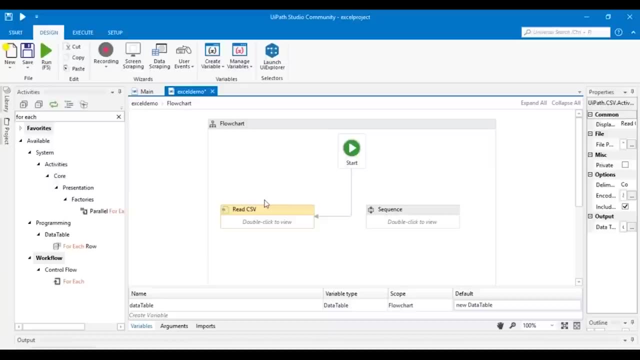 sequence in which it will open the Google Forms and start filling in the data right. So now that we have configured our read CSV activity to the file pathway from where we have to fetch data, It's observed that it only fetches data for one time. 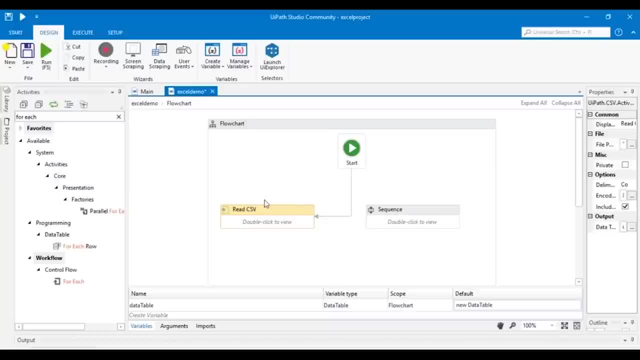 right. But now, if we want to create a loop of iterations of records from our database, what we have to do is you have to drag and drop the for each row activity from the activity pane. So let's just search for for each row activity and then let's. 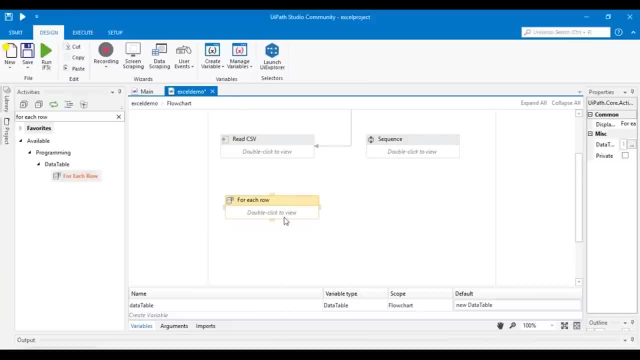 drag and drop it here. Once you drag and drop it here, double click to view it and then in this activity you have to mention: for each row in a particular data table, You want to iterate everything that is present in the body of the loop. 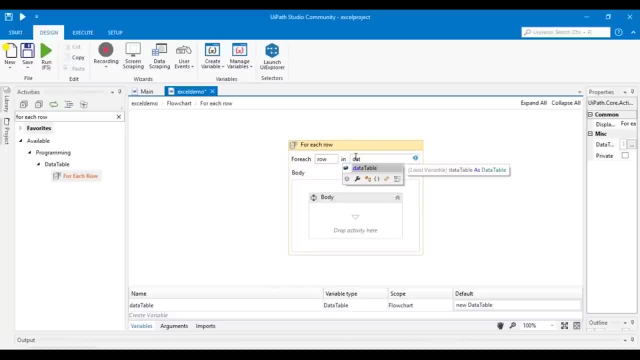 right. So let's just mention the output data table, that is the data table variable in our case, and then let's go back to our main workflow. That is the Excel demo over here. Let's just right click on this activity and then cut this. 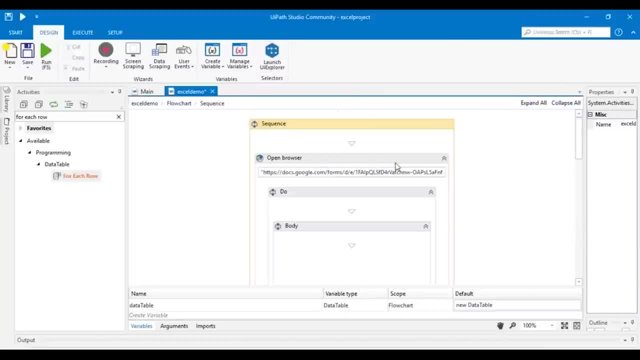 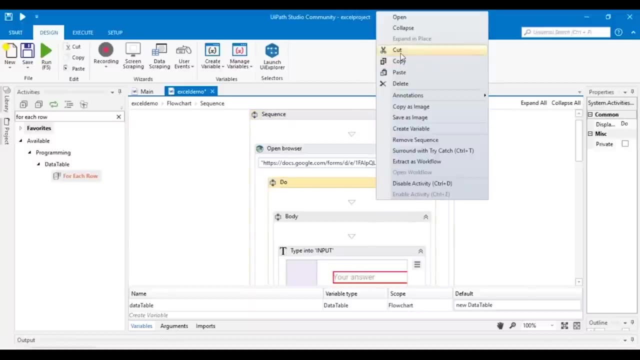 activity All right, and then open the sequence activity. Once you open the sequence activity in the do section of the open browser, you have to include the for each row activity, right? So let's just paste this activity here In the body section of the for each activity. 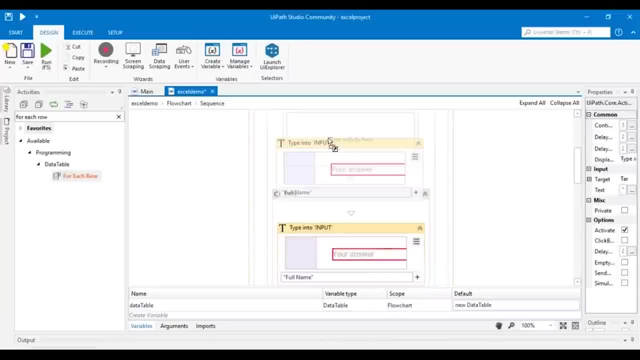 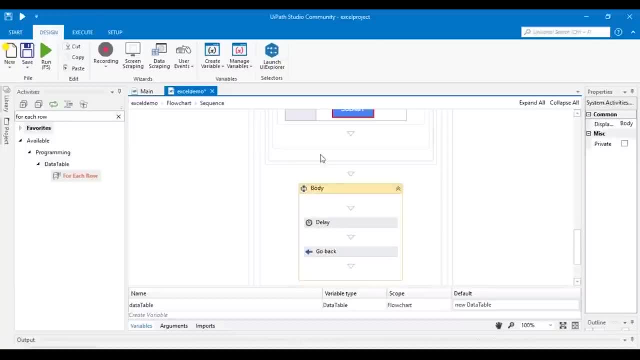 So let's just drag and drop everything that's beneath it. So let me just drag and drop it here one by one, And then let me just delete this body section. Now let's just summarize what all is happening in the sequence. Well, 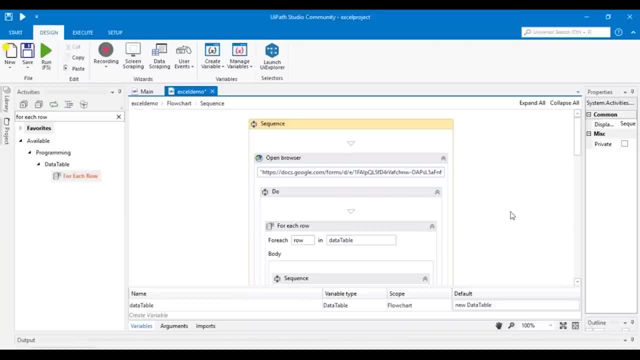 the open browser activity is going to open the Google Forms link that we mentioned. after that, it's going to perform everything that is present in the do section of its body, right? So in the do section of its body, we have mentioned that for each row in the data table. 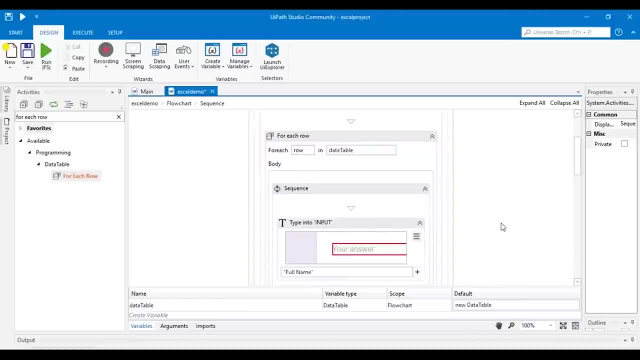 that is, from the each row in the Excel file. We're going to read data and then give it as input to the Google Forms. All right, so that's what's happening. So now let's go back to our main workflow, and then let's. 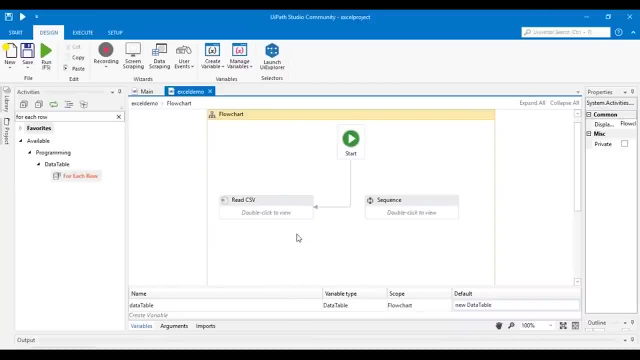 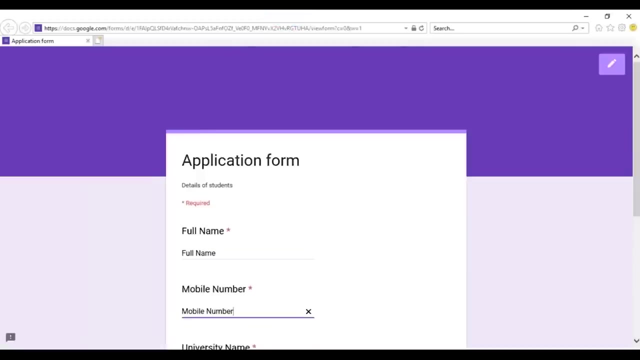 connect the read CSV activity to the sequence so that the data can be fetched from the Excel file, right? So let's just connect this activity now And then let's run again. What's happening here? It's filling the text again and again. that we mentioned in the 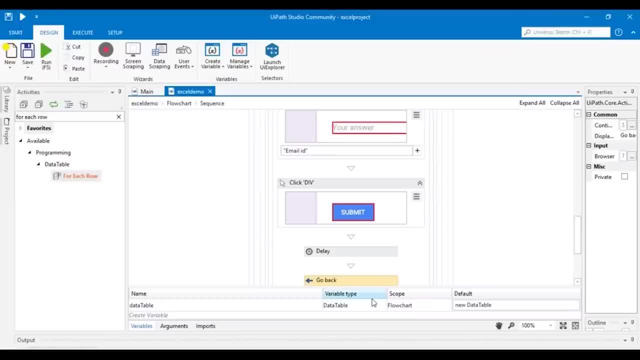 type into actions, right? So we don't want this to happen. We want the data to be fetched from a read CSV file, So for that we have to mention the row names of our CSV files. So let's just mention so for that in the type into field. 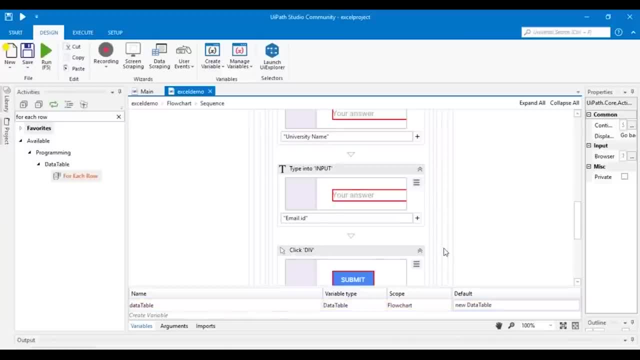 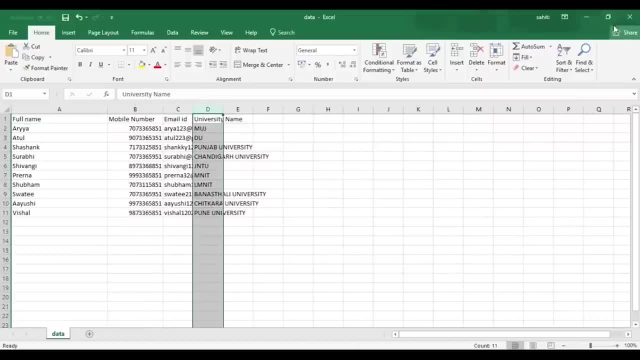 we will place the information of the row names of our CSV file right. So let's see What are the names that we have given in our CSV file. Well, we've given full name, mobile number, email ID and University name. 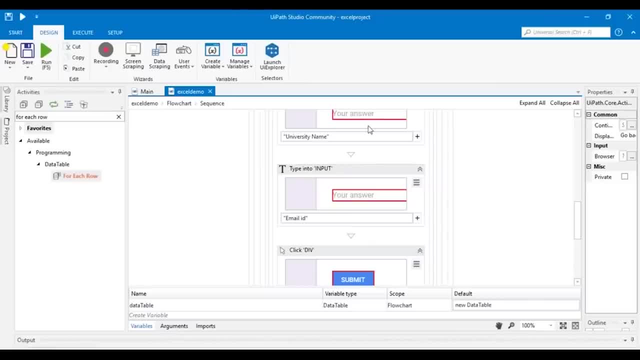 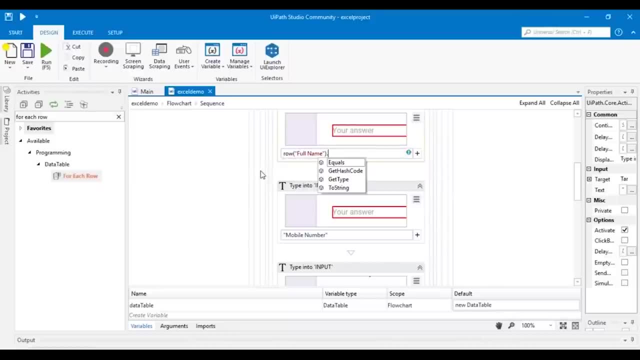 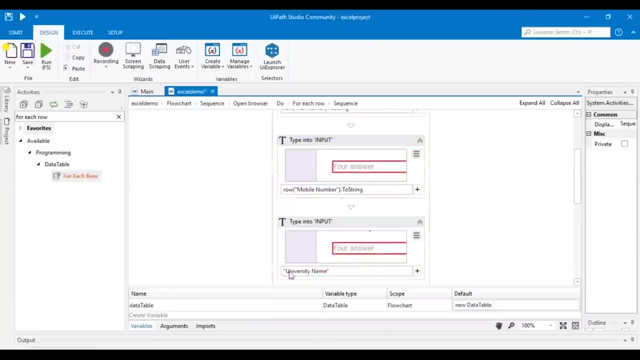 right, Let's mention these in the type into fields. So for that let's go to the first type into fields. type in row and in bracket. type in full name and convert it to string. Similarly do that for mobile number. University name. 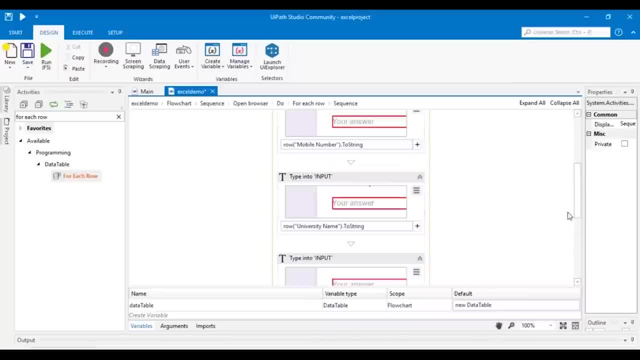 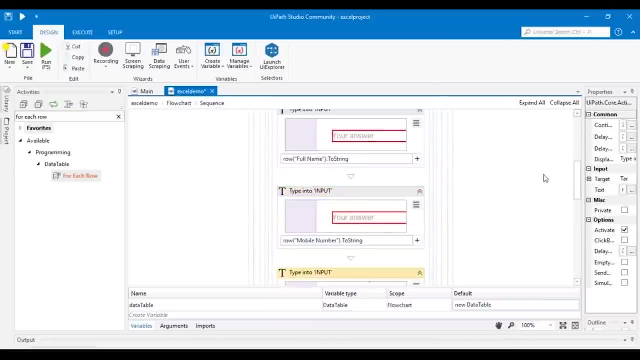 And then the email ID right Now. once it is done, let's click Out of the sequence and check for errors. Well, you can see that there are no errors, right? So let's just open the complete sequence and check for exclamation. 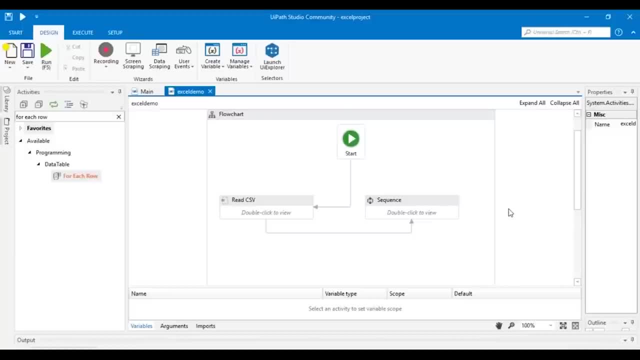 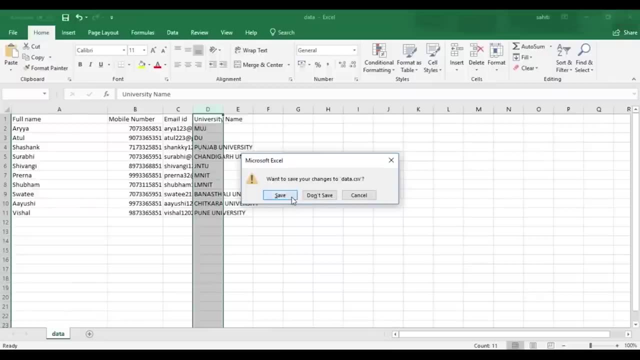 marks, There are no errors. So let's go back to our main workflow and run the project. But before that let's close our CSV file, right? So let's just close a file And then now let's run the program. 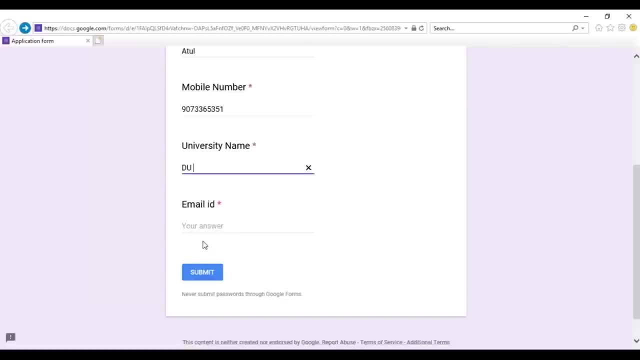 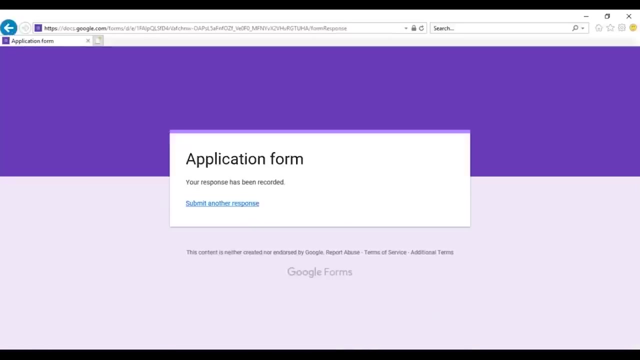 So when you run this program, you can see that all the fields are filled automatically in the Google form, right? It's not just happening once, it's happening until the time it's able to fetch the details from the Excel file, right? So after the project has run successfully, 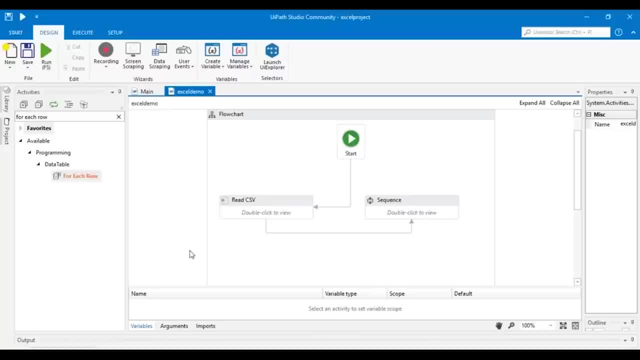 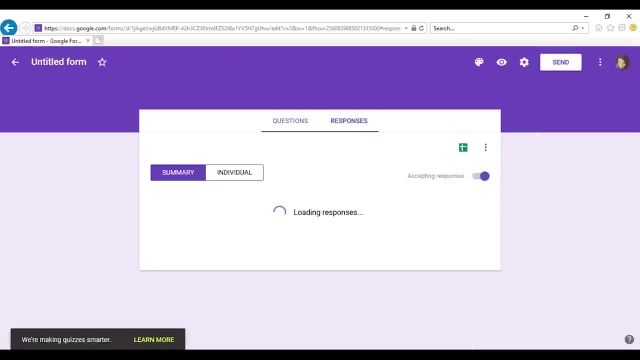 it will return back to the uipath tool. So now let's open the Google forms and see the number of responses. right? So let me just open the Google form So you can observe all the responses here. So that means a project was successful. 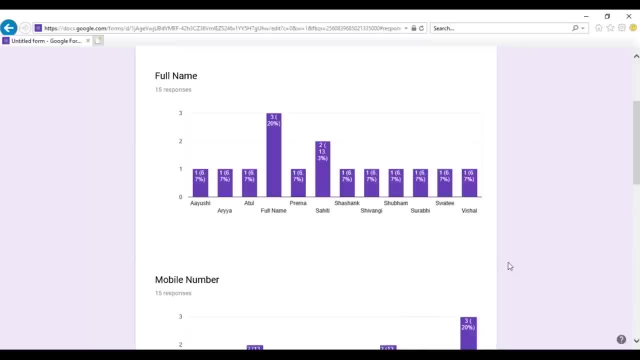 So, guys, you just saw how a simple Excel activity got just automated. You can implement this at a large scale. So let's go back to the industry, where many hypergrowth companies are using it to automate the task, to save time, money and also get the task done with high accuracy. 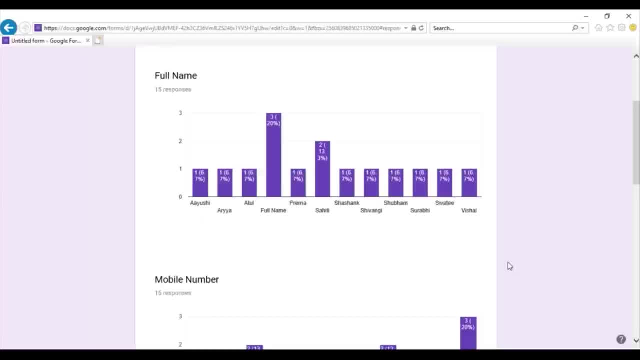 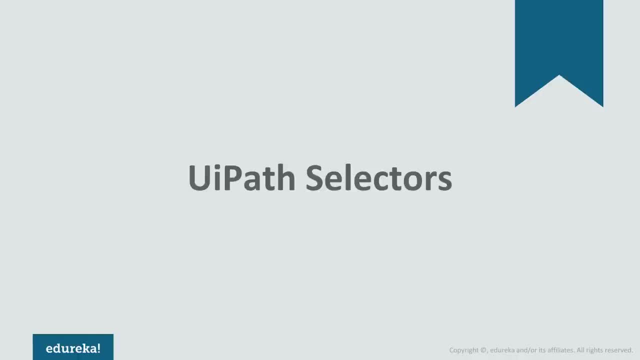 right. So that's how automation will help you to enhance your businesses in the scaling industry. Today, in this session, we are going to see what are selectors exactly and why do we need them in uipath, right? So, without wasting any time, 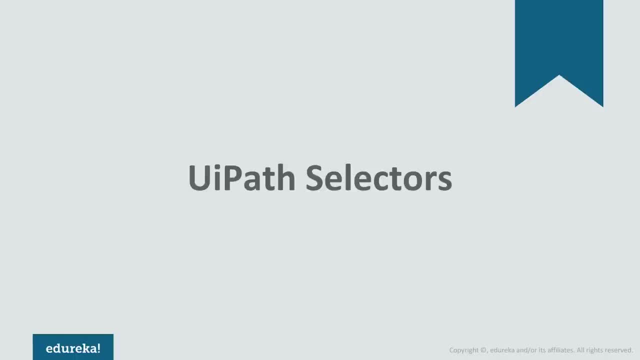 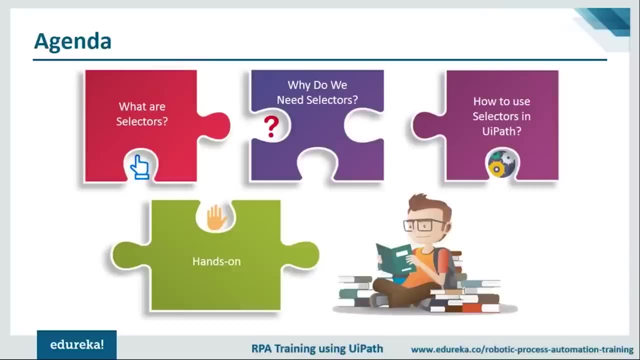 let's move on to the agenda. all we'll be covering in today's session. So we start this session by first discussing what are selectors and then we'll see why do we need selectors in uipath. After that we'll see how to use selectors in uipath and ending our session. 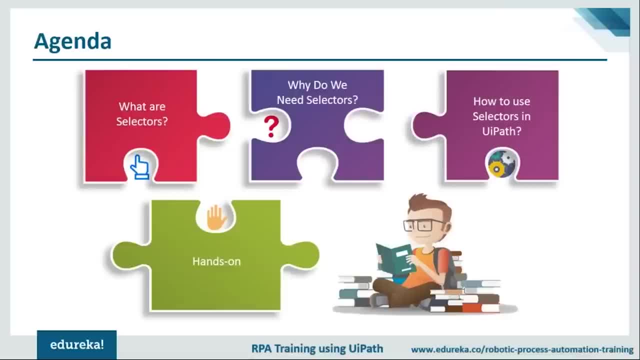 with a hands-on right. So today's session is going to be a quick one, but we are going to know a very important topic in the uipath studio, which is selectors, which is going to help you in doing a lot of automations in. 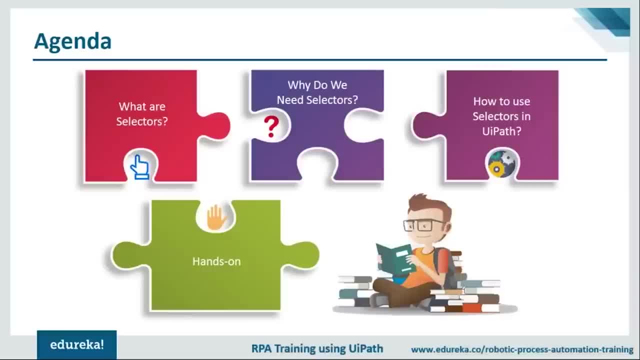 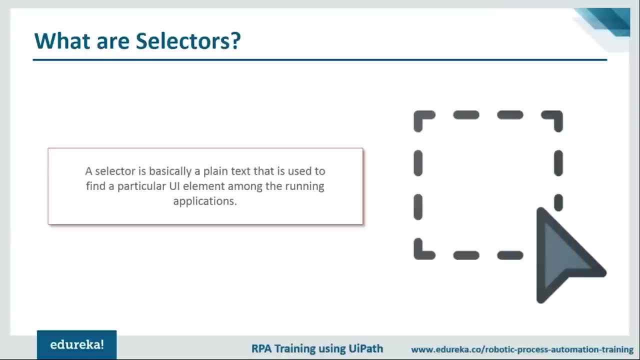 your day-to-day life. All right. so, without wasting any time, let's start with the first topic of today's discussion, which is: what are selectors? So, guys, selectors are nothing but basically a plain text which is used to uniquely identify an element on the screen. 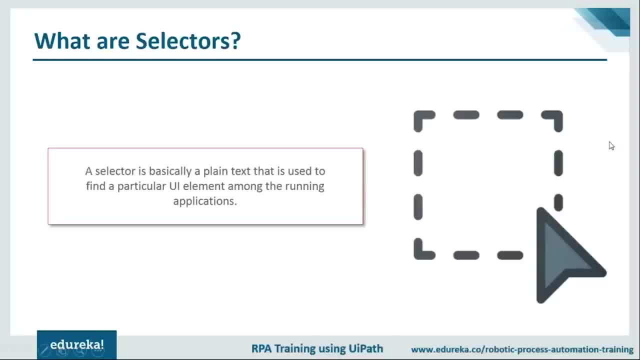 For example, if I am to talk about this particular image that you can currently see as a human, I would say: you know, this is an image which has gray outlines and it has a arrow which is of a semi gray color. right, 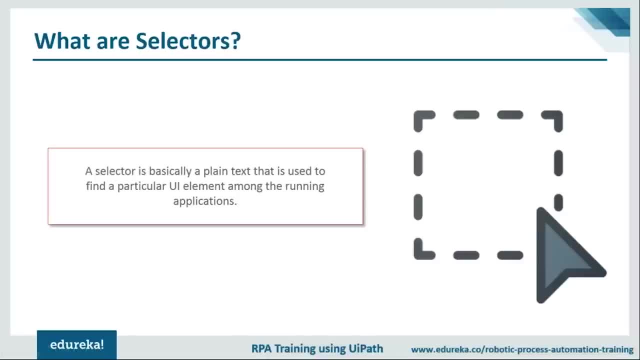 It's on the right side of the screen And it is aligned in the middle of the presentation. So this is the way another person who would like to recognize this particular object on the screen. Now imagine it telling it to a computer. So if you were to tell it to a computer, 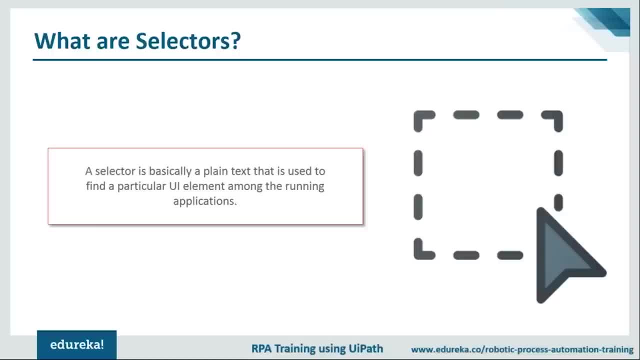 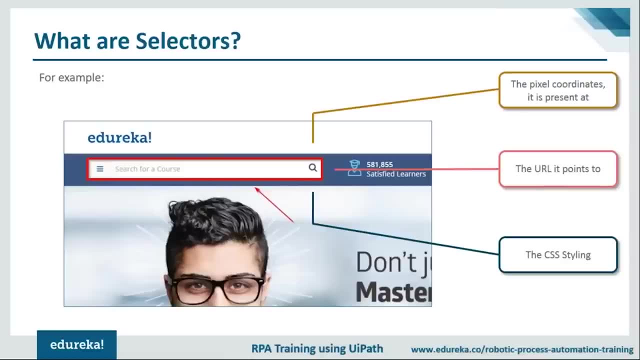 you would do that using plain text of code, right? And you would tell them. for example, if you want to identify an element for a website, let's say for Edureka, there is this element, which is a search box on the website. 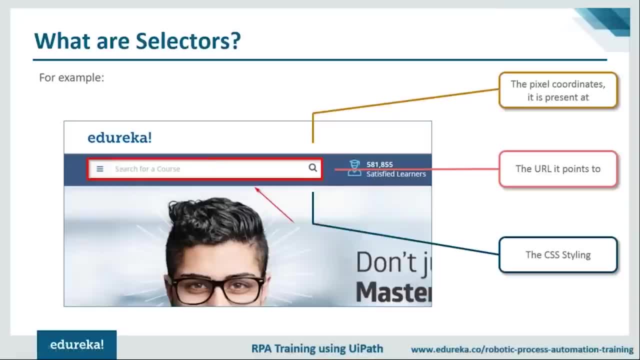 Right Now, if I were to identify this particular element on the screen, if I want to tell the computer that this is the element that you have to identify, let's see how the computer would look into it, or how the computer would actually identify this particular element. 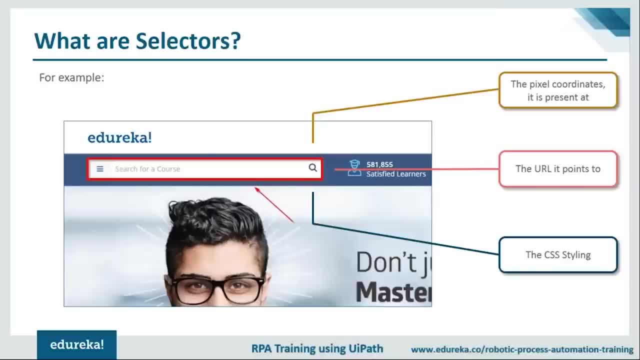 The most generic way of you know identifying elements on a screen is by noting its pixel coordinates down right. So once you have the pixel coordinates, you know where exactly to look for that particular element on the screen And you can easily identify the element there. 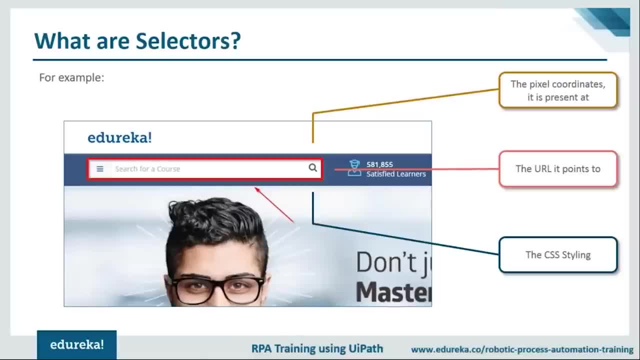 The other way for your computer to identify it is by looking at the URL it is pointing to. For example, if you were to search anything inside the search box, it will always point to something like edurekaco slash search- slash, the search term that is searching for. 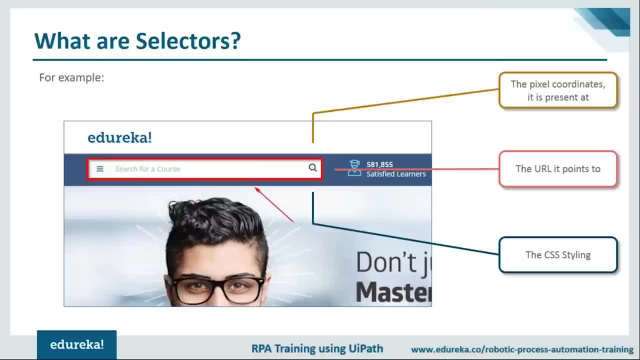 So it will always have this particular URL attached to it, right? So you can easily identify the element on the screen by identifying the URL with which it is Assigned to. the next way You can identify this particular element is by the CSS. All right. 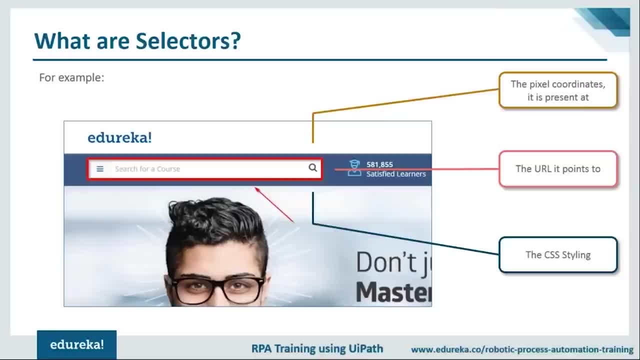 so you can look at the CSS of the search box and you can say, okay, so this particular way, any element that is looking this particular way, is what is to be selected or is what my target element is. All right, So these are all selectors. 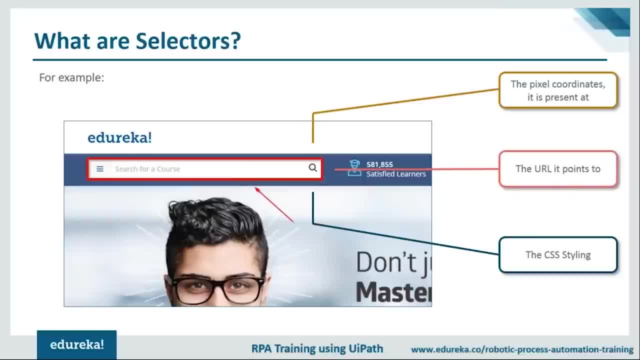 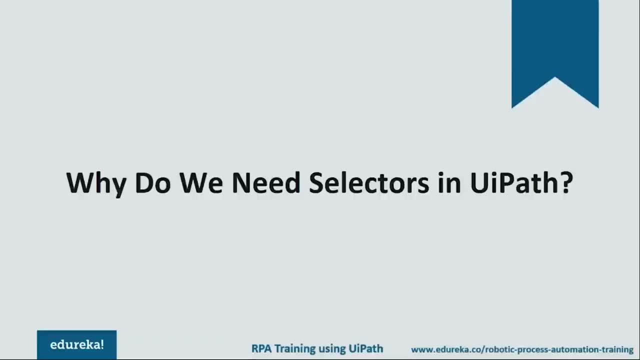 These are all ways of identifying elements on the screen of a computer, and they are called selectors. All right, Now the question that you might be asking yourself is: why do we need selectors in the iPad? So you might be wondering. this is a UiPath session. 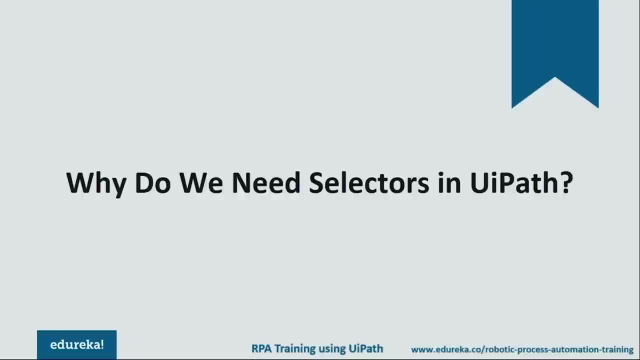 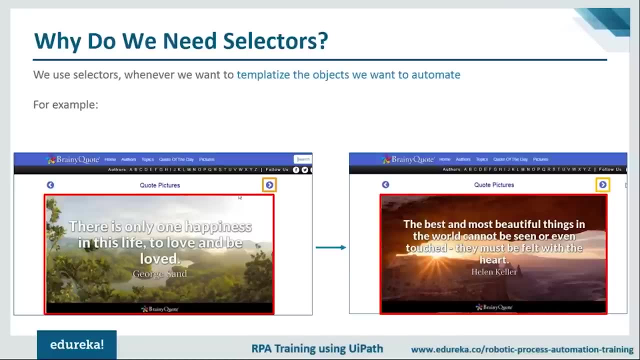 Why are we learning about selectors? All right, So let me explain you how. let me explain you why. so you need selectors, because sometimes the content that you're trying to access, or the content you're trying to automate, is not static, All right, for example, websites. 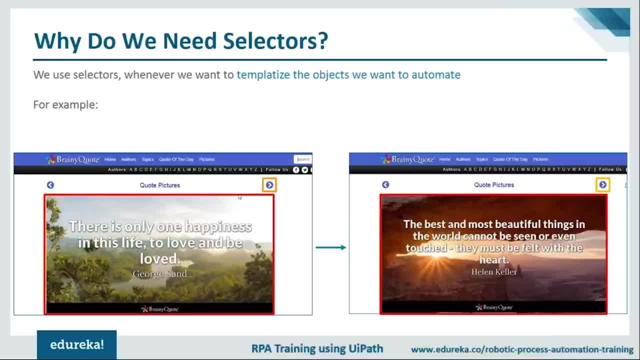 So websites are not static. Everything changes on every page, right? If the whole page is being reloaded, right. For example, this particular website. on this particular website, you will see that the URL of the page changes every time I click on. next. 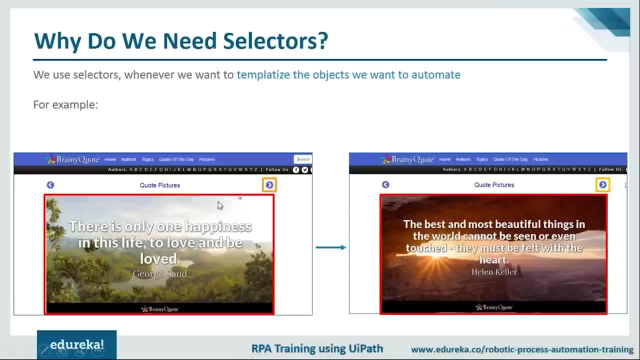 All right. Also, the element like, for example, what I want to do on this particular website is I want to identify this particular image, All right. So whenever I click on next, the properties of this image will change, or the properties of this image box will change. 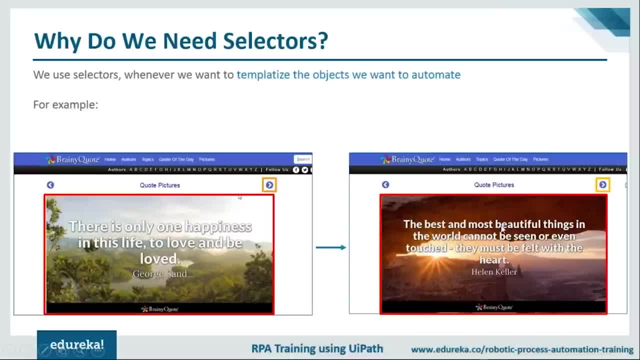 It will not point to this particular image, which might have a different source, origin, It might have a different name, It might have different dimensions, and all of that All right. so everything changes whenever I'm changing the webpage and I want to solve this. 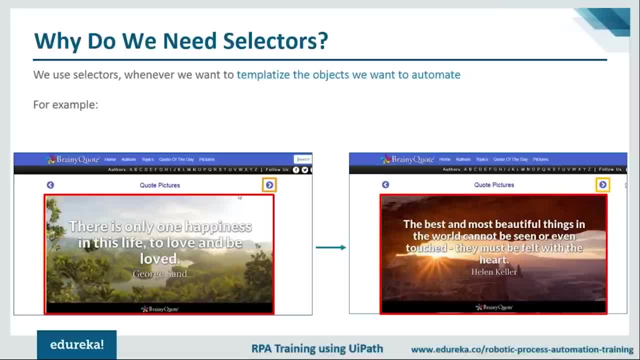 I don't want to automate this part wherein I can easily identify the image, the main image on screen, All right. So if I were to do that, I would use selectors, because using selectors, I can tell you a path that these are the properties that I want to focus on and these are the properties that I don't want to focus on. 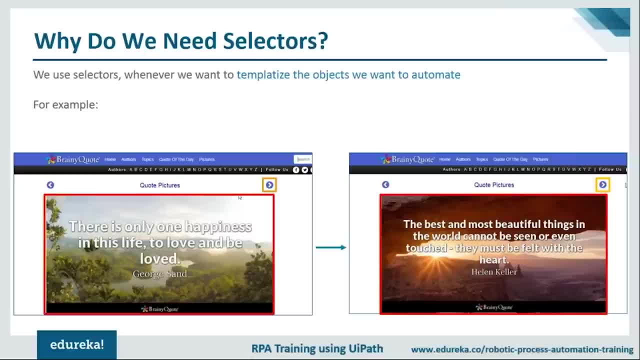 For example, since the name is changing on every web page that I'm getting or I'm pressing next to, I can ignore the name property of this particular image. I can maybe import or I can maybe use some other property which is not changing throughout the website. 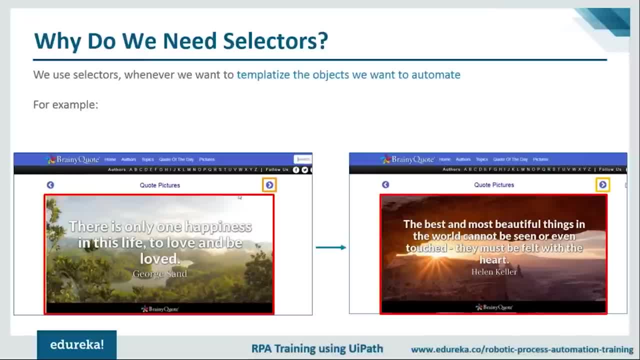 you know, irrespective of whether I'm clicking on next or not. So our aim is using selectors. We have to select the properties which will never change on each, In every page, right? So this is the motive of using selectors in UiPath. 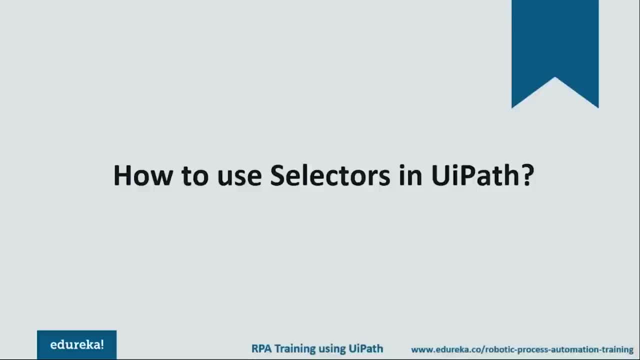 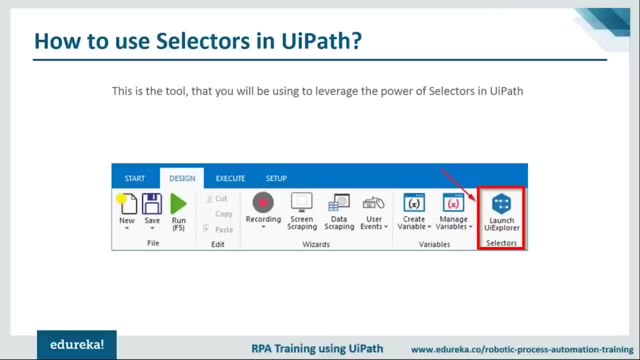 Now, how can you actually use these selectors in your path? if you were to do, or if you were to analyze the selectors of a particular element, how you can do that using UiPath. So let's share a light in that. So in UiPath. 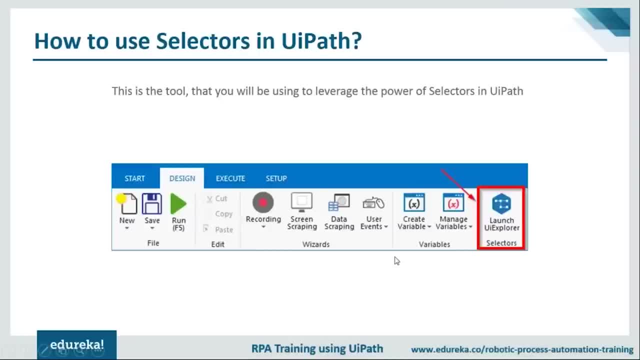 you must have noticed this ribbon which is there on top of the screen, and you must have noticed this particular tool inside UiPath studio, which is called Launch UI Explorer. Now, this is where all the magic happens, guys. This is where you can see all the selectors that your UiPath will be identifying or will be fetching to basically identify that particular element on the screen. 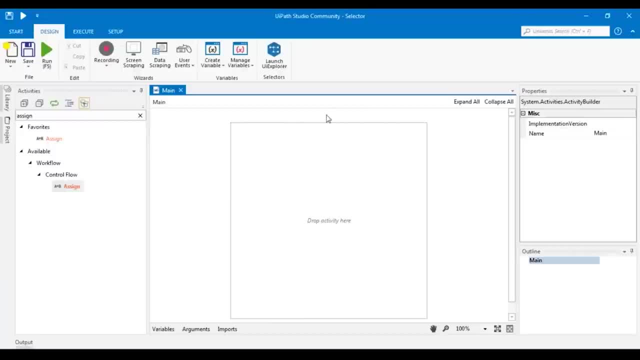 So let me quickly jump to my tool so that I can show you what I basically mean. So this is the ribbon that I was talking about, guys, and this is the tool. This is the magic tool that our video is based on today. So, if you want to analyze a particular element on the screen, 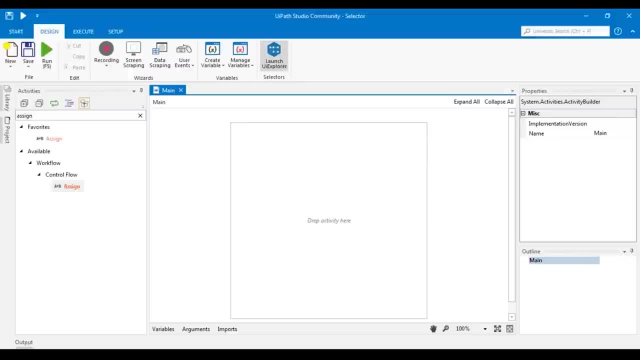 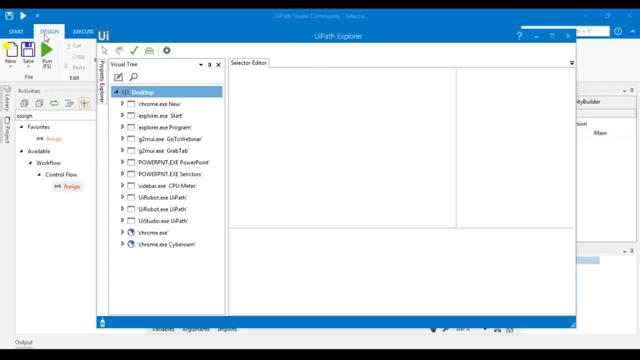 you simply just have to click on Launch UI Explorer, All right, which will give you this particular screen. Now, if I want to identify or if I want to analyze, say, the run icon on the UiPath studio, let's see how I can select or how I can list the selectors for this particular element. 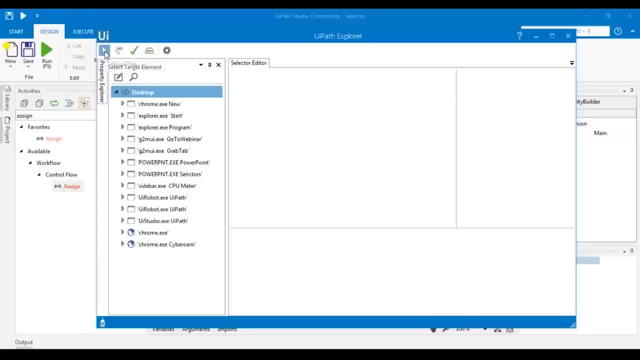 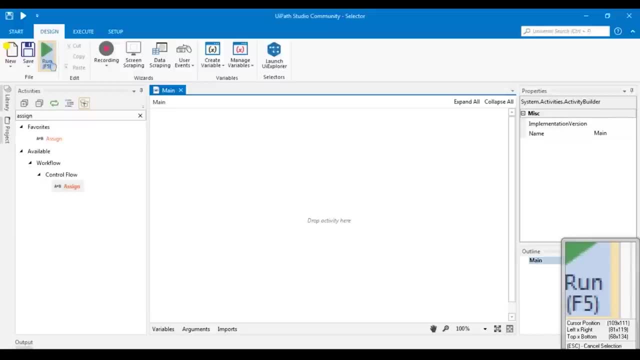 So you will click on this particular icon which says select target element. I'll click there and then I'll select or I'll hover on the element which I want to identify using selectors. So say, I want to identify the run icon on UiPath Studio. 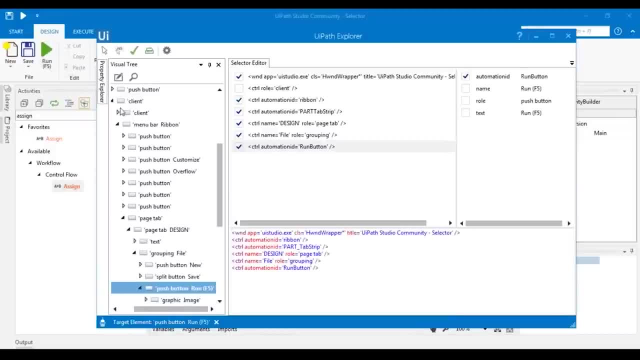 I click on run right and then it will give me all the selectors which are related to that particular element. Now, the way selectors work, guys, is like this. Now, I understand most of you guys must be from non-programming backgrounds and I don't want to scare you with the code. 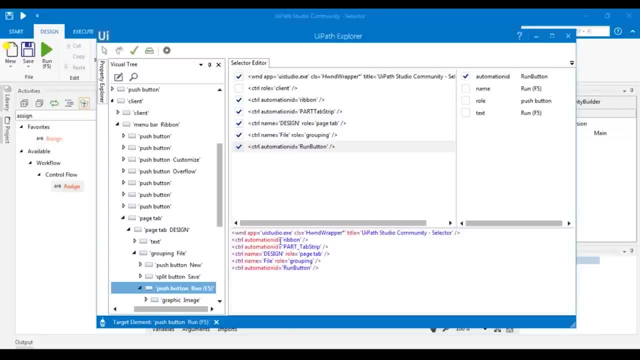 right. So it is very easy to understand if you try to see what is happening. So the way this particular icon has been recognized is like this. So the first line which comes in selectors is basically the window which will have that particular element. So if you look at it, 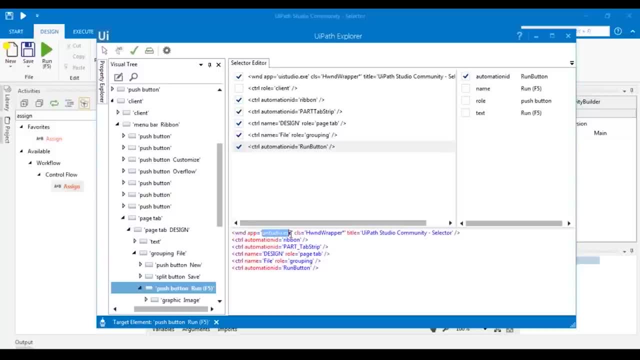 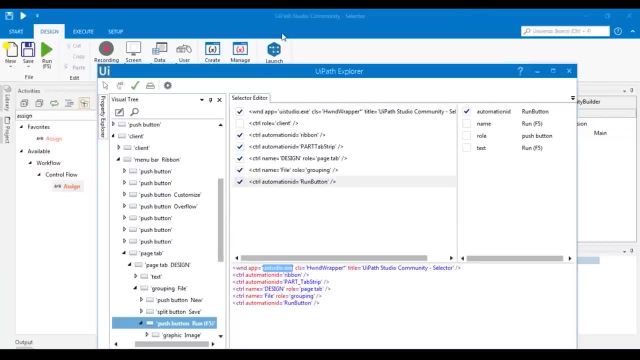 it is looking for a window whose title is UiStudioexe, which is basically this. So this is the window which is being, you know, recognized in the whole of the desktop or on the whole of the screen. Once it finds UiStudioexe window, it will look for the title which is UiPath Studio. 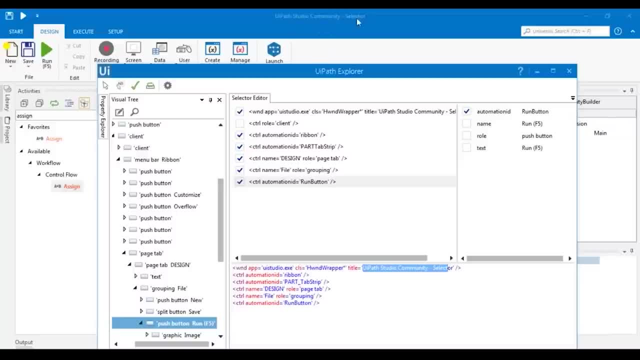 Community hyphen selector. So, as you can see, it is matching this title. So, if all these things match, it has successfully identified the window. Once it identifies the window, it will go into the ribbon. So, as you can see, the ID of that particular element is ribbon. 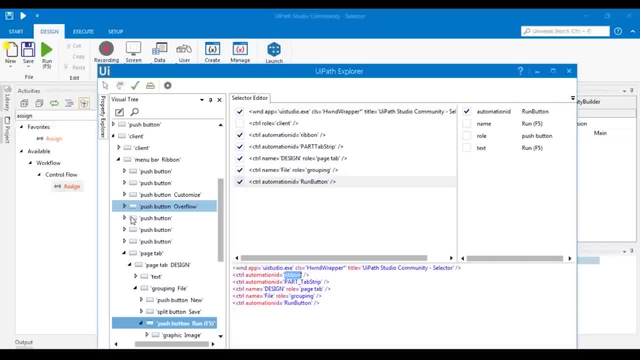 So this is the ribbon for your particular element. right inside the ribbon There is one more ID which is called part underscore, tab strip. So basically it would point to this particular space on the ribbon And then so on and so forth. in the end, 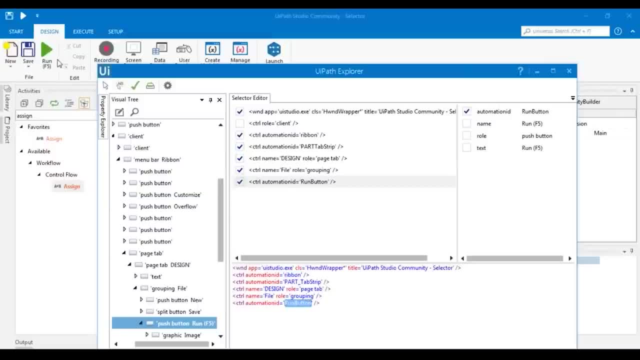 it will have the run button right and this is how you will reach the run button. Or this is how your UiPath Studio is recognizing the run button. It is taking a top-down approach. It starts from the window, drills down into the components and then gets that particular element. 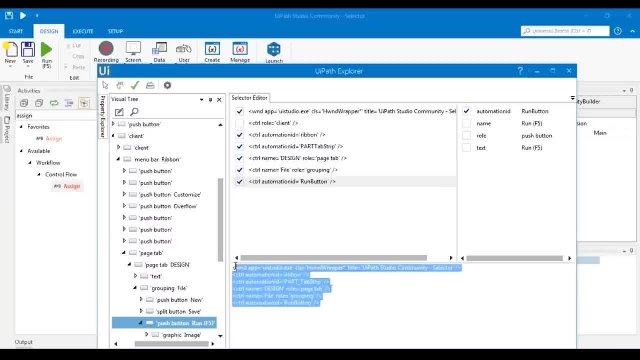 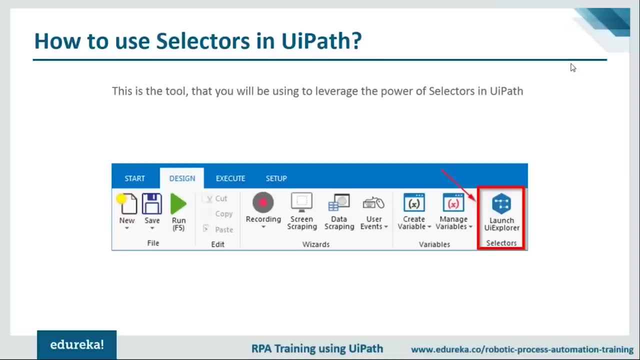 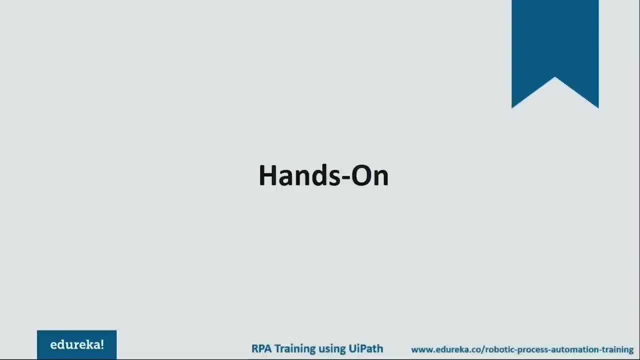 right. So these are the selectors guys. This is how you can identify selectors for a particular element on the screen. Now moving on, this is a very general example. This was just to teach you how you can identify the selectors in UiPath. Now let's move on to the hands-on part, wherein we'll be actually seeing which exact places will use selectors to solve them. 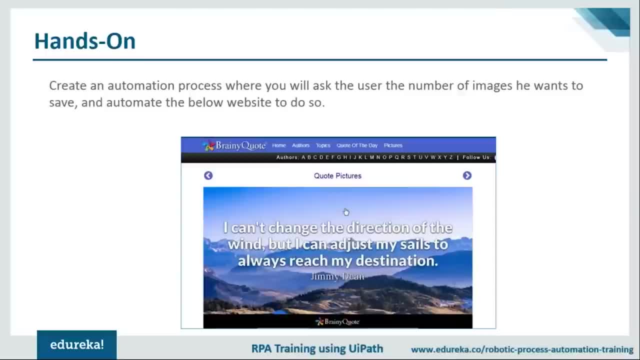 All right. so let's look at the problem statement. So let's take the example for word that we took before, right? So this is a website which basically gives you nice quotes on images. right now, I like the images, guys, So I want all these images, or I want a particular number of images, to be. 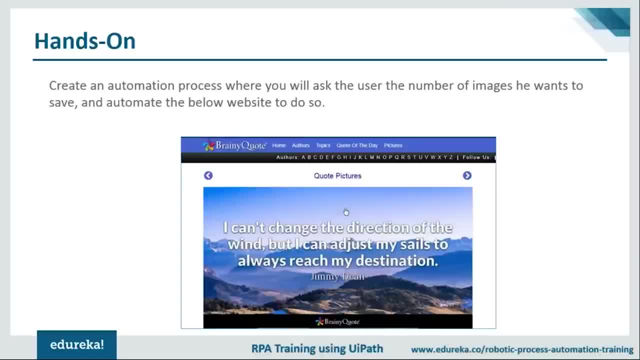 downloaded from the site automatically, right? So if you were to do it as a human, if you were to do it, you would basically right click on the image, save image as, and then give the name and you know, save it in a particular folder that you want. 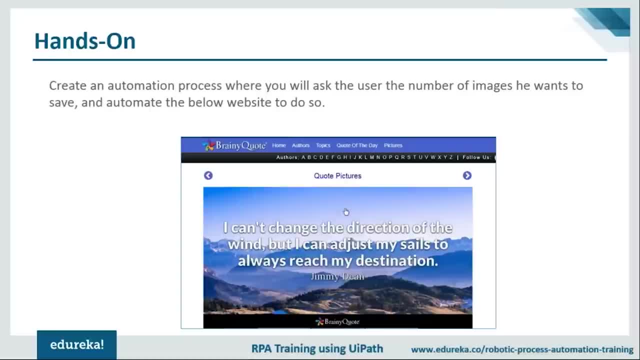 Now say, I want around 50 images from this particular website. So if I were to do so, it will be a very cumbersome task for me and I want to solve that All right. So if I were to solve that, I would be using UiPath Studio and in the UiPath Studio 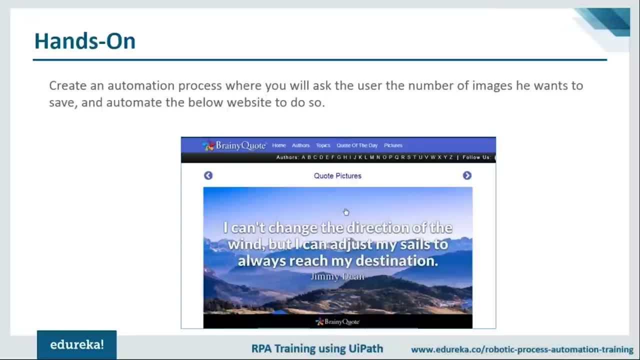 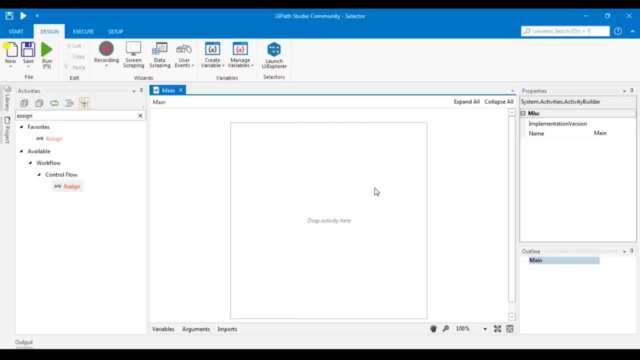 I will be designing the automation for this Particular demonstration. So let's see how we can do that. So let me go to my tool, All right. So, guys, this is the tools where you will be, or this is the area where you will be designing your automation. 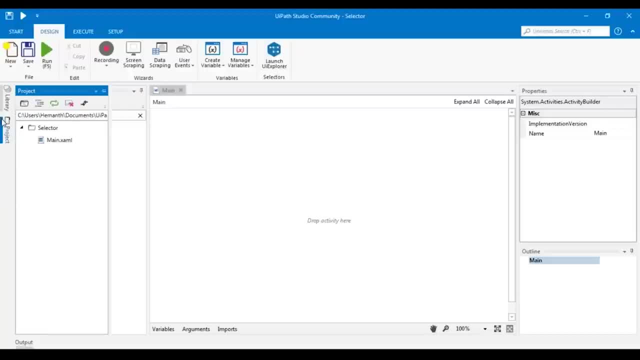 So the first thing that you need to have is a sequence. So you need to have a sequence of steps. So let me type in sequence, All right? So the first thing that you need is a sequence of steps, right, The first thing that I need to have. 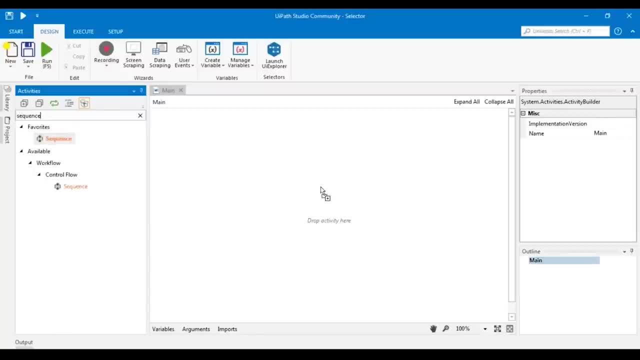 In my workspace area is a sequence. Let me drag and drop the sequence over here. So I have a sequence. now. inside the sequence, I'll have a series of steps that I want to execute one by one. So the first thing that I want to do is go to this particular website. 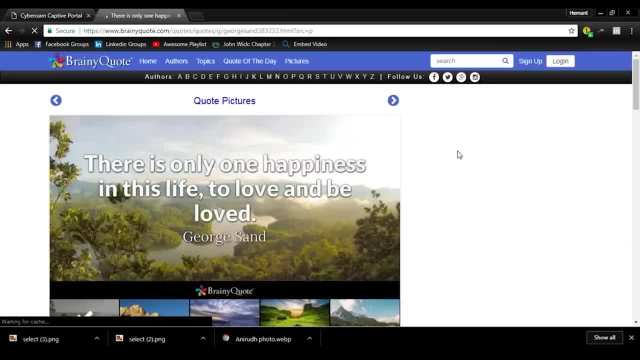 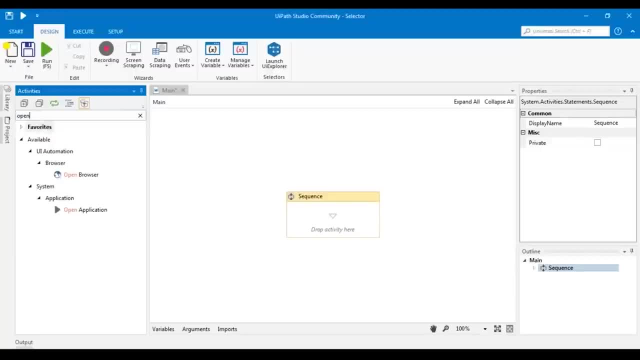 which is having the codes for me, right. So this is the website that I want to go to. Let me tell my UiPath Studio how to go to this particular website. So, basically, I have to open a browser and inside that browser, I have to go to this particular link. 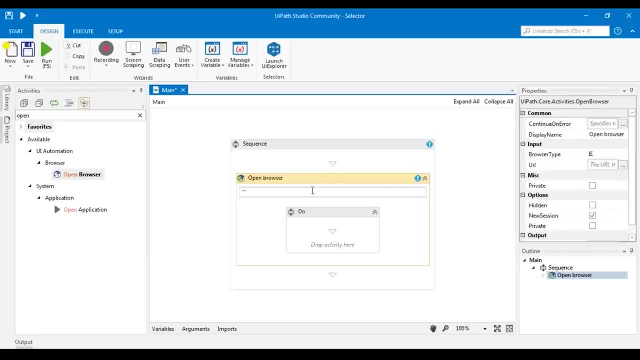 So let me copy the link from here and paste it inside the URL bar. All right, So once I have the URL bar, now my sequence. the first thing that will do is open a browser and it will go to this particular link. Now, which browser do I wanted to open? 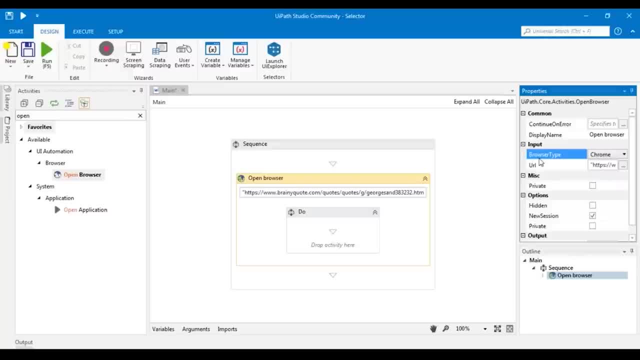 I want it to open me Chrome. All right, so I'll select Chrome from the browser type of properties of this particular element. next that I want to what I want My UiPath Studio is take a screenshot of this particular image, All right. 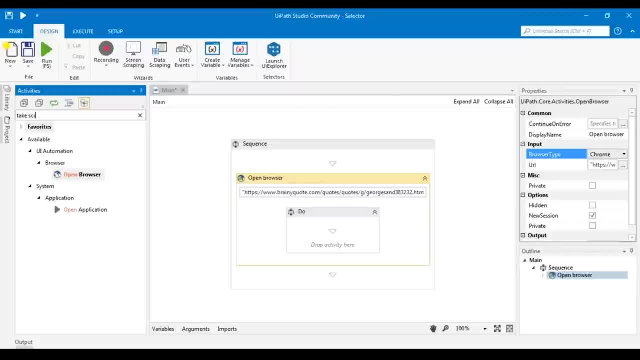 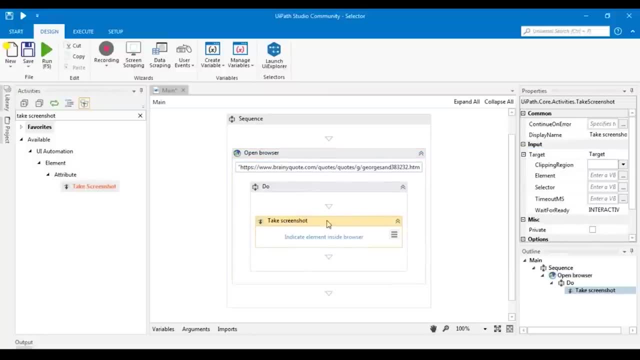 So what I do is I'll simply write take screenshot- right, I'll get this element or I'll get this activity and drag and drop it here And now. I have to tell the take screenshot activity What exact thing do I want the screenshot off. 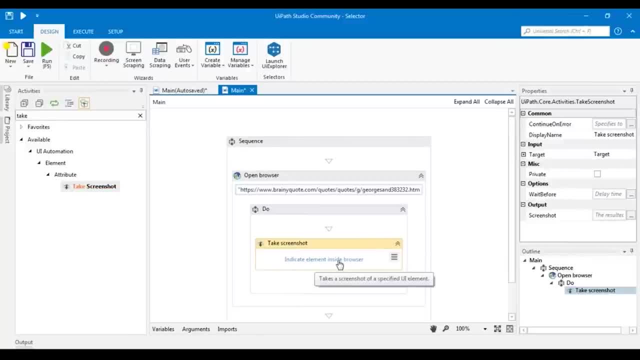 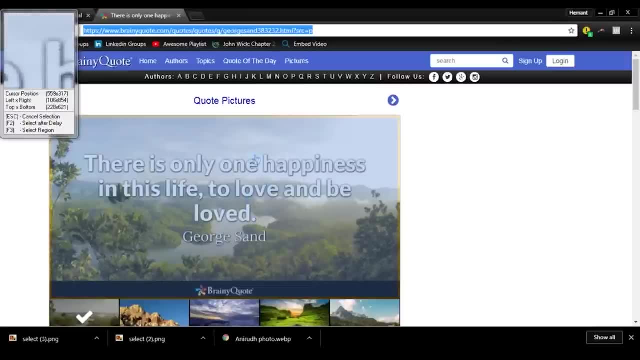 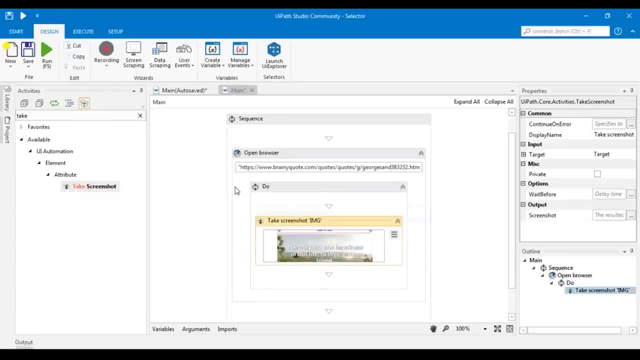 Right. So now I'll click on indicate element inside browser. So once I click here I have to specify which image they want the screenshot off. So, for example, I want this main image to have the screenshot right, So I click on it and the screenshot is taken next. 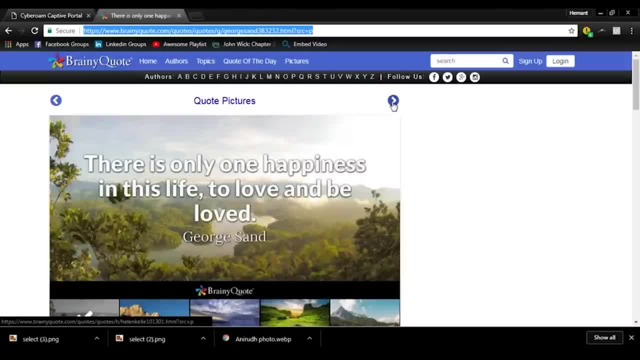 What I want to do is, once I've taken the screenshot, I click on. next, I'll go to the other page and I'll take the screenshot again and do it as many times as I want, Right? So the next thing that I want to do is click on next. 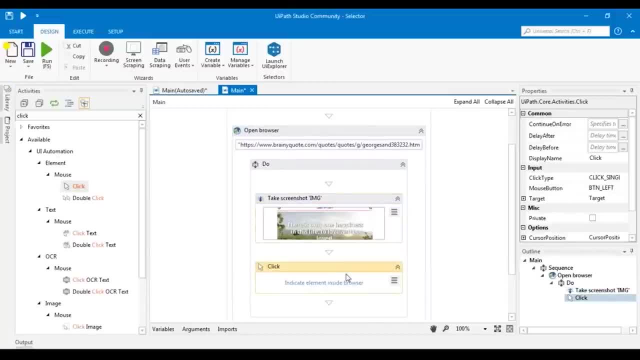 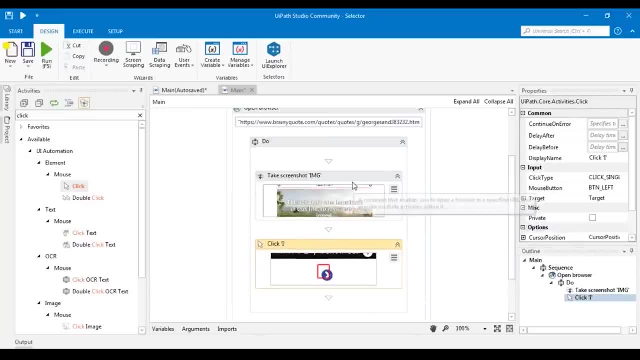 So I type and click a drag and drop it here, indicate the element inside browser which is here, and that is it, Right. So now my UiPath Studio knows that I have to take a screenshot of the image And once I take a screenshot, 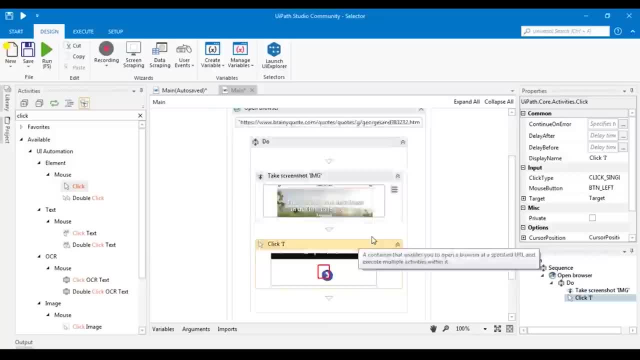 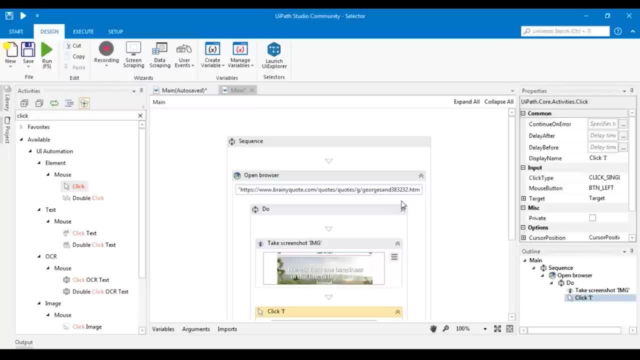 I have to click on next and do it again. Now I want the input from the user as in: how many images do I want, right? So the UiPath should understand that, say, I want 10 images. So it should have a interface to interact with me. 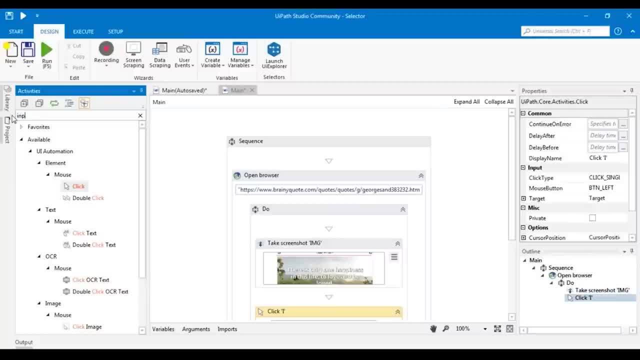 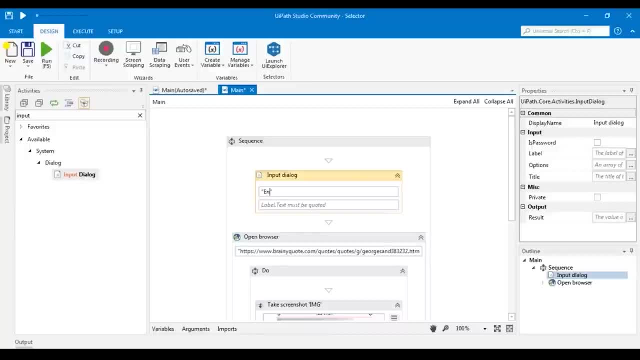 So that interface is basically input dialog. All right, so we type in input and you'll have this activity over here, Just simply. just simply drag and drop it here. It's very simple, and specify what all details do you want your dialect to display to you. 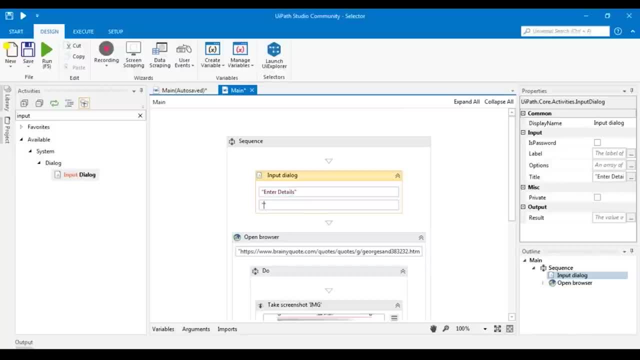 So I'll tell my data to tell me that: enter the details or enter how many images do you want to download. All right, so I've specified that now, whatever entry or whatever number I'll be putting it in this particular input dialog, has to be stored somewhere. 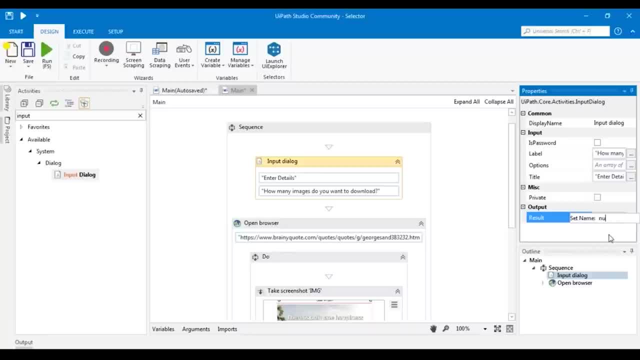 right. So I'll be specifying a variable Here which could be saying: now right, All right. So now whatever I'm entering over here or whatever values I'm entering into the input dialog is being stored in a variable called now. 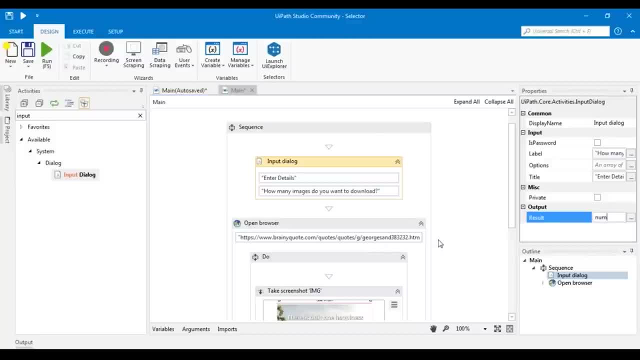 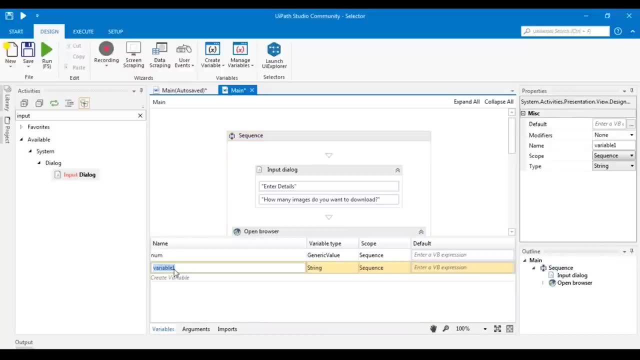 Now, guys, there is two ways to declare a variable. One way of doing it is by clicking on variables and clicking on create variable, and then specifying the name of your variable and then selecting the type of your variable, right? The other way to create your variables is like this: 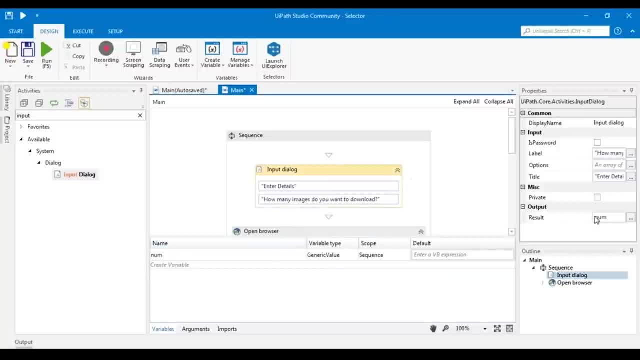 So you know, if I want to delete this variable, just delete it. Say, I want to declare a variable over here, So I'll just simply hit control K And once I've hit control K I can specify what variable do I want my UiPath to store over here? 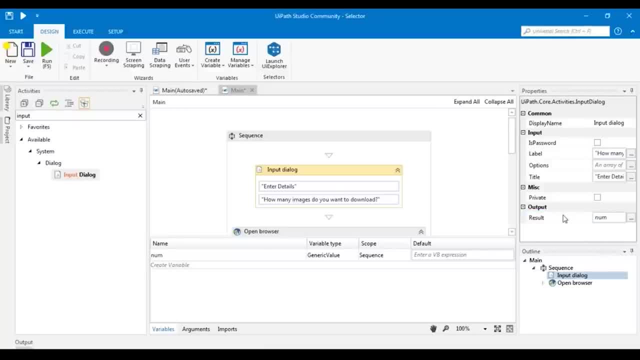 It's very simple. So once I've specified these variable where my value will be stored, the next thing that I want my computer to do- or my I want my UiPath robot to do- is take the screenshots. So, basically, I've told my UiPath robot to take the screenshot and hit on next. 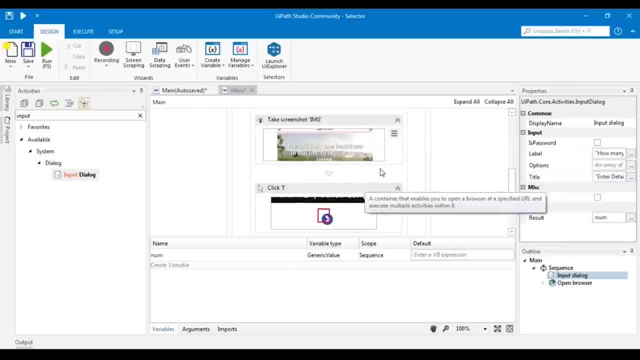 right. But once I do that, I'll also have to save that image in a particular location, So I haven't specified that. So to do that, I will simply say: save image over here and drag and drop the activity here, right? 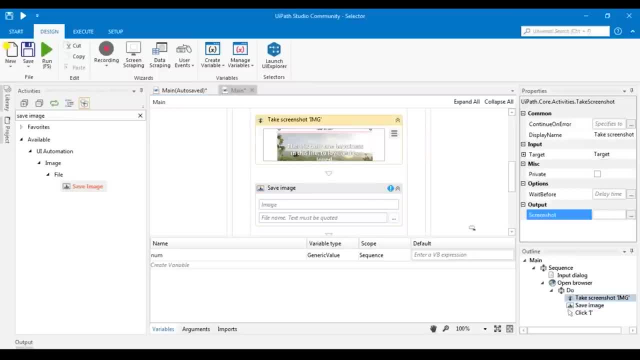 So if it's taking a screenshot, where is it storing? I have to define a variable for that as well. So I simply hit control K. I will specify the variable name as image. It will automatically identify where or you know what type of variable type has to be assigned to this variable. 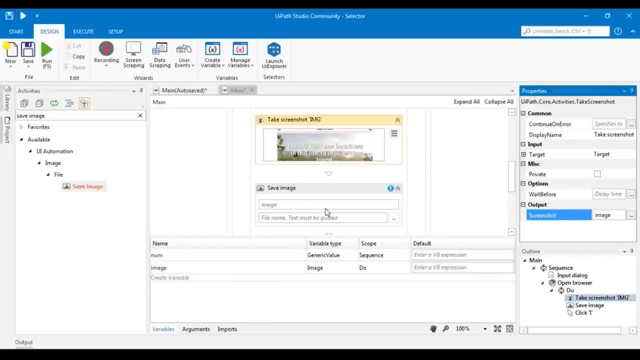 So once it does that it will store that image in this particular variable. and I want to save this variable, or I want to convert this variable into file. So my save image activity will help me doing that. So first I have to specify the variable over here in the first tab. 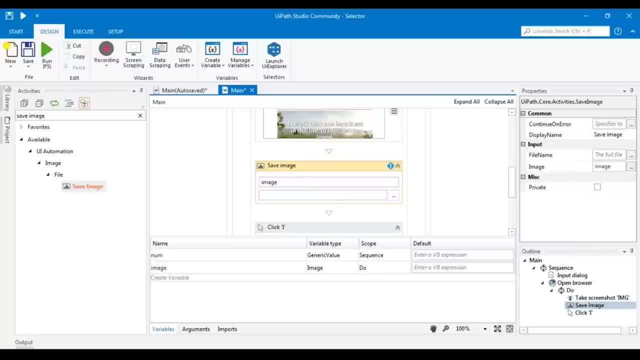 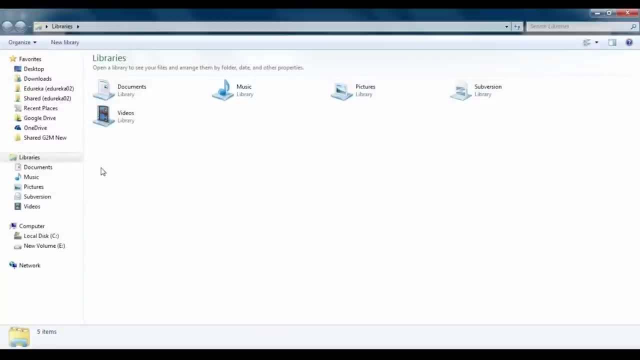 and then the location where I want my select To be or where I want my image to be saved. So for that, let me say I want my images to be stored inside pictures library and say I create a new folder here with the title images. 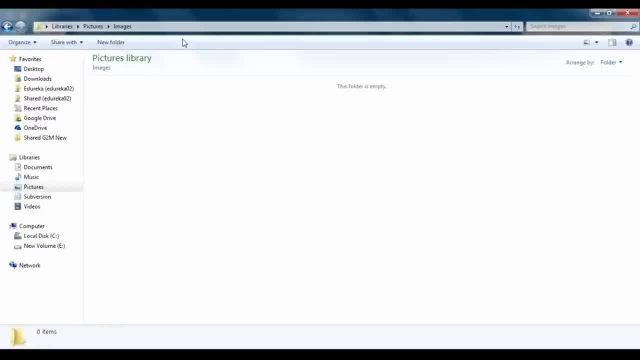 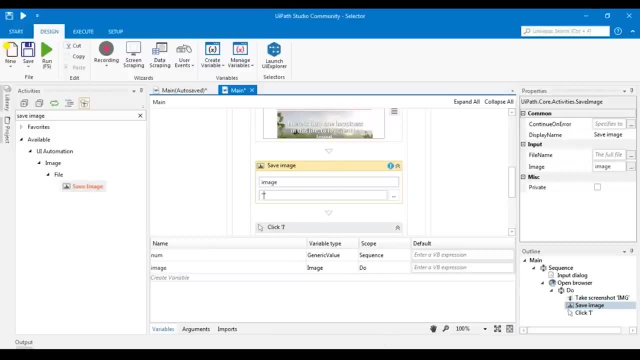 All right, so I want my images to come here. So what I do is I'll simply copy the address from here and save it over here. All right, Now I specify the name Of the file that I want to save, so say it will be image dot PNG. cool, seems fine. 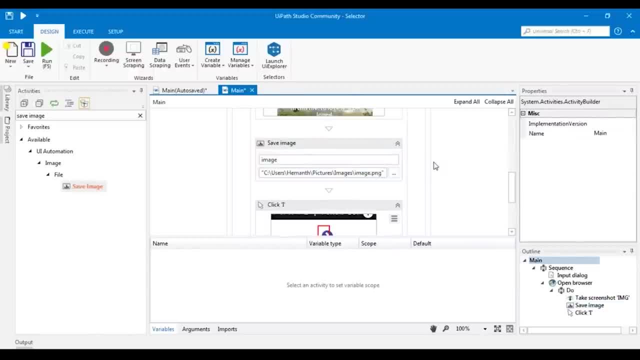 Right now I want to do this process again and again till my number of images that I've specified here is met. So to do that, I'll have to run a loop. Now. There's a loop in UiPath called to while, which basically means that you will do something while that condition is true. 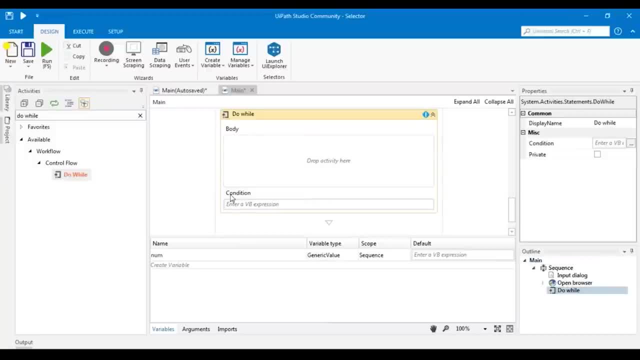 right, So let me drag and drop it Here. So, while this condition is true, it will execute a small or a sequence of steps until the specified condition is true. All right, So what will be the condition? So the condition should basically mean that there will be a variable. say, I create a variable called Val. 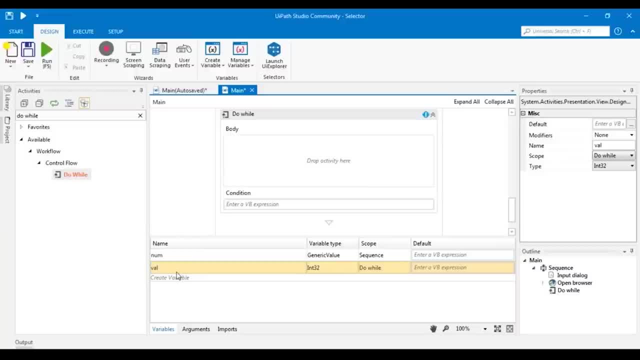 which would basically be an integer, and this integer, till the time it is less than num. That is the number of images that I have provided. It should keep on taking screenshots And once the number of screenshots reach the number of images that I wanted, it will come out of the loop. 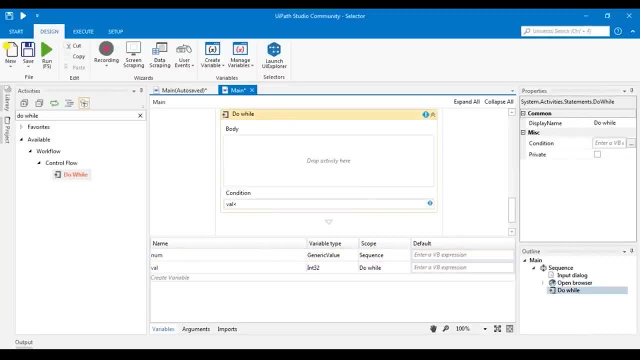 So basically, my condition should be: Val should be lesser than num. All right, Now my num is basically a generic value in variable, So I have to convert it into integer so that it can be compared with Val, right? So the way to convert your variable into integer is C, I, N, T. 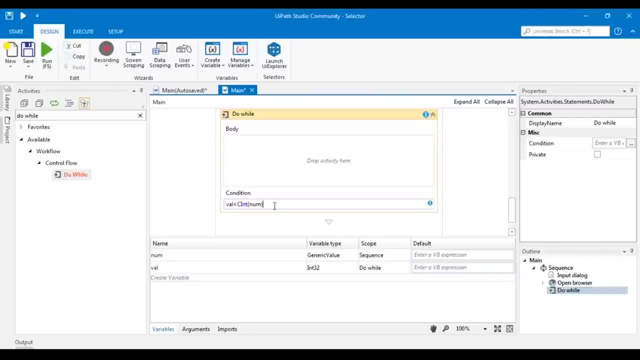 And then brackets. it basically means convert this particular variable into integer. All right, So once it is converted into integer, it can be compared with another integer and, you know, it can be termed as a condition. Now, while this statement is true, 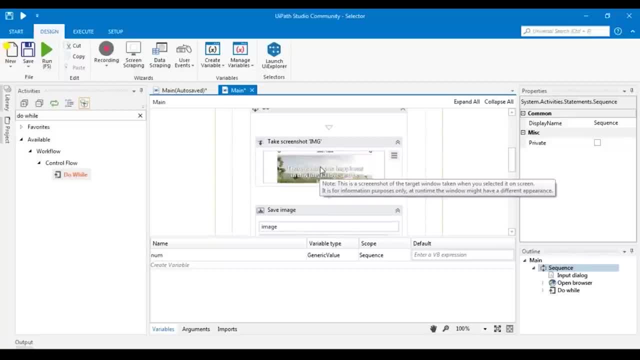 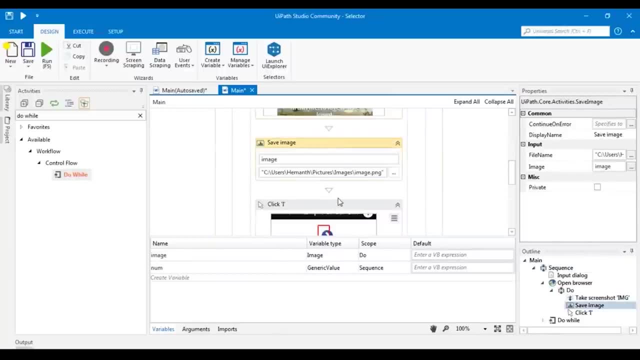 I want to execute these set of steps, So let me copy these set of steps and paste it inside my for loop, right? So let me copy these steps, Right, and paste it here inside the for loop, and my for loop will basically go inside the do component of my browser. 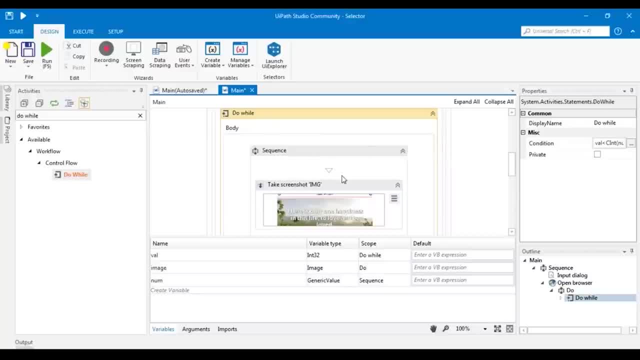 So, whenever my browser will open, it will basically execute a loop, which will execute until my number of images have been taken or the number of images have been downloaded. All right, So now, as I can see, it is taking a screenshot, It is saving the image and then it is clicking next, right now. 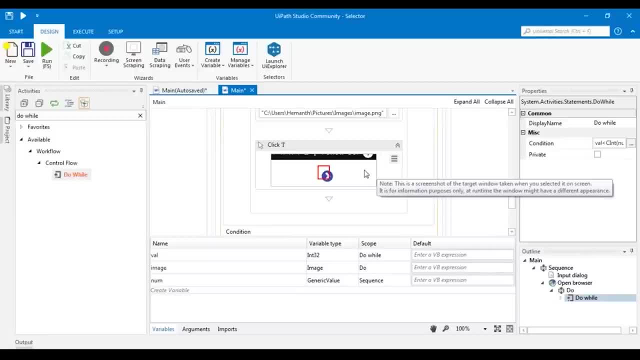 The only one part is left, that whenever you're doing these kind of automation, or whenever you're doing this kind of automation, you are dependent on the website, right? So the website should be loaded fully, So let's give a delay over here. 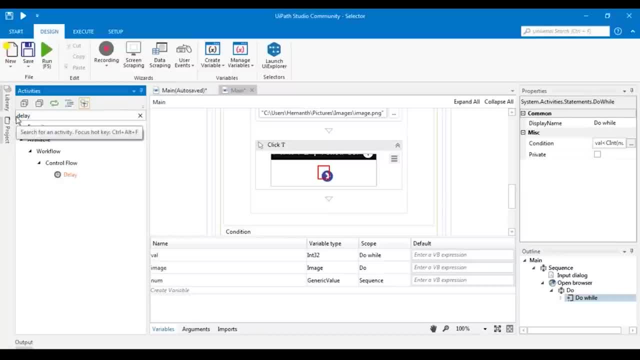 which will basically give our website the time to load properly. All right, let's drag and drop an activity here called delay. I hope you guys understand why I'm adding delay Because, say, I go to this particular website and hit on refresh right now. 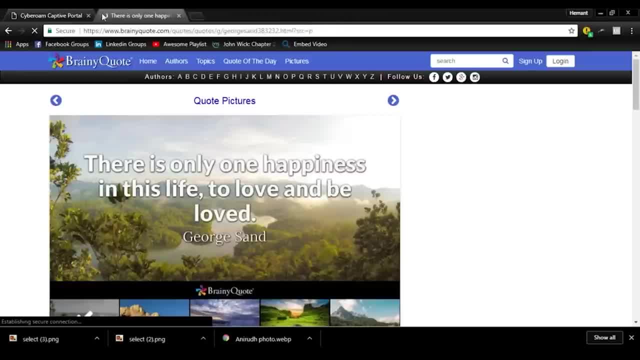 it's taking some time to load, So my computer should give this much time to my machine to load the webpage so that it does not give me an error that the element has not been found, For example, it clicks on next. now My website is taking time to you know. 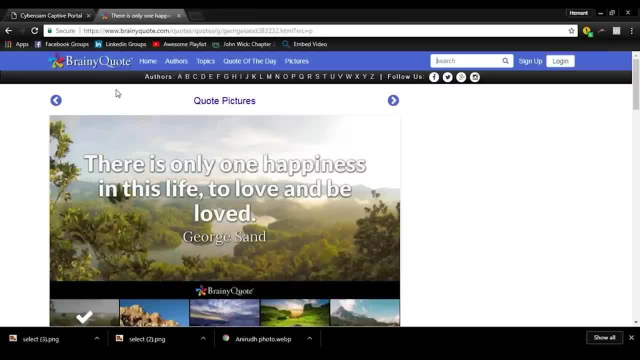 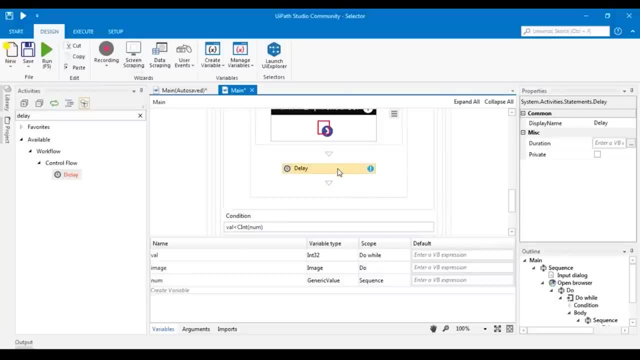 reload and there is nothing on the screen and my UiPath may go crazy that I cannot find the element that you have specified. So, to avoid that, we will use the delay statement, which is basically delay, or will basically, before going to the next iteration of taking the screenshot. 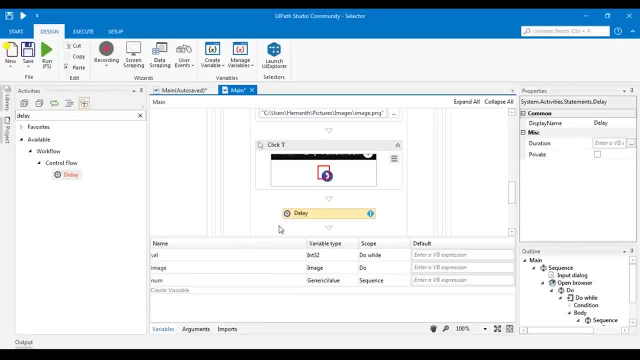 It will wait for three seconds for the website to load, All right, So let's specify the time over here for which it should wait. So the duration should be three seconds. So let us configure it to be three seconds, which will be like this: 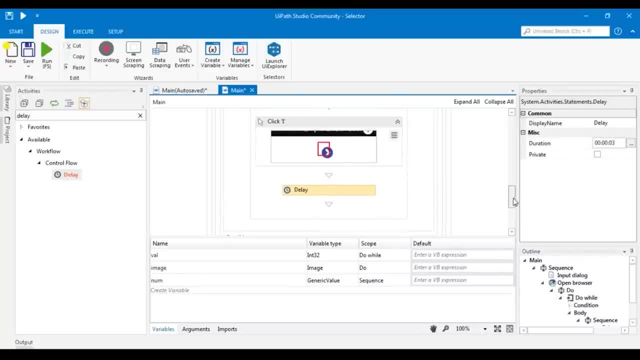 All right, So now my sequence will wait for three seconds before going on to the next iteration. Also, I would want my val integer to be incremented, because only then it will. you know, there'll be a stage when val and num will be comparable, or when they'll be equal. 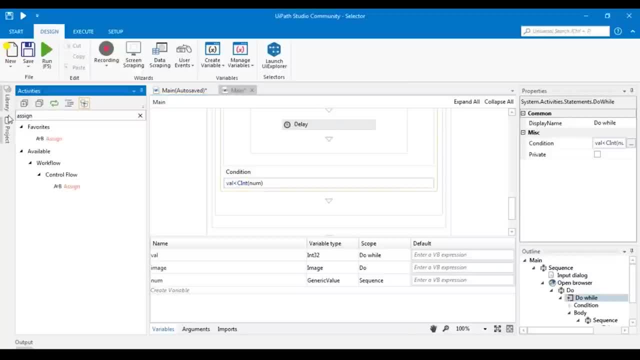 So what I'll do is I will again search for an activity called assign right. I'll drag and drop the assign activity here And let me increment my val by val plus one. I hope you understand this, because my condition is that until and unless my val. 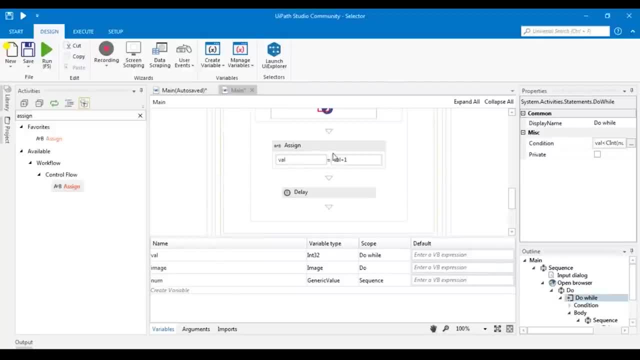 is less than my num variable, this particular loop has to be executed. For example, I want around three images to be downloaded, So my num variables value becomes three right and a val. you know it's default value- Let's specify it here- would be zero. 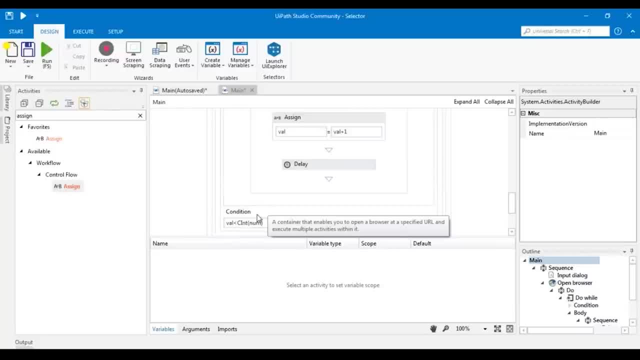 right, So my val's value is zero and my num's value is three. So it will go to this iteration. It will take a screenshot, It will come here and the it will assign the value of val to be plus one, which is so now. it was zero before. 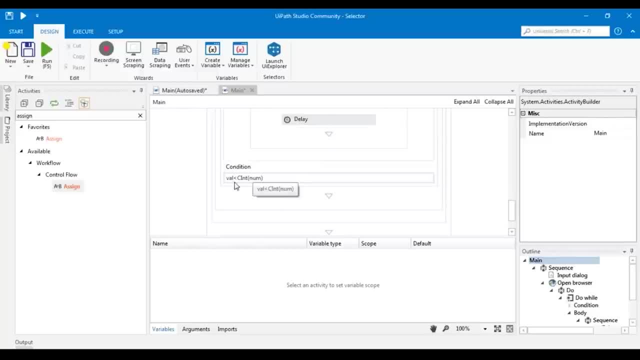 Now it becomes one. right, It again checks the condition. one is less than three. It will again go take one more screenshot. come over here. you know, increment the value of val by one, So now it's two. If it will again compare. 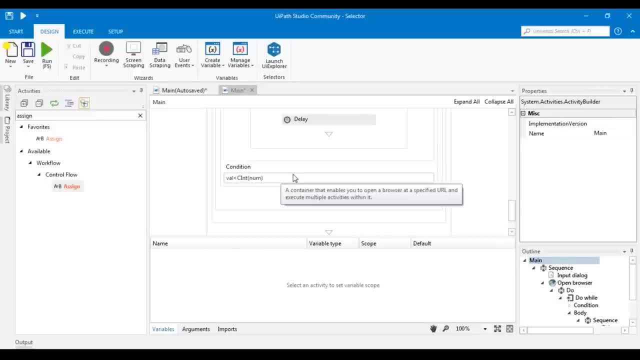 so two is less than three, again do the iteration, So then it becomes three, And since three is less than three is four, it will come out of the loop and end the program. So basically, you get and you end up with three screenshots. 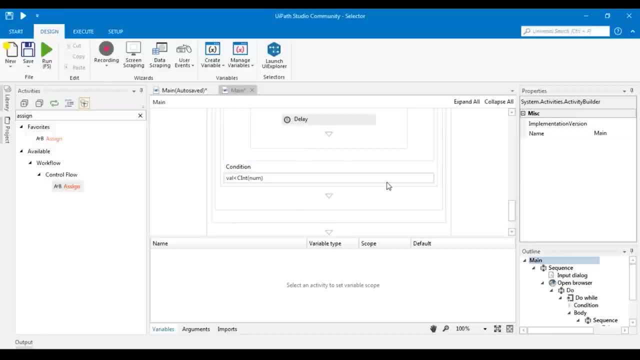 which are the ones that you want, right? So I think this activity is complete now. Now let me show you how this particular program will run. So obviously, this program will not be able to run because at every time the click image or the click button is pressed. 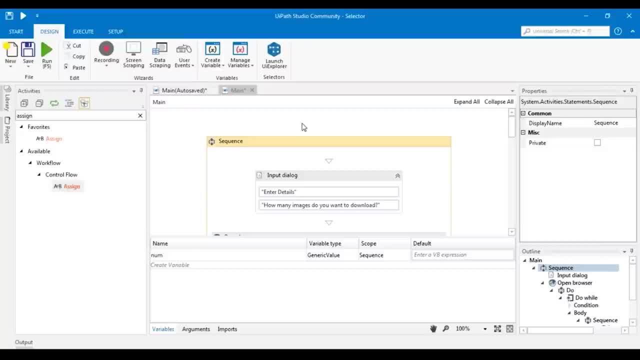 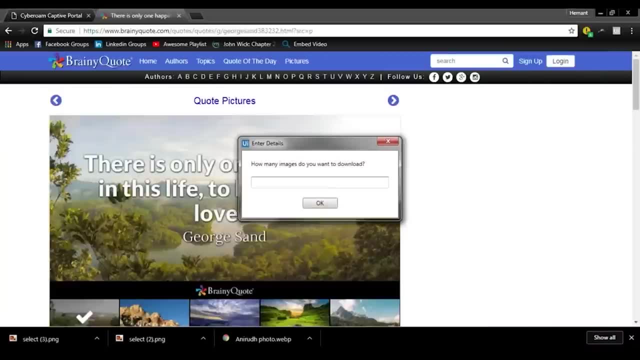 every element on the screen changes. All right, so let us see what we get right now. So let's hit on run. So if I hit on run- this is the input dialog That I was talking about- It will ask me: how many images do I want to download? 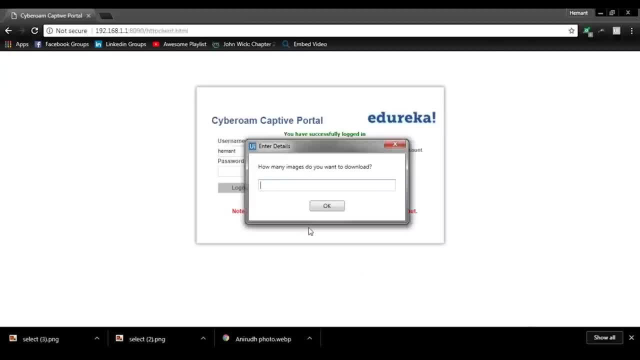 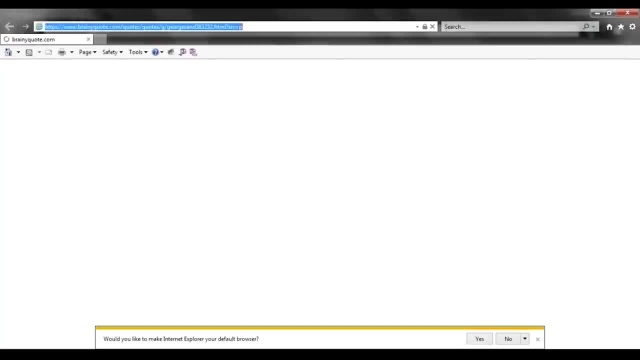 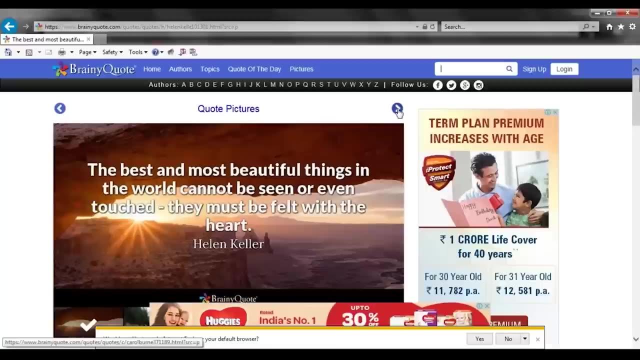 So let me quickly close this tab, so that there is no confusion, and click hit three. Three is the number that I want, So I'll click on Okay. so this will basically open browser. So now it is trying to identify the image on the page and it's hitting next. 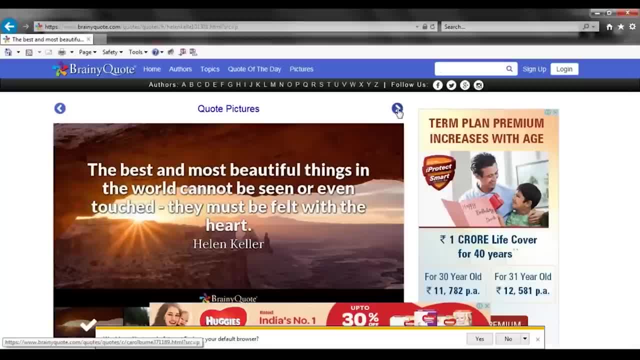 But the thing over here is it can only hit it once right. It cannot identify the image again because everything, all this particular web page, has changed, right. The text of that image is saying: and maybe the source of that image has changed as well: 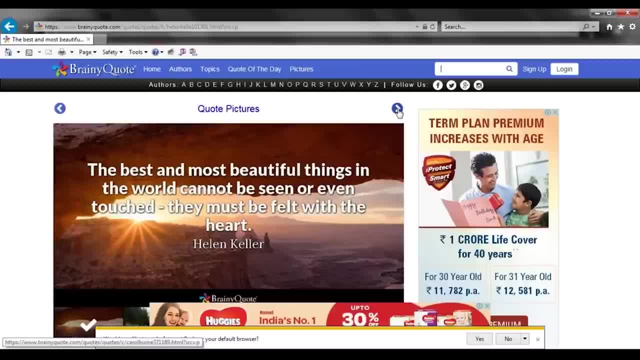 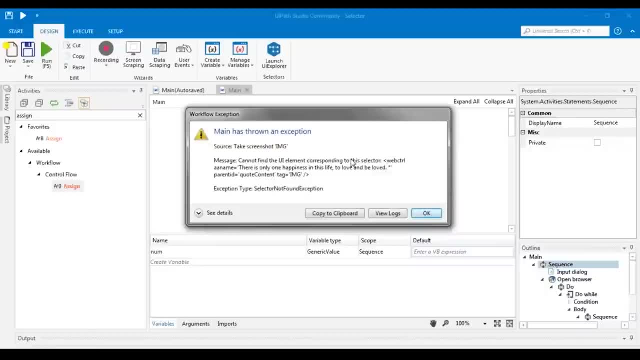 So now it is not able to identify the image on the screen, and hence you see that it is not automating or it is not doing anything anymore, right? So it will take a few seconds, It will keep on trying and then it will give you an error that it is not able to find the UI element corresponding to the selector. 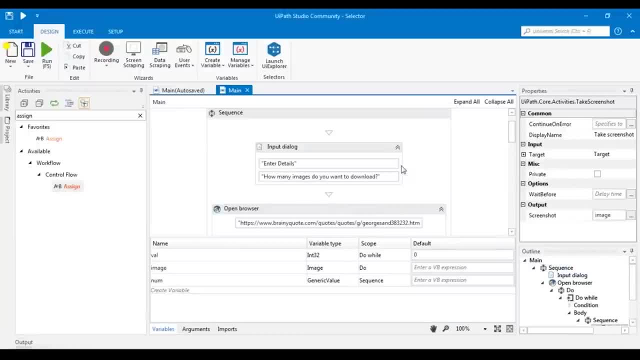 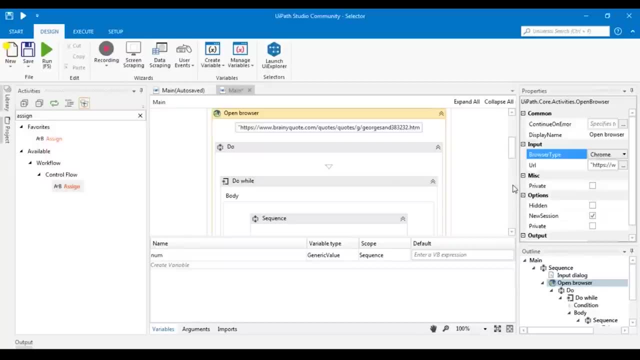 right. So this is the error That you are getting when you're trying to solve it. So let me quickly fix one thing, which is: you know, I want my Chrome browser to open, So I have selected Chrome now, So whenever I'll be doing, 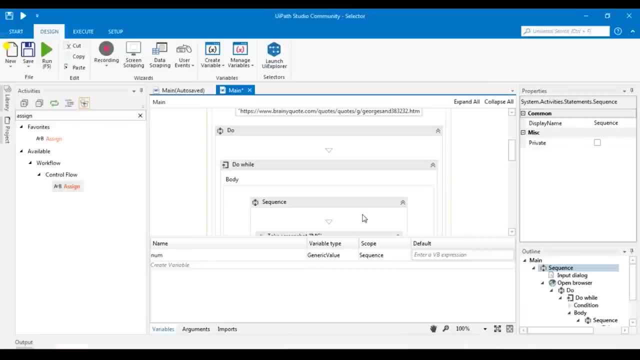 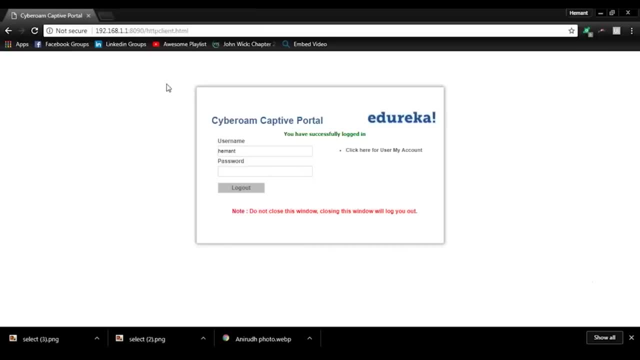 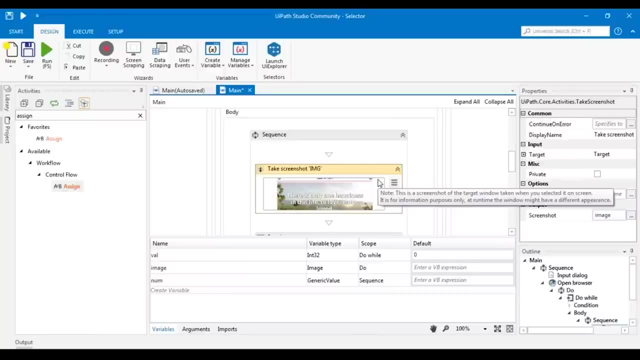 I'll be running this project Now my Chrome browser. I don't want IE. All right, so now let us configure how, or let us see how we can actually template: is this particular image that we had right? Or how we can identify this particular image. 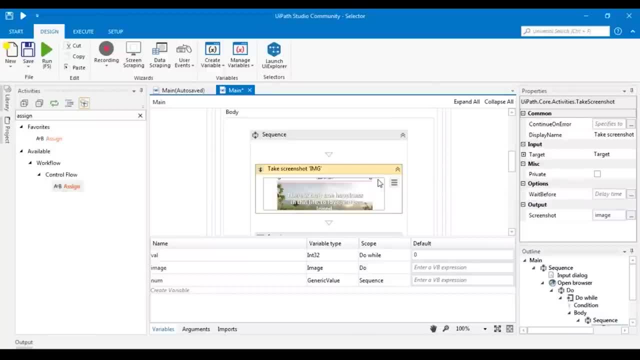 Irrespective of what page we are on or irrespective of what quotation image is there right? So to do that we have to go into selectors. So the way you can select or you can see the selectors for this particular image or that particular image container on that website is going to target right and hitting, and you know. 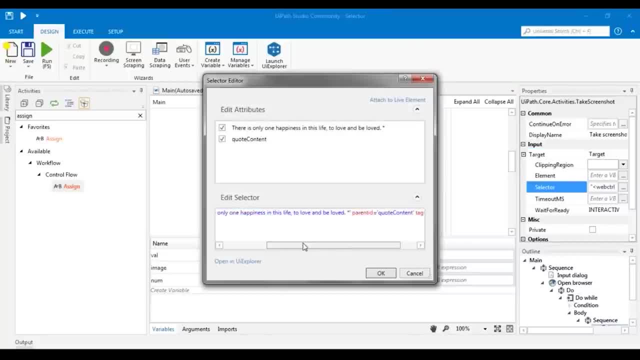 selecting the selector option over here, which is this. So, as you can see, the current selector of this element is including the name, The image as well. So, guys, this is where the problem is right, Whenever we clicking next on the web page. 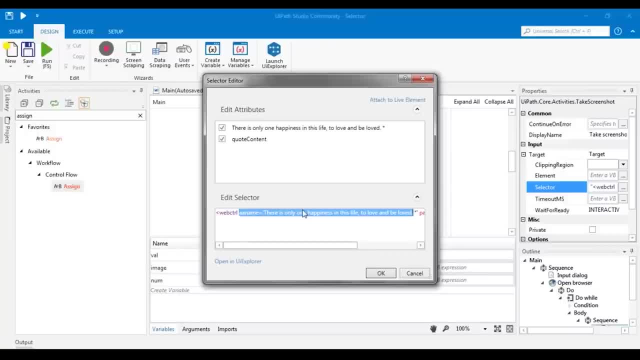 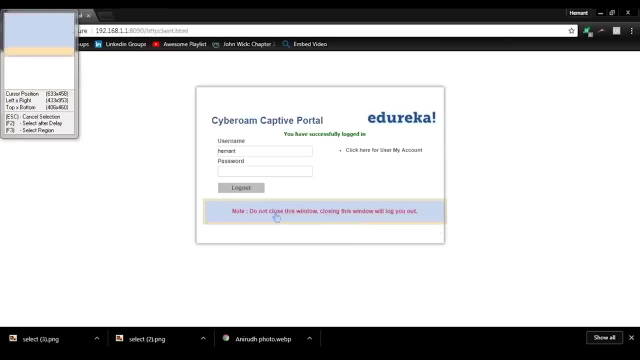 a new image is coming in and this name changes and it is no longer able to match this particular name to that image, right, And that is why we are getting an error. So let's see how we can fix it. So, basically, now what I'll be doing is I'll be clicking on launch UI Explorer. 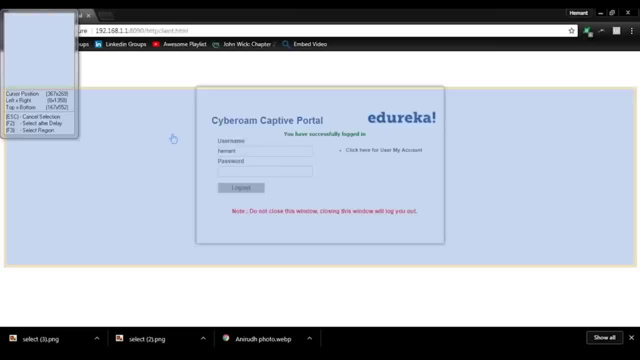 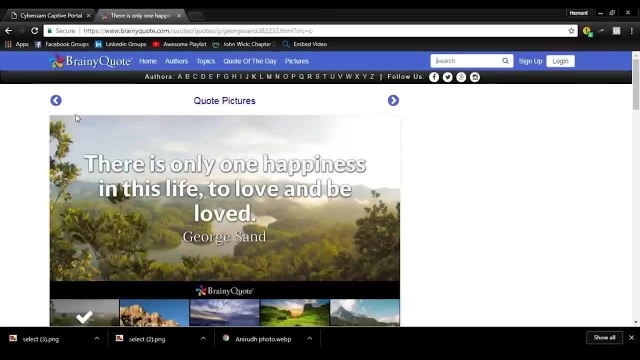 So it is asking me to indicate an element on the screen, So let me hit escape right now to cancel the selection and let me open the web page where my image was. So, basically, I want to template is this particular container which will have the image. 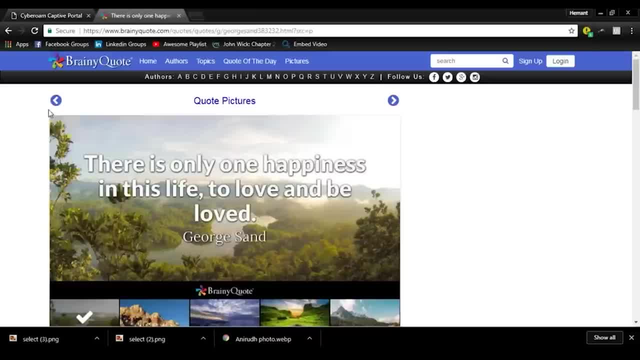 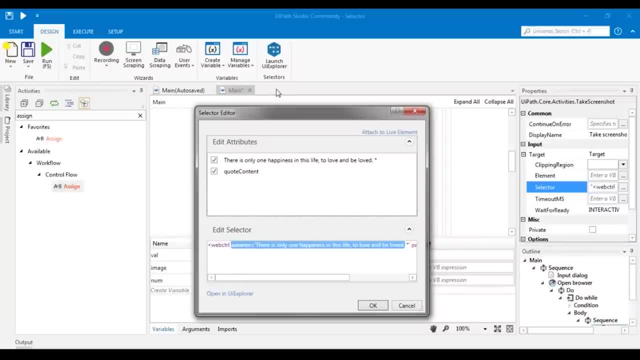 So whenever, whichever page I am on, I want a screenshot or whatever is there inside this particular image container, right? So let's see how we can fix that. So I will click on open UI Explorer and let me indicate that this is the element. 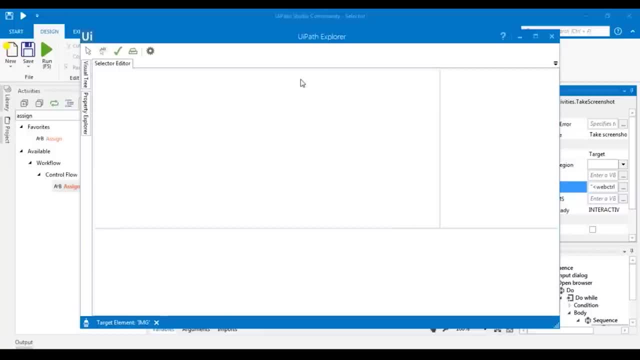 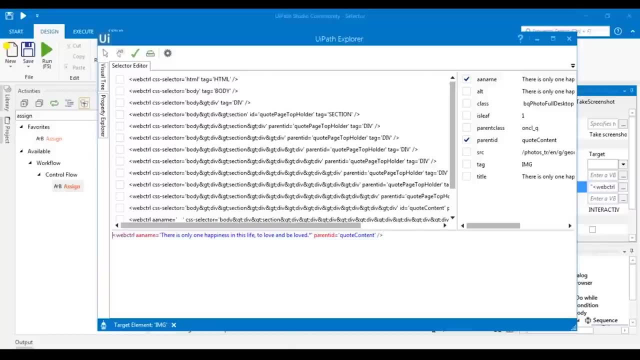 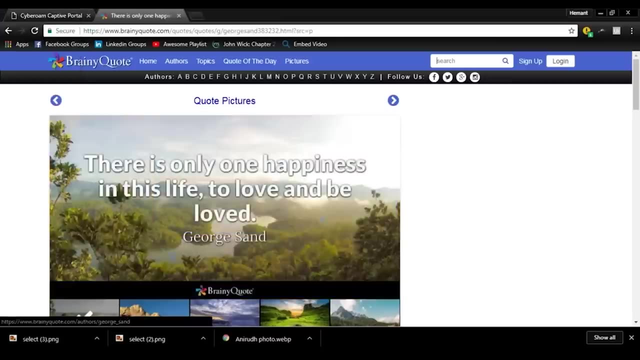 Where I am wanting the selectors to be off. right, So it will open the UI path Explorer and, as you can see, this is the selector that we want to be changed. All right, so let me quickly select the target element again so that I get the original selectors for my image. 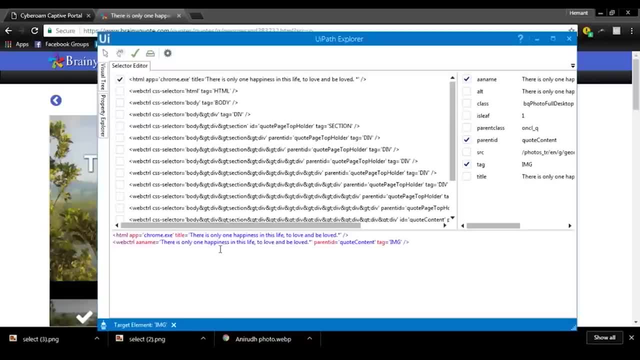 So these are the original selectors- will give me a top-down approach, from the browser till the element that I'm trying to target. Now, as you can see, even the browser has a title which is something like this, which is based on the image that it is showing, right? 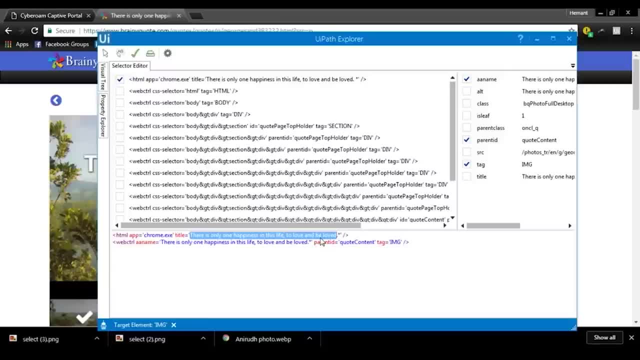 So this is again not good for me, because every time I hit next, this title is changing. All right, so I don't want this title. Now, this is a new thing that you'll be learning, guys: that whenever you are saying that, whatever the right will be or whatever a particular element be, do this. 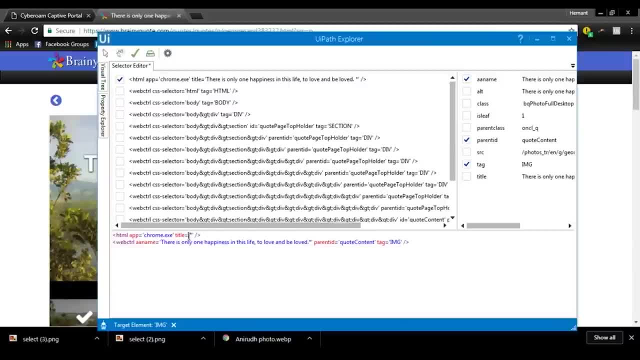 right, So that anything, that placeholder for anything which can come into the existence, Is called star, for example. in this particular case, I'm saying whatever in the Chrome browser, whatever the title be, search for this particular element, All right. the other way to say this could be: or let me give you some clarity on you know. 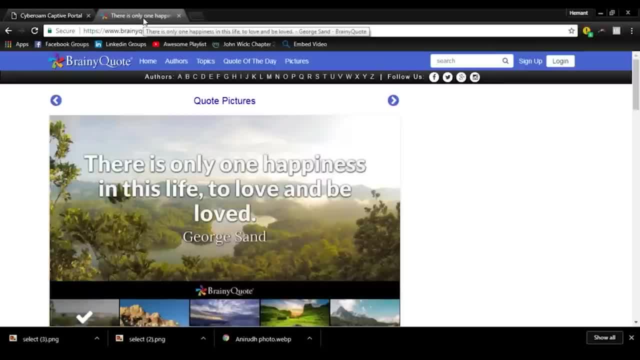 what I'm trying to explain. if I go to this particular browser, you can see that there is a quote over here, and after that brainy quote is being written. All right, let's see if it is same on the next page as well. 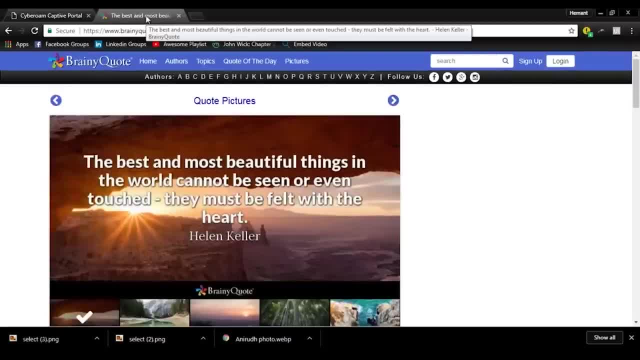 I'll hit next And if I see the title now, I'll again see that the quote has been changed. But what not has changed is the end statement of the title, which is hyphen brainy quote. All right, So if I come back to my selectors, 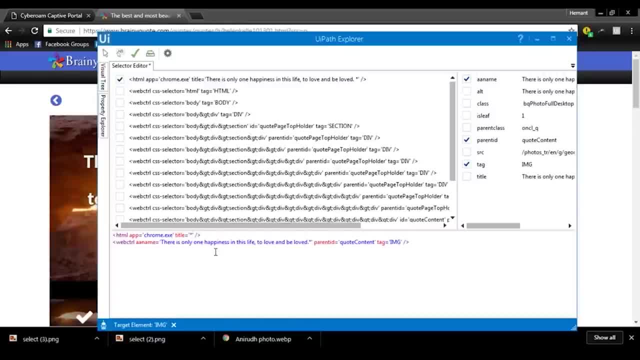 I come back to the title section of my selectors. I say star space, hyphen space, brainy code, which basically means anything can be before this particular you know word which is brainy code. I'm not bothered with that, but the title should always end with hyphen brainy. quote. 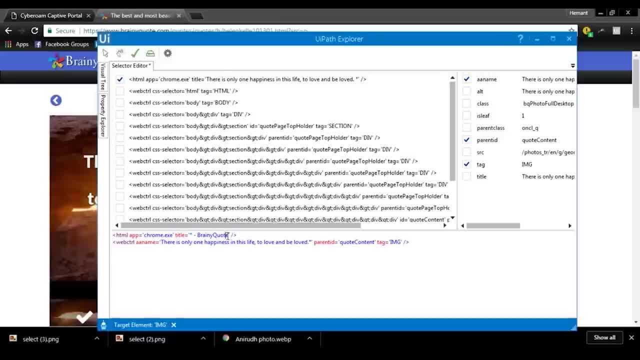 All right, So this is the significance of star over here. This is what the star is basically me. It's a placeholder for anything. It could be anything that is being filled before hyphen brainy code: Right, So now how it is identifying this particular element. is so any HTML page? 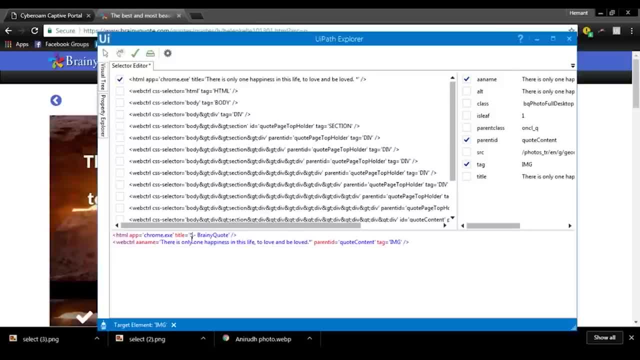 which is, you know, in the Chrome browser. if it's having a title in which in the end it's hyphen brainy quote, go inside that particular tab right. So this seems to be fixed. We can also further strengthen it by giving the URL as well. 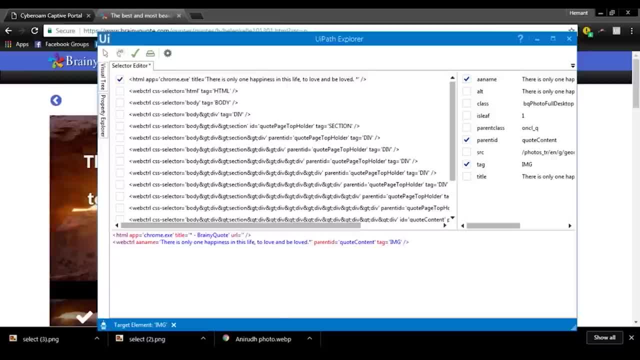 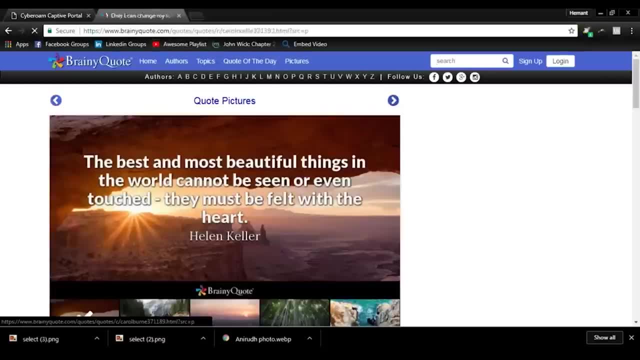 So I can give the URL for that tab as well over here. And if you see the URL, guys, so let's try to see if the URL is changing or not. So if I hit next, I can see that this particular section of the URL is always same. 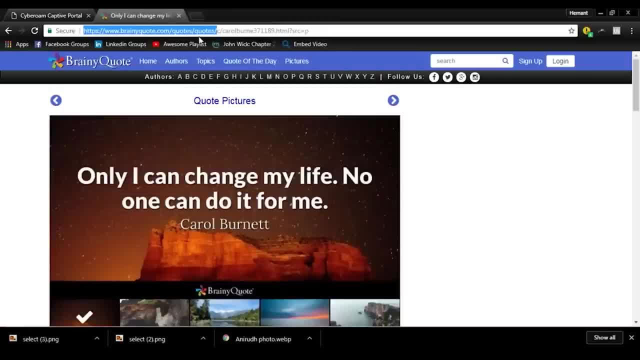 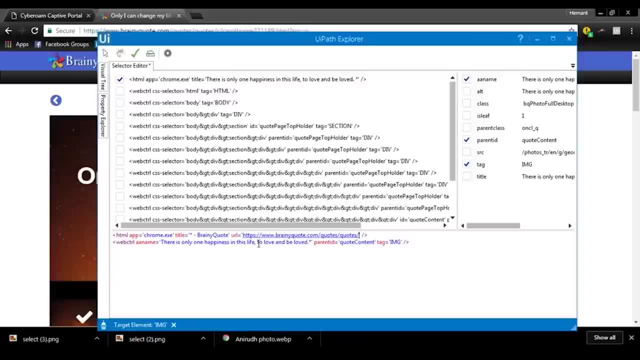 and this particular section of the URL is changing. All right, So what I do is I'll copy this section of the URL, go to my tool and specify the URL here and say star after that, which basically means anything which is before star is this: 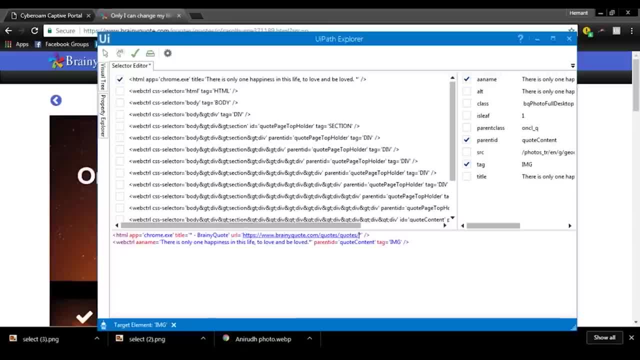 and anything after this could be anything right. anything after this is, I'm not bothered about it, but the start of the URL should be something like this: And if it is like this, go inside that particular tab. right now you can validate whether it is still. 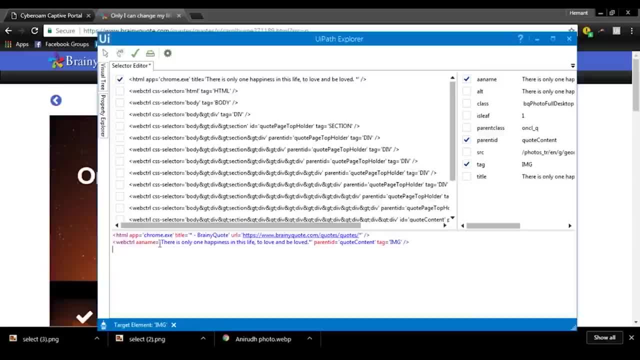 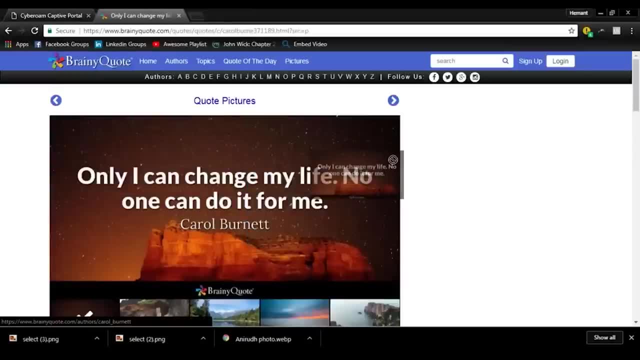 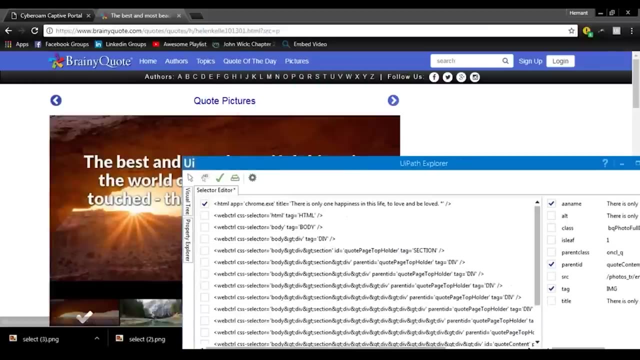 able to identify the element on the screen by hitting this validate selector. So right now, as you can see, the image has changed right. So let me hit back right And let me see if this is the same image that my selector is pointing to. 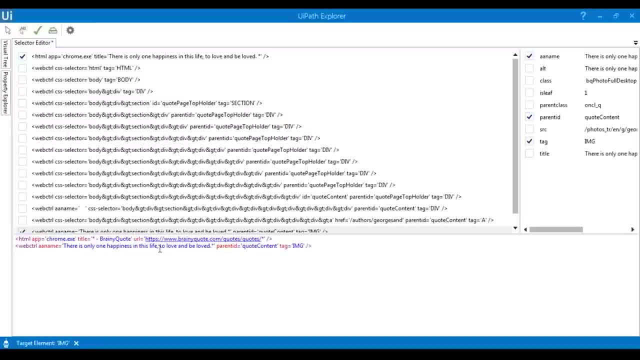 All right. So I feel this is the same. So it says there is only one happiness in this life, and it's also said there's only one happiness in this life. So right now, if I hit on validate selector, it should tell me whether it is pointing to this image or not. 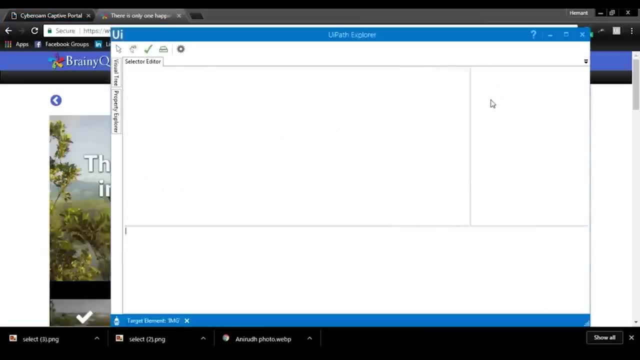 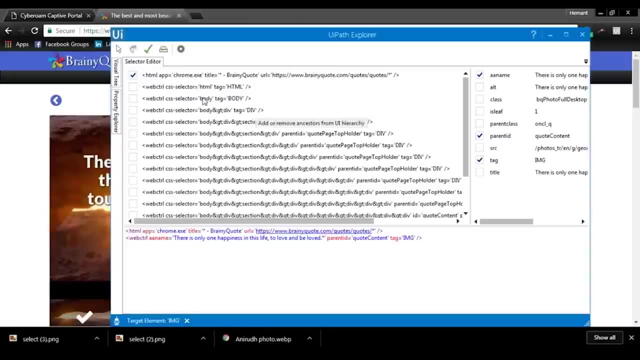 So I'll hit validate selector. It was pointing to this particular image, All right, but the moment I click on next and if I go to my ui path selector now and I say validate selector, it will say it cannot find the UI object for the selector that I have provided. 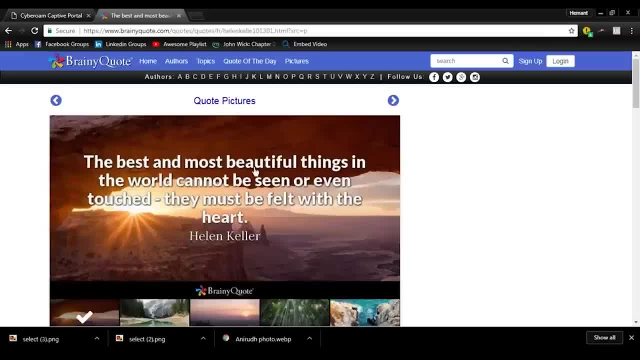 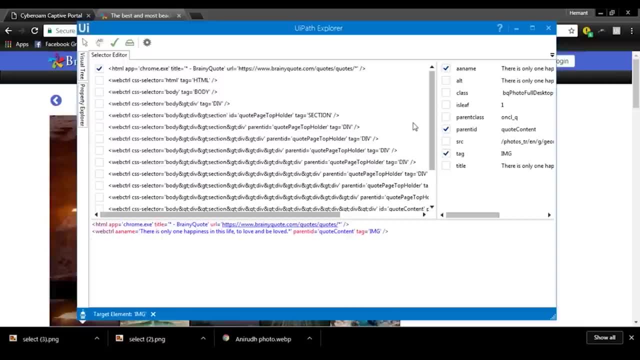 because now this particular image of this browser is having a different name, right, So we have to fix that. So again, since the name is changed, changing at every page, I would not want the name property to be included when I'm trying to identify an element. 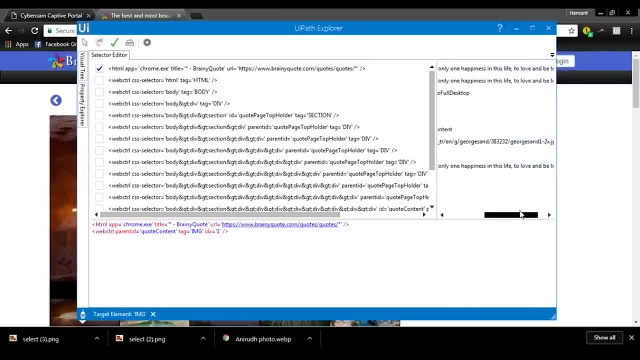 right. So let us see what. all other things I have over here which I can actually use, the title I cannot use because again, the title will change the source. I cannot use because the source of the image will change as the image changes. 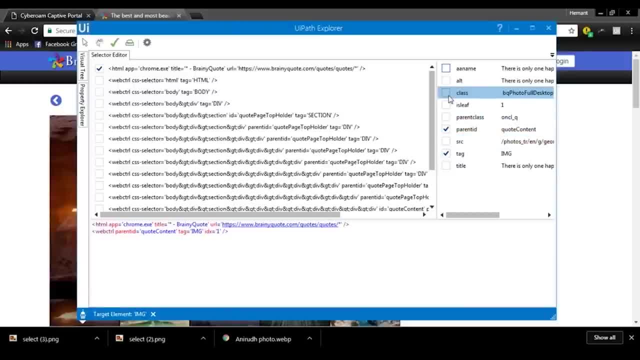 right, The parent class. I can consider the class of the file. I can consider the class of the image container. This is basically the class of the image container which is there, and I think this will do good If you select this as our selector. 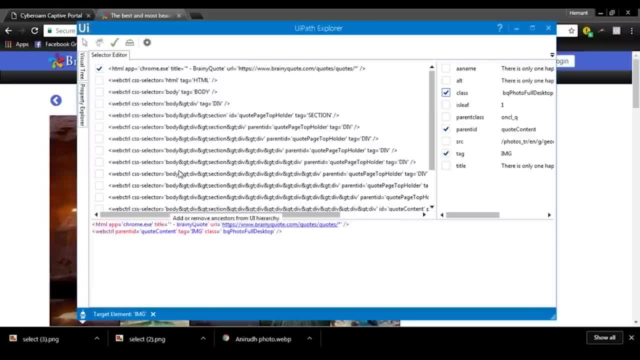 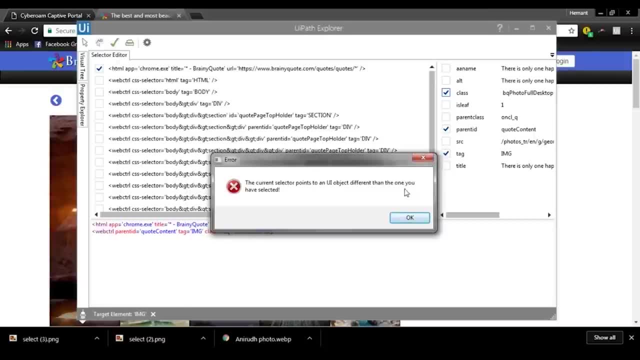 I think it will be able to recognize that element on the screen. Let's see if we are right or wrong. So we will click on valid selector. the current selector points when you are different than when you have selected. that is fine, because previously we had some other image. 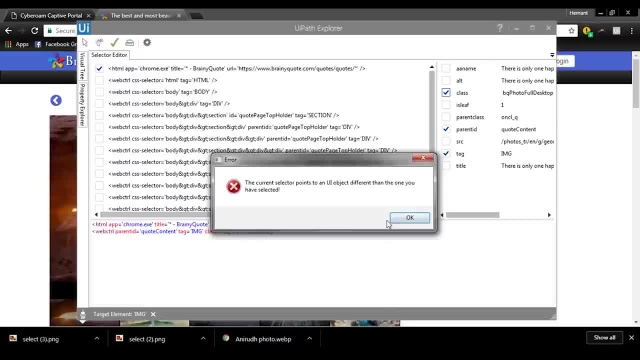 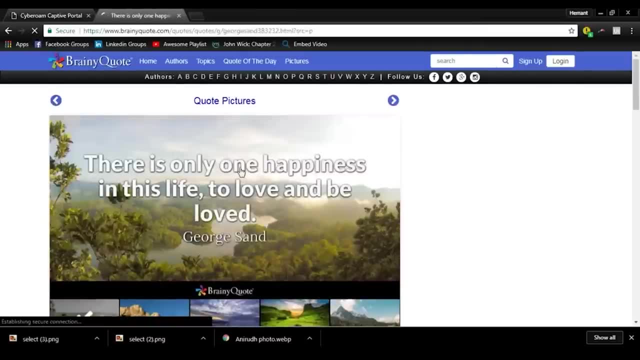 So this warning basically tells us that now we are being pointed to some other element, right? So to fix this, what we can do is we can go back to the image That was Originally the source for the selector that we have modified and click on validate selector. 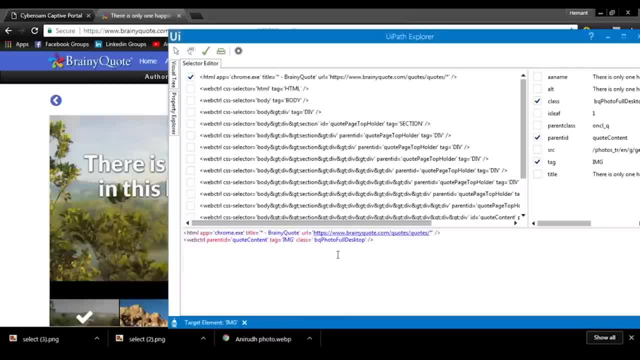 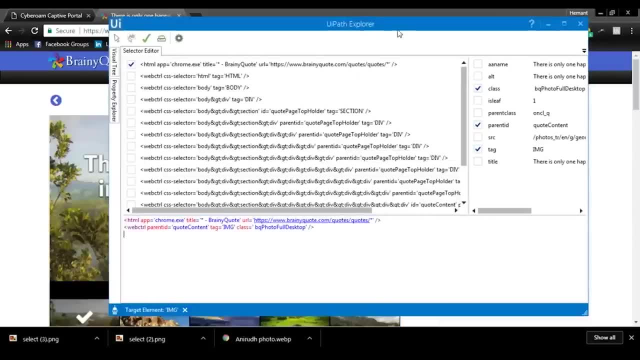 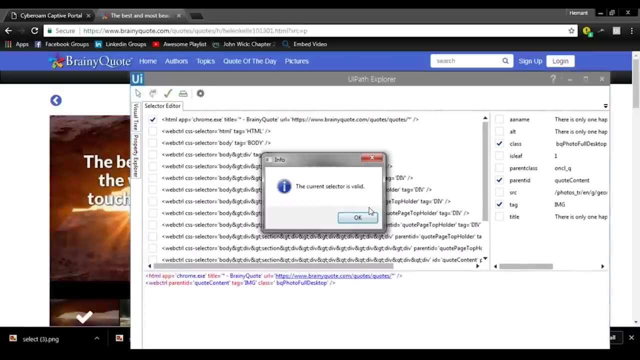 So, yes, the current selector is valid for this selector as well, which we have just modified. So I think this selector should work, or is working, right. If I click on next now and again validate the selector, It is: the current selector is valid. 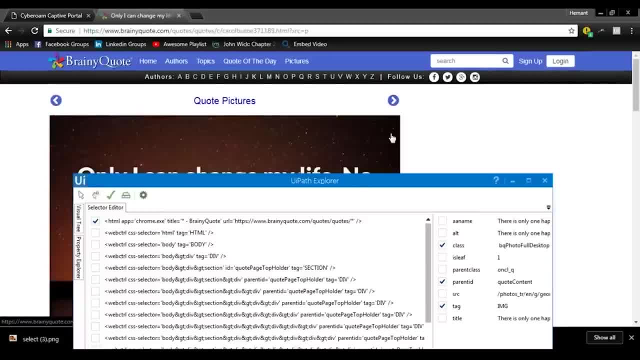 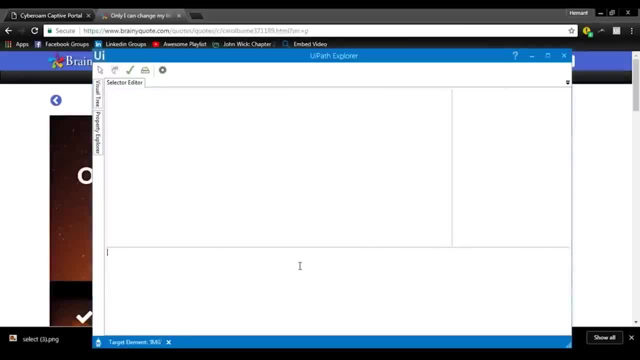 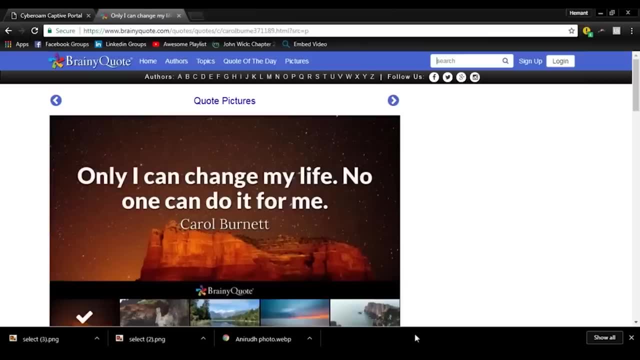 If I again change the webpage and I click on valid Selector, it again can validate the image container that I have templatized using selectors. So this code now is usable. I can copy this code and I can close this and I can paste it over here. 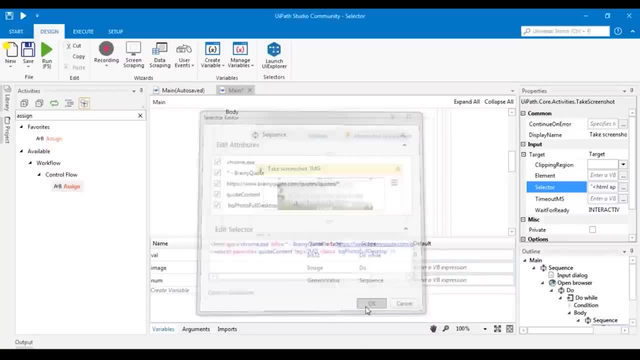 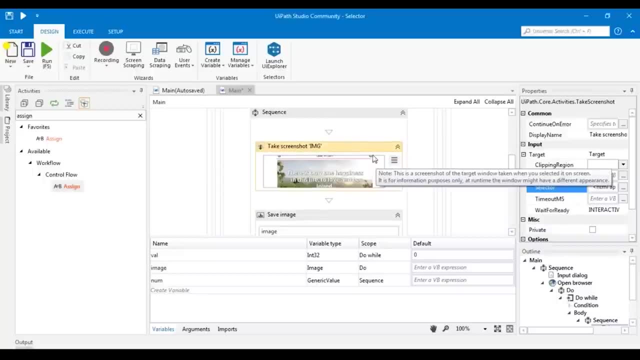 So now my image container has been templatized, So on every page it can identify the main image right. So this is why selectors are important guys. Now again, if I scroll down a bit and I see the click button, this again can be a problem. 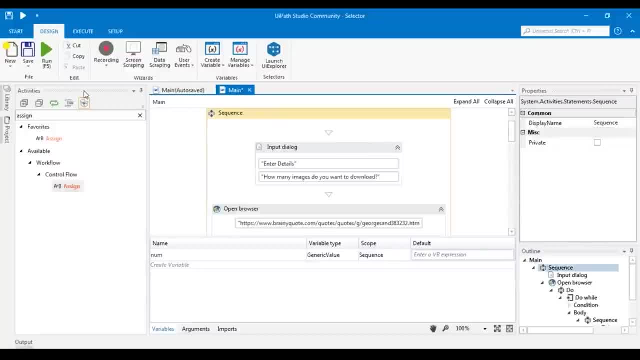 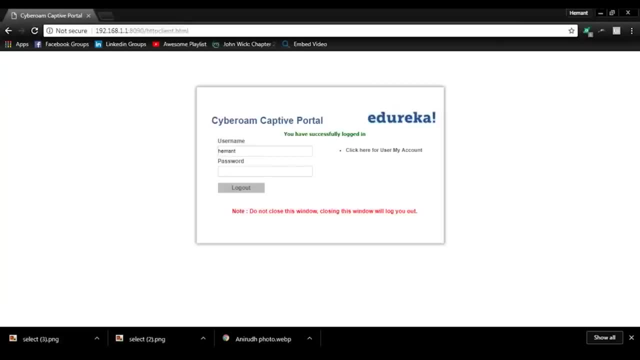 But for now let's try to run it and see if we need to implement selectors in button as well. So we'll hit run it. Let us close this tab and let's enter say I want around four images and I'll hit Okay. 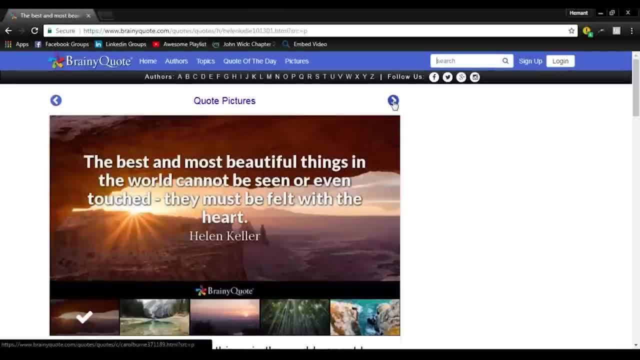 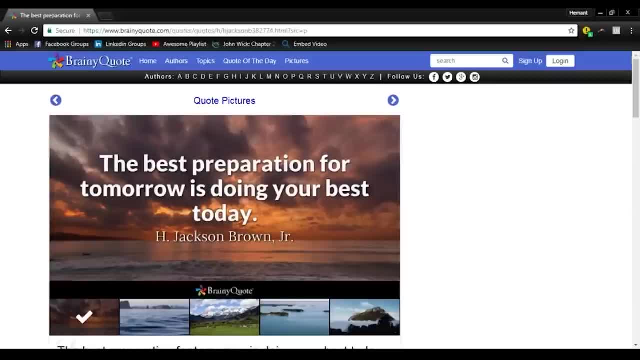 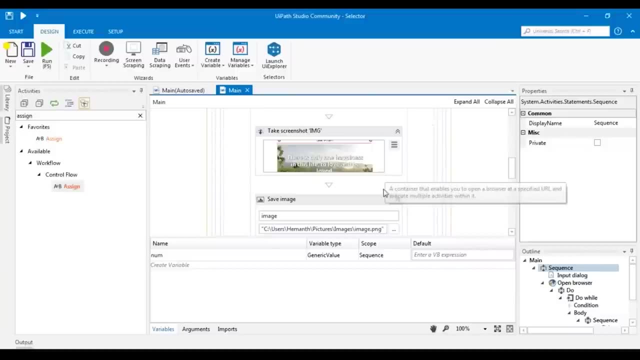 Okay, So my Chrome browser has opened, So now it has seen my website and, as you can see, it is waiting for three seconds and then clicking on next, Taking the screenshot and alright, so our automation works. So now the one thing that I forgot to do over here is change the image. 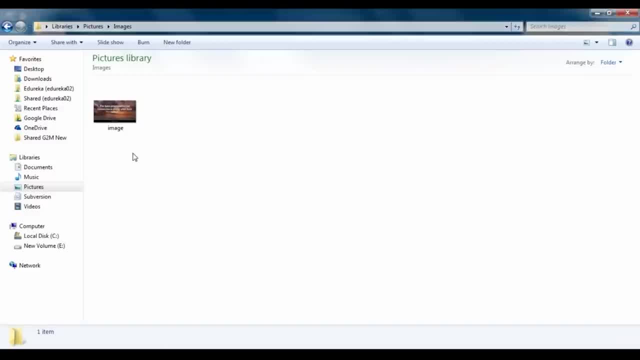 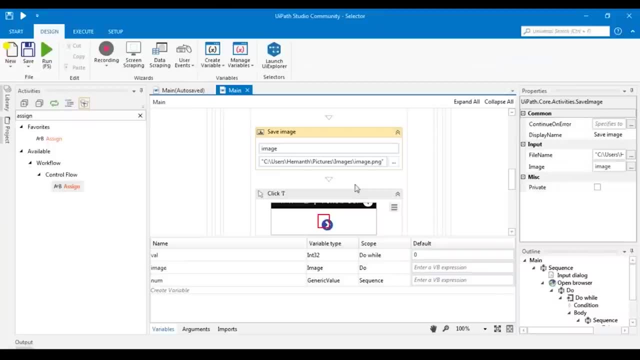 So if I were to see how many images I have in my folder, it's only going to show one, because every time that it is trying to save an image, it is saving it by the same name, that is, image dot PNG. So I have to fix this now. 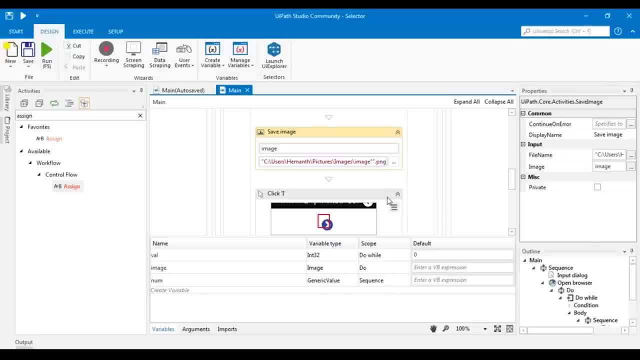 So to fix this I can do a simple math problem which is basically something like this: So I can add a number in front of the image name. So what number? so what better than our own variable, that is Val. right, So that Val has to be converted to string if I'm trying to store it as a name. 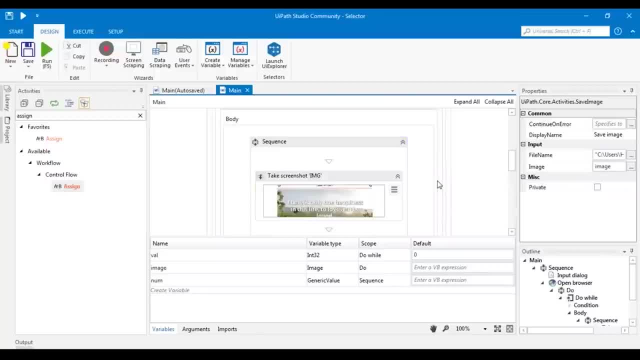 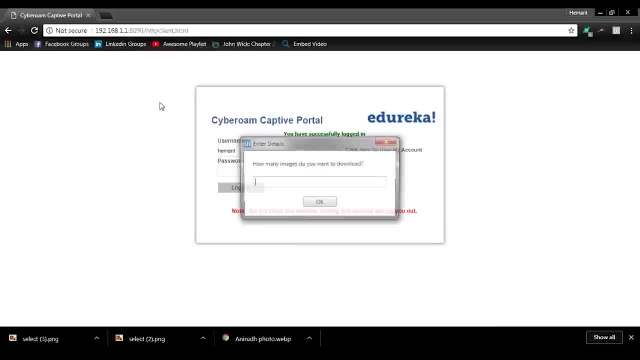 So let's enter the Val variable here and now save the project. All right, So now let's try to run our program and see if you're getting different files. So it'll ask me the number of images that I want to download. I'll say around five images. 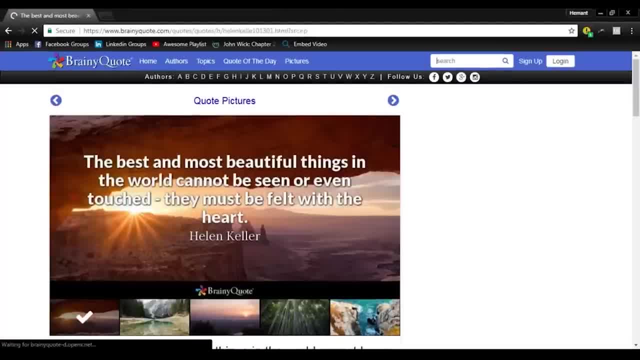 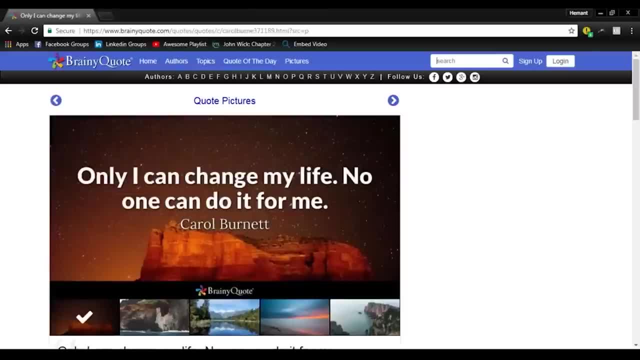 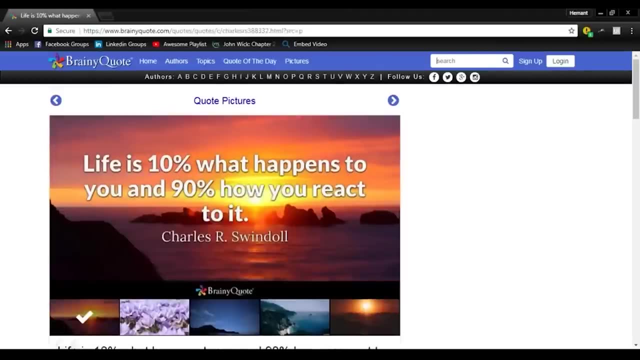 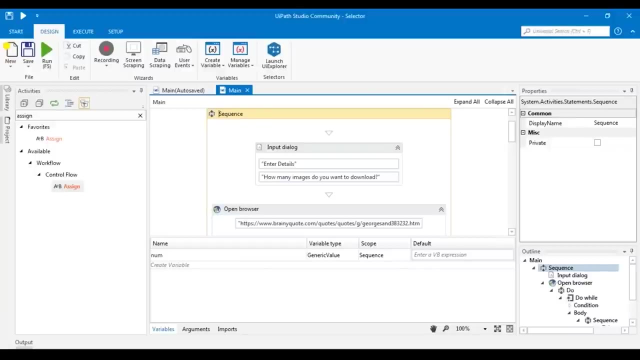 Let's head. Okay, We'll go to the page. It has saved one file, Save the second file, Save the third file, The fourth file and then the last image. after this And once it has finished the automation, it will close the browser and return to my uiPath studio. 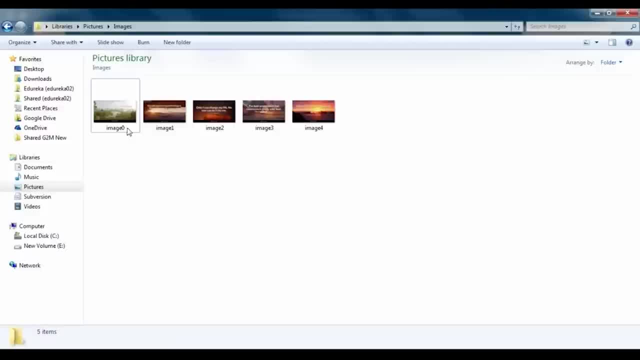 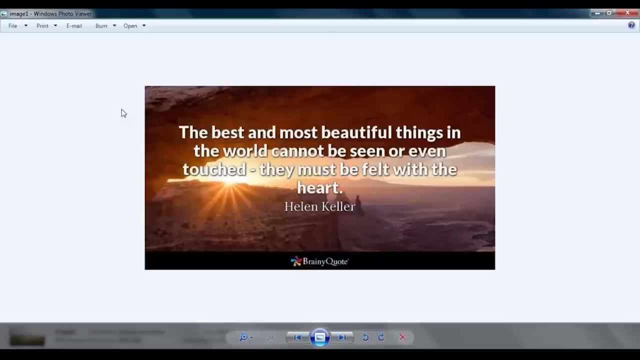 So let's see if I have five images in a folder now. So yeah, Yes, I have around five images. So let's check if these images, I can see these images. So yes, I have successfully automated this particular website by templatizing the objects. 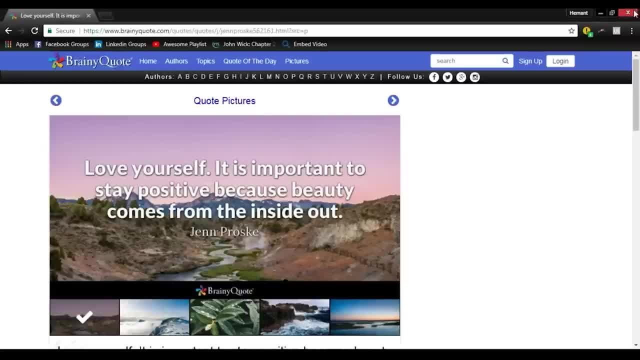 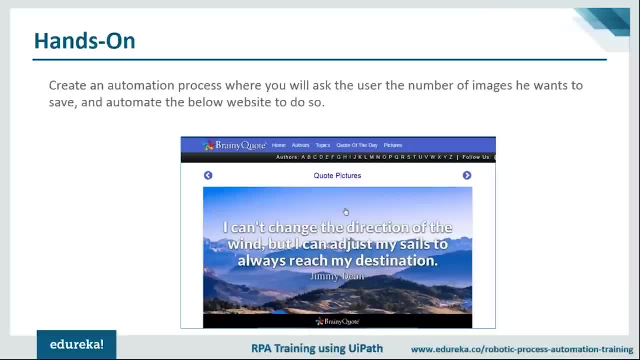 that are there on this particular website using selectors, right? So with that guys, congratulations on your first project on selectors. So I hope you guys have learned something new and basically this opens a lot of scope In terms of automation. You can just think about automating something and using selectors. 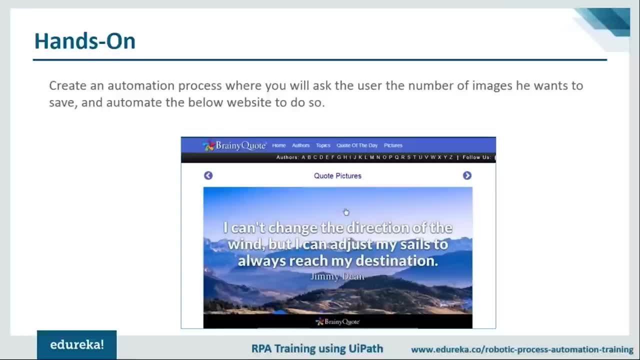 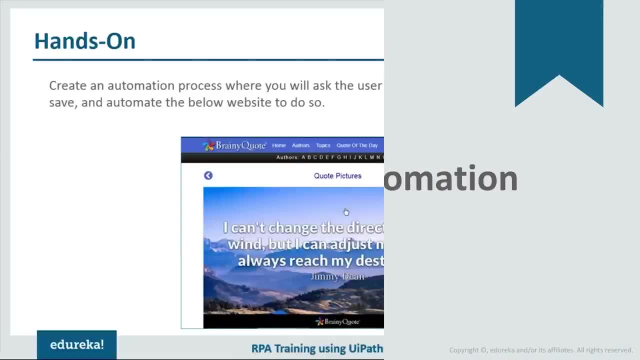 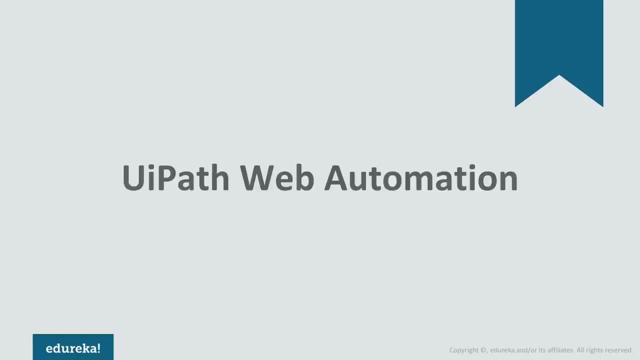 You can do that. It is a very powerful thing that uiPath has given to us and we can basically implement it on any website that is there on the web. What do you understand by the term web automation? Well, as you know, businesses and applications today are widely structured on web-based systems. 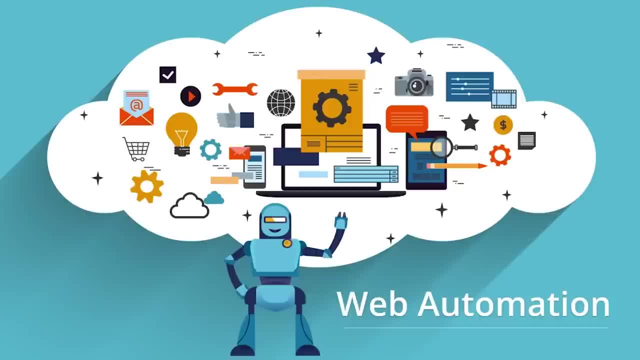 Informations that populate these systems are dense and demand extensive processing, So many companies in this large scale industry have repetitive tasks which are tedious and take a lot of time. So this is where web automation comes in: from form filling to screen scraping, data extraction. 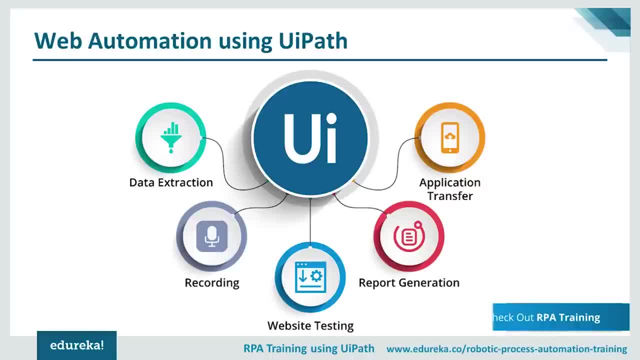 and transfer between the applications, or web testing or any periodical report generation, right. So now that you know why do we need web automation, or not only at an individual level, but also at a higher level, Let's look into how can we use web automation in the uiPath tool, right. 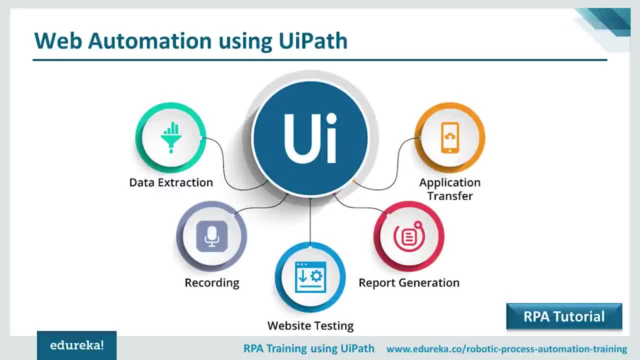 So let's move on. So, basically, let me just brief you a little bit about the uiPath web automation tool. Well, uiPath web automation uses a built-in recorder that can read and enact web-based activities. It identifies web elements by their attributes. 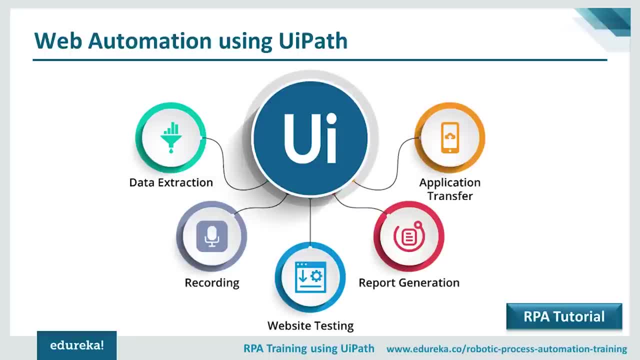 and accurately manipulates them while keeping up the website changes, right. So if you open any website- let's just say Flipkart or Amazon or anything, right- And if you want to collect data from those websites, you just have to click on the web automation tool. 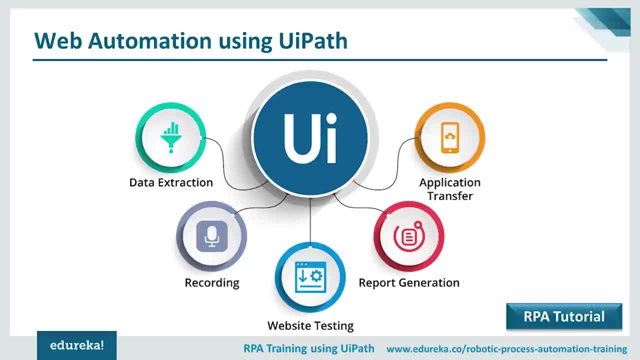 and then you can start recording. it works with any website, no matter how complex, and can remotely deploy on various machines in the network. So any IT professional can also go forward and use the web automation tool. by automation web-based workflows with uiPath, you save time, money and energy. 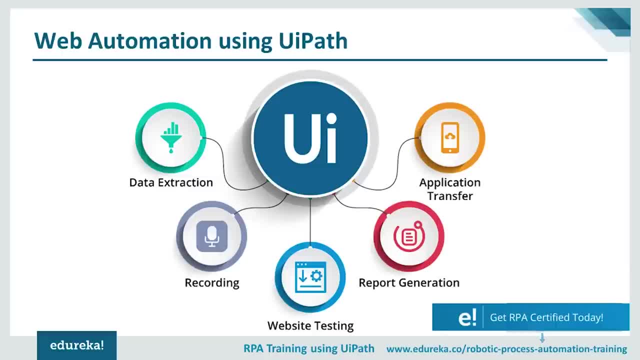 So you need not spend lots of money in paying employees whose sole work is either put data entry task or perform any basic task. So you just have to ensure that the accuracy requirements are always met and your web automation is done. So now that you know how the web automation works, 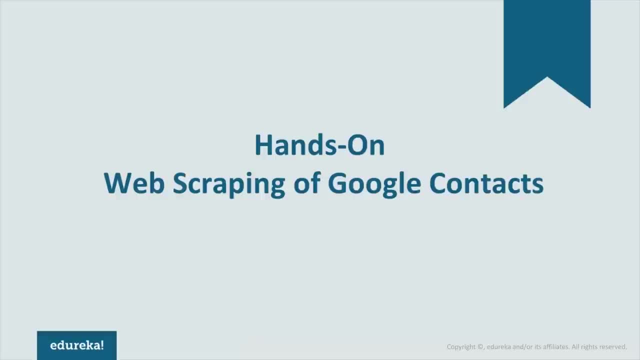 and why do we need web automation? Let me just move on to the hands-on part and show you how we can use web automation. So web scraping can be used for various types of web page formats. right, So you can use web scraping for HTML formats. 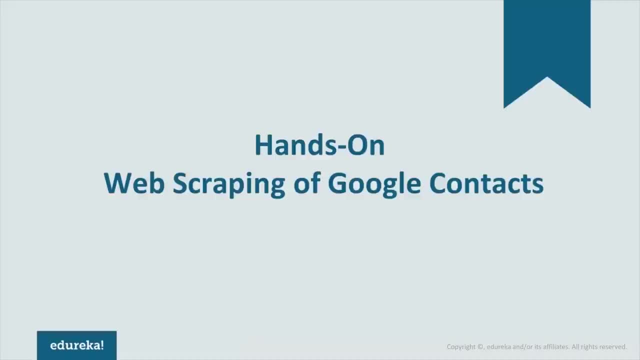 or JSON formats or any other types of formats. So now let's just look into What demo where we'll be running web scraping using HTML web page formats, right? So what we're going to do is we're going to extract data from Google contacts. 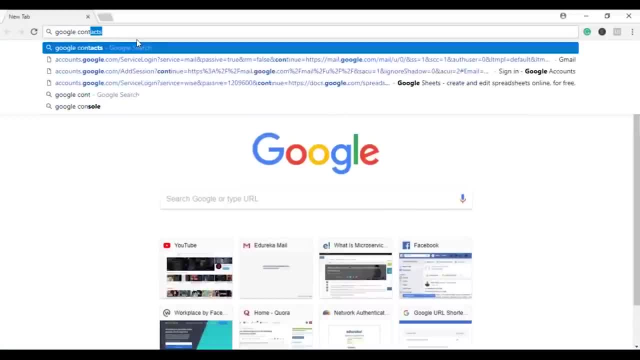 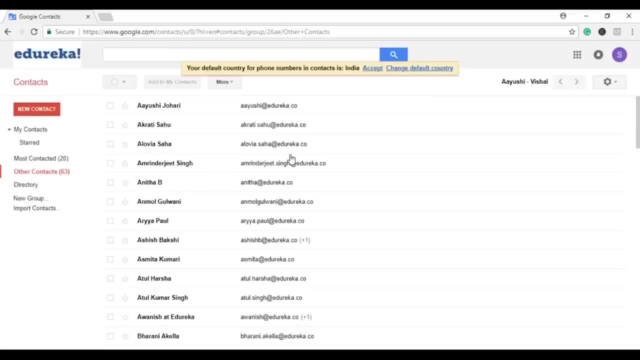 So let me just open Google contacts now. So, as you can see, these are my Google contacts, right? So what we're going to do is we're going to scrape the data out of this page and then store it in our file. So now let's open our uiPath and then scrape the data for this page. 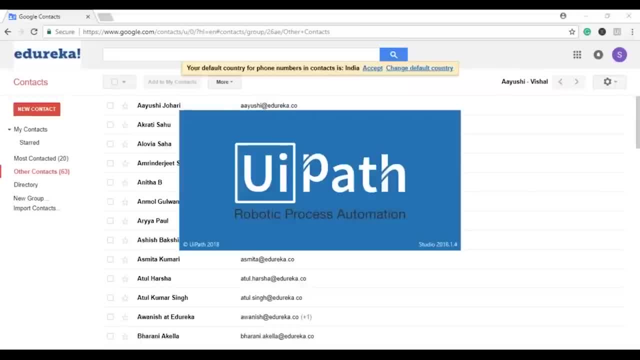 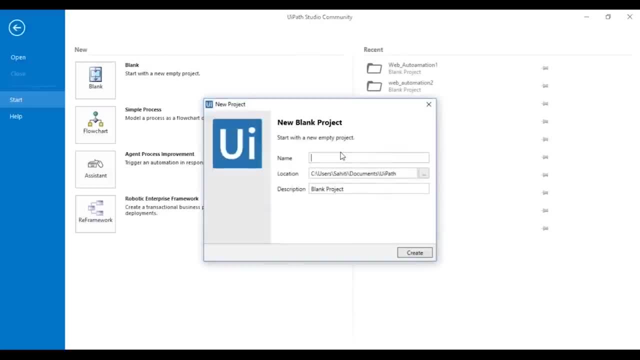 So let me just open the uiPath. So let's just open a blank project. So let me just click here. So let's just say I choose the name of the project as demo project one, and then I'll click on create. So once I click on create, this creates a simple project for me. 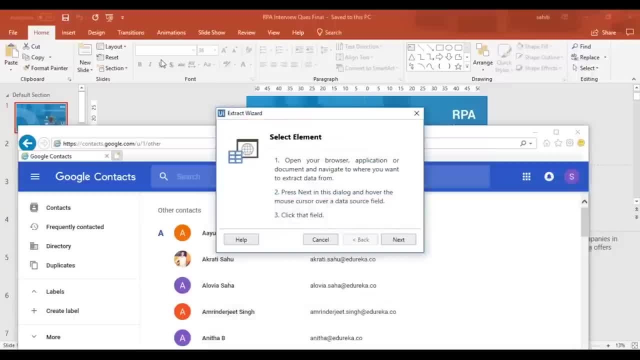 Now let's go to the design tab and click on data scraping, So this will pull up a wizard in which you have to click on next. Basically, this wizard is to select the element Right, So let's just click on next and then hover the mouse over the elements. 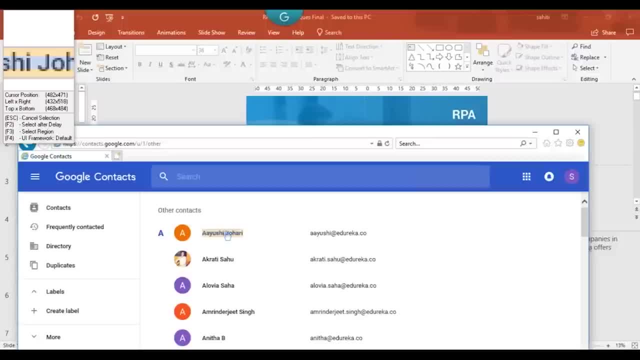 We want to choose. So suppose I want to choose this name. I'll select this name and then click on next. once I click on next, the second name I'm going to choose is to tell the uiPath to create a pattern. So it will basically create a pattern in which all the names would be stored automatically. 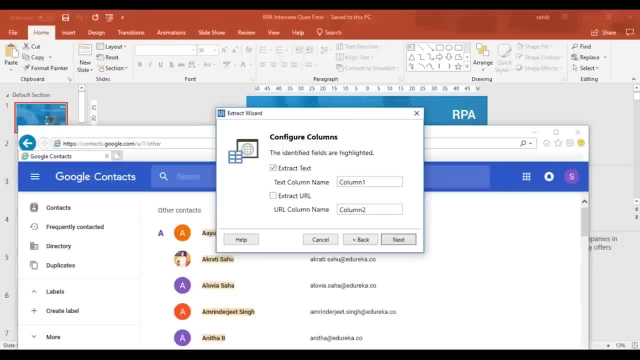 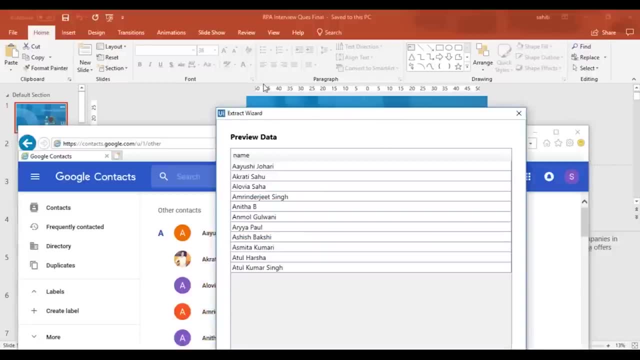 Now. after that, you can put your column names in the wizard right. So let's just say I put the column name as name and then click on next. Once it is done, you can see that it has extracted in this sheet. So now, if you want to extract any other information, 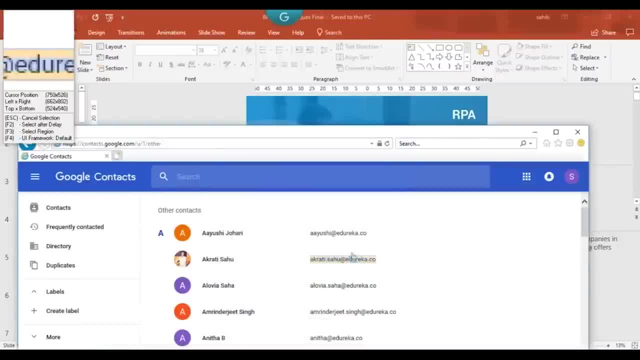 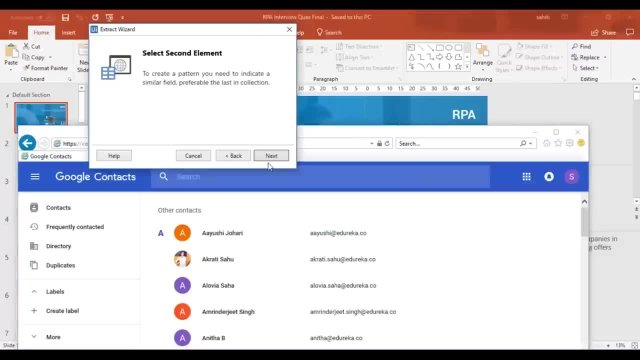 then you have to click on extract correlated data. So once you click on that you can extract information here. Let's just say, I can extract information about email, So let me just click over there and then click on next so you can extract any correlated data. 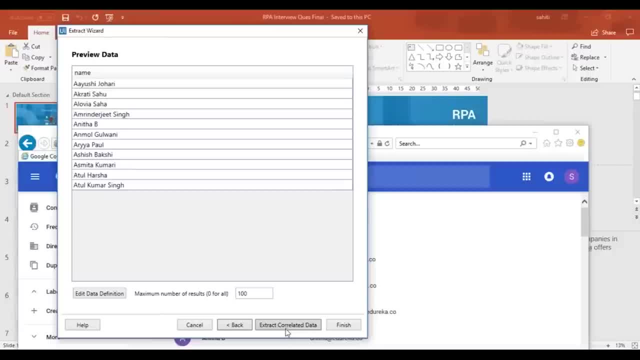 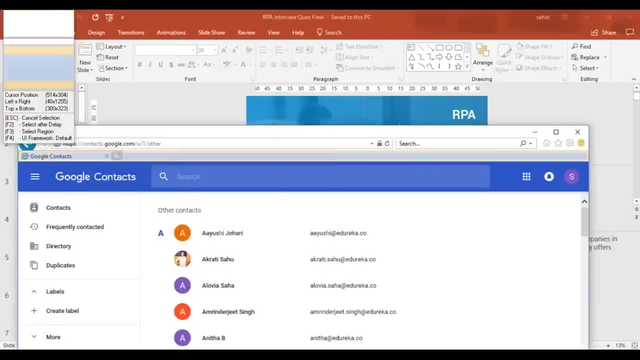 by clicking on this radio button as extract correlated data, right? So let me just click on extract correlated data and then show you so I can choose the email ID and then click on next. once I click on next, I again have to choose the email ID so that I create a pattern. 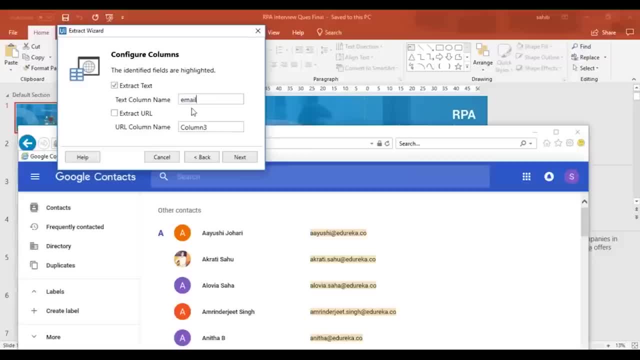 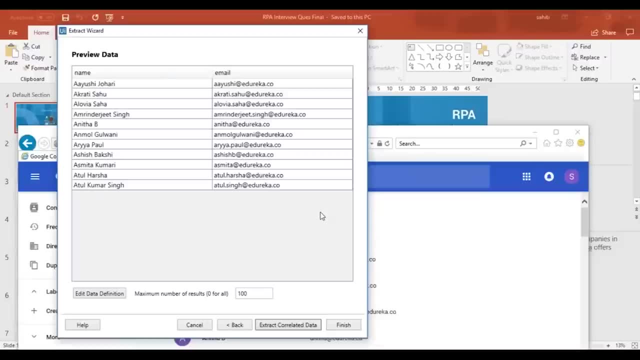 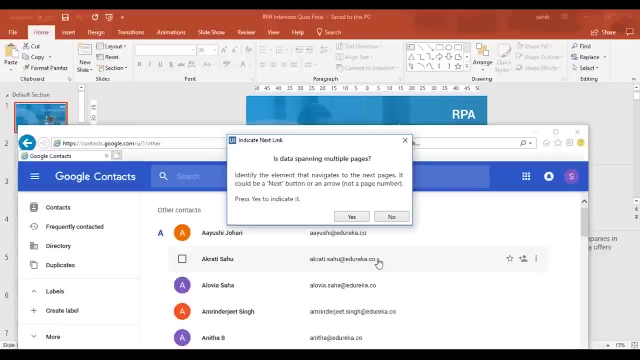 So let's just say I renamed this column as email and then click on next. So once this is done, uiPath automatically detects the page is in the HTML table format. after you're done with that, You just have to click on finish. So once you click on finish, you get a dialog box. 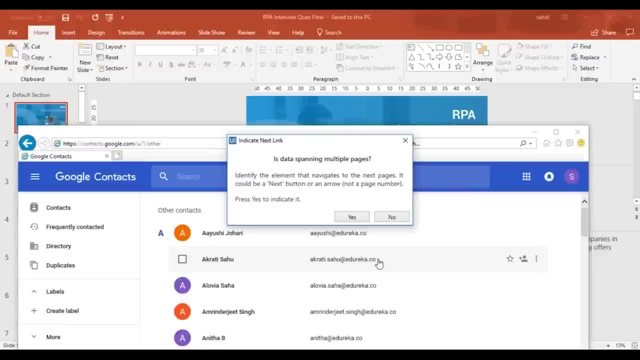 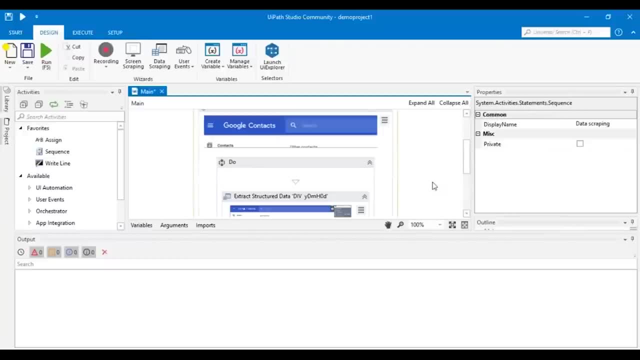 which says: if you want to span the data among multiple pages, since we do not have the data among various pages, let's just click on no. Once this is done, it gets you back to the uiPath tool, where you can see that all your steps are stored, right. 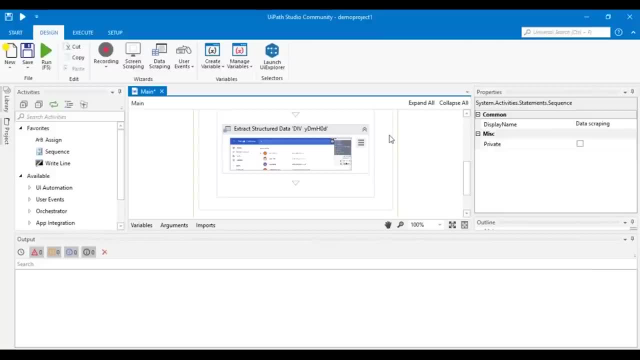 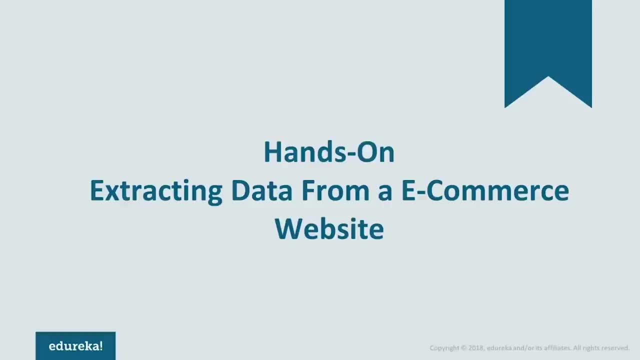 It automatically records all the activities that you perform when you want to extract data from websites. So, guys, this was a short demo on web scraping. now, moving forward, Let's look at a large scale, where we are going to create an application which will read the email. 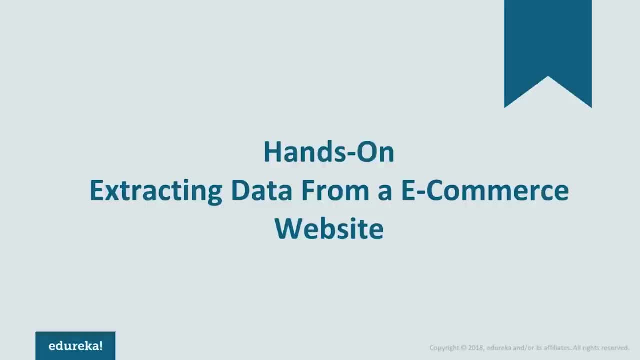 It's going to take the subject line of the email and it's going to put inside a search query of an e-commerce website and then extract the results from the scraping technique and put it inside a CSV format file, right? So after this is done, 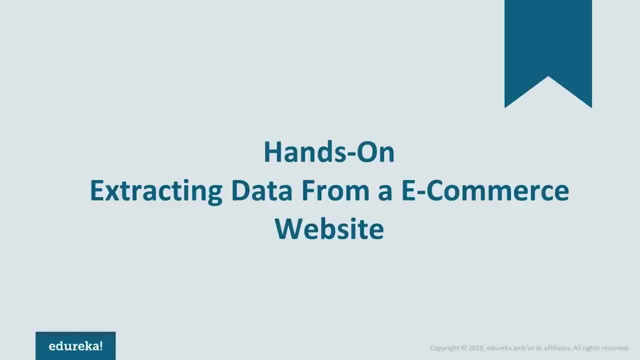 what it is also going to do is that it's going to save the file and send it back to me via email. So if we have to automate this task, let's just see how we're going to do it. So let me just go back to start and then choose a blank project. 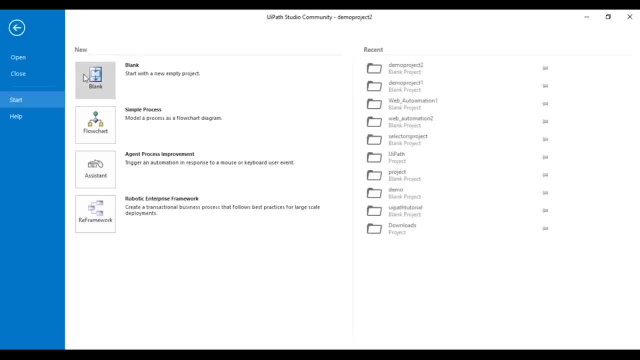 which would basically create a simple blank project for me, right? So let me just click on it and then give the project name. Let's just say I give the project name as demo project and then click on create. So once it is done, 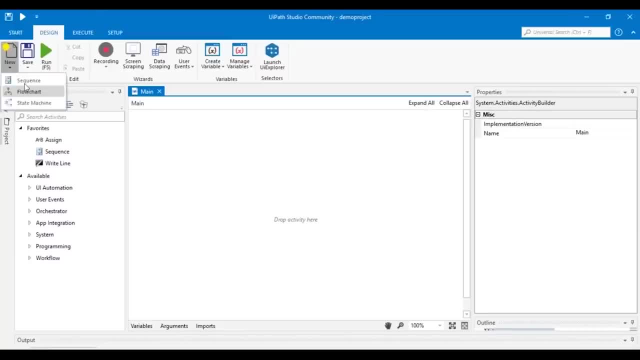 let me just go to the design tab and choose to create a new sequence. So let me just create a new sequence and let me just name the new sequence as demo, and then I'll click on create. So I've got this new sequence here. 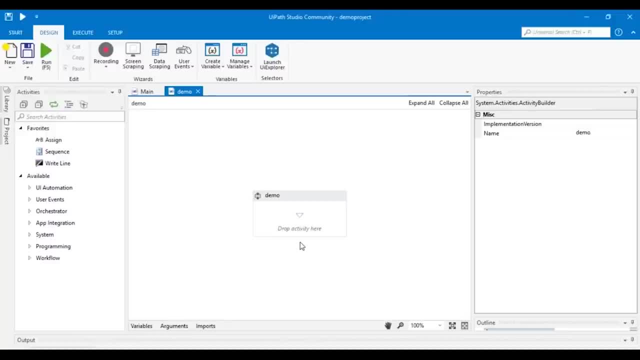 So, according to the problem statement, now what I want to do is I want to get an email with the subject line of my requested data. Right So? but before that, let me just give you a short demo on how can we scrape data from websites. 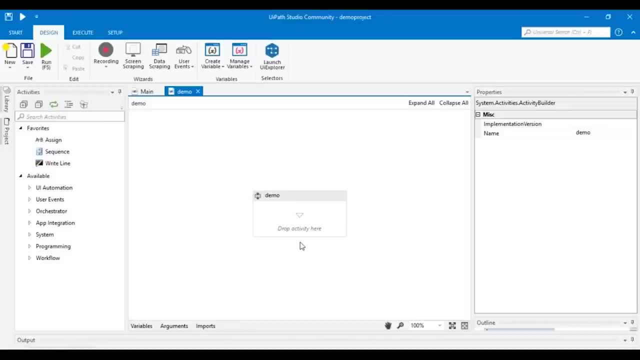 So it's pretty interesting to learn with the first time how the data is extracted from the website. Just imagine if you can extract all the data that you have on online websites. So for that you have to click on the data scraping, So to extract data from websites. 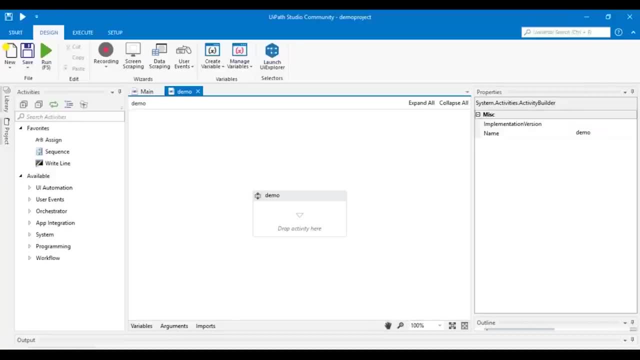 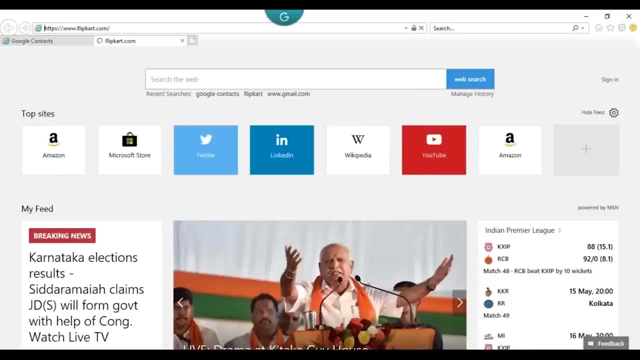 you have to click on the data scraping tool, But before that you should open your website. So let's just open that website, Let me just click on it. Let's just say I open flipkartcom and then search for it. So let's say I want to search for any phone. 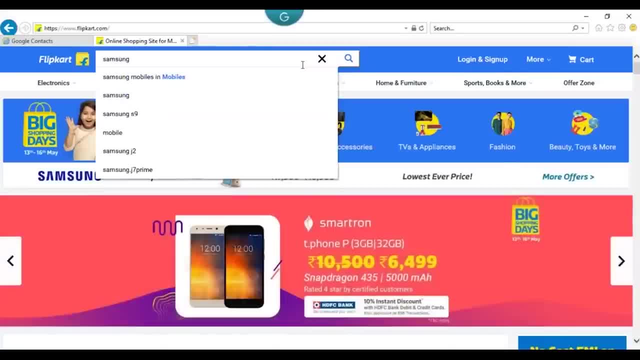 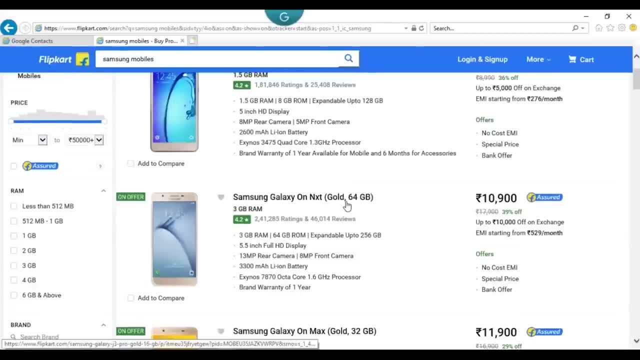 Let's just say I go for the Samsung brand, So I'll type in Samsung So you can see that flipkart shows you a list of all the Samsung phone. So if I want to scrape the data of all the Samsung phones, how do I do it? 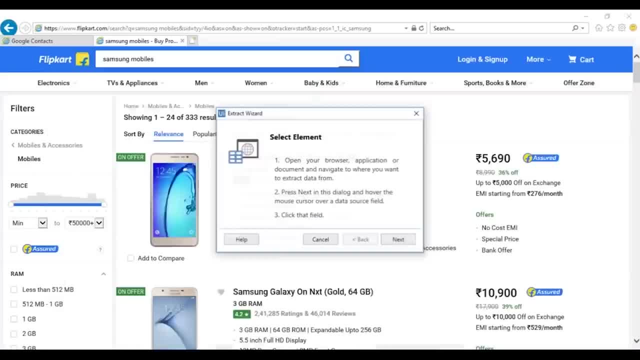 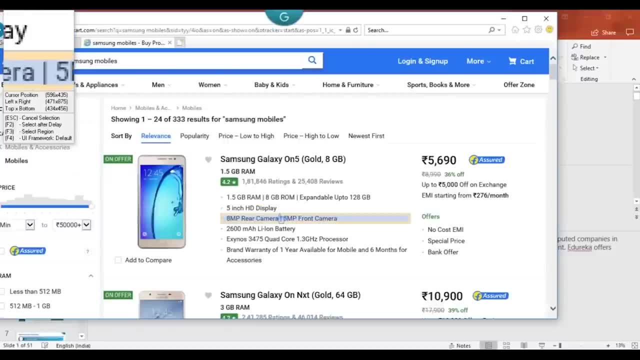 So for that you have to go back to the tool, You have to click on data scraping and then, as I told you before, you have to click on next on this wizard. Once it is done, you have to choose the parameter you want to retrieve right. 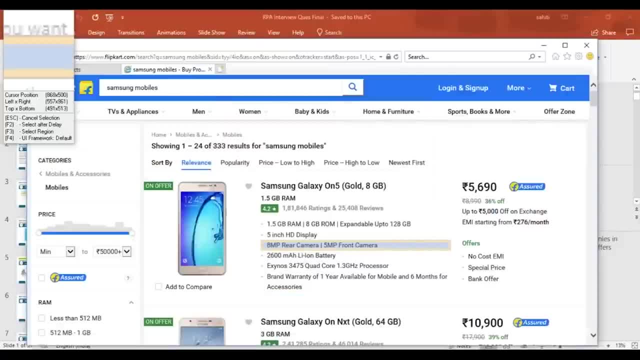 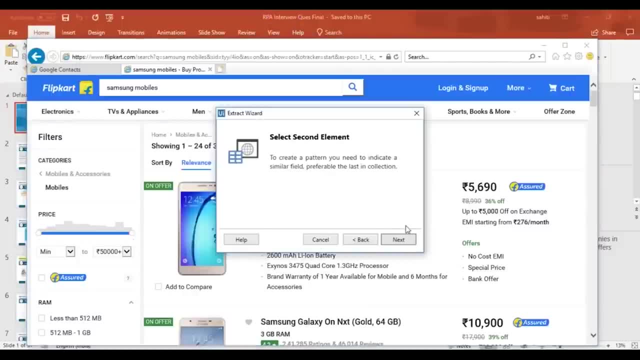 So let's just say I want to retrieve the name, right? So I'll click on next and then I'll hover the mouse over here. Once it is done, I'll again click on next to make a pattern so that we can indicate a similar field in the collection, right? 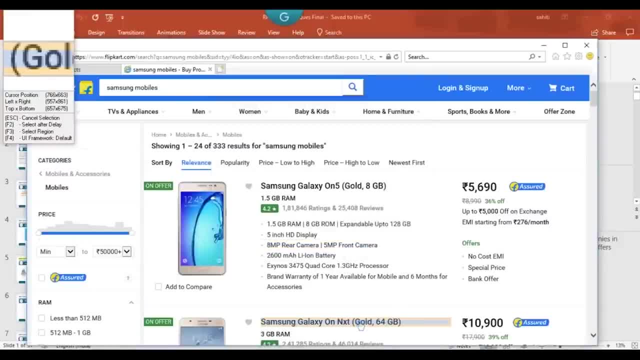 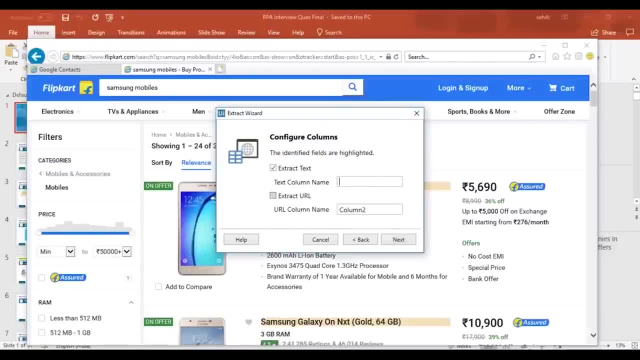 So let me just click on next, Let me just choose the second option. So this would basically identify all the phones starting with Samsung, right? So let's just say I mentioned the column name as mobile name and then I can also extract the URL by checking on this button. 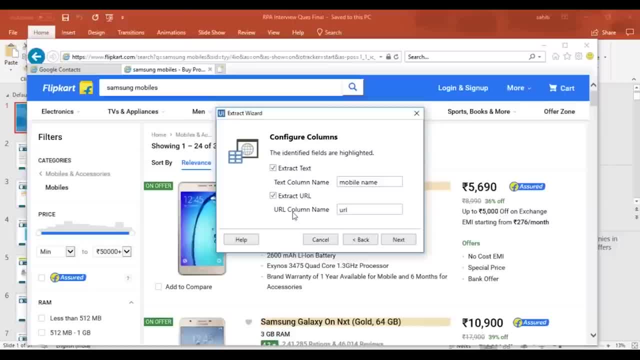 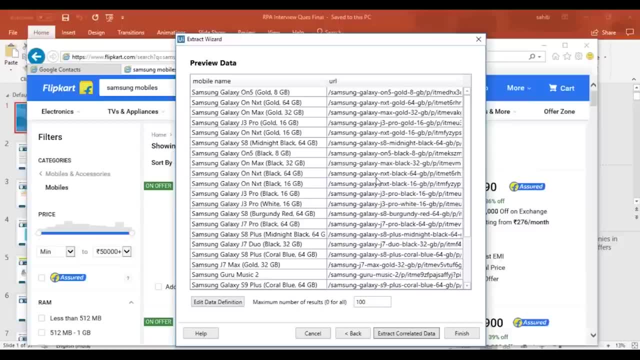 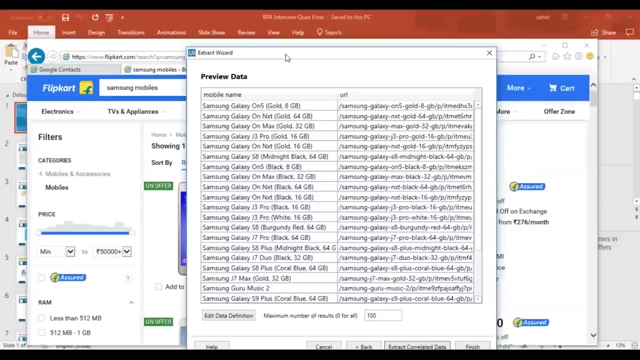 and then I renamed the column as URL and then I'll click on next. So, as you can see, it has extracted all the data of mobile names and the URLs. So if you want to extract any correlated data to retrieve information such as the rating or your mobile configuration or the price, 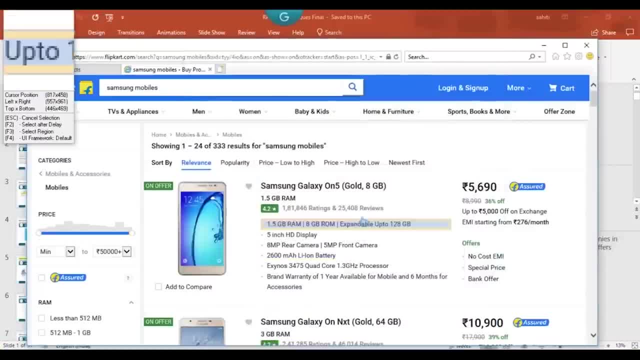 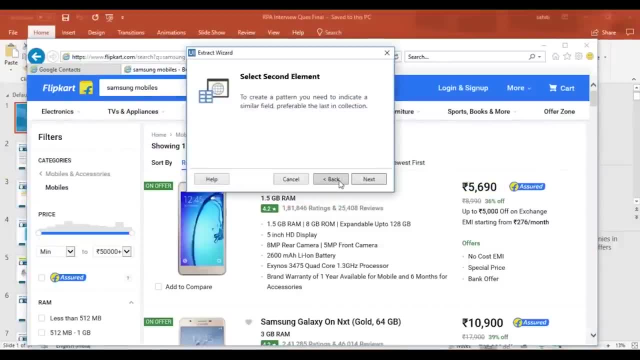 you have to click on this extract correlated data option and you just have to hover the mouse over there. So if I want to extract the prices, I'll hover the mouse over here and then I'll click on next. Once I click on next, as I told you, it will start creating a pattern. 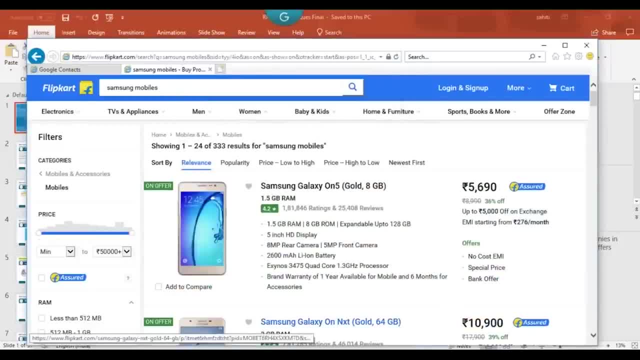 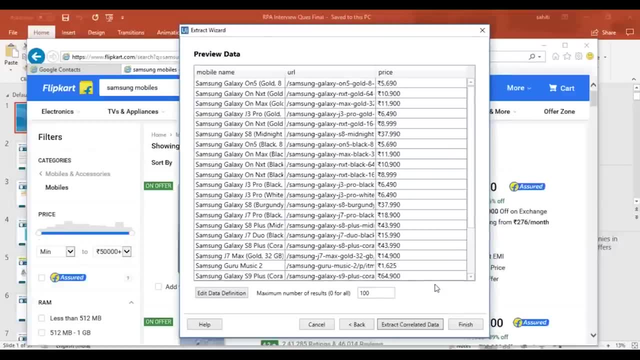 So let me just click on next and then choose the second option. So let's just again rename this column as price and then click on next. Now you can see that the mobile name URL and the price has been extracted. after this is done, You just have to click on finish. 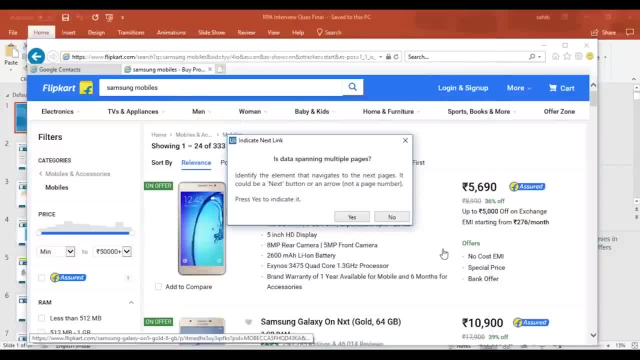 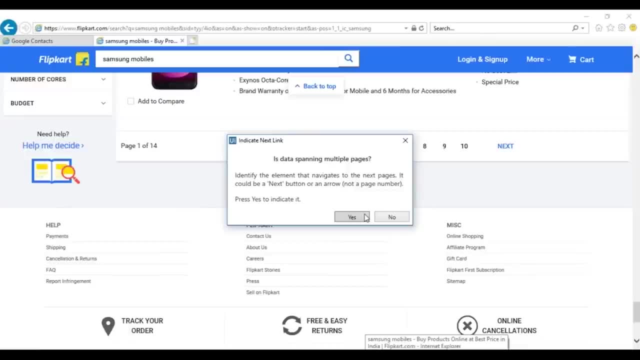 Once you click on finish, you get this dialog box which says: if you want to span the data among multiple pages, that is, if you want to scrape the data among multiple pages. So once you click on yes, you have to choose the next option, because that is the option that we use to span various pages. 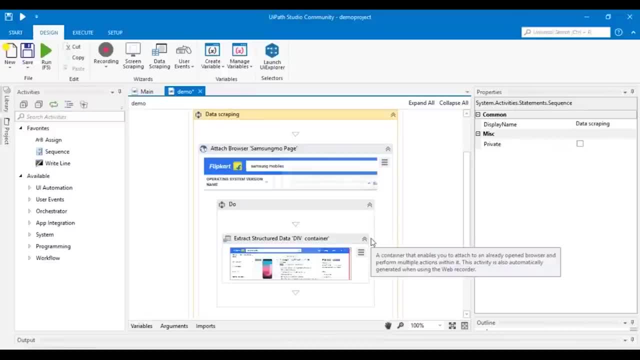 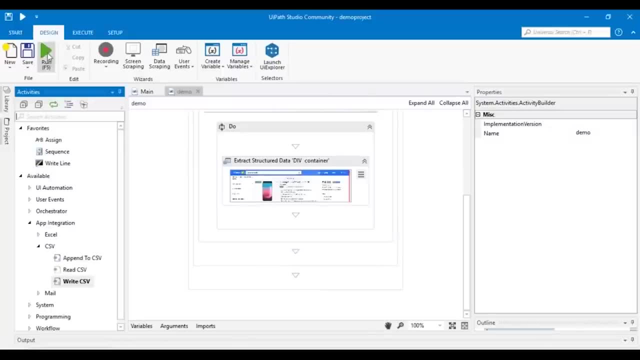 So you just choose this option and that ends your data scraping. So that's: our data scraping tool is ready now. So now let's just run this program and then check. So when you run this program, you can see that it is spanning around various pages. 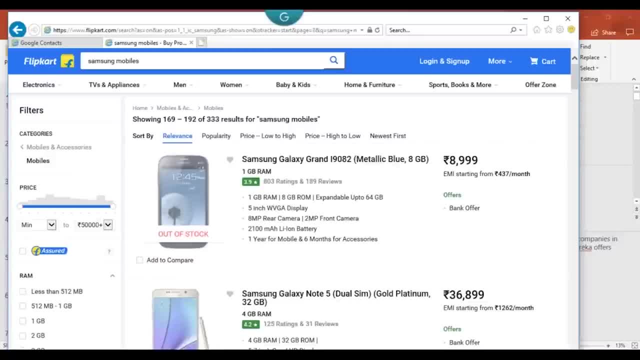 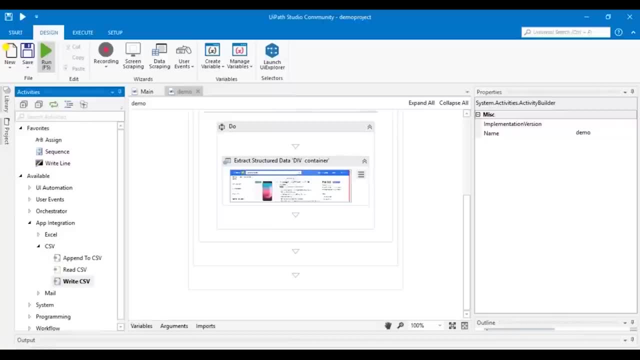 for Samsung mobiles right. Once it is done, it gets back to the UiPath tool. Now, if you want to save the scraped data in a CSV file, what we have to do is we have to go to the activities pane and then search for an activity called write CSV. 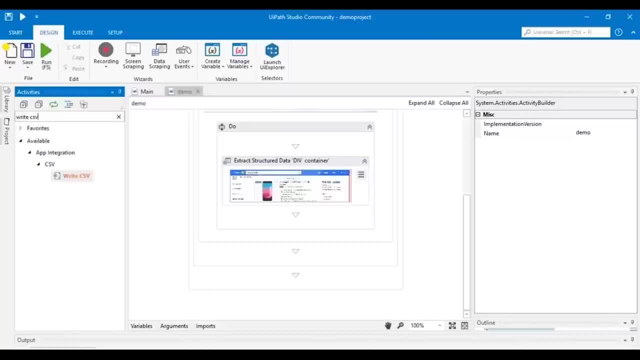 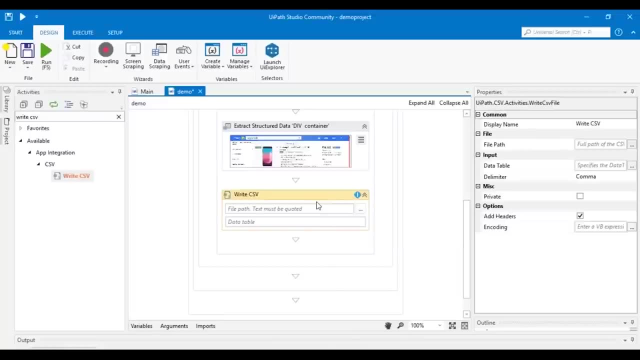 All right. so let's just search for write CSV and then drag and drop it here. Now, in the write CSV file, you have to mention the path name where you want to save your CSV file. So let's just select this path name. 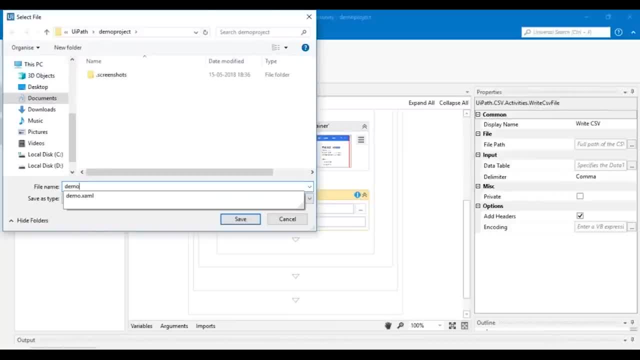 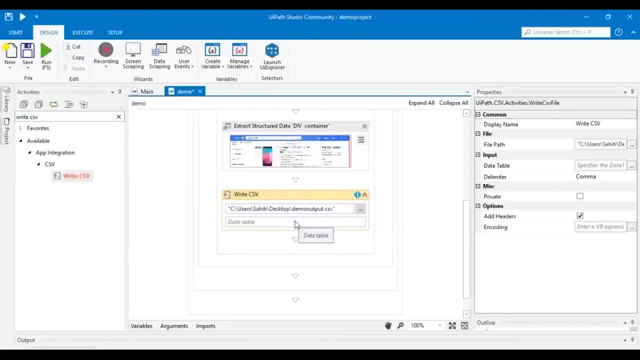 Let's just say, I mentioned the file name as demo output, and then I put it on my desktop and then I save this file. Once it is done, you have to mention the data table also. So let's just say, this data table is stored. 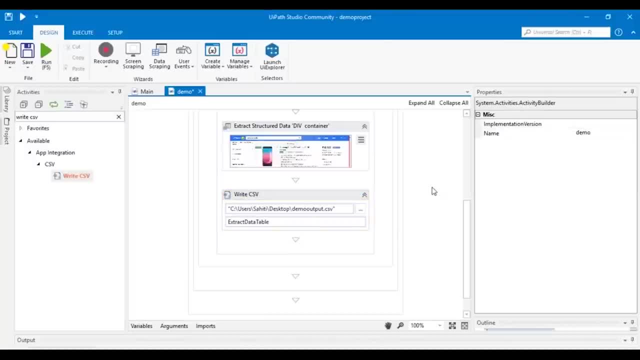 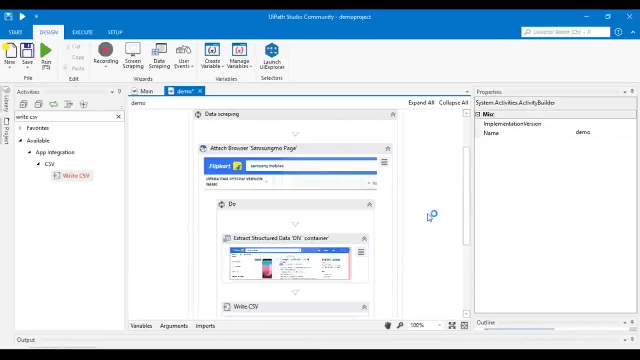 and extract data table. All right. So if you have to check if there are any errors in your sequence or not, you have to click out of the sequence and check for the exclamation marks. You can clearly see that there are no exclamation marks. 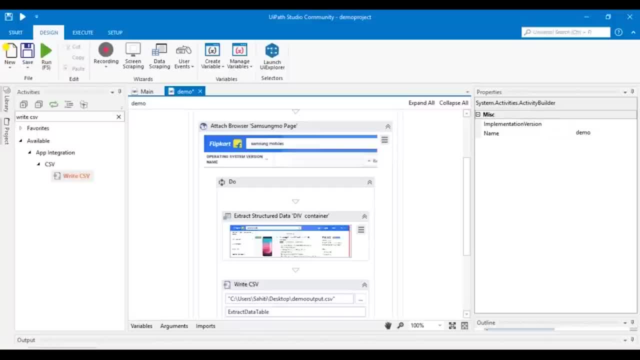 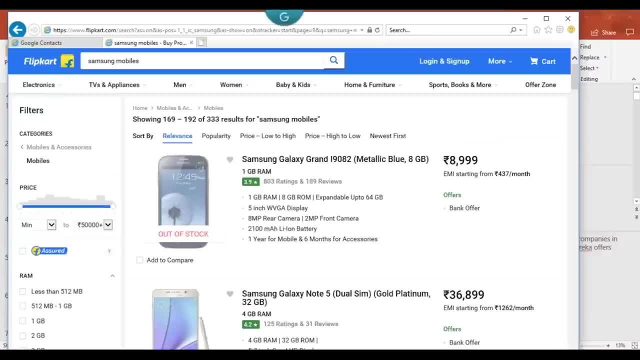 So that means our program is error free. So now let's just save this file and then let's just run this file. So when you run this file, you can see that the data is extracted from the websites and it has reached the last page. 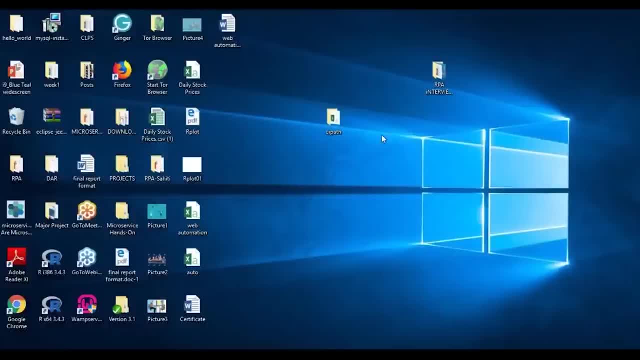 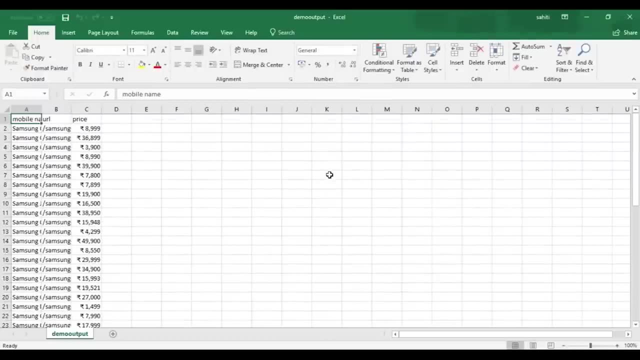 Once it is done, let's just go to this file now, where we have saved the files, and now you can see that all the information regarding Samsung phones is saved: The mobile name, the URL and the price, Not only these three parameters. 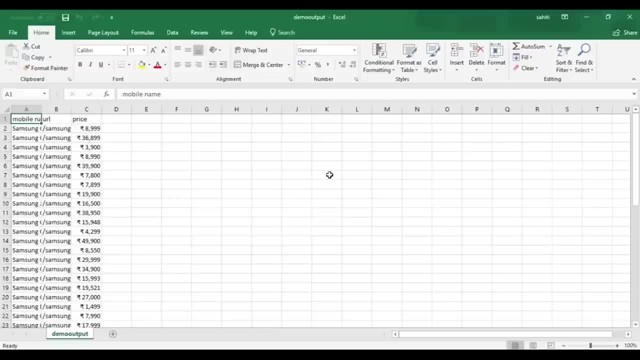 you can also extract n number of parameters, such as the rating, the mobile configurations, the EMI- if EMI is available or not- any such parameters right. So this has no boundations of how much data you can extract. So, guys, that was a short demo on data scraping. 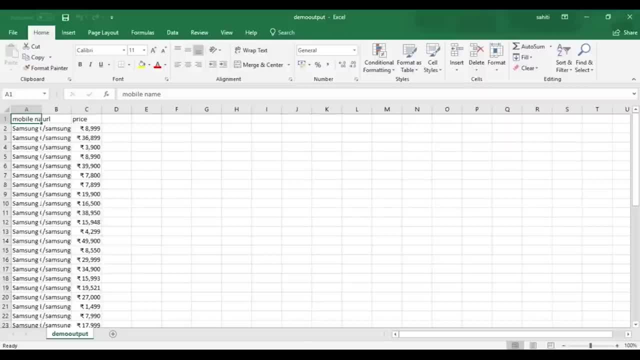 But our problem statement was to do custom search right. So I basically want to take data out from my email and then take the particular search subject line of my email and then search it in the specified e-commerce websites. So if I just say I choose Flipkart, 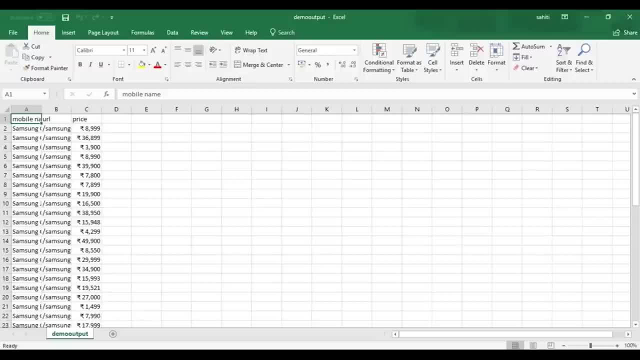 then I want my automation tool to take the subject line of my email and then search it in the Flipkart. So if I just say LG TVs, then I want the automation tool to search LG TVs in Flipkart. I basically wanted to do the custom search. 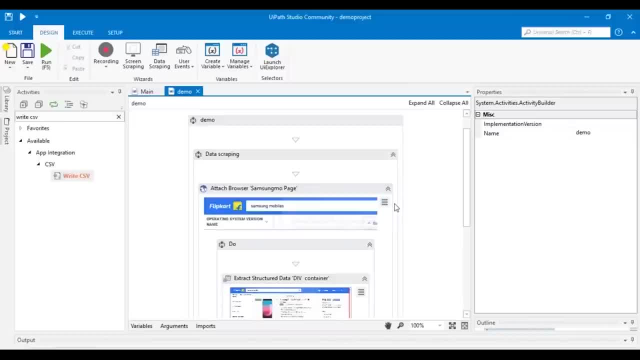 But to understand how that's happening we have to first get an email right. So for that in the activities pane we have to search for the IMAP activity. So let me just search and then drag the get IMAP mail messages. 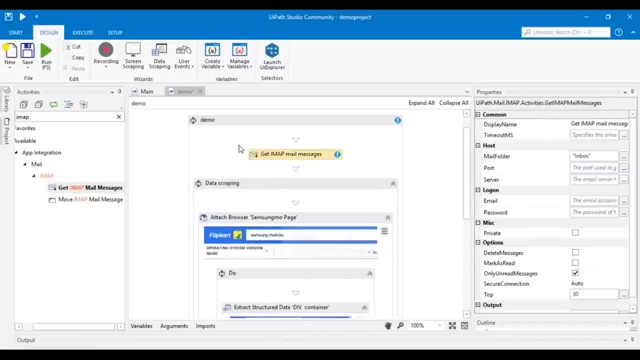 So this activity would basically enable you to get an incoming mail right. So once I drag and drop this activity, I have to configure this activity. So for that you just have to click on this activity and go on the right side of the section. 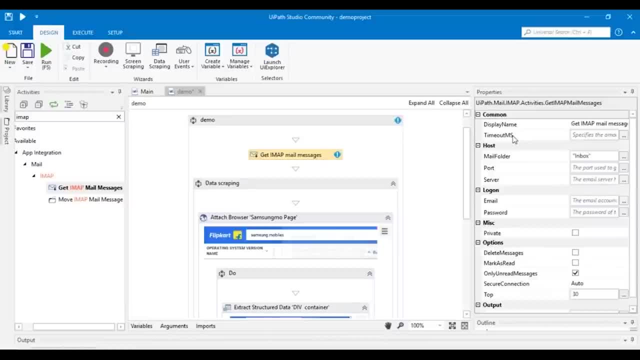 that is the property section where you mention all the properties right. So on the properties pane you can mention the email ID, the password, the port number, If you want the messages to be deleted or you want to read only the unread messages. 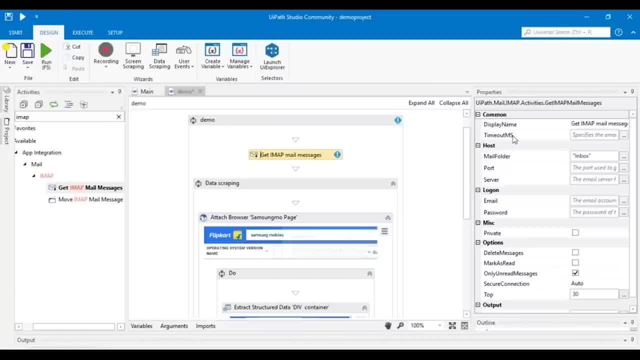 any such options, right? So for the IMAP protocol, the port number is 993.. So let's just mention the port number as 993 here, And then we have to give the server name. So before giving any server name, let me just tell you that any text 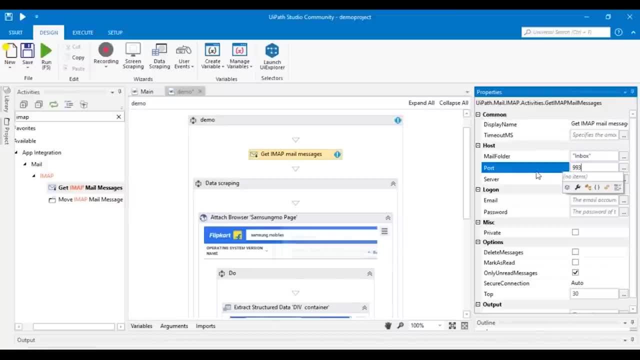 that you include in the UiPath tool must be in double quotes, all right? So let's just include the server name in double quotes. So let's say so. let's just include imapgmailcom. So this is the address of your server now. 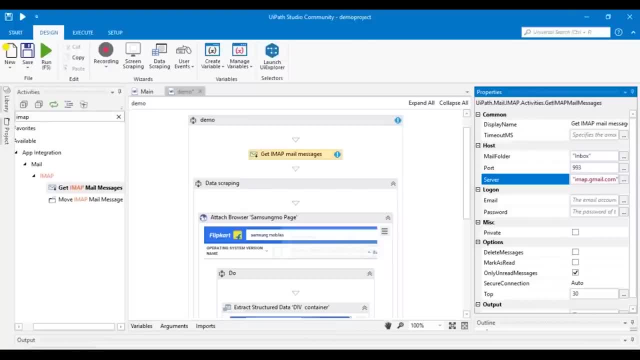 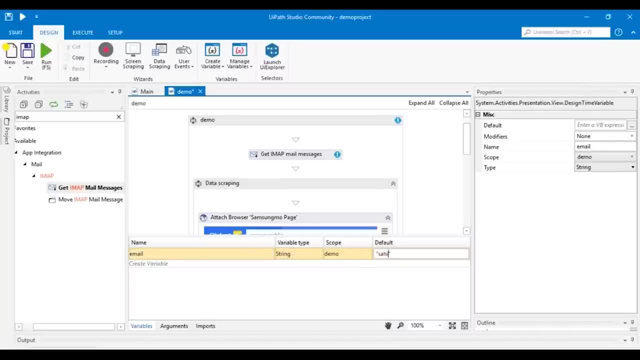 Now it will ask you for your email and password. So let's just create a simple variable for email and password. So let's just create a variable named email and password. So if I type in email of string type and by default it should be my email ID. 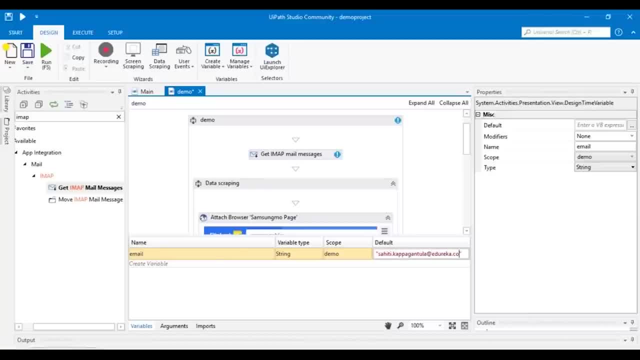 So I'll just type in my email ID and the password. Let's just create a variable named password. So now, once you've created the variables, you have to mention them in the IMAP activity. So let's just click back on the IMAP activity. 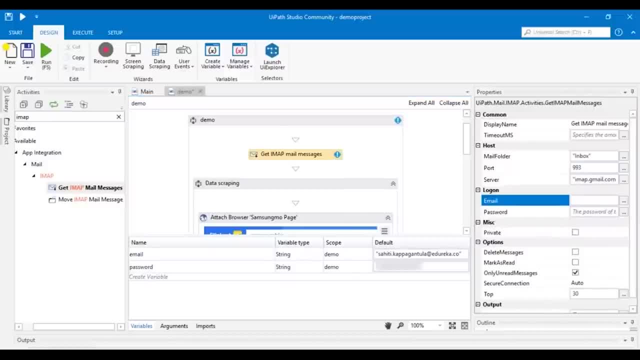 go to the property section and in the login details enter the variable name as email and in the password section let's just enter the password variable. right Now. let me tell you one thing here: Any variable that you mentioned in the UiPath tool. 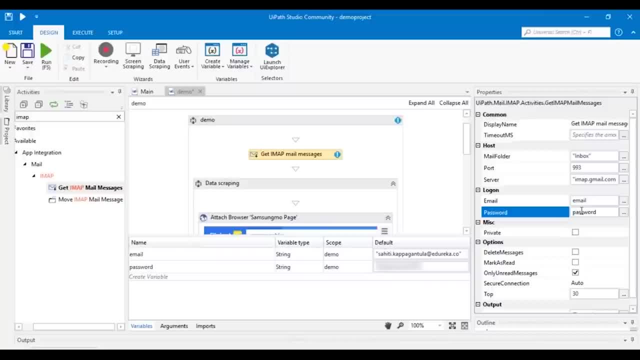 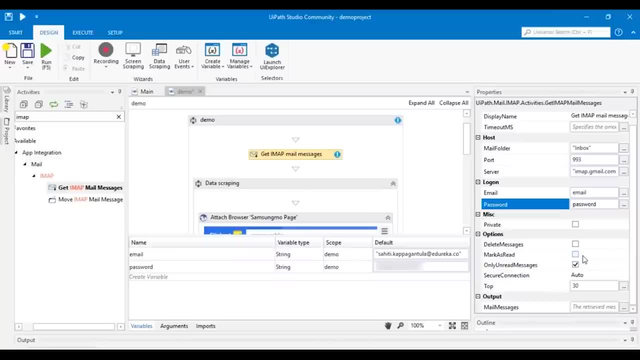 need not be included in double quotes. It's only the text that you have to include in double quotes. All right. After this is done, you can configure various options, such as if you want to delete the messages or if you want to mark it as read. 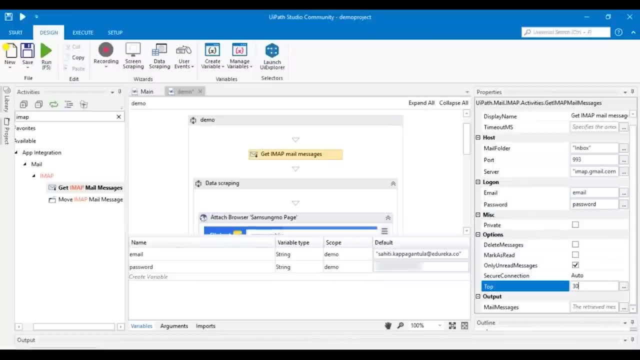 or if you want to read only the unread messages. So, from top, if I want to read only one message, I'll choose one, All right. So once you have set the properties for your IMAP activity, the next thing that you have to think about is: 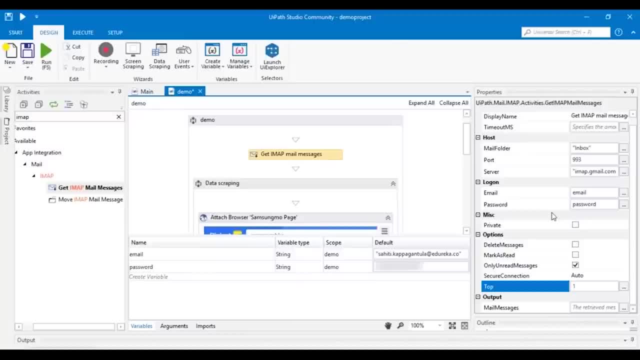 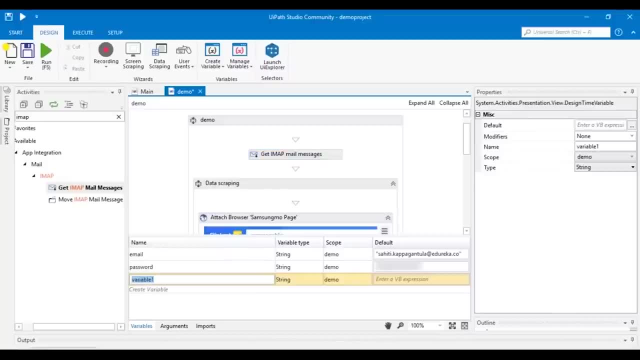 whatever you're getting familiar with, the email has to be stored somewhere, right? So to store somewhere, you have to create a variable which is of list type. So let's just create a variable mail messages of the variable type list, right? 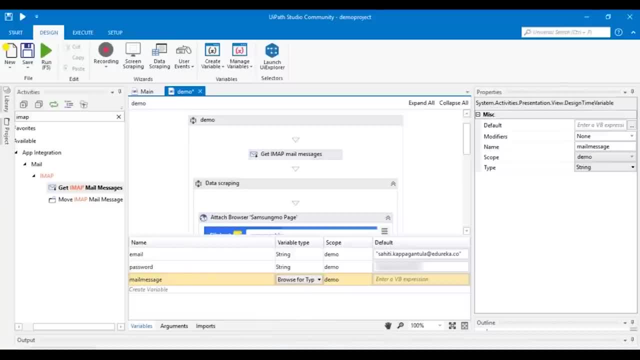 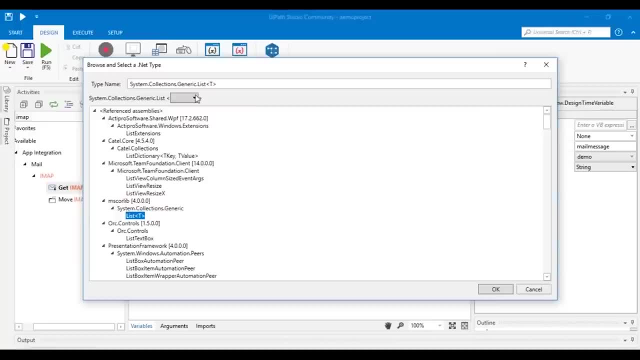 So for that you have to click here and choose browse for types In the search option, search for list, and under the system collections, generic, you'll find the list option and then you'll choose list of T. So now, what is T? 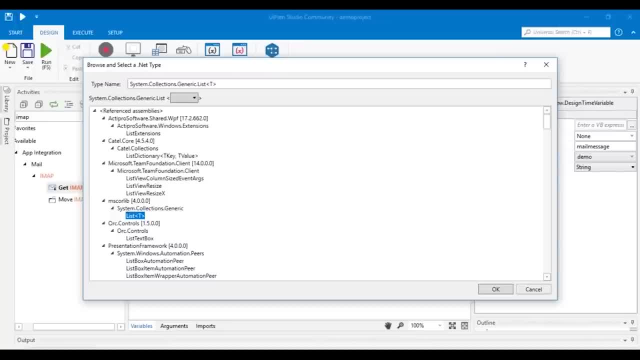 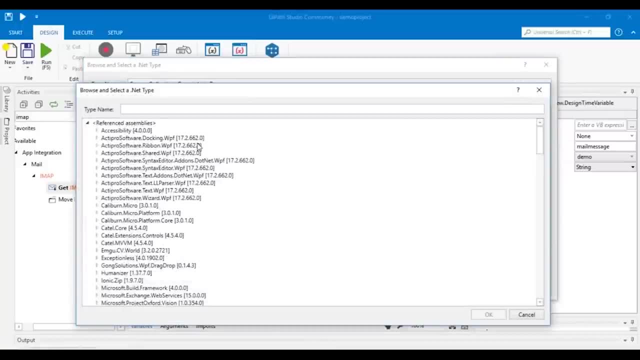 We have to define it here. That is the mail message. So I'll just go to the dropdown and then search for mail over here. So for that let's just go to browse for types again and let's search for mail and under the systemnetmail option. 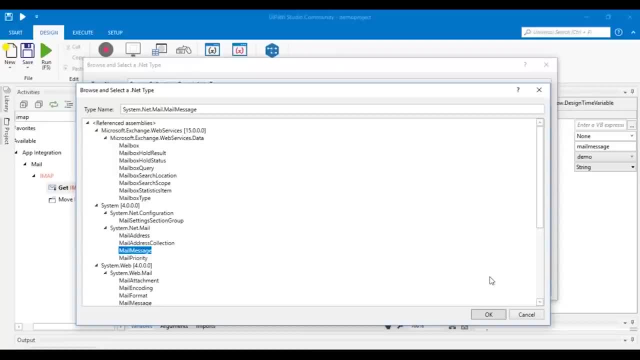 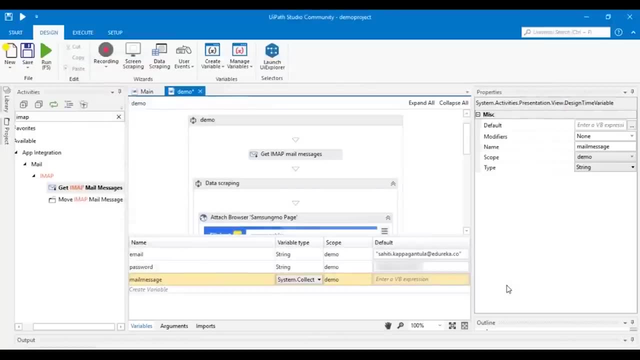 you have to choose the mail message option, right? So after that, just click on OK and then again click on OK. So after this is done, I have to specify this variable name in the properties of IMAP activity. So let's just click back on IMAP activity. 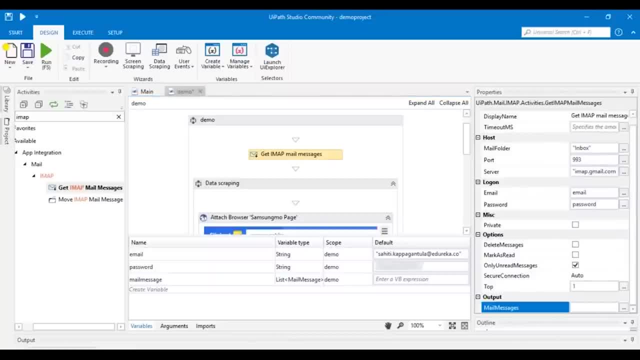 go to the property section and in the output section, mention this variable name. So once this is done, our IMAP is configured to receive emails right Now let's just check in. If you're able to search, you can observe that there's no activity to search, right. 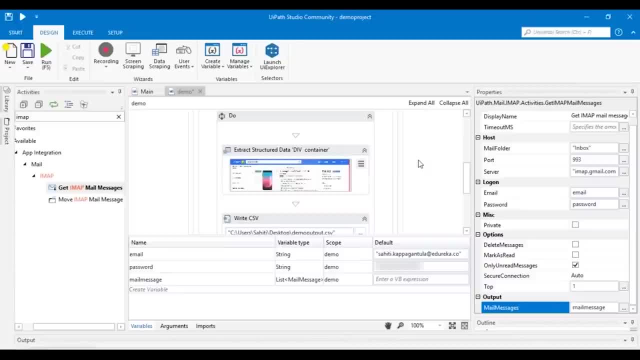 So that's because I'm not passing the information anywhere. So to pass the information I have to pass the emails that I'm getting through the IMAP activity. So for that I have to use an activity called for each. So in the activities pane. 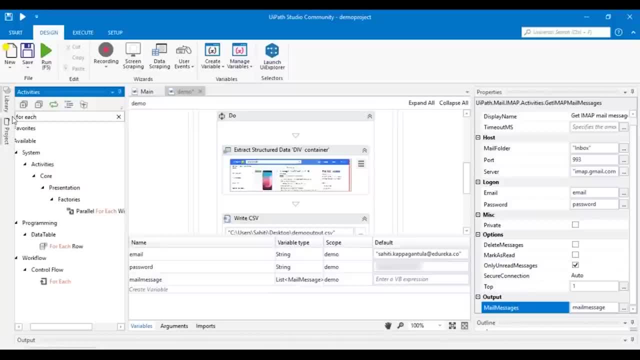 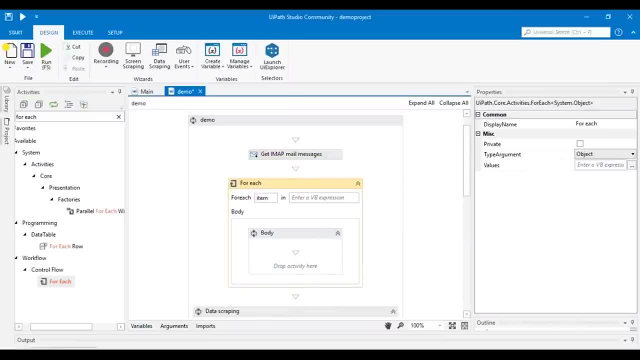 let's search for the activity for each and let me just drag and drop it here. So, basically, what are we trying to do with this activity for each? So the for each activity would enable us to get information from each mail, right? So there's one email that I'm using right now. 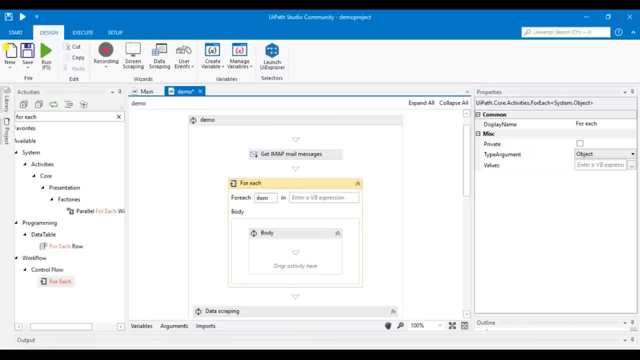 but for future uses, you'll be using various number of emails, So that is when I would need this activity Now. in the for each activity, you can observe that it asks us for each item in what? Basically, in that we have to include a variable. 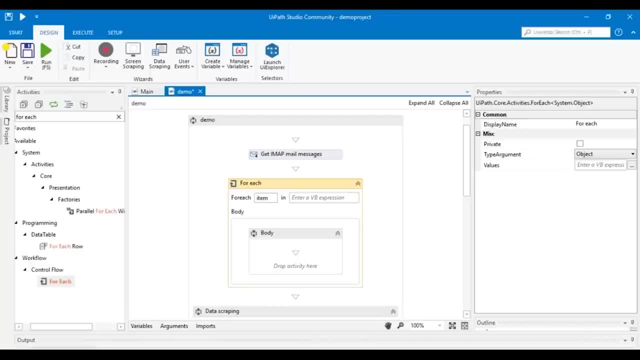 So basically for each item in my mail messages, right? So the mail messages is basically the output that we're getting from IMAP, So we're going to include that. So let's just include mail message variable here and in the item section. 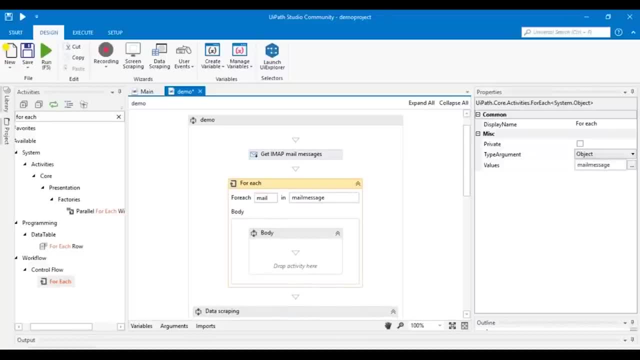 let's just say we include mail. So basically this would mean for each mail in the mail message we want to do the repetitive task. All right. Now in the properties pane of this activity you have to make sure that the type argument is of mail. 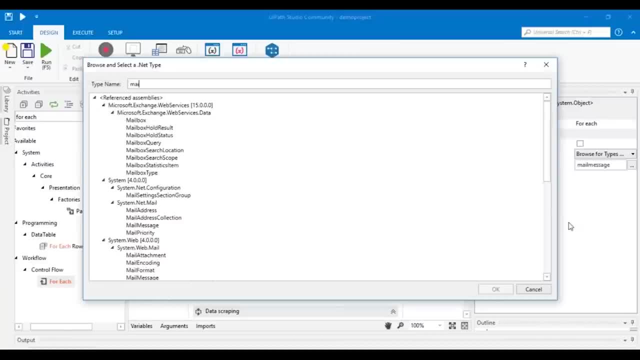 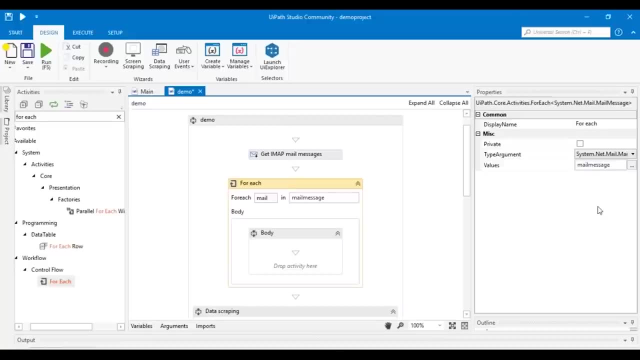 So let's just search for mail here. So by mentioning the type argument as mail, we are identifying this argument is of type mail message and is looking inside the variable which is of type list of mail messages, right? So basically, you're trying to search a mail. 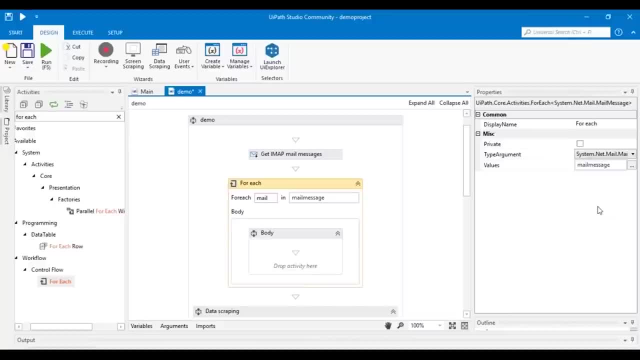 in the mails you have Now. this for each activity will execute anything that is inside the body time and again. Now what the for each activity will do is it will execute anything that is inside the body, So each time it receives a mail from its list. 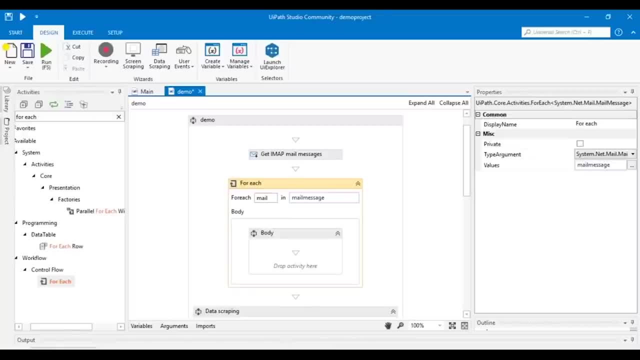 it will execute the action specified and then go back. All right. So if I specify this, I will specify the activity to open a browser which will point towards my custom search page for now, And then I'll be going to the e-commerce website. 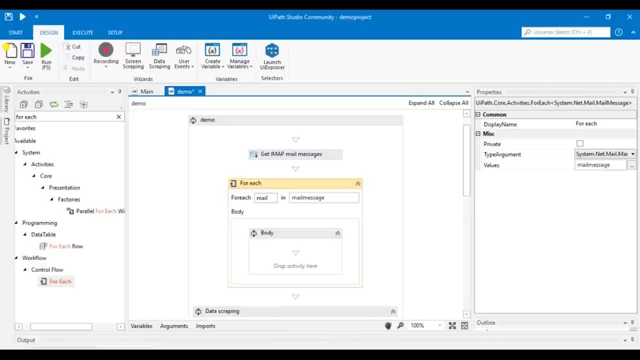 I'll scrape the data, So the complete task will go again and again each time it finds a mail. All right, So now to perform this task, let me just go back to my e-commerce website. So let me just say I search for the product. 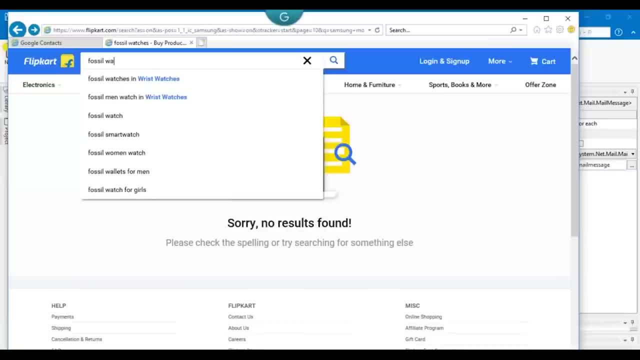 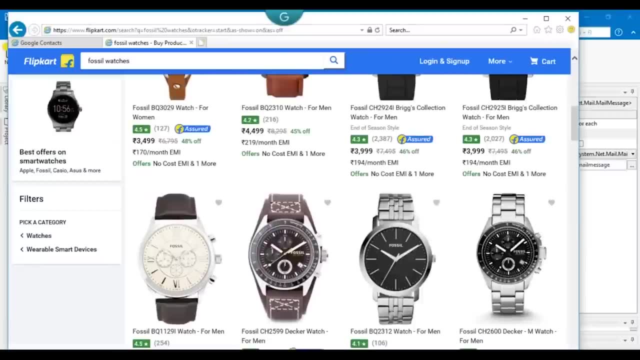 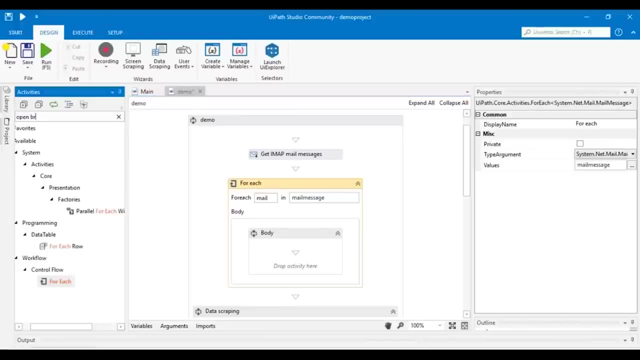 Let's just say I search for fossil watches. So let me just type in fossil watches and the search results show all the watches related to the brand, right? So I will just copy this link and let me go back to the tool and then search for an activity as open browser. 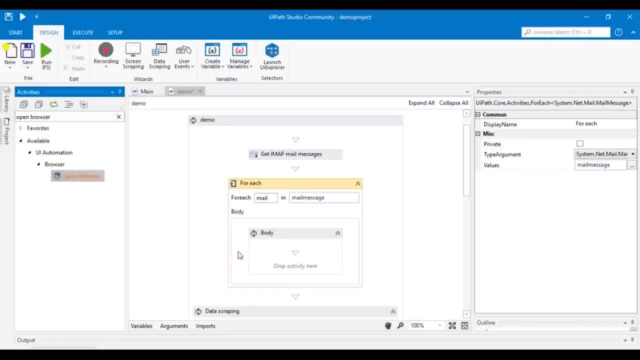 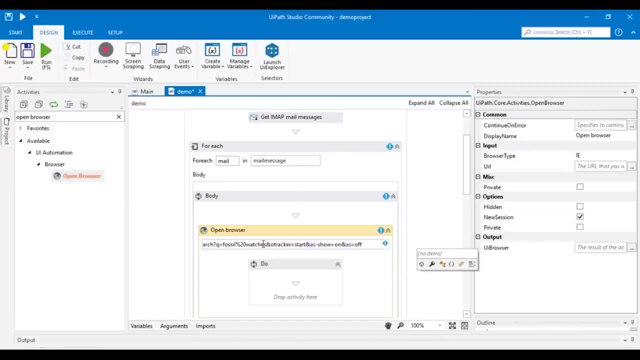 and then drag and drop it in the body section, right? So let me just drag and drop it here and then let me just paste the link that I've copied. So basically now, whenever it finds the mail inside the list of mail messages, it will open a browser, right? 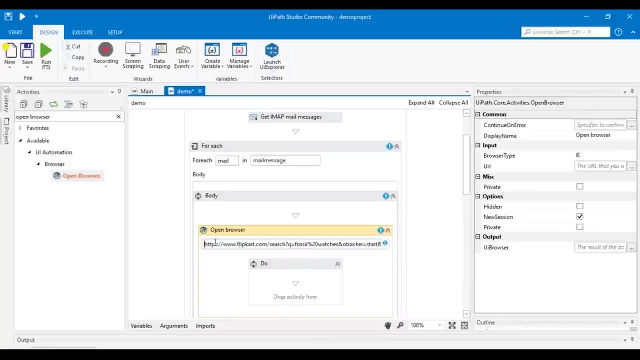 So it will point to this particular address. Now again, if you observe that the address is a string, right? So, as I told you before, all the strings must be included in double quotes. So let me just include this in double quotes. 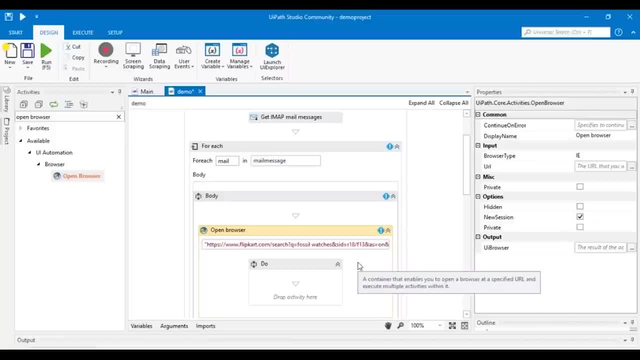 Now, if you observe here, this address only searches for fossil watches. Now, if you want to do custom search, what you have to do is you have to close the double quotes here, open the double quotes here and then remove this part, and then you have to search for each item. 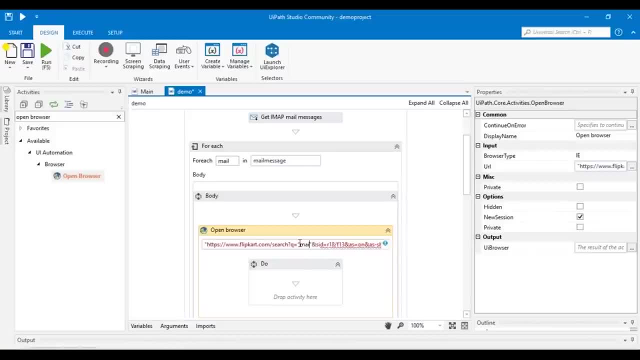 in the subject line, right? So for that you just have to include the mail variable dot subject so that it identifies from subject. All right, Now you can see that there's some error because of the exclamation marks, So to remove that. 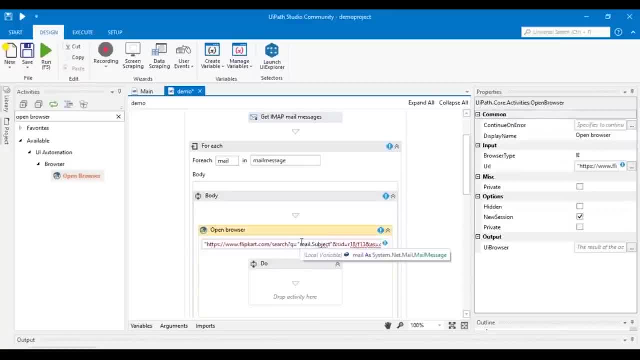 let's just see that the error is here. Okay, So what you have to do is, when you concatenate something, you have to include the plus signs, right. So now you can see that the exclamation mark is gone Once you click out of the sequence. 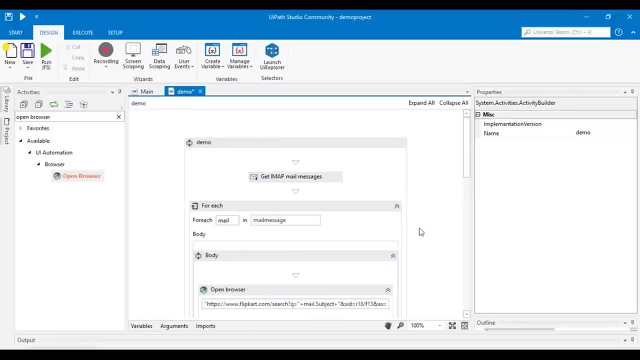 you can see that the exclamation mark isn't there. That means our program is running error-free. So now what's happening here? Basically, I wanted the subject line of my mail to be identified for the search query right, So I just replaced the text in the search query. 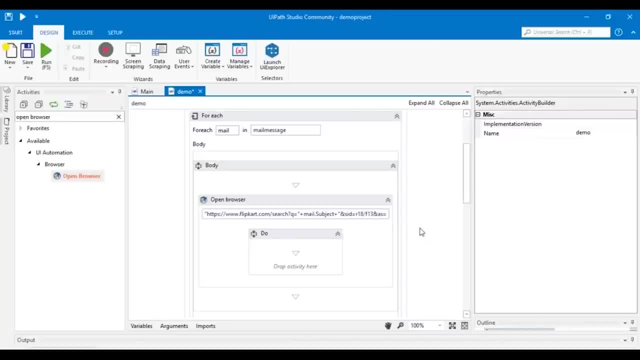 and then I included the variable for subject line. So this will read the mail and it will store everything in a list of mail messages. So suppose if I give the subject line for LG TVs, it will go to this custom link and it will scrape the data for LG TV. 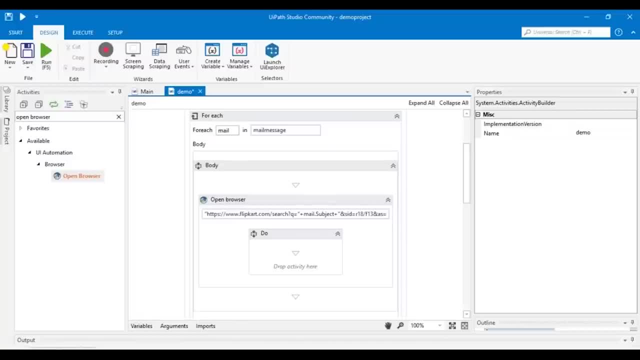 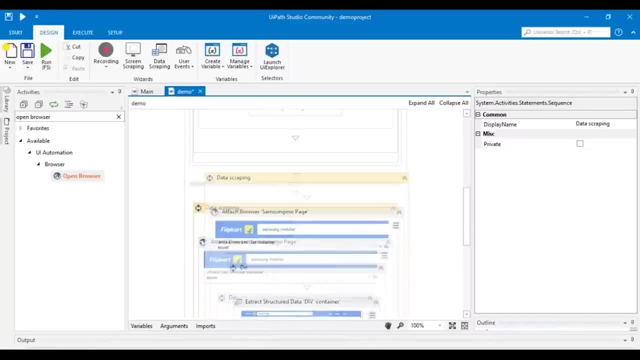 in the Flipkart website, right? So I've already done this data scraping part for you, So now let's just drag and drop this data scraping part over here. Let me just drag and drop it in the do section over here. After I drag and drop it here: 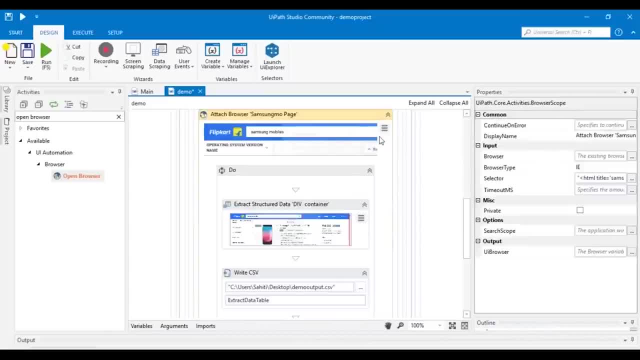 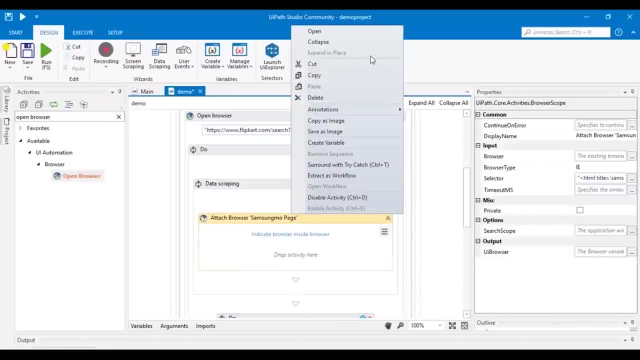 I'll just remove the part where I've searched for Samsung Mobile. So let me just go here and let me just remove this. So let me just drag and drop this here. Let me just delete this part and let me just drag and drop it. 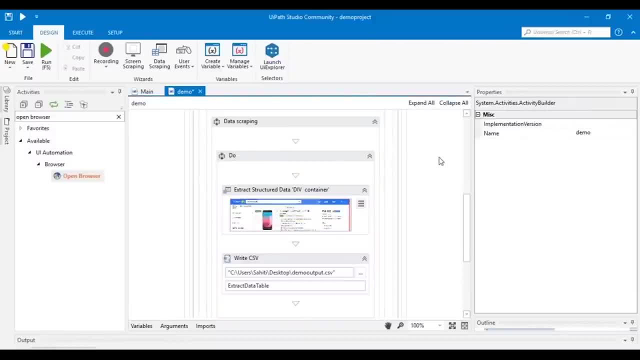 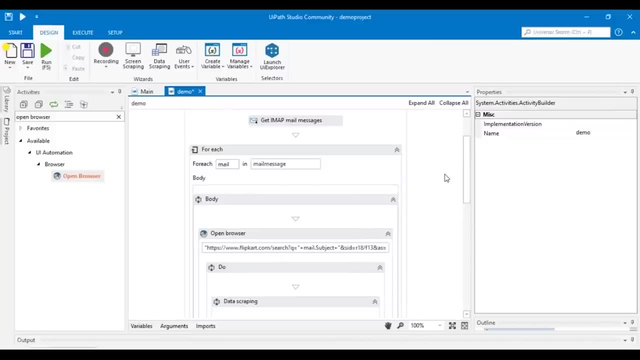 back here. So, guys, let me just click out of my sequence and check for any errors. There are no errors. That means our data scraping is fixed right. So now let's just go through what all we have done. We have created an activity to receive emails. 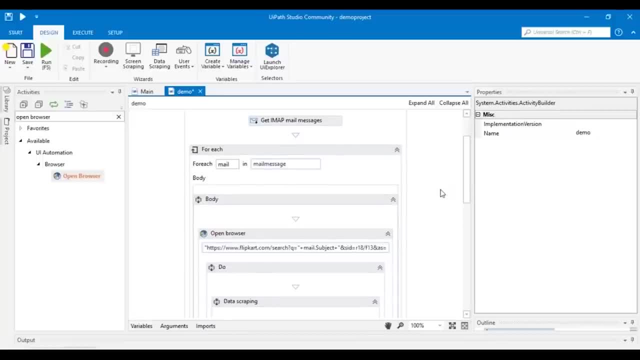 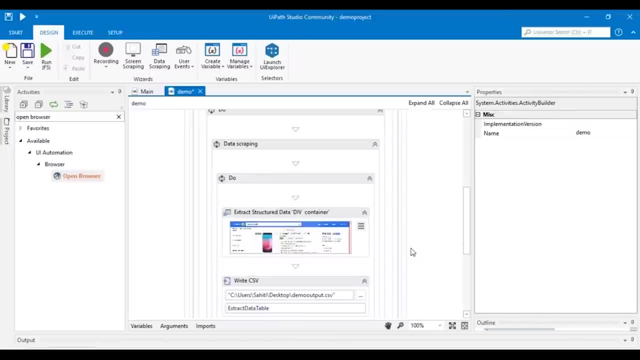 and for each mail we have decided a process to do, right. So we'll go to the Flipkart website, We will do the custom search and once the custom search is done, the data will be extracted and then it will be stored in an output file. 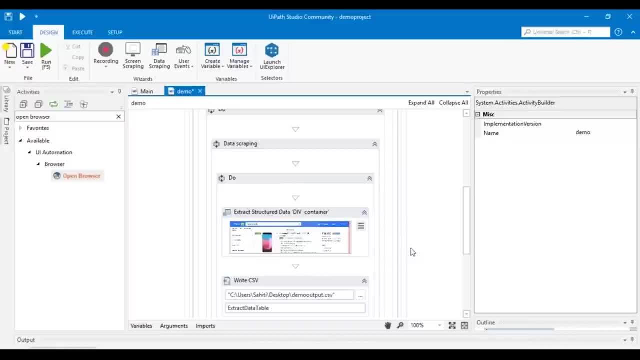 So now let's just bring this back and let's make it more interesting by trying to get an email back with all the data scraped right As of now. it will just take the email, it will get the search query. it will search for it. 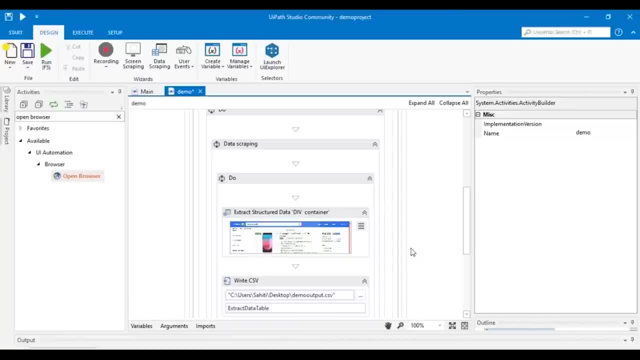 and it will store it in the CSV file mentioned. But now I want to get an email back with all the data scraped. So for that we have to search for the SMTP protocol in the activity pane. So let me just go to the activity pane. 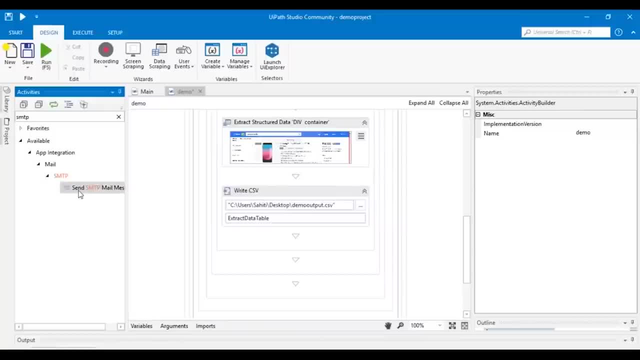 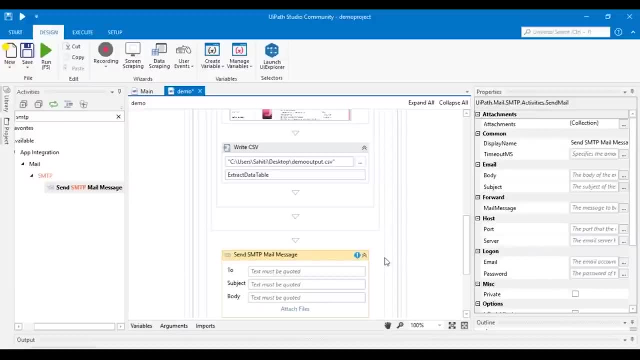 and search for SMTP protocol. So once this is done, let me just drag and drop it here. So once this is done, you have to specify whom do you want to send the email, right? So since I want to send the email back to me. 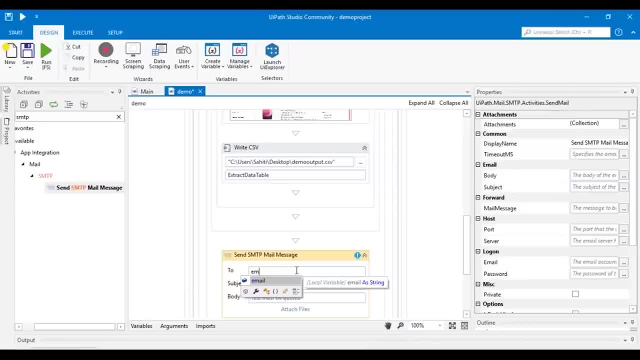 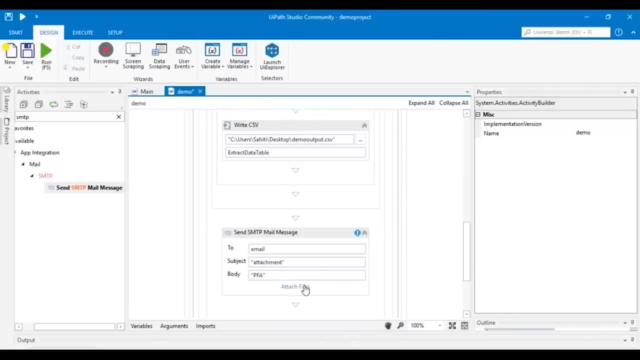 I'm going to mention my mail ID, So that is email variable. Let the subject be attachment and the body be PFA. All right, So now let's just attach these files. So to attach the files, we have to click on this option: attach files. 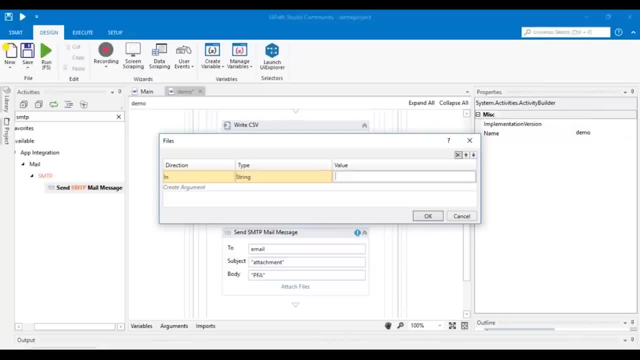 So in the argument you have to mention the file path, right? So let's just search for the file path here. The file path must be included in double quotes, So let me just go back to the documents where I've stored this file. 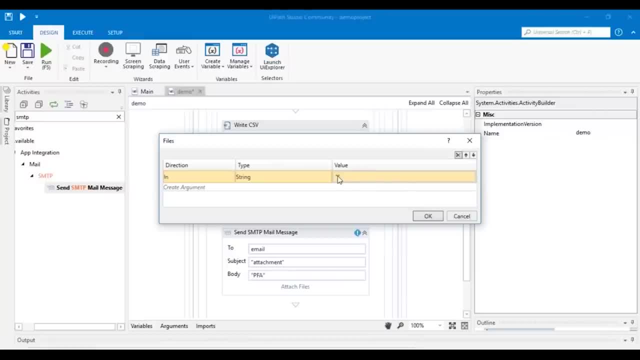 Let me just copy the address. Let me go back to UiPath tool, paste the address and then include the file name. all right. Once it is done, click on OK. All right. So what's happening here is it will pick up the file from this particular address. 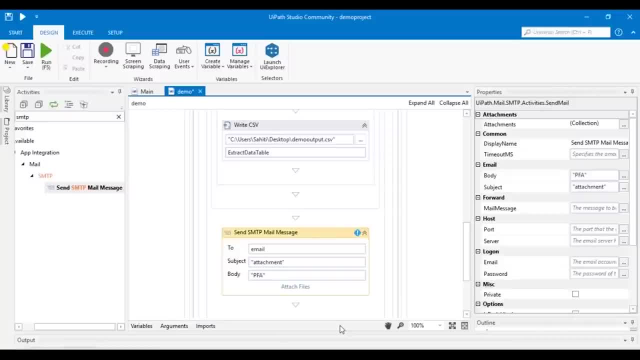 and send a mail to me, But again you see an exclamation mark here, right. So that means there's some error. So for that you just have to configure SMTP. Let me just click on the SMTP activity. Let me just go to the property section. 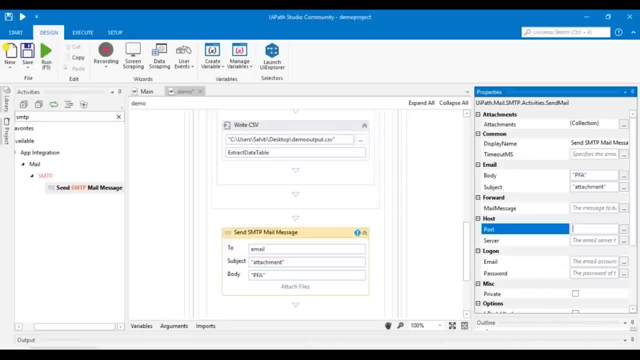 and in the port number you have to mention the SMTP protocol port number. that is 465.. All right, And the server name as smtpgmailcom. All right. After that it will ask me for an email, So inside the email option. 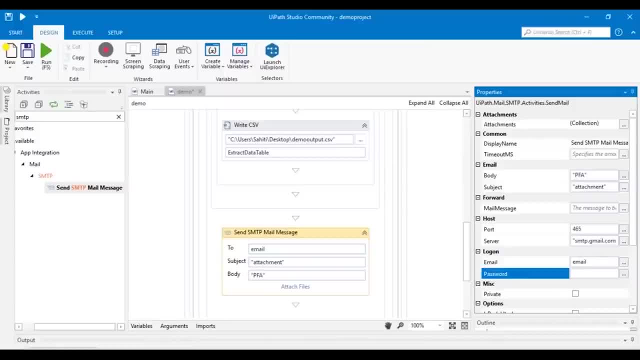 I'll put in my email variable and in the password option I'll include my password variable. Whom will it send to? It will send to myself and it should come from me. That's the property section that you have to configure. All right. 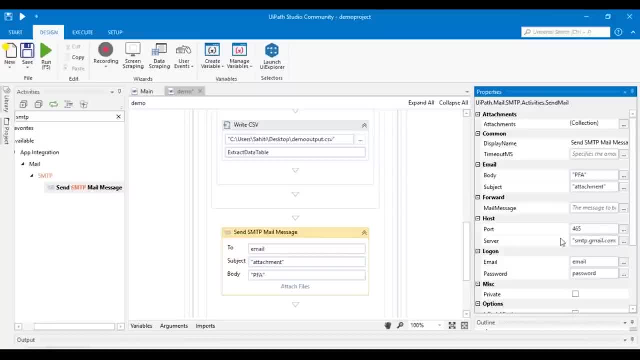 So, guys, this was a basic demo. You can actually play around with it and create an advanced version of it, But for now let's just look into how it runs. All right. So let's just click out of the sequence and you can see. there are no exclamation marks here. 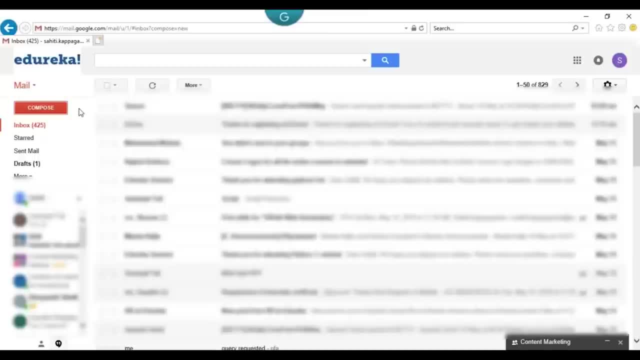 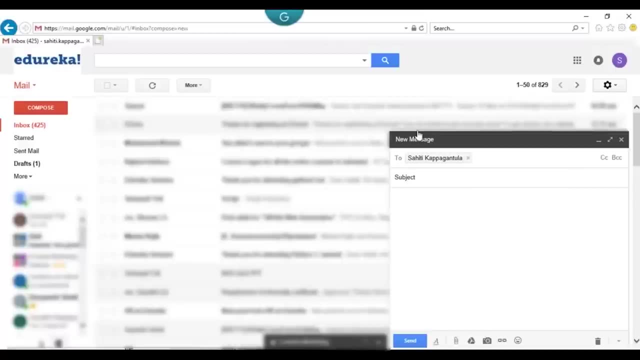 So now let's just go back to our email ID. So let me just go back to my email ID and then let me compose a mail to myself with the subject line of the search query, right? So if I want to search for LG TVs, 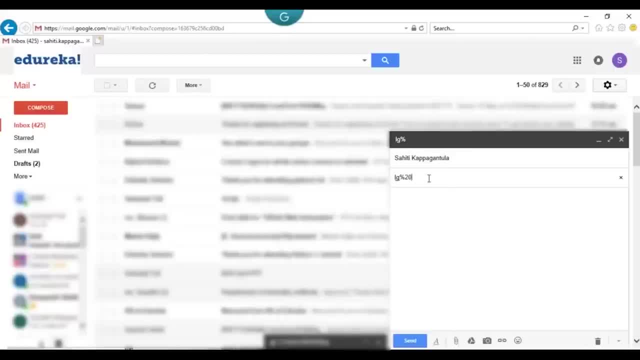 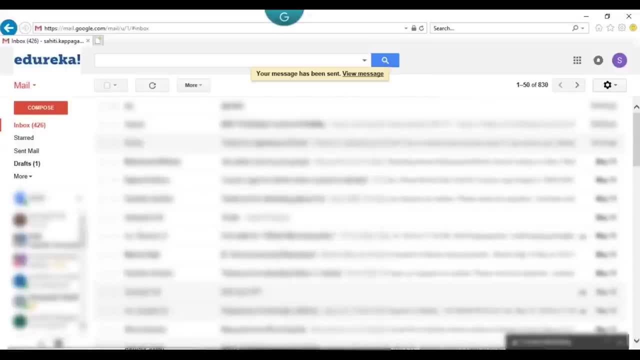 I'll type in the subject line for LG percentage 20 TV and then send. So why have we included percentage 20?? That is because anytime you want to identify a space in UiPath, you have to include percentage 20.. All right, 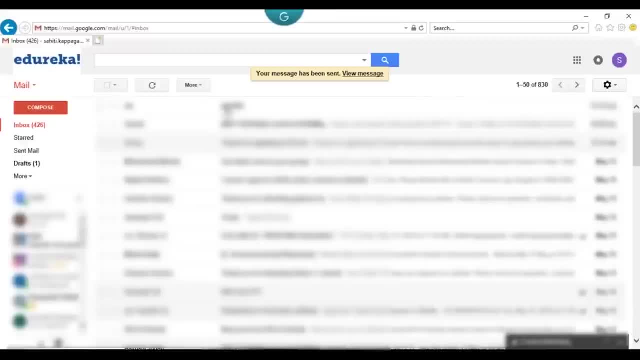 So once it is done, you can see that you have received a mail with the subject line: Now let's go back to the UiPath tool and let's just run this program. So now let's just check if you've got any mail. 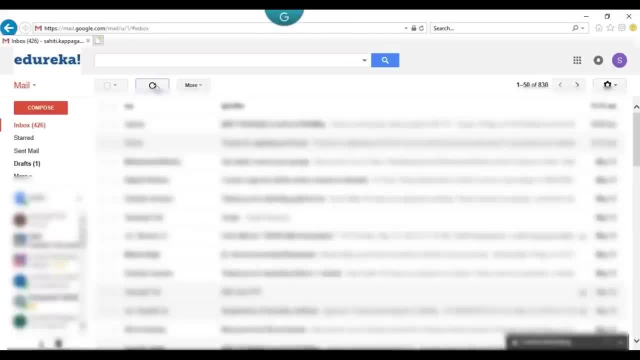 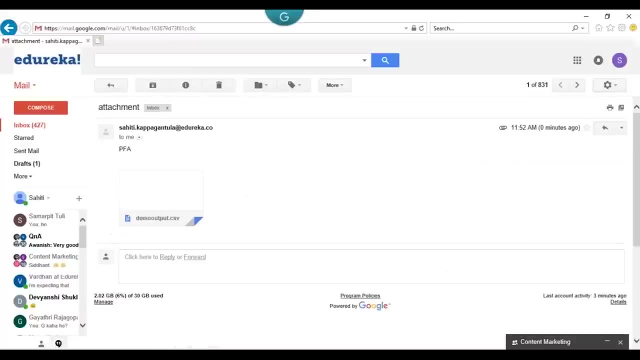 So let me go back to my email ID and let me just refresh this. So once you refresh this, you can see that you've received a mail with the attachment, right? So let me just open this and download this file for you, All right. 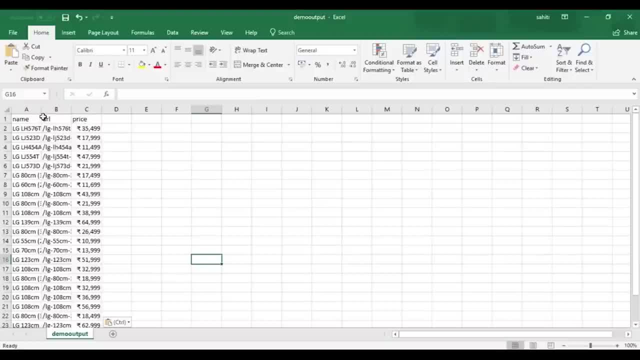 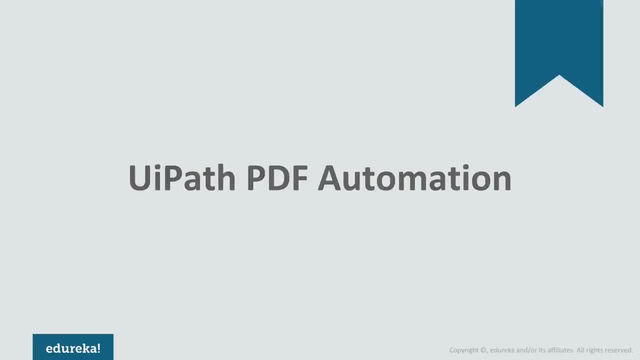 In the demo output file you can see the name, the URL and the price right. So that is the data which is extracted and it was sent to you. The session will basically brief you on all the activities that UiPath offers to extract data. 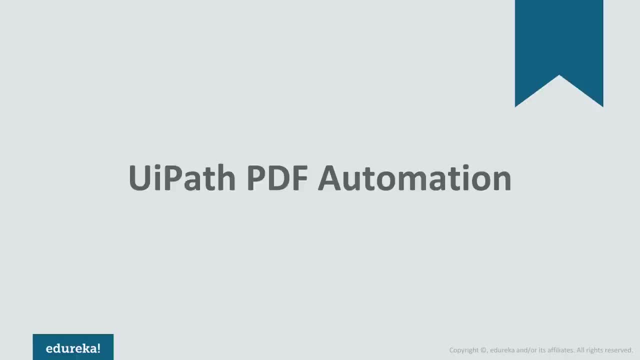 from whether PDF is in the native text form or even in the scanned images. Now, before we start extracting our data, you need to first install our PDF activities from the manage packages section. So for that, let me just open my UiPath. 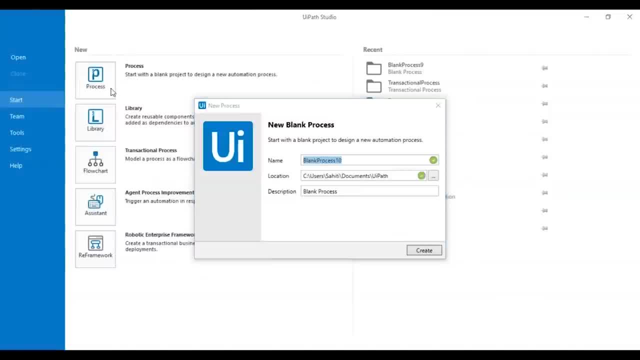 All right, So now I'll just choose the blank process and let's say I'll create a new blank process, Let's name it demo for PDF extraction and then I'll mention the description to be demo again and I'll click on create. So this will basically create my process. 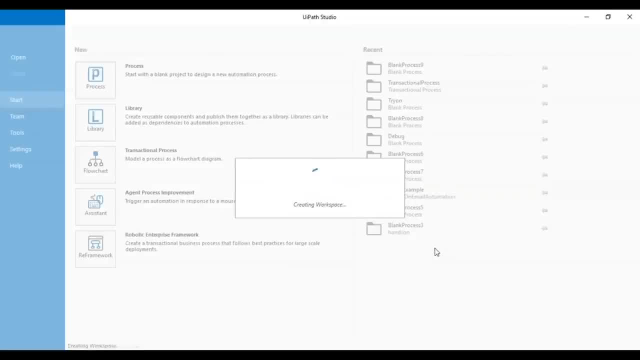 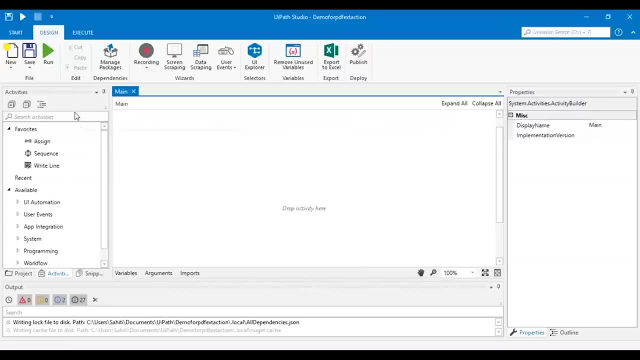 or you can say the project. Now, inside this particular project, I'm going to install the PDF activities and perform all the extractions that you're going to see in the session. All right, So, as I was mentioning before, you start extracting data. 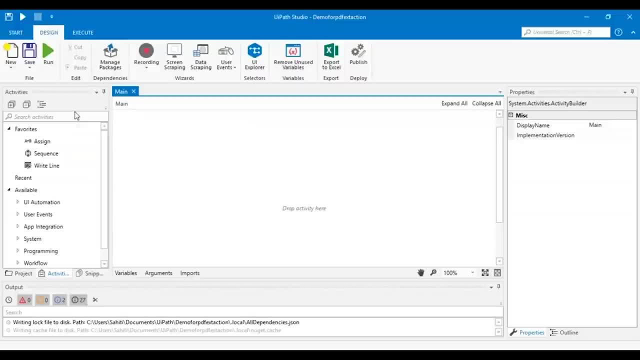 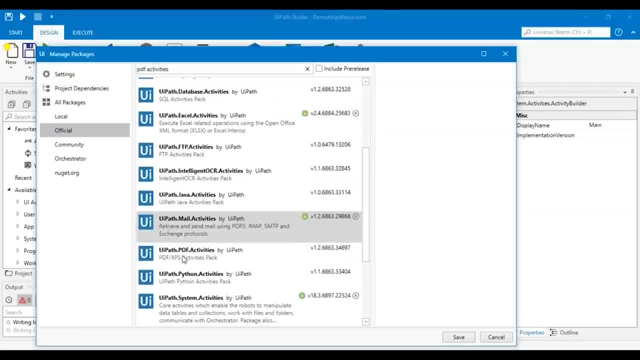 you need to install the PDF activities, right? So for that, you'll just go to this manage packages and then you'll search for PDF activities, All right? So, as you can see, you have to install this particular package. So for that. 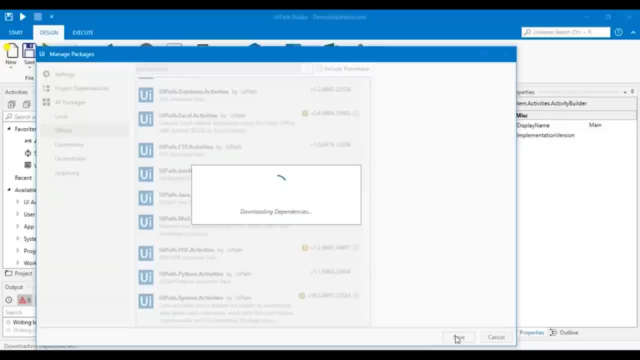 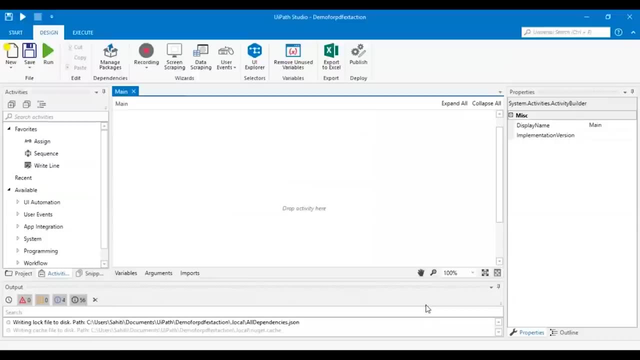 you'll just click on this small arrow button that you see and then you'll click on save. So once you click on save, you can see that you know your dependencies are getting downloaded for the workspace. Now, once the dependencies are downloaded, 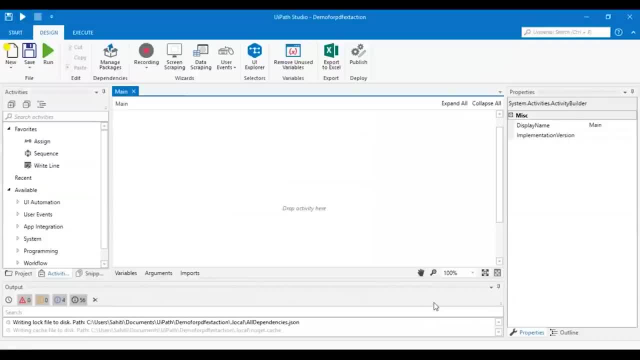 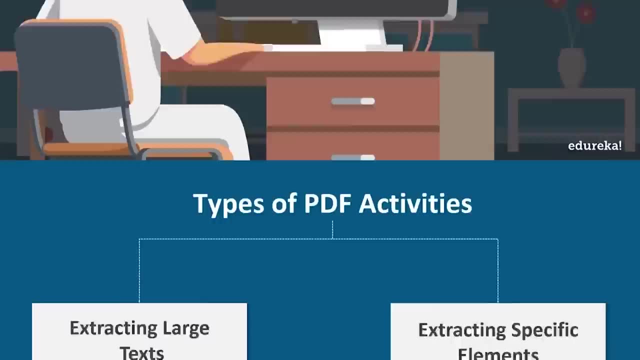 you'll see that. you know you'll be redirected to this particular window. So let me just quickly go back and explain you the topics for PDF extraction and then I'll show you how you can do it with UiPath right Now that you have your PDF activities. 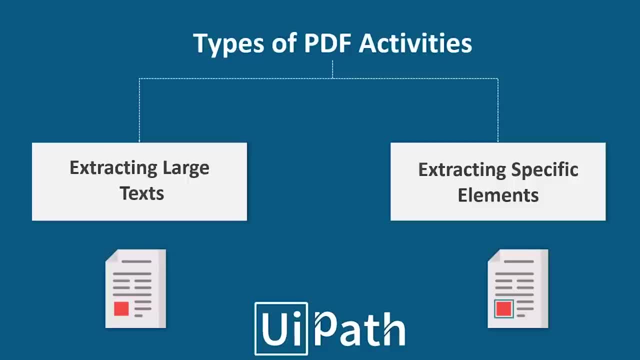 installed on your UiPath. let me tell you that there are basically two ways to extract data from PDF. That is basically extracting large text and also extracting specific elements. Now, when I say extracting large text, I mean that either you want to extract a complete text document. 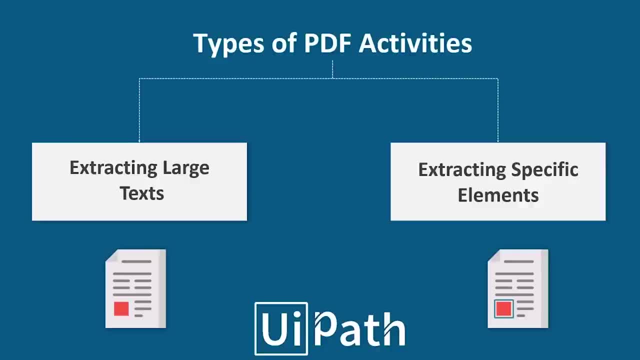 or it can happen that you want to extract the text document which also has images, right. So extracting large text would be extracting either the complete text from the document, based on the number of pages that you give for the document, or you also can extract images. 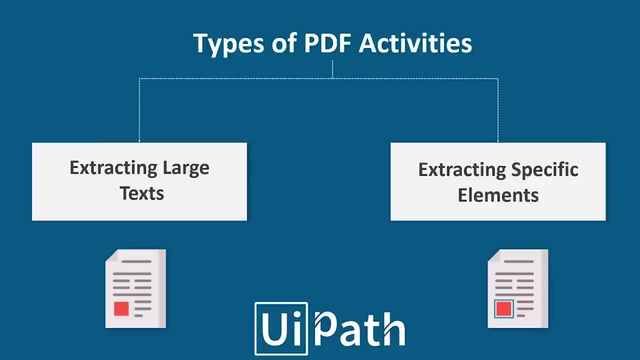 and text together of a large document- And when it comes to extracting specific element. by extracting specific elements I mean that whenever we want to extract some specific variable or something right. So let's say if you have any invoice and I can extract the invoice number. 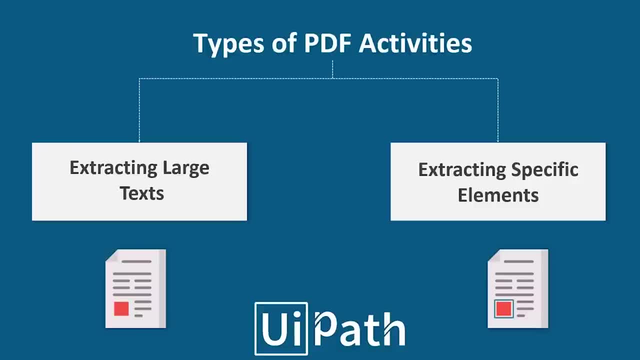 or you can extract the grand total or the tax saved and so on. right, So I'm going to talk about both of them one by one. So, initially, we're going to start with extracting large text and once we're done with that, 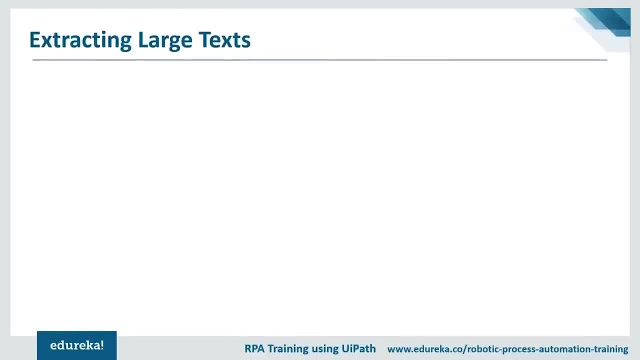 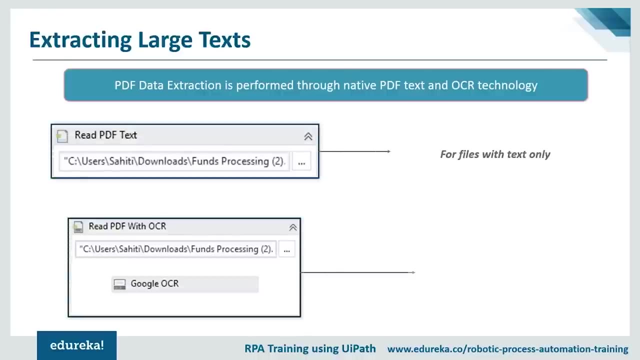 we'll move on to extracting specific element. right, So let's start with extracting large text Now. to extract large text, there are mainly two options in UiPath. that is, either to use the read PDF text activity or to use the read PDF with OCM. 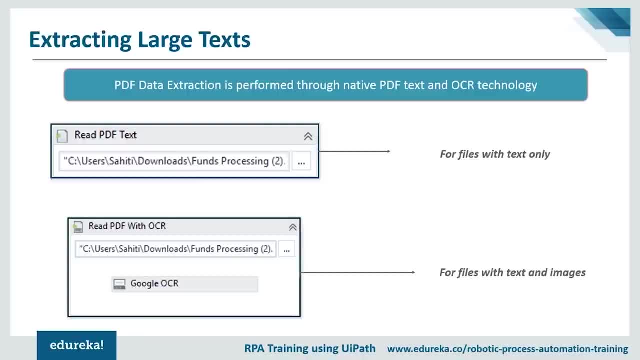 Now what happens is the read PDF activity is used to extract the data from those PDF files which have only text. So this particular activity is basically used to extract data from those files which have text only, But when it comes to read PDF with OCR activity, 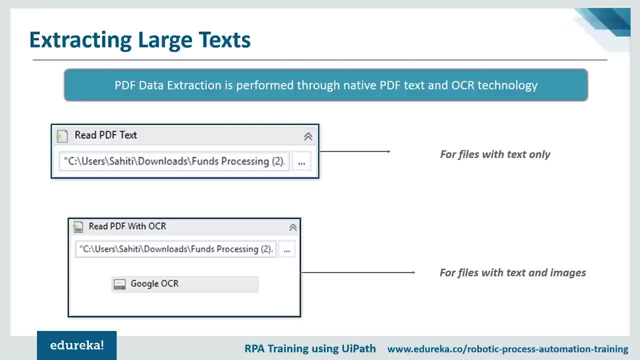 this particular activity can be used when you want to extract data with those kinds of PDF files which have a combination of text and images, right? So just in case, if you have any image in your PDF, then remember that you have to use the read PDF. 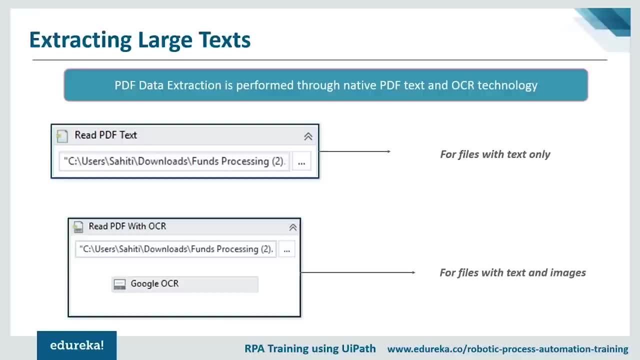 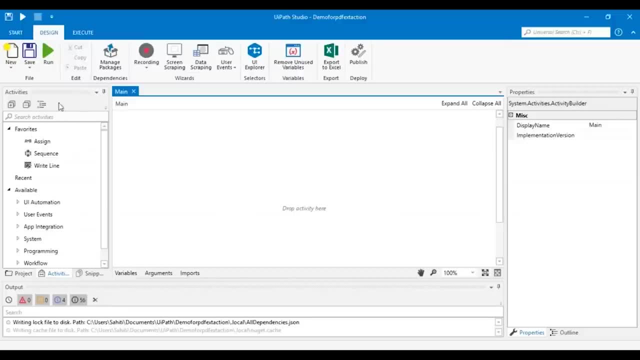 with OCR activity, else you're going to have to go forward with read PDF text, right? So let me just quickly shift back to UiPath and show you how that's done. All right, So now what initially I'm going to do is I'm going to drag a sequence. 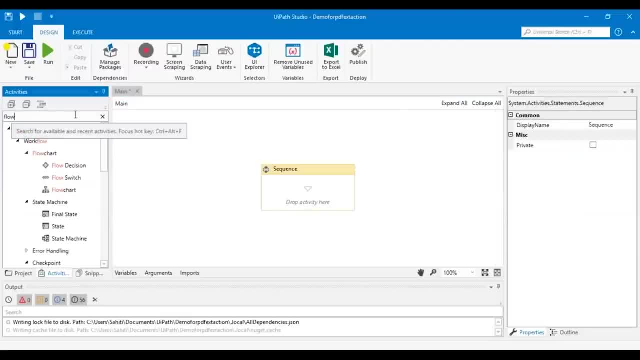 And then, in this particular sequence, what I'm going to do is I'm going to drag a flow chart. Now I'm dragging and dropping this flow chart, since we are going to perform various activities, So I'm just going to use all these activities. 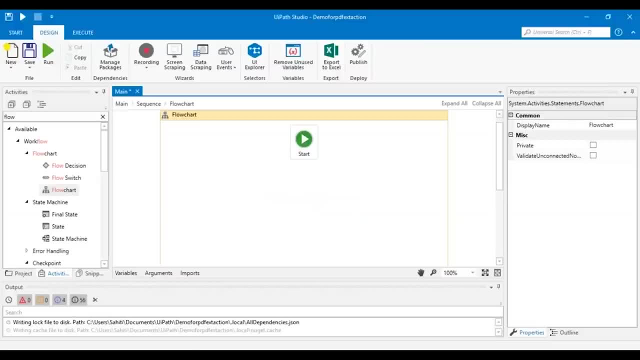 in the single flow chart. So whichever activity that I want to run, I'll just run that particular activity. So this is one way you can do your work easily. Now what I'll do is I'll again drag and drop a sequence, And let's say I start with the read PDF activity. right? 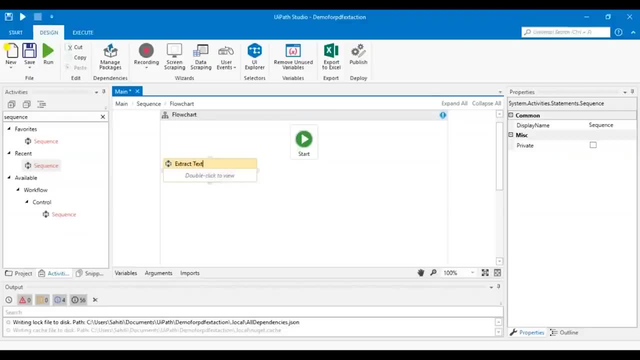 So let's say, extract text. So I'll rename this particular sequence to extract text and then I'll double click on it And then over here I'll search for read PDF activity. So, as you can see, when I search for read PDF, 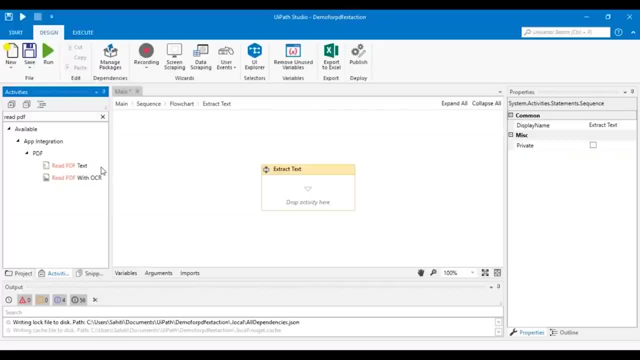 we get two options, That is, the read PDF text and read PDF with OCR, right? So first I'm going to show you how you can use the read PDF text, So I'll just drag and drop it over here Now. once you drag and drop it over here, 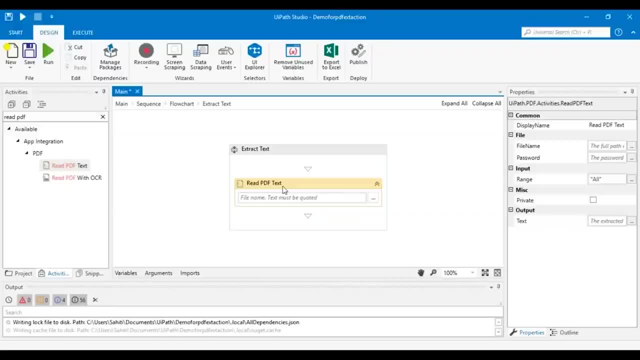 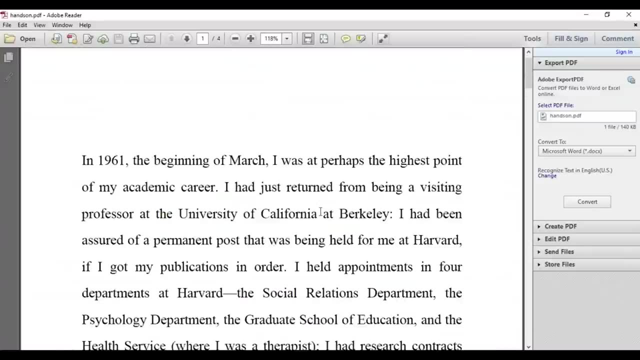 what you have to mention is the file name or the PDF from which you want the data to be extracted. So let me just show you my sample PDF. So I've opened the sample PDF that I've created to extract the data. So what you see from this particular paragraph, 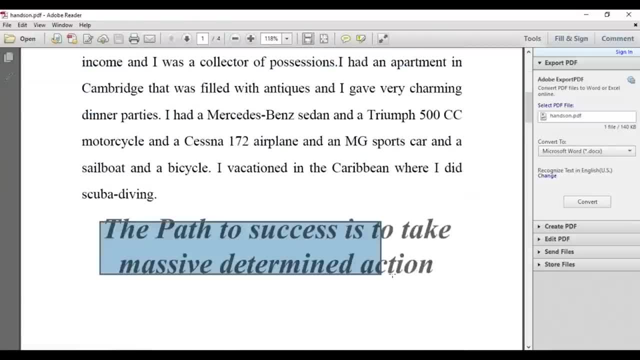 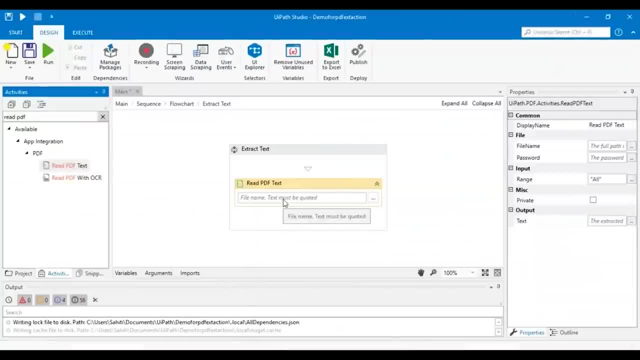 that this is the complete text and this particular code is an image right. So what we're going to do is, first, we're going to extract the text from here. So what I'll simply do is: I'll just mention the part for this particular paragraph. 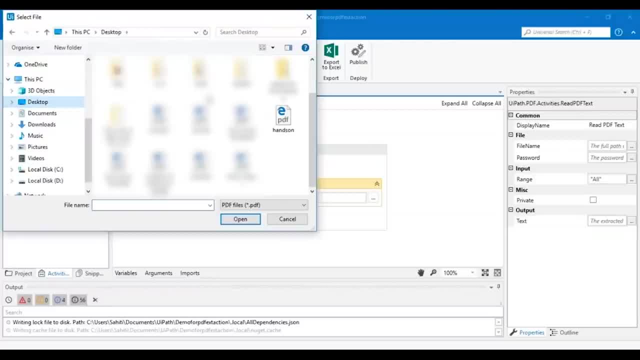 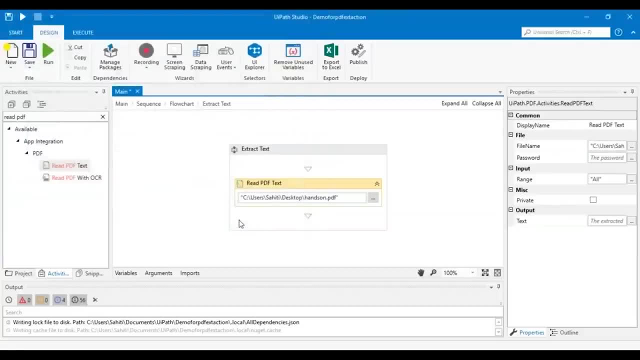 in the PDF. So I'll go to this three dots option, I'll go to desktop and then I'll choose the name of the PDF that is hands-on and then I'll click on open. So now this activity knows which PDF has to be read. 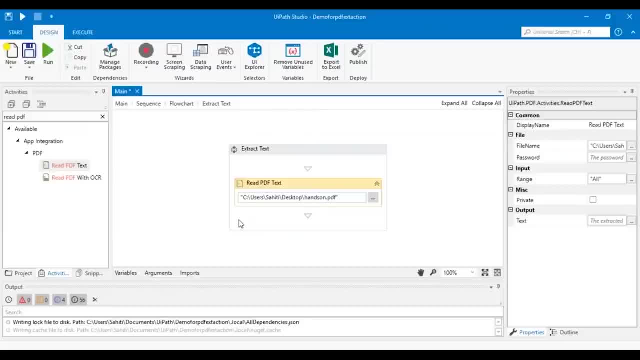 and from where the data has to be extracted. Now to see the output, what you can do over here is either you can put a message box or you can put a write text activity right. So let's just search for write text and then I'll drag and drop it over here. 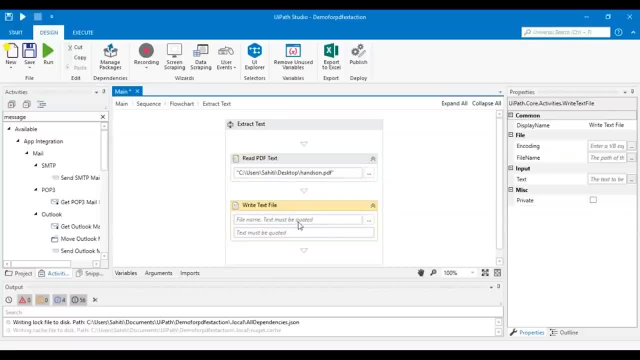 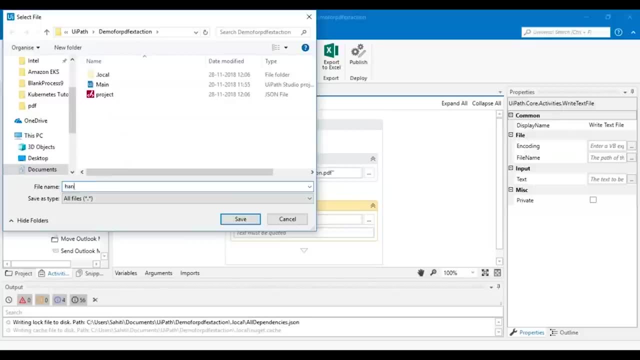 So I'll just drag and drop this write text activity. Now what I have to do is I'll have to mention the file name for the write text. So let's say, I'll mention in this particular folder and I'll mention the output file, to be hands-on, right. 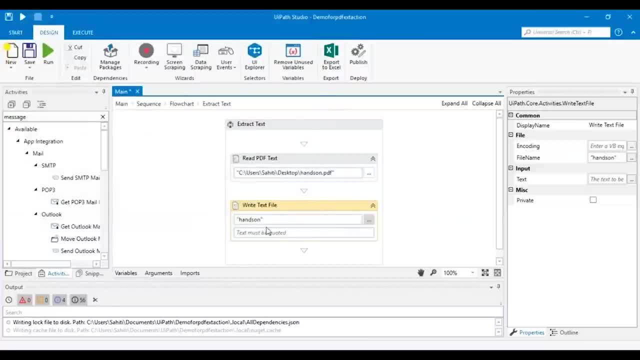 And then I'll click on save. Now, after I'm done with that, I'll have to mention the output. So before you do that, you have to mention the output variable in the read PDF text activities. So you can just go to the properties pane. 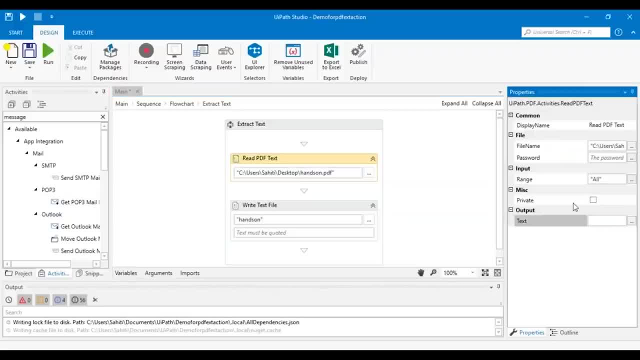 that is on the right side of the window, and to just set a variable, you can just press on control K and then mention the variables name, Let's say output, and then we'll mention the output variable over here, right? So what the UiPath understands. 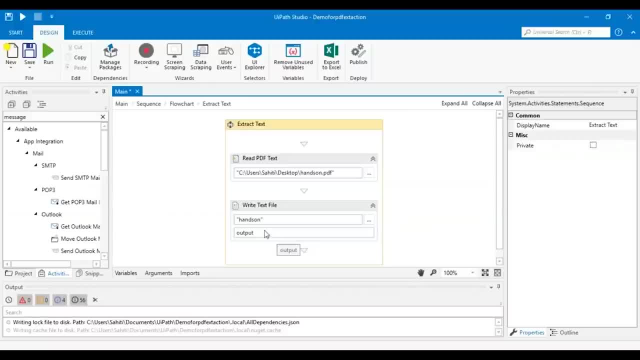 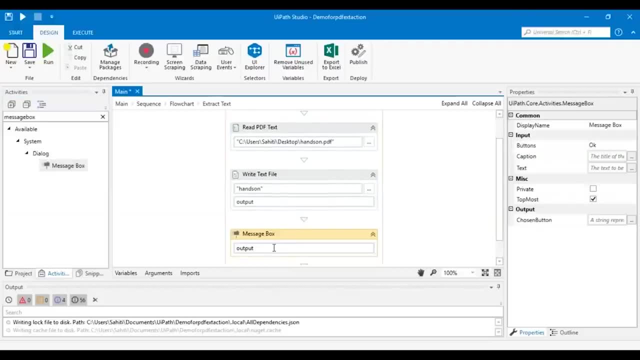 that we want the data that has been extracted to be written into this particular text file. Also, let me search for a message box and I'll drag and drop it over here and then over here will again mention the output variable, right? So I hope that you know. 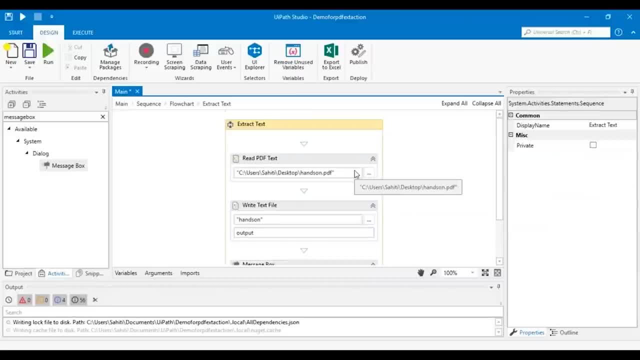 the read PDF text activity is clear. You just have to mention the part of the file, that from which the data has to be extracted, and then you can write the output to a text file message box or any other string activities. So I'll just click on debug. 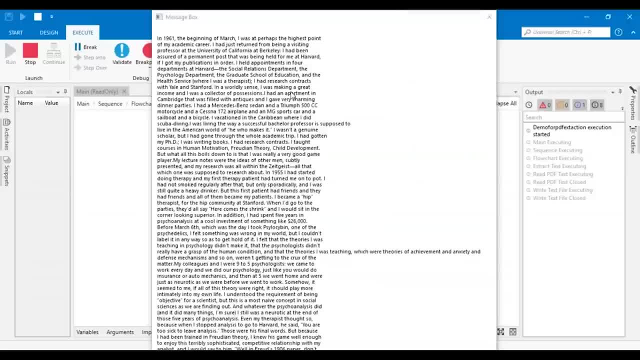 All right. So, as you can see that the complete text present in the PDF has got extracted, So you don't understand where the images or even it got extracted, or not, right? So for that, what I'll simply do is I'll go to the read PDF text activity. 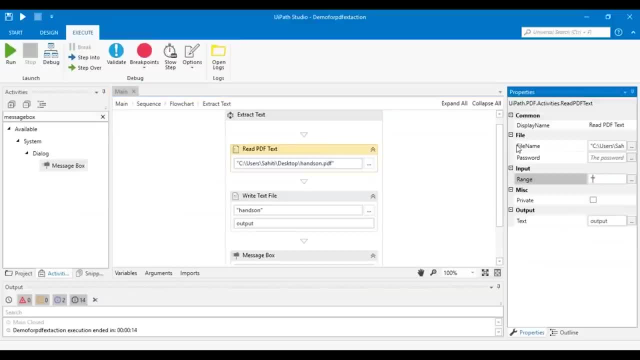 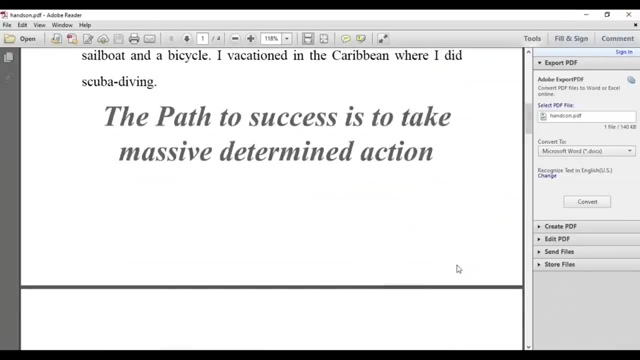 in the range section. What I'll do is I'll just mention one. Now I'm mentioning one over here. That's because you know our image is in the first page. So I'm just mentioning one so that we understand if the image is getting extracted or not. 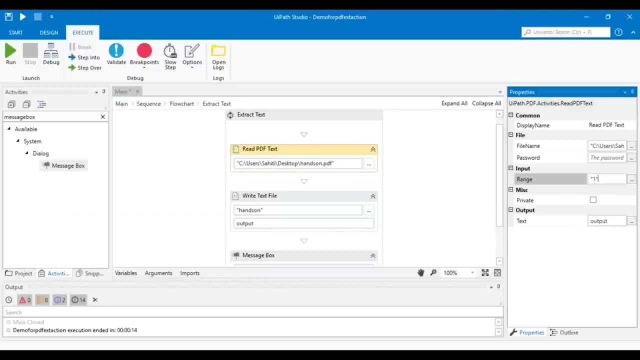 So all right Over here, Let me tell you one more thing. You can mention n number of pages that you want, Like initially I had mentioned all. that means all the pages in the PDF. Now I'm just mentioning the one. that means the first page. 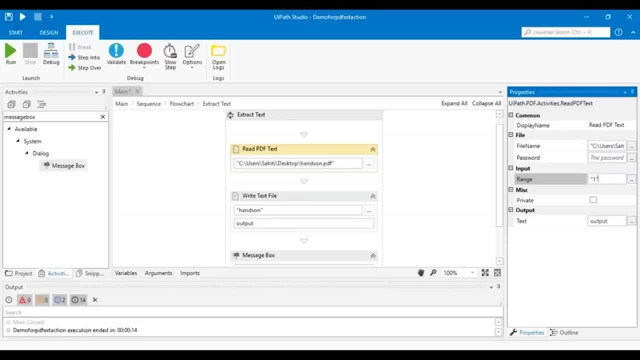 or you can also mention a range like 1 to 5 or 5 to all. that means, you know, from the fifth page it would get extracted to all the pages left in the PDF right. So that's how you can do. 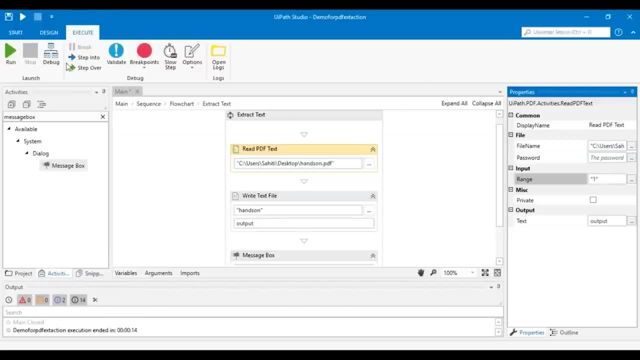 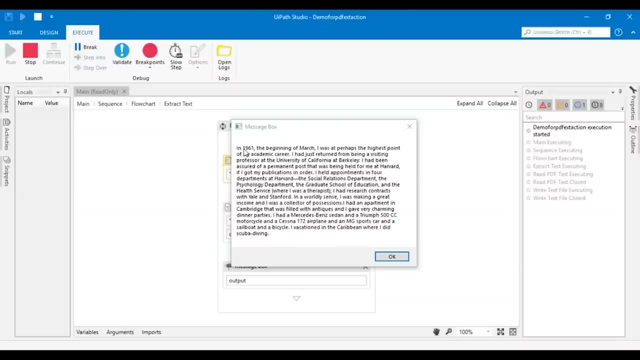 So I'm just mentioning one over here so that it's clear to us. Now I'll again click on debug to see the execution. All right, so you can clearly see in the message box that you know the data has got extracted. 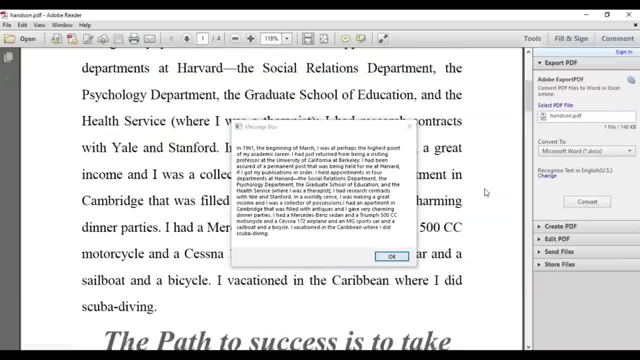 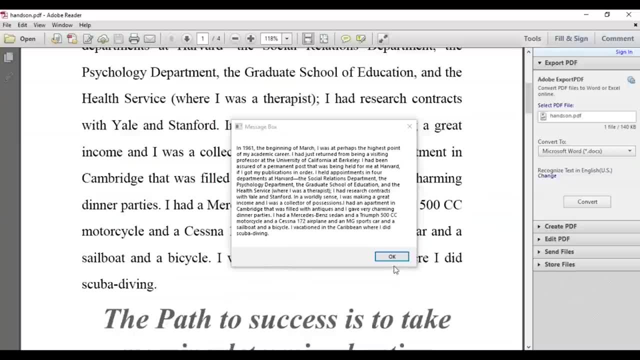 Let's just compare it with the PDF that we have, So you can see that you know our text has just got extracted and the image did not get extracted right. So that's how it's really clear that you know the image doesn't get extracted. 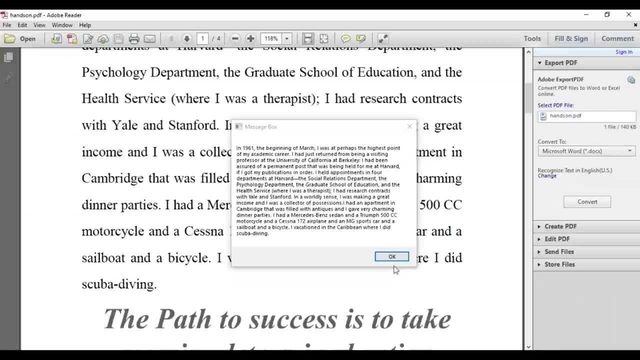 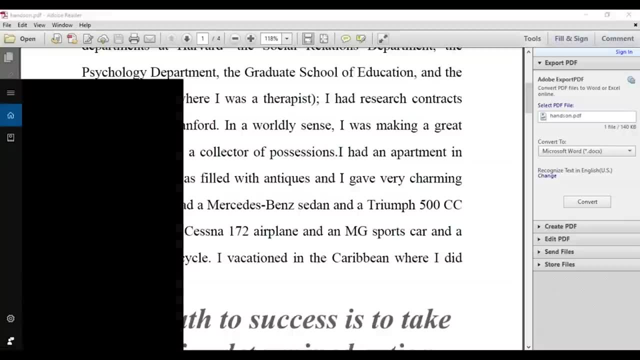 with the read PDF text activity. So, just in case, if you just have only text in your PDF, then I would suggest you can go for this particular activity. Now, apart from that, let's also see our hands-on file that we created, So I'll just search for hands-on. 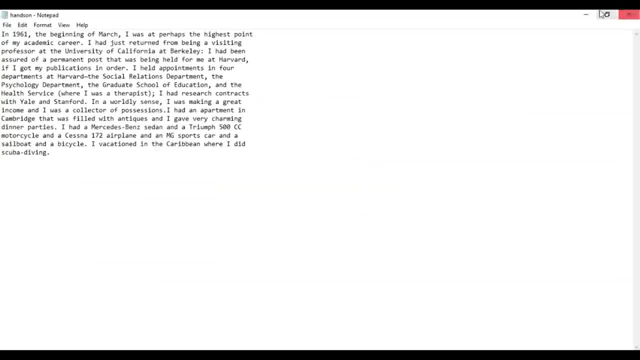 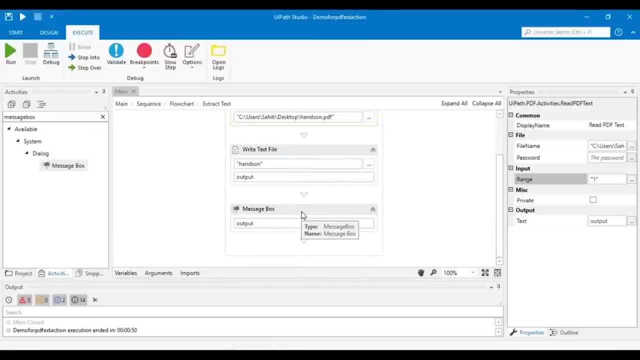 and you can clearly see that text has got extracted right. So that's how, guys, you can use this particular activity. Now, moving forward to the next activity, that is, the read PDF with OCR activity. What I'm going to do is I'm going to go back to the flowchart. 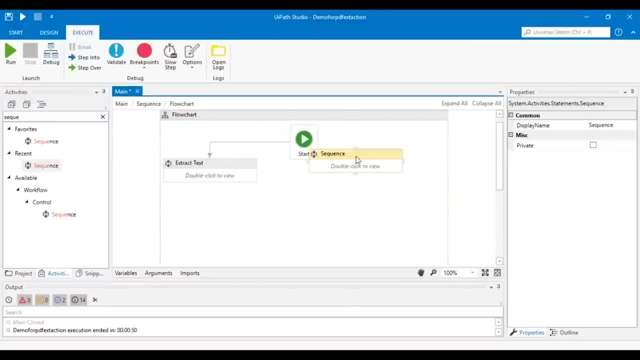 and over here I'm going to again drag and drop a sequence and then let's mention the name of the sequence to be extract images also, Right? so I'm going to just mention it to be extract images and I'm going to put the flowcharts arrow. 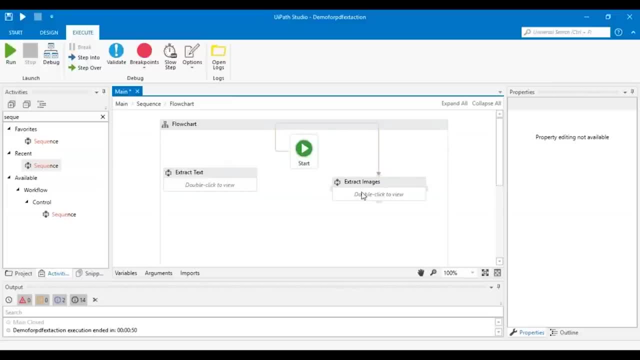 to be over here so that the execution starts from extract images. Now I'm going to double click over here, go to the sequence and then I'm going to drag the read PDF OCR activities. So I'm going to drag and drop it over here. 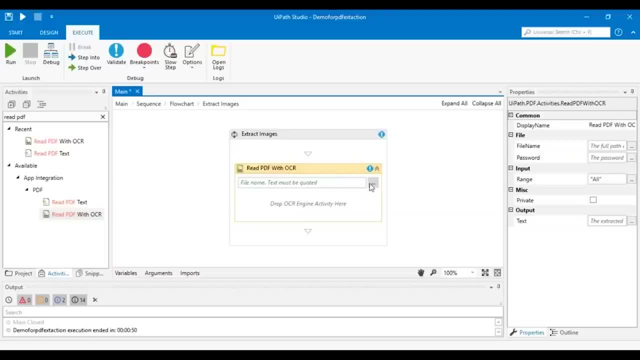 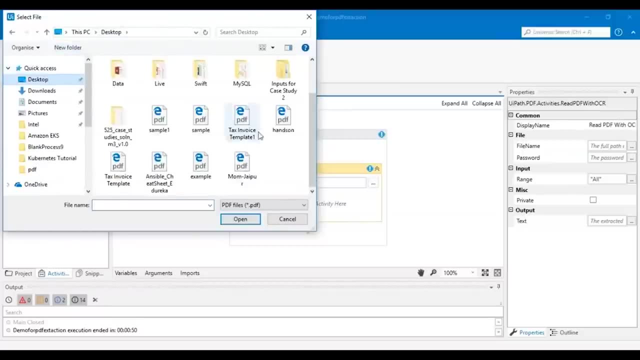 Now again, what I'm going to do is I'm going to mention the file part from which you know the data has to be extracted. So I'm going to mention the same file, that is, our hands-on file. So let me just quickly do that. 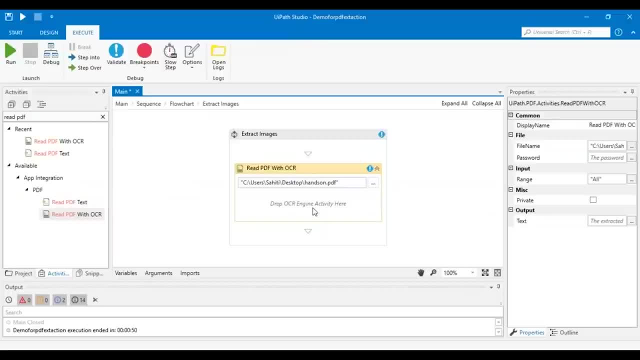 Right Now. one thing that I want to tell you over here is the read PDF with OCR: activity needs an OCR engine to execute this particular automation. So for that, what you can simply do is you can just search for OCR in your activity section and go to the engine section. 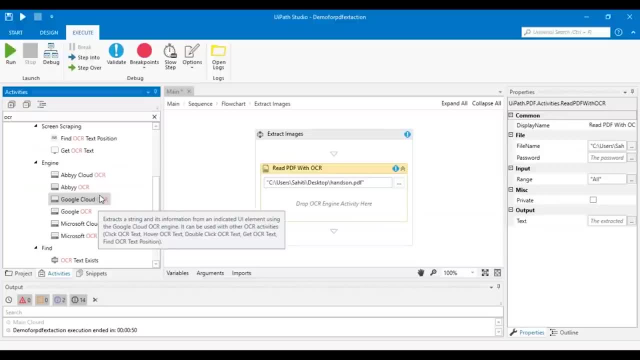 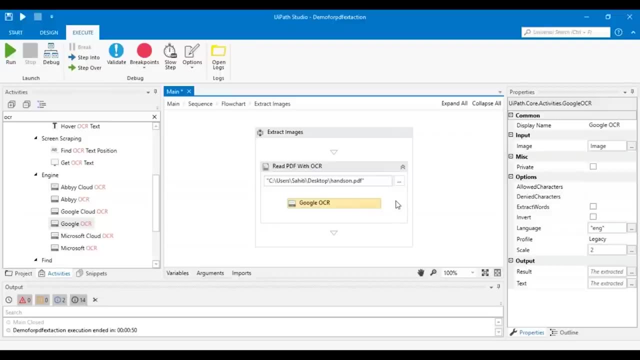 that you can see. over here You can see all the engines that you have installed on your UiPath, So I'm going to just use the Google OCR engine. So, as you can see in the properties section, every engine has its own parameters, like the allowed characters. 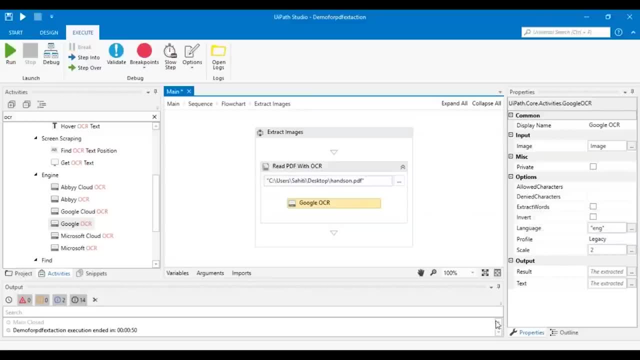 the denied characters, the exact words and word, language, profile and scale. Right Now, what I'm going to do is I'm going to just again use a message box and a write text activity so that we can see the output. So I'll just search for it. 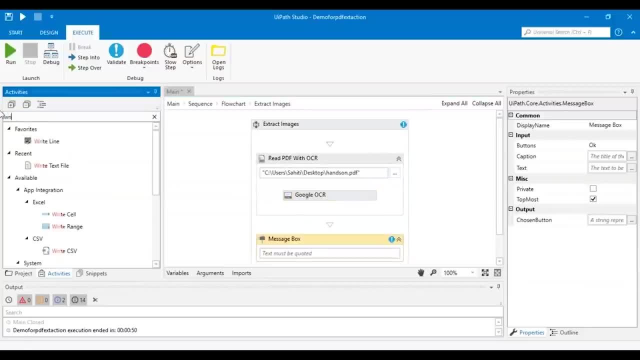 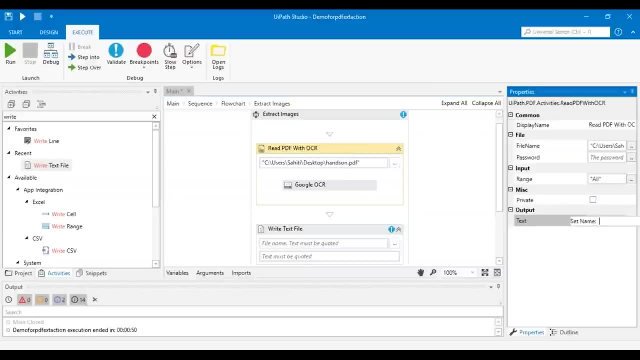 for message box and drag and drop it over here and also the write text activity. Right Now, in this particular section I'll mention the output variables. So for that again you can press on control K, mention output. that is basically the output variable, and then I'll use. 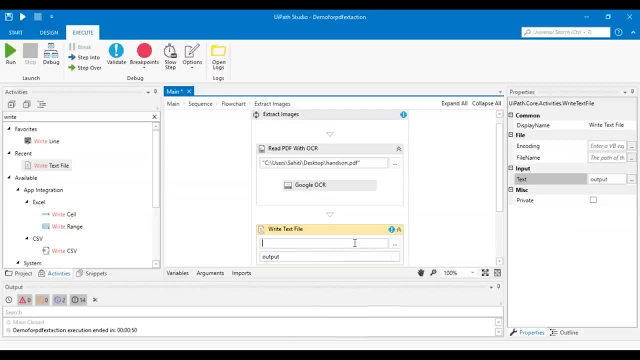 the output variable over here and mention the file name. So let's say, you know we mentioned the file name. to be hands-on too, Right Now. similarly, in the message box I'll mention the variable name Right. So that's how you can do. 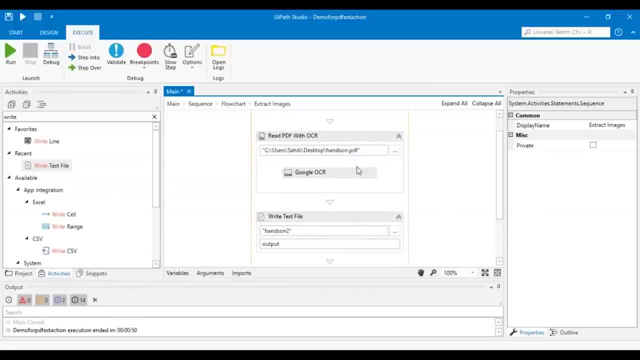 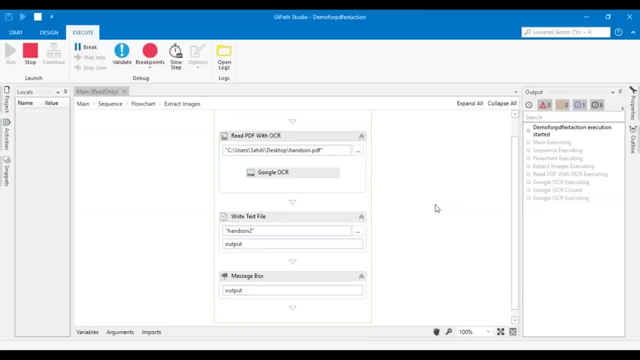 Now what I'll say is what I'll simply do is: I'll just execute this particular section so that you understand. So I'll click on debug. So on the right hand side you can see that you know the execution is happening. So once the execution is executed, 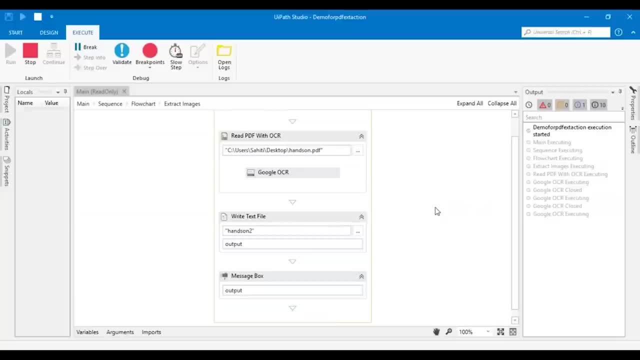 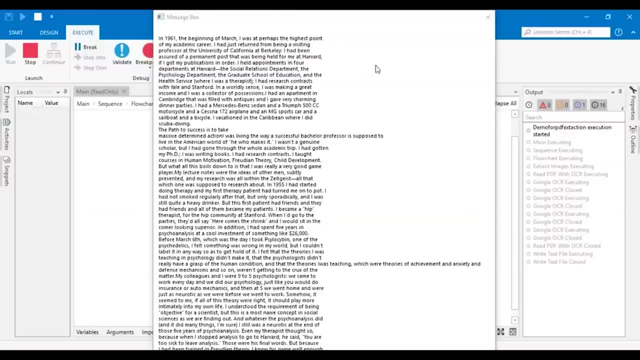 you'll see the output in the message box that you know. even this text from the image is getting extracted, All right. So again, what happened is our complete PDF got extracted. Now, to get a better understanding of what is getting extracted or not, I'll just go to the read PDF with OCR section again. 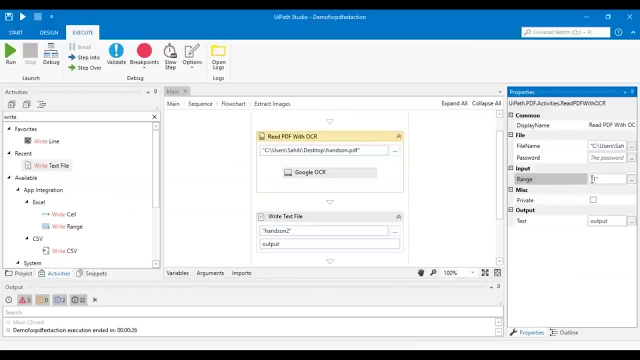 and mention the range to be one. That's because you know the images in the first page so you can play around it with it. So if you have the image in your 10th page, you can extract the data till the 10th page. 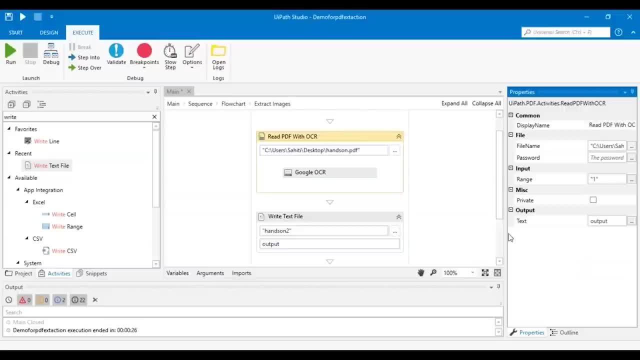 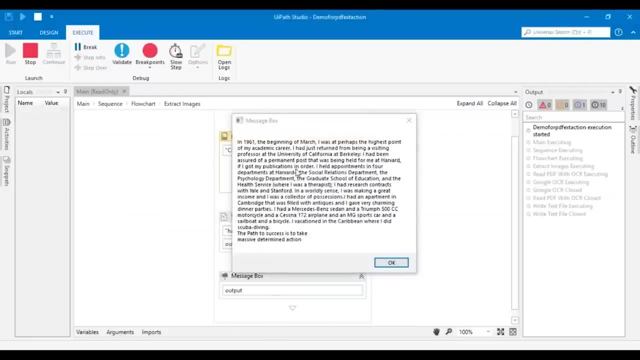 or you can just extract that particular page to understand the concept, Right? So I'm just going to mention this one over here and then I'm going to click on debug again. So, as you can see the output, the date has got extracted. Now let me just open our file and show you. 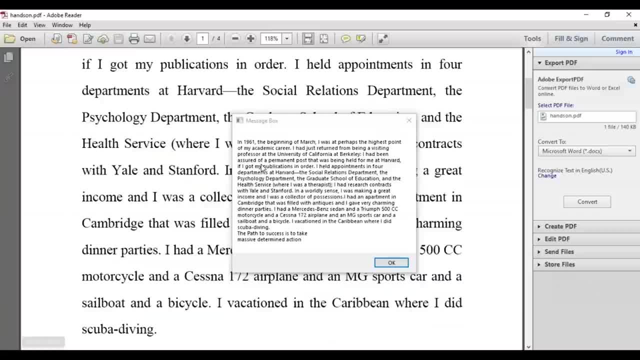 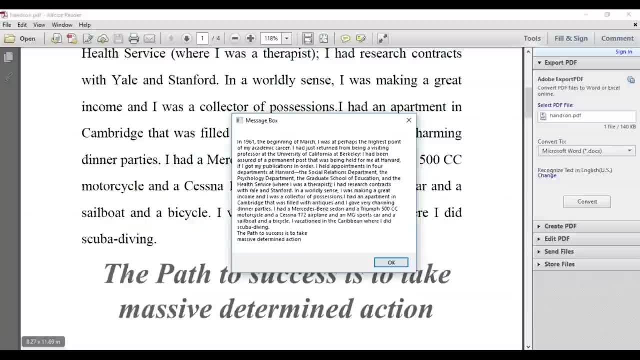 So, as you can see, in 1961 to scuba diving is our text which has got extracted, and also after that we had an image which says the part to success is to take massive, determined action. So that has also been converted to text and it has got extracted. 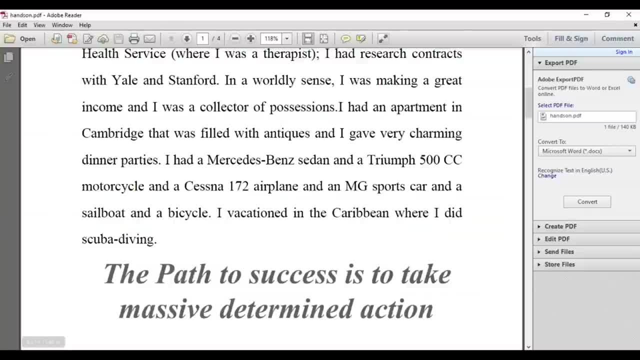 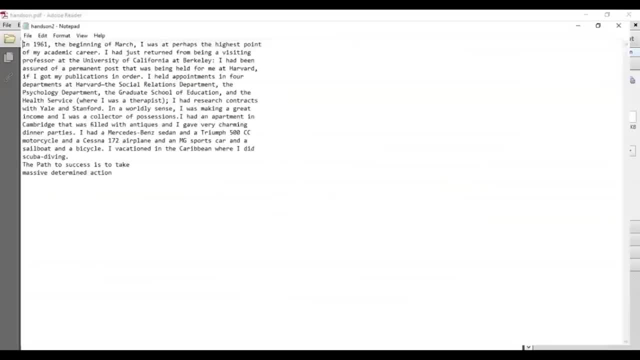 Right. So let me just quickly confirm this over the dry text activity also. So I'll just search for hands-on 2 and then I'll open it. So see the output. So if you see the output, you can clearly see that you know. 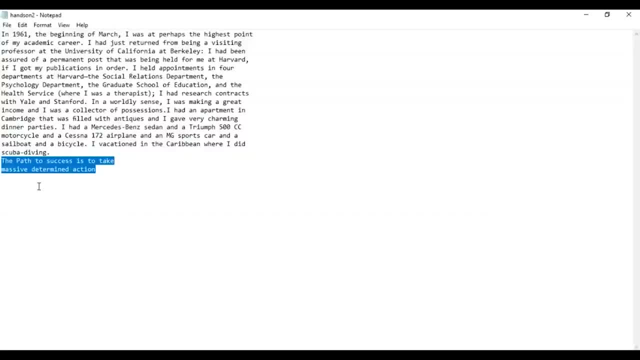 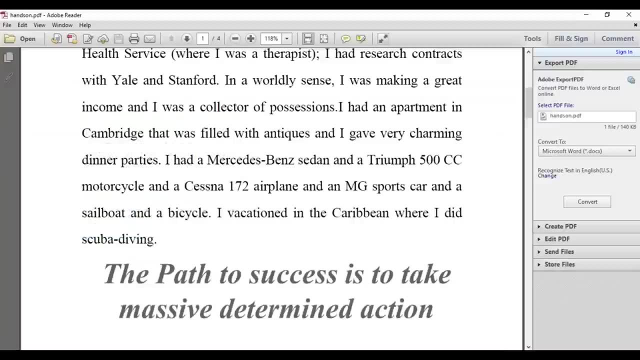 the part to success is to take massive, determined action. that is, which was an image, has also been extracted, Right? So that's how guys: PDF with OCR activity extracts both the image and the text. So, as its name suggests, this activity basically uses the optical character recognition. 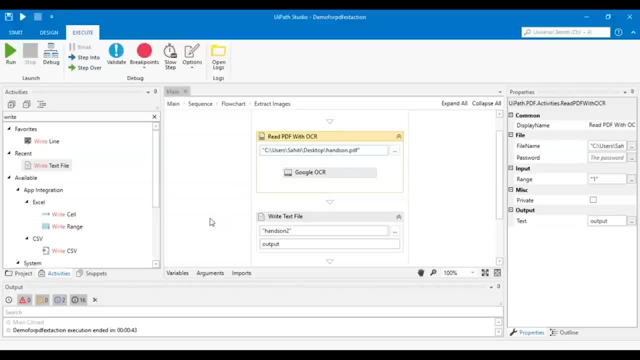 to scan the images inside the PDF document and then it outputs all the text as a variable that we mentioned over here. Right? So that's how you can use both these activities, guys. Now, before I close this section, let me tell you one more interesting thing over here. 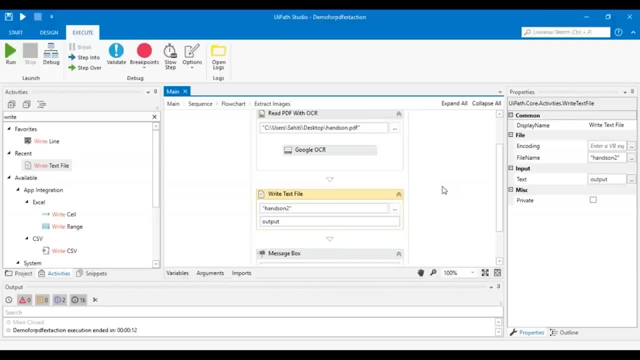 that is basically both the read PDF text activity and the read PDF with OCR activity are self-contained. So when I say self-contained, I mean that you don't need. the application is open, Right. So even if a PDF was closed and it was not open, 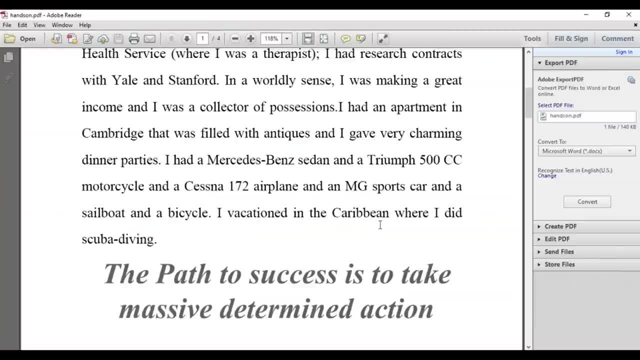 it will still extract the data from the PDF and would give the output Right. So that means you know both these activities can run in the background, which is one good plus point when you want to extract data Right. So now, apart from both these options, 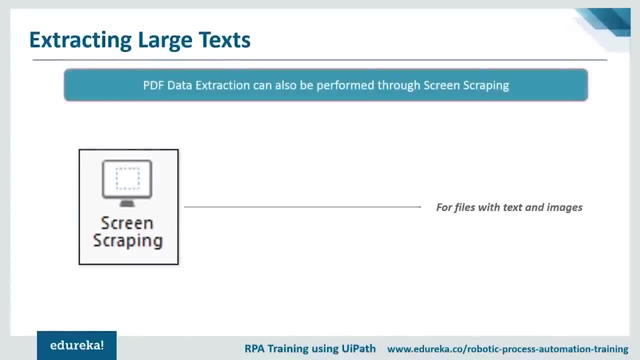 there's also one more interesting option, that is, using the screen scraping wizard. So you might be wondering, right, how you can use the screen scraping wizard, So whenever you want to scrape the data from your image or you want to scrape the data from text or any particular document. 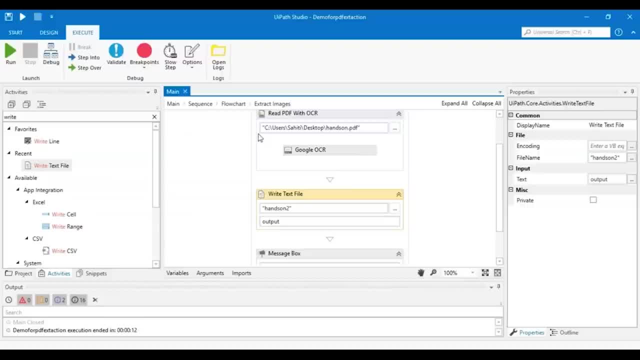 you can just use the screen scraping wizard. So if you open your UiPath tool, you can clearly see that you know you find your screen scraping wizard in the design tab of ribbon and that's how you can use the screen scraping. So I'm going to show you how you can do that. 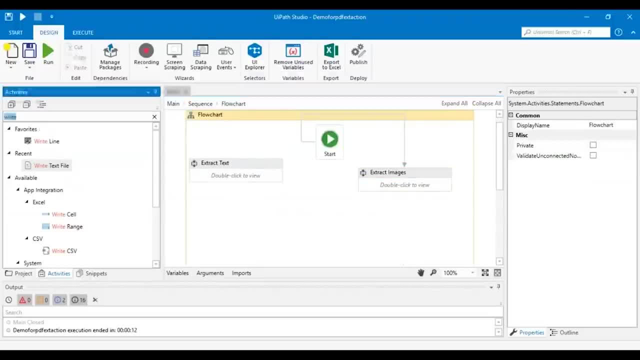 So I'll again go to the flow chart. I'll just create a new sequence and let's say, you know, I rename it to screen scraping and then I'll connect the start node to the screen scraping sequence. So I'll double click over here. 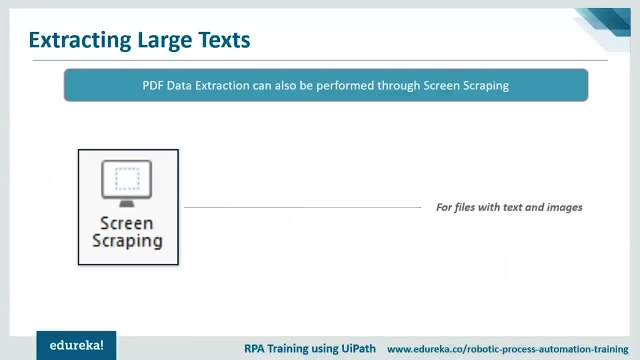 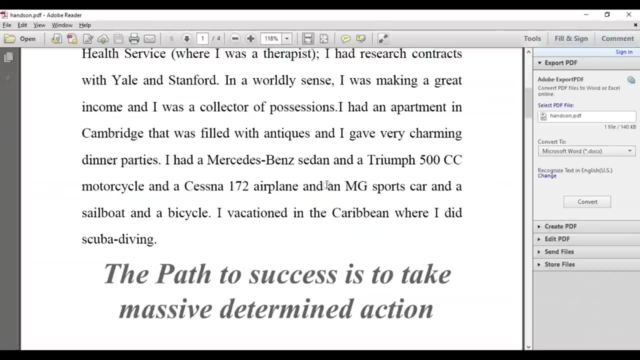 and now what I'll do is I'll just click on the screen scraping, and then I can scrape whatever text that I want, Right? So what I'll simply do is I'll open my PDF, All right, and then I'll go back to UiPath tool. 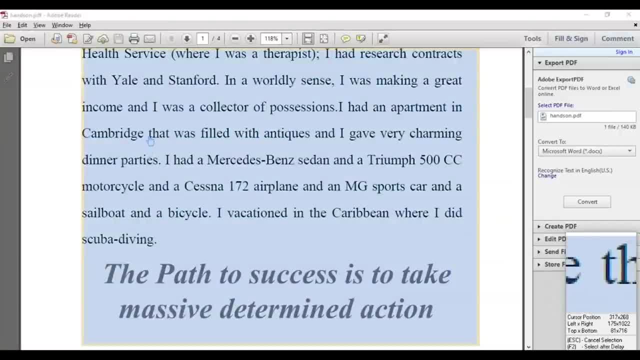 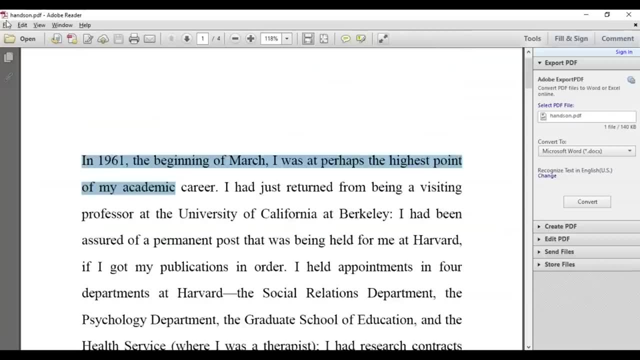 I'll choose screen scraping and then I can mention whatever I want to scrape. Now, before I start scraping, let me tell you that you know it's always good practice that you mention your PDF document in the actual size, For that you go to zoom. 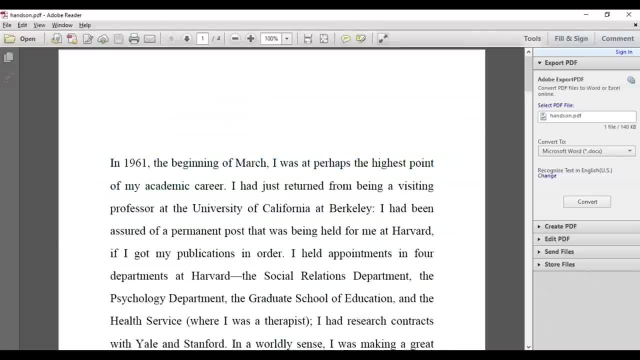 and fix this to actual size. Right Now let's go back to UiPath tool, Click on screen scraping and then we'll mention whatever we want to scrape, Right? So I'll click this particular section So you can see that. 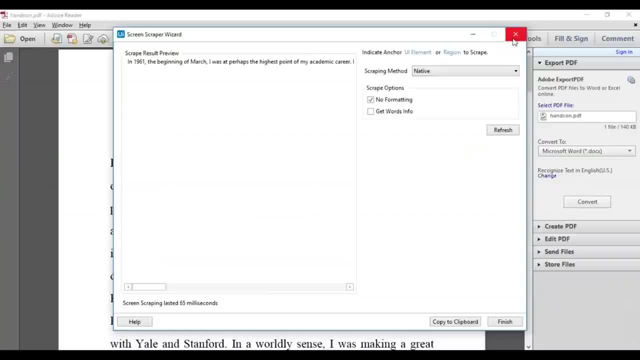 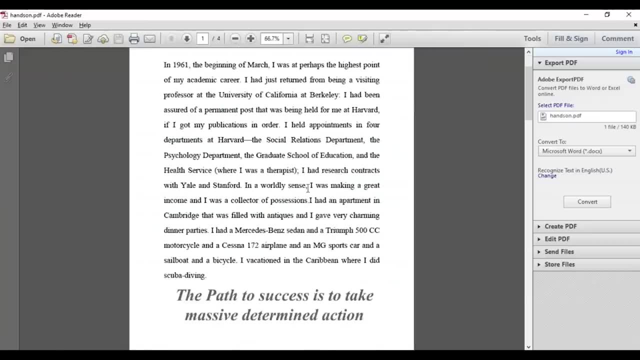 you know this particular section got scraped Else. if we also want to scrape again, you can just, you know, close this particular section again and then mention whatever you want to scrape. So I'll just zoom out and let's see. 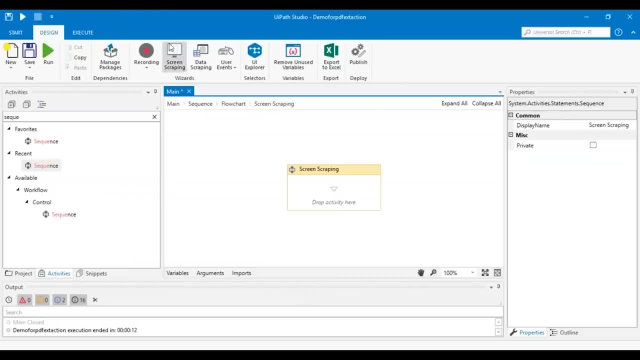 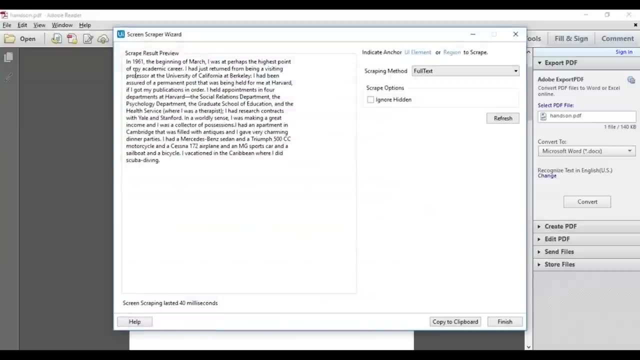 We're going to scrape the complete first page, Right? So I'll go back to screen scraping. I'll choose the complete section that is from here to here. So I'll just drag and it opens up preview window If you're scraping for the first time. 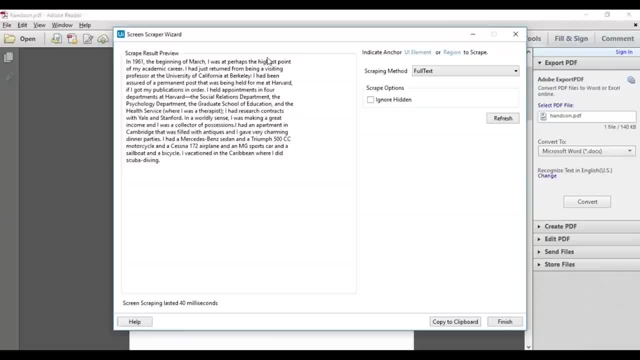 let me tell you that you know these are the ways option that the screen scraping wizard offers in the preview window. So this is basically the screen scraping preview wizard that you can see. So on the left hand side, that is basically the scrape result preview. 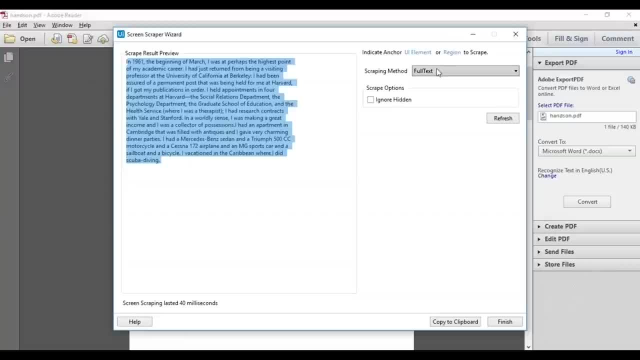 So whatever has been scraped, So this is completely based on the scraping method. So since it was full text, only our text got scraped. Now, if I change it to OCR, you can see that. you know, the OCR engine is Google OCR. 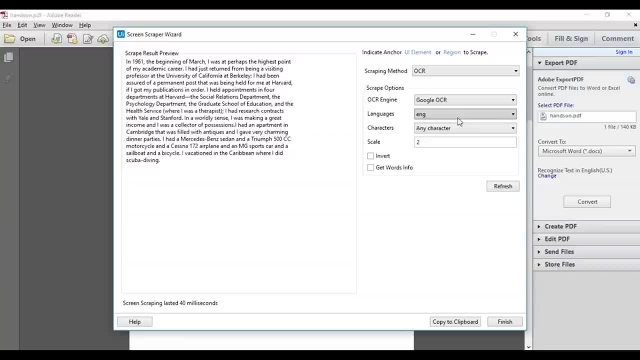 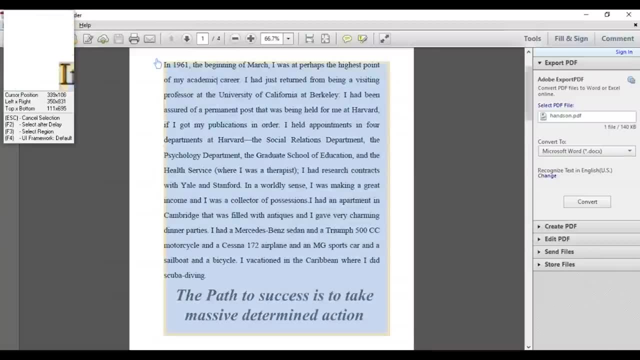 Languages could be whatever language that you want to mention. Characters: I've mentioned any characters and scale. Now again, if I want to scrape again, what I'll do is I'll again go to UI element and then I'll choose the complete section. 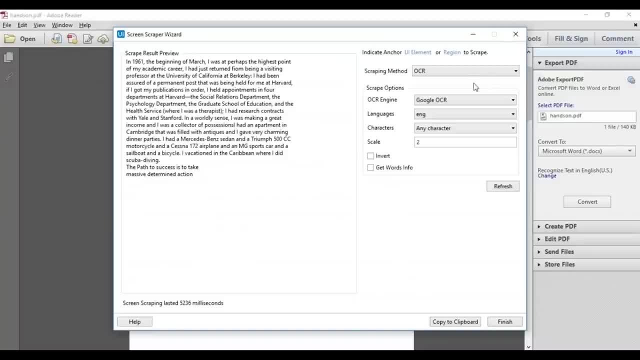 All right. When I choose the complete section again and when I choose OCR, you can clearly see that you know the image is also got extracted. So that was about the preview of the screen scraper wizard guys. So now, once you're done dealing, 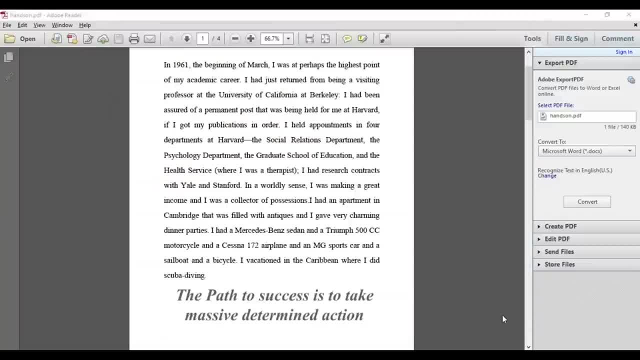 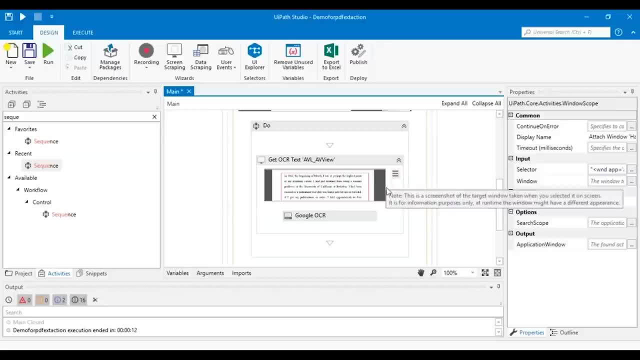 with all these properties. you can just click on finish and this will redirect you to this particular window, So you can see that you know we've got attached window do and whatever has to be scraped, right? So since we have chosen the OCR engine, 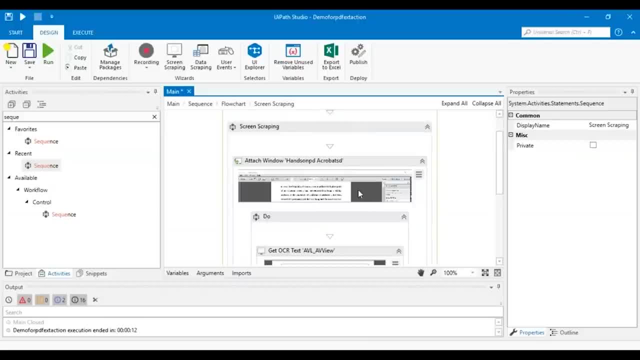 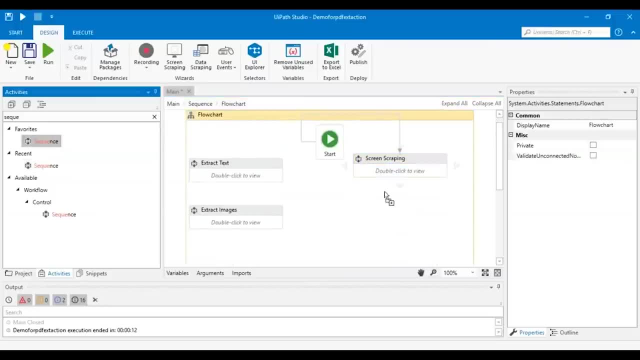 we've got the workflow like this Instead. if we would have chosen the scraping method to be full text, we would have got the workflow different. So let me just quickly do that part also. So I'll again create a new sequence and let's just quickly go into that. 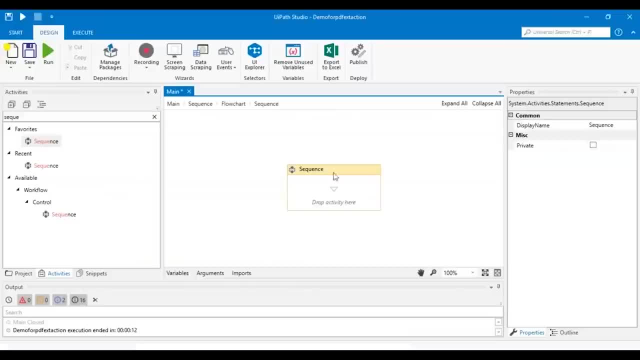 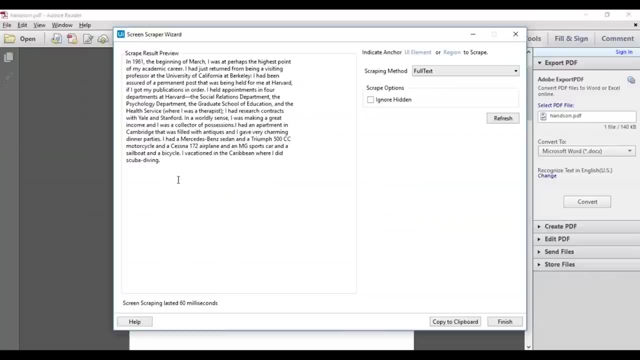 and then I'll choose for screen scraping. So let me just open my PDF and then I'll choose this particular section again and then I'll choose full text. That means you can clearly see that your screen, you know, your image- is not got extracted. 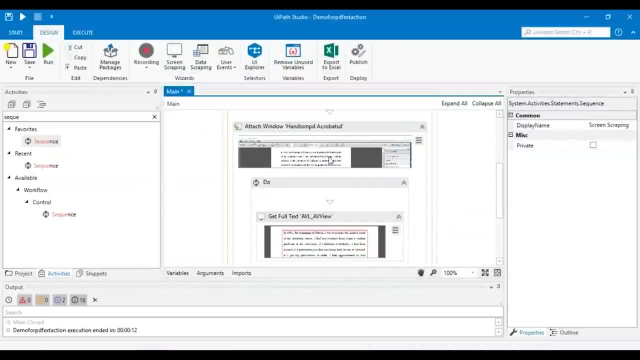 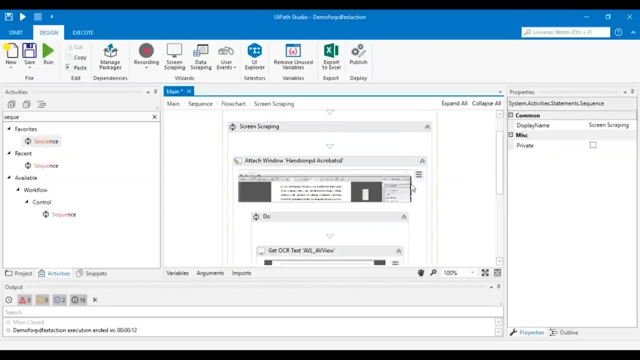 After that I'll click on finish. So this will basically redirect me to this particular full text screen scraping workflow. So it's clear that you know you don't find your OCR engine here, right? So what I'm going to do is: 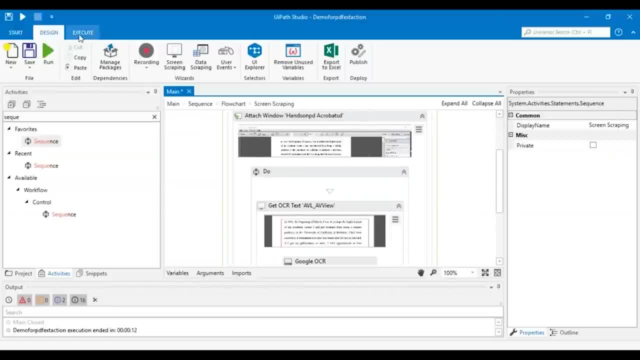 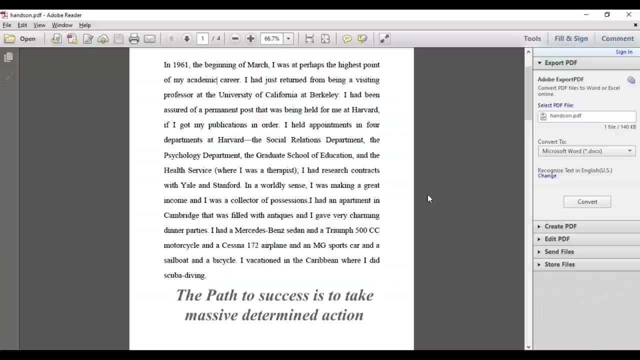 I'm going to just run this particular workflow, that is basically the OCR one, and I'll click on D bar and you can clearly see that you know your data is getting scraped right Now. obviously we cannot see the output because we have not mentioned. 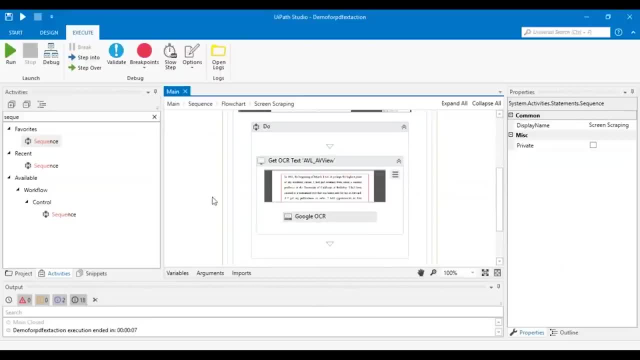 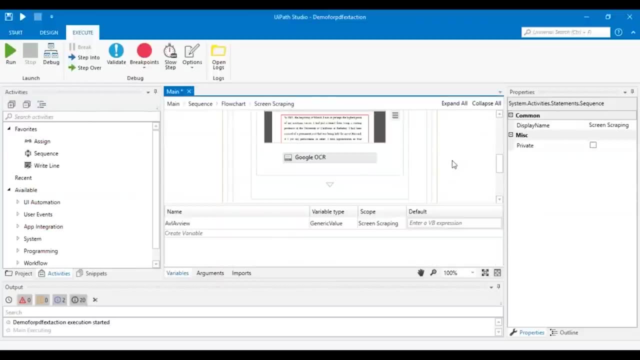 any message box or a write text file. So for that what we can simply do is let's just mention a message box so that you know we see the output. So once you add a message box, whatever output variable was generated in, get OCR text. 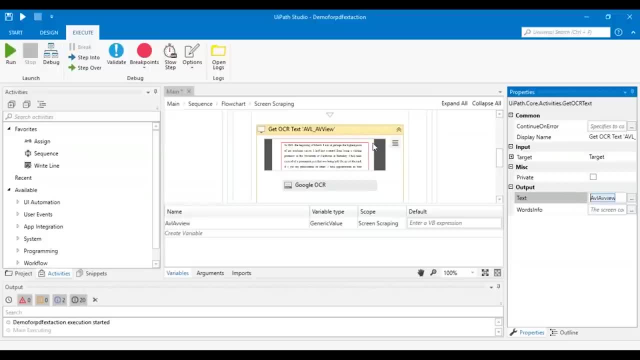 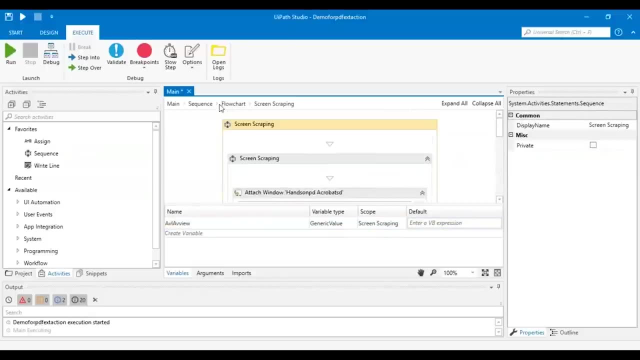 that is basically the AVL AVV view over here. So I'll just copy that and then I'll paste it over here And what I'll do is I'll change the scope to screen scraping. That is basically the complete sequence, right? 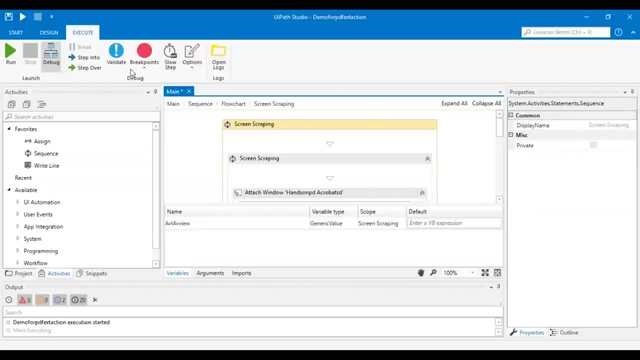 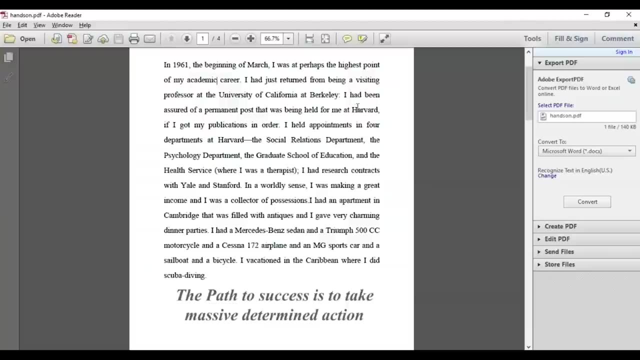 So you have to change the scope for the variable Now, once you're done with that, you can just click on debug and let's just wait for it to run All right, so you can see that you know it's getting extracted. 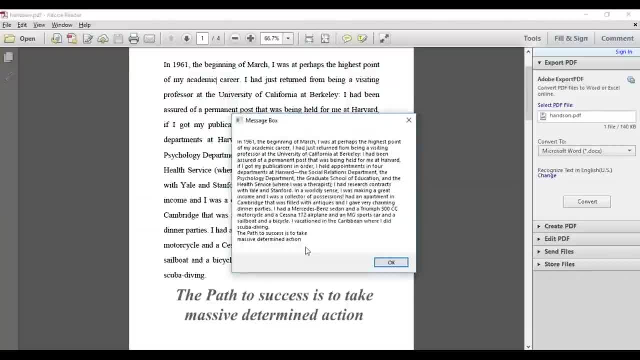 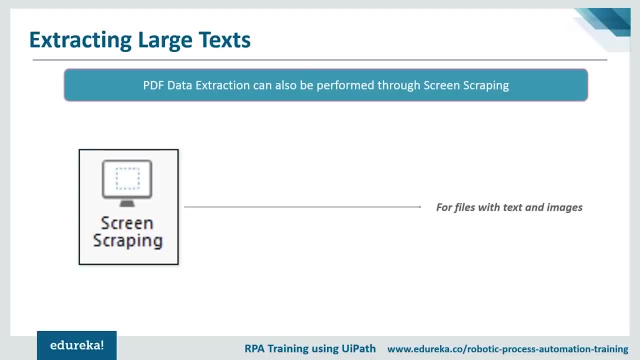 and now you'll see an output of the message box, of all the text, right? So, as you can see the complete text and also the image has got extracted right. So, guys, that's how you can use the screen scraping wizard. 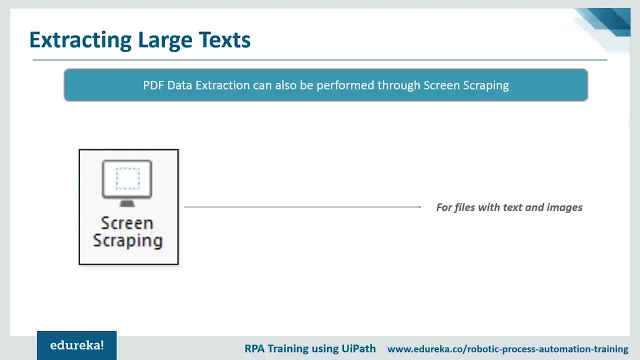 So this was also one way to extract large text, guys. So basically, as I mentioned, there are mainly three ways through which you can extract the last text, That is, the read PDF activity, the read PDF with OCR activity and the screen scraping wizard. 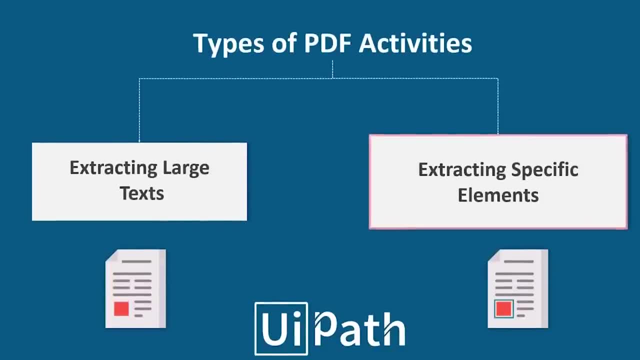 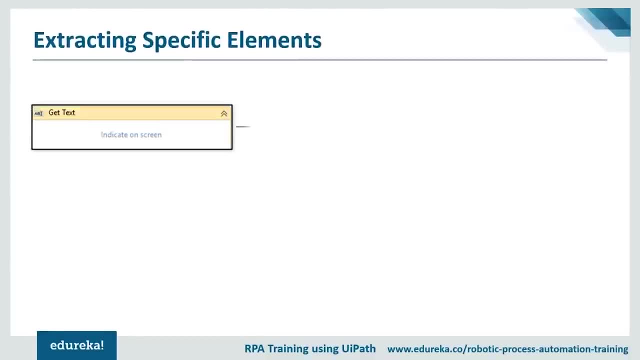 Now let's move to the next type of PDF activities, that is, to extract specific elements. So when you want to extract specific elements, there are again mainly two types of activities that you can use, That is, the get text activity and the anchor based activities. 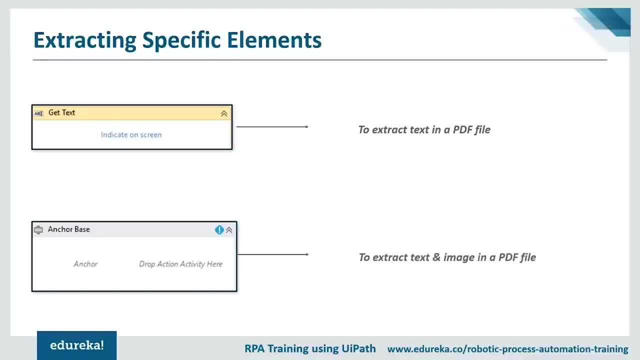 So the get text activities are basically used to extract the text in the PDF file, and the anchor based activities are again used to extract the text and the images in the PDF file. So initially I'm going to show you how you can use the get text activity. 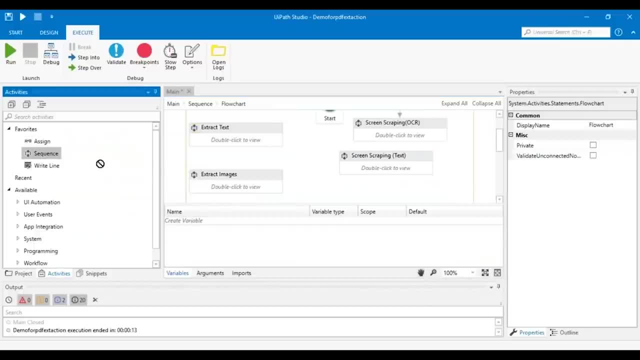 So let me just quickly shift back to my UI path, Then I'll again show you how you can add a new sequence. And let's say, you know we rename it to get text activity. So for that I'll just mention: extract specific elements. 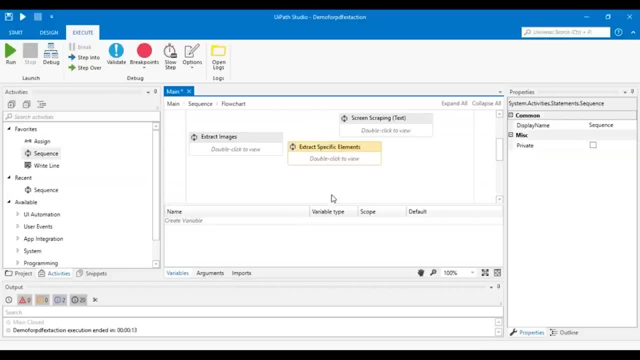 And what I'll do is I'll open this and now I'll add the get text activity, So I'll search for get text and then I'll drag and drop it over here. Let me tell you that you know your PDF, from which you want. 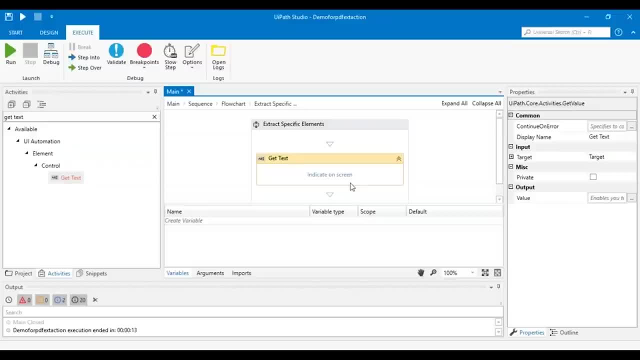 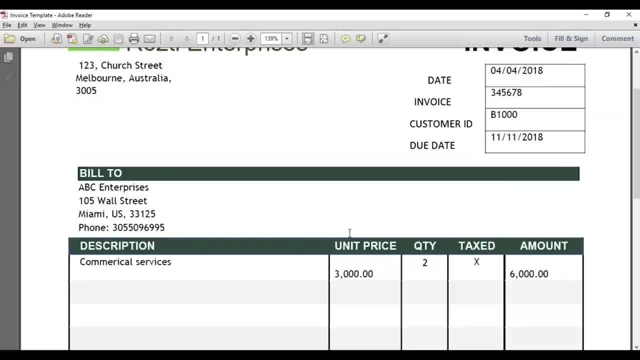 to extract any particular data or any particular text has to be opened. So for that purpose, what I've done is I've added the get text activity and then I've created a sample invoice to which I'm going to extract specific elements. So let me just shift. 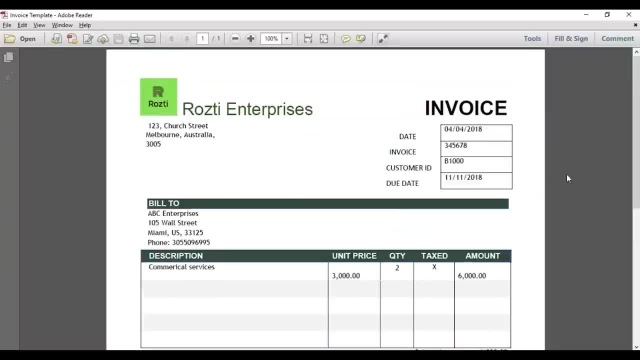 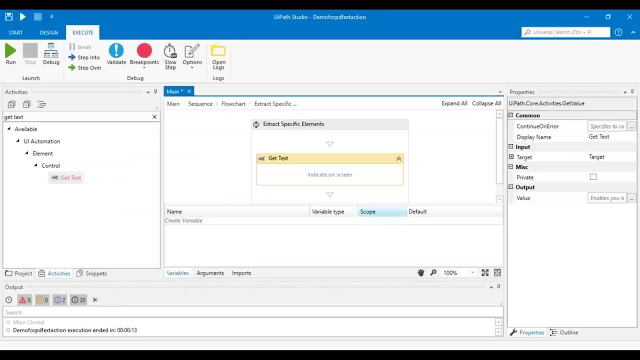 back to actual size So that you can see. So we have date, invoice, customer ID and the total amount and the tax due, right? So now I'm going to shift back to my UI path and then I'm going to indicate on the screen. 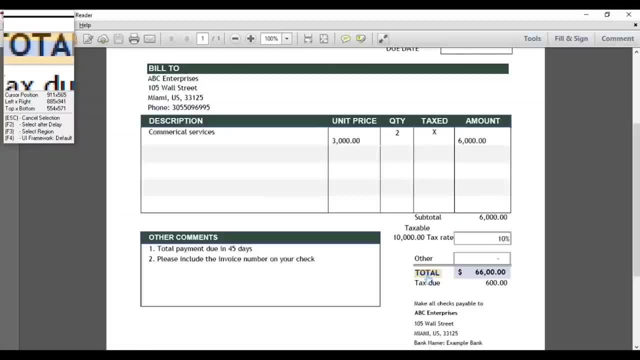 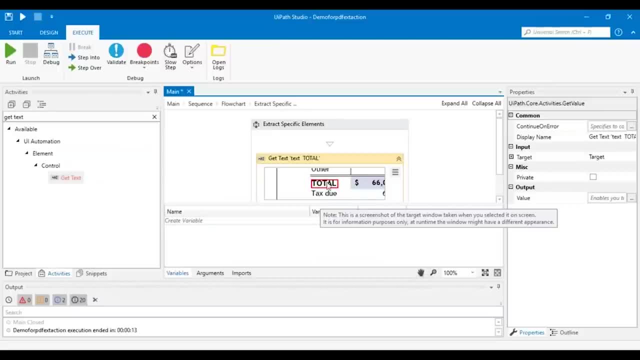 So, as you can see, we can indicate anything. So let's say, you know I'm going to indicate total, right, So I'll just choose this total and you will clearly see that you know this particular section has got indicated. 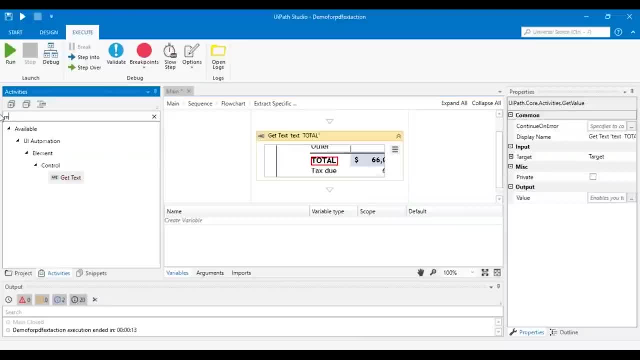 right. So now, if you want to- just you know- get the output, you can just search for message walk and I'll create a variable for the output. So I'll click on control K, mention output and then over here again, I'll mention output. 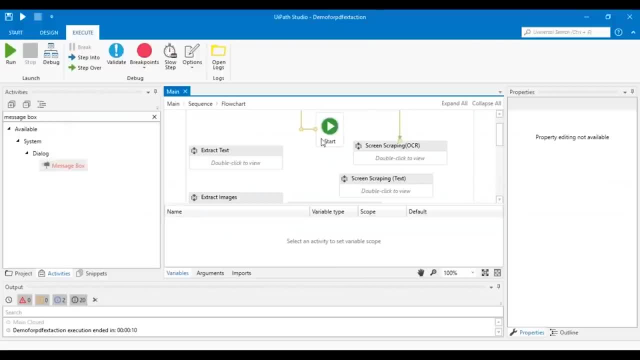 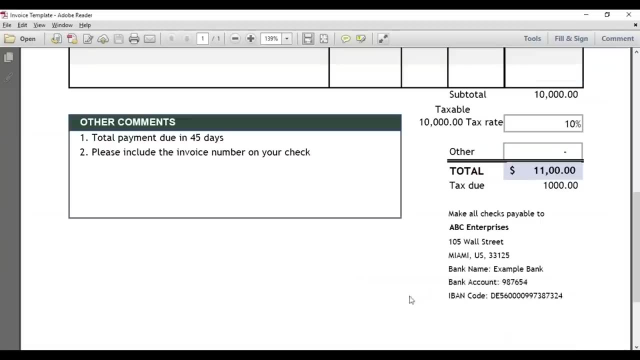 So let me just quickly change the workflow to the extract specific elements so that the start node is connected over here. Now let me just quickly click on debug. So before that, make sure that you know your invoice is open, right. 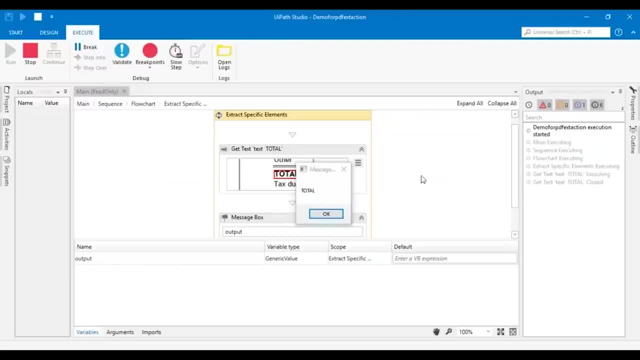 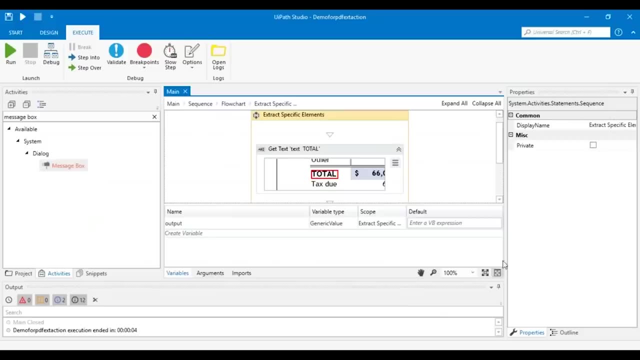 So UI path and then I'll click on debug and you can see that. you know you've got the message total, So to make it more app, let me just extract the total value, that is, the 6600 that you see. So I'll go to this. 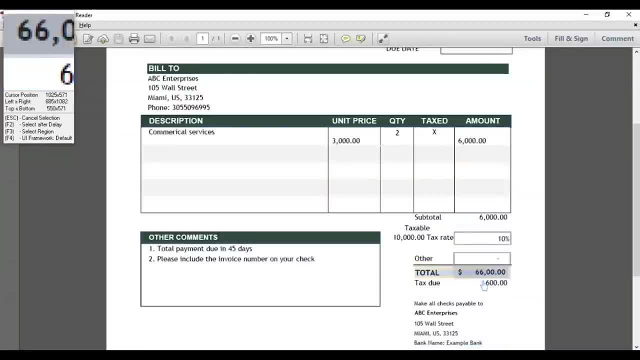 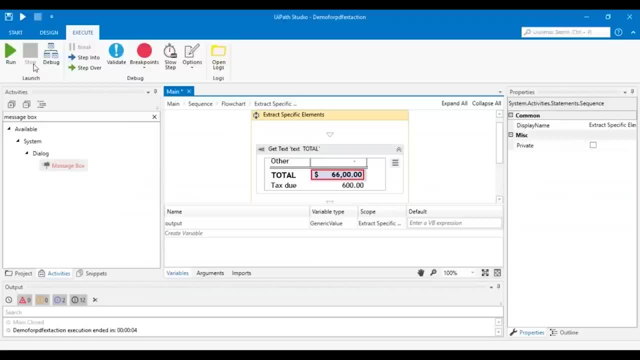 particular option over here. I'll again click on indicate screen and then I'll choose this particular section right, So you'll clearly see that you know this particular value would be extracted. Now I'll again click on debug to show you. 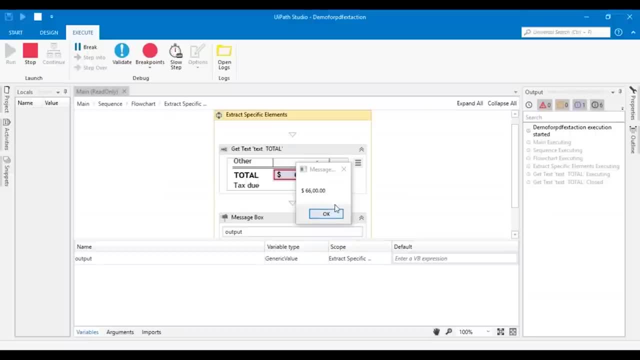 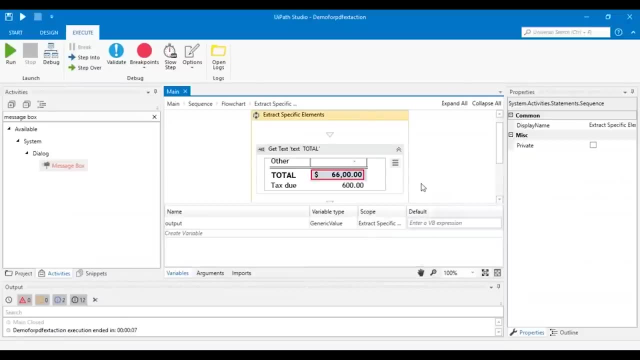 So once you click on debug you can clearly see that you know this particular value has got extracted right. So if you clearly observe this is generally used to, you know get the text value or to just extract the specific element. 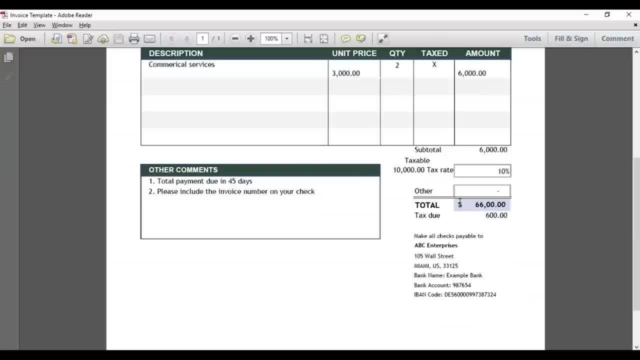 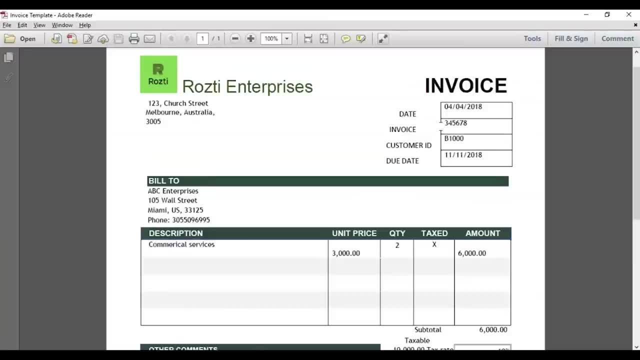 So in the complete invoice that you had you can extract anything that you want. I extracted this particular section so you can either extract the other comment section or the name of the company or the date, the invoice number, the customer ID or due date. 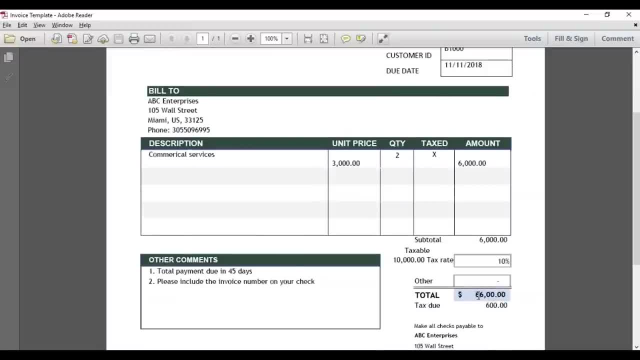 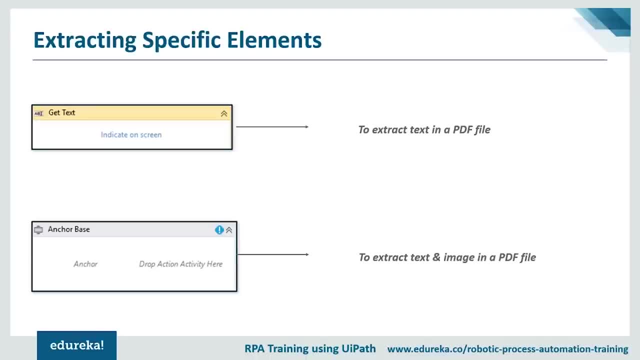 or any other such parameter right. So, for the demonstration purposes, I've just extracted this particular section. So that was about it. Now moving on to the next type of activity, that is, the anchor-based activity. So, as I mentioned before, the anchor-based activity. 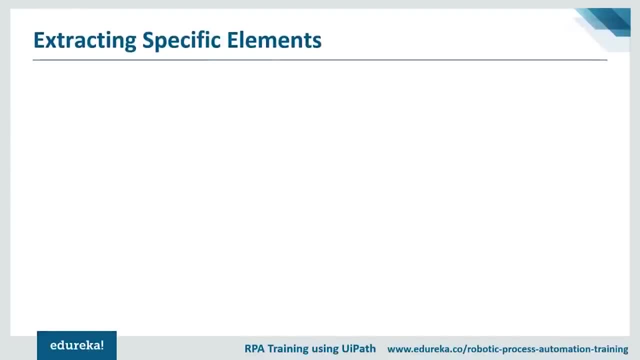 is basically used to extract the text and the images in the PDF file. So the anchor-based activity basically has two sections. that is basically the anchor and to drop the action activity here. So when I say anchor in the anchor, you can either use the find element activity. 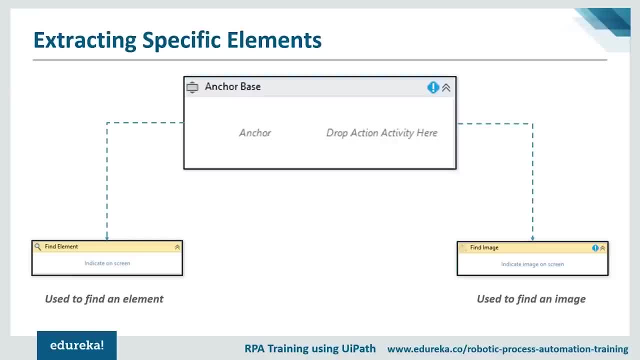 or the find image activity. Now, the find element activity is basically used to find any element and the find image activity is specifically used to find the image. and the drop action activity over here is basically what you want: to give an idea of where the activity is. 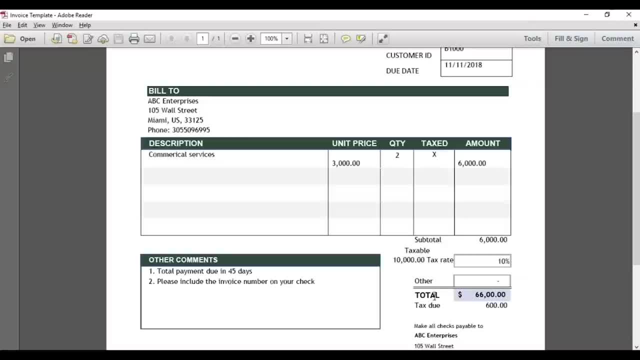 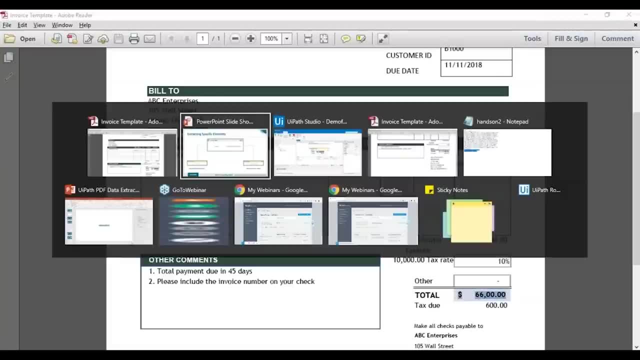 right. So suppose in our invoice example what we can do is we can use the find element activity to get the total and the get text activity to extract this particular value, right? So I'm going to show you that how that's happening. 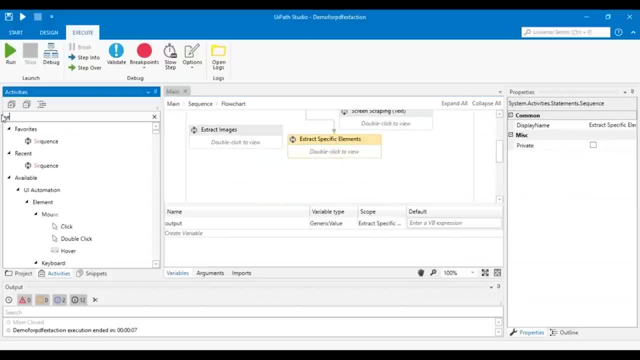 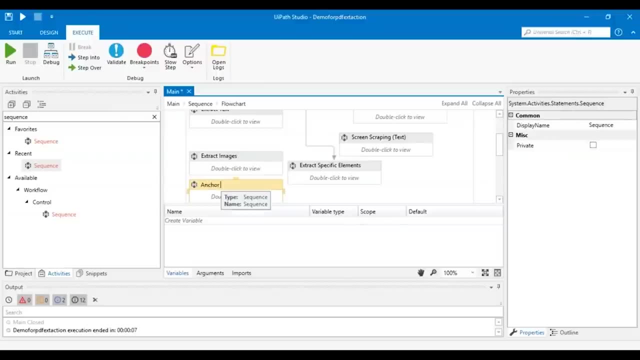 So what I'll do is I'll again go back to flow chart and let's just quickly create a new sequence, and then I'll just rename this particular sequence to anchor example Right, And now I'll just put the start note to this particular activity. 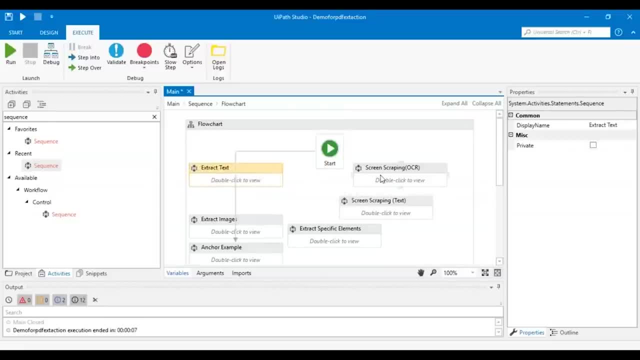 And let me just quickly arrange them so that you have a clear understanding. So we started with extract text and extract images and we did screen scraping. that is, screen scraping text, and now we're doing anchor. right, So I'll just do anchor. So I'm just going to open. 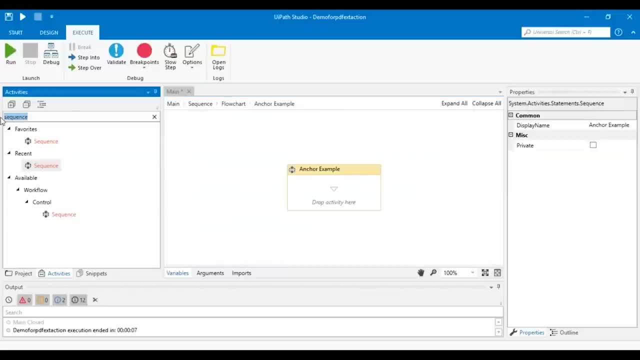 this particular sequence. and now what I'll do is I'll drag an anchor based activity. So I'll just type in the search box for anchor and you'll see that you know you can drag and drop this anchor base. Now what you can do is: 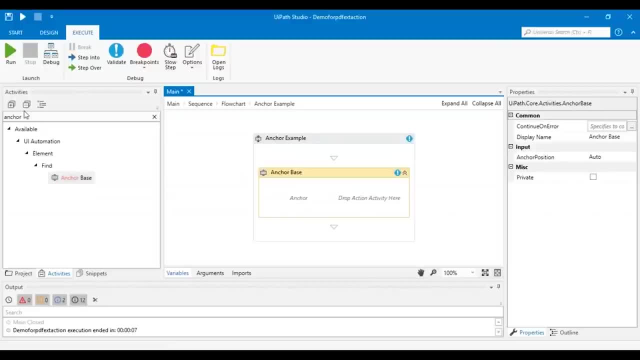 you can drag two activities, that is, the anchor and the drop action, over here. So initially I'm going to drag and drop the find element activity. So I'll search for find and you can see that you know you can drag and drop. 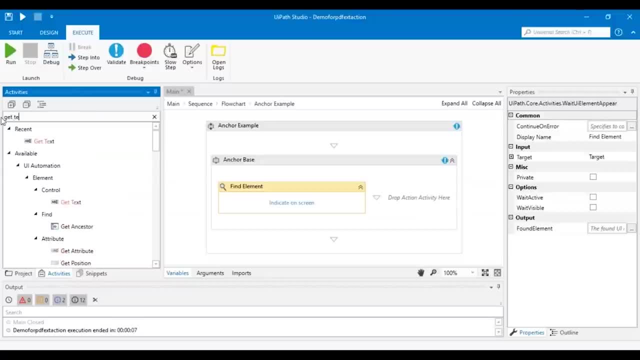 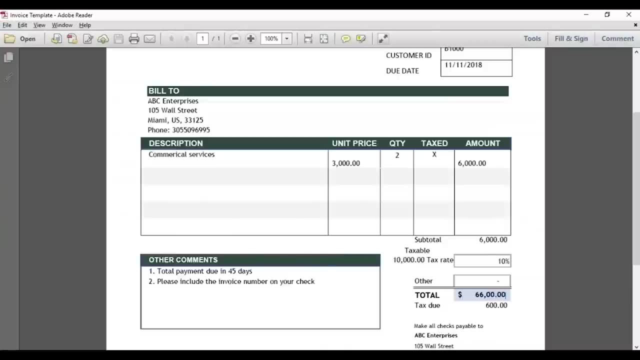 this particular activity And then, on the right hand side, I'm going to drag the get text activity. So let me make sure that you know my PDF files are open. All right, So they're open. Now what I'll simply do is: 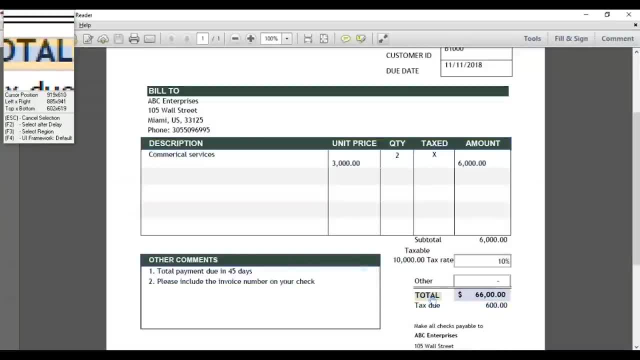 I'll just go to find element activity. I'll indicate on the screen. So let's say total is what I want to find, and then in the get text activity I just hold my mouse over the 6600 over here. So apart from that, 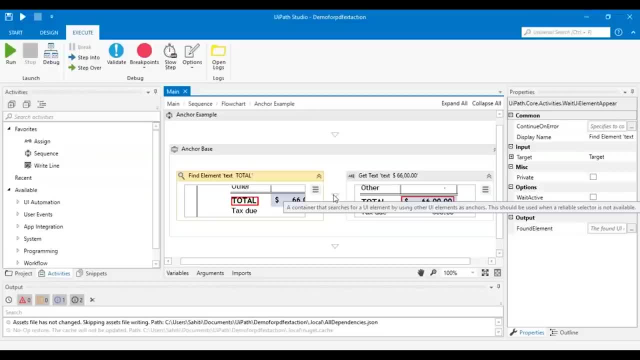 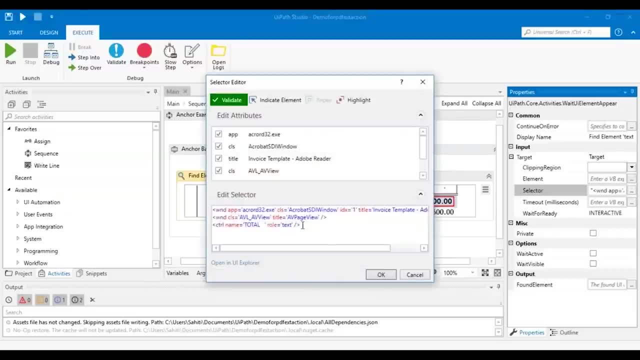 let me tell you one more thing over here, that is, you know you can play around with the selector. So if you just go to the target section and then if you choose the selectors, you can clearly see that you know you can change as per your need. 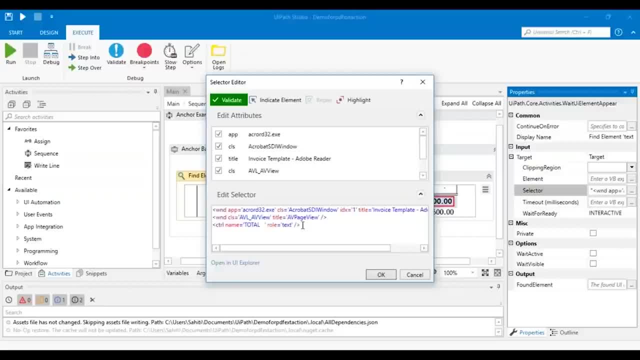 So if you just want to scan across various PDFs and going to extract the same values, then you can also indicate the elements and play with the selectors. Well, I'm going to leave that part for you so that you guys can explore how you can do it. 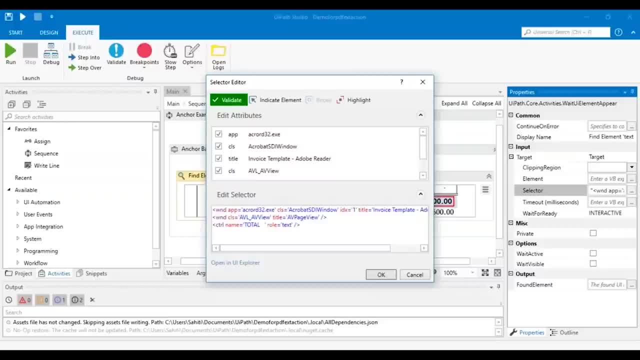 And if you don't get how to do that, please let me know in the comments section and I'll tell you how you can do that. So now let me just quickly, you know, add a message box over here so that we can see the output. 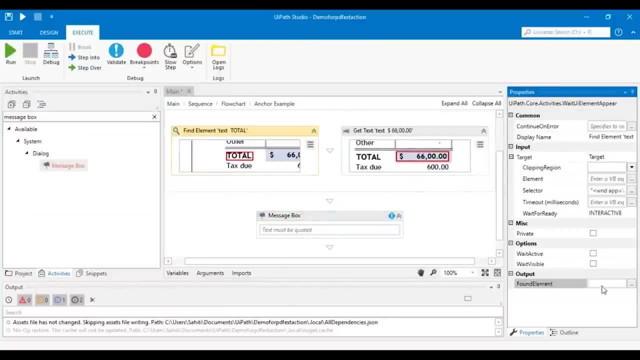 So I'll just search for message box. So in the section what I'll do is I'll just mention the output variable. So let's say we mentioned the output variable to be output and then in the section I'll mention the output variable. 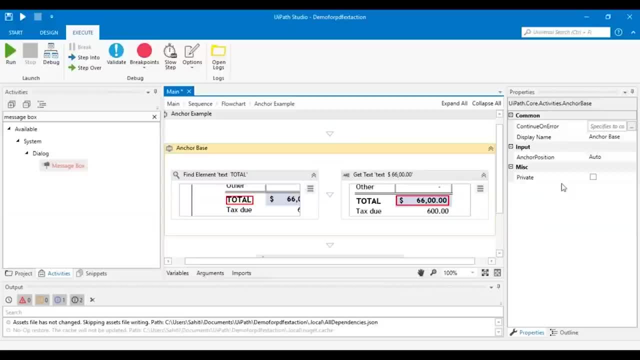 Now one more thing I like to tell you over here is that in the anchor base activity, if you see in the input you can see the anchor position right. So whatever text that you want to extract, you can mention the anchor. So for example: 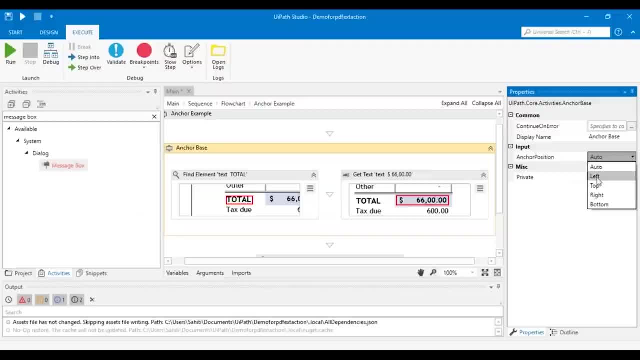 over here. we're using the auto. that is by the default. but yes, you can mention the left top, right bottom. So if you have your anchor on left, then what text that you want to extract which is on the left side? 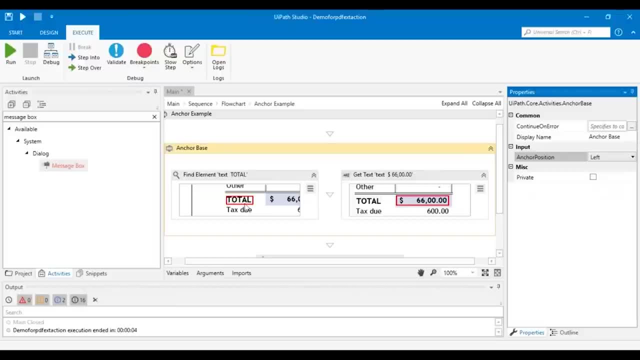 on the right side you can mention like that. I'm going to just mention left. that is because you know the anchor that we have mentioned: total. it is on the left side of whatever value that we want to extract. That is over here. 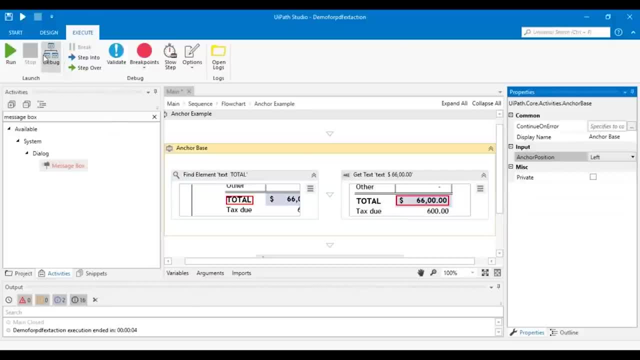 That is 6600.. So I'm going to just mention left over here and then I'm going to click on debug. So once you click on debug it's clearly seen that you know the output is 6600. That is you know. 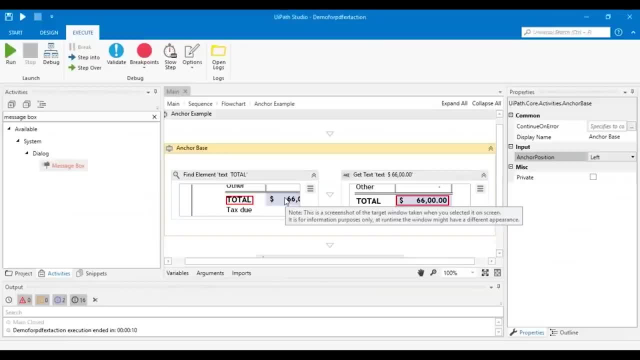 data has got extracted right. So that's how you can use the find element activity to get whatever you want to a specific element or at a specific position. Similarly, you can use the find image activity. So if you just search for the find image activity, 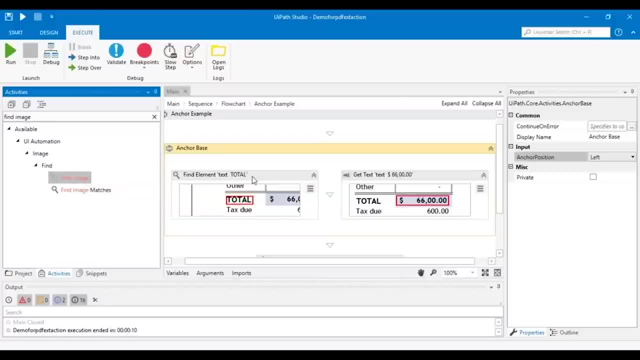 you just get this particular activity. You can just drag and drop it over here in this particular section. So I'm going to click on find image activity and I'm just going to, you know, drag and drop it over here Now, over here. 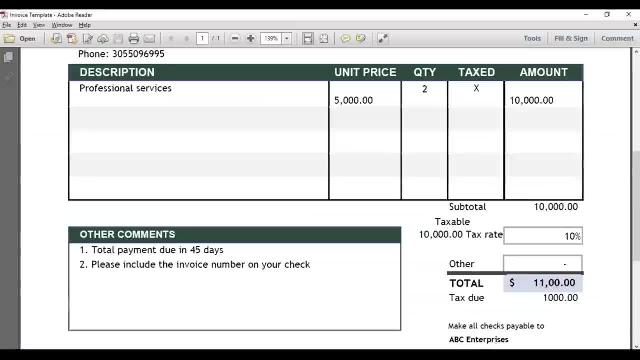 you can again indicate on the screen. So I'm going to leave that part for you, but let me just quickly show you how you can indicate it on the screen. So what I'll do is I'll just close this and then I'll just 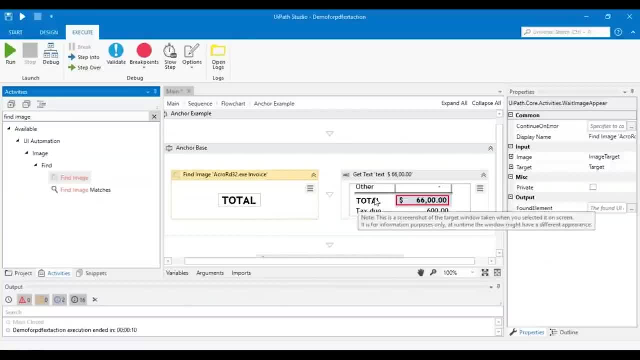 you know, indicate it on the screen. Let's say total, And once you mention that it will understand that you know it has to search for this particular image. That is the total and based on the anchor position on the left hand side. 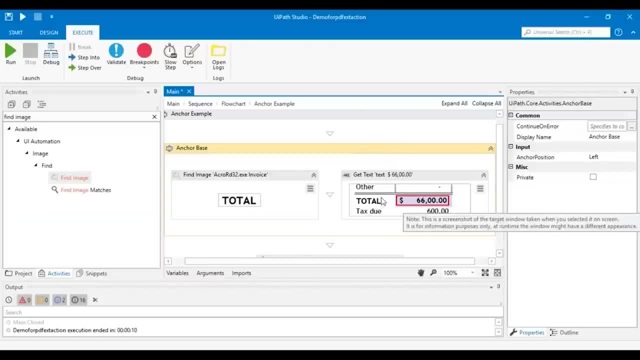 whatever action that you want to do. suppose I want to extract 6600, I'm going to just use find image activity again, and then you can just select that particular section to extract the values, right? So that's how you can use the find image activity. 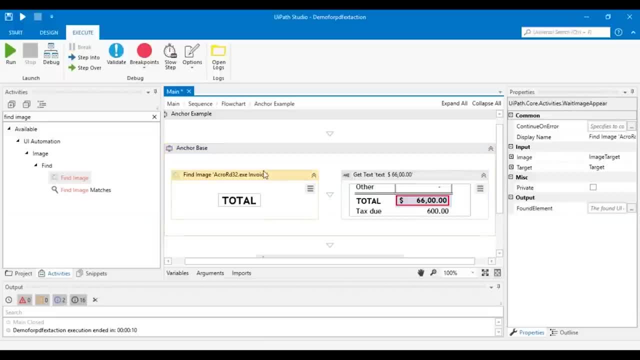 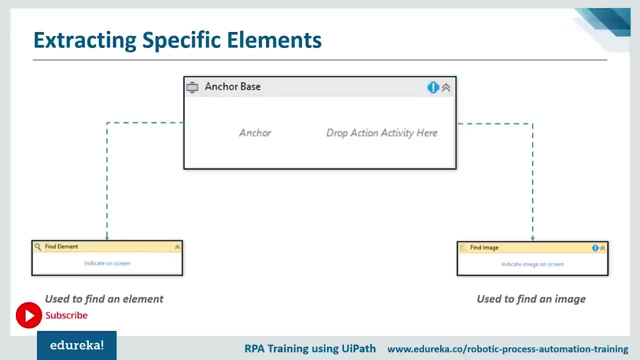 Also, guys. well, I'm going to leave the find image activity part to you so that you guys can explore. So, guys, that's how you can extract various elements or, you know, you can say specific elements using the activities in UiPath. 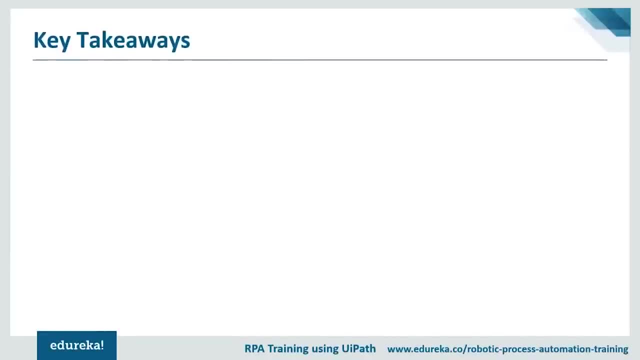 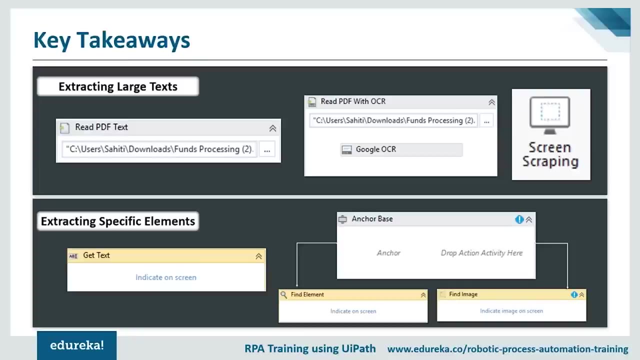 So that's an end to the session. Now, before I just end the session, let me just quickly brief you on all the activities that you've learned. So to extract data from PDFs. there are mainly two types of activities. One is extracting large text. 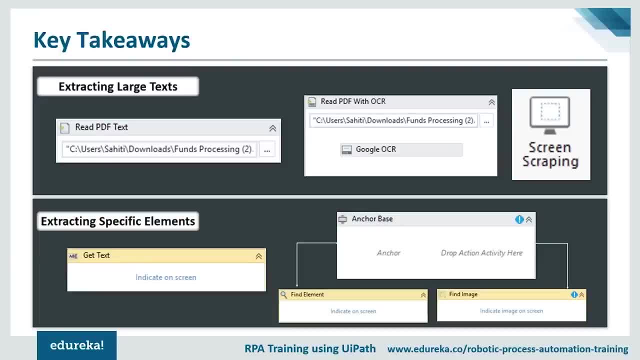 and extracting specific elements. So in extracting large text there are mainly three activities, or you can say two activities and one scraping wizard. So that is the read PDF text activity mainly used to extract text from the PDFs, and the read PDF with OCR activity. 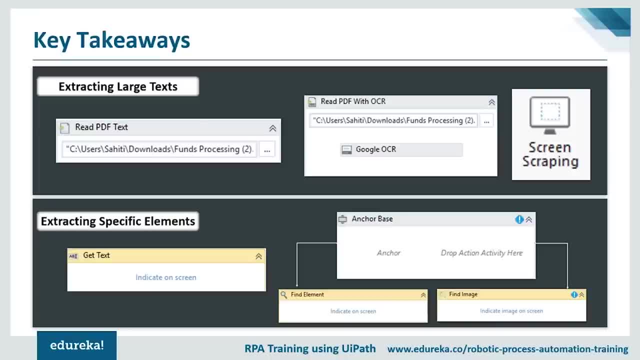 through which you can also extract the images in PDFs. The screen scraping wizard is to just scrape any data that you want, if it's a text or the image, based on your need. Now, coming to the extracting specific elements, you mainly have two types of activities. 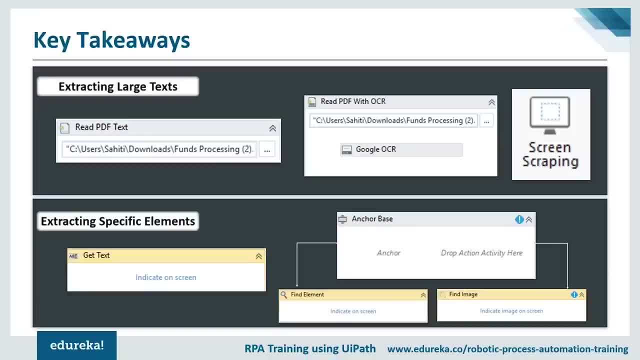 That is the game scraping and the screen scraping wizard is to just scrape the get text and the anchor base. The get text is basically again used to indicate element on the screen to get the action, or you can say to get the text and to use the anchor based activities. 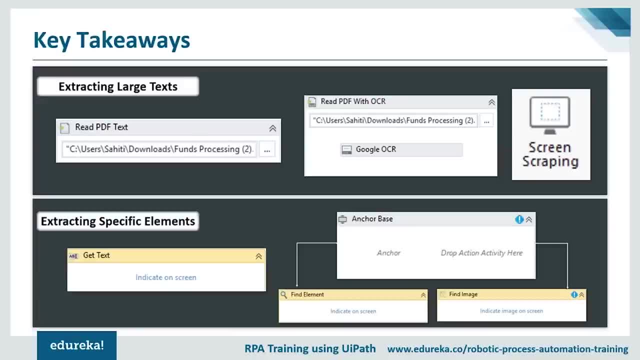 the anchor base that mainly consists of two sections, that is, the anchor and the drop action activity over here. So in the anchor section you can use the find element activity and the find image activity to extract any image or the element and based on that 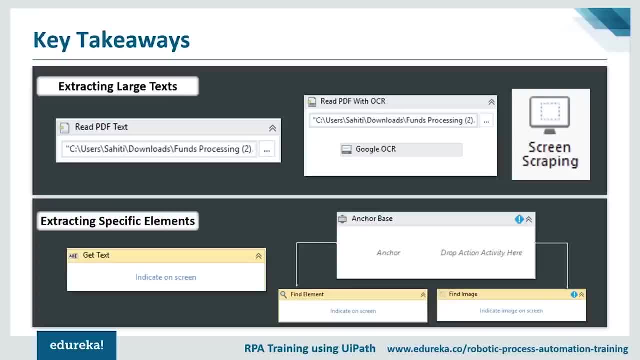 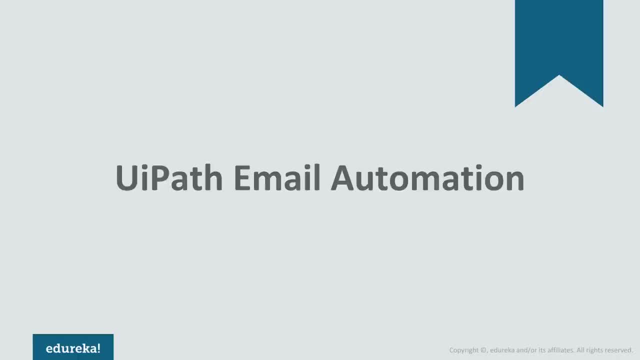 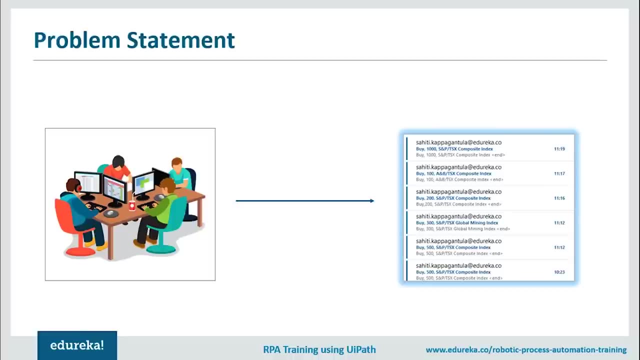 you can just mention the position and whatever action has to be mentioned that can be mentioned in the get text activity. Welcome to this session on UiPath email automation. So we're going to start today's hands-on. Let's just say we consider a team. 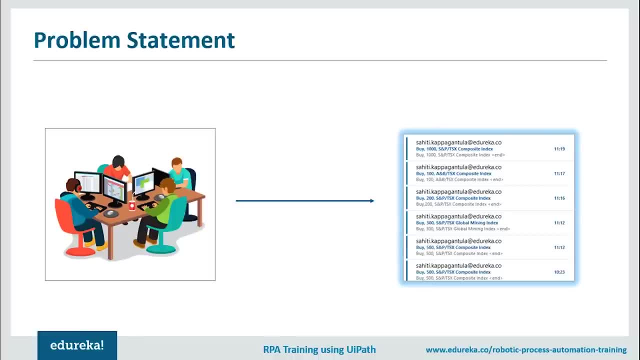 which is responsible for you know, to only respond to the email request for the funds to be processed and then report them in the same time manually. So I repeat the problem statement again: We have a team whose own work is to, you know, to just go through. 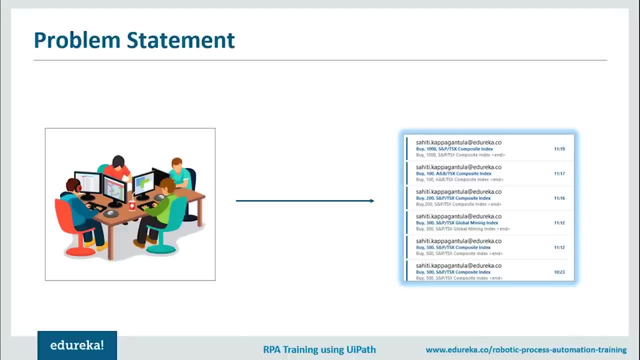 the mails and then you know they have to process those mails and then respond back to you. So now you know, when you see this scenario in a large scale industry, you get thousands of mails based on the funds right. So this is not practically possible. 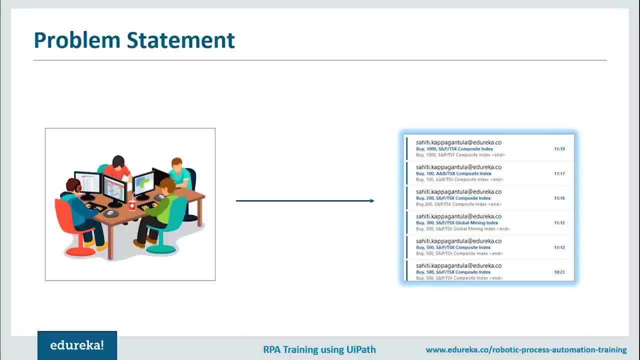 to do it manually. You have to automate it because if you don't automate such tasks then there could be a lot of errors. like you know, your emails could be mess read or, you know, the information stored could be wrong, or some people can just skip some emails. 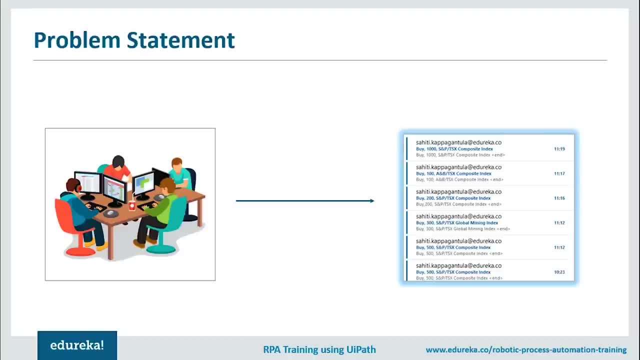 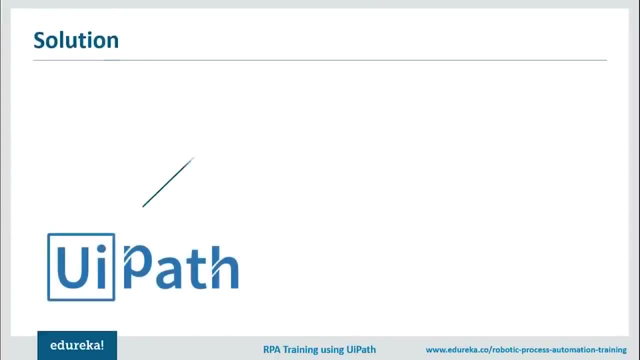 or you know, there could be a lot of problems storing each and every emails information, right So, to avoid such, you know, problems, we can just automate these tasks that I just mentioned. right So, to automate these tasks, what I'm simply doing is: 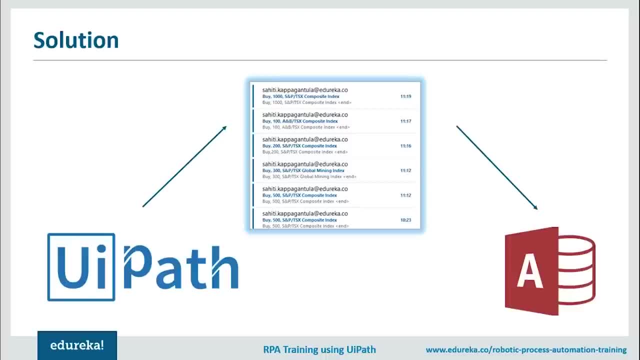 I'm going to use the UiPath Studio that I just showed you, and then we're going to read through all the emails. So, once we read through all the emails, I'm going to, you know, store all that information in a database. So over here. 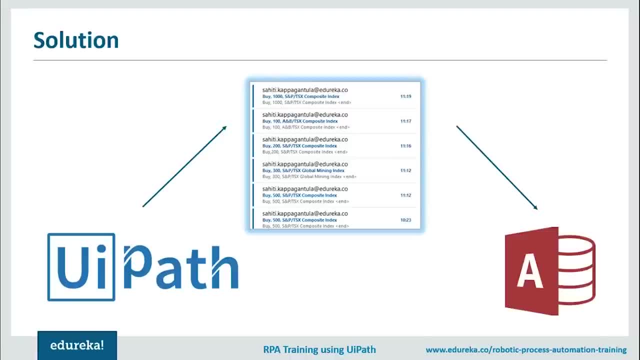 I'm using the Microsoft Access database. So that's how I'm going to, you know, automate the task, and then I'm going to store these values in the database, right? So, before I, you know, shift back to my UiPath Studio and start automating the task. 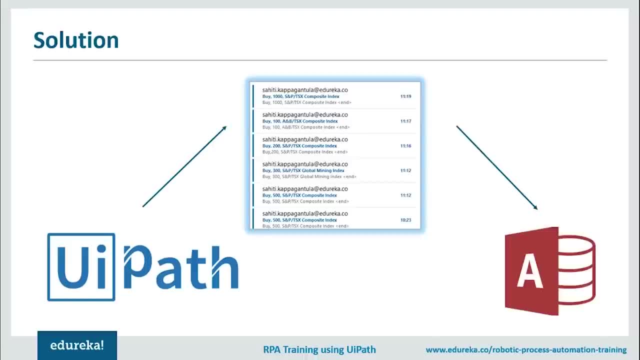 let me tell you the steps that I'm going to do first. So first I'm going to create an MS Access database file. So that's basically: I'm going to create an MS Access database Now after that, for this particular hands-on. 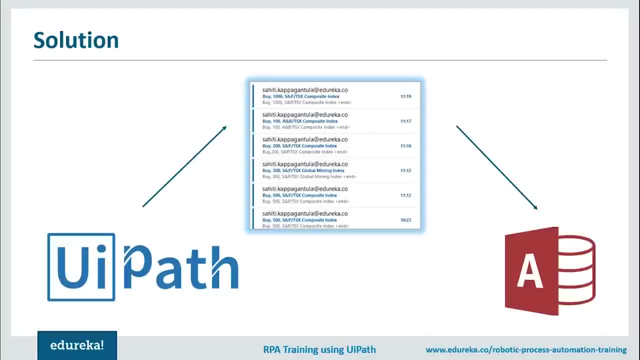 I'm going to assume that you know the trained fund emails are generated by a standard software. So over here I'm going to use the Outlook. So you can use any other software that you wish. So you can also use Gmail. but yes, over here. 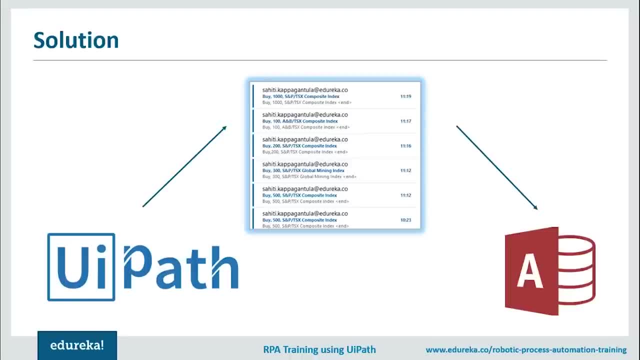 for this particular session. I'm using Outlook and I'm also considering that the subject of the email and its content are in a proper format. So the format that I'm going to talk about I'm going to show you when I open my Outlook. 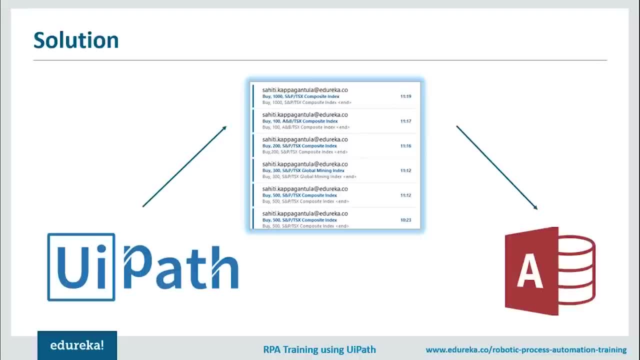 So they're in a. all the mails that have to be read are in a proper format, right, Then? what I'm going to basically do is I'm going to create a rule to identify all these emails, right? So when I say rule, 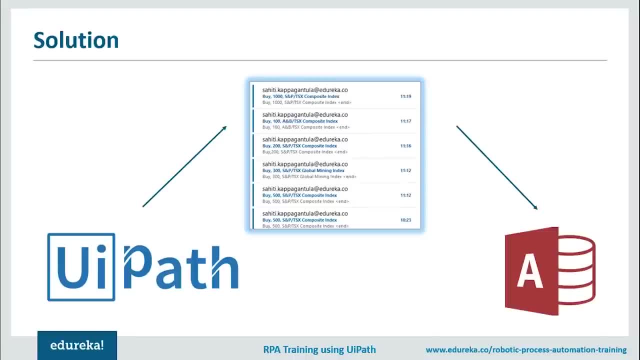 I mean that you know I'm going to make sure that all these emails which have to be read are read from a particular folder, and the emails that are in that particular folder also should have a proper format of the subject. Only then they would be read. 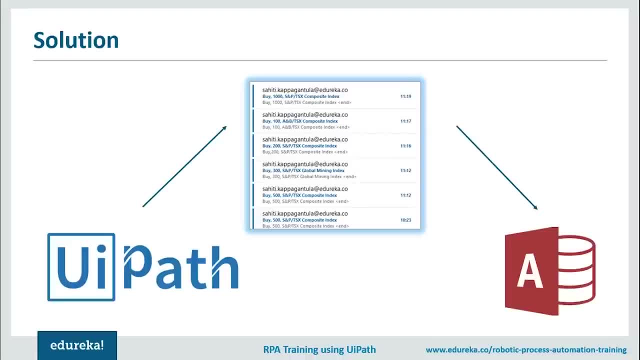 and then they would be stored, Else there would be an exception and the loop would stop right. So that's what I'm going to do Now. after that, since you know we the problem statement said that you know the team had to respond. 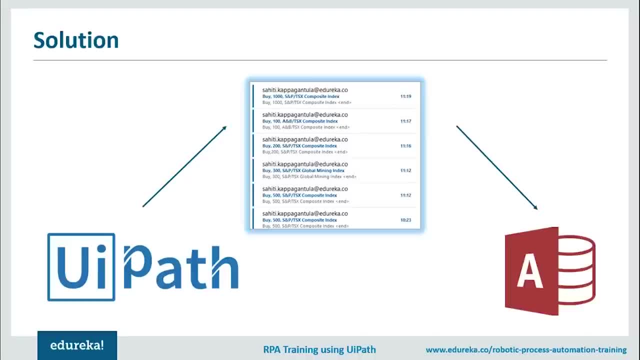 to the email also. So basically, we wanted a response status. So in the database that I'm going to store, I'm going to have a column which says: you know, receive. that means you know this email has been processed and yes, we've got the information. 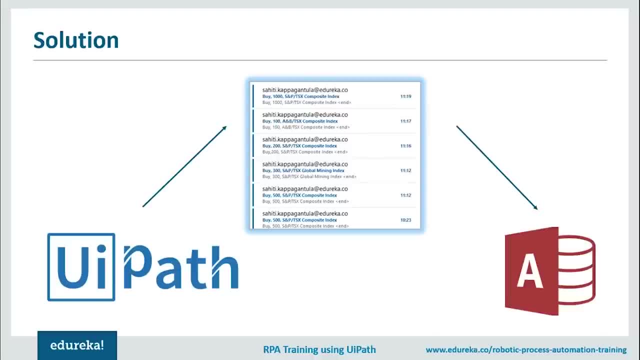 and then, finally, we're going to just automate the complete task and I'm going to show you how that is done so that all the emails are read right. So I hope that you know the steps are clear to you guys. So let's go to. 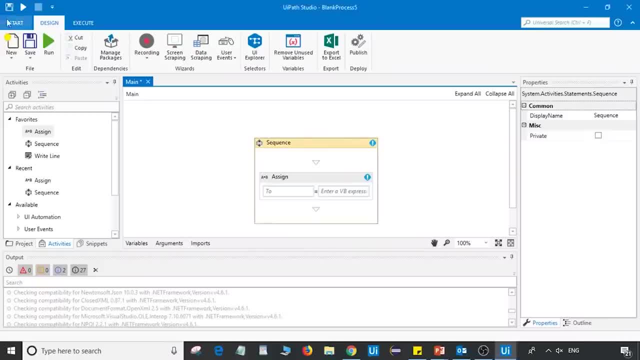 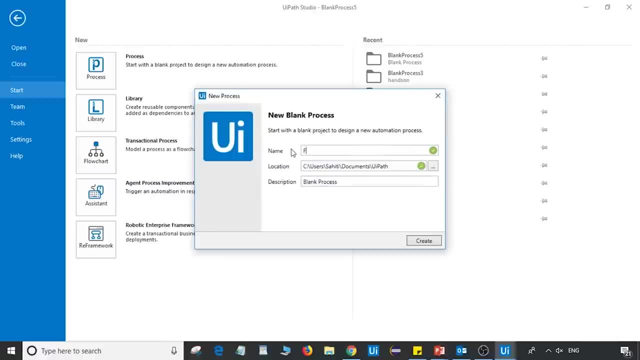 our sidebar studio and then let's start with our hands-on part. So I'm going to do a fresh start, So I'm going to create a new project, So I'm going to go to process and let's say, you know, we have this projects name. 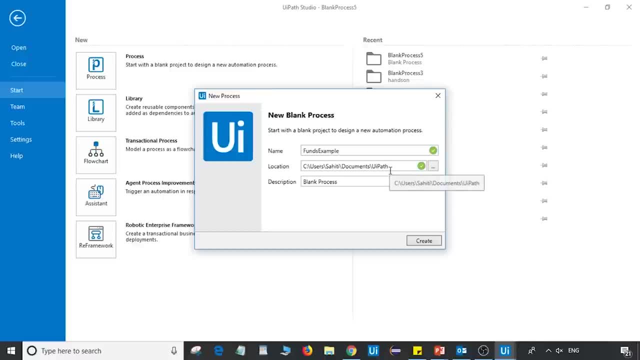 to be funds, example, And let's say the location stands the same and in the description, and let's say I have hands-on right. And then I also mentioned email automation, so that it's clear. Now, once I'm done with that, I'll come back. 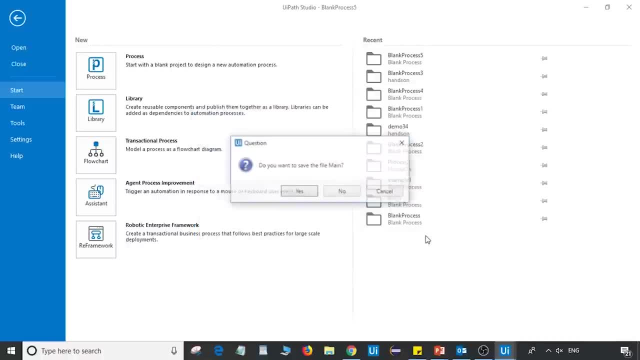 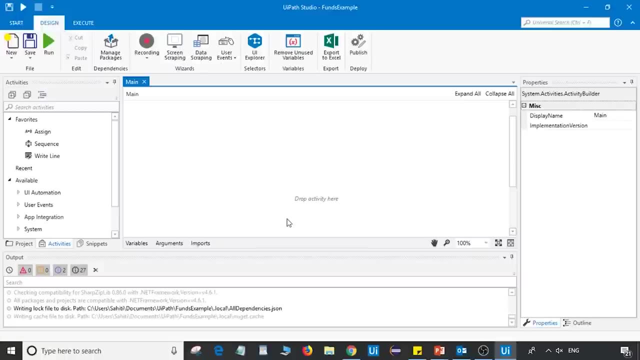 and let's say, I have hands-on right So I'm going to click on create. So once you click on create, you can see that you know your project is getting loaded and your project is getting created. That is basically a blank project. 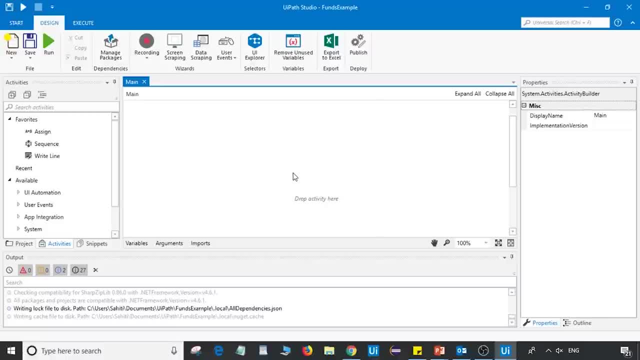 So, as you can see on the screen, a blank project has been created right Now before we start by with the activities in the UiPath Studio. first, what I said was I'm going to create a database, right. So for that. 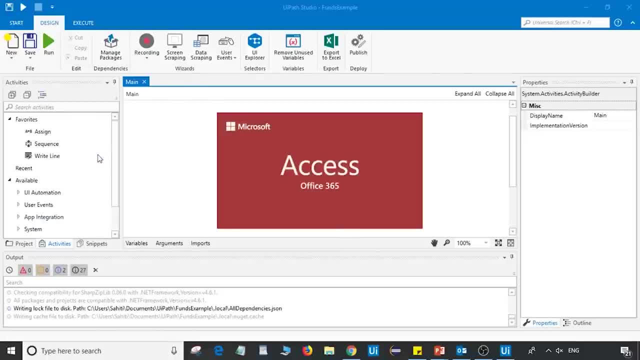 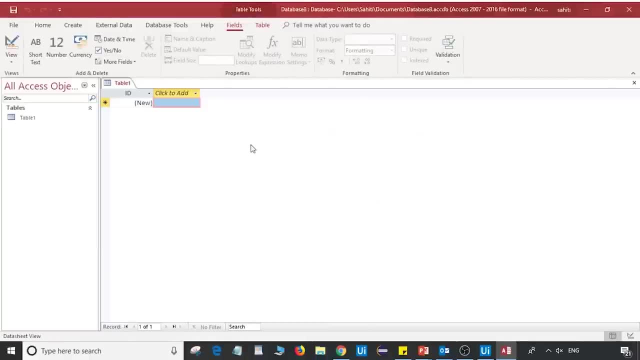 I'm going to search for access in my system, So let's just open access. after that I'm going to choose blank database and then over here I'm going to mention the table values. that is basically: I'm going to choose a table and then 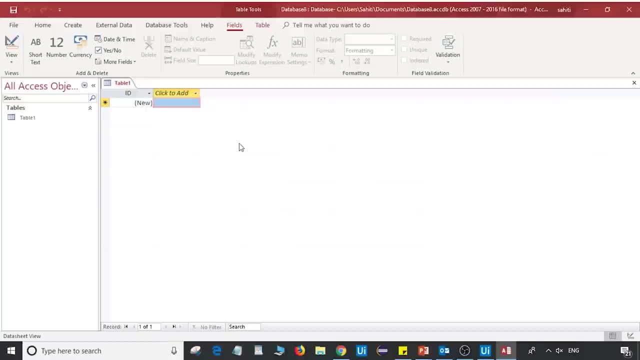 I'm going to have a lot of columns so that you know I store all the values right. So that's how it's going to be done. So over here let's just say: we choose the default table, So I'm going to choose. 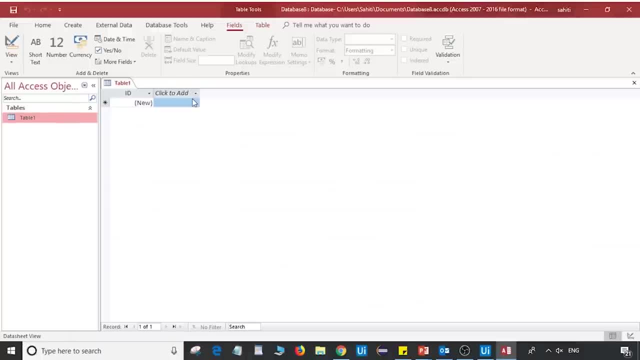 this default table, that is table one, and after that I'm going to start adding columns. So let me just quickly add the columns once I open my Outlook and also open my UiPath Studio, right, So you won't get confused. So let me just quickly. 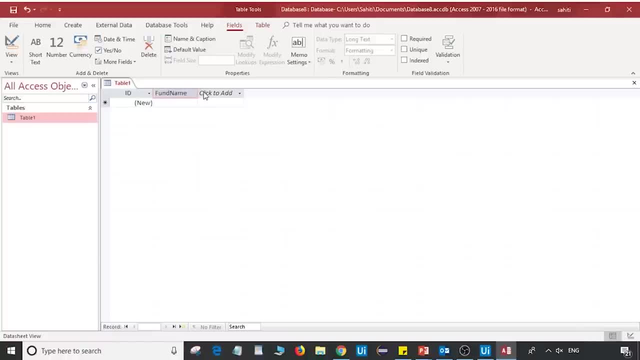 add columns. So first column would be fund name. So that is basically the fund name that I want to store. Then I want to store the request type. that is basically my action right. Then I want to store the request from. that is basically. 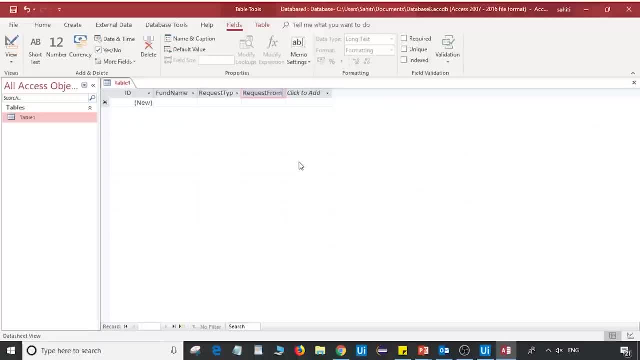 the from mail address that I want to store, Then I want to store the request status And then I also want to store the quantity right. So I'll just type in quantity right. So I have these various columns. that is the fund name. 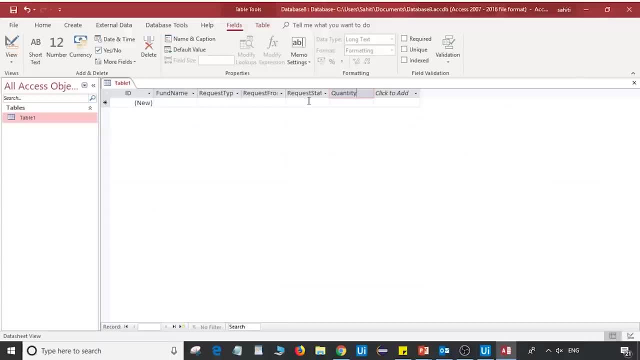 the request type, the request from the request status and the quantity right. So let me just you know, extend these column names so that you clearly see them Right Now. once this is done, I'll just go to view and choose design view. 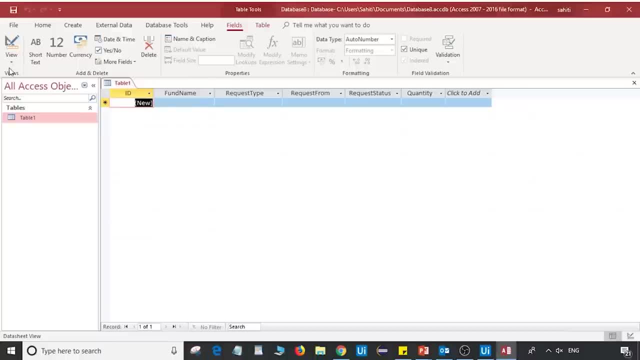 and then I'll mention the table's name, Let's say fund transactions, right? So that's basically the table name that I'm giving, And over here you'll see all the column names and their respective data types, right? So, starting with, 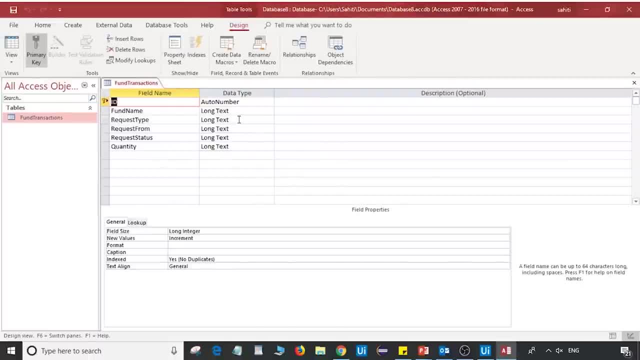 the first column name, that is ID. that is basically a pre-generated column that will be used to identify every tuple that you want to store, right. So let me just identify every tuple uniquely in that table. So this column will basically act like a primary key. 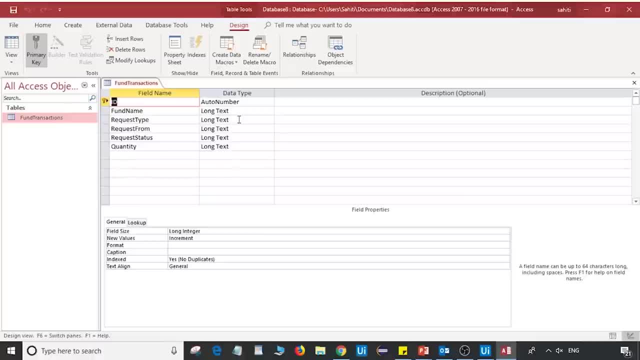 So when I say primary key, so for every record in that table would be uniquely identified with this particular column. So, since you know, for every record that has been added, a new number has to be generated, So I've used the data type. 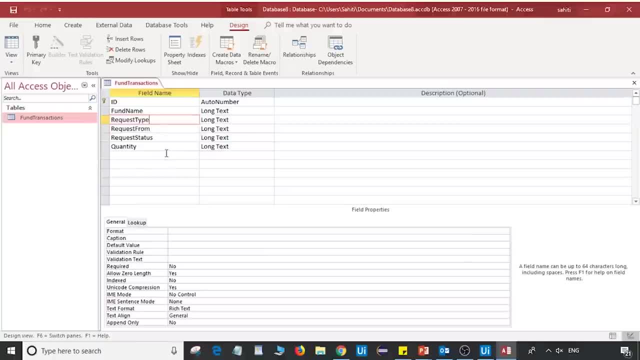 to be auto number. Similarly, I have the fund name, the request type, the request from the request, status and the quantity right. So I have all my column values. so after that, what I do is I'll just save this database file. 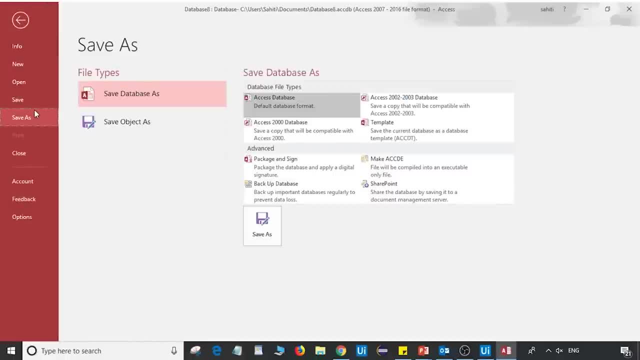 So I'll go to file, I'll open, save as, and then I have various options to save right. So I'm going to choose access 2000 database. I'm doing this because you know sometimes what happens is when you want. 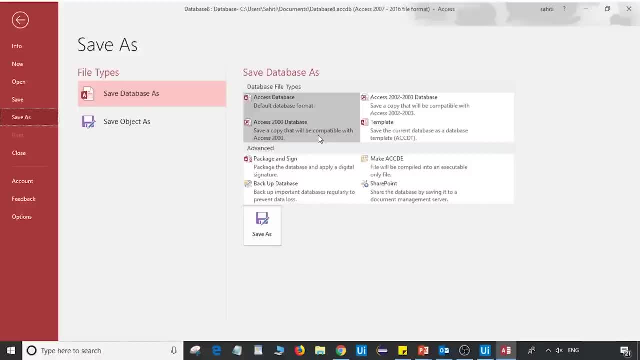 to connect your database file to your UiPath Studio, you get an error that you know unrecognized database format. That's because you know your access version present in your system is not compatible with your database, and then I'll click on save as. 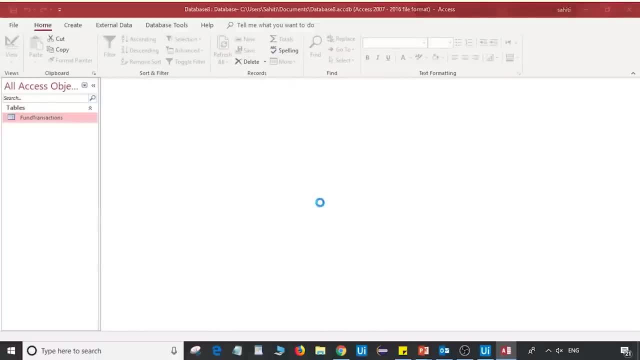 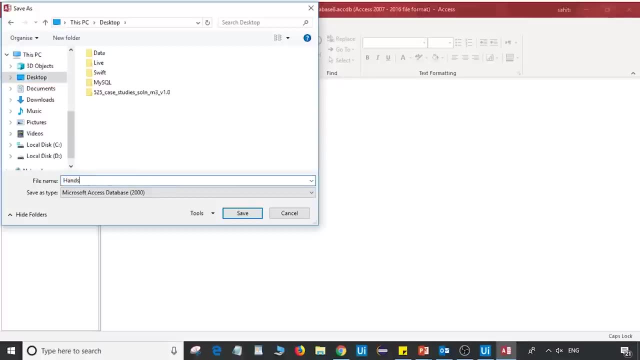 So I'll just choose this option, yes, in the dialog box. and let's say: you know, we save it to desktop and we have hands-on right, So I'll just click on save and you'll see that you know. 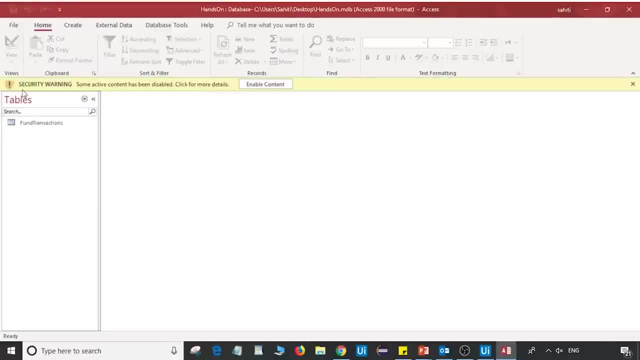 our database has been saved right, So you can just enable the content and you'll see that. you know. we have a table with all these columns. since our database has been ready, Let's just shift to our Outlook so that we understand. 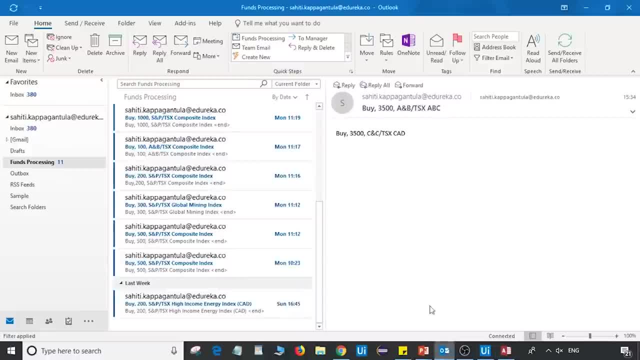 what emails are being read and how. the email subject format is right, So I'll just open Outlook. Alright, so this is my email. So this is basically the email from which all the emails would be read and you know the values. 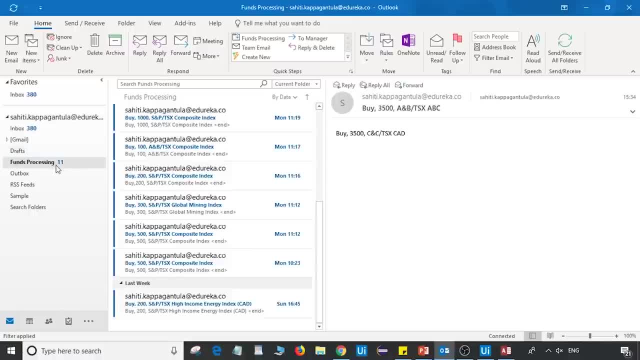 would be stored in the database, right? So what I've simply done is, for this particular session, I've just created a new folder from which all the mails would be read, right? So you choose new folder and then you just rename your folder. 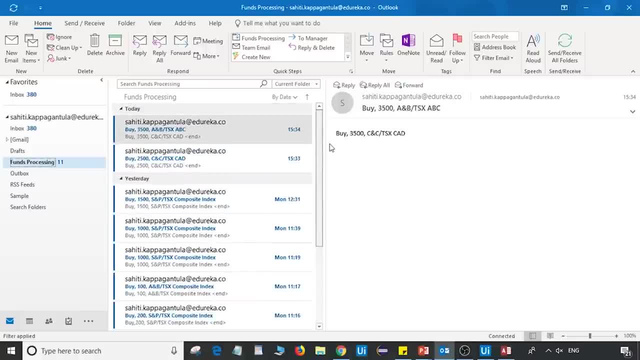 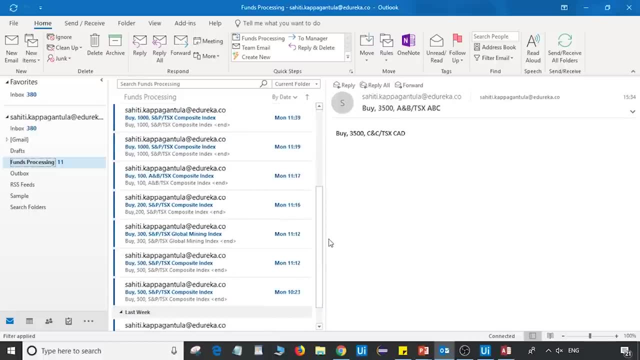 based on your wish, right? So I just chose it as funds processing, and you can see that you know I've already some pre-generated emails that I'm gonna read and whose values will be stored in my database, right? So I have around 11 emails. 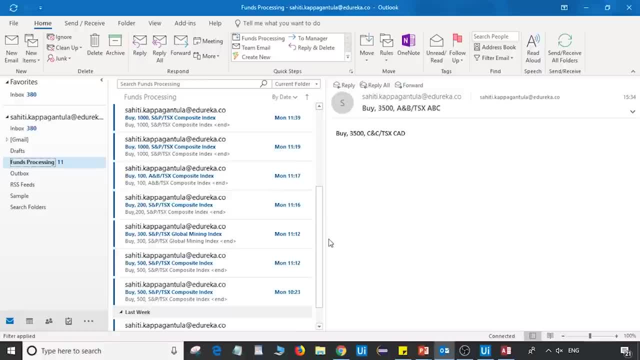 Now, one thing that I want to make sure is that you know you have to, you need unread emails so that you know you don't only the unread emails, and once they're read, we just want to mark them as read. 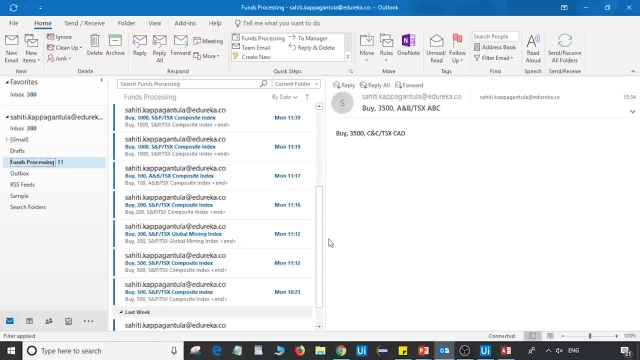 right So that all those parameters would be applied in the UiPath Studio. Now, if you observe any all the emails, you'll observe that you know the subject format stands the same. That is basically. we have three parameters. that is the by. 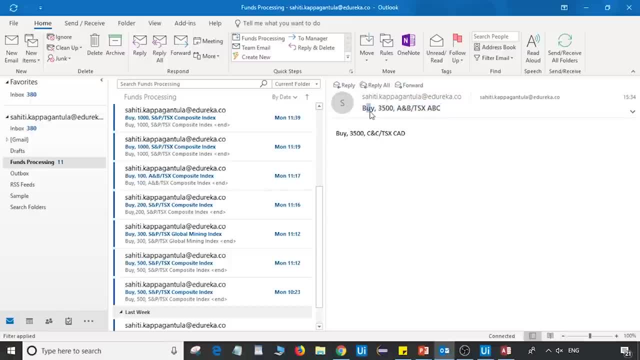 the quantity and the fund name right. So by is basically our action, that is basically our transaction type. Quantity would be any quantity that I've mentioned and the funding Now. so any mail in this particular folder without this particular format would not be processed. 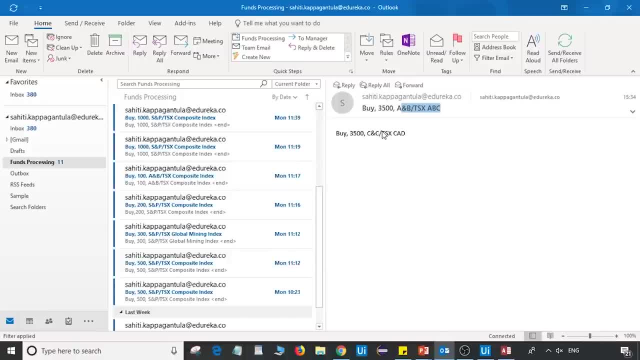 and obviously the loop will stop then and there and an exception would be shown right. So that's how we can, you know, create a rule to read all the emails. This is just a general rule that I have created You can have. 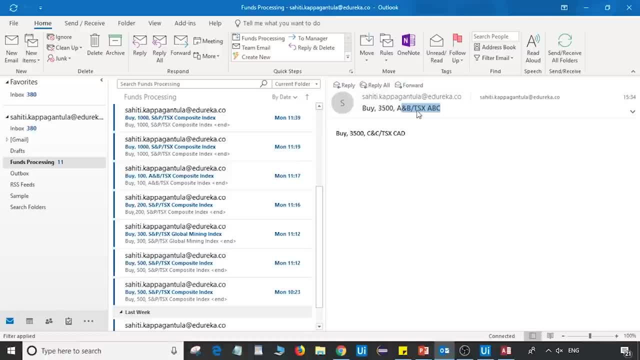 any rule that you want. So you can just have two parameters, or you can have ampersand or any other symbol that you want to choose. right? So that was the basic format of the email. right Now let's shift back to our UiPath Studio. 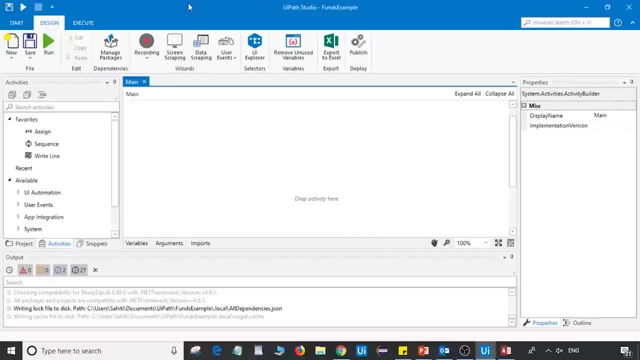 and let's just start automating Now. to start automating, what you simply have to do is you have to first drag a sequence. So when I say a sequence, all the tasks that you know you're going to perform, or all the actions. 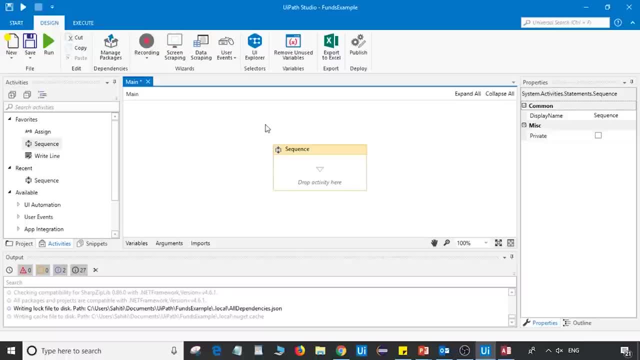 that you're going to perform are going to happen inside this sequence. That means, when you execute your UiPath Studio's project, the sequence is going to get executed right. So we'll just mention sequence and then after that, what we'll do is: 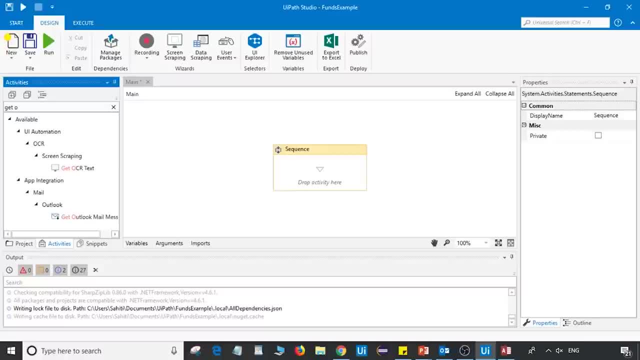 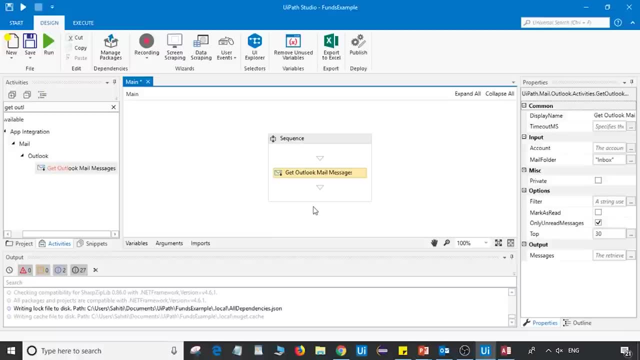 we'll drag a getOutlook activity, right? So we'll just search for getOutlook. So now I'm dragging this activity because I'm using an Outlook software. So if you were using a Gmail software, then you drag and drop a Gmail. 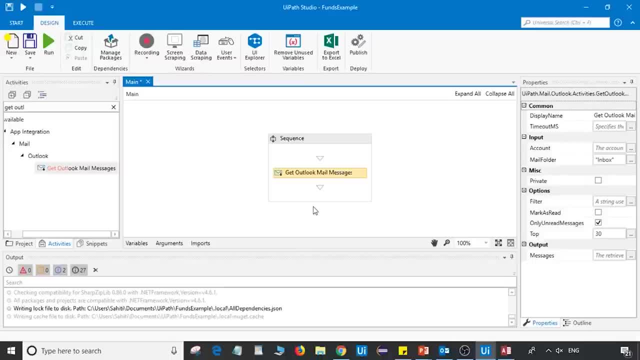 getOutlook Gmail mail messages, right? So that's how you can do. or if that is not the activity, then you can drag. then you can drag any activity from the packages folder, right? So in the getOutlook mail messages, what I'll have to do is 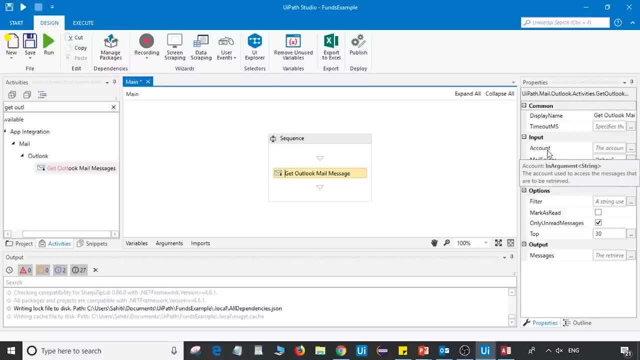 I have to mention the account from which all the mails have to be read and the folder's name, right? So that section is my present account that I'm using. that is my email ID, So I'll just type in my email ID, right? 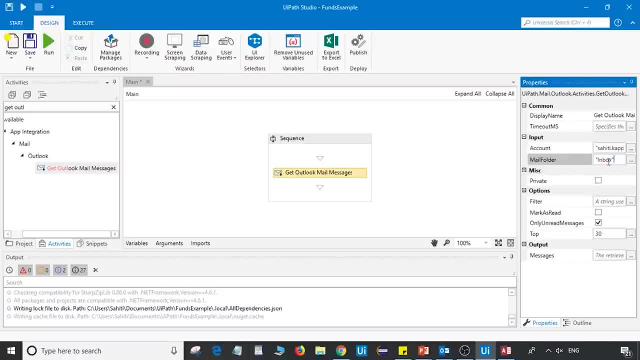 Now, once this is done, you have to mention the mail folder. By default, it would be inbox, but yes, since our mail folder had funds processing, we're going to mention that. So I'll just type in funds processing, right, So you can open this. 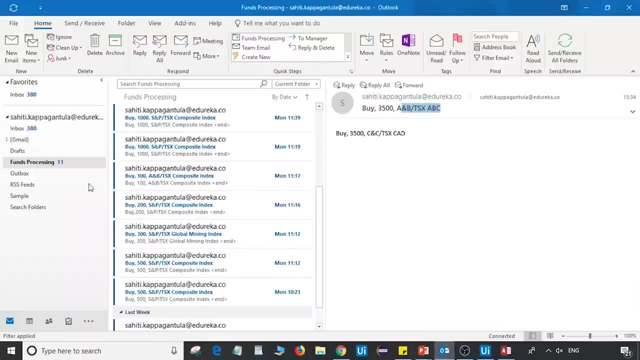 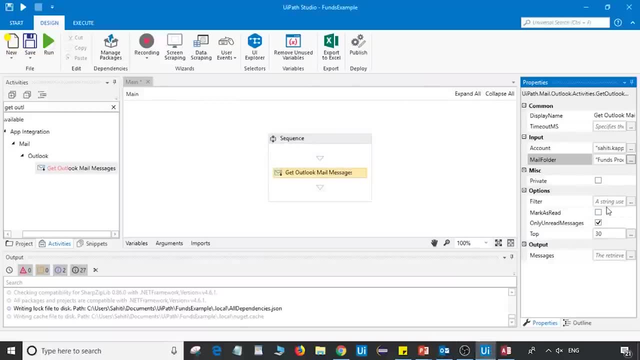 and you can make sure that you know. it's mentioned funds processing, So let's just check again. Yes, it's funds processing. Now, after that is done, you have to mention, you have to mention all the filters. So we want to read only unread messages. 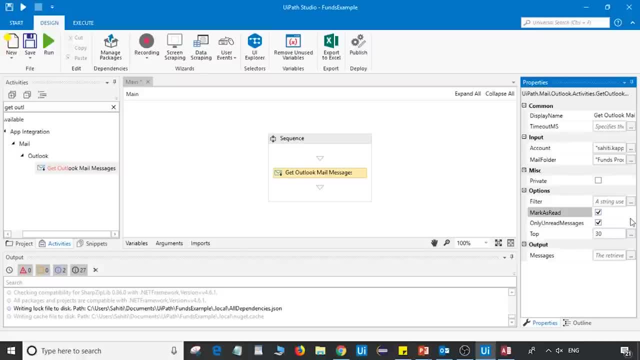 So I've chosen that and then I've chosen mark as read. So once all your messages have been read, they'll be just marked as read and only top 30 are considered right. So top 30 messages that you can see over here would be considered. 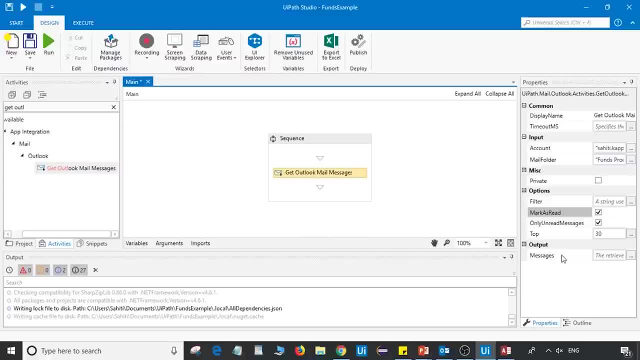 but yes, if you have hundreds of emails, you can limit it to hundreds of emails as much as you want. Now, after this is done, what you have to do is you have to initialize, or, you know, you have to create all the variables. So, to create. 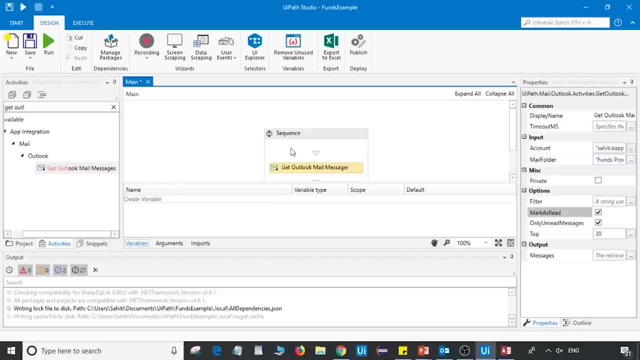 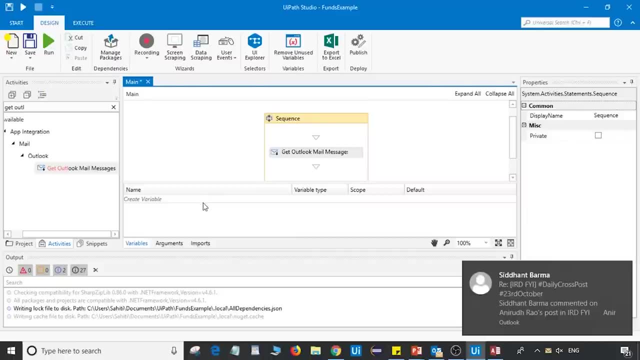 all the variables, we're just going to use this variable option over here and then we're going to choose sequence. So that would be the scope, would be sequence for them and to create a variable, you'll just choose this option of create variable right. 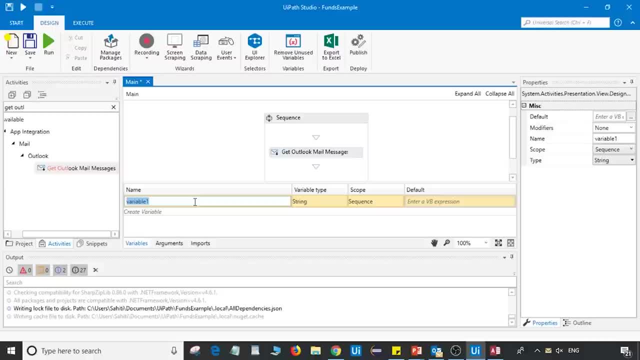 So let's just start mentioning all the variables. So I'm going to start mentioning all the variables and I'll explain you why we're using all these variables. So I'll start with the array: fund details. So basically, I'm using this variable to store the values. 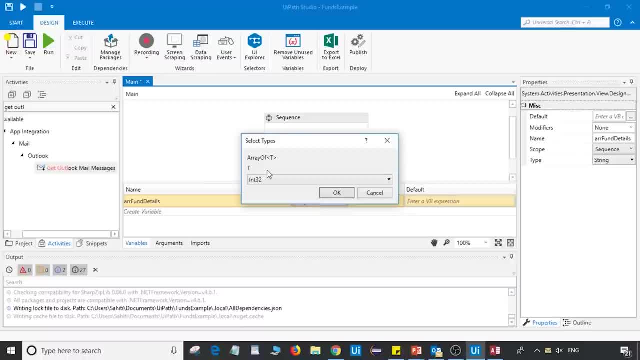 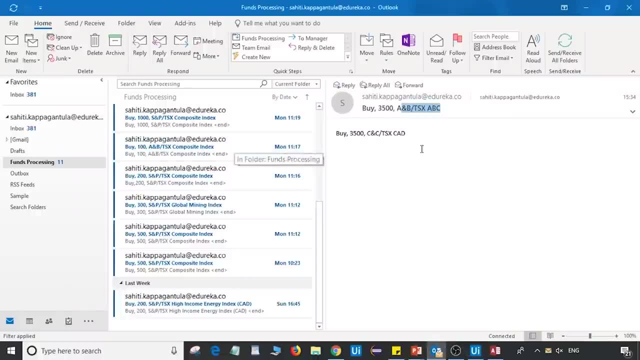 of the subject, So I'll just tell you how that's happening. So in the array of T I'll choose string, because this is of a string array, and when I say array, fund details. so, as you saw in the outlook, you have these values. 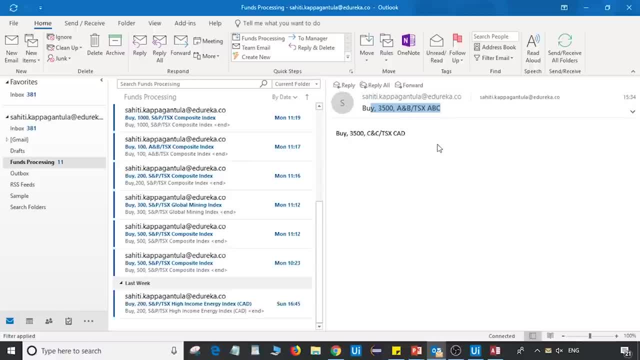 right? So you have three values by 3500 and A and B. that is basically the fund name, right? So basically, what I'm going to do is I'm going to divide the subject into an array, So by would be. that is basically. 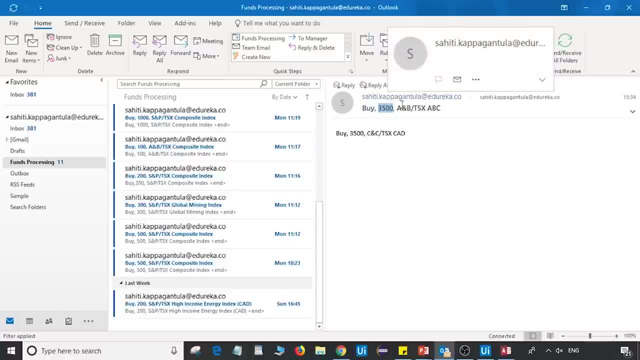 the action would be stored in array of index 0, the quantity would be stored in array of index 1 and the fund name would be stored in array of index 2, right, So that's how I'm going to divide the subject, and that's how. 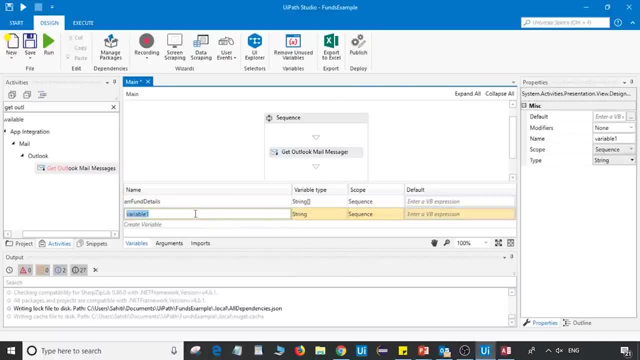 we're going to retrieve and store it in our database, right? So that's the reason we're using this. Then I have to create a variable to connect to the database. right Now, this has to be a variable type database connection, So I'll just browse. 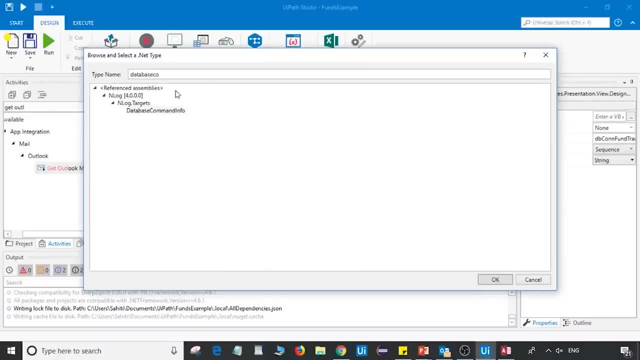 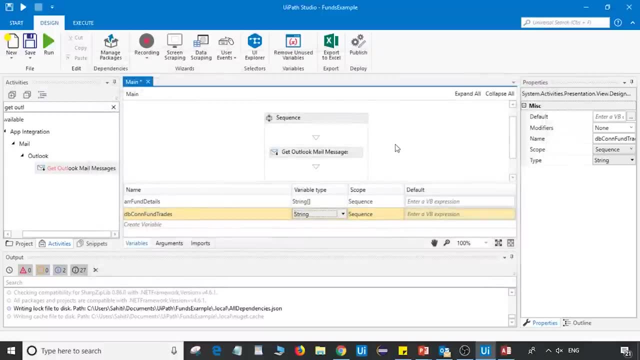 for types and choose database connection. All right, So you can see that. you know, I don't find any such variable type, So I'll just close this. and now what you have to do is you have to install them. So you have to install. 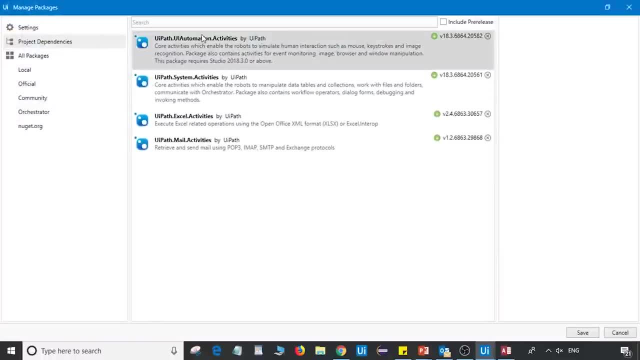 those packages. So you go to manage packages option and then you can start searching for the packages that you want to install, right? So basically, since we are connecting to a database, we need a database activity. So I'll search for uipathdatabase. 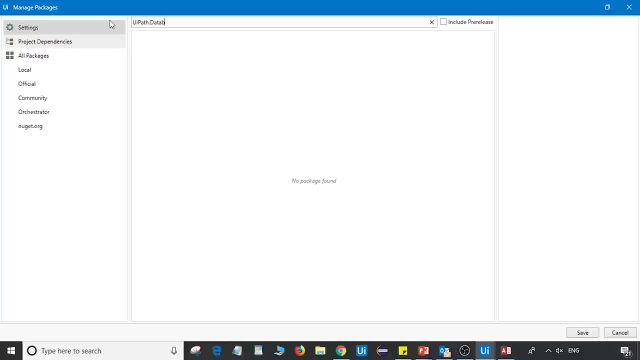 and then I'll click on that. Okay, Let's just quickly search. Yes, So I'm going to choose this arrow option over here to install the package. So that would be chosen, And after that I also want to choose the Microsoft activities. 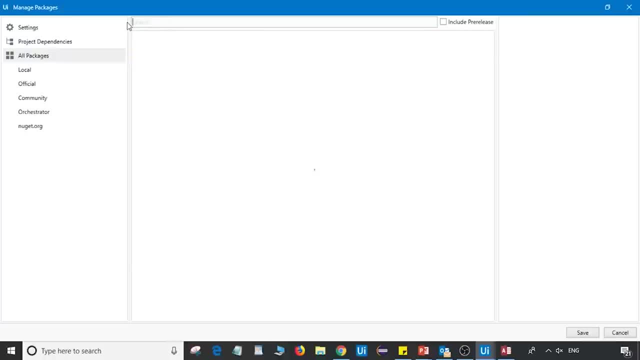 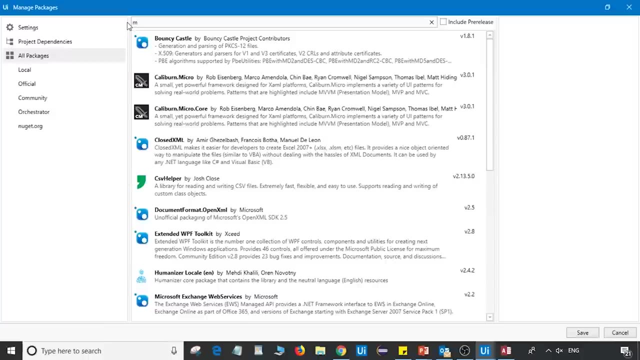 extension package because I'm using MS Access database, right? So I'm going to use search for Microsoft Access extension. All right, So I'm going to just click on this and I'm going to search for Microsoft Access extension. All right, So I'm going to. 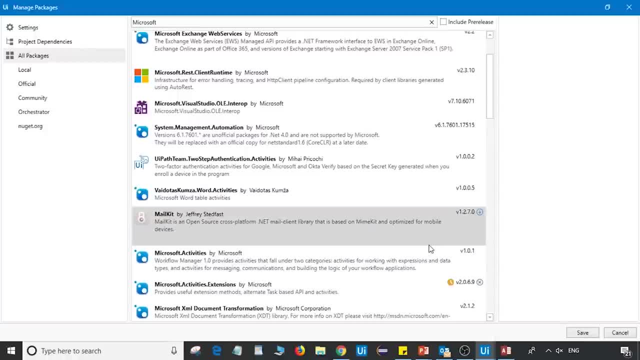 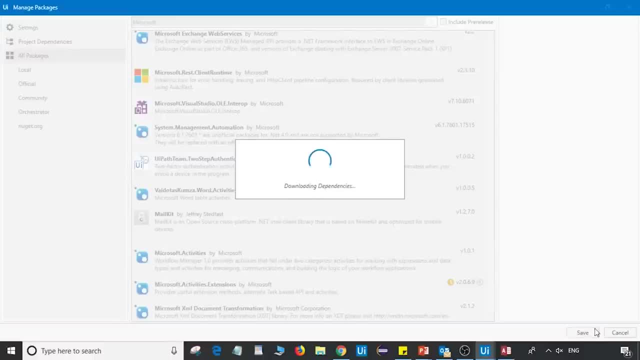 just click on this arrow, So once I choose the packages that I want to install, I'll click on save. Once you click on save, you can see that you know your dependencies are getting downloaded for the project, So let's just wait. 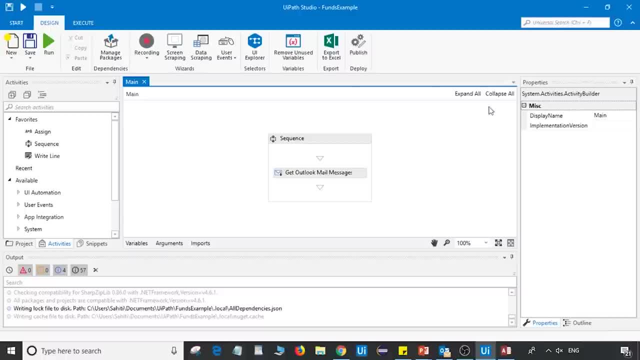 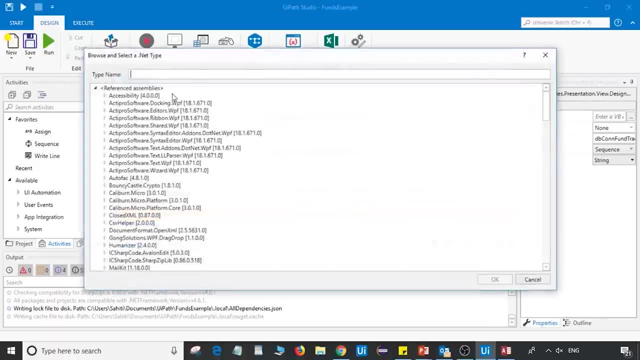 for that. All right, So you can see that you know all your dependencies have been added to the project, right? So now let's just again go to the variable section and then let's search for database connection. right, So we'll go to. 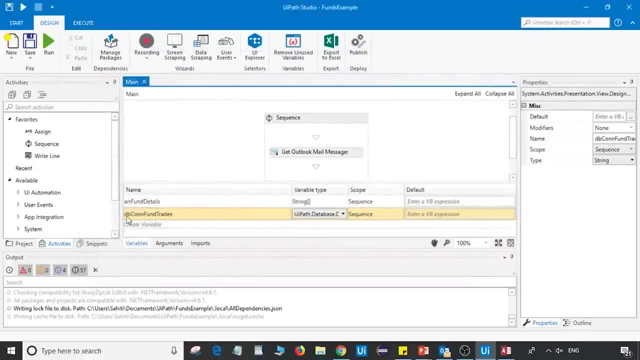 browse for types and we'll just click on OK. So that's how you can use this variable type. Next, we're going to create another variable for mentioning all the tuples, or you can say, to get the output of the database. So I'm going to use: 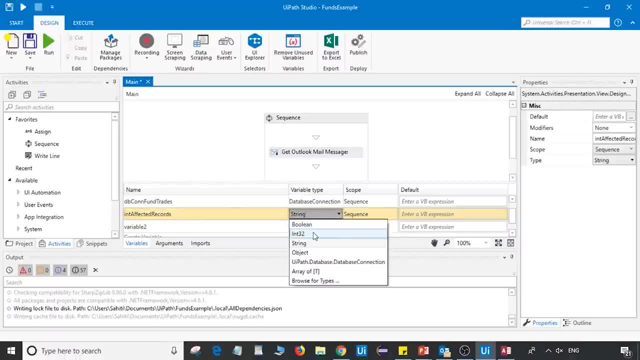 this particular variable. for that, And let's say to be of n type, Then we're going to create variables to list all the emails which have to be read right? So for that I'm going to choose the name to be: list fund emails. 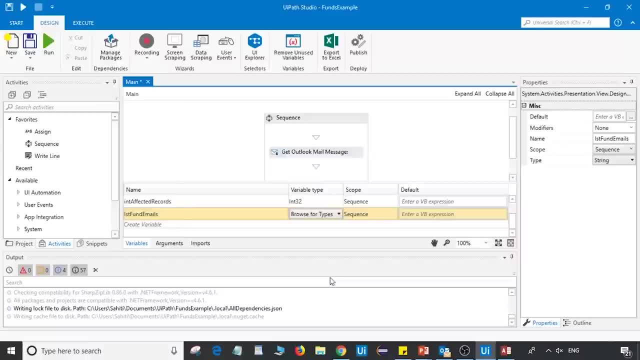 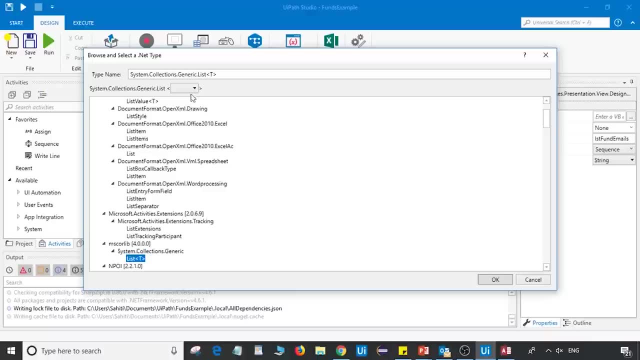 And then we have to mention it to be of list type. So we'll browse for types, we'll search list and you see an option of list of T right? So in that we have to choose the option of systemnetmailMessage. 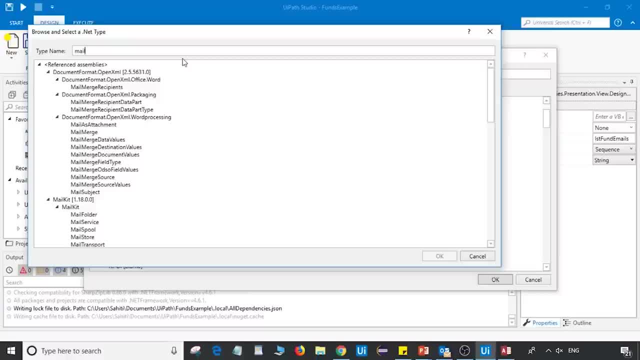 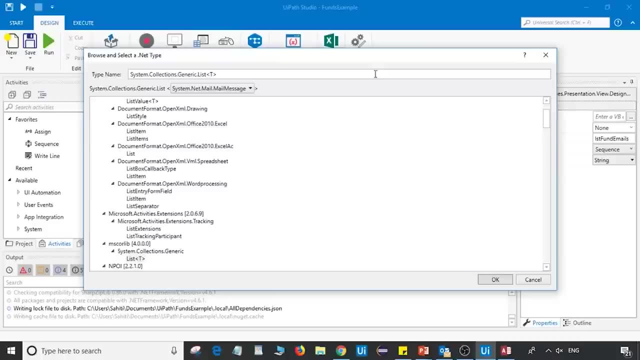 because that is what we want to read. that is mail. So I'll just type in for mailMessage, All right. So I'll just select this and then I'll click on OK. So once I click on OK, this particular variable is also. 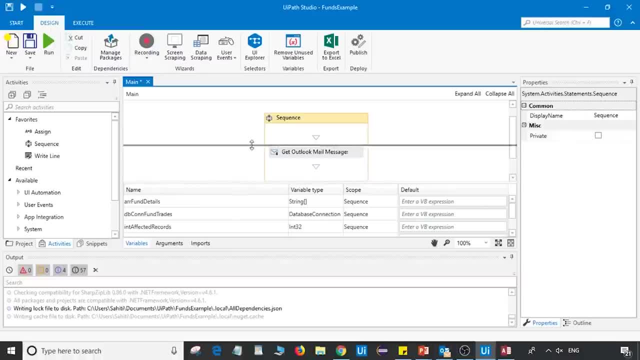 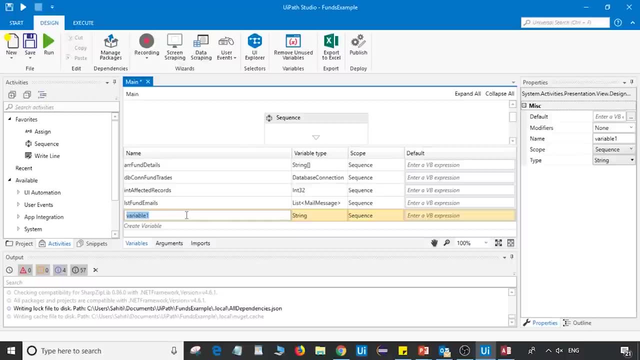 created. I can expand this and show you right Now. after that I'm going to create variables to you know, to read the from address, that is, the from email address, the email subject, and also store the fund transaction type. 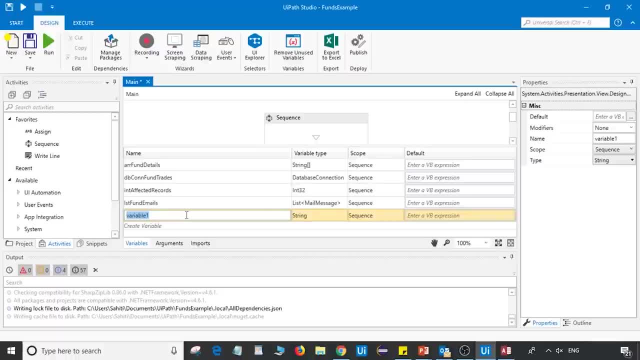 the fund quantity and also the fund name right Now, apart from these. so I'm also going to create another variable for the string query. So first let me just create these variables Now. similarly I'll create for the email subject. 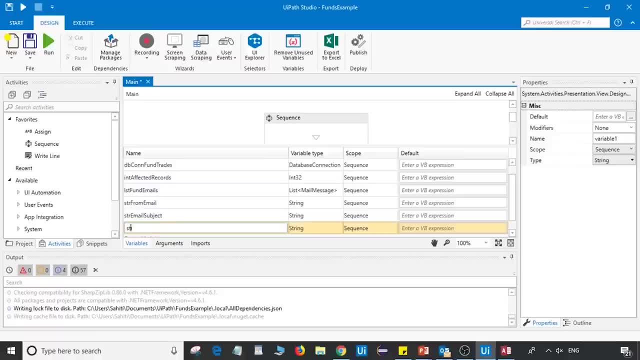 Again to be of string type. then we have variable for string fund transaction type, Again of string type. then we have variable for quantity, Again of string type. then we have string fund name, to be of string type again. So 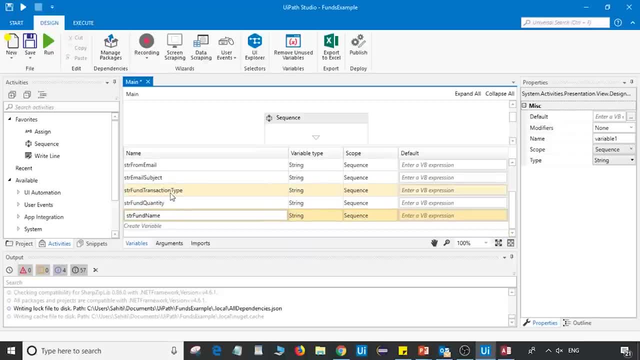 as I mentioned, we're going to create a variable to assign to the query that we're going to use to insert the values into the table. So I'm going to just create a variable saying string query, Again of string type, and finally, 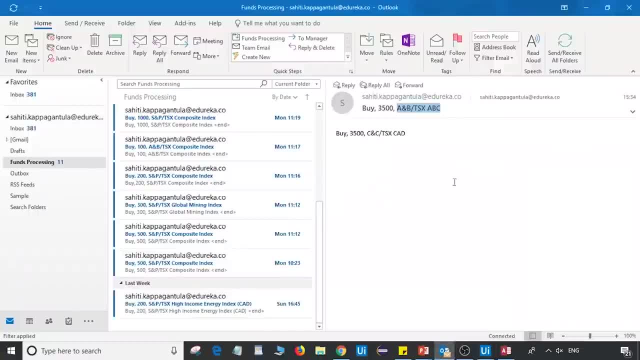 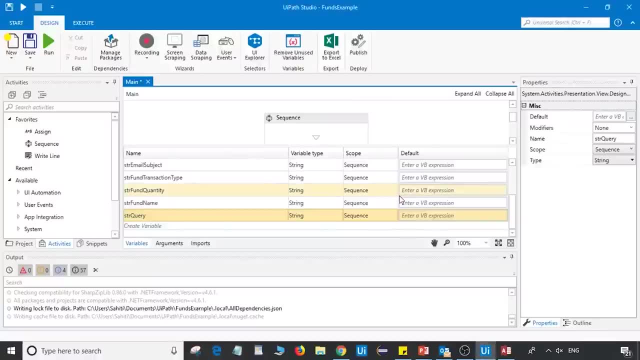 we're going to create one more variable of in type, so that you know, it counts the number of values into the array, right? So in our case, we have maximum value to be 3, right, So we're going to. 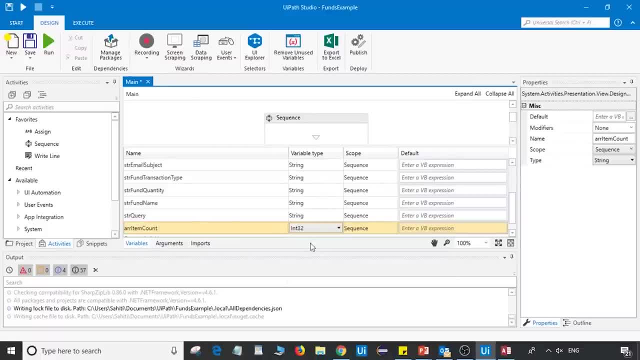 create a variable of in type, right. So now, once the variables have been created, what you can simply do is you just have to start using them, right? But before that, let me just summarize these variables for you again. 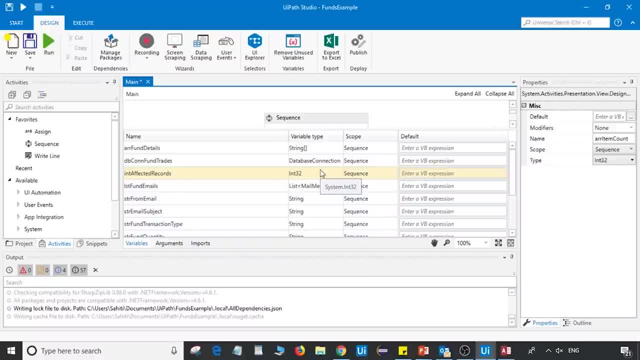 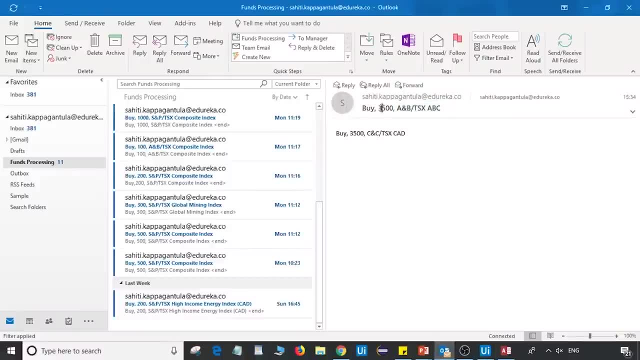 So we've created the array fund details variable, that of you know string array type, to store all the subject values, like value. array of index 1 would store this particular value and array of index 2 would store this particular value. After that: 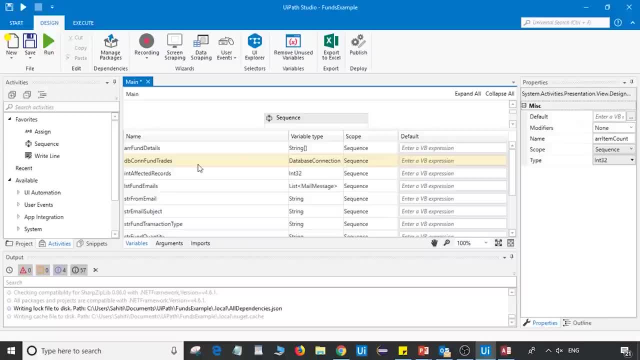 we've used a variable to connect to the database and then we've used a variable to store all the values, or, you know, to print out all the values that we've stored in the database. Then we've used and we've created a 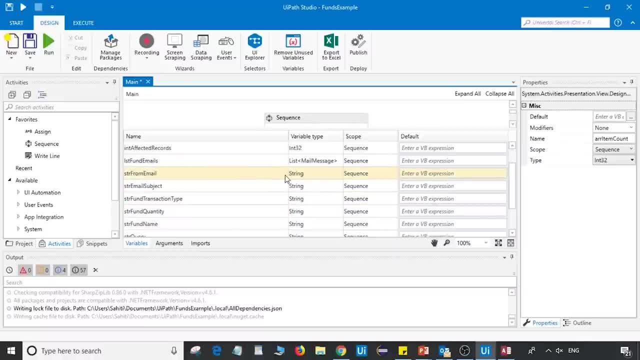 variable to list all the mail messages, So it's of a list type. and then we've created variables for to read the from the list. Similarly, we've again, you know, created a variable to be assigned to the query which has to be used. 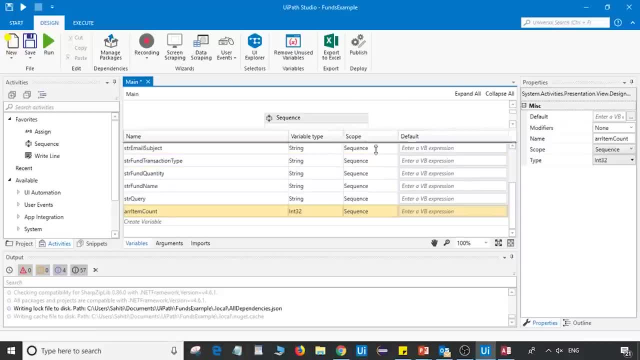 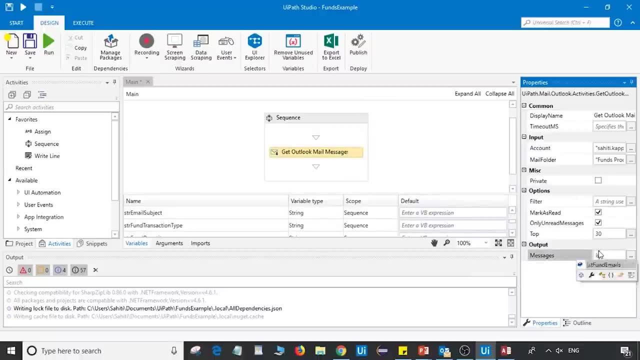 to insert values into the table. and then, finally, we've created a variable to avoid the array range out of bound exception, right, So now let's just start using these variables. So go to the get outlook mail message you have to mention. 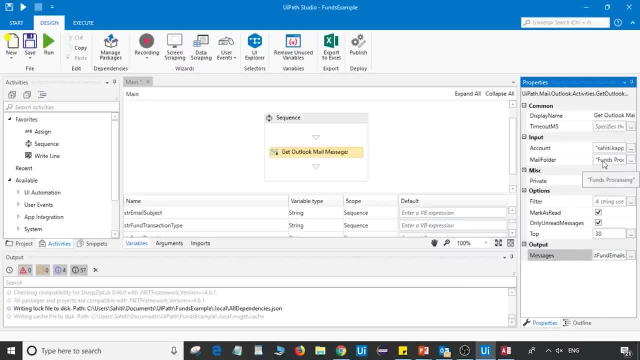 in the output of list fund emails, right? So what's basically happening over here is that we have a list of all the emails and then, once they are read, they would be marked as read and only top 30 would be read. and all these output. 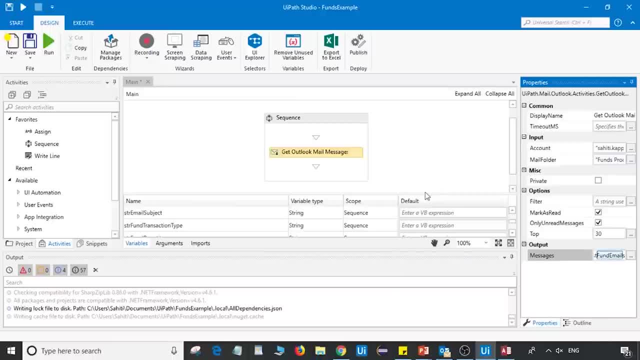 like all the information that is extracted from there would be stored in the variable list fund emails. right Now, what will happen is, for every item in list fund emails, we want a set of actions to be performed right. So for that, 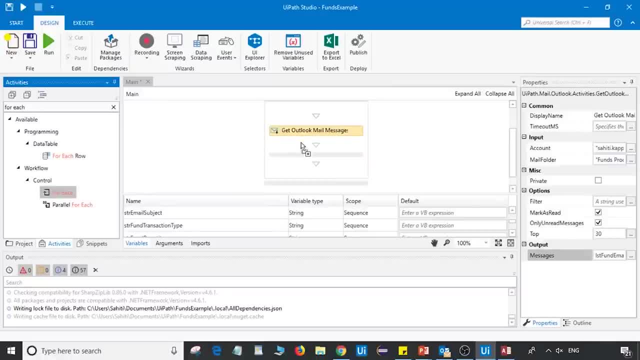 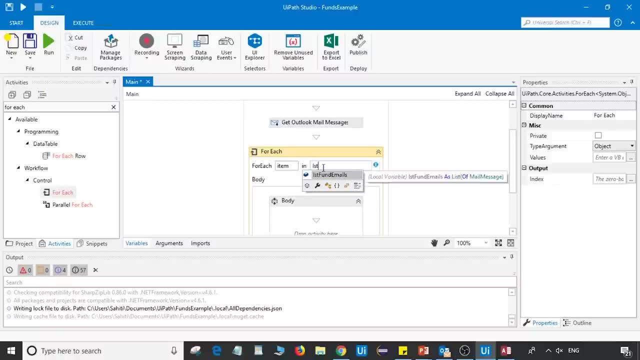 we have to use the for each workflow, So I'll just search for for each. so now what we can do is we have to mention for each item in list fund emails, that is, for each item in every mail we need to perform. 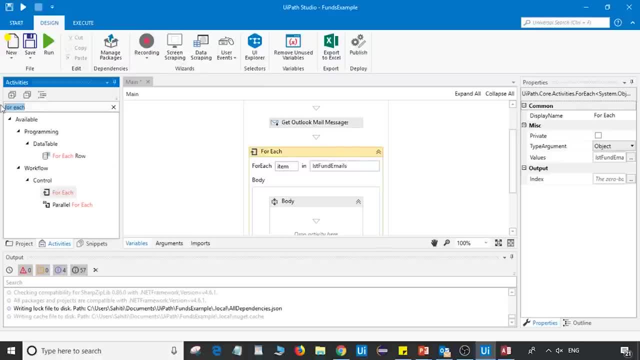 few actions, right? So I'm going to mention that So quickly. I'm going to drag some assign activities and I'll then show you why am I dragging so many assign activities, right? So that's basically I'm going to assign. 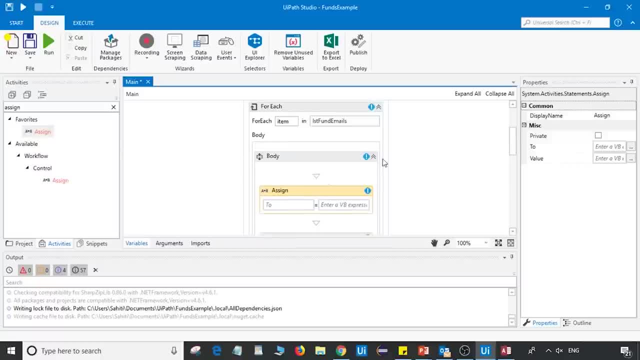 all the variables that we created to some values. So I've dragged around seven activities. So let's see what is happening with this. So, starting with the first assign activity, what I'm going to do is I'm going to assign. 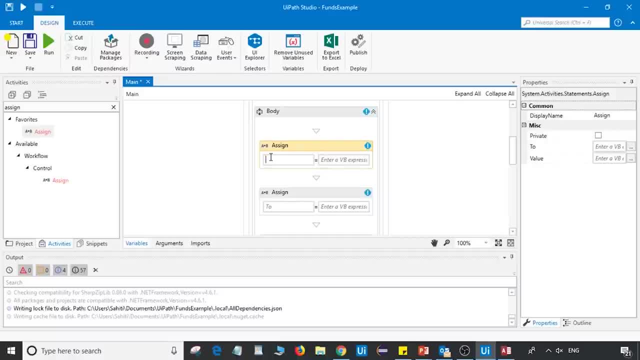 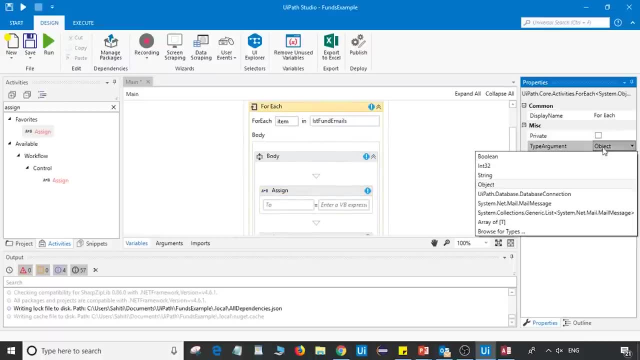 the from email address. So that is basically the first value that we want to be read. So we want to store the from email address and then we want it to be retrieved right Now. before we start with that, one more thing. 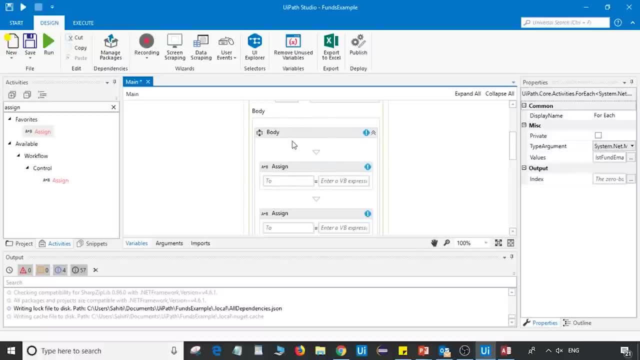 that you have to mention over here is in the type argument you have to choose systemnetmailmessage. Only then you would be able to retrieve the from email. So we'll use that variable and then we'll use for every item that is. 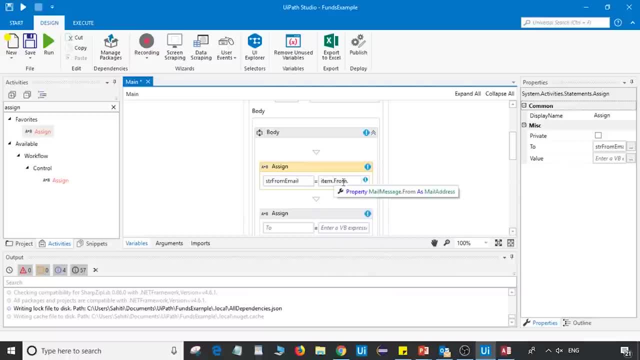 itemfrom- that is basically from address- would be retrieved, right? So we're going to mention address, So I'll just choose address over here right Now. similarly, I want to retrieve the email subject also, So I'll just assign. 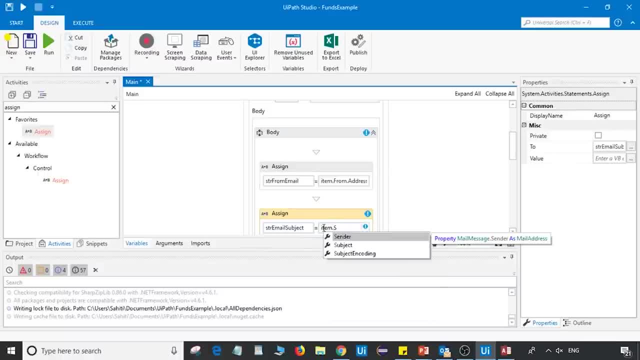 to this particular variable that the string email subject right. So what's happening is, for every item, that is, for every email, the subject would also be retrieved and would be stored in this particular variable right Now, after the subject has been retrieved. 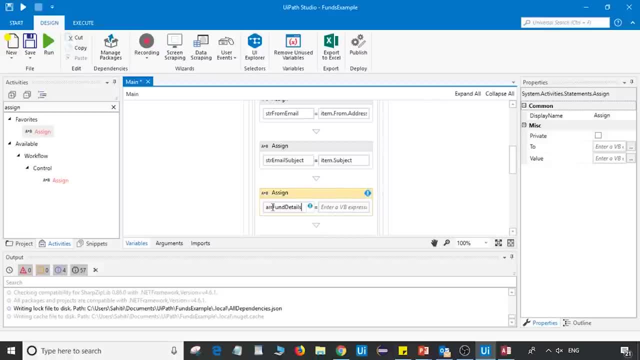 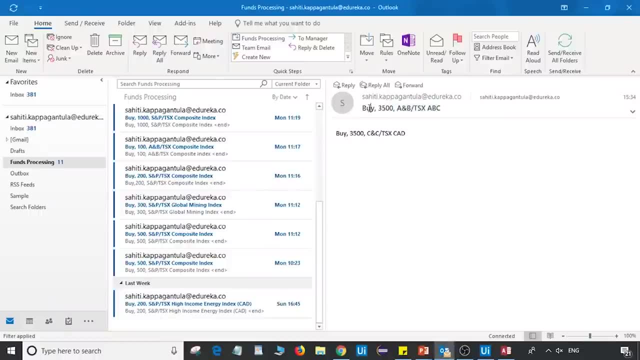 we want to store it in an array, right? So what we'll do is we'll use this array fun details and then we'll assign it to the string email subject. But yes, there's one more thing you have to remember over here. 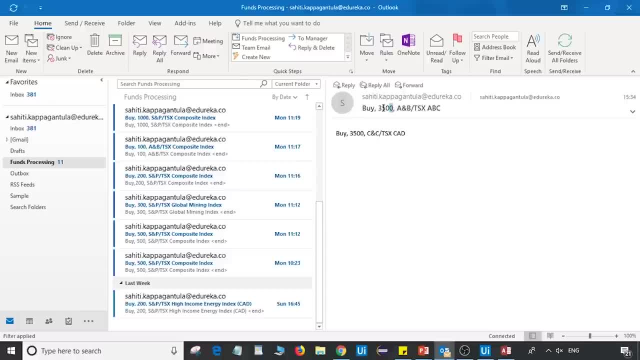 If you see, the string email subject is separated with the commas and all of them have to be stored in an array, right? So you have to mention this splitting of commas, So for that you have to use the split operator. So. 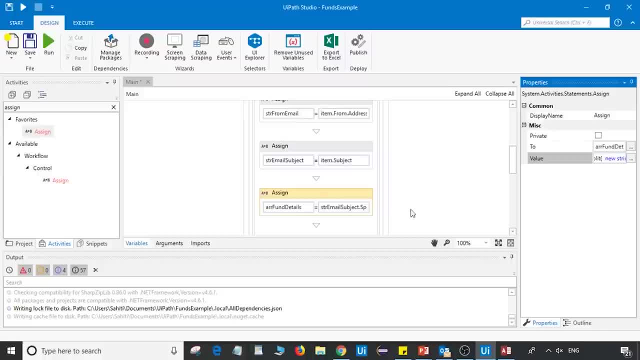 since I've already stored it over here, I'm just going to, you know, copy this and then I'm going to paste it over here. So, don't worry, I'll explain you. So let me just open this and show you. 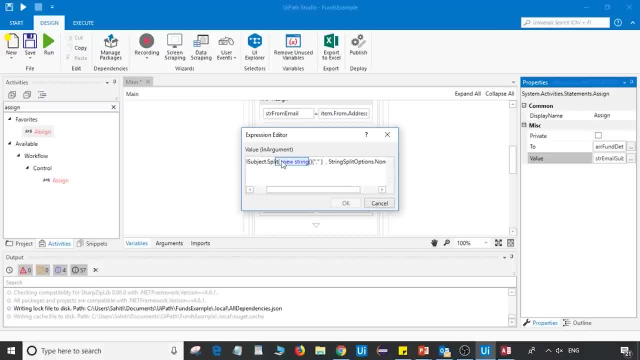 So you can see that every string or every string that is in front of the comma or after the comma would be considered as an array value. So that's what I've mentioned over here. Now, after this is done, we have to. 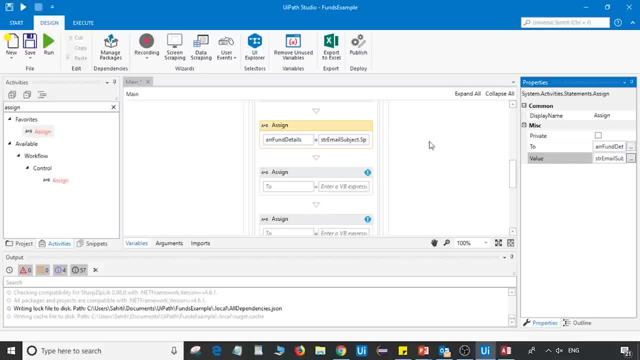 you know, store all the values into the array right Now, but before that you have to use the variable of array item count so that you avoid the exception. So I'll just use array item count and then I'll assign it to the length. 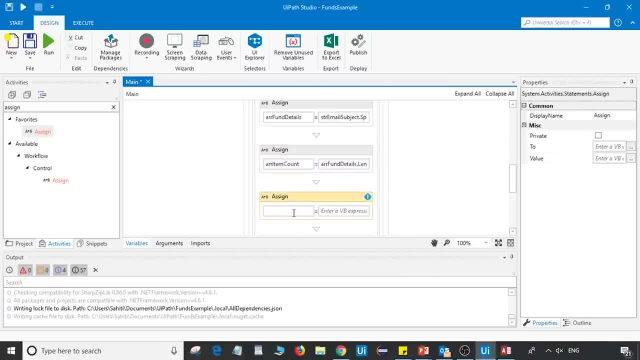 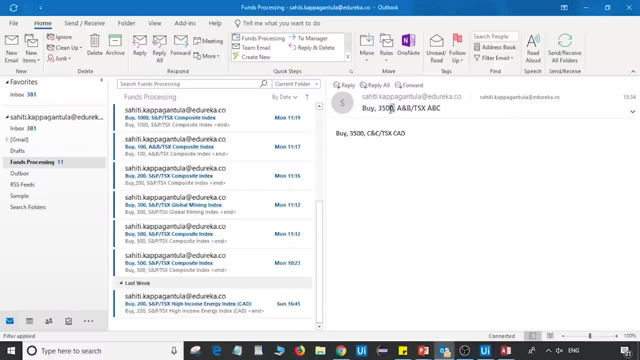 we are going to assign the values of array index 0,, 1, 2.. So when you open your outlook, you can see that you know array index of 0 would be assigned to fund transaction type. array index of 1. 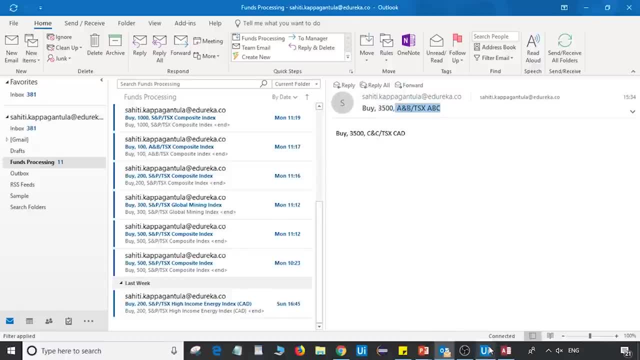 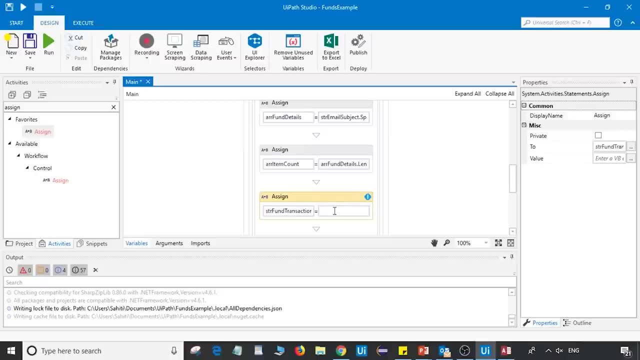 would be assigned to the quantity and array index of 2 would be assigned to the fund name, right? So let me just quickly do that. So let's say string fund transaction type would be assigned to array index of 0, right? 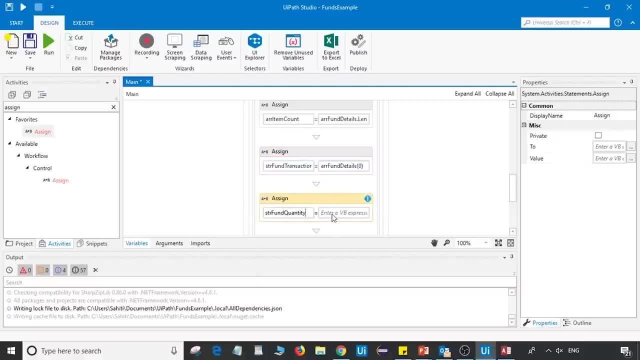 So basically you have to mention the quantity. So I'm using this fund quantity variable and then I'll use array index of 1 and over here I'll use string fund name and use array fund details of 2, right. 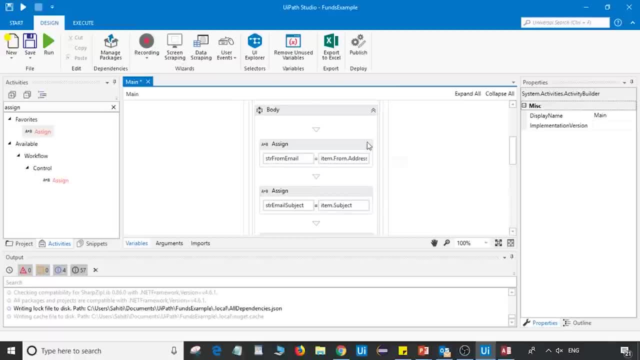 So that's how you can store basically. So this is how, basically, I've used all the assigned activities. So what I've done is, for each item I've assigned over the length of the array we have assigned the array of index 0. 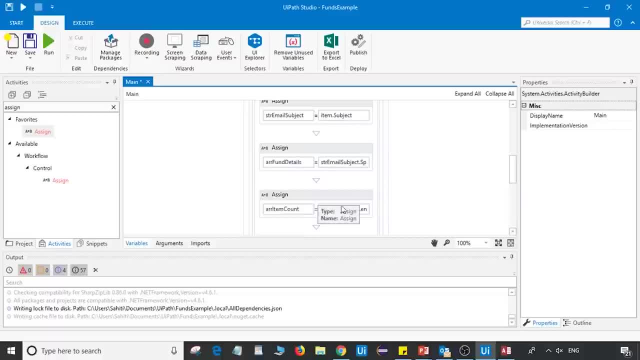 to be called feeder, and then the array of index 10 is assigned to be the name right. So the array of index one is assigned to be the name, and then the name of the item is assigned to the address and then the name of the value. 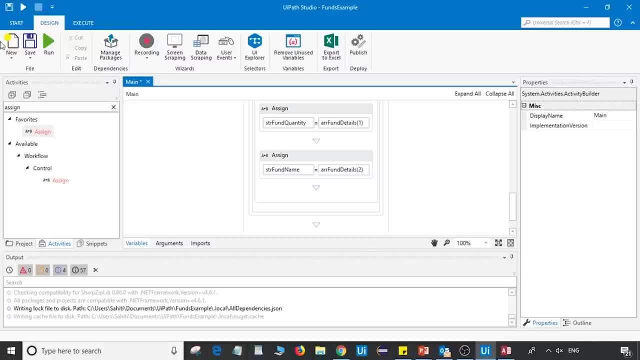 of that value is set to right. so that is basically the database that you have created. but before that you have to, you know, execute the query right. so for that, what you do is we'll first create a sequence that is basically a sub sequence, and then I'll 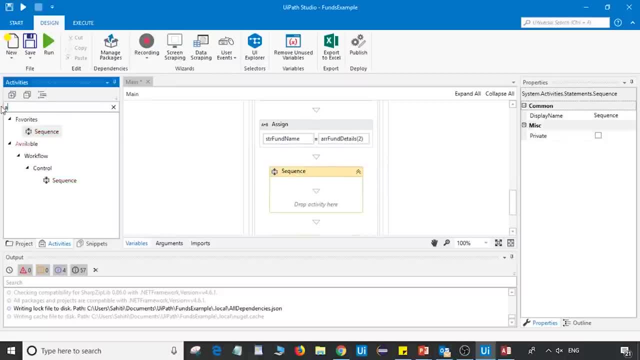 drag and drop it over here, and after that I'll just search for the assign activity and then and again drag and drop it over here. now what I'll do is I will basically assign the string query variable that I've created to be used for inserting the query. so I'll just say string query and then I'll mention. 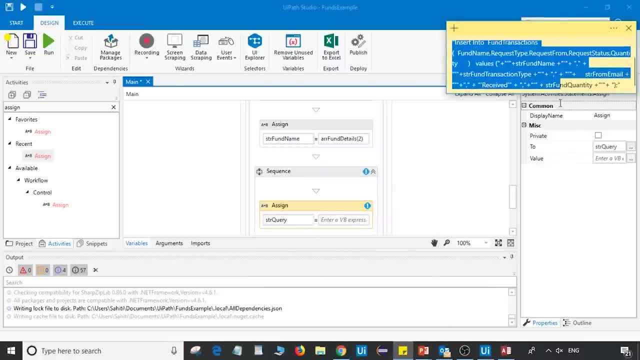 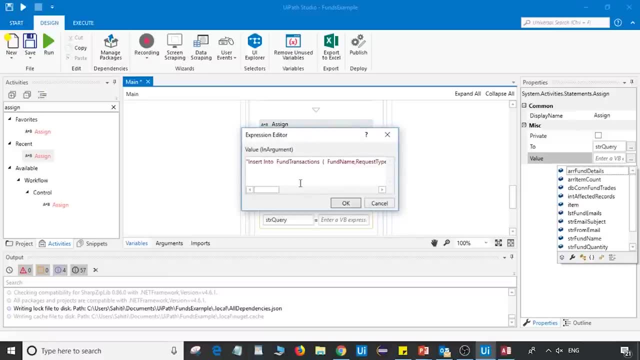 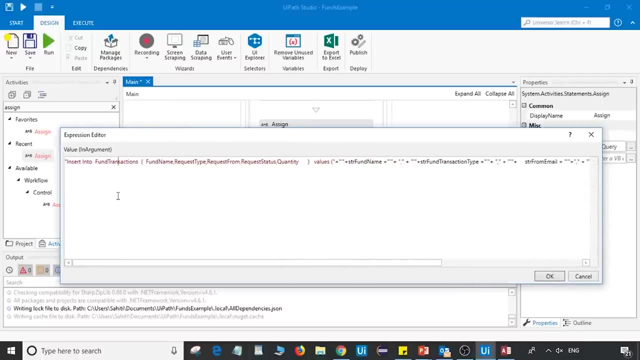 the expression, right? so since I've already saved it over here, I'll just copy this and then I'll choose this option, choose the three dots and then paste it over here. so what's basically happening is: let me just you know, expand this section so that you clearly see all right. so what's basically happening is: 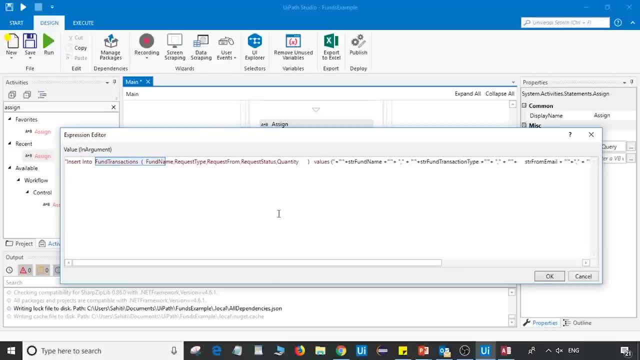 you can insert into the fund transactions. that is basically a table table of contents. that is basically a table of contents. that is basically a table name. so if you see, we have that as a table's name, that is fund transactions. so that's what we're going to insert. so we're going to insert into this table. 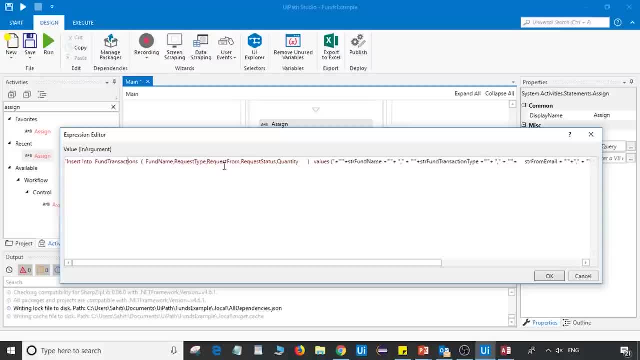 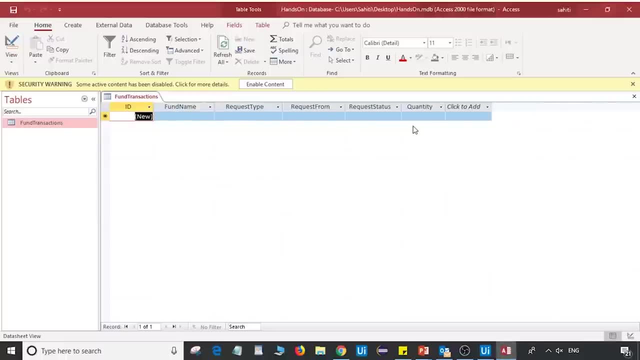 and then we have the names, right. that is the fund name, the request type, the request from request, status and the quantity. so let's just quickly check that. that is the fund name, request type, request from request status, quantity, right? so that's basically the columns that we have now. we'll use the keyword. 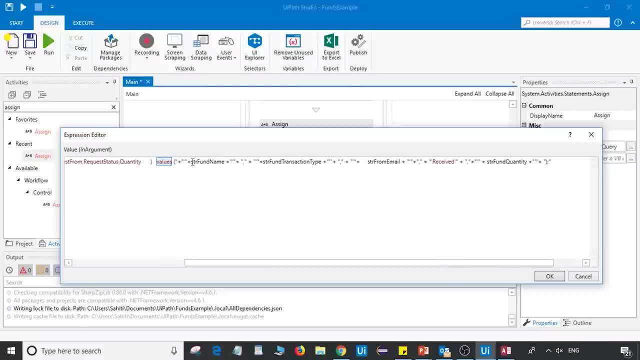 values and then over here we'll mention all the values, right? so since we do not have any static values and all the values are static, we'll just say that all the values will be assigned to the variables. we have mentioned all the variable names that we've used, that is, the fund name, the fund transaction type. 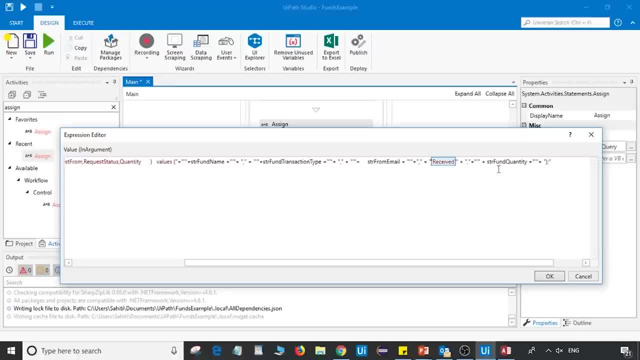 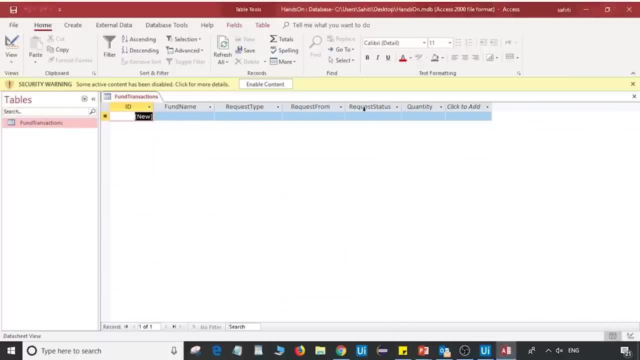 the front email and then we've used this keyword received and fund quantity, so this received text is used to as a response to this particular request status column. so as soon as you know the information is, you know, received into this database. that is basically. we get all this information. we also get a. 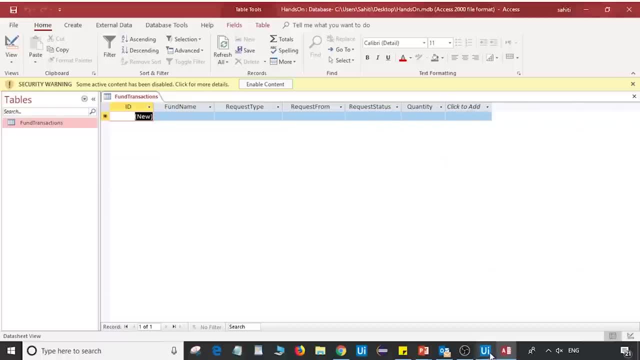 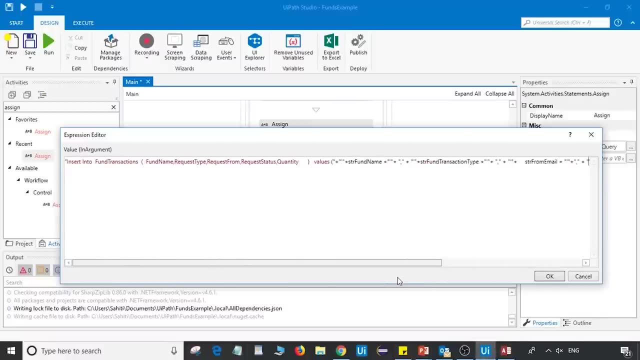 response status, that unit is received and the quantity would be displayed right. so that's how you know you can insert this. you can use this query to insert values into the table. so if you have to understand in simple SQL form, it's basically insert into the table's name. 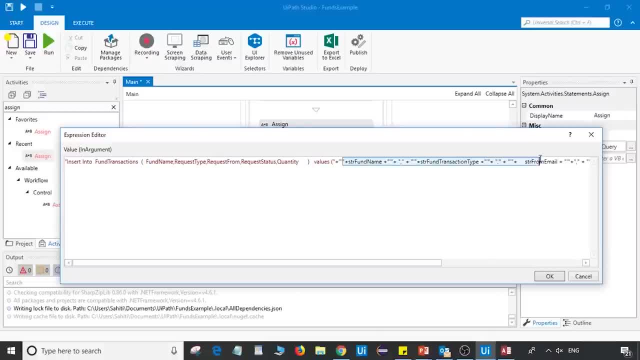 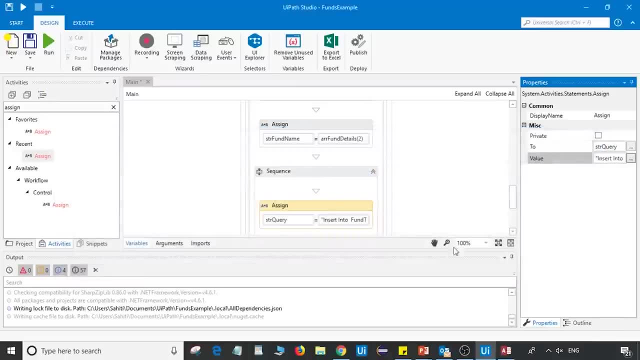 and you have the columns name values and you have all the values which have to be inserted into the respective columns, right? so I hope that I'm clear with this. now I'll just click on. ok, and we have. you know, we've put the query. now we've. 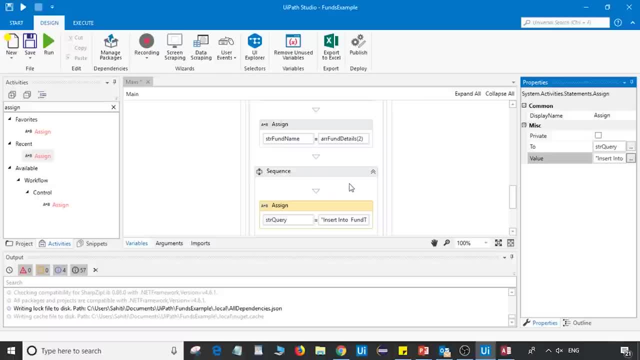 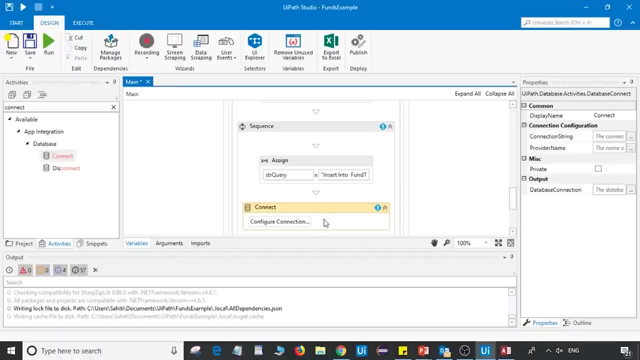 all, we have just assigned this query to a specific variable, right. but before this query starts running we have to connect to the database. so for that you will use the connect activity. so I'll just search for connect and then you'll drag and drop it over here. so once you drag and drop it over here, you have to. 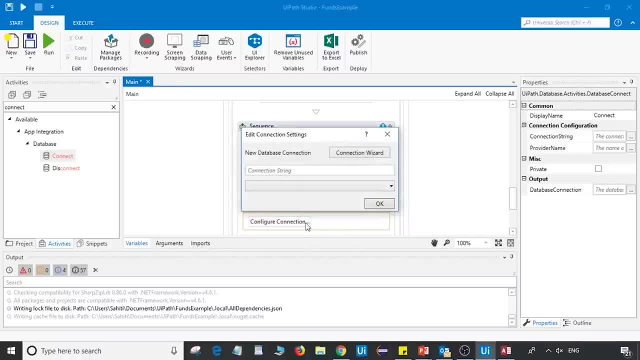 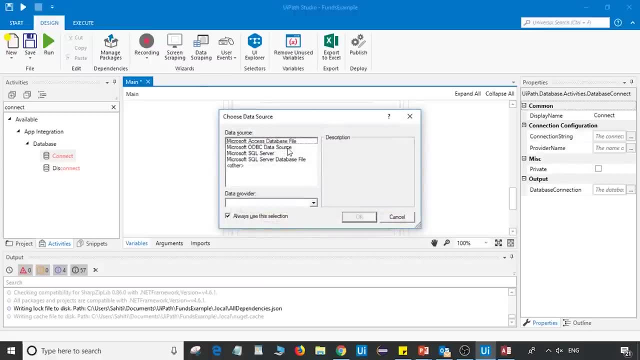 configure your connection right. so you'll just choose configure connection, you'll go to connection wizard and then you'll choose Microsoft Access database file. I'm choosing this file because I'm using an MS Access database file. well, if you're using any other data source, like the ODBC data source or the SQL, 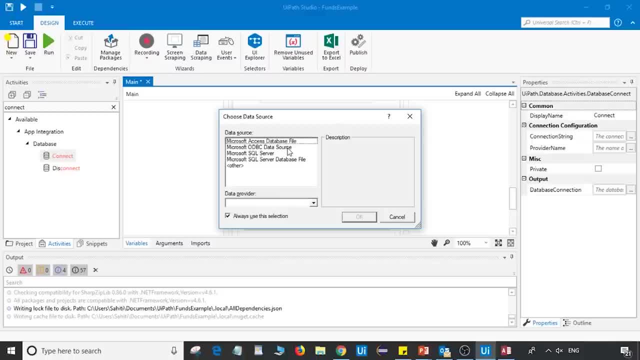 server or the SQL Server database file or the SQ αν any other file, then you can use uh with respect to that. so i'm going to use microsoft access database file, so i'll just choose this option and then i'll click on ok. now, once i click on ok, i have. 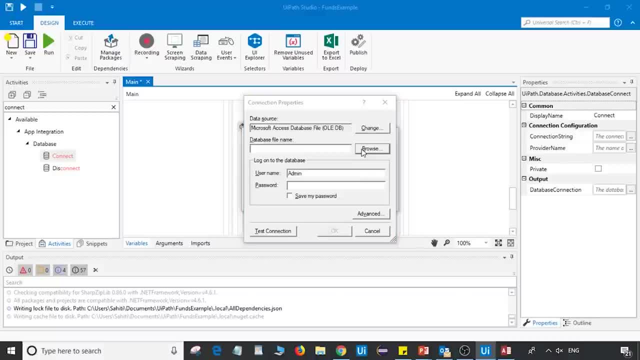 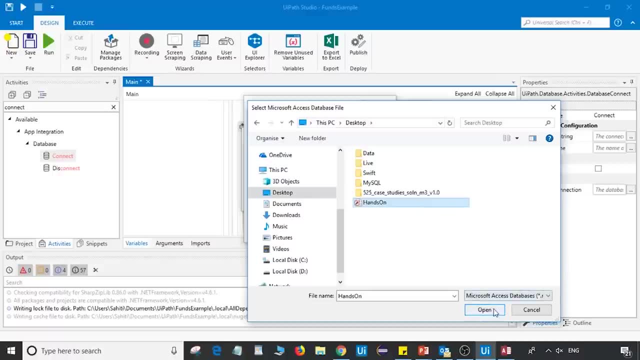 to connect to the database that i previously created. so i'll go to browse and then i'll just go to desktop and choose hands-on. that's what i created, right? so i'll just click on open. so once i click on open, you know we have given the part to the database file name. now, after that, you can. 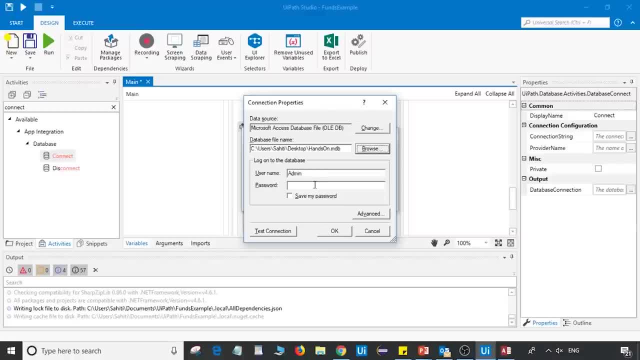 also mention the username and password to make sure you know your database is secure. in this section i'm not going to do it, so i'll just click on test connection after that. so if it says test connection succeeded, that means your database is ready to get connected to the ui part studio. 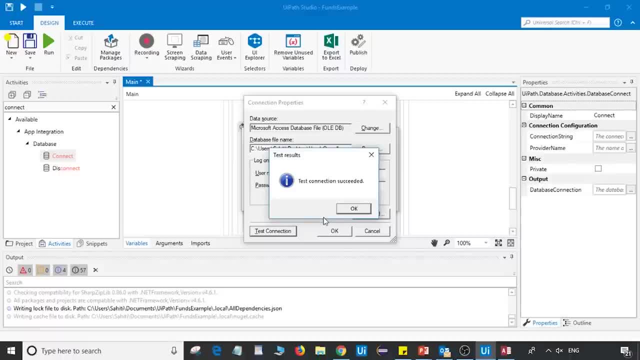 right. so now, in this scenario, you know, if you get an error that you know the ui part does not recognize the database, or you know the database format is not recognized, that means there's a problem with your access version, right? so you just change your access version, which is compatible. 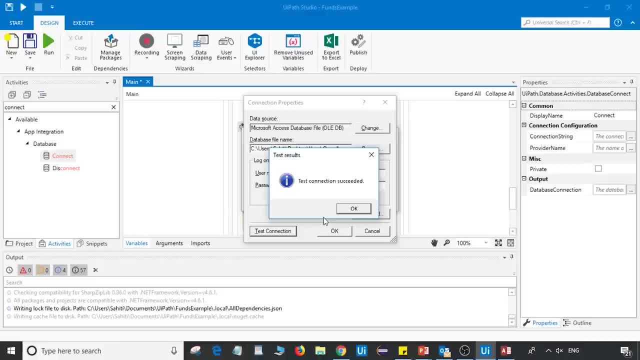 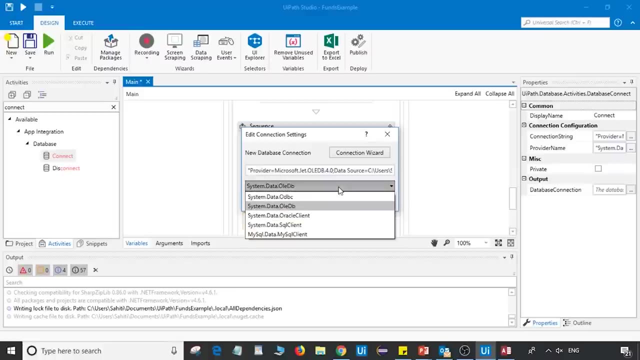 with your ui parts studio's version, and then this connection would be successful. so, since our connection is successful, i'll just click on ok. now, once i click on ok, i'll again click on ok and then i'll choose this option to be of systemdataoledb. so well, i'm going to choose this option because i'm using a microsoft. 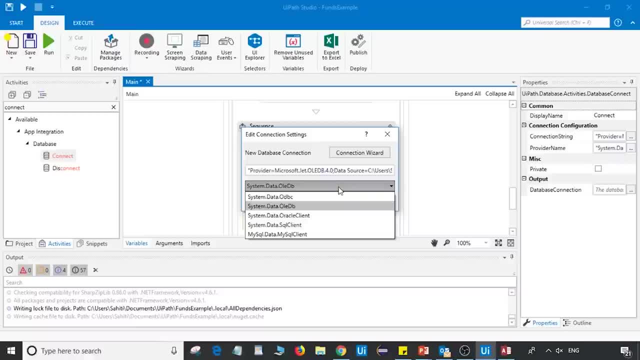 access database file. if you were using an oracle client or an sql client, or if you were using an mysql database, then you would choose the options accordingly. so i'm going to choose this option and then i'll click on. ok, all right, so let me just quickly. 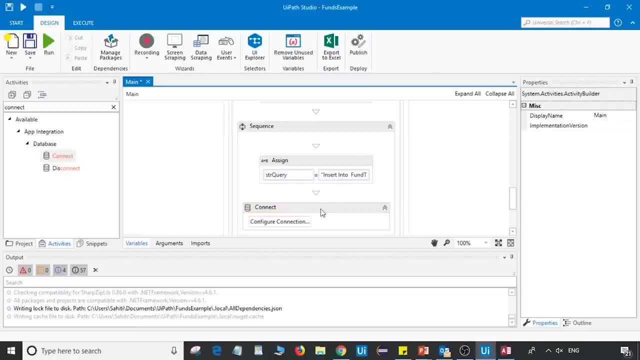 choose it again. it was not selected, all right, so that's how you know you can connect. now in the output section you have to mention the database, which has to get connected right. so over here, what we have done is we have mentioned the path of the database, we haven't mentioned the database. 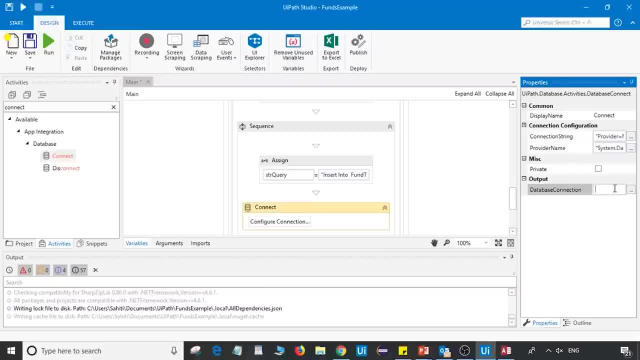 variable name anywhere, right? so that's where you have to connect. so in the output section of the connect activity you can just, you know, mention the database. so i'll just mention the database: connect fun trades. that is basically the variable that is used to create the database and over here. 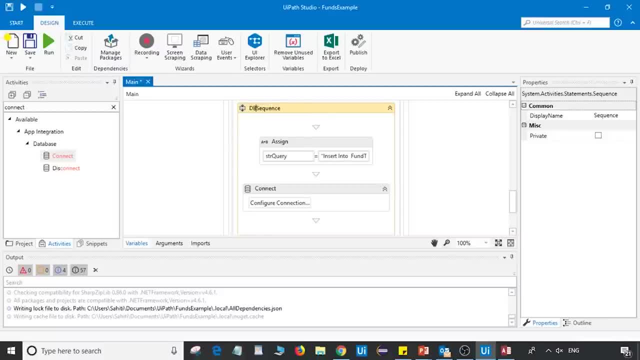 say: you know i'd rename the sequence so that you know it's clear. so i'll just type in db connect sequence, right? so that's basically. it makes it clear for you guys to understand what exactly we're doing in the sub sequence. now, once your database is ready to get connected, what you also 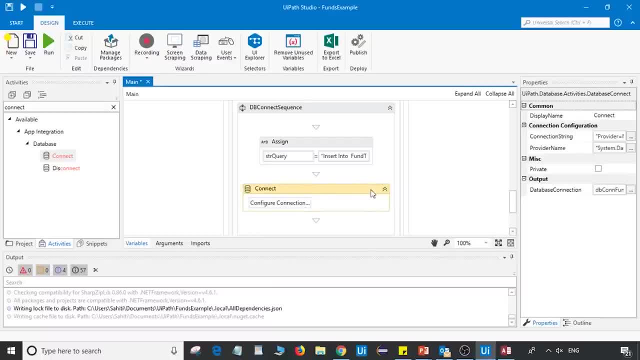 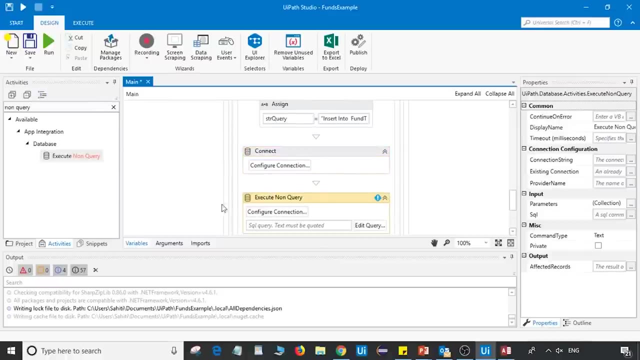 have to make sure is that you know your query is executed. right now, since we've, you know, assigned our query to a variable, we can use a non-query to execute. so we'll just use non-query execute activity. so i'll drag and drop it over here. so, in this section, what i'm basically going to do is i'm going to 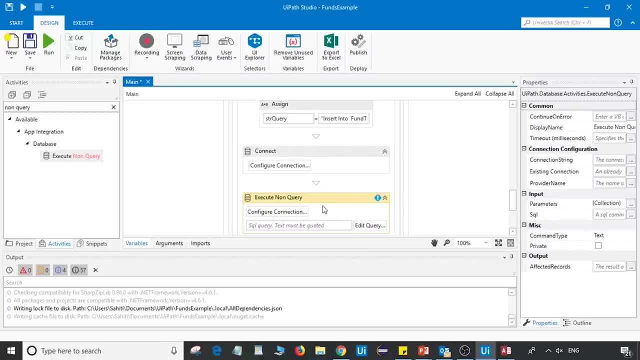 execute my query. i'm using this activity because i'm executing a non-query right. my query has been assigned to a variable, so i just have to mention that variables name. so i'm going to mention the variables name, that is, str query, and then in the properties section i have to mention the. 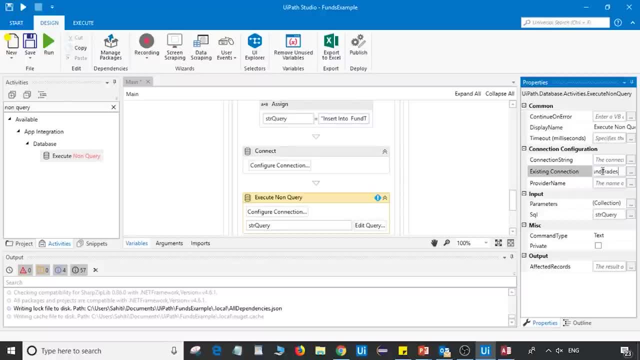 database name. that is basically the database connection fun trace. that is the variables name. and then what we're going to do is, in the affected records, i'm going to mention the int affected records output. so that is what the output that we're going to mention right, this variable will. 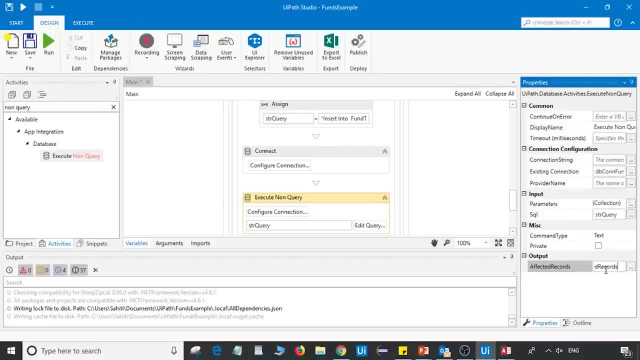 basically give you the output of all the values that were inserted into the database. right now, once this is done, let me just quickly, you know, make sure that you know you can print these values, that you know you can view all the values that are inserted into your table right. so for that you'll. 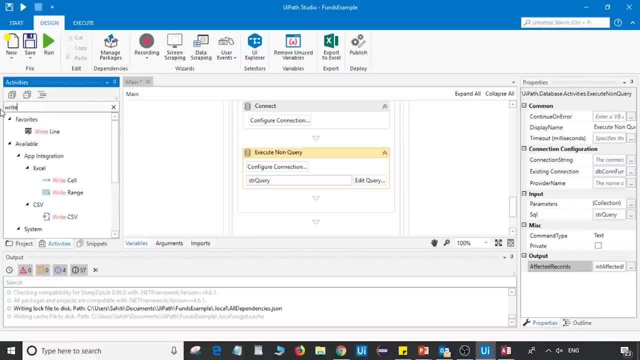 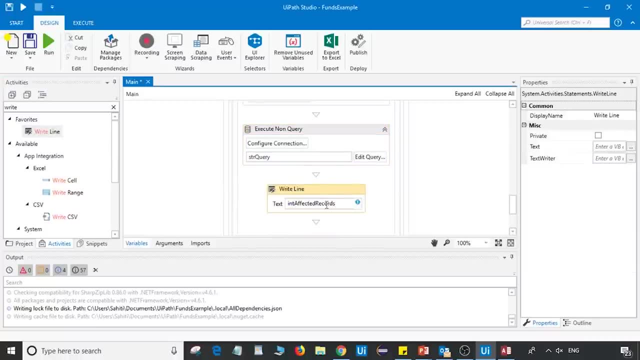 just insert a right line activity and then you'll say int affected records- that is basically our variable name- and convert it to string because it gives an output of a string value, right? so this is how you know you can create your complete sequence to automate these tasks. so let me just give you a 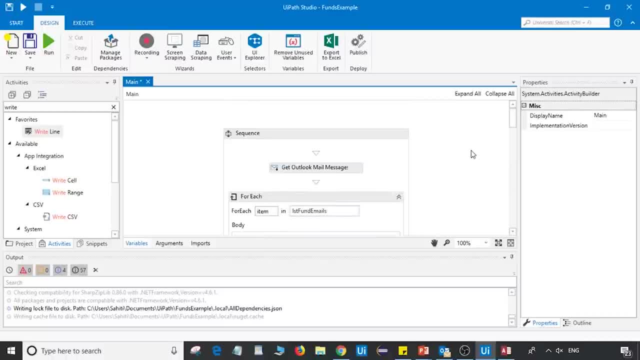 review of all the steps again. so we started by creating a database, that is the ms access database, and after that we made sure that you know, our outlook had few mails and we made sure which folder had consisted that mails. after that, coming back to the ui path studio, we created a sequence. 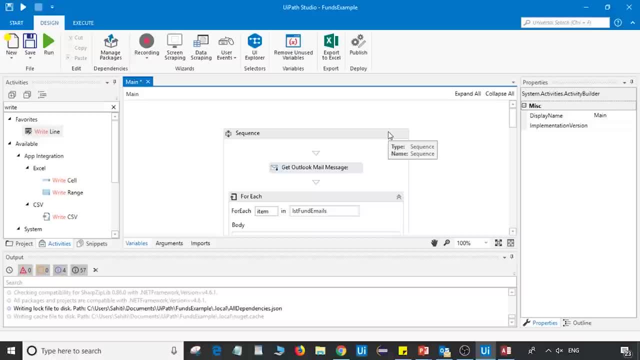 inside, which basically all the tasks, or you can mention all the actions that would be performed, and after that we started with the get outlook mail message. so here we mentioned the account that is basically my account over here, and then the mail folder through which it has to be read. 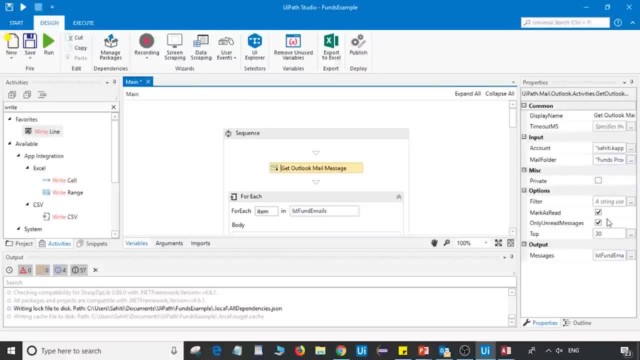 and i've also mentioned the filters- that is, the only unread messages, the mark as red and the top 30, right? so basically what would happen is only unread messages would be read and once they're read, they would be marked as red and only top 30 would be read. after that, we mentioned the output. 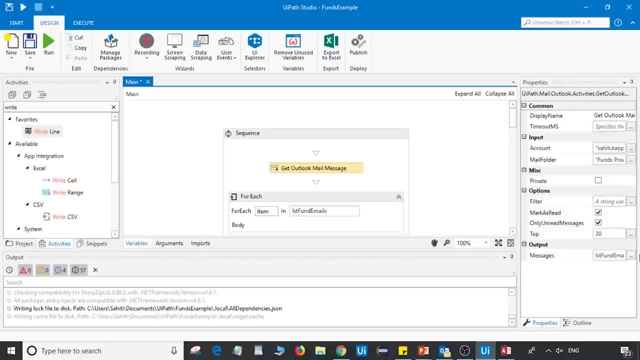 to be of list 1 email. so all this output would be stored into this particular variable. now, for each item in this table, we are going to create a new item and we are going to create a new item in this one: emails. we wanted a set of actions to be performed, so i've mentioned a for each loop that. 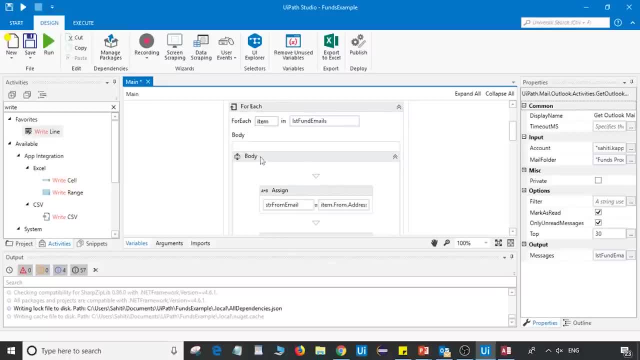 is basically a for each workflow over here, and then in the body section we use various assign activities, right? so we wanted the from email address, the subject, the fun details, and then we use this variable, for you know, to avoid the exception. then we also store the array index. 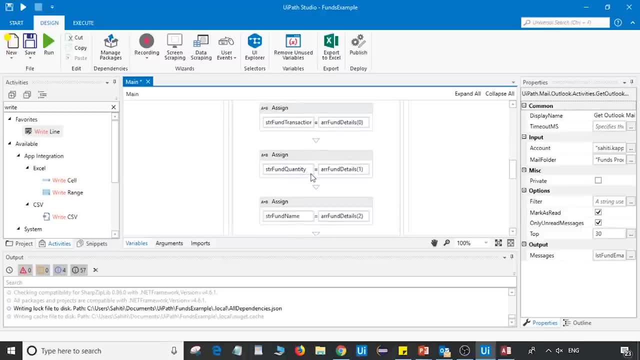 values into the assigned variables- that is basically the fund transactions, fund quantity and fund name. and once we have assigned all the variables- that is basically all the values- to the variables, we had to make sure that we had all the variables that we had to make sure that we had all. 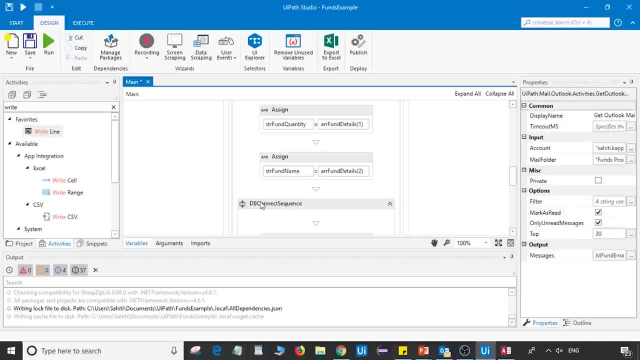 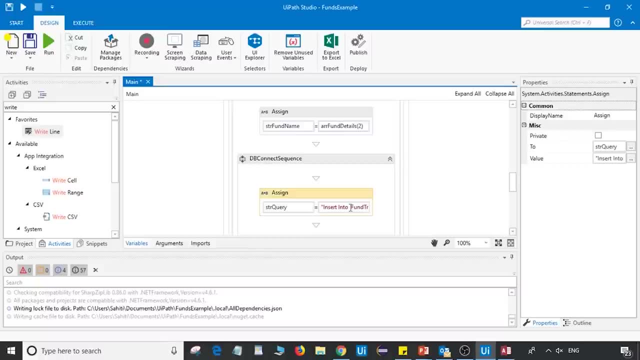 the variables we had to connect to our database right. so for that we created a new sub sequence, that is the database connect sequence, inside which i put in an assign activity to which i inserted the values right. so i've mentioned basic. i've basically, you know, mentioned the query. so if 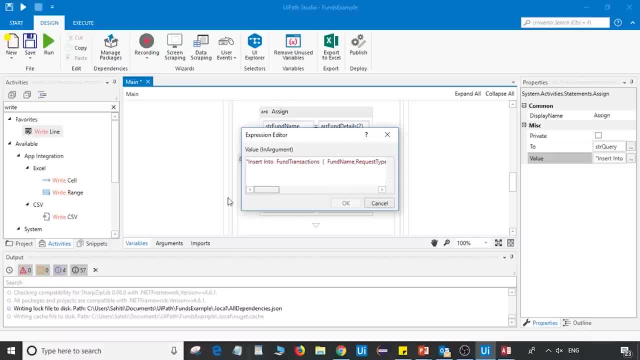 you see over here, i mentioned the query to be insert fund into fund transactions and the values right now. once that was done, we had to connect to our database. so i just configured the connection and then our query would be executed. once our query would be executed, we 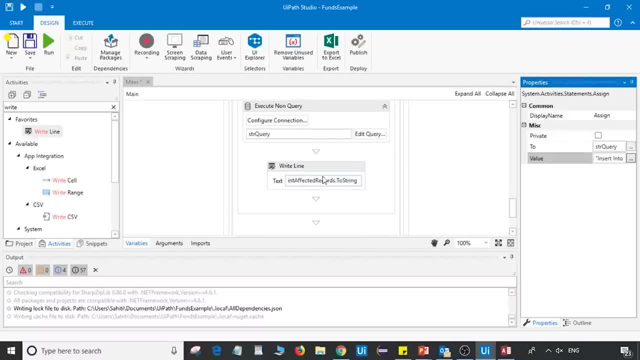 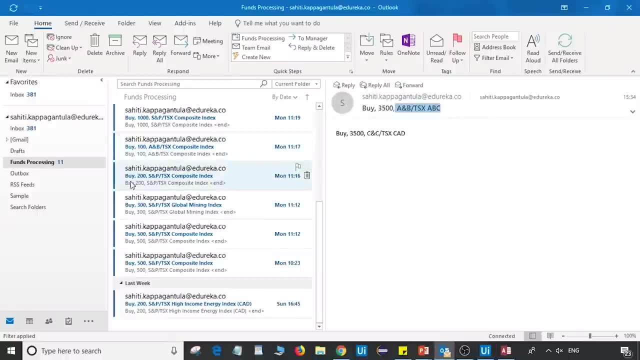 wanted the output to be printed, that is, the output to be visible. so we just use the right line activity. so i hope you know. the sequence was clear to you right. so now let's just quickly check if our outlook has some unread emails so you can see that. you know our outlook has few unread emails. 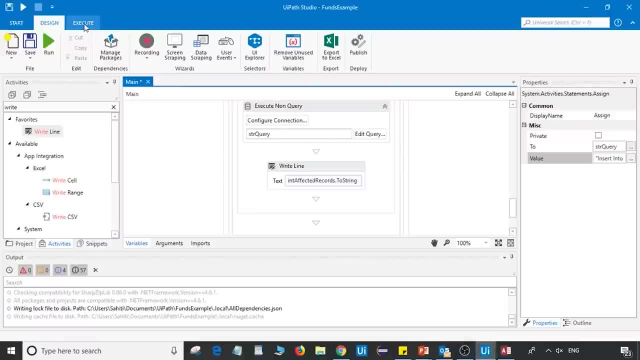 so now i'll just quickly run this sequence. so for that i'm going to go to execute and choose debug. so i'm choosing debug because you know, even if you have any error, then you can clearly understand which step is giving you an error and then you can quickly solve it and you can understand the. 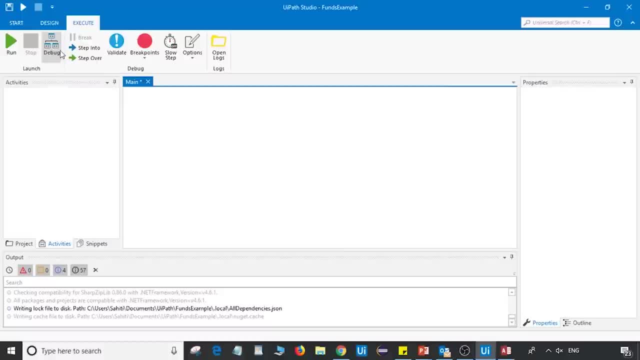 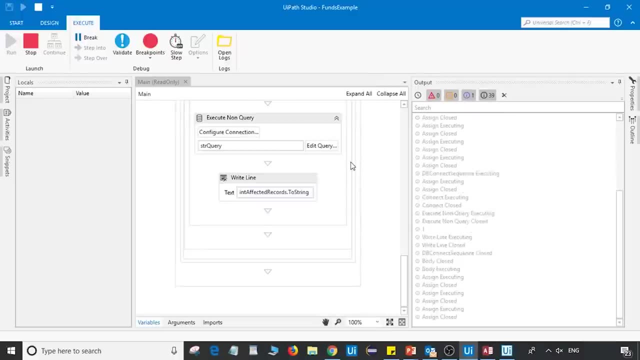 workflow of each and every step, right? so you will just choose debug so you can see that you know the debug has started. that means our program has started executing. once it executes, you'll see that you know it automatically closes and you just go back to your dashboard, right? so let's just wait for that. 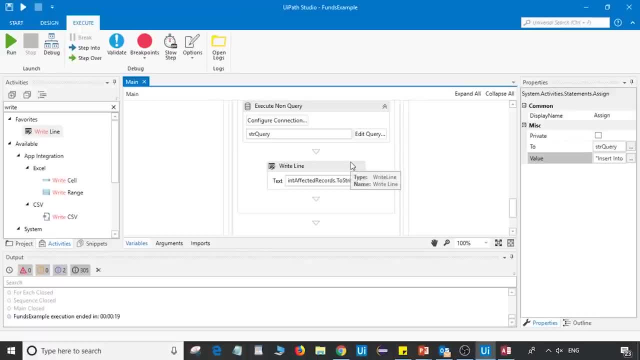 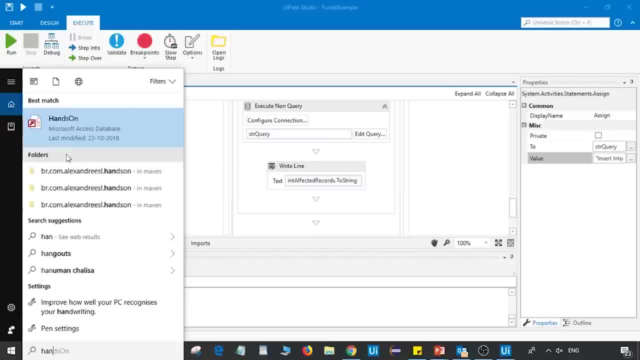 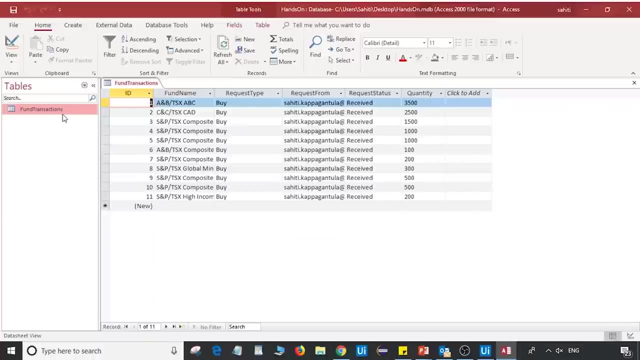 all right, so you can see that you know our execution has completed, right. so now let me just quickly close this particular hands-on database and now we're going to open it again so that we see, we see the output. so i'm going to enable content and i'm going to enable the table's name. all right, so as you can, 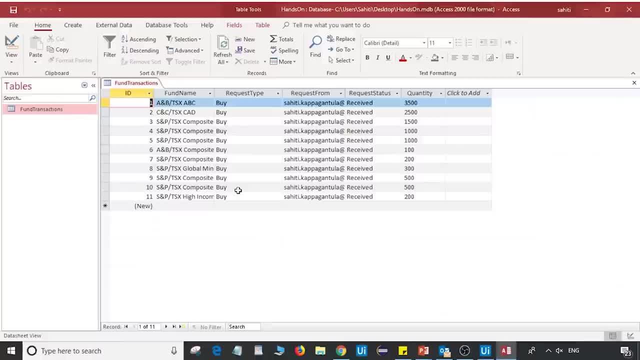 see that you know all your data has been retrieved to this particular database, right. so you. we stored the fund name, the request type, the request from the status, the quantity, right. so all the id was generated automatically as and when the mails were read and the information was stored: the fund name. 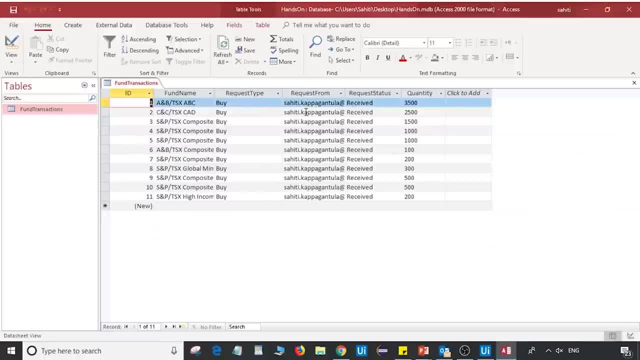 the request type was taken from the email subject. the request from was basically the from email address, since i had sent it to myself. i'm sorry, since i had sent it to myself, my email address is visible and then the status is received. that means the information has been received and. 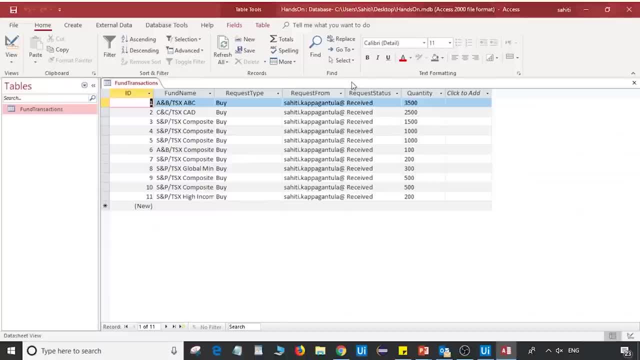 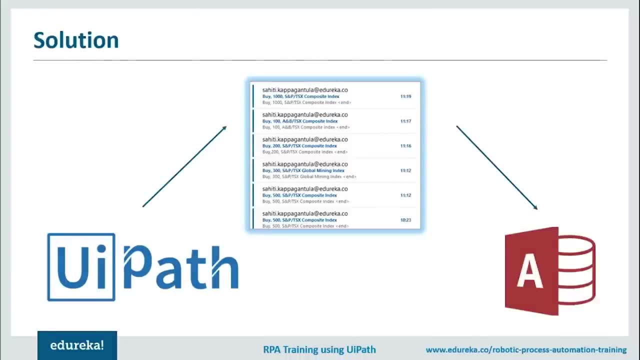 the quantity is also mentioned, right. so that's how you know. i think you know you can automate your task and make sure that you know the team did not have to do such humongous tasks manually. i showed you an example of around 11 emails. but, yes, you can do the stars for you, the thousands. 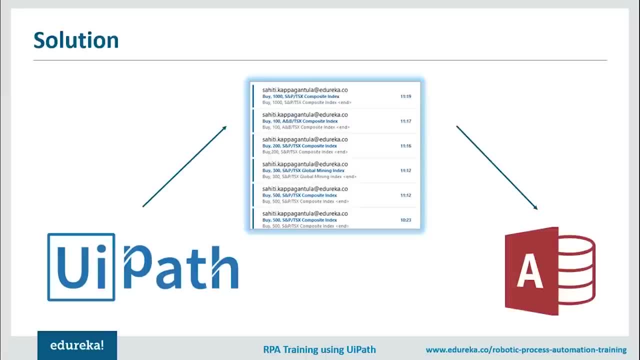 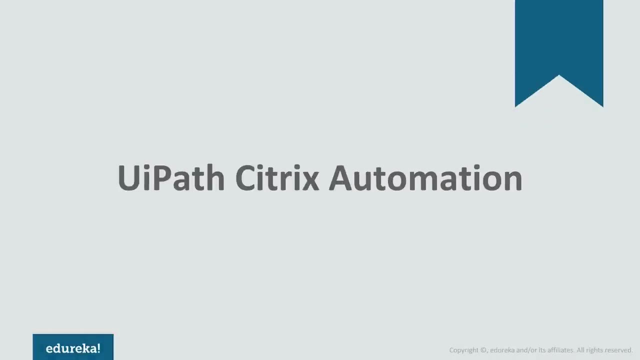 of emails at a large production scale, so that you just don't employ people who just have work to, you know, manually sit and process emails and then waste the time and energy. right, so you can just automate this task and this happens quickly and this saves you time. also, the screen is a 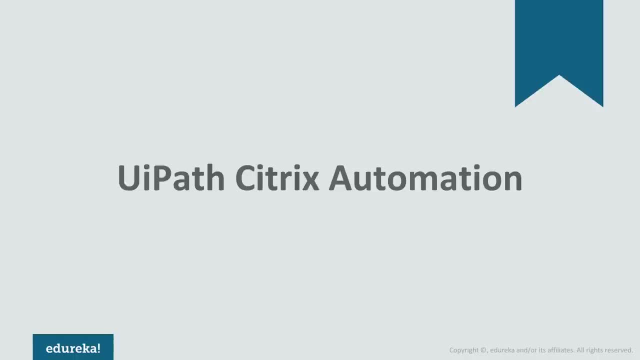 window through which one sees a virtual world, and if you have to automate your tasks in this virtual world, then you need something known as citrix automation. now that you know what rpa means, a question may come onto your mind on: how do we automate tasks on virtual environment? 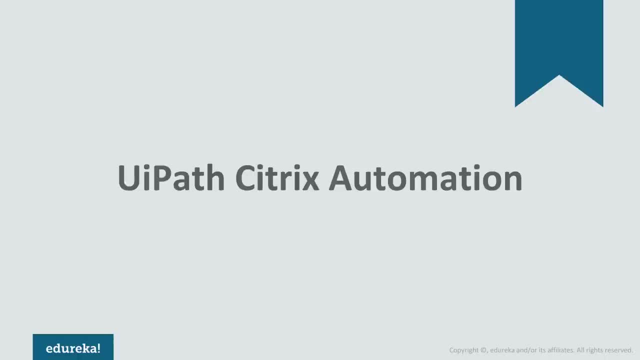 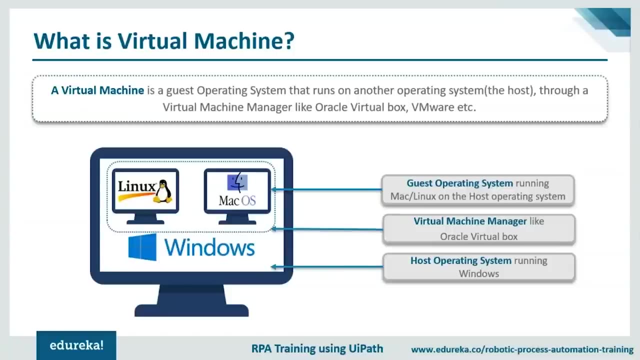 but before getting into how to automate tasks on virtual environment, let's see exactly what virtual machine is. so, if you talk in layman terms, any machine that is remotely located or any kind of machine that is created inside your computer is set to be a virtual machine. all right, so now? 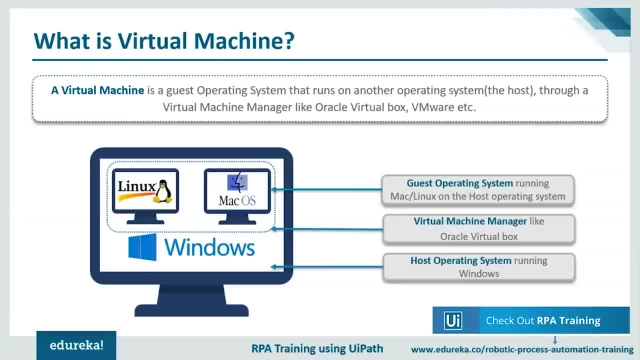 let's look at a virtual machine now. with that просто 좋아 on the machine, we are inside a virtual machine, alright. so let's look at a virtual machine, all right. so now let's look at a into a proper definition of what virtual machine is. a virtual? 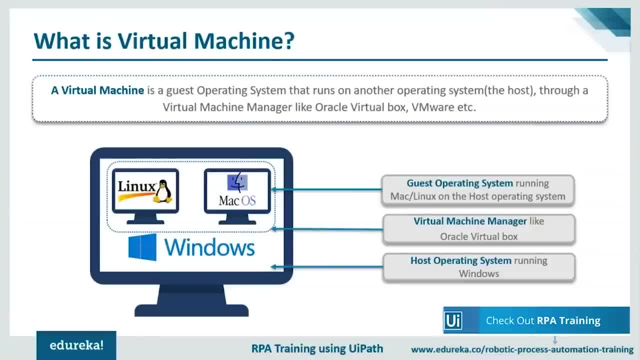 machine is a guest operating system that runs on another operating system to a virtual machine manager. This virtual machine manager could be a Oracle virtual box or a VMware Etc. So if you talk in real-time scenarios, most of the time you have servers or any company operating online to host a. 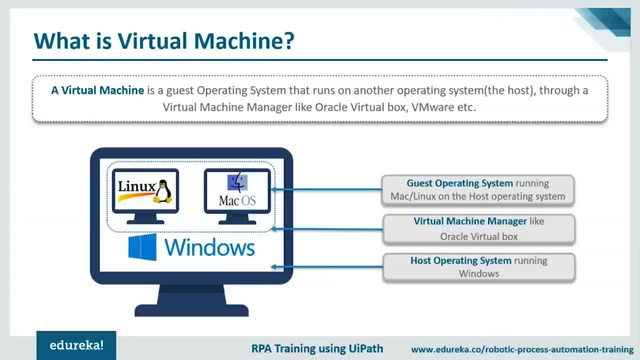 website somewhere. So the somewhere is basically the server. usually what happens is you take the server on the cloud and whenever you want to access that server, you can access it using the remote desktop connection. So in this kind of scenarios, if you want to automate anything, 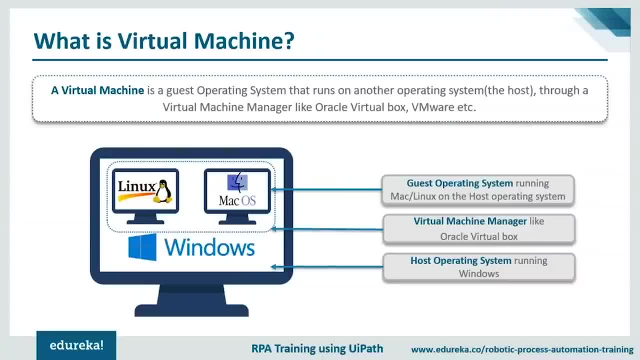 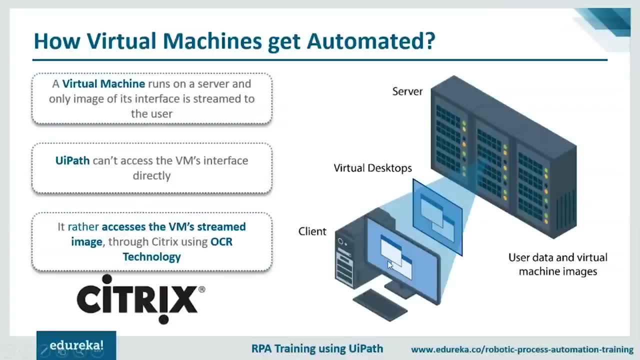 on your virtual environment, then you need Citrix automation. So what exactly I'm talking about? Let's look into it. It basically implements a Citrix technology with this, All right. So basically any server that you're trying to access on your 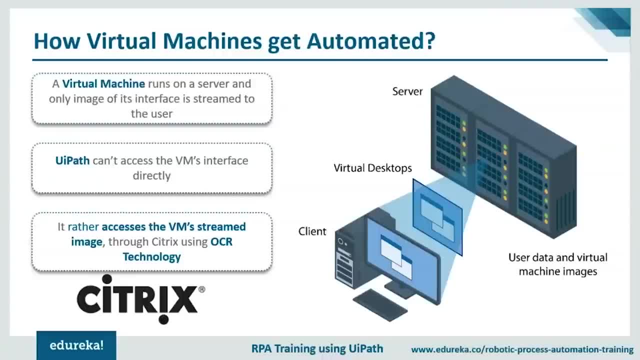 computer, You basically get the image of the screen of the server right now. What happens is, whenever you click on something, that image or pixel is sent to the server and then in that server it is exactly clicked over there. So if you talk in the technology terms, this is the process. 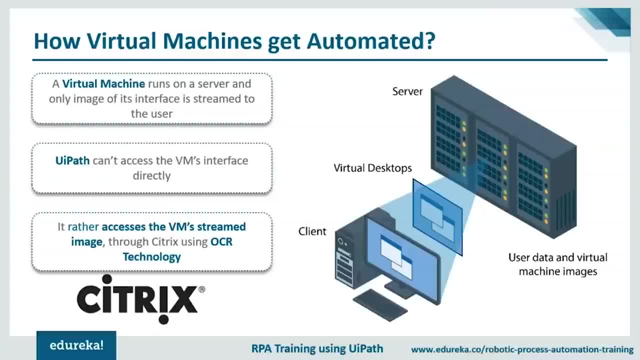 for automation of remote desktop connection. All right now. the same process is applied even if you have a virtual machine. So if you have a guest operating system on your own operating system, for example, if you have hosted Ubuntu on Windows or Mac on Windows or any guest operating system. 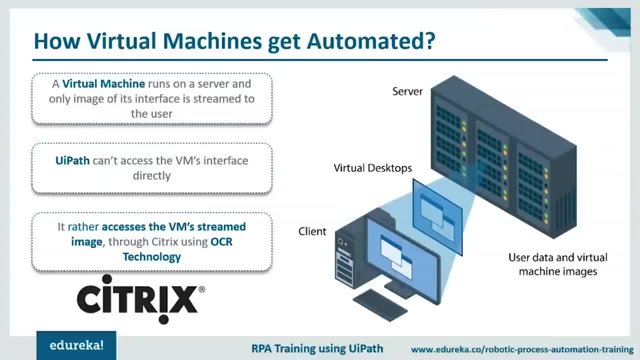 On your own operating system. What you get is you get a screen and then inside that screen you work. So if you host Ubuntu on Windows, you get an event to screen on which you have to work. So similar to the remote desktop connection you're getting. 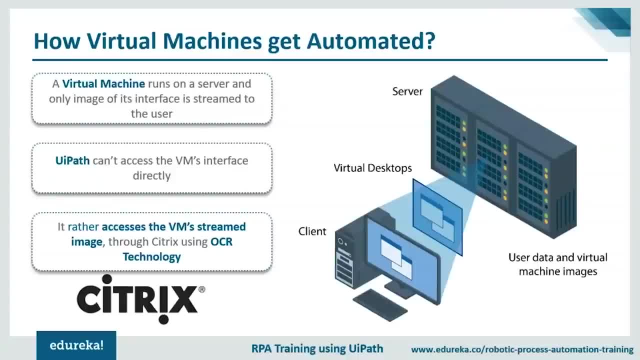 the images and on those images you're clicking on something. So whenever you click on something, those pixels go to the actual screen of the actual operating system. Now, when you want to automate this kind of stuff, that is, if you want to automate working on a server from your own company, 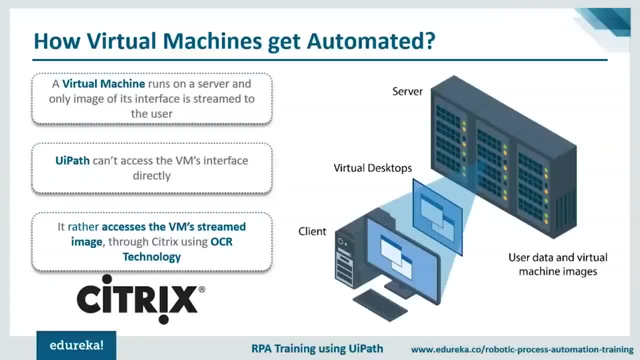 Computer or you want to automate something that is connected with the remote desktop connection or that is connected to the AWS server or any kind of stuff. You can do it by using the uipath studio, and then the technology which can do this is the Citrix automation, so you can collaborate. 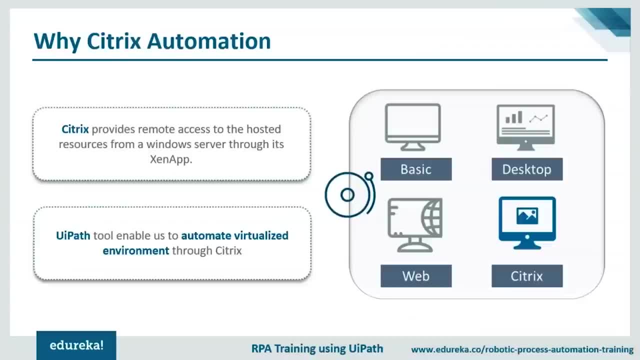 using the Citrix automation with the uipath studio. Now you might be wondering: why are we using a different technology right? Why do we separately need Citrix automation? Why can't we just do it with a simple recorder on the uipath? 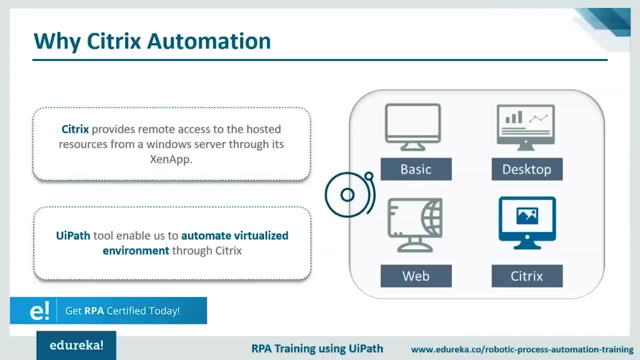 studio. So, as I told you before, when you work on virtual environments you only get images right. You do not get elements or objects. So uipath studio offers basically four types of recorders, that is, the basic desktop, web and Citrix. 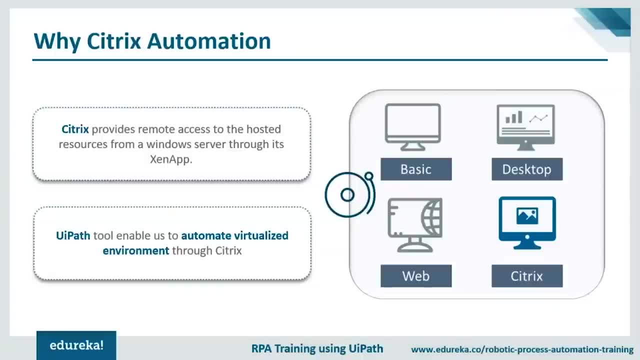 Now, the first three recorders are for recording actions manually, that is, you cannot use these recorders to record something on the virtual machines. But if you look into the fourth one, that is, the Citrix, this can be used to record actions on virtual machines. 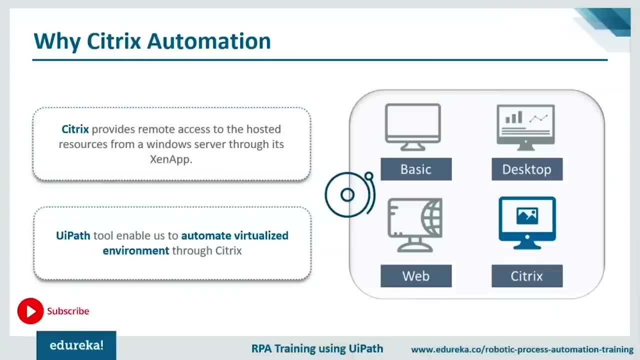 But there's one limitation with this recorder: You cannot automatically record a set of actions and have them played back. You have to hold the robots hand and show them what to do, at least for now. So how do you do that? Well, you just have to try to teach it how a human does. 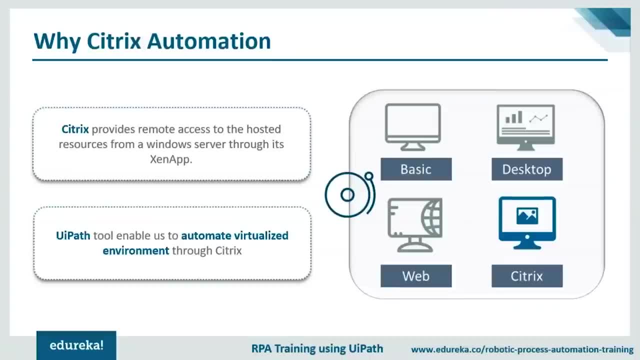 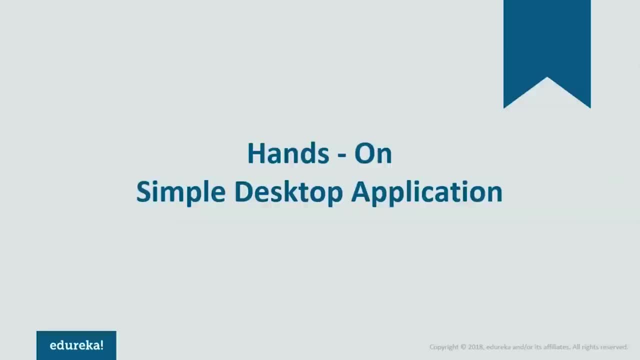 by finding elements on the screen like buttons or text fields, or doing something in relation to those text fields by clicking on controls or using the keyboard shortcuts. right. So now let's see a practical example. So we're going to first start by automating text. 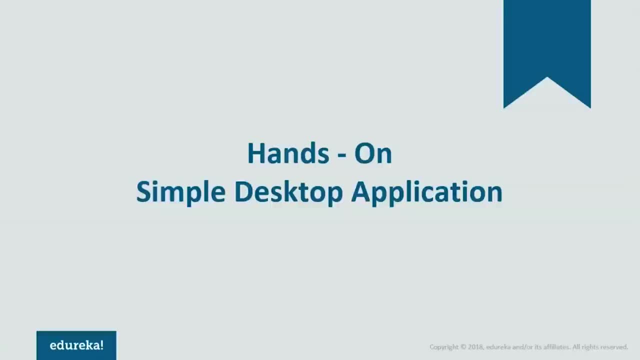 Text and image in the virtual environment. So suppose, if you want to open a notepad file in the virtual environment and you want to type in something, how will you automate that task? So let me just open my uipath tool and show you how can it be done. 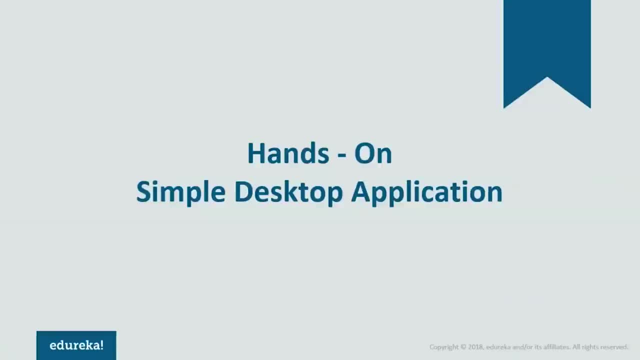 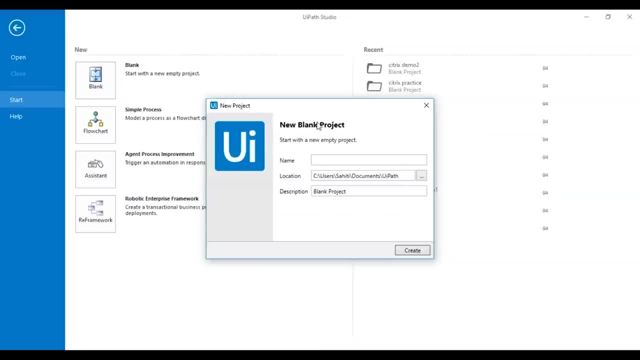 So let me just go back to my uipath tool and open it. So let's say I create a blank project and let's say I put the name as Citrix demo, right? So let me just type in Citrix demo and click on create. 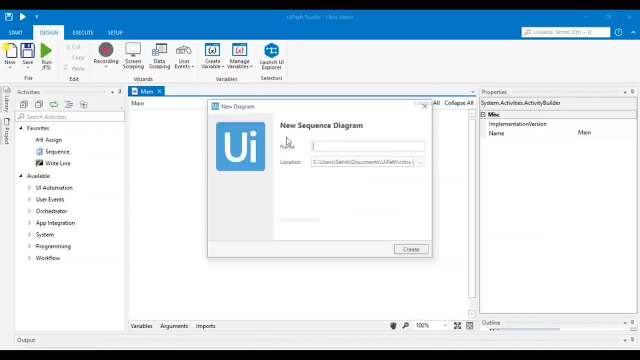 All right, Now let me just create a new sequence here and name it demo one and then create it. All right, So inside this let me just drag and drop a sequence in which basically all the activities would be recorded. All right, Now, let's go to the recording tab. 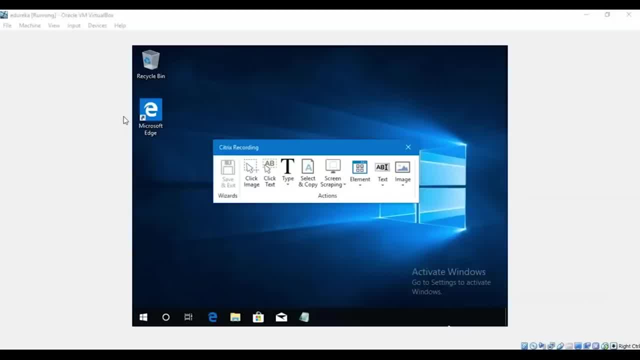 and choose Citrix recorder, right? So let me just choose a Citrix recorder and then you can see my virtual environment. Now what I want to do is: I want to open a notepad file and I want to type in something over there, right? 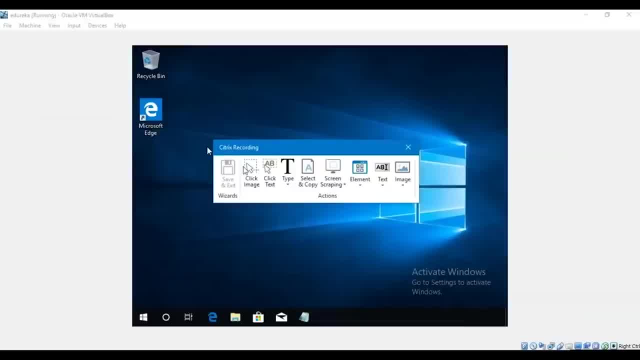 So how will I Automate that task? So for that you have to choose the click image option and then go to the notepad icon, right. So I'll select this notepad icon. Once I select that, I'll click on Okay. 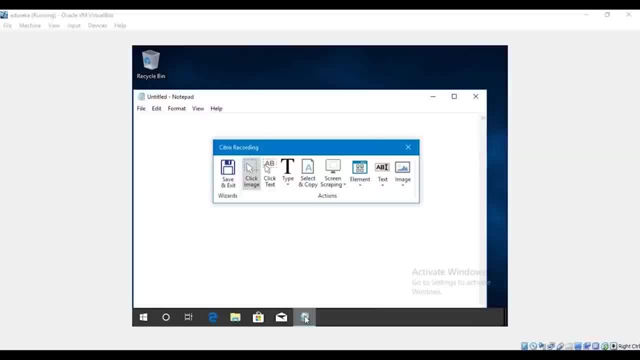 Now this will open my notepad file for me. after that I want to type in something, So I'll choose the type in option and then I'll mention the region where I want to type in. So suppose I want to type in here. 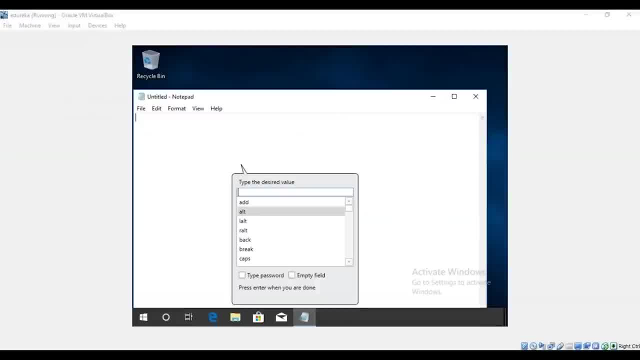 I'll mention the region here and then I'll mention the text. All right, So let's just say I mentioned the text, as hey everyone, And then I'll click on enter so you can see that our text is entered in our notepad file. 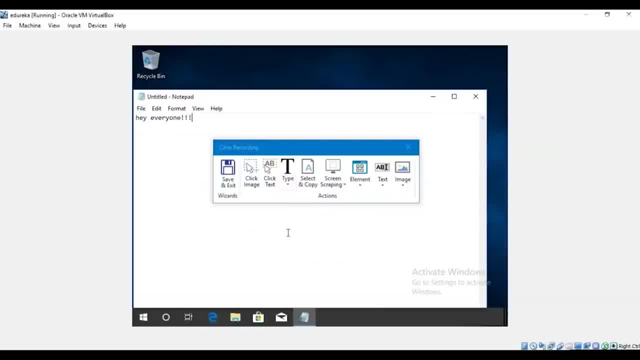 All, right Now. if I want to close the notepad file, I'll choose the option click image and mention the region across this cross button right. So let me just do that and then I'll indicate on the screen. So this will give me an option to save the file or not. 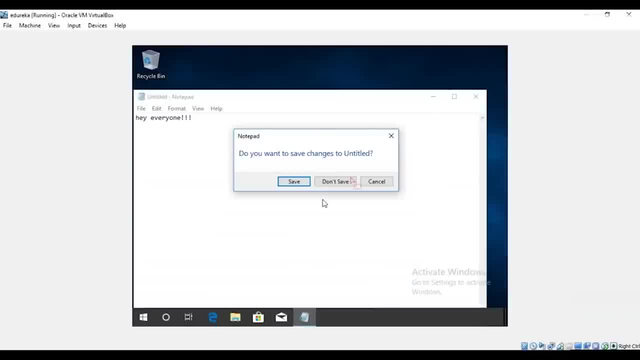 So, since I don't want to save this file, I'll choose the option for don't save, right? So I'll click on the option of click image and then select this region. Once I choose that, you can click on OK. So this will not save my file and it will close my file. 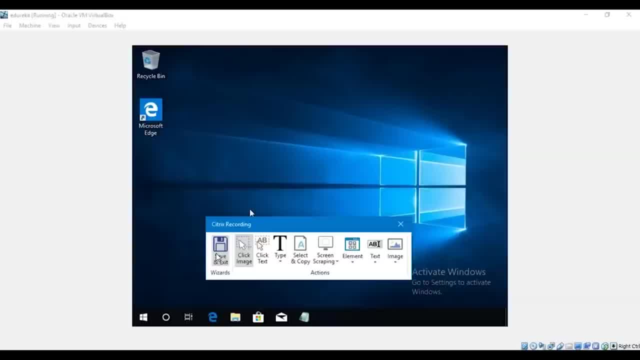 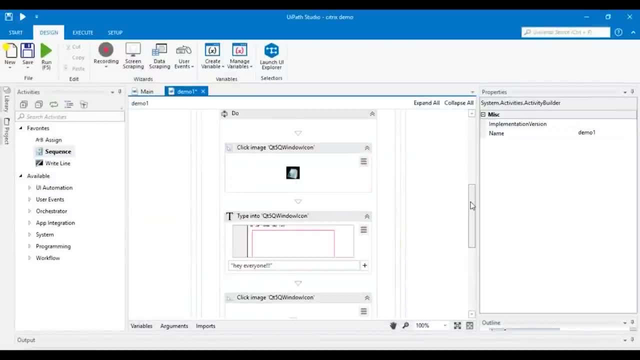 All right. So once you're done with all the work, you just have to click on this option for save and exit. All right, So let's just click on this option and this will save and exit my file, So you can see that UiPath has recorded all your actions. 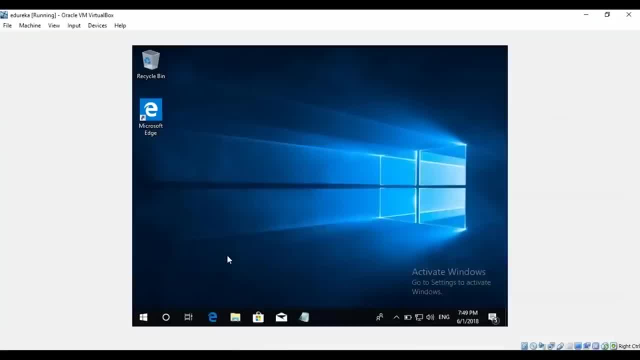 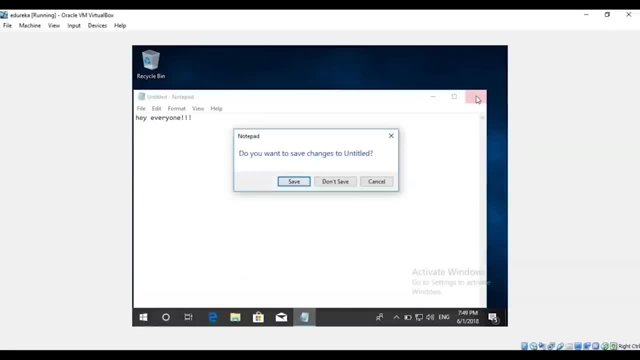 So now let's just run this program and see. So when you run this program, you can see that the notepad file is open. It is typing the text that is required and then it is not saving the file and it's also closing the file, right? 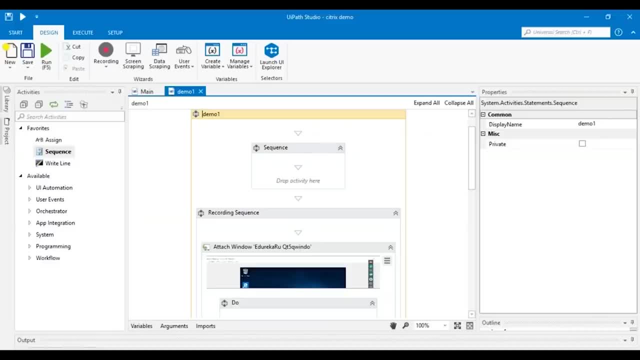 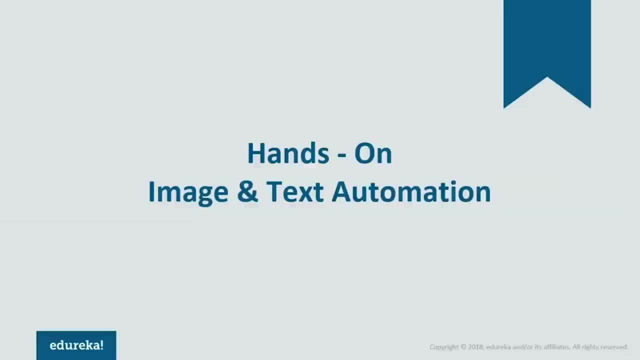 So that means our actions were successfully recorded on the virtual environment. So, guys, that was a basic demo on recording all actions. Now let's try to do something more interesting. Let's try to automate a task of an application running on a virtual environment, right? 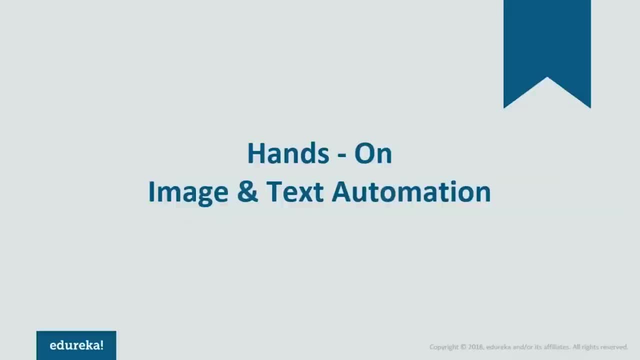 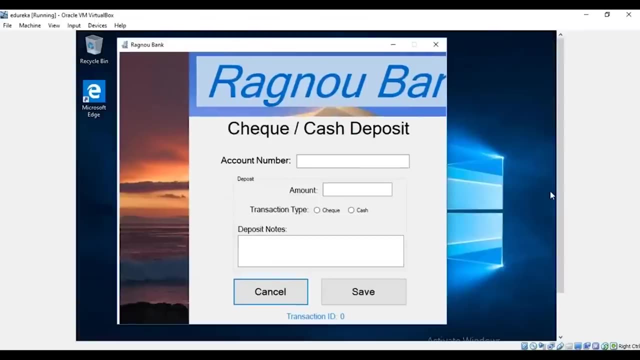 So let me just show you that application, So let me just go to the virtual environment and then open the application for you. So, guys, this is the application running on the virtual environment in which we have to automate the task. All right, So basically, I'll be entering the account number. 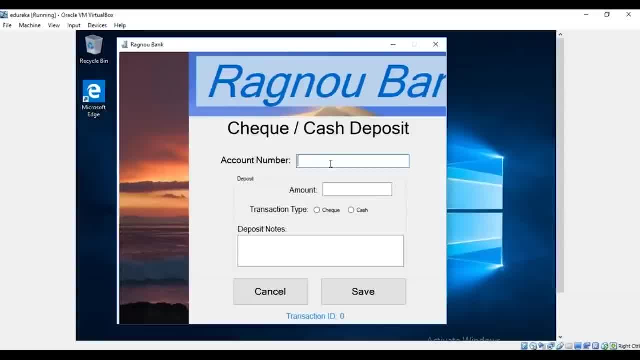 So suppose I enter the account number S, 3, 4, 5, 6, and the amount could be around like hundred bucks, suppose, and then the transaction type to be chosen as check. So once you're done with that, and then I'll click on save, 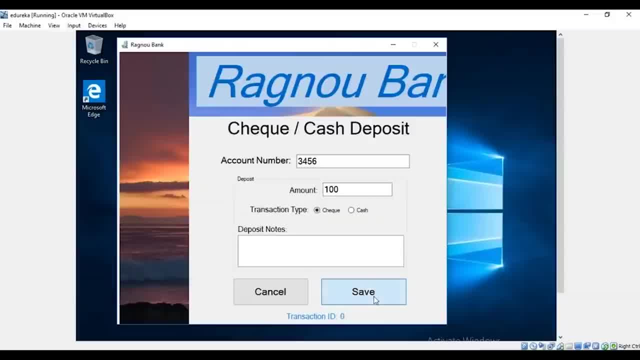 All right. So once you click on save, you can see that the transaction ID is generated. Now what I want to do is: I want to make sure that the transaction ID is generated. So what I want to do is I want to display this transaction ID inside a message box. 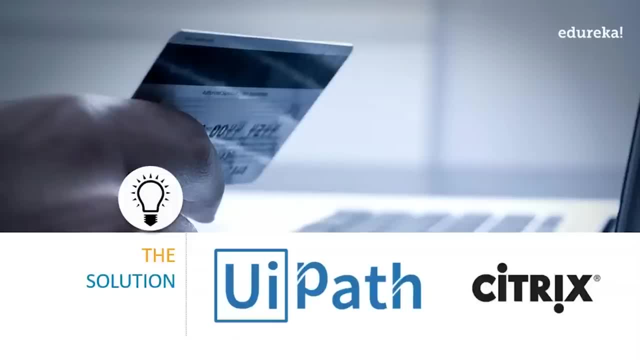 Once my transaction is successfully completed. So to do this, we're going to use the UiPath studio and the Citrix automation. So let me just open my UiPath studio and then let's start doing this, All right? So let me just create a new sequence here again. 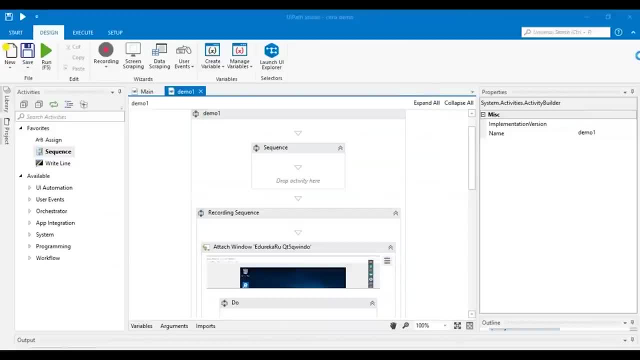 Let's say demo 2, and then click on create. Now, once you're done with that, let me just drag and drop a sequence inside this, basically, inside which everything would be done, All right. So once I'm done with this, let me just go to the recording tab. 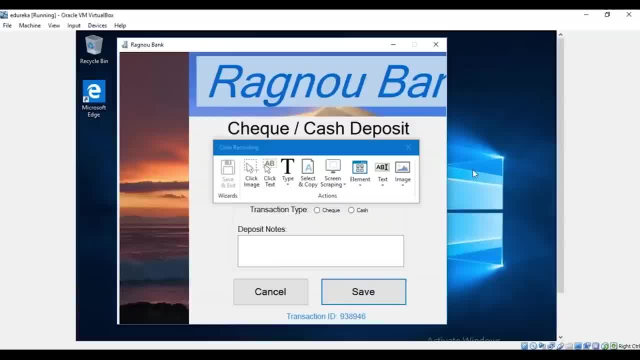 and click on Citrix recorder. All right, So let's just go back to the virtual environment where our application is running and then record all the actions. All right Now. what I showed you in the previous demo was to how to use the click image button. 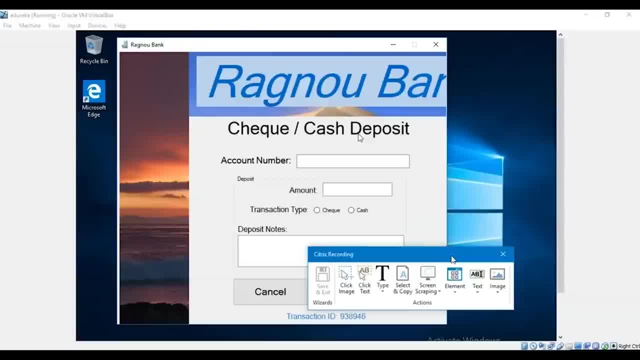 But as you can see in the application we have three text boxes and all look the same. So if you use the click image activity it might get confused on which text box to focus on right. So to work around with this, you'll use the click text option present here. 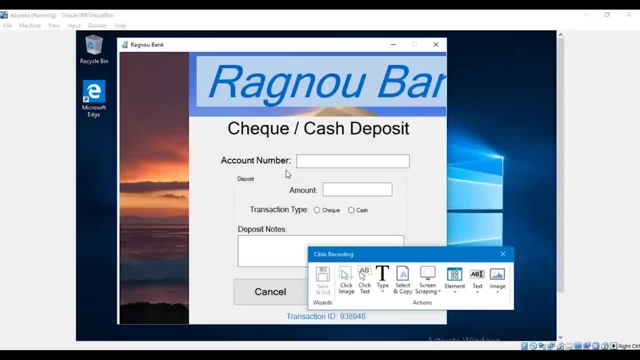 So with the click text option, you can search around this particular text and in front of this text you can specify where you want to click. right, So let me just choose the click image option and select account number. right, So let me just choose the account number. 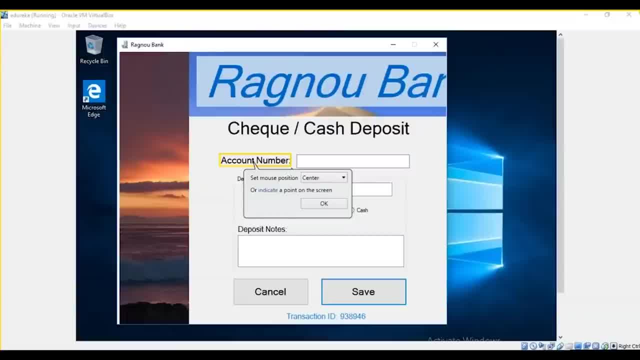 and then indicate a point on the screen where you want to click. basically, right, So I want to click before the account number. So I'll choose, indicate and I'll choose here. Once I'm done with that, I want to type in the account number, right? 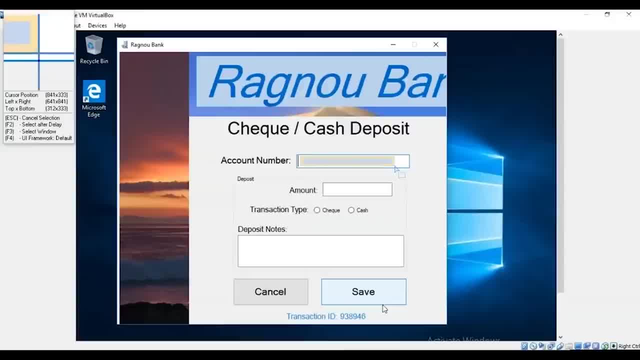 So I'll choose the type in option and then select the area to type in right. So I'll choose this area and then I'll type in the account number. So let's say I type in the account number as 34671239.. 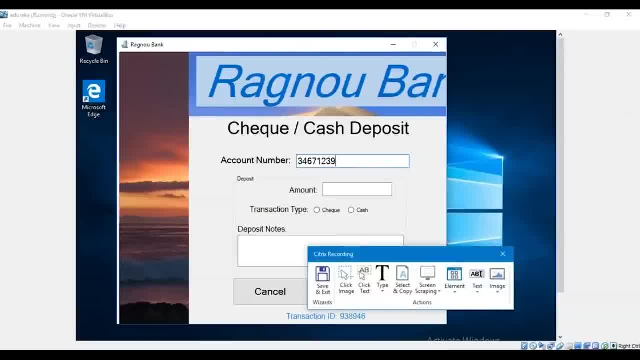 All right, and then I'll click on enter. This will basically enter my account number. then, similarly, I want to enter the amount also right, So I'll again choose the click image option and select amount. Once I'm done with that, I'll indicate a point on the screen. 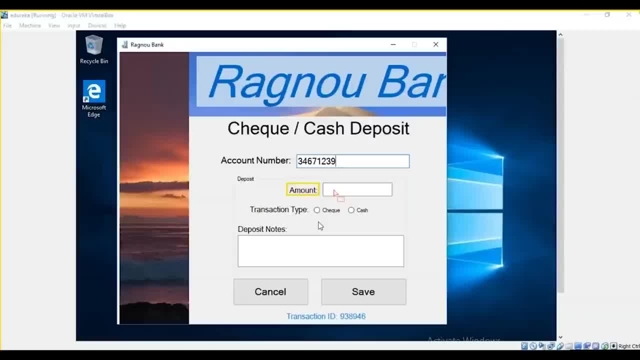 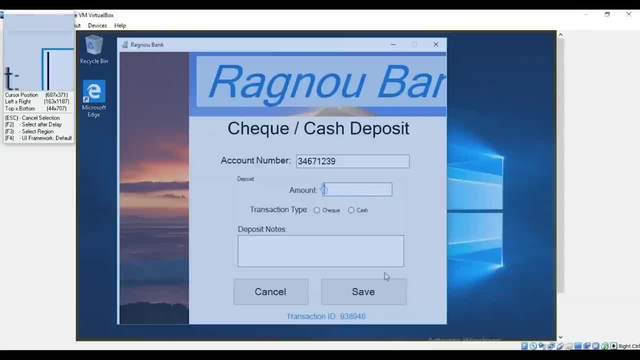 that is, I'll indicate where I want to click. I want to click before the amount, So I'll click in here, and then I want to type in the amount, right? So I'll choose the type option and then I'll mention it here. 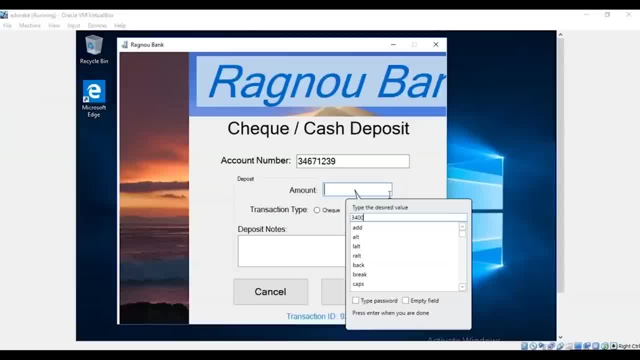 So let's say, I enter the amount as 3400 and then I'll click on enter. once I click on enter, this amount would be entered right now. after I'm done with this, I want to select the transaction type. It could either be a check or a cash. 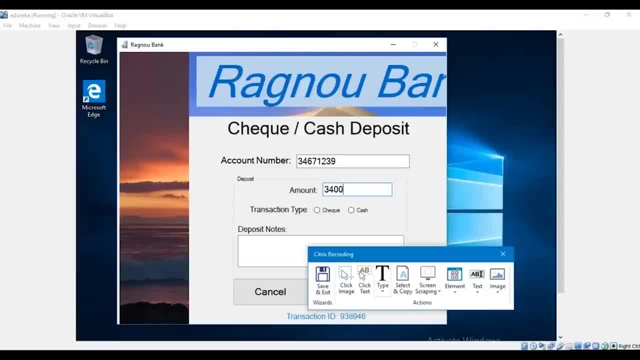 So here I can either choose the click image or the click text option. So when I choose the click text option it will basically apply OCR on this particular image, and if the text matches, it will click that option. So let me show you how that's done. 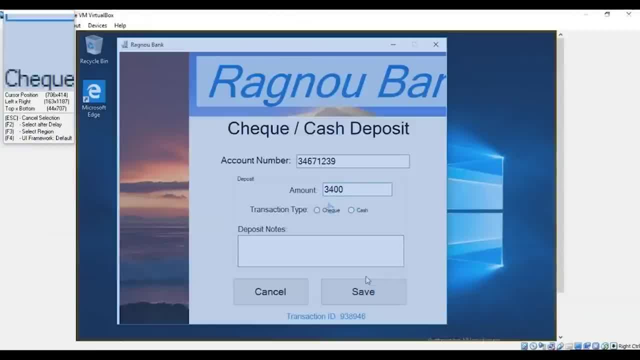 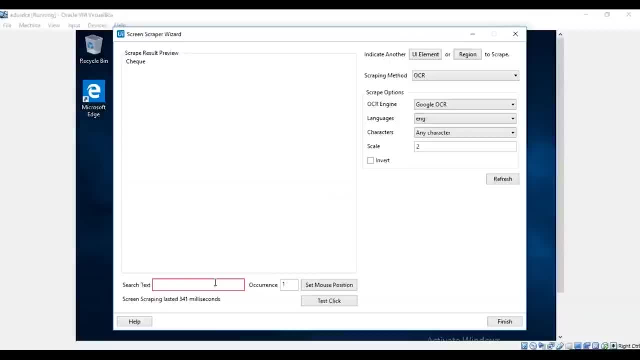 All right, so I'll choose the click text option and I'll select the region around check. So let me just select the region around check. Once it is done, in the screen scraper wizard I'll match the text to check, right? So let me just type in check here. 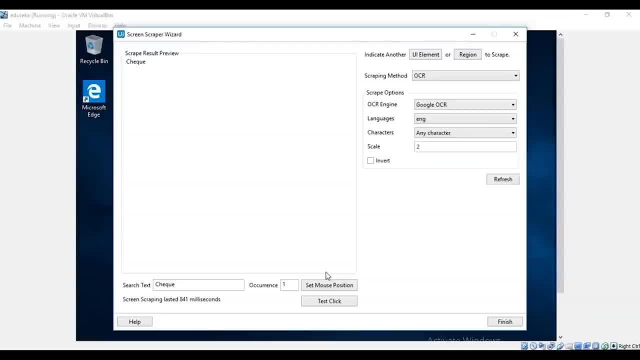 and then I'll choose the test click option to see whether it's working or not. All right, So let me just click the test click option and then you can see that the check option has been selected. All right, Okay, that works perfectly fine. 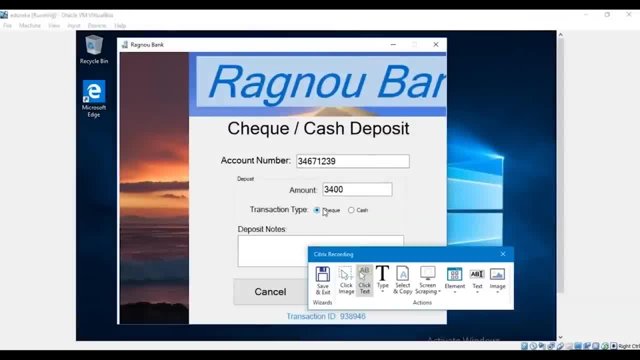 So let's click on finish. All right. Now, if you don't know what OCR is? well, OCR is a feature offered by Google which you can use it in the UiPath studio, right? So if you want to know more about OCR, 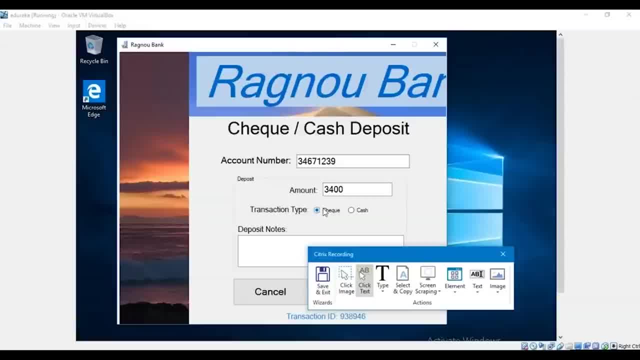 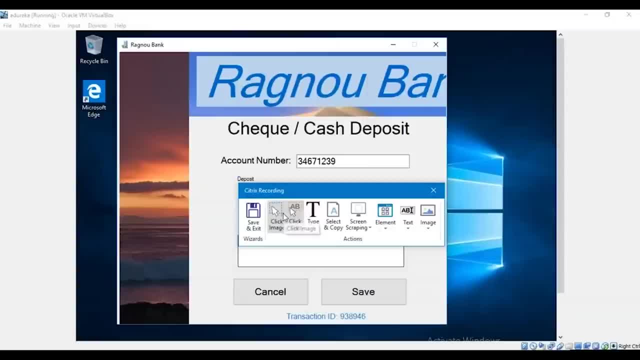 then you can refer to the official website of UiPath studio. All right. now getting back to the demo. after finally choosing the transaction type, I want to click on save. So I'll choose the click image option and then I'll select the region for save right. 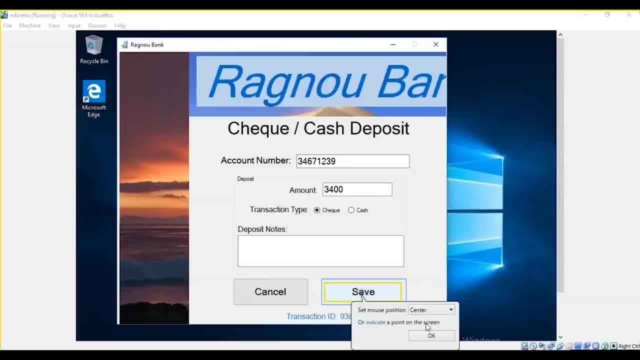 So this will basically click on save. So once it clicks on save, you can see that you've generated a transaction ID. Now I want to read the transaction ID, So I'll be clicking on the screen scraping wizard and choose scrape relative. Now why am I choosing this option? 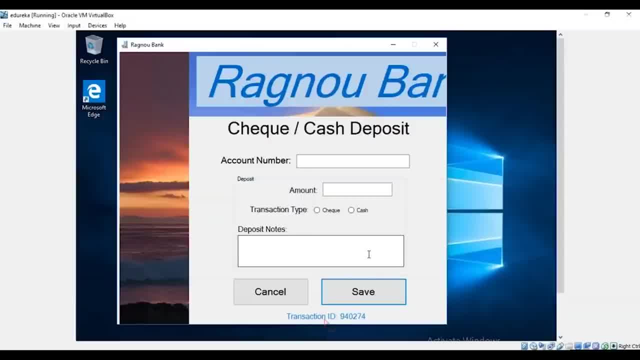 That's because I want to read this transaction ID and then I want to read what's there before it. right? So this part will remain static for each transaction and this part is going to change for every transaction that you make. So that is the reason that you choose scrape relative. 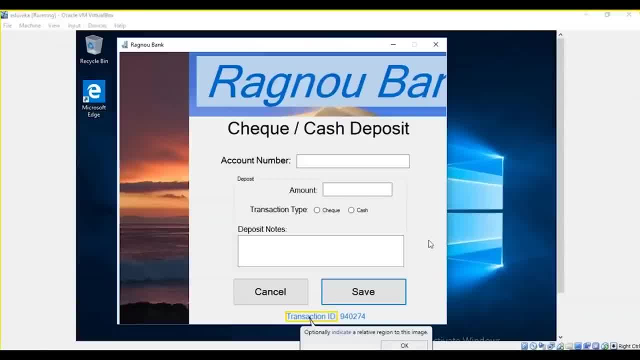 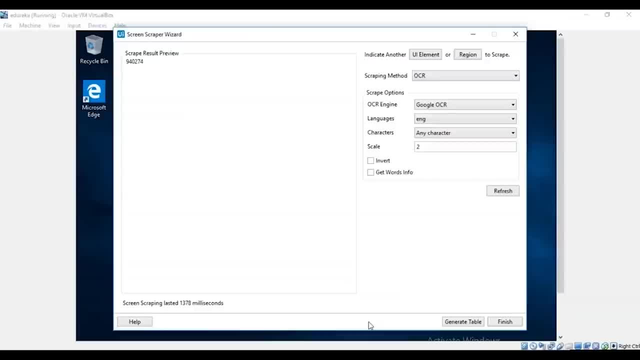 So let me select the transaction ID. Once it is done, I want to indicate the relative region, right? So I'll indicate it over here. So in the screen scraper wizard you can see that the transaction ID has been scraped, right. 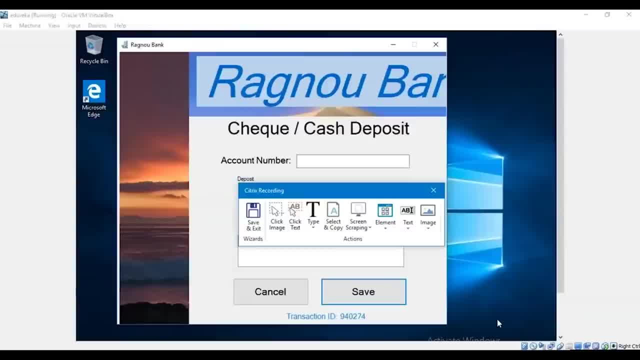 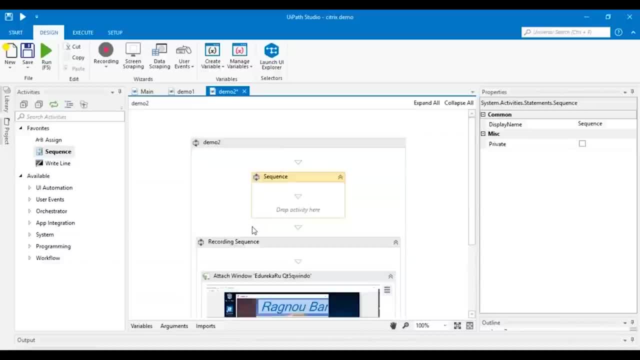 So after that, you'll just click on finish. Now, once you're done, you just have to click on save and exit, and this will get back to the UiPath studio, right? So let me just click on save and exit and let's go back to the UiPath studio. 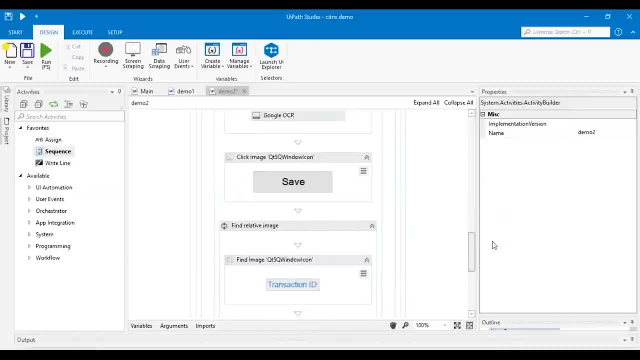 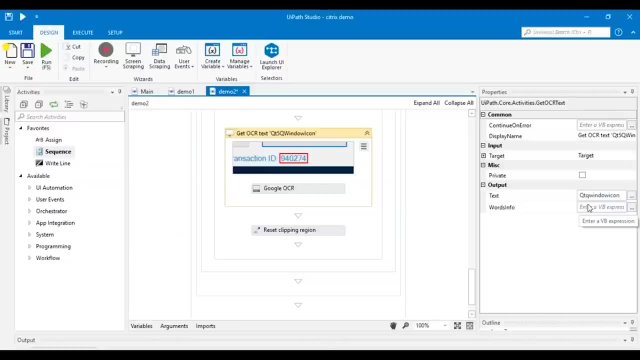 Now over here You can see that in the recording sequence all your actions have been recorded. All right. Now if you see here, you can see in the output option that the text scrape is stored in the variable of qtq window icon, Also in the variable section. 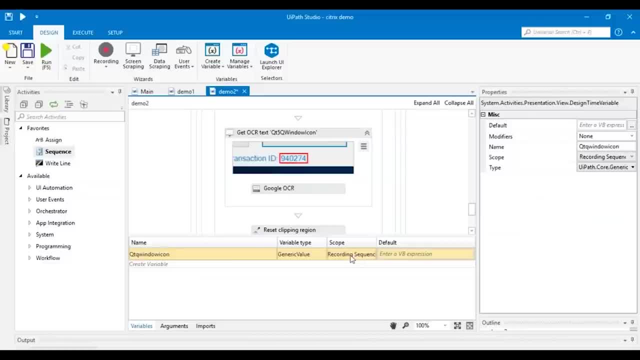 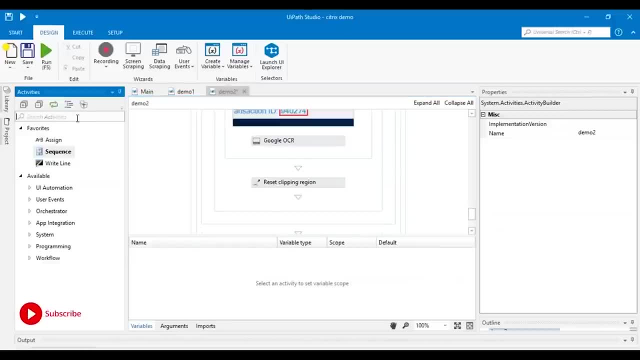 You can see that the variable is created, All right. So now let me just increase the scope for it. So let me just make it demo 2, so that it's there for the complete sequence, and then search for a message box in the activity pane. 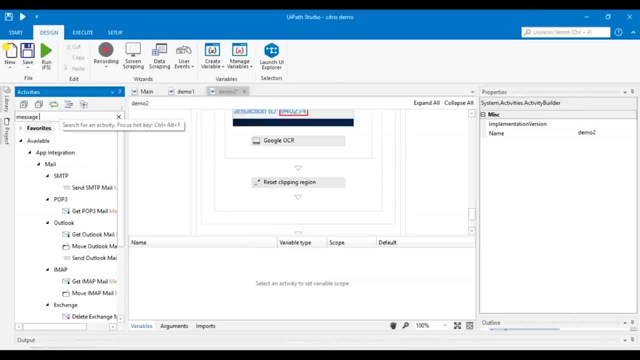 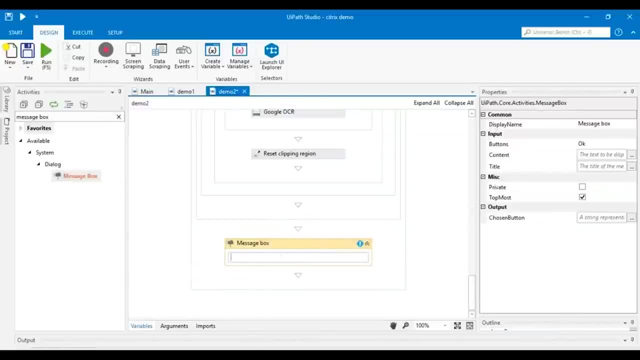 So let me just search for a message box And then let me just drag and drop it here In the message box. I want the transaction ID to be shown, So let me just include the variable name and done So. now let's just run. 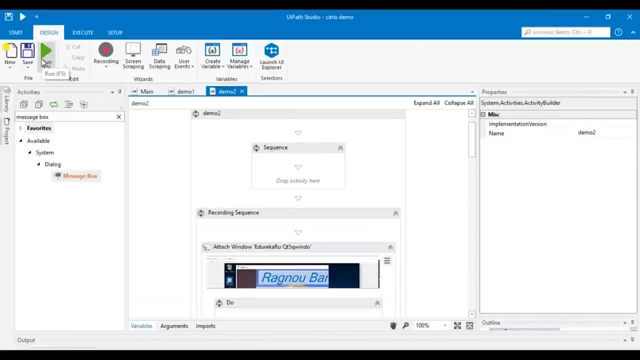 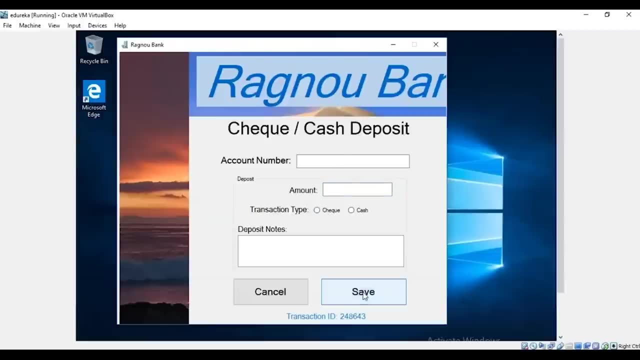 and see if our program is running fine or not. So now let me just click on run. You can see that the account number is entered, The amount is entered, The transaction type is chosen as check and then it's click on save. Once it is clicked on save, the transaction ID is generated. 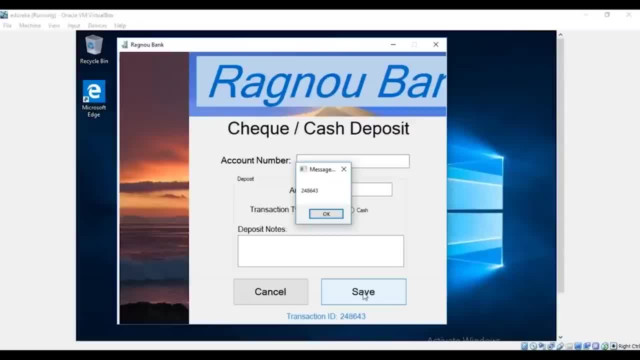 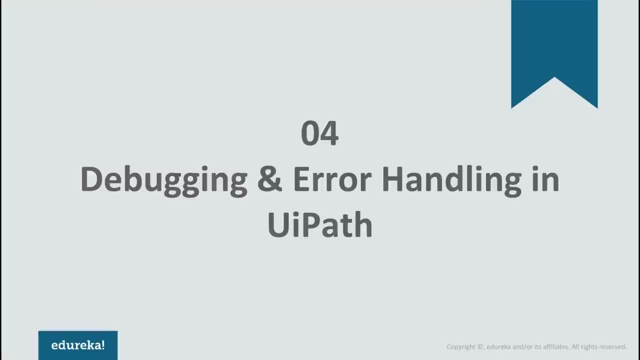 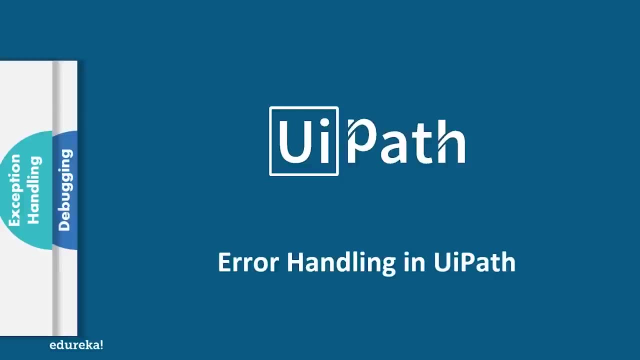 and then the ID is displayed in the message box. All right, So that means a program is running absolutely fine. All right, So now let's click on OK. So in error handling you mainly have two topics to understand, that is, debugging and exception handling. 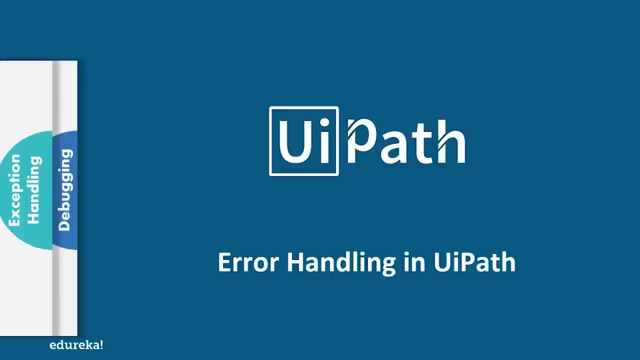 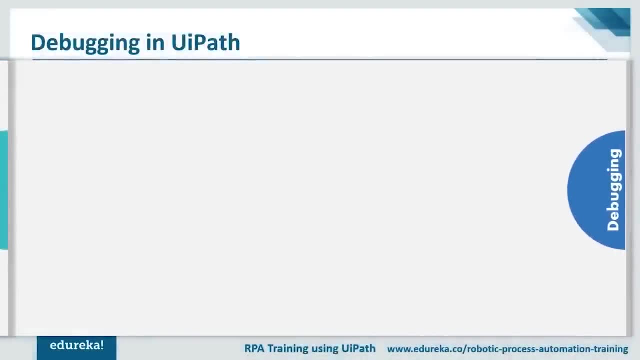 So we'll get started with the session by understanding debugging first, and then I'll tell you how you can perform exception handling right. So let's just get started with the session. So, as I said, we'll start with debugging first. So debugging is basically a process of identifying. 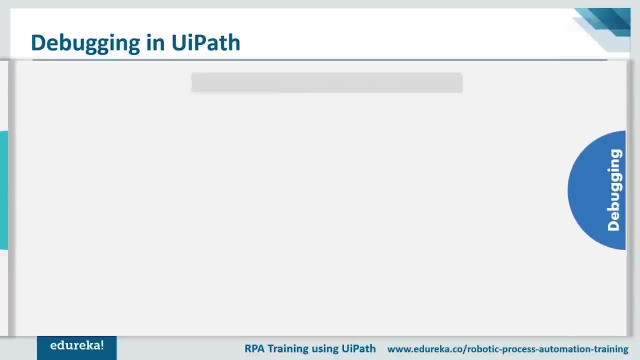 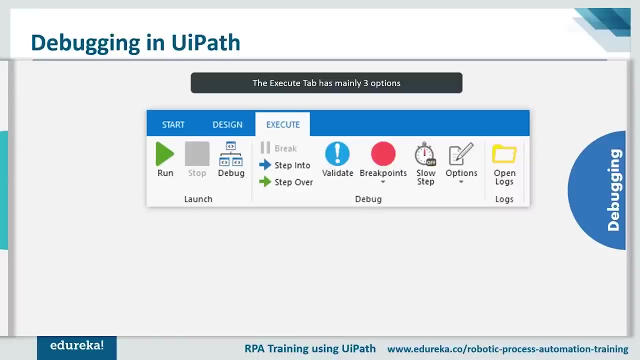 and removing errors from your projects. How would you do that? So, when you open your UI path, you would see various tabs, out of which one tab is the execute tab that you see on the screen right. So when you open the execute tab, 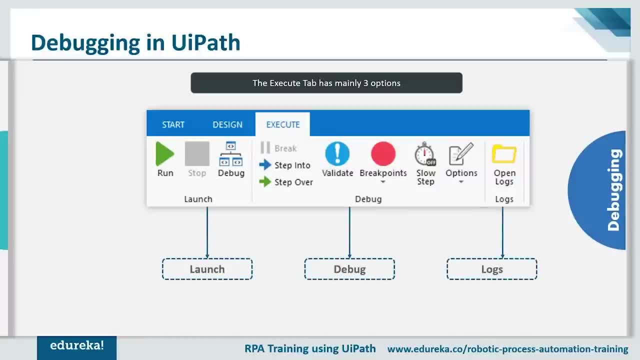 you will see these sections, that is, the launch section, the debug section and the log section. So these sections are basically used to you know, to debug your errors. So I'm going to explain each of these sections one by one and their respective functionalities. 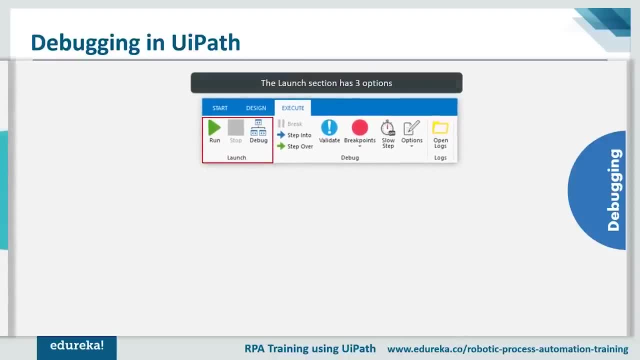 So, starting with the launch section, the launch section has mainly three options, that is, the run option, the stop option and the debug option. So the run option is basically used, you know, when you want to simply execute your project. So with this option, 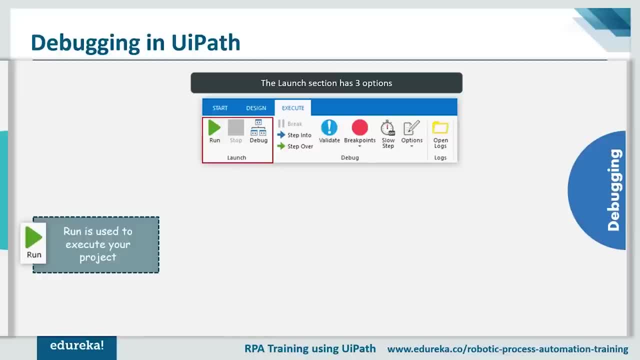 you would not see step-to-step execution, but you would directly see the output, right? So whenever you don't want to see step-to-step execution and you just want to see whether you know your automation works or not, You can just go for this option. 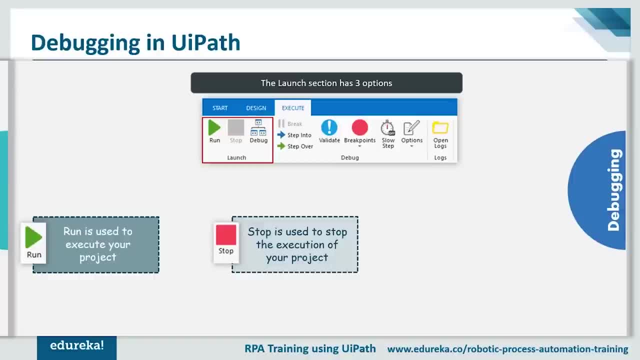 The next option is to stop option. So the stop option is basically used to stop the execution of your project. So, just in case you know, if you've started the execution of the project and you want to change something, or you know you want to add something more, then you can just cancel. 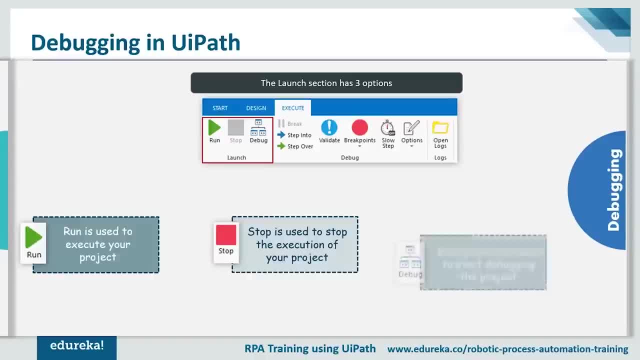 the execution of the project in the middle by clicking on this button, And the third option that is available is basically the debug button. So this button basically helps you to debug the errors, or you can say you know the faults in the project. So when you click on this debug button, 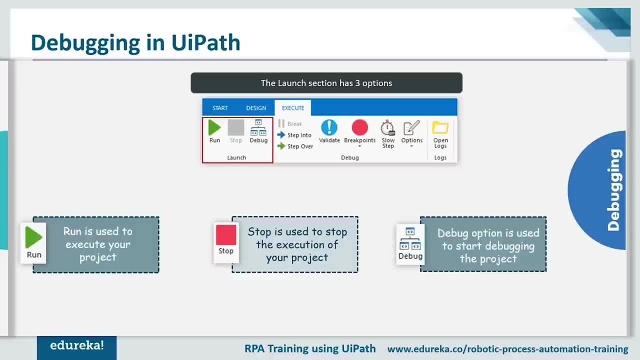 this will basically enable all the debugging options of UiPath right. So in the launch section I'll again repeat: you have three sections, that is, the run, the stop and the debug options. Now moving on to the debug section. the debug section basically has five options. 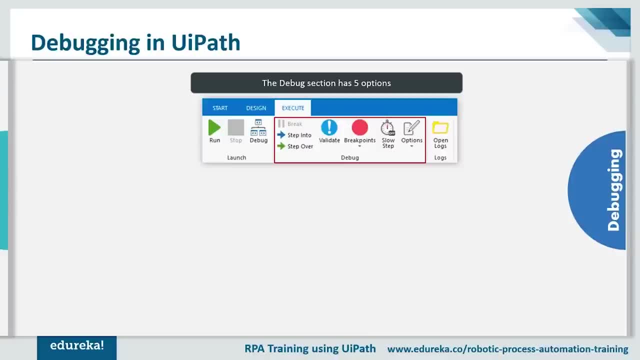 That is, the steps, the validate, the breakpoints, the slow step and the options itself. So, starting with the steps: the steps are used to execute your project step by step. So when you click on the step in, or you know you click on the step over, you'll see that. 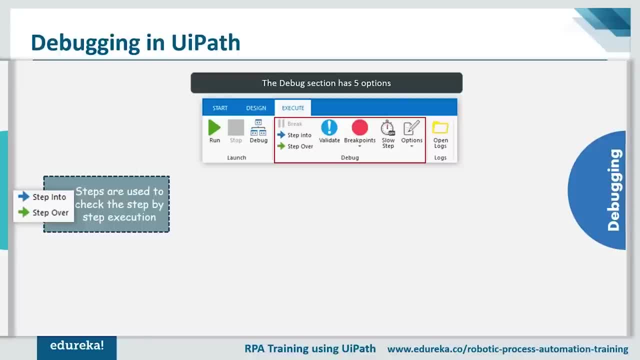 you know you go to the next step and it waits. So when you click on to step into, you'll see that you know wherever you have stopped your automation. when you just click on to step into, you'll see that you know. 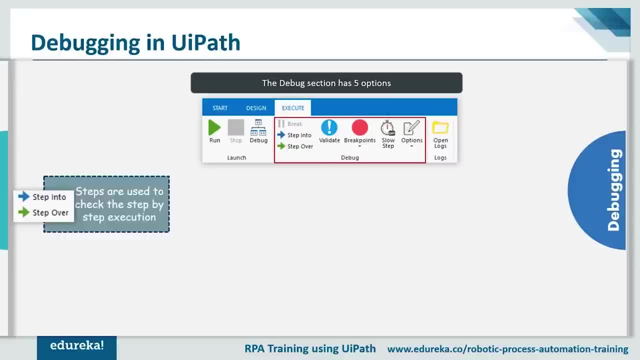 you go to the next step and it again waits for you to click on to the next step, right? So that's how you can see the step-to-step execution and move forward and debug your errors, moving on to the next Option that is present. that is validate. 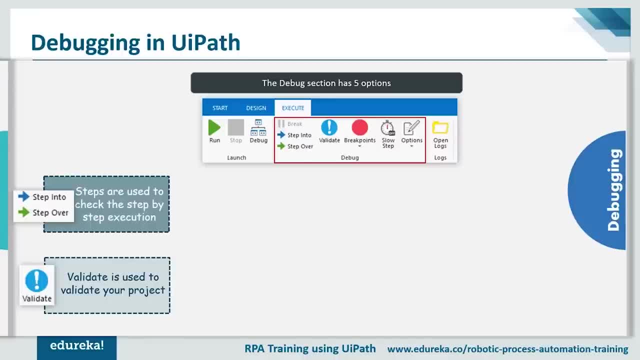 So validate is basically used to validate your project. So with this button you can basically make sure that you know you have errors in your project or not. So whenever you choose this option, I would say that you know it will just check the automation if it has any errors. 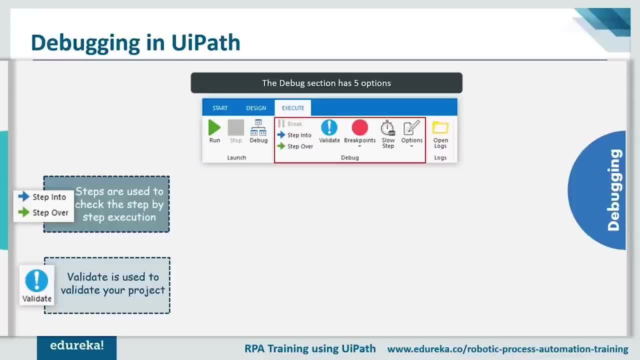 or not. and if it does have any errors, then it will return to you those errors so that you debug those errors right. So now, how do you debug those errors? Well, I'll tell you when we move on to the hands-on part. 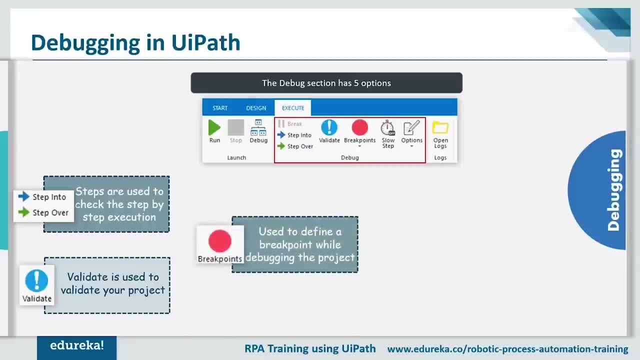 but before that let me just tell you what breakpoints are. So breakpoints are those points at which you want to stop your execution. So just imagine, you know you have 10 steps in your automation. So if you want to stop your execution at the fifth step, 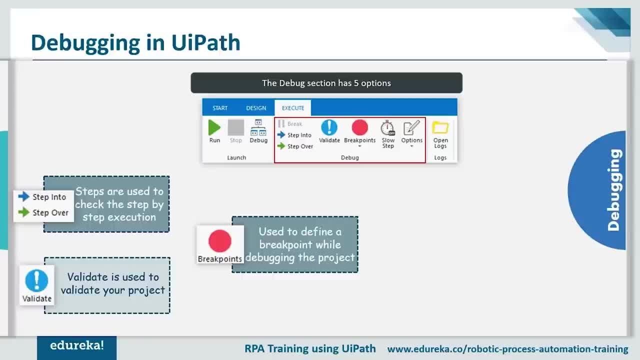 then you can just use this breakpoint option to just stop the execution of the fifth step and then after that, then you can use the step into option to see the step-to-step execution right? So that's how you can use the breakpoints. now moving on to 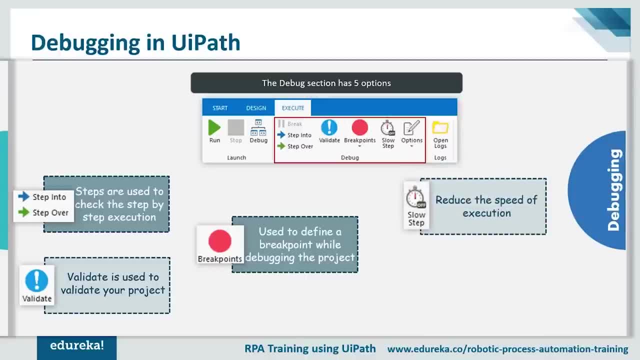 the slow step. The slow step is basically used to slow down your execution. So, as all of us know, that boats are very, very, very fast in executing the task and even if it's a large task, that they have to execute it within the seconds. 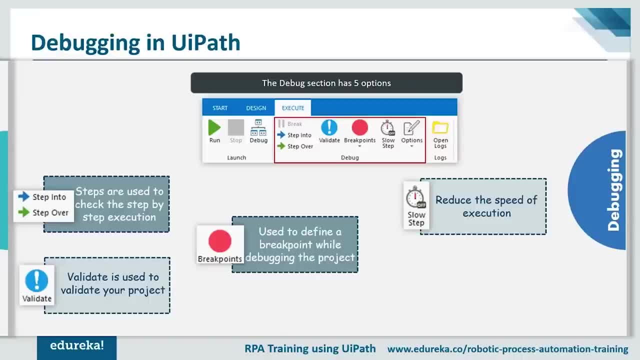 right. So to see the execution one by one and to make sure what step is running and what step is not, so you can just use the slow step option. So this will basically slow down your execution and it will be visible to your eyes which step is executing right and 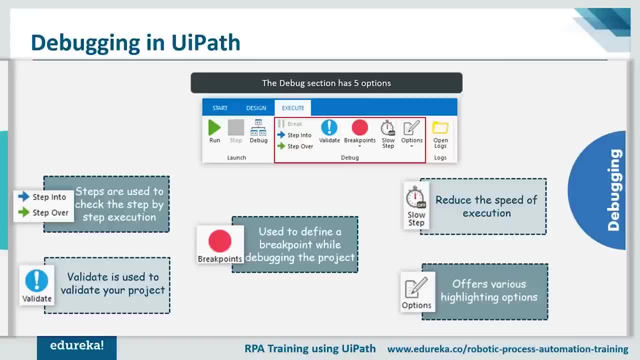 moving on to the last options, that is, the options itself. So this basically offers ways highlighting options to highlight the activities. So when you highlight your activity, you can clearly understand which activity is running presently, or you know which activity has any error or if you want to maintain any. 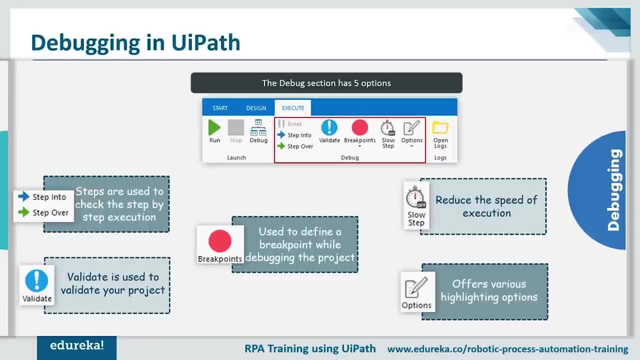 specifications in that particular activity that you want to remember while you're debugging: errors and so on. right, So that's what the debug section offers, guys. It offers steps option, It offers the validate breakpoint, slow step and the highlighting options itself. right now, moving on to the last section of this, 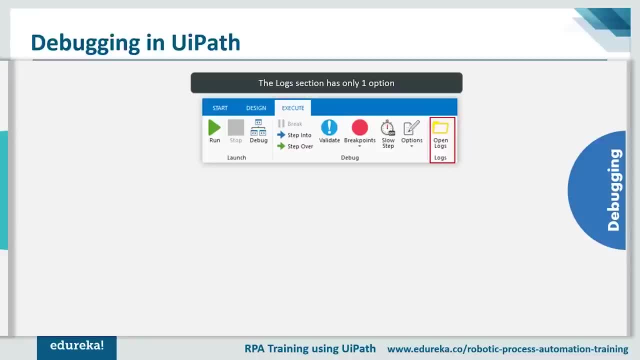 tab that is basically the log section. So the log section has only one option. that is basically to open the logs of your browser. So you can just consider this option as a shortcut to open the logs of your project. So you might get a question over here. 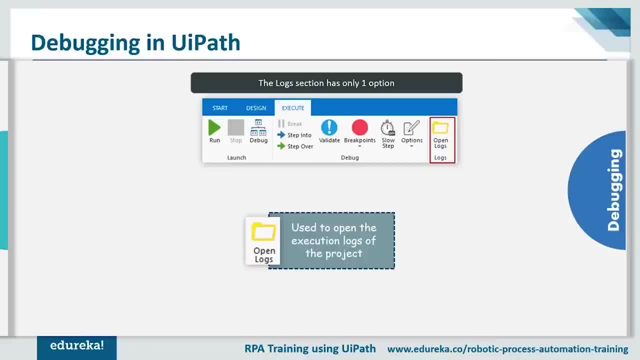 Why do we need logs? You know when we have so many options over here, right? So well guys, let me tell you if you're from an IT background and you would understand that you know when logs are there, you clearly understand which variable is running or which variable has been assigned. 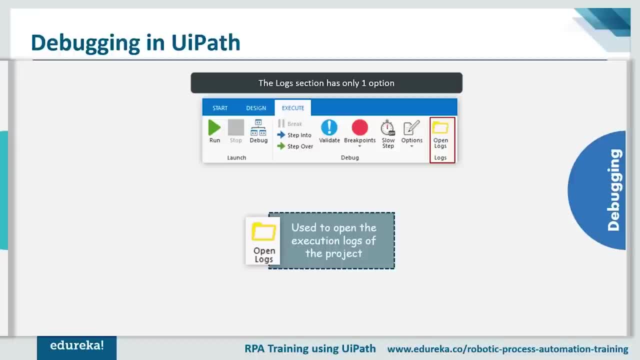 to which value or what activity is running, What is the output, come and so on. right, So logs make it very clear Where is the problem coming from and with those logs you can make sure that you don't have any Errors. right, so you can start debugging with the help of logs. 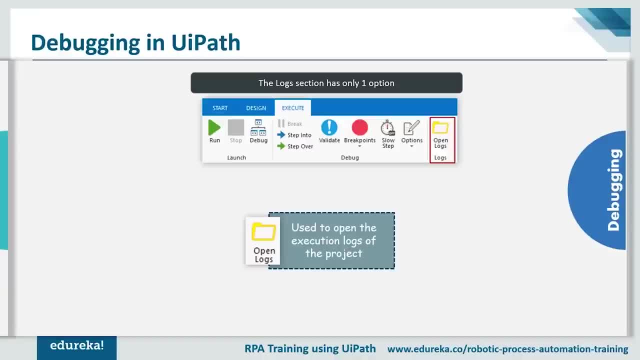 also. So, guys, these were the various options that you have to debug errors in UiPath. So we basically have the execute tab in the ribbon, which offers three sections, that is, the launch to debug and the logs, and these three individual sections also offer again the various 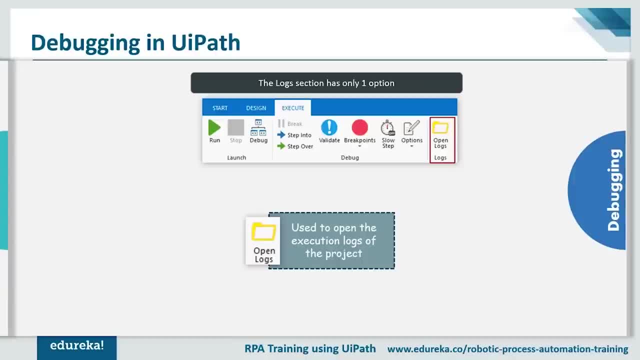 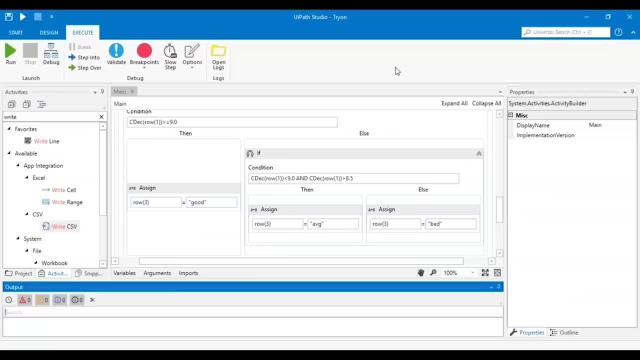 buttons through which you can debug errors. right now, to show these options in practical, I've created a demonstration for you, So let me just open that demonstration, All right? So what I've done is I've created a project, So this project, basically, 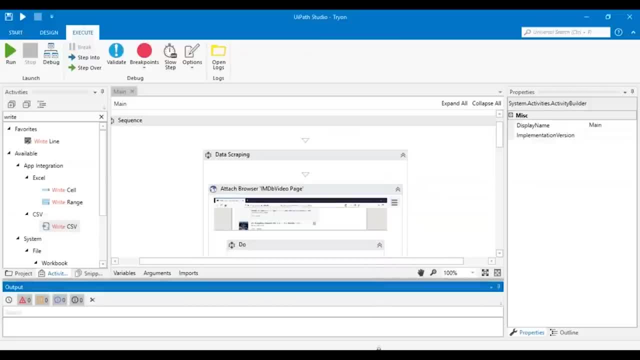 Scrapes data from the imdb website. So, as you can see on the screen, I've basically performed data scraping from the imdb website, which basically scrapes the top key video games in the list and then, once it scrapes the list, it just stores them in the data column or you can say an excel. 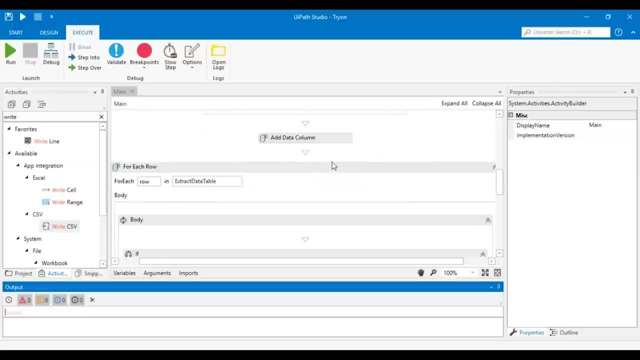 sheet where I want to store this data. So now what I'm going to do is, for each video game, There's a rating that is given right. So, based on that rating, what I'm doing is I'm reading the game: if it's good, it's bad or it's average, right. 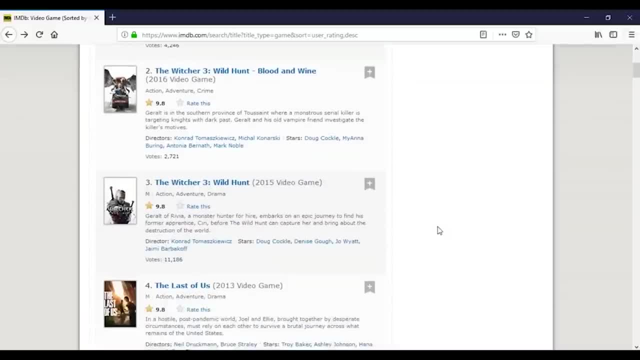 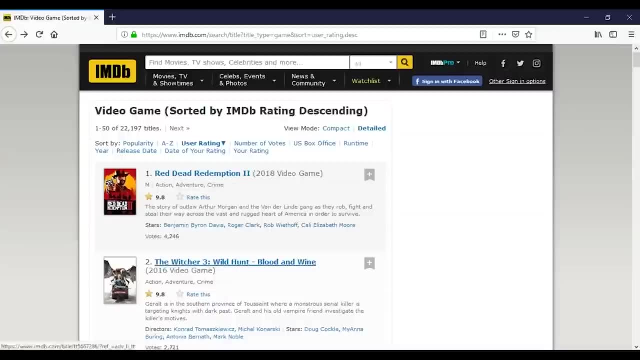 So let me just open the website and show you. So, As you can see, this is the website which is being scraped. So what I'm scraping is the name of the game, the rating and the upwards of the game now based on these ratings. 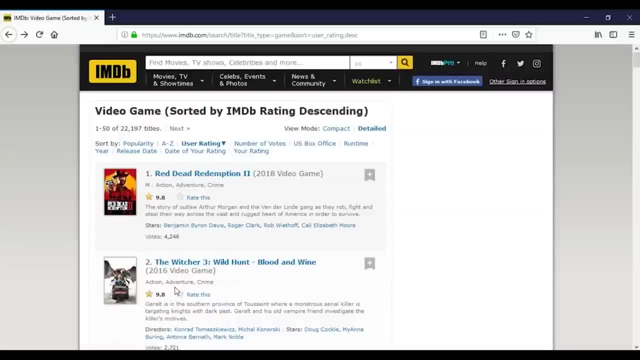 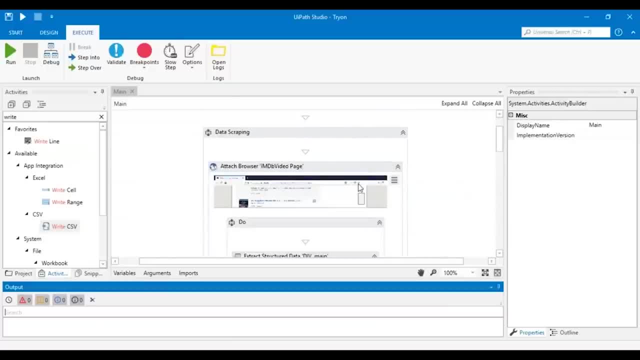 I've basically divided the games or, you know, I've categorized the games into good games, bad games or average games. So let me show you the sequence that I've created. So over here I've created a data scraping sequence. So how do you do that? 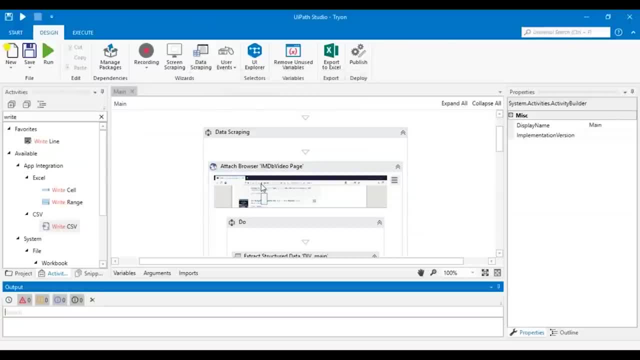 You go to design and then you can just choose data scraping option. So if you want to understand how do you perform data scraping, I'll leave a tutorial in the description box and then you can understand how do you perform data scraping. now, after data scraping is performed. 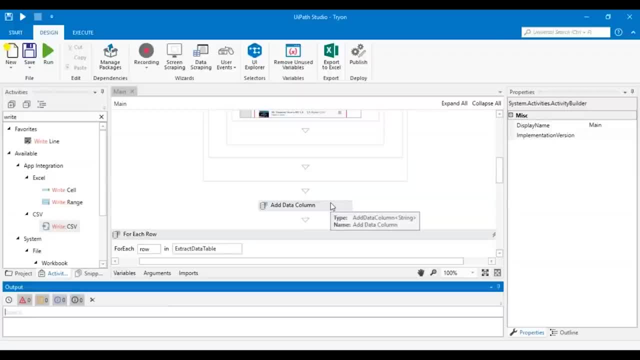 I've added a data column that is basically to store all these values in a table format, or you can say, in a data table format. and now, for each row in this data table, What I want to do is I want to grade the games, right. 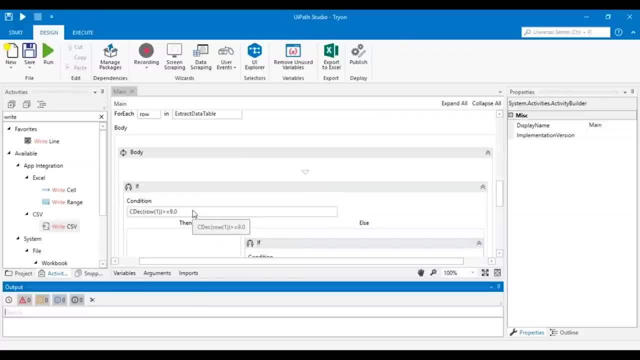 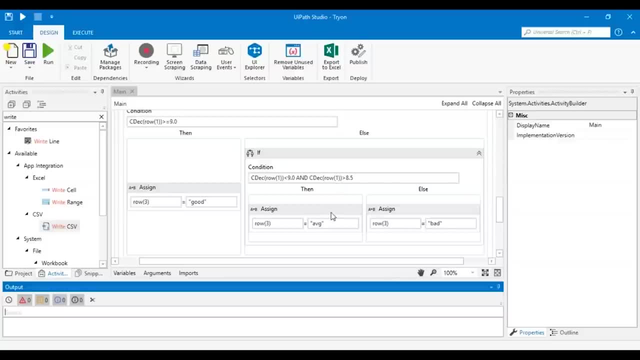 So suppose if any game has a greater than 9.0, so that game would be rated as a good game. And if any games rating lies in the range of, you know, 8.5 to 9.0, then it would be rated as average. or if any game less than. 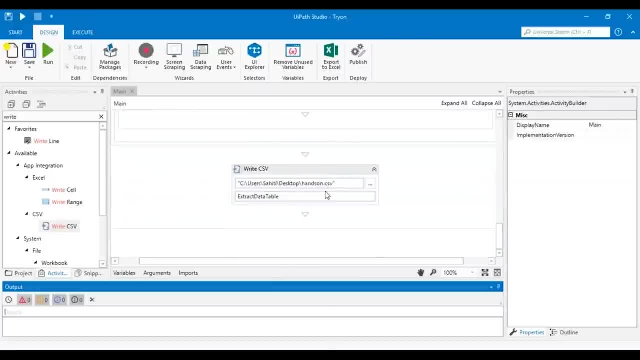 8.5.. 5 would be rated as bad, right? So that's what I've done over here. Now, after all these ratings are done, all the data would be stored in a hands-on dot CSV file, right? So let me just execute this part of the program so that you. 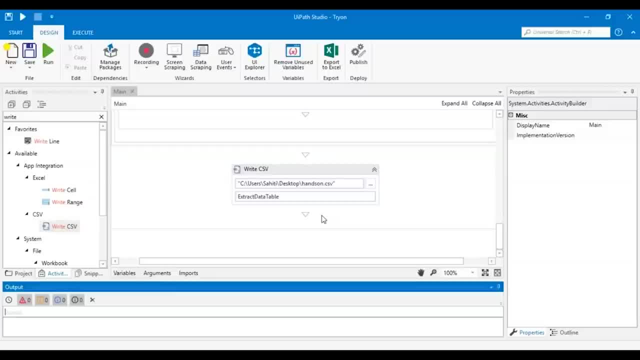 understand what kind of output that we get, and then I'll show you how you can debug errors, right? So let me just open this. This is on the first page. Now I'll just click on execute and run, So let's wait for it to execute. 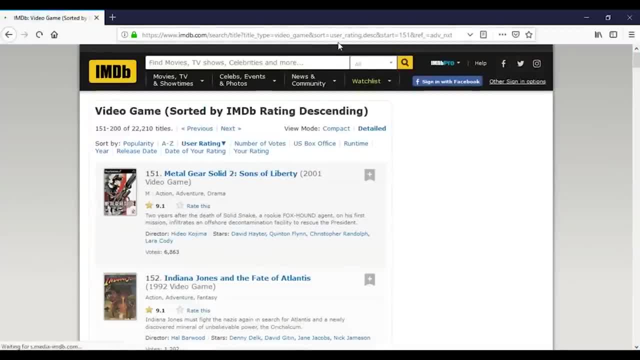 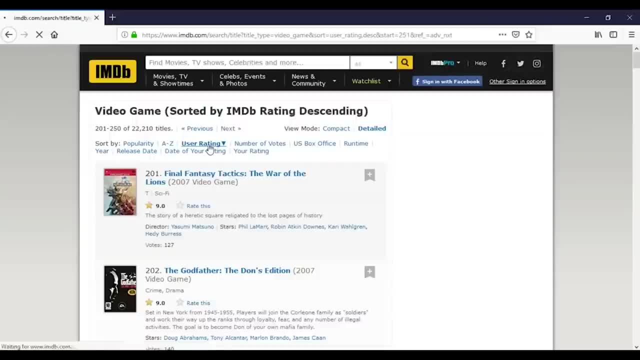 So, as you can see on the screen, the data is getting scraped over here, So as the pages that you see are getting loaded over here and all the data is being stored somewhere. So once this completely executes, I'll show you what's happening. 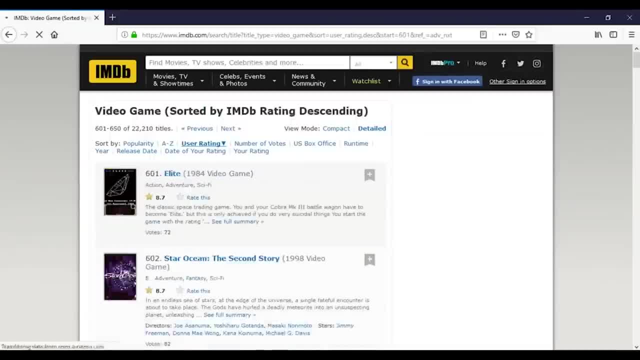 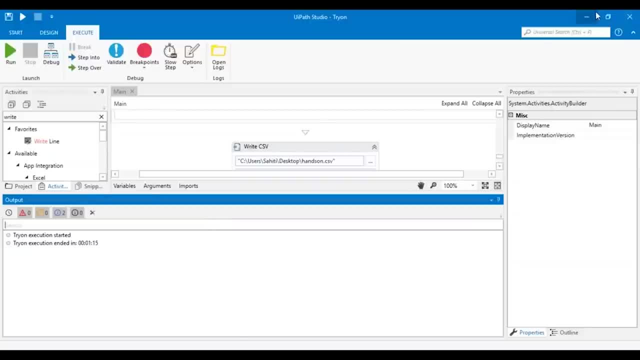 So let's just wait for it to execute, All right. So as you can see in the output pane, we've got the output that UiPath has executed a complete sequence in a minutes. Now let me just open that CSV file. All right. 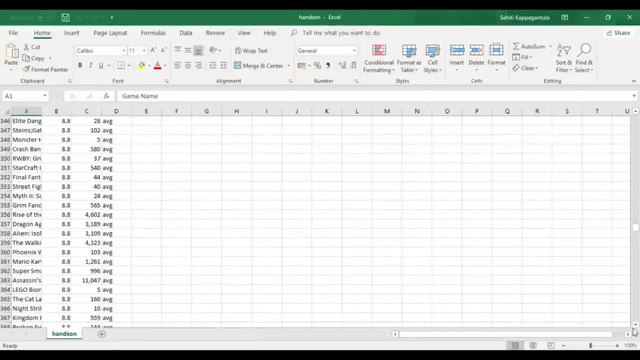 So, as you can see in the screen, you know we've got few values through which it has been rated. So, as I said over here, if the rating is greater than 9.0, then it's going to be rated as average. 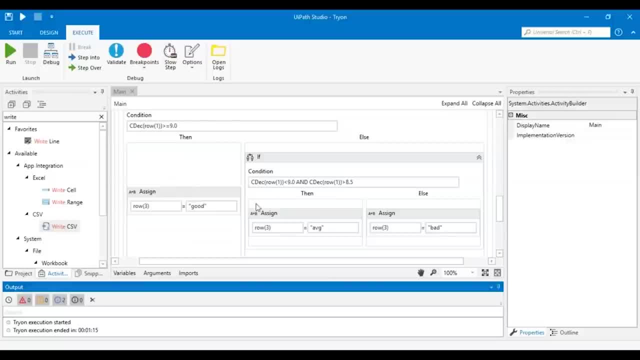 And 9.0, or it is equal to 9.0. It would be rated as good, or if the rating is between 8.5 to 9.0, then it would be rated as average and less than that would be rated as bad right. 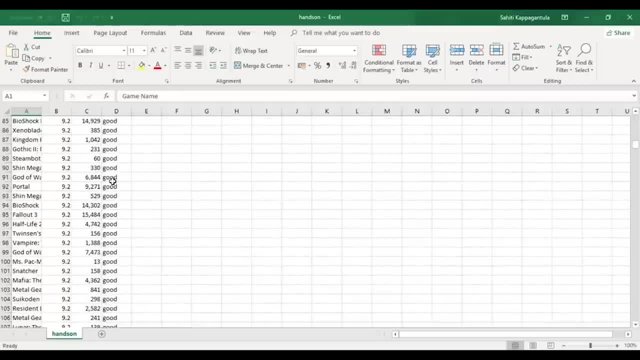 Let's just see what the output comes. So all the games which have a rating greater than or equal to 9.0 have been rated as good. Now let's just see the section between, you know, 9 to 8.5,. 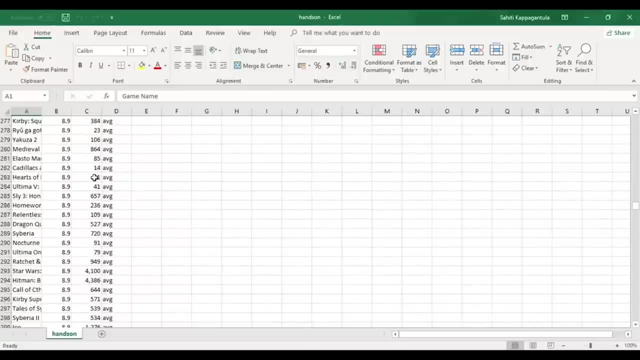 which means 9 is not included. right, So you see the games with ratings 8.9 and 8.8,. right, So all these games have been rated average. So that means our UiPath execution of automating task is running. 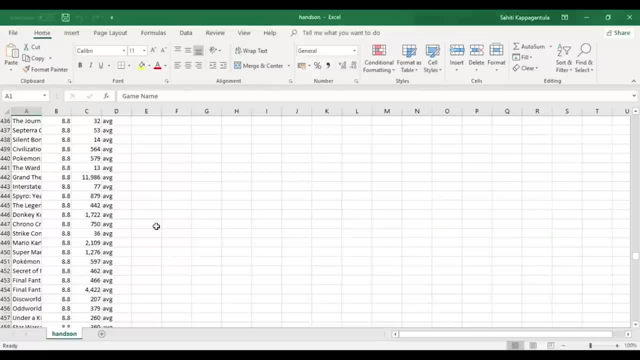 absolutely fine, That means we have automated. well right, So it's scraping all the data, It is storing all the names of the game, the rating of the games, the words, and then it's giving a final output based on the ratings. 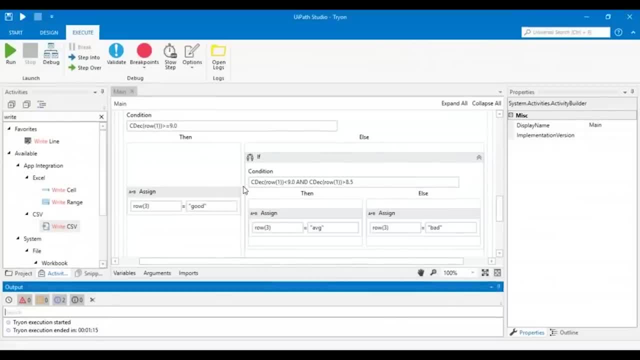 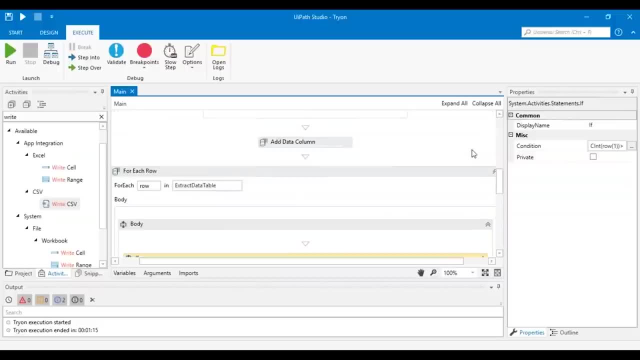 right Now, what I'll do is I'll intentionally do some errors, and you guys don't know right What errors I'm doing. All right, So what I've done is I've intentionally done some errors on this sequence. So now let's see how we'll debug these errors. 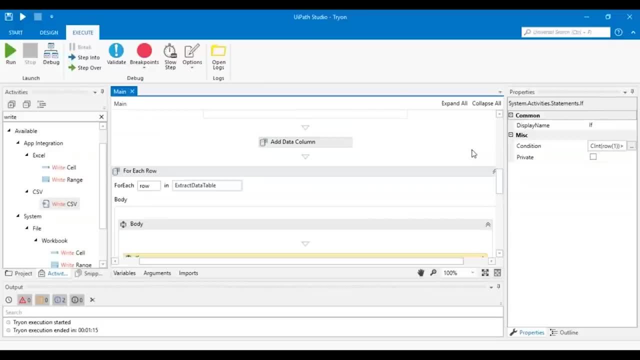 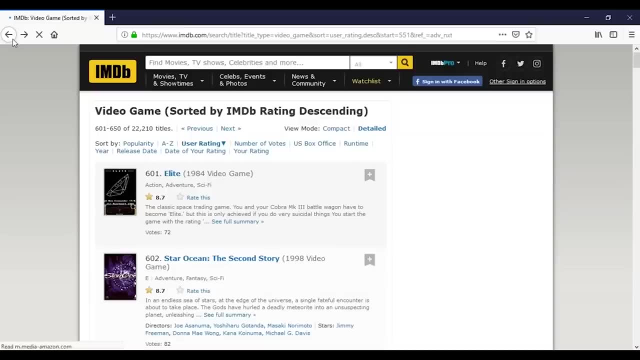 But before that, what I'll do? I'll again execute this particular sequence so that you understand what's the problem, right? So let me just quickly delete this file and then I'll go to the first page over here. Now we're ready to execute. 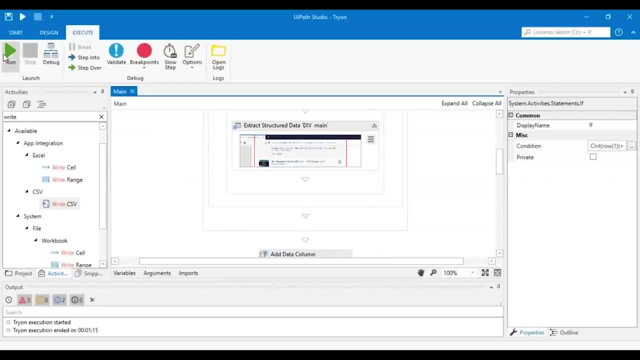 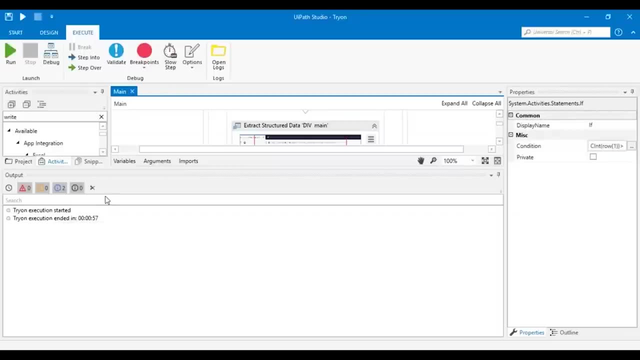 So I'll again execute this particular sequence. So I'll click on run. So in the output pane, if you clearly observe, it shows a status that you know it has started executing. All right, so you can see an output that you know, the execution. 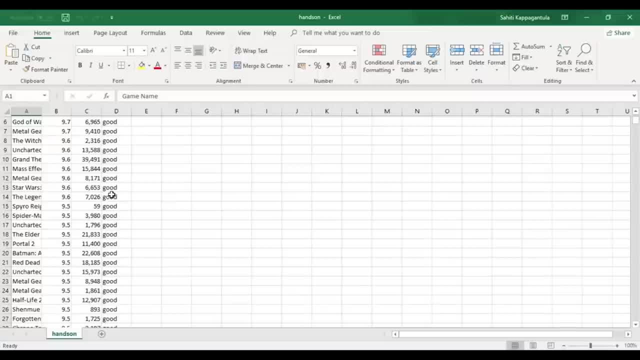 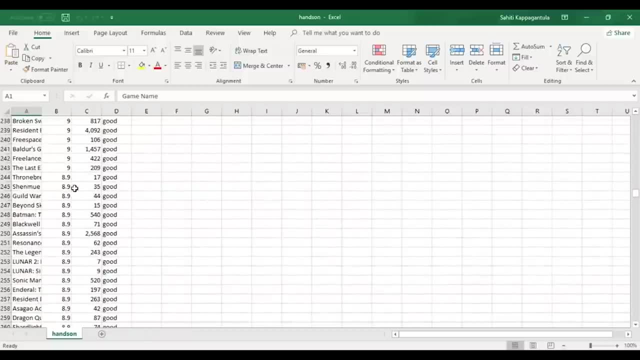 has ended right, So now I'll again open that file. All right, So you can see that. you know we've got all the games with the ratings greater than 9.0 to be good, But the games with the ratings between 8.5 to 9 have also got. 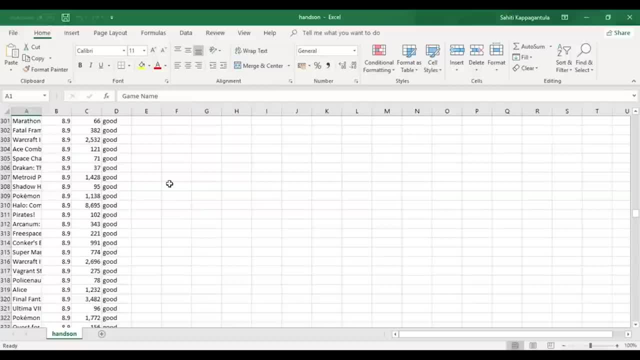 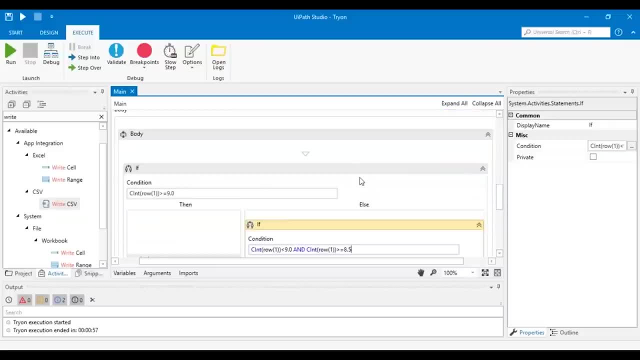 the output as good right. So that means they've also got rated as good, which is not correct. According to our sequence They must have, you know, been rated as average right. So as you can see over here all the games with the ratings, 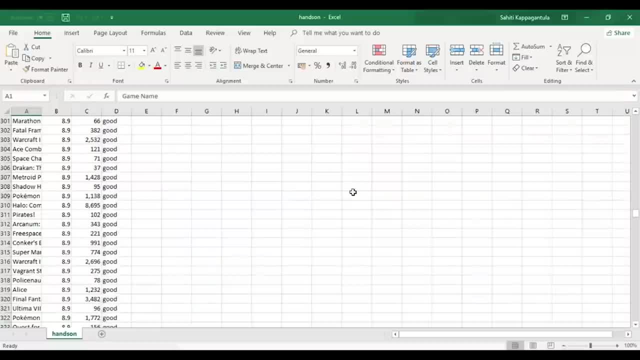 between 8.5 to 9.0 must be rated as average right, But yet if we see the output over here, all have been rated as good, That means there's some error in the output. We need to debug this. 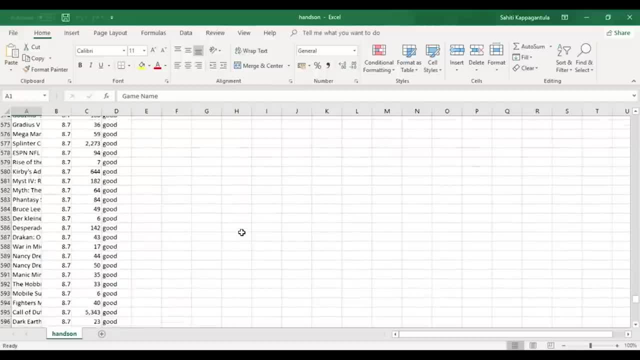 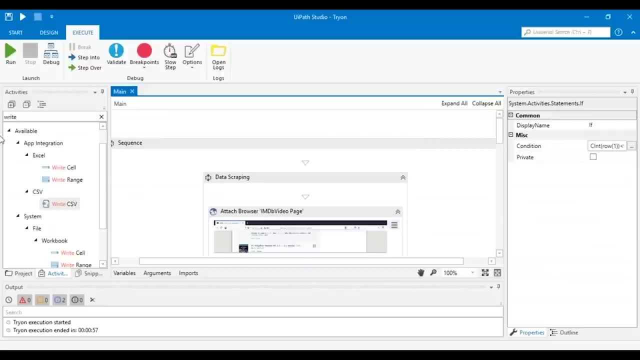 Now, how do we debug this? So, for that, we're going to use all the options that I just had mentioned before. So I'm going to go back to my sequence over here. Now, what I'm going to do is I'm going to start, you know, using 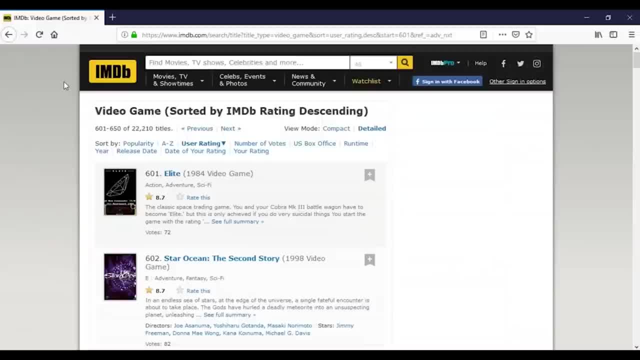 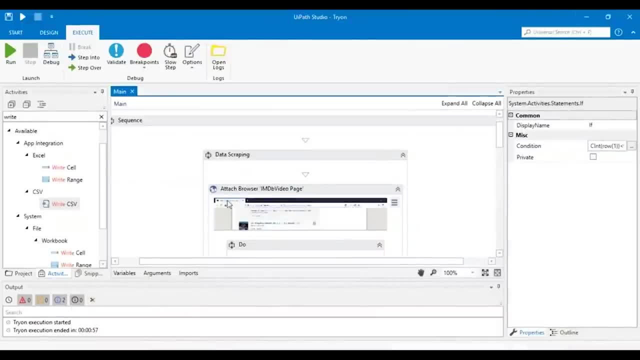 all these options Now. initially, if you observe, over here, games that are present in this particular website have been scraped. absolutely fine, right. So that means we have no problem with regarding to the data scraping option over here. But, yes, after that we have an add data column again over here. 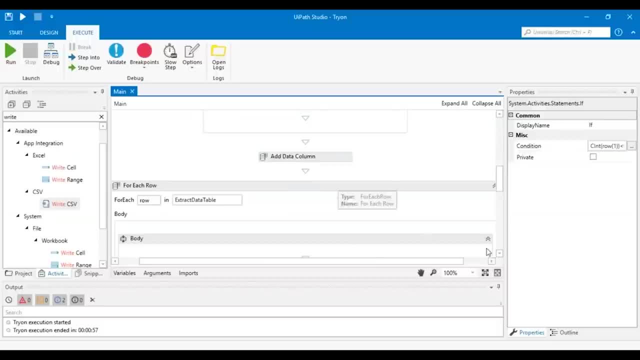 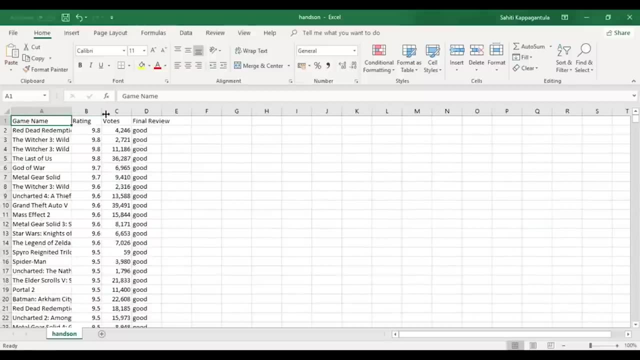 We don't have any problem. That's because you're not. data is getting added in form of a table and we see that in our Excel file, right? So if you scroll up to your Excel file, you can see that. you know, all the data is being stored in the form of a table. 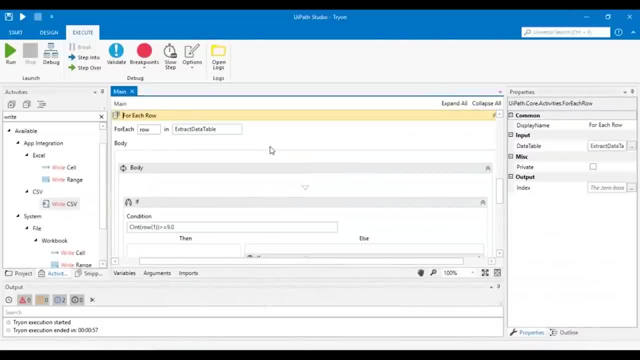 So that means there's no problem over here also. But yes, there's a problem over here because for each row we have some problem in the loop, right. So that's because- a final review, that is, if it's a good game or. 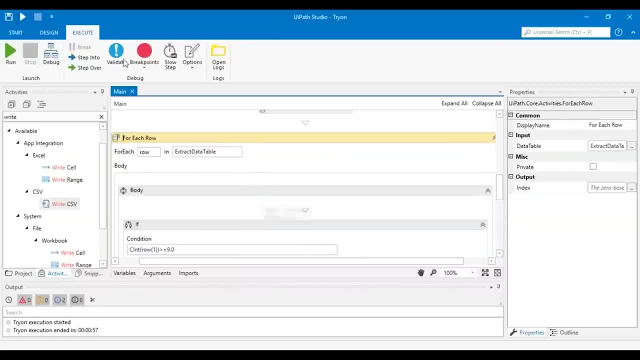 a bad game or an average game is going wrong right Now. what I'll do is I'll basically add a breakpoint over here. So when you click on this breakpoint option, you'll see two options, that is, toggle breakpoint and remove all breakpoints. 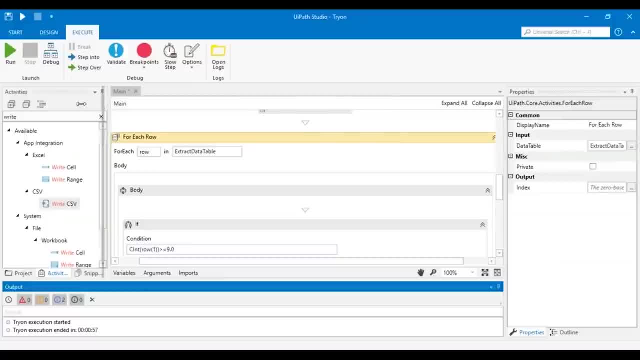 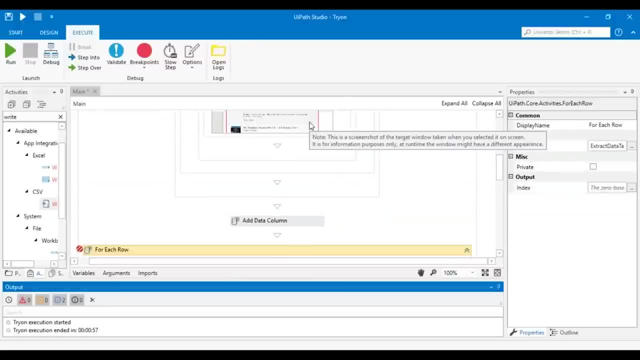 So I'll add toggle breakpoint over here. So when I add toggle breakpoint over here, you'll clearly see that you know this particular section is where the execution will stop. So when you start your execution all the data would be scraped. 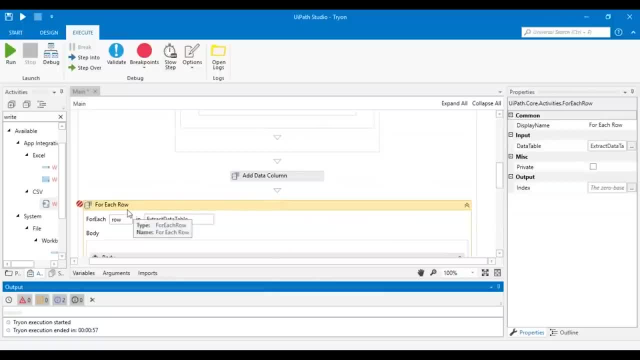 It would be added to a data column and then the execution would stop over here. After that we have to, you know, click on to step into execution so that we see step-by-step execution, right? So I've added a breakpoint over here. 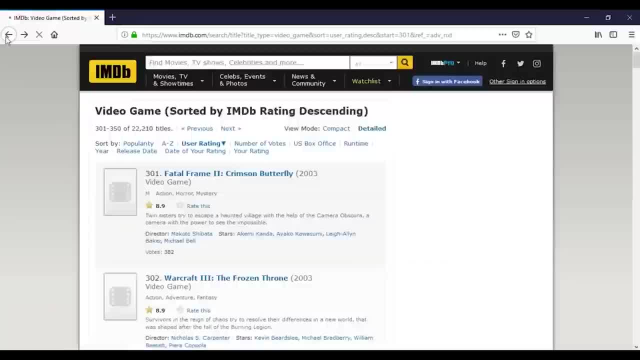 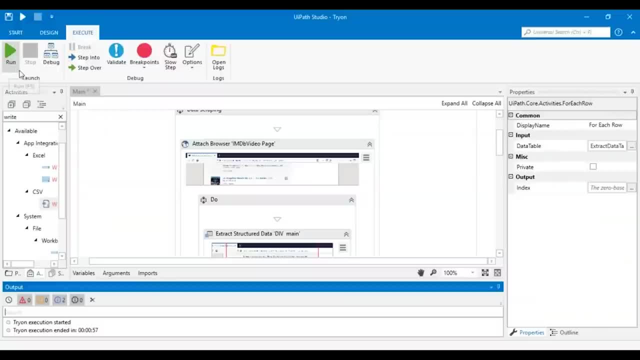 Now what I'll do is I'll go back to my Excel file, Back to my first page over here, And then I'll close this file and then I'll start executing again. Now, instead of just run, what I'm going to do is I'm going 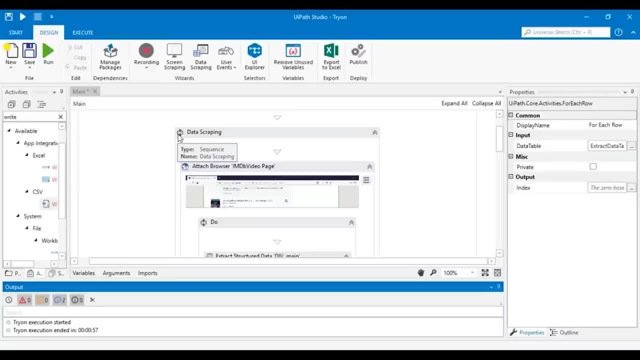 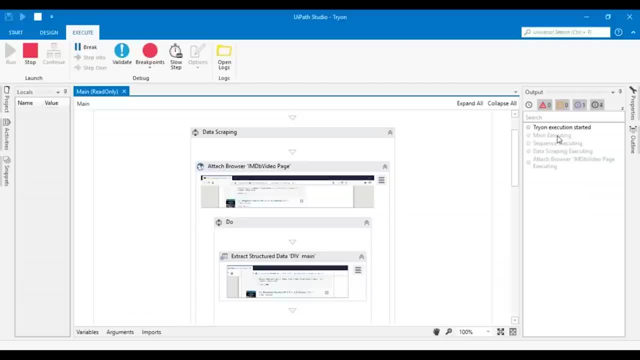 to choose the option of debug so that I clearly understand what is happening in the execution part. So I'll go to execute tab and choose debug. So when you choose debug you can see that you know in the right hand side in the output section that you know the. 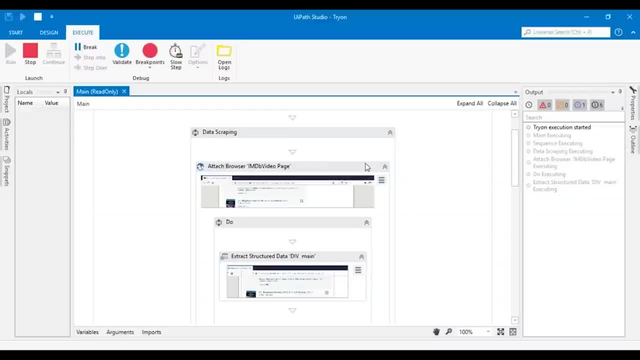 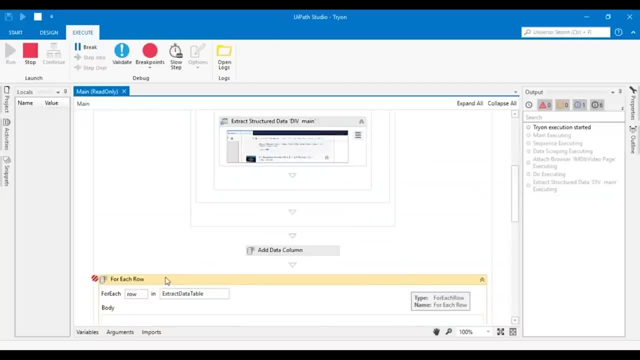 execution has started and the main is executing. the sequence is executing and the data is getting scraped right Now. once the data is gets scraped, you'll see that you know the execution stops at this particular activity. that is, the for each row activity. 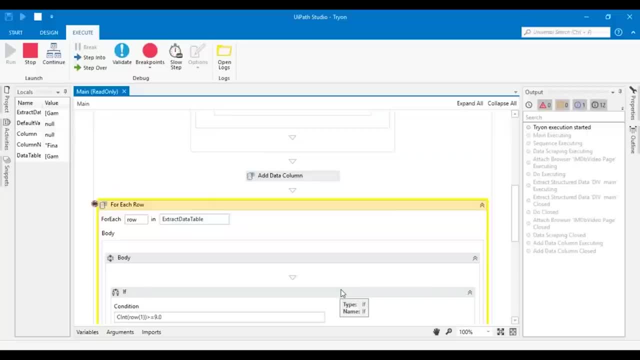 All right. So that means from over here, we can have a manual execution, by which I mean you can control your execution and see step-by-step execution. Now, what I'm going to do is I'm going to choose this option of step into and then I'm going to see step-by-step execution. 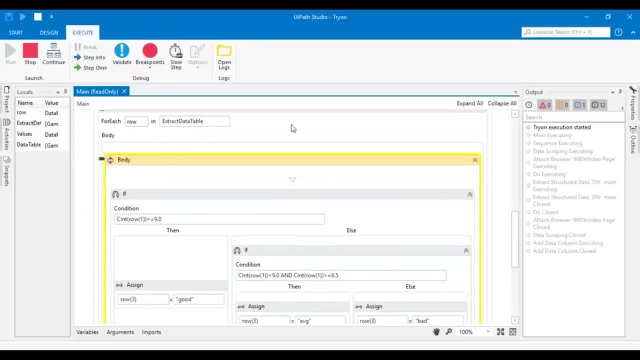 right, So I'll click on step into and then you can see that you know this particular part has been executed, and then it's waiting for a next step into so that you know the body section gets executed. Right, So I'll again click on step into and you can see that you. 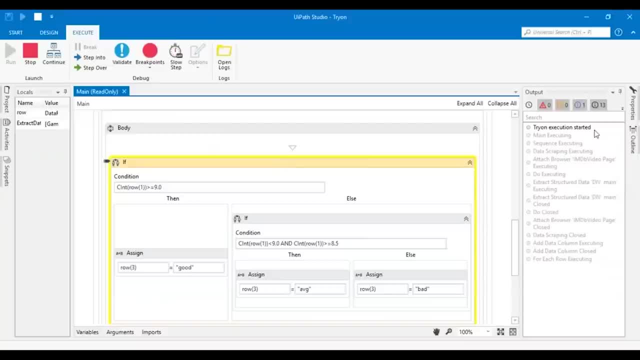 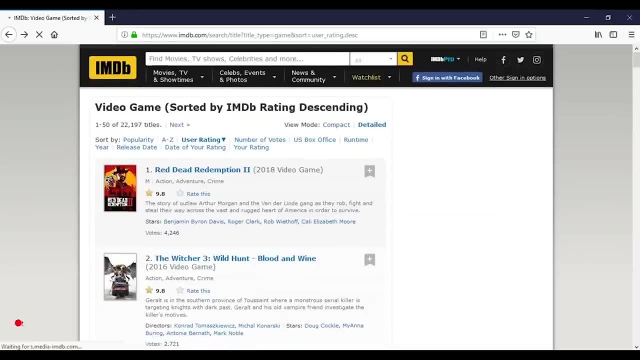 know for each row has getting executed and then the body will get executed and then again the execution would stop until we click on step into again, right? So in the first page that you see, our first game had a rating greater than 9, right. 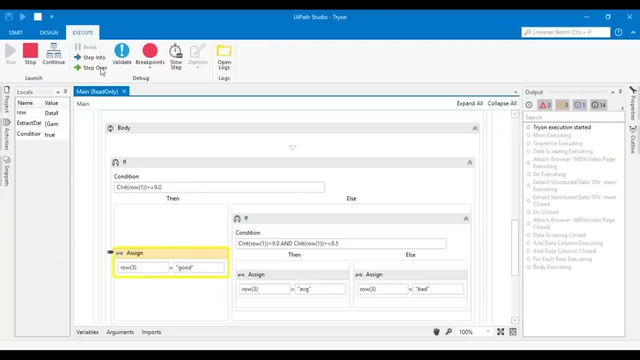 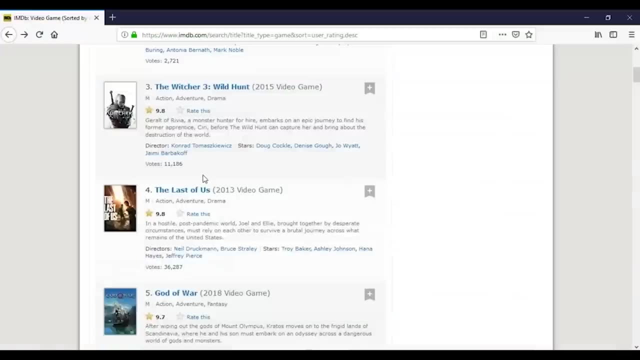 So that means it should go over here, So that means it's going fine. Now let's again click on to step into and let's see so again. and if condition is getting checked, and then it means the second game is getting checked, So the second game. 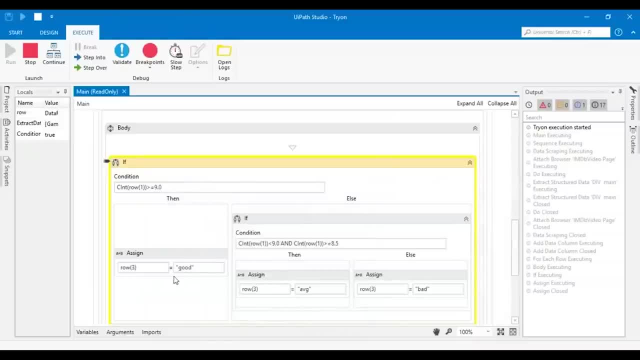 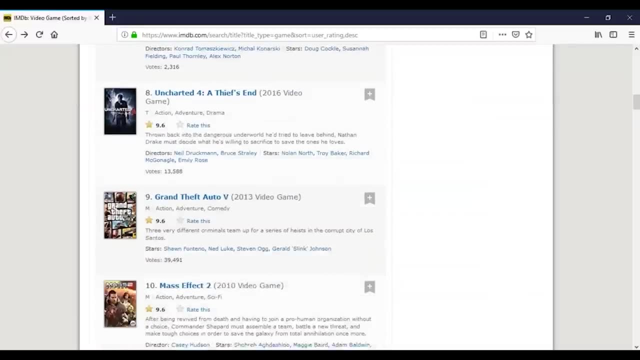 Rating is also greater than 9. So it should again go over here and should be rated code, right? So let's just see that. so that means it's running fine, right? So now let's just check into some game which has rating less. 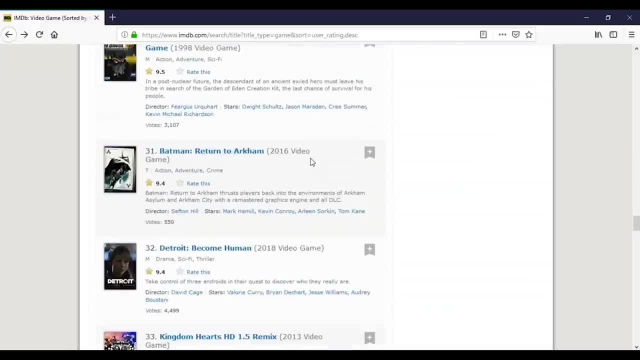 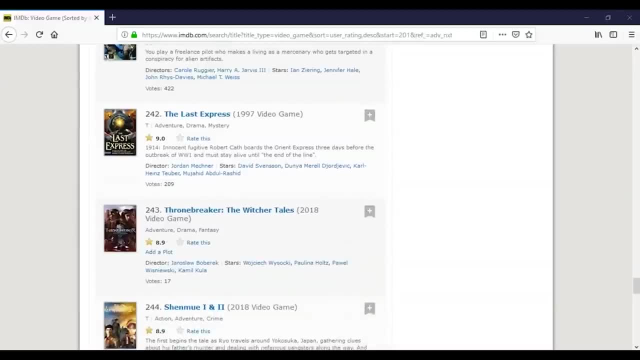 than 9.0, right? So we'll move on to the next page, I guess. So over here you can see that you know this particular game has less than 9.0 rating, right? So now let's just click on to step into and then, if you keep, 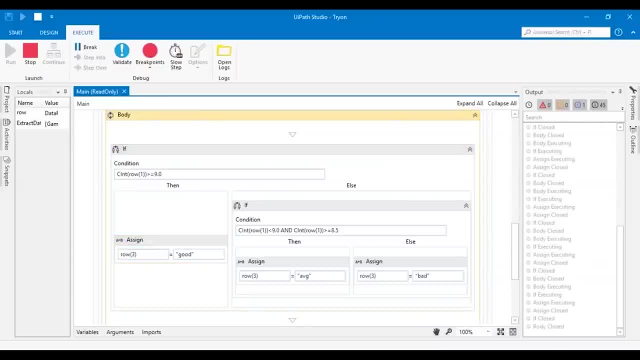 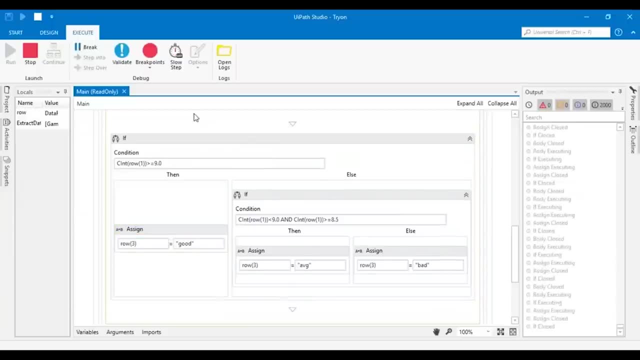 doing this, you'll see that you know until we go to the game which is rating less than 9.0.. So you won't understand where the error is right. So let's just do that, All right. while it's executing, let me show you one more feature. 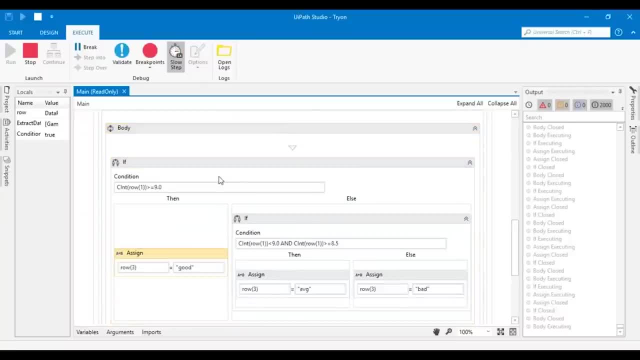 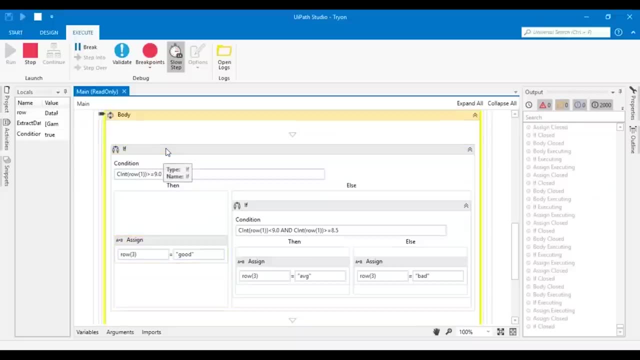 over here. That is the slow step. So now you can use the slow step, you know, to understand which exactly activity is running. So, as you can see on the screen, the activity which is getting highlighted is basically getting executed. So you can, you know, increase the speed of slow step. 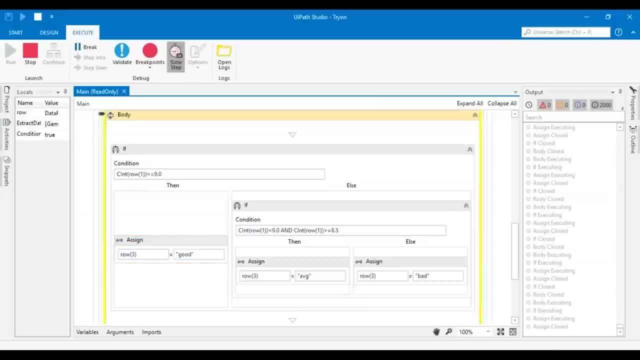 Now it is like it's 1x, So if I click on it again it will be 2x, 3x and 4x, right? So that's basically the speed of activities, Of how it is running. 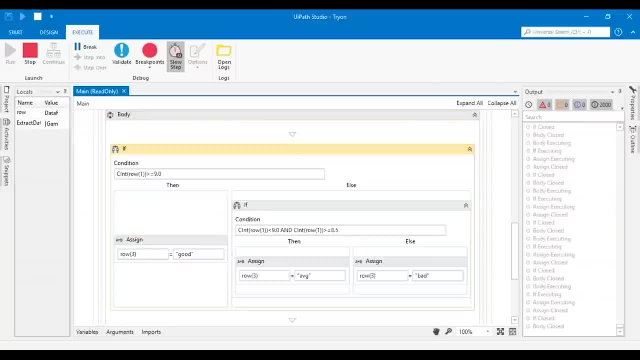 So with the slow step option, it makes it clear for you to know understand which particular activity is running. So, as you can see on the screen, so many activities are running. Now, if you observe over here, what is happening is it's never. 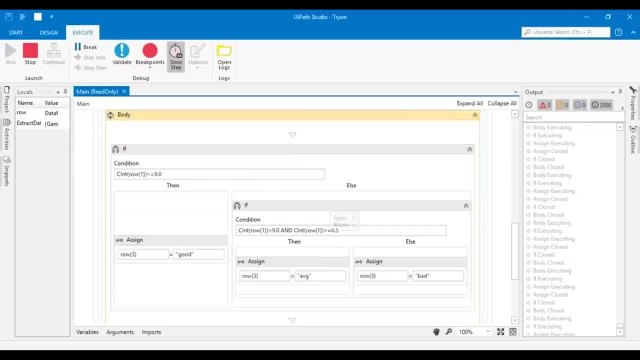 going to the else loop. It cannot happen, right. That means there's some problem over here at the else condition. So basically, if you observe over here, what I've mentioned over here is C int row 1 should be greater than equal to 9.0.. 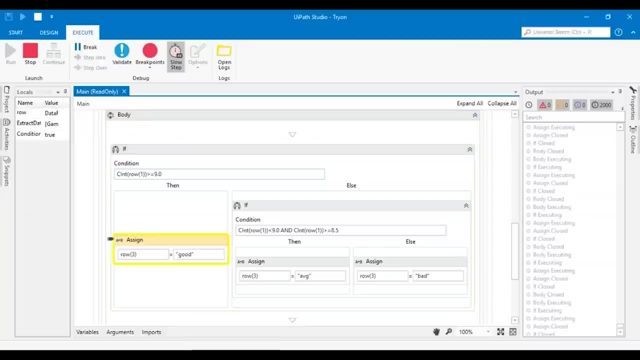 Now, row 1 basically consisted of all the games rating. So games Rating is greater than or equal to 9.0 and it should be an integer right, So it would just consider 9.. It would not consider anything after the decimal right. 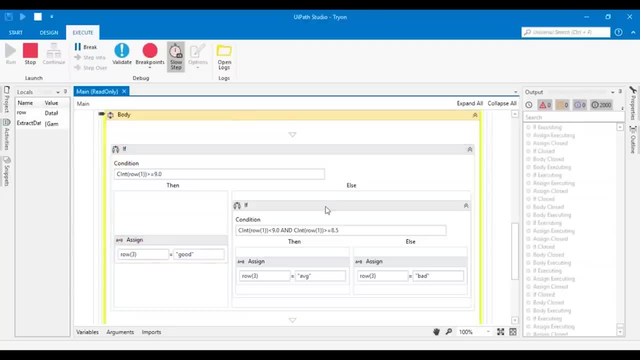 So all those games would be rated as good. Now, Similarly, if you go to the else condition over here, I've again mentioned that you know all the gratings: less than 9.0 and greater than or equal to 8.5.. 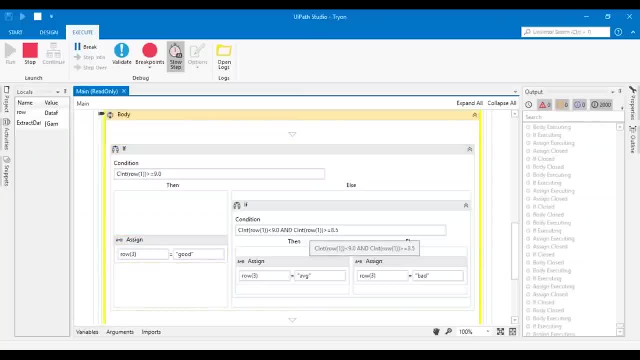 But yes, if you observe over here, what I've mentioned is C int. That means it's again considering an integer and not a decimal right. So 0.0 and 0.5 will not be Considered. It will just consider only 9 and 8, and that is the reason that you know. 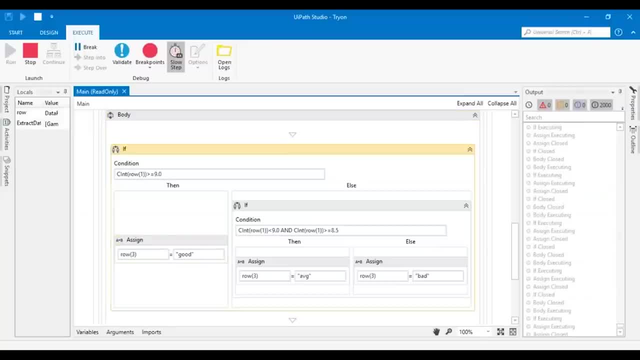 you're getting all the errors, That's because you know it's not considering the 8.5 ratings to be considered as average. It's just continuously taking all the ratings into the good values. So that means this would never go into this particular loop and all the 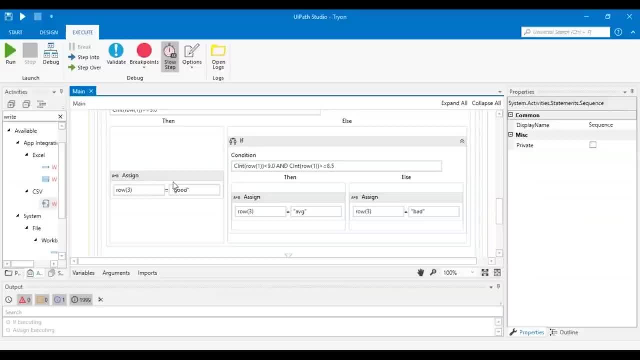 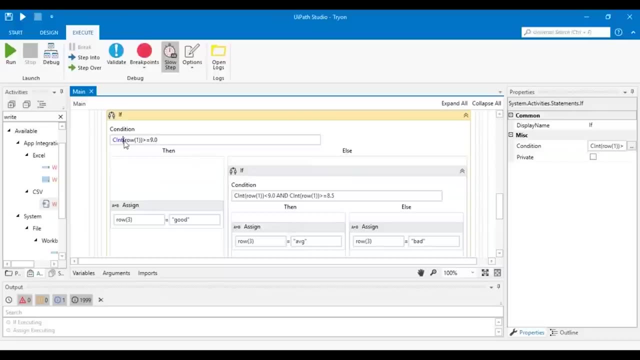 games are getting the values assigned as good, right. So that's how you know. you understand that. you know this particular loop was causing the error. That's because the conditions that we have mentioned over here are C, int, right. So now, if we just see the output since it has executed, you'll see that. 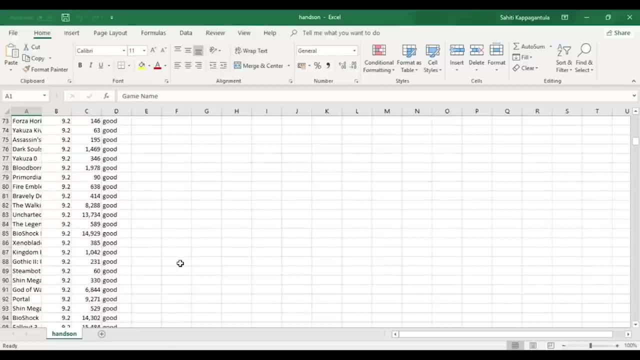 you know we've got all the good values and no values are considered as average or bad right. So if I scroll it down for you, you can clearly see that you know all the games which have ratings also less than you know. 9 have also got. 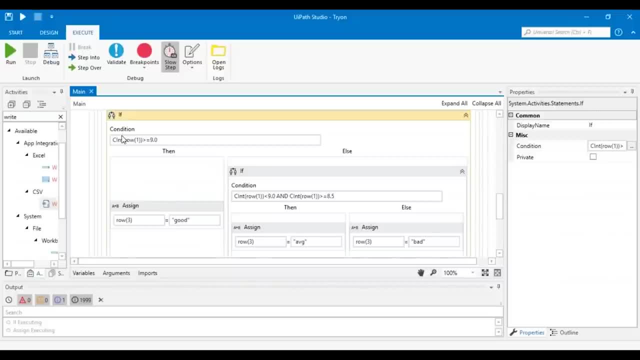 good. So now what you can do for this is you can just change this to C decimal. So that means this would consider the decimal values also. So I'm just going to change it to C decimal And over here also, I'm going to change it to C decimal. 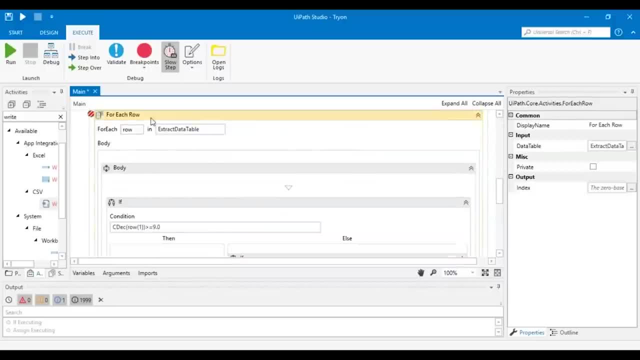 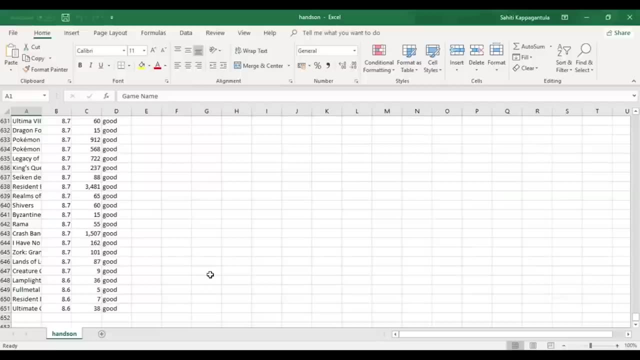 And what I'm going to do is I'm going to remove this breakpoint. So I'm going to go to breakpoints and choose: remove all breakpoints so that the execution stops nowhere, And then I'm going to delete this particular file, so that you know. 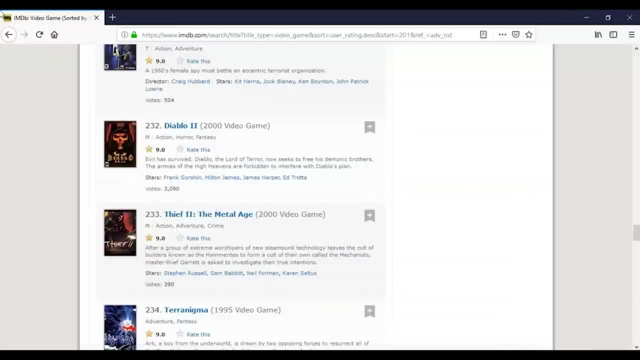 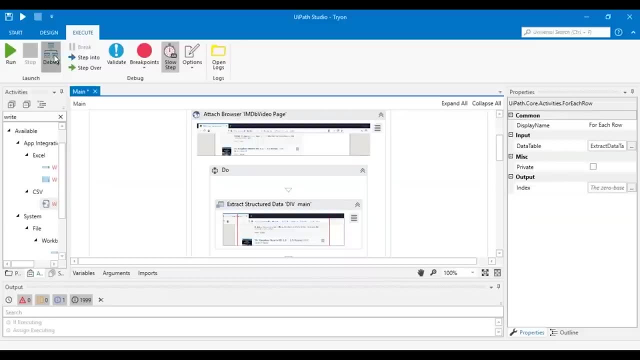 the execution does not cause any error and we'll go to the first page. and now let's execute a program again, right? So when I execute the project again and I click on debug and let's say, you know, we highlight the options. 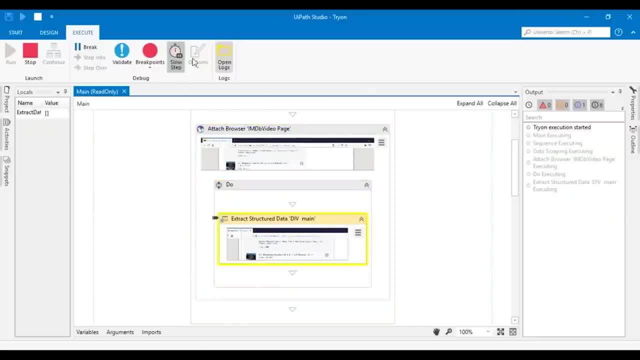 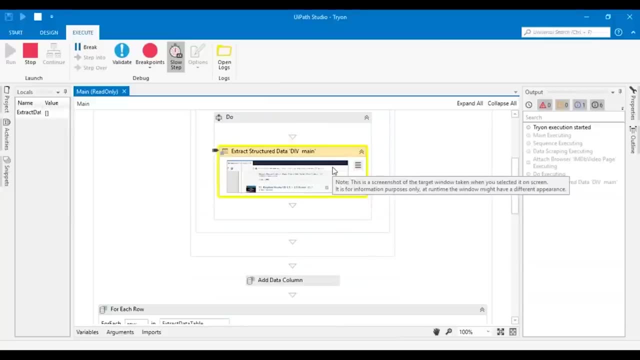 So I'm going to use slow steps. So you can see that. you know it's continuously debugging, right? So I'm just going to remove slow steps so that it runs fast for me. So, as you can see, the data is getting extracted. 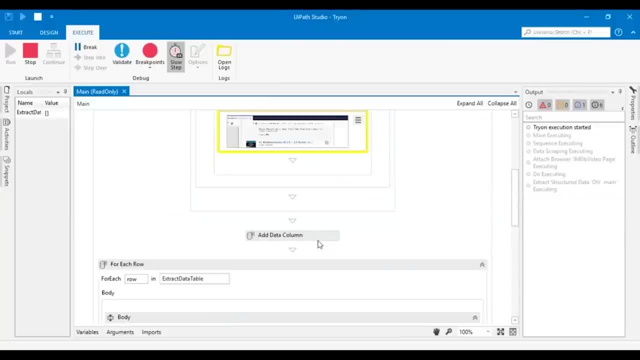 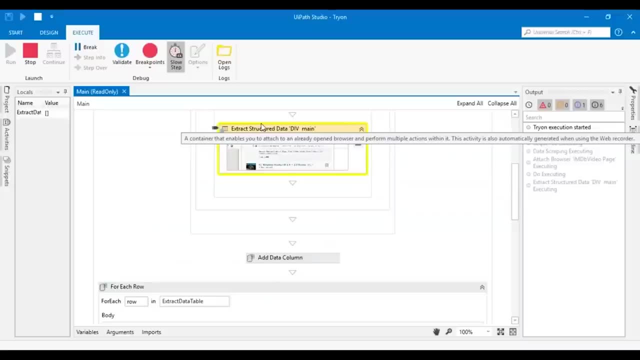 So once the data is been scraped from the website, it will be added. So you'll see the next step, and once it is done, I'm going to just remove that slow step so that it gets executed in a really fast way and we see our 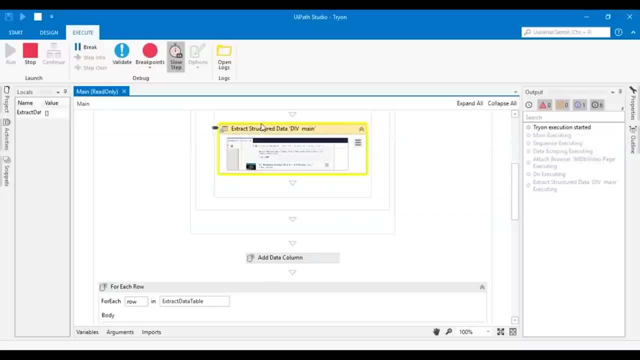 output right. So that's how guys, you can basically, you know, debug the errors. So as and when it's executing, let me just again revise all the options for you. So the run is basically used to run the project, Stop is used to stop the execution. 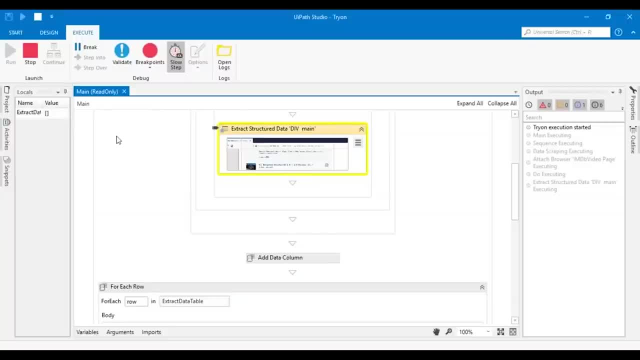 So if I just click on stop over here, the execution will get cancelled over here itself. continue is to you know, continue debugging break is to give us hold to the execution, so that you know if you want to add something, or you know if you want to change something or if you want to see any. 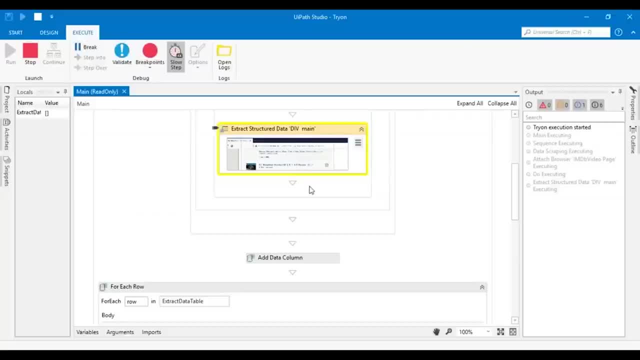 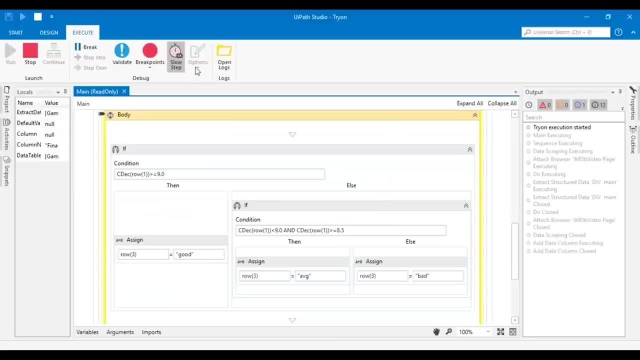 errors, then you can see the errors step into. as I mentioned before, is to go to the next step and then validate is to check, validate all the errors, breakpoints is to add breakpoints and then slow step is to reduce the speed of the execution right. 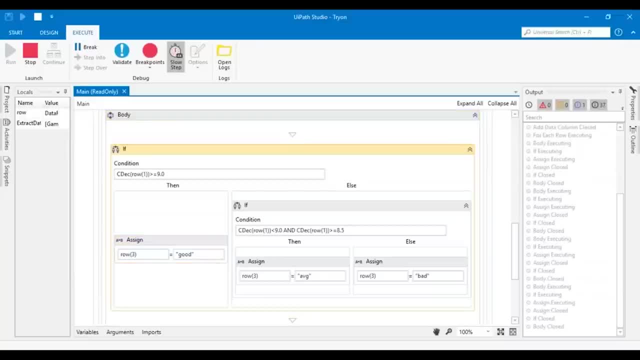 So, as you can see, It is common to our if loop and it is getting executed. That means all our games have been scraped and all the game ratings has been given. So, based on these ratings, all the games are getting rated as good, or 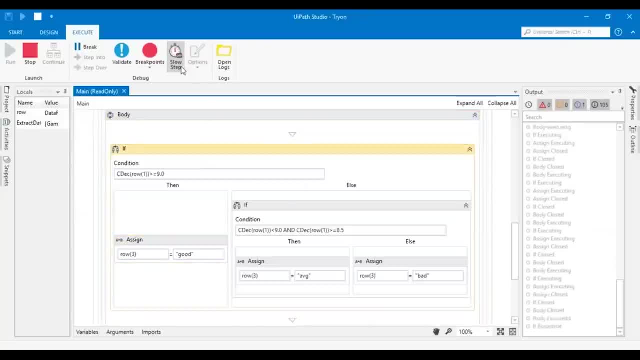 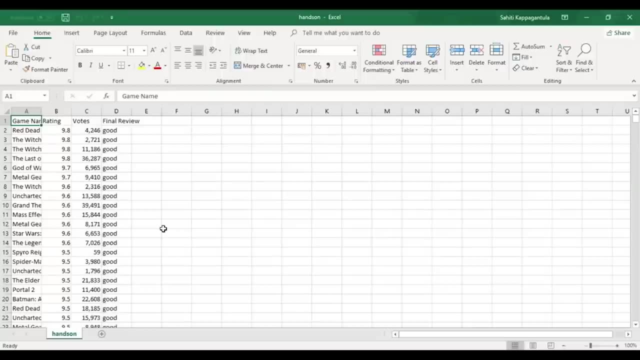 average or bad right. Let them just get executed, All right. So, as you can see, our project has been executed. So what I'll do is I'll just open that file And you can see that you know all the games whose ratings is greater. 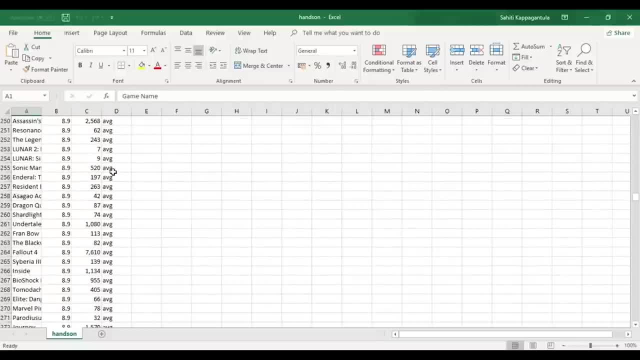 than 9.0 has been rated as good and then when the rating falls below 9.0. You can see that you know they've been rated as average right. That means we have resolved our errors and that's how you know you. 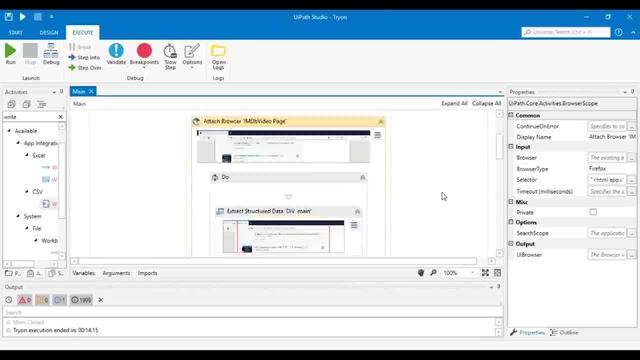 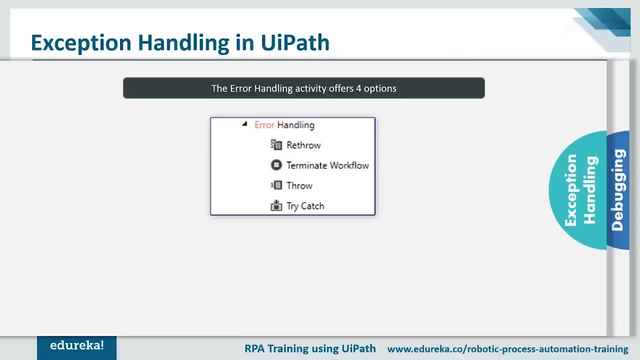 can debug your projects. So, guys, this was a short demo on how you can debug your projects. Now, moving on to the next part, That is, the exception handling. So to perform exception handling in the error handling activity, You mainly have four options. 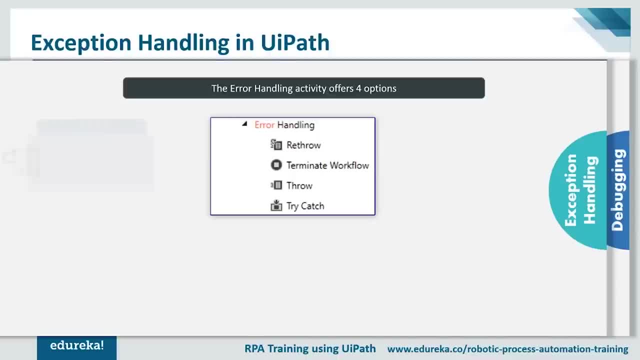 That is the retro, terminate workflow, throw and try catch. So the retro is basically used when you want the activities to occur before the exception is thrown. So whenever you want the activity To be executed, even if it has any few defaults or errors, and only 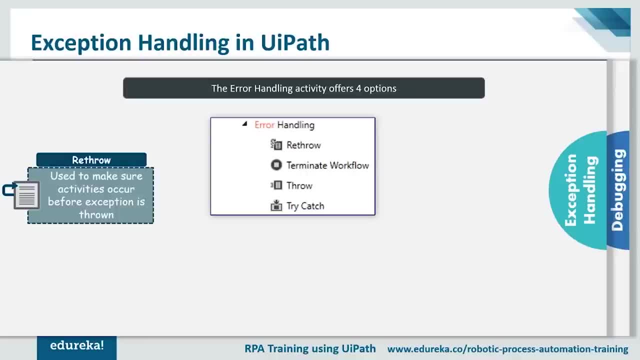 after that you want the execution to be thrown, then you'll use this retro activity. Then after that we have the terminate workflow. So terminate workflow, as the name suggests, basically terminates the workflow the moment the task encounters any error. if you're performing an automation of 10 tasks and then if any one of the tasks encounters, 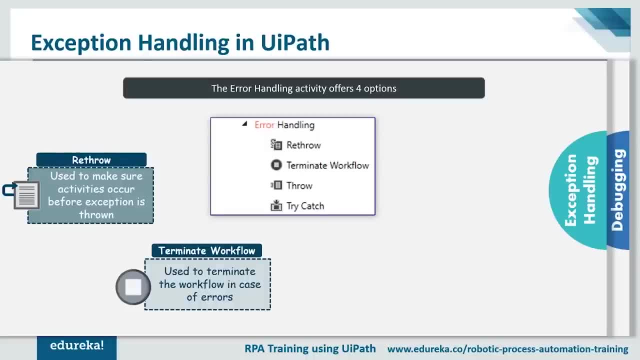 any error and you use this particular terminate workflow handling activity, then at that point you know the workflow would be terminated And that helps you to resolve your errors. Now, after this, we have something known as the throw activity. So with this, throw activity is used whenever you want to throw your error. 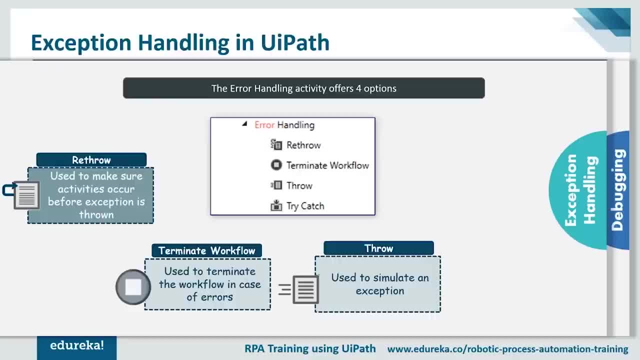 before the execution of the step. So when you want to, you know, throw your error and then you want to throw it before the execution of the step, you use this throw activity and then we finally have the most popular one, that is, the try catch activity. 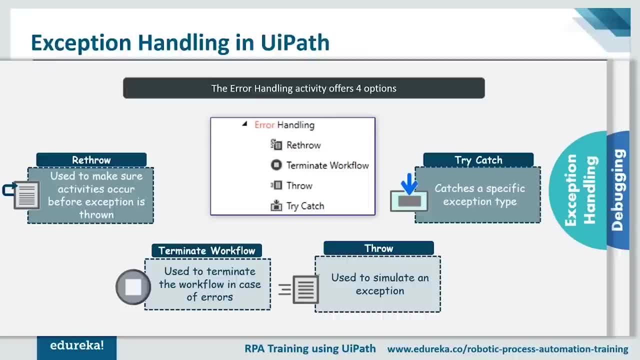 So the try catch activity is basically used whenever you want to perform error handling and you want to catch a specific exception type. So when you use the try catch activity, Whatever you want to test or you can consider whatever activities or you know maybe a list of activities that you want to test- you can just 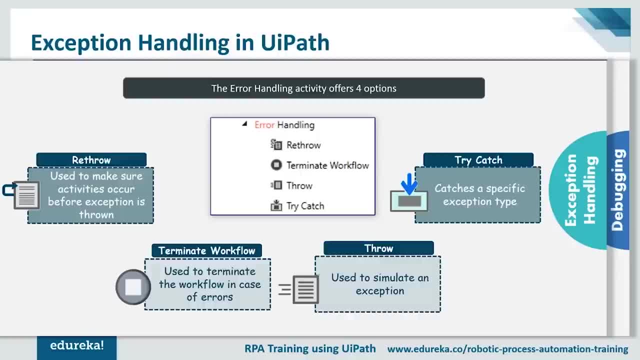 put it in the try section and then if any error occurs in those activities which are put in the try section, those errors can be handled by using the catch section. So in the catch section you can either put a message box or a login page or any such assign activity or anything that you know that handles. 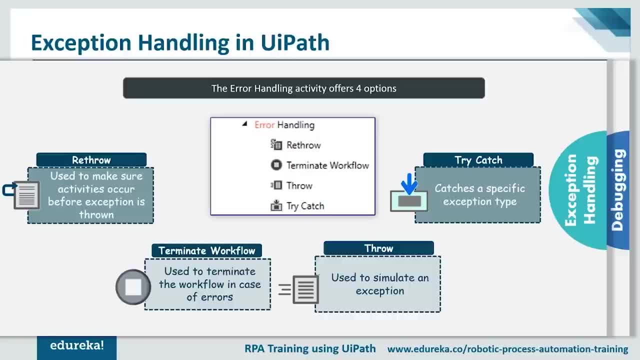 your errors. So I'm going to show you how you can use this activity. when I move on to the hands-on part, And in this try catch activity, Let me also tell you that you have a third section, that is the finally section. So the finally section is basically used to mention the activities which 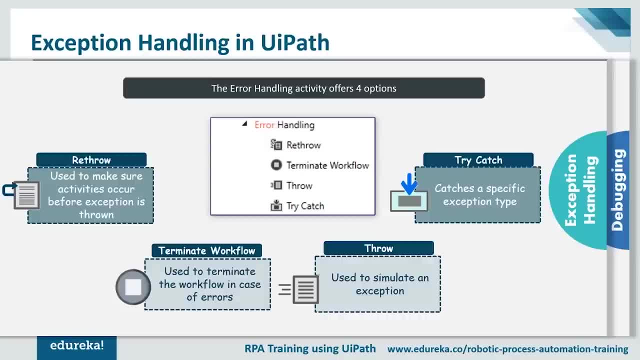 have to be performed after the try and catch, a perform right. So I hope, guys, all these four activities are clear to you. That is, the retrow, the terminate workflow, the throw and the try catch. So let's go back to the demonstration part again. 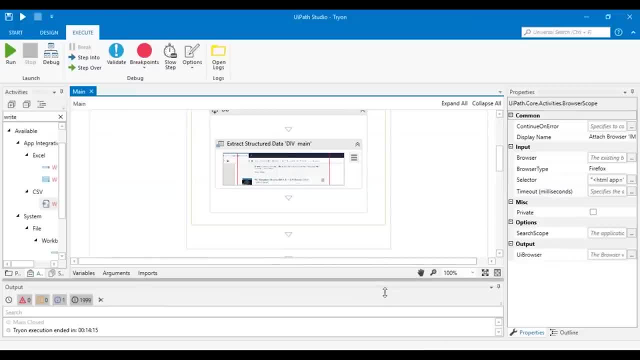 So over here, as you can see, I'm going to use the same demonstration part. Now what I'm going to do is, let's say: you know our Excel file will be open when- the when- we execute the project. So that means it will show an error that you know our Excel file is. 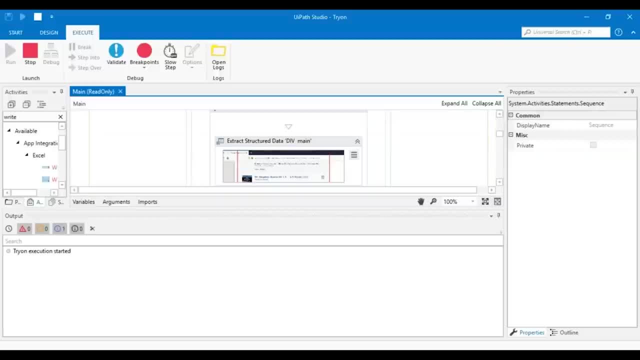 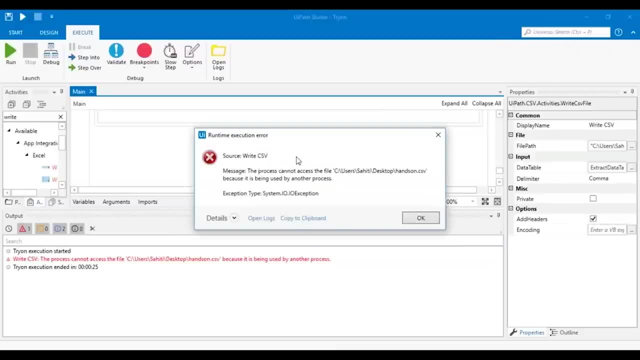 open. So let me just run the project for you so that you see the error. All right. So, as you can see on the screen, this is the error that you basically see that you know your right CSV file. that is basically our output file. 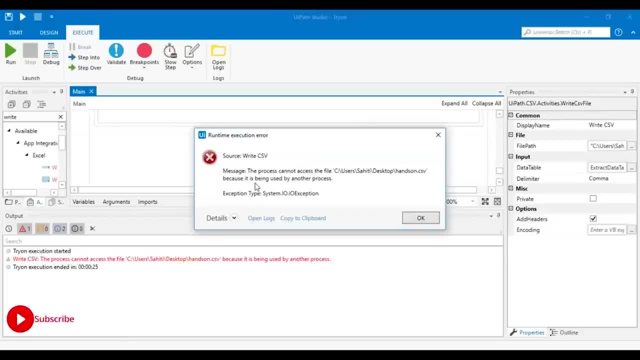 cannot be open because it is already being used by another process. That means it's open right now. to avoid such kind of errors, You can use the exception handling. So what you can do is you can just add a try catch activity. So what I'm going to do is I'm just going to search for try catch. 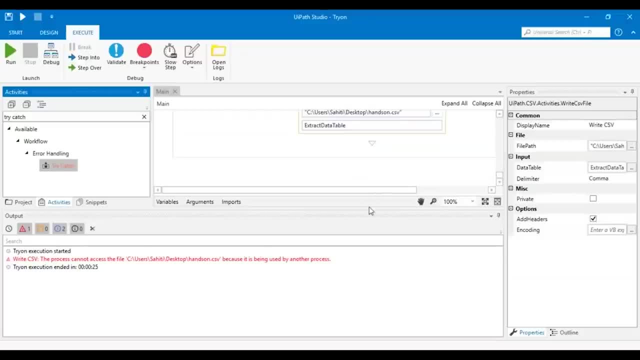 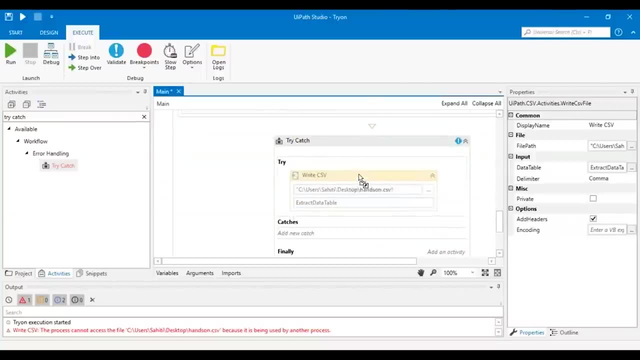 So we here, and then I'm going to add it over here. So I'll just drag this down so that you clearly see Right now. what I'm going to do is I'm going to put this right CSV file into the try section and in the cat section let's say: you know we. 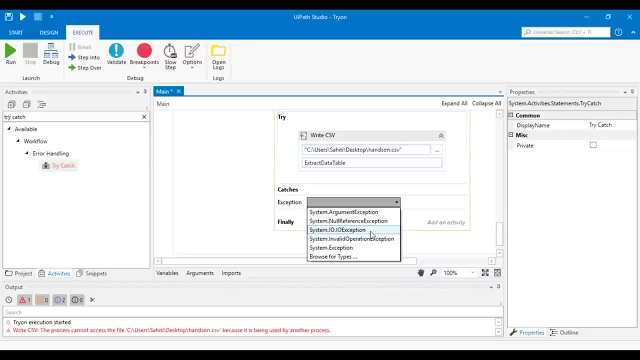 want to deal with the error of IO exception, right, Because that is the error that has come up. So I'm going to choose the exception of IO exception and then I'm going to add an activity, right? So let's say, we want to add the message box. 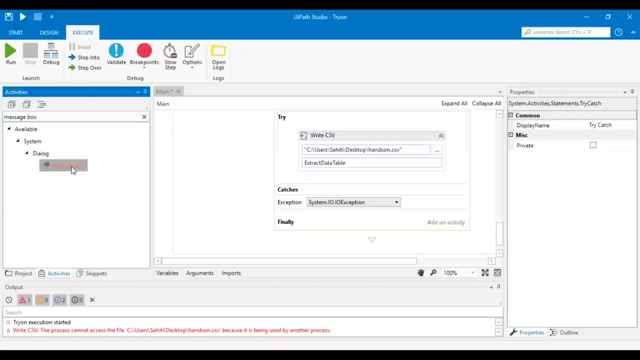 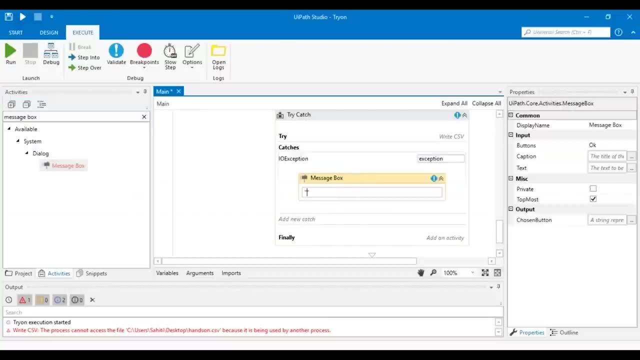 I'll just search for message box so that it displays an error Once the exception has been found, and I'll drag and drop it over here Now, once this is done, I just mentioned the message. Let's say, you know, Excel file is open. 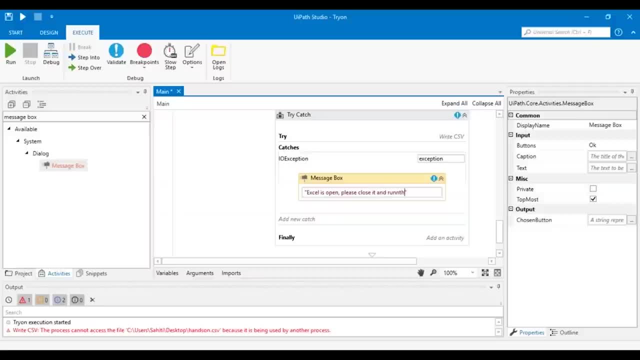 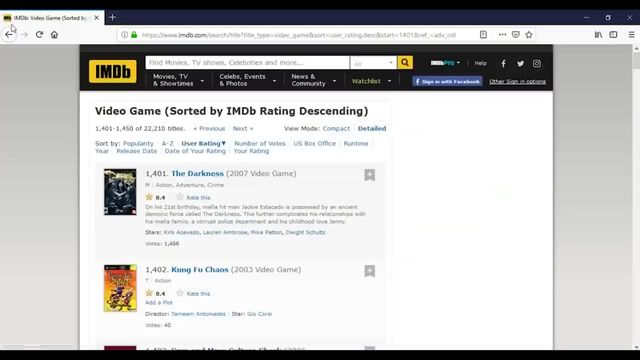 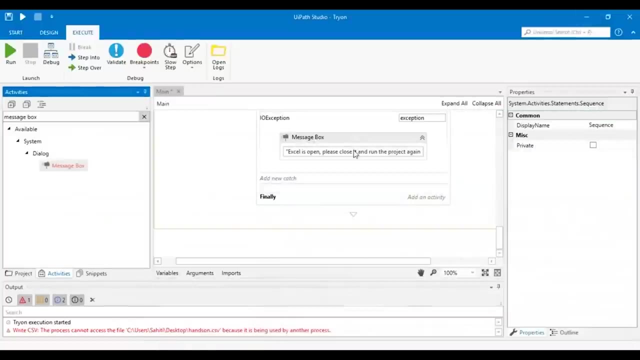 Please close it and run the project again. So I'll just do that, and then let's just run the project again. So what I'll do is I'll just go to the first page And I'll keep this file open. That is basically my CSV. 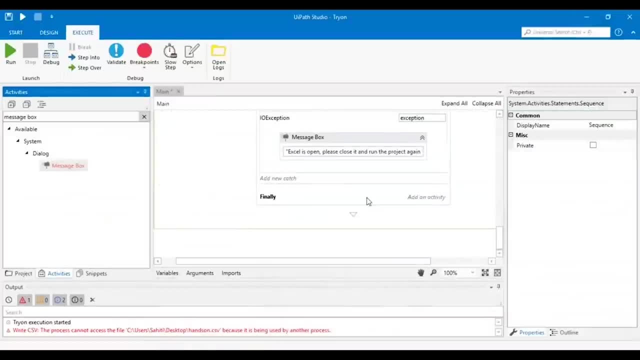 File to which you know all the data has to be scraped and it has to be stored inside the CSV file, and then I'll click on run right. So let me just do that. All right, So, as you can see, you know, since our Excel file is open, the exception. 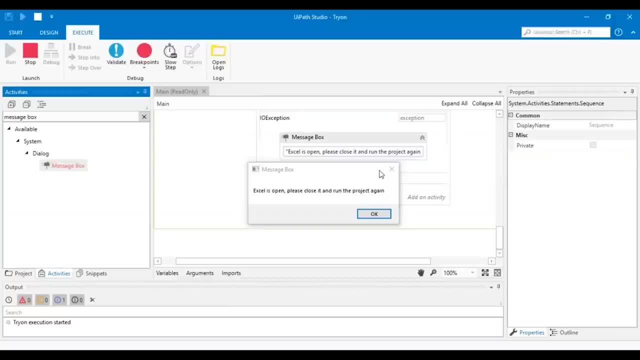 is getting handled. instead of an error that comes out, instead of error that you saw before, this message box displays which says Excel is open. Please close it and run the project again. right? So that's what we mentioned over here. So you can just click on OK and then you know what to do. 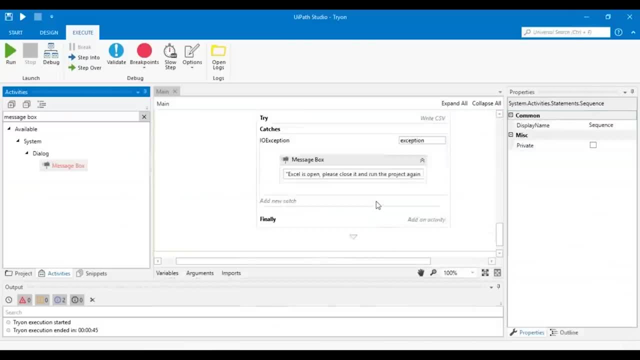 So I'll just close My Excel file and then I can run the project again, right? So, guys, that's how you know you can perform debugging and error handling. So I hope that you know you've understood both the concept and both. 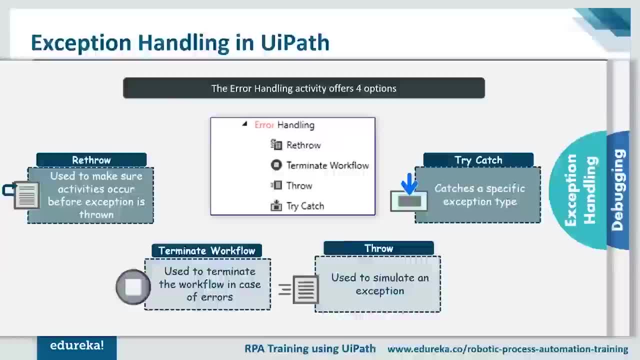 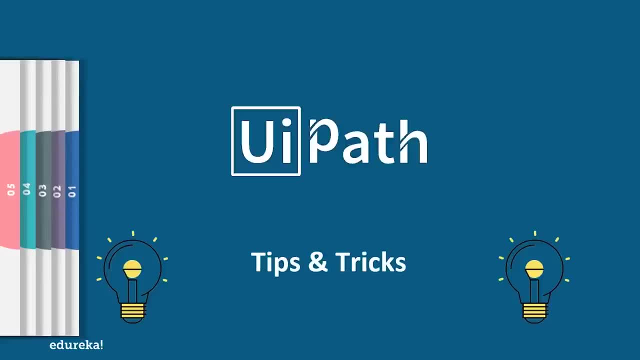 their functionalities. Now let me tell you something more interesting over here. So what I'm going to do is I'm going to discuss few tips and tricks So you know, you can say something like a key takeaways that you need to know and some few errors that normally people do. and how do we? you 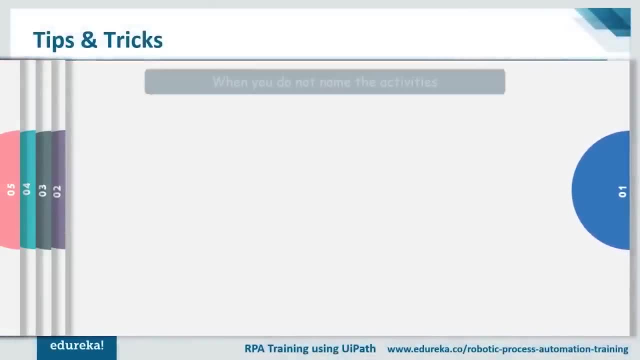 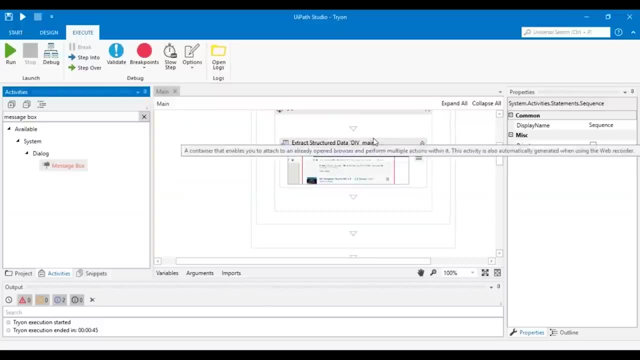 know, resolve those errors right. The first thing that comes up is: you know, when you do not name the activities, by which I mean that you know I open my UI path. we've dragged and dropped so many activities, right? 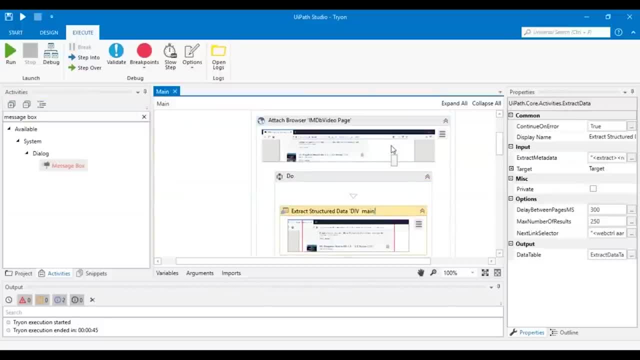 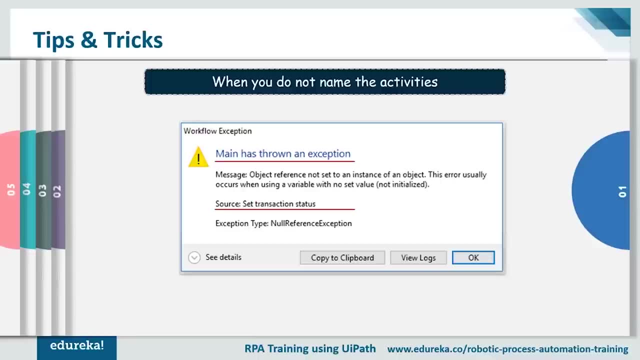 But yet we haven't named any of them. We don't name them and we just drag and drop them right. So it's always advised to name these activities, because you know, if you do not name any activities and you would see some error like this: 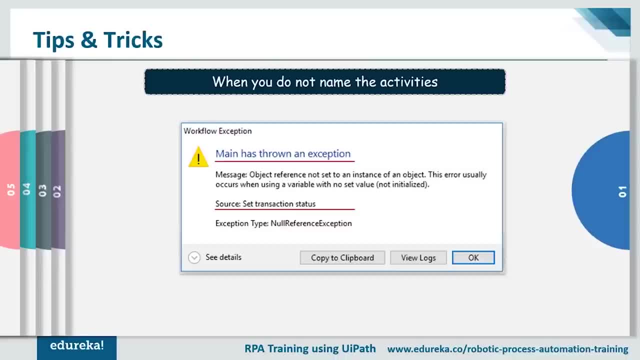 that you know main is thrown an exception and the sources set transaction status or any other status. So anybody from a non-IT background would never understand that you know what is a main and how the main is throwing an exception or even. 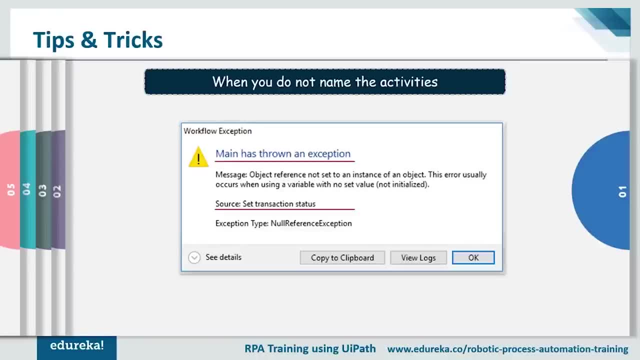 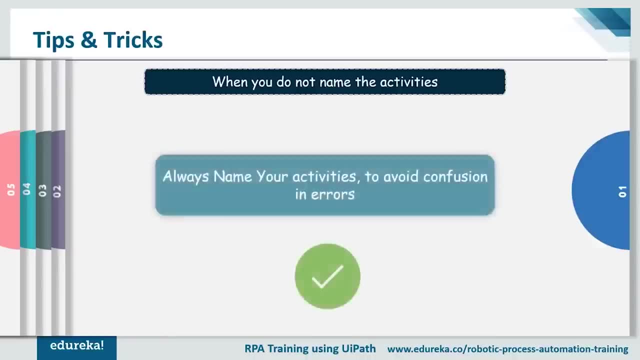 from an IT background person would not get into. If it's a big automation task, of which, exactly which activities throwing an error right? So to just avoid such kind of errors, What you can simply do is you just name your activities to avoid any. 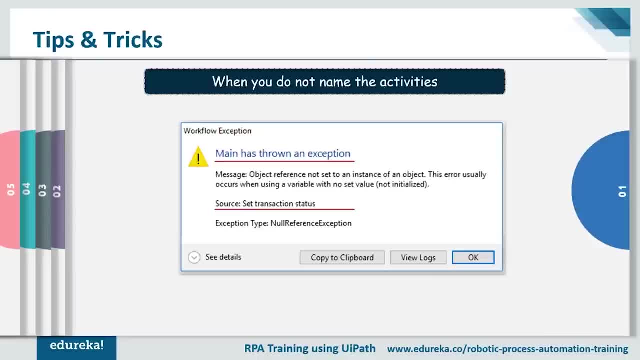 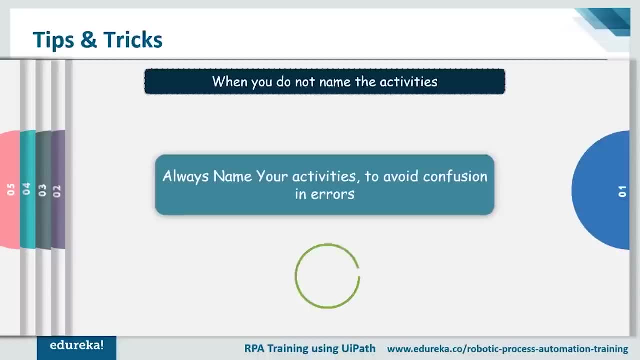 confusion in the errors. So once you just name the activities, you would get an error that you know. this particular activity with the name is throwing an error or is throwing an exception. So that's one key takeaway that you can take that you should always name. 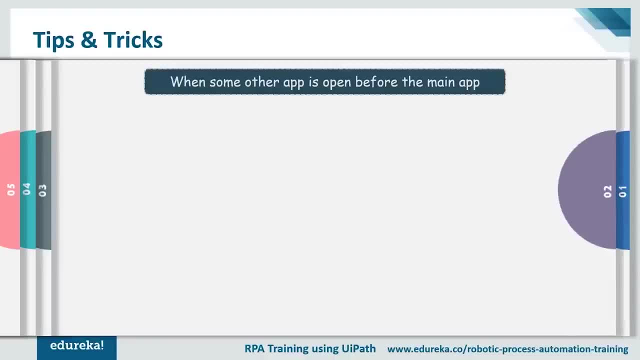 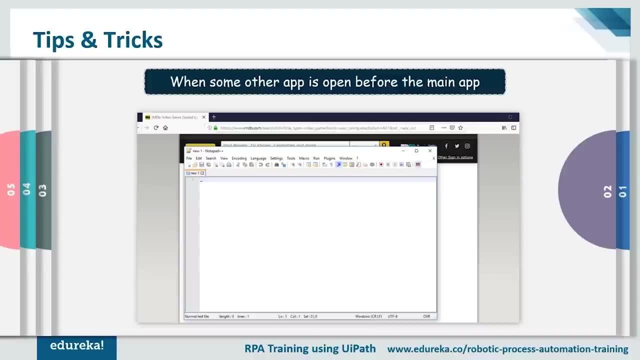 the activities. now moving on to the second one, which is basically when some other app is open before Main app, like for the example over here, for the demonstration, I use the website right. So instead of the website, if I have a website over which I have my 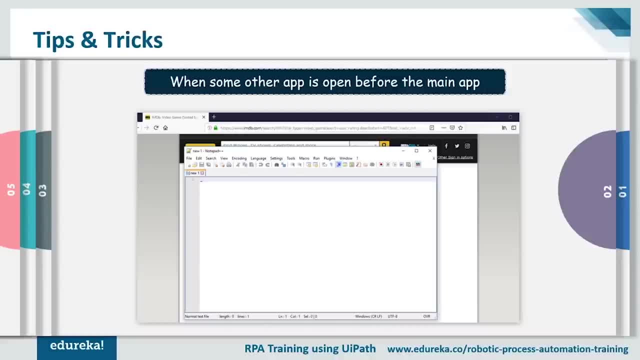 notepad plus plus open, then obviously UiPath would not understand from where it has to scrape the data. right? You need to make sure that you know your website is open and no other application is open. So this is one of the most common error that everybody does. 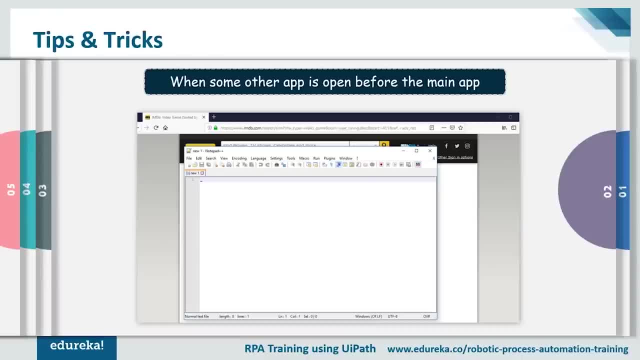 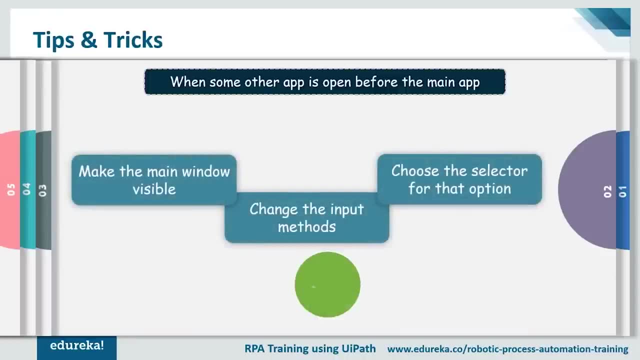 They just open few apps and then they expect you- I part to understand from which. do you know they have to scrape the data or to any other activity, right? So in such errors you basically have three options: either You just close all the apps and then you know you make sure only your. 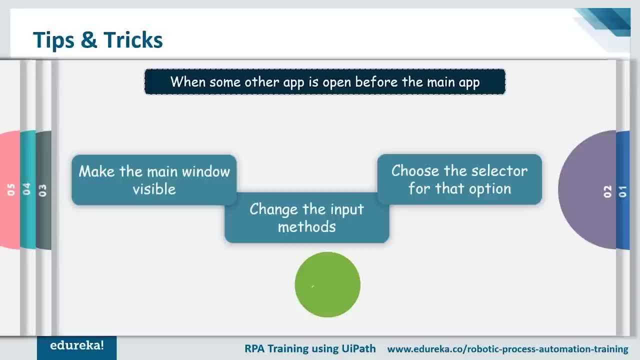 main app is open. So we are. in my case, I would just make sure that you know my Mozilla Firefox is open, with the website open, and then the data would be scraped. else You can also change the input method. So when I say input methods, I mean that you know when you have any. 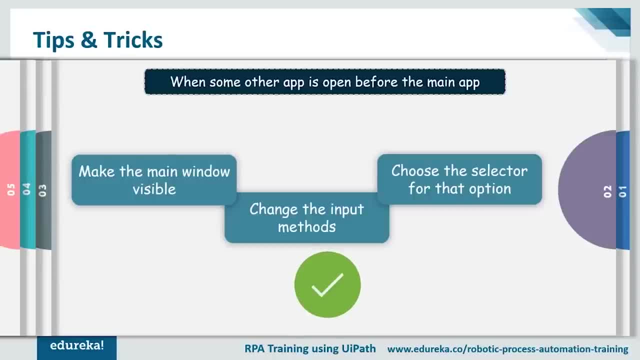 click action enabled in your UiPath Automation task, then you can make sure that you know that click action simulates the click. you can make sure that wherever you want to click, That is allowed to click. and the third option is obviously choosing the selector for that particular option. 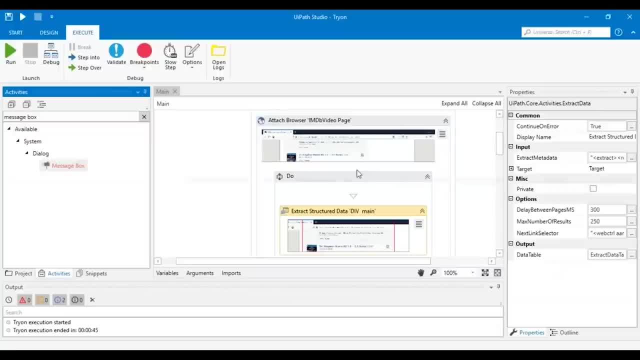 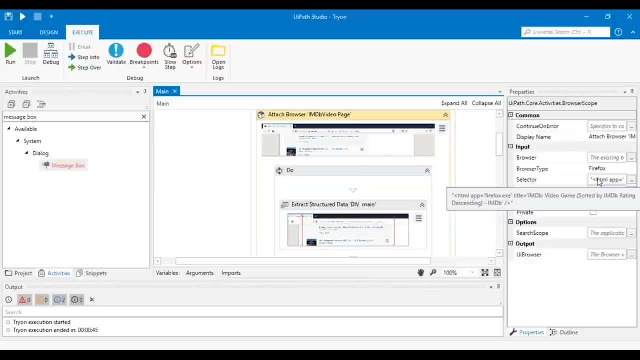 So if you see my UiPath, you will see that you know there's a selector for attaching web browser, right? So that means you know this is a specific selector by which the website is being identified and the data is getting scraped, right? 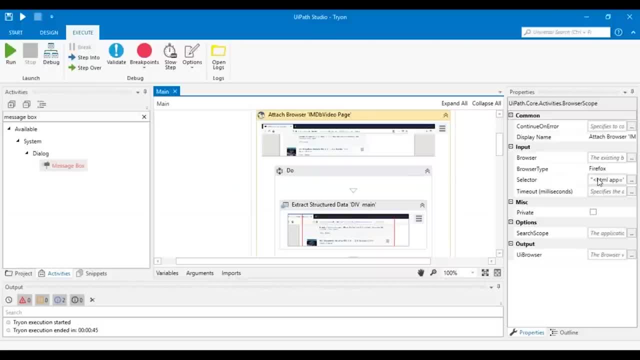 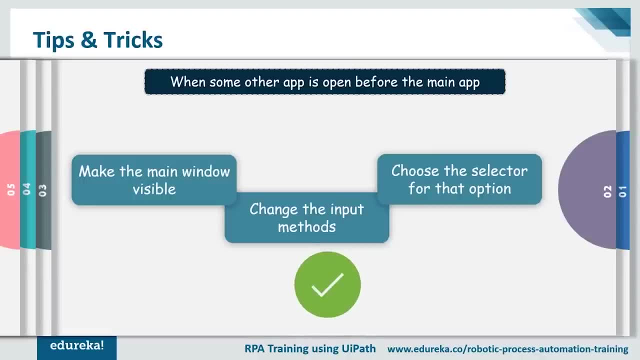 So you can just make sure that you know the selector is the right option through which all the data is being scraped and data is not scraped from any other application, right? But, guys, these are the mainly three options that you can go for that. 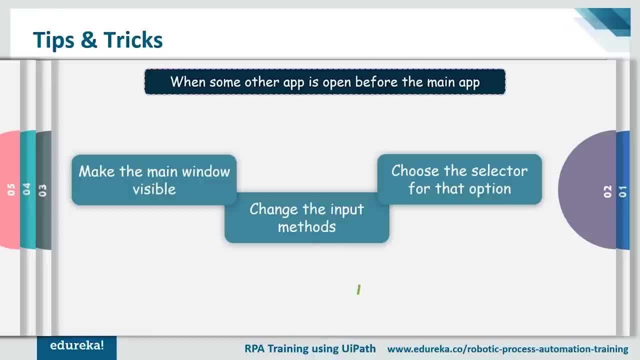 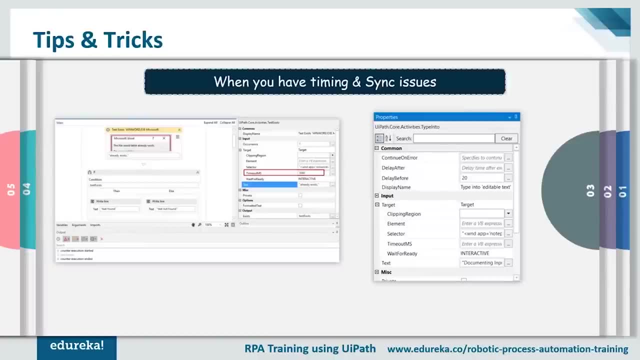 is make the window Visible, change the input methods and choose the selector for that particular option. Now, moving on to the third mistake that people do is basically, when you have time and sync issues right now, I would not say that you know, this is the problem of a user who does it. 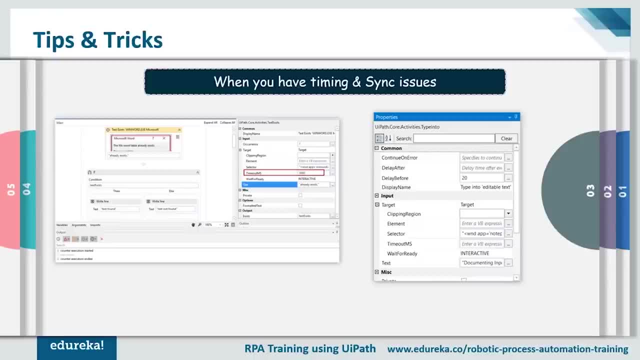 But, yes, it's a problem of the app that we are relying on, right. So sometimes it can happen that you know my web page is not loading on the right time, or sometimes you know my web page just crashes, or you know it just takes longer than expected, right. 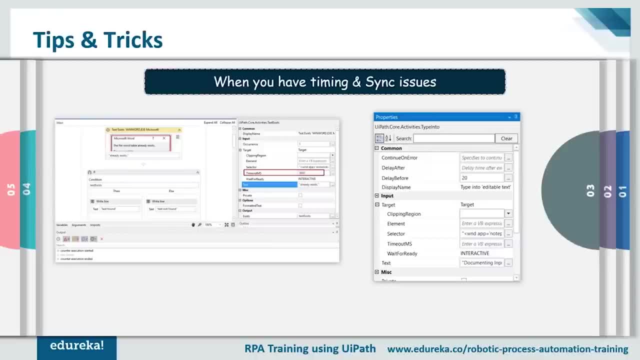 So then UiPath does not understand what to do, right? So by default, if you observe this timeout MS section, it would be 30 seconds. But if you change it, you know, if you change it to zero, then obviously the time for loading would not be considered by UiPath and that would. 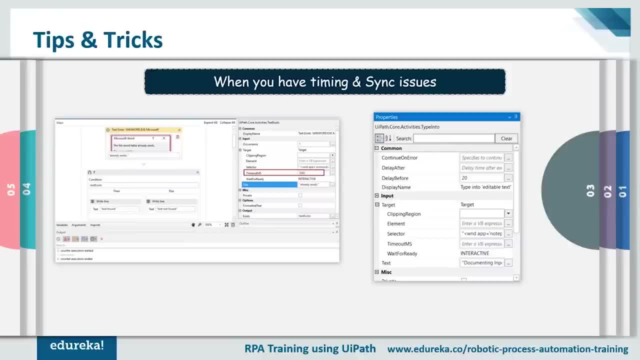 throw an error right. You always have to make sure that you know. you put a little bit of timeout- milliseconds- so that you make sure that you know if it's 30 milliseconds or three seconds or anything. you know all those timings. 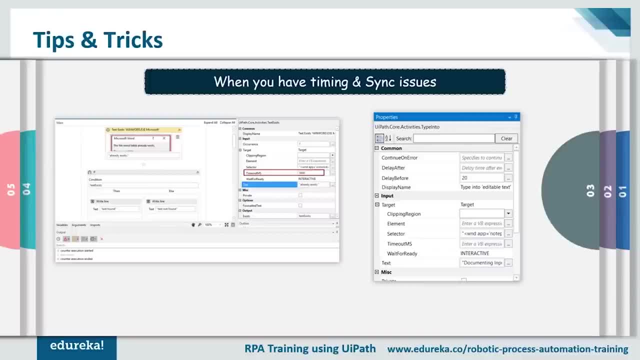 and all the timing for loading of web page or, you know, opening an app is considered. So this is one more key takeaway that you need to Understand. that you know are your timing should be proper. Now in this, there are three more things that I need to mention it for. 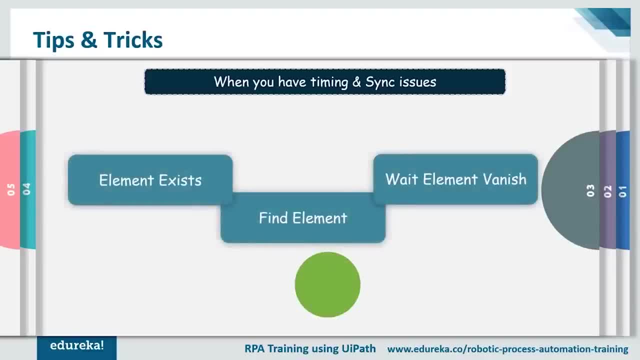 you guys. That is, the element exists, the find element and the wait element vanish. Now these three are basically the activities in UiPath. So what element exists does is element exists does not affect the running of a workflow in any way. right? 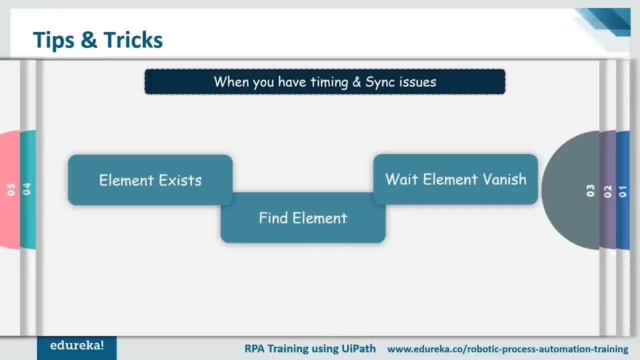 But find element and wait element vanish do affect the running of workflow. So what element exists does? it just returns true or false value, depending on whether the Element exists or not. So basically, what will happen is: you know the element exists, will also tell you that you know if the element is existing or not. 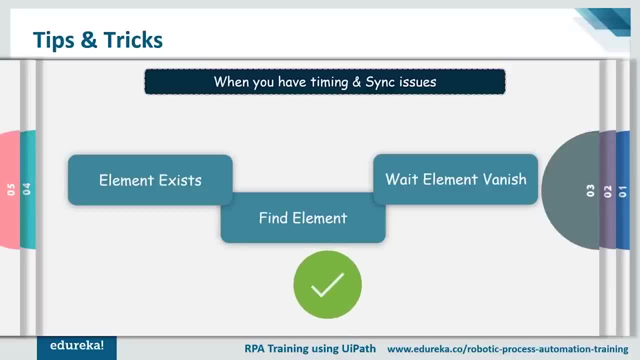 So this is basically for the syncing issue. So it can be, you know, a button or a pop-up or a message or any other components of application that you want to consider. Now, the find element basically stops the automation until an element is found right. 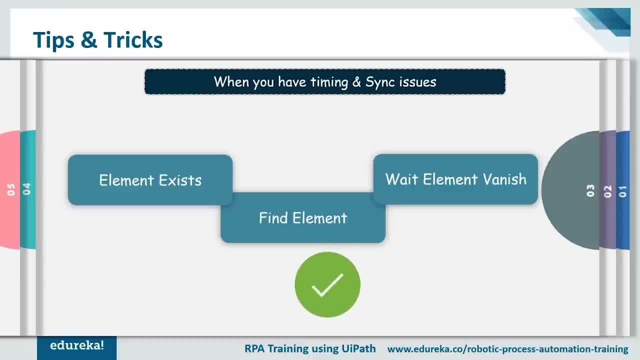 So until an element is found, you can use this find element and the wait element vanish obviously waits for an element to disappear before continuing right. So for the Timing issues, you can consider the timeout parameter in UiPath where you need to mention those milliseconds or the seconds where you make. 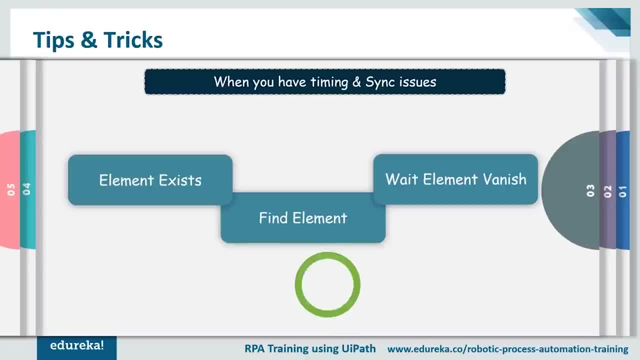 sure that you know, UiPath considers so much amount of seconds before throwing an exception. and for the syncing issues, or the synchronization issues, you can consider the element exists, the find element and the wait element vanish activities. right Now moving on to the fourth one, that is, when your browser crashes. 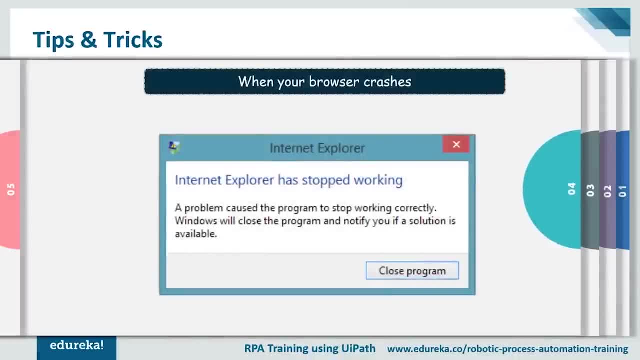 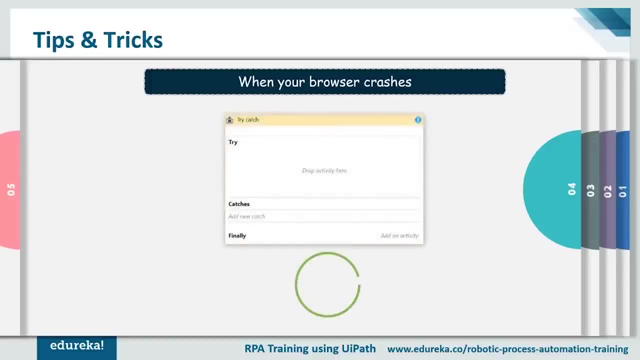 right. So, as I was working on a browser, it can always happen that you know your browser is not working and your browser crashes at the last moment, right Now. in such scenarios, what you can simply do is you can just use a. 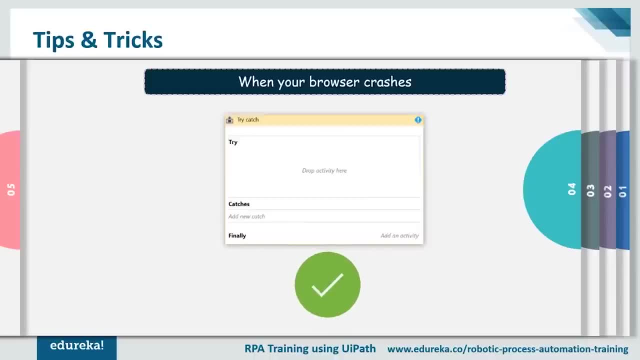 try-catch activity. So with this try-catch activity, what you can simply do is you can just put your browser and whatever activities that you want to perform with the browser into the try section and in the cat section you can just choose the exception type, and then you can make sure that you know. 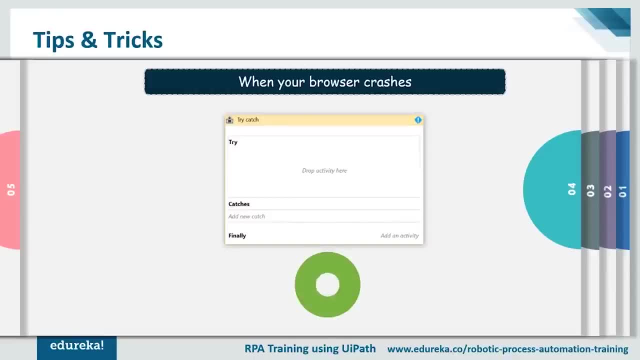 you can add a message box that you know your browser is not working. Please try again. or you know you just have to wait some time. Please try again. And then you reload your browser, check your browser and then you perform the. 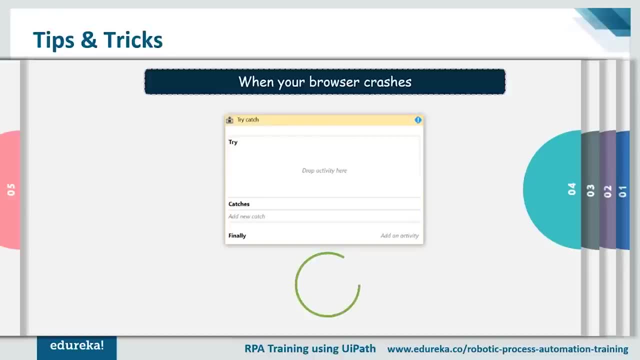 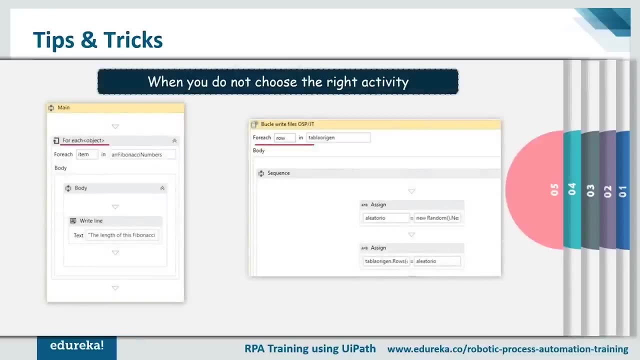 Automation right. So that's how you can handle when your browser crashes. Now, moving on to the final one, That is the fifth takeaway, That is, when you do not choose the right activity. When I say right activity, I mean that you know when you open your 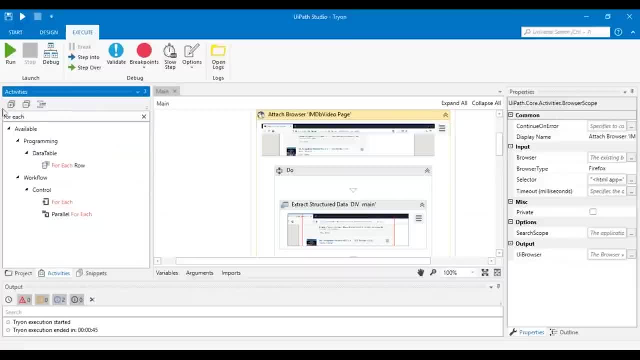 UI path and let's say you know, you search for the for each activity. you get three options, That is, the data table for each row or the control for each and the parallel for each. Now, anybody would have any confusion because you know all the for each. 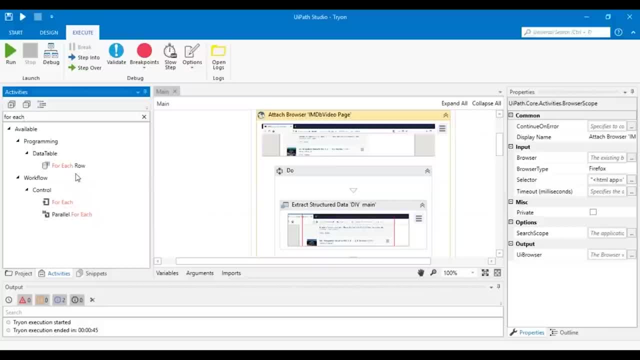 activities have same parameters, right? So now the data table For each row is basically for each row in the data table and the control for each is basically like a for loop which runs to the complete loop, right? So if you see into the presentation, you can see that you know the. 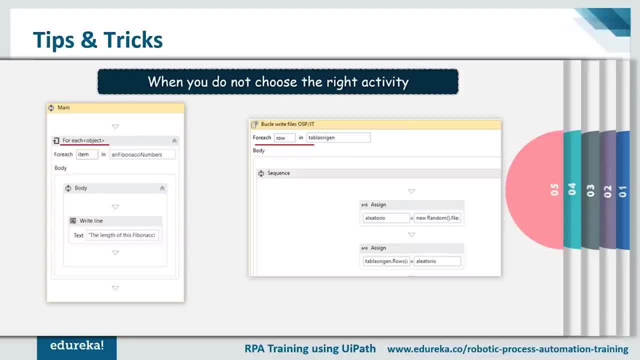 parallel for each one. basically, is used for each item in. let's say, you know to build an array, Then you have a body and then you can have XYZ in this, but for the activity in which you know, it is for each row in the data table and you. 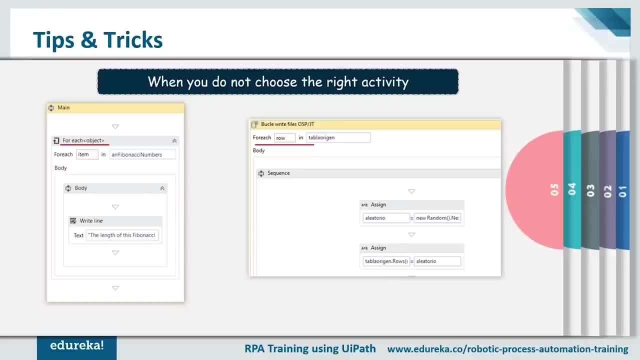 have to mention the data table, right. So generally people get confused by the name that you know. somebody says just use for each activity. They don't understand if they have to use the for each flow activity or they have to use the for each row in the data table activity, right. 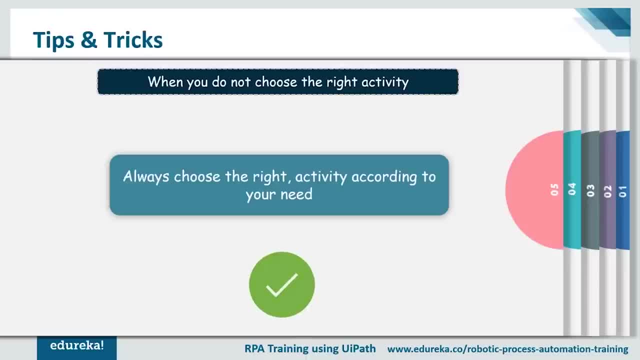 So you have to make sure that you know this is perfect and you need to understand what is your requirement, right? So, guys, that with a few tips and tricks or you know, you can say few key takeaways for error handling and debugging in UiPath. 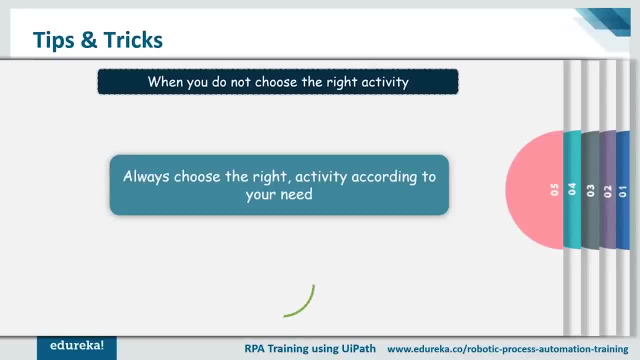 So, guys, before I end this session, I would just say that if you want to debug your errors or if you want to perform error handling, then you need to clearly understand all the concepts, or you can say all the tasks or activities That you've mentioned in your automation, so that you know, you understand. 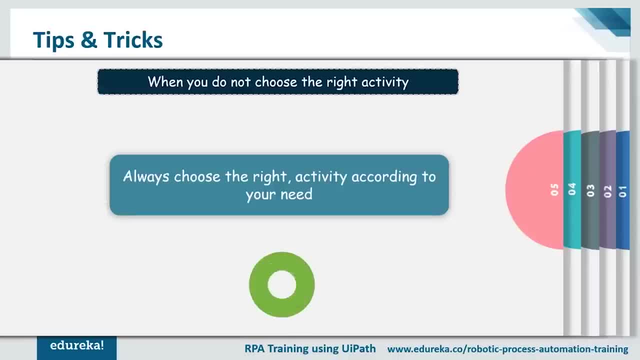 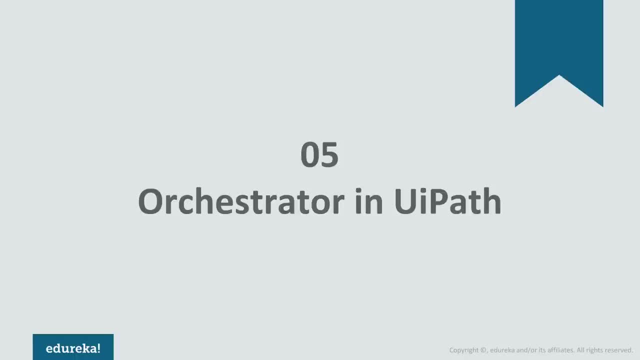 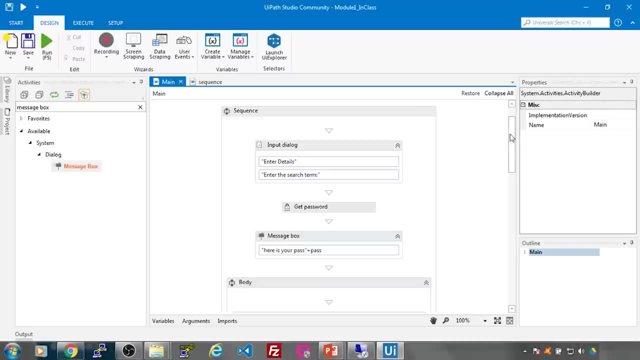 from where what is happening, and then this would easily, you know, help you to debug and handle your errors. Welcome to this session on UiPath orchestrator. So I have created this particular program which which does scraping, which which basically involves extracting information from a particular 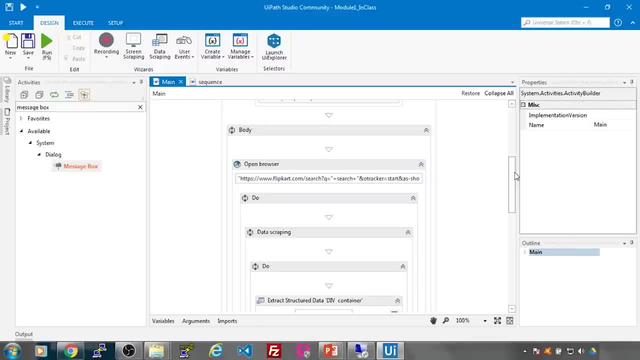 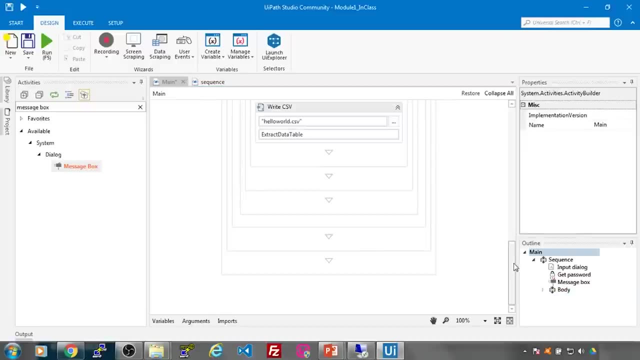 e-commerce website and storing it Inside an excel file. All right, So let's see how this goes, how this is actually happening. All right, So let me edit some part of it and let's see how it happens. All right, so I'll hit run. 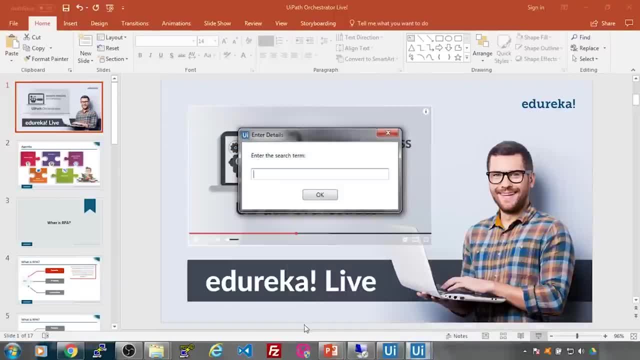 And you know it'll ask me for the search term. Now what? what is the product that I want to search on the e-commerce website? Say, I want to search for a blackberry. All right, I'll hit and I'll enter blackberry. 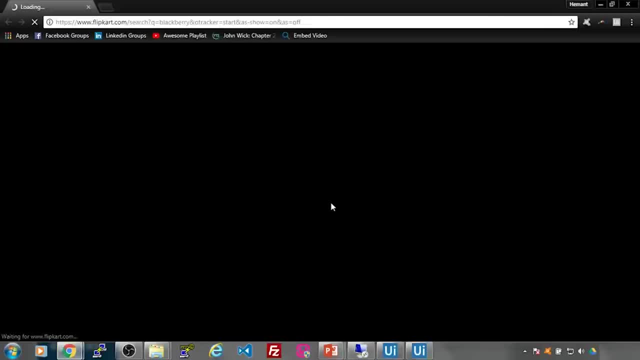 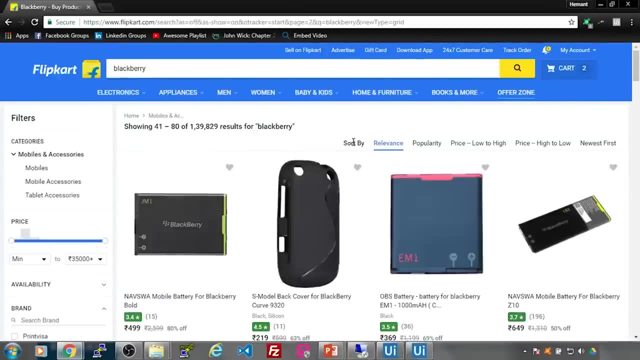 I'll click on Okay And it will go on and it will now open the e-commerce website. It has searched for blackberry over there Right, and now it will go over there and search for each and every product on that particular website. 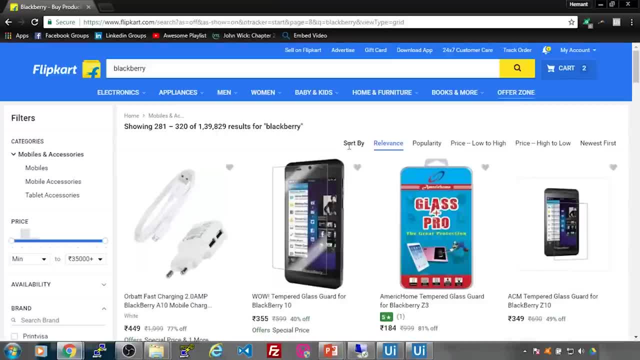 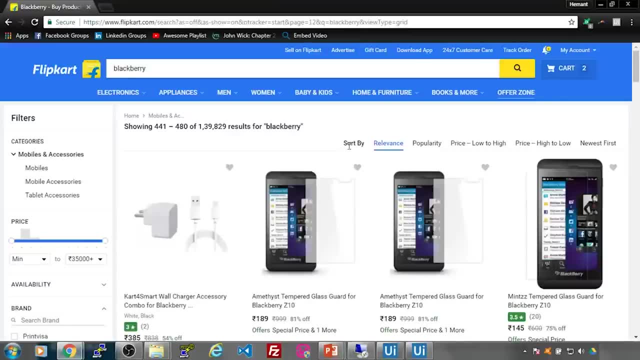 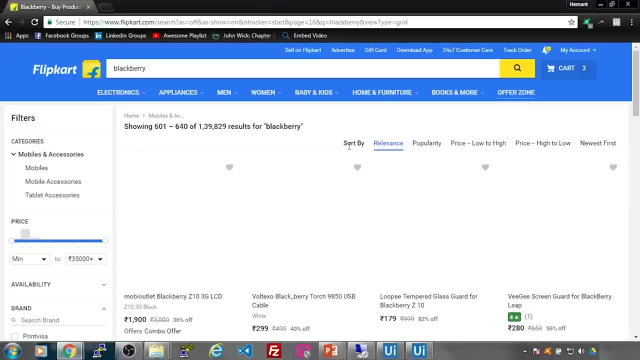 Once it had got that product, it will store the information inside an excel file and that is what I'll be getting. All right, So let's see how it ends. All right, so I can see there are now around 1 lakh results for this. 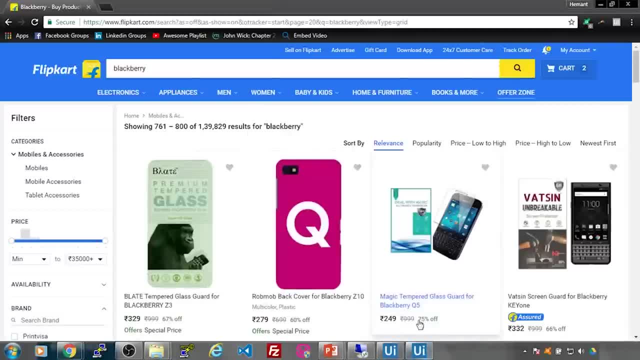 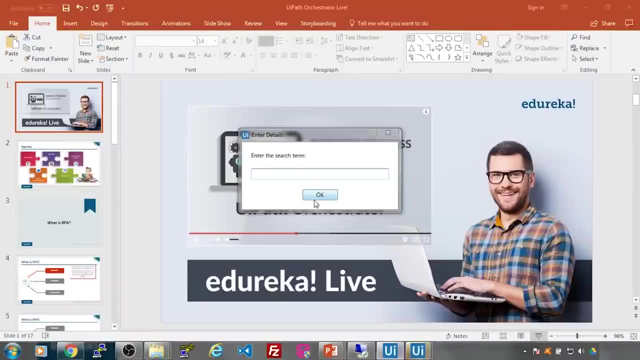 Let me try some other search term, because this will take a lot of time. So let me close this particular automation. Let us run this program again with this different search term, All right? so let's enter the search form search term as say iPhone. 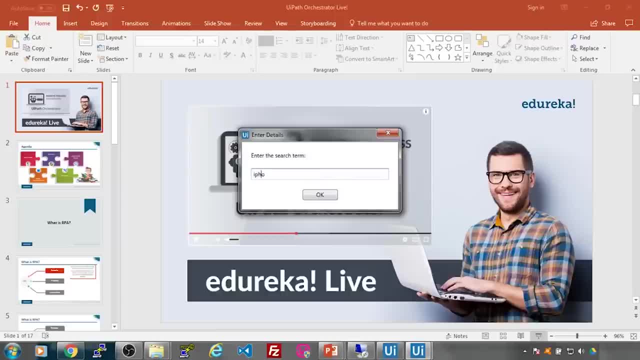 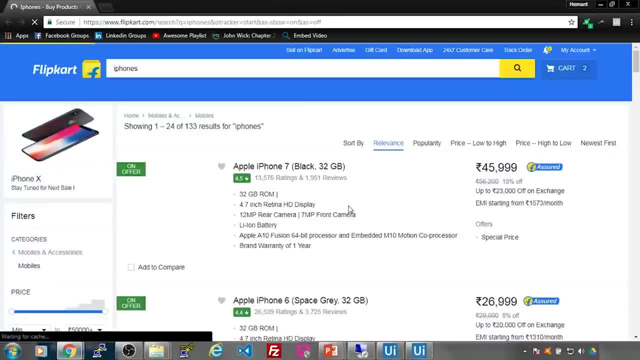 Let's search for iPhone. I hope there are not more iPhones Then blackberry, So all right, let's see How this is running. All right, so there are only 133 results, which is a good thing for me. 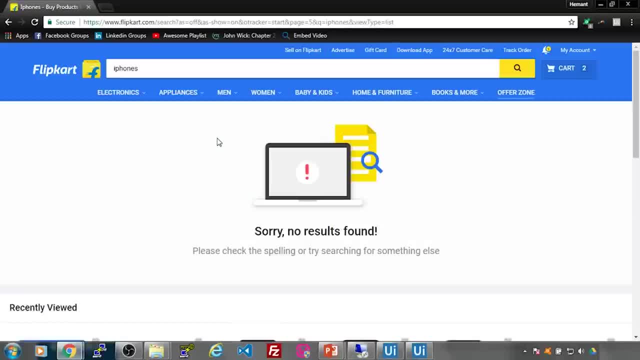 So now it's running the automation and once it reaches the end page of the of the of the search, it will recognize this page and say: okay, my search has ended. Now it will take all the results which has just scraped from the website. 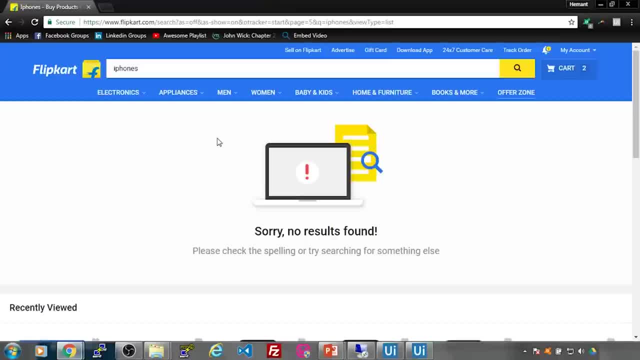 and now store it inside An Excel file. Now imagine, guys, if you were to do this manually. if you were to do this manually, how would you do it? So for doing this manually, guys, you know you will go to each page. 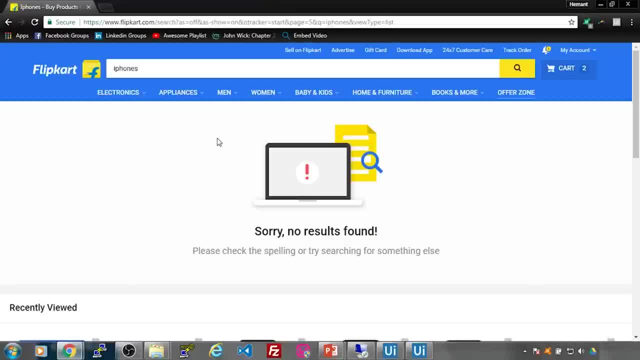 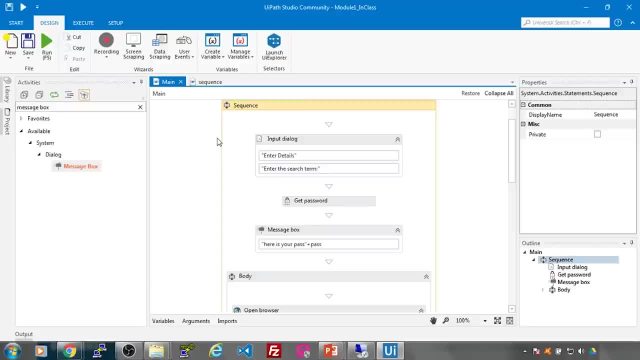 You will copy the name, You'll copy the price and you will do that for each and every product which is there on this e-commerce website. right, And doing that will take a lot of time. right, And we don't, and we have. we guys are very short of time, right? 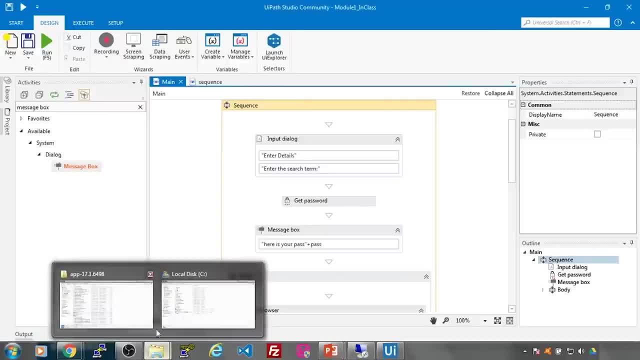 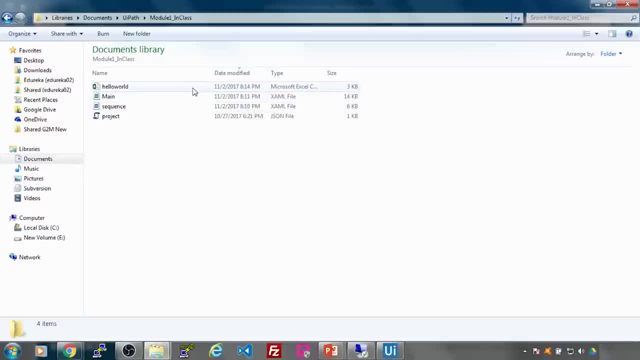 It took around, I guess, a minute to actually get everything. So let's check If we got our CSE file. So this is the CSE file. as you can see, it's 814 right now and it's just been modified. Let's open the CSE file here. 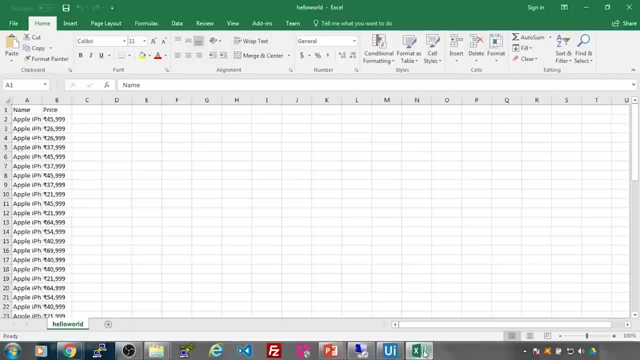 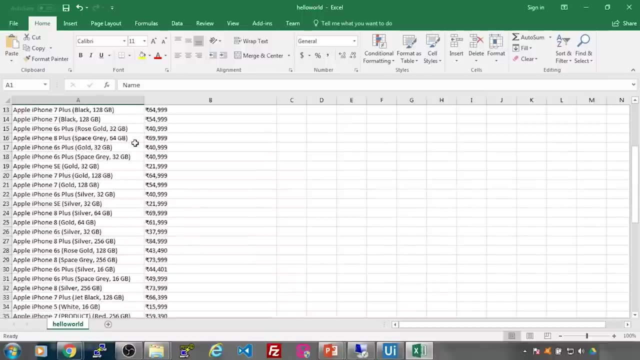 And yes, as you can see, the name and the price prices have been extracted from that particular website and now I have a list of iPhones with their prices. right? So this is the kind of automation that you can create in your iPad, Right? So this is the kind of automation that you can create in your iPad. 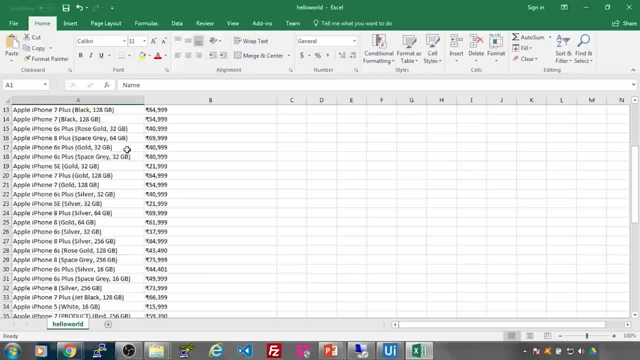 And I think it only took me around 15 minutes to create this automation. and don't worry, guys, I'll be teaching you guys how to create this automation, maybe in some other session, right? But today, since it's an introductory session and it should be about the 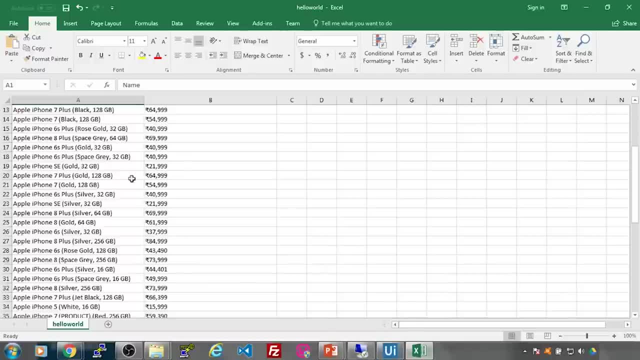 UiPath orchestrator. I'll teach you how you can, you know, execute this particular project on some other client machine without even downloading this project on the client machine. right? And for that, what I've done is I've created an AWS server. 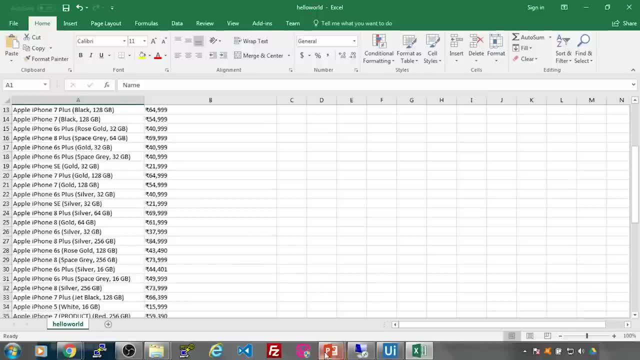 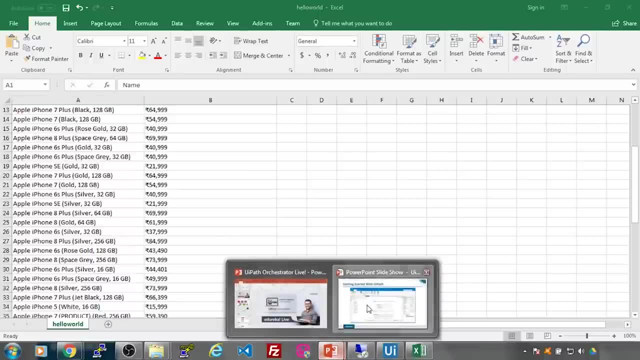 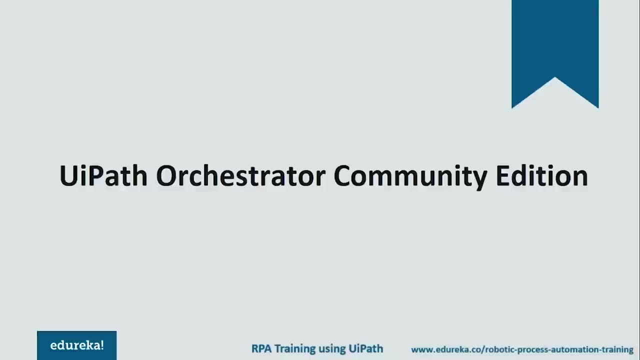 And I've installed UiPath on it. Now what I'll be doing is I'll be running the command from this particular machine to my UiPath orchestrator and my program will run then on the AWS machine. All right, so this is our agenda for UiPath orchestrator. 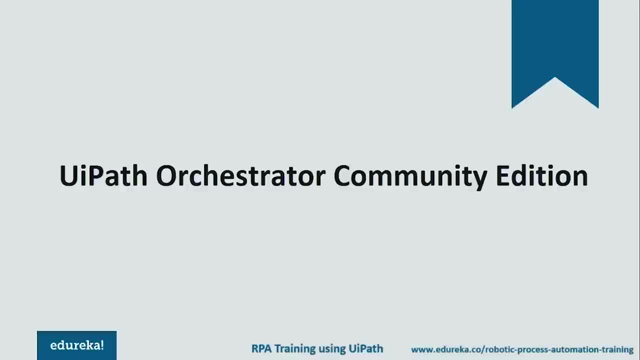 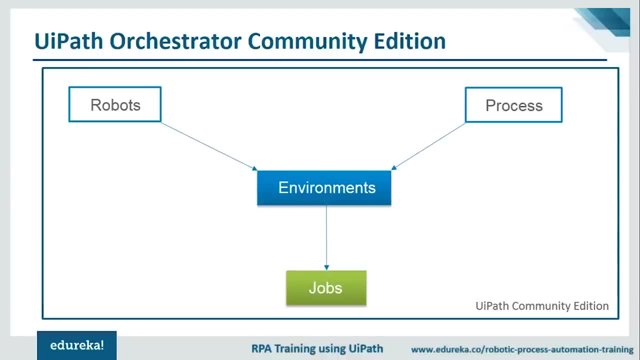 But before that, let's understand what UiPath orchestrator actually is. All right, so UiPath orchestrator typically has this kind of process, which is designed around it. So first, inside the orchestrator, you have to define robots. So what are robots? 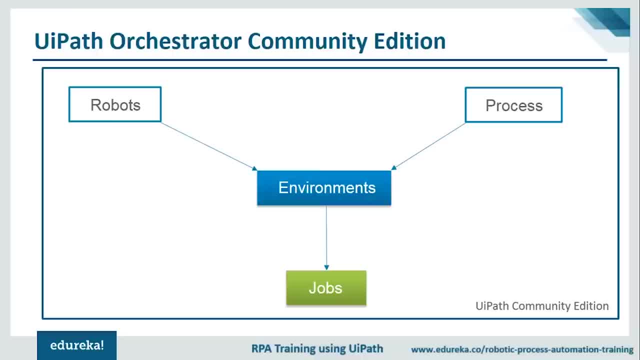 Robots are nothing but the part of your automation which will be executing everything. For example, in the automation that I just showed you, there was a part of the program which was scraping everything which was clicking on next right And then in the end it saved everything in the excel file and then ended. 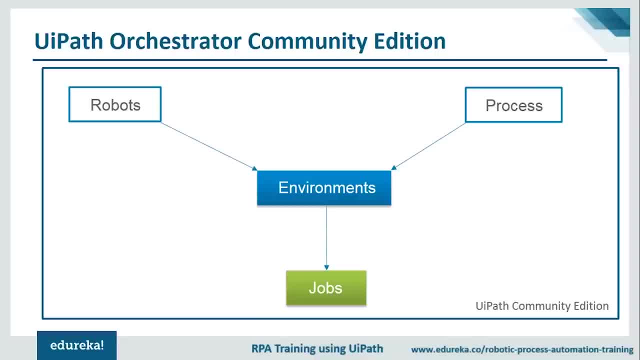 the automation. All right, so that entity is the robot, That entity is known as a robot. Now I have to define inside the orchestrator, where my robot actually is, which machine it is running on. So I've defined all of that and I hence create a robot. 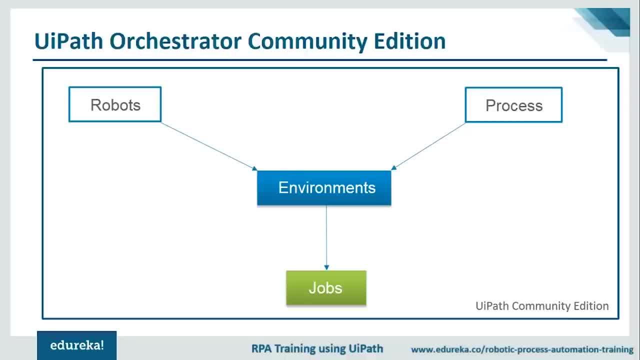 So, once a robot is defined and your orchestrator is connected to your machine, the next thing that you have to do is create an environment. Now, what is an environment? An environment is basically a playground where you have put your robots. Now, the next thing that you'll be doing is inside that environment. you'll be 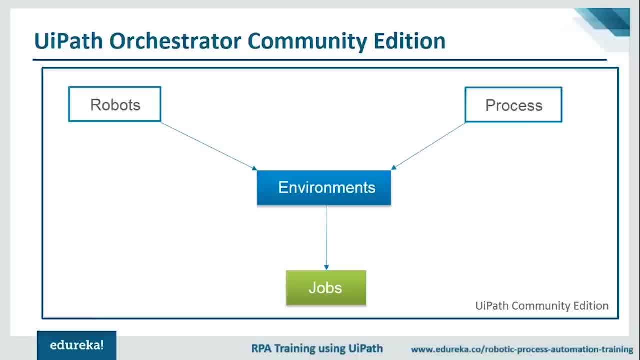 putting the project that you want to run all right. So that project in UiPath Orchestrator is known as a process. So you'll be putting the process or you'll be putting that project inside that environment and then the robot is able to see that project right. 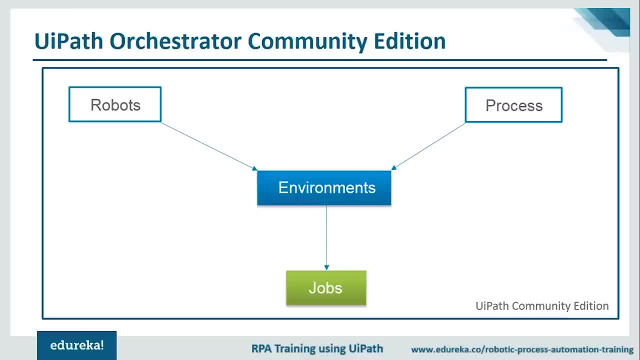 And it is inside the environment. and then you go to jobs, which is the third part of your UiPath environment or the UiPath user interface, and inside jobs you just try to run the project And define which robot should execute that project. Now, the robots are nothing but machines. 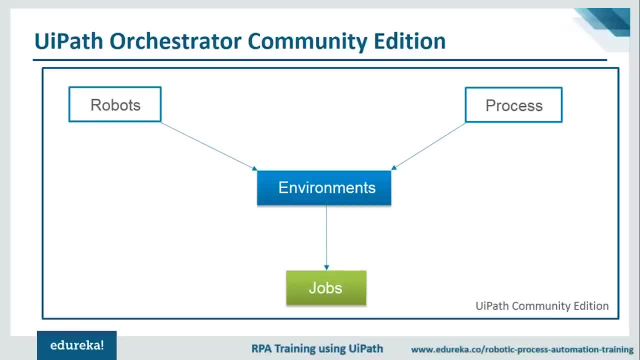 They are different client machines that you have defined in UiPath Orchestrator And whatever machine you specify, it will run on that particular machine, the project that you have specified or you have uploaded inside your environment. All right, So this is basically the whole story behind UiPath Orchestrator. 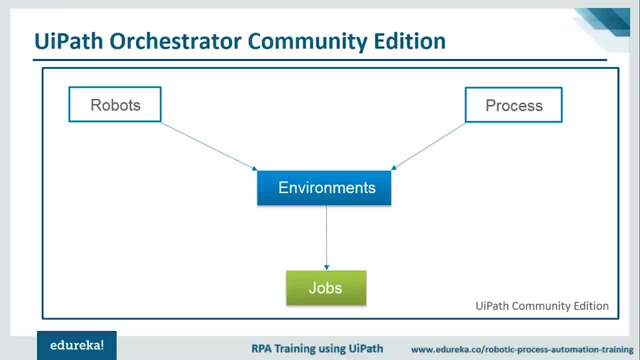 And don't worry if you don't understand anything what I've just told, the story that I've just told. We'll be doing that in demo And I'll take you from each and every step for creating your environment. you're creating your robots and hence executing your jobs inside UiPath Orchestrator. 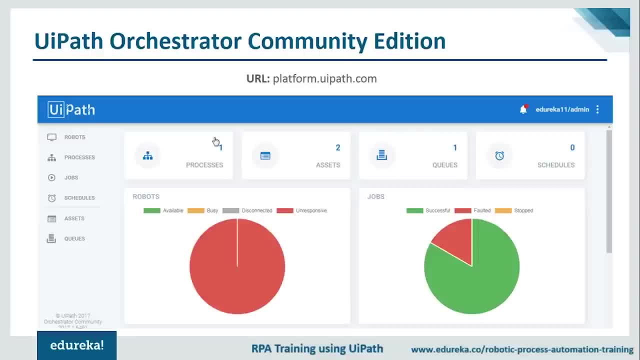 All right, Now let's move ahead, guys. So this is the Orchestrator page. This is where your Orchestrator is actually located, So you have to go to this URL, which is platformuipathcom. Once you have reached this URL, you will have to register yourself on the Orchestrator. 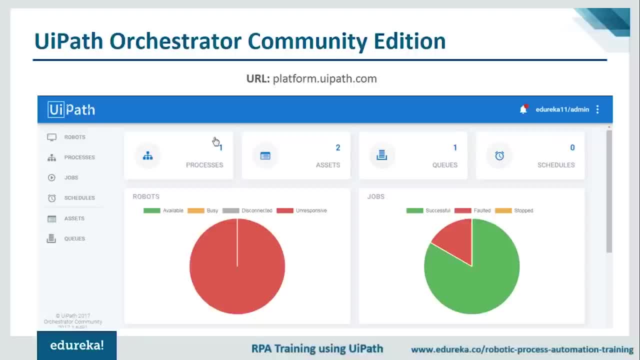 So it is a very simple, straightforward process. You enter your email ID, your password and the relevant details and you just click create. And once you click create, you will be prompted with this screen. This is basically the dashboard of your UiPath Studio. 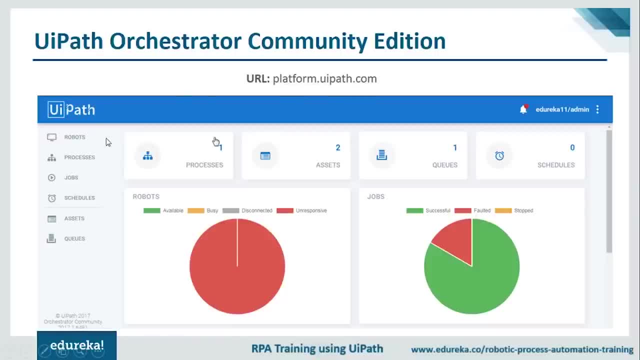 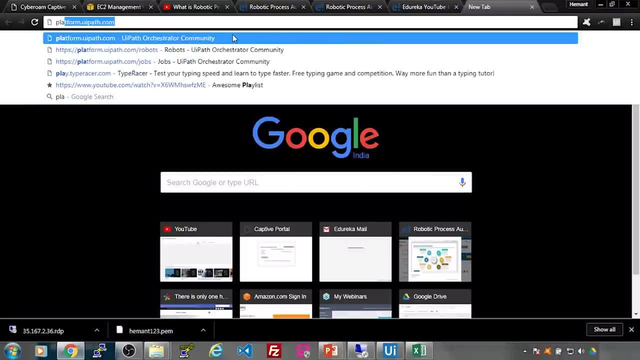 All right, So let me quickly show you the user interface for UiPath Orchestrator inside my browser. So give me a second. All right, So we'll go to platformuipathcom. I'll hit enter And, guys, this is the user interface for your UiPath Orchestrator. 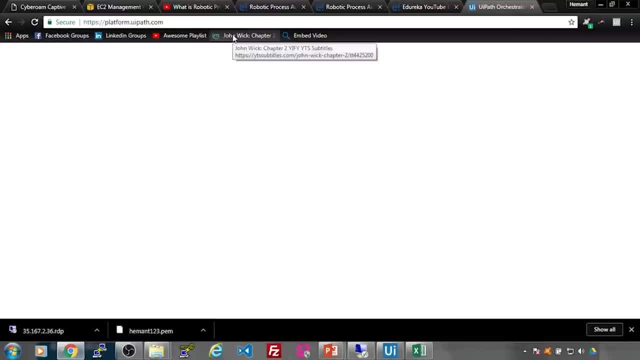 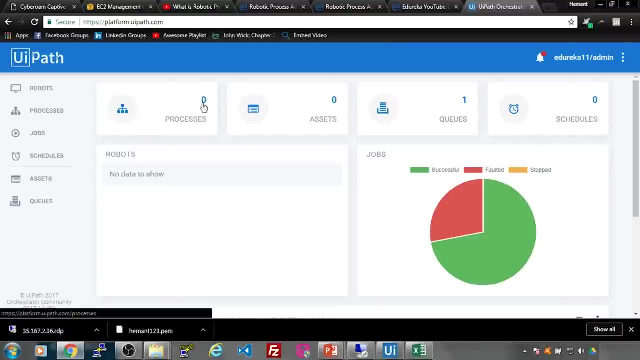 Right Now. you have robots here, You have processors, You have jobs, You have schedules, assets, queues. What are these? I'll be explaining in a moment. All right, So the first thing, like I said, if you would refer to the diagram is, you know, creating. 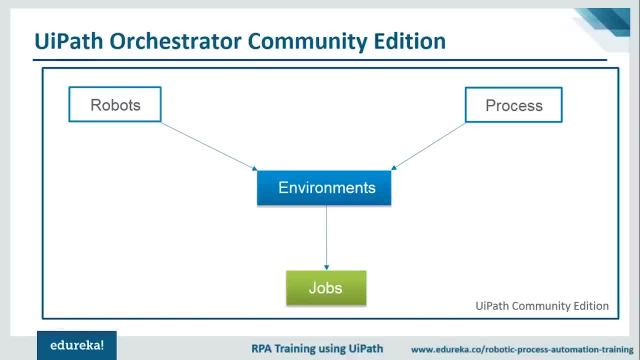 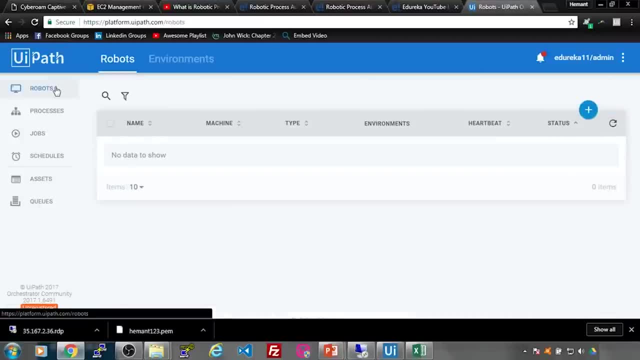 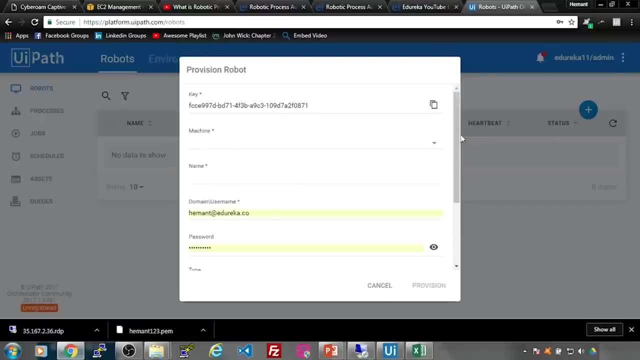 a robot, All right. So let's create a robot first. So for creating a robot, you will go to the robot tab by clicking over here And you will be clicking on the add icon. Once you click on the add icon, this is the screen that you get prompted with. 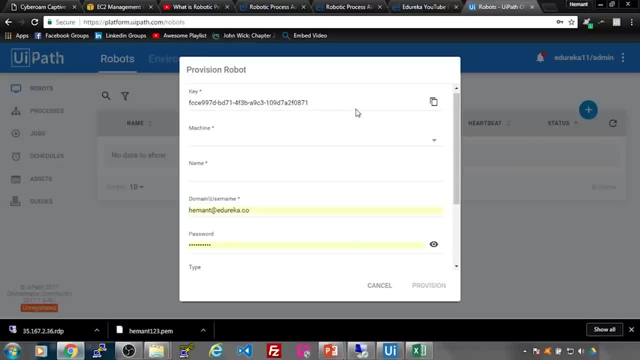 This is the key that you have to copy and paste on your machine so that your UiPath Orchestrator can recognize. Okay, So this is the machine I have to connect to. All right, Once you connect to your UiPath Orchestrator. 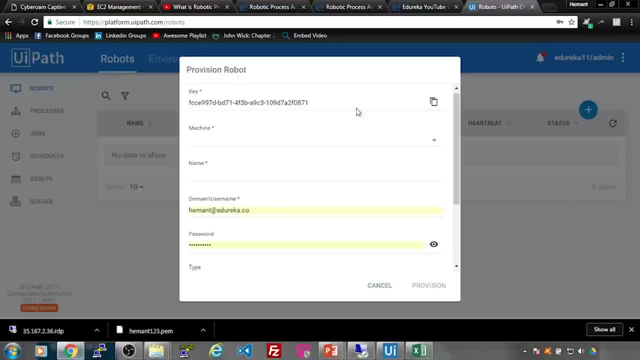 Your robot, that is, on your machine. you have to specify the machine name over here, So machine name. You can get your machine name basically by going into start computer, Right click over there Properties, And you know you'll have the machine name over there. 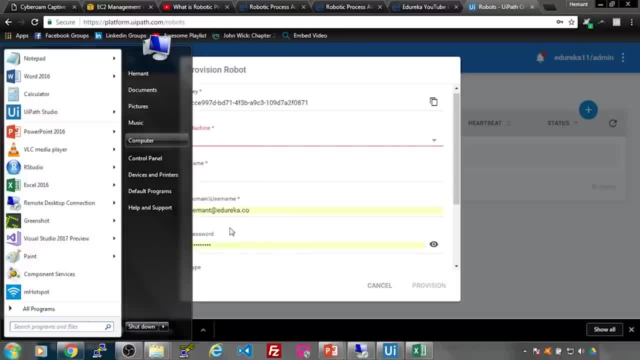 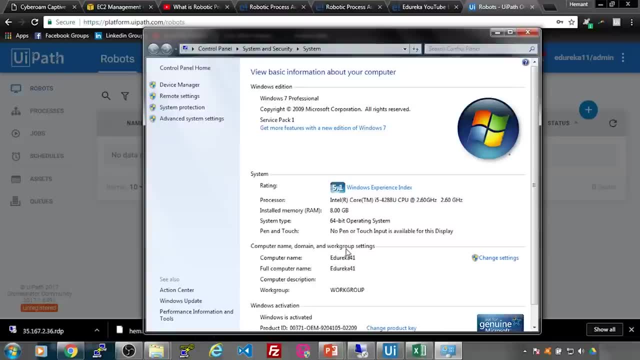 So let me quickly show you the machine name from my computer. So if I click on properties, this is the machine name. for me, The computer name is the machine name, which is Edureka41.. All right, So I'll be entering that over here. 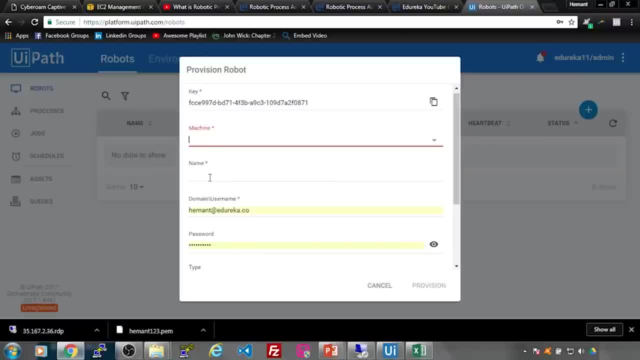 And then you know, If you want to name your robot- something you have to enter the name of your robot- Then the domain. So domain basically means the account name that you have for your computer. For example, my domain name would be Hemant. 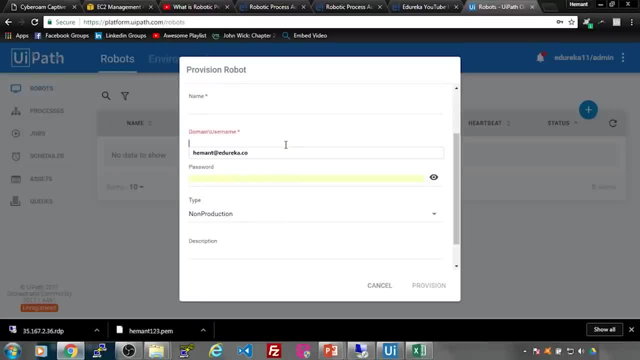 Right For you. it would be the username that you have used for your Windows machine. After that you have to enter the password over here for your machine and then click on provision. All right, So let us do that for my machine first. 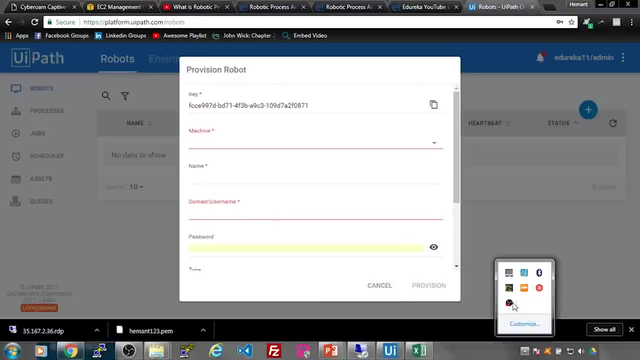 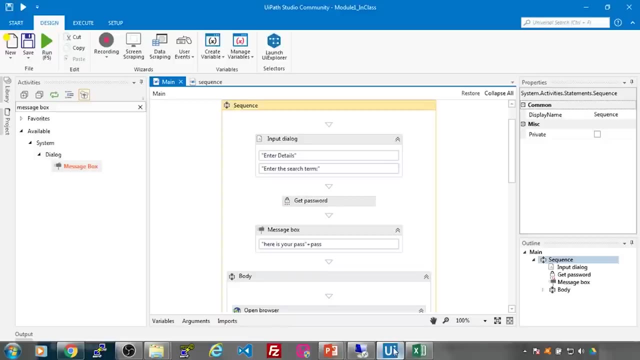 So let me quickly show you how you can launch a machine. You can launch the UiPath Studio or the UiRobot on your machine, Right? So by default, guys, your UiRobot service is not running on your computer. If you want the UiRobot service to run on your computer, there's a little something. 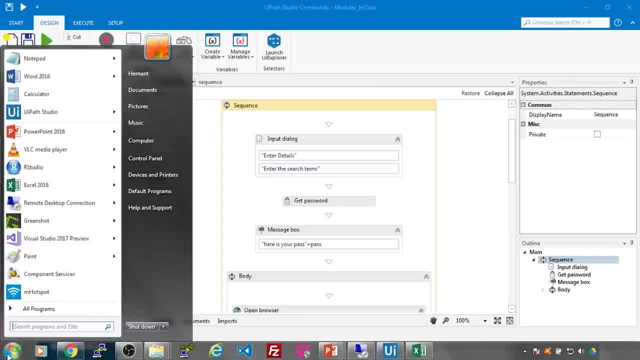 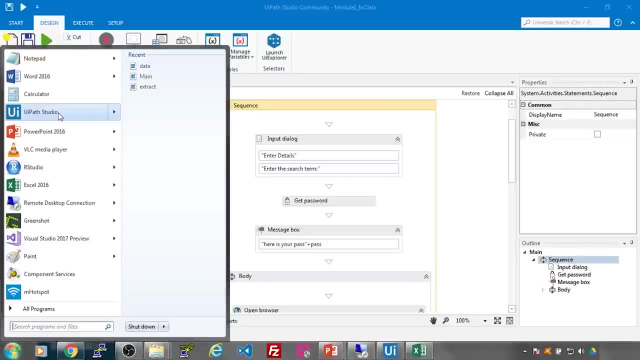 that you have to do extra, which is you will be going to. you know the path where your UiPath Studio EXE is located. For that you know. just go to your UiPath Studio icon, Right click on it And go to properties. 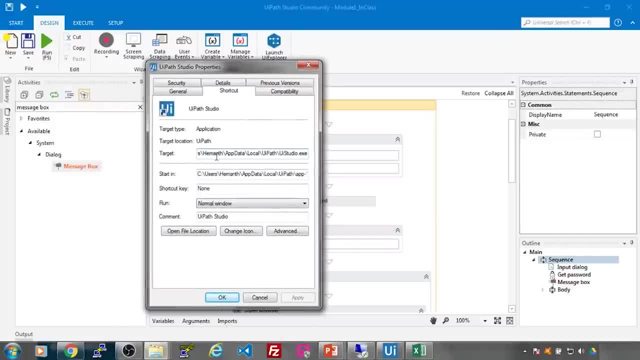 So this is basically the shortcut that you'll have on your desktop Right And you have to take this path and you have to go to this particular path. Right, I'll copy the path. I will go to this particular path. Let's go from here. 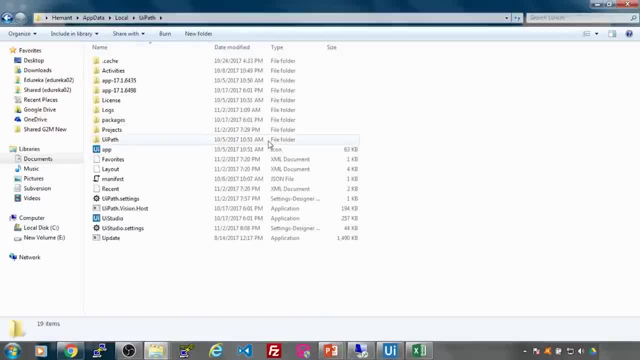 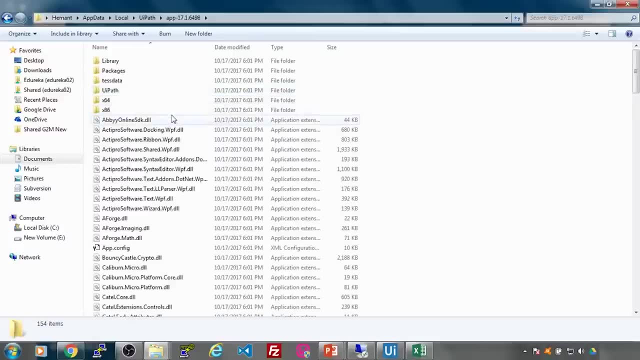 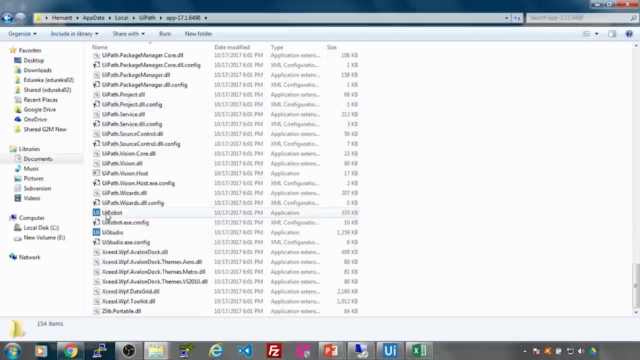 All right, This is the. this is the place where your UiPath has been installed. Now you will be going inside the app folder, So let's go inside the app folder And once you are there inside the app folder, You will scroll down and you will find an icon which is known as UiRobot. 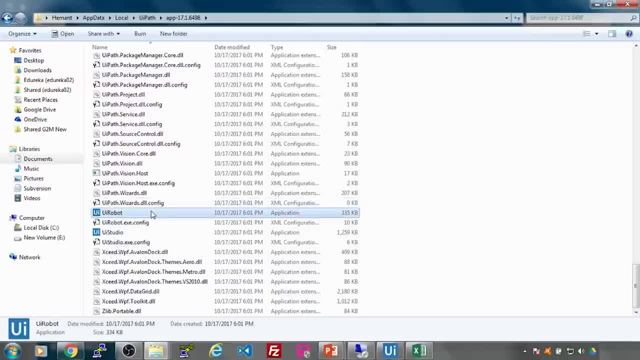 All right, Once you find it, double click on it to run it And it will run as a service in your system tray. All right. So, as you can see, I have a UiPath robot running over here. All right, So now I have to connect this robot to the orchestrator. 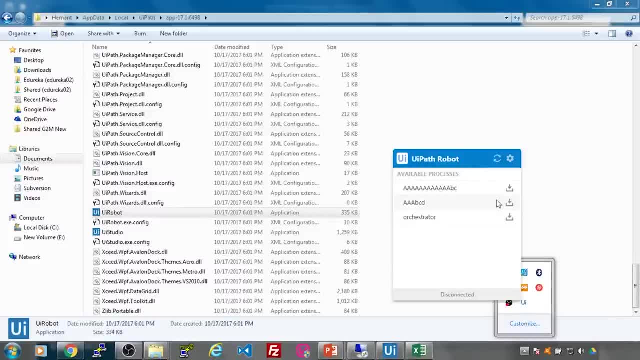 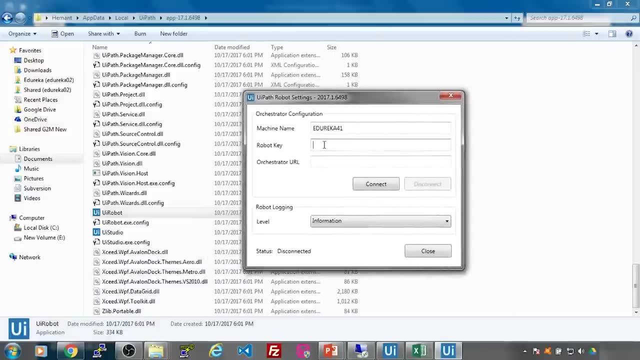 So, for doing that, I will right click on the robot, I will click on settings And I will get this page. So this is the page where you will be entering the robot key that you will be getting from orchestrator, And you have to enter the orchestrator URL over here, which is platformuipathcom. 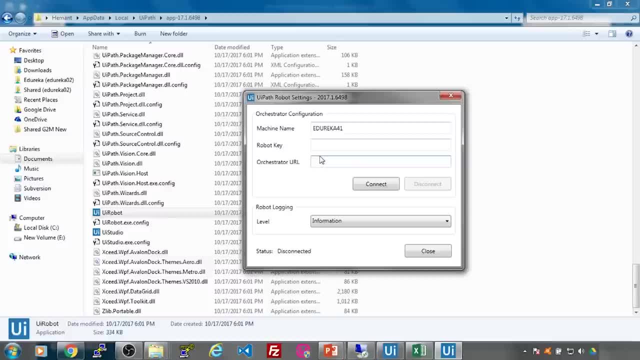 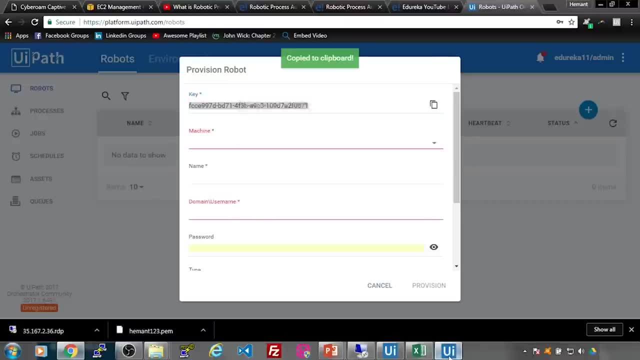 All right, So let's try to connect this robot to my orchestrator. So I will go to my orchestrator. I will copy the key. I will again go to this page. I will paste the key over here. All right, Done. 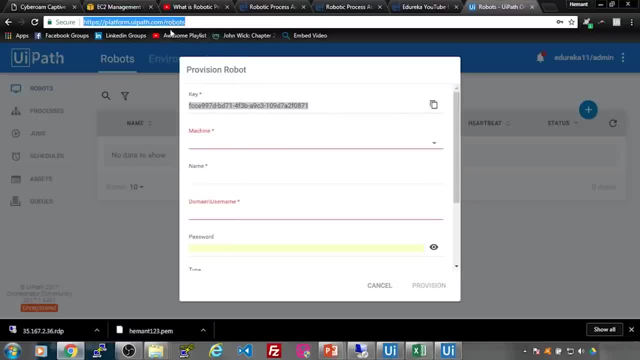 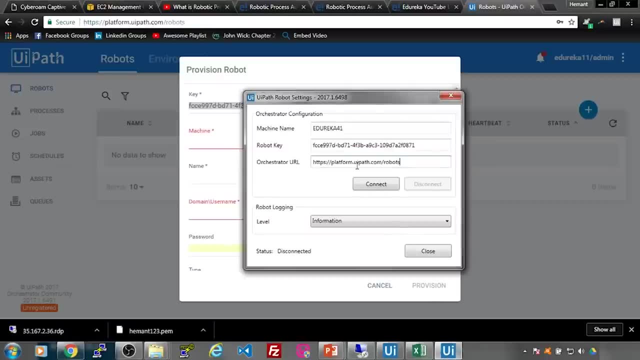 So let's go to orchestrator URL and now over here, I have to specify this particular URL. All right, So let's specify the URL over here. Done Now. robots is not required. All you have to enter is platformuipathcom. 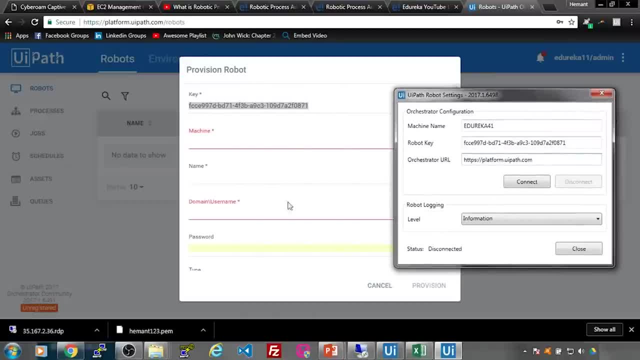 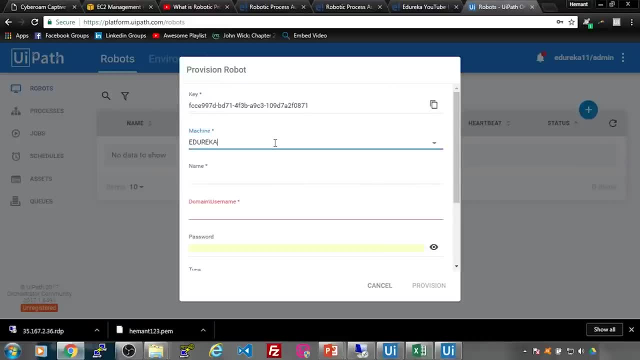 All right. So once you have created your robot over here, you will click on connect. So let's create the robot here. So let's enter edureka41, which is the machine name for me, All right, And the name that I want to give to my robot. let me give it as local system. 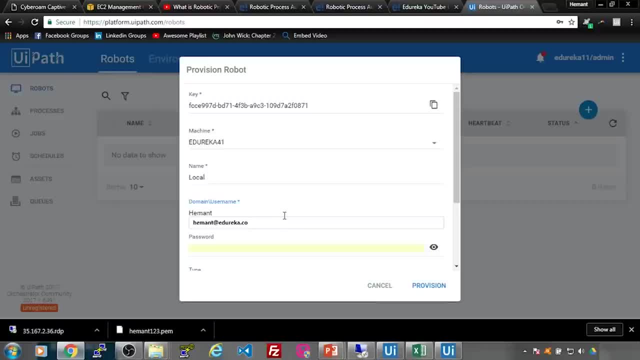 Right, The domain is hemant. That is my account name, And let me give the password now. So my password is this. All right, Now let's go down And that is it. That is all you have to configure for creating a robot. 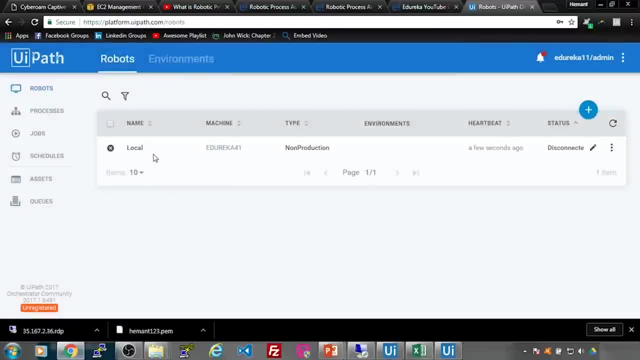 Once I click on provision, it will list my robot over here with the name local that I've given to my robot And the status is right now disconnected, All right, So what I'll do now is I'll go here, I'll click on connect. 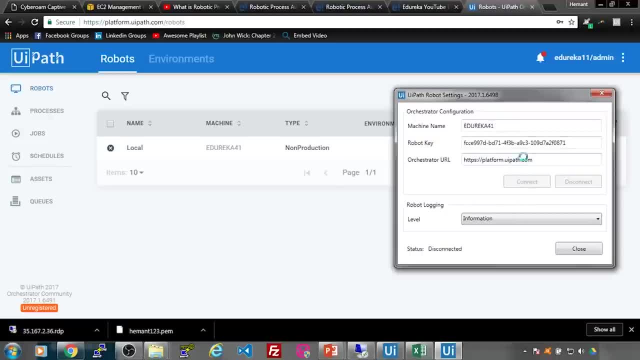 Now, if all the information that you have entered is right, you will be successfully connected to your UiPath Orchestrator. So it takes some time to connect. All right, So it has connected And if you see here, the status is available now. 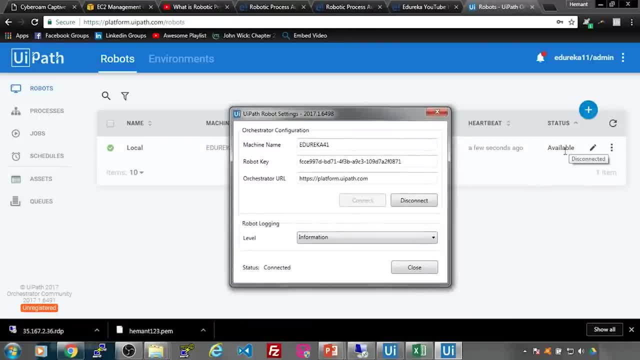 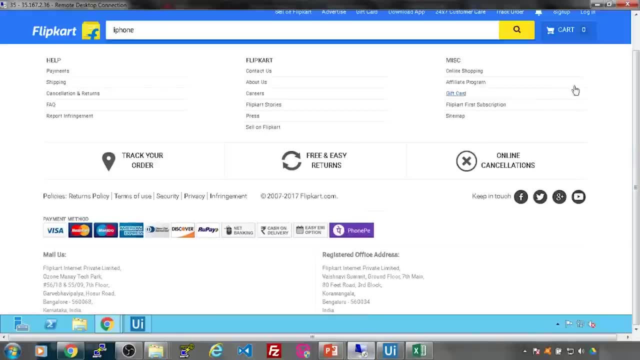 So you have successfully connected your robot to your orchestrator. Now let's connect the AWS services website. All right, So this is my EC2 instance. So this is the EC2 instance that I'll be connecting to Right now. the UiRobot service is running over here. 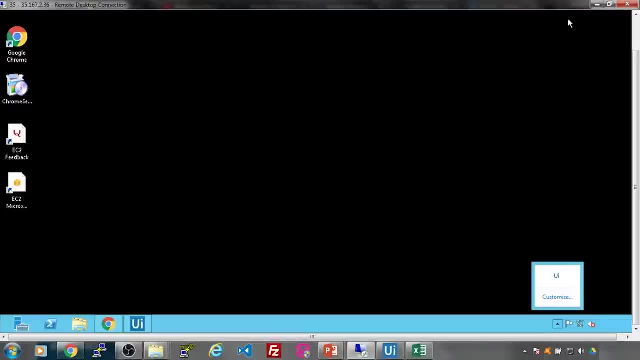 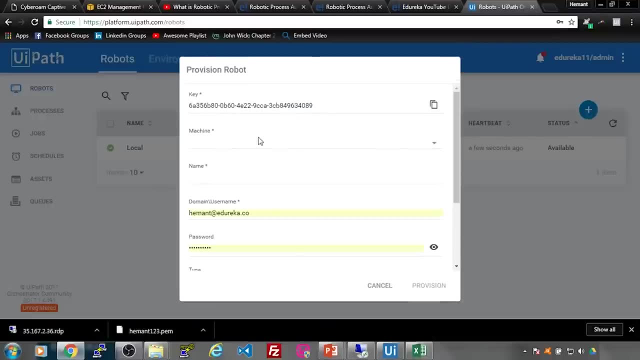 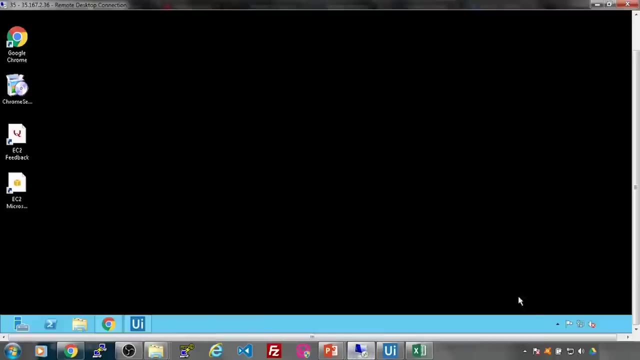 So let's connect this UiRobot to my orchestrator. So I'll click on add icon. I will add the machine name. So I have to get the machine name from there, But I have the key here. So let's copy the key and paste it inside my UiRobot, which is running over here. 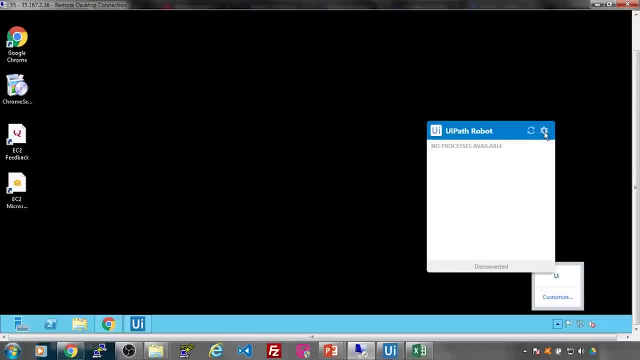 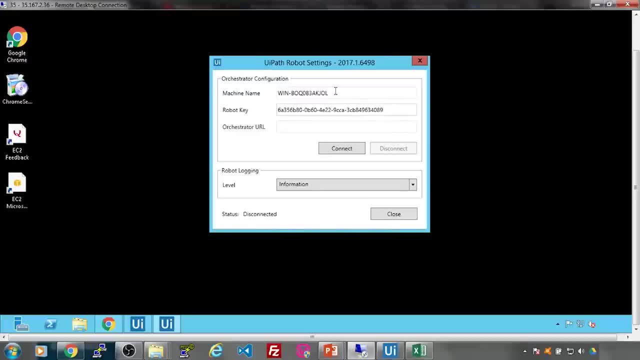 All right, So I have the robot which is running over here. Let's go to settings. All right, This is where I'll be entering the robot key. Now, this is the machine name that I have to copy. So let's copy the machine name. 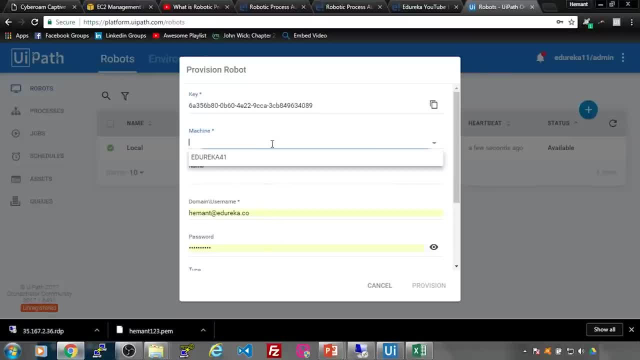 Let's go back to my UiPath Orchestrator. Let's paste the machine name over here. All right, Done. Now what name do I want my AWS machine to have? So let's give it the name as AWS. What is the domain name for this? 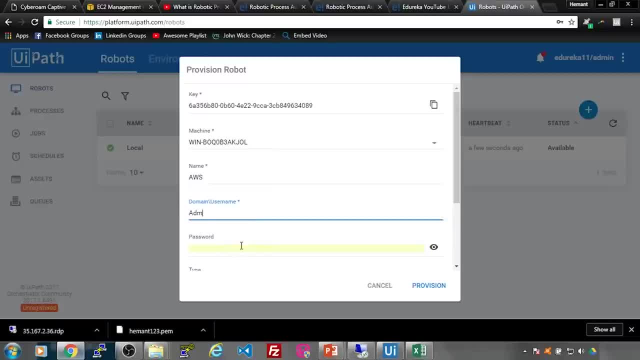 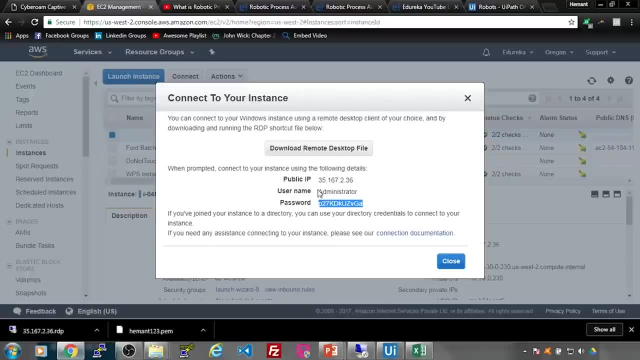 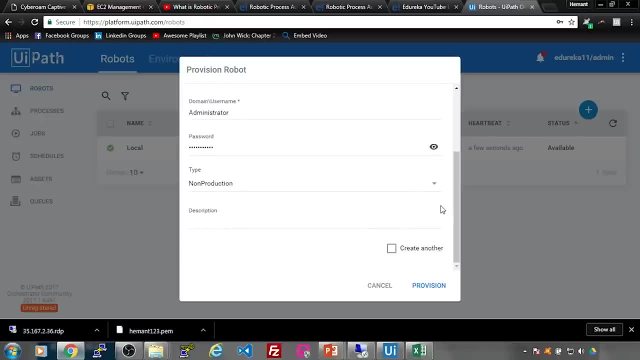 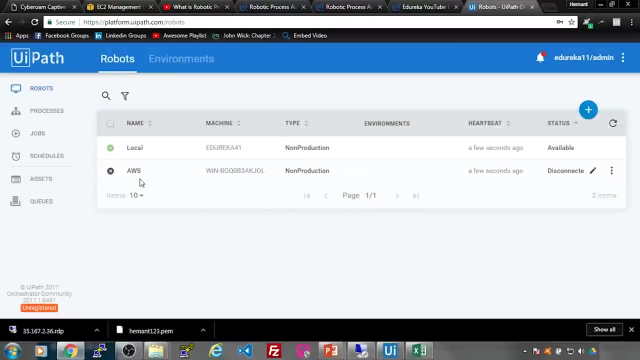 it is administrator, so let me control a and put administrator over here. all right. now i have to give the password, so let me get the password from my aws console. i come back here, i'll put the password, and that's it. now let's click on provision. all right, so my aws robot has also been created. 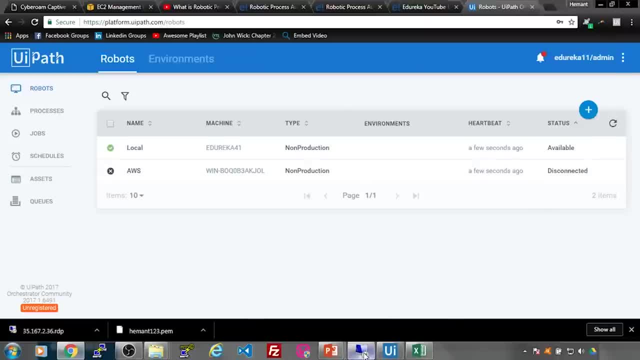 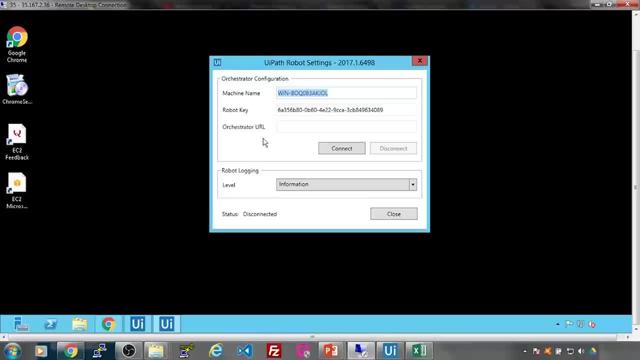 but it is right now in the disconnected stage. so let's create, let's connect our ui parts robot to orchestrators. for that i have to again verify the orchestrator url. so let's copy the orchestrator url from here. which is this: right, let's go back, paste it here, remove the slash from the end and 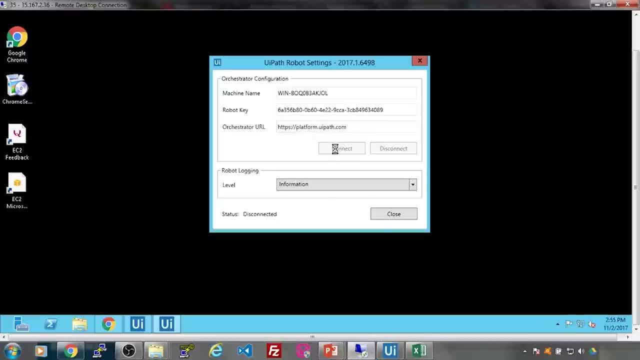 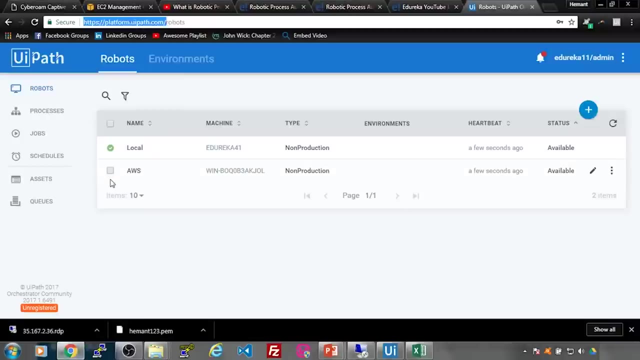 click on connect. all right, so it will again take some like two, three seconds to connect and, as you can see, it says disconnect over here, which basically means my robot has connected. let's verify that in my orchestrator page. all right, so my aws machine now is saying it is available, which is awesome. now i want to, since my robots 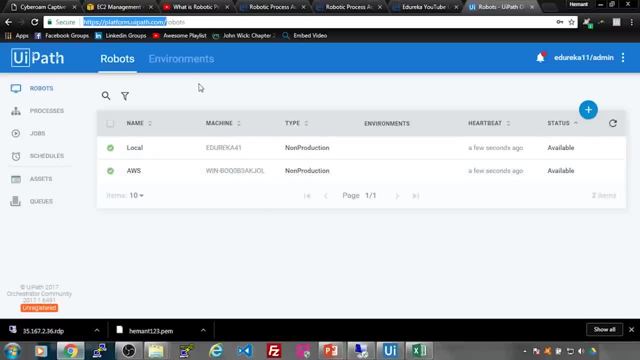 have been deployed. now i don't have an environment right now which i have created, right, so i'll go to environments. so this is an environment that i created earlier. let me quickly delete it so that i can teach you from fresh. all right, so i've deleted the environment. now let's create a new environment and name this. 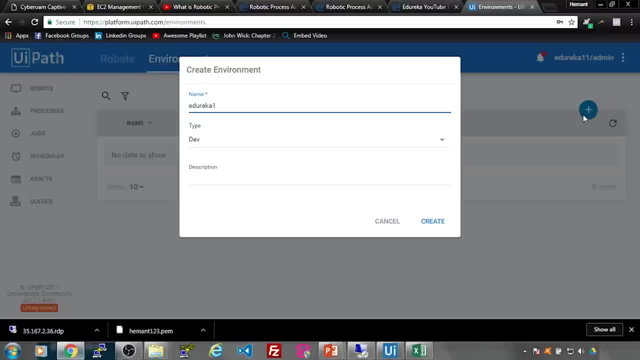 environment, say as edureka one. all right, and let's hit create. so this will create a new environment. now, what robots do i want in this particular environment to be deployed? so let us deploy the aws server and my local machine as well. all right, so with you just have to click on the check box. 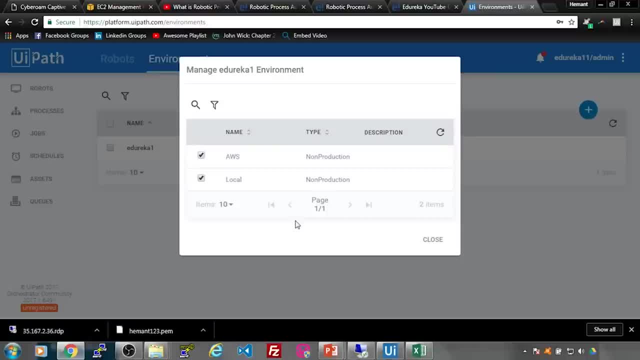 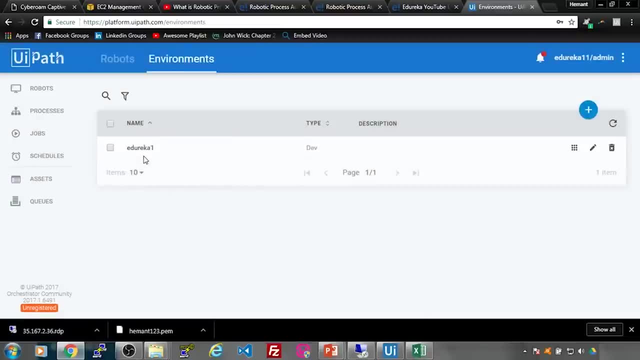 and this will deploy your robot in your robot environment. so let's create a new environment in your machine, in your environment, and you can click on close after that. all right, so your environment now consists of two robots, which have been deployed. now what is left is a project, which 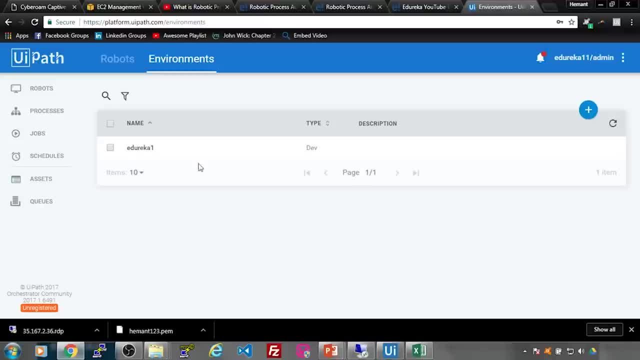 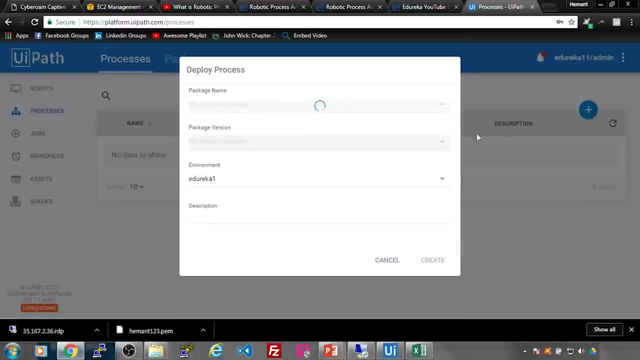 has to be assigned to your environment. for that you will go to processes right and you will click on add. now, once you click on add, this basically points to a common repository which, which uipath community edition or uipath orchestrator community edition, has provided us with all right. so when, whenever you'll 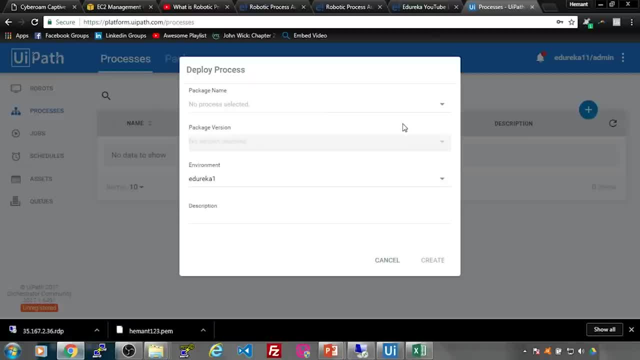 publish your projects to the uipath orchestrator. it will get published inside your uh, this particular depository right, and whenever you upload your projects, you will get your projects listed over here, all right. so this is the list of projects that people have uploaded, or you know? 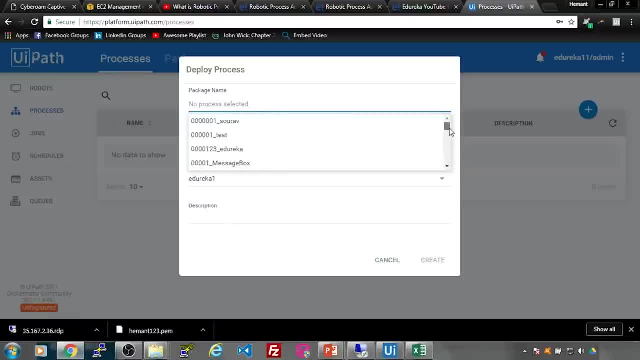 people like you who are trying to use uipath orchestra orchestrator have uploaded right, so these are the pages. now there's a glitch in uipath orchestrator guys- let me point that out- that it can only show a limited number of names over here. all right, so you, when you're naming your project anything, you have to be very 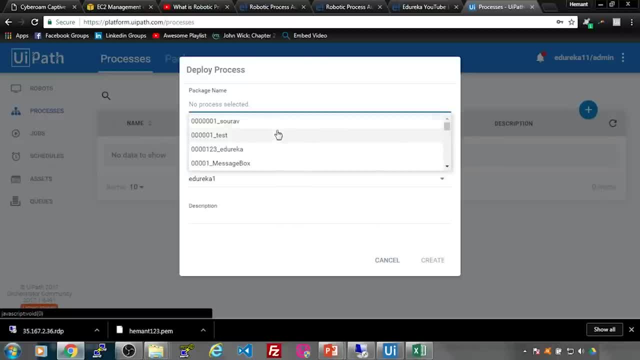 sure that, uh, the naming convention is such such that it get listed over here, all right. so, for example, the sorov guy, he, he made the name as triple zero, triple zero, one underscore sorov, and it got on the top, and maybe that is the reason he'll be able to use it. but if you scroll down, guys, 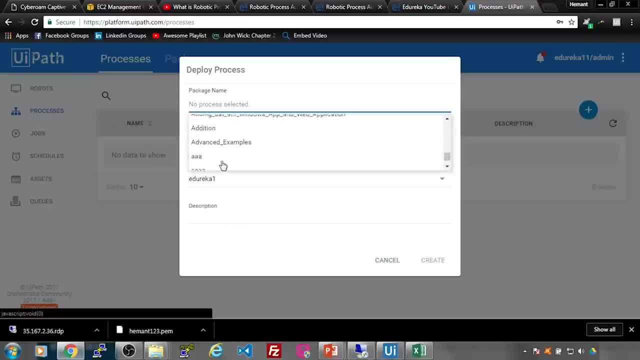 cannot see anything beyond a right. so these are all the projects that people have uploaded. anything beyond is not being reflected, and that that is because, um, you know this, this particular list can only show a few names. so, uh, like i said, you have to give the naming convention very carefully. 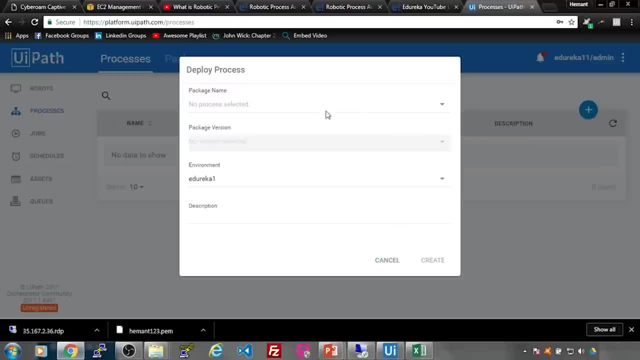 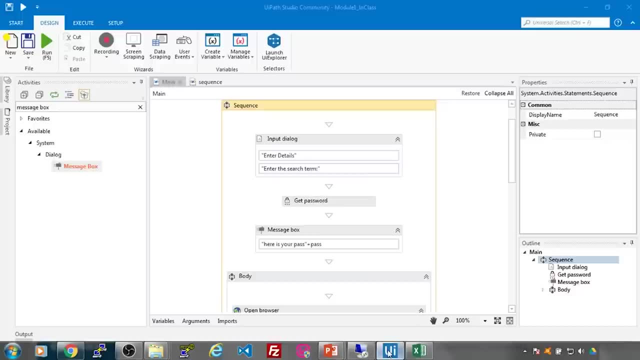 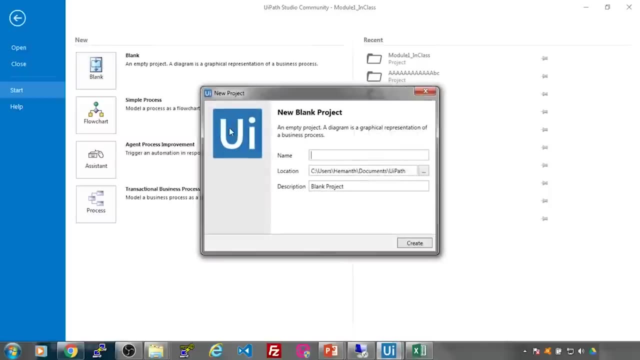 so that it get lit, it gets listed over here. so, before deploying a project, let's create a simple project that we want to upload. all right, for that. let's go to my uipath studio and let's create a new project. uh, let's name it as say: zero, zero, zero, zero, zero, zero and let's give one more zero that. 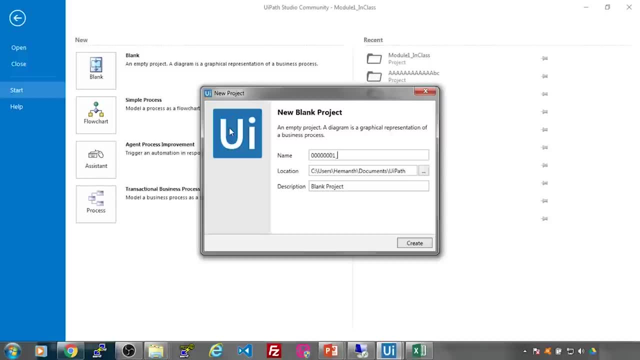 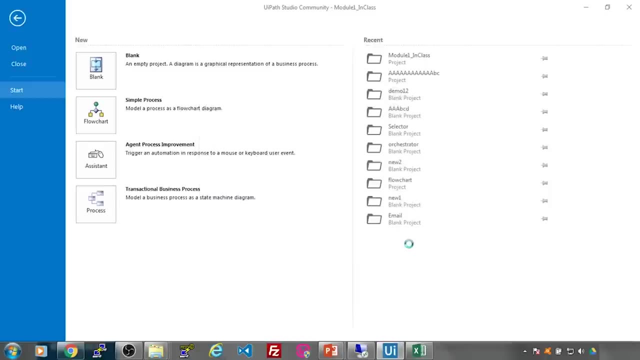 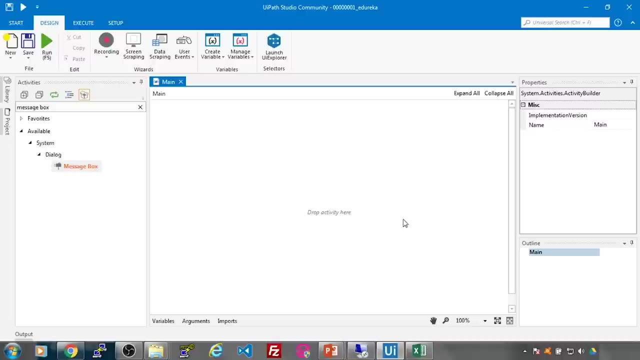 is seven zeros and then one underscore: edureka, all right, so let's give it. give it this name and hit create, all right. so this basically, uh, creates a project folder for me. now i want to publish this project folder to my orchestrator, which i will do once i have created this particular automation right. another cool. 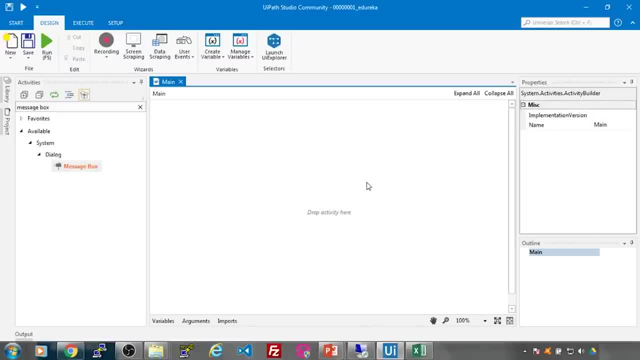 thing that you need to notice in orchestrator guys is that you'll be creating your project only once. you don't have to copy your project on each and every robot that you have deployed inside, deployed inside orchestrator. all right, you will be creating a project once you will. 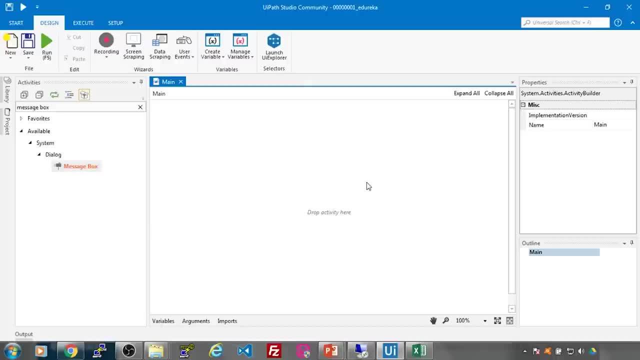 be uploading it onto the repository. and any robot that you want to be and that you want your project to be deployed on, you just select that robot, hit run and it will run on that particular machine without even being downloaded over there. all right, so let me drag and drop something, some some kind of automation, all right, so let's, let's. 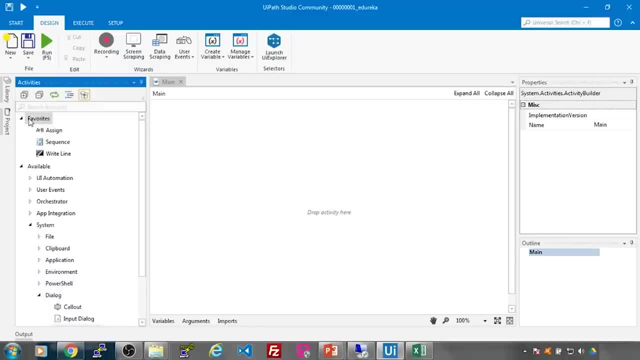 try to run an automation on our aws server. so let's run a very simple automation that i created earlier. let's first drag and drop a sequence. so let me search for a sequence. it's here. let's drag me to drag and drop it here. all right, then let's ask for an input. 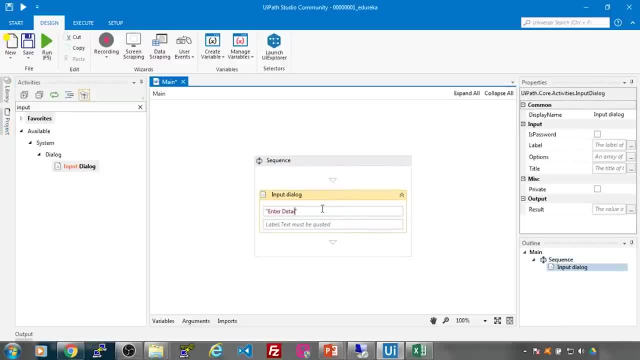 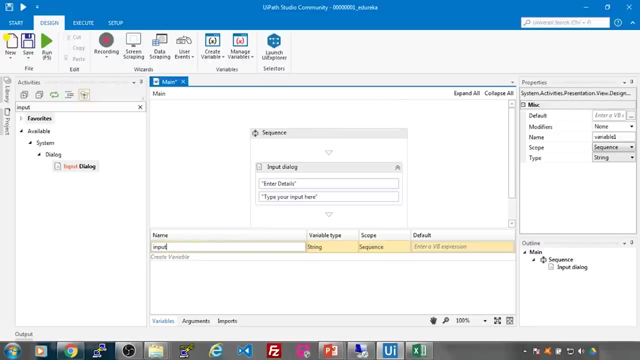 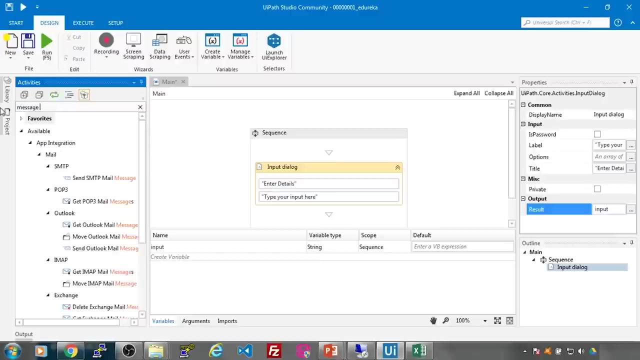 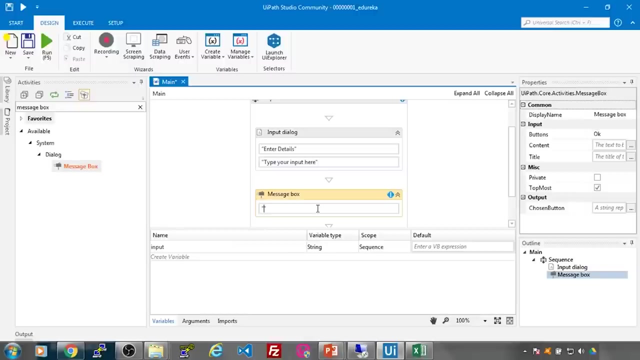 let's enter. let's say enter details and type your input here and let's create a variable for your input. let's give this variable as here, alright. and then let's create a message box. Let's drag and drop it here. let's specify that this is your text, that you entered, alright. 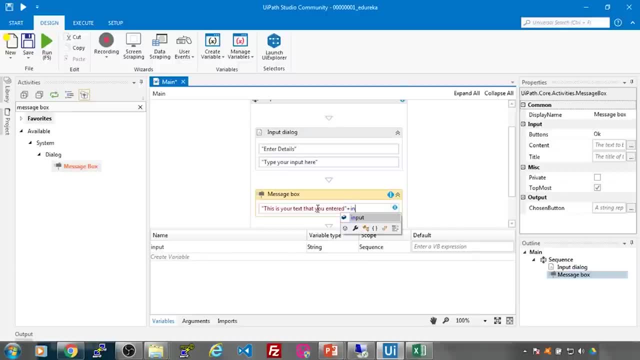 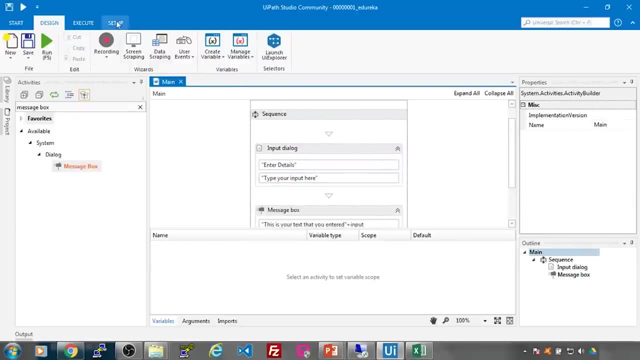 and specify the variable with it, which is input. alright, done, So it's complete. let's save this project and let's now publish it to the orchestrator. So for that, I have to click on publish, and this will basically publish my project to. 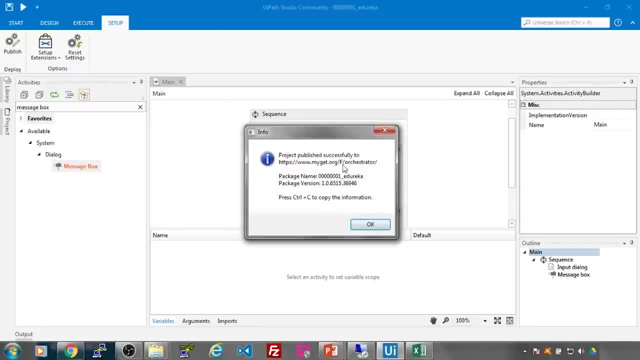 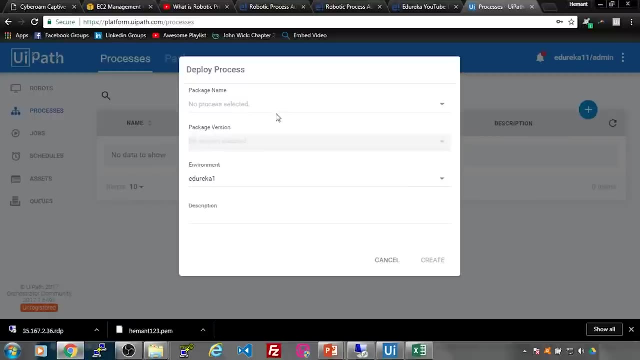 the. this is basically the repository where it's being saved on and this is the package name, that is 0000001, underscore edureka. Alright, so we have successfully did that. let's click on ok. and now let's hope our package gets listed over here. alright, so let's try to add a process. so it's refreshing the list. 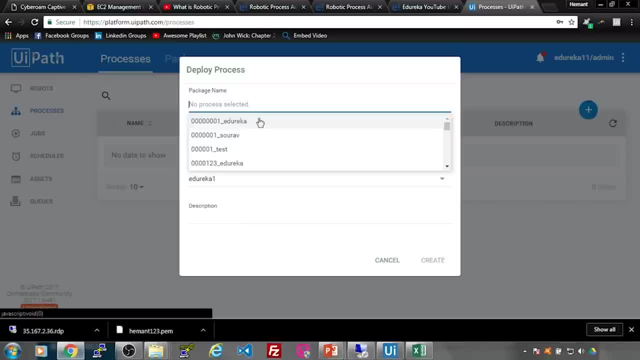 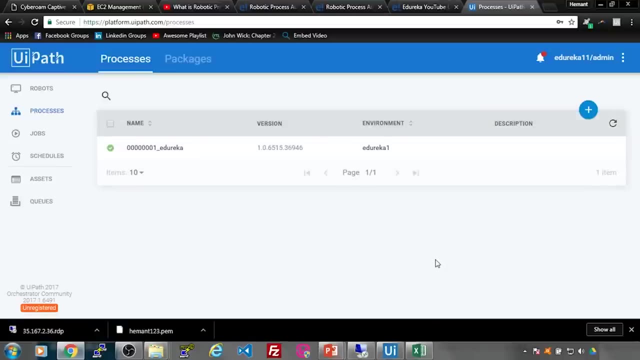 Alright, so the list has been refreshed. so, as you can see, my project is listed over here now, So I'll click on the project. alright, My environment is edureka1, so let's hit on create now. So this will basically import the project that is there on the repository to your environment. 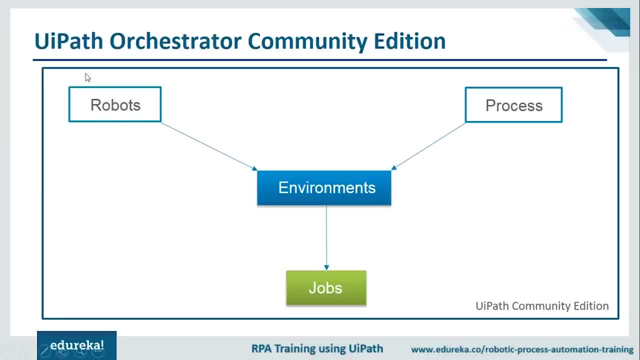 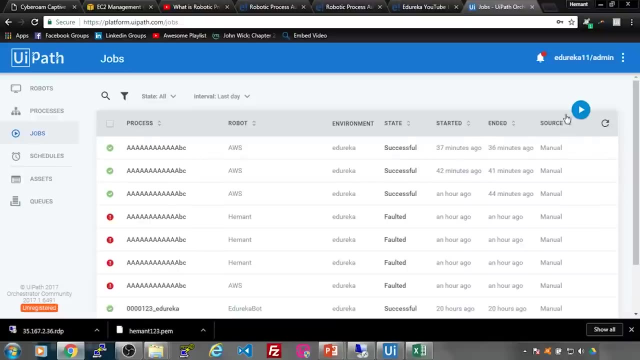 alright. So this is what I was telling you. so now your robot and your process is inside the same environment. Now the next step for you would be to execute a job. so let's do that. Let's go again to our UiPath orchestrator and go to jobs. alright. 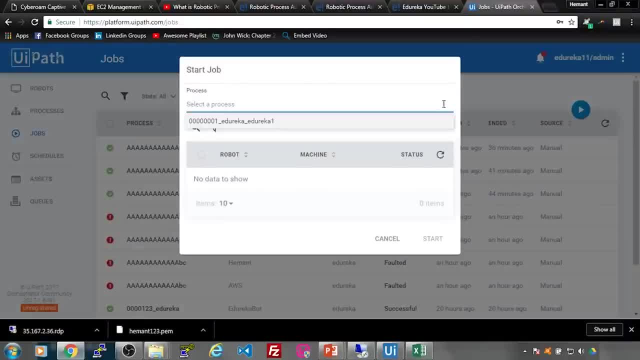 Let's try to execute a job. So I have to select. what job do I want to execute? so this is the project that I have deployed. alright, So these are servers where I can execute my job. so let's try to execute it on the AWS. 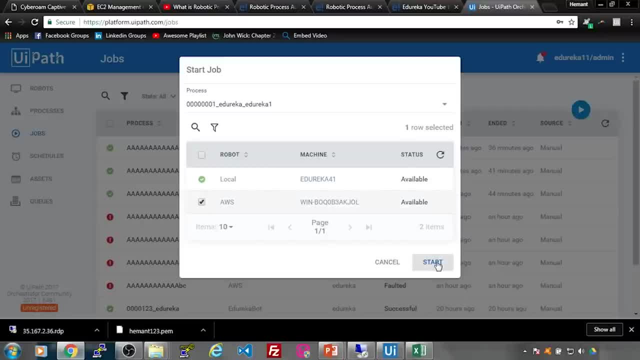 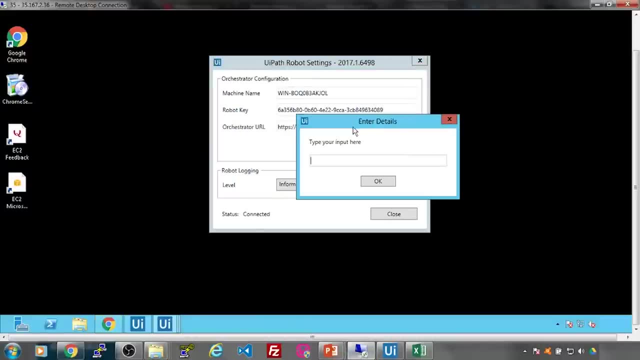 server. So I'll select AWS and I'll click on start. let's see what happens. So if I go to my UiPath orchestrator so, as you can see, it automatically launched the message box over here, alright, It will ask me for my job. 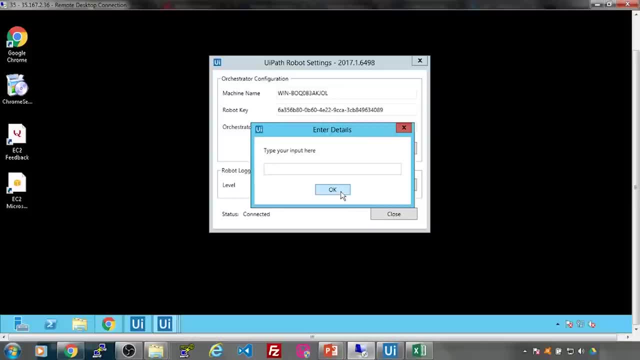 Alright. So for my input, let me specify. the input say: I am on AWS server. alright, Let me click ok and this is your text that you entered: I am on AWS server, alright. So I created my project on UiPath studio, which is on a local machine. 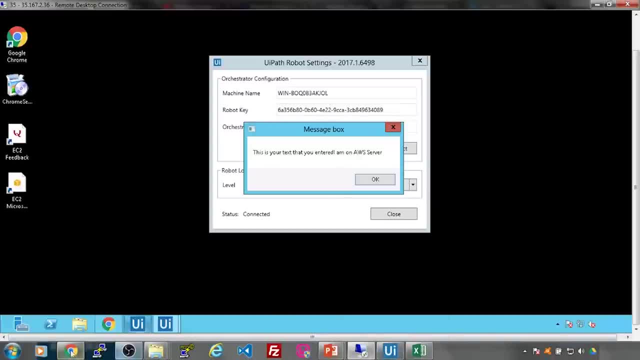 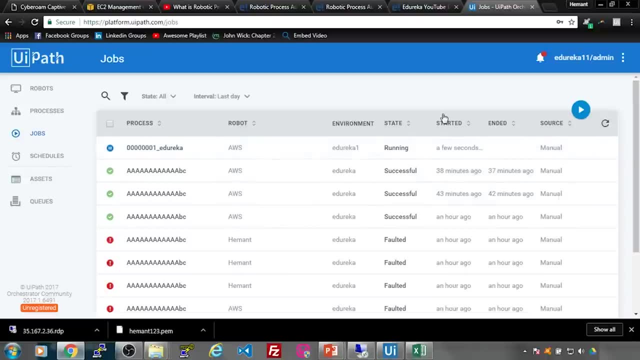 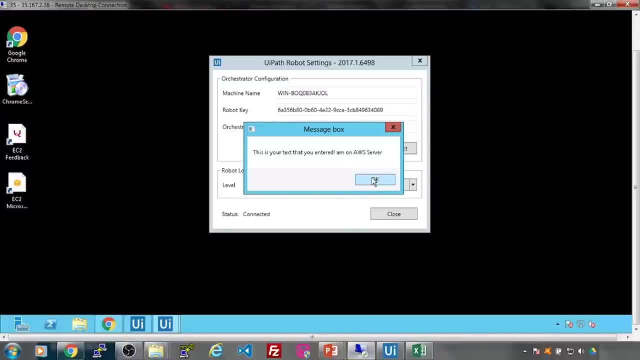 I uploaded it on the repository and then I deployed that particular project from my machine, from my orchestrator, to over there, and you know, it just gets executed automatically. So this is what I wanted to do. So congratulations on your first project on orchestrator. now let's try to do something. 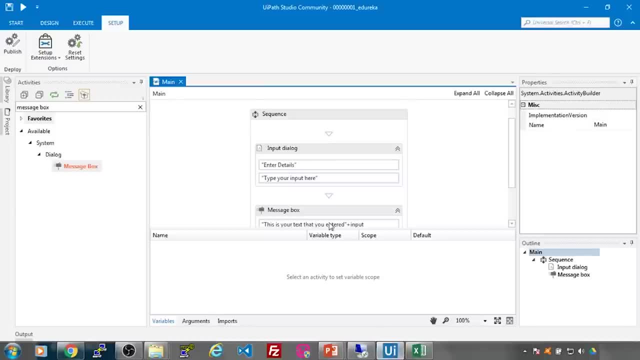 more interesting. Let's try to, you know, create one more project here. Let's try to create a Gmail login, alright, So let's see how we can do that. So for creating a Gmail login, guys, the thing that you have to do is: first, I would want. 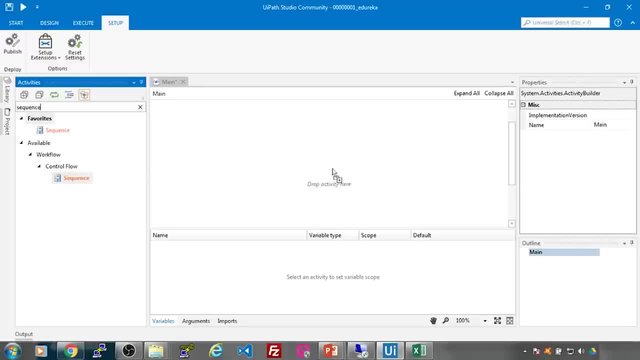 a sequence, Alright, So let's drag and drop the sequence over here. and then I want to open a browser, right? So let me specify the browser over here. Now, what browser do I want? it? do I want my project to open? 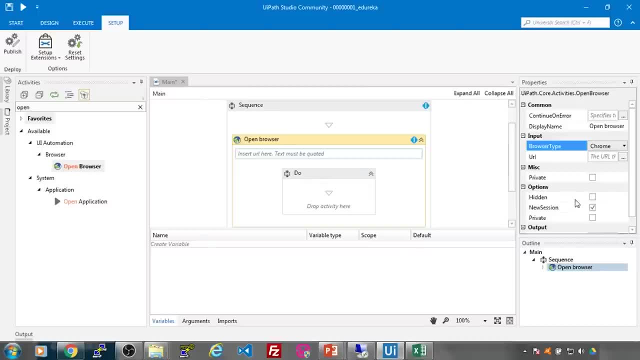 Let's select it as Chrome and let us open it in a private window. alright, And what is the URL that I want to go to? I want to go to gmailcom, So this has to be inside quotes, Alright, Once I'm on gmailcom, I want to click on the enter your email address text. right? 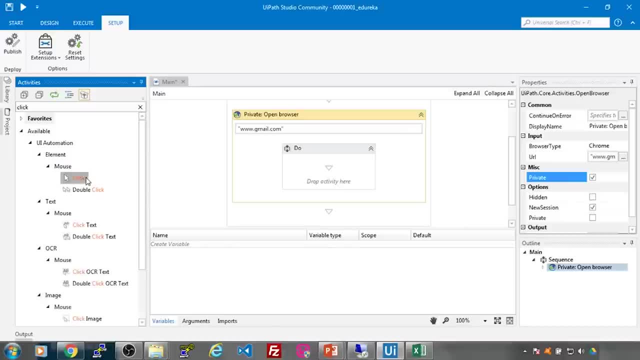 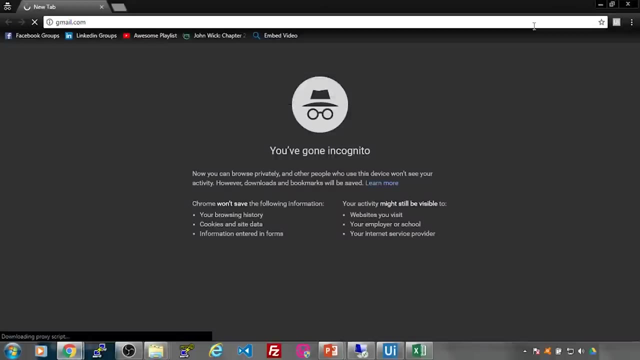 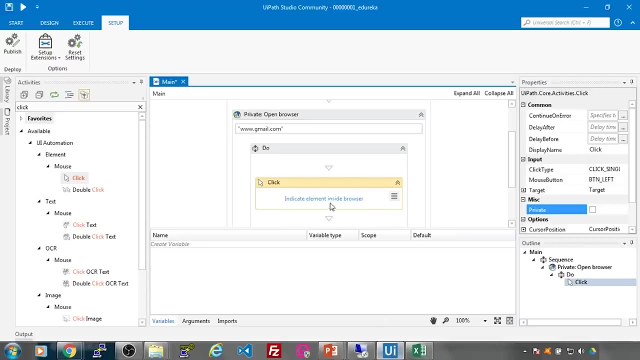 So I'll search for a click activity. I'll drag and drop it here. alright, So now I have to indicate it inside my browser. so let me open it inside a private window. Alright, So let's go to my UiPath. 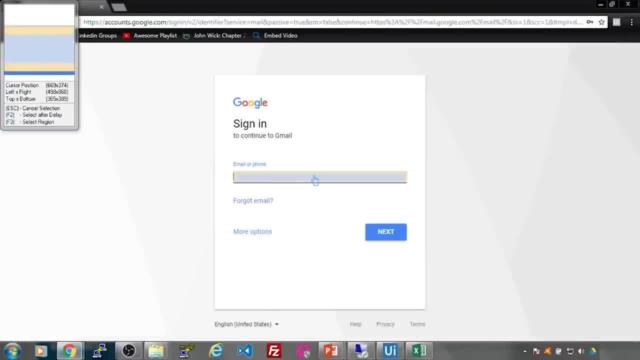 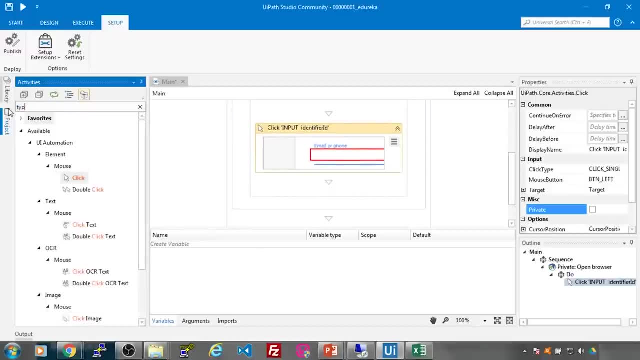 It is asking me where do I have to click? so it has to click inside this particular text box. Once it has clicked over there, I want to type something right, So type. I'll search for an activity called type. I'll drag and drop it here. 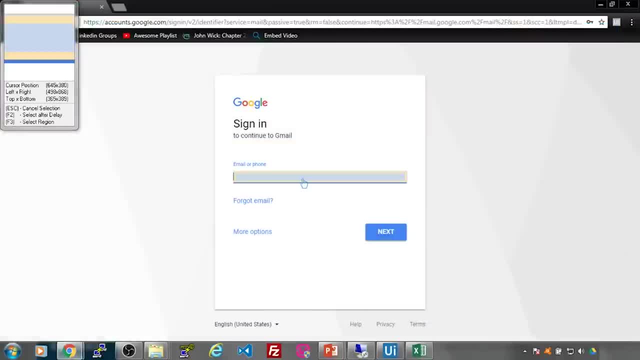 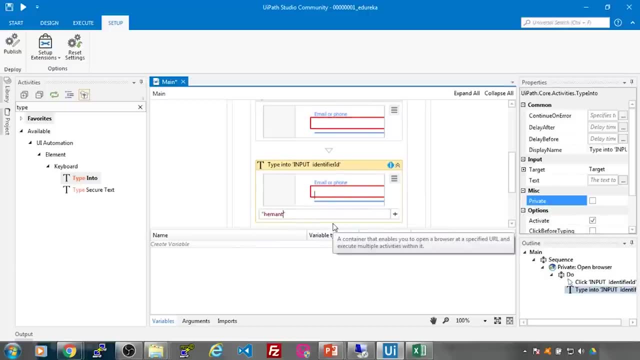 Where do you want to type into? I want to type into this text box, So let us specify the email address over here. So what is the email address that I want to log into? It's hemant, at the rate, edurekaco. 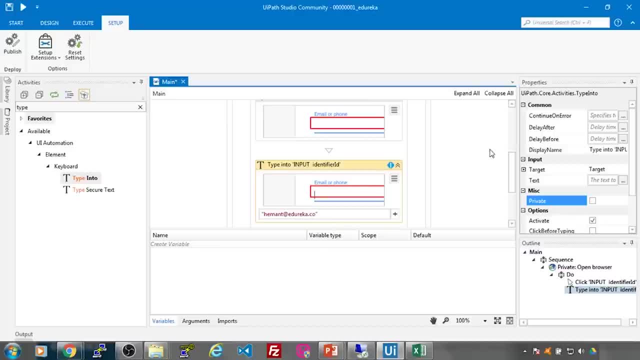 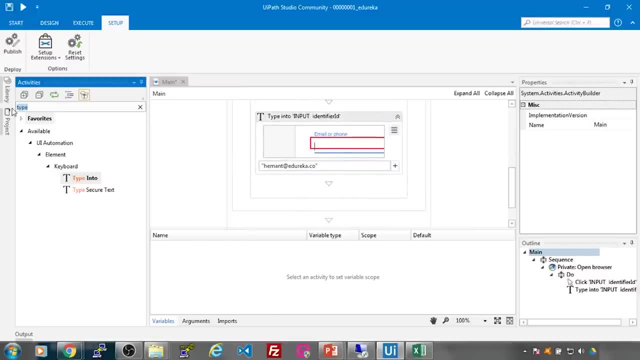 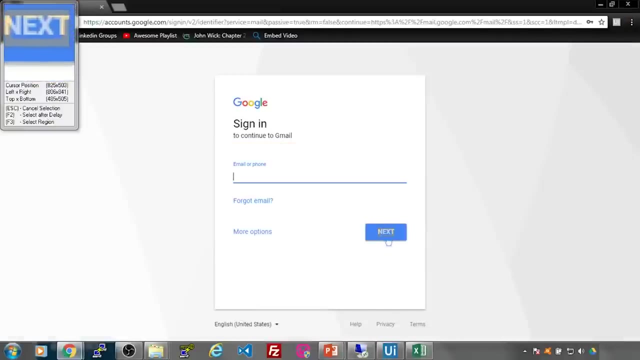 Alright, Okay, So once it has entered here, it again has to click on next. So I'll drag and drop an activity for that. Let's indicate it inside the browser. So this is where I have to click once I've entered the URL or once I've entered the email. 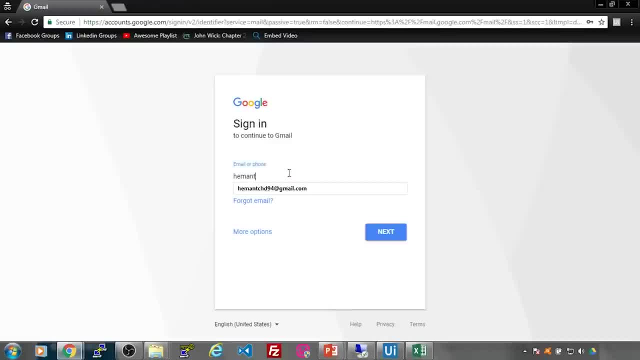 address. So let me enter, say, my email ID, Alright. So this is where I have to click And click on next. This is the next screen that I get. Now I have to enter my password, Alright. So this is something very interesting, guys. 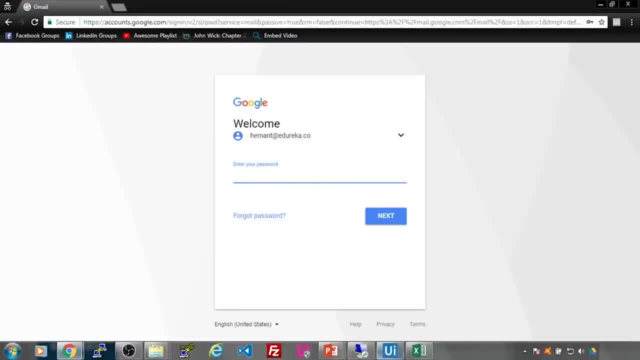 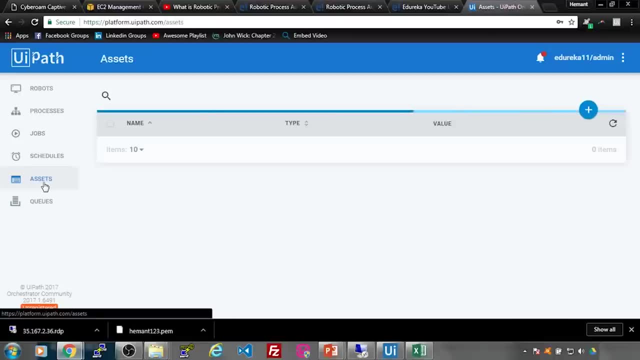 Now what you can do is you can go to your orchestrator- Alright, You can click on assets, And once you click on assets, you can create your own variables over here which you do not have to mention in your projects, Alright. 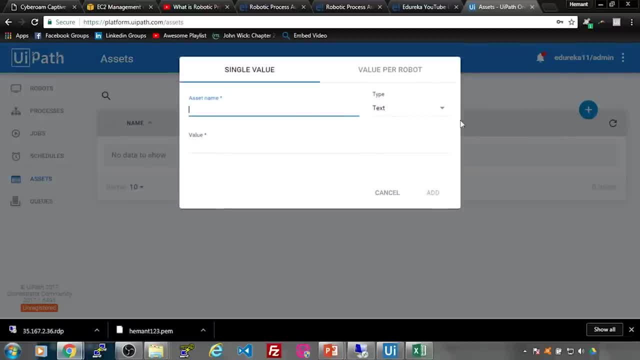 So for that I will click on plus. Alright, I will give my asset name And the type should be Client ID, the type should be credential and my asset will be gmail underscore login. all right, okay, so the username is hemant aderade edurekacom and the password is this. all right, let's click on add. 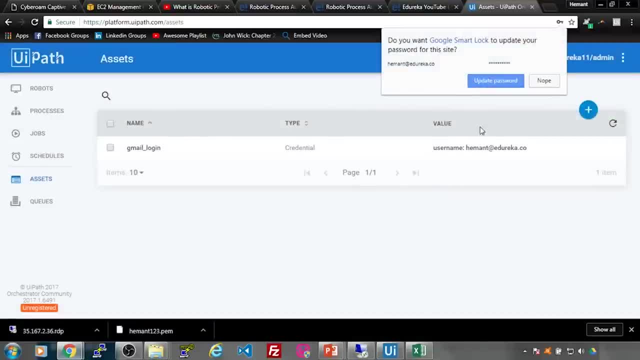 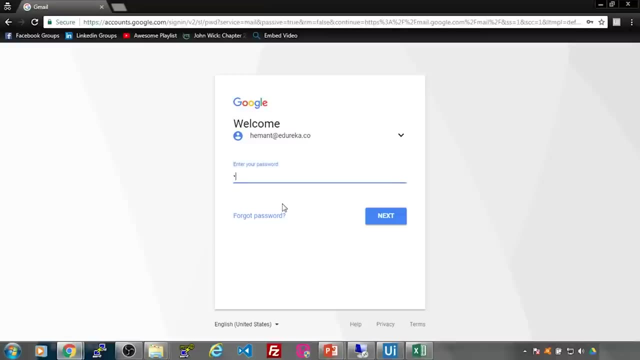 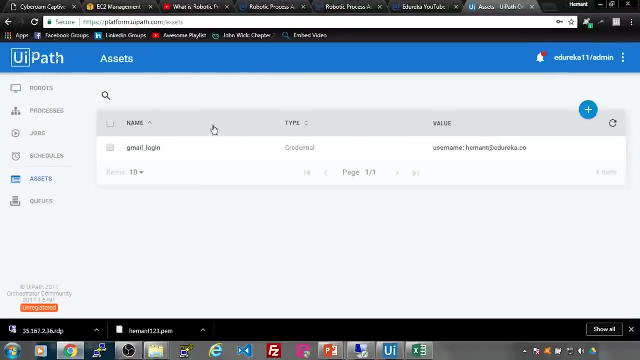 awesome. so it has now- uh, you know- created a gmail login asset for me, which basically is the off type credential and has a username: this: let me quickly check if this is the correct password for me. i ought to forget my passwords very frequently. all right, so, yeah, it was the correct password, so i've entered it over here and now all i have. 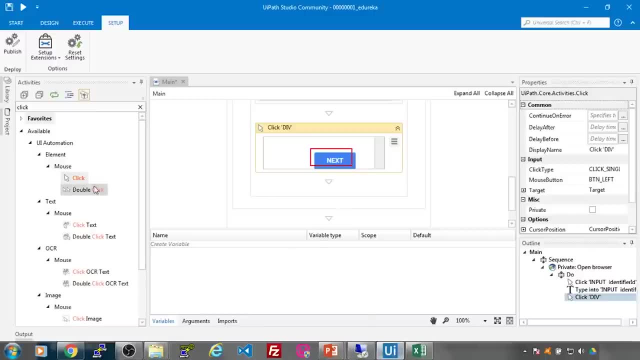 to do is i have to come back to my project and over here i have to go to the main screen, and over here there is an activity called orchestrator. i'll go inside orchestrator. i will find an activity called assets. i'll go inside asset, and there's a thing called get credentials. all right, so let me drag. 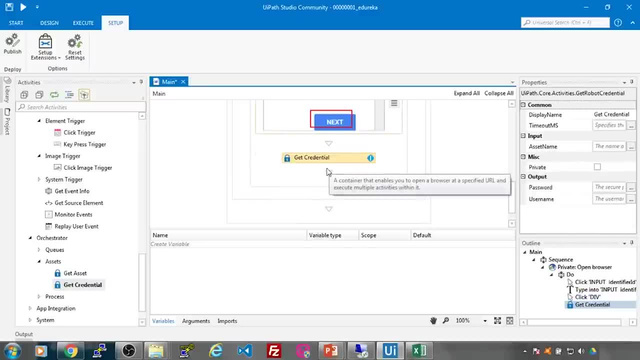 and drop it over here. awesome. now it is asking me the asset name, so the asset name is gmail. underscore login that i mentioned in my orchestrator. all right, and the password. where should the password go? the password should go inside a variable, so the variable should be: 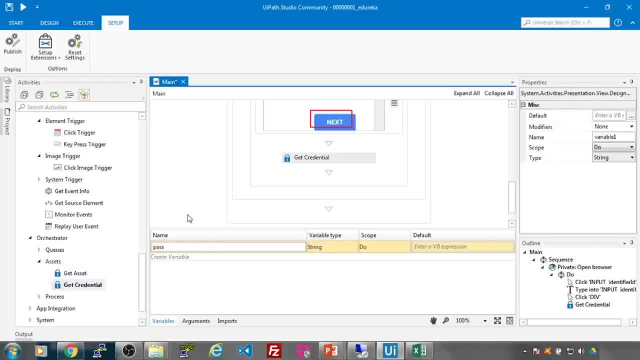 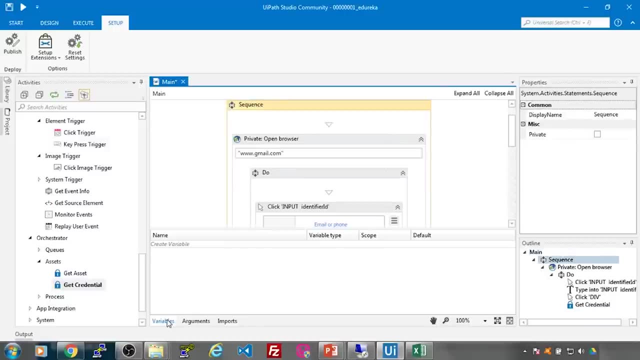 pass right, so i've specified the variable for my activity, so let me define it again. it was not saved, so it's pass all right. all right now. this pass has to be of the variable type password, right, so let us try to. let me quickly show you how you can, you know, come around. 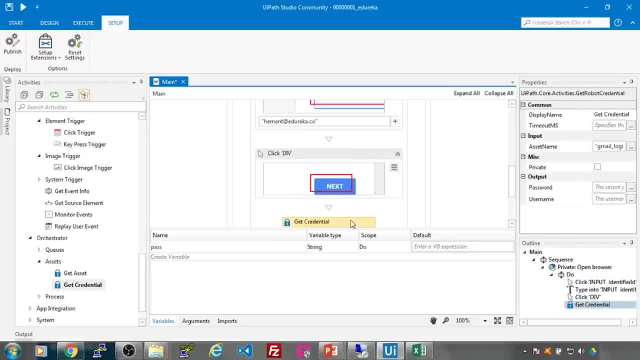 or you can see what type of. how do you identify which type of variable type you have to define? so whenever you will enter a wrong type of input, it will show you this blue icon right. so it says value of type string cannot be converted to system dot. 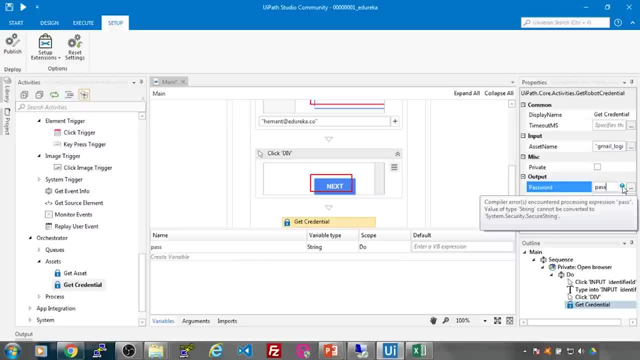 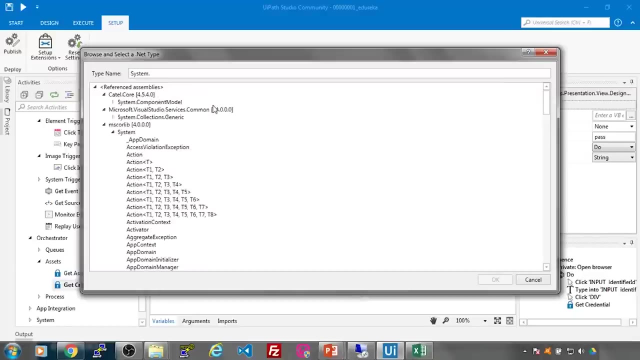 security dot- secure string. so this give basically gives you a hint. okay, so this is the kind of activity or this is the kind of variable that you have to declare. so we will go to variable type, will go to browse for types, will go to system dot- security dot- secure string. right, so it's system dot- security dot. 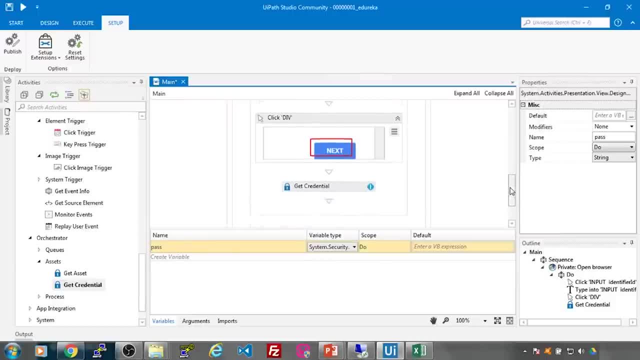 secure string. I'll click on OK. and now, if I go here, you can see the blue icon has gone and has successfully- you know exactly successfully- accepted my variable inside the password. all right, so why am I doing this? I'm doing this because I want to get the 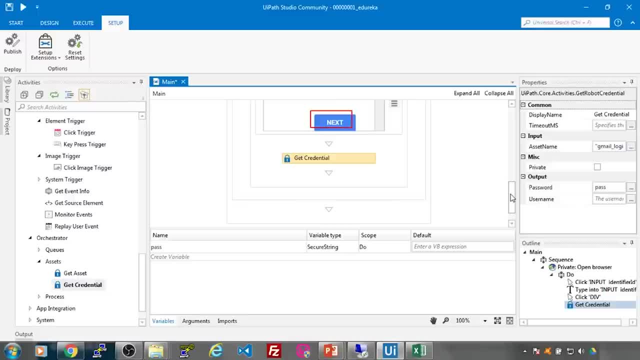 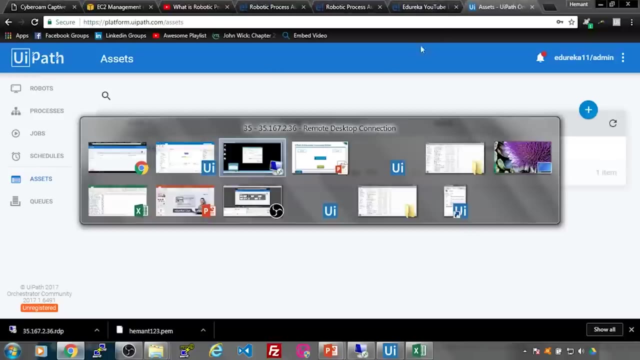 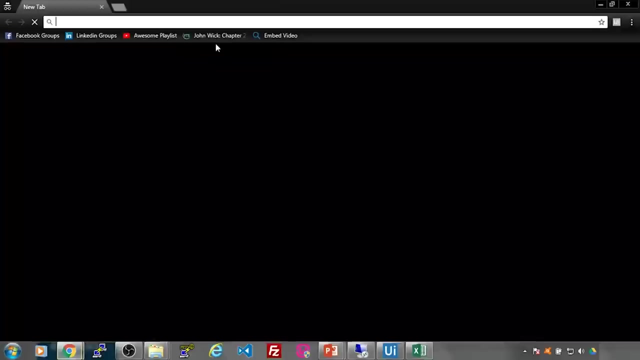 password directly from the orchestrator rather than going to my. you know defining it over here in the system. ok, so I've done that. now the next step is putting this variable that is passed inside my. let me quickly open one more incognito window so that I can show you. 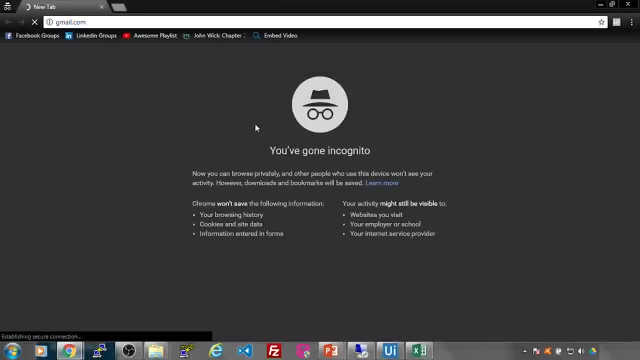 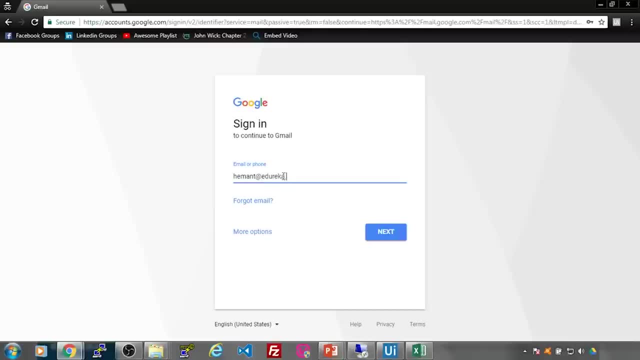 where is the incognito window, so that I can show you where is the incognito window inside my. let me quickly open one more incognito window so that I can show you. it has to be entered right. so this is the email. so let me specify the email first. all right, and 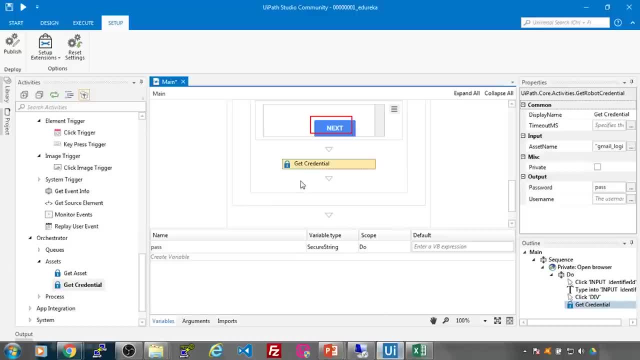 this is where my password will go right, so I have to tell you a path. this is where you will be saving the password, so let me type type secure text. so, because we are entering a password, we have a different activity for entering the password inside my password field, which is type secure text. where do I? 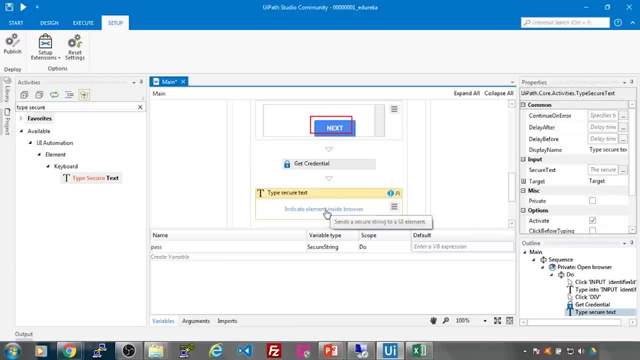 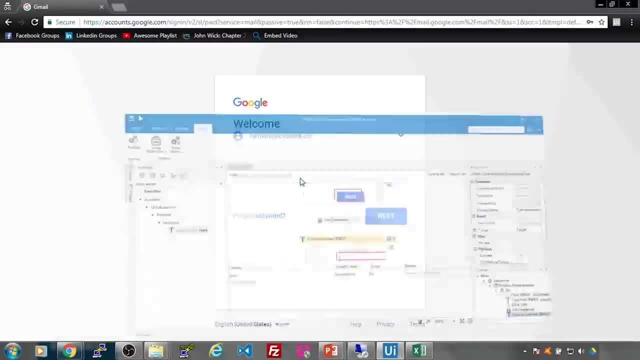 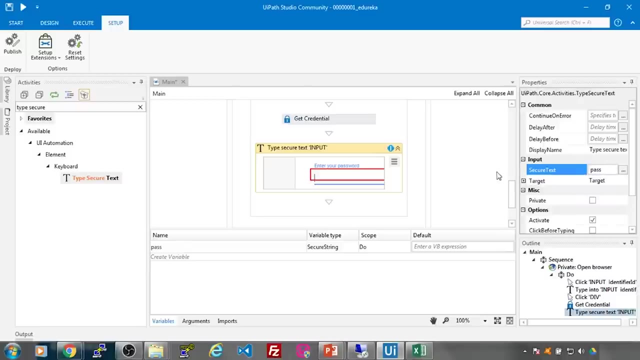 want to enter the password, I have to indicate that inside this particular activity. so I'll indicate element inside browser which is here, right, and then I have to specify the secure text over here which is pass, all right. this basically will enter your password on that page and now you have to click on. 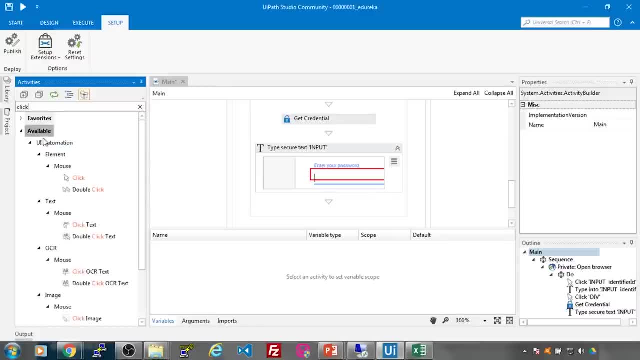 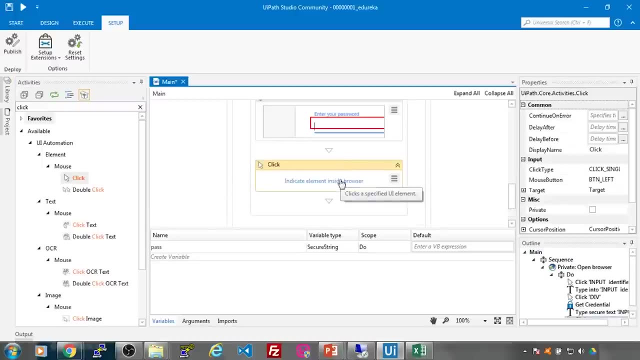 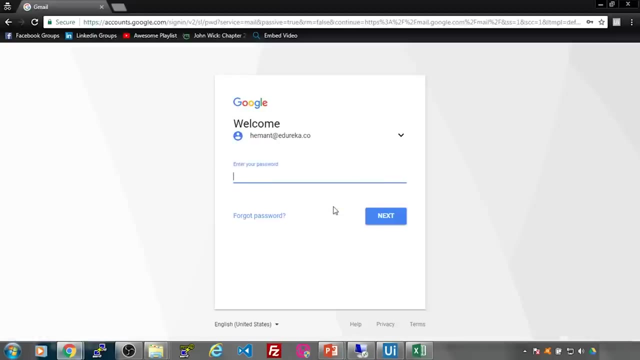 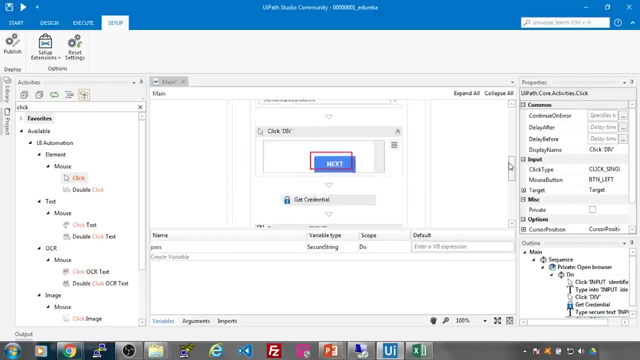 login to successfully execute your automation or for successfully logging into your Gmail. so let's select next over here. so this will basically make you enter or this will basically log you into Gmail. so my activity is done. guys, I have successfully active, created my activity now so let us try to publish. 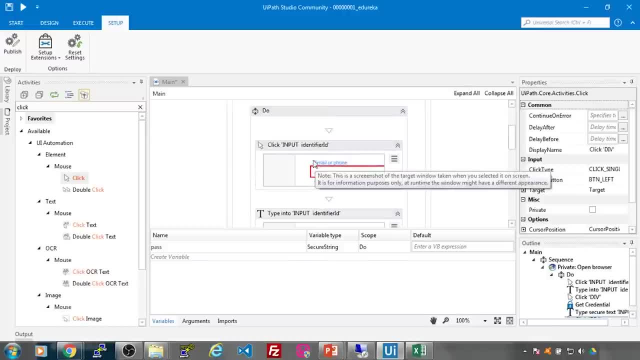 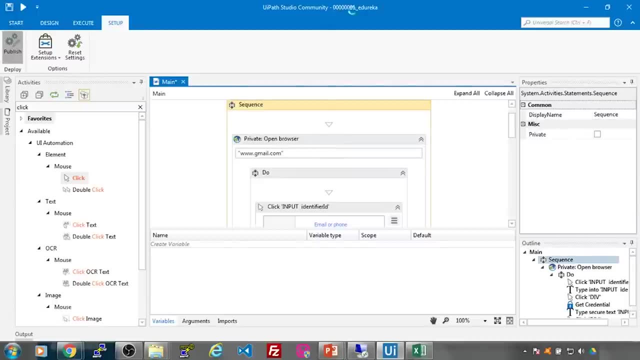 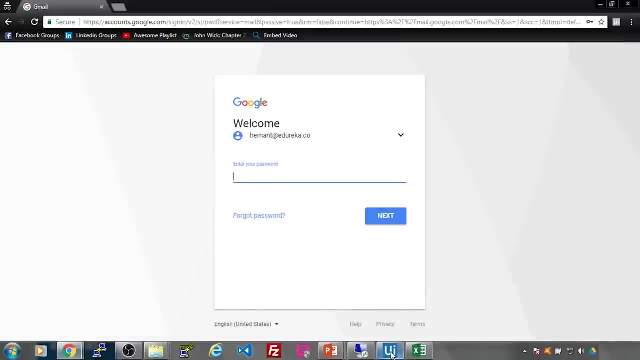 it now and let's see how it actually happens. all right, everything seems fine, let's publish it. so it will get published in under the same folder, which is this. so it has been published to this particular repository with this name. so now again it again: a very important concept inside. 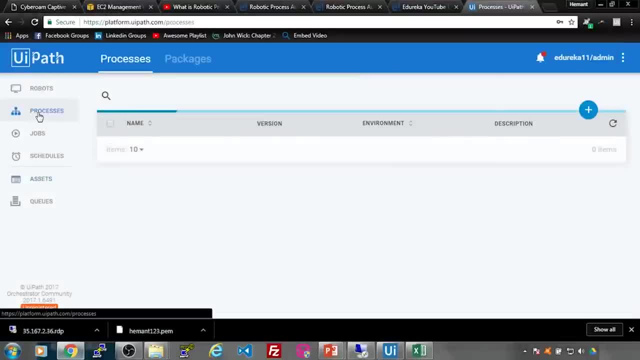 UiPath orchestrator, which is, you know, once you update your package, what do you have to do once you update your project? what should you do? so? once you update your project, guys, you again have to go here inside processes and go to this particular tab, which basically 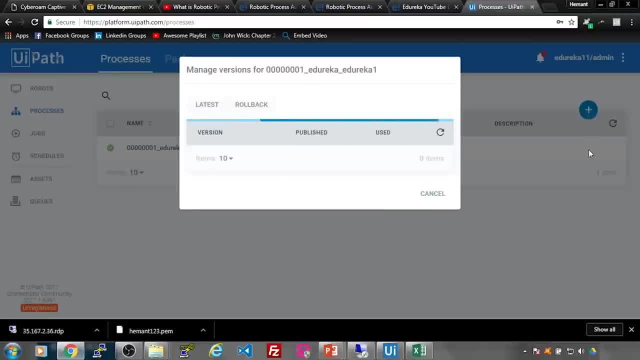 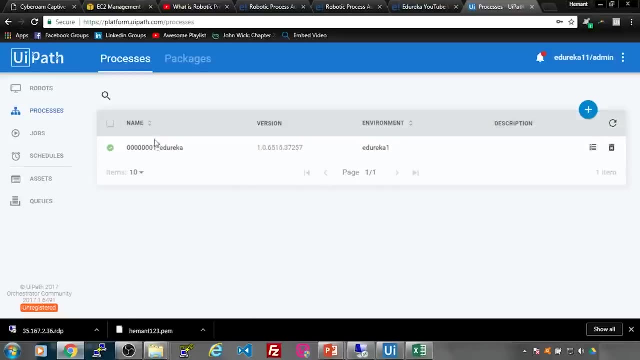 means view versions, right? I'll click on view versions and over here you can see that a new version has just been published a few seconds ago, so I will use this particular version and now my project or has been uploaded, has been updated inside my environment. let's try to run this process now on my API. 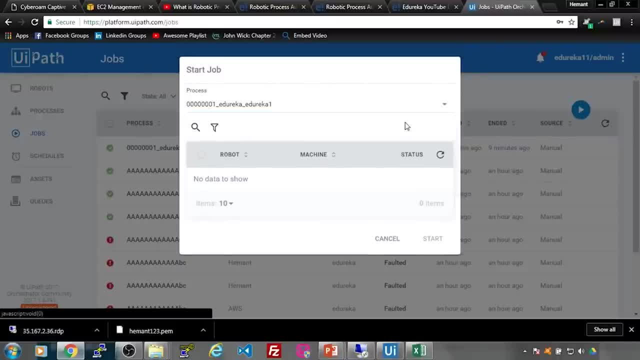 AWS machine. all right, so I'll select the process, which is this: I'll select the machine where I wanted to run on and I'll click on start. and let's hope for the best, let's hope our project runs. so I'll click on start now. so the command. 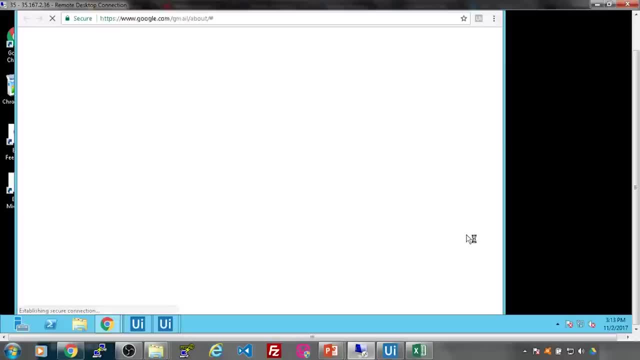 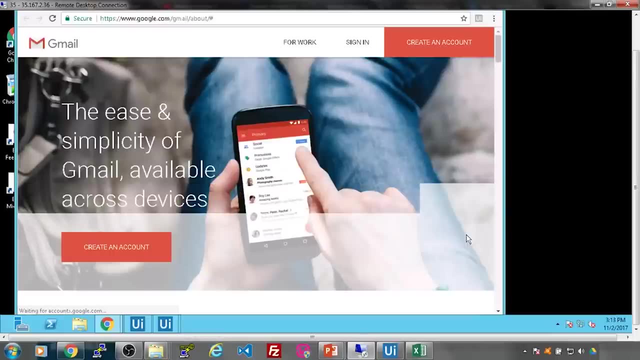 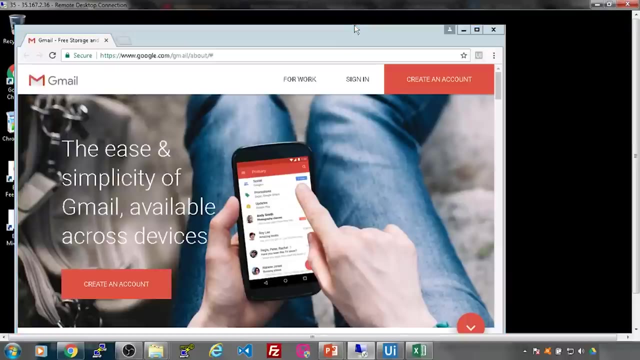 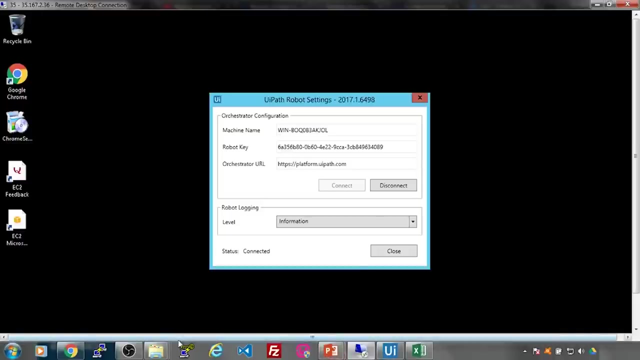 has been sent. so let's see, let's wait for, okay. so basically, over here we are getting a different kind of window, so I'll have to update the URL that I've updated in my page, because this will not work. so to do that, let us close this automation right now and let me again go. 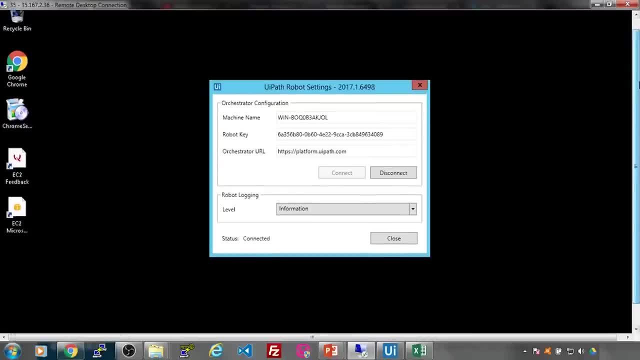 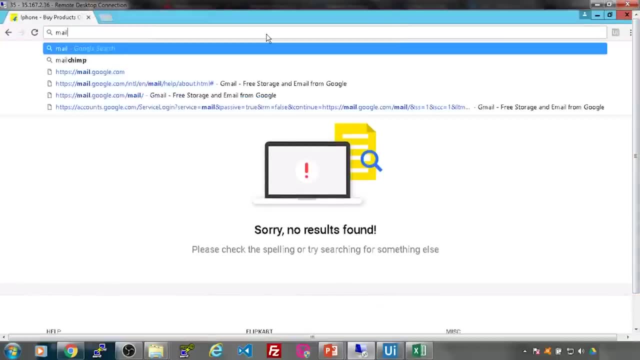 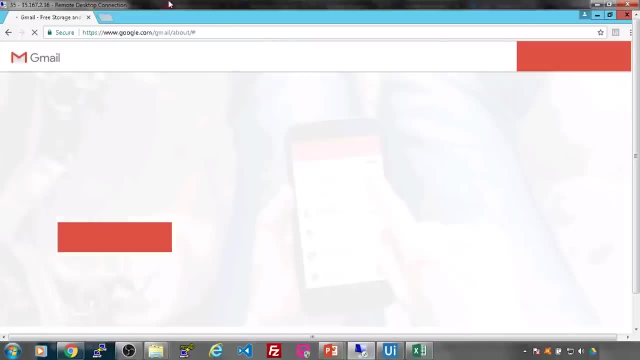 to my UiPath page. let's see which. if I type in mailgooglecom, how does it actually function? so if I type in mailgooglecom, okay, so again, I'm getting this page. I'm getting this page. I'm getting this page, so I have to click on sign in. all right, so this is the page that I have to go to. 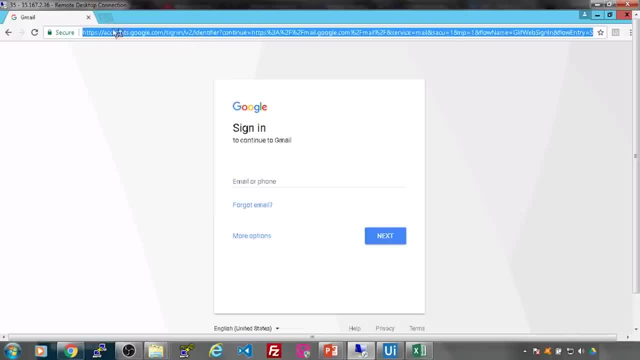 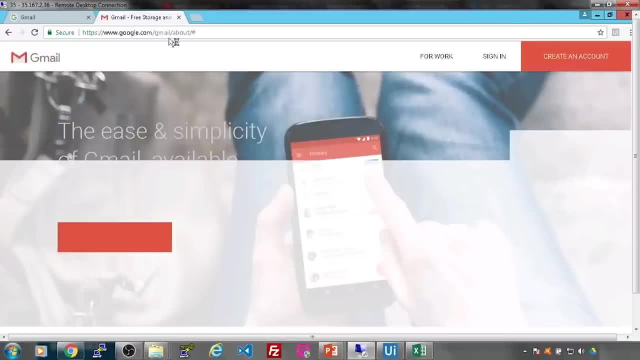 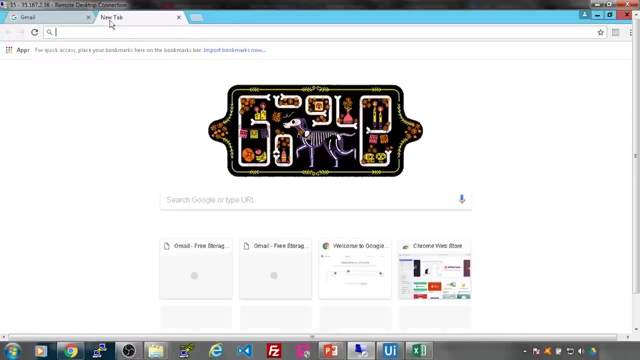 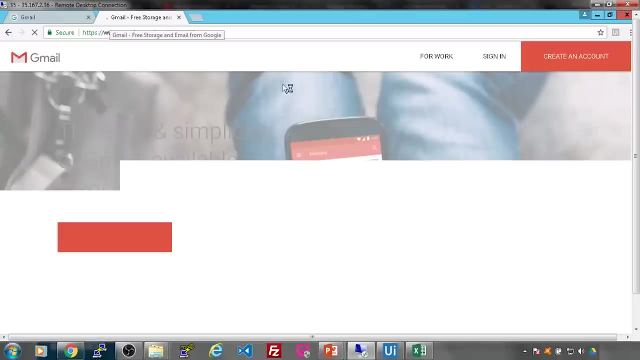 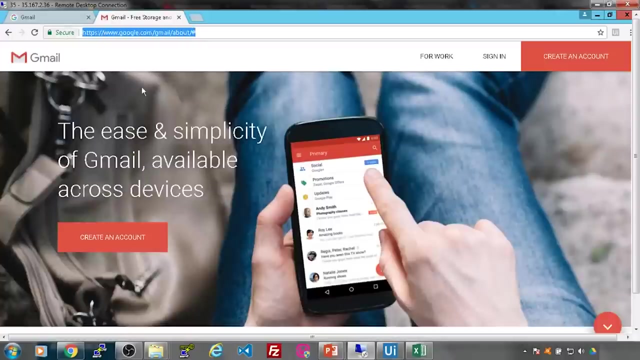 all right. so if I again enter gmailcom here, let's see if it redirects me to this page. okay, so let me enter this URL. then I'll go to this page. that is gmailcom, and let me tell my automation that you have to click on sign in. all right, so let me copy this particular URL. copy it. 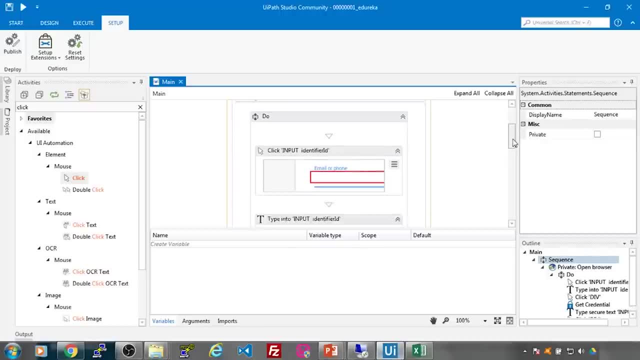 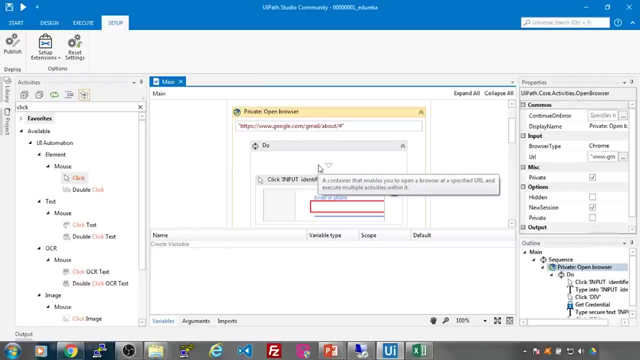 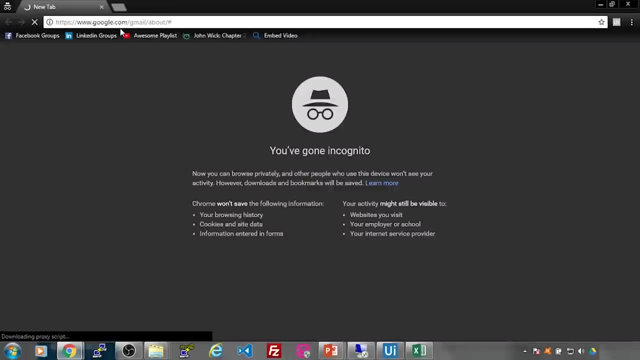 and let me go to my project. so, basically, before you know, going here, I have to enter this particular URL and once it goes to this particular URL, let's see how it looks on my browser. all right, so this is the page now I have to click on. 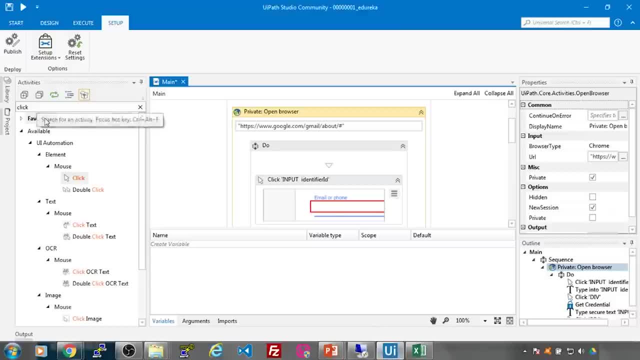 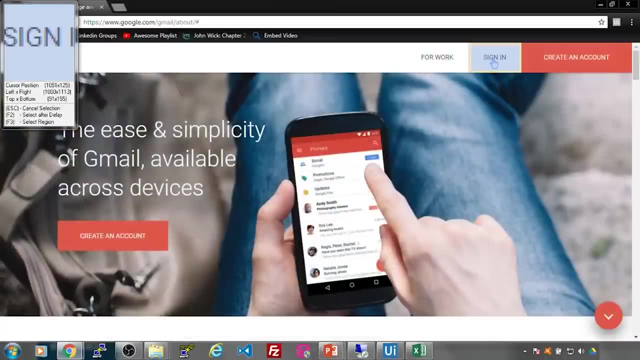 sign in first right. so let's let us specify that. let us include one more click activity and drag and drop it here and indicate where do I have to click on. so I have to click on sign in. so once I've clicked on sign in, I will reach. 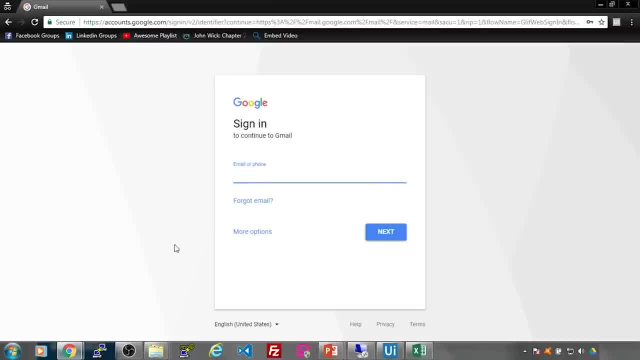 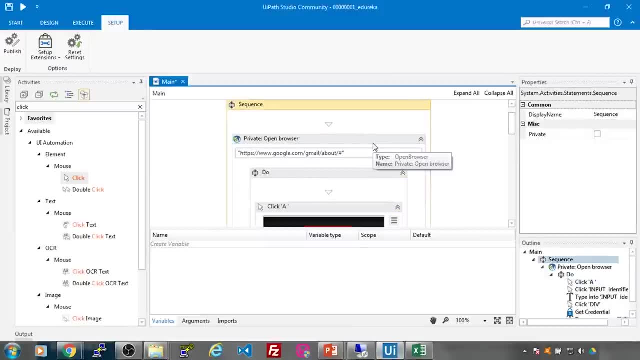 this page and everything seems the same after that. all right, so let's update our project, which we have just modified. so let's save this project and click on publish. so the project has been updated in the repository. now we'll go to UiPath orchestrator, which is here, and 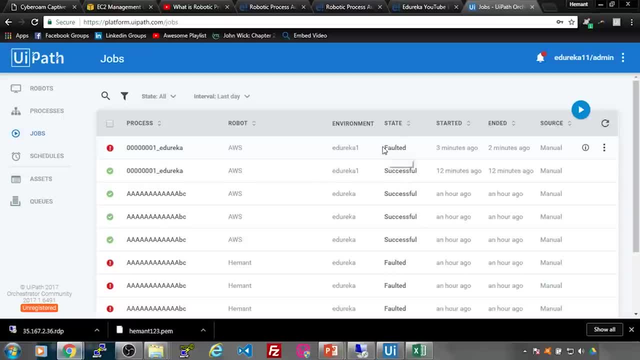 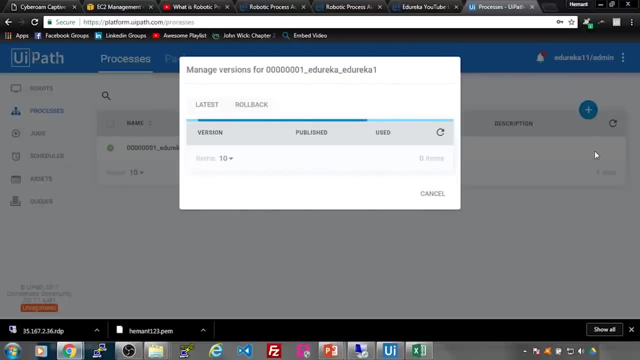 see where you got faulted because it could not execute successfully. so now I go to processes. I'll update my version by going to view versions, and it basically takes time to get reflected over here. so what I do is I'll click on refresh and it takes some time. let's wait for our 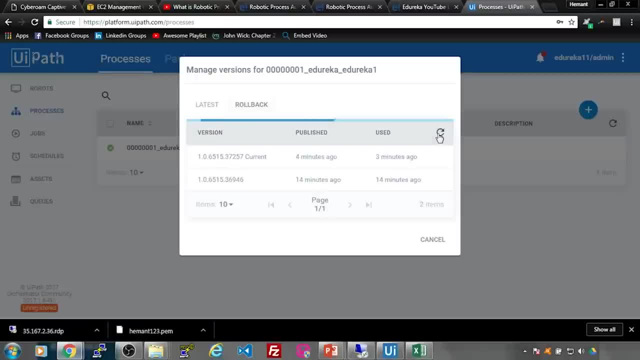 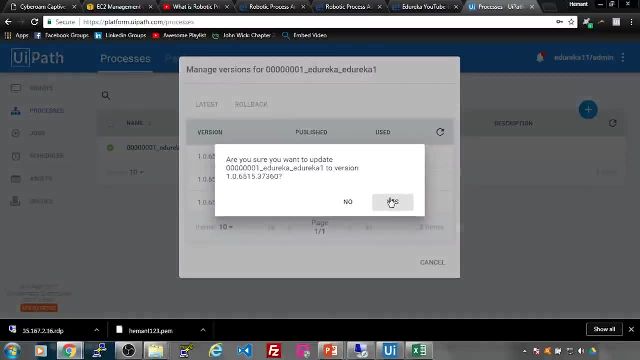 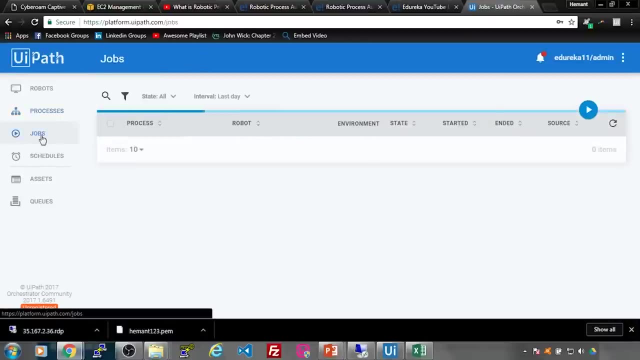 version to be reflected over here in the repository. okay, so my version is now updated over here. let's click on use and let's click on yes. so this will update my project inside my environment. let's again go to jobs again. let's try to execute it. 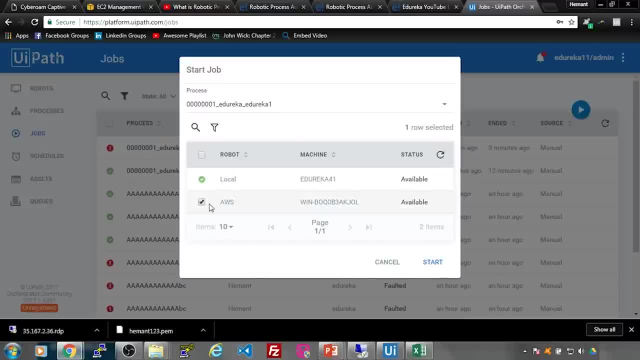 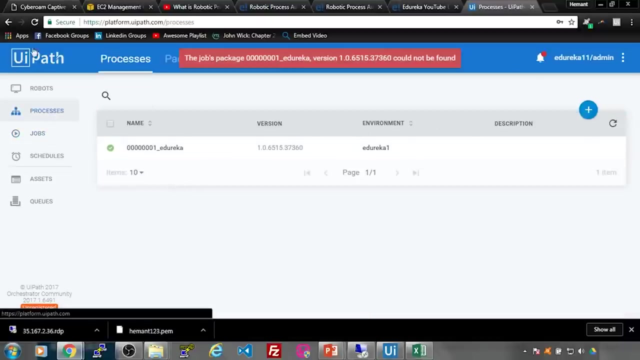 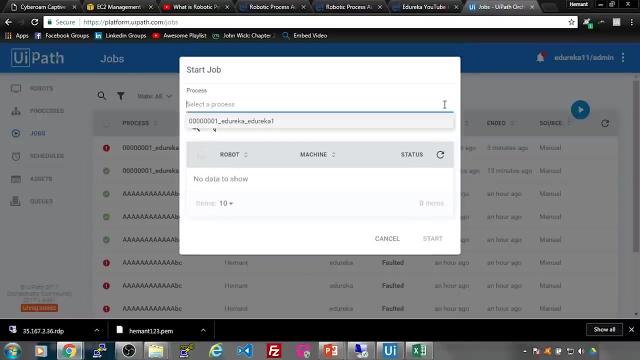 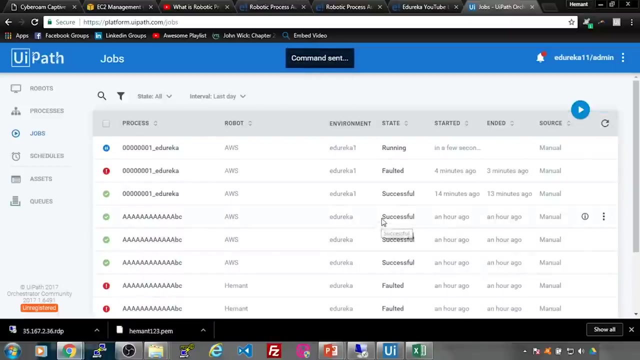 by going to my project and executing it inside the AWS machine. let's click on start, okay. okay, there seems to be some problem. let me quickly refresh it. all right, let's go to jobs again. all right, so the command has been sent. now let's go to my AWS server and see if it's working. 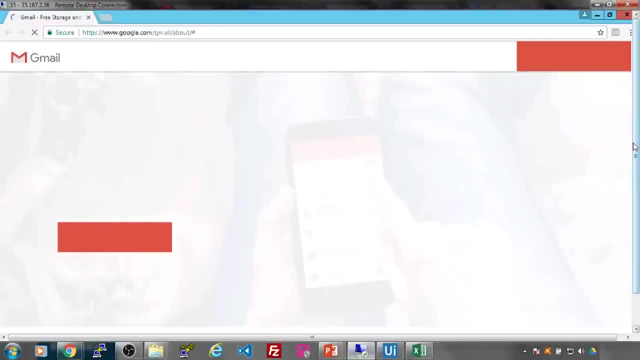 fine now, all right, so it has come here. it has clicked, entered my email all through, pivot to my account. all right, now we've finalized the command and what we've got to do is just workout our. So it is now not entering my password. The system seems to be working a little slow. 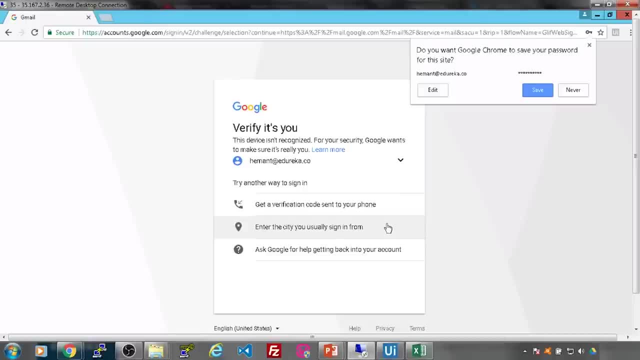 Alright, so I guess that is it, My automation completed successfully. It is asking me one more sign in because you know it is being logged in into some other page, some other server, which is in a different region, and that is why it is asking me to. 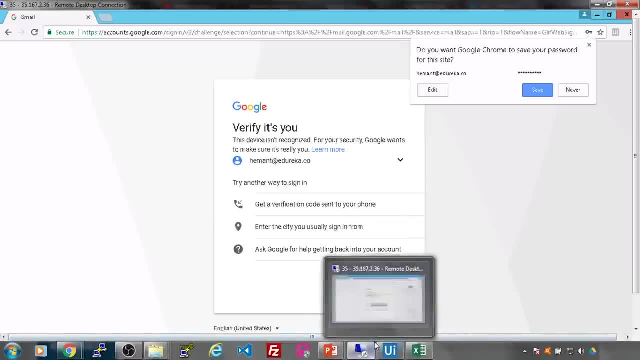 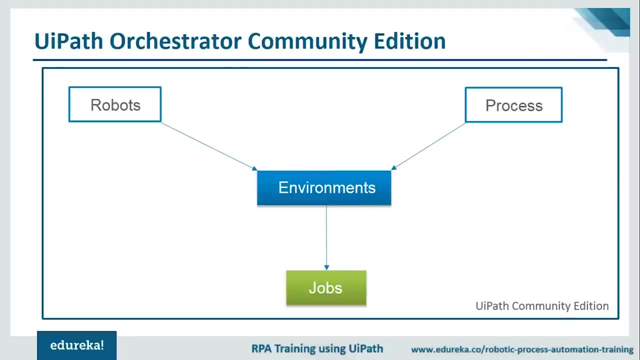 verify myself. But the thing is, we successfully executed our project on a different machine that was in a remote location. we executed from the orchestrator and we were able to execute the project from our end by, you know, publishing it on to the repository and then executing. 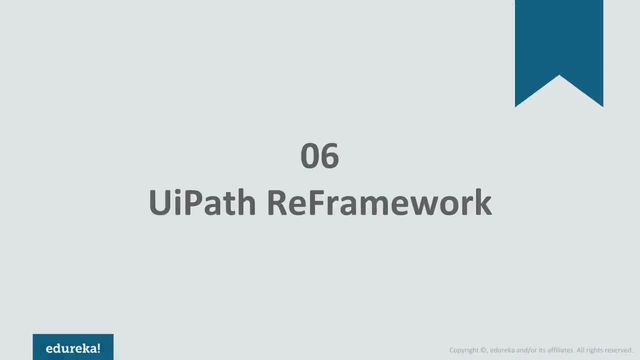 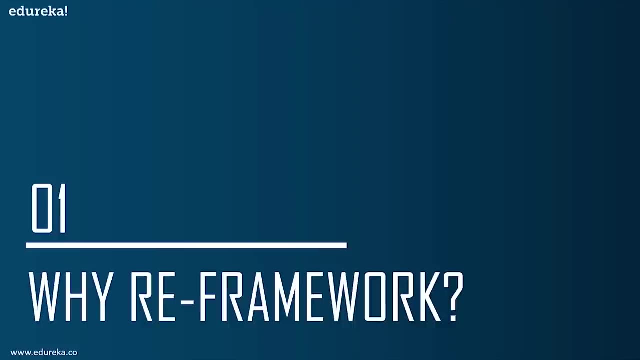 it from the orchestrator? Why do we exactly need the AARI framework? So let me just explain you with an example. Now consider a scenario wherein you are automating a particular task, let's say the process of extracting the data from various invoices. right, 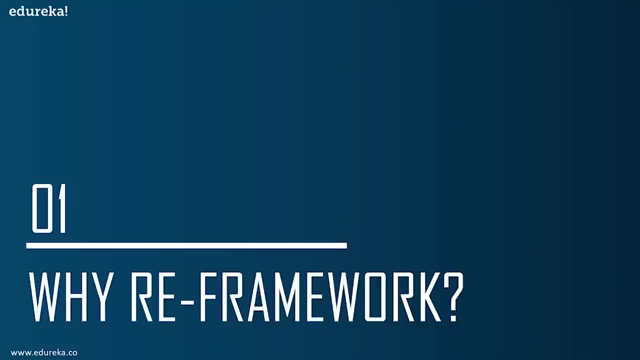 Now, to automate this process, we need to mention the folder from which we are automating. the invoices have to be read, then identify the fields, basically all the fields from which you want the data to be extracted right. So obviously, if you just observe into this task, you cannot completely automate the process. 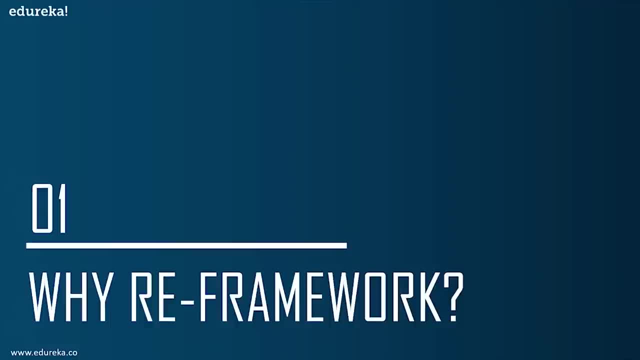 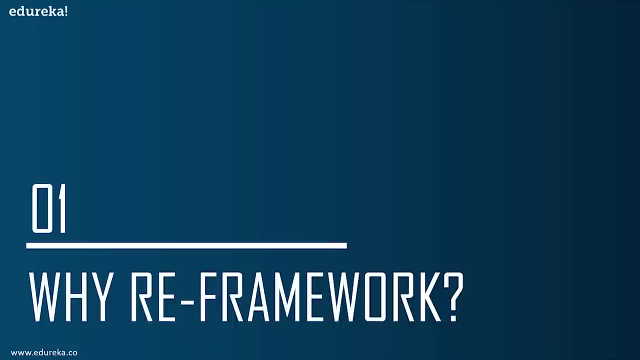 These invoices are already read and which are not right. So, basically, to avoid human intervention, We have to define the robots in such a way that they can be used in every possible situation, and this is where, basically, the re framework comes into the picture. This framework is basically a template that helps the user define the process that offer. 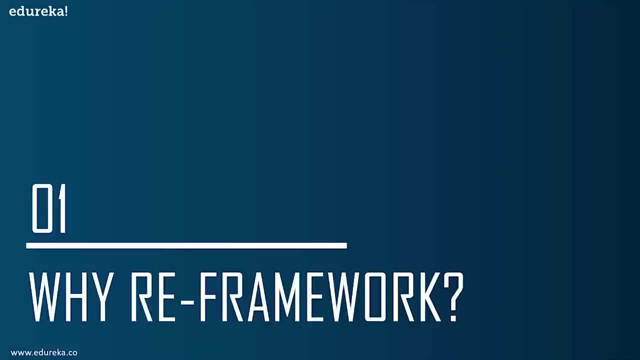 a way to store, read and easily modify the project configuration data, with robust exception handling scheme and event logging for all the exceptions and also the relevant transaction information. this framework logs messages at each and every relevant step towards solving a business transaction and since those logs to the orchestrator server. this. 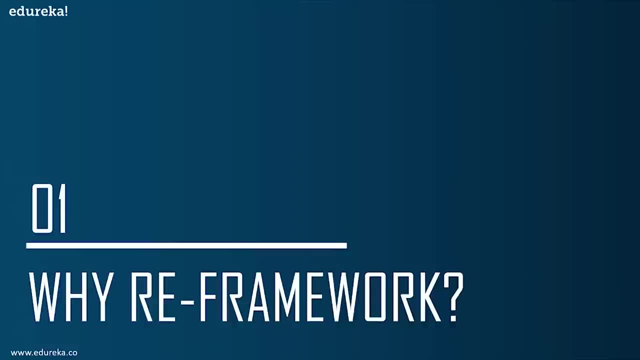 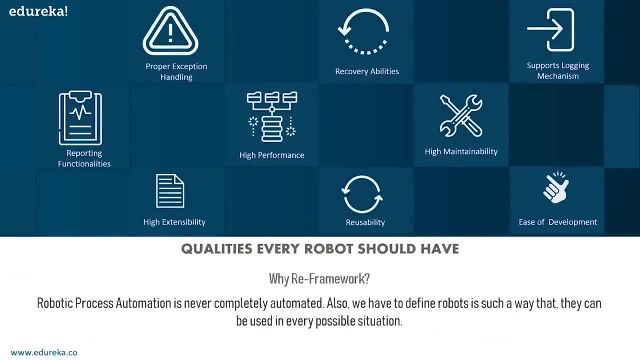 in turn, can be connected to a database, to where all the data can be stored, right? So if I have to summarize the need of re framework for you, then it directly implies to the qualities that each and every robot should possess, right? So the reasons are as you can see on my screen. 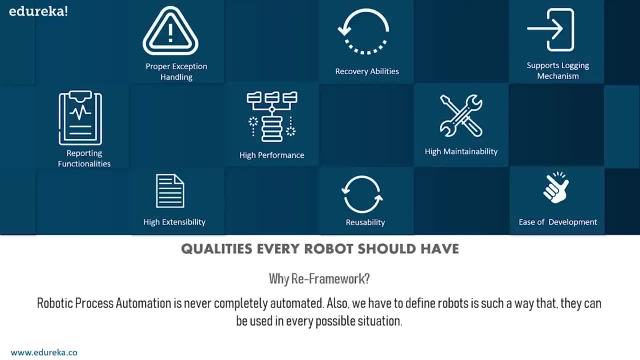 that is basically the proper exception: handling, recovery abilities, supports, locking mechanism, reporting functionalities, high performance, high maintainability, high extensibility, reusability and, finally, the ease of development right. So the need of free framework is really simple, guys, Whenever we want to remove the human intervention completely. 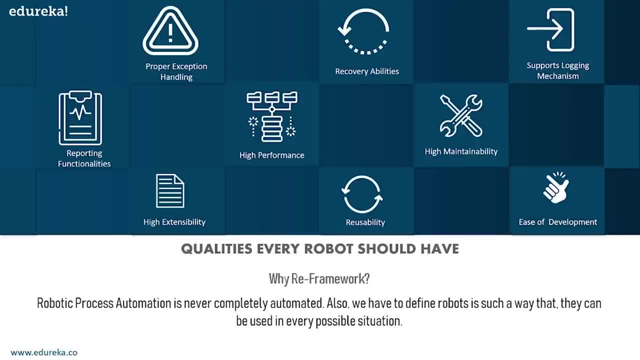 and design a robots in such a way that they can perform in each and every situation is basically where the reframe work comes into the picture, right? So now that you know why we need reframe work, Let's look into what exactly reframe work is right. 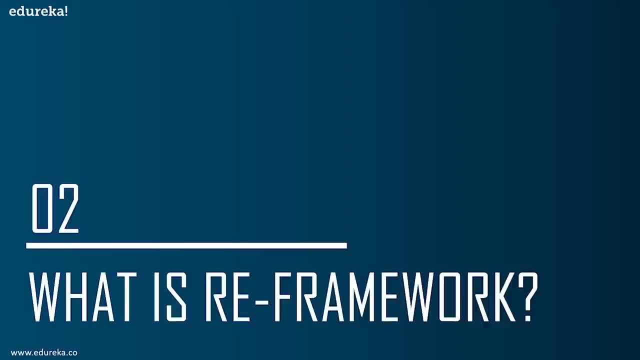 Well, if I have to explain reframe work for you, then reframe work can be considered as the starting point of every project. So to explain you this point, let's consider the scenario of a business process. Now, before I move on with our business process, 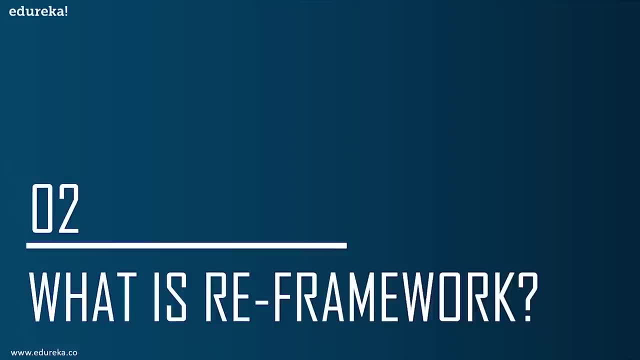 let me tell you that each business process consists of multiple distinct in scope and in-purpose collection of components, and each components can have many transactions right. So a business process can have around five, six components, or even maybe more, More than that, or maybe less than that. 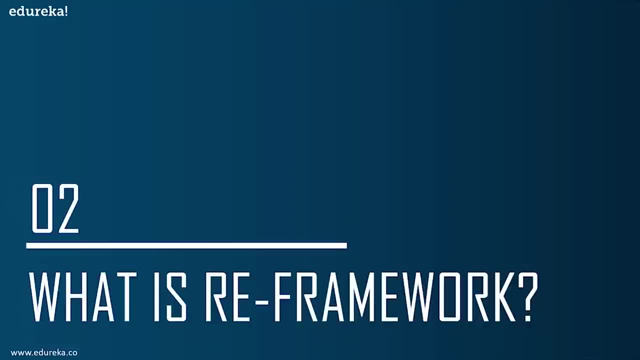 and then each component can again have a set of transactions. So a collection of relatable business transaction forms, of business process component and a business component is a part of the complete business process that you're working on. So now to explain you further of consider the scenario. 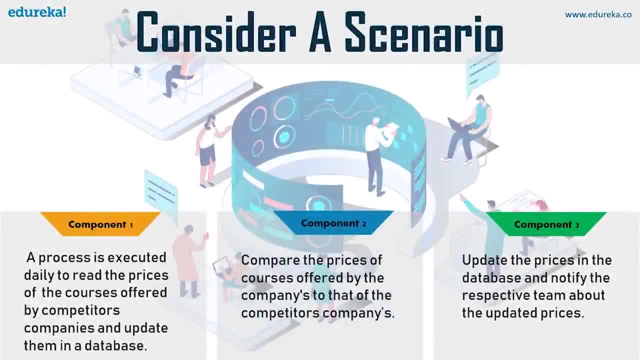 that you can see on my screen. So our scenario is basically to update the prices of the courses of the competitors companies into our database so that we can compare and then we can understand the market values of each and every course and our company. right now, the business process that I have considered will basically 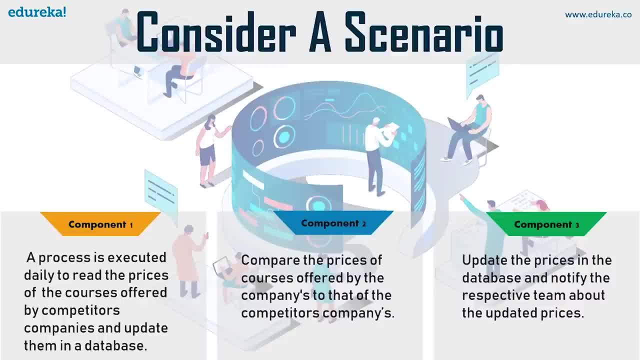 have three components. The first component will basically consist of a process which is executed daily to read the prices of the courses offered by the competitors companies. right After that, the second component will basically compare the prices of the courses offered by our company to that of the competitors company. 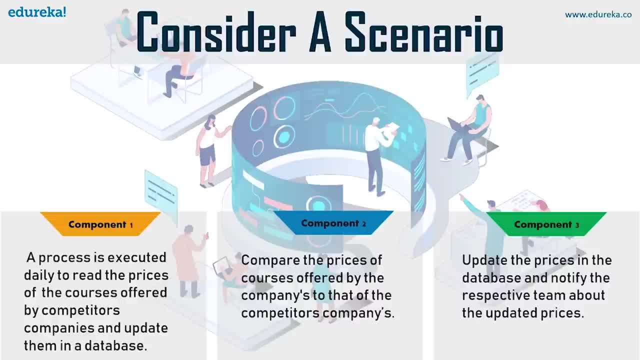 and finally, the third component will update the prices in the database and notify the respective team about the updated prices. right? So, guys, these are basically the three components that our business process will consist of. so now, once you've figured out the components, each component can be further divided into business transactions, right? 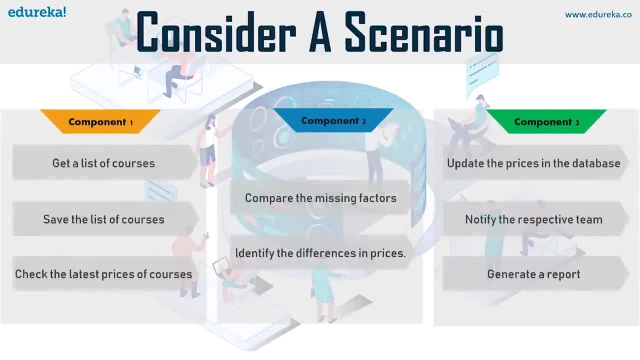 So in our scenario, I have considered the transactions for each component to be as you can see on my screen. So our first component will basically have three business transactions. That is, the first transaction is to basically get a list of courses to which we want to compare the prices. 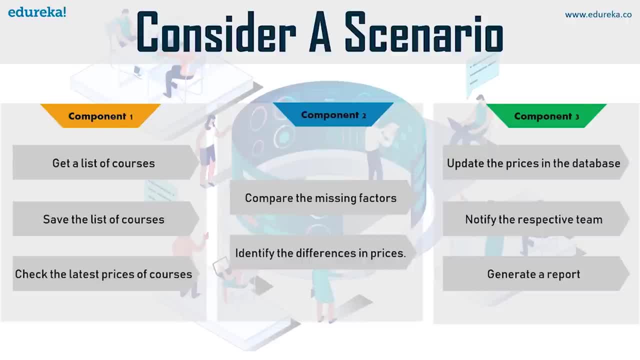 after that second transaction will basically save the list of courses and the third transaction will basically check the latest prices of the courses. The second component will basically compare the missing factors. So, for example, let's say you know the competitors have some course live on their website. 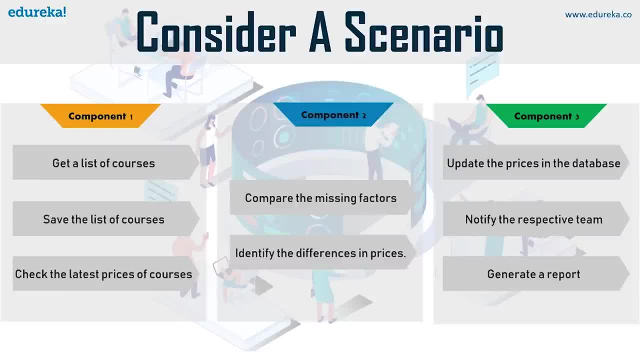 but they haven't released the price of the course either in India or maybe any other nation, right? Also, the second transaction of this component will basically identify the differences in the prices of the courses offered by our company to that of the competitors company. and finally, coming to the third component, 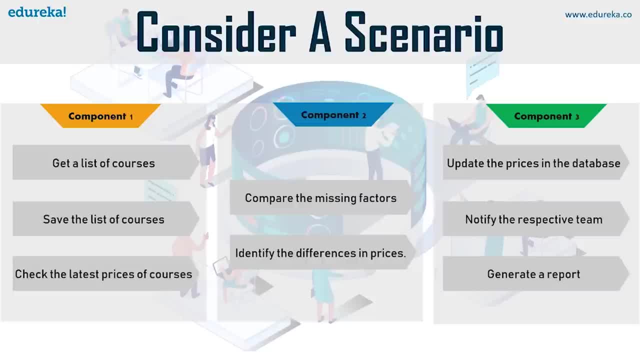 in the third component. The first transaction will basically update the prices in the database and then notify the respective team about the updating of the prices. So basically the notifying part is done by the second transaction and finally, coming to the turn transaction, The third transaction is basically used. 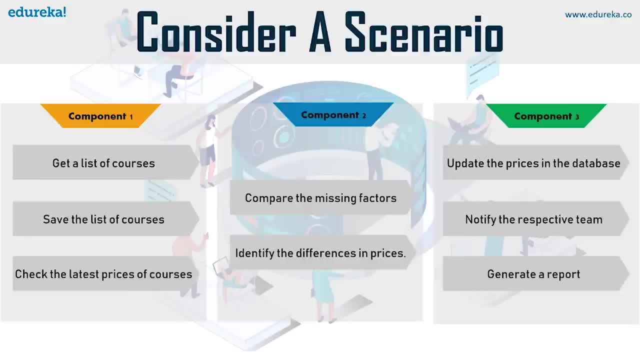 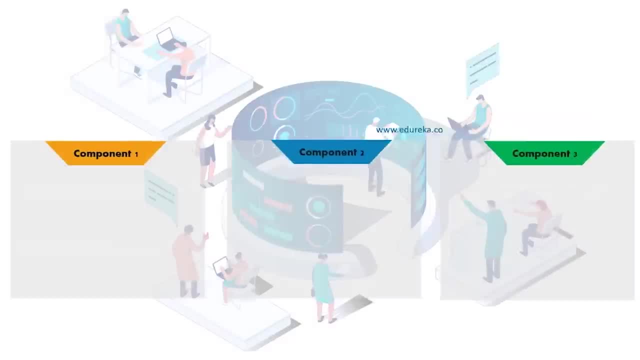 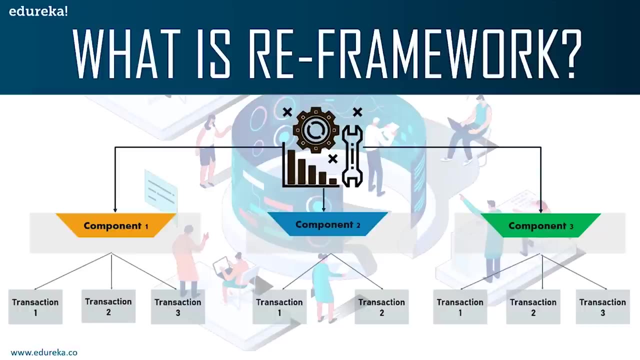 to generate a report of those prices, right? So basically, guys, in our scenario you can have three components and then each component can have these transactions, right? So basically, if you have understood from my example, then each business process is basically a collection of components and further the components. 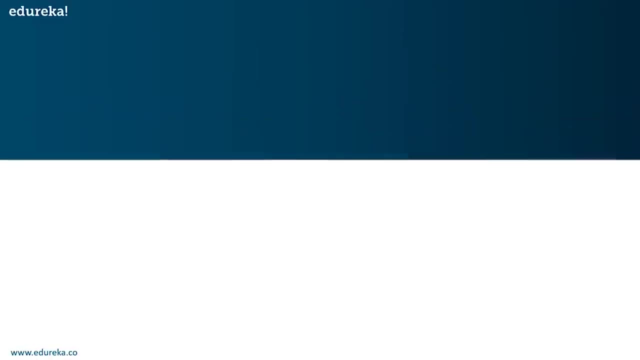 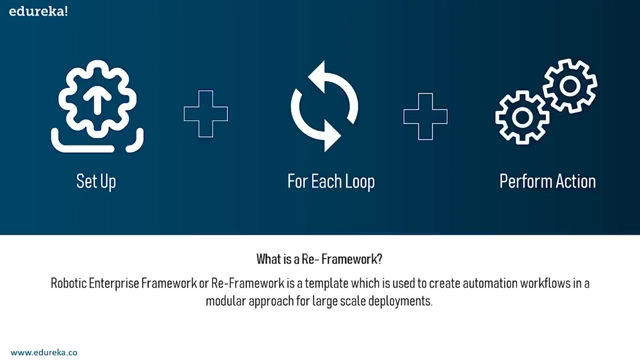 are a collection of a transactions. If you're wondering where does reframe work come into the picture, then let me tell you that the robotic Enterprise framework, or the re framework, is a template which is used to create automation workflows in a modular approach for large-scale deployments. 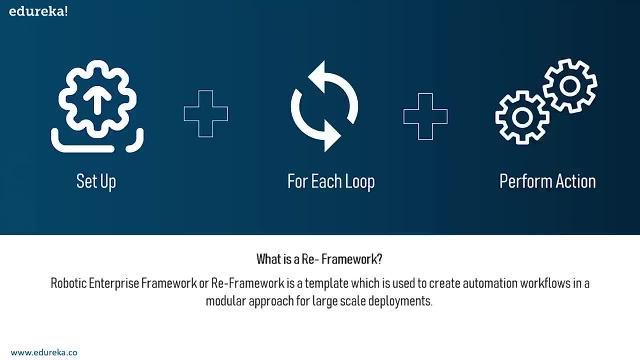 So basically, it is used to set up the project configuration for each and every loop to perform a set of actions. So when you start working on re framework, you'll basically understand that you know: set up a set of actions for each and every loop. 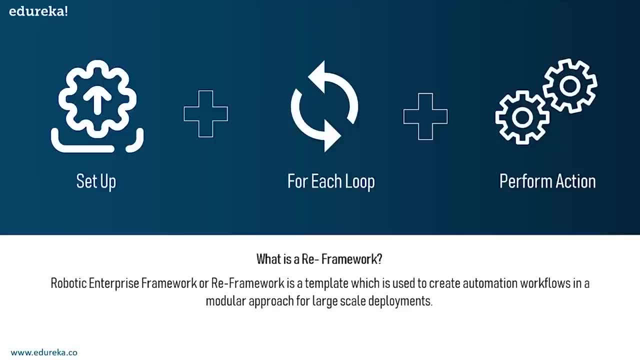 So basically, those set of actions will iterate for each and every loop and then, finally, the action will be performed or maybe you'll see an output, right? So basically it goes for a loop. So, don't worry, I'm going to explain you the different components. 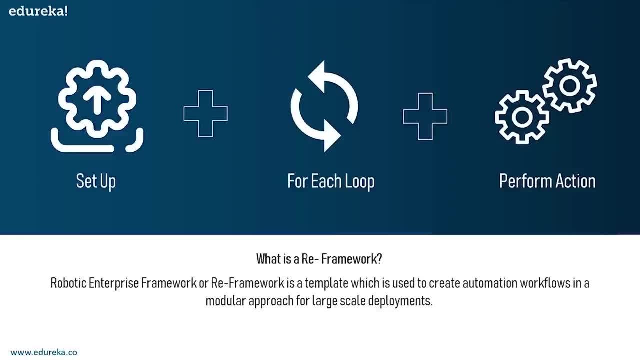 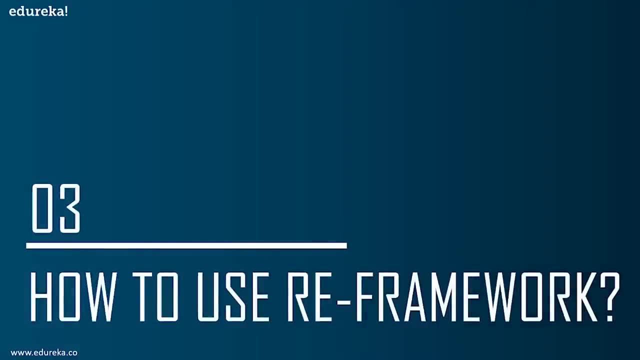 of the re framework to understand how you can actually do the stuff right. So now moving on with our session. next, Let's look into how to exactly use this re framework right. So, to use re framework, what you have to do is you have. 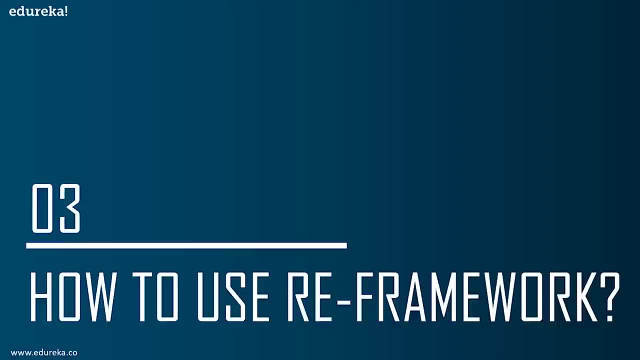 to first identify the components of your business processes and then understand where could be the areas of exceptions and reporting of locks. after that You have to open your uipath studio and you have to start the uipath robotic Enterprise framework template, and after that you have to start just. 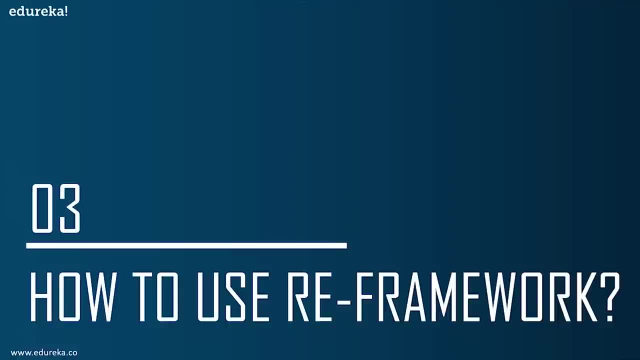 customizing the blocks which are present already in that framework, right? So the customizing part of these blocks is basically how you want your transaction or basically how you want your business process to work on, Right? So I'm going to explain you about each and every component of that re framework very soon. 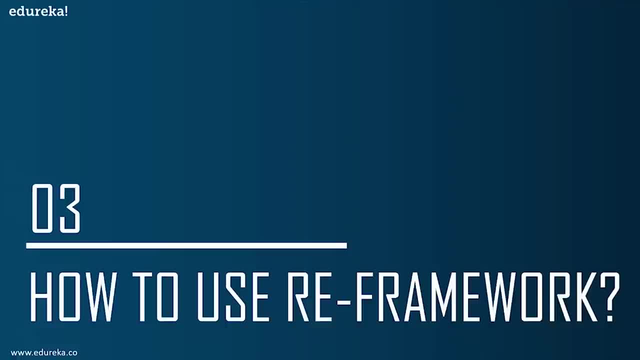 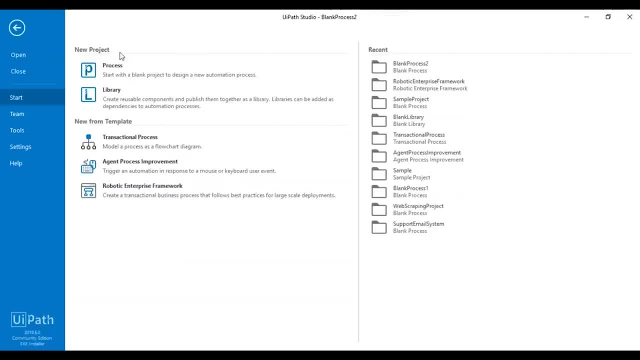 So now, before I just move on with the explanation part of those components, let me just quickly open the project and show you so. when I click on the start button on the left hand side you'll see various kinds of projects and templates you can use in uipath right. 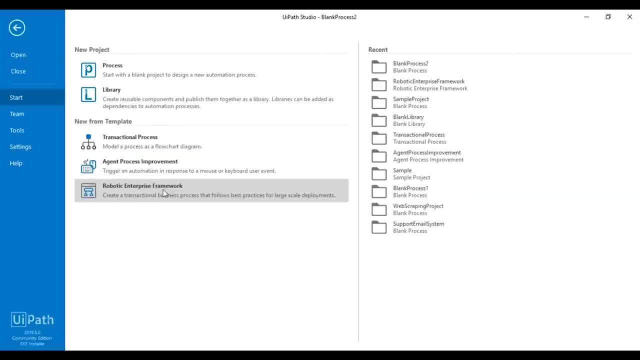 So over there you see an option of robotic Enterprise framework. So if I just double click on that, you can just mention the name, location and the description of your project. So let's say we just mentioned robotic Enterprise framework Demo and then let the location and description be the same. 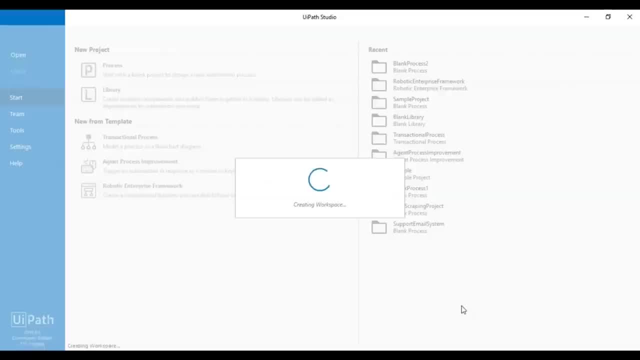 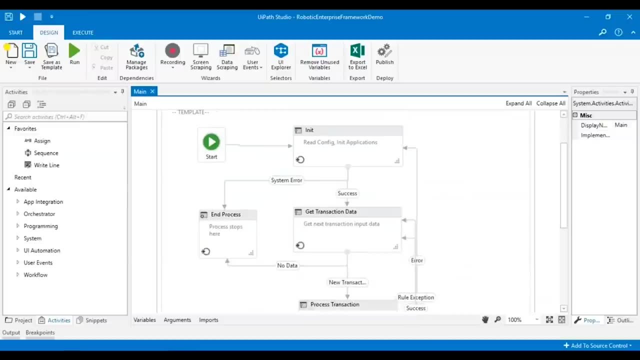 and then I'll just click on create. So once I click on create, you'll see that you know your project is loading, So let's just wait for that to happen. All right, So, as you can see, this is how your re framework looks like. it has various states. 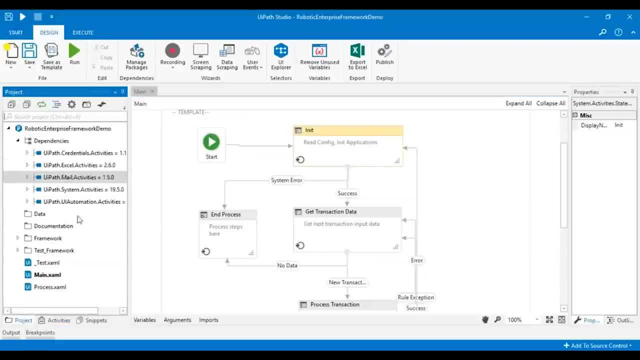 and machine. So now, if you just go back to your project tab over here, you'll clearly see the various dependencies and the ways files this particular process has right now over here. out of all these files You don't have to change the settings for all the files. 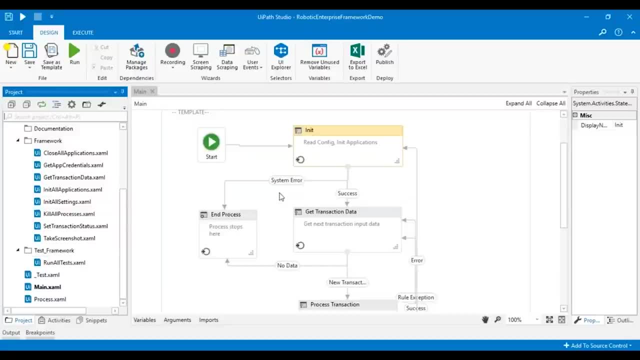 You just have to change the settings for few files, So some files remain the same as they are and some basically get changed based on your business process. Right apart from that, we have this main file, So the main file is basically the file which executes. 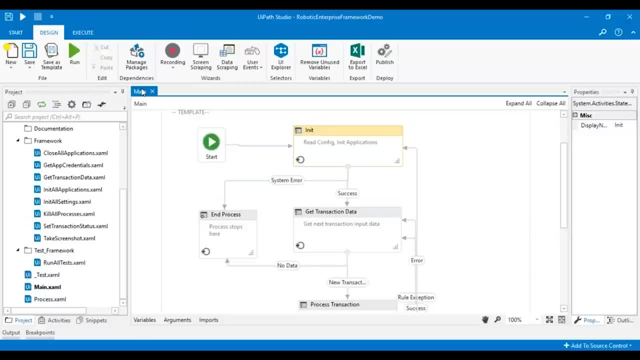 when a project is deployed and published onto the orchestrator server. So this is the file which basically executes. right, So over here you have to configure the file based on your business processes. again, All right, So this was all about how to use re framework next. 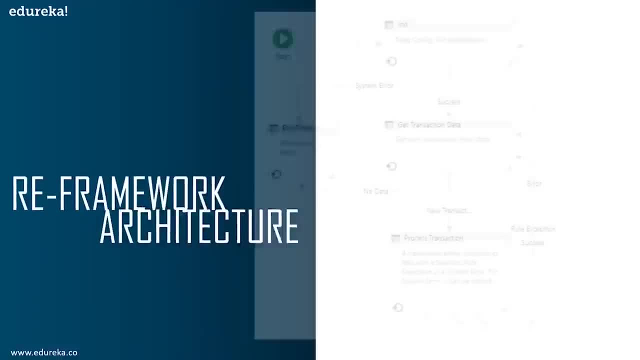 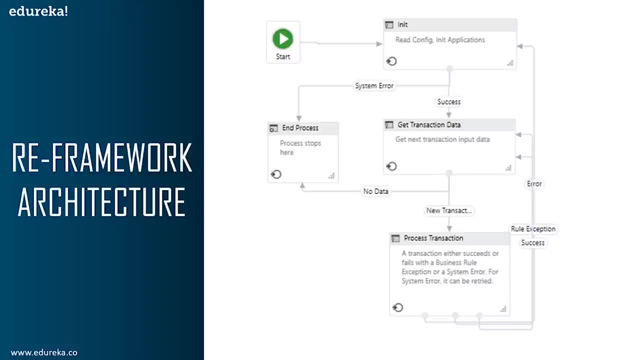 Let's look into the re framework architecture. So the re framework architecture basically uses the state machine diagram, as you can see on my screen. So it basically has four states, that is, the init state that get transaction data state, the process transaction and the end process state- right, 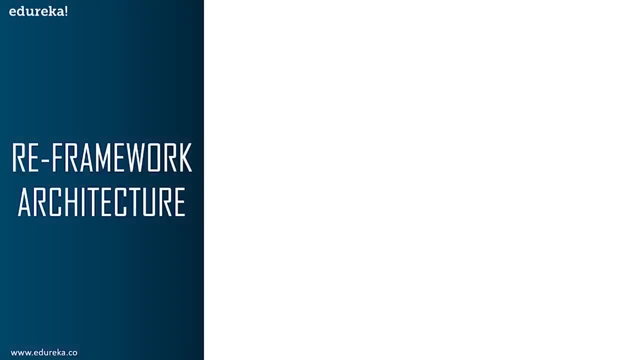 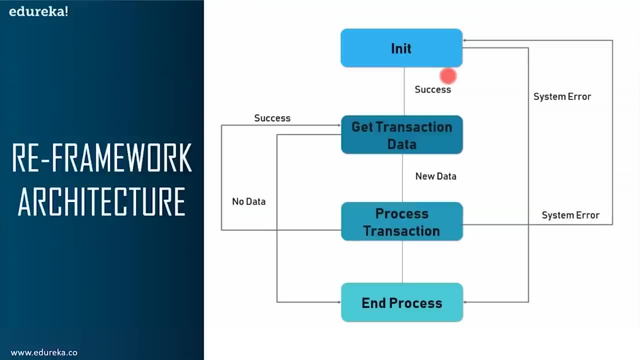 So now, before I move forward with the explanation of each and every state in detail, let me just give you an overview of the complete workflow of this re framework right. So any project that you create on re framework basically starts true in state right. 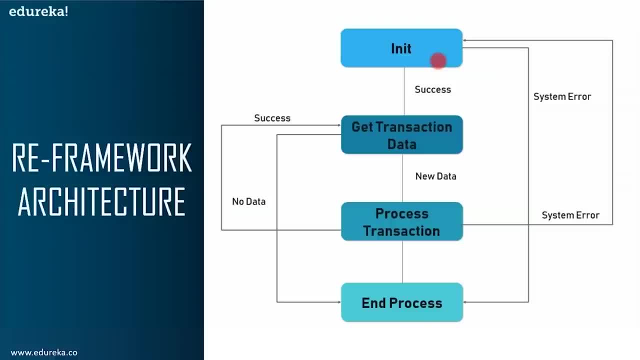 So the init state is basically the state where the robot reads to configuration and initializes the application. So if the configurations can be read and all the applications are initialized, then the state is meant to be successful. So if the state is successful, then it goes to the get transaction data state. else, 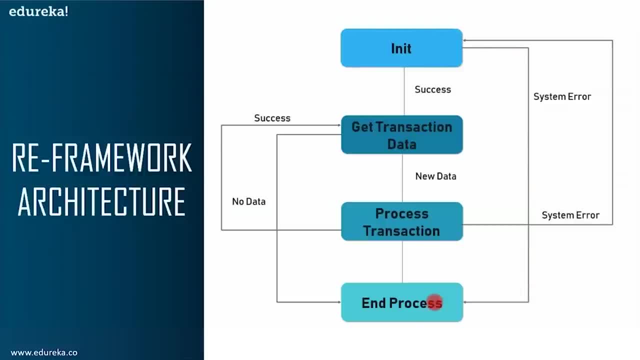 It just directly ends the process by showing you a system error. right now, let's say you know our state was successful, then we would land on to our get transaction data state, right? So in the get transaction data state you have two possible actions. 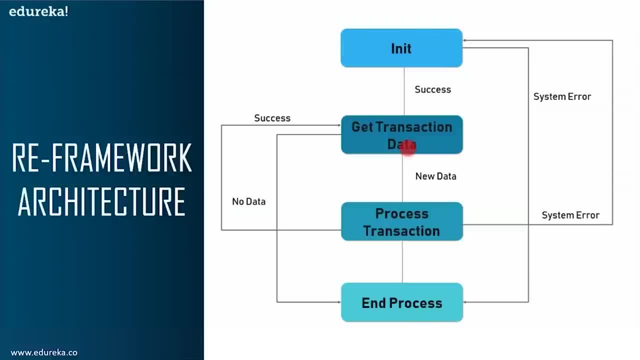 that is, either the new transaction comes into the picture, So basically the new transaction that comes next is processed by the report. So once you know the transaction is retrieved then it goes to the process transaction. that is basically our next day. else, if all the transactions have been operated, 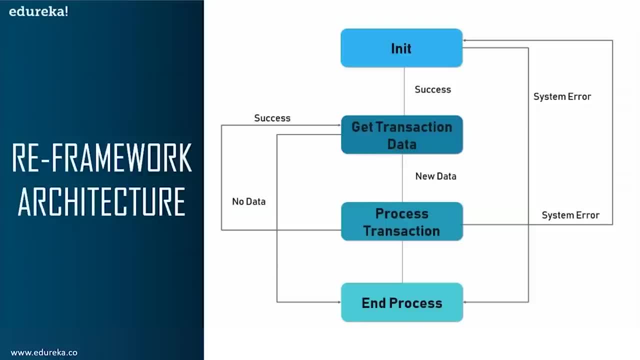 and then there's no more data left, then it basically goes to the end process, right? So there are basically two possibilities that you have to understand in the get transaction data. One is basically if there's a new transaction or if there's any new data that has to be processed. 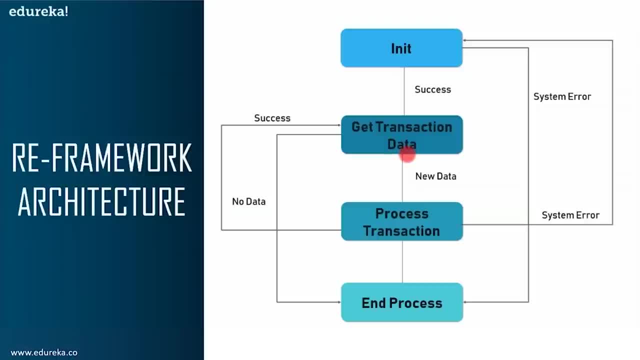 then it goes to the process transaction else, if there's no data, and then all the transactions are taken into account and it directly goes to the end process. but the process end right now. let's say you know we are in the process, transaction state now. 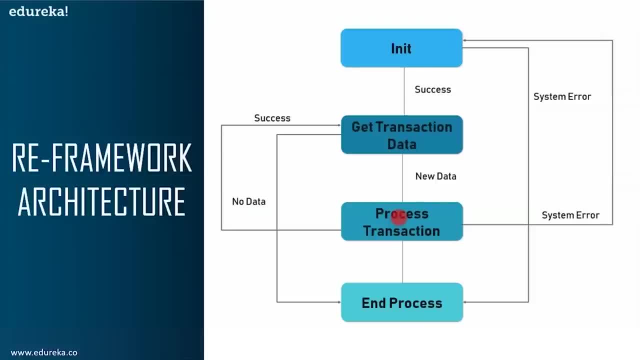 in the process transaction state. There are again three outcomes that can come. that is either the success, the business rule exception or the error transition right. So the success is basically where the loop is performed and the next transaction data is taken into account. So if you remember when I was explaining you, 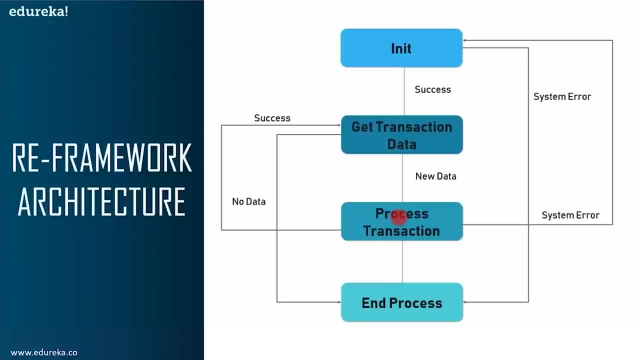 about what this reframe work. I was telling you that when the setup is initialized and then for each loop some actions have to be performed. So that particular part where we are defining for each loop that is basically happening in our process transaction state, and where we are talking about setting up our basic requirements. 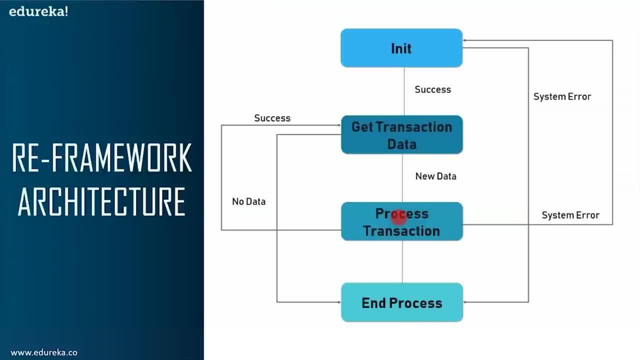 that basically happens in our init state, after which we basically get the transaction data right now, as I was talking about the process state. So, as I just mentioned, the success state is basically used when the loop is performed and the next transaction data is taken into account. moving. 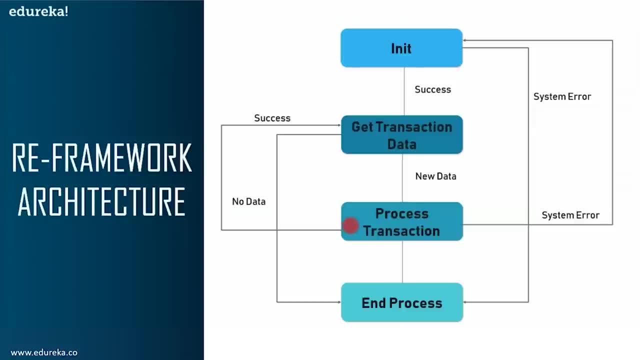 on to the business rule exception. So, in the business rule exception, some specific action needs to be taken, after which the execution loops back to the get transaction data state right. apart from that, coming to the third one, that is, the system error transition, This is through which you can take all the necessary steps. 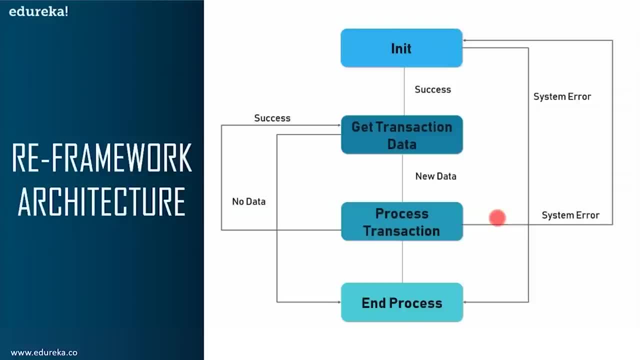 to receive from an error, right? So basically all the applications are closed and the execution loops back to the init state, right? So when all the applications are closed and the execution loops back to the init state, basically in the init state again, since the applications are initialized, the applications 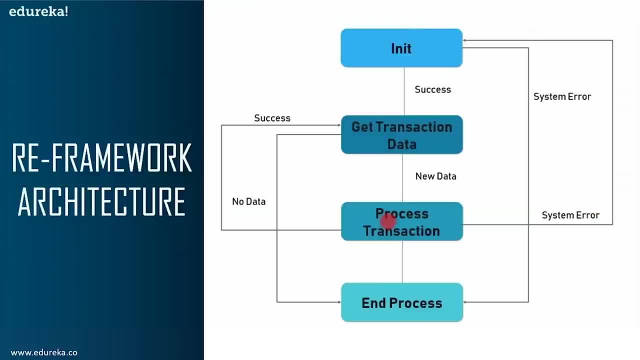 are restarted right. after all the actions that perform over here, We finally have the end process, which is basically used to end the process right. So I hope you have understood the workflow of the re framework right. Let's take a look at all the four states of the re framework. 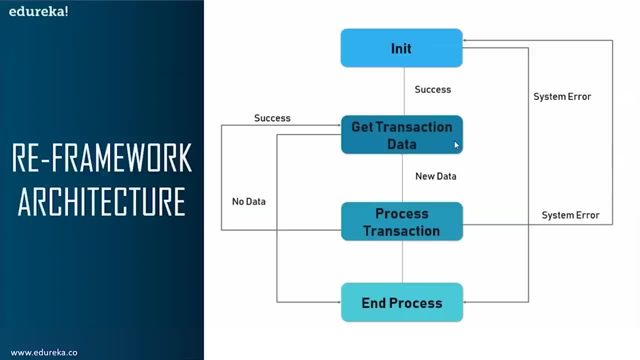 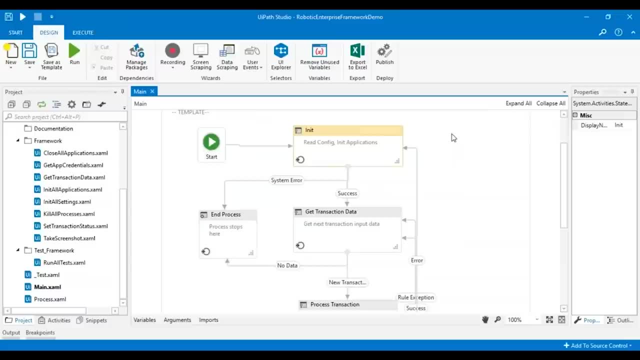 That is the in it get, transaction, data process, transaction and end process. Let's start by taking a closer look at the init state. So let me just quickly shift back to uipath studio, right. So now, if I just double click on the init state, 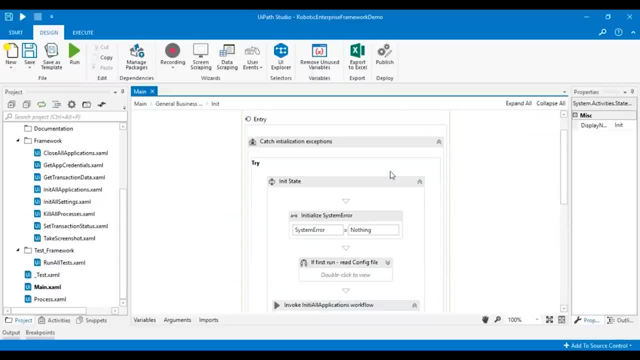 you'll see how it expands, right? So basically, as I was telling you, the init state is used by the robot to read the settings and start all the applications. So this is basically where the robot reads all the configuration that you must have mentioned and then it initializes all the applications required, right? 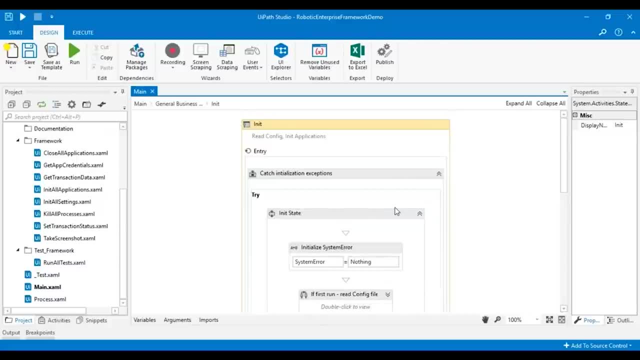 So, as you can see, we have the exception handling schema placed inside each framework. So this is why, basically, we have the try-catch blocks presented each and every state. So here, what happens is that, basically, the robot will try to initialize and if it fails to, then the process will end right. 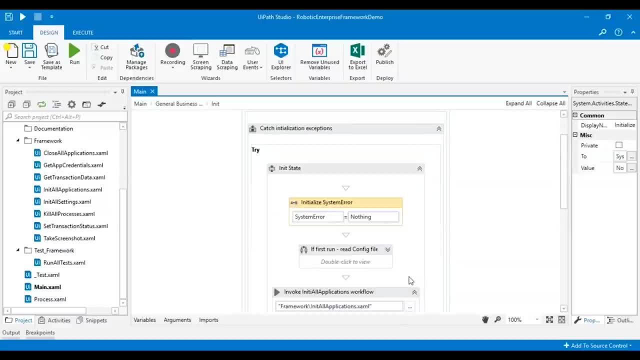 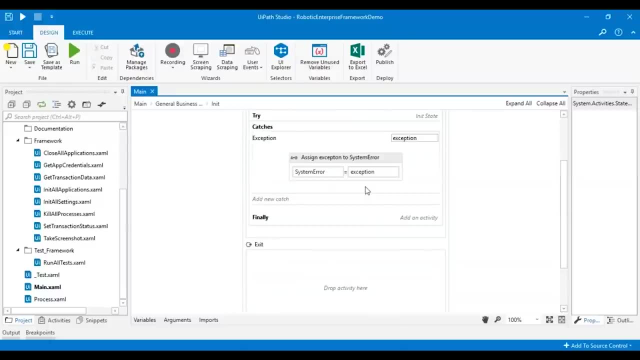 So, basically, whatever we are mentioning in the dry section is to initialize the actions and then, if the actions are failed to be initialized and it directly just ends the process, right? So it just gives you an exception and then it finally just ends the process, right? 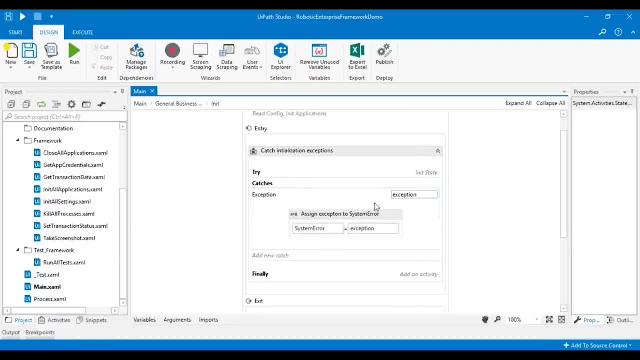 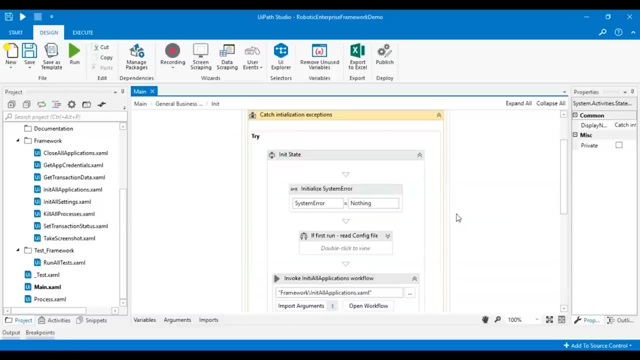 So if I just scroll up then you can clearly see that you know, in the first section that comes- that is the price section- What is mentioned is initialized system error. So basically that's an assign activity that is used. So this is used to basically check. 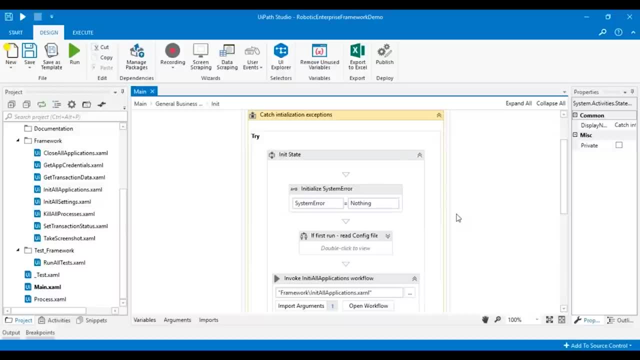 whether there's an exception or not. So for that we set the exception object to the system error and then we just initialize it with nothing, right? So basically, over here we're just initializing a system error variable to nothing after that, as I just mentioned, 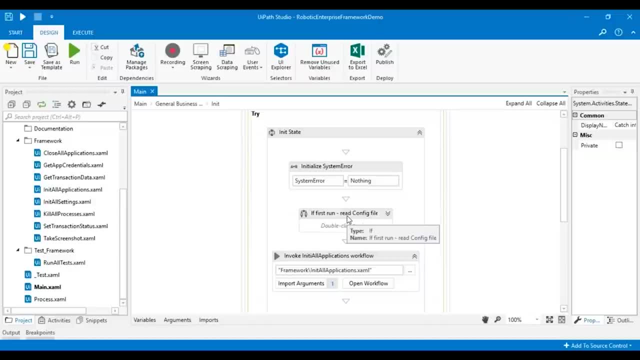 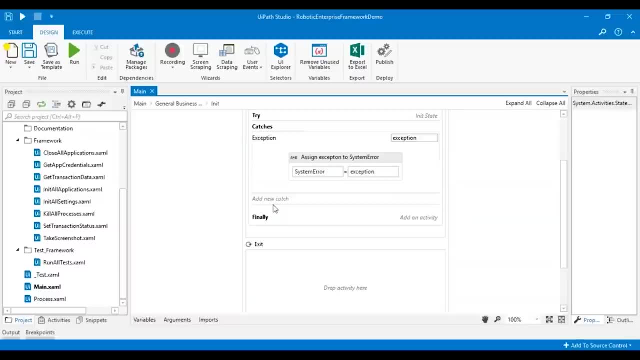 that the reward has to read the configurations. Our next step is to read the config file and then start all the applications And finally our step is to basically catch any exception that comes into pictures. So over here that's what is mentioned. that is basically an assign activities foot. 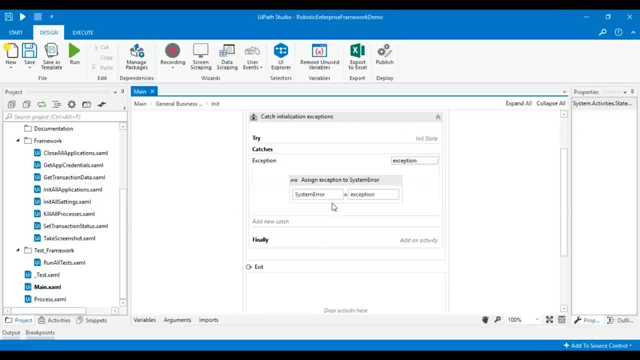 and then the system error is assigned to the exception value and the exception type to be any common exception right. So, depending on the value of the system error, that is basically the variable that we have assigned in the try block and also in the catch block. 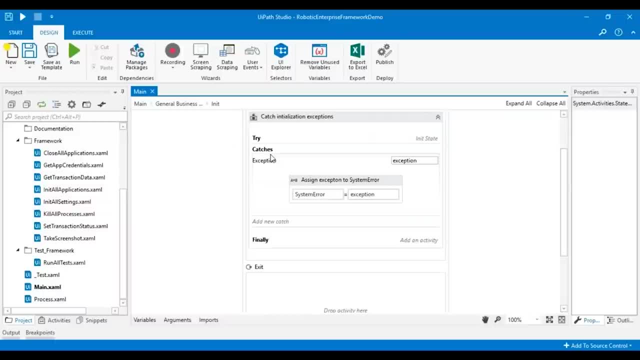 So, depending on that particular value, what happens is that either you go to the next day- that is, the get transaction data state, or basically the process ends right. So if it is successful, then it goes to the get transaction data state, as you can see over here. 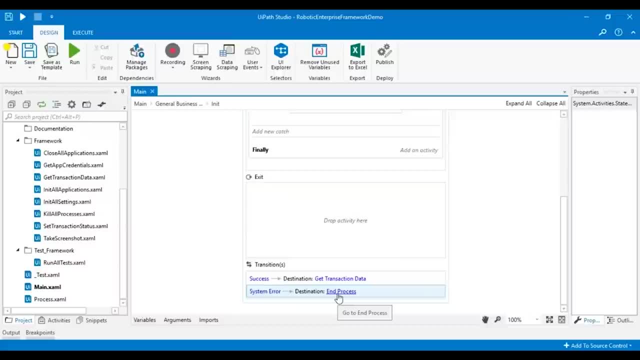 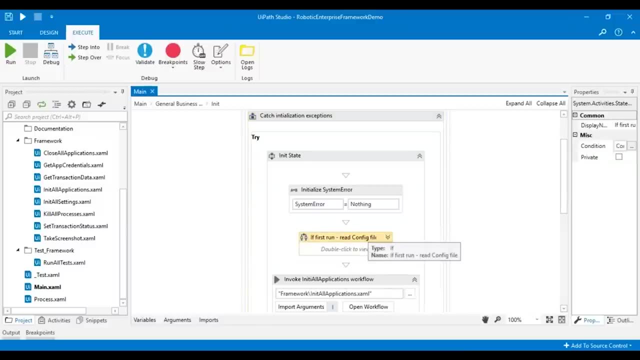 if it is not successful and then there's some error throw, then it basically ends the process right now. Let me just quickly scroll back over here again and then let me give you a better understanding about reading the configuration file. So over here, if I just double click you'll see that. 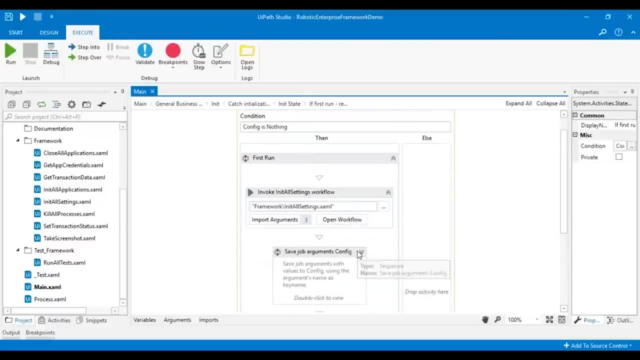 you know, it again opens a different sequence in which you have various other options. So, basically, if you have to just understand the step, then you can just understand by the fact that you know the step is used to read the configuration file. now, reading the configuration file only happens. 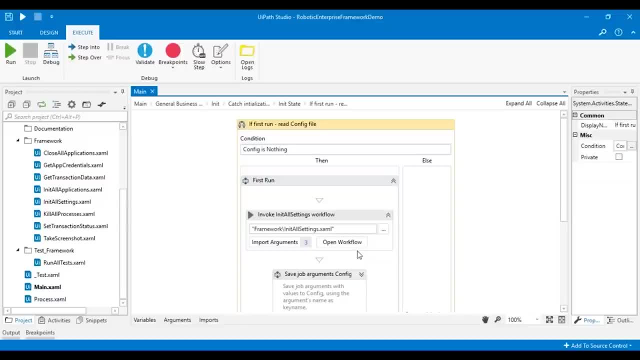 at the beginning of the execution. So basically, when the configurations are read by the robot, then that is basically done at the initial state of the execution. only it doesn't happen at the end, because it's obvious that you know the robot doesn't understand the configuration. 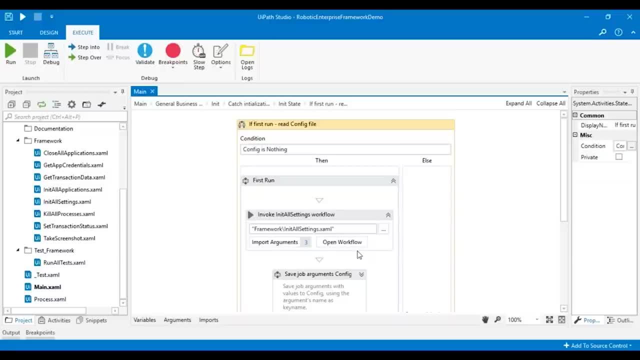 then obviously execution cannot happen, right. So that is the reason this happens at the beginning. Now over here, if you observe, there's an if condition. that is mentioned. so over here it is mentioned that you know the config is nothing. now, if you look. 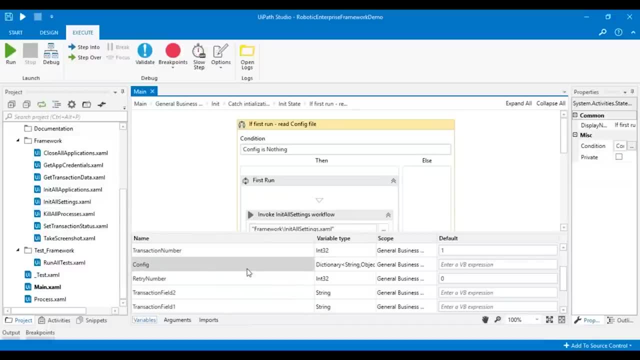 into the variable pane of this particular section, you'll see that you know the config is available. So it's basically a dictionary and then the dictionary has the string and the objects. So the string is basically the key and the object is basically the value of the dictionary. right now. 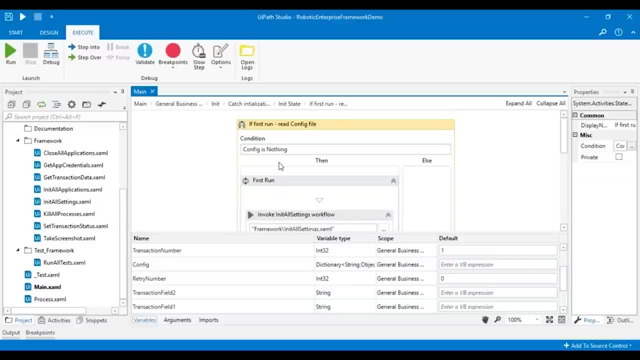 in this particular dictionary. that is basically in conflict. You can store any kind of data, like you know: number, string data, time values and so on. right, So now, when you mention the condition that you know the config is nothing, you move on with the next step. 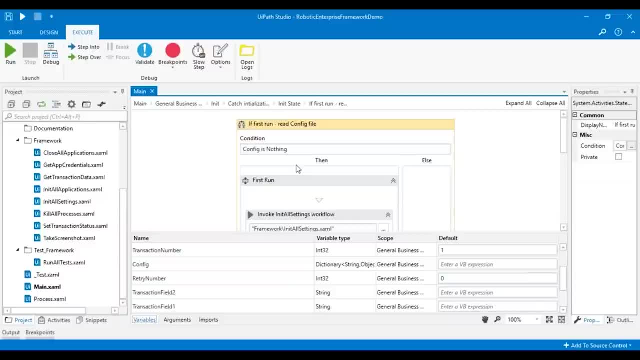 that is basically, if this condition is successful, then then section of the if condition is executed. So in the then section, what your first step is? to basically invoke the in it all settings to XAML file, right? So this basically happens from the framework folder. 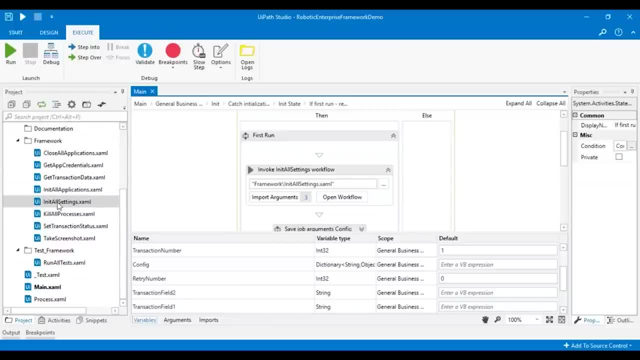 that you can see on the left hand side. So we hear this is basically the XAML file that is being invoked right now over here. If you observe this particular activity, you also have you input arguments right. So if you just double click over here, 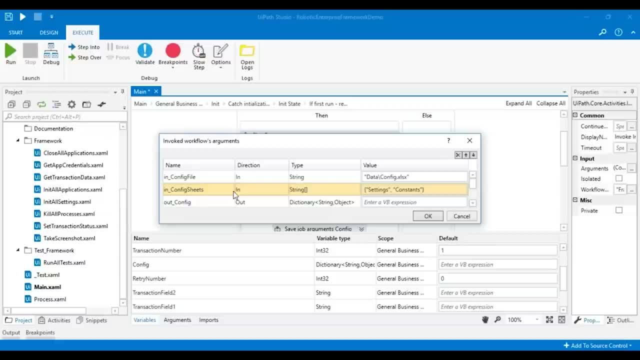 you'll clearly see that you know you have to input arguments. That is, the in config file and the in config sheets. Now, the in config file basically consists of the path of the configuration file located in the default data folder and the in config sheets indicates the sheets. 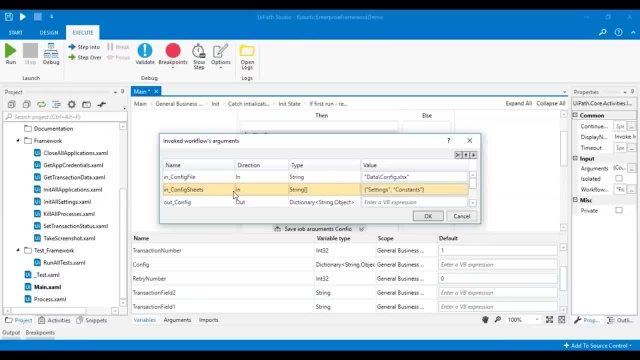 which contain the configuration data right. So that is basically the different sheets present in the configuration file, And also those particular sheets have the configuration data right now. apart from this, We also have the output arguments. Now the output argument is again the out config. 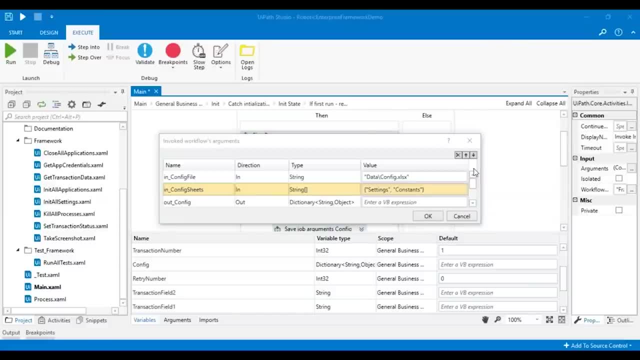 which is a dictionary value again, in which the spring is the key and the object is the value right? So if I just click on, okay, this gets closed right now. before I move on with the next activity, Let me tell you over here that you know. 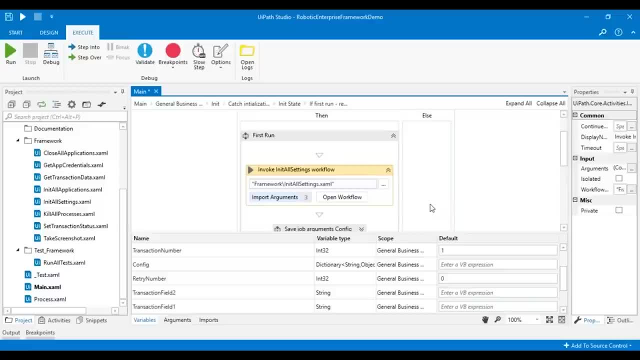 the in it all settings. that XAML file is basically the plug-and-play, so you basically don't have to change anything in this particular file when you're working for your business process. It's got to be the same for each and every business process and then you don't have to configure much. 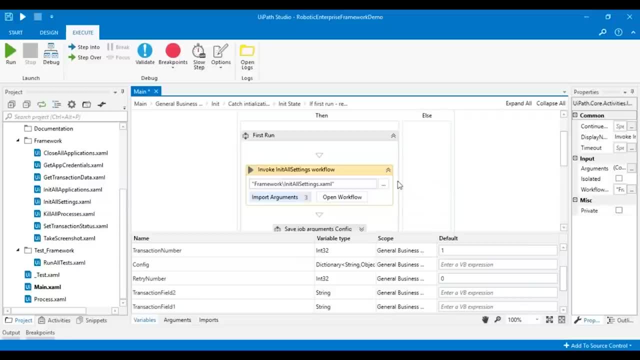 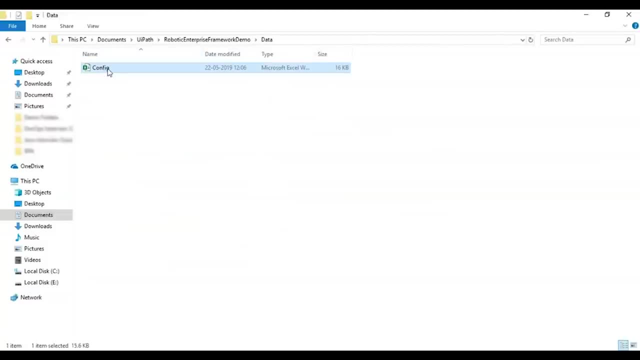 about it, right? So, as I was talking about the configuration file, so before I move forward, let me just open the configuration file and show you project folder, is this? So if I go to data, you see the config file over here, right? 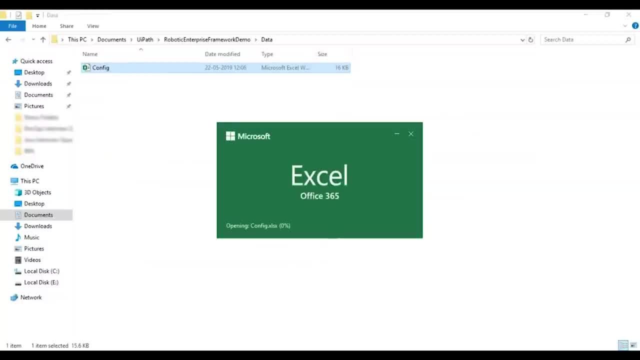 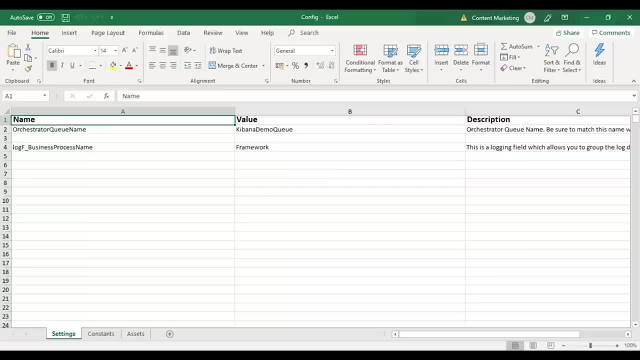 So if I just double click over here, you'll see that in its opening. So let's just wait for that to happen, All right, So once it is open, basically, guys, this is how your config file looks. So it basically has three sections. 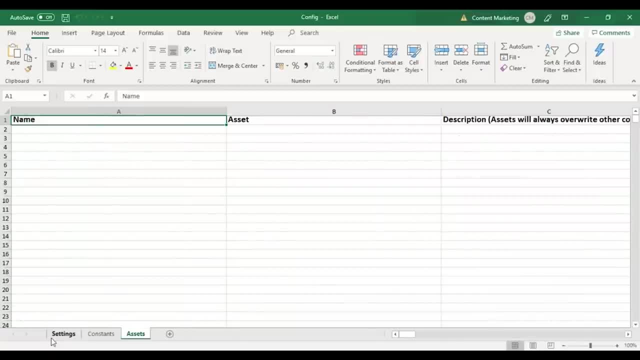 That is, the settings, the constants and the assets, right? So all these sections have their own functionalities and features. the settings is basically used to put any configuration related to the business process, like you know, URL, file pass, credential names or anything which is specific to that particular business process, right? 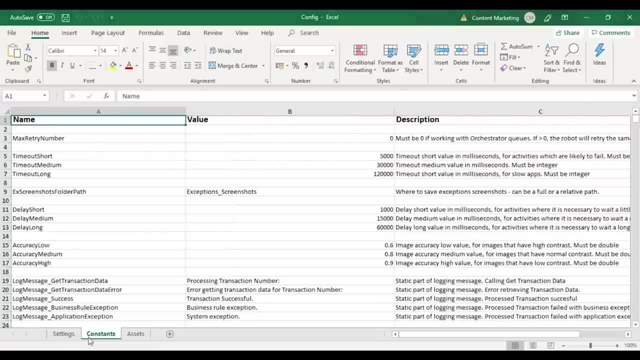 Coming to constants. constants is basically used to store the technical settings for the developers. Like, when I say technical settings, what I mean by that is, you know, you can store the number of retries, timeouts, delays, image accuracy settings, static log message bars and so on. 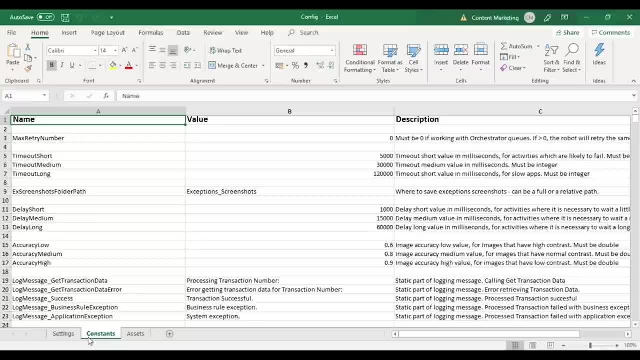 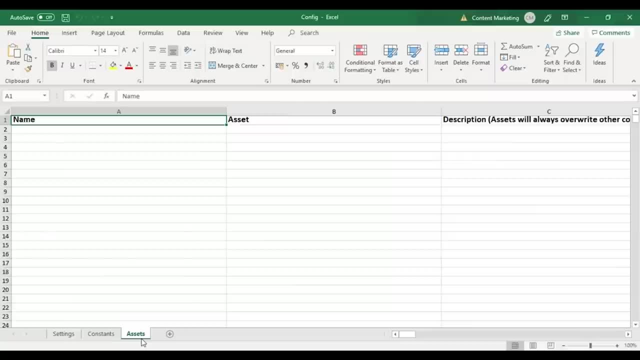 Right. So basically, the constants part is basically used to store the technical settings for the developers. and finally, coming to the assets part, So the assets part is basically used to store the values which override the default settings. right Now, if I just shift back to the settings part over here, 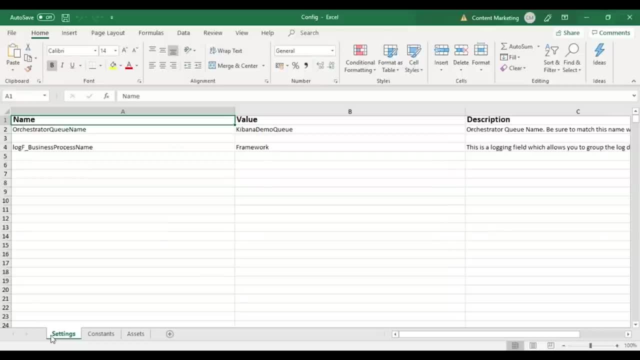 you basically see three columns right. That is the name, value and the description. So the name basically always contains spring. that is the key in the dictionary. So, if you remember, I was talking about the config variable, right? So the config variable was a dictionary. 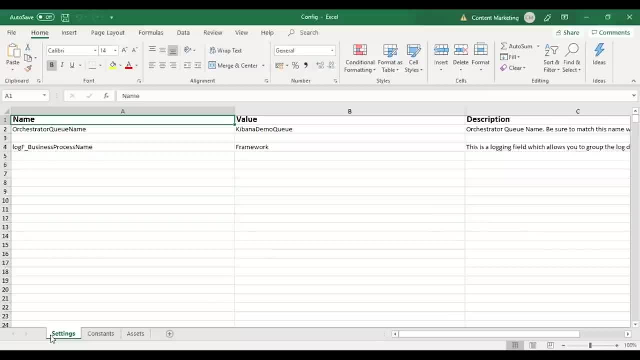 in which we had string and object and the string was a key right. So basically, whatever is present in the name folder is considered as a string and that is present in our key section of our config variable. coming to value, the value holds the dictionary value. 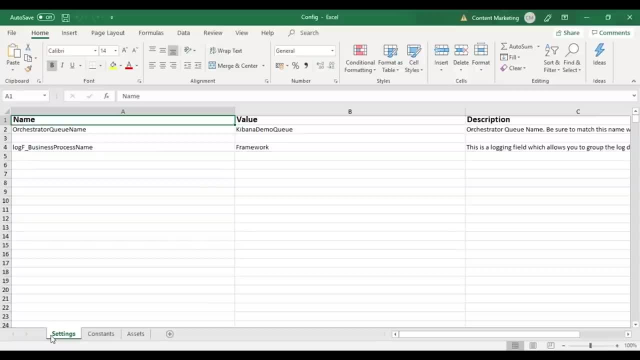 So, in the config variable, whatever was object is basically our value. and finally, coming to the description, So the description provides a detailed account of each and every spring. right now, moving on to the next sheet, that is constant. So the constants, as I was telling you, basically consists: 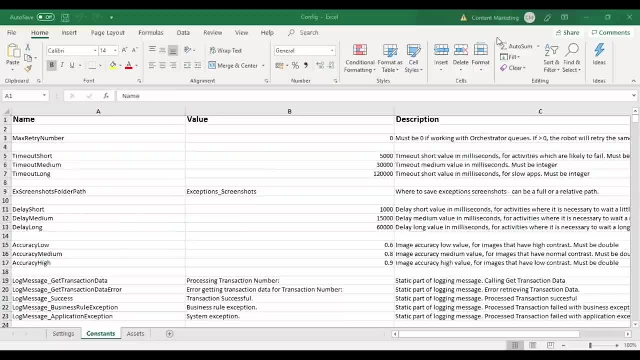 of the technical stuff that is required for the developers. So these are basically used to avoid hard coding and time delays. So these config objects basically allow easy global value adjustments. right, You can just, you know, define the configuration over here and then you don't have to define it again. 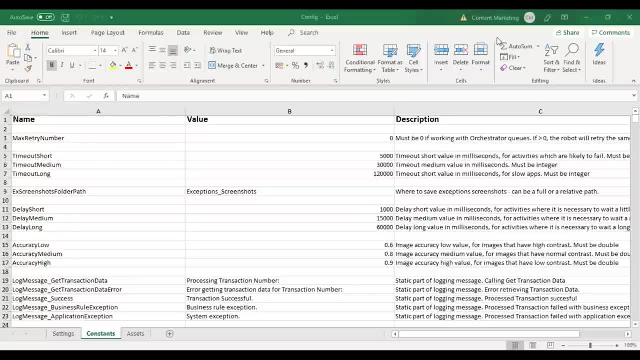 and again and again. right, So with these we can improve the performance and also find you in the projects for different environments. right Now, if you observe the columns, then again it has the same columns. that is the name value in the description. 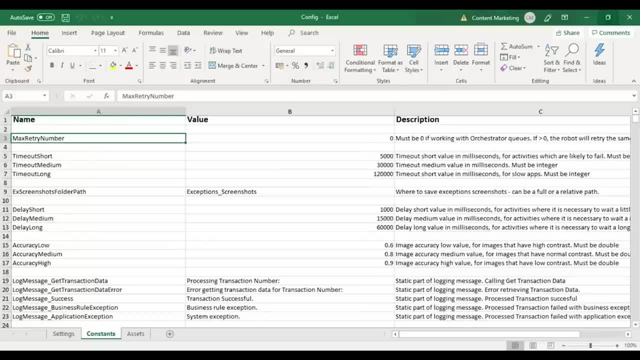 So, for example, if you just consider the max pretry number, the max retry number is basically used to keep account of the retries of the transactions which have failed due to an application exception or a system error, right? So, since we're using the template of the reframework, 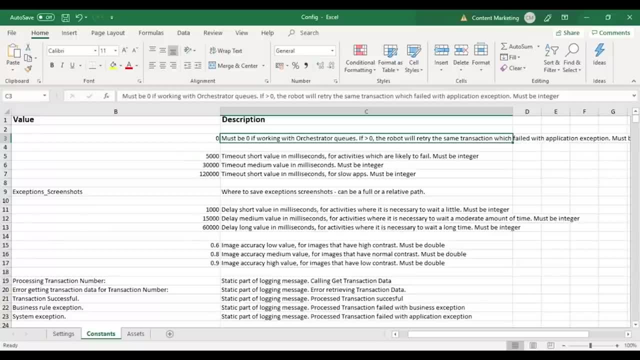 and this template is basically designed to, by default, work with the orchestrator queues, but then it can also be used to suit other types of input data, as the can, Excel, email folders and so on. right, So by default, the max retry number is assigned to 0. 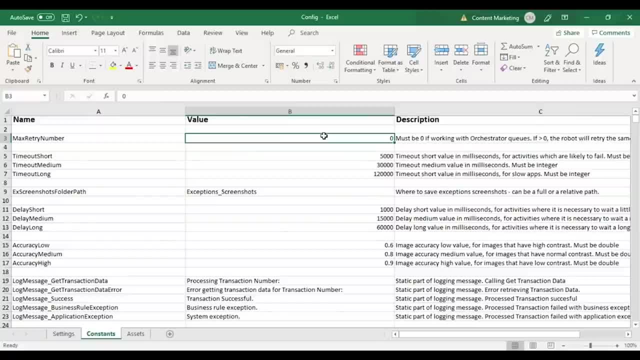 and the number of retries is set in orchestrator. Of course, this number can be changed, allowing the robot to retry the field transactions If the queue functionality does not work right. apart from that, We also have others such as timeout- short, timeout, medium, timeout, long. 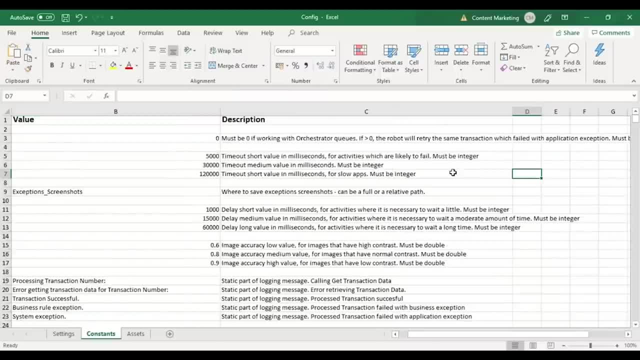 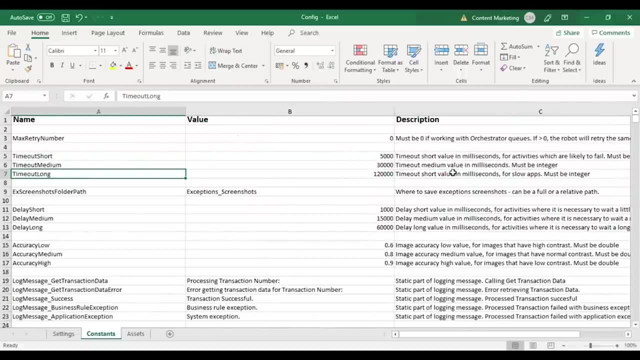 This is basically used to find out the timeout value in milliseconds for the activities which are likely to fail. So they basically have a limit. So the timeout short has a limit of 5000, the timeout medium has a limit of 30,000 and the timeout long has a limit of 1 lakh 20,000,. 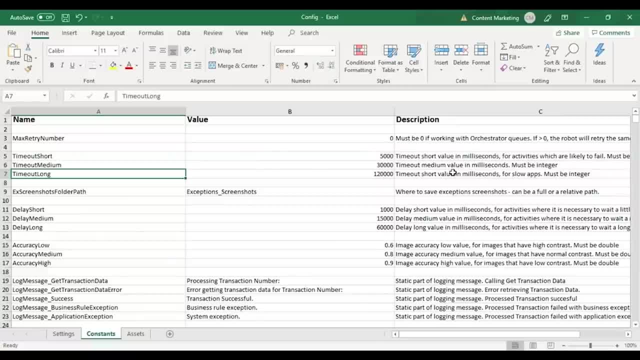 right After this we have the X screenshots folder part. So the X screenshot folder part is basically used to save the exception screenshot and that particular screenshots can be used to solve out the exceptions If any exceptions occur in a business process coming to delay short, daily, medium and delay long. 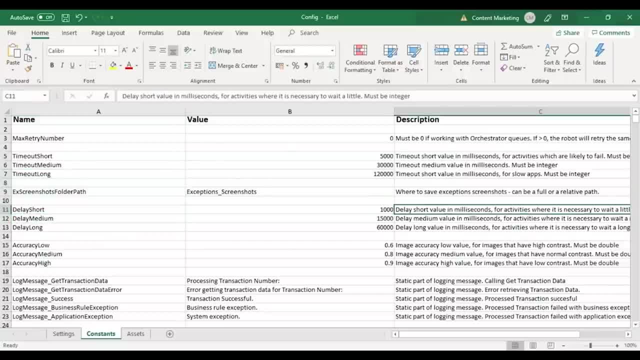 So the delay short, daily medium, daily long is basically used for the activities where it is necessary to wait for a little while, right? So again, the delay short, delay medium and delay long basically have their own limits. So the delay short, as you can see, 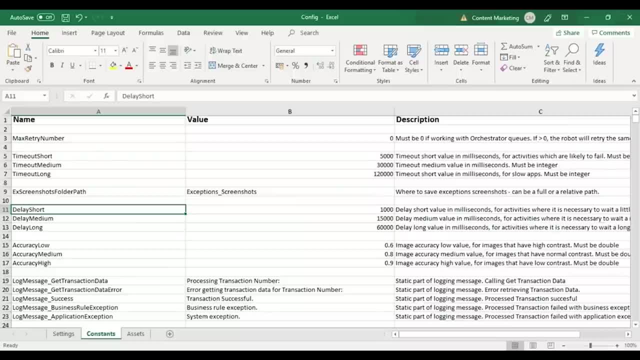 has thousands. really, medium has 15,000 and delay long has 60,000. right after that We have the accuracy low, accuracy medium and accuracy high. So this is basically used to define the image accuracy. So either the image accuracy can be low, medium or high rise. 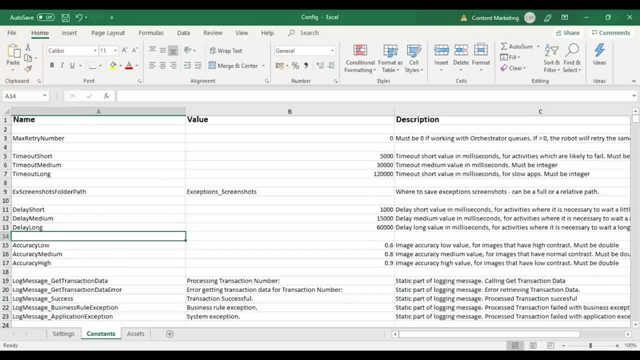 So the images which have high contrast basically have accuracy low. the images which have a normal contrast, which have accuracy medium and the images which have low contrast, have accuracy high, right. So again, these particular strings have their own value set. So the accuracy low is at 0.6, accuracy medium is at 0.8. 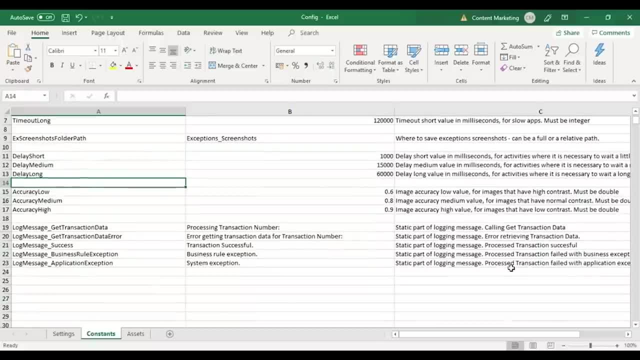 and accuracy high is at 0.9. and finally, coming to the log message: get transaction data. log message: get transaction data. error success business rule exception and application exception have the functionality of static part of logging message. So the first one, that is the log message: get transaction data. 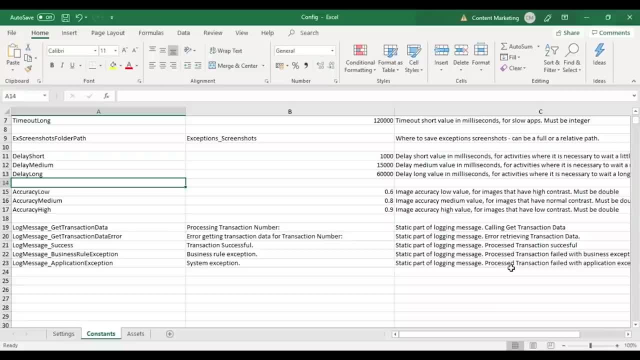 is basically used when you call the get transaction data and that particular processing transaction number value is stored. coming to log message: get transaction data error. This basically logs the error retrieving the transaction data over. here We basically store the error getting transaction data for transaction number. coming to log message: success. 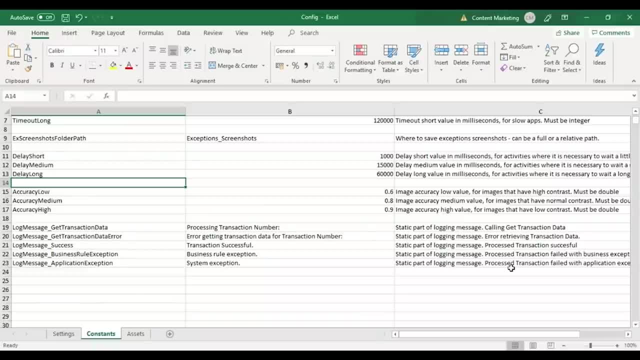 So the log message Success is basically used to process the transaction successfully. So whatever transaction is successful, that particular transaction value can be stored. coming to log message business rule exception, This is basically use to log the part where the process transaction filled with business exception. 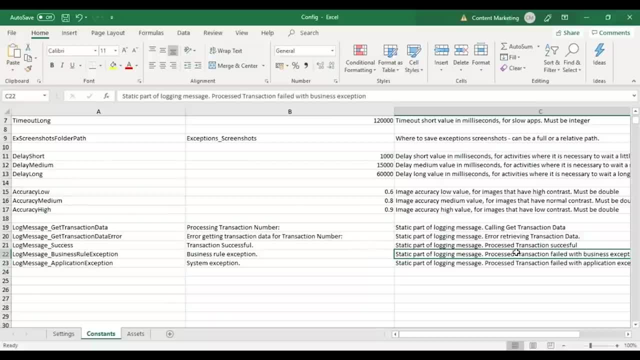 So we are, you store the business tool exception. finally, coming to log message application exception. So the log message application exception is basically used to log the message of process transaction failing with application exception, right. So over there, you store the system exception, right. 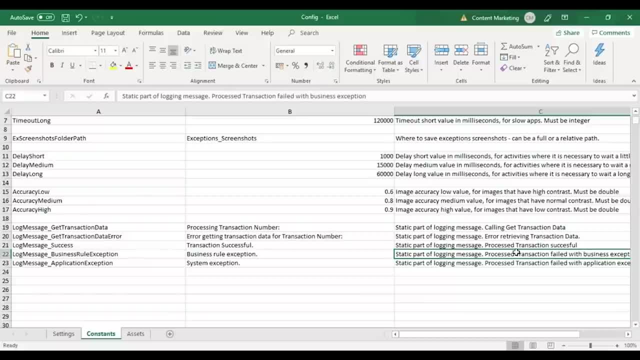 So, basically, guys, this was all about the config file. So, guys, with this we come to an end to understand the config files. over here We understood three main sheets that the config file has, that is, the settings, constants and the assets. right now, once the config file is basically read, if you move back, 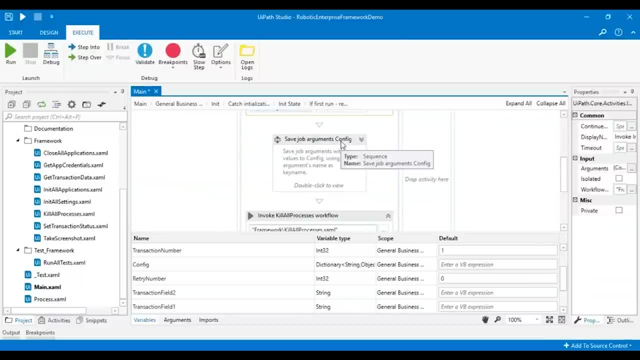 to our uipath studio. the next step that comes into picture is to save the job arguments config, right? So this is basically used to save job arguments with the values to config using the arguments name as a key name, right? So if I just double click over here, you see that you know. 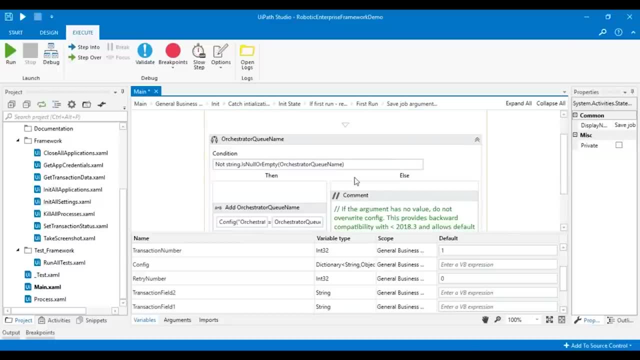 we have an if condition where the if condition says: not spring is null or empty. and then you mentioned the orchestrator Q name, right? So as I was talking about the configuration file, so once the configuration file is read and then the robot understands the arguments. 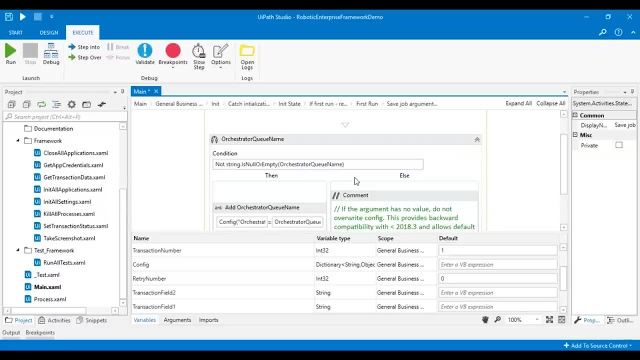 which need to be considered. it basically saves the arguments over here, right? So it basically keeps adding all the arguments to a dictionary with strings and objects as key and value, right? So that is basically happening in the den condition where we are basically assigning the config orchestrator Q name. 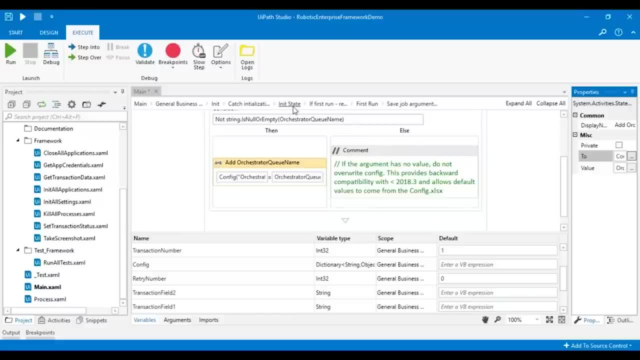 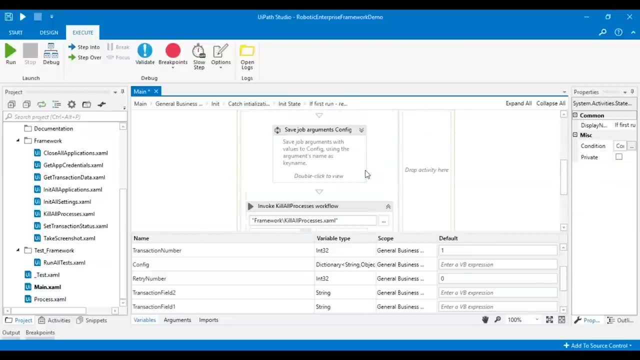 to the orchestrator Q name value, right? So that is what is basically happening over here. Now, if I go back to the init state and then if I go back to the read config part over here, the next step that we see after save job arguments: config. 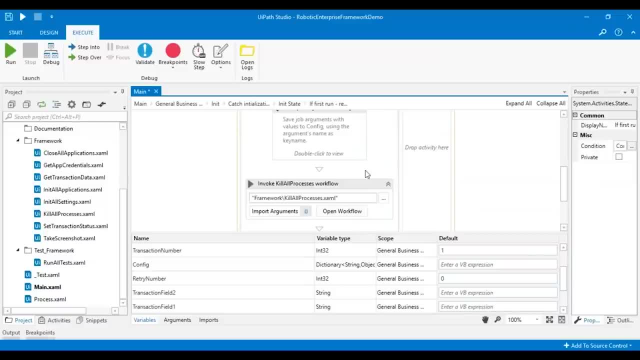 is basically to kill all the processes, right? So basically, we are invoking the kill all processes- XAML files on the framework folder again. Now what happens is that the robot has to start in a clean and a concise environment, right? So what you do is you add the log fields. 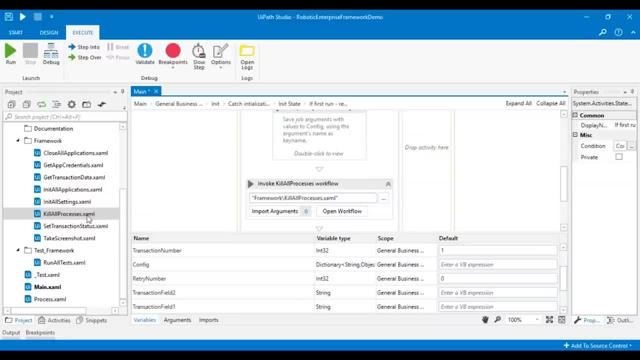 that is, add the business process name to store the log of the process. So whatever processes are not working and then they're not for further use are basically killed. So it's really simple. You just have to go by the name. that is to just kill all the processes. 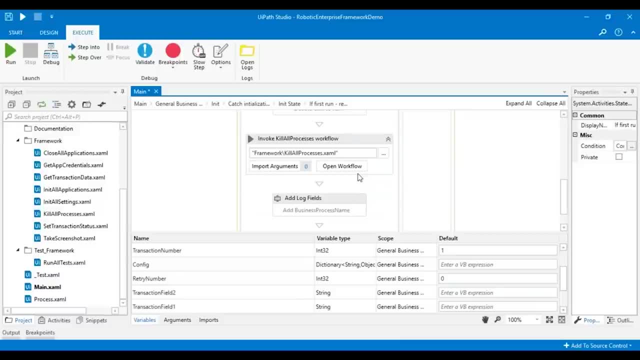 after you kill all the processes. next, What you have to do is you have to add the log face. So the add log fields is basically used to add the business process names. This is used to log the data: what business process is going on? 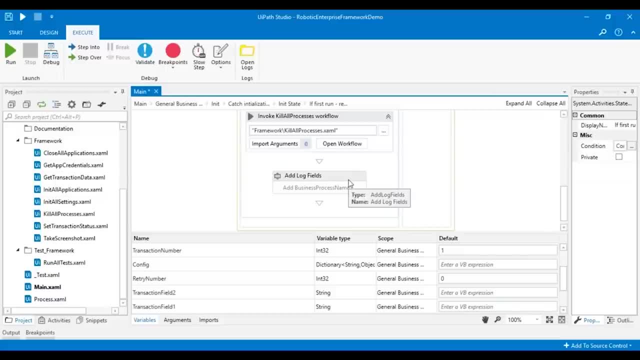 So this is just for exception handling, to understand, if there's any exception, then which business process is creating a problem right Now, once you read all the country file, you kill the process and then you add the log fields. if you go back to the image state, the next stage that comes. 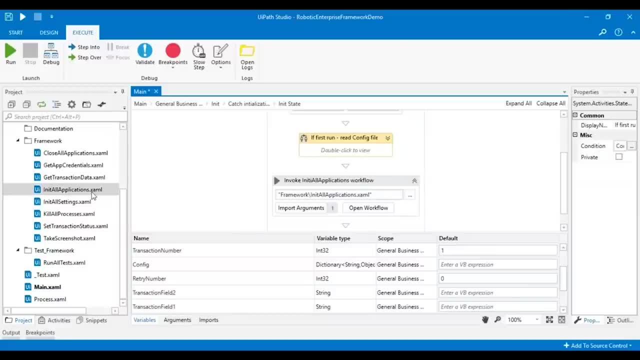 into picture is to in it all the applications, right? So the in it all applications also happens with the XAML file present in the framework folder, that is, the in it all applications. Now, this is where basically all the applications are initialized, or you can understand that, you know. 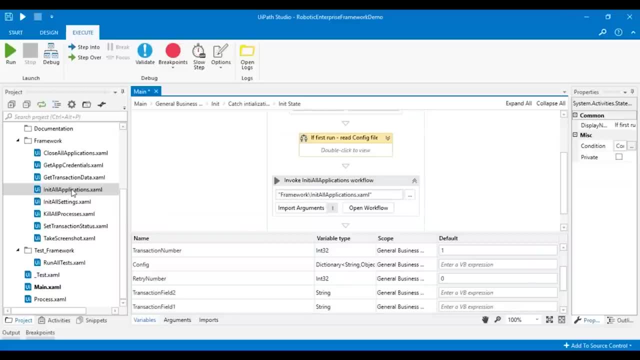 the applications have started. right now, This particular XAML file is basically parameterized depending on what applications are used in the process. So this is where, basically, you'll have to change the configuration based on your requirement. right, It should be basically parameterized on the business process. 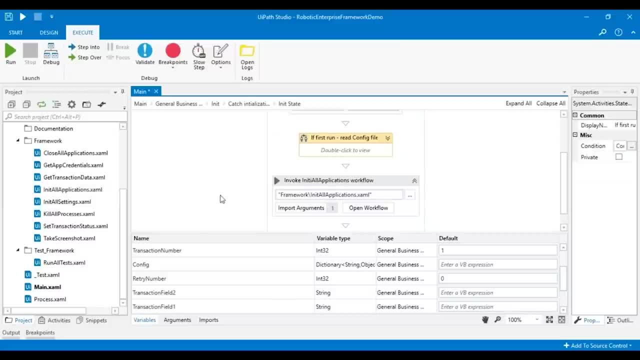 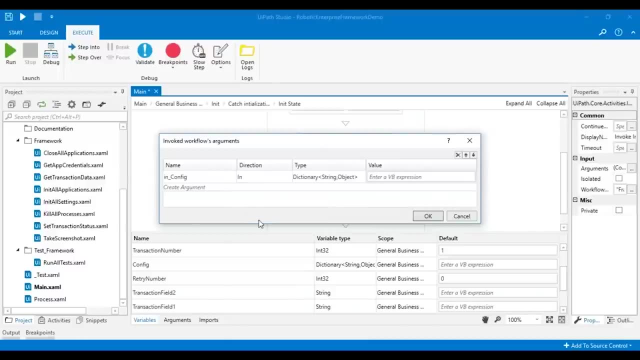 that you have what values that you want to use and so on. right. So over here, if you just see the arguments, then we have the in config value as the input dictionary. So basically it is a dictionary value with the key as the spring and the value as the object. right, 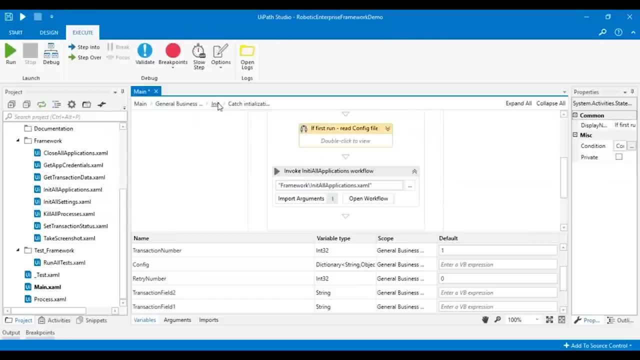 So if I just click on okay and if I just go one step back and then go to in its state- this is where basically are in its state completely ends, And then you know if all these steps are successful, and then there's no system. 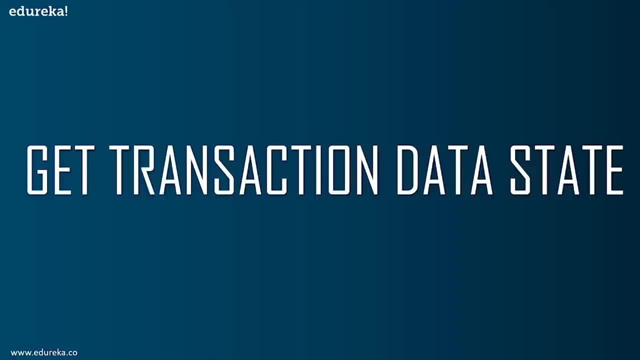 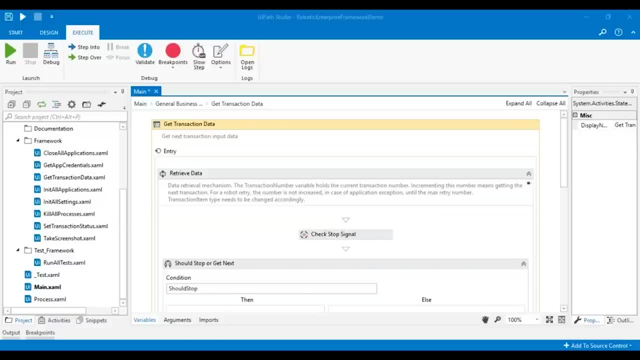 Error. the next state that comes into picture is the cat transaction data state. So the get transaction data state is basically a data retrieval mechanism which is necessary to complete a transaction in a process. So the transactions are basically defined as repetitive part of the processes with each. 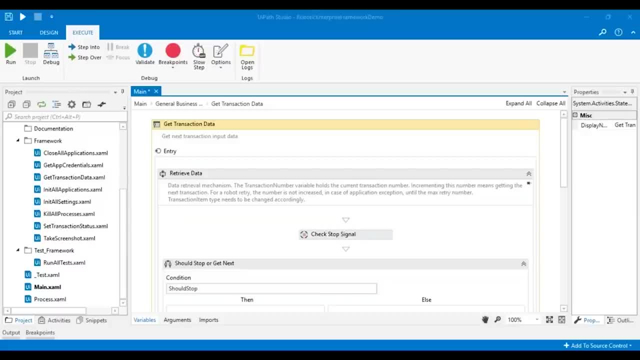 and every execution of the transactions numbered right. So, for example, if you just consider the example of, you know a support system, right, So they have a lot of tickets coming up. right, So each ticket has a different number right. 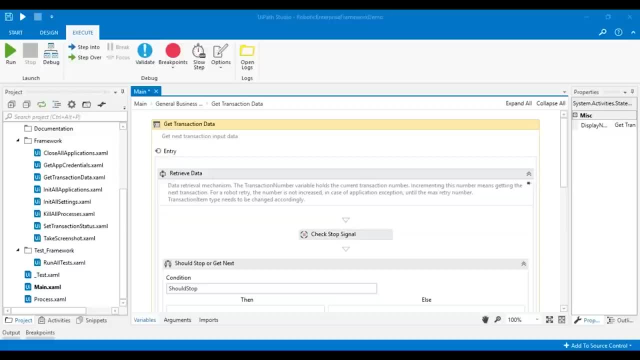 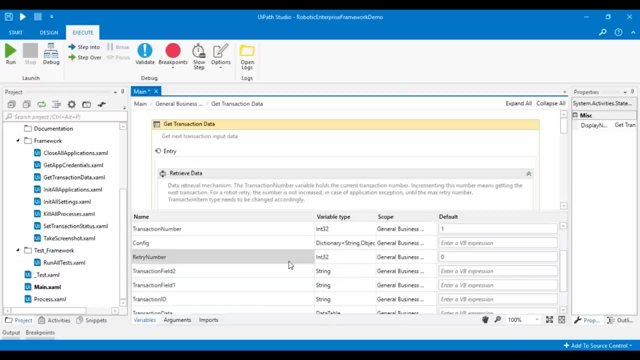 So those particular ticket numbers are unique and therefore they can be used as the transaction numbers, right? So the value stored in the transaction variables is by default one. So if I just drag the variable pane you can clearly see that. you know, the value stored in the transaction number variable by default is one day. 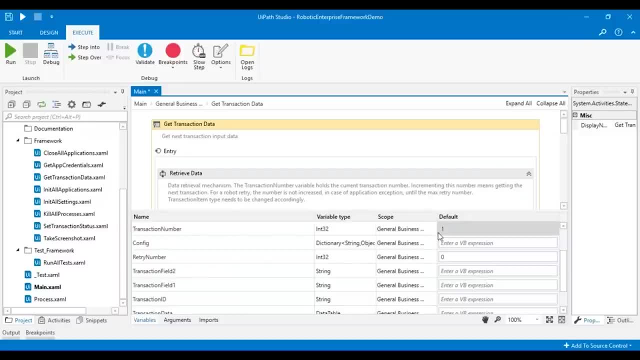 So it starts with one and then it gradually increments within counter right. So the next variable that you have to understand again over here is the transaction item. So the transaction item is a basically a Q Item by default, and then you can change this type of data type. 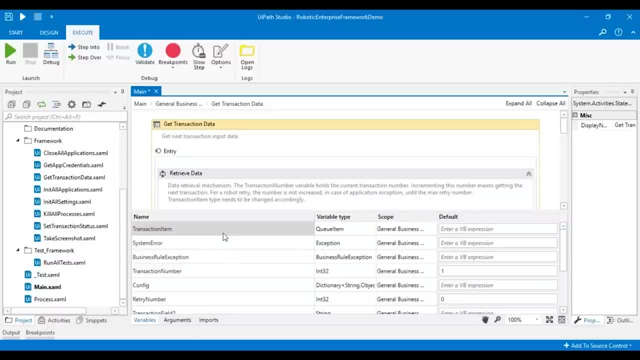 that is, you can make it either email, Excel folders and so on, right, So that's completely your call and based on what kind of business process that you're working on. but by default it has the Q item right Now if you just start with the activities of the get transaction data. 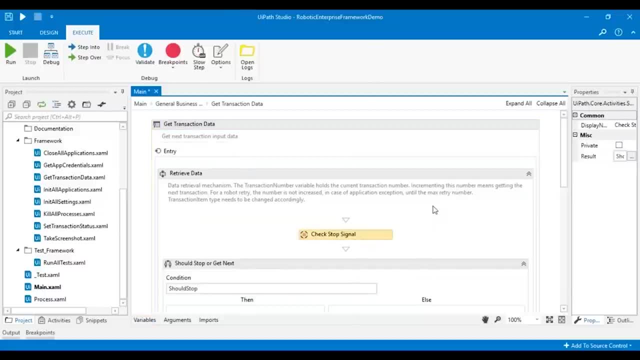 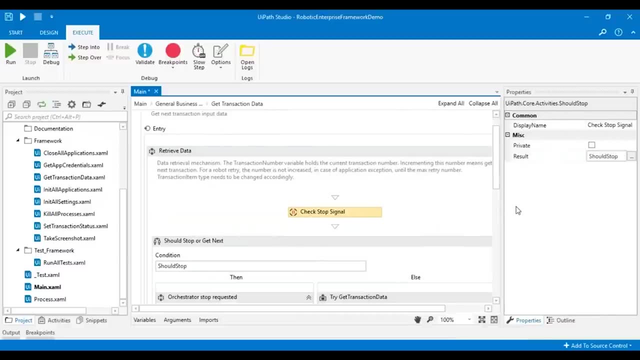 then you'll see that you know, the first thing that comes into picture is the check stop signal. So the check stop signal is basically used to check you know whether our robot is working or not. If you basically stop our report, then it would directly go to the end. tosser state. 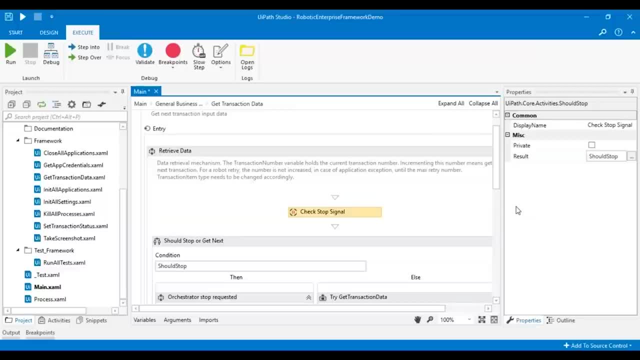 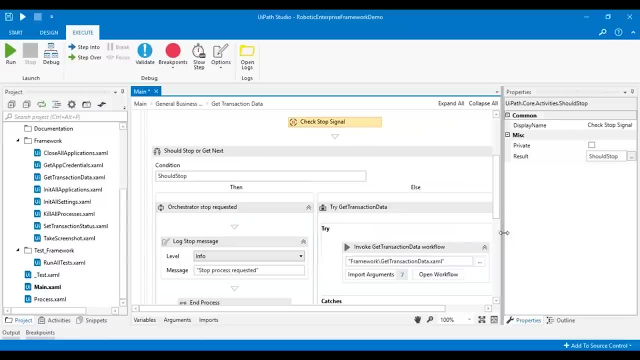 to basically end the process. But yes, if no stop signal is received from the orchestrator, then basically what happens is that we have to perform the further steps in the get transaction data state right, So over here, if you just scroll down. 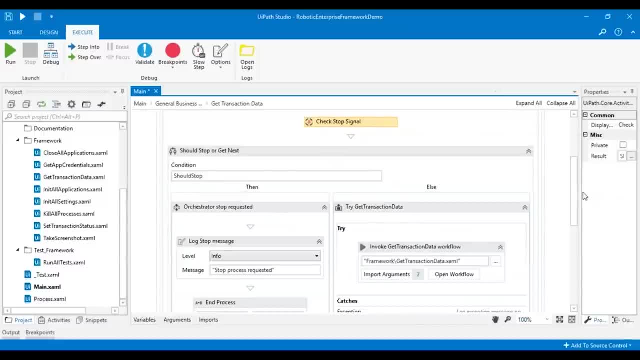 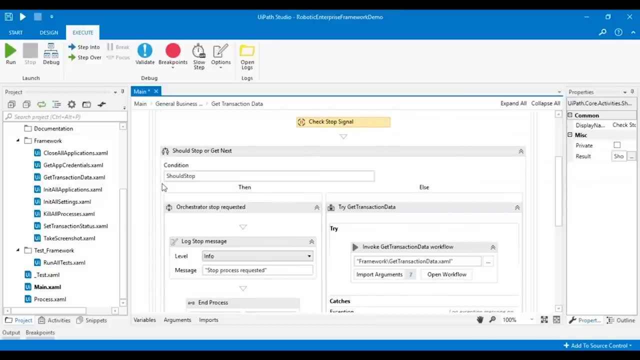 you'll see the condition should stop right. So over here in the check stop signal, if I drag the property section, you'll see that. you know the result is stored in the shirt: stop variable right. So if that particular variable is successful, 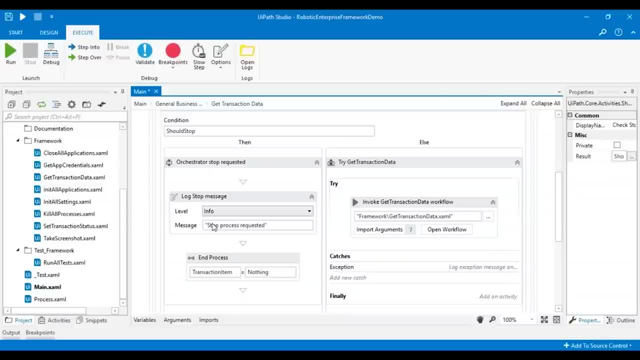 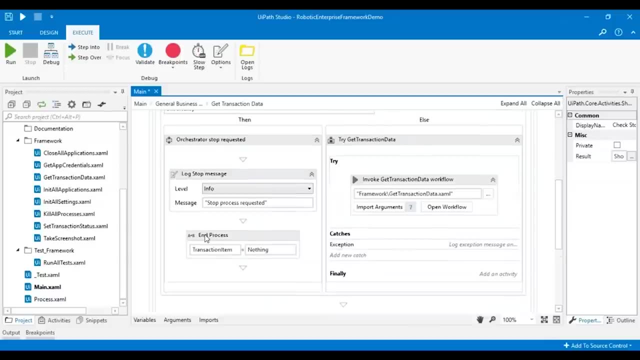 that means our report has received a signal to be stopped. then a log message will come up with saying that you know the stop process requested. So basically, that particular log message will be stored into your log folder and the transaction item will be assigned to nothing, right, apart from that. 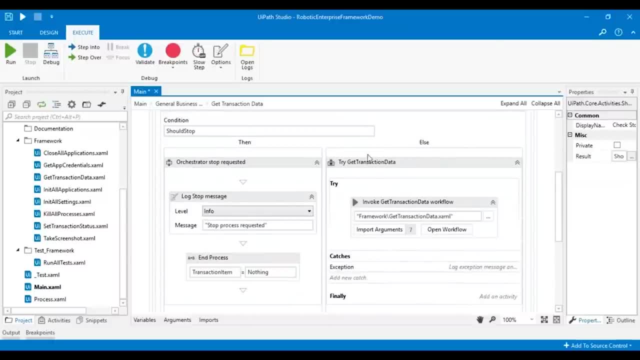 if we do not receive any should stop folder, then you can see the else section will be executed. So in the end section what will happen is that we'll move forward by invoking the get transaction data XAML file, right? So if I just double click over here, 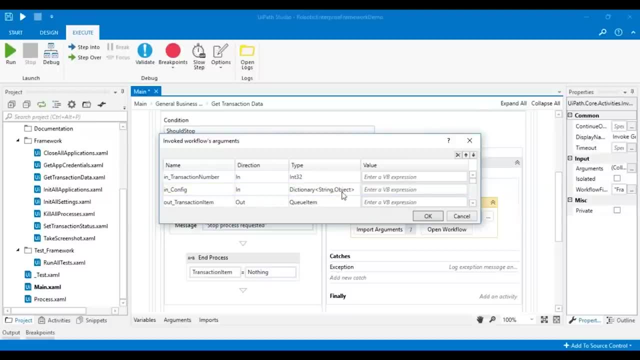 you mainly see two input arguments, right, So that is the transaction number and the config. so the transaction number is an integer data type where you basically store the transaction number, and the config is basically a dictionary, as I previously mentioned, which consists of string and object in the key and the value section. apart from that, 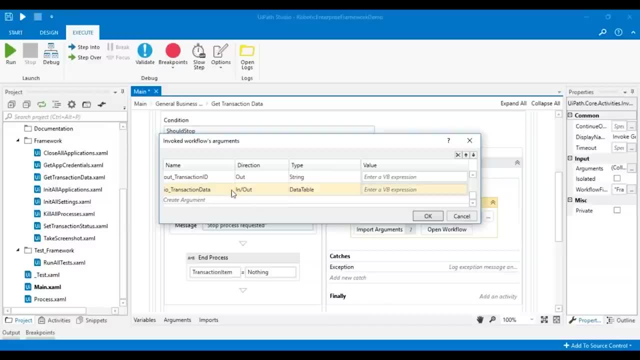 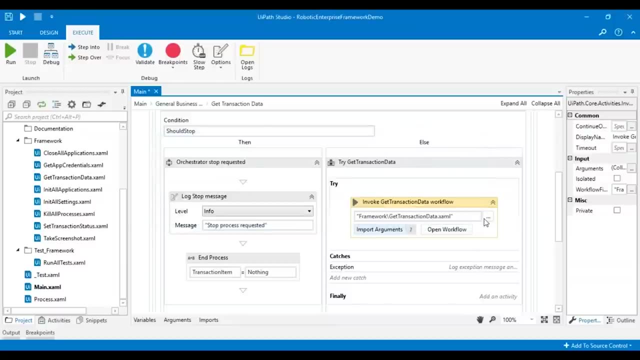 We have the out transaction field, one field to our transaction ID and data, all other as output arguments which are basically used for logging purposes. right, So now if I just, you know, right click this activity and then if I just click on open workflow, 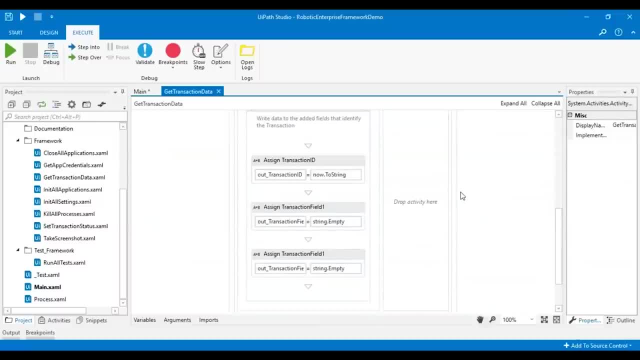 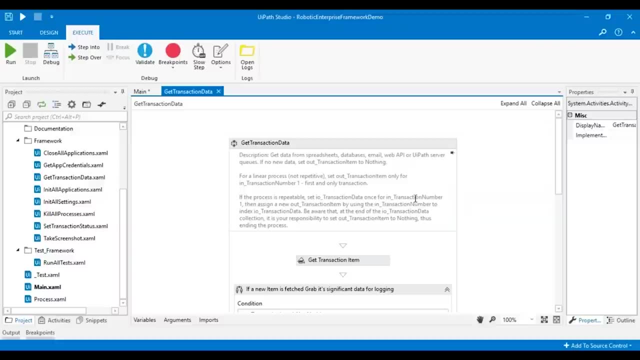 so you'll clearly see that in this opens a different workflow which is stored in that particular XAML file. right, When you open this workflow, you clearly see a description which says that you know this particular workflow is designed to get data from spreadsheets, database, emails and so on, right, 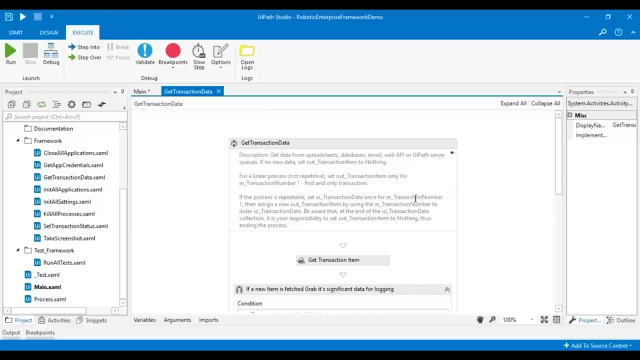 So if no new data is set, then set out transaction item to nothing. if there's new data, then we have to configure over here, right? So for linear processes which are basically not repetitive, the set out transaction item only for one transaction number. 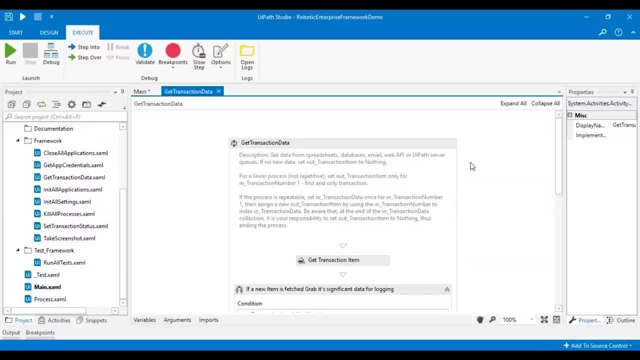 That is the first transaction only. but, yes, if this transaction is reputable, then what happens is that you have to assign a new out transaction item by using the transaction number to index the transaction data, right? So I'm going to show you what's happening over here. 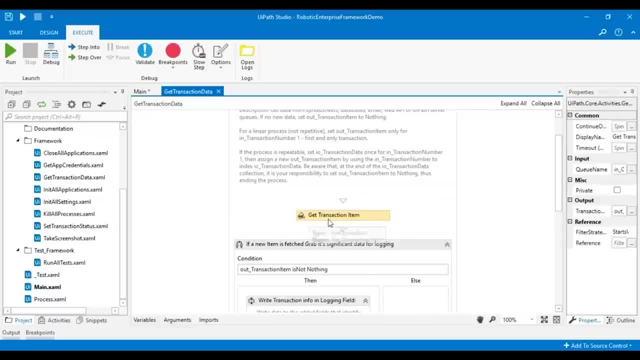 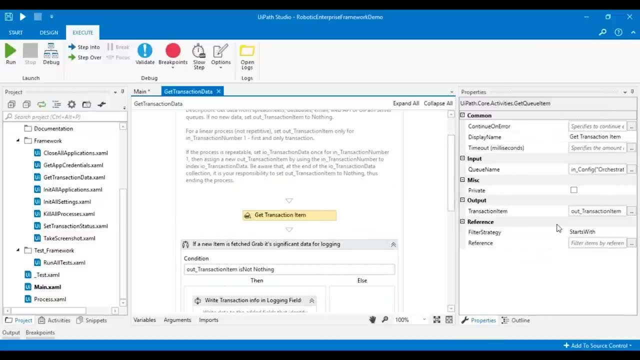 So the first thing that comes into picture is the get Q item, So basically the get transaction item. So in the get transaction item what happens is that if you see the properties section, you'll see that you need the output is basically a cue item. 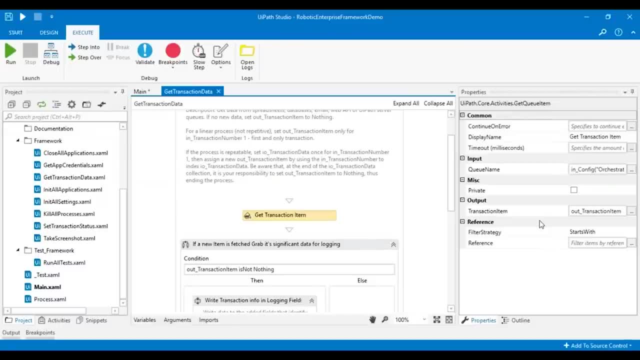 right, That is basically a transaction item in the form of Q. Now this particular transaction ID output argument should be unique for each and every transaction, right? So obviously, if you have around 10 transactions, so this particular ID should be unique for each and every transaction. 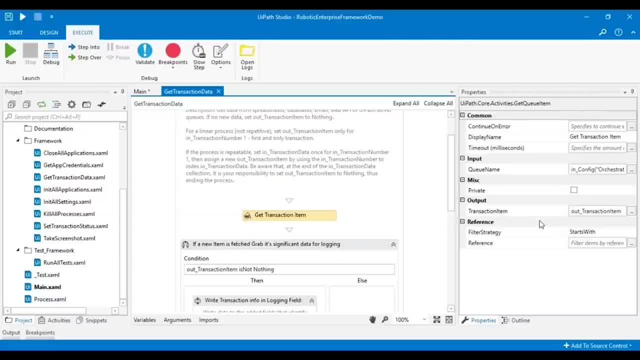 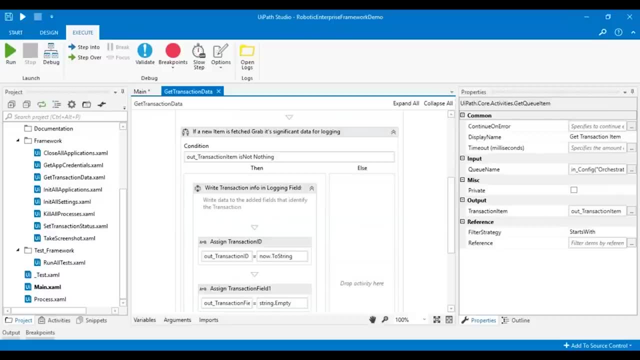 so that the actions with respect to that particular transactions are successful right now. if there's no data- like, for example, let's say, there's no new data- then obviously the process stops and then if there is new data, then we move on to the process transaction right now. apart. 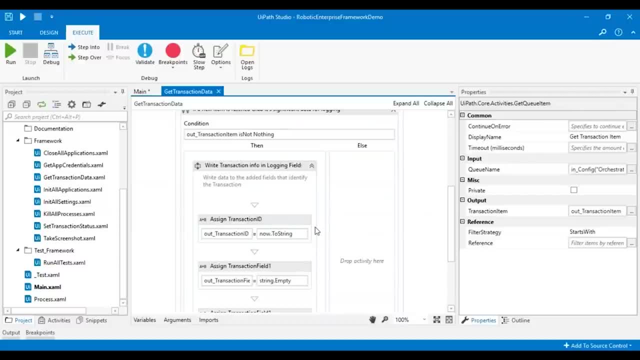 from that, at some point of time of the workflow, What happens is: all of the transactions are being already processed, right? So there are no new transactions which have to be processed or which have to be read by the report, right? So then what happens is that the report should stop. 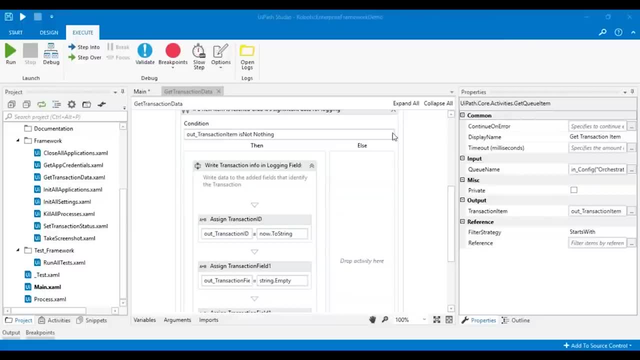 and then you should go to the end for the state. So this basically occurs when the transaction item becomes nothing or null. or when you use the orchestrator Q, that happens by default when there are no more new items to be sent, right? So that's what we are doing with: setting a condition. 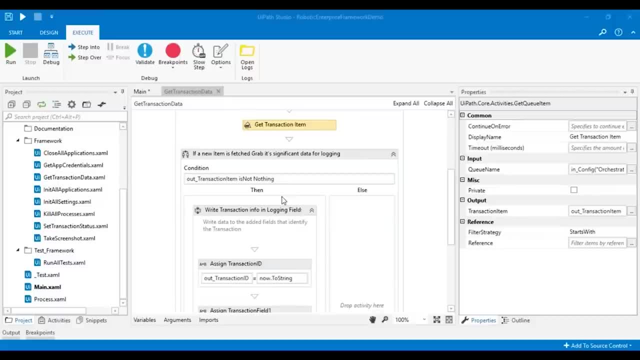 which is our transaction item, is not nothing, Right? So if it is nothing, then what happens is that you know your report should stop and then it should just directly go to the end process, right? But yes, if it is not nothing and there's some new data. 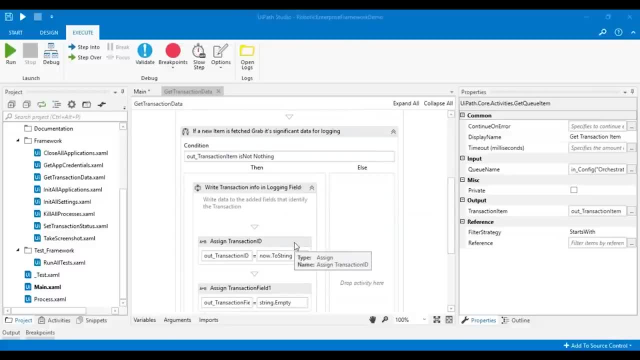 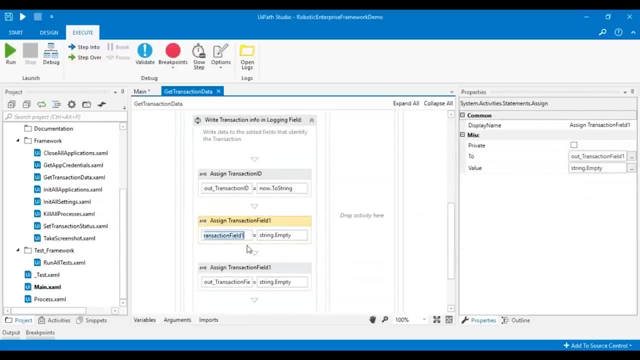 then what happens is that you write the data to the added fields that identify the transaction right. So the out transaction ID is assigned to now dot string and the out transaction field 1 is assigned to string- dot empty, and the out transaction field 2 is again assigned to string, dot empty. 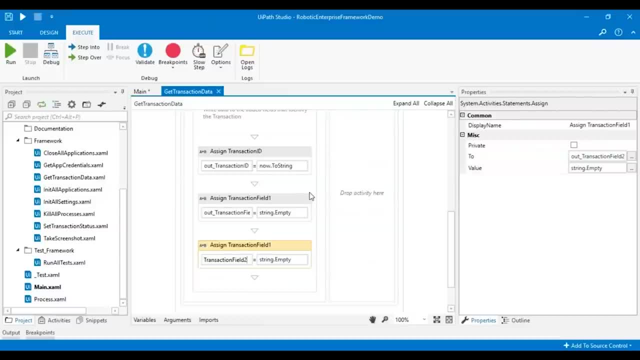 Right now, before I move back to my main file, I would like to tell you one thing here, that is, you know, if you change the type of the transaction type, So we are. it was Q item, right? If it was not that, then you have to assign it to null. 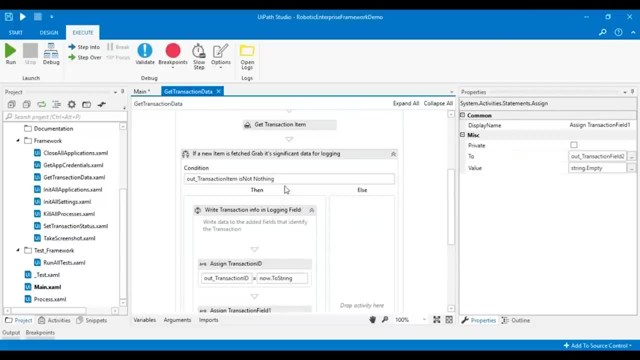 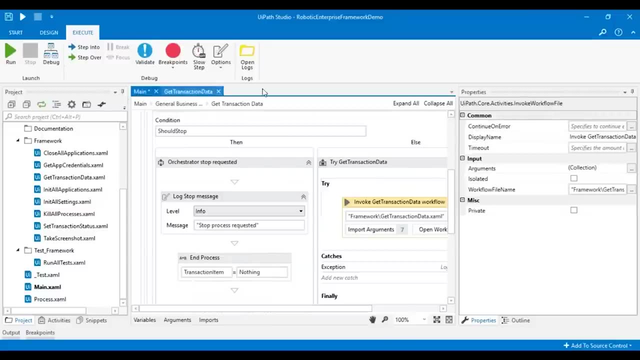 and not nothing. and then what will happen is the report will identify whether it has take you forward to the next step or if it has to end the process. right now, let me just shift back to my main file and then let me just you know. 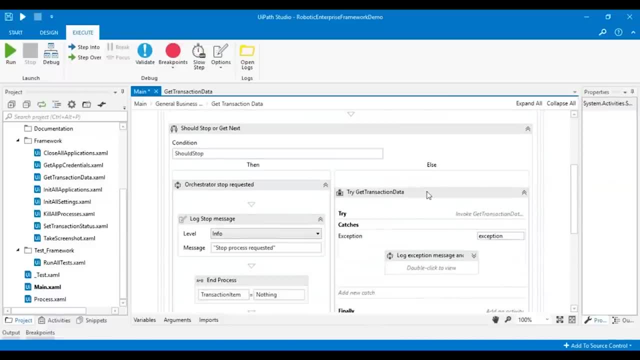 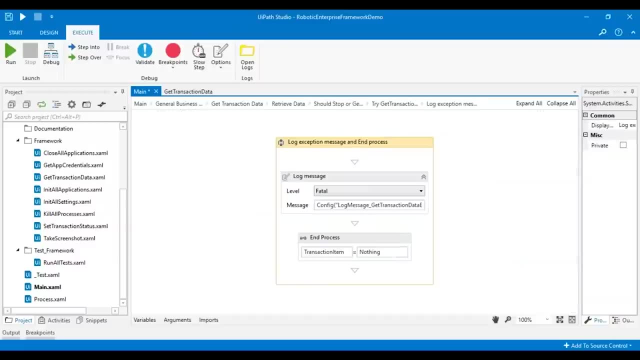 drag the property section back and in the else section of this particular activity. Let me just show you the catch block. So the catch block has an exception. So basically, what we're doing is we're just logging an exception which says: you know, 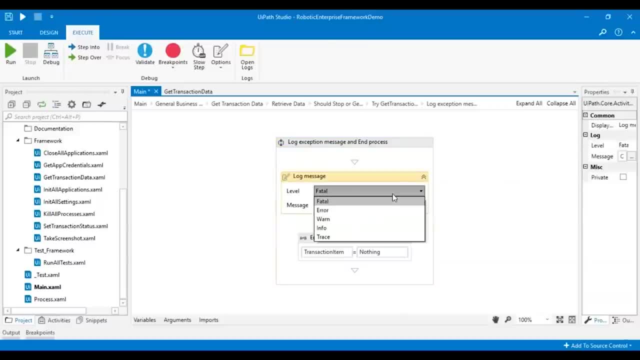 the level is fatal. So over here, if you observe the level in a log message, activity is used for the user's perspective, to understand if it's an error, if it's a warning, if it's a trace and so on. right, so it's just for the user's perspective. 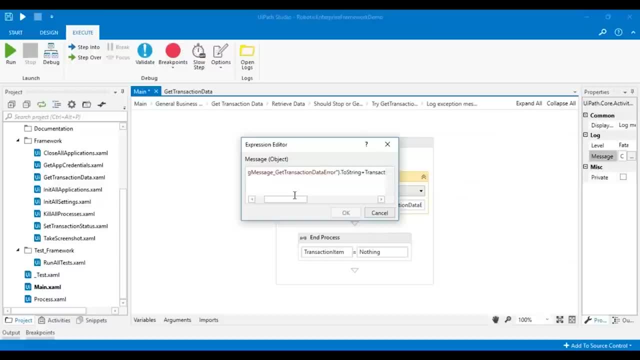 So if you just mentioned fatal over here, and then the message is mentioned that the log message get transaction data error to string, and then we are mentioning the transaction number, also the exception source, right after that We just ending the process, that is, we are just assigning. 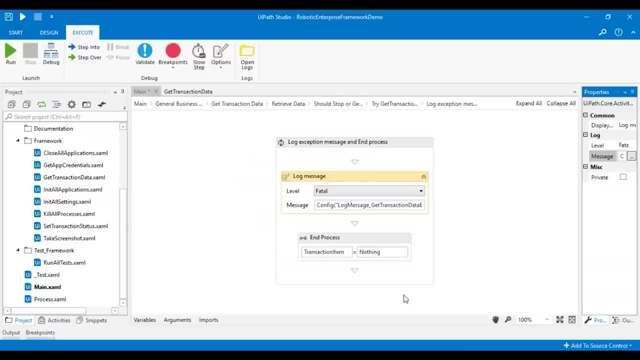 the transaction item to nothing. So as soon as you assign the transaction item to nothing, you'll understand that you know that particular process is going to end and there's no more new transaction data that has to be processed right. So now, if I just go back to this part, 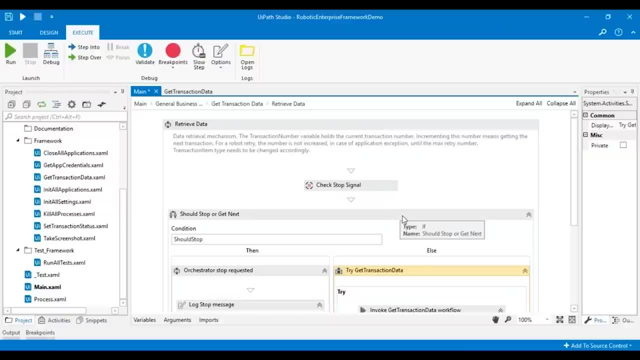 this is basically the workflow of how to get transaction data works. Just remember the fact that for every transaction that you process, the transaction number should be unique. So now let's move forward with a next date. So, as I was telling you, if this particular part is successful, 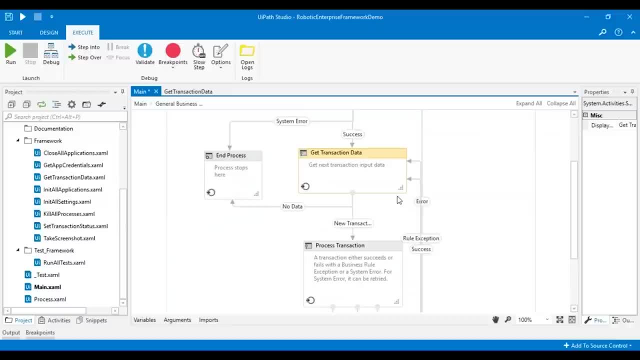 that means you know, if the get transaction data throws a new transaction, so that means there's a new transaction which has to be processed, then the next factor that comes into picture is the process transaction state. else, If there's nothing to be processed, 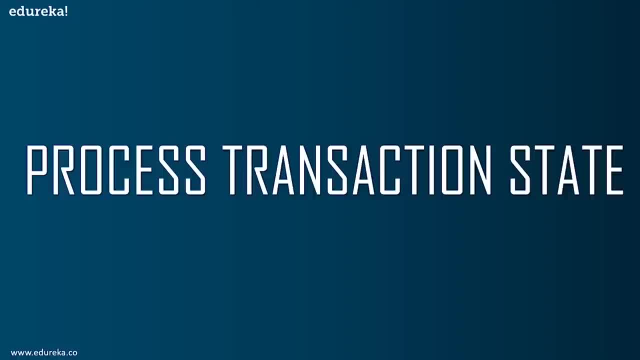 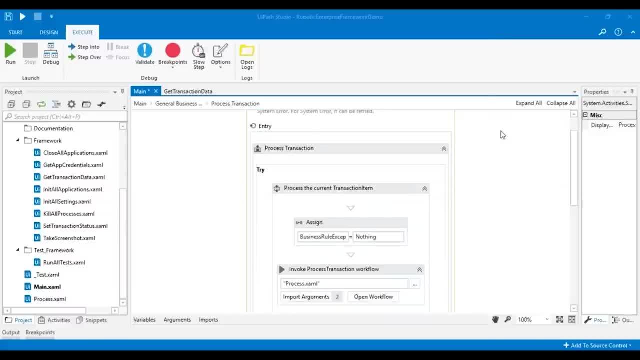 and it directly goes to the end process date, right? So now let's take a closer look at the process transaction state. So, as you can see, the process transaction also has a try-catch block in which we invoke various kinds of XAML files. 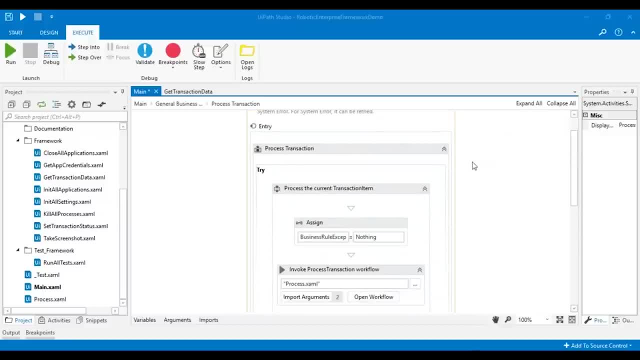 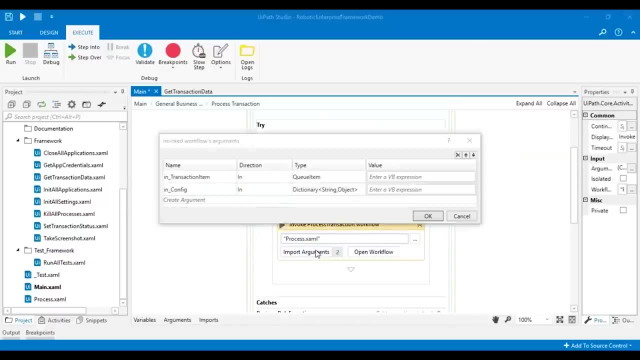 right. So let's understand each one of them. So, starting with the try block. So the try block basically starts by invoking the process to XAML file, right? So over here we basically need to input arguments. that is the transaction item. 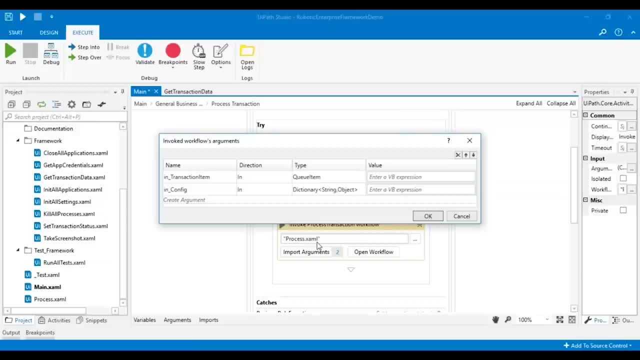 which is basically the cue item and in config dictionary. So that is also an input argument. It again has the spring and the object as the key and the values in the dictionary based on the execution of this particular process, We catch a business tool exception. 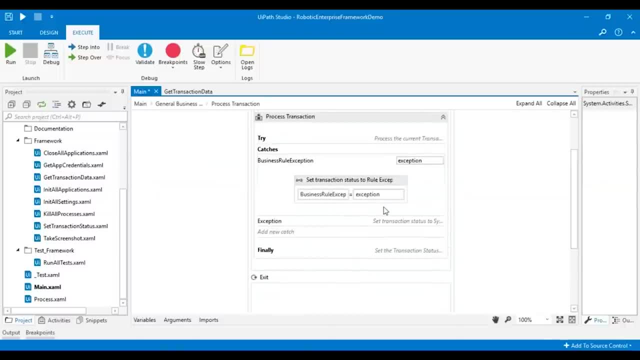 So in the catch block you can clearly see that you know we catch this particular exception. That is basically a business tool exception which is thrown by a throw activity right now. after that we also have a system exception to handle any unhandled exceptions. 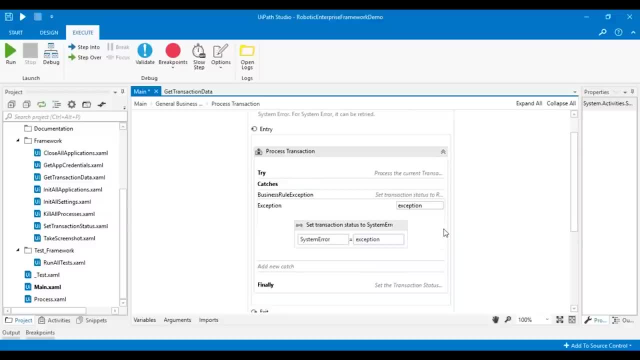 thrown in the process or in the activities, right. So whenever there's any unhandled exception, that is, the system exception handles that particular exception right now based on the one of the three outcomes. that is basically, if you observe in the main file. 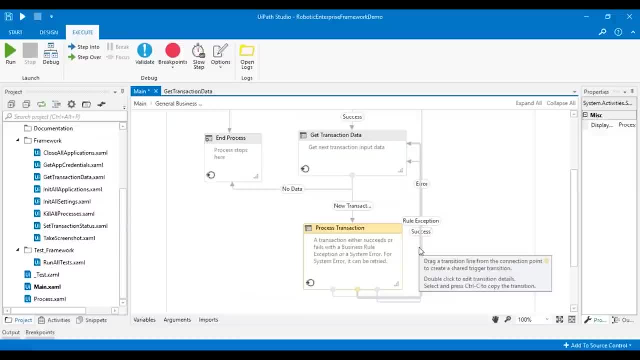 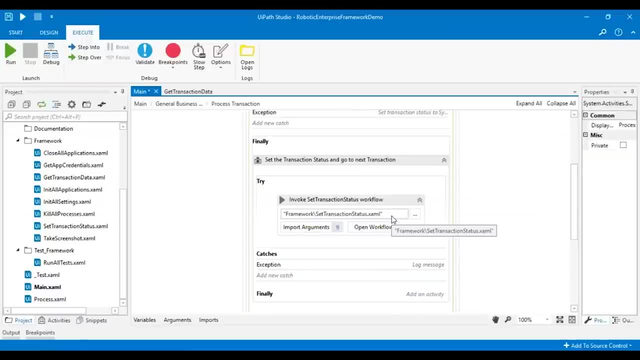 there are mainly three outcomes, that is, the success rule exception and the error. the new state is selected. So over here, if I just go back to my process transaction. so over here, if you go back to the finally section, you'll see that 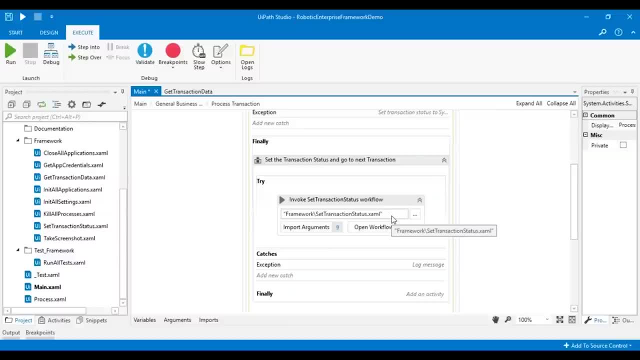 you know, we invoke the set transaction status workflow. So again, this particular XAML file is invoked from the framework folder and basically in this, as soon as the transaction is completed, We need to set the status with appropriate logging mechanisms, right? So basically we'll have to mention that. 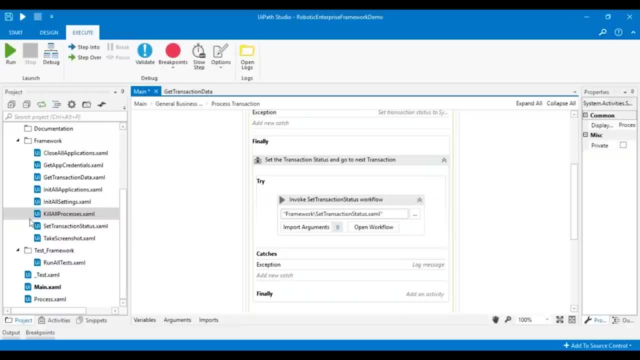 you know that particular transaction is done and then maybe we'll have to set the transaction status that you know. yes, it is successful and all that right. So over here, if you just see the arguments of this particular workflow, 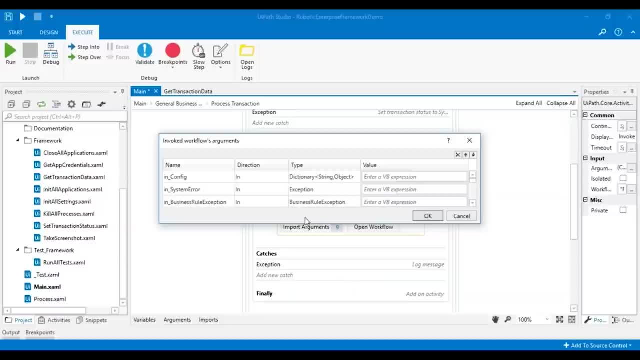 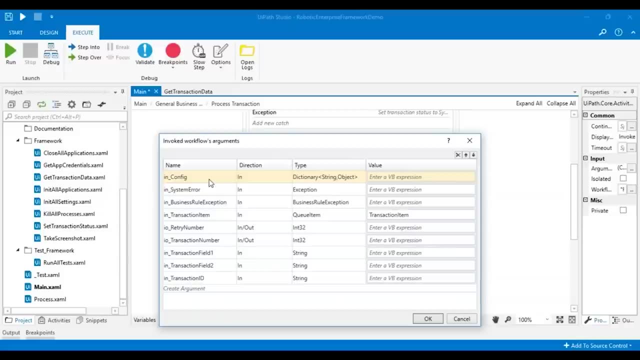 you'll see that. you know we have the config file, the system error, the business role exception as the input arguments and basically these three arguments are used to determine the next date, That is basically whether it has to go to the end processes. 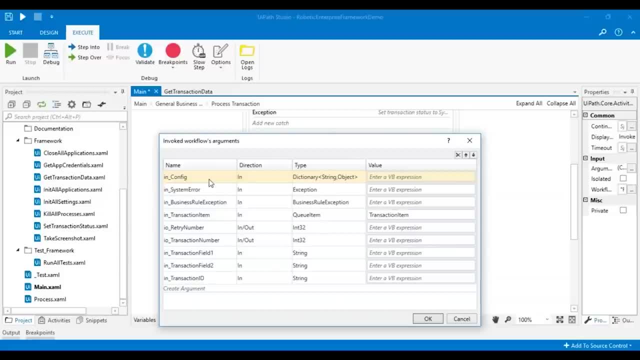 or maybe it has to go back to the in its date, or maybe again it has to go to the get transaction data state right. apart from that, We also have the other input arguments, such as the transaction item, the transaction field 1, field 2 and the ID. 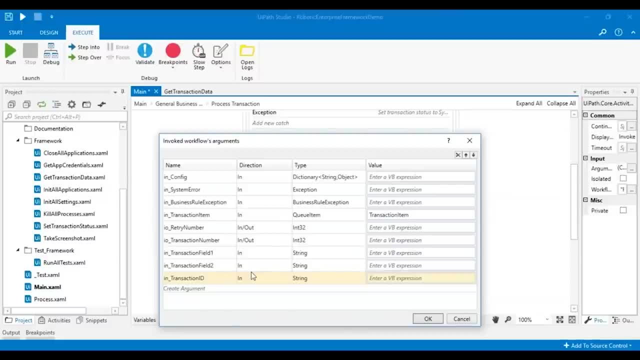 So basically these are used to basically keep a track of the transaction that is happening, and then they can definitely be altered in the transaction XAML file. So whenever you want to order the transaction, you just have to go back to the transaction XAML file and then alter it over there. apart from that, 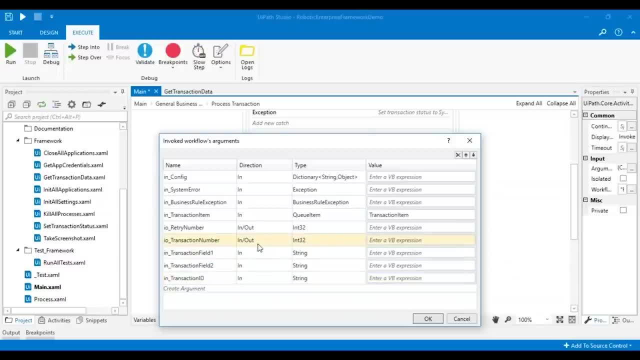 We also have the retry number and the transaction number, which are used as both input and output arguments. So the retry number, as I previously told you, is to basically keep a track of the retries of the field transaction and the transaction number is to keep track of the transaction number right now. 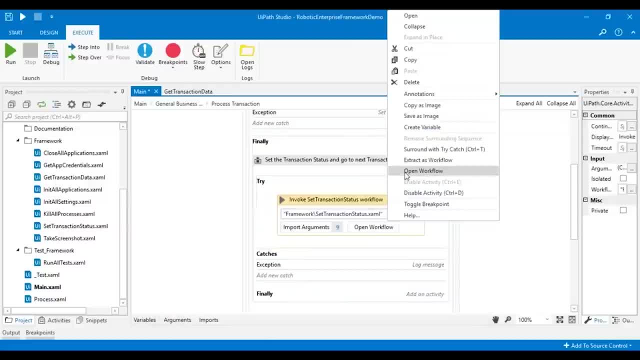 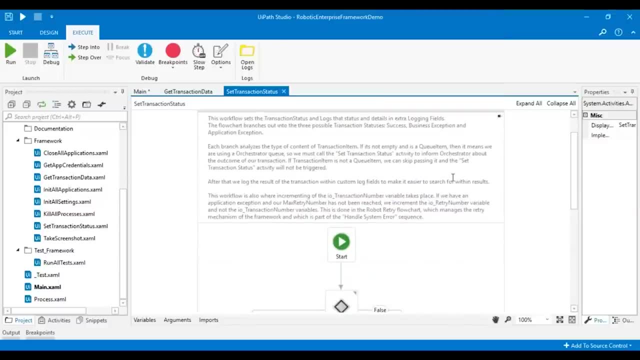 if I just close this particular dialog box and then if I just right click on this particular activity and open the workflow. So if I open the workflow of set transaction status XAML file, you'll see that in it's a simple flow chart executing three possibilities. 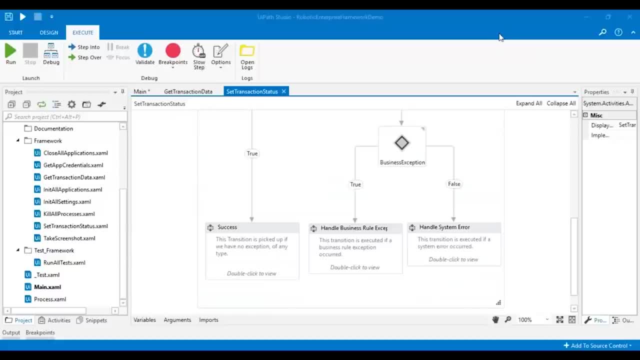 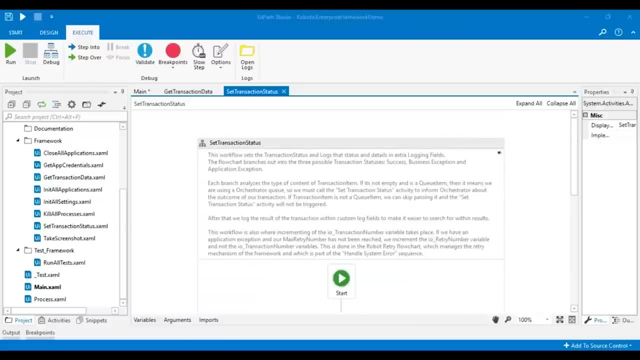 that is success: handle business tool exceptions and handle system errors. So we'll discuss each one of them one by one. So let's start with success, But before that, what you see over here is a flow chart. So, basically, if the process is going on on a success node, 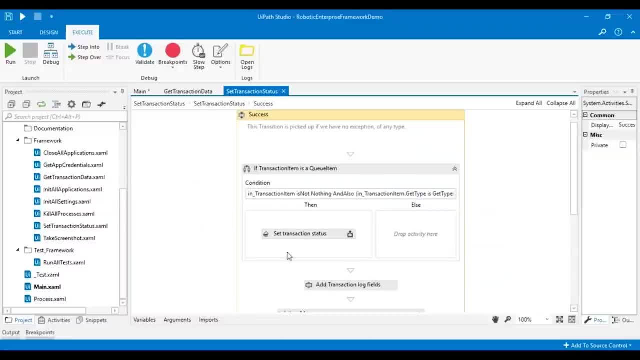 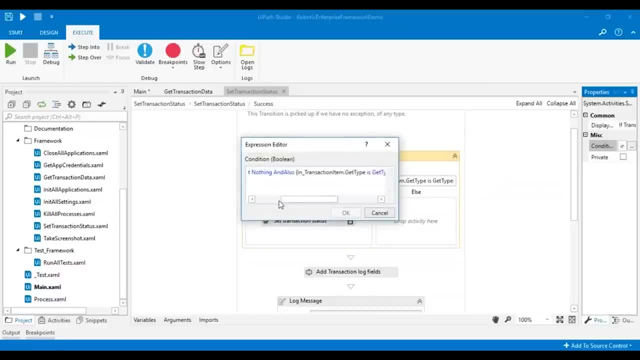 and then it is true. then if I just double click to view this particular activity, you'll see that you know there's an if condition mentioned over here, right? So the if condition, you basically have to mention the condition. the condition mentioned is basically in transaction item. 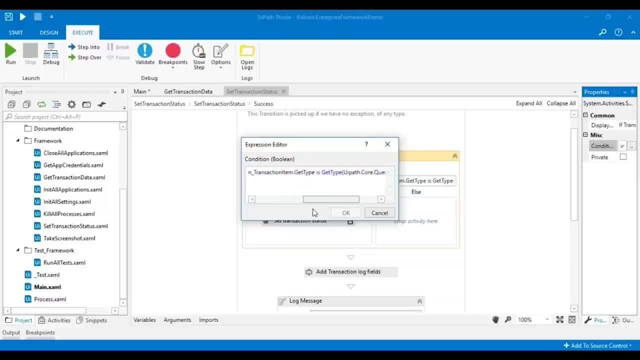 is not nothing. and also in transaction item dot get type is get type according to the QI, right? So if that is the condition, and then if it is successful, then you set the transaction status as you don't do anything, right? So basically, this condition says that you know. 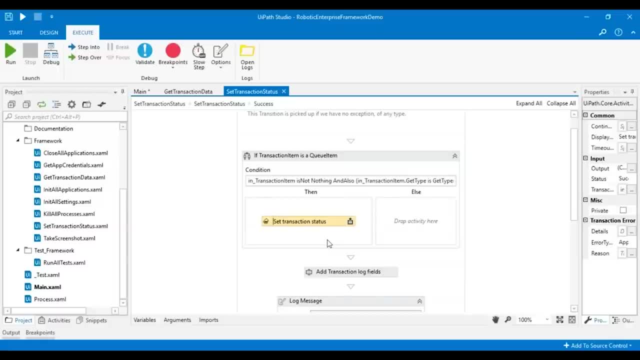 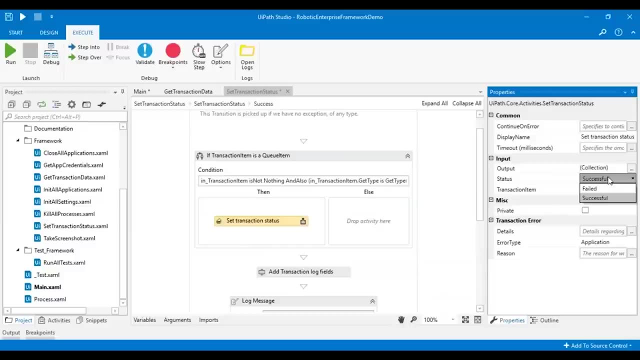 if the transaction item is not nothing and the transaction type is basically the Q item, then you set the transaction status to be successful. So if I just drag the property section, you'll see the status to be successful, right, So that's what is basically done over here. 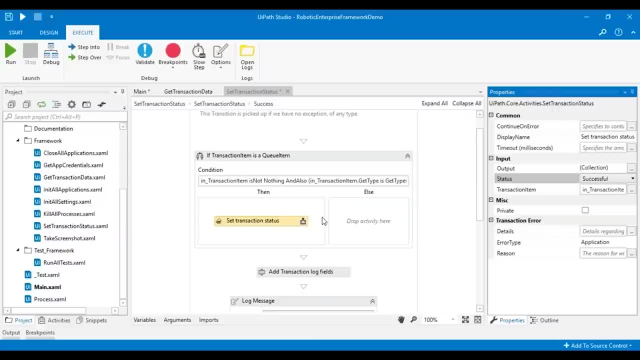 You will set the transaction status to be successful And then, if you want to change the type of the transaction item, then you have to first delete this activity and then you have to change the type of the transaction item right. Apart from that, moving forward with the workflow, 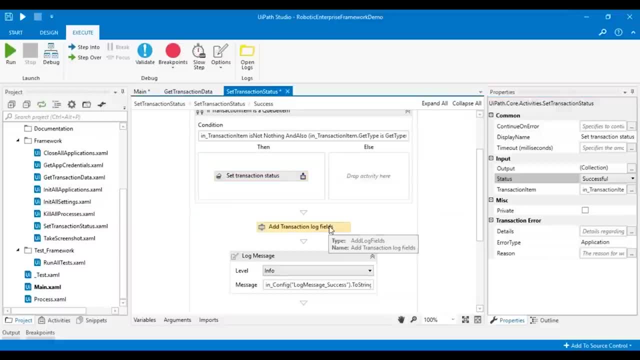 The next activity that comes is the ad log fields. So this is basically used to log the successful message. So whenever there's a transaction which is set, then automatically the log fields would be logged where it would say that you know it is successful right now to set this message of log. 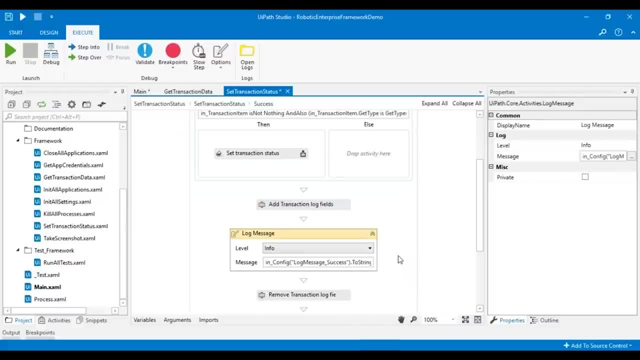 to be successful. You basically use the log message activity. So, as I was telling you previously also, the level is basically for the user experience to understand: if it's an error, if it's a fatal, if it's a warning and so on. So we are, it is mentioned. info. 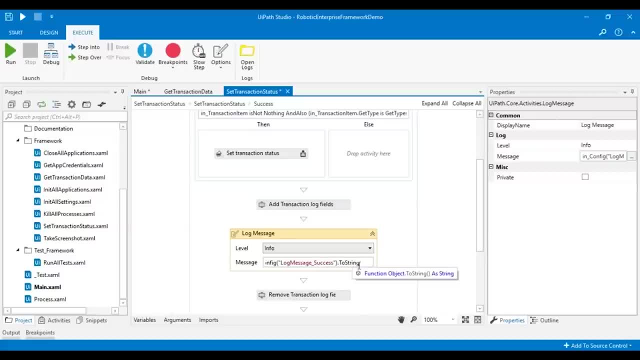 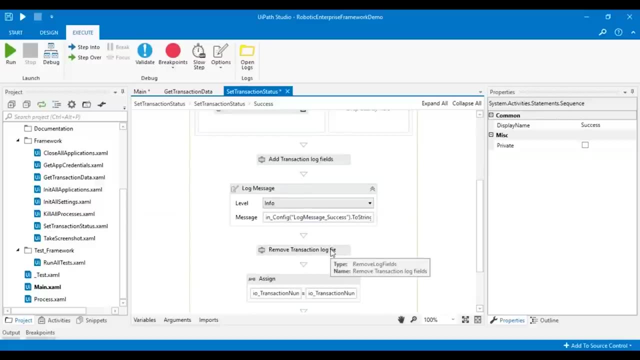 and in the message it is mentioned that log message success to spring that. so basically, log message success would be displayed into your log file. That's right now. after that, what happens is that we remove the transaction log file. So this is basically to remove the custom log fields. 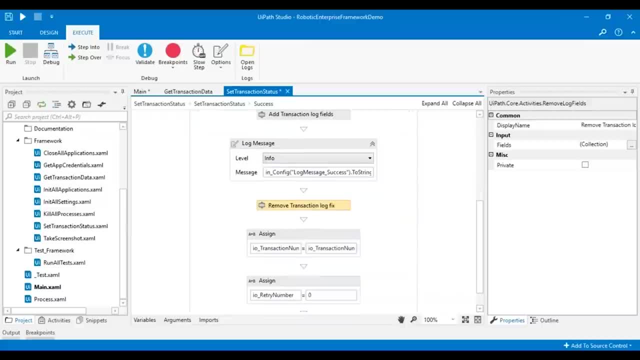 to each log message, right? So that is done and moving on. Finally, we assign the transaction number to the next transaction, right? So basically, we are assigning the variable of the transaction number to the next transaction, so that you know the next transaction is checked. 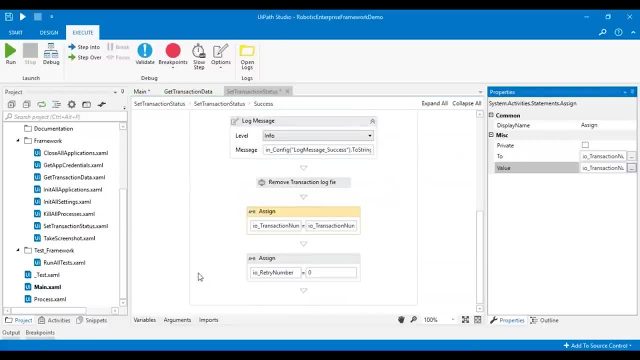 So that is basically it is initialized by the counter right now. after that We also set the retry number to be 0. So if you remember, in the config file also the retry number was by default set to 0. So we are will just assign that particular variable to be 0. 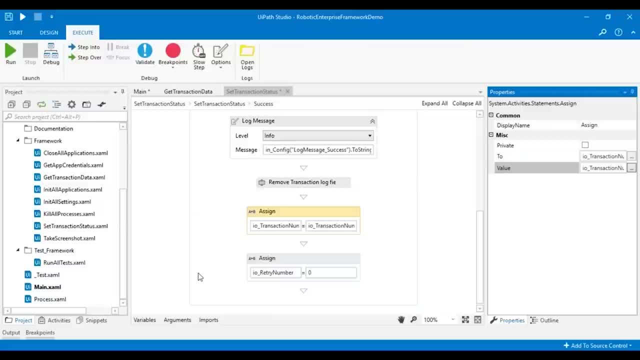 so that initially, the count of retry starts with 0 and then, if there are any retries for a specific transaction number, then the count is increased, right? So, guys, this was all about the success state. now moving back to the set transaction status, You'll see that you know. 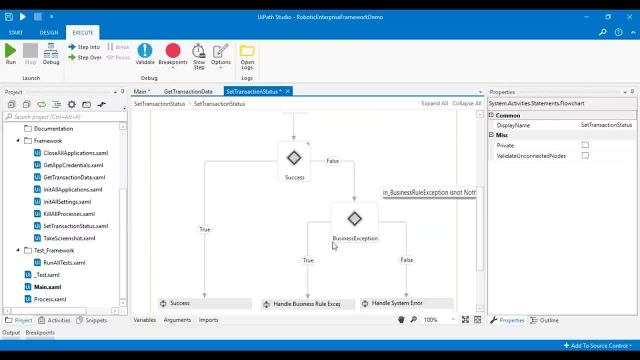 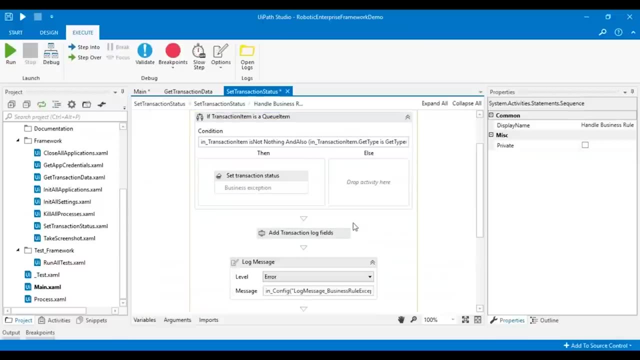 if the success is not successful, right. So basically, if that state is not successful, then we go to the business tool exception. now in the business tool exception- If I just double click over here you'll see again- and if condition, and then the same steps are executed as that of the previous one. 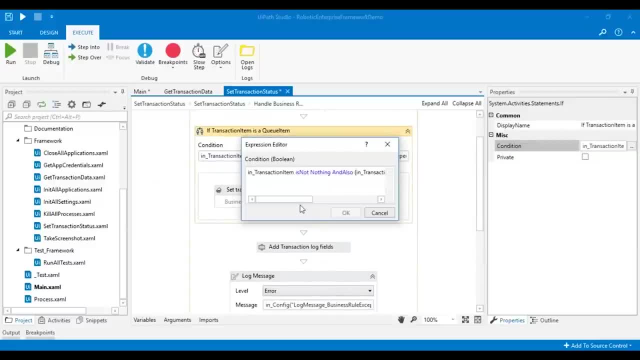 right. So we are in the condition section. The same condition is again mentioned, that is the. if the transaction item is not nothing and also the transaction dot get type is basically a cue item, Then what happens is that we have to set the transaction status. 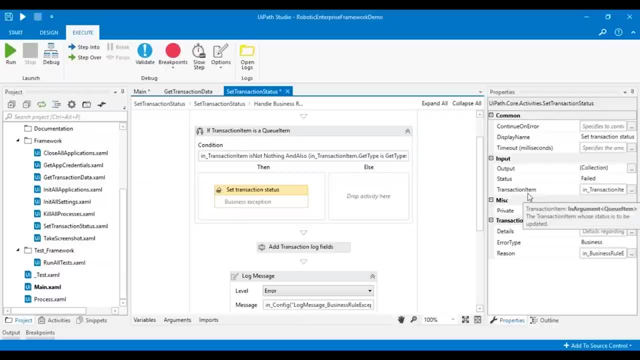 to be failed. Now, This is basically. we are mentioning the fact that you know there's a business rule exception that has occurred and the transaction has been failed to be processed, right. So that is the reason. in the set transaction status, We set the status to be failed. 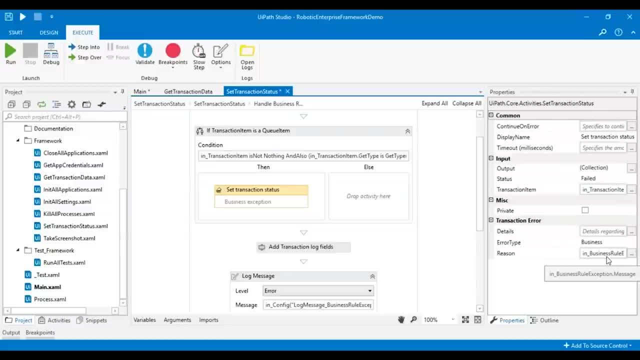 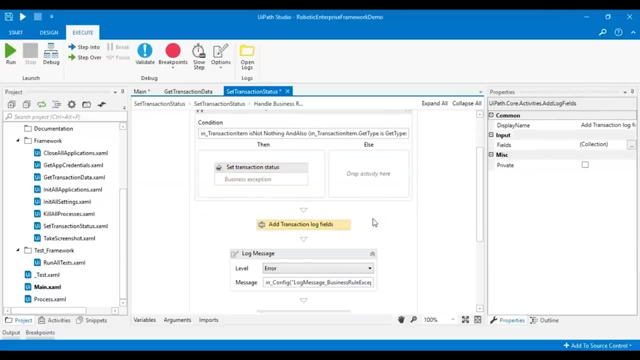 and the error type to be business and the reason to be business rule exception, so that it's clear that you know it's because of the business rule exception that you know that something is gone wrong. after that We again just add the transaction log field. 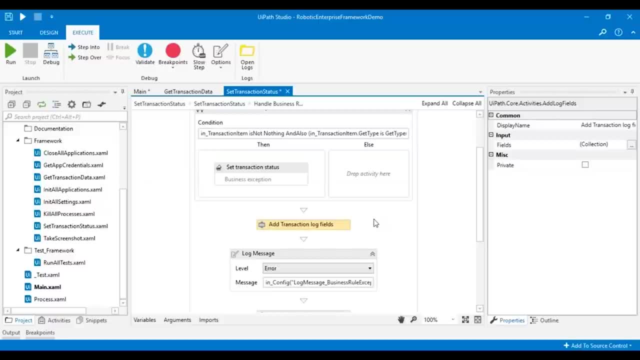 So basically we add the custom log phase to log the message and to log the message will use the level to be error now because it's an error and in the message will say: you know, log message: business tool exception. So basically, when the execution is occurred, the log message. 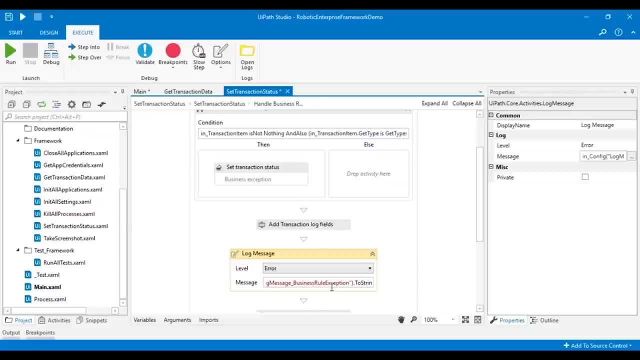 would be stored saying that: you know, log message, business tool exception. So anybody who is coming back to look into this project and understand that you know because of the business tool exception something has gone wrong, right, So after that- will again similarly just remove the transaction. 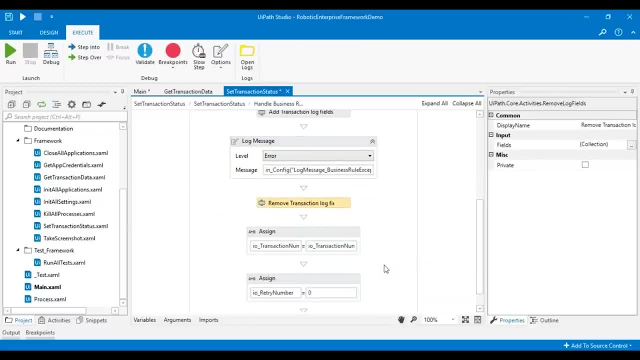 log files to remove the custom long fields of each log message and finally assign the transaction number to the next transaction number. right, So we basically move on to the next transaction number with the help of this assignment and then also reassign the retry number to be zero. 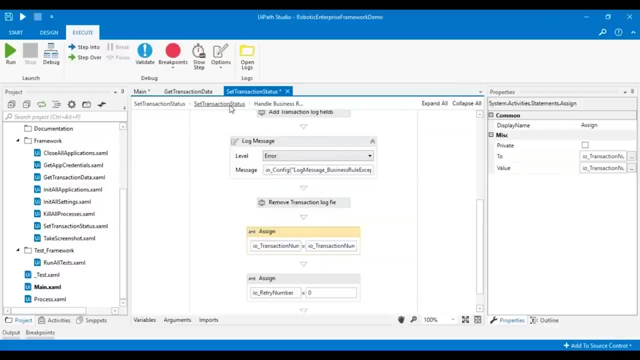 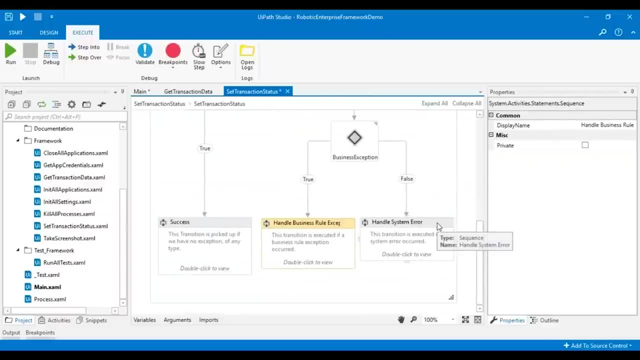 right. So, guys, this was all about the business tool exception. Now, if I go back to the set transaction status and look into handle system error, so if the business tool exception is true, then this particular business tool exception part is executed. else, if it is false, 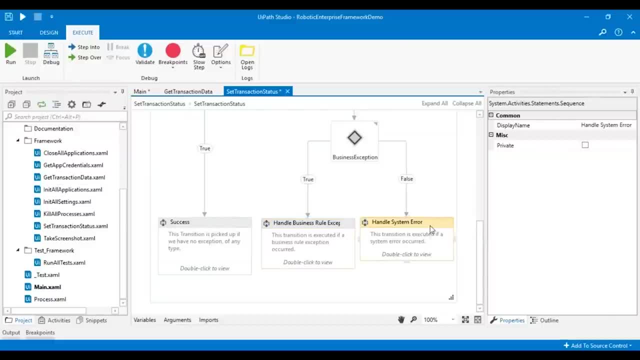 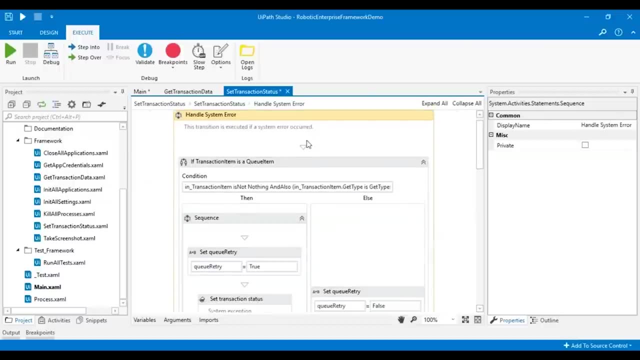 and the third part is executed, that is, handle system error. that is because you know that is the only possibility that can occur if it is not success and business tool exception right. So if I double click over here, you'll see this again in the condition that has to be mentioned. 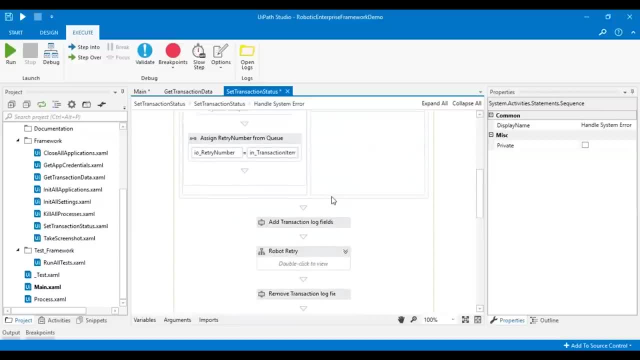 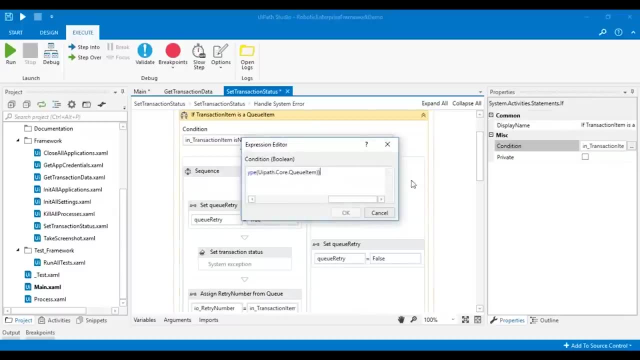 and then there's a little bit change in the sequence of the workflow of this particular activity, right? So let's look into the same, So starting with the condition. So the condition is the same as the conditions that we just discussed previously, that is. 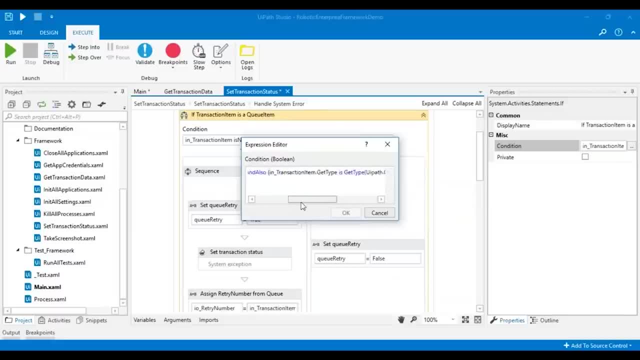 if the transaction item is not nothing and also in the transaction item get type is not a queue item, Obviously, then we'll set the queue retry to be false. But yes, if it is the queue item and then the transaction item is not nothing, then some steps would be occurring. 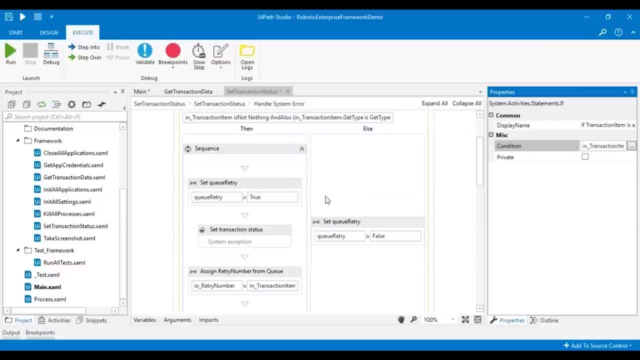 right. So what we'll do is we'll consider an extra variable over here, that is, queue retry, right? So this is basically used to log a warning message if the queue item is being retried and also an error Otherwise. right now, one thing that you have to remember over here: 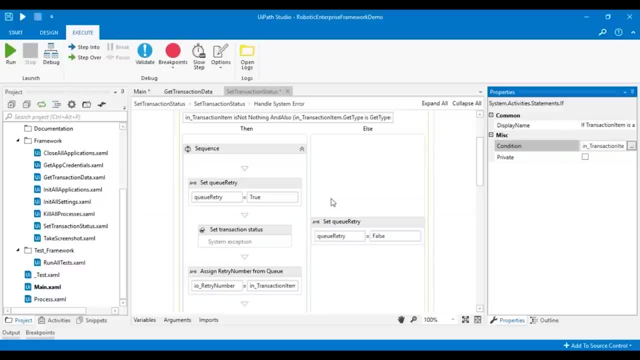 is that, basically, that you know, if we use the queue items, that the flag is always true. else it is false, right? So that is what is happening over here, Since we're using the queue item that I've initially assigned the value to be true. 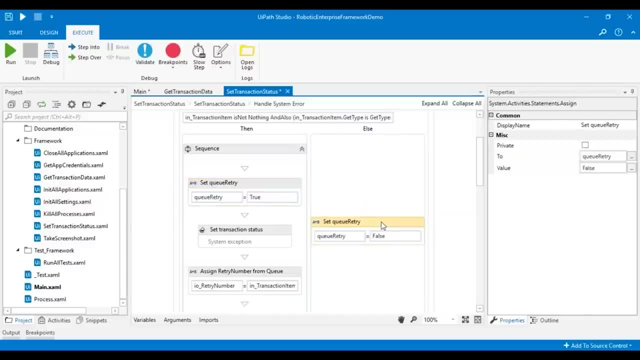 That is the flag is true. else, If it is not true, then obviously it is false. right, But if we would want to change the type of the transaction item to something else, then we need to remove this entire sequence, as I also was telling you previously. 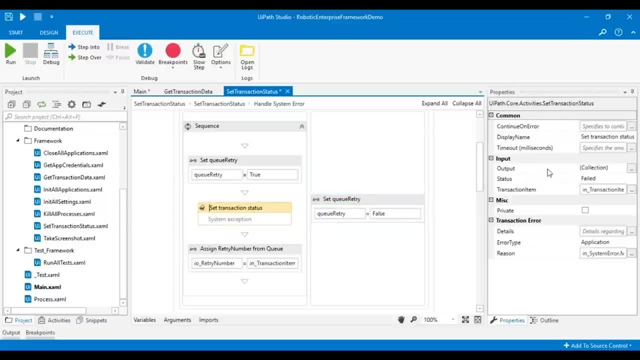 right now. after that, what you have to do is you have to set the transaction status to be failed again, obviously because we are throwing an error right. So that is the reason we mentioned the fact that you know the transaction status has been and the edit type to be application. 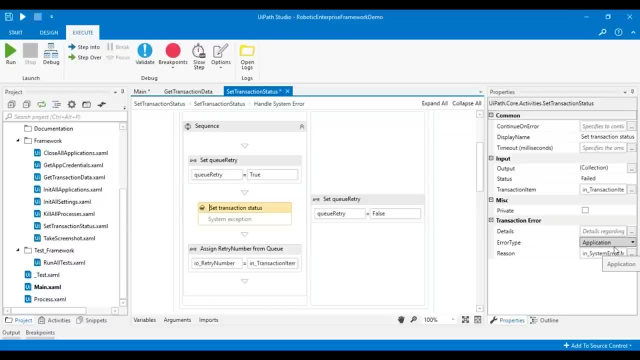 because if this is not happened because of the business rule application- but yes, it has happened due to the error in the application, right? So that could be the error type and the reason to be system error message, right? So basically, we just mentioning the fact that you know. 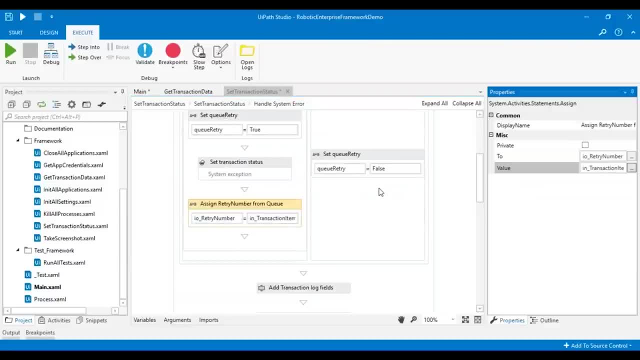 it's a system error. after that, What you'll do is you'll basically assign the retry number to the transaction item- dot retry number, right? So basically, you're counting the number of retries that is happening for a specific transaction number And then, finally, you will add the transaction log fields. 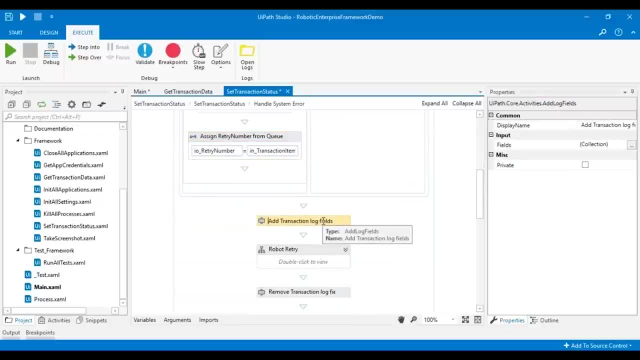 that's basically to log your messages. So this will basically add the custom log phase to the report execution logs And then finally, you'll put in the robot retry flow chart, right? So when I say the report retry flow chart, this is basically a flow chart. 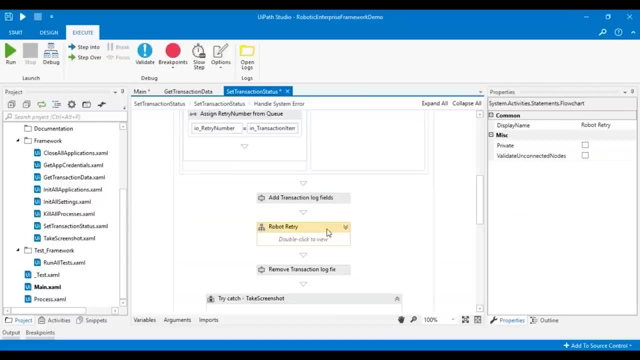 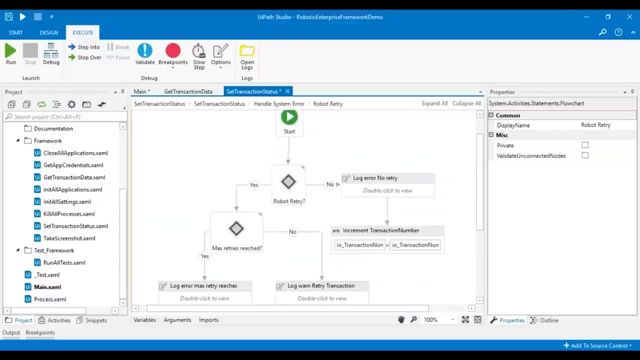 which will talk about all the retries that will happen for a specific transaction number. So if I just double click this for you, you'll see that you know there's a particular flow chart that happens, which only talks about the retries. if you know if there's any maximum retries. if yes, 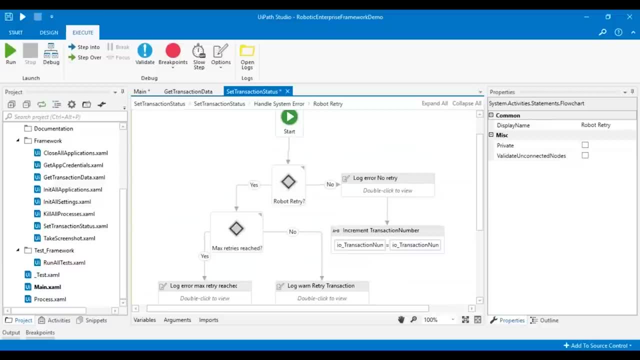 if, initially, if the robot has retried or not. if not, then what is the message, if yes, then what is happening, and so on. right? So remember by default that you know we're using the orchestrator queue, in which the max retry number that we assigned 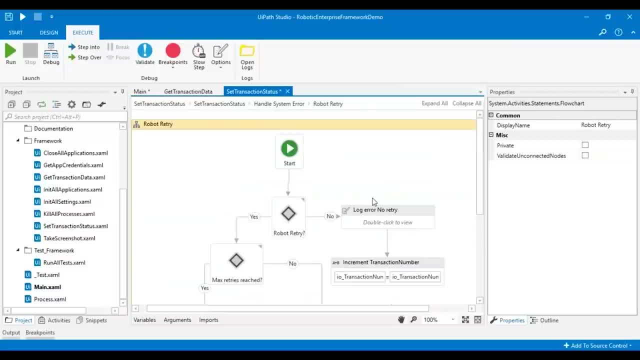 in the config value was zero, right. So now, if you just look into this flow chart, you'll understand that you know if the retry number is not enabled after the first floor decision, then the no branch of the robot retry would be executed. 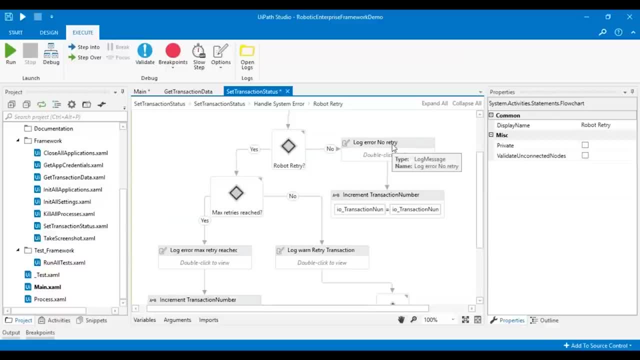 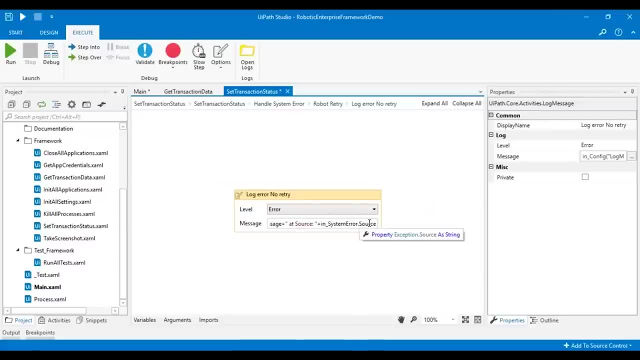 So over here if you look into, there are mainly two activities that you look into- that is, the log message activity with the level error, and then it displays message saying that you know the log message application exception, the source where you know the exception is happening. 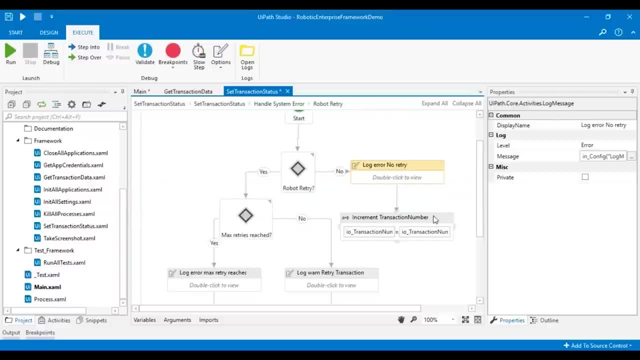 right. So that is one thing that comes over here. apart from that, There's also an increment in the transaction number, so that you know the robot does not retry the same transaction, but instead it just moves on to the next one, right? So, basically, what's happening over here? 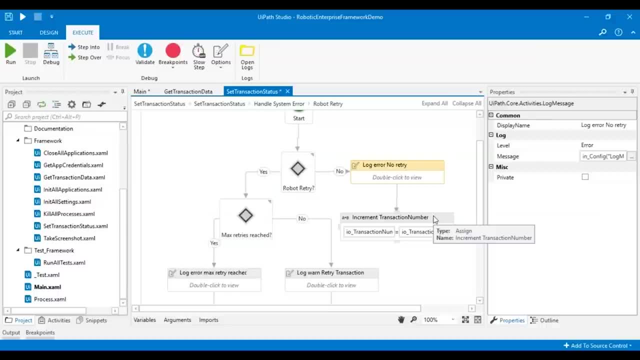 is, we're just defining if the retry has to happen or not. If it has to happen, then we move on to the retries. If it does not have to happen, then we'll say that you know, there's no retry required for a specific transaction. 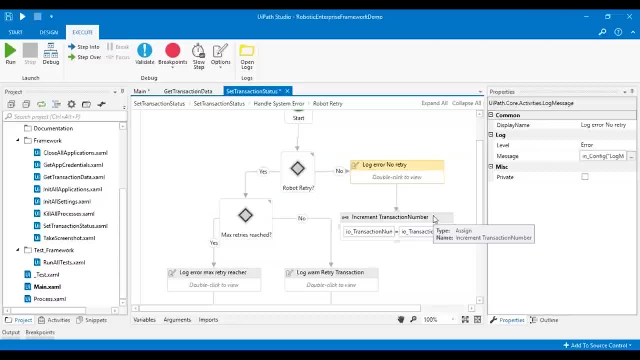 and then the robot can just move forward right now. Similarly, if you consider the scenario where we are not using the queue, we can just set the max retry number in the config value to be greater than zero. right, The yes branch of the robot retry will be executed. 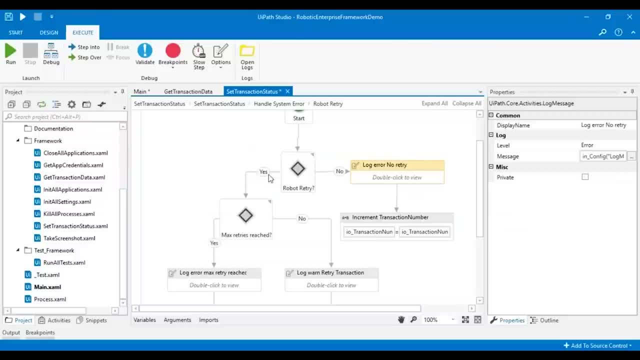 So initially, what you have to understand is the yes branch is executed when, in the config file, you assign the max retry number to be greater than zero, and the no branch is executed when in the config file, the max retry number is put to zero, and then it is a queue item for the yes branch. 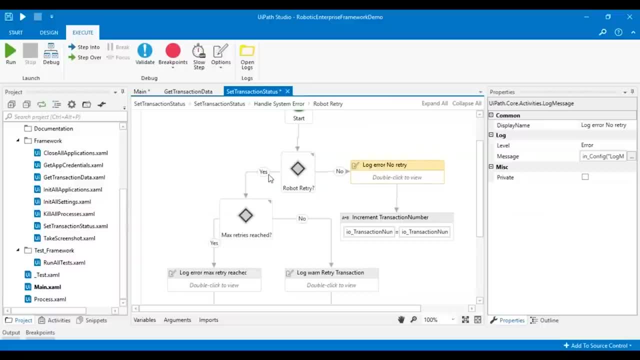 It is not a queue item that is getting executed. So when we are talking about the execution of the yes branch, what happens is that the report checks if the max retry number has been reached or not. right, So this is basically used to understand the fact that you know. 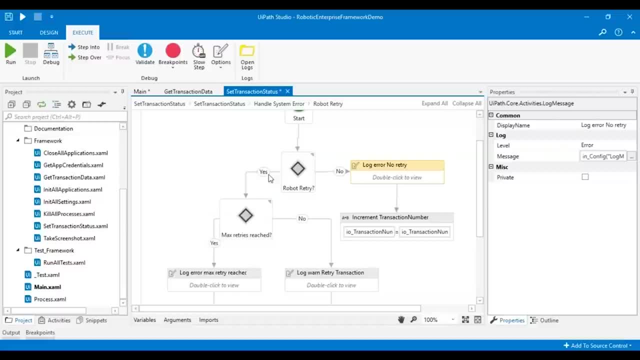 the retries of a failed transactions should not happen forever, right? So if the current retry number reaches the maximum value, then the report logs a message again. So if I just double click the view, you'll see that you know. the report logs an error message saying that you know. 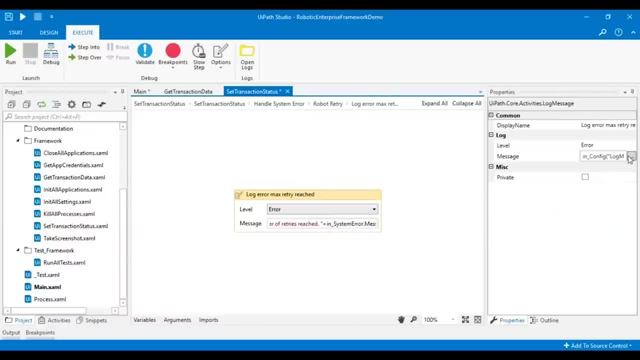 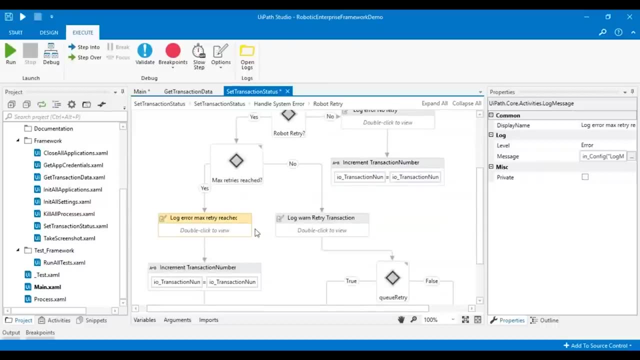 the log message: application: exception of the maximum retries have been breached, right. So that basically logs a message. and then what happens is the transaction number is moved forward. So basically we move on to the next transaction. But if the current transaction has not reached the maximum number, 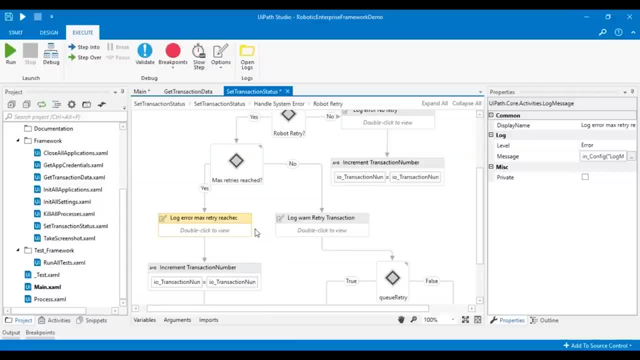 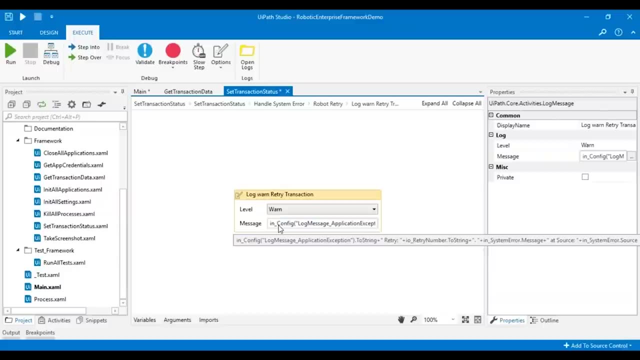 of retries and it has been retried only a few times, then the max retry number indicates that the robot simply logs a warning. So if I double click the activity you'll see that you know the level is one and the message says the log message: application exception. 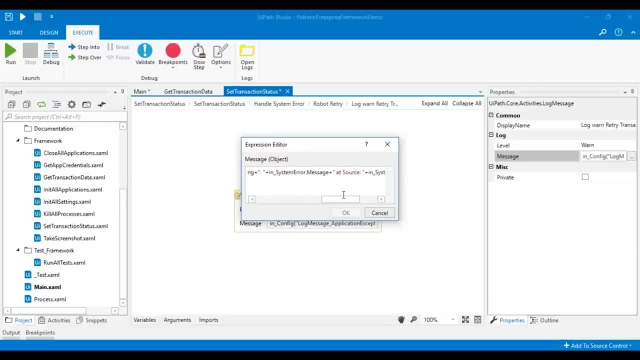 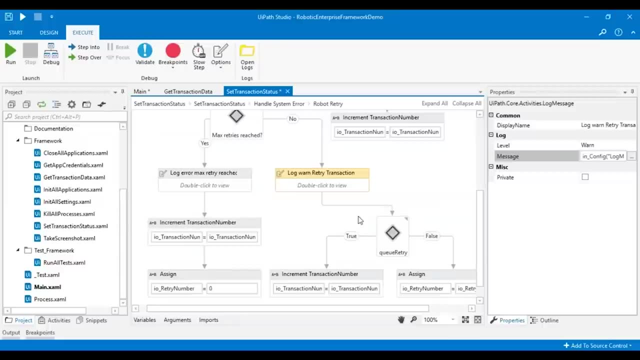 to spring is basically has not reached a maximum of retries, right. So that's basically it's going to be printed at source right now. after that, what happens is that another decision comes into picture, that is, the queue retry. So in case the type of the transaction is other than the queue item, 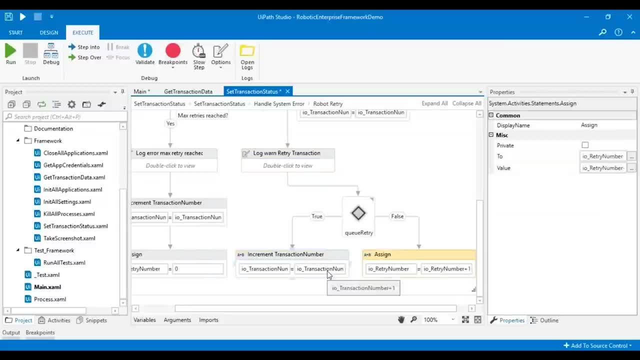 then the robot increments the current transaction number right. As you can see, in the assigned part of this activity, the transaction number variable has been assigned to the increment of the next transaction number, right, So it's just goes to the next transaction. 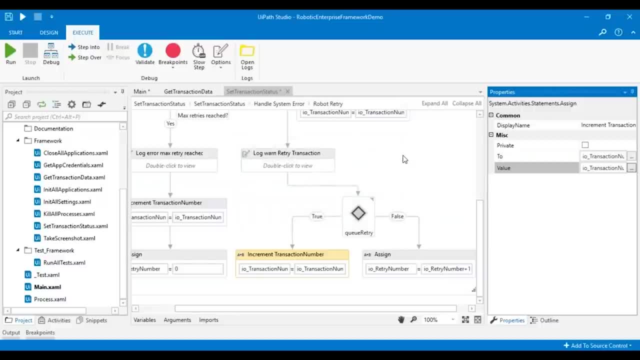 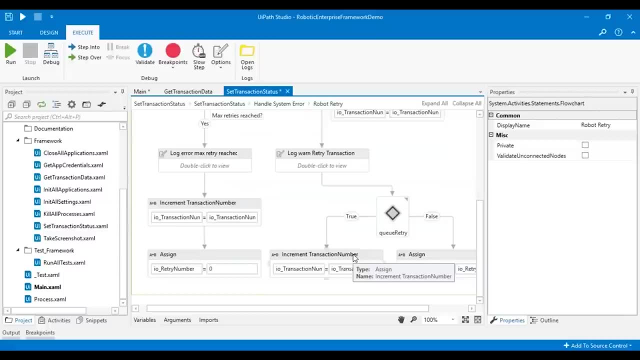 Similarly if it is false. So in that case, when the type of the transaction is the queue item, then the retry number is just incremented by one right after restarting the application. The same transaction is basically in the get transaction data right, So because of this the transaction number has the same value. 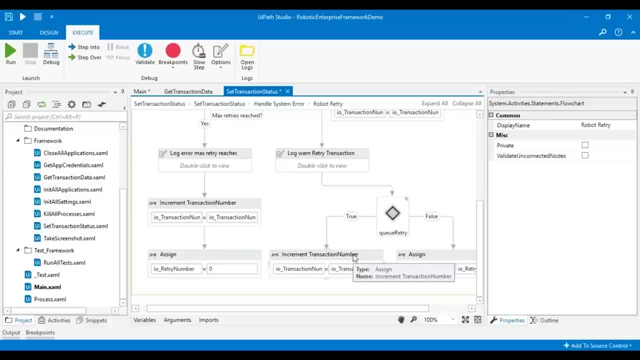 So, just in case the queue item variable is processed, the orchestrated deals with retries, So it increments the transaction number, right? So that is what is basically happening in the true section of this particular activity, where the transaction number is increased by one. and if it's false, 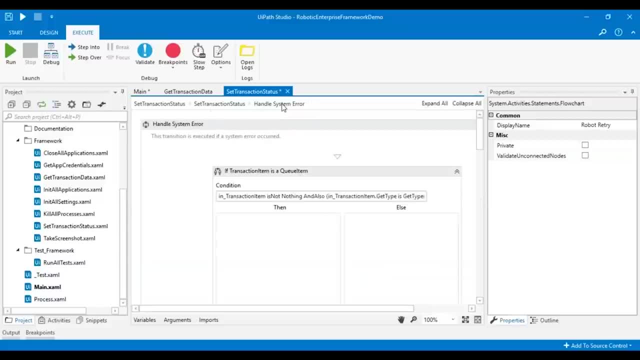 then the retries are increased by one. right now, if I go back to the handle system error, the next step that comes into picture is to remove transaction log file. So basically, that is to remove the log custom fields of each log message And finally we have a try-catch block. 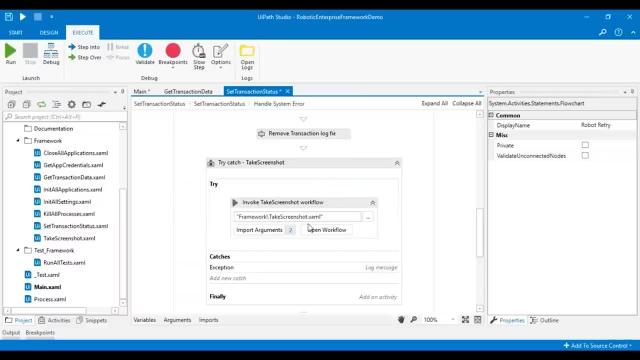 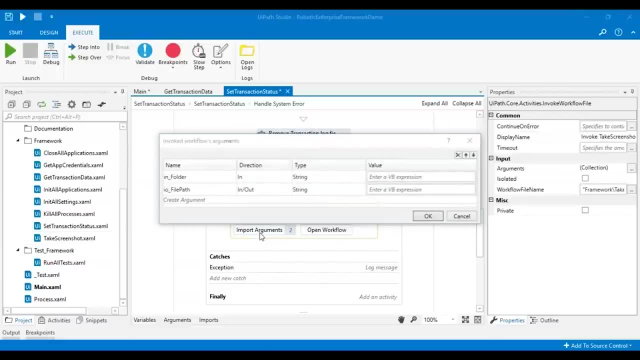 which talks about taking the screenshot of the workflow. So over here we invoke the take screenshot, that sample file from the framework folder Again, and then over there we have two arguments. So let's look into the same. So the input argument is basically in folder. 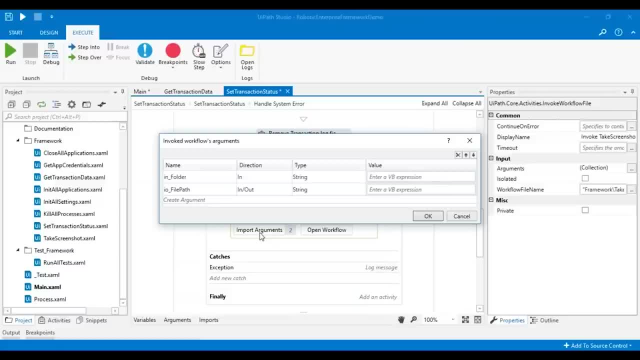 which consists of the folder and the file path is basically an input and output argument, which consists of the file part where you want to store, right? So that is where basically the screenshots are taken. and now, if you have a question, why exactly the screenshots are taken, 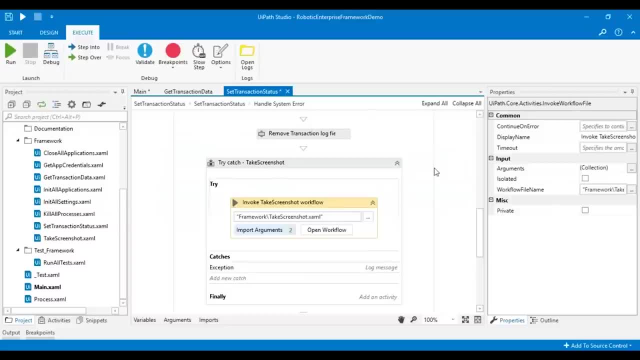 so you can just understand, with the fact that you know the screenshots are taken at the time of the exception, so that any user looking back into this or maybe anything happening with the business process can be understood with that particular time of the exception, right. 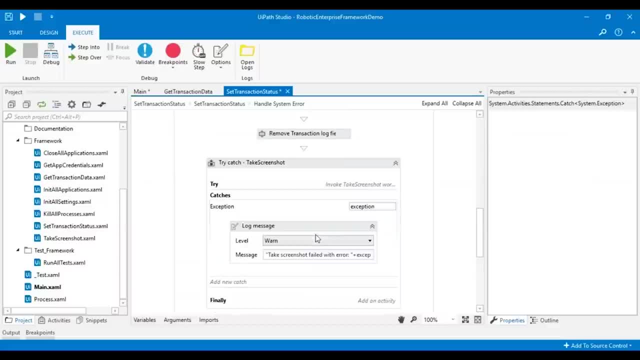 So this basically makes life easy for the users. apart from that, We also have a catch block, So basically, if the screenshot cannot be taken, then it shows a warning saying that you know the take screenshot failed with an error, right, So that's basically happening over here after that. 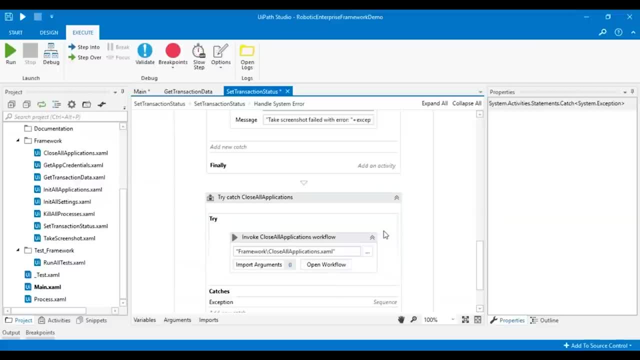 What you'll do is, after you define all the try-catch block of screenshots. Also, you have to finally close all the applications, right? So to finally close all the applications you invoke, to close all applications to XAML file from the framework folder again. 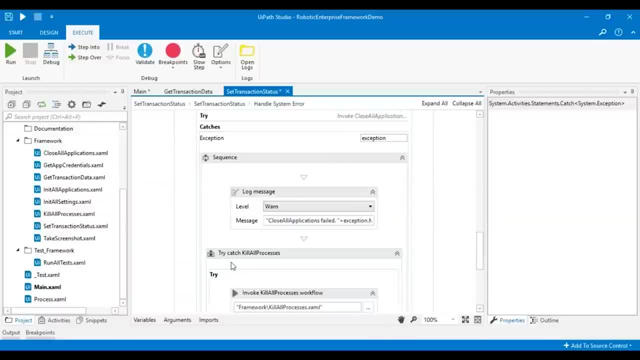 which basically closes all the applications. and then, if this also fails, what you can do is you can log a message of warning where you basically display a message saying that you know, close. all applications have failed, and then you again have a try-catch block which is kill all processes, right. 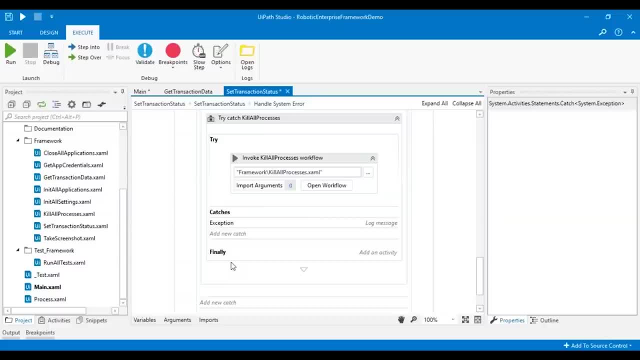 So if the applications cannot be closed, then you just kill all the processes to make sure that everything is closed, and then, if that also has a error, then you again throw an exception showing that you know there's some warning happening and then kill all processes. field right. 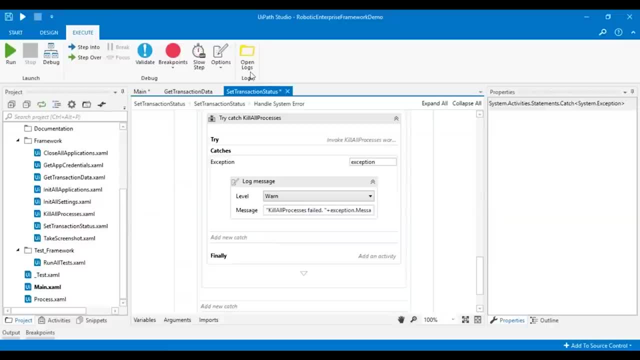 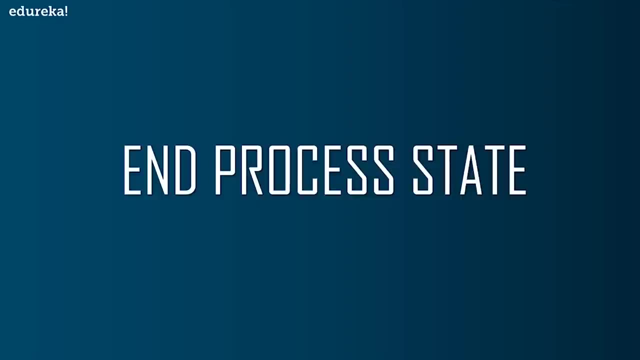 So this is where, basically, you want to close all the processes that are happening, right? So, guys, with this we come to an end of this process. transaction state. Now, finally, let's go to the final state, that is, the end process state. 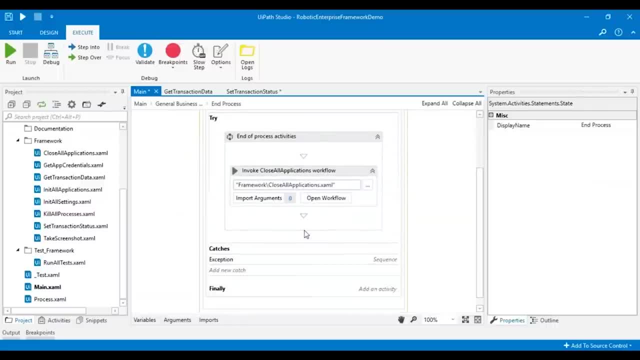 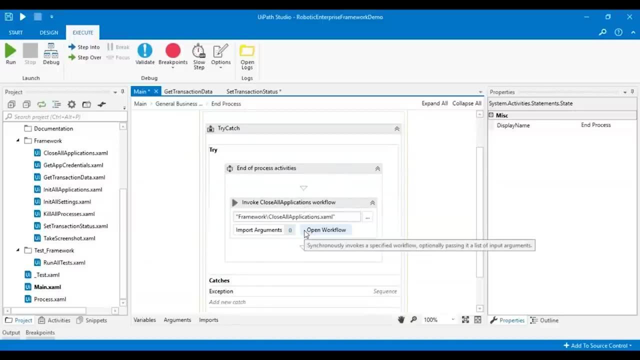 So end process state, as name suggests, basically is used to close all the applications. So it simply has a try-catch block. So the try block basically has invoke close applications workflow basically, which is used to close all the applications, and then if there's an error in that, then you just log a message. 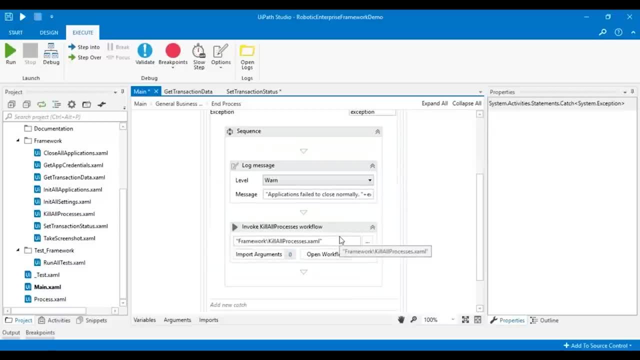 saying that you know applications close to pay normally. So then you have to basically invoke the kill all processes XAML file to just kill all the processes running right. and the kill all processes is against invoke from the framework folder, right? So with this, guys, we come to an end of the understanding. 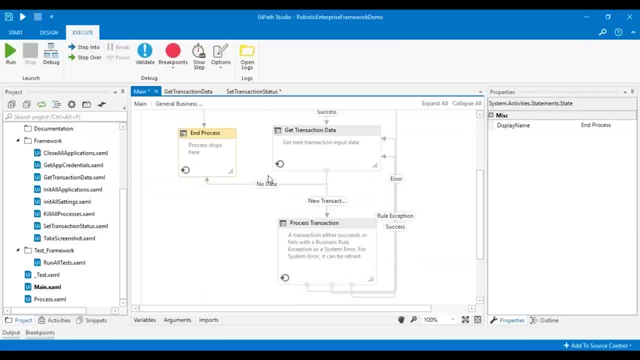 of the workflow of the reframework. I hope you've understood all the steps in detail and understood how the workflow of the reframework works. So, based on this concept, what you can do is for your business processes, you can change few files and then you can. 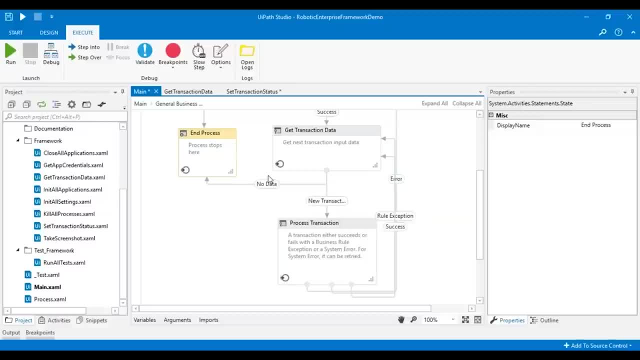 make sure how your process works in large-scale deployments, right? taking an example of a support ticket system: for every ticket that is generated, Maybe we just want to send an email, right? So, for example, we want to send it automated generated email saying that you know. 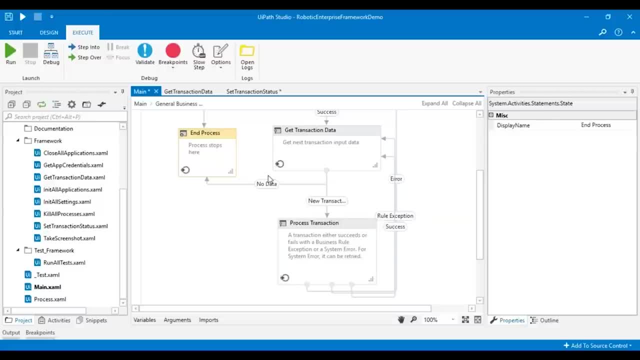 hi will be taking care of your problem, right. So what you can do is for each transaction item that you have. So over here the transaction item will be the ticket number. So for each transaction item, what you can do is you can just in the process transaction part. 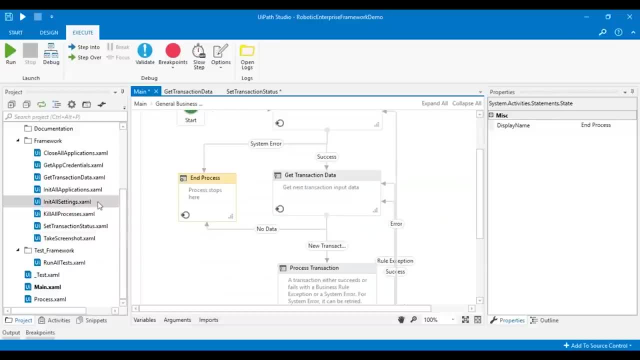 What you can do is you can configure the files of in it all applications where you basically initialize the application from where you want to send the email and then you finally can close all the transactions right. So this part I leave it to you, how you want to figure out. well, 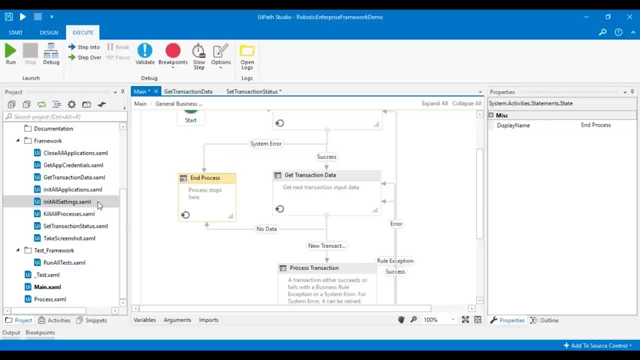 if you have any further queries related to the working of the re framework, please comment in the comment section. But before I close with the session, let me just take you through one more XAML file that you know you need to understand. that is basically the get app credentials. 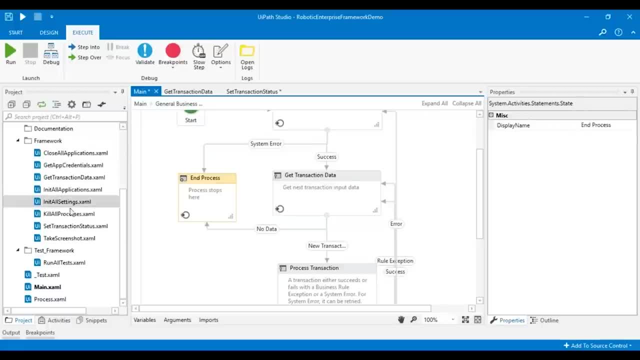 So, if you observe, in my session I've completed, I've explained you all the XAML files, All the XAML files that are present in the framework folder, but I skip the get app credentials XAML file, right? So let me just open this particular XAML file. 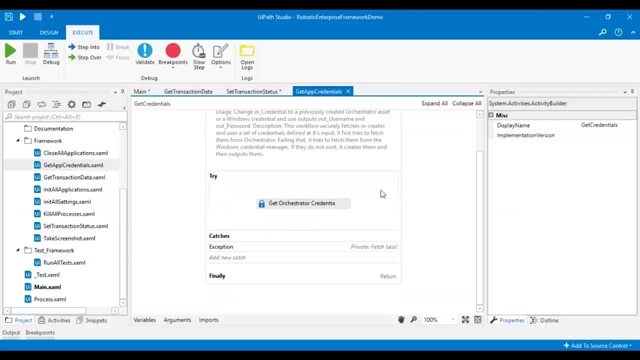 So when I open the XAML file, what you basically see is this: as the name suggests, is basically used to retrieve the credentials used by the robot to access different applications, right? So basically, we want to retrieve the data of a robot so that the robot can access different applications, right? 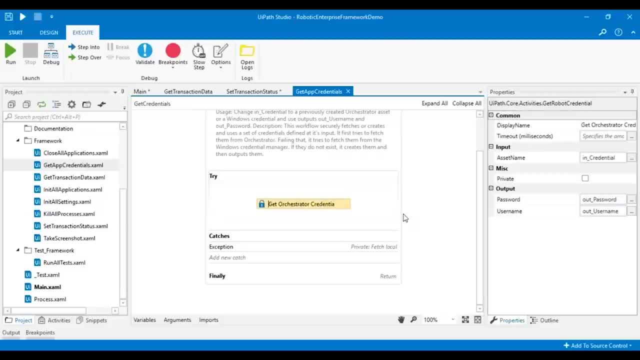 So a few ways to store the credentials is basically to store them in the orchestrator assets. So when we store the orchestrator credentials we can basically have a password and the username. if the retrieval of the orchestrator fails, then we basically can just directly catch an exception. 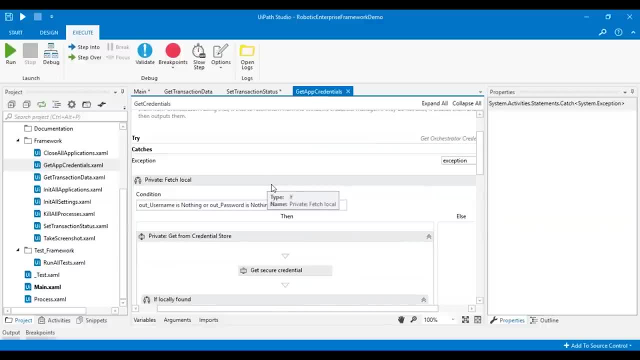 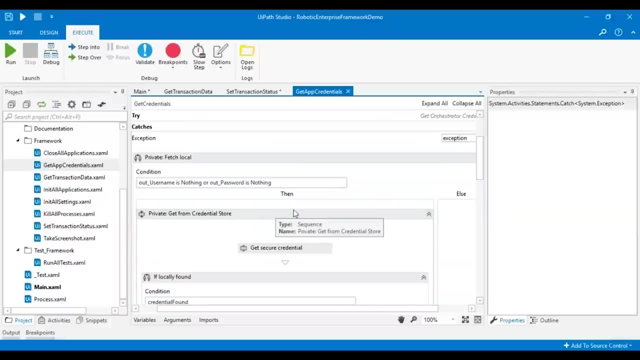 So over here in the exception folder, if I just click over here in the cat section, if I just click on that, you'll see that is an exception. It has a proper if condition. So if I use a name is nothing, or if our password is nothing, 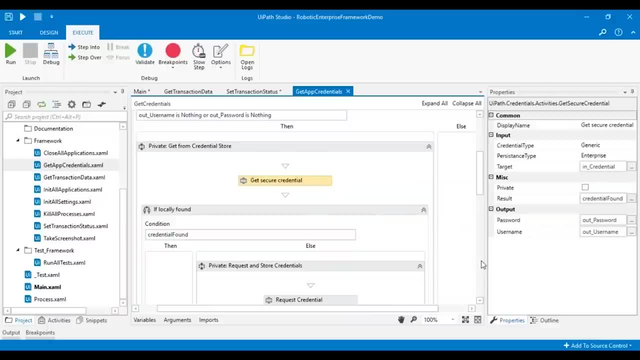 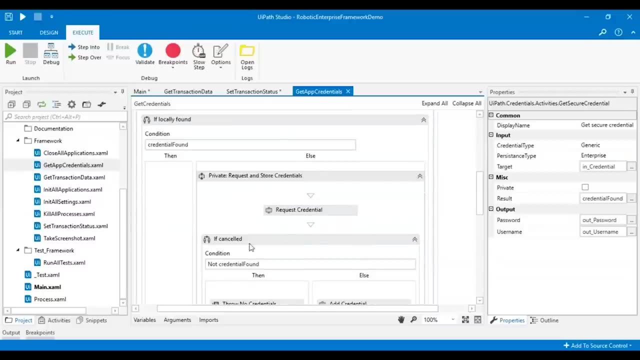 then what happens is that, basically, we have to get the credentials from the Windows Vault. So we are. you'll basically get the output of the out password and the username And then, if credential is found, what you basically do is you don't do anything. 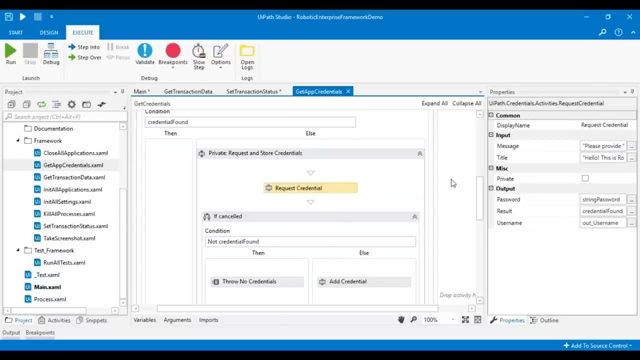 But yes, if you do not find the credential, then you again request a credential and then you can display a message saying that you know, please provide the credentials for access, and then the title of the message could be: hello, This is a robot. then you can mention the user name. 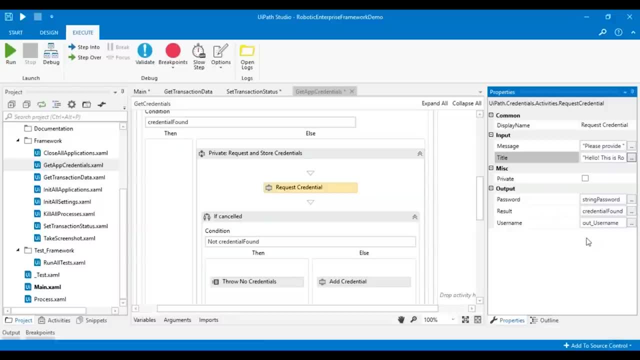 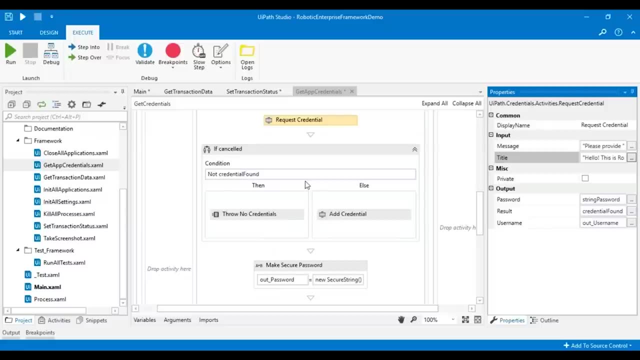 and password and those will be stored in the string password and the out username variables right now, once you give the credentials, you know, if it is not found again, maybe you know there's some error. Maybe you just might have skipped by not mentioning anything. 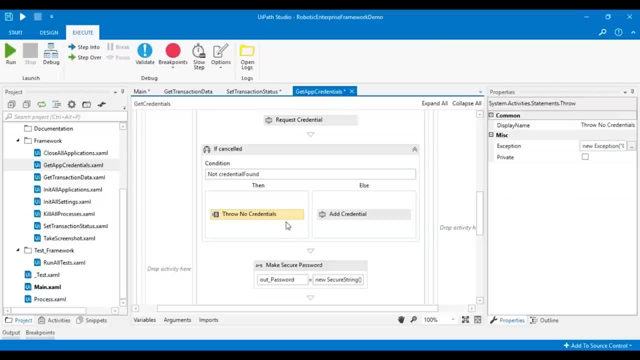 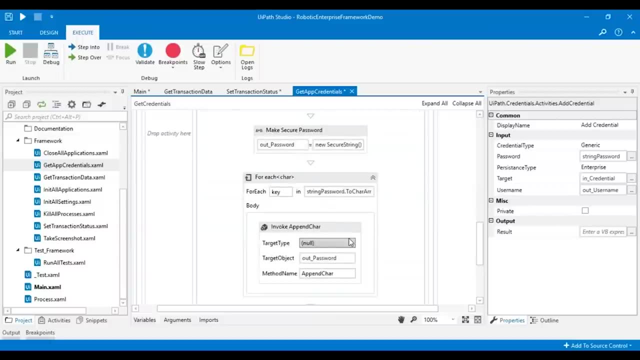 You can just throw an exception saying that you know it, there are no credentials, but else if there is data that you have mentioned, then you can just add this credential and then make the password to be secure now for each key in basically the password. what you can do. 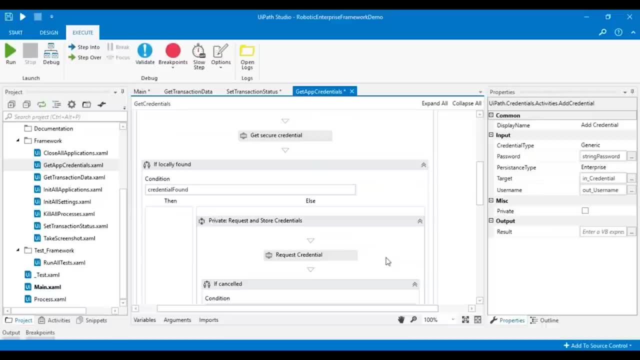 is, you can just encrypt that particular password and then finally use those particular credentials to access the rewards, to get the credentials of the rewards to access various applications, right. So basically, guys, this particular XAML file is just to retrieve the credentials used by the report. 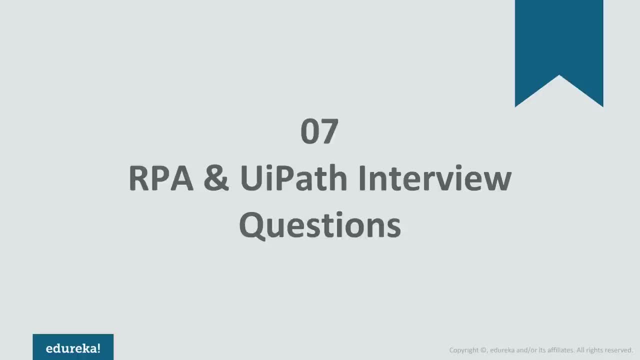 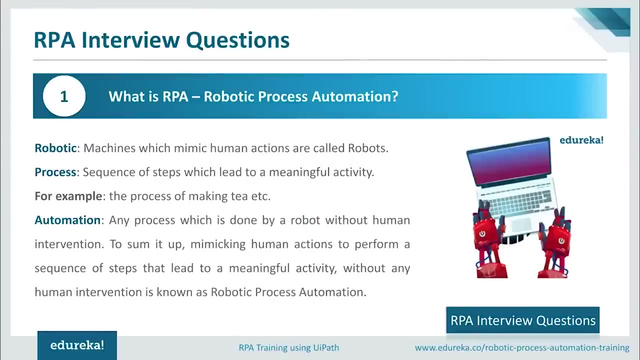 to access different apps Applications. So at number one, we have the most basic question, that is, what is RPA? RPA is an acronym for robotic process automation. So now let me explain you these terms- robotic process automation- one by one. when it comes to robotic, robotic are machines. 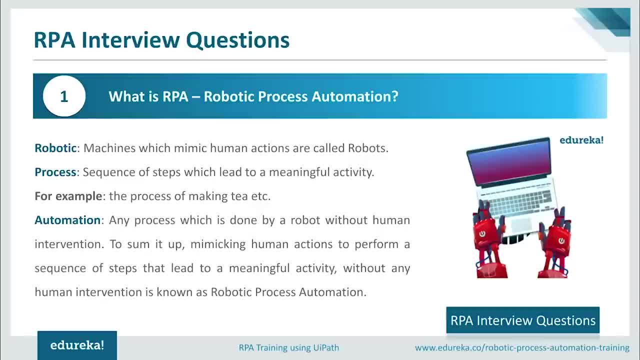 which mimic human actions. right So, all the machines which mimic human actions are called as robots. with robotic, It helps the human force to reduce their task force. right So, the robots do your work. You need not put your energy to do all those works. 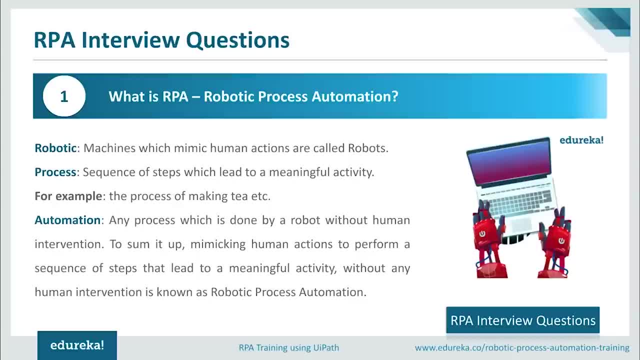 when it comes to process, process is basically a sequence of steps which lead to meaningful activity, right? So it could be a process of making tea, making coffee, making your cake or making your favorite dish- any process, right? any sequence of steps which lead to a meaningful 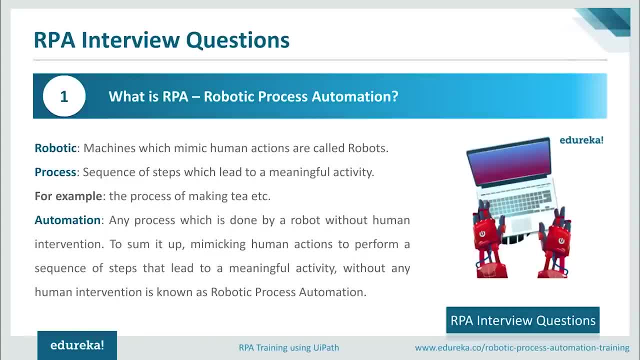 activity can be termed as process. So, for example, if you have to make tea, what is the process that you guys follow? you put in Milk, you put on tea leaves and then, once it is done, you just add a little bit of sugar and your tea is ready. 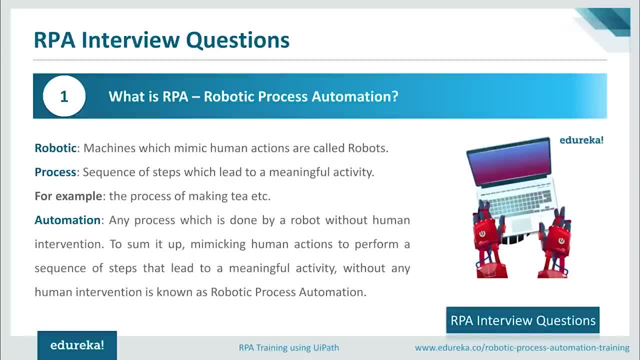 right. So if you have followed a sequence of steps to get the tea done, so that is process. So, when it comes to automation, any process which is done by a robot without human intervention is said to be automated. So any kind of process. it could be a simple one. 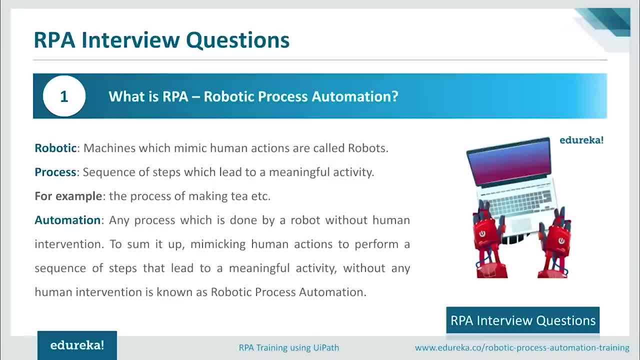 It could be a complex one. It could be any number of processes, right? So any number of processes which are done by robots without the human intervention is said to be automated. All right, Now, if you have to sum all the three terms together: mimicking, 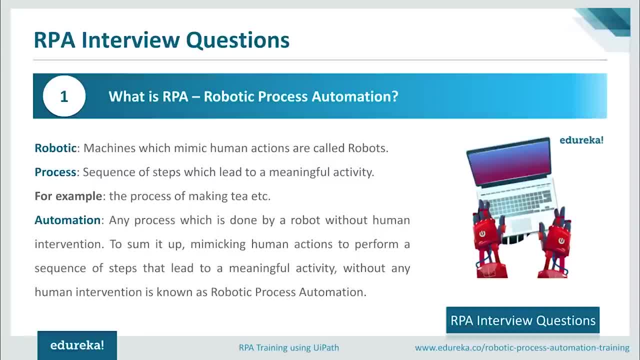 human actions to perform a sequence of steps that lead to a meaningful activity without any human intervention is said to be robotic process automation. So I hope the definition is clear for you. It's simple, right? each term has its own definition and you just have to sum all the three terms together. 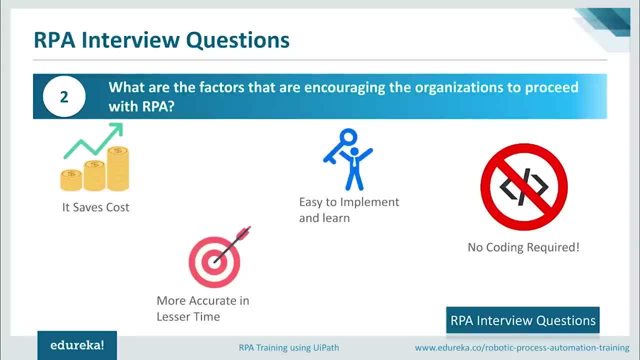 So now that you know what RPA is, let's move on and see what are the benefits offered by RPA. when you talk about benefits Of RPA, You obviously know that many large-scale companies like cab, Gemini, Deloitte, IBM, Accenture, use RPA in the scaling industry. 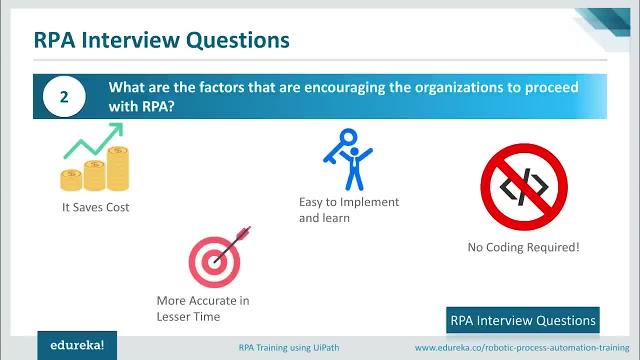 to run with their businesses, right. But why do they use RPA? That's because it saves costs, It's easy to implement and learn, It's more accurate in less time and there is no coding required, right? So once a company starts using RPA, it need not hire employees. 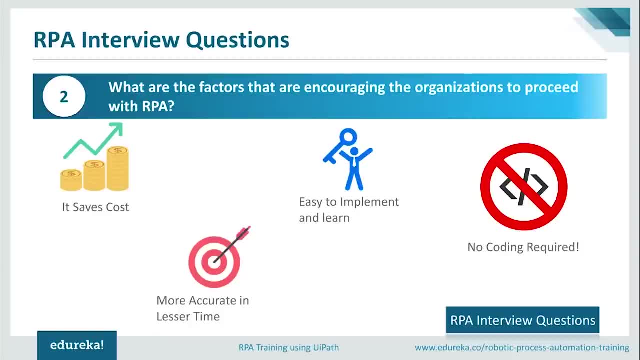 whose sole work is to do simple tasks. All they have to do is they just Have to get their work automated. So any company's goal is to get the maximum work done with less amount of time and less amount of cost right. So RPA is the solution to all these problems. 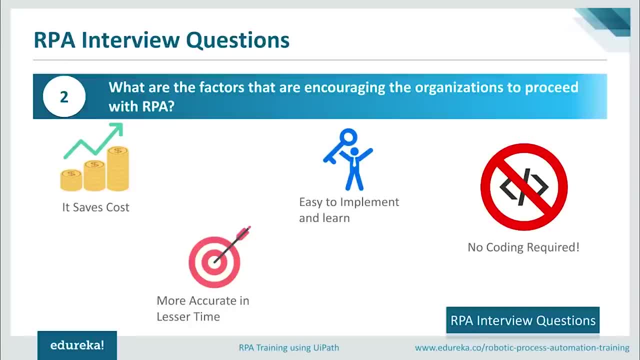 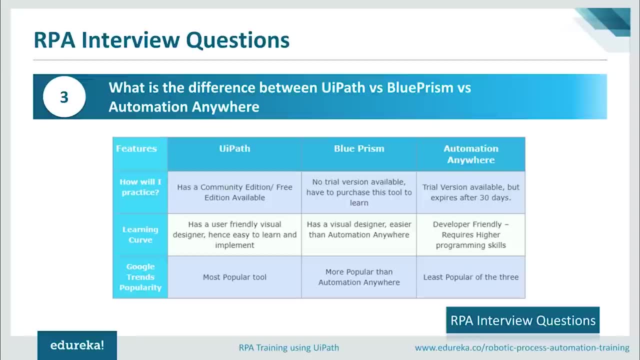 Now that you know what RPA is and what are the benefits offered by RPA, It's an obvious question that how do we implement RPA right? So to implement RPA, there are various tools like UiPath, Blue Prism, Automation Anywhere, Pega, WorkFusion and n number. 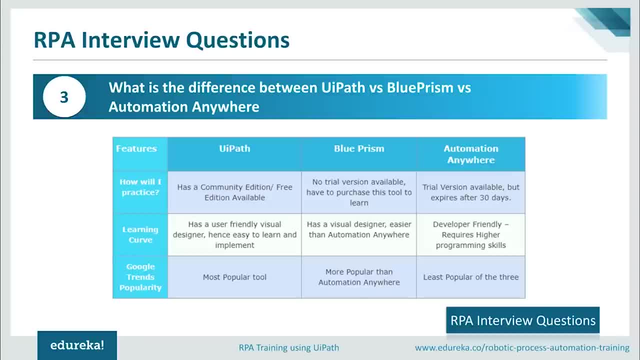 of tools, But the top three tools in the market are UiPath, Blue Prism and Automation- Anywhere. Now, this creates a confusion between all our minds on how do we choose between these top three tools, right? So when it comes to the trial version, UiPath offers a community. 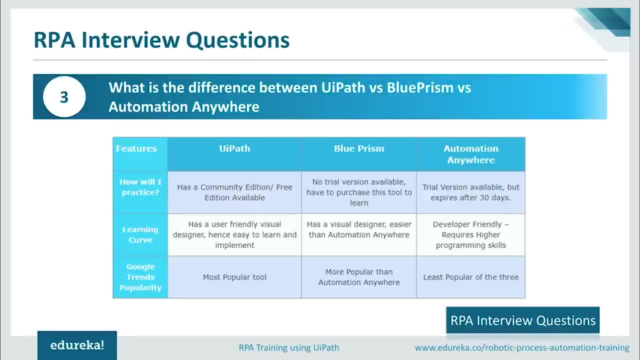 edition, which is basically like a trial version, where you can practice n number of tasks And once you think that you've gained expertise in the tool, you can buy the pro edition. When it comes to Blue Prism, Blue Prism does not offer any trial. 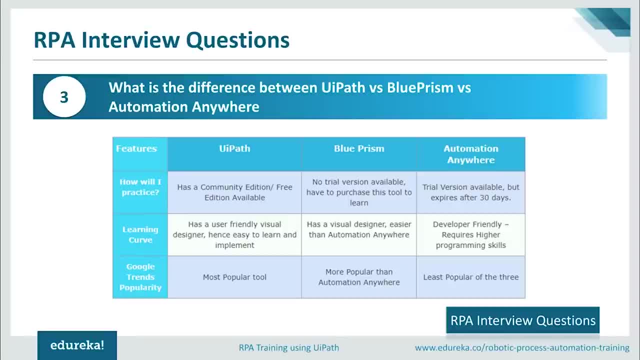 version. You can only request a company for the edition And if you think you'll purchase the tool, they'll send you with the license. After that, the Automation Anywhere tool definitely offers a trial version, but that is only limited to 50 tasks, right. 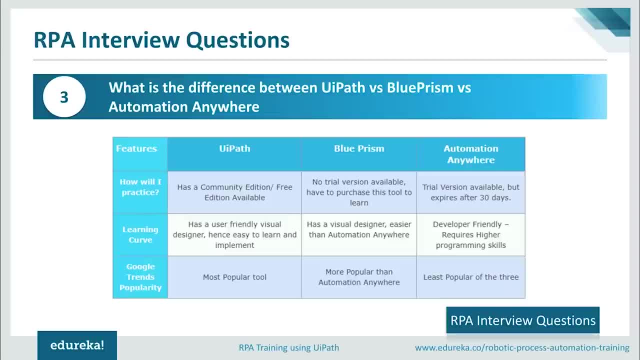 So 50 tasks are not enough to learn any tool. So that is the reason UiPath gains one point extra here. Now, if you go to the learning curve, UiPath is user-friendly, So it makes it very easy to learn and implement. Coming to the 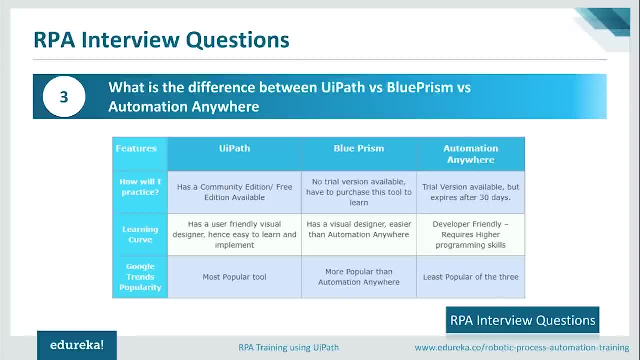 Blue Prism. Blue Prism has a visual designer And is easier than Automation Anywhere, but it is not better than UiPath since it does not offer trial version. And finally, the Automation Anywhere software that is definitely developer friendly, but it requires high programming skills, right? 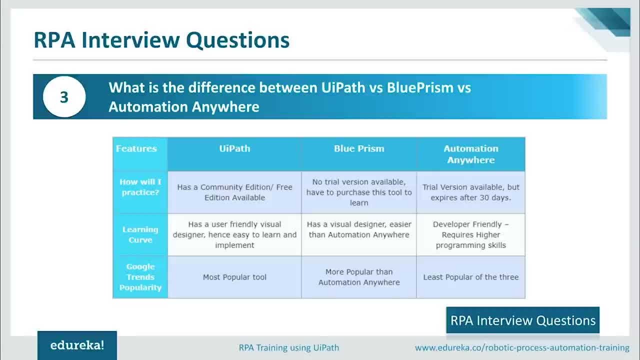 So any non-IT professional cannot go for this tool as they would not have any coding skills. And finally, if you compare on the note of the popularity, UiPath is the most popular tool because of its features. So I would say all the three tools are good enough to compete. 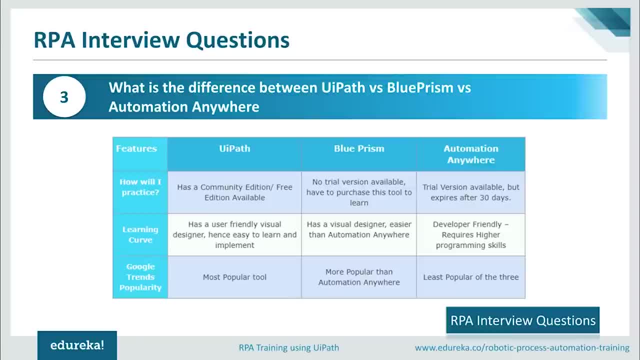 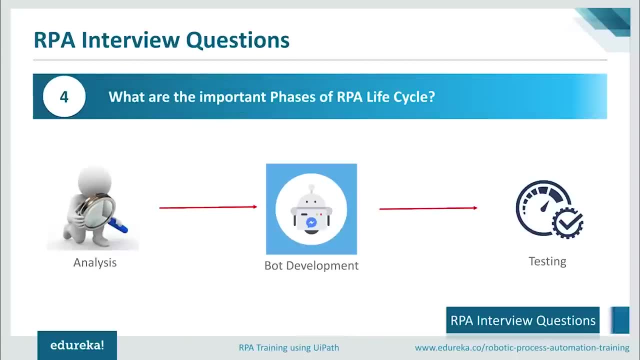 with each other, But I would say that you should choose for UiPath, since it helps you in all the ways right. So now you know what RPA is, what are the benefits, How can we implement RPA? But now let's get into the important phases of RPA life cycle. 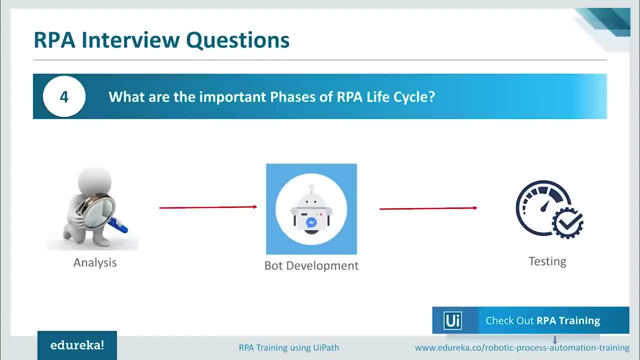 When it comes to the RPA life cycle, there are basically three phases. It is the analysis, the board development and the testing. When it comes to the analysis part, this is the first phase in which RPA begins with analysis, So business teams and RPA architects work together to 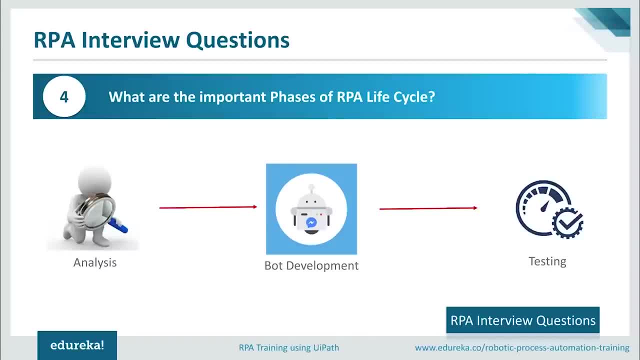 understand the business process for RPA development. The first phase is to analyze what is the problem and how do we solve it with RPA. So that is what we're talking about here. The next phase is the board development. So the RPA developer team starts working on the requirement in. 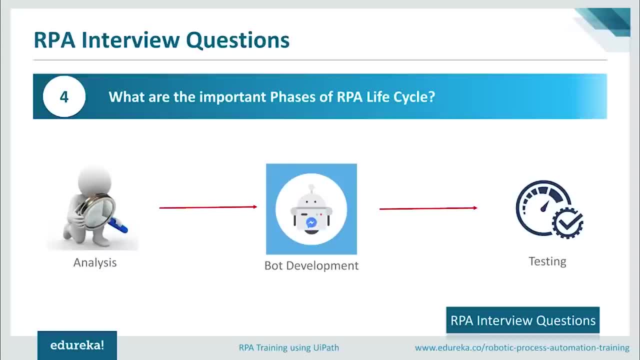 their environments right. So whatever input they get from the analysis phase and they understand what environment has to be built, It is in the board development phase that they start building the environment. Now, after the analysis and board development phase is done, It comes to the testing phase, where they have a separate testing. 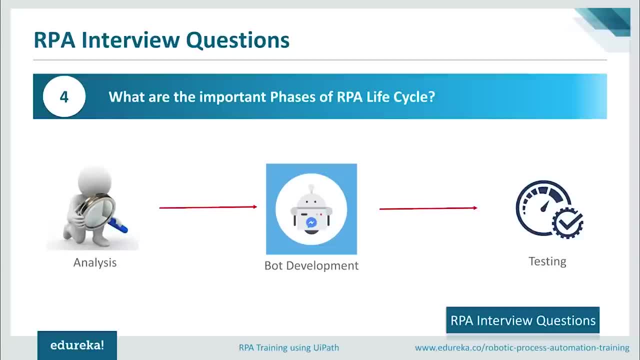 team which performs the quality analysis like the normal STLC flow right. So the best practice is to have a dedicated testing team which performs the quality analysis on the develop board. So in this testing if they find out any errors or bugs, it goes. 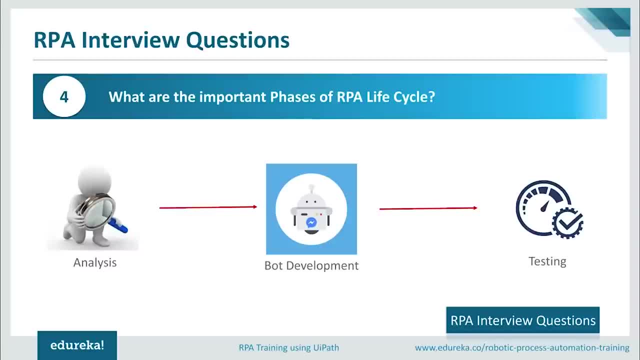 back to the board development team and they again start improvising on the built board. Now, after these three phases are done, the board is ready for distribution and enters the maintenance phase, where the board is performing the automated task and is maintained by the maintenance team. 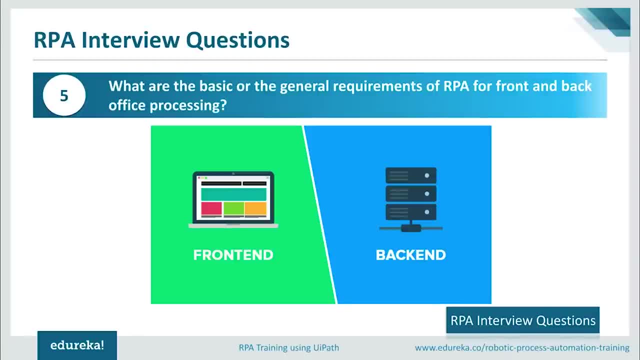 Now, after understanding the phases of RPA lifecycle, what are the basic general requirements of RPA for a front-end and back-end office processing right? So it's a fact that RPA is well known for its flexibility and its capability to meet the robust IT standards without compromising. 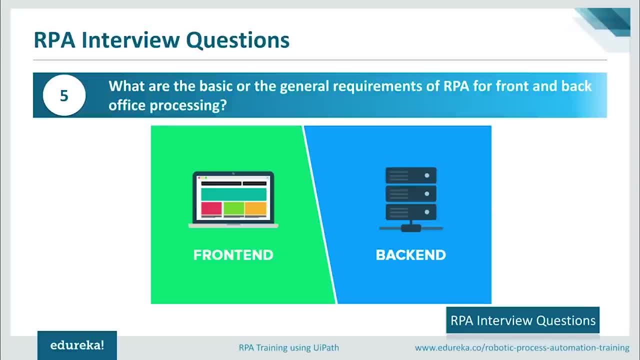 the security right, It is possible to use the robotic software for the front-end and back-end office. Now, what are the requirements required for For the front-end and back-end office is the question. Well, the answer to this question is that most of the requirements. 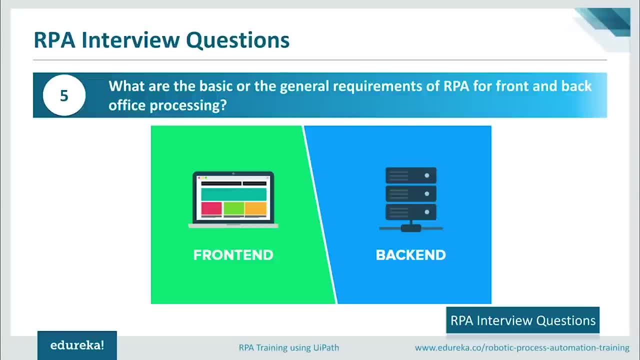 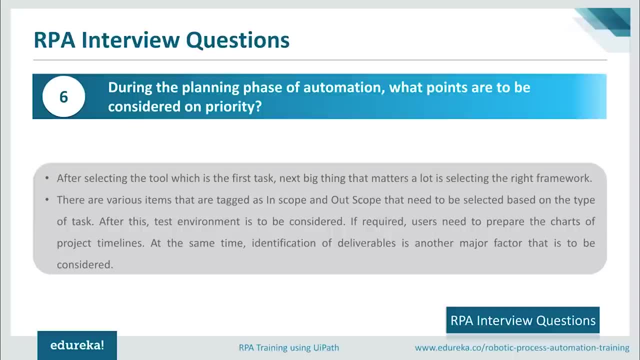 are same for both, So the users need not worry about different configurations, as the same configuration can be easily deployed and the results can be derived as needed. So now let's move on to the next question and see what are the points that are to be considered on priority during the planning. 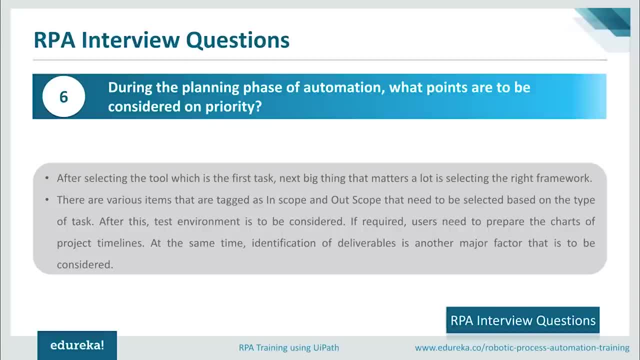 phase of automation right. So well, I could say, after you select the tool, which is the first task, The next big thing- That is a lot- is the selection of the right framework. There are various items that are tagged as the scope and out of. 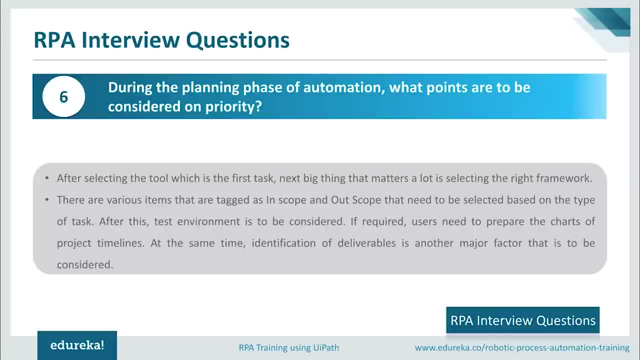 scope that need to be selected based on the type of task, right? So some things would be under the scope and some things would be out of the scope. So you have to decide on that matter, on the framework and the scope, after you're done with that. 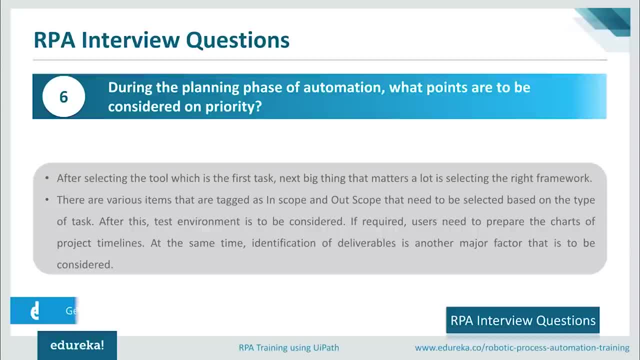 You have to test the environment, which is considered right. So suppose you take an example of a company trying to automate a task. What are they going to do? As I told you before this, first analyze the problem and then they'll build a board. once they're done building the board, 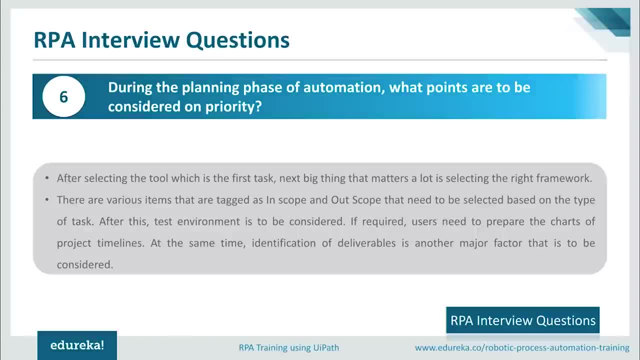 They have to test the environment, which is considered. only. if the considered environment matches the requirements, It moves on to the next phase. as they still need to consider various environments right If required. users also need to prepare the charts of project lines so that they have a proper timeline on by which time 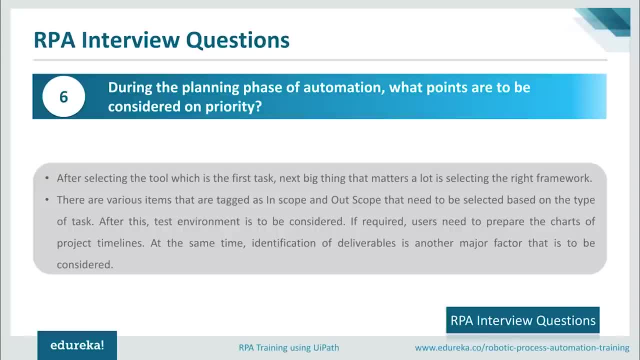 they're going to solve the problem and then automate the task. So, in short, you have to select the right tool for the task and then you have to select the framework. Once it is done, You have to check on the scope. which task are out of the scopes? 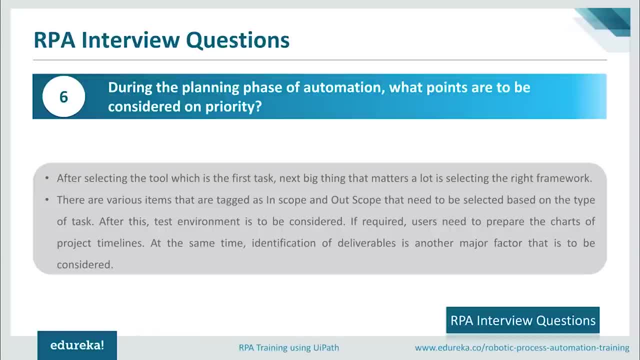 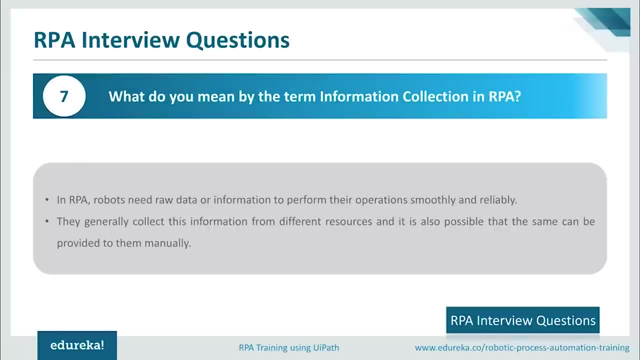 and which task are inside the scope. Once you're done with all of them, You have to test the environment which is considered, and then you have to identify the deliverables right. So, moving on, we have a question, that is: what do you mean by the? 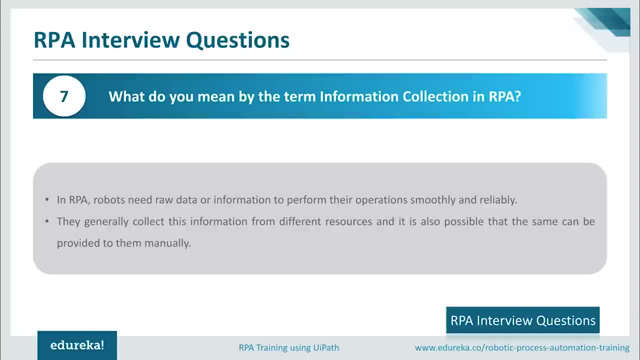 term: information collection and RPA. It's a known fact that any task that you do, you first need to collect a lot of information based on it right. So what is the meaning of information collection in RPA? Well, in RPA, robots need raw data or information to perform their 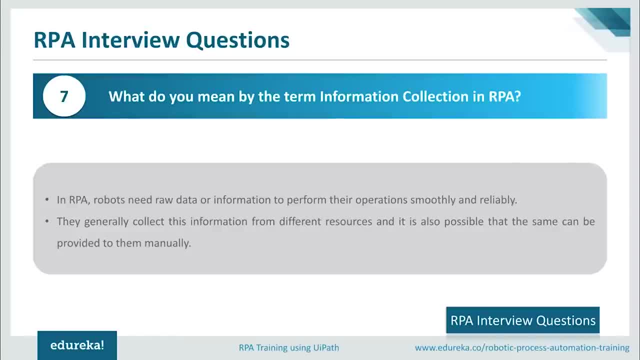 operations smoothly and reliably. That's because they're not dependent on humans, right? So they need all the information already stored in the system so that they can function properly. Generally, they collect this information from various sources, and it is also possible that the same information can be. 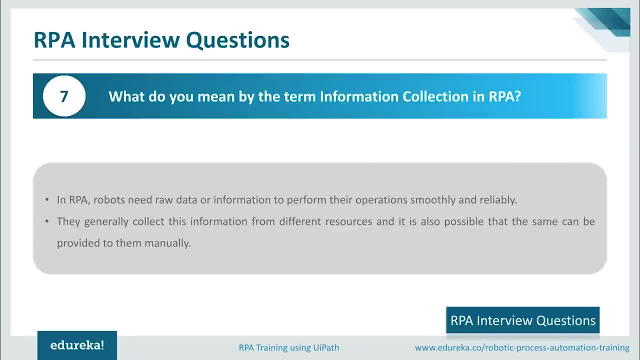 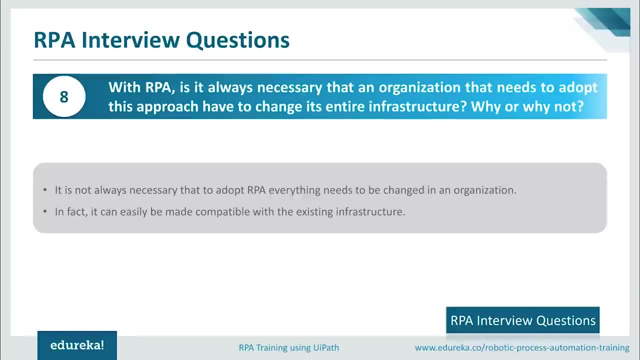 provided to them manually, right? So humans can provide this information to their boards, or they generally collect information from various resources. So that is the meaning of the term information: Information collection. All right, So now let's move on to the next question, which is a myth. 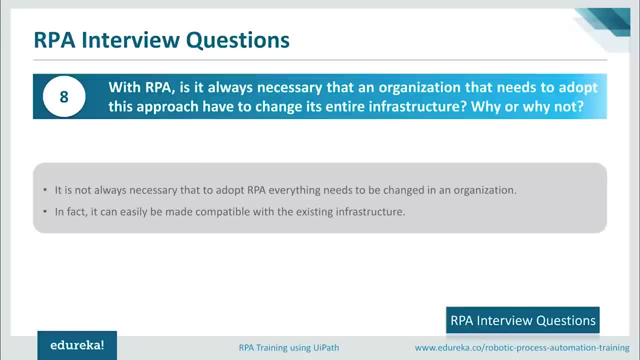 about RPA, that is, is it always necessary that an organization that needs to adopt this approach have to change their entire infrastructure? if they have to change, then why do they have to change? or if they don't have to change, then why not? Well, the answer to this question is very much scenario based. 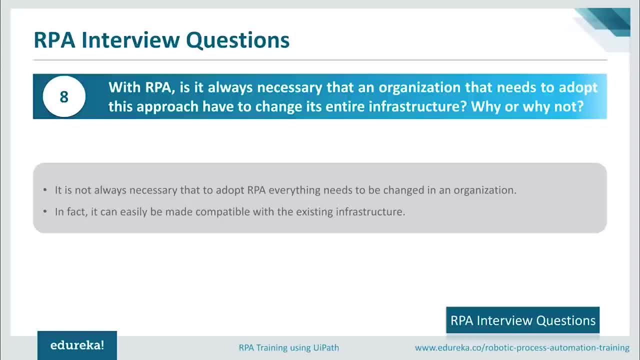 right. So there could be scenarios where the company is wanting to adopt RPA, have to change the entire infrastructure, and they could be scenarios But the companies need not change. Well, let me tell you, guys, that it is always not necessary to change everything to adopt RPA in an organization. 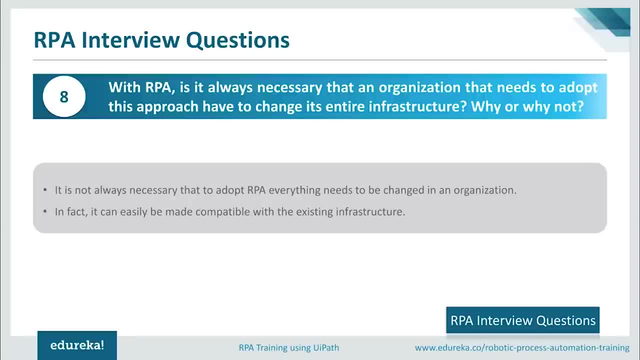 In fact, it can be easily made compatible with the existing infrastructures. This is mainly due to the fact that the latest robotic software and the tools in RPA do not face any compatibility issues easily and can simply enable the organizations to keep up the pace. 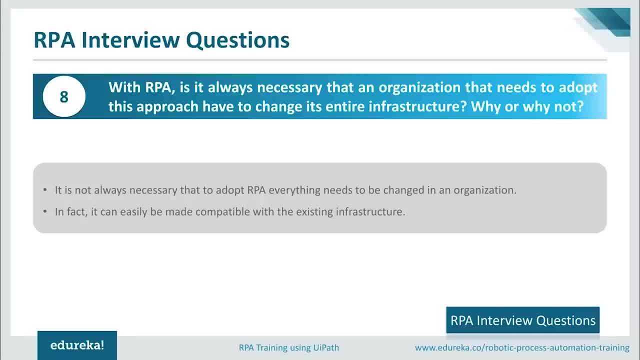 right. So if any company is trying to go to the approach of RPA, then that doesn't change. It doesn't mean that they have to pull down the complete systems to deploy RPA. In fact, RPA doesn't face any compatibility issues and makes 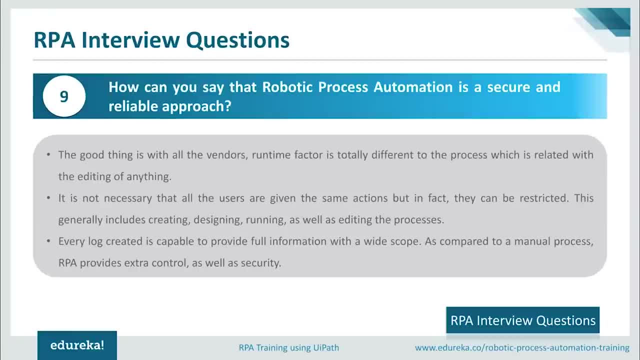 it easy to deploy this in their organization. Now, once a company has gone for an RPA approach, how do you say that the robotic process automation is secure and a reliable approach? So there could be a lot of questions about security, reliability and everything. 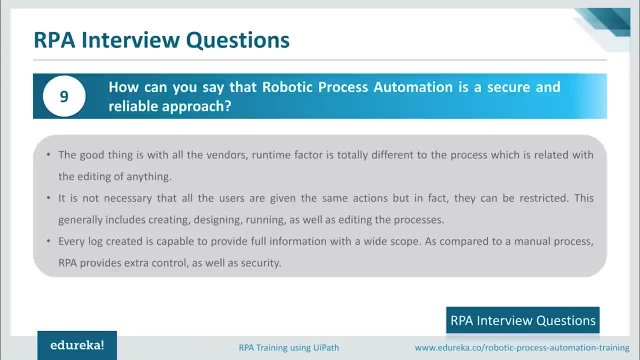 But how can we justify the fact that robotic process automation is a secure and reliable approach? Now, when you talk about the factors such as reliability and security in RPA, the good thing about RPA is that the runtime factor is totally different to the process which is related with anything of editing right. 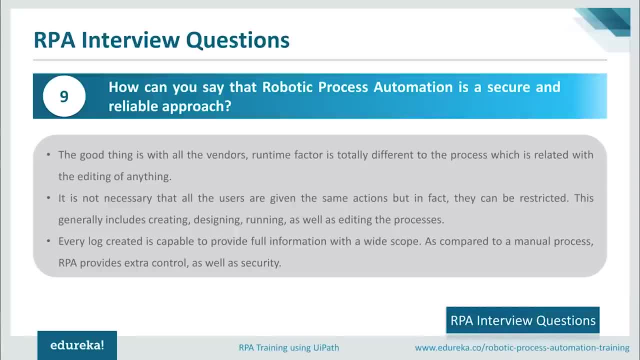 So it is not necessary that all the users are given the same actions, but in fact they can be restricted. So what I'm trying to say here is that a user carrying out a task will be only given access to that particular task. He or she will not be given access to any other task. 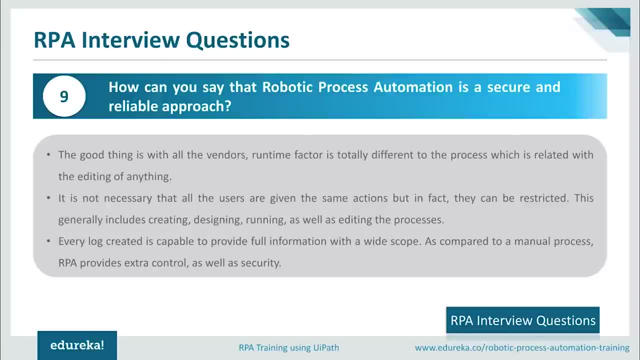 So this generally includes creating, designing, running, as well as the editing the process. Every log created is capable to provide full information with a wide scope, So there's complete information about every activity performed, All right as compared to the manual processes RPA provides. 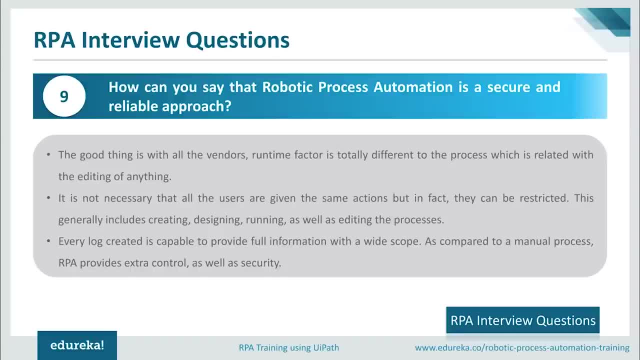 extra control as well as security. So when you compare to carry out a task with a human approach and an RPA approach, I would say RPA approach is always better in the matter of security and reliability. as humans can fall sick, There could be a leak of security with humans, but when? 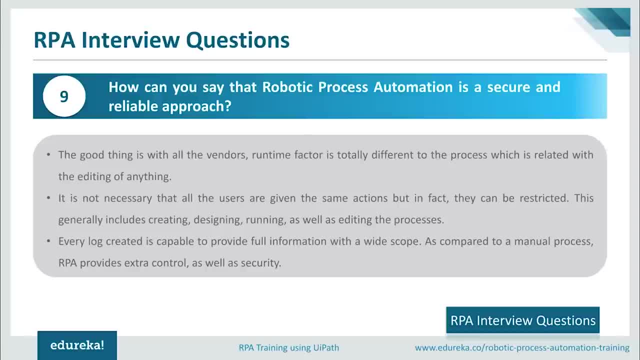 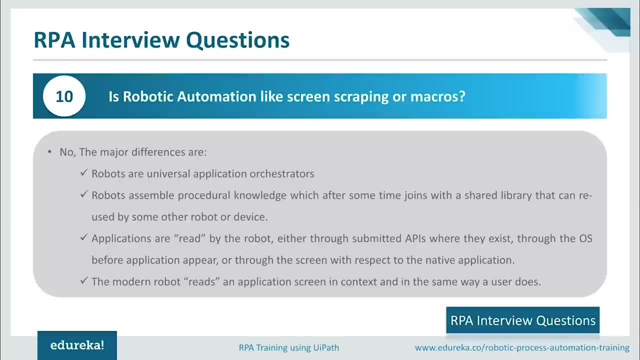 it comes to robots, they're always working 24-7, with more accuracy and also with more security. Now let's move on to the next question, which is: is robotic automation like screen scraping or macros? The answer to this question is no, as managerial robotic automation. 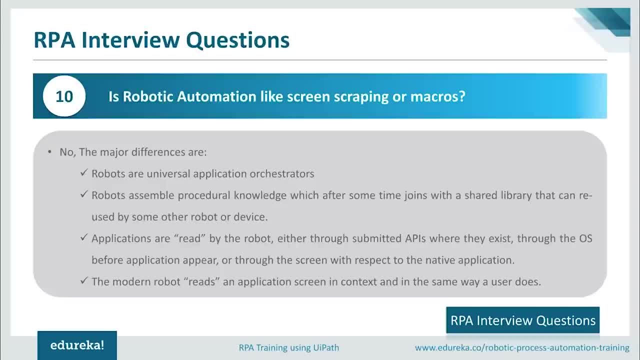 is a generation on from old technologies like screen scraping or macros. The major differences between these two are: robots are universal application, So any application that can be used by a man can be used by a present-day robot, whether mainframe or bespoke application or web service enabled application or any other third-party. 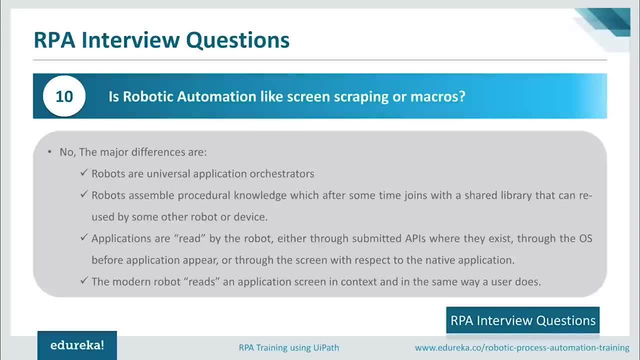 API hosted service. robots assemble procedural knowledge which after some time joins with the shared library. that can be used by some other robot or a device, right? So if you store some information in one robot, that can be reused again and again with n number of robots, now also applications. 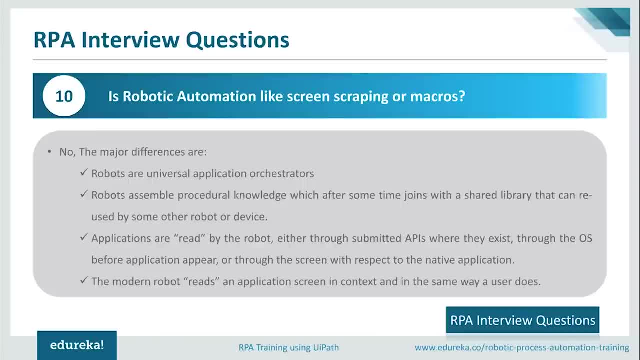 are read by the robot either through the submitted APIs, whether they exist through the OS before application, or through the screen with the respect to the native application. So therefore, I would say robotic automation is not like screen scraping or macros. Its work is to automate the components deal with perceptibility. 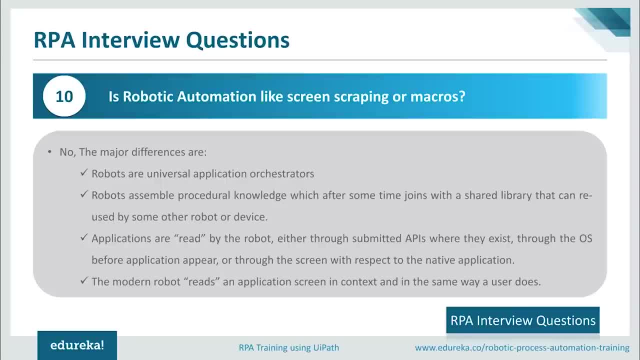 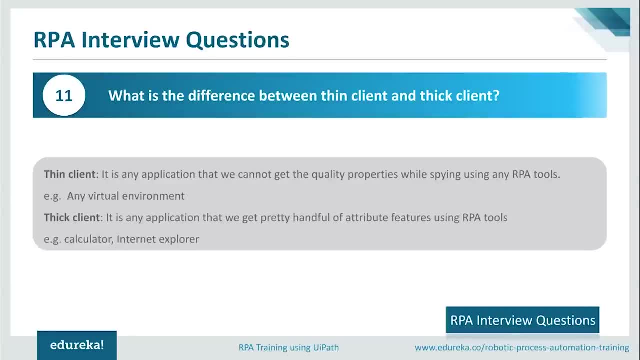 also work on configure management and also deal with debugging right alive. So now moving on to the next question. the next question we have on the list is: what is the difference between a thick client and a thin client? The term thin client is used to describe an application that. 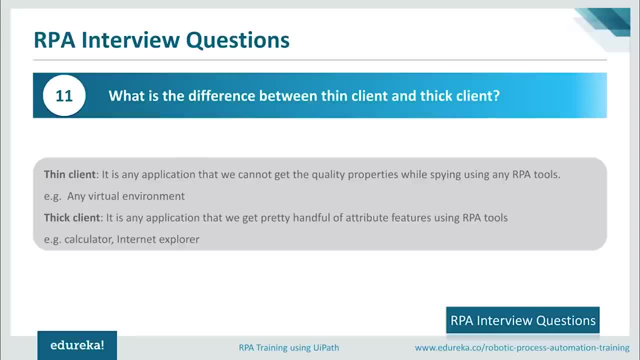 does not run on any local environment, right, So it basically uses a client server architecture. in this kind of applications, We do not get the quality properties while using any kind of RPA tools. So, for example, if you talk about Citrix or any virtual machine, 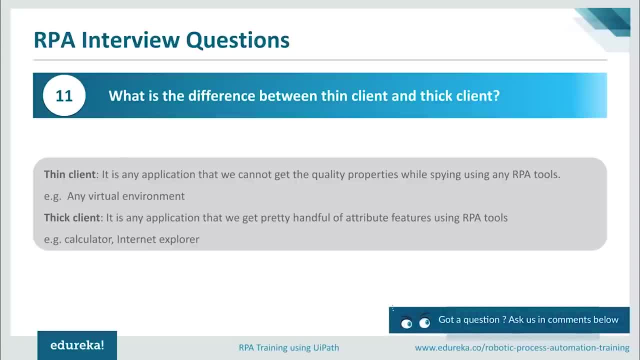 then these kind of applications to come under thin client, whereas a thick client application is the one in which it is directly installed on the local machine, like blue prism itself, Right. So in thick client applications we get a pretty handful attribute of features using RPA tools. 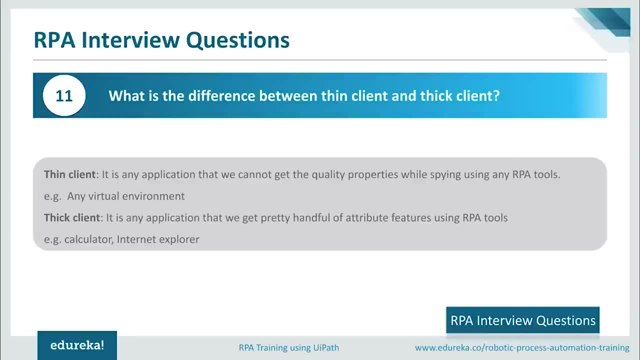 So, for your better understanding, let me give you an example of a simple analogy, and analogy could be to think of a service of a thick client application as having a landscape made of buttons, fields and checkboxes right, Whereas a thin client application is smooth and featureless. 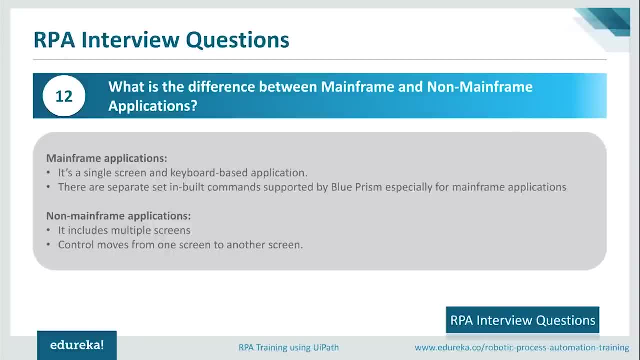 Now moving forward to the next question on the list we have: what is the difference between a mainframe application and a non-mainframe applications? Well, guys, this is the basic question that is always asked, that is, what is the difference between a mainframe and a non-frame? 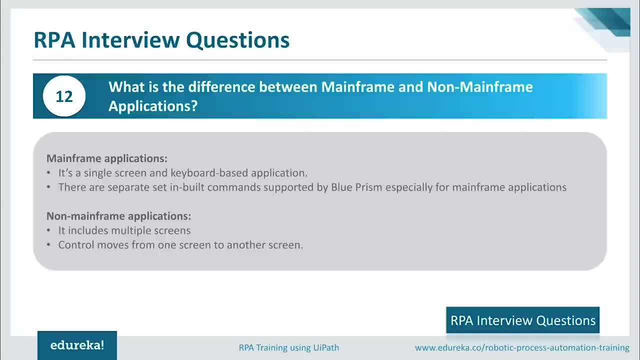 application. Well, when you talk about mainframe applications, they are single screen and keyboard based applications, right. When it comes to a non-frame applications, these kind of applications include multiple screens, So control moves from one screen to another screen. So it basically depends on the complexity of the task that makes. 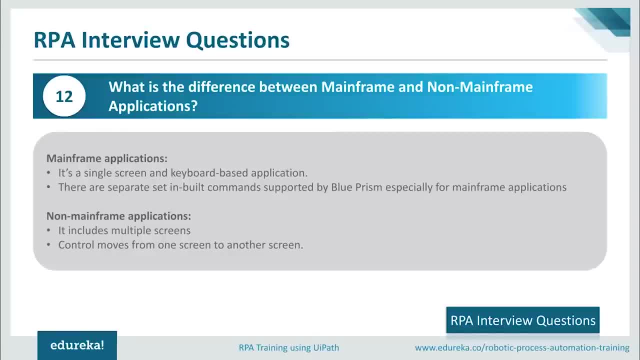 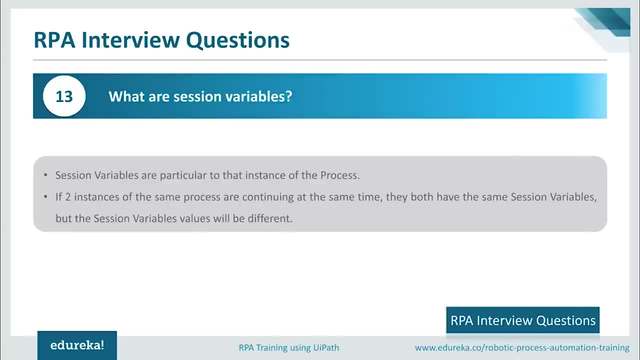 you choose between the mainframe application and the non-frame application. All right, now that we have looked into various different kinds of questions, Let's move on to the next question, which is: what is session variable? Well, when you talk about session variables, session variables. 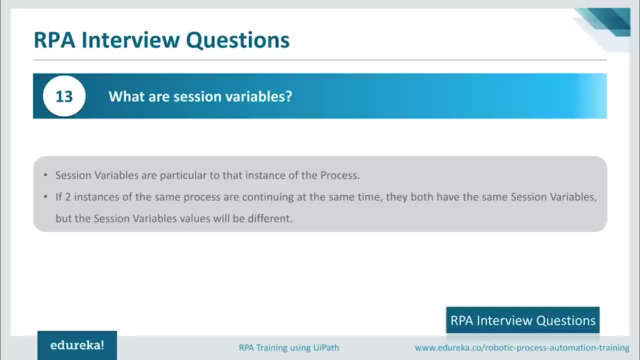 are particular to the instant of the process, right? So if there are two instances of the same process continuing at the same time, they both have the same session variable, but the session variable values will be different. that is because there are two different instances. 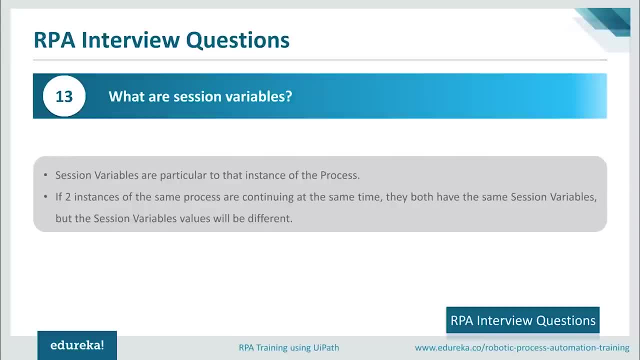 All right. So a session variable is very much particular to the instance of the process. So if you have one process running with M number of instances, all these M instances would have the same session variables but with various values. All right. so, guys, that were some basic questions related to. 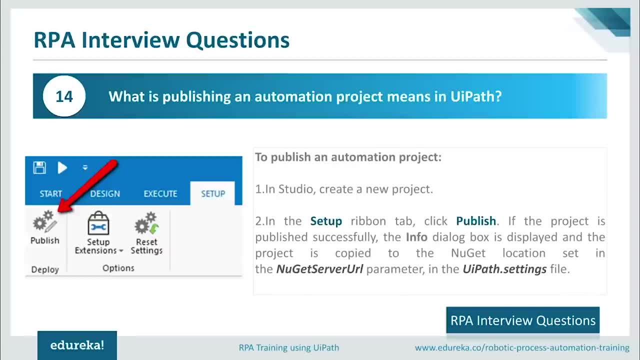 the RPA technology Now moving forward. Let's look into some questions related to UiPath. So the first question that we have here is: what do you mean by publishing an automation project in UiPath? right? So for any interview that you go for a RPA developer role, the 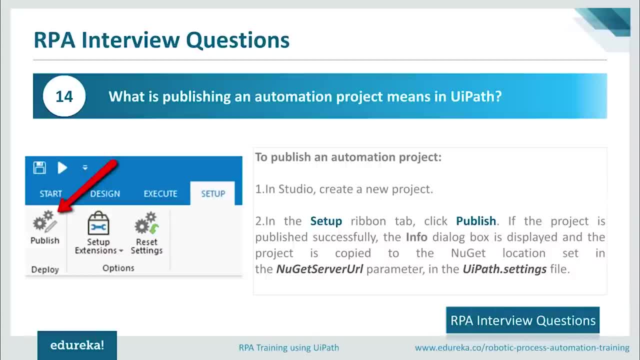 basic questions that you would be asked Would be about the basic knowledge that you have on RPA. after that, they would be interviewing you on the basis of the tools that you have explored. So over here we have a basic question, that is: what do you? 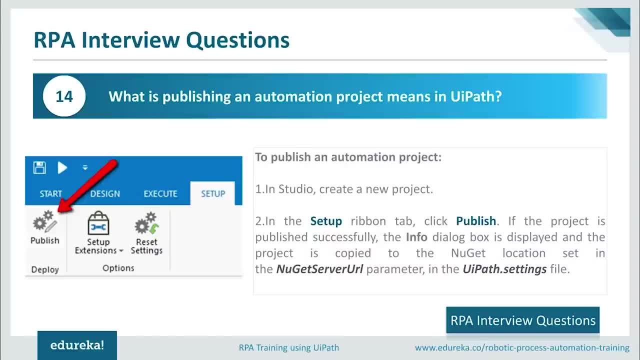 mean by publishing an automation project in UiPath, Right? Well, publishing an automation project means archiving it and all the other files in the folder so that it can be sent to the robots and then be executed, right? So it basically means that you archive all the files in your 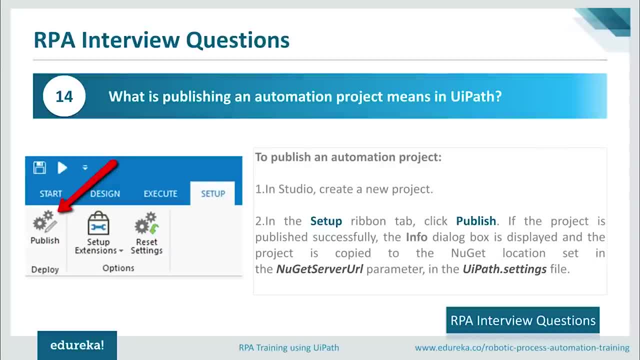 project and then you send it to a robot so that the robots execute your work. If you're connected to the orchestrator through a robot, the automation project is sent to the orchestrator feed and then it is displayed in the packages page from here. 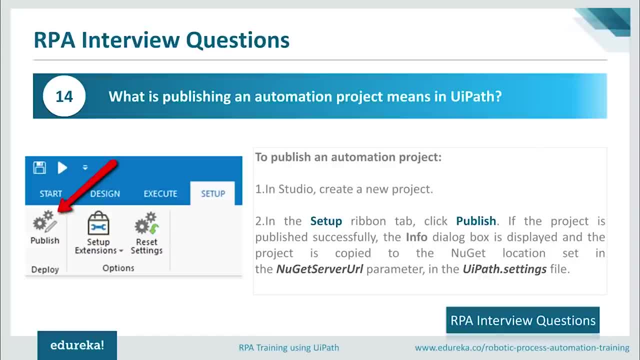 You can distribute it to all the robots by assigning the package to the environment, right? So basically you're trying to create a process here. If you're not connected to the orchestrator, the automation project is sent locally to the studio feed. So basically this can be done really easily by using the 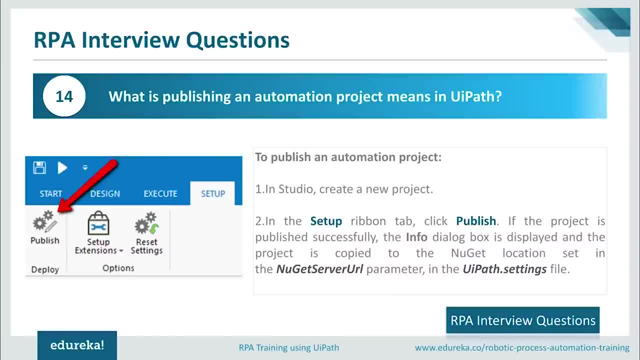 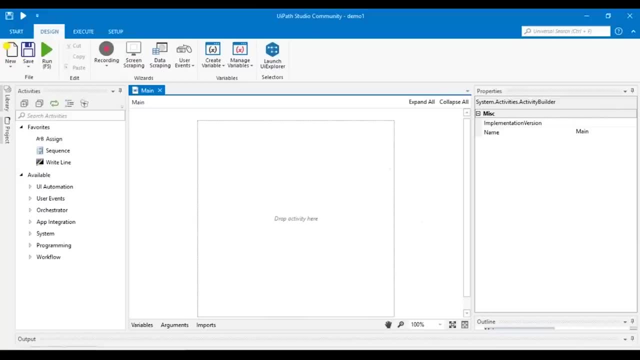 publish button on the setup ribbon tab. So let me just open My UiPath tool and show you where is this button right. So this is what I was talking about. This is the ribbon part, and when you open this ribbon you see this publish button. 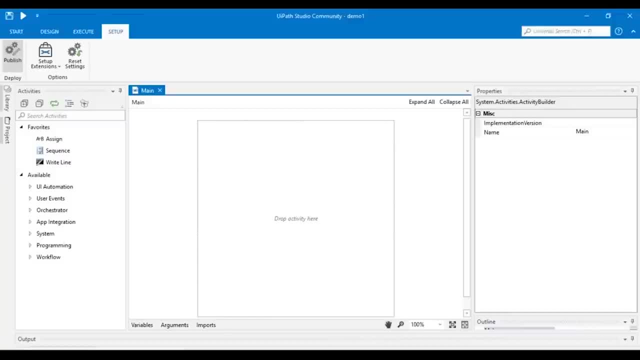 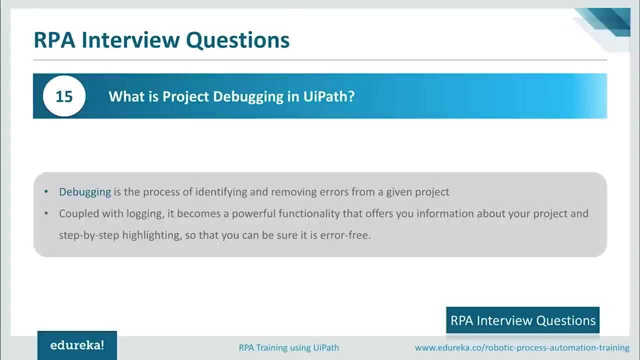 So this is where you have to press to publish your automation project. All right, So, as you guys know that we're discussing about the UiPath tool, sometimes many interviews ask you on the different activities that you can perform on the tool. So now let's look at the next set of questions in which we're 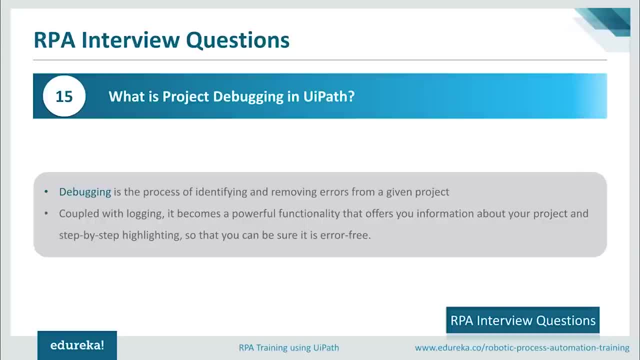 going to discuss How to perform various steps for different activities, right, So next in the list We have: what is project debugging in UiPath? when you talk about debugging in layman terms, what do you understand by debugging? debugging is the process of identifying and removing errors. 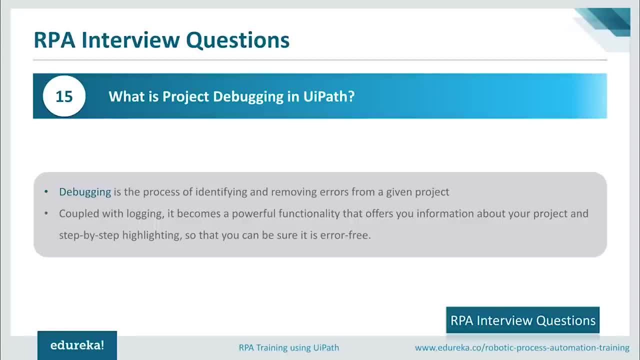 from a given project right. So whenever you identify the errors and then you remove it, that process is known as debugging. So when you couple it with logging, it becomes a powerful functionality that offers you information about your project and step-by-step highlighting right. 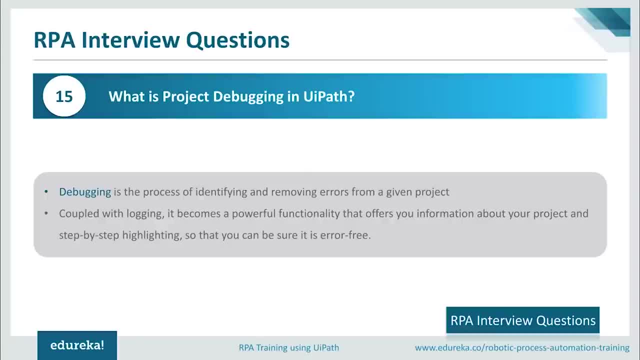 So if you perform a complex task with debugging, you can ensure that your project is error-free. So I've told you this term logging here, right? So what does logging enable us to do? logging basically enables us to display details about what is exactly happening in your 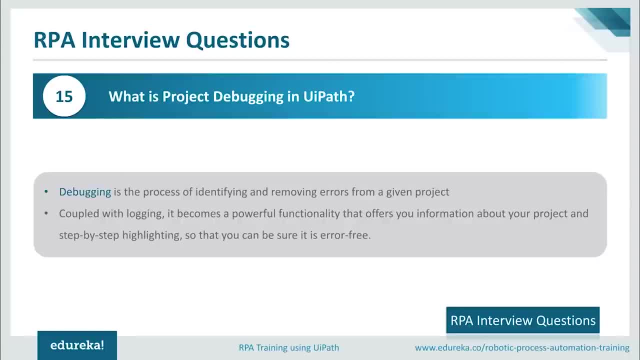 project in the output panel. I'll just show you in the demo in a while. This in turn makes it easy for you to debug the automation. So debugging makes your project error-free and logging enables you to display the details right. So both of them make a good combination to. 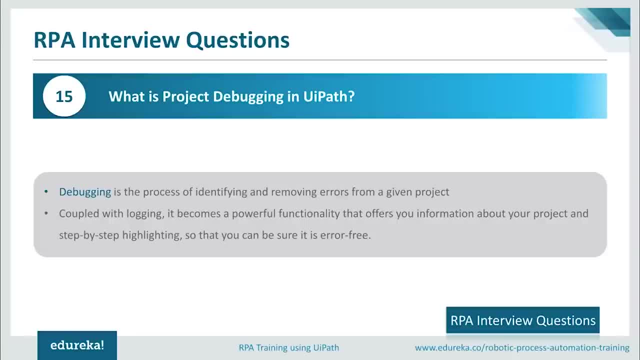 Secure to your project to be error-free. All right, now that you know what project debugging is, Let's look into the steps on how you can debug your projects. But before that, let me just preview a little bit about break points, right? 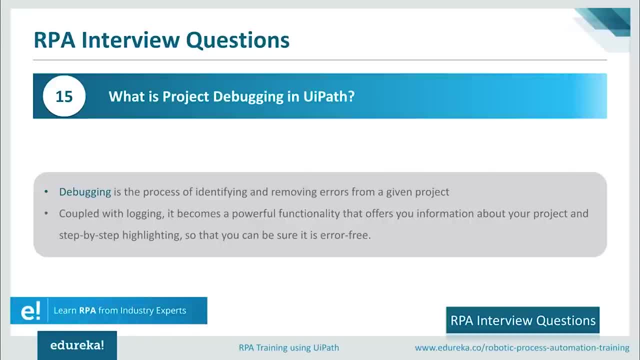 So when I've interview ask you about debugging, he asks you about all these terms: logging, breakpoints and debugging, right. So basically, breakpoints enable you to pause the execution of a project so that you can check its state at a given point. So when you run large, complex tasks, you can stop the execution. 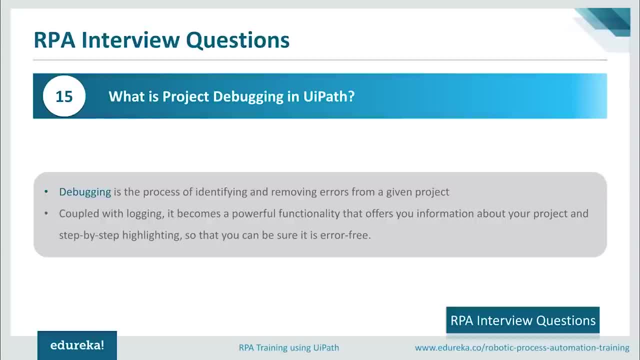 in between and check the state of its running, So that helps you to identify errors and debug them. So, as I said, let's look into the steps on how do we actually debug projects. So let me just go to my uipath tool. 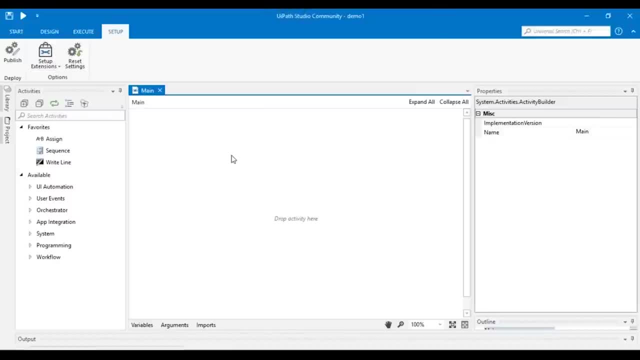 All right. so I'm going to create a short demo in which I'm going to show you how you can debug your project. So for that, I have to search for the flow chart activity And then drag and drop it in the workspace. All right, after that, I'm going to include an input dialogue. 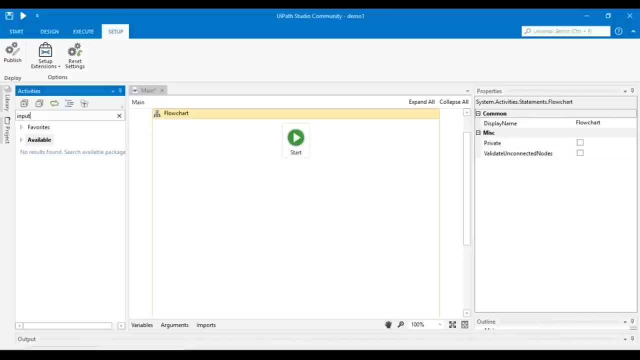 the message box And the log message. So let me just search in the search bar for the input dialogue. Let me just search for a log message And the message box. So guys don't worry about what all these are. I'm going to brief you a little bit about it. 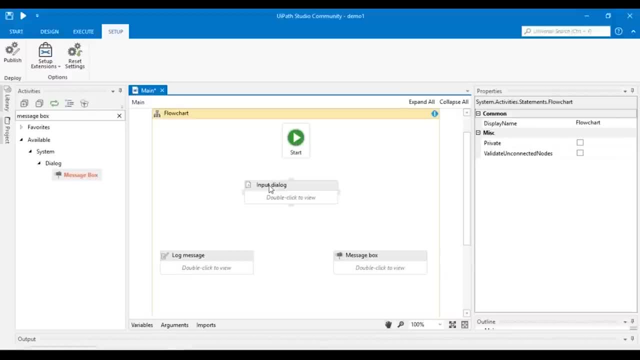 The input dialogue is basically what you want the user to ask. All right, the log message consists of all the log messages that would be displayed and when you talk about the message box, that would be after you give an input- What message you want to get displayed? right? 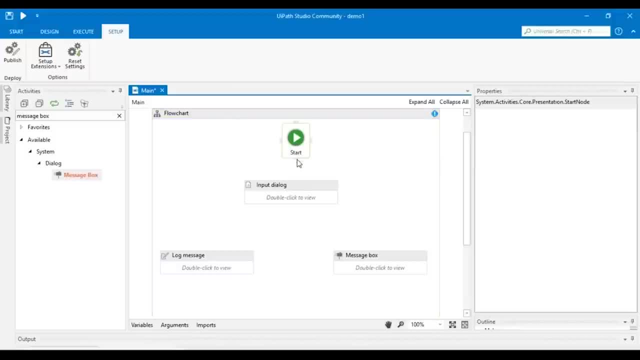 So now let's just connect this start to the input dialogue, Right, and the log message to the input dialogue that takes the input from this, And then let me just search for a decision box And then drag and drop it here. Right now let me just connect the log message activity to the. 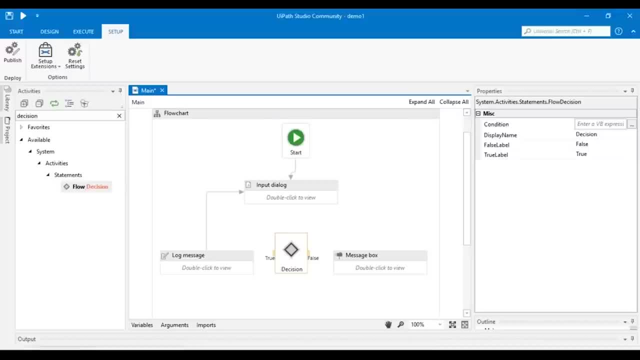 true branch of the flow decision and to the input dialogue activity. All right, so let me just connect them. Now, select the log message and go to the properties panel and update it accordingly, So in the levels you have to go for error and then click out. 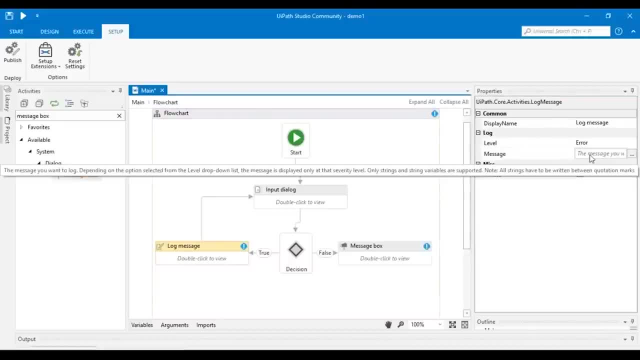 of the sequence, All right. and in the message field, type in what error message you want to be returned, right? So if I say, suppose invalid user, so we can type for invalid user. So basically what's happening here is that when you execute, 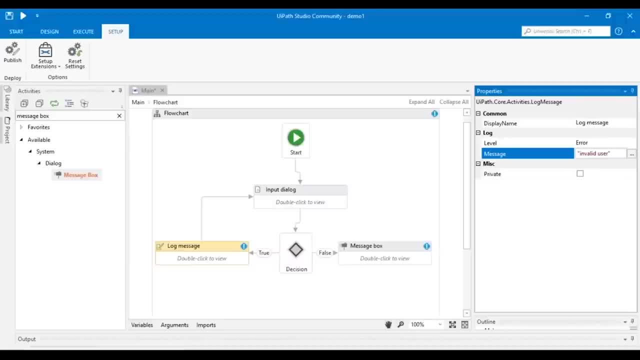 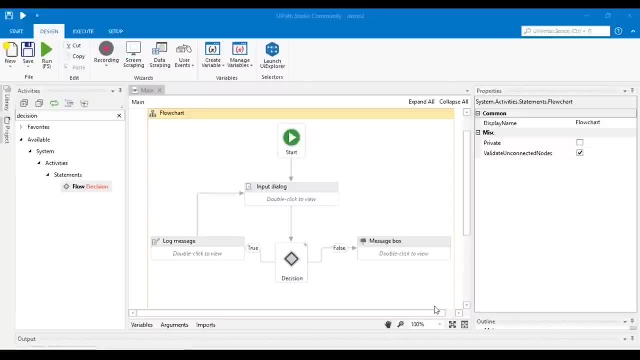 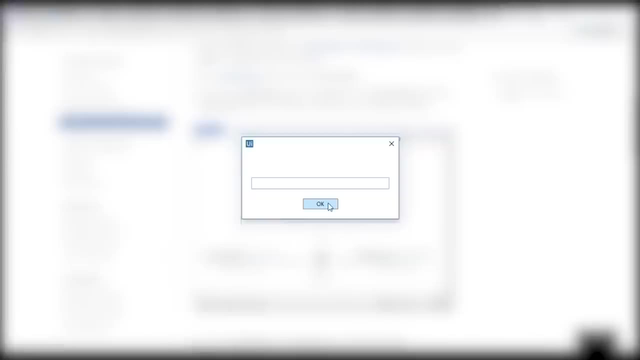 the project. the error message is displayed in the output panel every time The user does not fill in the input dialogue window, right? So now that we're done with the flow chart, let me just press on F5 to execute the automation. So let me just press on F5 and let me just not fill anything. 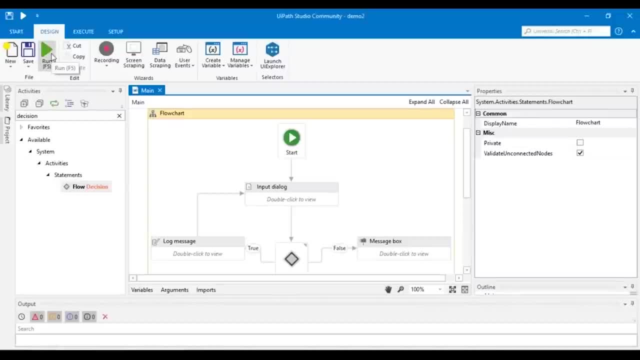 over here and click on Okay, All right. So now let me just run this program and show you. so. let me just say, if I type in hi, It shows that the execution has started, but there was an invalid username, right, So it locks. few errors. 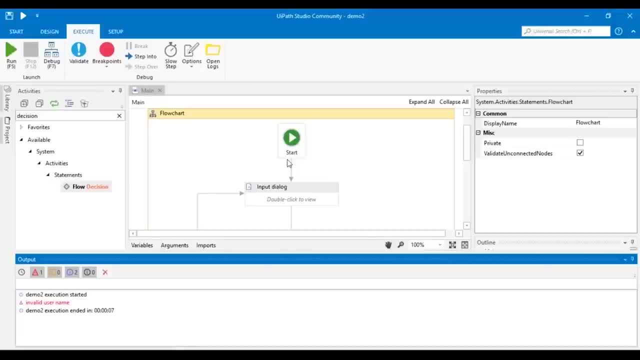 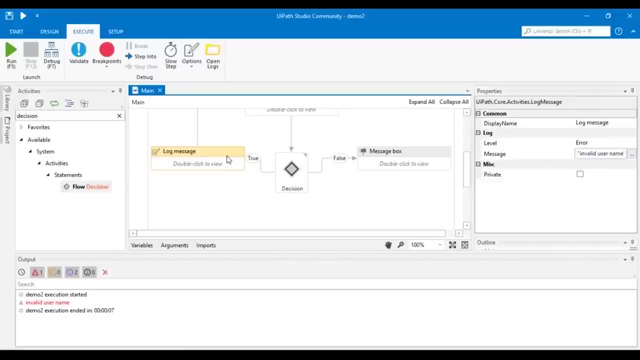 So on the execute tab with the debug group from the options menu you have to select log activities, right? So let's go to the options menu and select log activities. So it's already selected in my UI path. now select the log message activity and on the execute tab in the debug group, 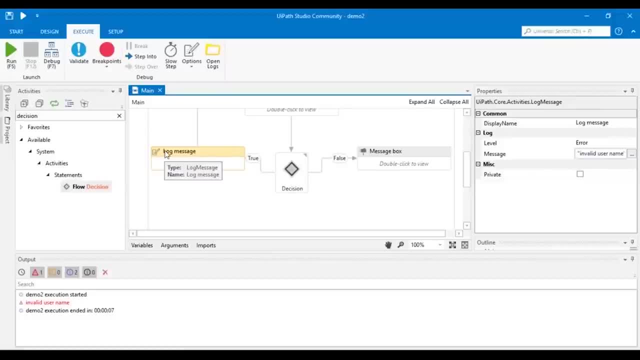 click toggle breakpoint. right, So the log message activity selected, and in the breakpoints I'll choose toggle breakpoint. All right, So you know that there's a small Red dot with white strips displayed next to it. right, The signals that the activity has a breakpoint applied. 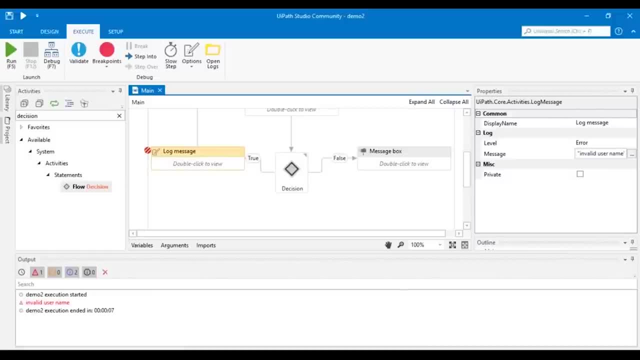 So when the interview asks you, how do you identify if an activity had a breakpoint or not? This is the signal: a red dot with white stripes. All right now to debug this program. on the execute tab in the launch group, You have to click on start debug. 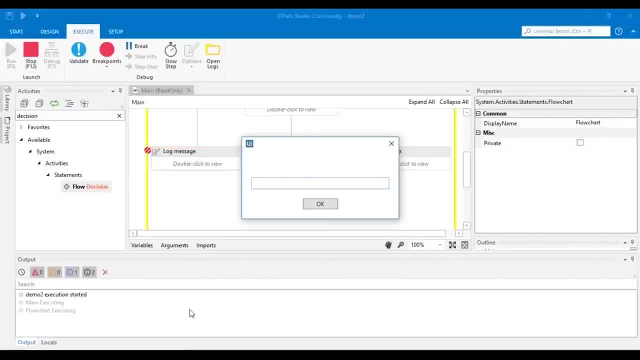 So let's just click on that and debugging starts right. So if I just mention a text here and click on okay, the breakpoint has been triggered and, as a result, the automation has stopped. now in the output panel the error and all the steps covered. 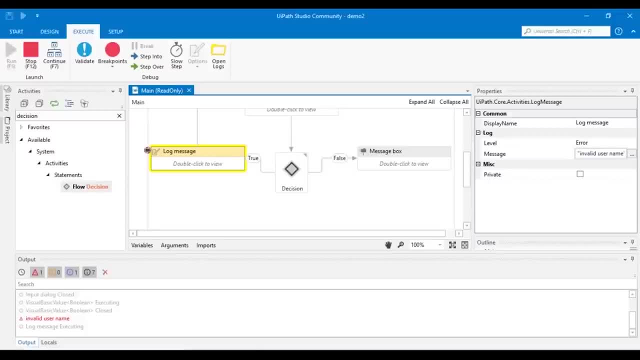 till now have been logged and the log message activity is highlighted. So this clearly shows that we have some error in the log message activity. Once it is done, Just click on the stop button to stop debugging and then we get an information dialog box which displays that the debugging 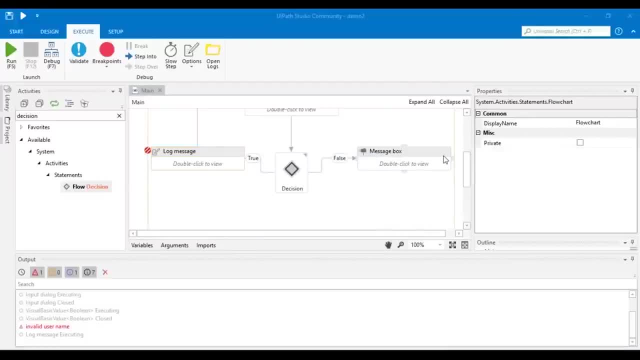 process has been cancelled. All right. so, guys, that's how you can debug your project. You just have to create your Project and then go to the execute tab to start debugging, right? So that was a basic information about how you can debug your. 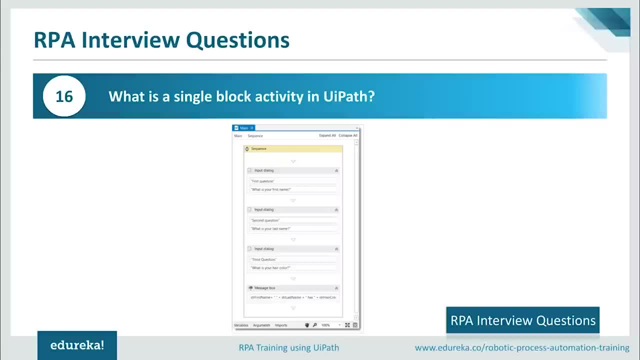 projects. Now, moving forward to the next question We have: what is the single block activity in UiPath? Well, before talking about a single block activity, let me preview a little bit about sequences, right? So why am I telling you? you'll just come to know sequences are. 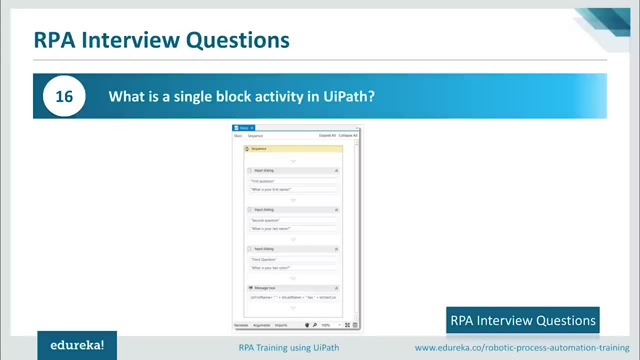 the smallest type of projects. So when you're asked in the interviews what are the smallest type of projects, Then your answer should be sequences. It is suitable to linear processes as they enable you to go from one activity to another activity. So basically, sequences act as single block activity. 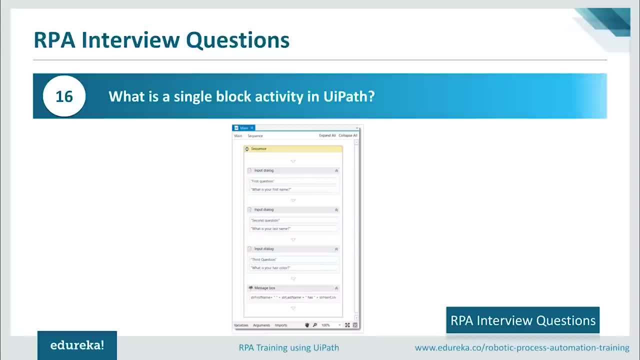 So whenever you are asked about a single block activity in UiPath, you should always talk about sequences. One of the key features of sequences is that they can be reused time and again as a standalone automation or as a part of state machine or flow chart. 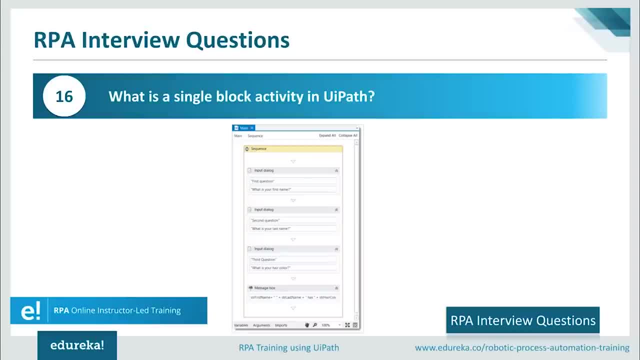 So, if you talk about examples, you can create a sequence to take information from PDF file or add it to a spreadsheet and reuse it in a different settings while changing few properties, right? So sequences help you doing the work in a very easy way, right? 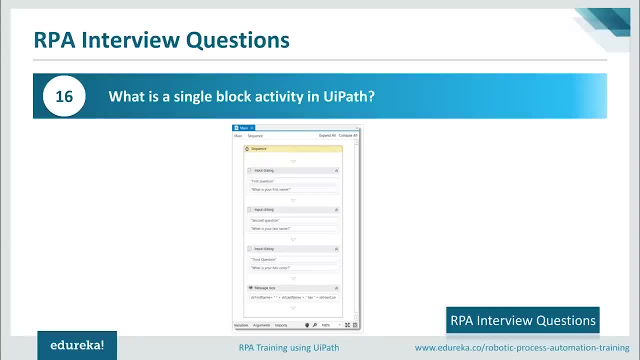 So now let's look into what are the steps that are required to create sequences. All right, So I'm going to show you a demo where we're going to create a sequence that asked the user for his first name and last name and his hair color, and then display the answers. 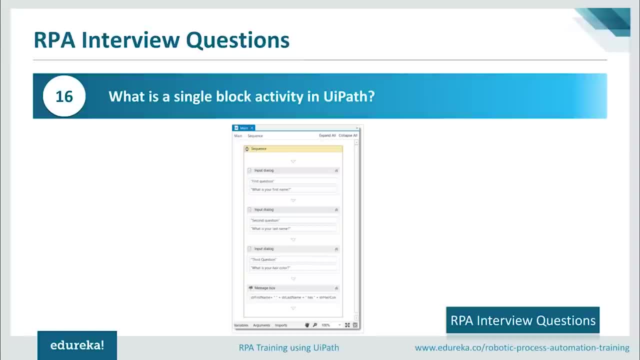 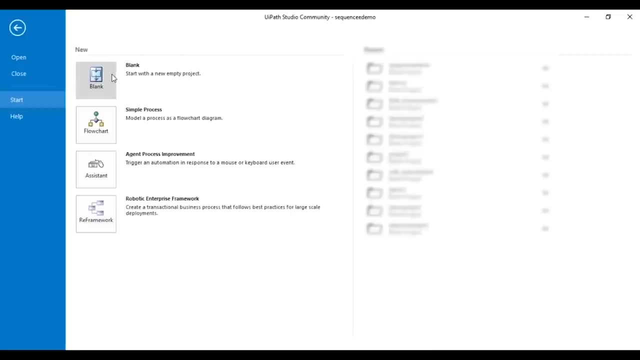 So to do the following, what you have to do is you have to open your UiPath tool. So let me just open this Now to create a sequence, Let us just create a simple blank project. So for that, I'll click on blank project here and then choose. 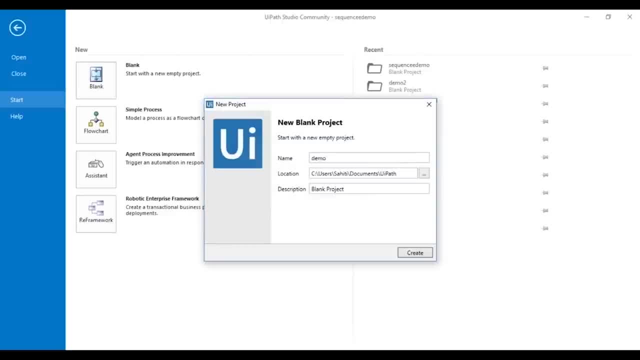 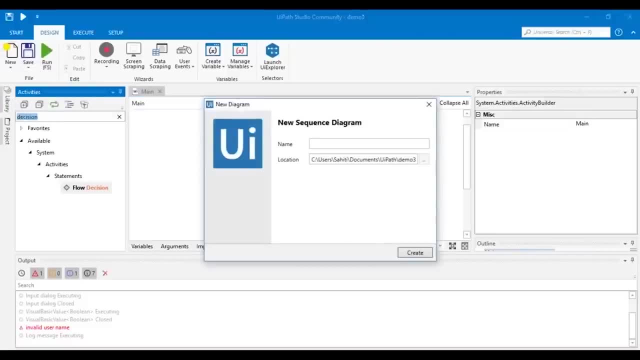 my blank project name. Let's just say demo 2.. Let's just say demo 3 and under the design tab I'll go for new and choose sequence. All right, I'll give the sequence name. Let's just say: I give the sequence name as sequence demo. 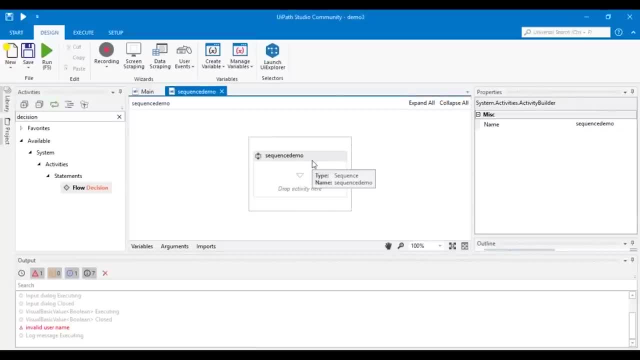 and click on create. So basically this creates a sequence for me now to identify the first name, Last name and the hair color. We're going to create variables. So to create variables you have to click here on the variable option and then choose to create a variable right. 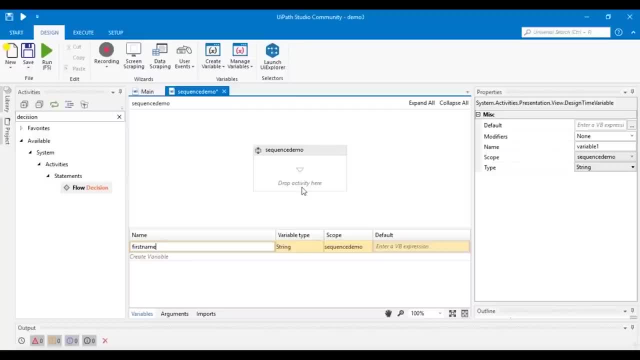 Let's just say I create a variable name- first name of string type, a variable name last name of string type again, and another variable, Let's say hair color. All right, So all the three variables are created. now to ask the user for his first name, last name and the hair color, you have to. 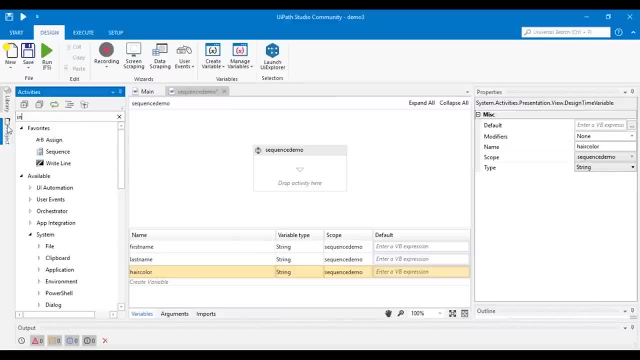 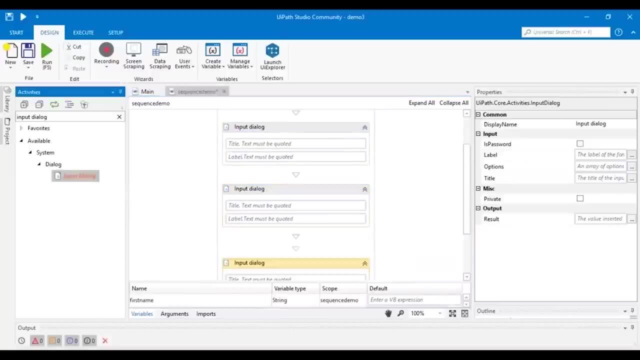 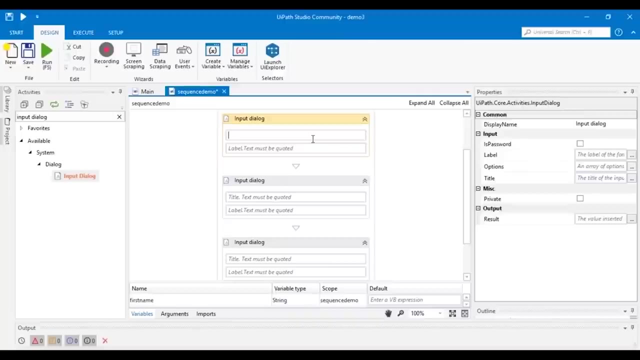 pull in three input dialogs. Let's just search in the activity pane for input dialog and then drag and drop it in the sequence. Now in all these three input dialogs you have to fill in the title and the label right. So let's just say I fill in the title for the first input dialog. 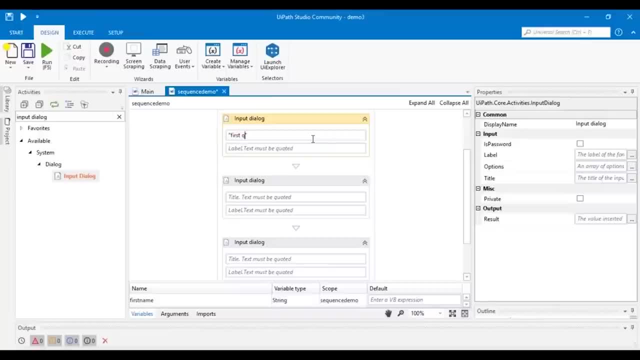 as first question. So if I type in first question and in the label I'm going to type in the question that the input dialog is going to ask me right. So I'm going to type in what is your first name. Similarly, 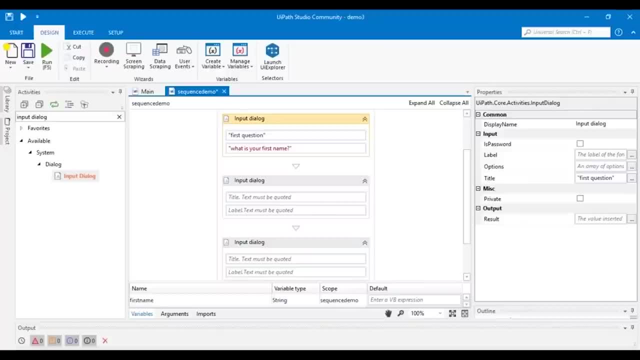 I'm going to do for the other two input dialogs, but I'm going to ask for the last name and the hair color, So I'll type in: second question: What is your last name? Third question: And what is your hair color? 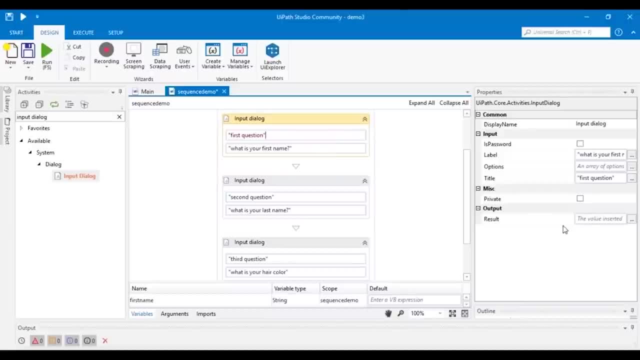 All right now in the properties panel of the first question, in the results section, you have to include the variable that we just created, right? So for the first input dialog we're going to include the first name variable. coming to the second input dialog, in the results. 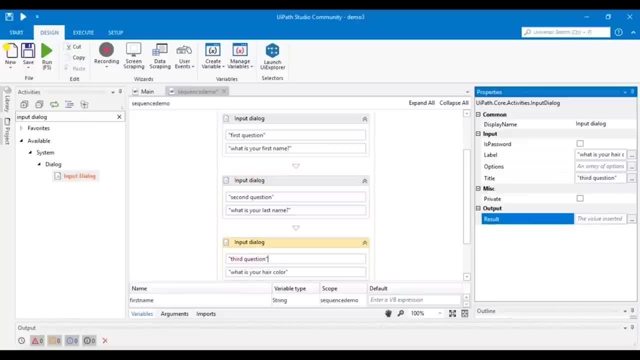 section will include the last name variable and in the third input dialog We're going to include the variable hair color. So what's happening in the results field? Well, this indicates that the variable is going to be updated with the value added by the user at every point, right? 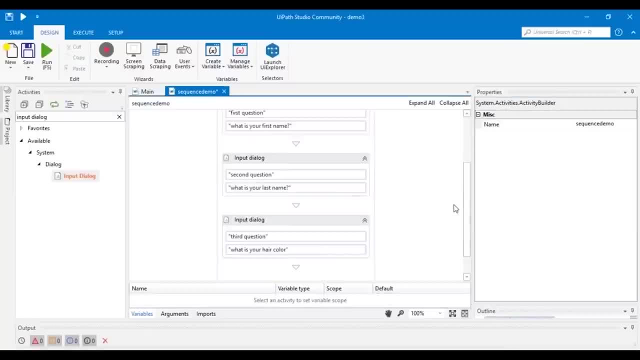 Finally, after we have given all the inputs, we want a message to be displayed right. So we're going to search in the activity pane For message box And then drag and drop it here. Now we're going to select the message box and it and in the 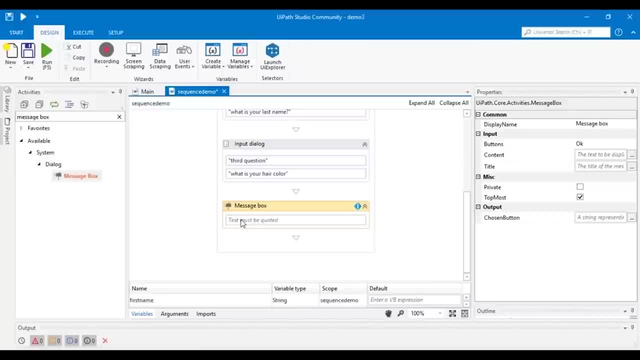 text field we are going to add the variables and a string to display all the information gathered from the user right. So in this case it would be the first name, the last name and the hair color. So let's just include the variables here with the string. 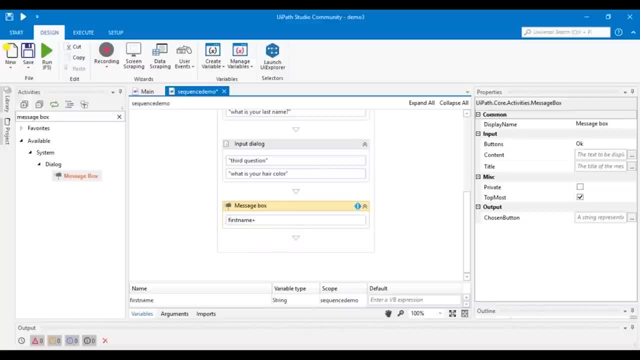 So, first name, concatenate it with a space, and then, last team, again concatenate with a word has and then include the hair color variable, right. And finally, let's concatenate it with a string hair, All right. So now, if you want to check if there are any errors in the 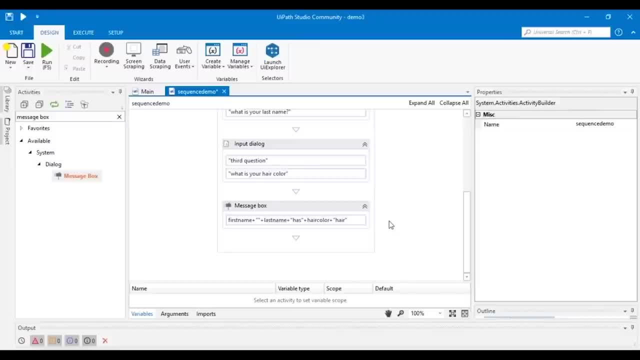 sequence. you just have to click out of the sequence and look for exclamation marks. So here you can see that there are no exclamation marks. So that means our program is error-free. now let's just run this program and see what's the output. 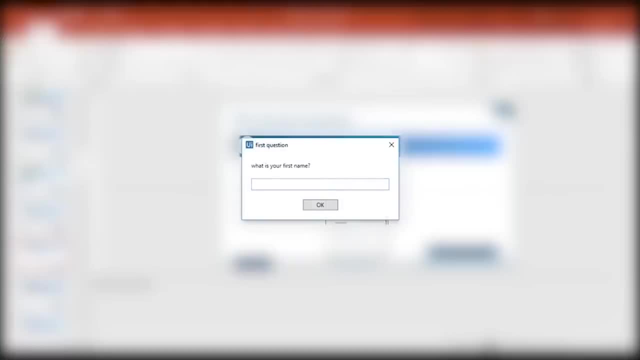 So, as we're going to give the input, The first question is: what is your first name, right? So if I say sahiti is my first name and I'll click on okay? and then the second question comes up, which is: what is your last? 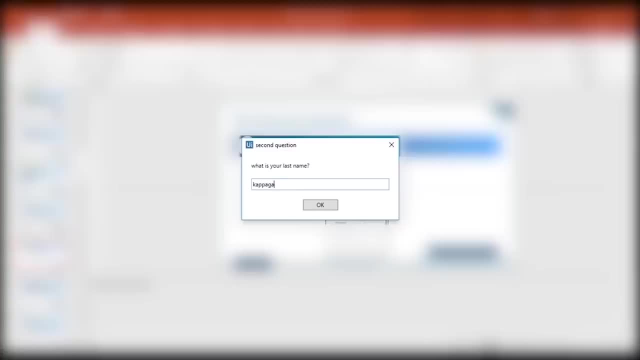 name. So let me just type in my first last name And then click on Okay. once it is done, I'll enter my hair color, So I'll click over here. I'll type in over here and click in Okay once it is done. you can see that the message box displays. 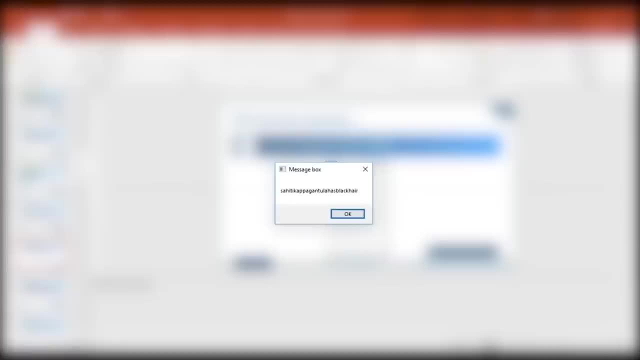 the output, but you can see that there are no spaces. that is because We haven't added any spaces, right. So uipart does not give space by itself, You have to give the input. So for that let me just go back to the uipart tool again. 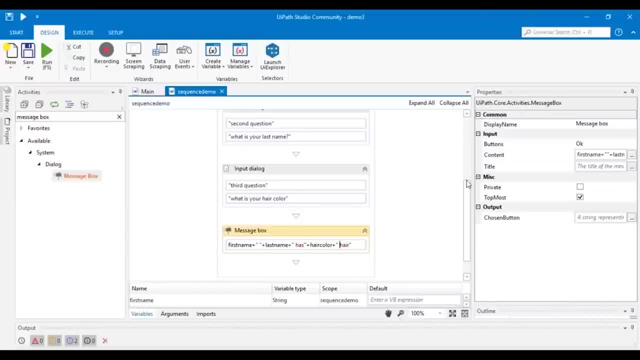 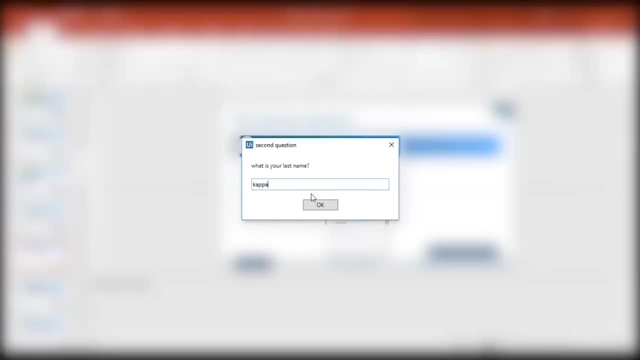 And let me just add spaces between the double quotes, right? So I'm adding space and let me just run this program again. So let me just enter the details again And you can see the output of my first name, last name and my hair color, right? 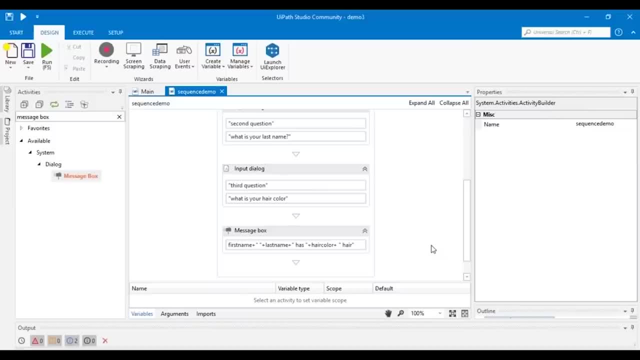 So that's how you can create simple sequences, And this is a single block activity, And this kind of examples can be termed a single block activity as everything is happening under one sequence, right? So it's always good to answer the questions with examples. 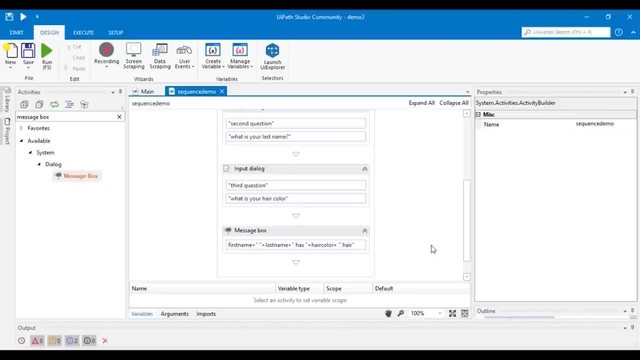 right. So when you're asked in interviews about the single block activity, always remember to talk about sequences and give them a proper example of how you can create sequences and then show them to run All right. Now, moving forward, We have the next question, that is, what is tracing and how do? 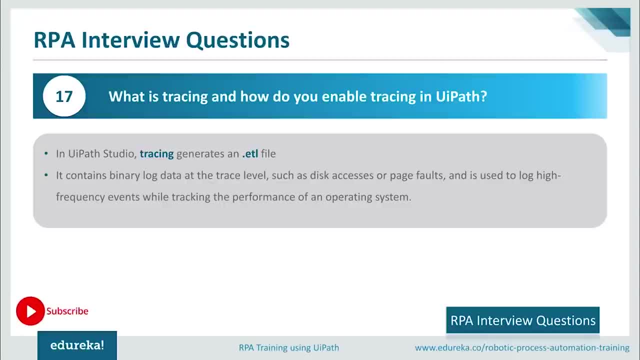 we enable tracing in uipart, So by default, let me tell you that uipart generates log files that track the activity of the studio and the robots right. These logs can be accessed from the execute ribbon tab by clicking on open logs button. 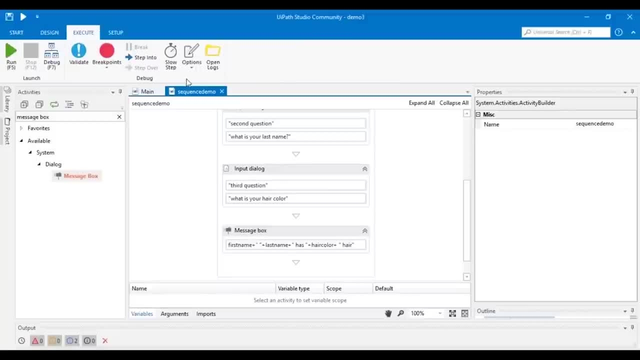 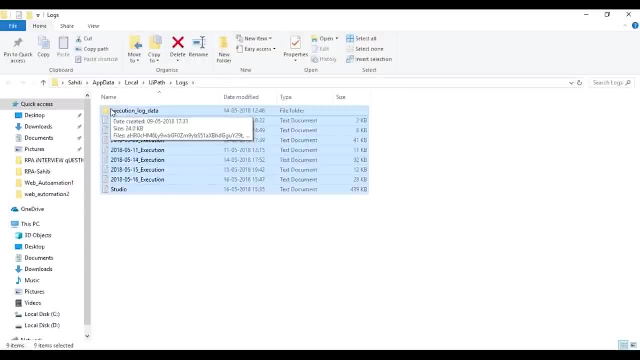 So let me just show you so, when I go to the uipart tool and then go to the execute ribbon tab and then if I open open logs, these are the log files that I was talking about, right? So for complex issues, more details about your automation is. 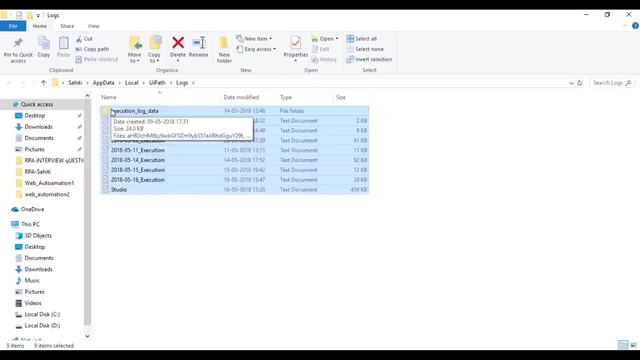 always needed, isn't it So to gather them tracing, We enabled in uipart studio tracing generates and etl file which contains binary log data at the trace level, such as the disk access or the page falls, and is also used to log high. 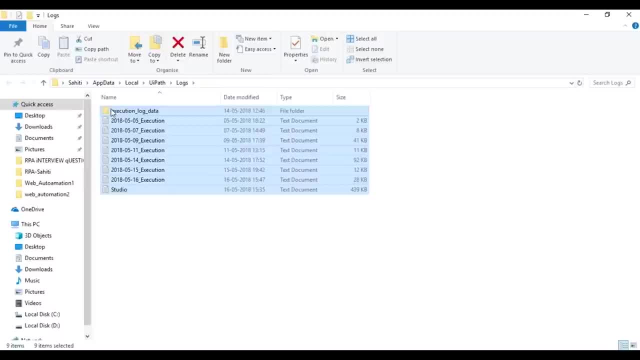 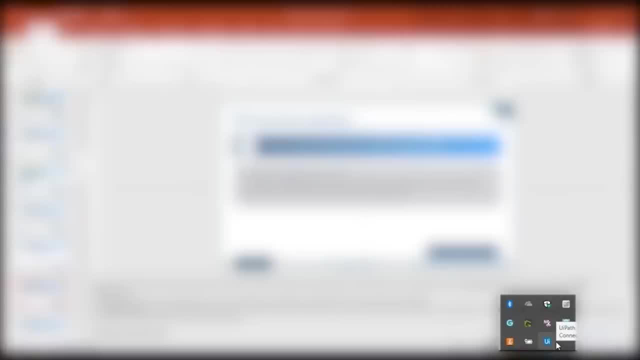 frequency events while tracking the performance of your operating system, right? So if you want to know how to trace the files, well, you can see that in your taskbar you find this icon of uipart robot, right? So you just have to open that window and go to the advanced. 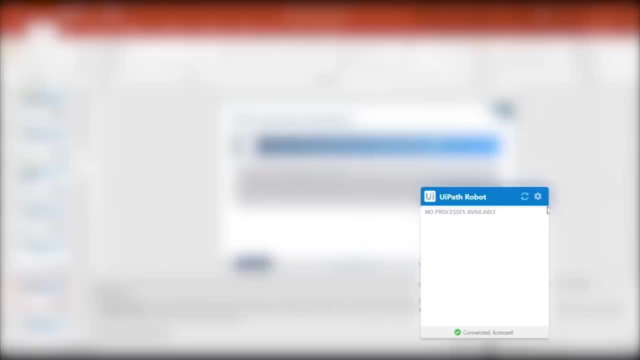 settings over there. Once the window opens, You just have to click on the start tracing button. that will trace every activity that you perform on the uipart studio, right? So tracing is really interesting when you talk in uipart studio, as when you deal with large, complex activities, it's really 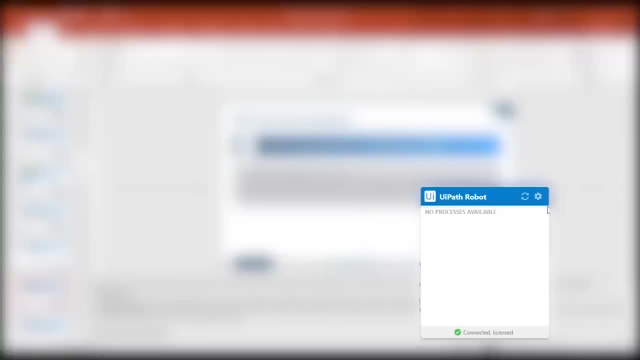 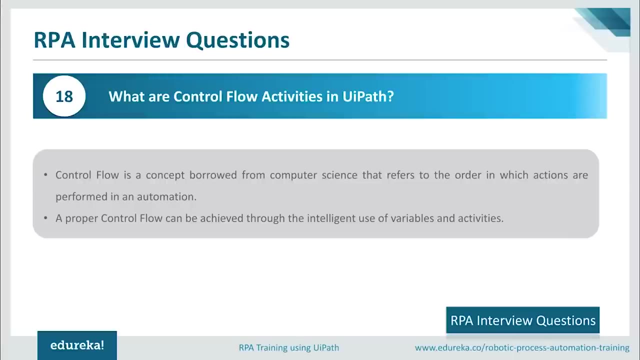 tiresome task to understand where the error is coming from, right. So debugging, logging, tracing- all of them together help you to solve these errors in a simple way. So for a long time now I've been talking about activities, right? So what are the control flow activities? 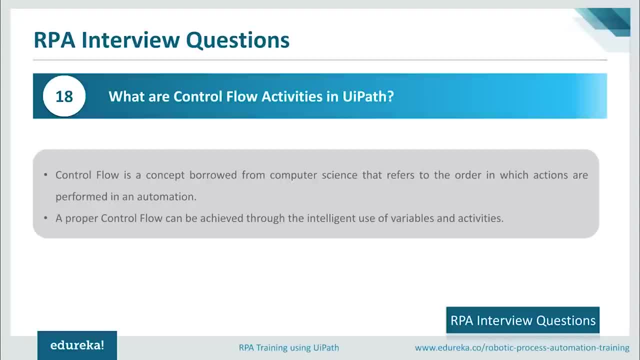 So that's our next question, Which is generally asked in interviews. So what are control flow activities in uipart? So when you talk about control flow in a layman language, it is just the order in which actions are performed, right? 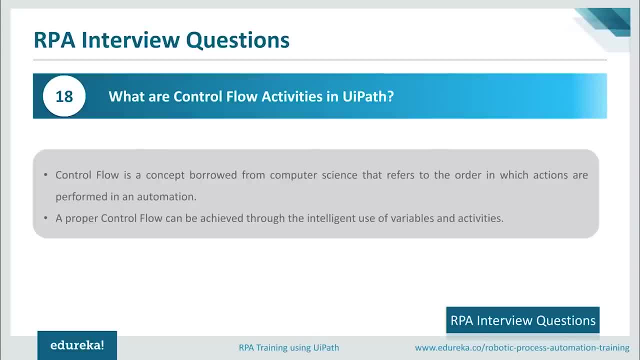 So control flow is a concept borrowed from the computer science field that refers to the order in which actions are performed in an automation. Let me tell you that a proper control flow can be achieved through intelligent use of variables and activities. So to understand control flow, 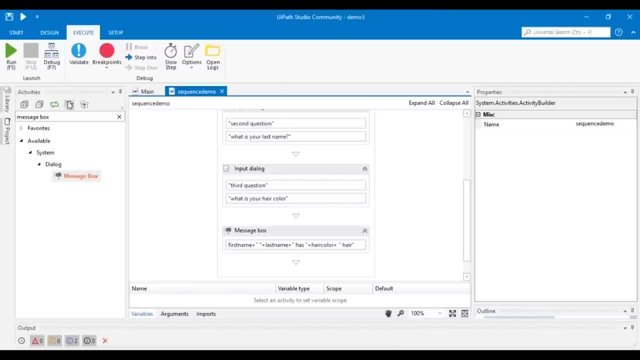 Let me just go back to my uipart tool and show you how that's happening, right? So when you go to the activities pane under the workflow tab, you have this control flow option, right? So if you observe the control flow option here, you can see. 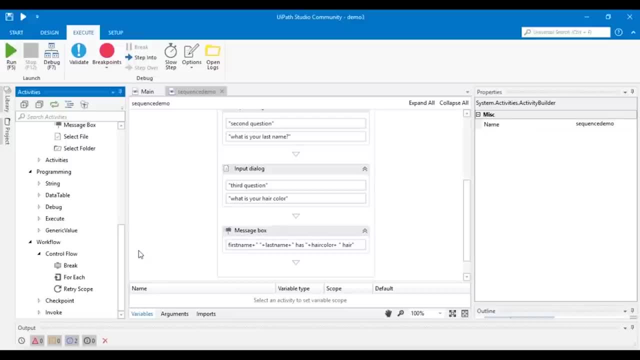 that the control flow option is for break for each retry, So you can apply different kinds of loops in layman language, such as the switch loop, the fall loop, the if-else loop, etc. right, So, basically, these activities enable you to define rules and 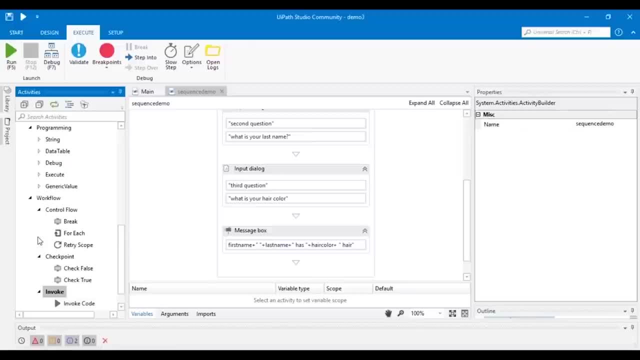 automate conditional statements within your project right. So, for example, delay can be added between the actions, or you can parallelly run for different projects, Or you can just pick up a particular branch and run it. or if you want to apply for a switch statement, you can do that. 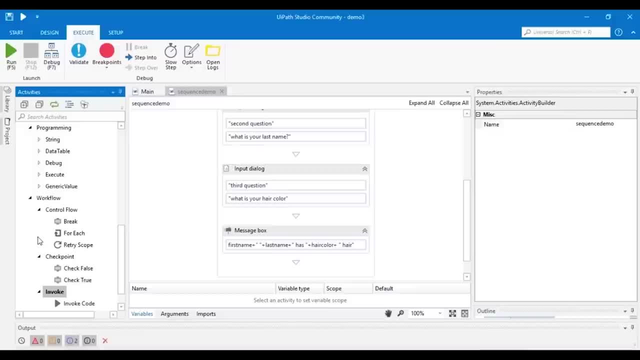 So, guys, that was a simple answer on control flow activities. If your interview asks you deep knowledge about control flow activities, then you can tell them about each activity. How do you implement it, What are the scenarios in which you choose which activities right? 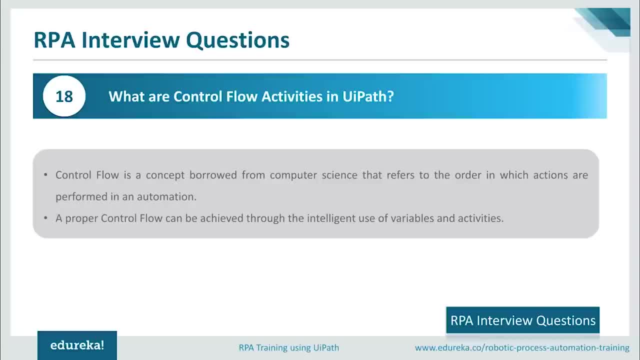 So, for example, if you have to run a loop again and again, you use the for each activity. if you just have to run the loop for different cases, then you use the switch activity. right? So you can explain the interviewer with such examples. 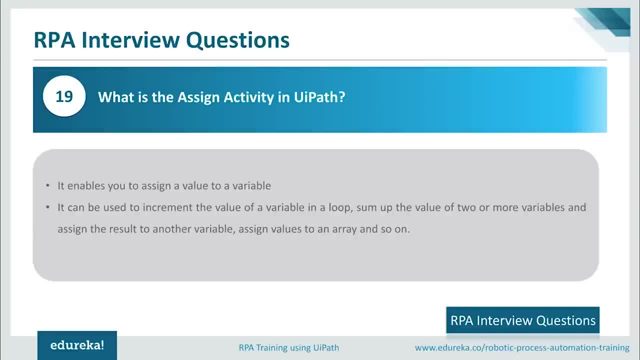 Now moving forward, We have the next question, that is, what is the assign activity in UiPath? So there are various type of activities that I just showed you. Now in those, what is the assign activity? Well, the assign activity is an important activity as it enables: 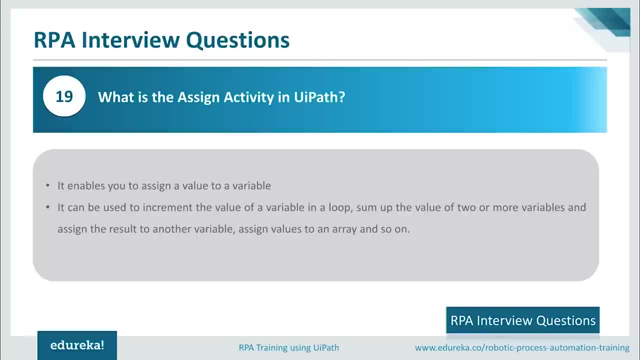 you to assign a value to the variable. right So it's used quite often. right So you can assign the activity to increment the value of a variable in the loop, or you can sum up the values of two or more variables and assign. 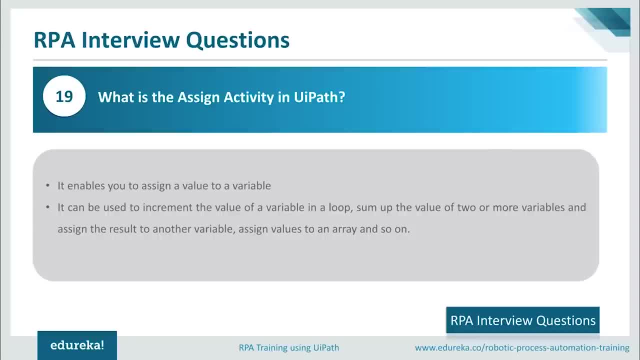 Result to it, or assign the values to an array, and so on. Right, So there could be many instances where you use the assign activity. So, by default, this activity is always included in the favorites group. Let me just show you that. So this is the activity that I was talking about. 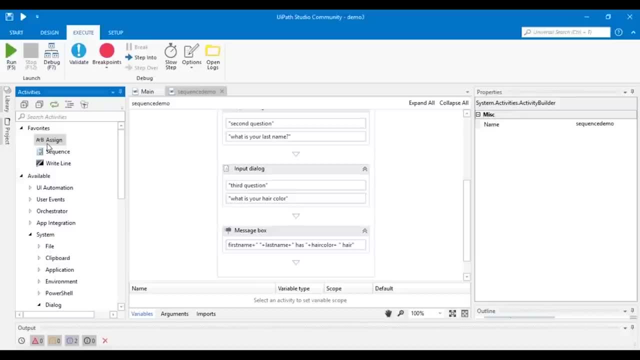 So whenever you're asked about assign activity, always give live examples, like how we can increment the value of a variable and then assign it to a particular variable, or in any scenario based questions where you can assign few values Or where you run a loop to assign the incremented value every. 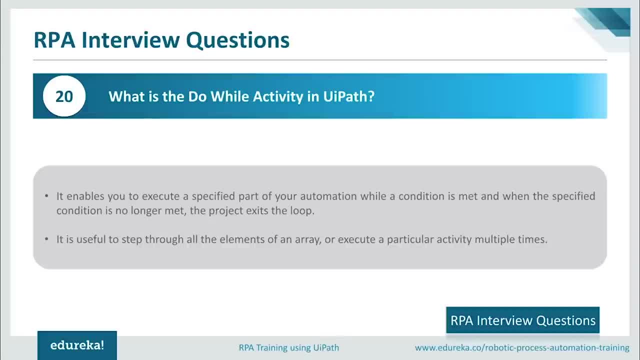 time right now. moving to the next activity type, We have the do-while activity. So what exactly is this do-while activity and how does it function? So if you're from the ID professional background, you do understand the meaning of do-while term, right? 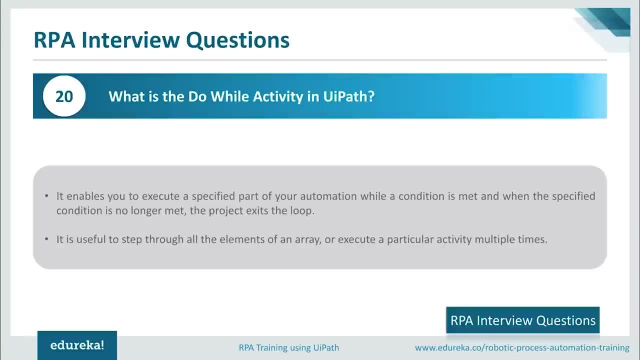 It basically goes by the name. you first do the task and then check the condition. So that's how it happens also in the automation field. So basically, the do-while activity enables you to execute a specified part of your automation while a condition is met. 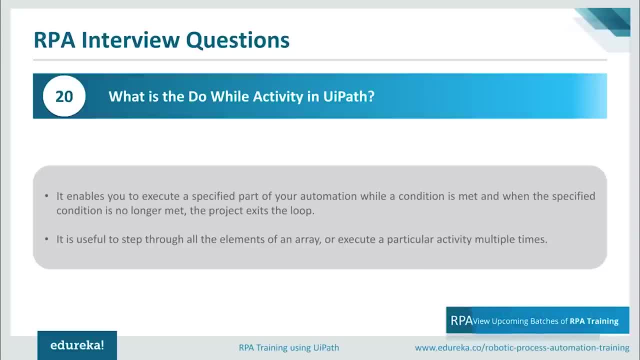 right. So when the specified condition is no longer met, the project exists to loop. this type of activity can be useful. Now, where is it useful? Well, this type of activity can be useful to step through all the elements of an array or execute a particular activity. 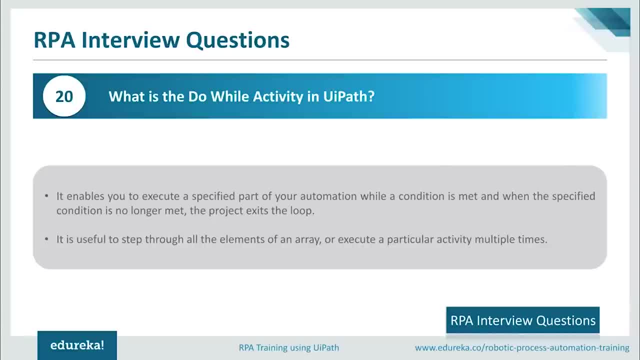 multiple times. You can also increment the counters to browse through array indices or step through a list of items, right? So there are various scenarios where you can use the do-while activity. So when the interview is ask you on when you should use the, 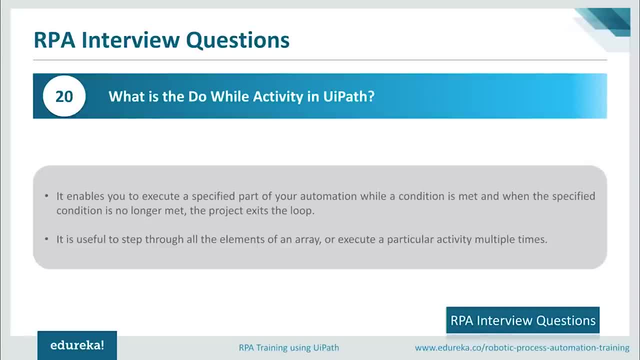 do-while activity. then you can give examples about how you can step through all the elements of an array or do a task particular number of times until the condition is no longer met right. So now let me show you the steps to create a do-while activity. 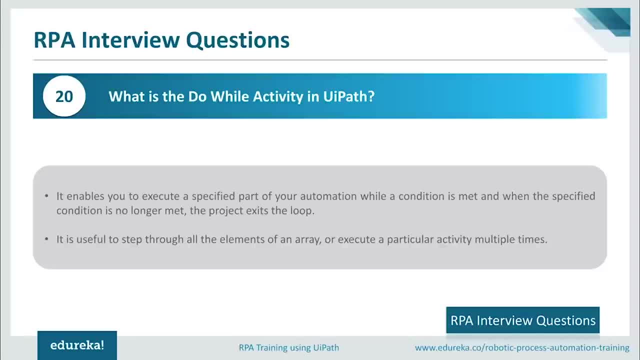 So for that, we're going to create a simple automation that increments integer variable from 0 to 10 and displays a message every time it is incremented, right? So for that, let me just go back to my UiPath tool. Let me create a simple. 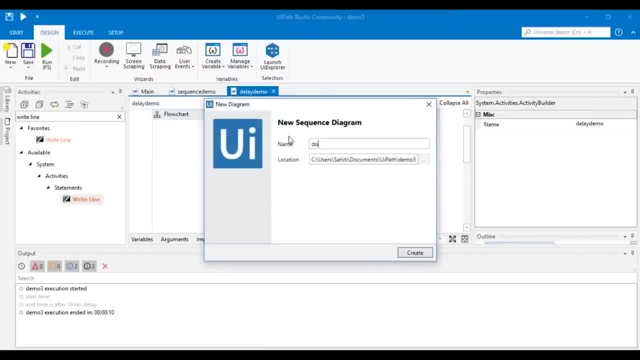 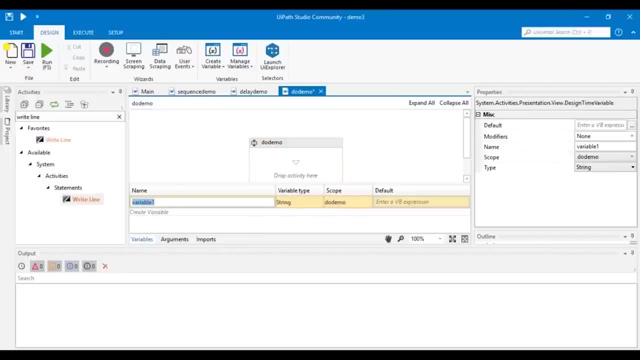 Sequence. Let's say I named the sequence as do demo and then select the sequence and create an integer variable. So for that let me just create counter of in type with default value as 0.. All right, Now let's add a do-while activity. 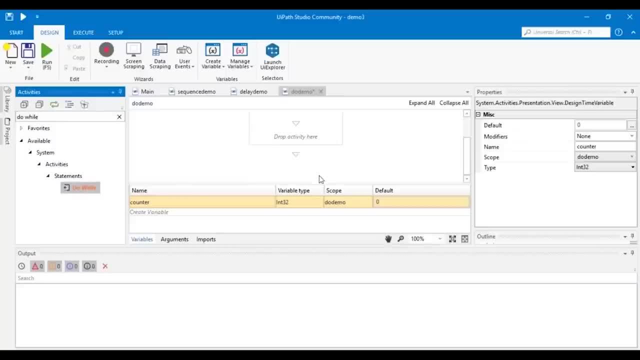 So let's just search for a do-while activity And then drag and drop it here. All right, now in the body Section you have to add an assign activity because we're going to assign this variable right. So in the body section you have to add an assign activity. 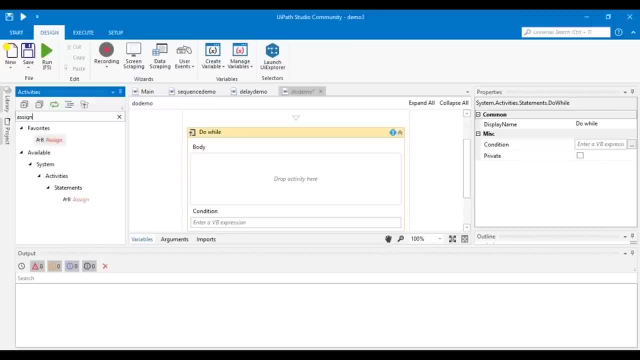 So for that let's just search for assign activity in the activity pane, drag and drop it here, and then in the value field Let's just include counter plus 1. that would mean each time the value is incremented It is assigned to this variable counter. 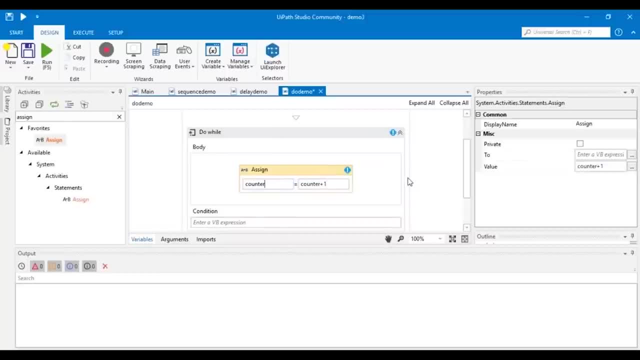 All right Now. once this is done, you have to add a right line activity under the assigned one right. So let's just search for Right line activity and add it here Now in the text field, we want a message to be returned every. 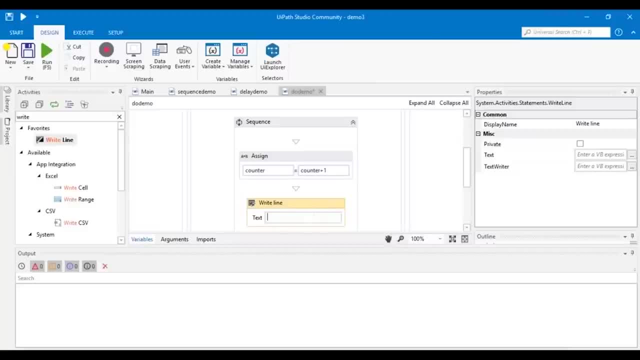 time it is incremented, right? So let's just type in that message. Let's say I type in: the counter is counter variable dot to string. So what's happening with this is that this writes the value of the counter in the output panel each time it is incremented. 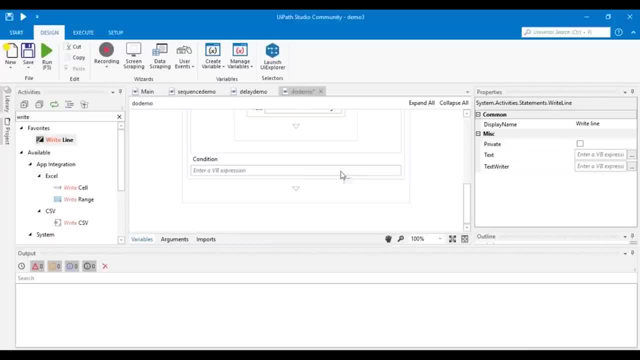 Now in the condition section of the do-while activity, type counter is less than 10, as we are performing this task till we reach 10.. Now the body of the do-while activity is repeated until the value of the counter variable is bigger than 10.. 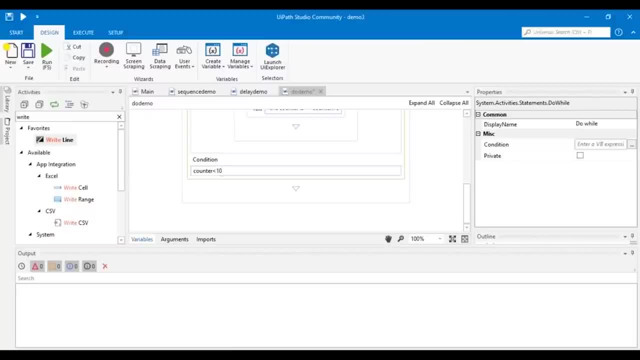 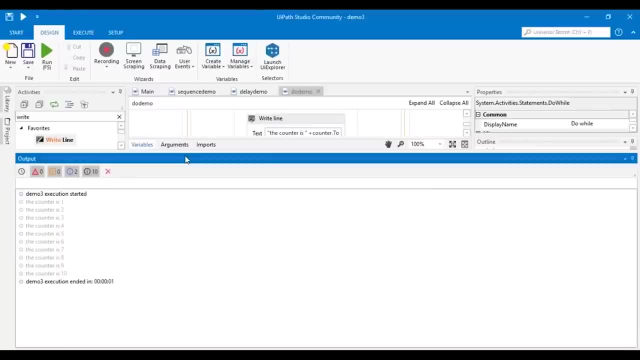 So the logic is very simple, right? This complete activity is repeated every time till the counter variable value is bigger than 10.. Now let's just run this program Now. if you look into the output panel section, it displays the message indicated by the right line: activity. 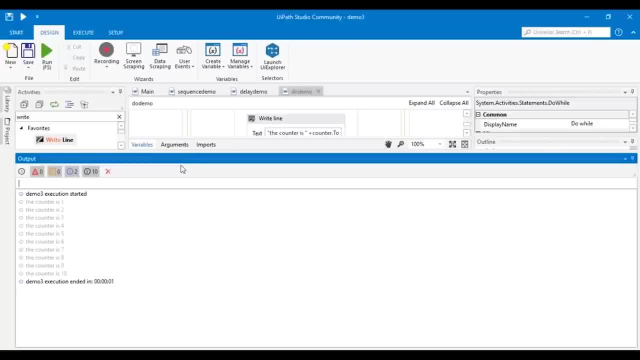 So you can see that the counter is one, two, three and is incremented till 10.. Once the counter value has reached 10, the execution stops. So that's how you can use the do-while activity to do simple tasks. All right, guys. now moving on to the next question. 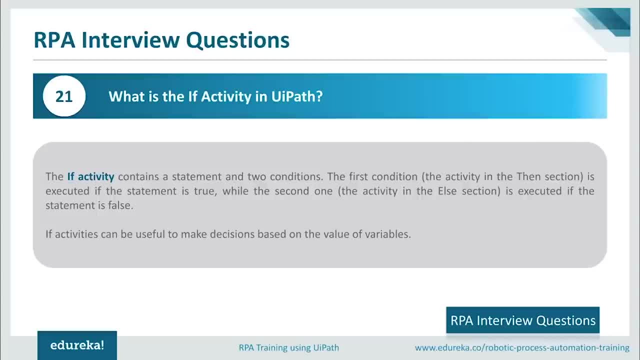 We have: what is if activity? now, when you talk about if activity, if activity contains a statement and two conditions, right. So the first condition is executed when the statement is true and the second condition is executed when the statement is false. right, So, when you talk about the if activity, if activity contains 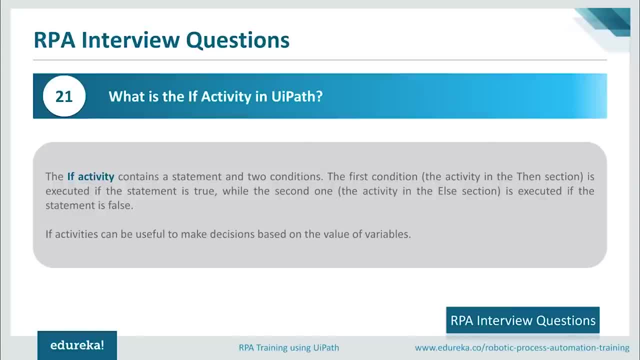 a statement and two conditions. The first condition is executed if the statement is true and the second and the second condition is executed if the statement is false, right. So there could be various scenarios, like you have to do this if the condition is true and you have to do that if the 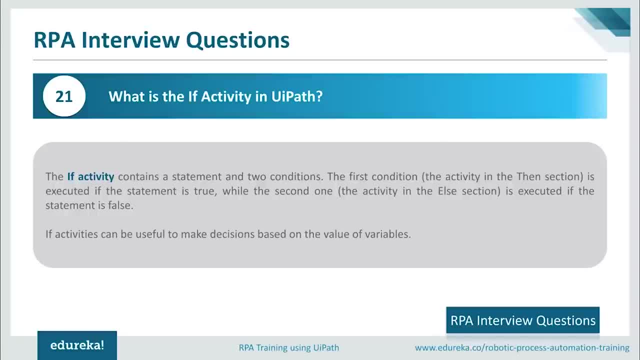 condition is false, right So if activities can be used to make decisions based on variables, arguments, values or any kind of scenario based questions, right So? let me simplify the if activity for you by showing a short demo on it. So what we're going to do is we're going to create a simple 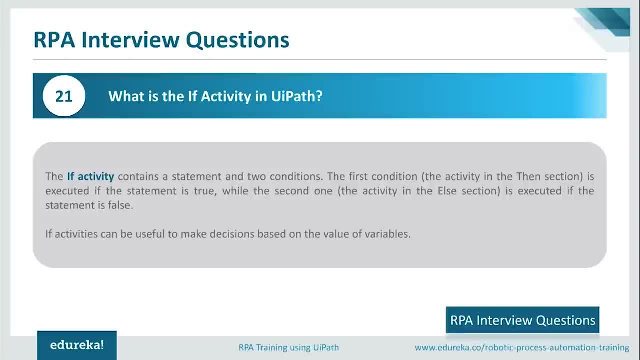 automation that ask the user for two numbers, and then we have to check if these two numbers are divisible by each other or not, and, depending on the result, it displays a different message in output. All right, So now let me go back to the uipath tool. 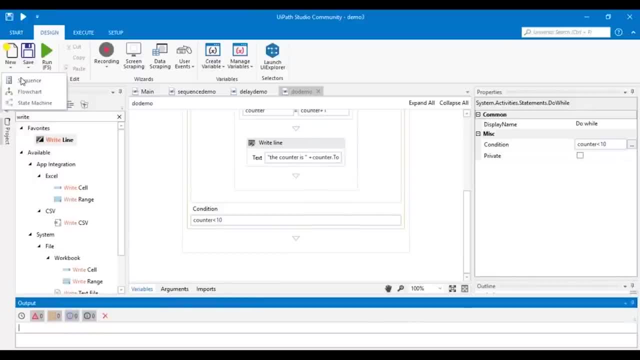 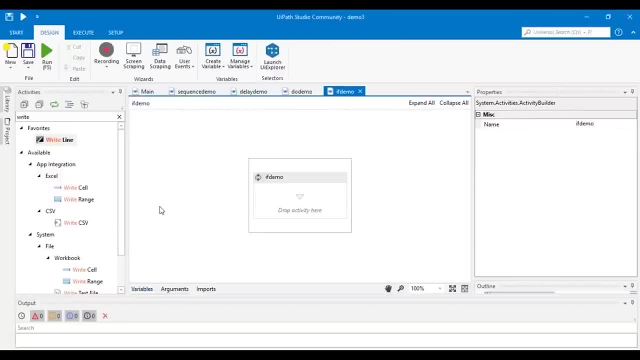 Let me close this. Let me create a new sequence here And let me just say, if I name the sequence as if demo and then click on create, All right, So this creates a new sequence. once you're done with that, We have to create two integer variables. 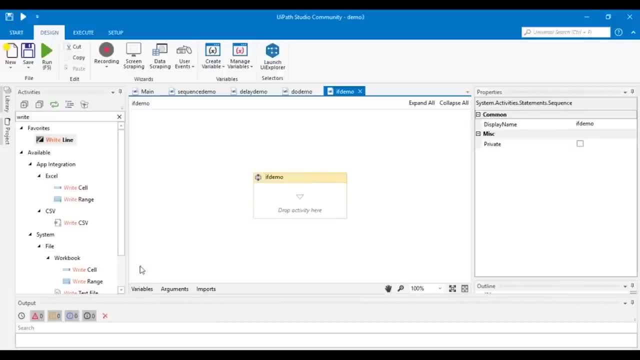 Right, So that is the first number and the last number. So let me just click on this activity, go to variables and type in. first number Of in type and last number of in type- again right, So let me just delete this extra variable here. 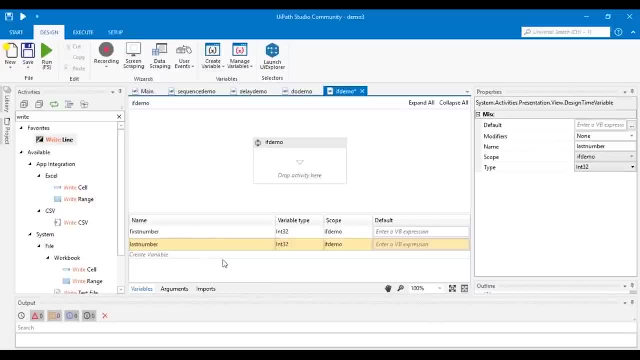 All right. So now what you have to do is you have to add the input dialogue to the designer panel, right? So that input dialogue would basically ask for your input of these two numbers. So let me just search in the Activity pane for the input dialogue. 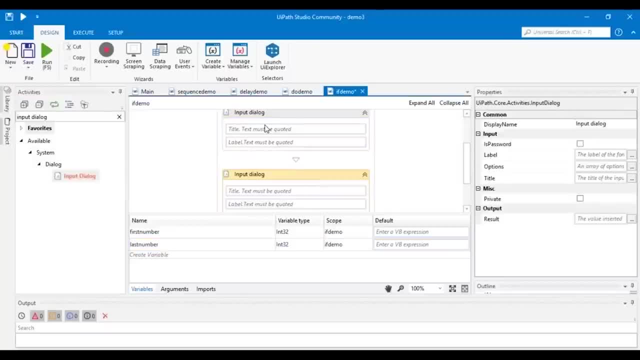 And then let me drag and drop it here Once it is done. Let's just say, in the title and the label of input dialogues I put the text as first question and the label to be what is your first number. Let the second input dialogue have the title, second question. 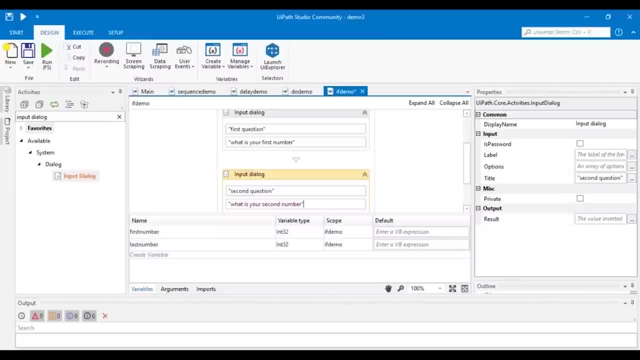 and the label to be what is your second number. Now, once it is done, in the results section of the input dialogue you have to include the variables, right. So for the first input dialogue I'll put in the first number variable and for the second input dialogue I'll put in the 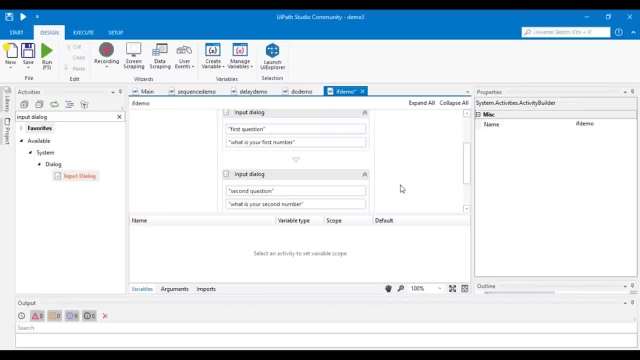 last number variable. All right, once it is done, you have to add the if activity, right? So let's just search for the if activity in the activity pane and then let me just drag and drop it here. All right, in the condition section of the if activity you 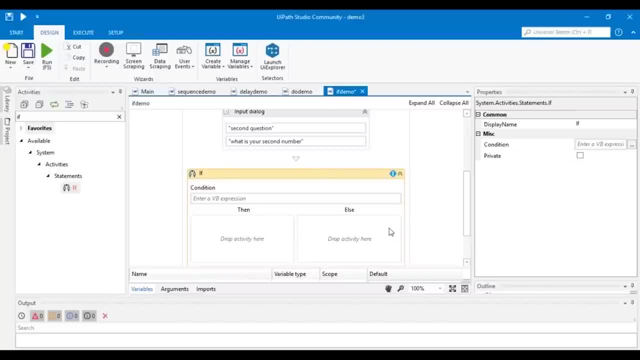 have to type in the condition, right? So here we're trying to find out if the two numbers are divisible by each other or not. All right, so we'll type in: first number, Mod. last number is equal to zero. So basically, when they're divided by each other, the reminder: 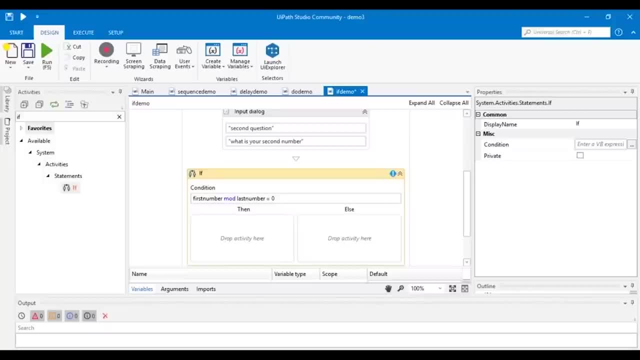 should be zero, right? So that is the expression. So basically this expression checks if the first number is divisible by the second number using the mod operator, and then in the then section we have to add a right line activity. So for that let me just search for right line activity. 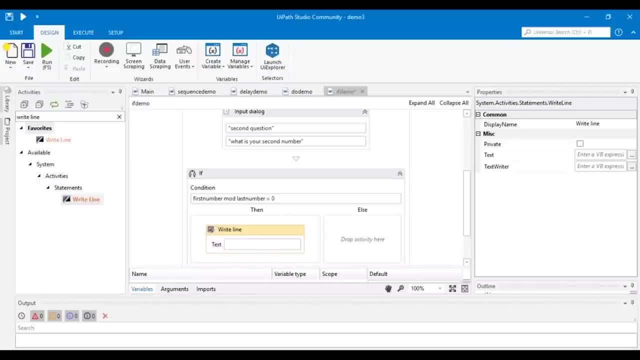 And in the text field let's just add first number to string and then concatenate it with a second number. So let's just type in: the text is divisible by- let me just give a space here- and then again concatenate it with the second number, as I mentioned. 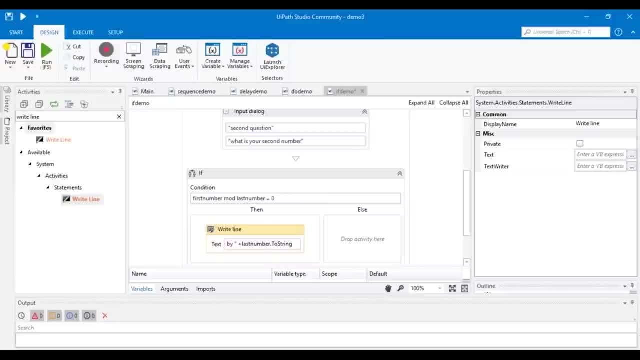 All right. so this is the message that will be displayed if the first number is divisible by the second number. else, if it is not divisible, then we again have to add a right line Activity in the L section. So let me just drag and drop it here and then let me just enter. 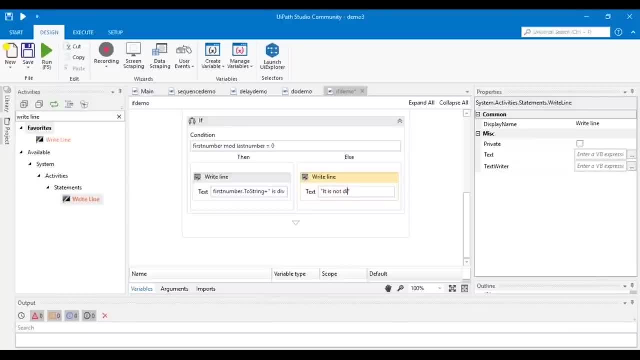 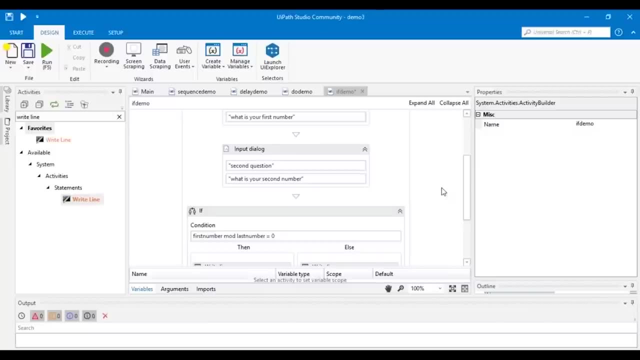 this text that it is not divisible. All right, So basically this program would function like this: We enter two numbers and then it will check if the first number is divisible by the second number or not. If the reminder comes zero, then it will print a message that 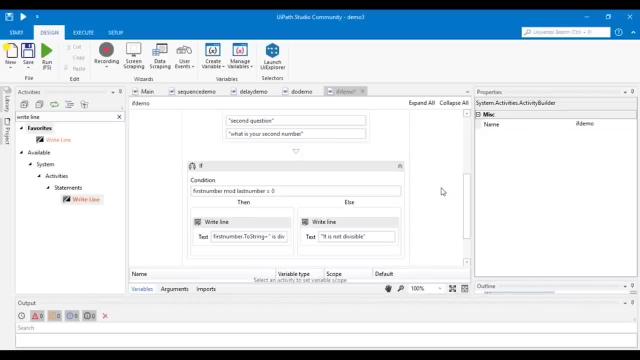 the first number is divisible by the second number. else, If the first number is not divisible by the second number, then it will display the message that It is not divisible, right? So let me just run and show you. So let me just input my first number as 34 and my second number 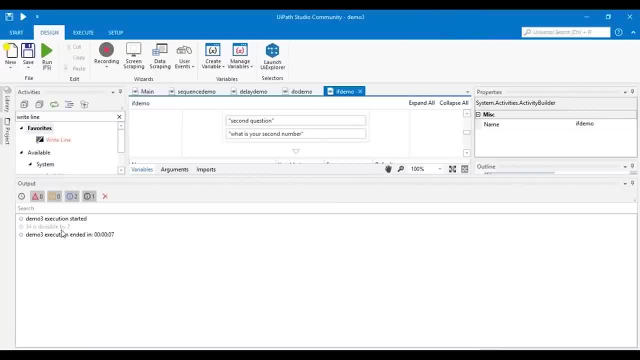 as two, All right. So in the output section you can see that 34 is divisible by two, right, That means the first condition has become true. So, guys, that's how you can use the if-else activity. So anytime an interviewer ask you, how do we perform actions? 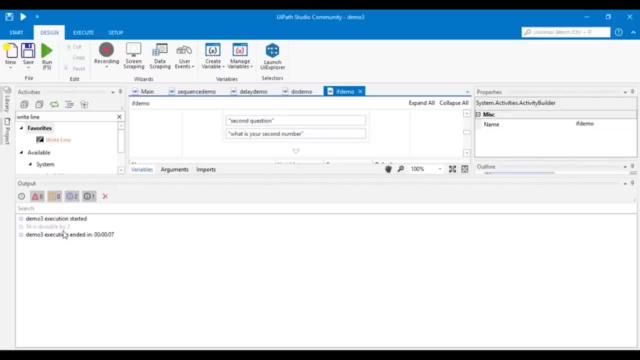 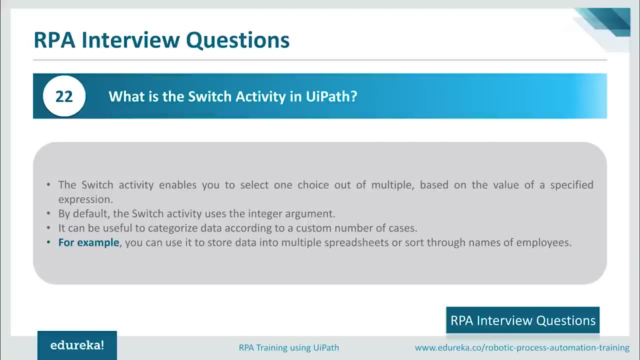 using the if-else activity. you can just show small demos on if-else activity Activities or you can just explain them to various scenarios. right, So now, moving on to the next question we have: what is the switch activity? So, if you have to define the switch activity, the switch activity. 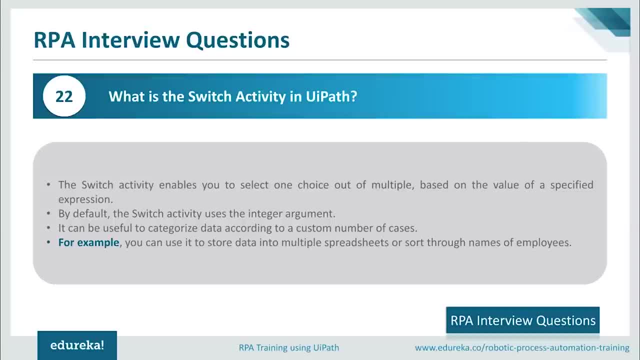 enables you to select one choice out of the multiple choice available based on the value of the specified expression. right? So by default the switch activity uses the integer argument, but definitely you can change it from the properties panel, from the type argument list, right. 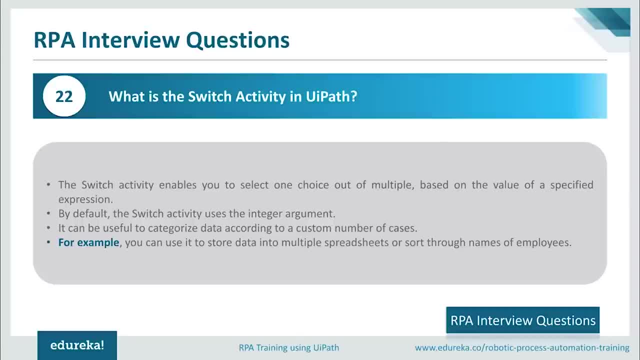 So when you talk about scenarios, when to use the switch activity, the switch activity can be useful to categorize data according to multiple number of cases. For example, you can use it to store the data into multiple spreadsheets or sort names of employees or any such scenario. 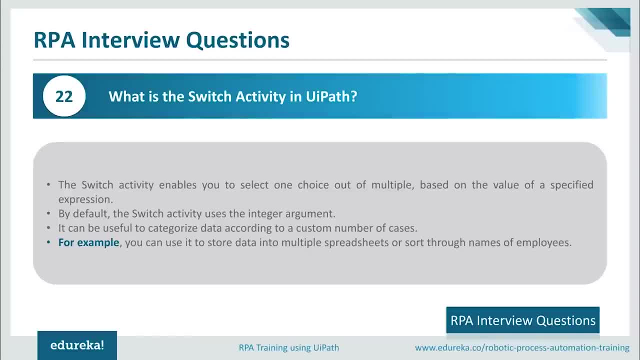 right. So now let me just show you a short demo on how you can use the switch activity in UiPath. So, to simplify that, we're going to create a simple automation that asks for a user, for a number, and checks if it is odd, or even, and, depending on that, a different message is written. 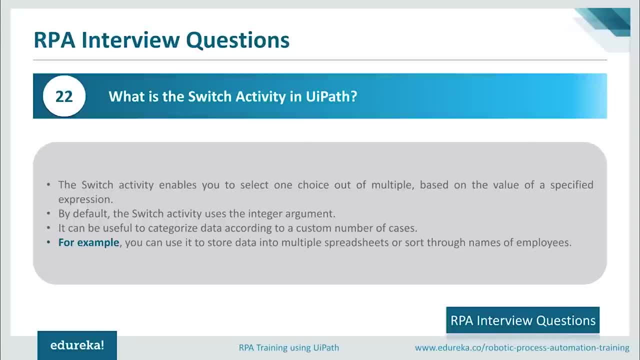 in the output panel, right, Since all of us know that the odd numbers divided by two have a reminder equal to one. So in this scenario, the project needs only two cases, that is, case 0 and 1.. So let me just show you how to do that by going back to the 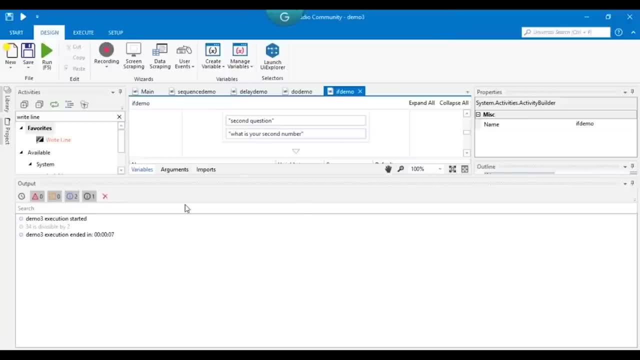 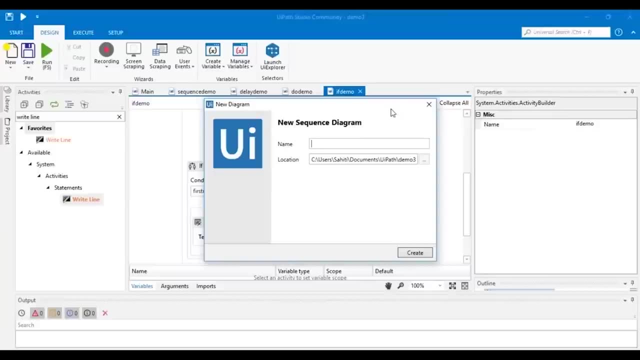 tool. So let me just go back to the tool and then let me just close this. go to new, create a new sequence. And let's say I named the sequence as switch demo, All right, So once you have created a sequence here, you have to create. 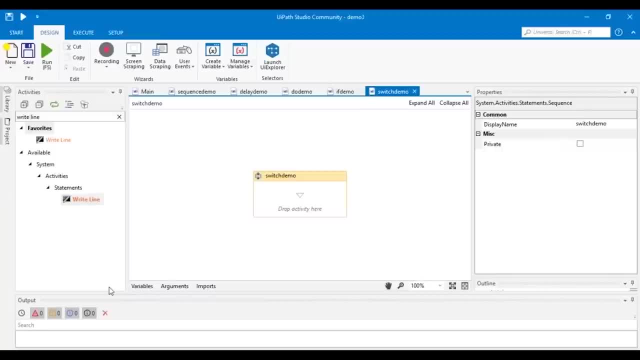 an integer variable. So for that, let me just click on the sequence, go to variables and create a variable name: number of in type. Once it is done, We have to add an input dialog that would basically ask us for the input of a number, right? 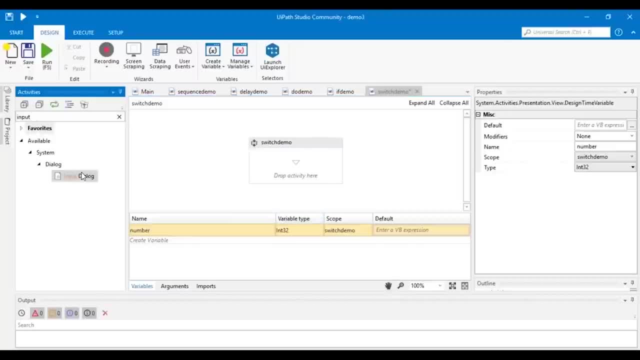 So let me just search for input dialog activity And then in the title, let me just say I put the title as input, your number And your label as What is your input. All right Now, once it is done, in the result field of this input dialog, 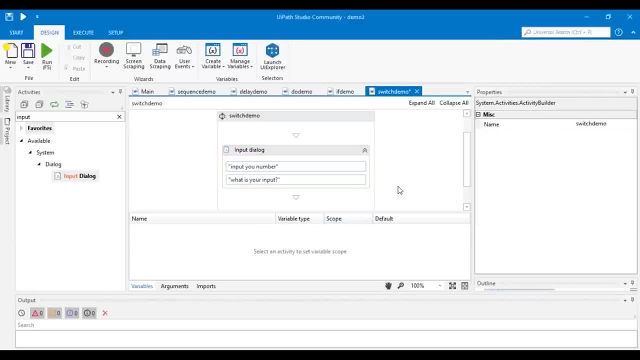 mentioned the variable name, that is number, here, and then we have to add the switch activity. So let's just search for the switch activity in the activity pane and then let me just drag and drop it here. All right, in the expression field of the switch activity. 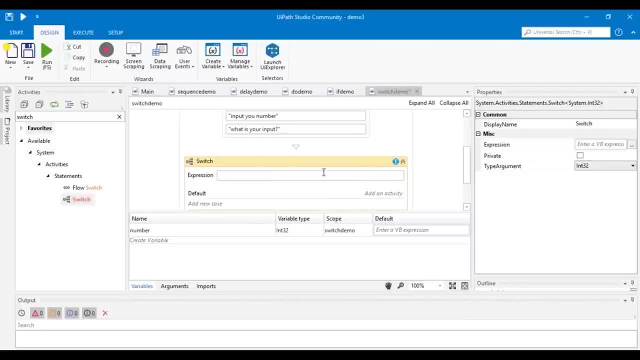 You have to type in the condition, right? So here our condition would be to divide the number by two. So let me just type in number mod To and then in the default section add a right line activity. So let's just search for right line activity and then drag and. 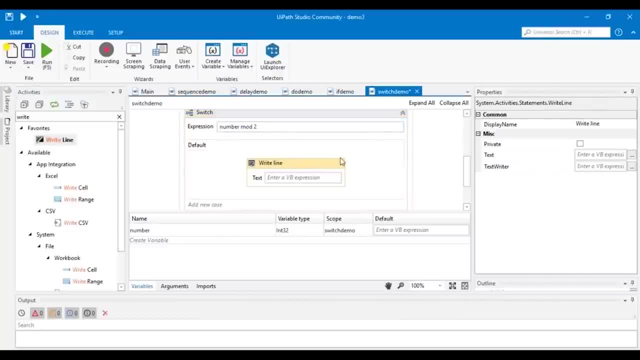 drop it here, All right in the text field. type in the expression as number to string and concatenate it with a string as is an even number. All right, after that, click on add new case and then mention the case value as one. Now again, add a right line activity here and then enter the. 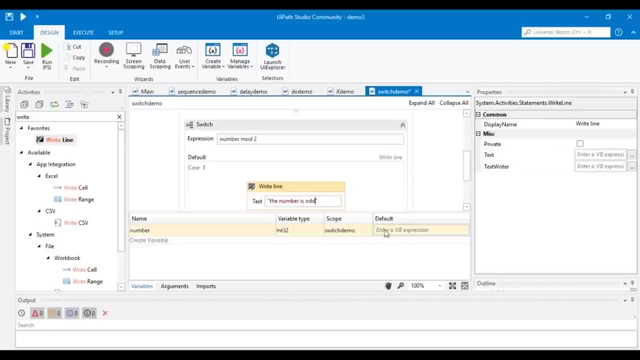 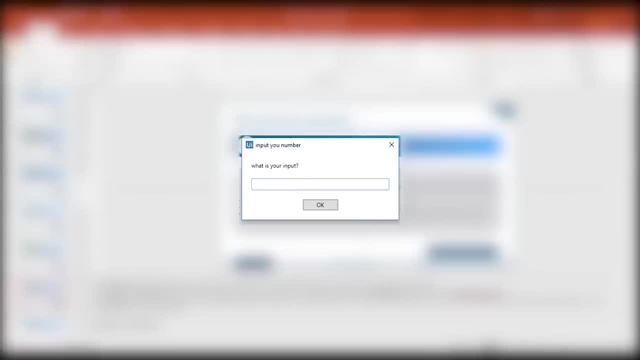 text that the number is odd. All right. So now, if you run this program, let's just see what happens. It's asking for my input, So let's say I put the input as 21 and click on Okay in the output panel. 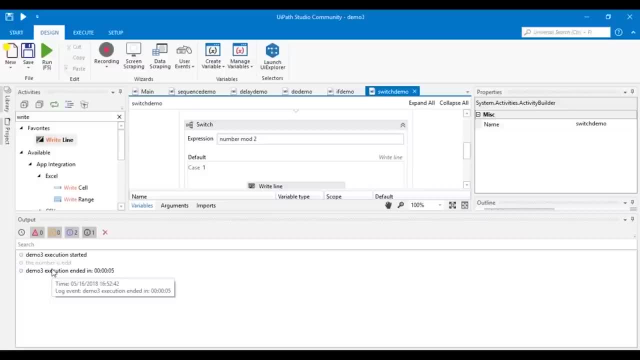 You can see that the number is odd is printed. That means it has gone to our second case, in which it is identified That it is getting a reminder right. So, guys, that's how you can explain the interviewer to answer questions related to the switch statement. 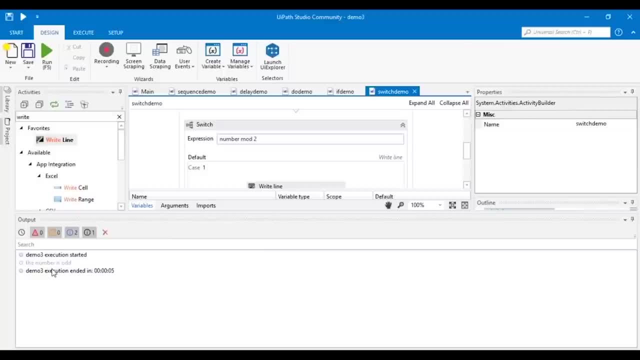 You can give a proper definition about the switch statement and then tell them about the basic syntax of switch statement and then after that, you can show different steps, how to create a simple project using switch statement. right Now, moving forward to the next activity, that is, the for each. 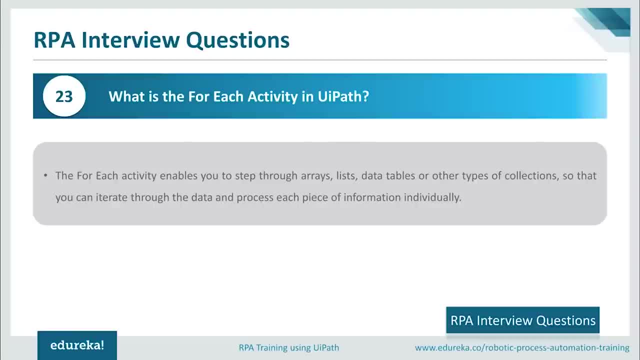 activity. So now, what is the for each activity in UiPath? Well, the for each activity enables you to step up the step through areas, list, data tables or any types of collections right, So that you can iterate through the data and process each piece. 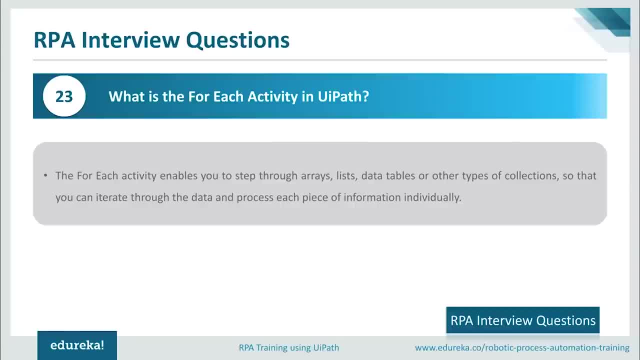 of information individually. So, basically, when you explain the for each activity, you can show the examples that for each item in a data table or any kind of data, You want the loop to run again and again, and again. So let me simplify it for you by showing you a short demo on. 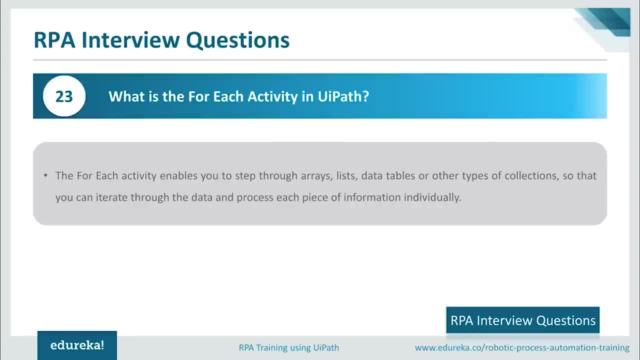 how to use the for each activity. So here we're going to create an automation that goes through each element of an area Integers and writes the length of an array and each element to the output panel, right? So let me just show you how to do that. 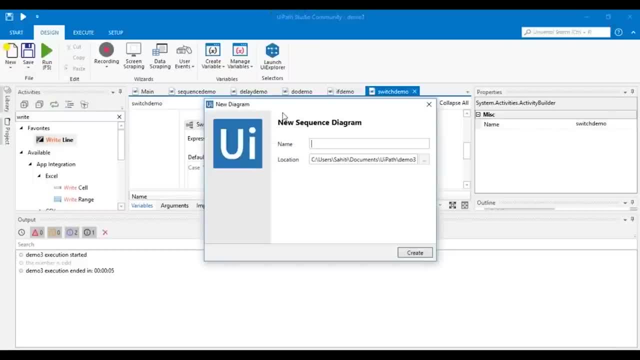 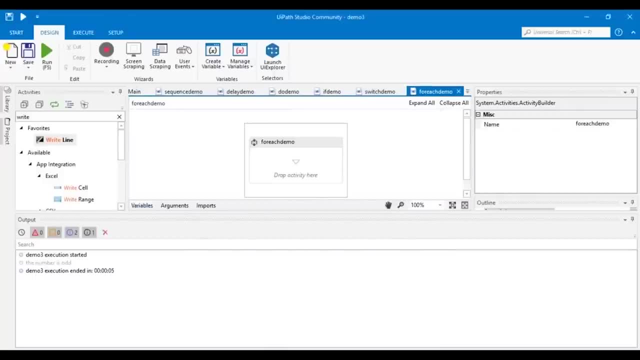 Let me just go back to the UiPath tool. Let me create a new sequence here. Let's say I create the sequence name as for each demo and click on create Once a new sequence is created. Let's create an array of integer variables. 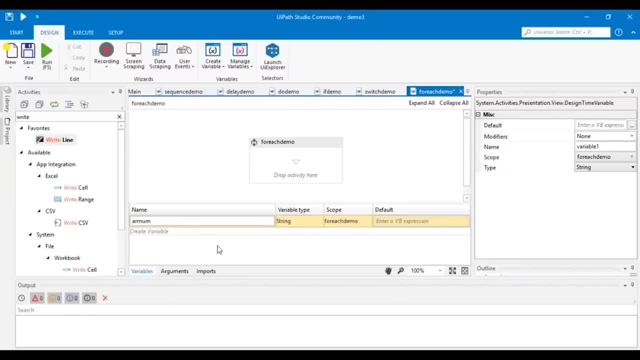 So if I mentioned the array name as array numbers of variable type, array of int, And in the default section let me mention some values, right? So let's just mention these values, All right. once it is done, let's add a for each activity. 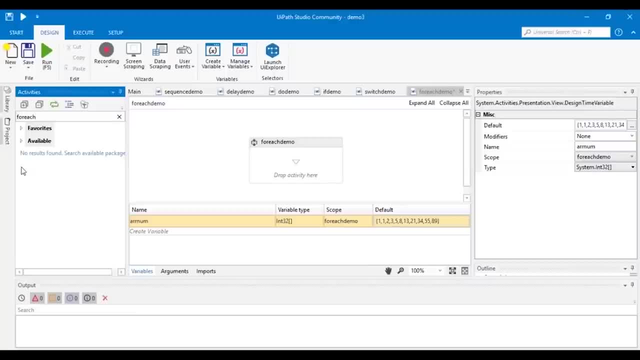 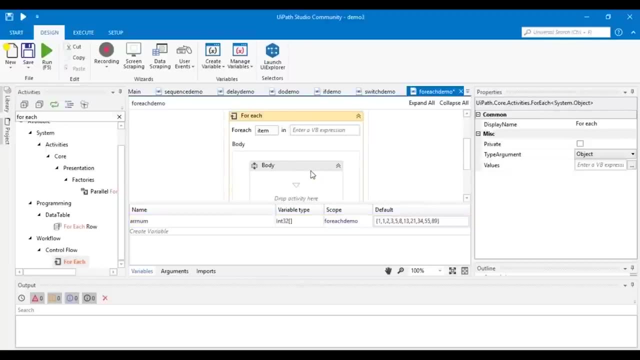 down. So in the activity pane let's search for the for each activity And then drag and drop it here. All right, So now in the infield of the for each activity we have to mention the array, right? So let's just mention this variable name. 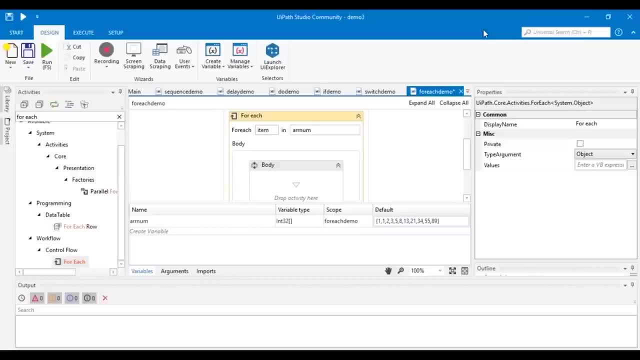 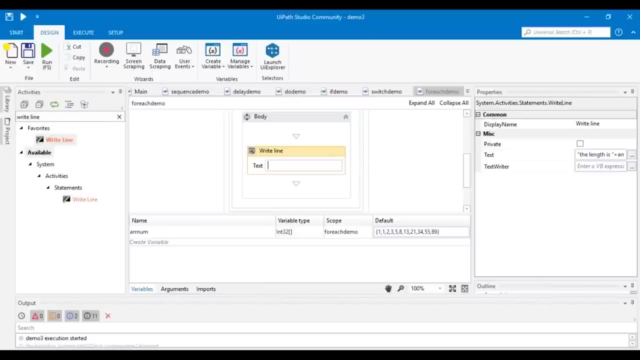 So basically, what's happening by mentioning the variable name is that this activity looks at each individual item in the provided variable. All right, Now in the body section of for each activity, let's add a right line activity. In the text field of the right line activity you have to. 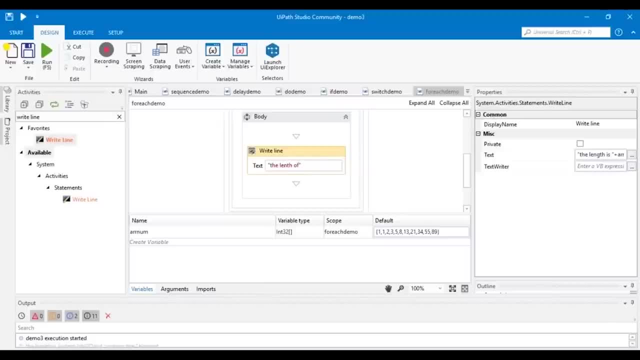 mention that string as the length of sequence is and concatenate it with the variable name and then mention the length option so that the length is calculated, and then again concatenate with a string With each item in the list, right? So let's just mention that. 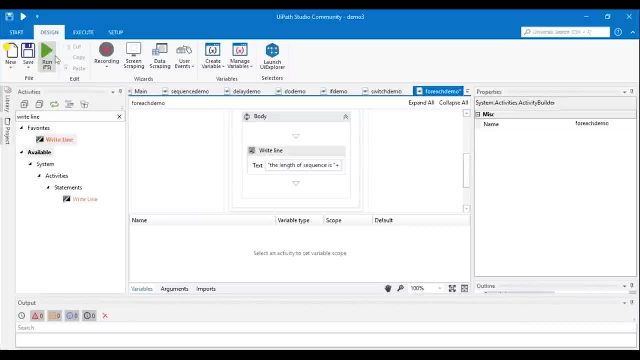 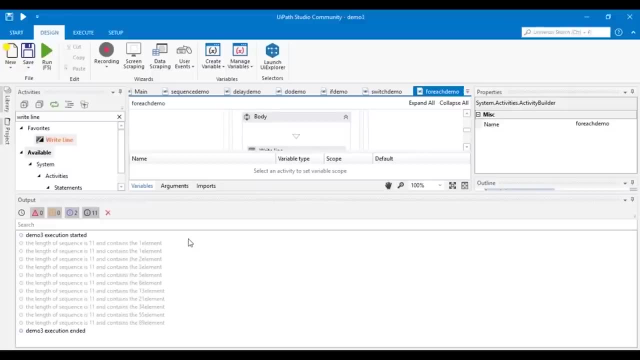 All right. So now, once it is done, let me just run this program and show you So. in the output panel you can see that the length of the sequence is 11 and contains the first element, the second element, the third, fifth, eighth, thirteenth and so on. 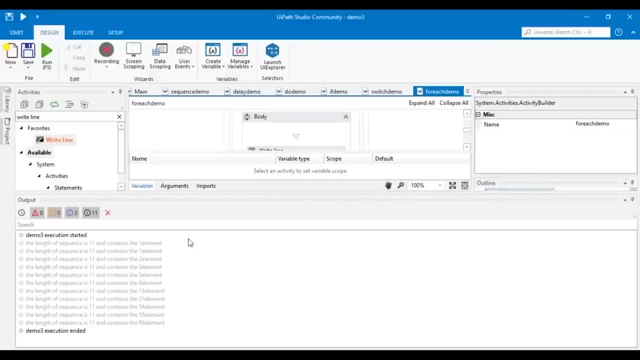 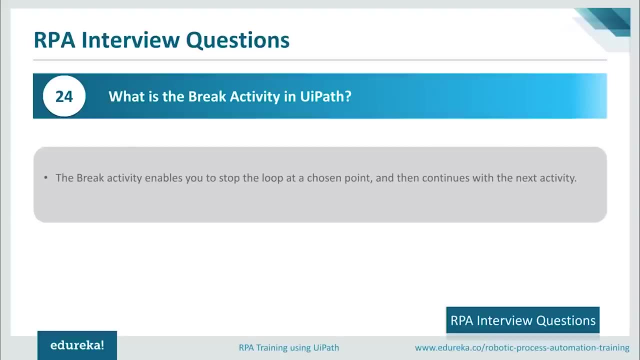 right. So with the length property you can find out the total number of array elements. Isn't it interesting? It's really interesting to answer this way, right. So now moving forward to the next type of activity we have on the list is the break activity in UiPath. 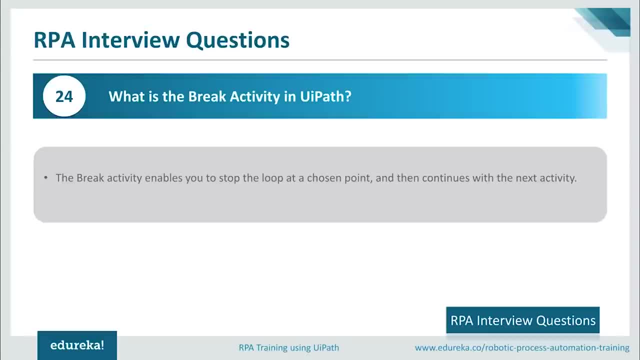 So the break activity enables you to stop the loop at the chosen point and then continue it with the next activity, right? So basically, whenever you use the break activity, you can stop complex tasks at a given point and then choose to run the next activity. 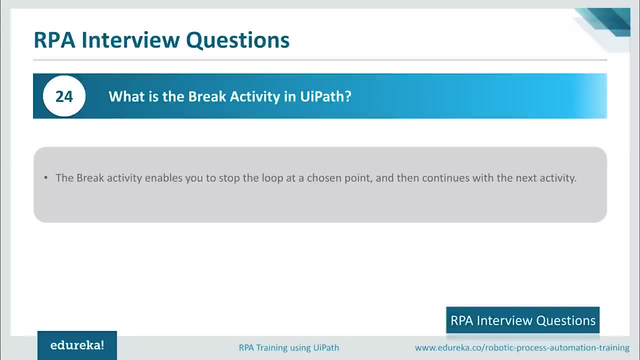 So let me just give you a short demo of how you can use the break activity right. So for that we're going to use the demo created for the for each activity and with this new project it only writes the first iteration of the loop and the few elements of array to. 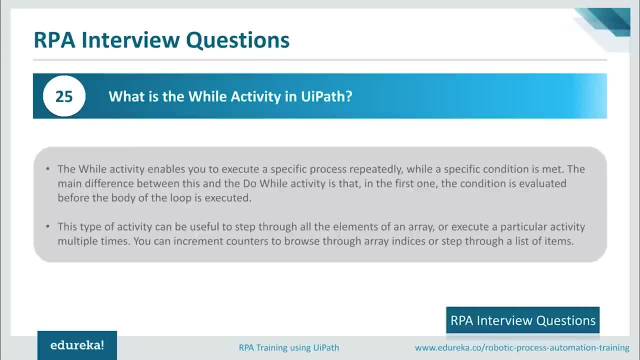 the output panel. So now let's move on to the next activity, That is, the while activity. So, guys, this is the last activity that we're going to discuss in the list. Until now, I've told you how to answer questions related to. 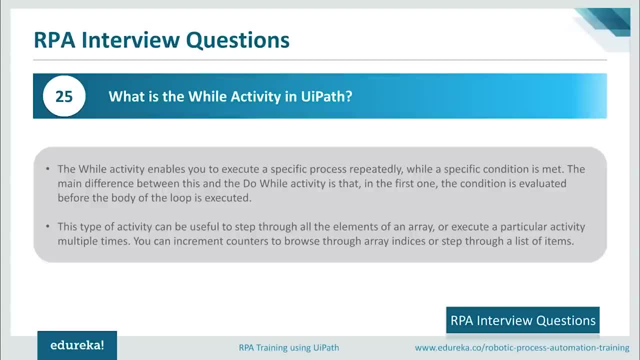 the if activity, the break activity, the do while activity, and so on. right, So now let's look into what is the while activity in UiPath. So when you talk about the while activity, the while activity enables you to execute a specific process repeatedly while. 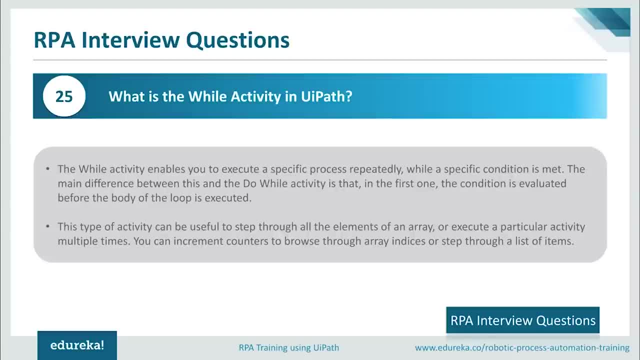 a specific condition is met. The main difference between this and the do while activity is that in the while activity, the condition is evaluated before the body of the loop is executed right. So this type of activity can be useful to step through all the elements of the array or execute a particular activity. 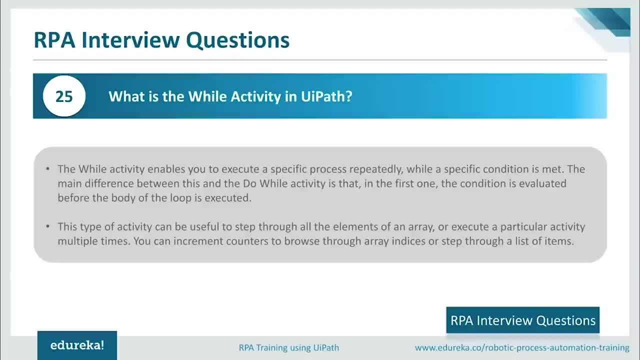 multiple times, or you can increment the counters to browse through array indices or step through a list of items, right? So basically, you can use the while activity when you have specific set of conditions and you want to perform that task if the condition is met. 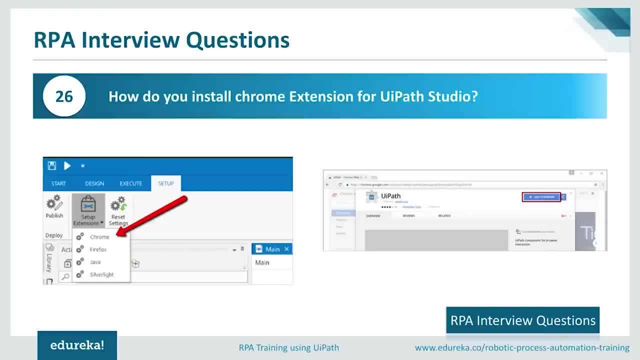 All right. now moving forward, Let's look into the next set of questions related to UiPath right. So now on the list, we have a question, that is, how do you install the Chrome extension for UiPath studio? Well guys, the steps to install the Chrome extension is really 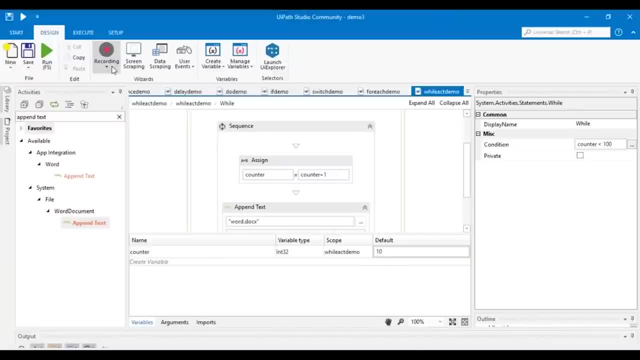 simple, All right. What you have to do is you have to just go to the UiPath tool, You have to go to the setup ribbon tab and then choose setup extensions, right? So in this option you can go for Chrome, Firefox, Java and silver. 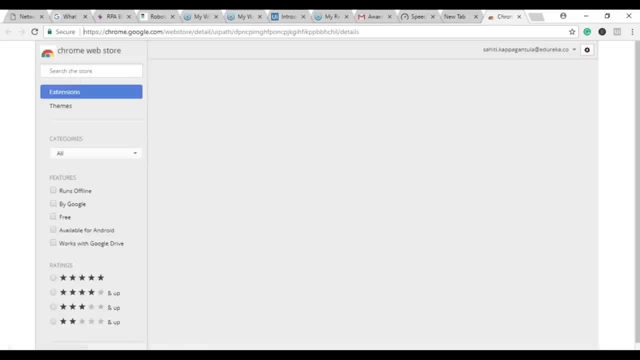 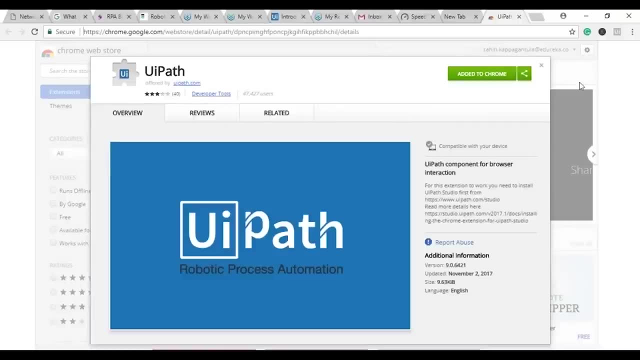 light. All right, when I go for the Chrome option, I'll be redirected to this page where there is a confirmation dialog box in which we have to click on the add to Chrome button, since I already have it added on my UiPath tool. 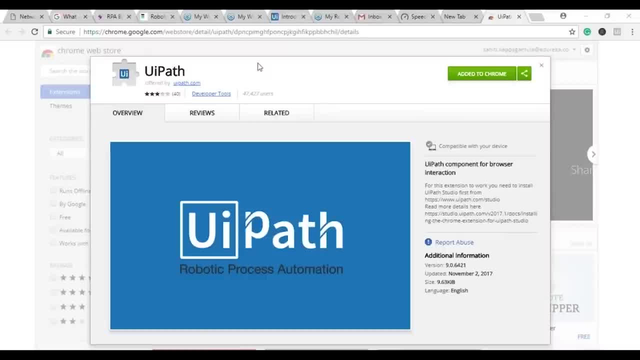 I need not do that, But else if you want to add this extension, you just have to click on the add extension button. So that's how you can install the extension. Now let me tell you one more interesting here. Once you click on the add extension button, the UiPath. 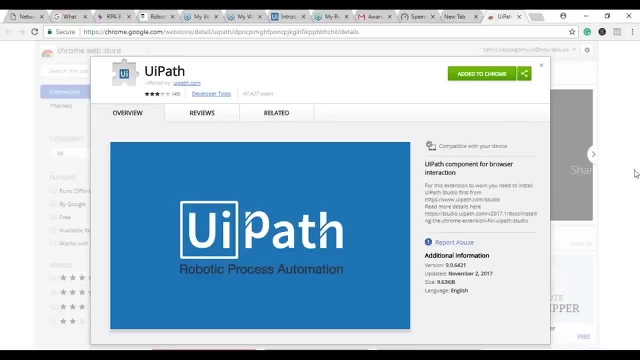 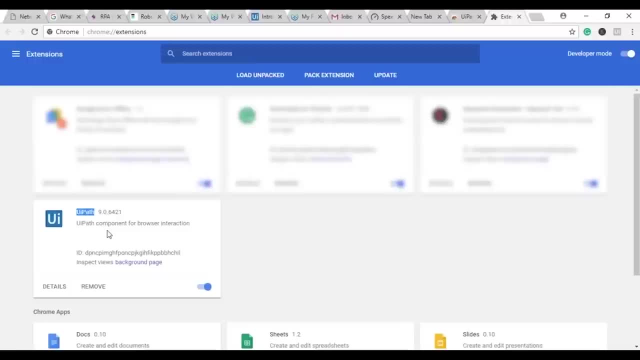 extensions are disabled by default. to enable them, What you have to do is you have to go on this site navigation bar, go to more tools, go to extensions. here You just have to click on this UiPath option and then give access to all the URLs, right? 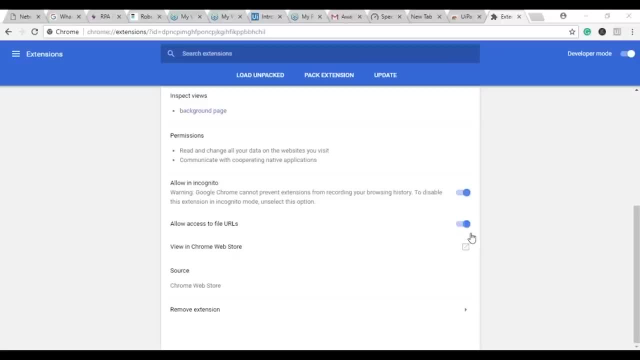 So I've already given access to all the URLs. If you haven't given the access after installing the extension, then the extension won't work for you. So this kind of questions can be also asked by the interviewer, which are basically scenario based or based on steps, Etc. 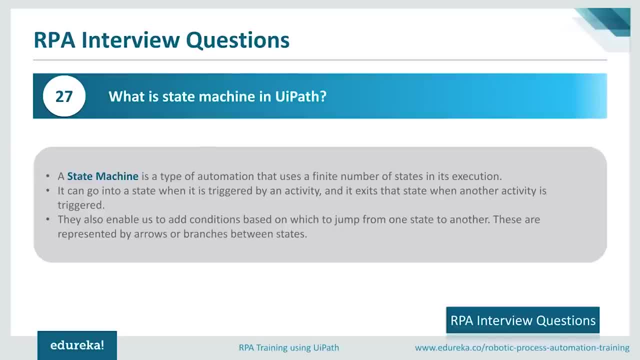 Right. So now let's look into the next question. So what is a state machine in UiPath? So when you talk about state machine, state machine is a type of automation that uses a finite number of states in its execution. It can go into a state when it is triggered by an activity and 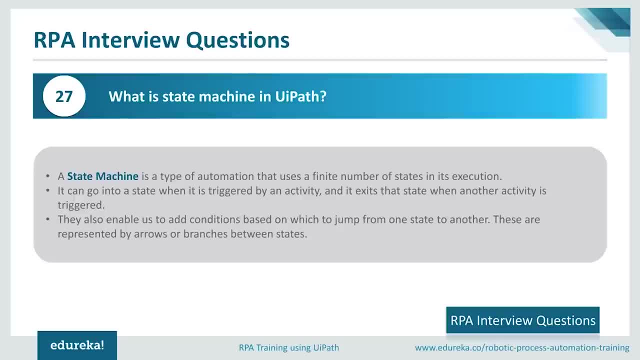 then it exits that state wherever other activity is triggered, right? So basically, in layman language, when you talk about states, when you travel from one state to the under the state, you trigger few activities, right? So that's what a state machine does. another important aspect: 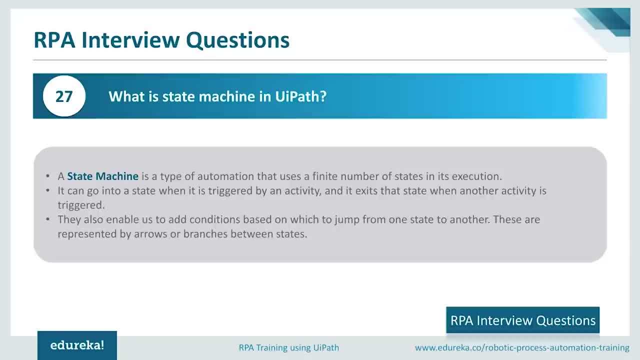 of state machines are the transitions, So they enable you to add the conditions based on which you have to jump from one state to the under the state. So basically, these are represented by the arrows or branches between the states. So when I interview questions you about the state machine. 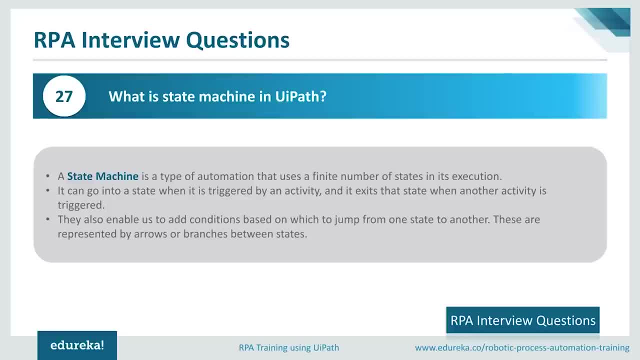 always remember to talk about the states, the transitions, the activities and all So, guys, there are basically two type of activities that are specified to the state machines, that is, namely the state and the final state, and to find them under the UiPath, you just have to go. 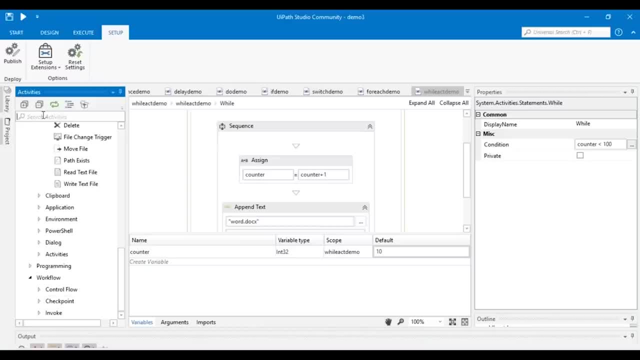 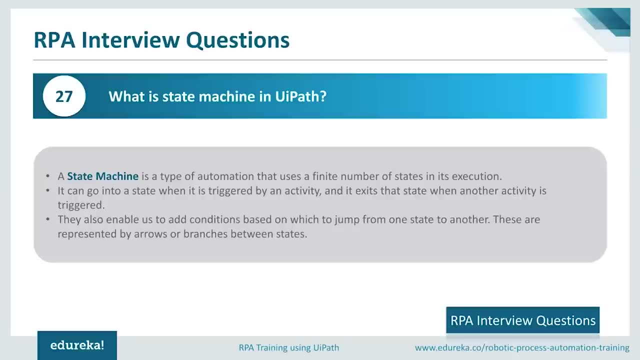 to the UiPath tool and then you can find it here under the state machine, right? So let me just type and show you see, this is where you can find your state machine. So basically, the state activity contains three sections, that is, the entry section, the exit and the transition section. 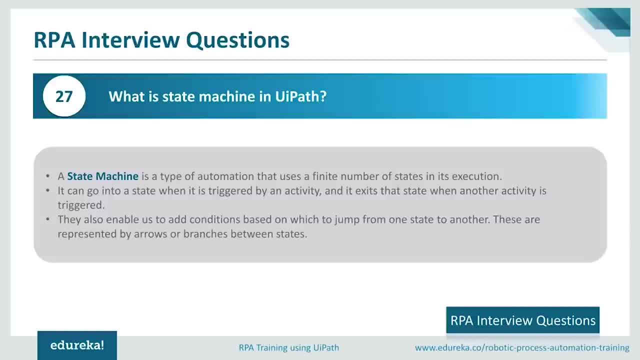 right. So when you talk about the initial state and the final state, the initial state contains three sections: The entry state, the exit state and the transition state- and when it comes to the final state, it only contains a single section, that is, the entry section. 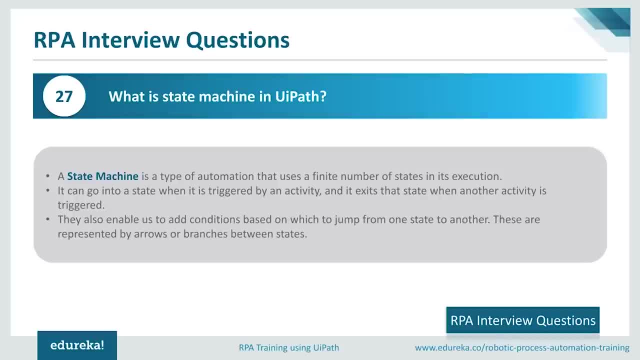 right. So that is pretty obvious that you understand that all the input from the initial state is passed on to the final state. All right. now talking about the entry and the exit sections. these enable you to add entry and exit triggers for the selected state, while the transition sections display all the transitions. 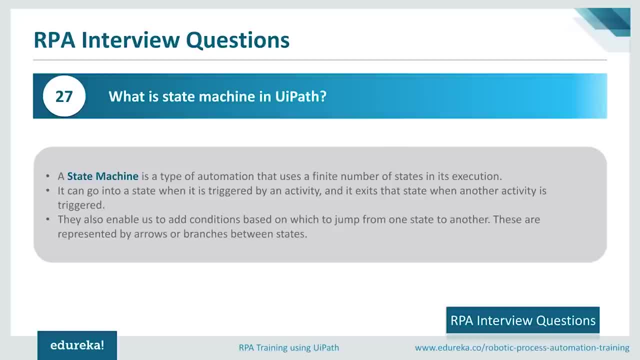 linked to the selected state. All right, if you're ever questioned about the state machine, you should always talk about the different types of states, how you can enable them in the UiPath tool. What do you understand by the term transition the activities, how many activities the initial state has and how many activities. 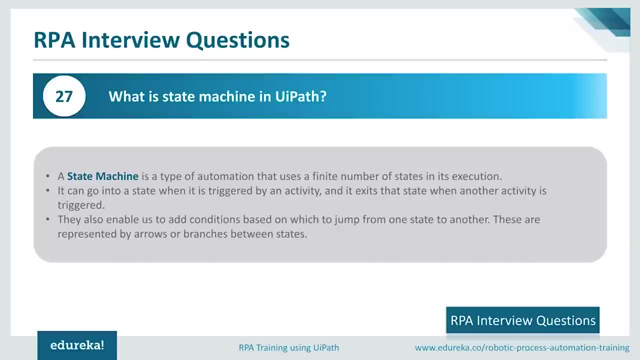 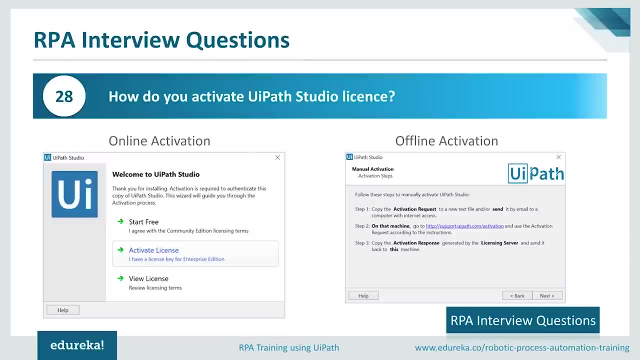 the final state has, and what do these each trigger right? So now moving forward to the next question. We have learned so much about UiPath tool, but how do we activate the UiPath studio license? Well, as all of us know that UiPath offers the community. 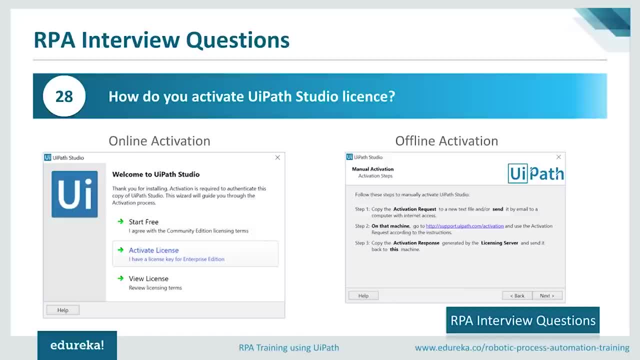 edition and the pro edition. the community edition is the basic trial version And, coming to the pro edition part, It is the licensed version, right? So to activate this license version you have to follow some steps. So, basically, these steps can be sometimes asked by the. 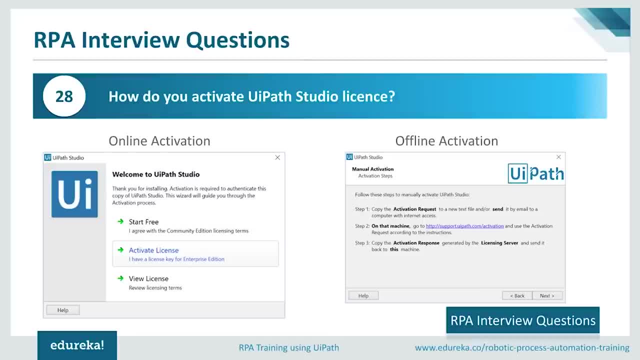 interviewers, as they would like to check if you have the basic knowledge about UiPath tool or not. So to activate the license, what you have to do is, after running and installing the studio for the first time, the user is prompted with the license activation wizard. 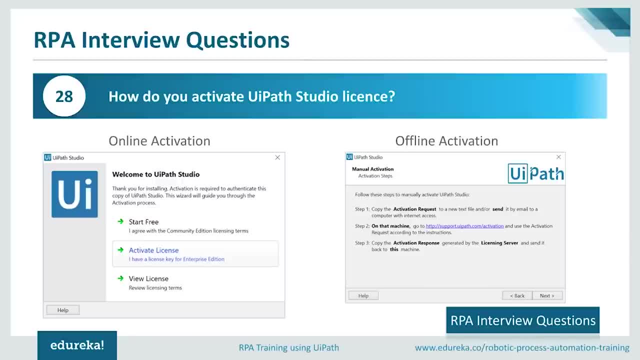 right. So in the wizard you have to choose the activate license button. Once you choose this, the UiPath registration window is displayed in this particular window. You have to fill in the email address, You have to fill in the license key which you have received. 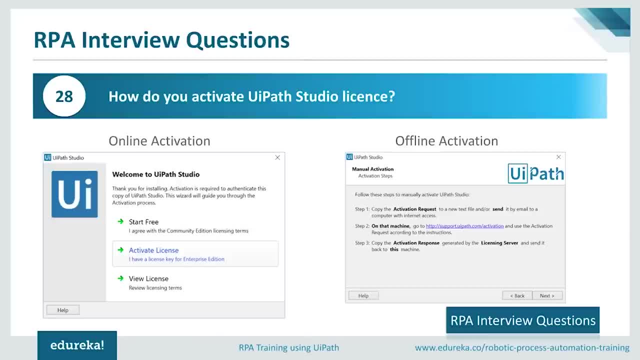 and then you have to select the automatic activation option. Once you select that, you have to click on the activate button and your UiPath license is now activated and you can start creating automation workflows. All right, So, guys, the steps that I just told you were for online. 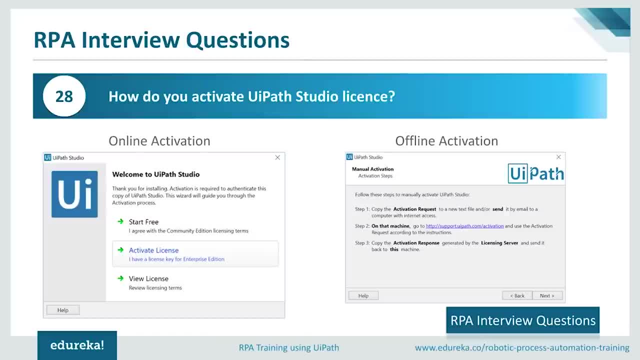 activation Now. if you want to activate your license offline, then what you have to do is you have to just click on that activate license button, as your UiPath studio opens, and then the UiPath registration window is displayed, In that you have to fill in the email address and then fill. 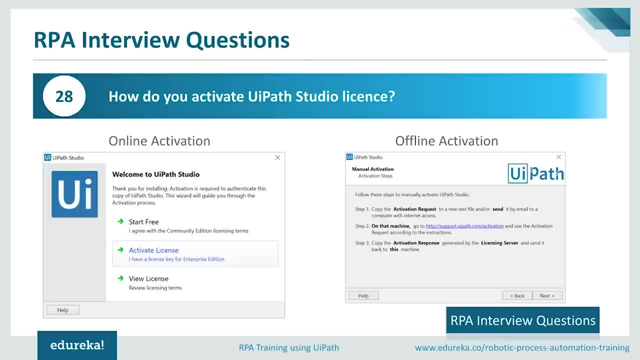 in the license key which you will receive to your email ID. Once this is done, you have to select the manual activation option and then click on activate. So once you're done with this, the wizard is updated accordingly and displays the next steps required to go through with the. 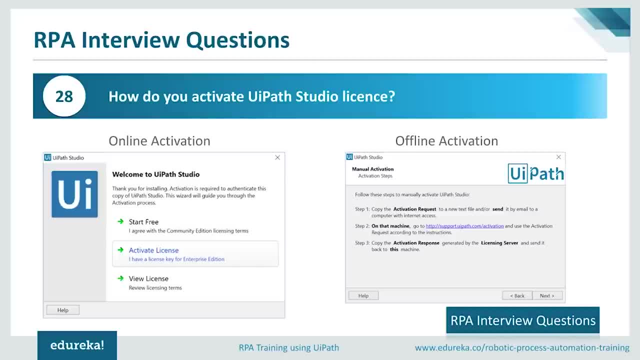 online activation right. So after that you just have to to click on next and then continue with your activation. So, in short, when you're asked about how to activate the UiPath studio license, you have two options: the online activation and the offline activation. So you just have to follow those steps that I just briefed you, else you will. 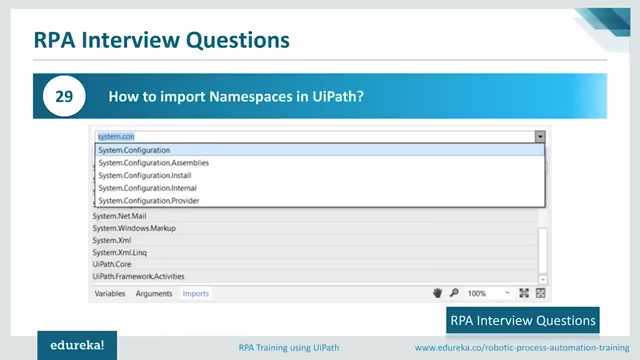 find them on the UiPath official website. All right, now, moving forward, we have a basic question here, asked by the interviewers on how to import namespaces in UiPath. So to import the namespaces in UiPath you have to follow some steps right? So for that let me just go back to my UiPath studio. 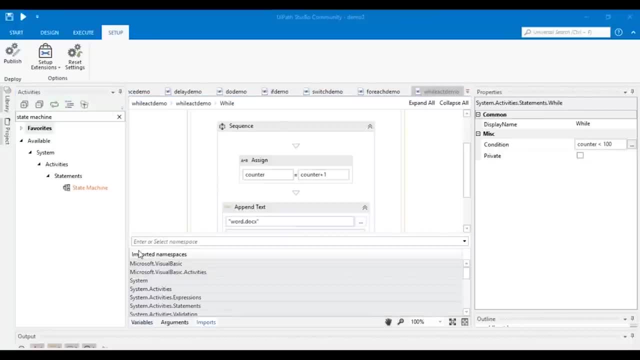 and then let me just open the imports panel here. Once you open this imports panel here in the enter or the select namespace field start typing the namespace that may interest you. So suppose I type in system dot configuration. So once you type in something in the select or the enter namespace, 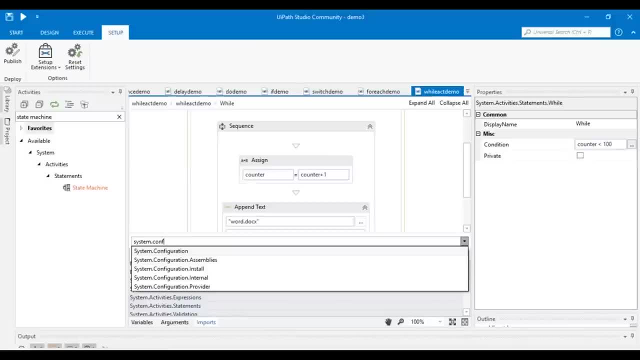 field, you'll get a drop down arrow to view all the namespaces available, right? So you have to just select the desired namespace and then the namespace is added to the imported namespace list. All right, and just in case, if you want to remove a namespace, then you just have to. 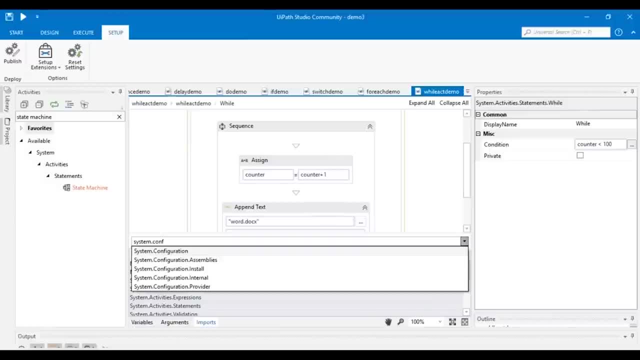 select it and press on delete. All right now let me tell you one interesting fact here: that the namespaces can be only deleted if they aren't used. For example, you can delete a namespace if the assembly that contains it is no longer referenced by the project. So these are the basic steps to 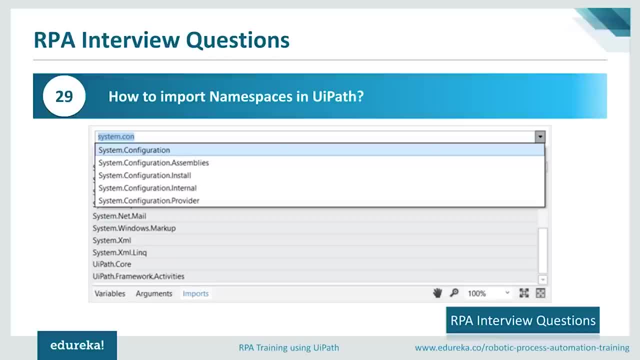 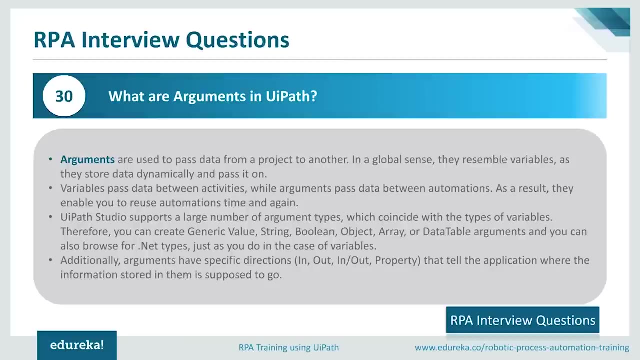 import the namespaces in UiPath. You don't have to go to the imports panel. you have to enter the desired namespace and it will automatically get imported. If you just want to remove it, then you just have to press on delete. All right, So now, moving on to the next question. Now that you know what variables are and what imports are, 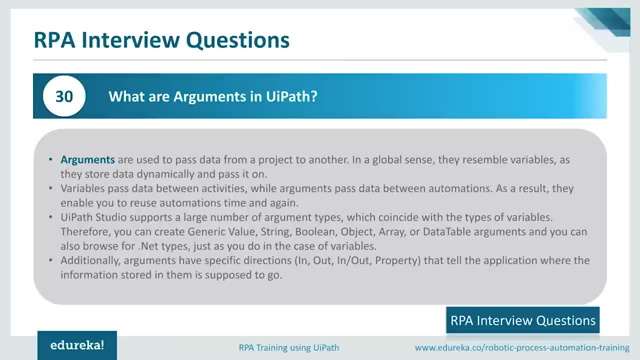 Let's look into what arguments are in UiPath. So when you're asked about arguments in UiPath, I would always suggest you to compare it with variables and imports. So in short, variables is something that always changes, right? It does not have a constant value. 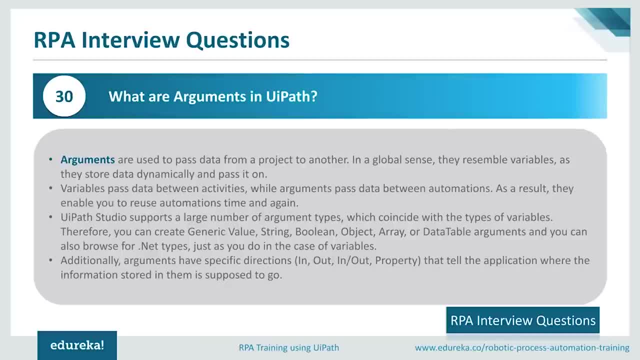 When it comes to imports, imports is basically that you want to import any namespaces, But when you talk about arguments, arguments are generally used when you want to pass the data from one project to another project. In global sense, there are simple variables, as they store data dynamically and pass. 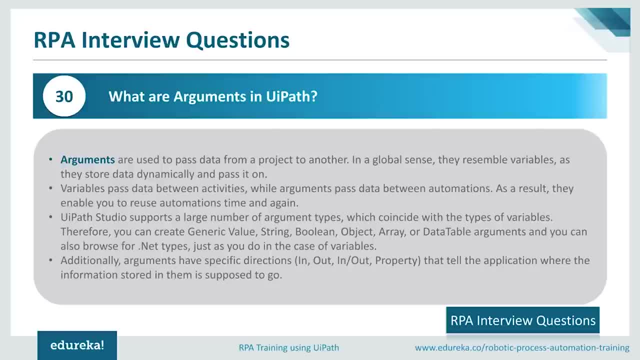 it on: Variables pass data between activities, while arguments pass data between automations, Right? So it's really interesting that you explain this way that variables pass data between activities. So it's really simple, right? There are hardly any activities And arguments pass data between automations. So when you want to pass something from one project to another project, 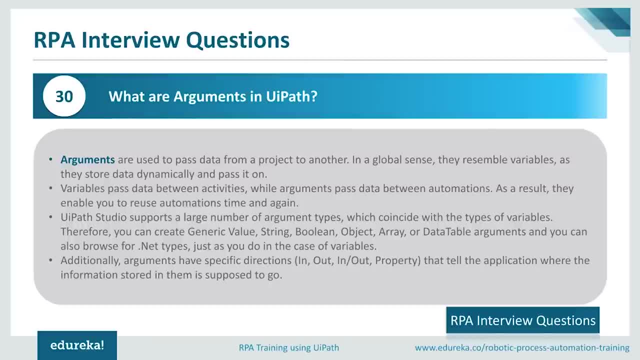 then you use arguments. As a result, they enable you to reuse automations time and again. So, to add to your knowledge, UiPath Studio supports large number of argument types which coincide with the type of variables. Therefore, you can create generic values, string, boolean, object array or data table arguments. 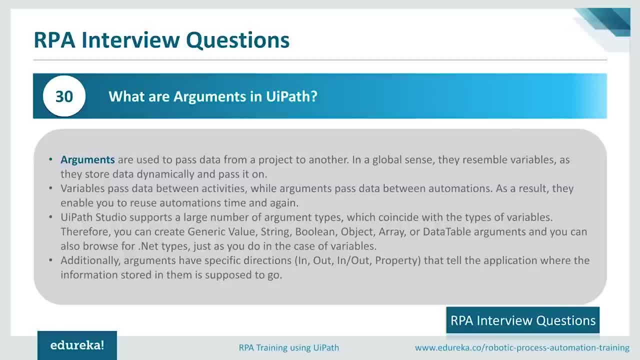 And you can also browse for dot net types, Right. So that is the same way you do in the case of arguments. is of variables, right? Additionally, arguments have specific directions, like in out, in out, property, etc. that tell the applications where the information is stored and where they're supposed. 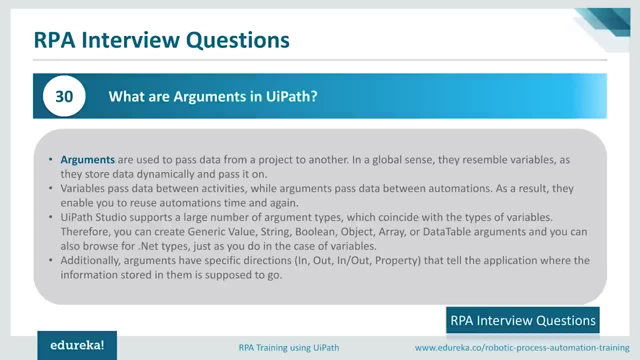 to go All right. So, in short, arguments are used when you have to pass data from one project to another project to automate it at a higher level. Now let's look at a short demo on how to remove and create arguments. So let me just go back to my UiPath tool: remove this. Let me go to the 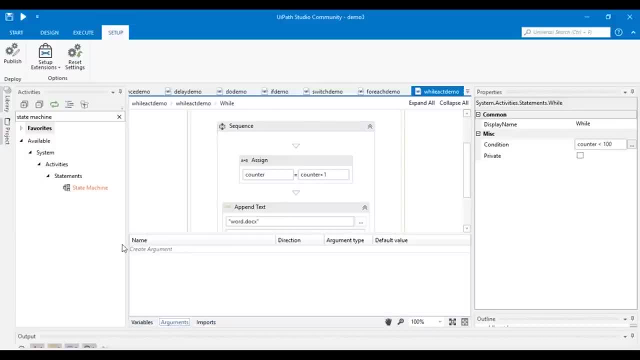 argument panel and then in the argument panel you can create an argument here, right. So to create an argument, you just have to type in something and then you can give the default values. the same way you create variables. to remove any arguments, You just have to right click on. 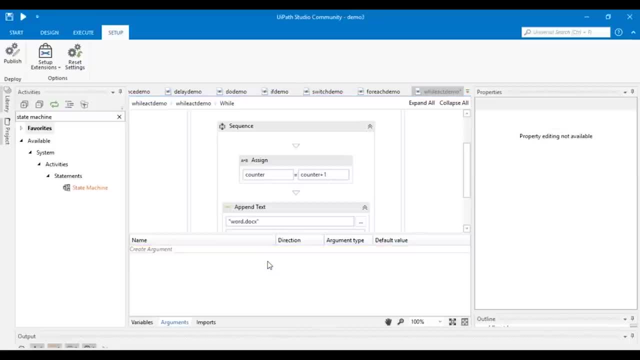 this created argument and then click on delete. this automatically deletes your argument, Isn't it simple, right? So whenever you're asked this question on what argument is, always try to compare between variables and arguments and then finally talk on how you can remove any arguments from your argument. So let's go ahead and remove any arguments from. 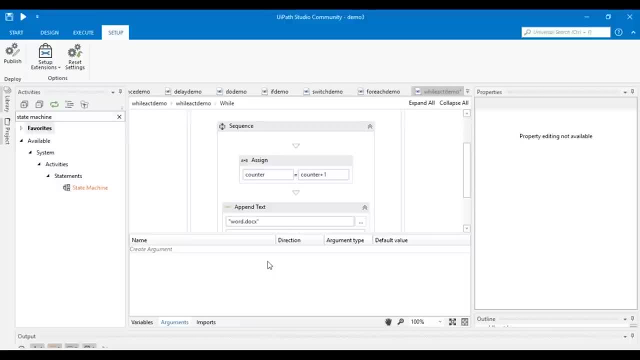 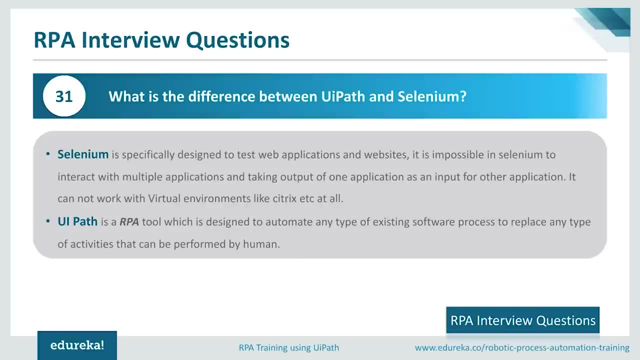 your argument. You can create and remove arguments in UiPath tool, All right. So now, next in the list, We have a very interesting question that is generally asked by the interviews, that is, what is the difference between the UiPath and selenium? So when you talk about selenium, selenium is. 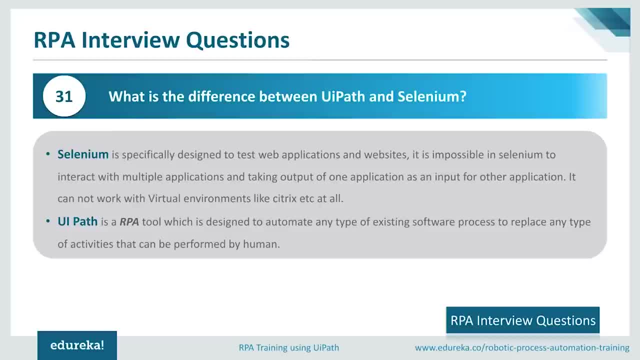 specifically designed to test web applications and websites. It's impossible in selenium to interact with multiple applications and take the output of one application as an input for the other application, right? So if you're dealing with multiple applications and you want to take an output of one application and give it as an input to another application, then you can never use. 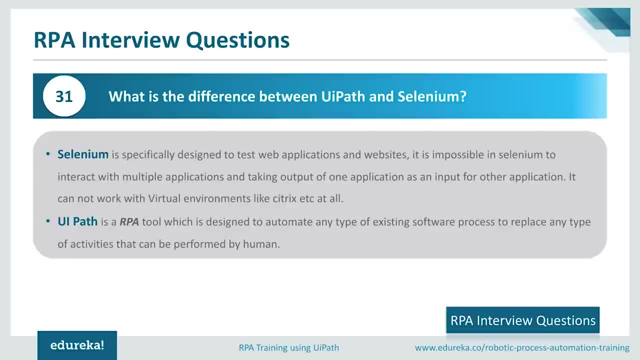 selenium. This is because it cannot work with virtual environments like Citrix, All right, but when it comes to UiPath, UiPath is an RPA tool which is designed to automate any type of existing software's to replace any type of activities that can be performed by a human being, right? So we? 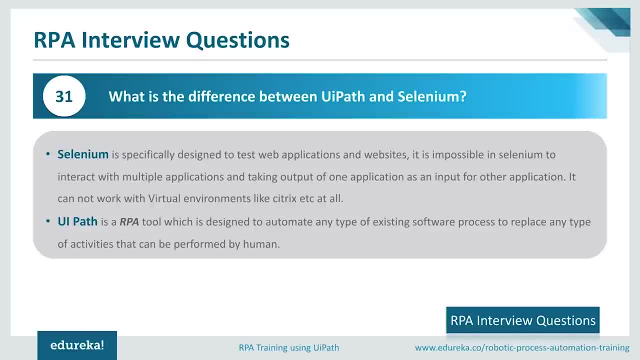 can see that RPA is the next level of existing automation tools, So it allows people to build complex, rules-based processes with very simple steps, with very little software development skills. You can do all things using UiPath, which can be done by selenium. 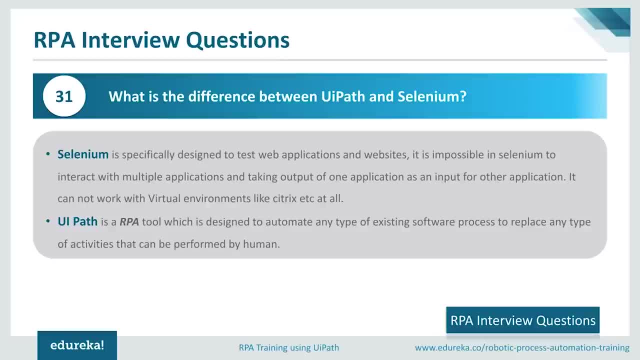 but vice versa is not at all possible. So I would say UiPath is better than selenium in some cases where we have to deal with multiple number of applications and we want to pass the output of an application as an input to the other. So now, next in the list, we have a question which confuses. 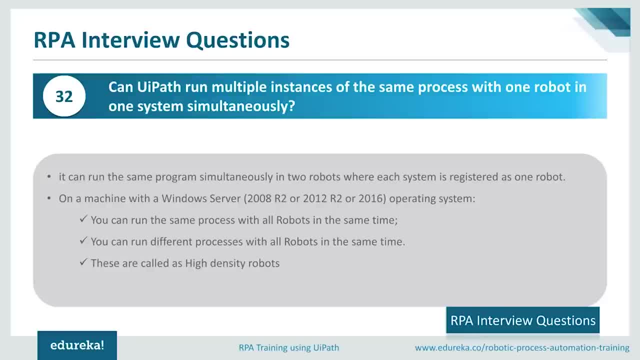 many people. Can UiPath run multiple instances of the same process with one robot in one system simultaneously? Well, the answer to this question is yes, as it can run the same program simultaneously in two robots where each system is registered as one robot, So the same machine can be registered as multiple robots. 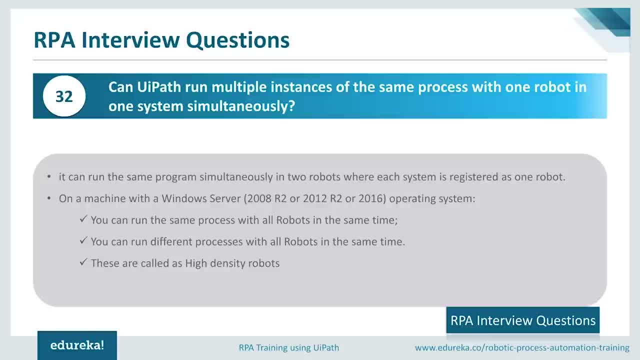 So when I'm talking about the machine, I'm talking about your desktop. on a machine with Windows Server, you can run the same process with all the robots, or you can run different processes with all robots, right? So these kind of robots are known as high-density robots. So if you're asked in your 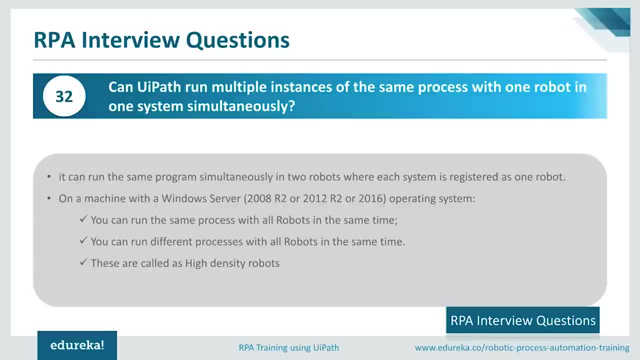 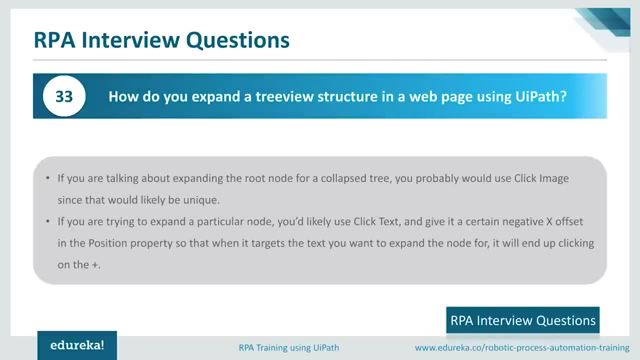 interviews about the high-density robots, then they're talking about n number of robots working on the same process or different processes right Now. next question in the list is: how do you expand the treeview structure in a webpage using UiPath? So when you talk about expanding the treeview structure, then there are various cases, right. 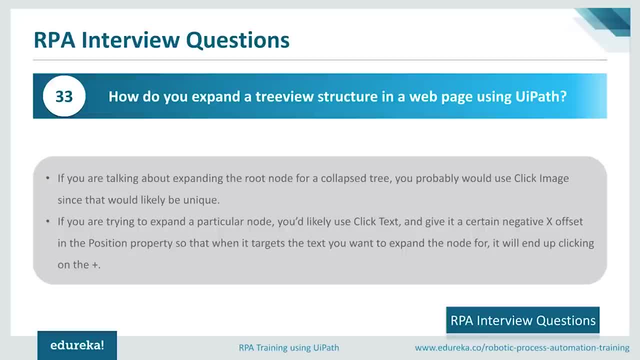 So if you're talking about expanding the root node for a collapsed tree, then you would probably use click image, since that would likely be unique. But if you're trying to expand a particular node, you would likely use click text And give it a certain negative X offset in the position properties so that when it targets the text you want to expand. 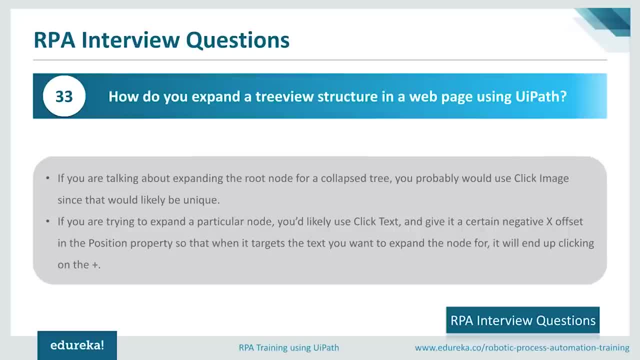 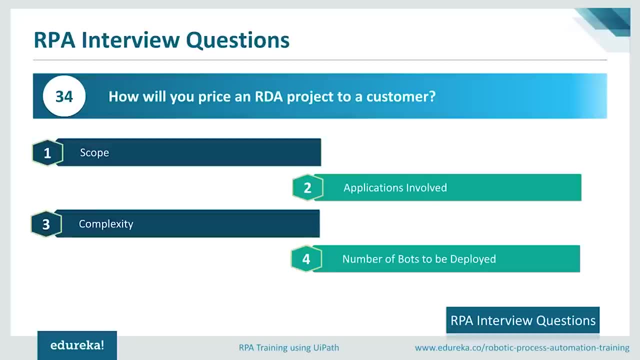 the node, for it will end up clicking on the positive sign. Alright, so that is how you can expand the treeview structure in a webpage using UiPath. Now, this is one of the most frequent questions asked in the interviews: How will you price an RDA project to a customer? 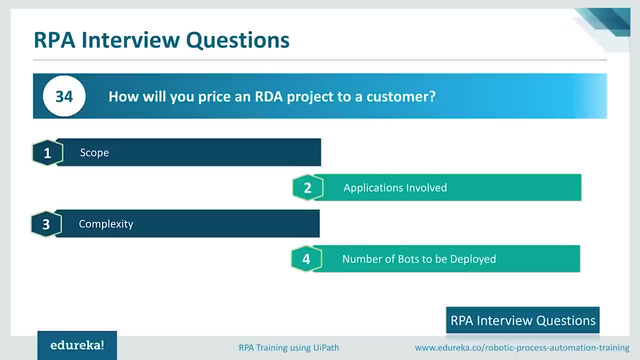 So if you are a RPA developer, then you should know how to price your RDA project to a customer. So to price your project, you have to consider four parameters: the scope, the application involved, the complexity and the number of boats to be deployed. 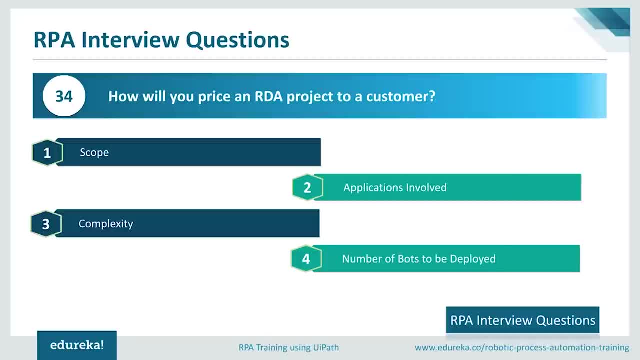 All right. So first we identify the scope of the automation, like how business processes flows or how many applications are involved, or how complex are the interactions between these applications. Once we know all of these, we will work out the number of boats to be deployed and then estimate the cost for each boat to develop and deploy. 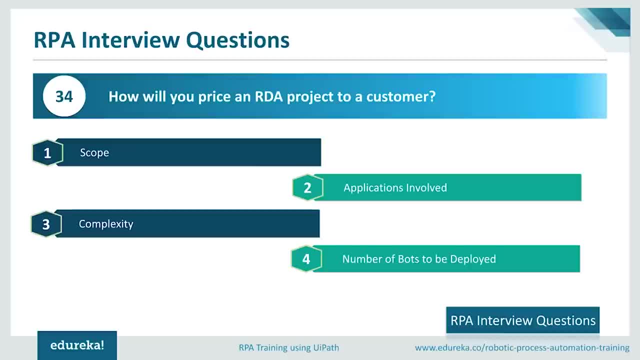 This is how we do at a high level, that is, I'm talking about a large scale company, Right? So usually, based on the complexities involved, the project may go anywhere between 6 to 12 months. So this should be your answer to price an RDA project. 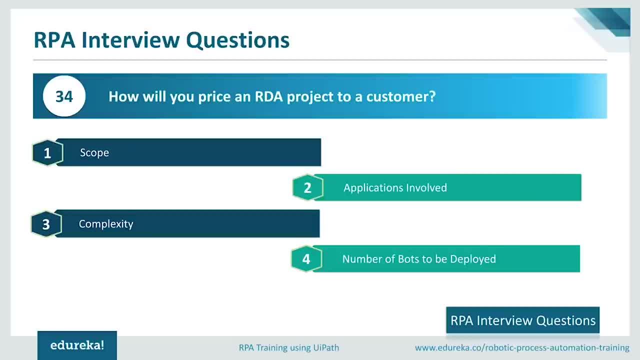 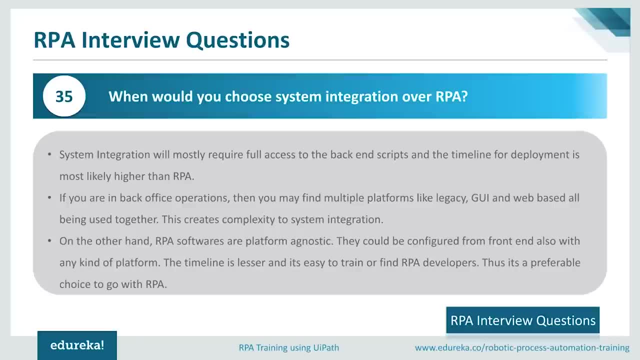 You have to consider the scope, applications involved, complexities and the number of boats to be deployed. right now, You must have heard about system integration, right? So our next question is: when would you choose system integration over RPA? Well, I would say we would prefer system integration. 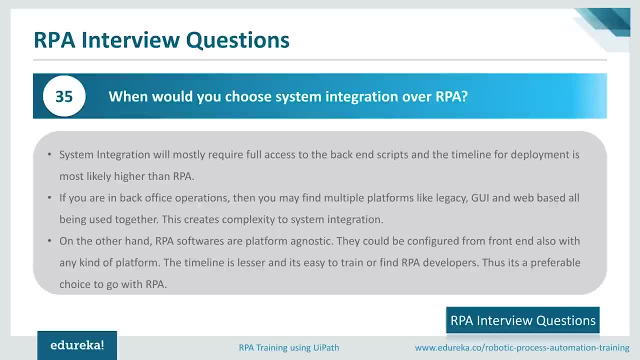 if the return on investment is better than deploying RPA. but obviously you will find only few projects which will have that kind of scenario. So I would suggest if you're working in the local environment and have similar kinds of platforms or software's, then you should go for system integration. 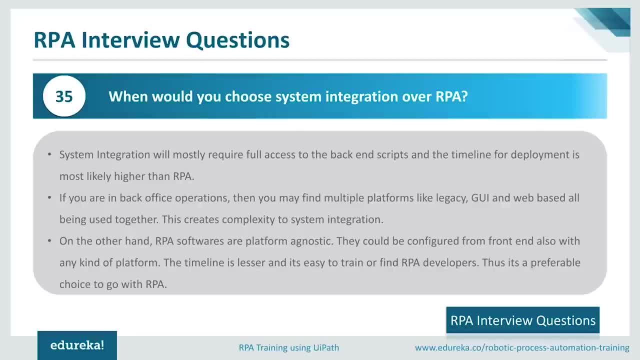 System integration will mostly require full access to the back-end scripts and also the timeline for deployment is most likely higher than RPA. So if you're in the back-end operations, then you may find multiple platforms like legacy, GUI and web-based all being used together. 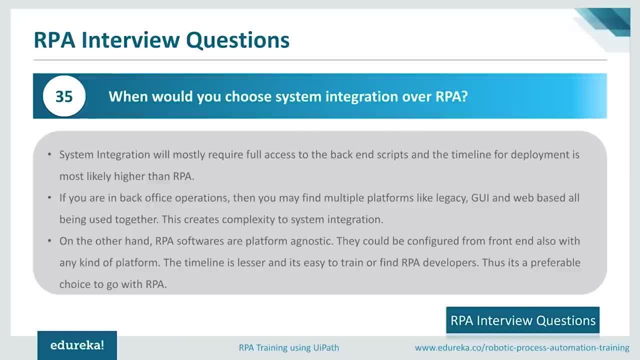 This creates complexity to the system integration. On the other hand, when you compare RPA, RPA software's are platform agnostic. They could be configured from front-end also with any kind of platforms right. So the timeline is lesser and it's easy to train or find RPA developers. 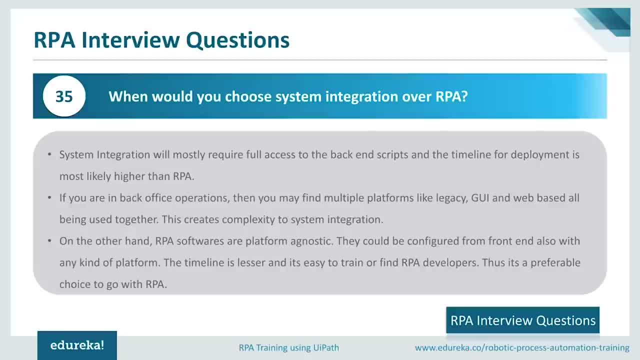 So therefore, I would say the preferable choice is to go with RPA, But yes, there are some cases that you need to use the system integration. So the answer to this question is completely situational based right. So whenever you have large projects, 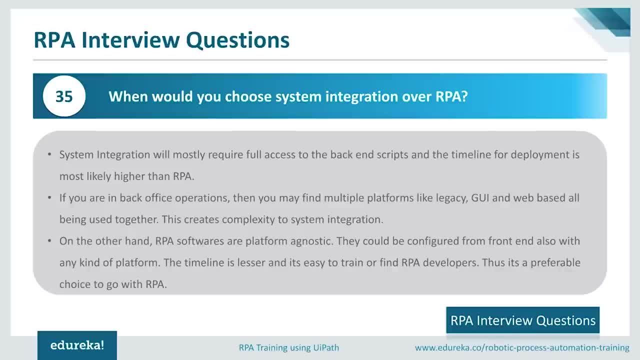 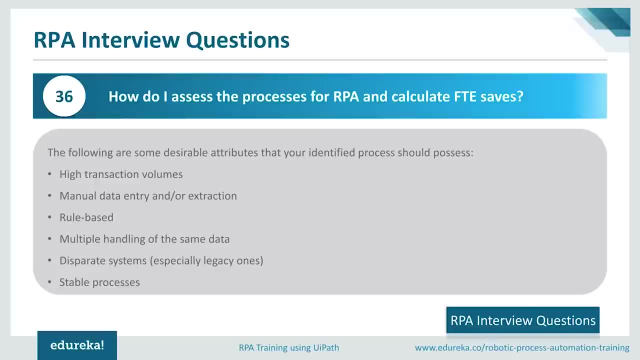 and you think that the return on investment is better than RPA, then you would use system integration, All right. So the next question on the list is: how do we assess the processes for RPA and calculate the FT? saves right So well. 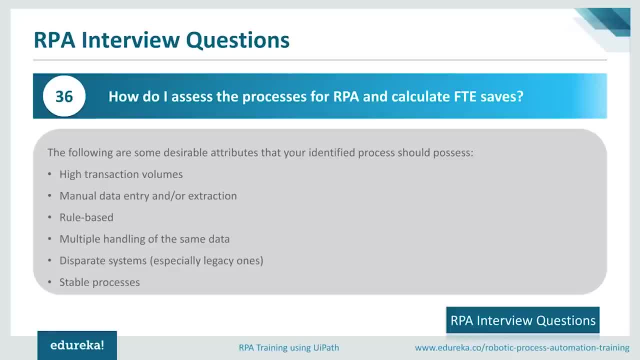 there are no hard and fast rules, but there are a few desirable attributes that your process should possess. It should possess high transaction volumes. It should have manual data entry or extraction. It should be rule-based. It should have multiple handlings of the same data. 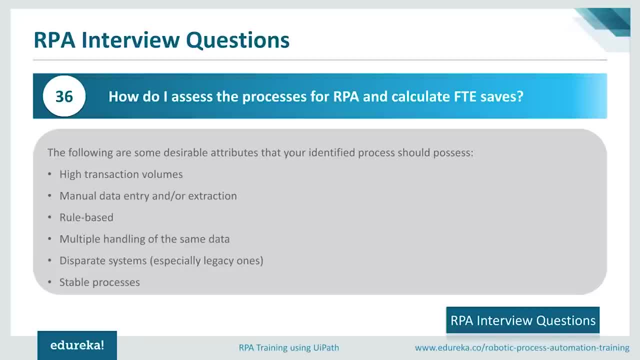 It should be discrete systems and stable processes right now. regarding the full-time equivalent savings, The concept is rather simple. You need to determine how long it takes an employee to complete the transaction currently and estimate the time it will take a board to complete the same transaction. 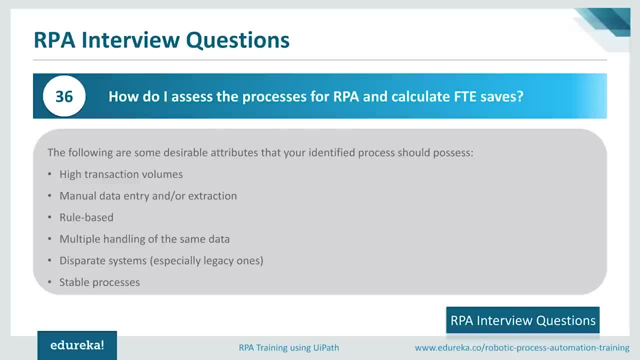 right. So you're basically going to compare the time a human and a board take to do the same transaction. The time savings per transaction completed, multiplied by the number of transactions, will give you the figure you need. Also, let me tell you one interesting fact here: that the challenge 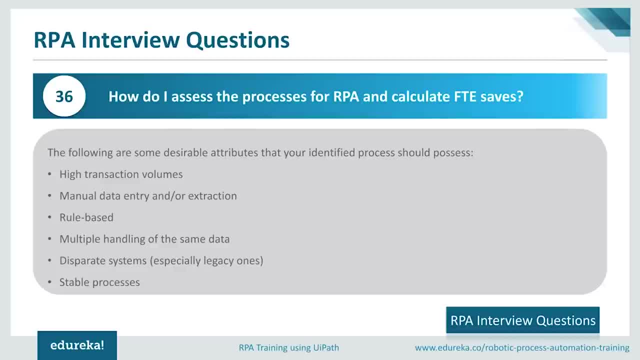 when calculating the FT savings lies in justifying and validating the assumptions you have made. So if you have to assess the processes for RPA and calculate FT, then you have to look into all these parameters. All right, So now moving forward to the next question. 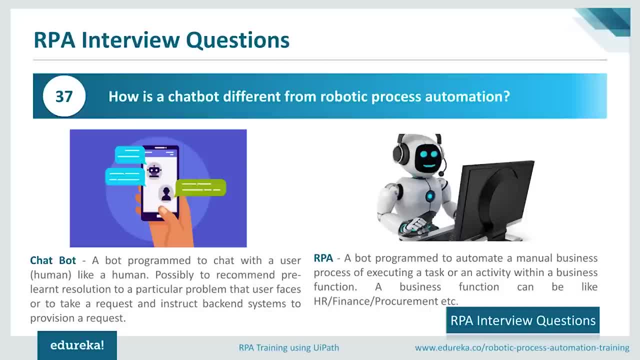 The next in the list is also very frequently asked question, That is, how is a chatbot different from robotic process automation? Well, to explain you the difference, the difference between the chatbot and a RPA engine is similar to the difference between a mouse and a mammoth. 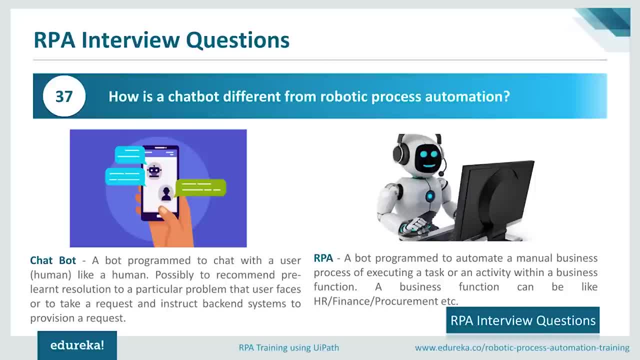 right, So by the names. the chatbot is programmed to chat with a user like humans, possibly to recommend pre-learned resolution to a particular problem that a user faces, to take requests and instruct the back-end systems to provision a request. when it comes to RPA, the RPA board is programmed to automate a manual business process. 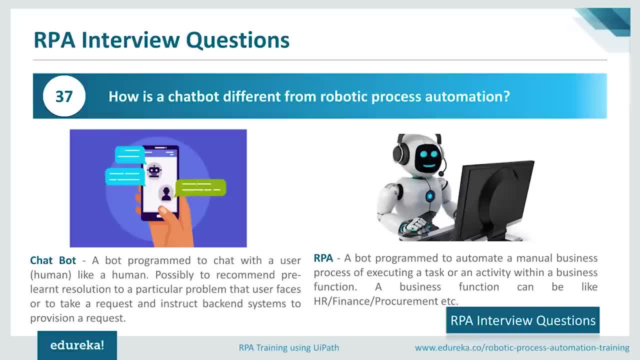 of executing a task or an activity with a business function right. So that's a huge difference between a chatbot and an RPA board. So chatbot basically helps the human, but an RPA board automates the manual business process and takes it on itself. 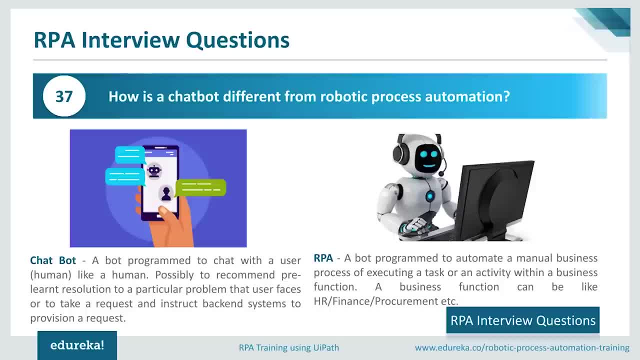 So, basically, a chatbot can be a medium to feed an input into RPA engine, but cannot replicate the features of an RPA engine. All right, So that is the basic difference between the chatbot and an RPA board. All right, Now moving forward. 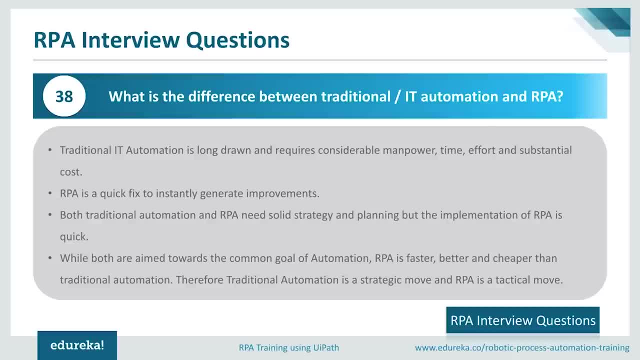 Let's look into another question which is frequently asked by the interviews, that is, the difference between a traditional automation and RPA. So when you talk about traditional automation, traditional automation is long drawn and requires manpower, time, effort and substantial cost, Whereas RPA is a quick fix to instantly generate improvements. both 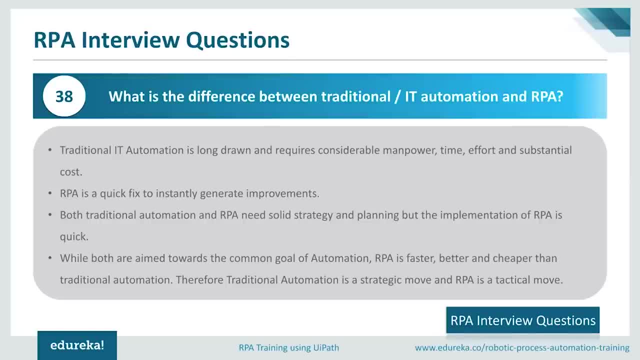 traditional automation and RPA need solid strategy and planning, but the implementation of RPA is really quick. while both are aimed towards the common goal of automation, RPA is faster, better and cheaper than the traditional automation, So you can say that the traditional automation is a strategic move. 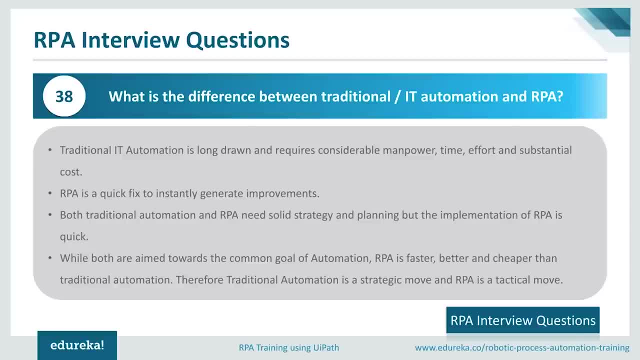 and RPA is a tactical move. in short, If you have the luxury of having time and budget, then you should go for traditional automation. else, If you have business pressures, then you should go for RPA. All right, So that was the basic difference between traditional automation and RPA. 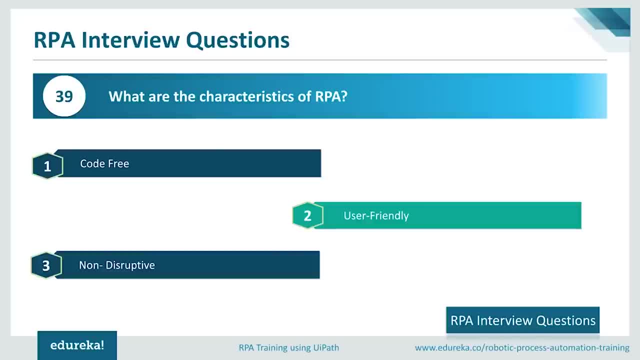 So now let's move on to the next question, That is, what are the characteristics of RPA? as I told you, the benefits before the characteristics of RPA are code-free, user-friendly and non-disruptive right. So when you talk about code-free, RPA does not require any programming skills. 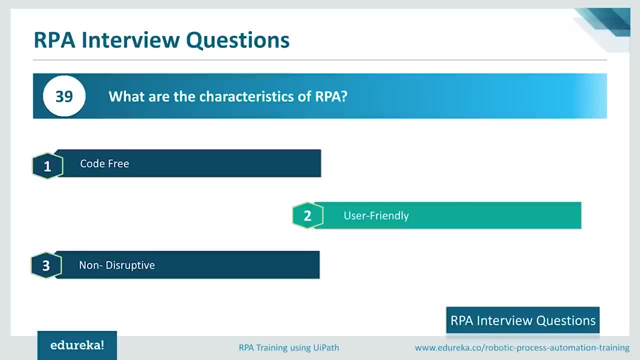 noise without any subject. expertise can be trained to automate the RPA tools instantly. the whole work that you have to do is just to drag and drop the functionalities to represent the steps and processes. So when you talk about user-friendly RPA, adoption comes within the business. 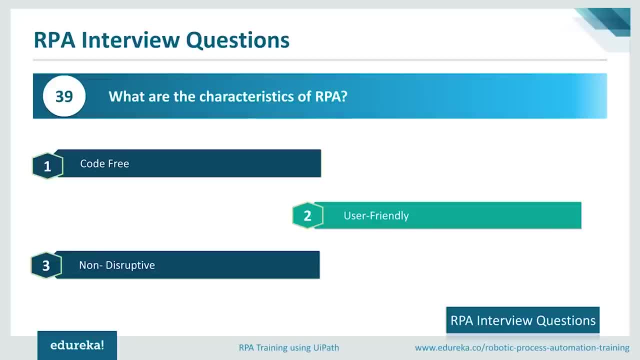 operations rather than IT departments. RPA projects require less IT skills and less investment. Eventually, the automation is lowered at a substantial rate. Finally, the last characteristic of RPA is non-disruptive. RPA avoids complexity and risk. The software robots access end-user systems via control user interface. 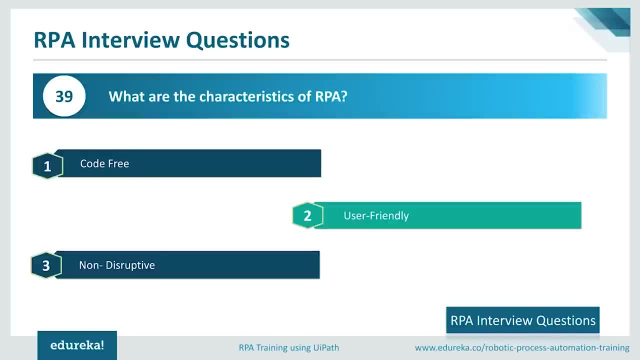 Hence they reduce the necessity of underlying the system programming. So when you're asked about characteristics, the answer is: RPA is code-free, RPA is user-friendly and it is non-disruptive. Now, moving on to the next question: How long does it take to establish the operational agility framework? 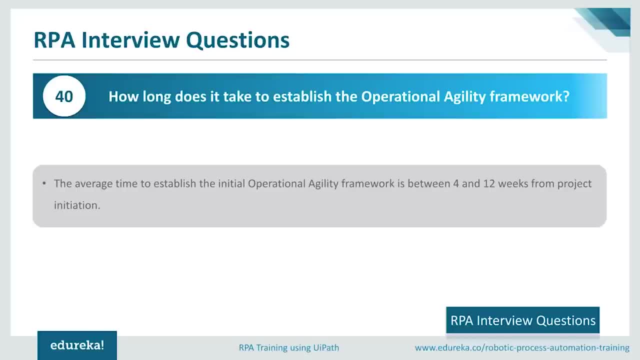 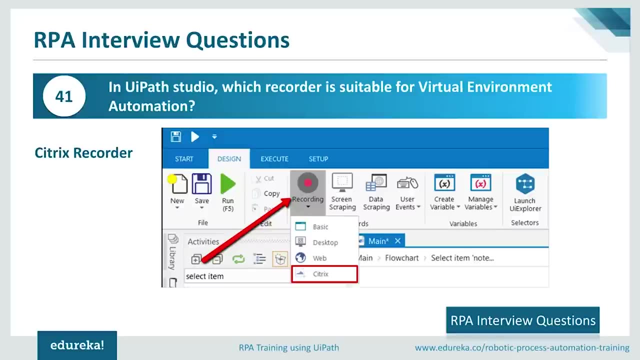 The average time to establish the initial operational agility framework is between 4 and 12 weeks from when the project starts right. So now moving forward. So now next in the list, We have a simple question based on the UiPath tool, which is generally asked by the interviewers, that is, in UiPath studio. 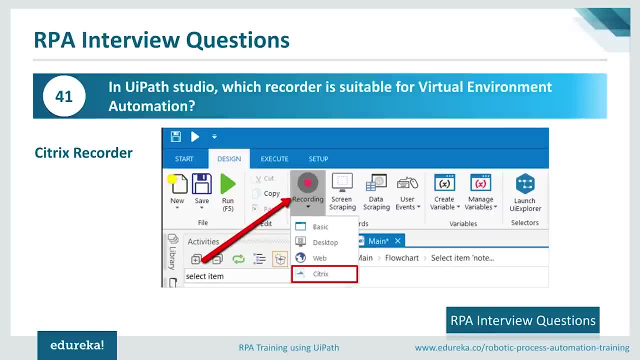 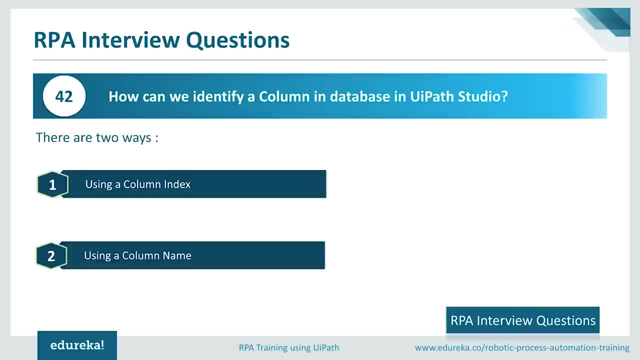 which recorder is suitable for virtual environment automation? The answer to this question is Citrix recorder. So now, moving forward, Let's look into a simple question, That is, how do we identify a column in database with UiPath studio? Well, basically, there are two ways. 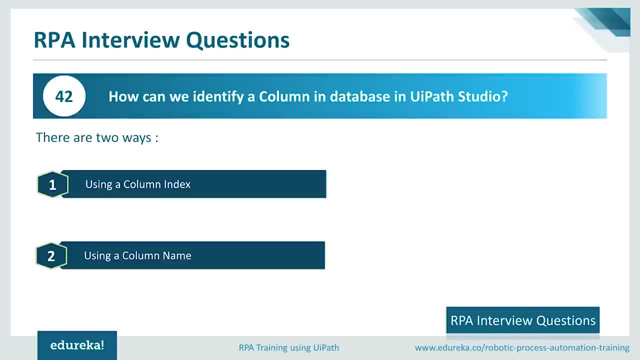 So to identify a column in database you can either use the column index or the column name. Next in the list is a very simple question to test your skills and activities. So the question is which activities can be used to iterate through an array in UiPath studio? 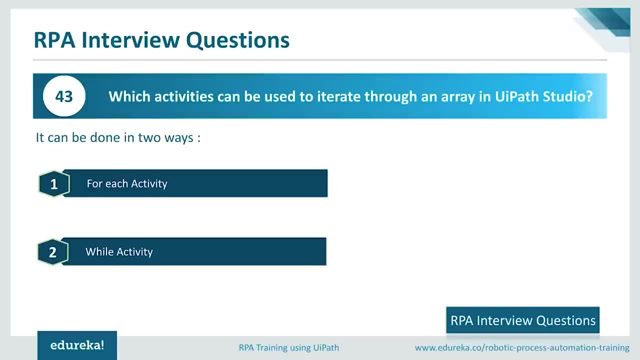 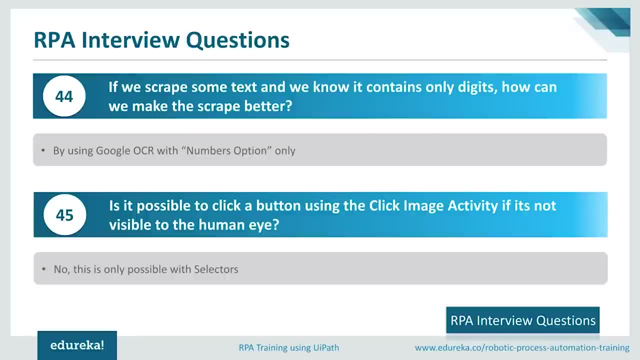 Well, to iterate through an array in UiPath studio, you can either use the for each activity or the while activity. Now let's look into some scenario based questions. That is, if you want to scrape some text and you know it only contains digits. 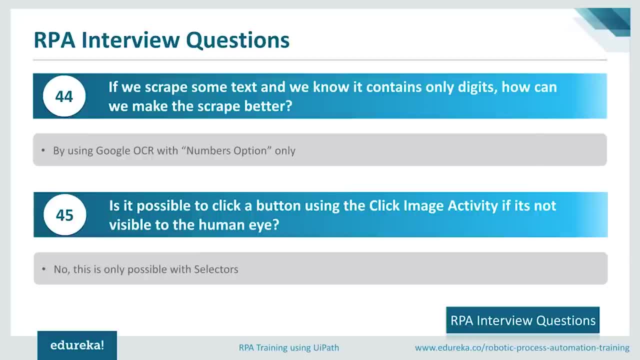 How can you make the scrape look better? So for this kind of scenario, you can use the Google OCR with the numbers option only Now. the next question that you can be asked is: is it possible to click a button using the click image activity if it's not visible to the human eye? 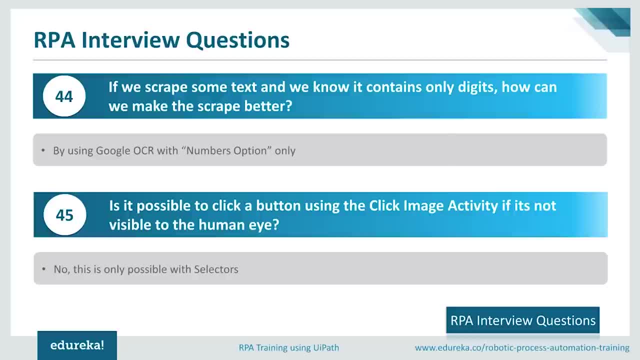 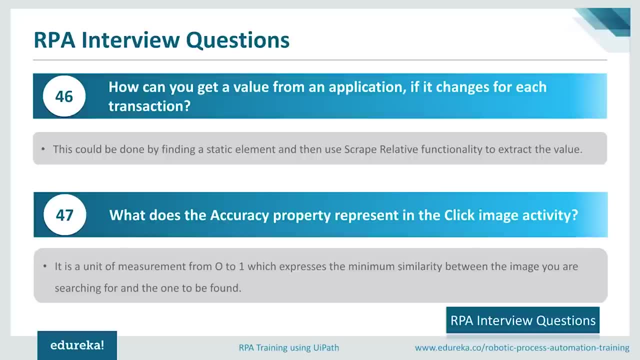 Well, the answer to this question is no. this is only possible with selectors. Now, how can you get a value from an application if it changes for each transaction? This could be done by finding a static element and then use scrape related functionalities to extract the value. 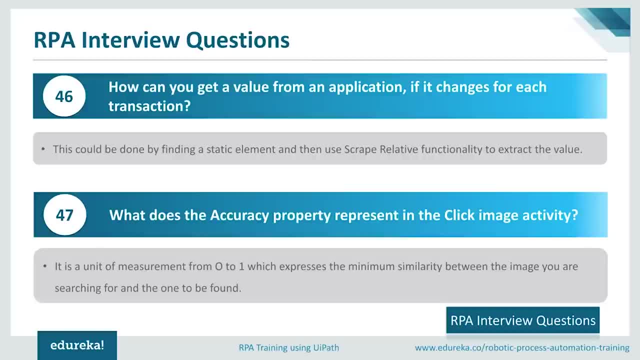 All right. So next in the list is now. if you explore the UiPath studio, you observe an activity known as the click image activity. So what does the accuracy property represent in the click image activity? It is the unit of measurement from 0 to 1. 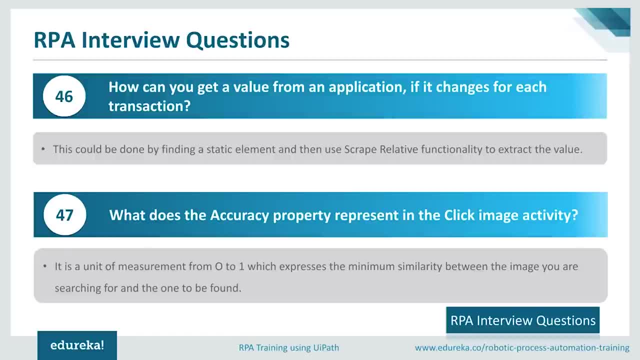 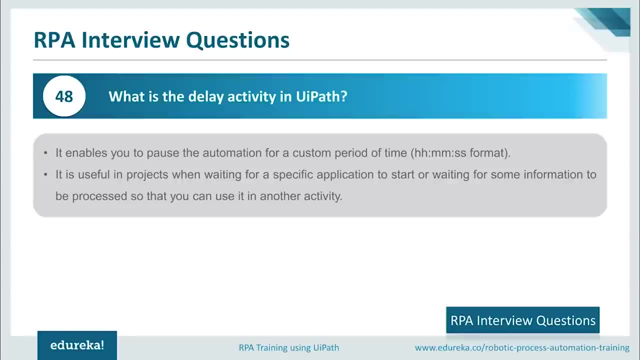 which expresses the minimum similarity between the image you're searching for and the one to be found. All right now. moving forward to the next question, That is, what is delay activity? right So now, when it comes to the delay activity, the delay activity enables you to pause the automation. 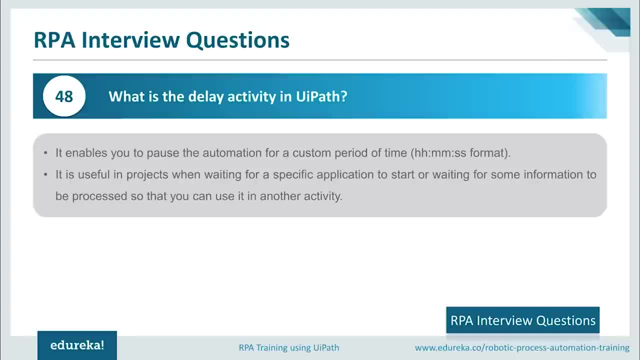 for a custom period of time, right? So, basically, if you're doing web scraping, sometimes the data isn't extracted at that moment. It takes a lot of time because of the net issues, right? So that's when you add delay or sometimes you want the task. 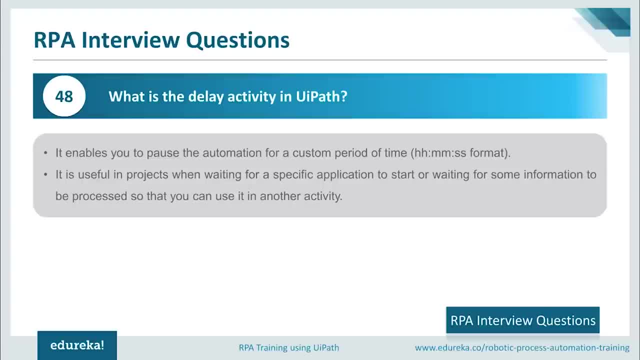 to be performed after certain seconds or certain minutes, So that's when you add delay, right. So this activity proves itself quite useful in projects that require good timing, such as waiting for a specific application to start or waiting for some information to be processed so that you can use it in any other activity. 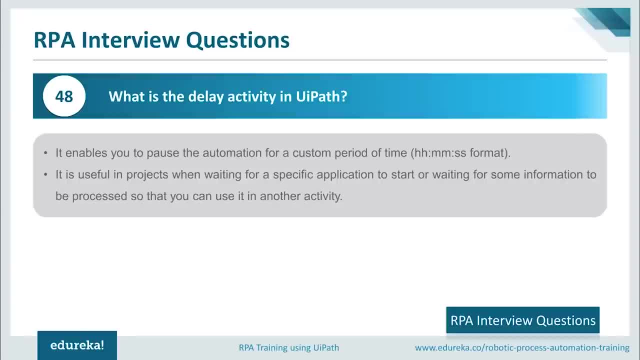 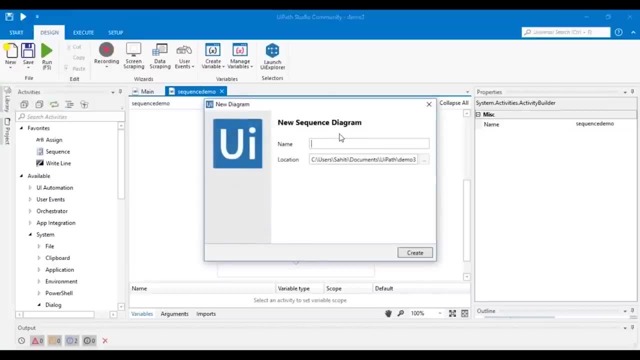 or any such scenario, Just like that. So now let's look into one such scenario. So for that, let me just go back to the UiPath tool, Let me go to the design tab, Let me add a new sequence and let's say I named the sequence. 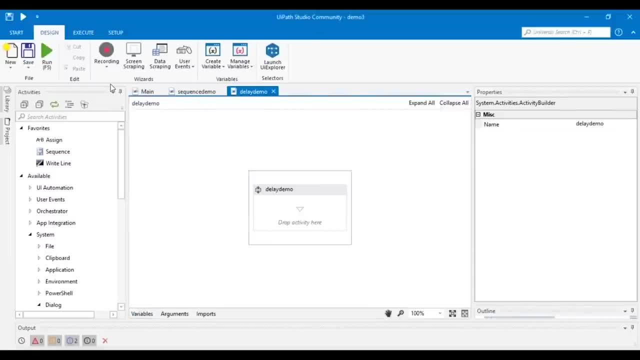 as delay demo. All right in this. let me just create a flow chart. So for that, let me just search in the activity pane for the flow chart. So let me just drag and drop it here. Once it is done, let me just add a right line: activity. 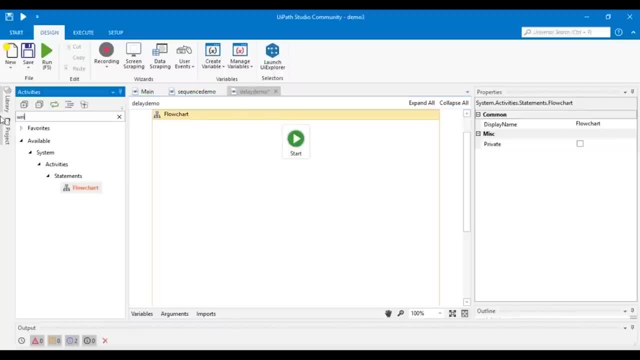 and connect it to the start node right. So let me just search for right line activity And connect it to the start node. After you're done with that, select this activity and in the text bar let's include the start time so that we understand how the delay activity works, right? 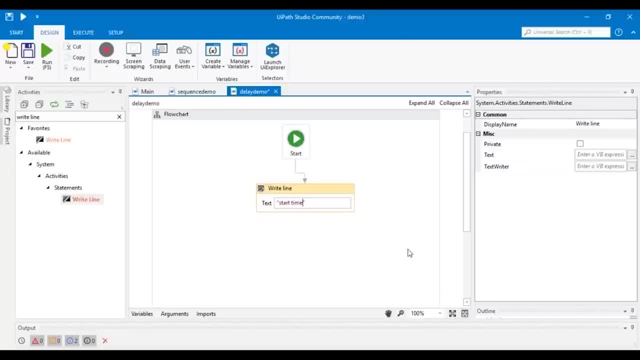 So let's just include a text- start time- and then add the delay activity. So for that let's just search in the activity pane and drag and drop it here. All right, so let me just connect this previous activity To the delay part and in the duration section. 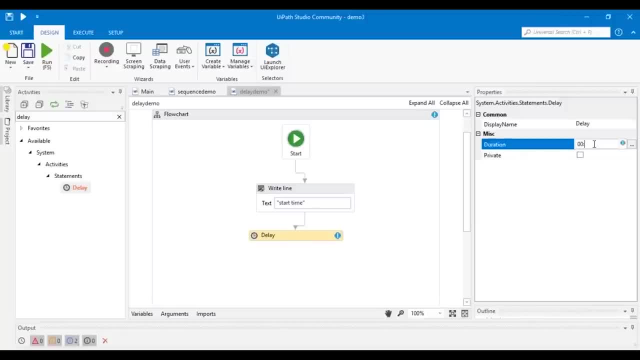 of this activity. let's just say I mentioned the duration for 10 seconds, right, So I'll mention it in this format, and by this what we're trying to show is that there would be a 10 second delay. that is going to be between: 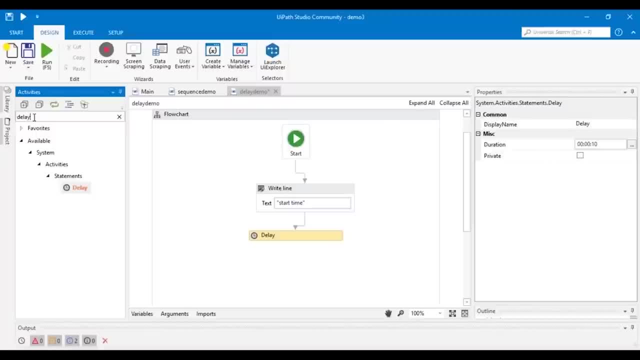 the two locked messages, all right. So now let's add the second locked message. So for that let me just search for the right line activity again and then drag and drop it here. All right, so let's just connect this activity and then in the text let's add this message: 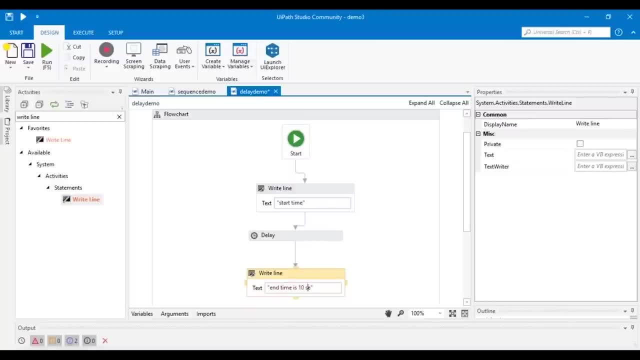 End time is after 10 seconds delay. So in the text field let's just add a message as end time is after 10 seconds delay. All right, now let's just run this program and let's see the output panel, right? 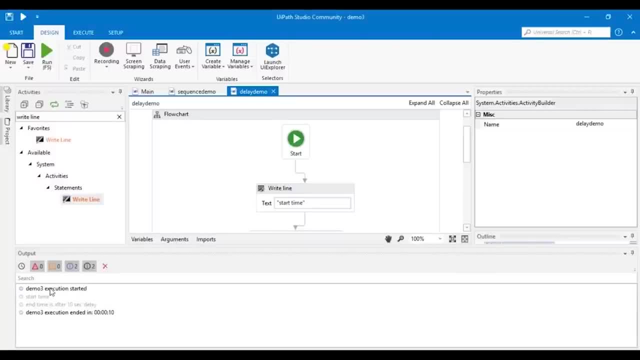 So we see that the demo has started as 22 seconds and once it has started, the end time is after 10 seconds delay, right, So just add 10 more seconds. That means it should end around 10 seconds. It should end around 33 seconds. 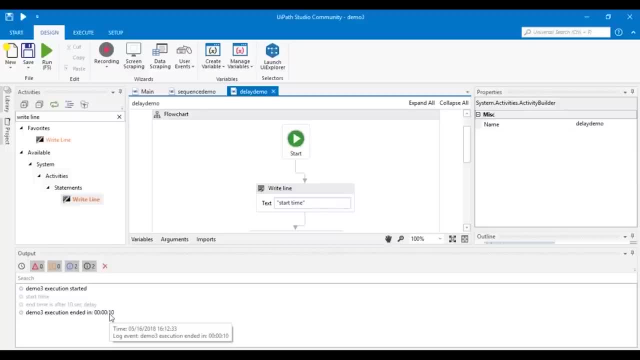 So let's just see if it has ended. Yes, it has right. So that's how you can use the delay activity, which causes the task to be delayed by few seconds or few minutes, or how much ever time you want right Now, moving on to the next question. 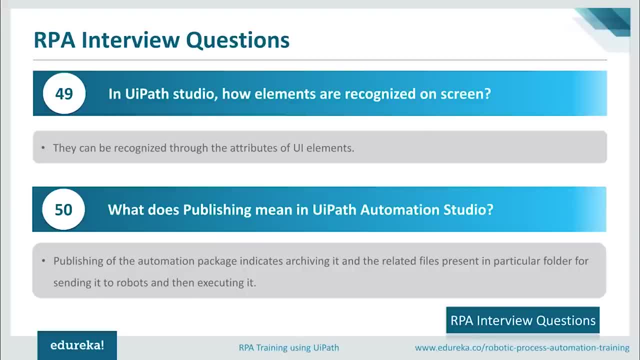 We have the question as: how are elements recognized on the screen using UiPath Studio? Well, the answer to this question is that they can be recognized through the attributes of UiElements, right? So whenever you're asked: how are elements recognized on the screen? 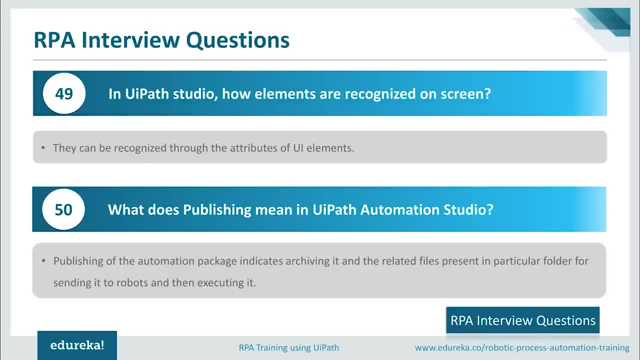 The answer is: they can be recognized through the attributes of UiElements. And finally, the last question for the session, that is, what does publishing mean in UiPath Automation Studio? So publishing of the automation package indicates archiving it and the related files present in the particular folder. 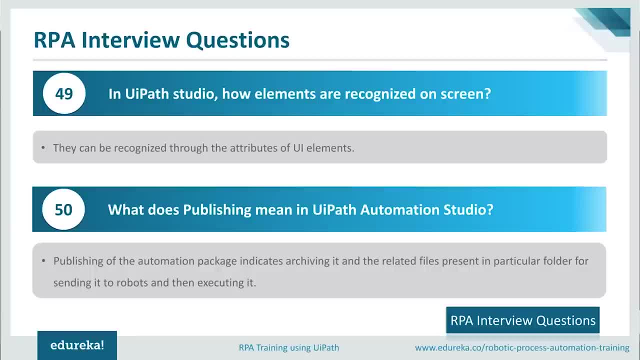 for sending it to robots and then executing it. So you want to perform a task each day at some time, right? So you just have to create your project for it, and then you have to just publish the project and then connect it with the orchestrator. 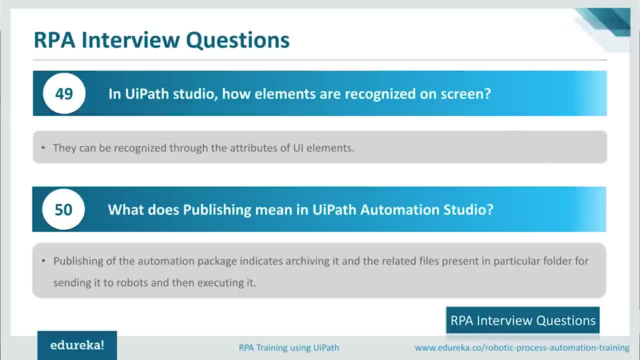 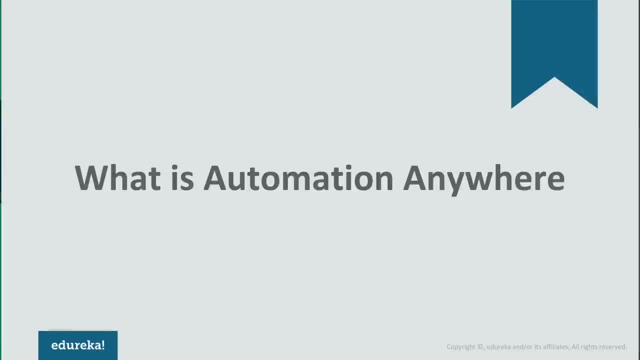 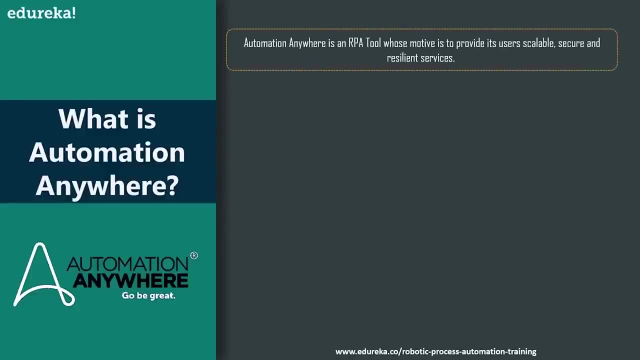 So every day, at the scheduled time, a robot would perform that task. Let's know what exactly Automation Anywhere is. So Automation Anywhere is basically an RPA tool whose motive is to provide its users with scalable, secure and resilient services. This tool offers a 30-day free trial. 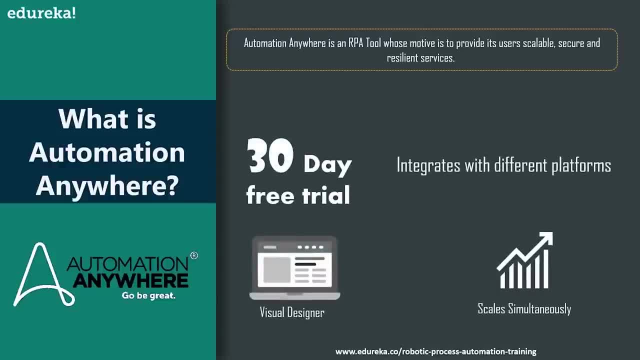 to let you explore the tool first and automate tasks, and then provides you with an enterprise service. Automation Anywhere also offers better performance, as it has the ability to integrate to different platforms and also scale simultaneously. This tool is meant to be used in the enterprise level. 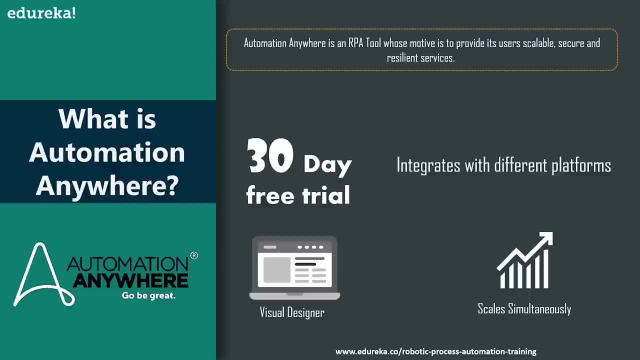 and is mainly designed for solving complexity issues. right? So if I have to just summarize Automation Anywhere for you, it's just an RPA tool which provides the users with scalable, secure and resilient services. It offers a 30-day free trial. 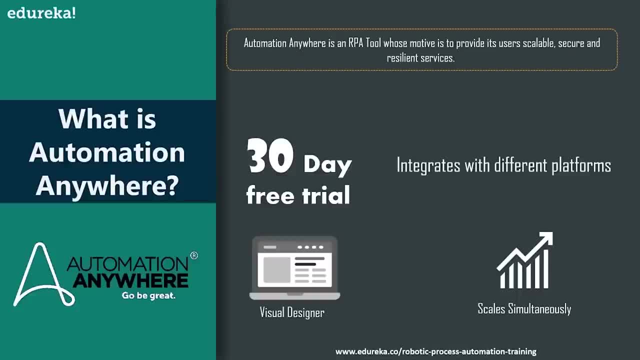 So if you just want to automate tasks, or if you're new to RPA and if you want to learn how to automate tasks, then you can definitely go for this tool, and this tool also integrates with different platforms, right? So, now that I've told you a little bit, 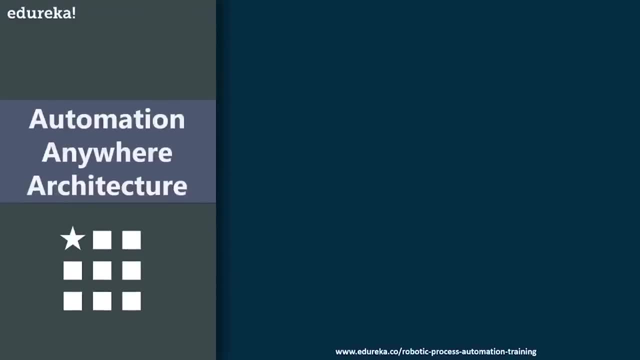 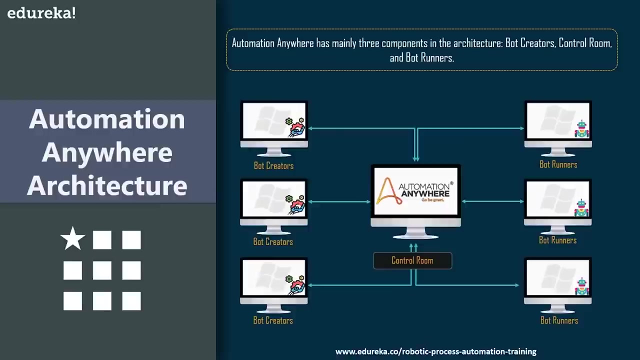 about Automation Anywhere. let me just quickly tell you how its architecture is. Automation Anywhere architecture basically follows a distributed architecture To this architecture. it mainly makes sure that you know centralized management is accomplished via Automation Anywhere's control room. So, as you can see on the screen over here, 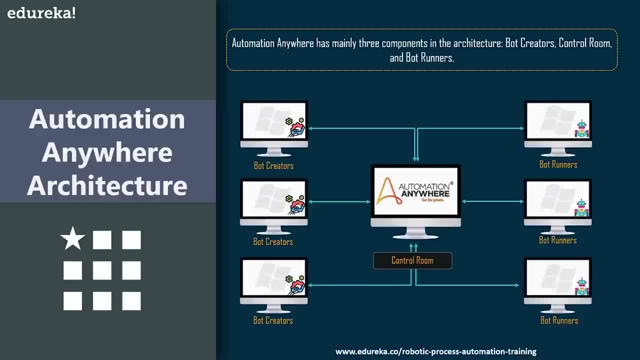 there are mainly three components of this architecture, That is, the bot creators, the control room and the bot runners, right? So let's just discuss about each of them one by one. All right, now talking about bot creators, as the name suggests, 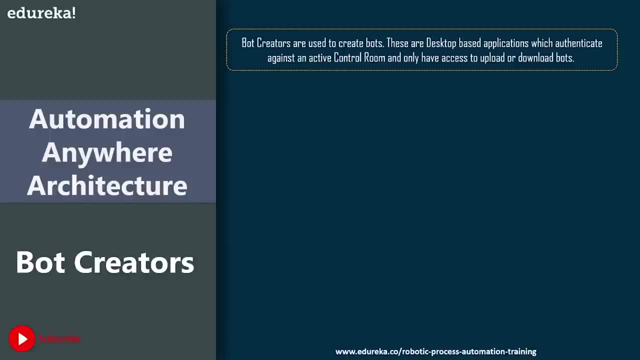 bot creators are basically used to create bots. These are basically desktop-based applications which authenticate against an active control room and only have the access to upload or download the bots. On configuring these bots for the control room, multiple developers can create individual tasks or bots and execute all of them at once. 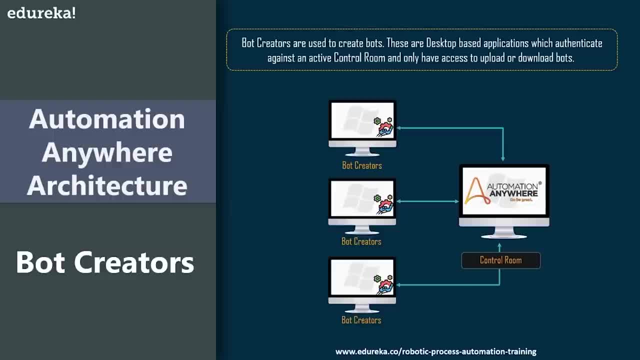 So basically, if you have to just understand what creators and what creators are basically used to create bots, and they are used to just upload and download the bots to the active control room, right? So basically, if you just look into the Automation, Anywhere's architecture. 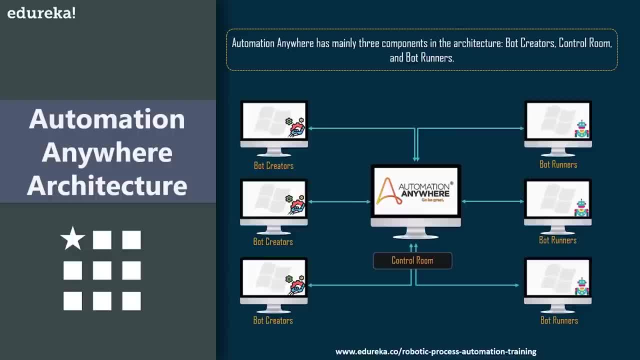 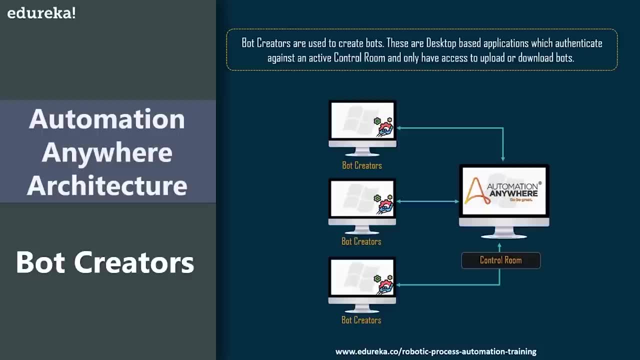 you'll clearly understand that. you know it completely revolves around the control room, right? So basically, the main component of this architecture is control room, and bot creators and bot runners are just subordinate components which help the architecture to run in a distributed manner, right? 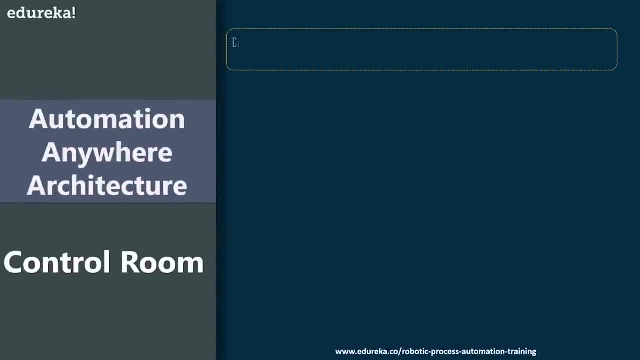 So now let's understand how exactly control room works. Control room is basically, as I said, the most important component of the architecture. It's a web server that basically provides the bots created by the bot creators. Now, as Automation Anywhere focuses on the centralized management, 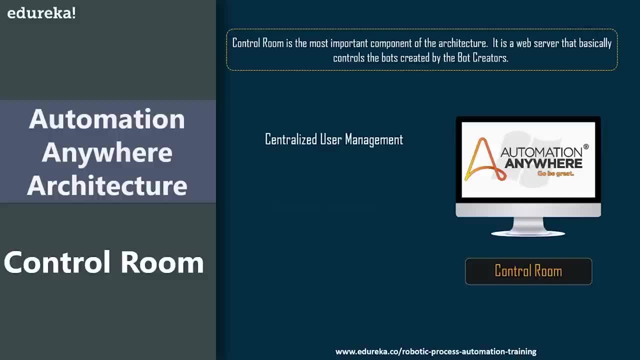 the control room offers features such as centralized user management, automation, deployment, source control, and also provides a dashboard. So don't worry, I'll show you what I'm talking about. We're going to install Automation Anywhere and then we're going to start working on it. 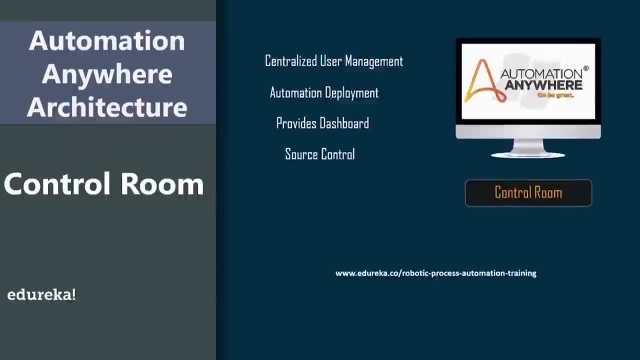 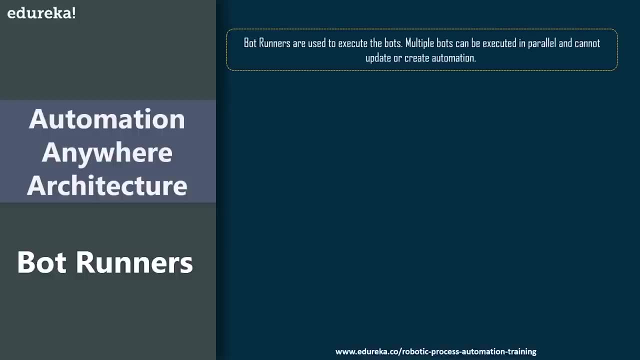 So don't worry about that, I'll show you how that works. So now let's move on to the third component of this architecture, that is, the bot runners. Bot runners are basically used to execute the bots, So multiple boards can be executed in parallel. 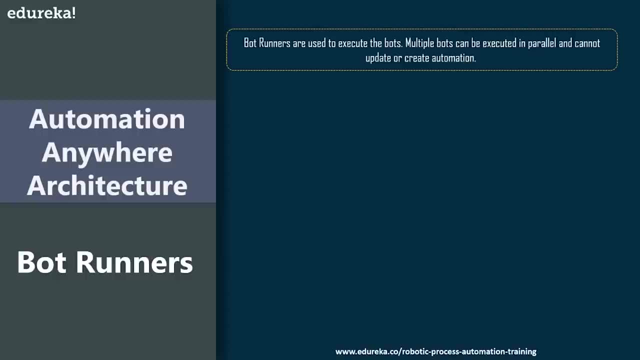 and they cannot be updated or they cannot create any automation right. So there are basically runtime clients which are installed on the Windows machines and can report back the execution log status to the control room. So if you just summarize all these three components together, 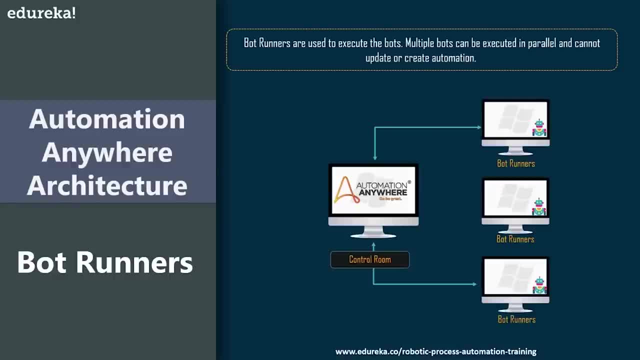 then once a developer creates a bot and updates onto the control room, the control room can hear by, schedule and execute these boards on the bot runners based on the requirements or are the priority of the enterprise, right? So I hope I'm clear and I hope the architecture is clear to guys. 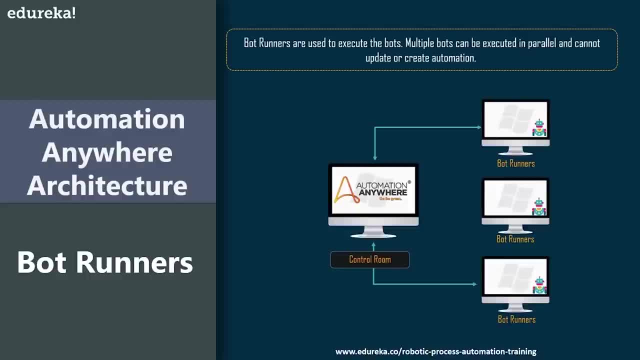 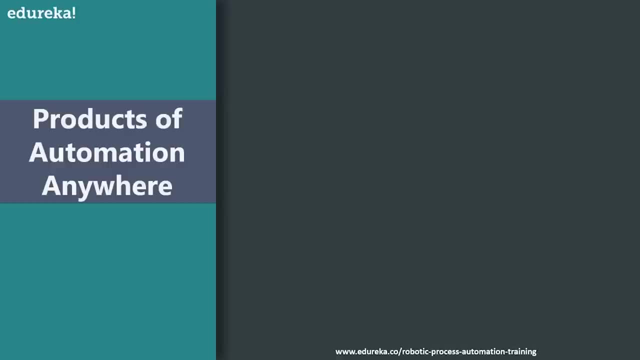 So, now that you know the architecture of Automation Anywhere, let's get into the products of Automation Anywhere. So, apart from the three products that I've told you, that is, the bot creators, the bot runners and the control room, There are mainly three more products. 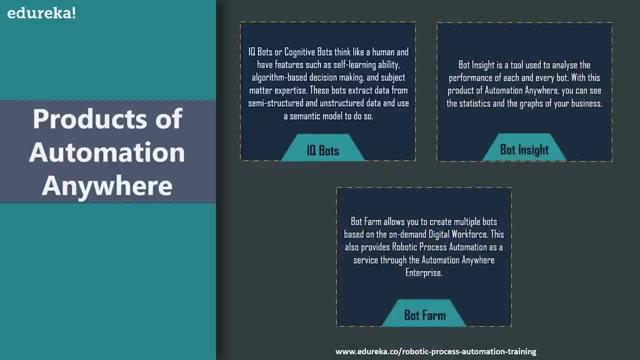 that is, the IQ bots, bot insights and the bot farm, right. So the IQ bots are basically cognitive bots that think like a human and have features such as, you know, self-learning abilities, algorithm-based decision makings and subject matter expertise. These bots extract data from a semi-structured 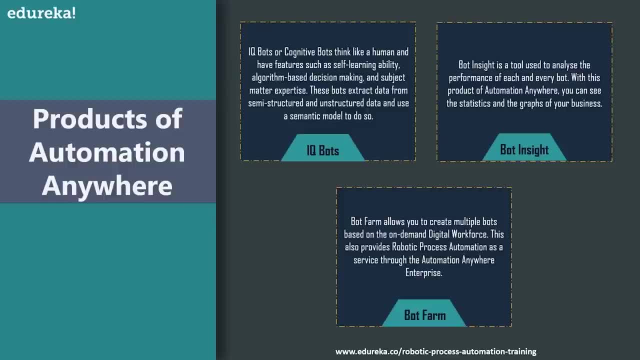 and unstructured data and use a semantic model to do so. Coming to bot insight, the bot insight is basically a tool used to analyze the performance of each and every bot. So with this product of Automation, Anywhere you can use the statistics and the graphs for your business. 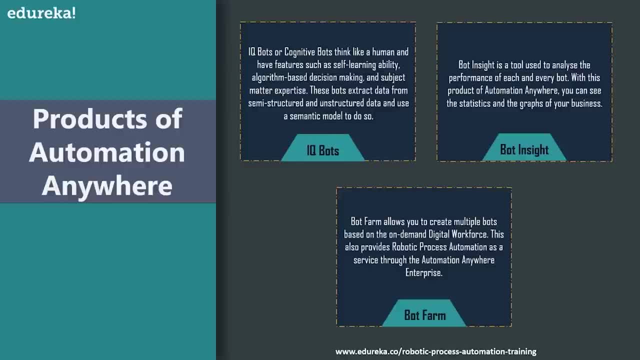 and coming to the final product of Automation Anywhere, that is, the bot farm. The bot farm allows you to create multiple bots based on the on-demand digital workforce, So this also provides robotic process automation as a service to the Automation Anywhere Enterprise. 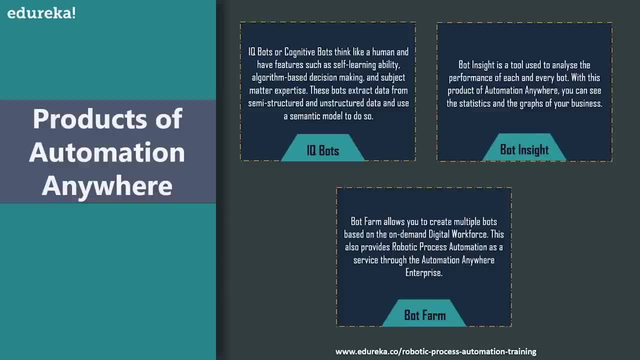 right? So, guys, that was all about Automation Anywhere. I hope you understood what is Automation Anywhere, What are the products of Automation Anywhere and what is the architecture of Automation Anywhere and how the components of the architecture work together, right? 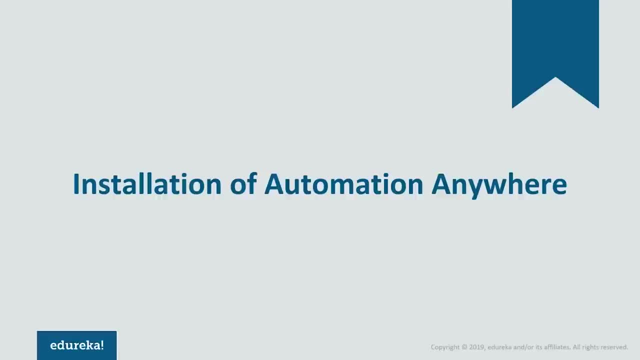 So now let's just move forward and let's see how to install this tool. So the installation of this tool basically implies the installation of two main components, That is, the IQ boards and the RPA Enterprise. So with the IQ boards you can basically create a learning instance. 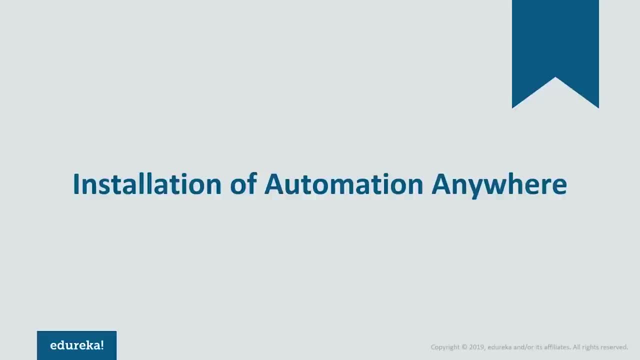 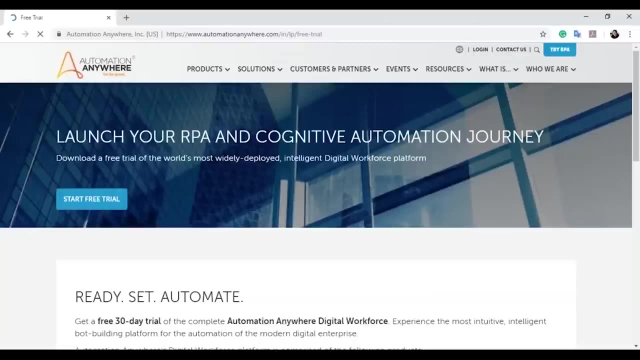 and the RPA Enterprise is like workbench or a dashboard which lets you automate tasks, right? So let's just start installing Automation Anywhere. All right? So to install Automation Anywhere, you basically have to go to the official website of Automation Anywhere. 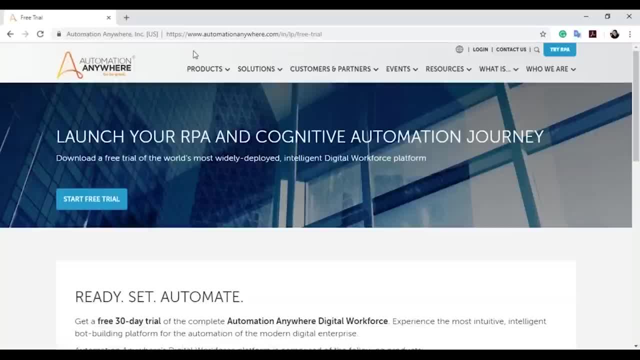 and then you have to just go to this link that is automationanywherecom: slash in, slash LP, slash free trial, And then you'll be redirected to this particular page, right? So, as I said, it offers a 30-day free trial. 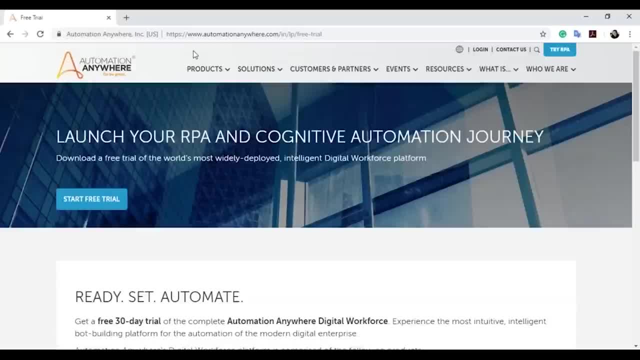 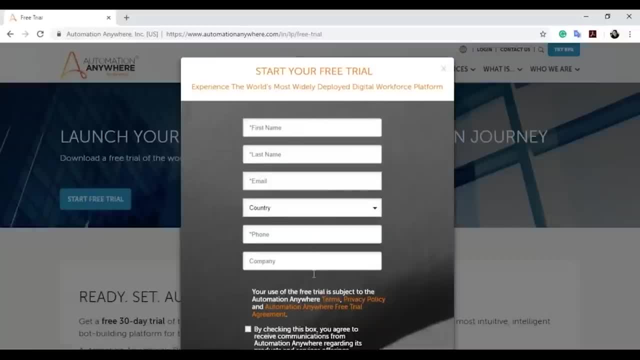 I'm just going to show you how you can start using the free trial. So if you just want to start using the free trial, what you simply have to do is you have to just click on the start free trial option, and then you have to mention all your details, right? 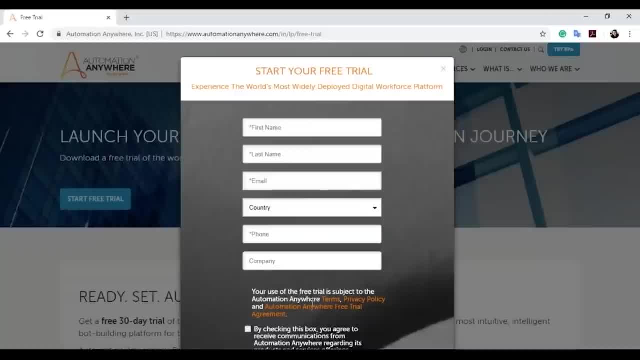 So since I've already installed Automation Anywhere in my system, I'm not going to do it. I'm not going to mention all the details and click on the button, But let me just tell you that once you mention all these details, that is your first name. 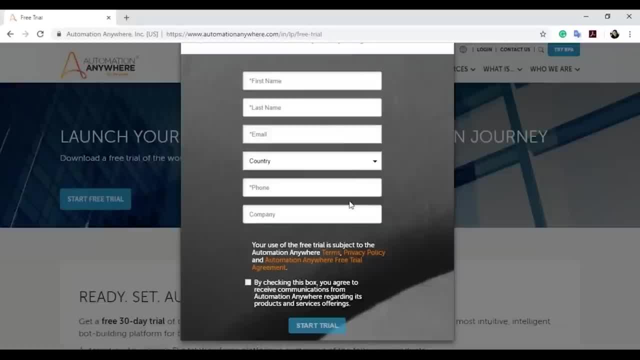 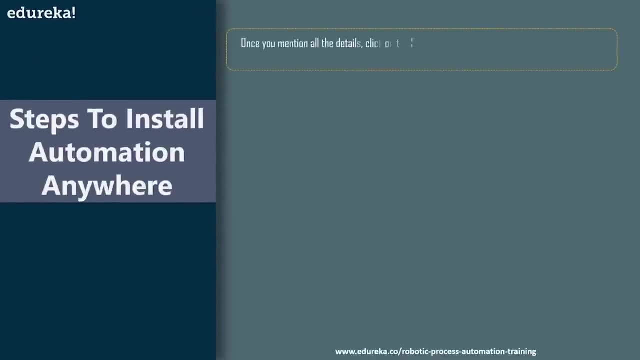 last name, email ID, country number and the company that you're working in. And then, when you finally check on this box and click on the start trial option, what will happen is you'll be redirected to a page you know, which will show you this particular output. 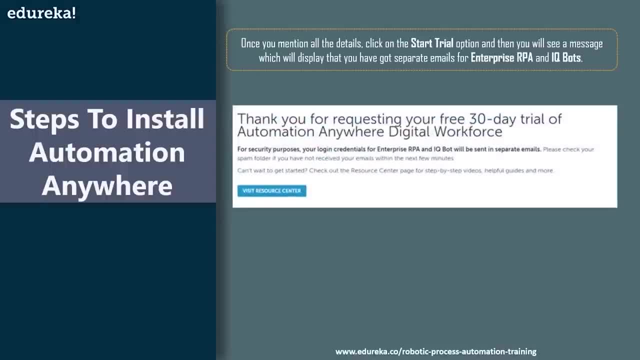 which clearly says that you've requested for a 30-day free trial version of Automation Anywhere, right. So for security purposes, what Automation Anywhere's franchise does is that you know it sends your login credentials for Enterprise RPA and IQ boards. 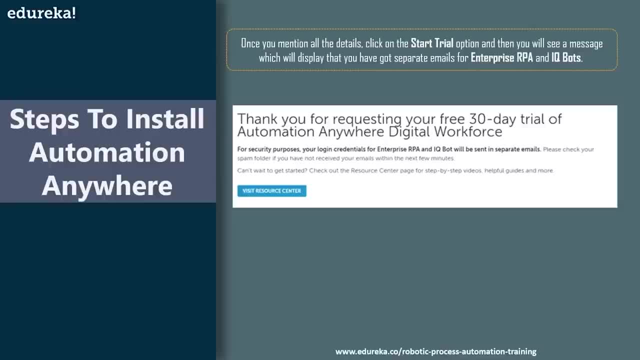 as separate emails, right? So basically, you would see that you know you would get two separate emails for downloading IQ boards and Enterprise RPA. So let me just open those emails and show you one by one. So I'll just open those emails. 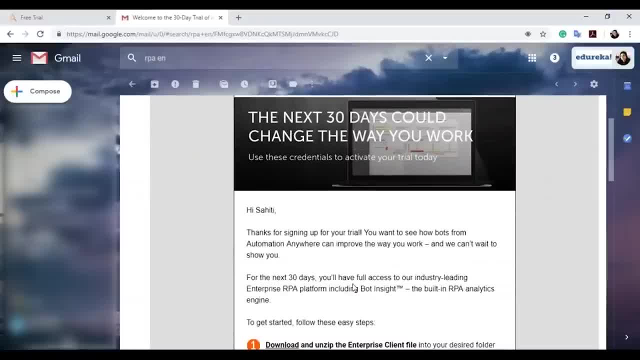 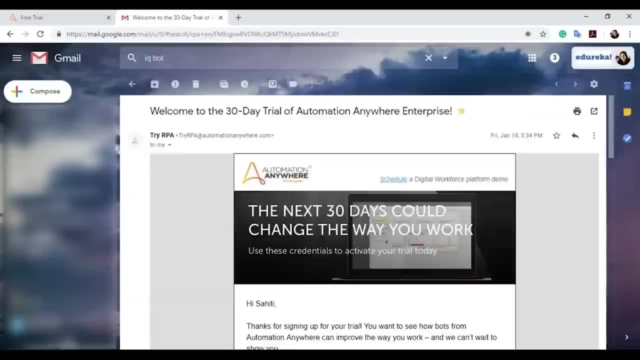 So, as you can see, I've got this email to just log into my control room. that is basically the RPA Enterprise, and similarly you would get a mail for the IQ boards. So let me just search for IQ boards and then you would see all the steps. 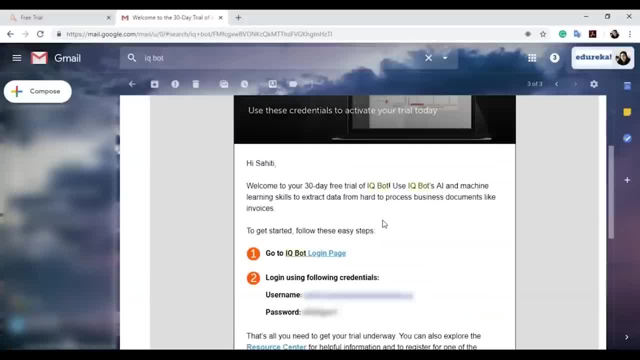 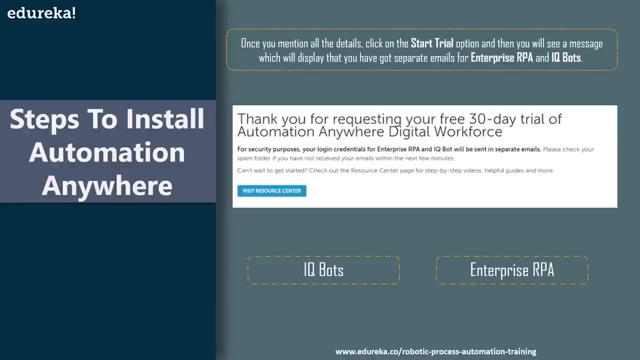 regarding how to install IQ boards right. So I'm going to show you how you can do that. So first I'm going to log into the IQ boards and then I'm going to log into the control room. that is basically the Enterprise RPA, right. 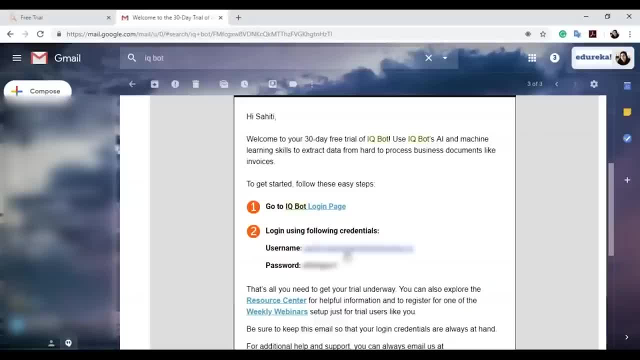 So let me just show you how you can log into the IQ boards. To log into IQ boards- as you can see in the mail it's very clear that you know- you just have to go to the IQ board login page. So I'll just open that. 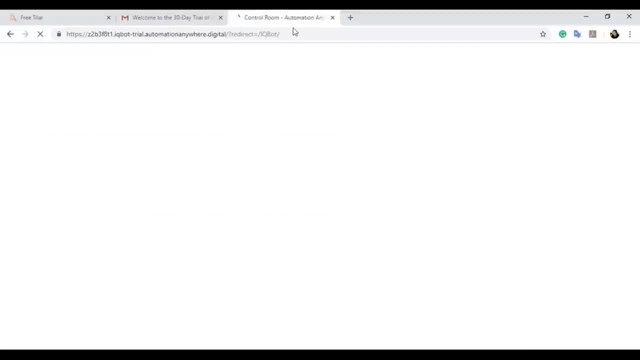 and then you'll have to mention the username and the password, right? So whatever username and the password you get in your email, that's what you have to mention. So I'll just open this page for logging into IQ board. Let's just wait for it to open. 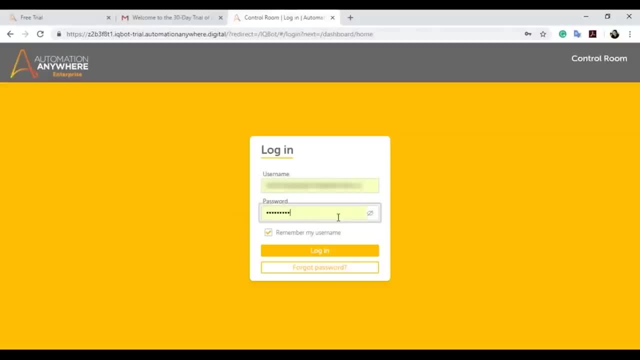 So, as you can see, we have been redirected to this particular page. that is basically the IQ board login page. So you just have to mention the credentials that you've got in your mail for logging into IQ board. Remember your credentials for RPA Enterprise. 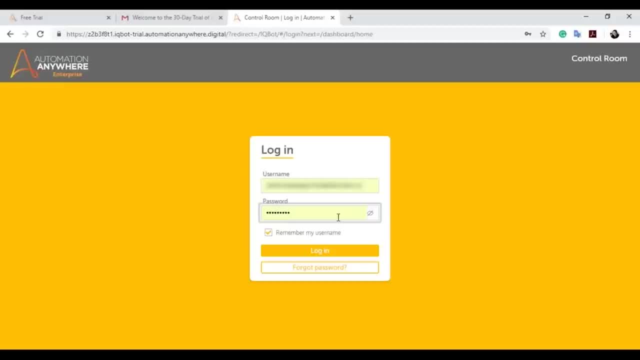 and IQ board are not the same. You have to make sure what you're logging into right. So if you're logging into IQ board, please make sure that you know you're using the credentials for the IQ board. Else, if you're logging into RPA Enterprise, 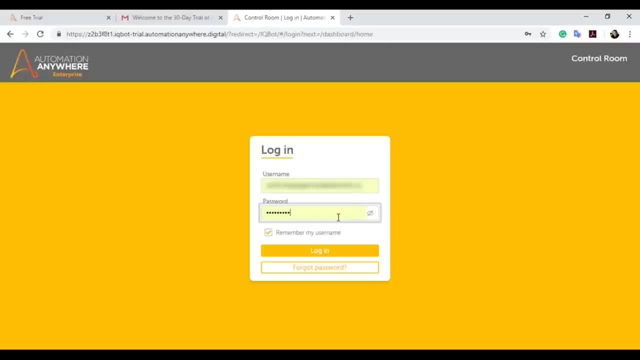 please make sure that you know you'll use the credentials for RPA Enterprise, right? So I've just mentioned the credentials for my IQ board. So once you mention the credentials for IQ board, you just have to click on this login button. 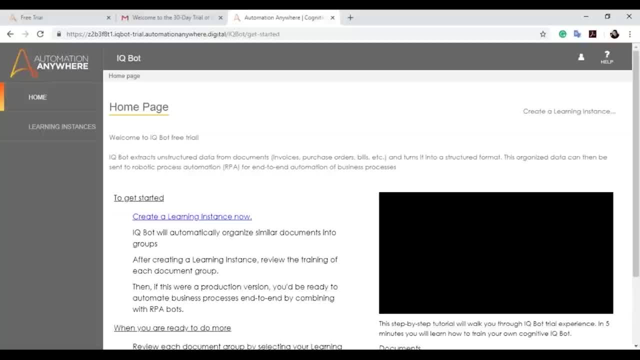 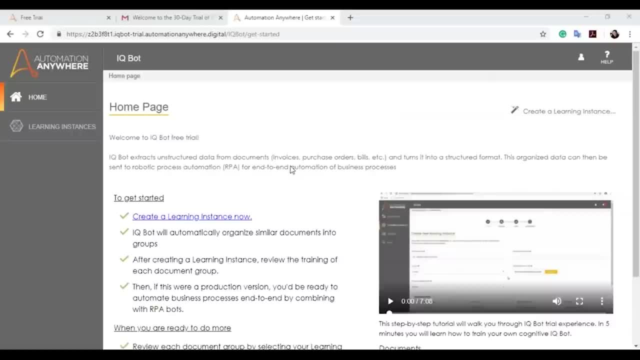 and then you'll be redirected to the home page of the IQ board, Right? So, as you can see, this is basically the home page of the IQ board. So now you can get started by, you know, creating a learning instance And then, if you want, to just automatically organize. 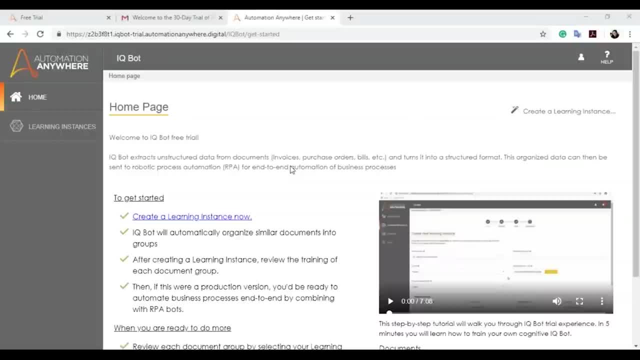 similar documents into groups. you can just get started with all these steps, So don't worry, you can explore this. Now, moving on to the installation of RPA Enterprise, As I said, you would have got a mail for RPA Enterprise. 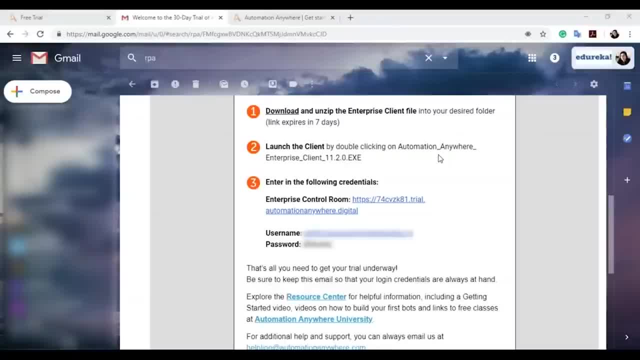 So when you see this mail of you know RPA Enterprise, the first step that you have to do is you have to download and unsub the Enterprise client file into your desired folder. So let's say: remember, guys, this particular link expires in seven days. 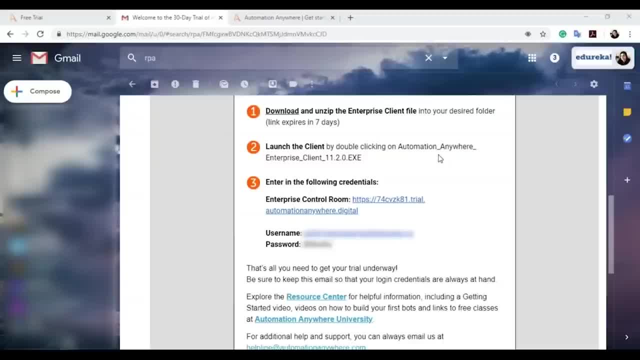 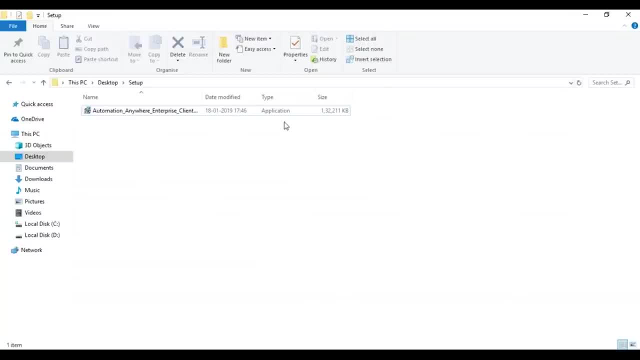 So make sure that you know you've downloaded this file within seven days, Right? So let me just open the folder where I've just downloaded this particular file. So, guys, this is basically the file that you know that you have to download and unsub. 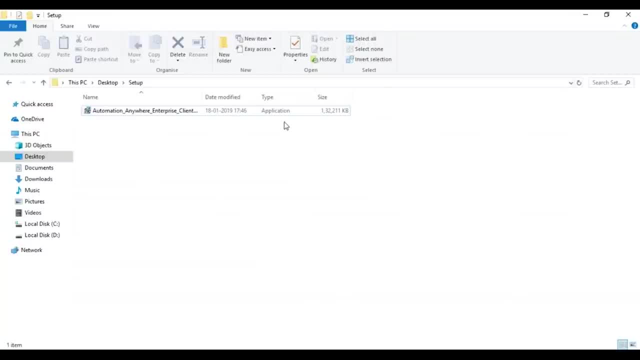 So that's what I've already done. So now, once you've just downloaded and unsubbed the file, what you simply have to do is you have to just double click on this file, mention the password if it's required, And then you'll see that. 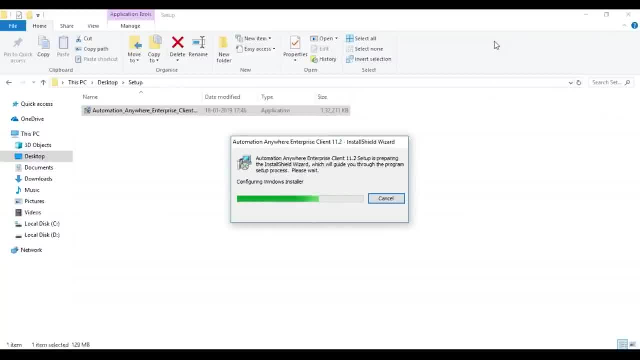 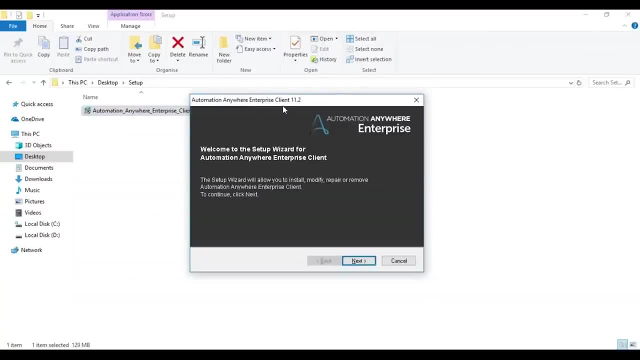 you know your setup is getting prepared to install, Right, So just wait for it to happen. All right. So once you double click on this particular file, that is Automation Anywhere Enterprise Client, you would see that you know your wizard is ready to get installed. 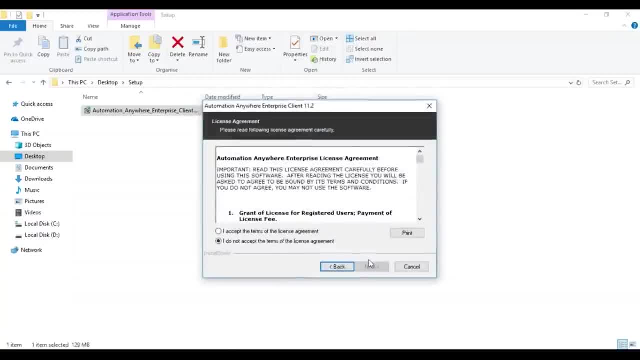 Right, So what you simply have to do is you have to click on next, Then you just have to accept the license, and if you want, you can just go through it and then you can click on next. Once you click on next, you can just mention the destination folder. 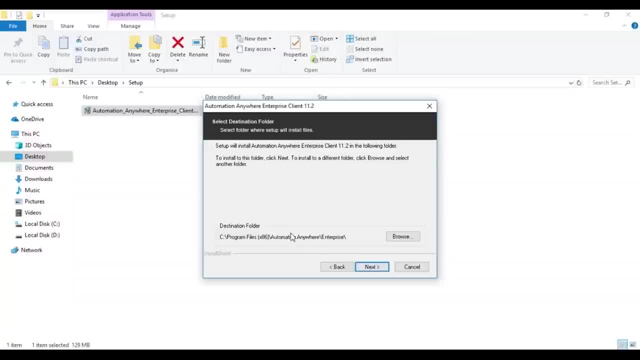 That is which folder that you want to make sure that all the files related to Automation Anywhere are stored. So that's C and program files for me. So I'll just keep that way and then I'll click on next. Once you click on next. 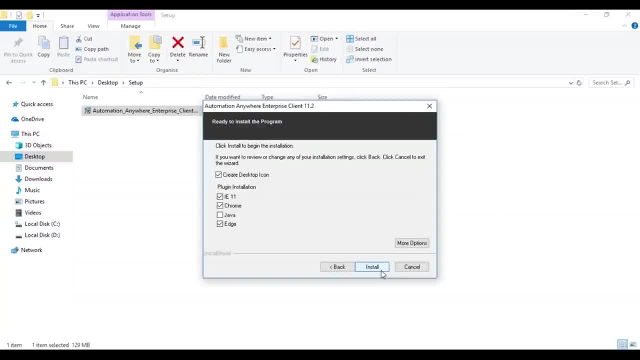 you'll see that. you know, you can just review your installation setting. So I want the desktop icon to be created and then I want the plug-in installations to be done. So I'll just click on install after this and you can see that. 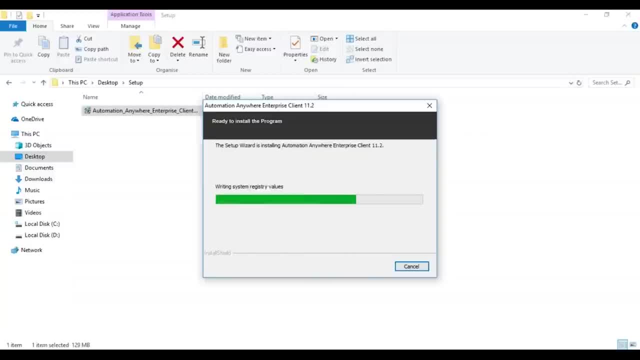 you know my Automation: Anywhere setup is getting installed Right, So let's just wait for that to happen. All right, Now, once your wizard is completely installed, you would just see this dialog box. that you know. setup wizard is complete. 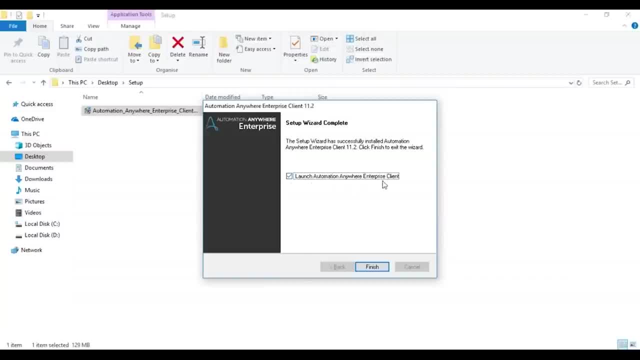 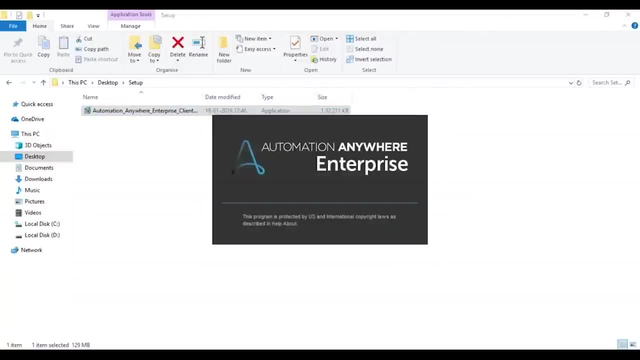 Right. So if you just check in this box of launch Automation Anywhere Enterprise Client, once it is done you just click on finish and you'll see that you know Automation Anywhere Enterprise Client will be launched. So let's just wait for that to happen. 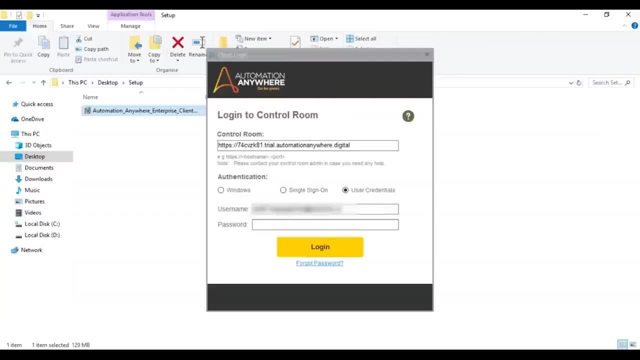 Now, once you see that you know Enterprise Client has been launched, you first get this option of client login. So this is where you have to log into your control room by using the username and the password that you've got in your mail. 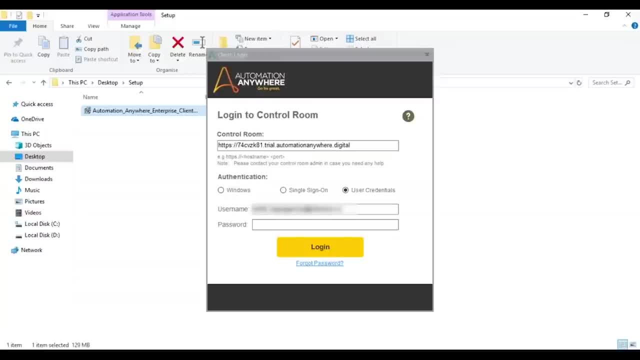 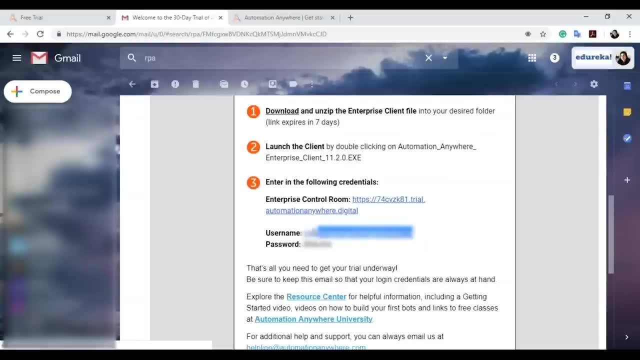 Right, So I'll just mention the username and the password and you have to mention the control rooms- login. So what I'll do is I'll just copy from here and then I'll paste it over here Again: copy this my username and I'll paste this. 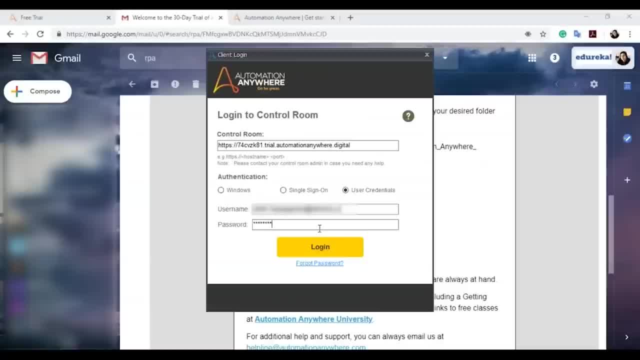 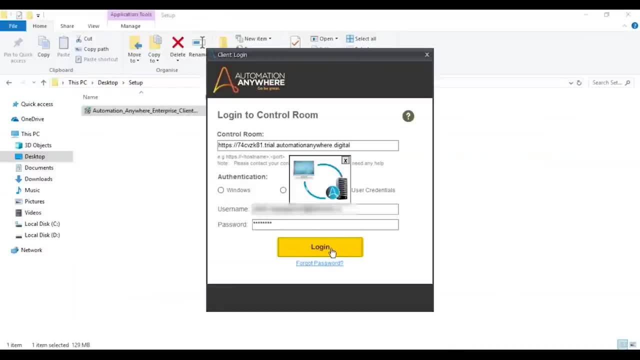 I'll copy this and I'll paste this Right So you can see that. you know I've mentioned my control rooms URL, the username and the password, So I'll just click on login after that, So you'll see that. 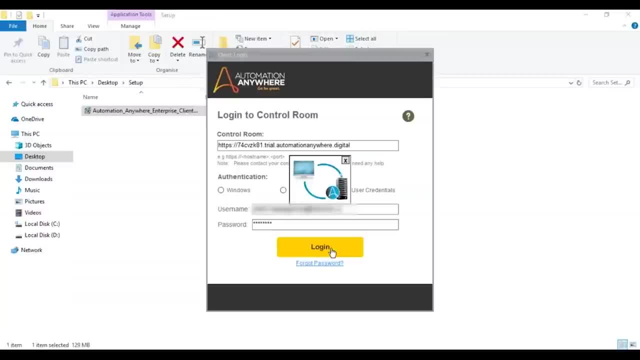 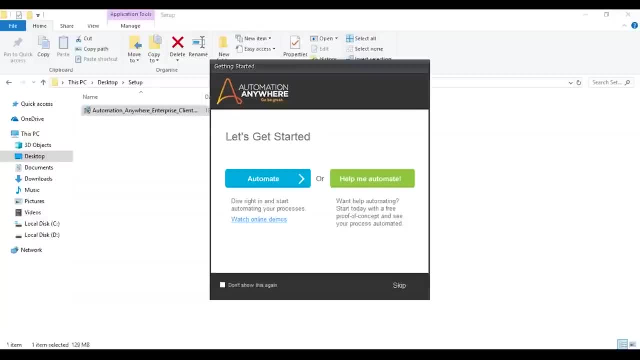 you know you'll be logged into the Enterprise Client, Right? So let's just wait for that to happen. Now, once you log into your Enterprise Client, you'll see this dialog box. you know where you have to choose: automate or help to automate. 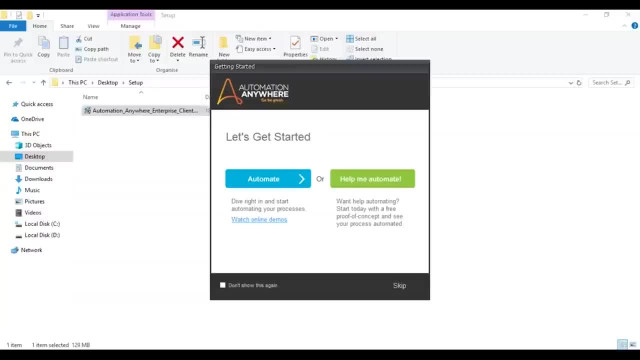 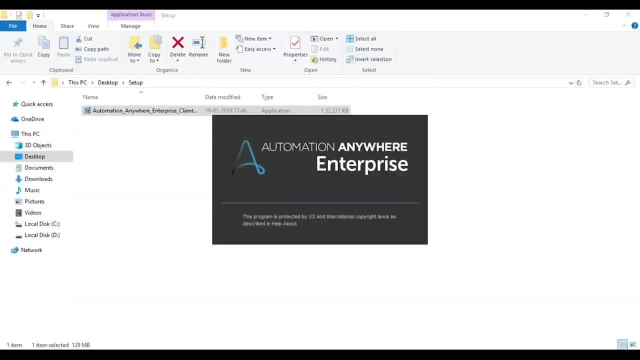 Right, So you can choose either one of them or you can just simply skip this step. So I'll just simply choose, skip. And now, once you choose, skip, you'll see that you know you'll be redirected to the Automation Anywhere dashboard. 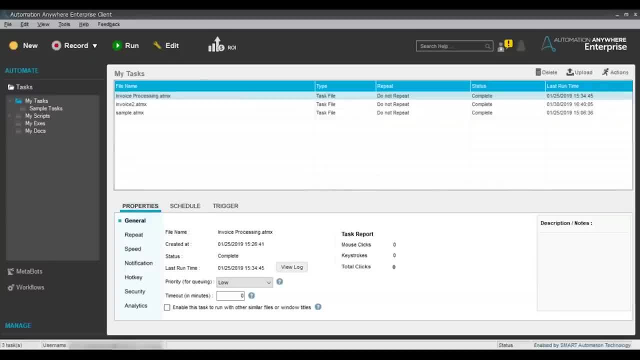 Right, So let's just wait for that to happen. All right, So, as you can see, the Automation Anywhere dashboard has opened up, Right? So, guys, this is basically how the Automation Anywhere dashboard looks like, So don't worry. 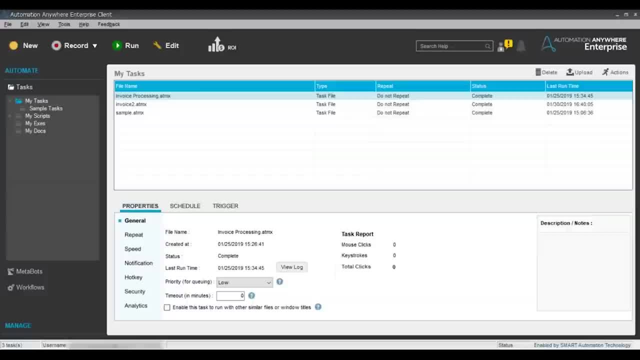 I'll show you how each of these functionalities of the dashboard work when we do the hands-on part. So I hope that you know. you understood how to install Automation Anywhere, Guys. the steps are really simple and clear. You just have to go to the Automation Anywhere's official website. 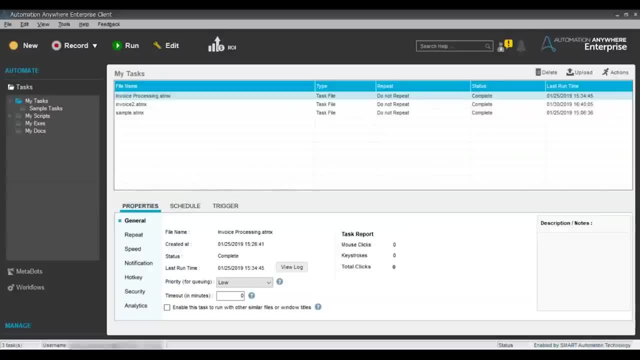 You have to mention your details. You have to just click on start trial option and then you'll receive mails for configuring IQ boards and RPA Enterprise. So just configure your IQ board using the credentials that you've got for IQ boards And after that, 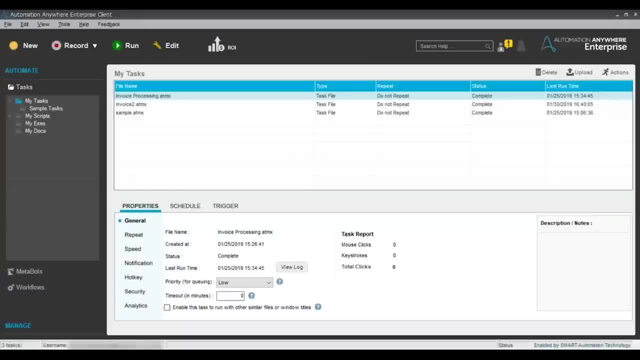 you just download and unzip the Enterprise Client file and then you again just accept the license agreement and just keep clicking on next review the installation and then you'll see that you know Automation: Anywhere Enterprise Client is downloaded right. So I hope that. 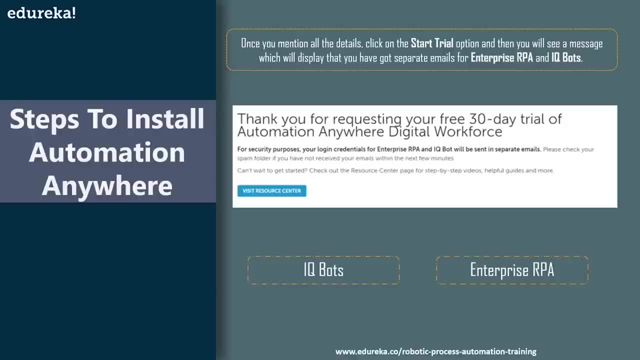 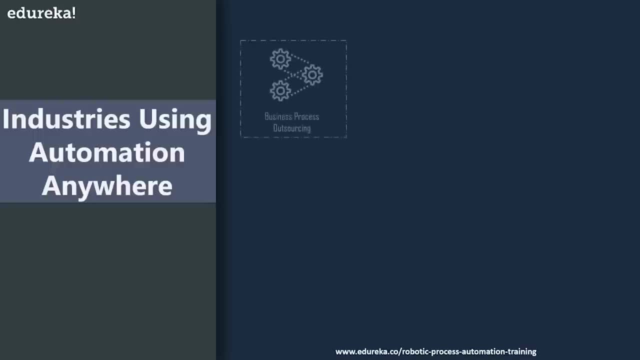 you know, you've understood how to install Automation Anywhere. Now let's look into the next topic, that is, top industry is using Automation Anywhere, right? So the top industry is using Automation Anywhere at the business process: outsourcing, telecom industry. 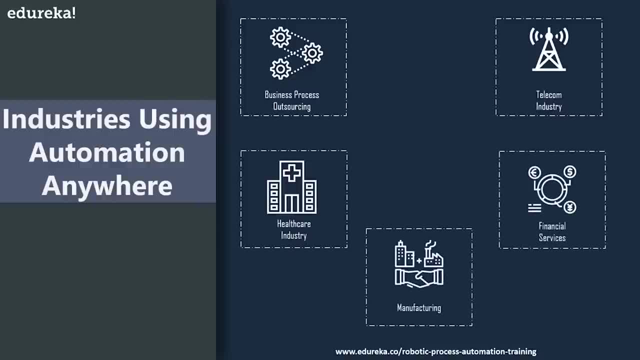 healthcare industry, financial services and marketing. Coming to the business process, outsourcing Automation is basically used in this industry to reduce the operational cost, improve operational performance and increase the capacity of the business. The telecom industry uses Automation Anywhere to provide support to the connected customers. 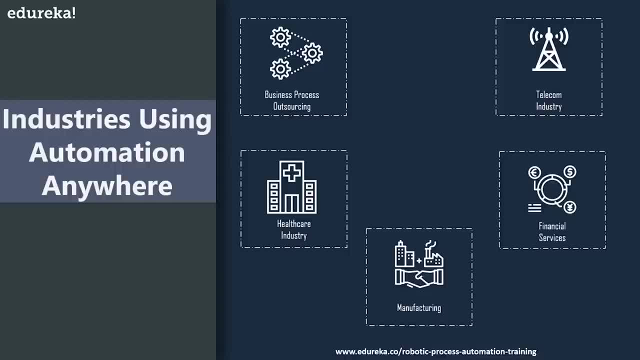 increase efficiency and also enable rapid growth. simultaneously, The healthcare industry uses Automation Anywhere to engage effectively with the patients, to reduce the risk and also analyze the critical healthcare data. The financial services use Automation Anywhere to improve the efficiency, reduce the fraud and also reduce compliance. 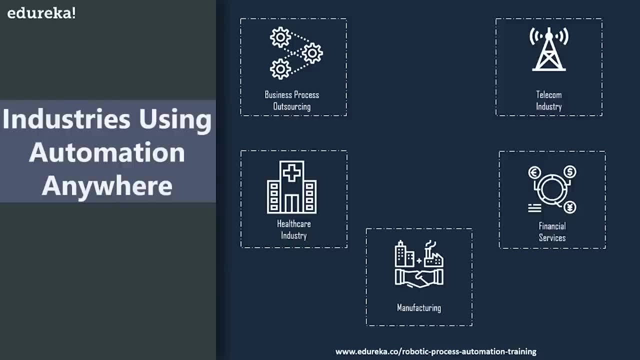 and manufacturing uses Automation Anywhere to streamline supply chain management, reduce cost and also accelerate production, Right? So, guys, let me just tell you that you know this is not the end to the story. There are various other industries using Automation. 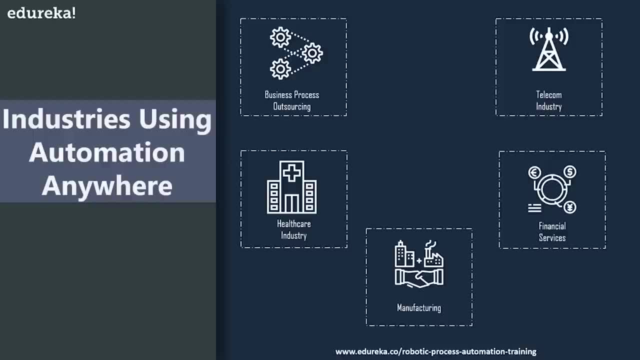 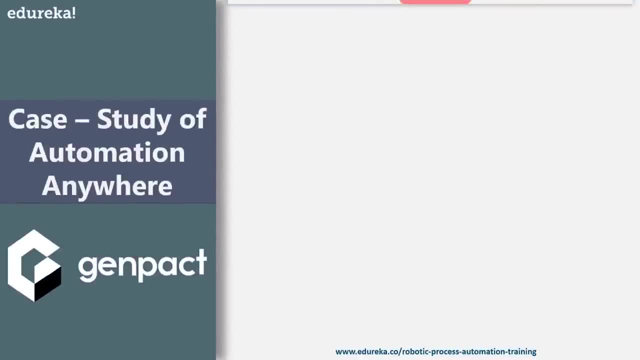 but yet I've just mentioned five over here, just for your knowledge. right Now, talking about industries, let me just next show you a company case study where a company started using Automation Anywhere and benefited by this right. So the company that I'm going to talk about is Genpak. 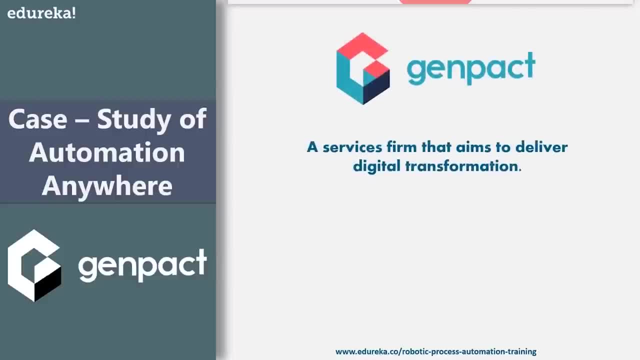 So Genpak is a services firm that aims to deliver digital transformation. A client of Genpak creates cameras, lenses and systems to the major companies. Now, the problem statement of this particular company was that that you know Genpak's clients order fulfillment procedure. 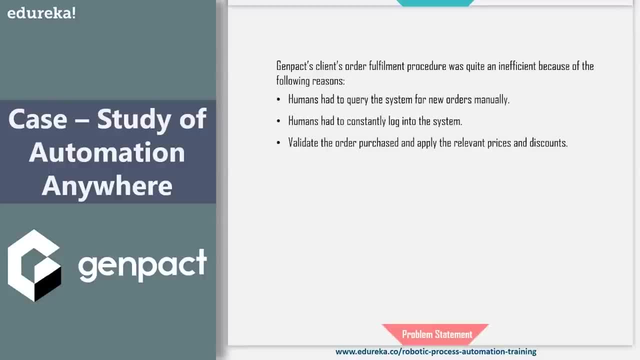 was quite an inefficient manual process, as humans had to query the system for new orders manually. This also caused quite a chaos, as humans had to constantly log into the system. Also, they had to validate the order, purchase and apply the relevant prices and the discounts. 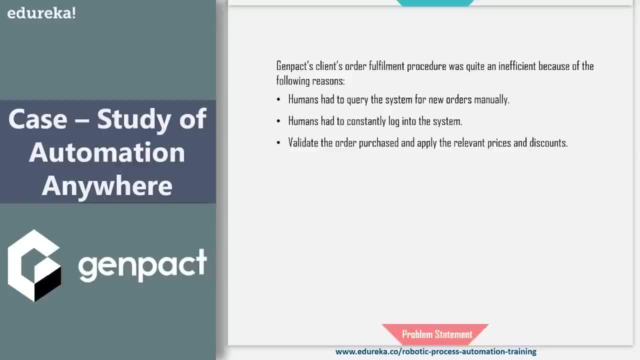 Now, obviously, this procedure was quite tedious, time-taking and was prone to errors. Now, to benefit their business, Genpak decided on automating their processes. Obviously, the solution was Automation Anywhere. So Automation Anywhere, and Genpak decided to re-engineer the process. 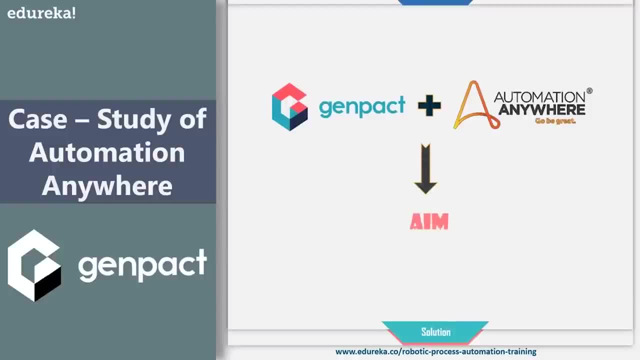 by using the smart enterprise processes. Their aim was to remove the inaccuracies, inefficiencies and the human errors caused in the system. So the execution team decided on to integrate the legacy systems with the Automation Anywhere and make sure that you know humans have an eye. 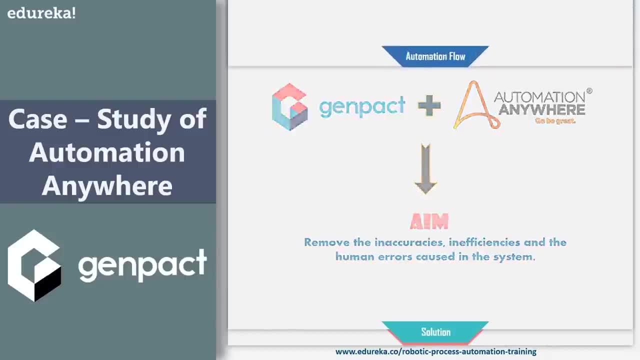 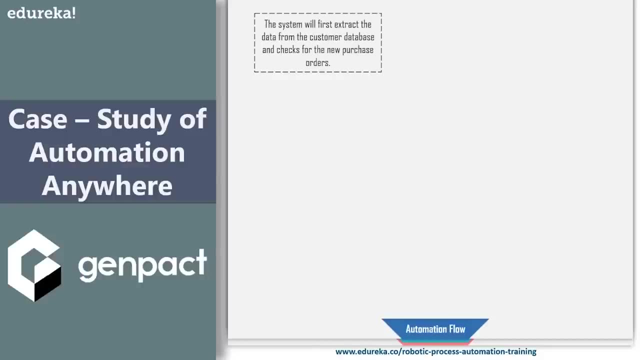 on the entire process getting executed right. So let me just tell you the flow of the automation. So the system would first extract the data from the customer database and then check the database for the new purchase orders. Then, once the purchase order gets downloaded, 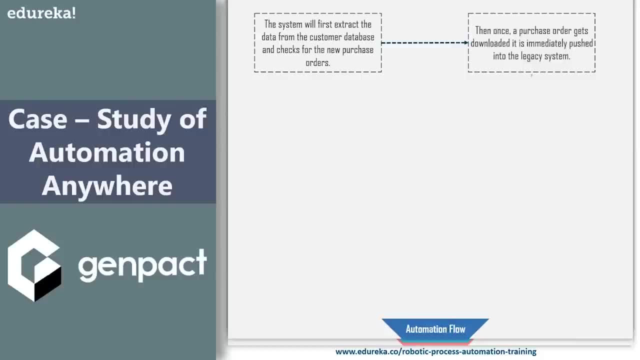 it would be just immediately pushed into the legacy system. After that, the agent would keep an eye on the process and manually validate the order for maintaining accuracy. And finally, Automation: Anywhere would upload the purchase into Oracle and then discounts would be automatically applied. 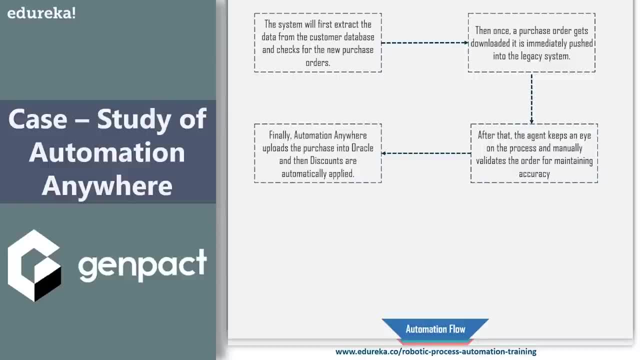 right. So, apart from all of this, let me also tell you that you know agents would cross check the full order then and ensure the quality control right. So what would happen is the system would first extract the data from the customer database, Then, once the data has been extracted, 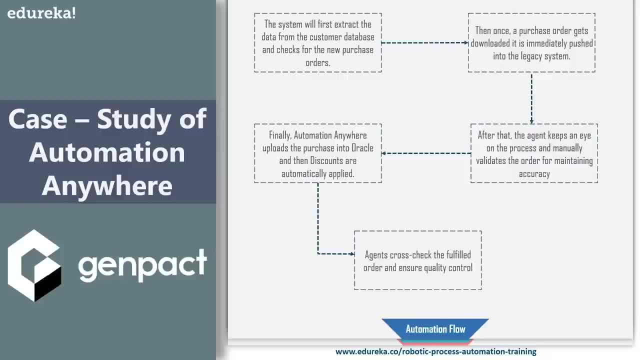 it would be pushed into the legacy systems. After that, the agent would keep an eye on the process and validate the data and finally, Automation Anywhere would upload the purchase into Oracle and the discounts would be applied as a cross check to the complete system. 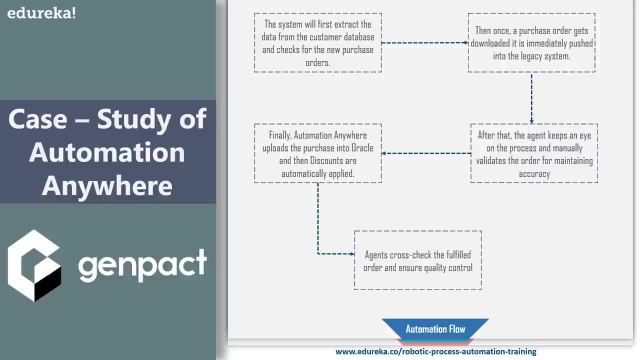 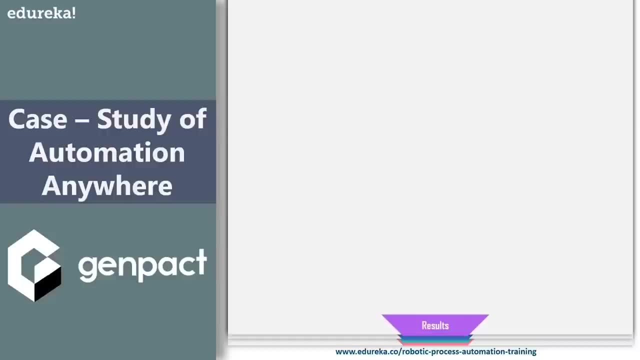 Agents would cross check the fulfillment order and ensure quality control right. So I'm clear with this point. Now, moving on to the results of this particular solution, the results observed are quite good. So the results were basically, like you know, there was 40% improvement in productivity. 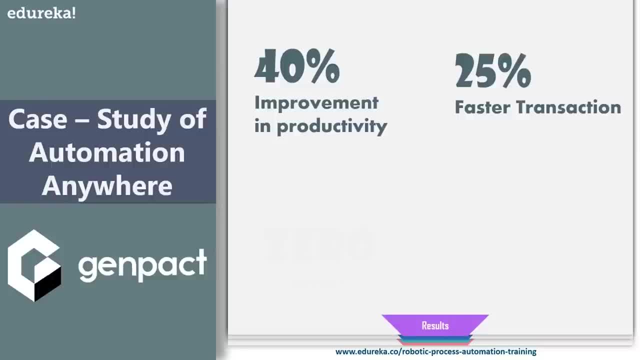 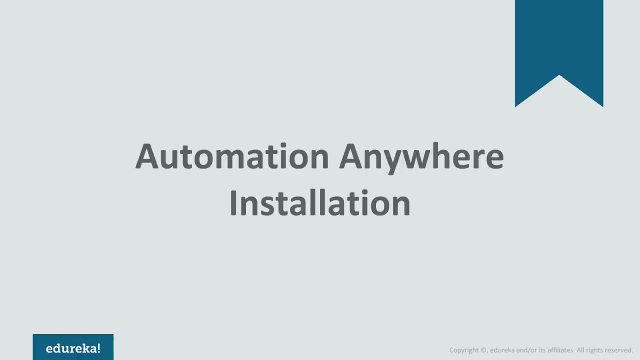 There was 25% of increase in the speed of the transactions. There was zero errors caused, as you know, manually. people would not do anything, So there was less chances of errors and 90% of manual labor was reduced. Welcome to the session. 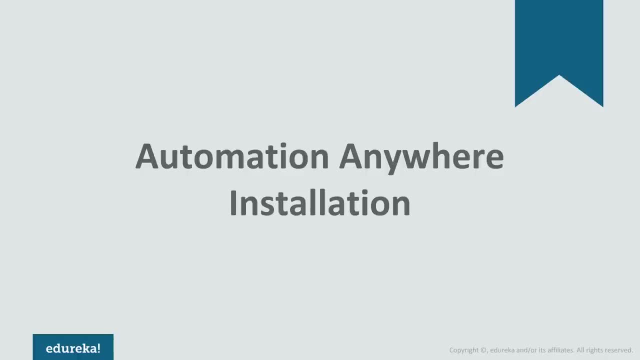 on installation and setting up of Automation Anywhere Enterprise Edition. right? So in the session, guys will see step-by-step how you can install and set up Automation Anywhere Enterprise Edition into your system. So let's get started. But before that I would like to request all of you to subscribe. 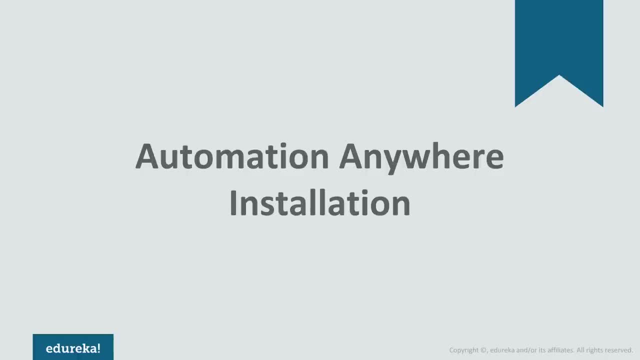 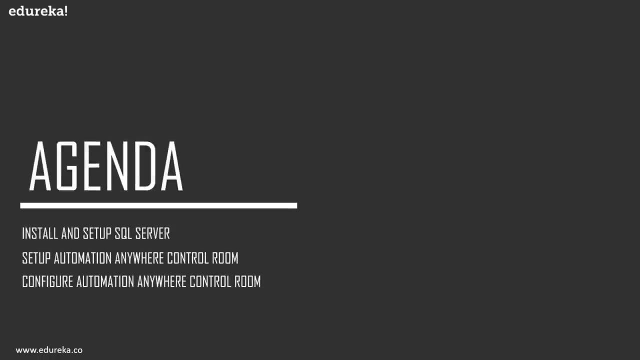 to our Edureka YouTube channel to get daily notified on the top trending Technologies. So on that note, let's start with today's session. So the topics for today's session are, as you can see on my screen, will first see how to set up. 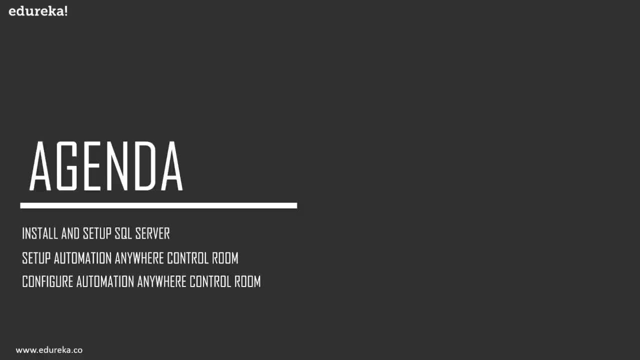 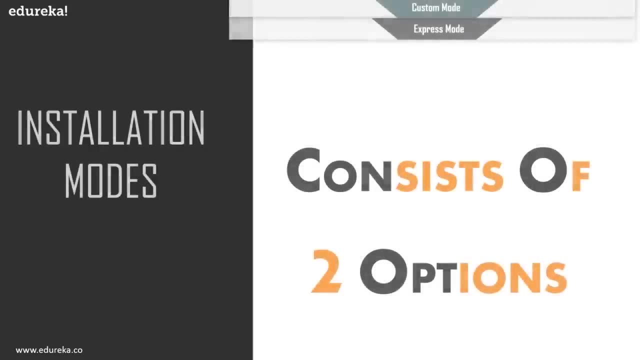 and install SQL Server, and then I'll show you how to do that, How you can set up your control room. Once both of them are done will finally see how we can set up our Automation Anywhere client. So let's get started, guys. 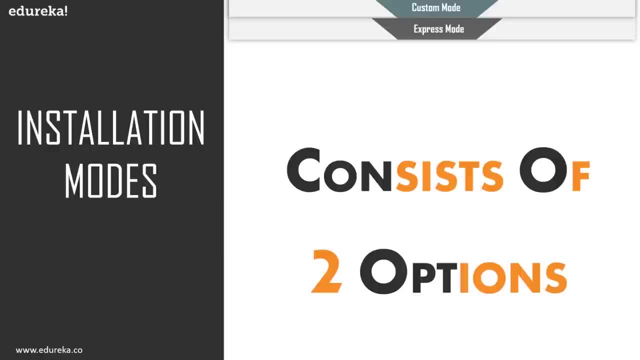 Now, before I start with the setting up and installation of Automation Anywhere, I would like to tell you one thing over here that you know: Automation Anywhere Enterprise Edition can be either installed in the Express mode or the custom mode. So we'll be going forward with the Express mode. 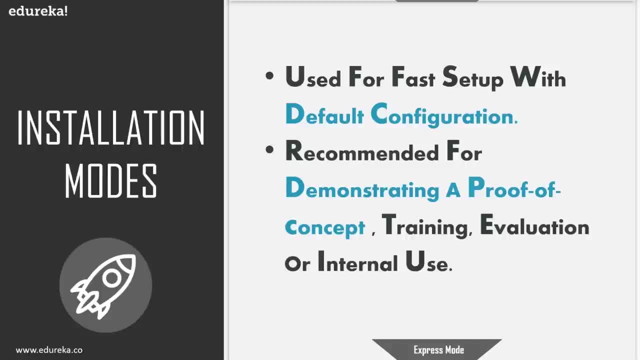 I've chosen Express mode because, you know, I just want to install Enterprise Edition on my system, right? I don't want to install on, you know, like, let's say, hundred systems or so, I just want to install on my system and I want the default configurations. 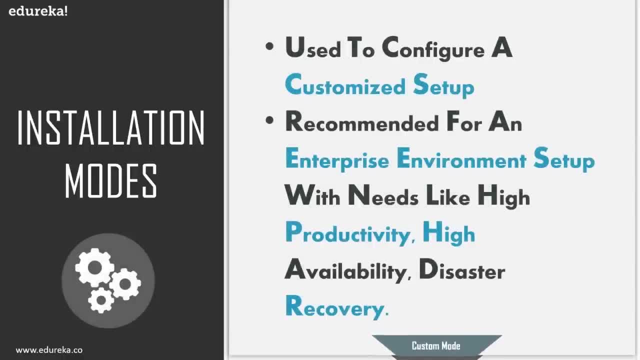 but when we go for the custom mode. custom mode is basically designed to install Automation Anywhere for an enterprise or maybe for a company where you know hundreds of PCs are using Automation Anywhere and the company wants few specific configurations. in that scenario We go for the custom mode. 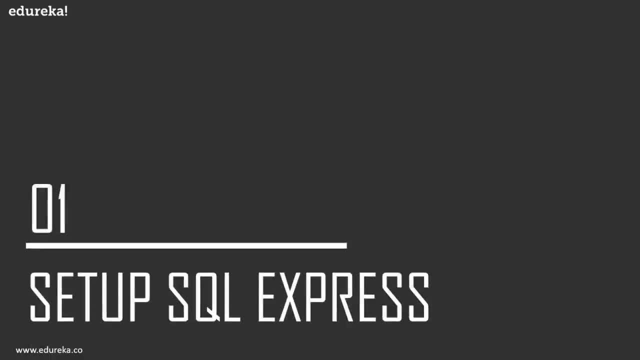 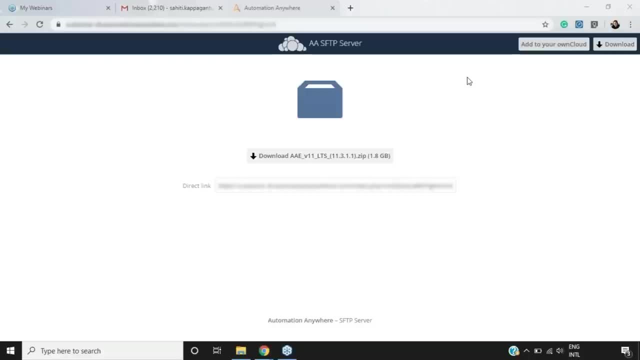 but since in this session we're just installing Enterprise Edition on our system, I'm going to choose for the Express mode. So when we choose Express mode to install Automation Anywhere will be basically redirected to this particular link, from where you can install Automation Anywhere. 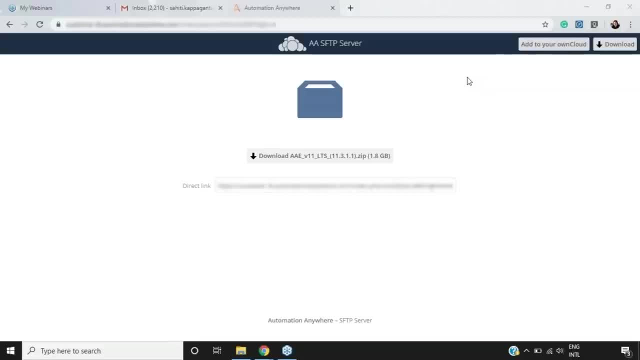 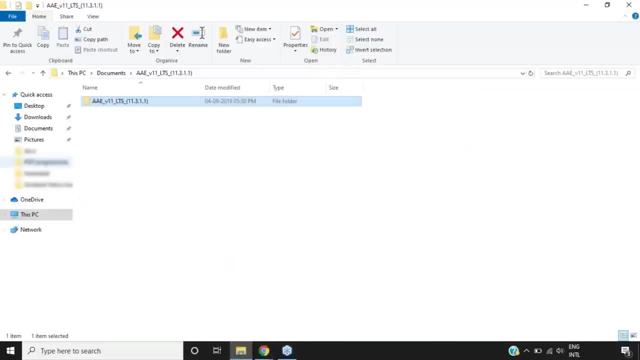 Enterprise Edition. Now this is the link from where you can download Automation Anywhere Enterprise Edition. So, since I've already downloaded on my system, what I'm going to do is I'm just going to use that particular file itself. So, once you download, Automation Anywhere, 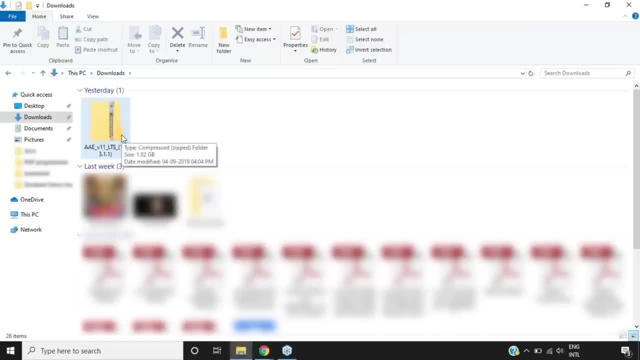 you'll basically see the zip file, right. So this particular zip file is downloaded and all the setup or and the required configurations are compressed under this file. So what we'll do is you basically have to extract this file. Well, I've already done that too. 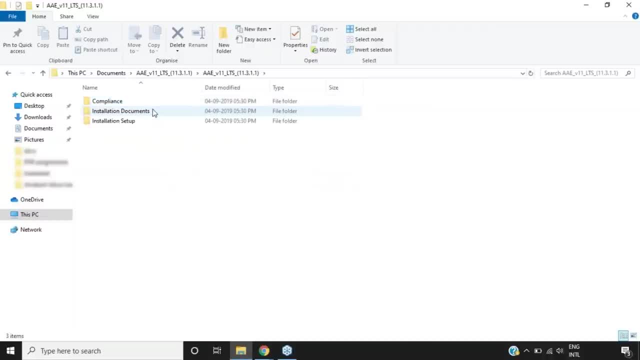 So once I extract, that is this particular folder which basically consists of compliance installation documents and installation setup and installation setup. We basically have client and control room. But before that, as I said, you have to install and set up sequel server. We also have sequel servers folder over here. 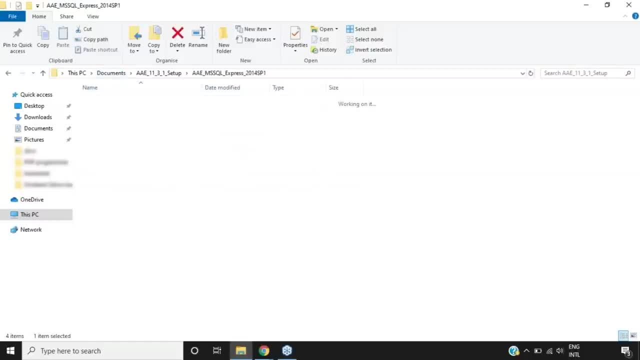 which is basically the setup folder from where you have to install. now, to start installing sequel server, What you basically have to do is you just have to double click on this particular icon, And once you double click on this particular icon, you'll basically see a dialog box which says that you know. 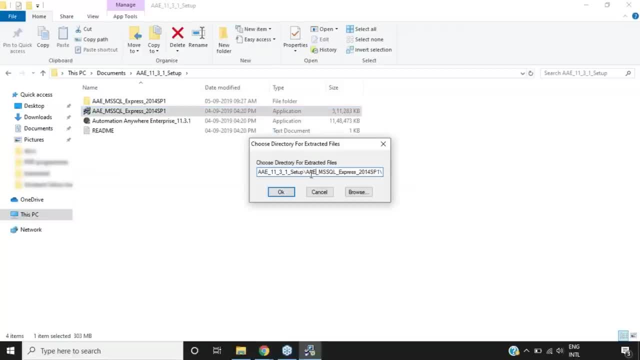 you have to choose the directory for the extracted files. So you can basically just choose the directory that is required. that basically chosen, see users and the username documents set up and then the sequel Express. So right, so I'll just click on OK. And once I click on OK, 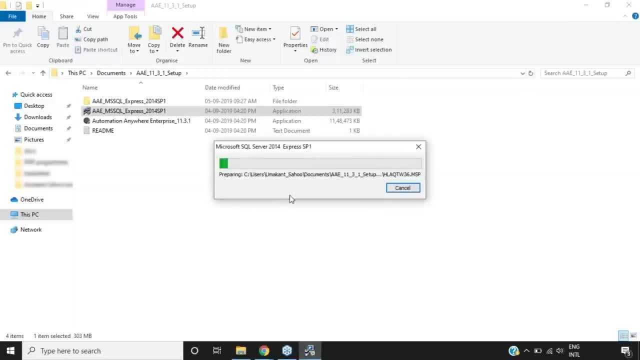 you'll see a dialog box which will basically show the status of you know how many files are getting extracted, So we'll wait for that to happen. All right, Now, once the files are extracted, this is basically the dialog box which opens up. 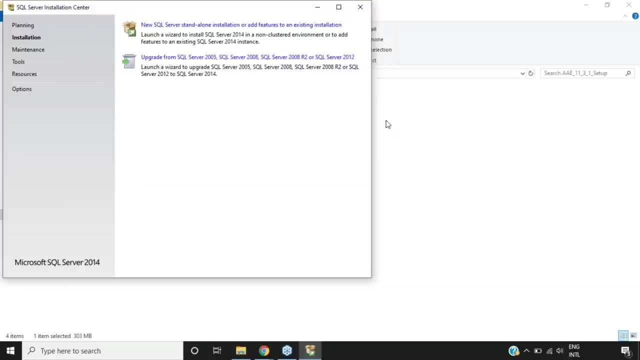 So it's basically the sequel server installation Center, where you have basically two options. The first one is the new sequel server standalone installation or to add features to an existing installation, and the second one is to upgrade from the existing sequel server, that is, 2005, 2008, 2008, R2 or 2012 version. 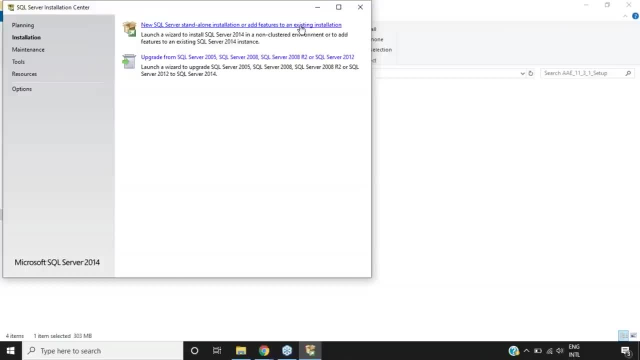 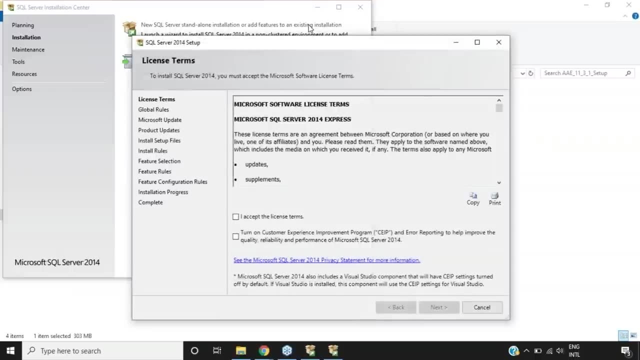 So since we're installing for the first time, we'll just choose the first option, that a sequel server standalone installation, right? So I'll just click over here Now. once I click on that particular option, you'll see a dialog box which will basically declare the license terms. 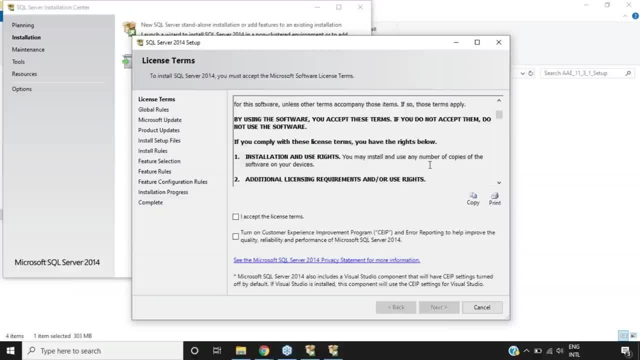 So it's your wish, You can go forward and read the license terms. Well, I'm not going to do that presently. I'm just going to click on I accept the license terms radio button and then I'll click on next. once I click on next. 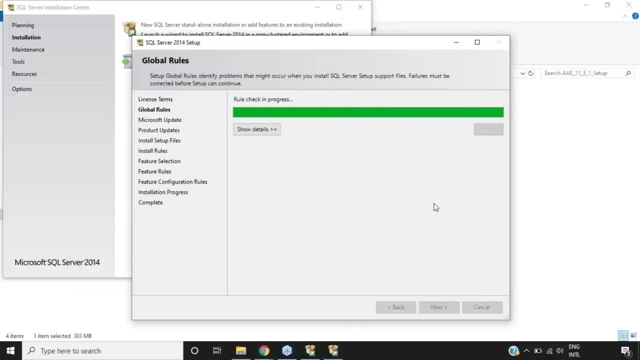 will be basically redirected to the global rules page where you know all the rules will be checked, and then we'll go to the Microsoft update option. in that particular option You don't have to check in anything and then you just have to click on next right. 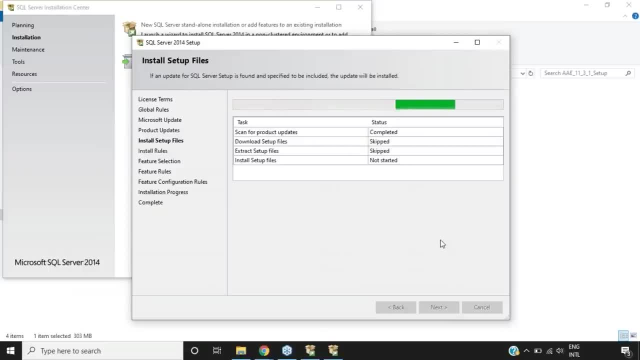 So I'll just click on next and once I click on next will be basically redirected to install set of files. Well, you see that you know all the set of files are getting installed and then few of them will be completed and few of them will be skipped. 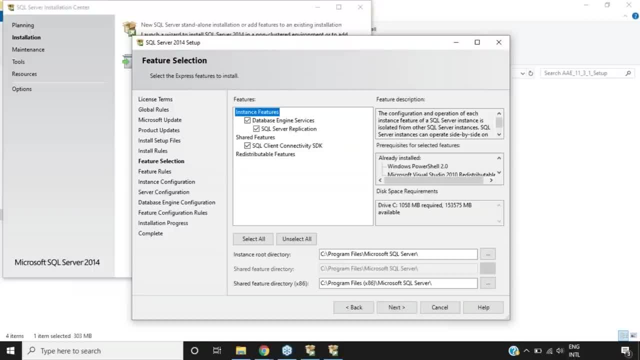 Now, once that is also done, you'll go to install rules, and one install rules are also done automatically. The next one which comes is feature selection. So, over here, what do you have to do is you have to make sure that you know. 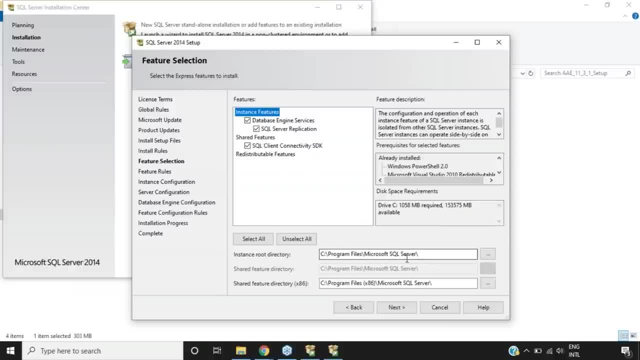 all your checkboxes are checked, and then you have to choose your instance root directory and the shared feature directory, right, Well, I'm going to keep it as it is. I'm not going to change any of them, and then what I'm going to do is I'll just click on next. 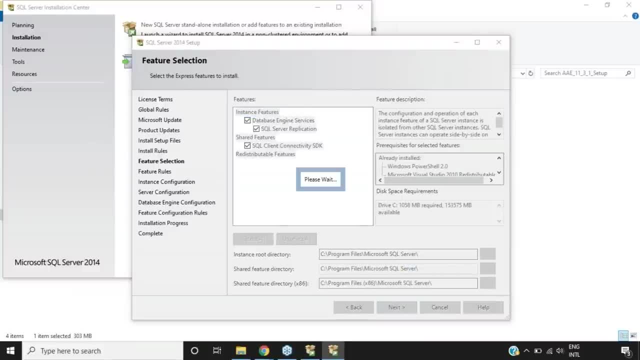 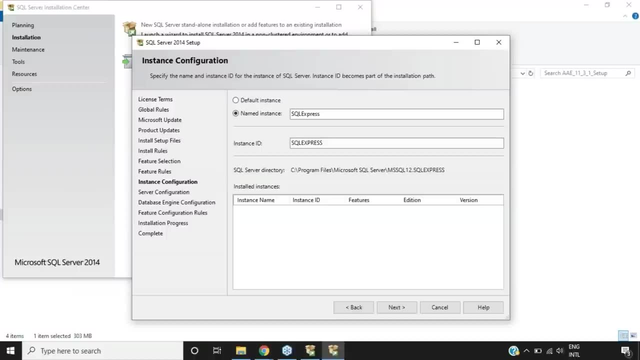 Once I click on next, the next thing that we have to choose is feature rules. So over there you have to basically give the name for your instance, right? So I'm just going to keep it sequel Express, which is by default, and the instance ID will be sequel Express, right. 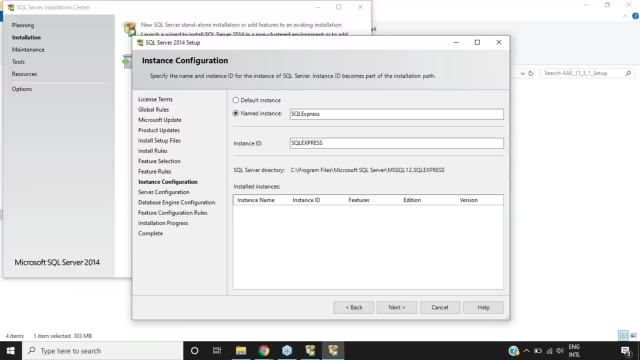 So with this particular instance ID will understand that you know this is our server through which automation anywhere will be connected. Please remember that you know the instance ID name is equal Express and the name of instance is also sequel Express. after that We have the server directory. 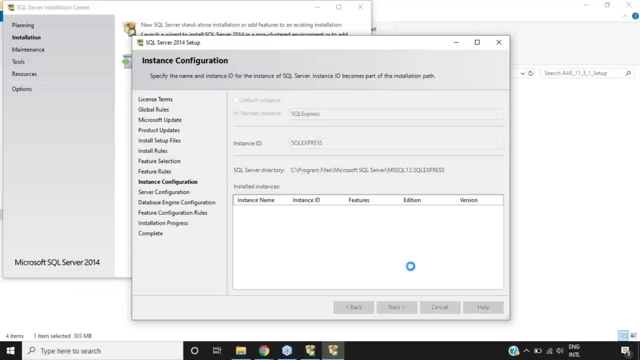 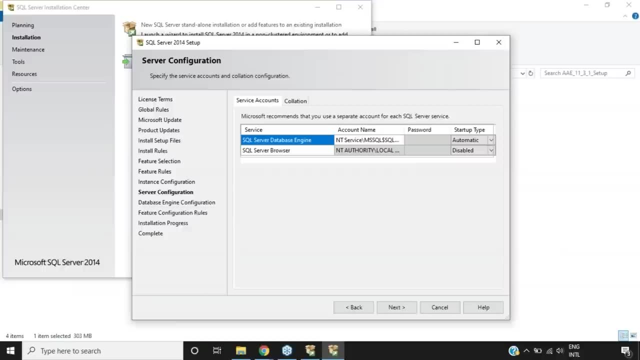 Now, once you think everything is fine over here, you just have to click on next again. Now, once you click on next, you'll be basically redirected to the server configuration, where you'll see the sequel server database engine and the sequel server browser. So we are. the startup type is automatic. 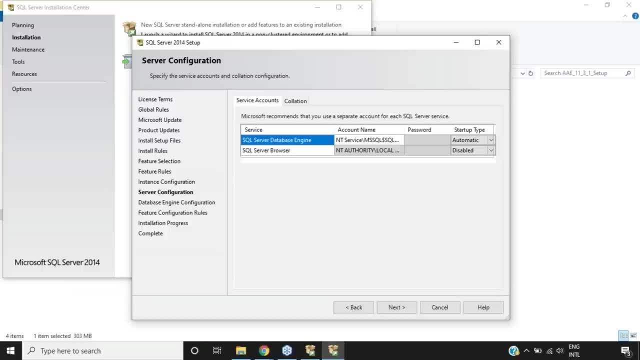 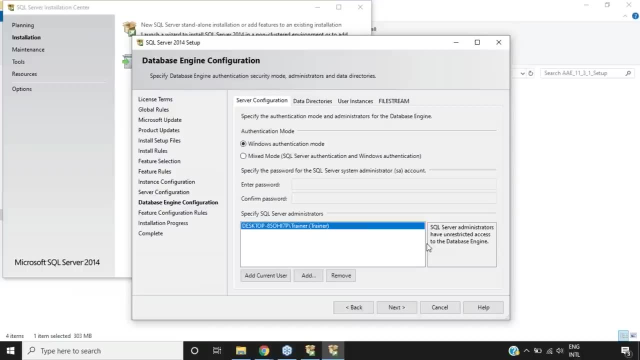 for the database engine, and then the browser is disabled by default. So I'll just keep it the way it is, and then I'll click on next. now, Once you click on next, the next thing that you have to configure is the database engine configuration. 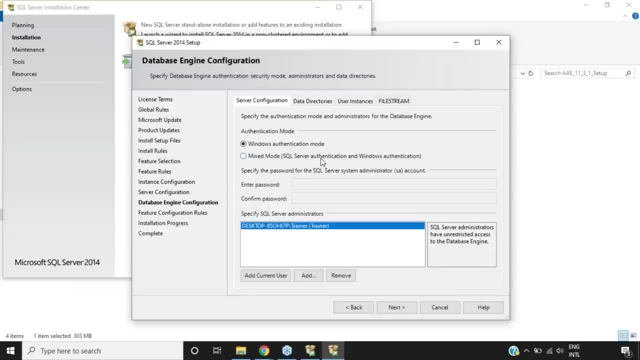 So over here, basically, we have two authentication modes, that is, the windows authentication mode and the mixed mode authentication mode. So I'll just choose the mixed mode authentication mode and then we can mention the password. So I'll just mention the password over here, Right? so I'll enter the password. 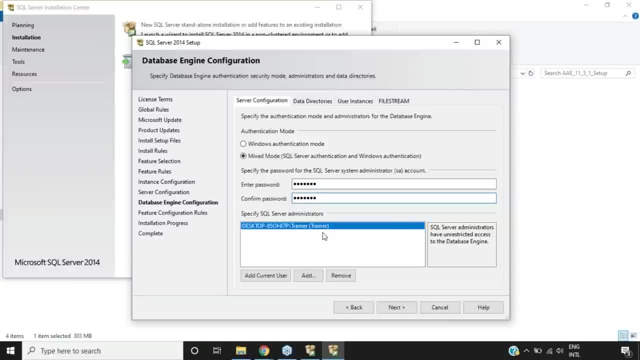 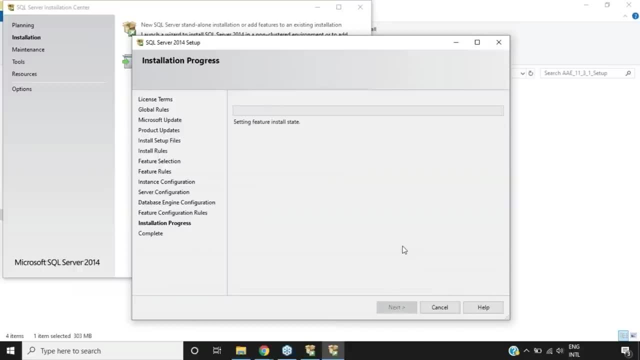 I'll confirm the password and then this is basically the desktop to which our sequel server is connected, and then what I'll do is I'll click on next. Now, once we click on next, automatically we see that you know feature configuration rules are done and then the installation progress is shown. 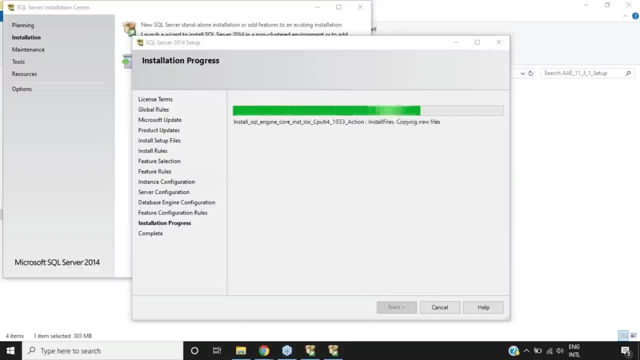 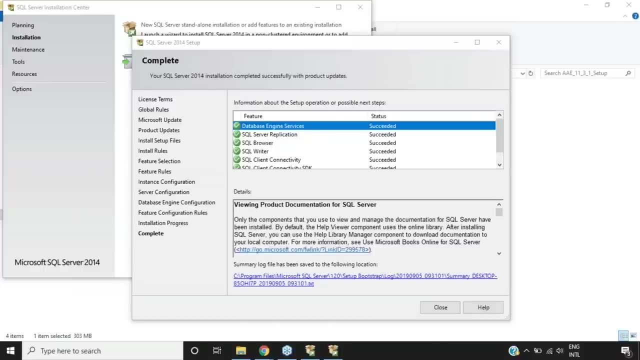 Let's just wait for that to happen. All right Now, once the installation is done, you see a dialog box which opens up and says it's complete and your sequel server 2014 installation has completed successfully. So over there you can see various features. 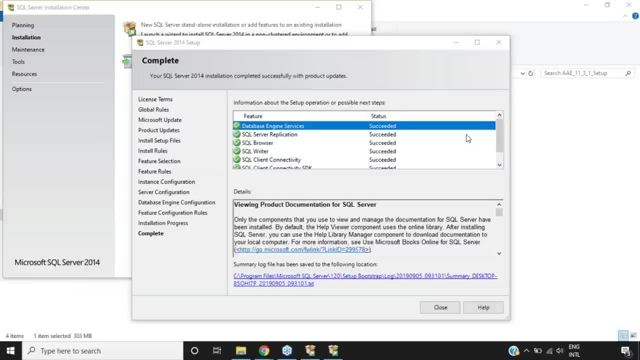 that have been installed, like you know: database engine services, sequel server application, the browser, the writer, the client connectivity, the client connectivity SDK and the support files. Now, once that is done, what you just have to do is you just have to check: everything is fine or not. 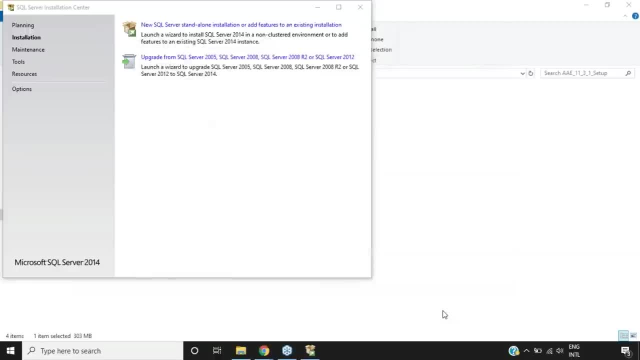 and then you can just click on close. now This is where your sequel server installation completes. but yet you have to make sure that you know your system is connected to the sequel server, right? So you basically have to enable the required services. So for that, what I'll do is I'll search. 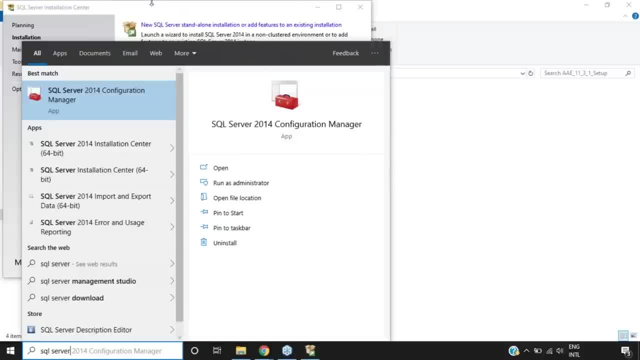 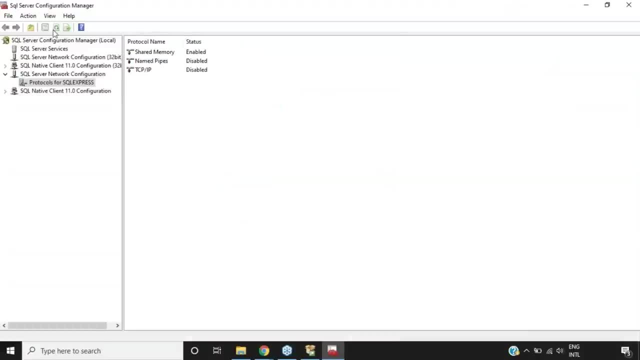 for sequel server configuration. So let me just search for sequel server configuration app, and then what I'll do is I'll just double click over here. Now, once I click on the sequel server configuration manager, this is basically the screen that opens up right now. 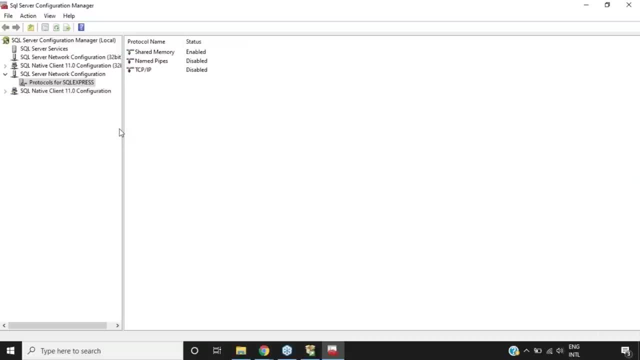 over here on the left side You see various options, like you know: sequel server services, the network configuration for 32-bit, the client configuration, the network configuration and the protocols for sequel Express, right? So this is basically what we had configured. if you remember right, the instance ID was sequel Express. 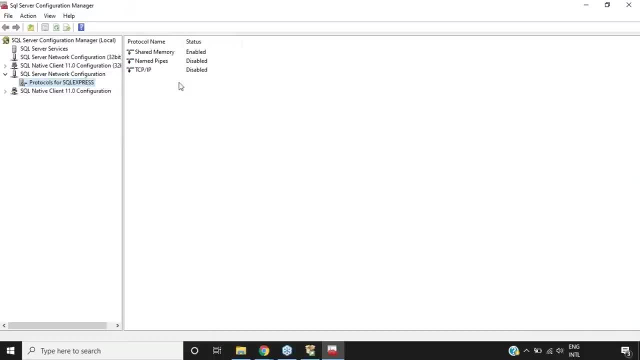 So over here, what you have to do is you have to go over here and then you see that you know the protocol name and the status on the right hand side. that is basically that you know the shared memory is enabled, The name pipes is disabled and the TCP IP are disabled. right, 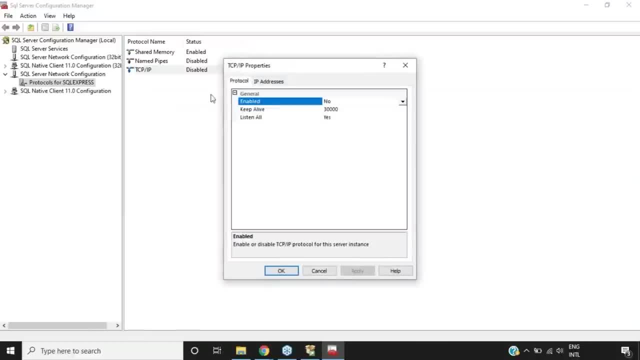 So what I'll do is I'll right click over here, I'll go to properties and then I'll go for IP address over here, right? And what you have to do is you basically have to scroll down completely and over here where you have the options of dynamic ports. 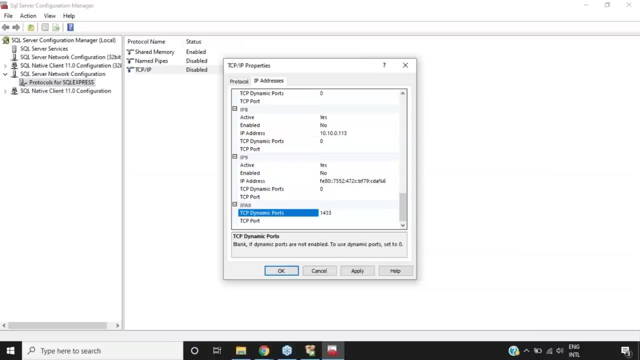 You just have to mention the port number. that is 1433, right. So remember that you know the TCP IP port for sequel server is basically 1433, right? So this is what you have to mention over here, and then you just have to click on. 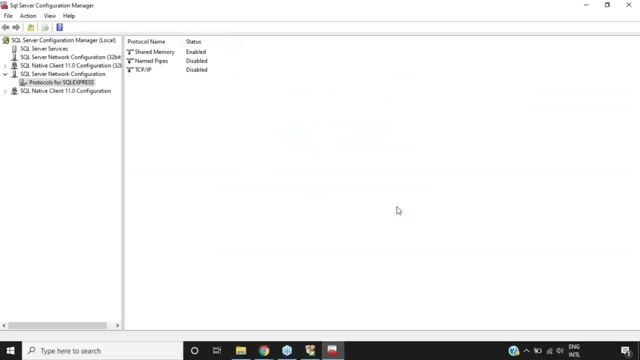 Okay, right now. after that you again have to click on Okay. and then what you do is you right click over here again and then you make sure the TCP IP port is enabled right now. So once TCP IP port is enabled, the next thing: 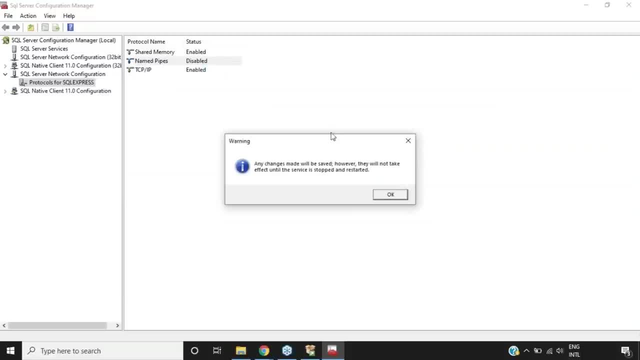 that you have to enable is the name pipes, So I'll again right click over here and choose enable. Now, once it is enabled, the next thing that you have to do is you have to go to the sequel server services option, and over here you basically see three options, right? 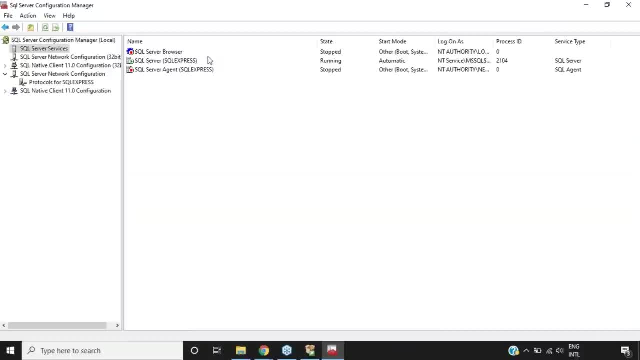 The sequel server browser, the sequel server for the instance ID and the sequel server agent for the instance ID over here. What you're going to do is you'll basically restart the service, right? So let me just restart this particular service Now. once this service has restarted, the next thing. 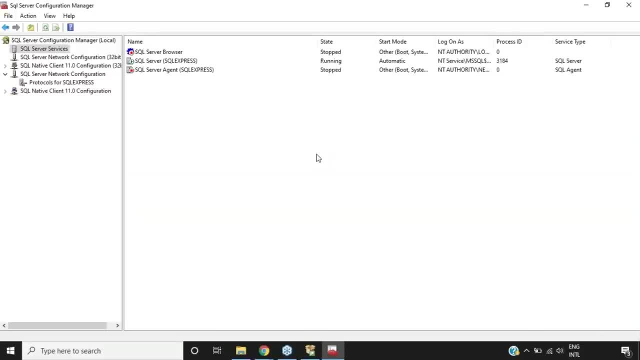 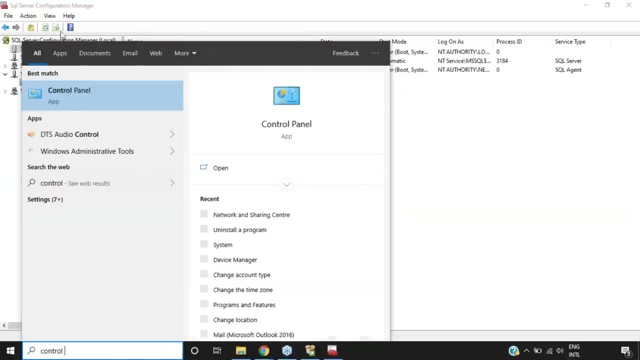 that you have to check is basically where you know where your system is connected to sequel server or not. So to do that, what you're going to do is you're going to go over here, right, and then you'll search for control panel, Right and in control panel. 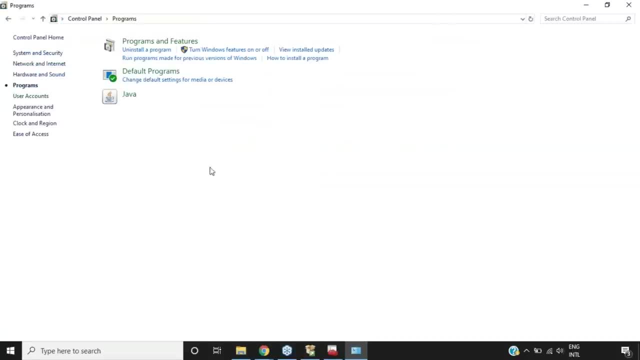 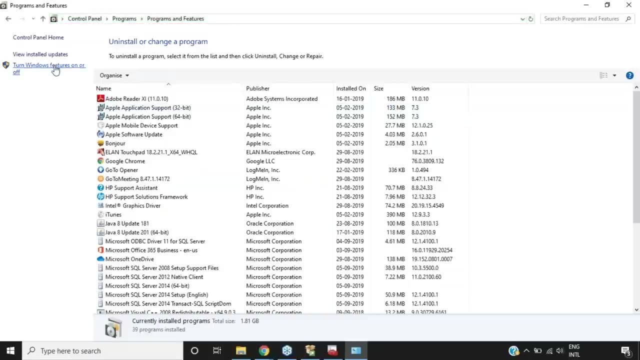 you'll basically choose programs and features, right? So you'll go to programs over here and then you'll choose programs and features, and then what you're going to do is you're going to choose this option of turn Windows features on or off, right. 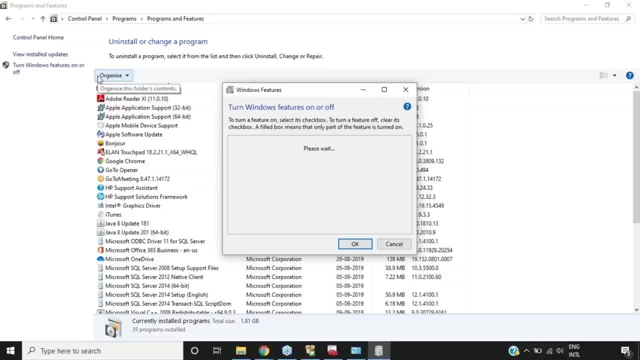 So I'll choose that, and then, once I choose that, you see this dialog box opening up. So over here you basically have to choose the telnet client, So let's search for that. My telnet client is already enabled, right, So just in case it's not enabled. 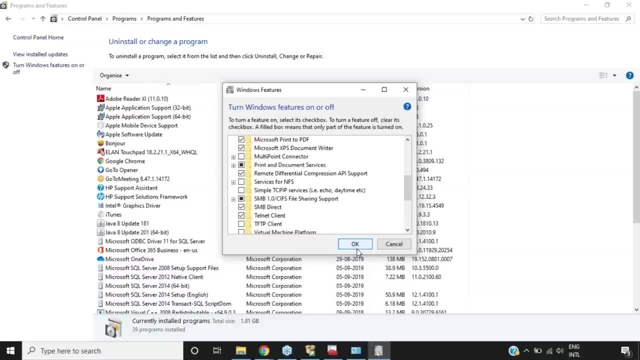 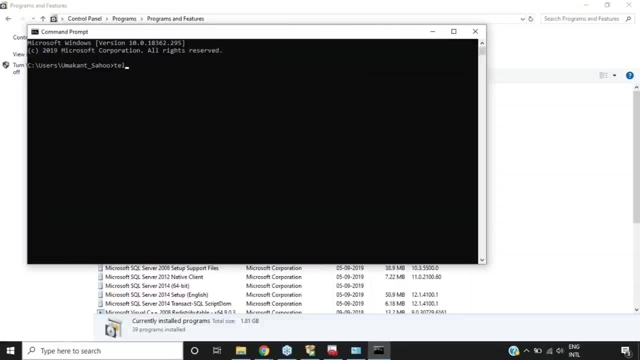 You just have to check into this particular box and then you have to click on OK. Now, once that is done, what you'll do is you'll go to command prompt And over here you'll basically type telnet, localhost and you'll mention the port number, that is 1433.. 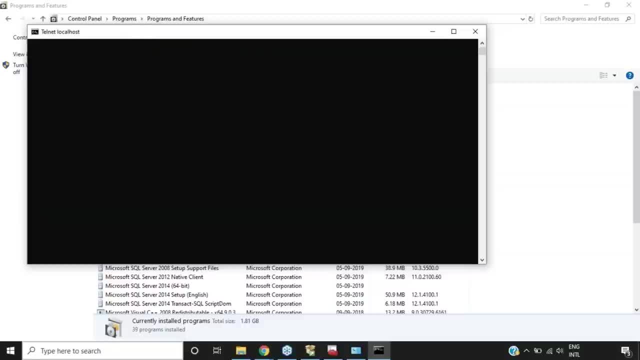 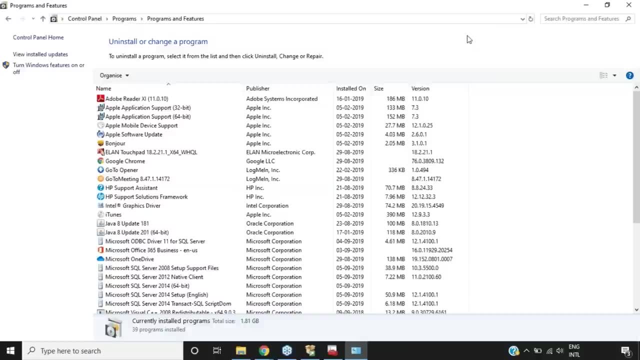 Now, once you see that you know this particular output is shown that is connecting to localhost, and it just vanishes. That means that you know your SQL Server is connected to our system. So this is where, guys, the SQL Server installation ends. I hope you've understood how you can install SQL Server. 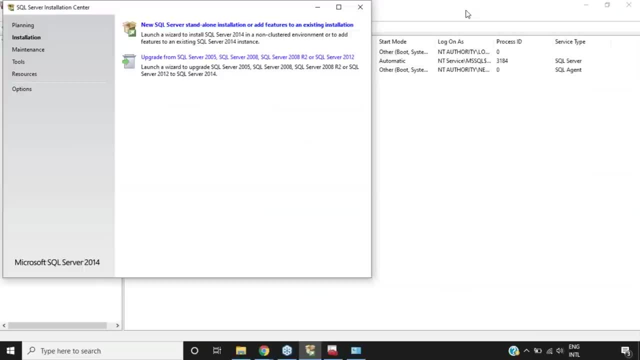 Well, it's really simple to install, guys. What you have to first do is you have to extract all the files from the automation anywhere folder and then put it in some file. after that You have to just choose the SQL Server application and then double click on that. 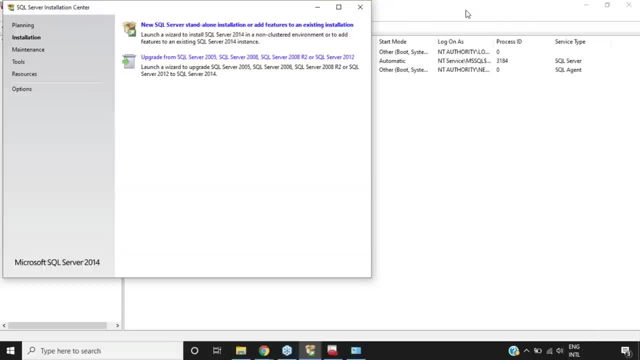 and then from there you'll see that you know the files will be extracted. after that You'll choose the option for new standalone installation. Well, you'll just accept the license agreements and then you'll just keep clicking on. next, The two most important things. 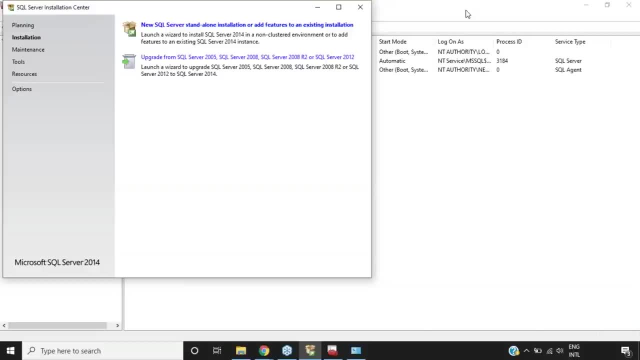 that you have to understand over here is that you know you have to check the root directory for SQL Server and also you have to check the instance name and the instance ID. now one, both of them are checked. You just keep clicking on next and then you'll see that you know installation is done. 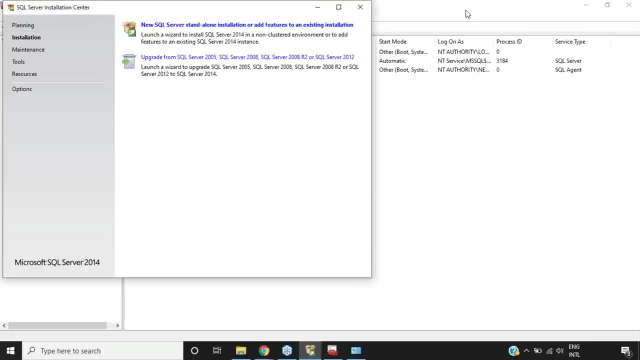 Once the installation is done You have to make sure that you know your SQL Server is a restarted right. So for that you'll go to the SQL Server configuration manager and in the protocol section you'll basically go to the TCP IP section, where you'll right click over there go. 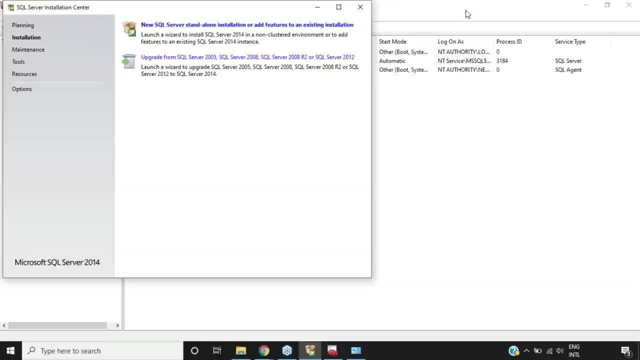 to properties and mention the port number in the dynamic port section. in the dynamic port section, that is 1433, and then you'll enable both the named pipes and the TCP IP. After that you'll go to the SQL Services section and then over there you'll basically restart the SQL Server. 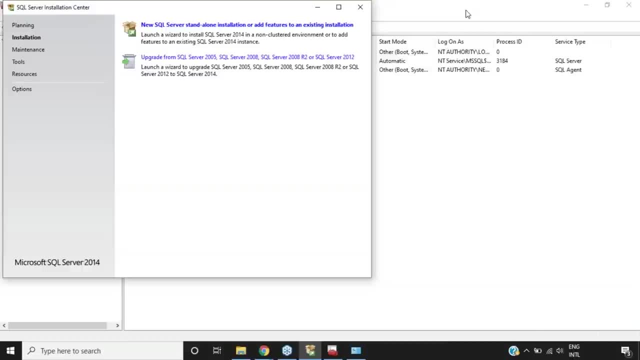 service and then, finally, to check whether your system is connected to SQL Server or not, You'll enable the telnet client and then in the command prompt you'll mention telnet local host and the port number that is 1433.. So that was about installation of SQL Server, guys. 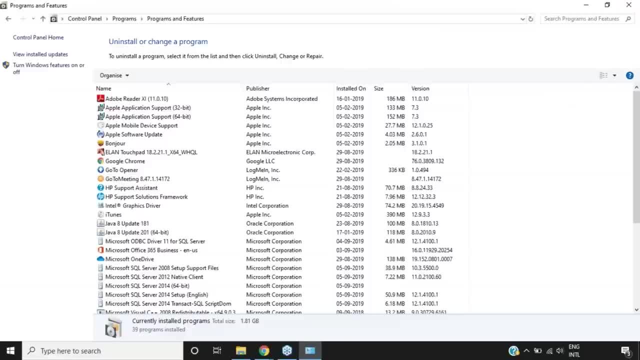 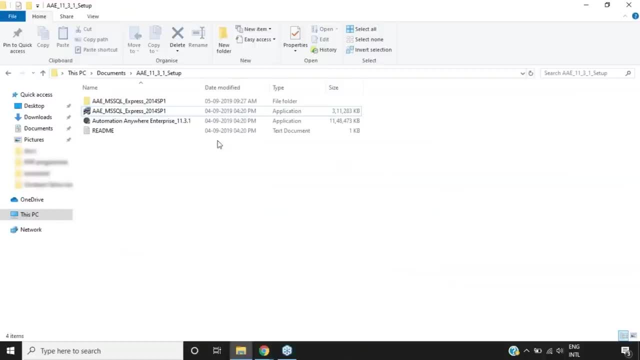 I hope you've understood. now Let's just close all these windows so that there's no confusion, right, and let's move forward and install Enterprise Edition. That is basically where you'll set up the control room. So for that, what I'll do is I'll right click over here: choose. 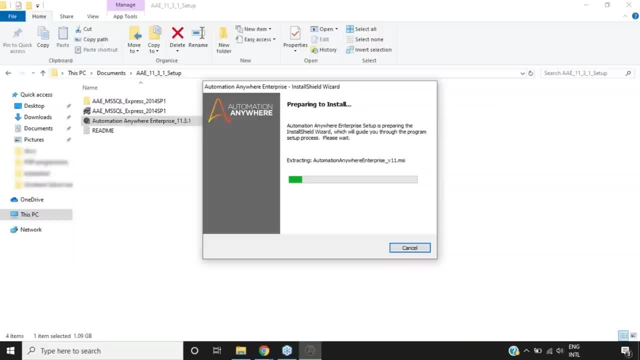 run as administrator. Now, once we choose run as administrator, we see this dialog box with says preparing to install. So let's wait for that to happen Now. once that is done, you get this option of you know unsupported OS detected. you see a message. 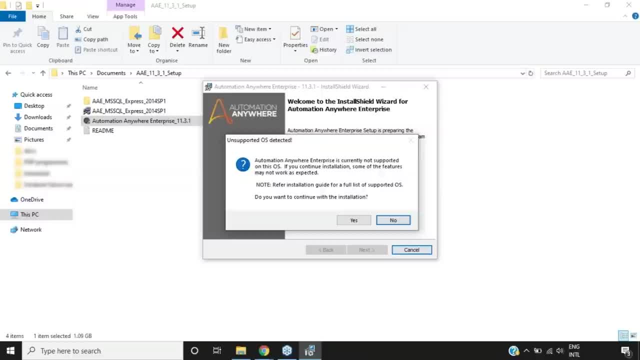 that you know. Automation Anywhere Enterprise is currently not supported on this OS. But yet, if you want to continue your installation, some features might not work right. So we just want to continue our installation. So we'll just click on yes over here, and then what will happen is that you know. 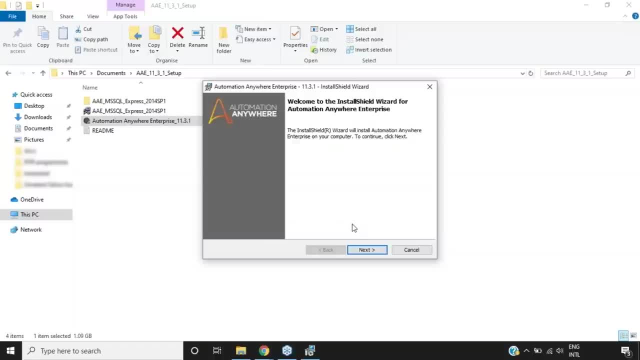 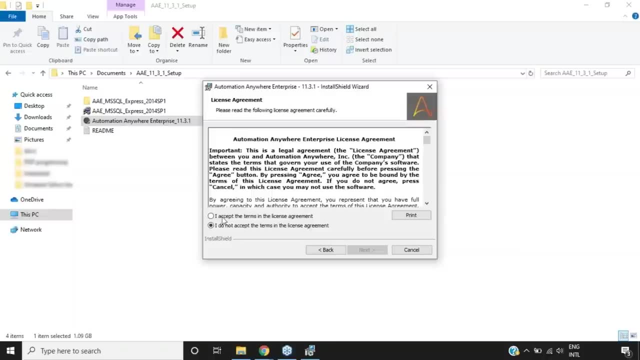 you'll see a dialog box which says welcome to installation wizard for Automation Anywhere Enterprise. So for this particular wizard you just have to click on next and then you see that you know you have to accept the license agreements, right, So I'll just click on: I accept the license agreement. 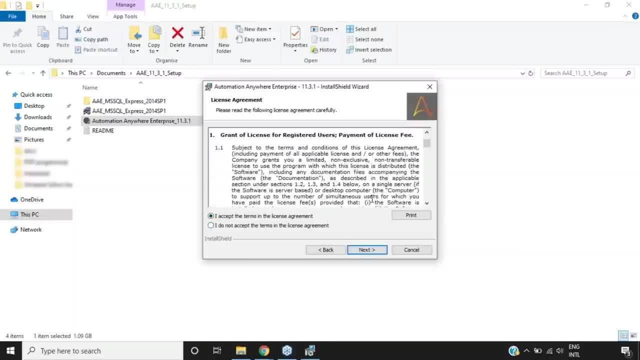 Well, you can go forward and read the agreements. Well, I'm not going to do that for this particular session and then I'll click on next. once I click on next, you see option of, you know, Express installation and custom mode installation. Well, these are two types of installation modes. 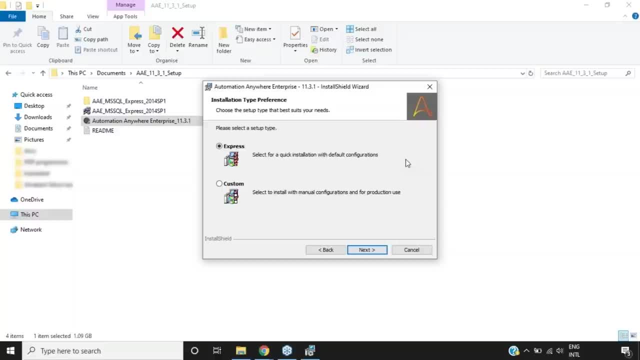 that you can use right. So since I have told you before also that you know I'll be going forward with the Express installation, I'm just going to choose the Express installation for a quick installation with default configurations. but if you want to manually configure way stuff. 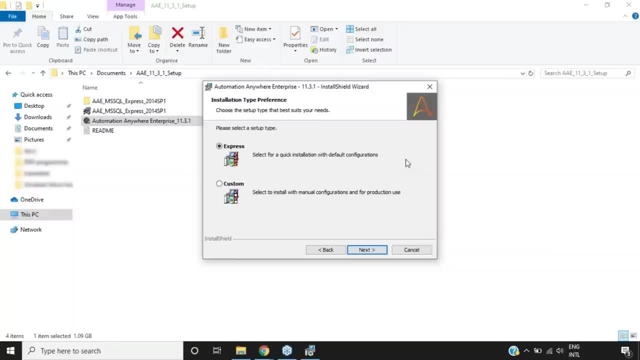 and then you want to use Automation Anywhere for production usage. you can go forward and choose the custom mode, But for this session, as I said before, I'm going to go for the Express mode, So I'm just going to click on next over here. 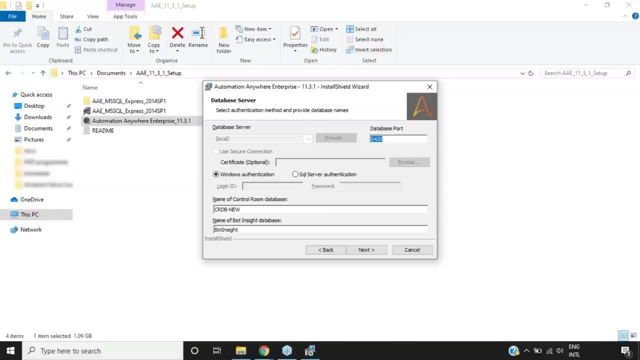 Now, once I click on next, the next thing that you see is the database server configuration. as you see on my screen, the database port number is 1433- that we had configured before- and then the name of the control room database will be CRDB new and the name of the bot inside database will be bought inside. 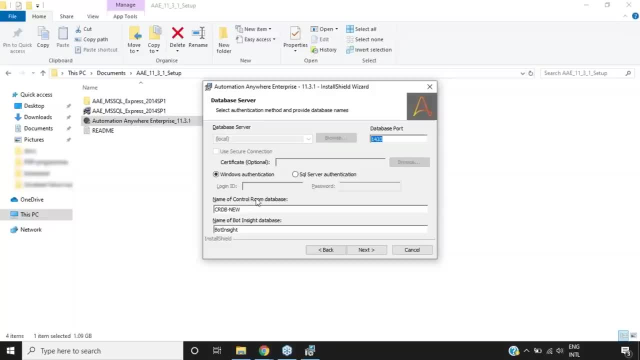 over here There are again to authentication modes: Windows and SQL Server. while I'm going to go forward with the Windows one, after that I'll just click on next. So please remember that you know you have to make sure that you know all these details are correct. 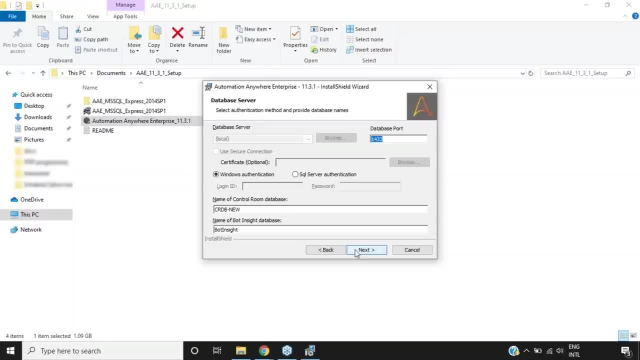 and then you find with all the details present, because once you install you cannot change these details. So the control room database will be CRDB new and the port inside database will be bought inside. So after that, I'll click on next. Now, once we click on next, we see an option. 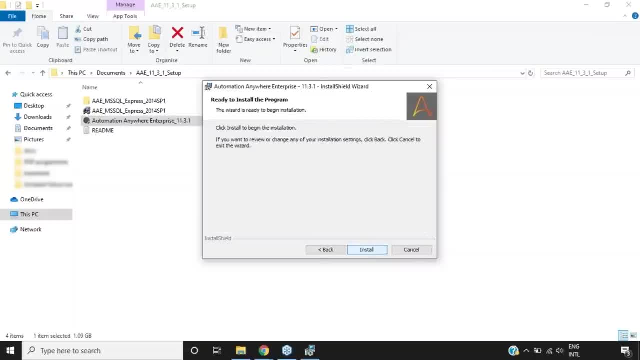 as ready to install the program, right? So if you're fine with all the details mentioned before, you can just go forward and click on install. But otherwise, if you want to just check again, you can choose the option of back, go back and check all the details. 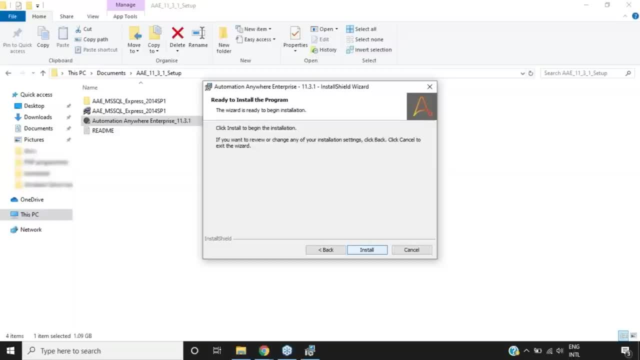 and then come back and choose the option of install. So I'm just going to choose the option of install over here, All right Now, once I click on the option of install, you can see that you know my installation wizard has started installing automation. 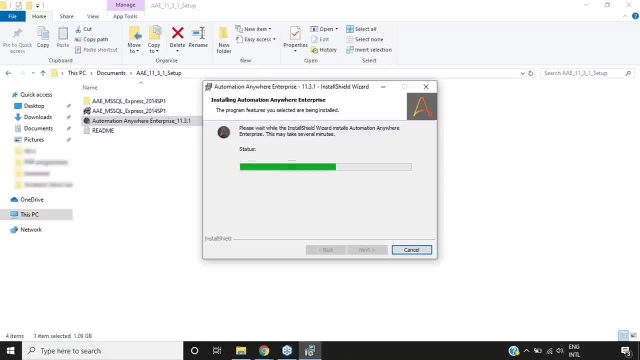 anywhere, Enterprise Edition. So let's just wait for that to happen. All right, Now, once the installation is complete, you see this wizard which says you know installation shield wizard is completed and then you get to check boxes where you know you can choose either to launch the automation 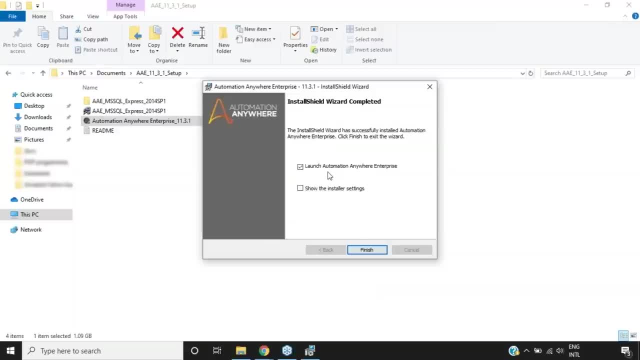 anywhere Enterprise and show the installer settings right. So I'm just going to check in the first box that is a launch automation- anywhere Enterprise- and then I'm going to click on finish. now, Once I click on finish, you'll see that you know automatically. 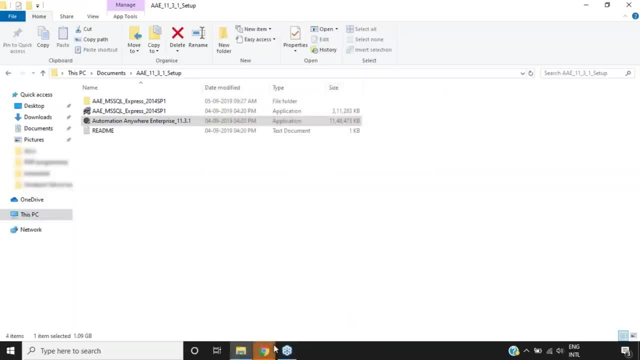 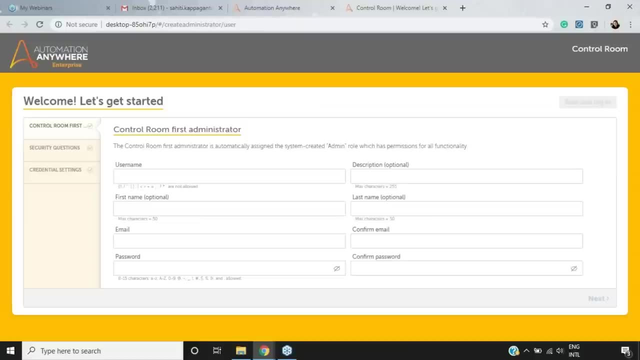 automation anywhere, Enterprise will be launched right. So you can see that control room is getting launched right. So let's just wait for that to happen, All right. So once the control room is launched, you see that you know the control room. 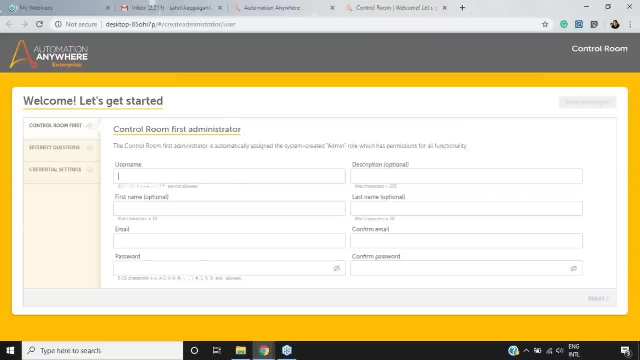 Administrator page opens up where you have to mention the username, the first name, email password and so on. So what I'm going to do is I'm going to make the first username to be Advent, because that person will be admin, and then first name to be, let's say, trainer. 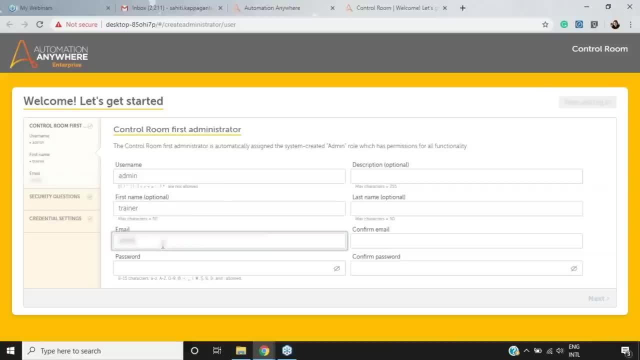 That is my desktop name email to be. let's see my email ID, Right, and then I'll just confirm the mail. After that I'll mention the password. So let me just mention the password. Okay. it says six to five characters with capitals, alphabets, numbers and then symbols, right? 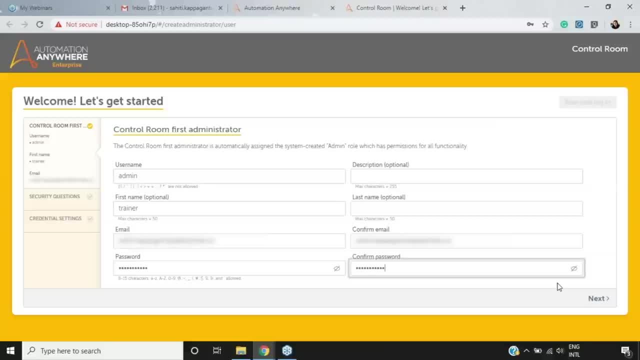 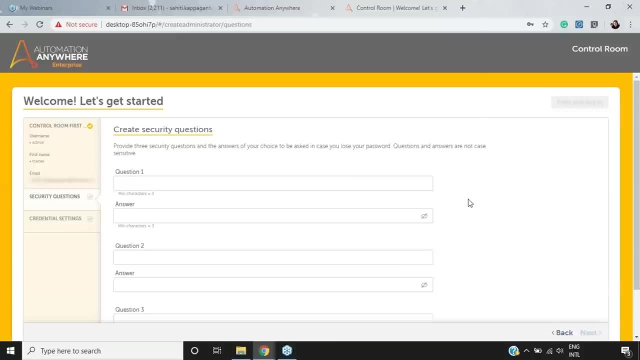 So I'll just mention, Now, once that is done, what I'll do is I'll just click on next. Now, once you click on next, what you see is that you know you have to basically create security questions, just in case you know you forget your password, and so on. right, 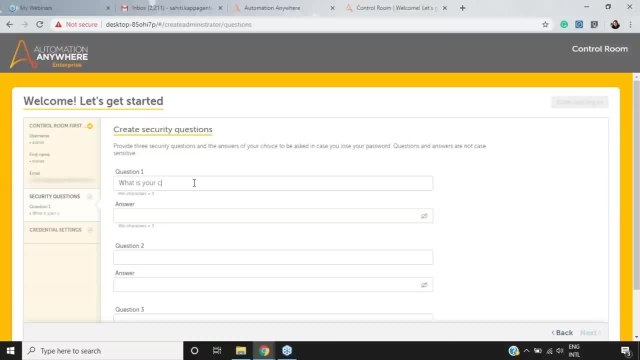 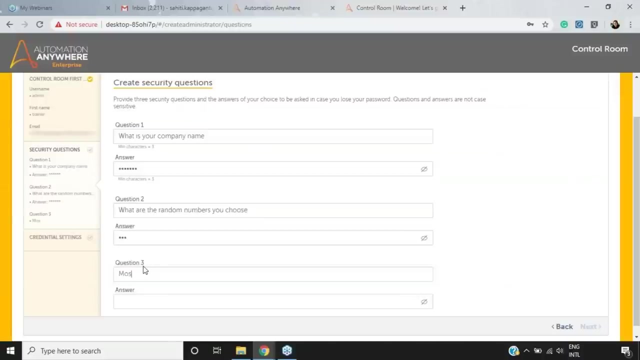 So I'll just mention what is your company name and mention the answer. I'll just mention the next question, which is what are the random numbers You choose and mention the answer, and then let's say most common symbol. I'll just mention the answer over here, right? 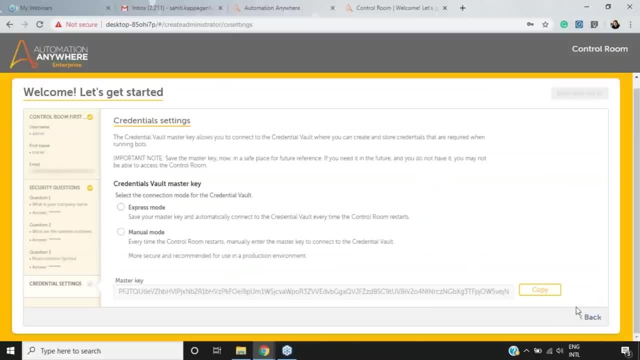 And then what I'll do is I'll just click on next. now, Once we click on next, this is the next thing that you have to configure. that is basically the credential settings. So the credential settings basically has a credential vault master key which allows you to connect. 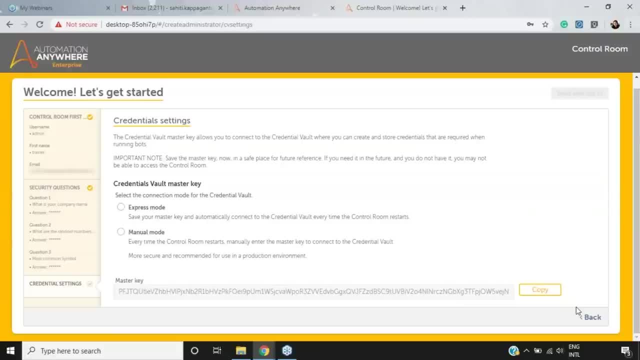 to the credential vault where you can create and store credentials that are required when running the bots. So you basically have to save the master key Now in a safe place for future reference. So since I've installed automation anywhere on Express mode, I'll choose Express mode. 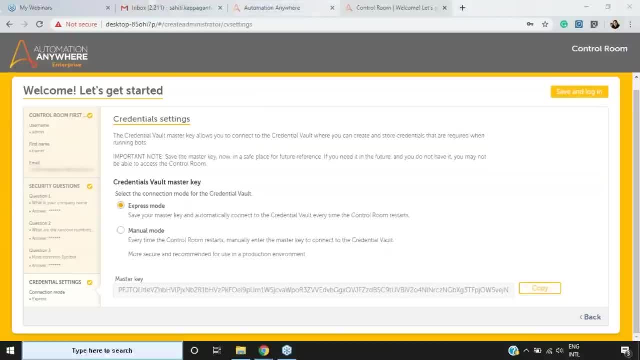 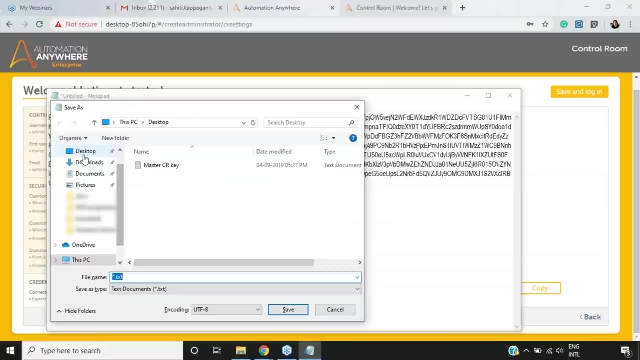 and then I'll just copy this particular master key. and let's say, you know, I open notepad and then I just paste the master key right, and then I'll just save this particular file right. So let's say, you know, 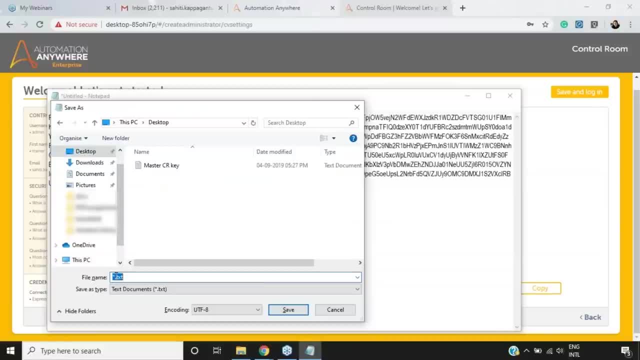 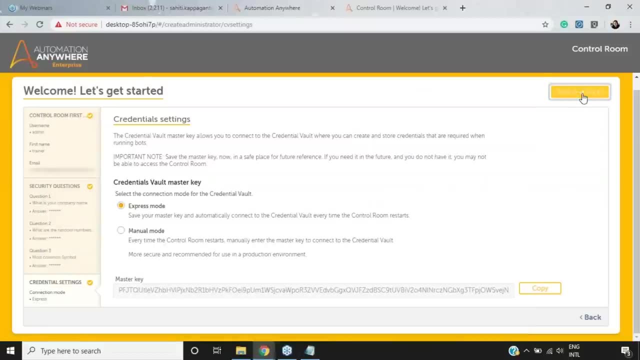 I save this particular file to desktop, and let's mention master right, and then I'll click on save. then what I'm going to do is I'm just going to choose this option of save and login. So I'm just going to log into my control room. 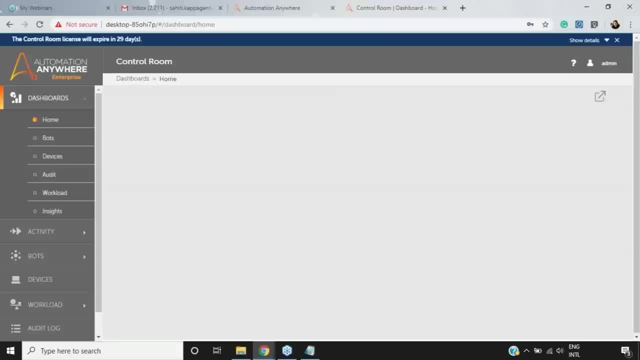 So let's just wait for it to open. Once you log into your control room with the admin credentials, this is basically how your control room looks, where you know you have this option of administration, and in the administration you can go and check your configuration URLs. 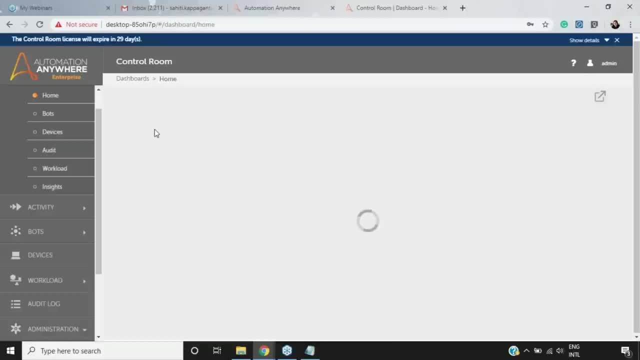 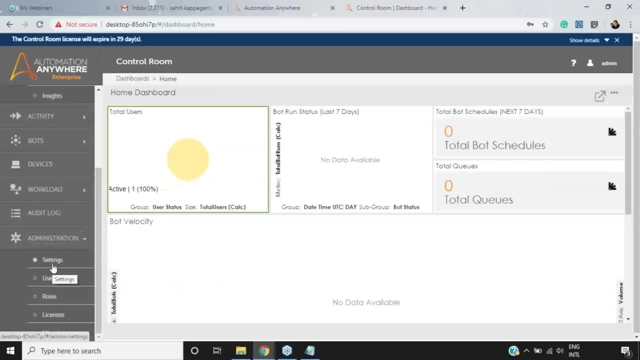 That is basically your control room URLs, right? So let's just wait for that to happen. Let's just wait for it to load, All right, so let's just click on administration now and administration over here. I'll just click on settings. 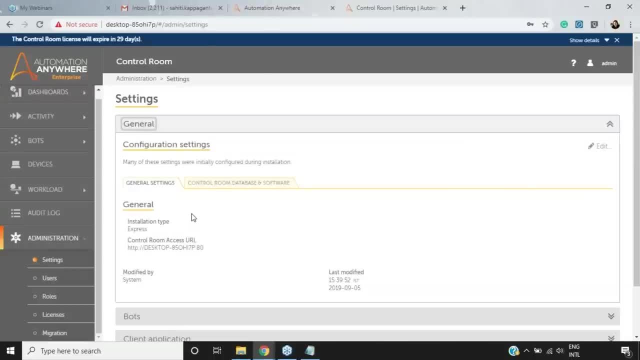 And in settings I'll just choose general and then, if I choose general, you see the general settings that you know. installation type is Express and the control room access URL is basically this particular URL. So, guys, this is basically the URL you have to use. 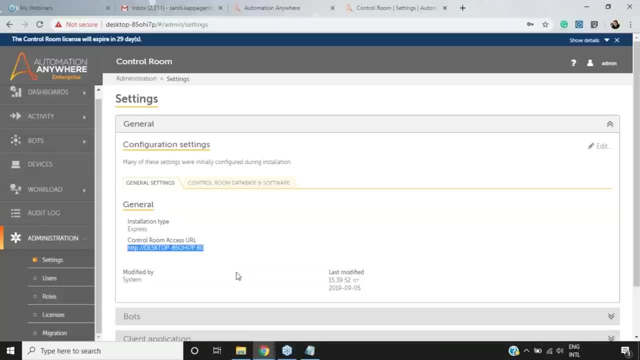 to log into your client Now. before that, I would like to tell you: don't worry if you're confused about the different features in control room. I'll be coming up with one more session on automation anywhere control room, but I'll talk about all these features in depth. until then, 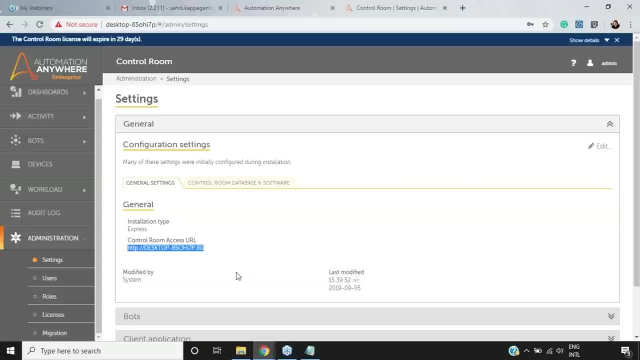 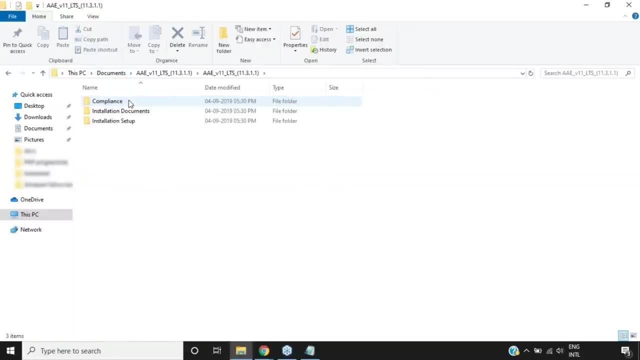 Let's move forward and see how we can set up our client. So we'll go back to our folders and in our folders What I'll do is I'll go back to documents over here and then I'll choose this particular folder. go over here. 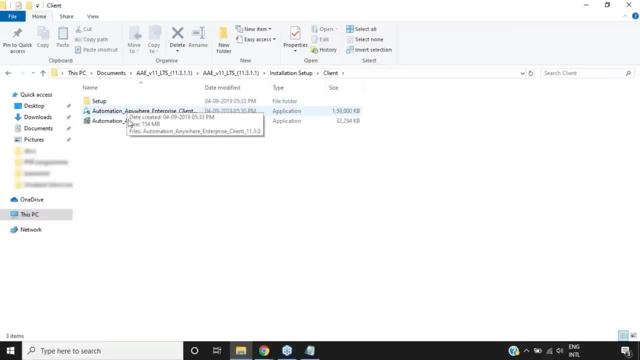 go to installation, setup, go to client and then in the client, I basically have two options, that is, the automation anywhere, Enterprise, client and application, and the second one. So we're going to choose the first one and then I'll just right click over here and choose run as administrator. 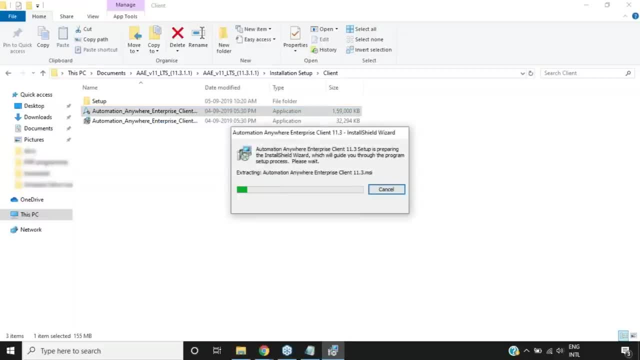 Now, once I choose it to be run as administrator, you see an installation wizard which has started extracting all the files, and then the installation will start soon, right? So let's just wait for that to happen. Now, once the installation begins, you see a welcome. 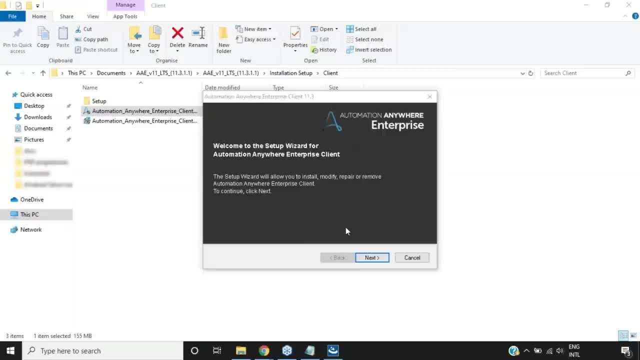 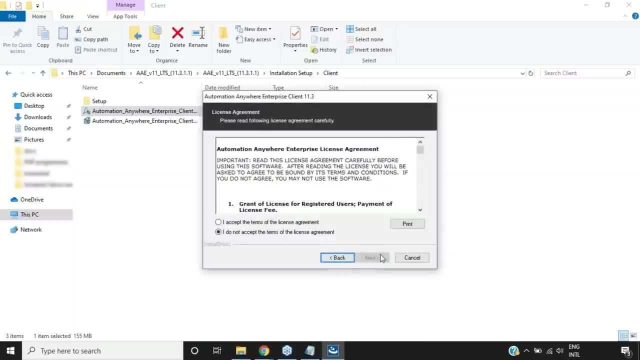 to set up wizard for automation anywhere. Enterprise client. since we want to set up the Enterprise client, What I'll do is I'll click on next. and once I click on next, you see this dialog box of you know license agreement. right, So you can just go forward. 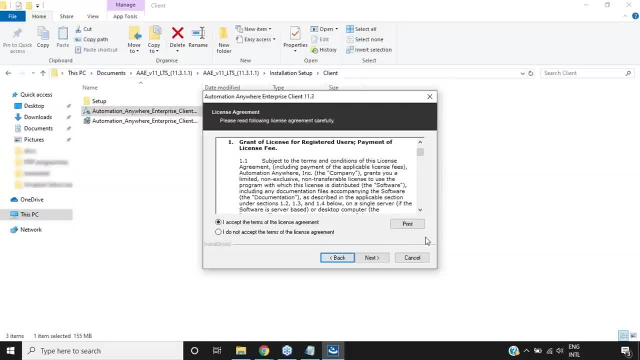 and read the license agreement over here. I'm not going to do. I accept the license agreement radio button and then I'll click on next. once I click on next, you basically have to choose the destination folder to download the Enterprise client. So this is what I've put by default at the C program files. 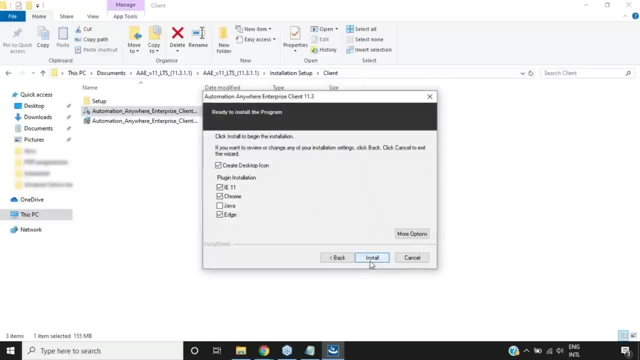 and then automation anywhere and Enterprise, and then I'll just click on next. once I click on next, you see a few options which can be installed. like you know, the desktop icon will be created and the plug-in installation will be for i11, Chrome and Edge. 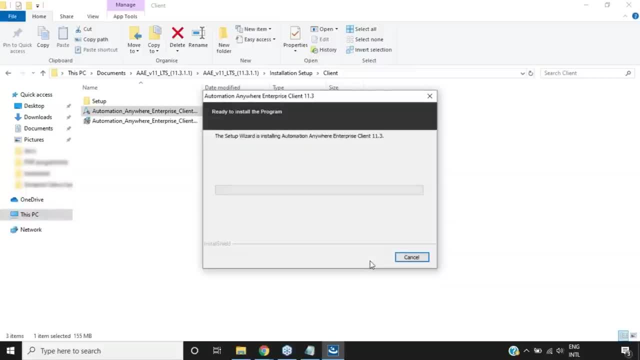 after that I'll just click on install. and once I click on install, you'll see that you know automatically automation anywhere Enterprise client will start getting installed. So let's just wait for that to happen. All right Now. once the installation is done, you see a set of wizard. 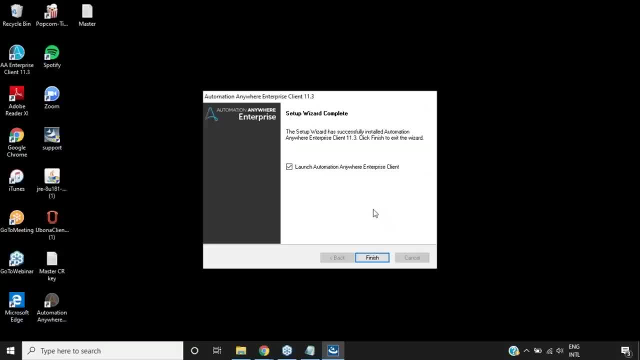 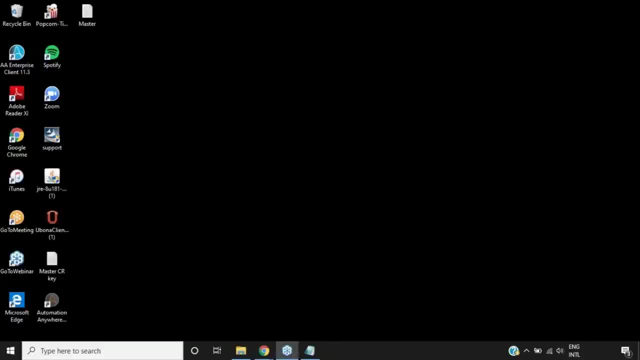 that which says: set of wizard complete and then we can launch automation anywhere. Enterprise client right. So for that you just have to check into this particular radio button and then you click on finish. once you click on finish, You'll automatically see that you know. 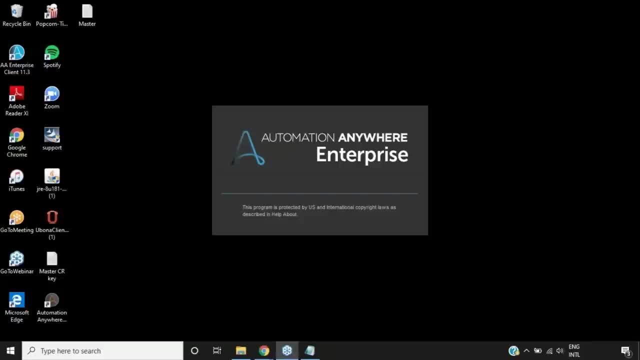 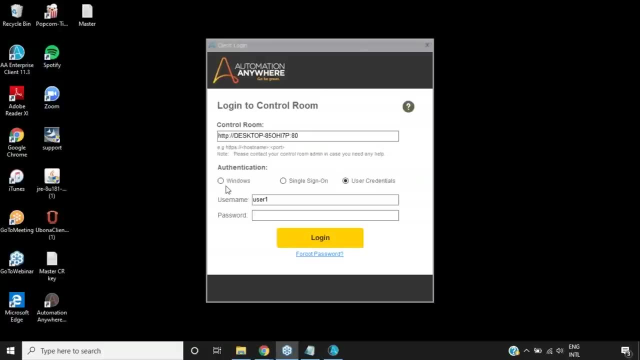 the client will start getting launched right. So let's wait for the client to be launched and then we'll log into the client. Now you can fetch the control room URL from the general settings of the control room, And then what you can do is you can just choose this option. 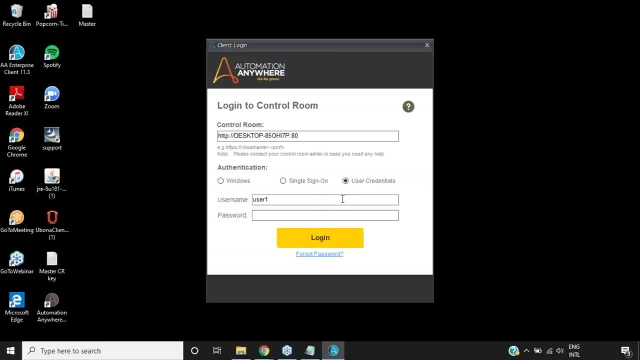 of Windows authentication or user credentials, and then you can mention the username and the password. So what I'm going to do is I'm going to create a user first, right. So for that, what I'll do is I'll go back to my control room. 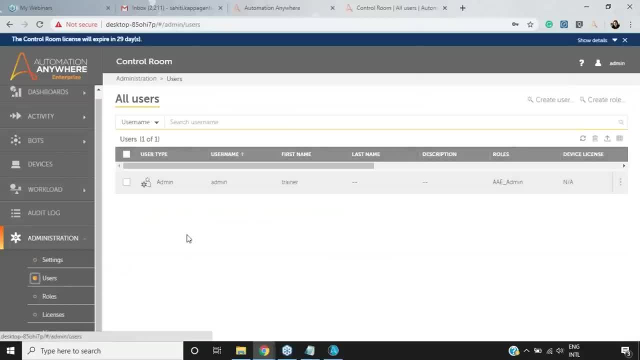 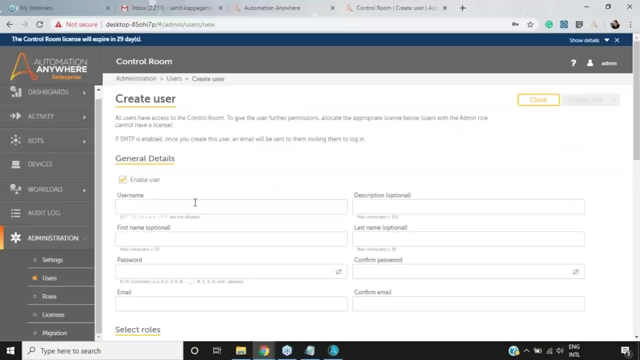 right. And then what I'll do is I'll go to users over here, right in users. What I'm going to do is I'm going to choose this option of create user right, So I'll just click on create user and then I'll mention user one. 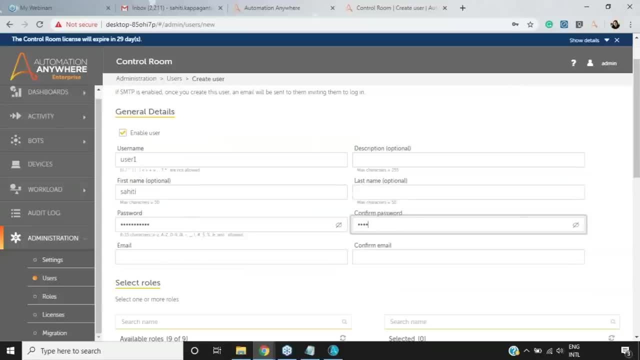 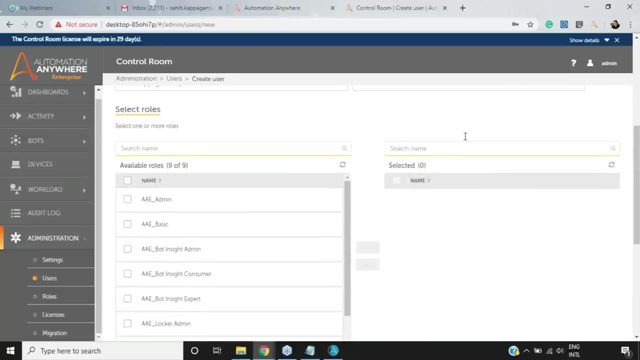 Let's say name to be sahiti, Then I'll mention In the password, and then I'll confirm the password, Right, and then I'll mention email ID, Right, and then what I'll do is I'll just scroll down and over here once you create the user you have. 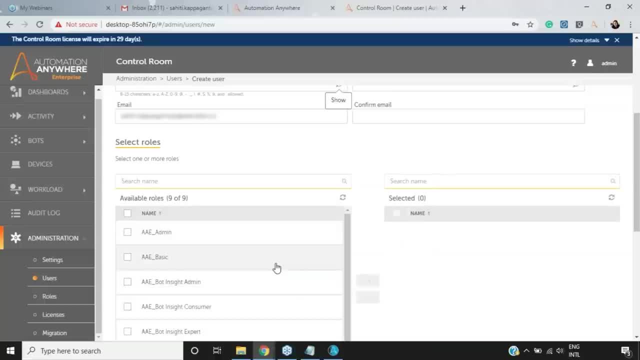 to select a role for the user. So over here what I'm going to do is I'm going to choose this role of a basic and then I'll just add it over here, right? So that means that you know this particular role has been added to this particular user. 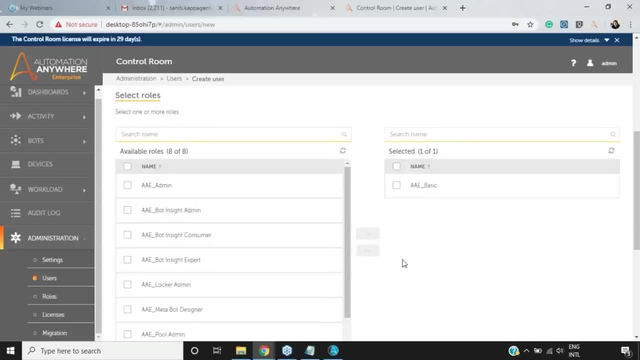 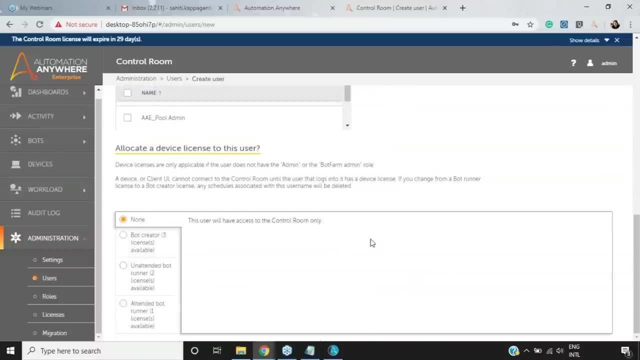 Well, it's not necessary that you know one particular role has to be selected for a user. You can select any number of roles that you want, right? So we are. I'm just selecting one particular role and then what I'll do is I'll go down. 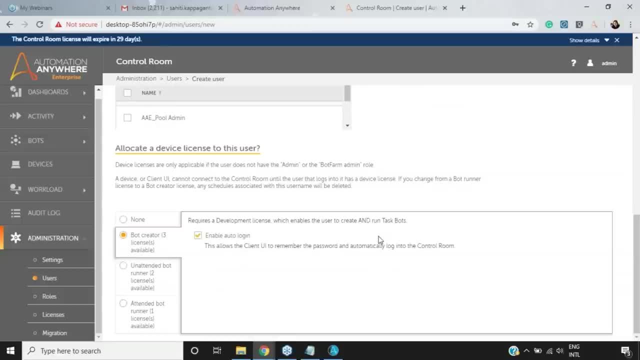 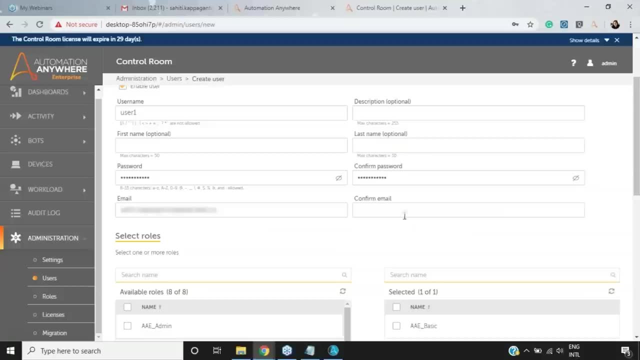 and allocated device license to this particular user. So for now I'm choosing bot creator and then I'll scroll up and then you can just check all the details. So we are. I'd forgot to confirm the email ID, So I'll just confirm the email ID. 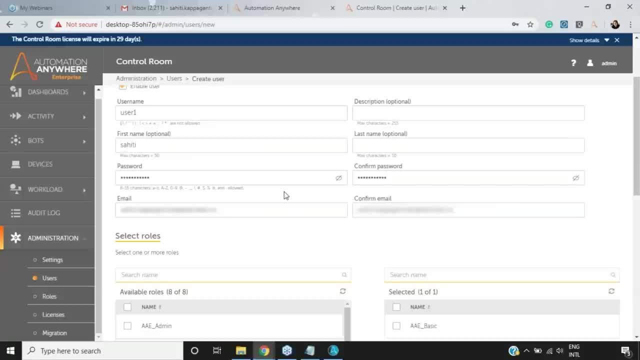 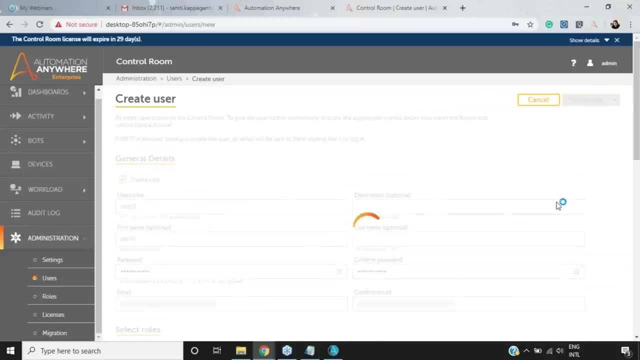 I've mentioned the password, the first name- Let's say sahiti- right, and the username is use one, and the role is a basic and the device licenses bot creator, right. So after that, I'll just click on create user now, since our user has been created. 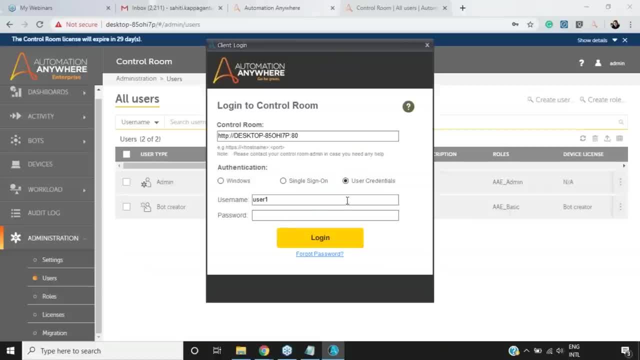 What I'll next do is I'll go back to my client login and I'll choose this option of user credentials and over here and mention username and the password. right now, Once the password is mentioned, I'll just click on login and you'll see that you know. 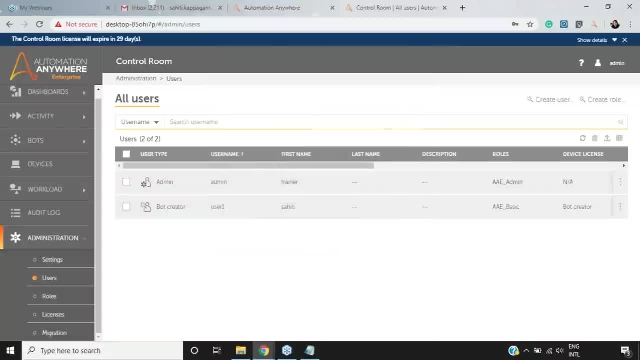 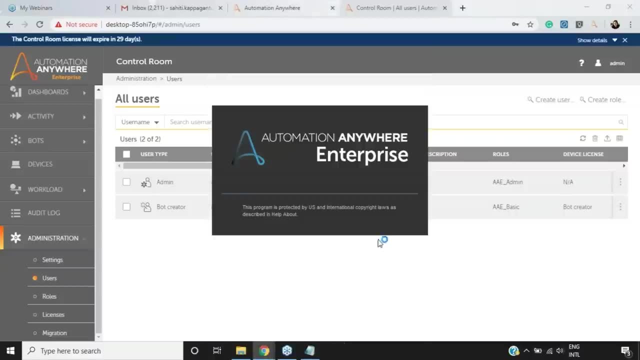 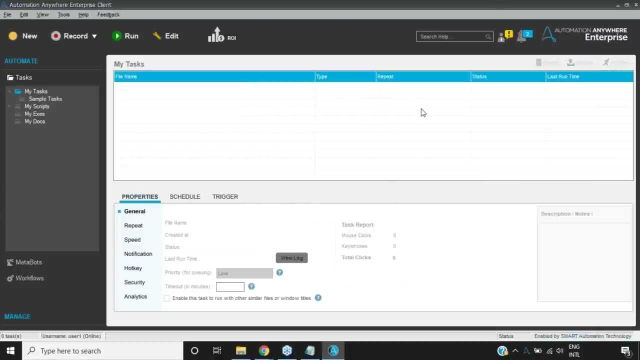 automatically the user with the user credentials, user one- will be logged into our client, right? So let's wait for that to happen, right? So we'll just get started Now. once the user has been logged in, this is basically the dashboard that the user sees. that is basically. 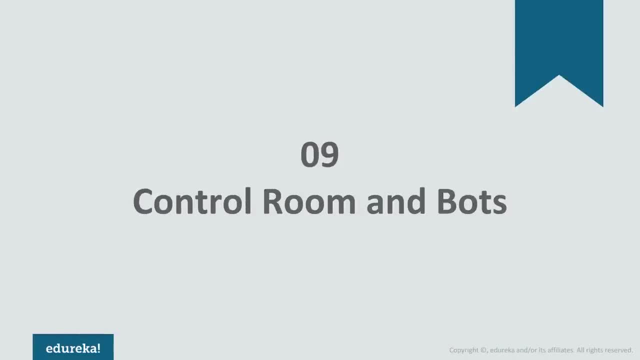 our Automation Anywhere Enterprise client. Since automation has came into existence, various tools have been emerging in the market. Automation Anywhere is one such RPF tool used by the industries to automate ways kinds of tasks. now, Automation Anywhere- control room is like the brain of Automation Anywhere. 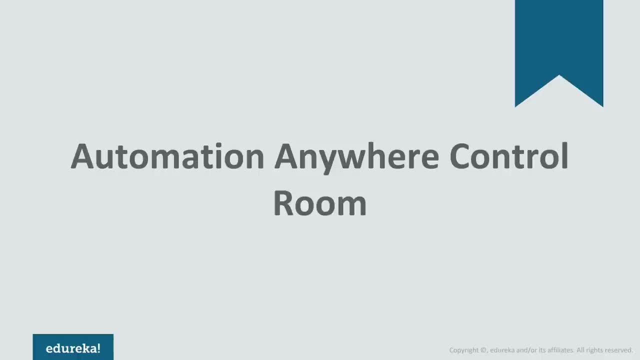 which basically controls everything that is happening with the tool and that is happening with the task. in the session, guys will understand what are the various features and functionalities offered by Automation Anywhere: control room. So before I talk about control room, let me take you through the architecture. 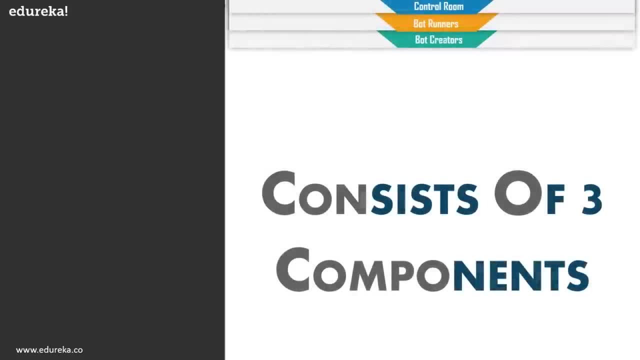 of Automation Anywhere. now, the architecture of Automation Anywhere is basically a distributed architecture. So this architecture basically has three components which work together to help the user to achieve his stars. Those stars are basically bought, creators bought runners and control room itself. Now the bot creators and bot runners are basically connected. 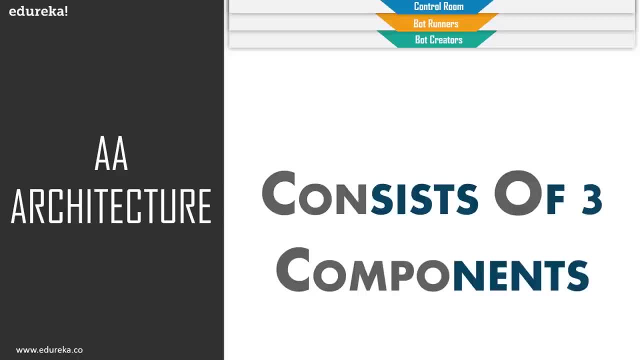 to the control room and the control room is the brain of Automation Anywhere. now, by this you can understand that. you know, control room is the place where everything happens and it is the brain of Automation Anywhere where everything is controlled. So, before I move forward and get into depth of control room, 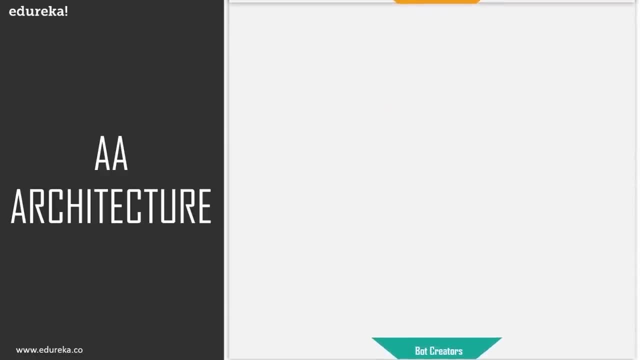 let me just tell you about bot creators and bot runners. Well, bot creators, as the name suggests, are basically used to create bots, So these are basically desktop based applications whose sole role is to upload or download bots and connect them to the control room. now, multiple users can create bots. 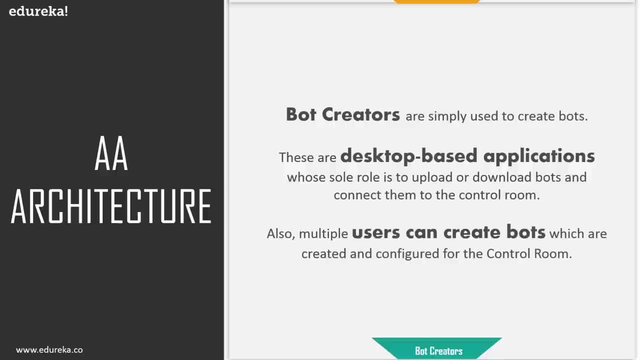 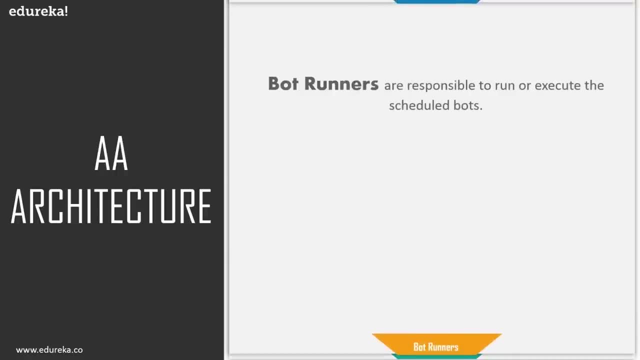 which are created and configured for the control room. So the bot creator is basically used to create the box. now coming to the next component, that is, bot runners. What runners are responsible to run or execute the scheduled bots? so multiple bots can be executed in parallel. 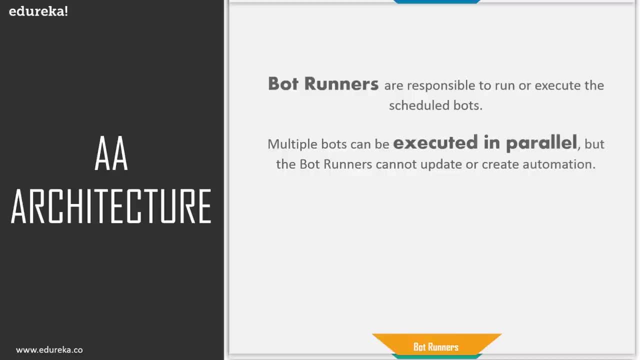 but the bot runners cannot update or create the automation. Now bot runners are also connected to the control room and have the ability to report back the execution log status to the control room. Now, finally, coming to control room. If you ask me what is control room, then control room. 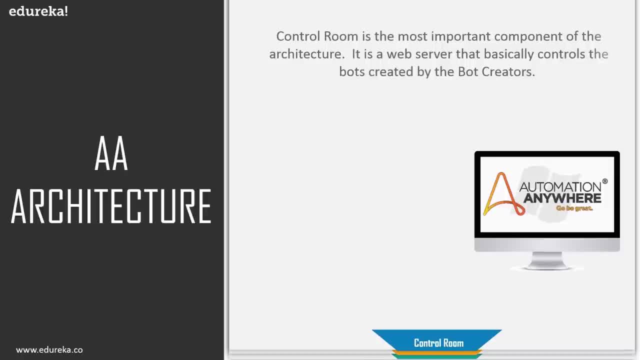 is the most important component of this particular architecture, that is, Automation, Anywhere's architecture. It's basically a web server that controls the bots created by the bot creators and also handles the automation executed by the bot runners. So the control room basically ensure centralized management. 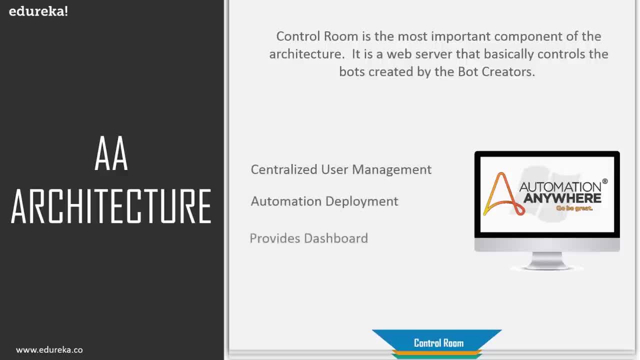 by offering features such as centralized user management, automation, deployment, source control and so on. if I have to give you a summary of control room, then you know control room is basically the brain of Automation Anywhere. it offers centralized user management. It provides a dashboard where you can see different stuff. 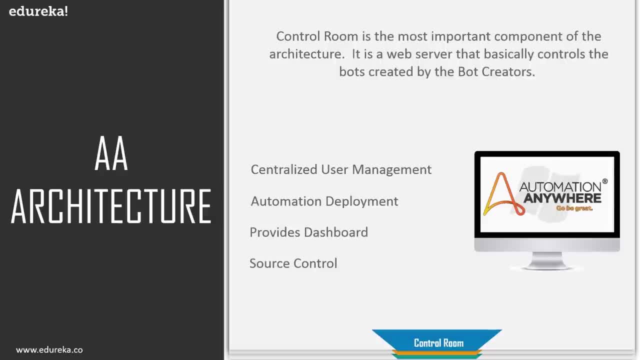 like you know, different analytics stuff and maybe how many bots are running, how many bots are not running, how much CPU is used by a specific board, What is the task happening, Which bot, and so on. apart from that, it manages the bot creators and bot runners and is completely web-based. 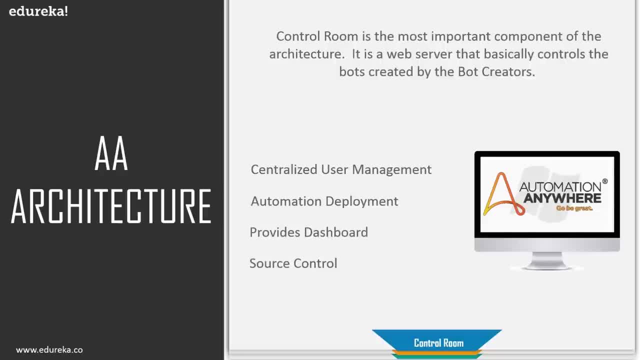 So now, once you have downloaded control room- that is, basically either to the Enterprise Edition or the Community Edition- You have to basically log into your control room. So since I've downloaded control room to the Enterprise Edition, I have this extra option of administration. 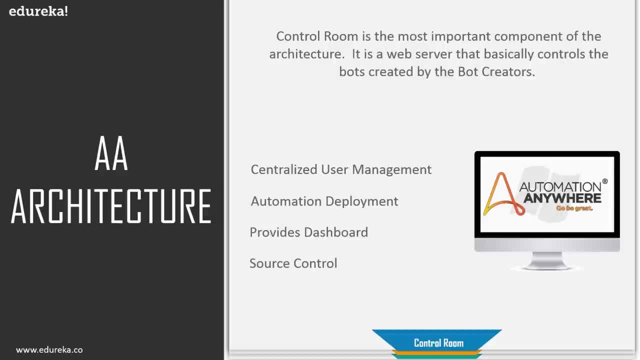 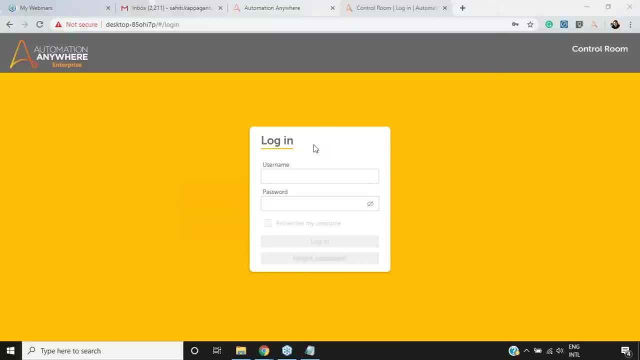 but if you use the Community Edition, you will not find the extra option of administration which you'll see in the dashboard. But before that, let me just log into the control room. So to log into the control room, you'll basically have a URL. 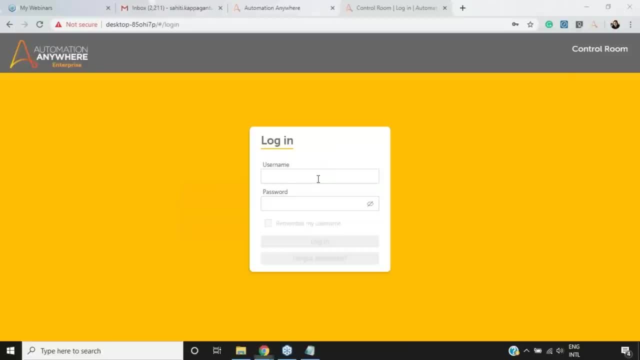 which will be generated when you install control room. So, apart from that, let's just log in over here. So I'll just mention the username and password, Right, and then I'll just click on login. Now, once I click on login, you'll see that, you know, automatically will be logged. 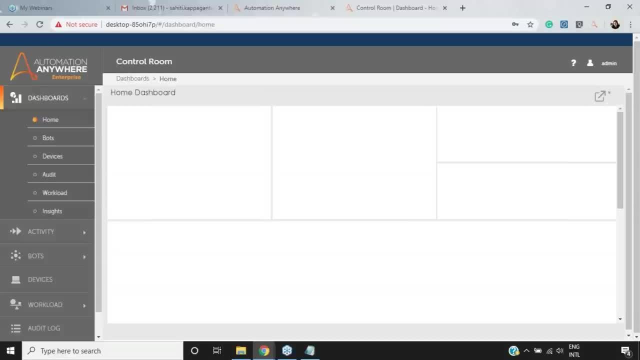 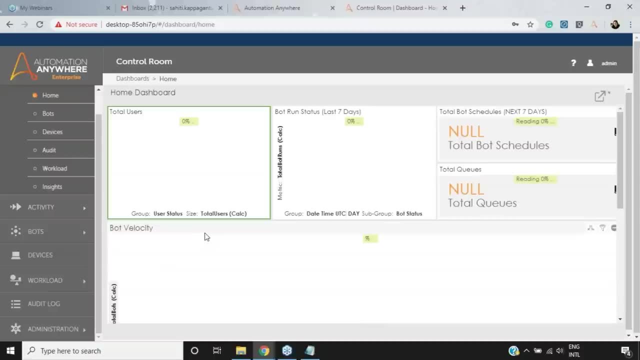 into our control room with the username and the password and once the control room loads, you see various features and functionalities on the left hand side and for the respective feature you have this particular dashboard. So don't worry, We're going to discuss each one of these in depth. 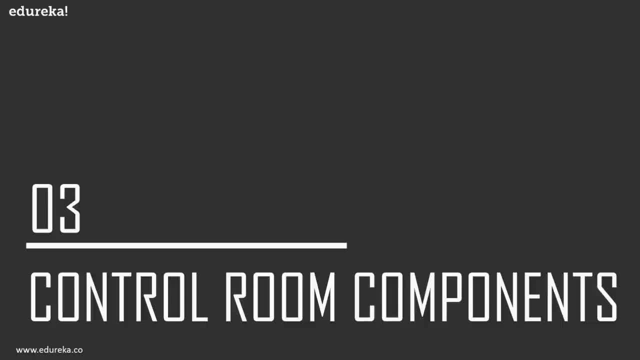 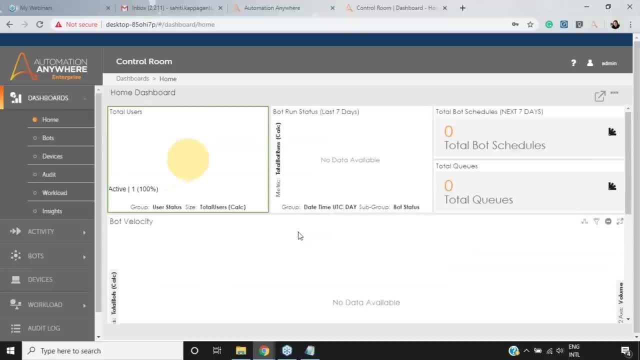 So, on that note, let's get started with the discussion on control room components. So, as I said before, control room offers ways, components like dashboards, activity bots, devices, workload audit log and administration. Now, since I've installed the Enterprise Edition, I have the administration option. else, 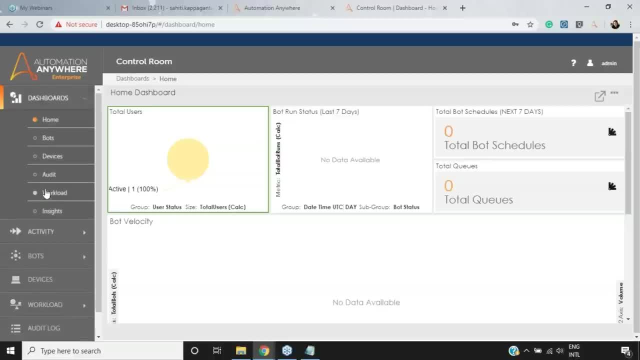 You will not find it in the Community Edition. But before I go to that particular option, let me just click on the dashboards option. So the dashboards feature of the control room is basically a feature which provides stats of various parameters. So it has various features, like you know: home bots, devices. 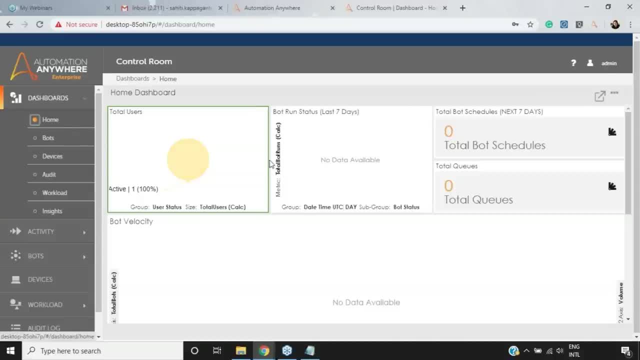 audit log, workloads and insights. So if I click on the home dashboard, you see that you know. the home dashboard shows the user bot run status, the total queues, the total bot schedules, the total users bot velocity and the capacity of bots versus the bot runners. 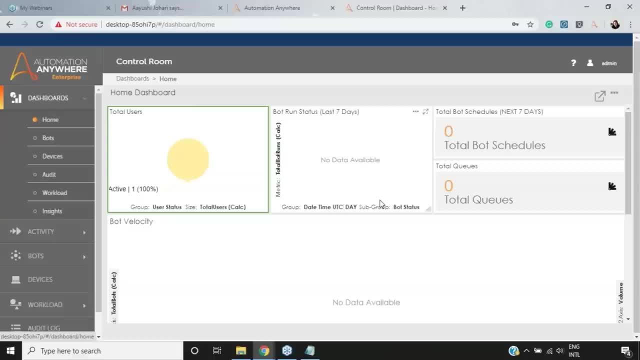 Now, since I have no tasks uploaded on the bots and then you know I have no running tasks present over here, There's no data available. else You'll see that. you know you'll have various options to represent data in various manners. like you know: chart filters, chart styles. 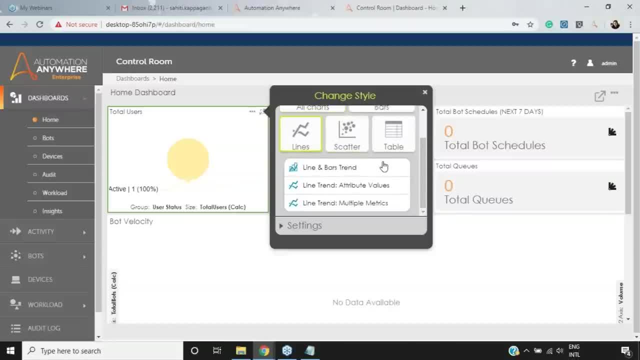 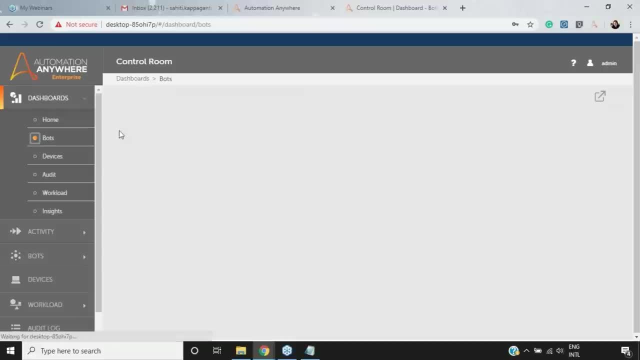 For example, I can choose all charts to be scatter type or maybe line charts. So it's completely our wish how we want to represent the data guys. This is what the home dashboard shows. coming to the bots, one the box dashboard shows the bot heartbeat, MVP bots. 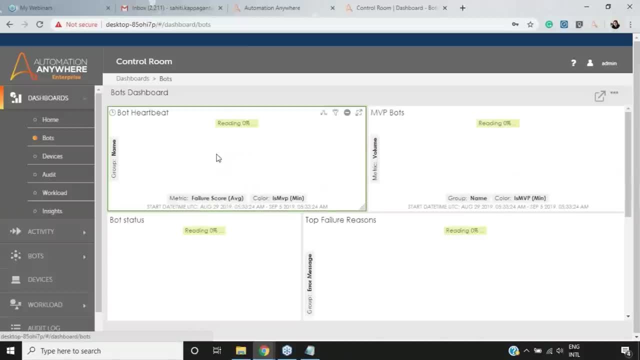 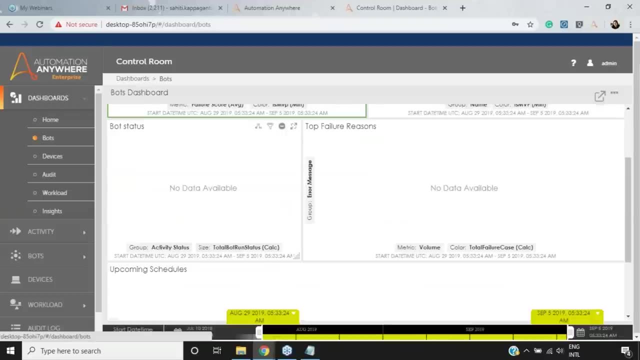 bot status, failure reasons and the upcoming schedules of the bots. So this basically keeps the information of all the bots that are running and maybe are scheduled in future. So you basically get an idea of all the boards deployed. coming to devices for the devices dashboard focuses: 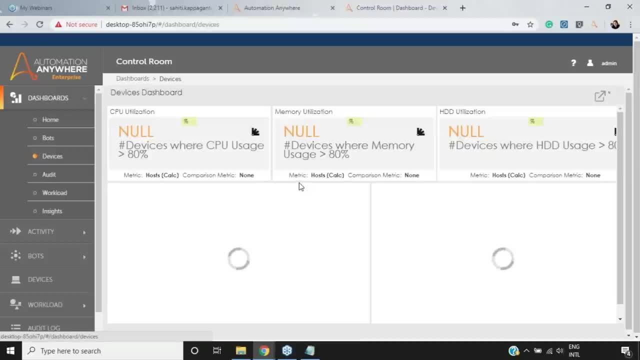 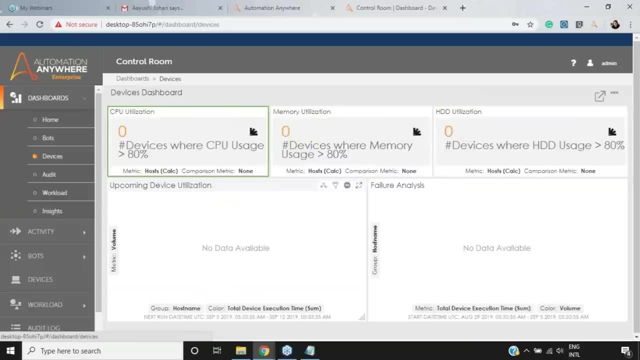 on the hardware utilization, like you know, the CPU utilization, the memory utilization, HDD utilization, upcoming device utilization and failure analysis also right. So, for example, if you upload a task on the bot, now a bot can use, let's say you know- 20% of CPU and maybe for memory. 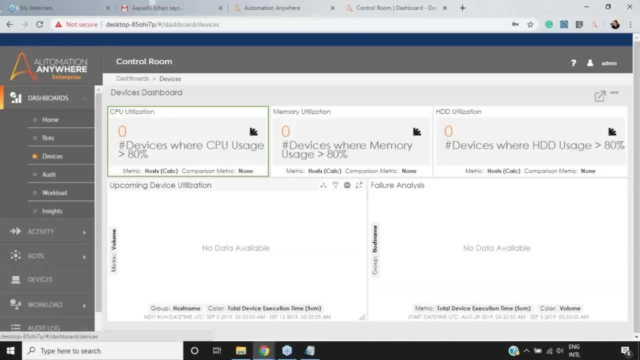 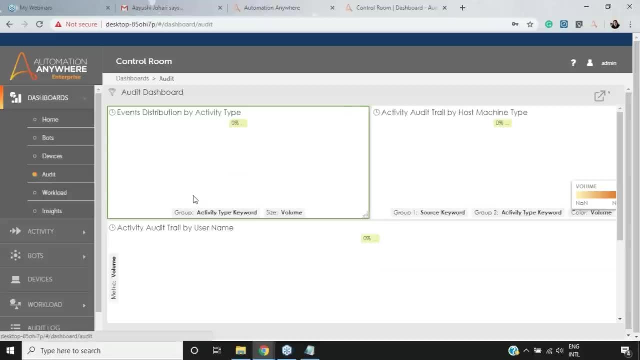 It's just using, you know, 500 MB and so on. So all these details will be present over here. Coming to the next one, that is audit tab, So the audit tab basically keeps a track of all the activities and actions performed by various users. 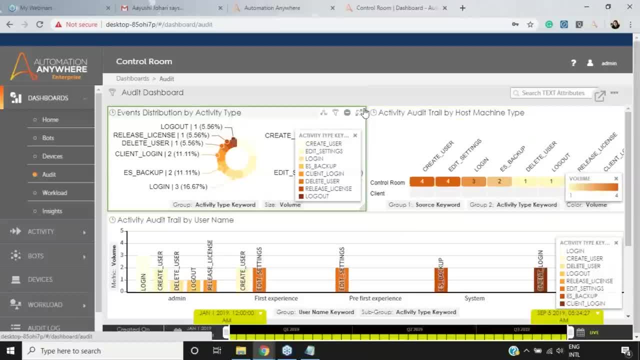 So basically all the different types of actions and the activities are basically tracked over here. So you can just see that you know the audit tab as a log file where you know you have all the actions perform. for example, let's say you know 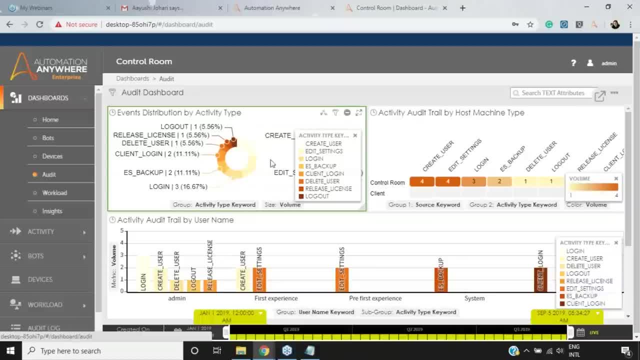 I have the client login over here, the log out, the delete user if we log in again, log out, release license and so on. So over here also you see activity audit trial by the username. For example, you have to check the activities for the username admin right. 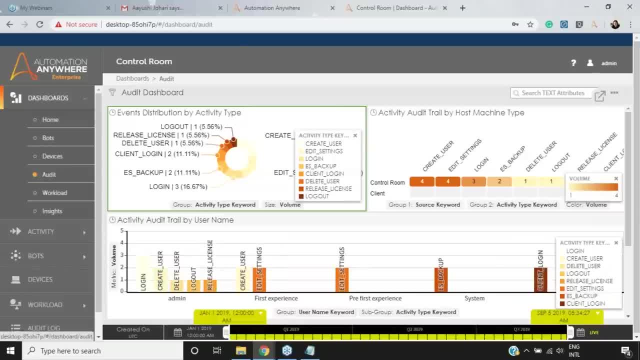 So these are basically the activities performed by the username admin and similarly comes over here that you know we choose the host machine types. So basically, guys, these are various filters that you can use to understand which user is performing which activity on which kind of bots or which kind of host machine. 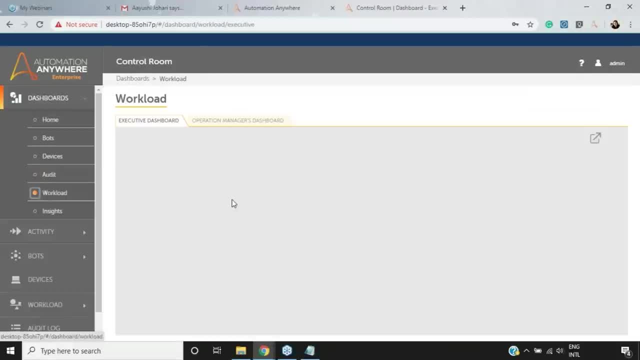 and what are the activities done? now let's move forward with the next dashboard, that is workload. Well, the workload dashboard has basically two tabs, that is, the executive dashboard and the operation managers dashboard. Now, the executive dashboard basically provides visualizations for queue status, queue with average time device. 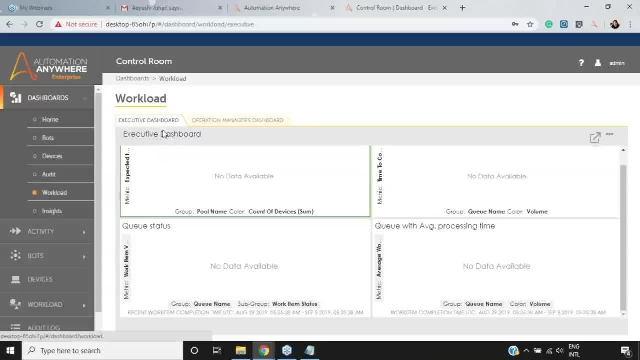 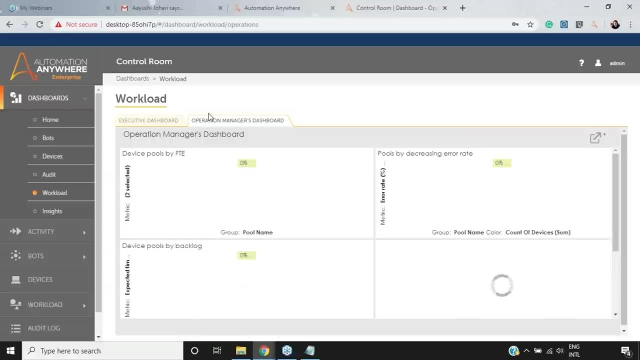 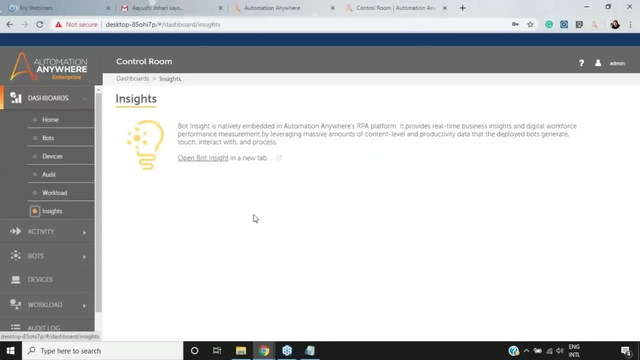 pulls by backlogs and queues by time to complete. coming to operation managers dashboard, the operation managers dashboard provides visualizations for device pulls by FTE pools by decreasing error rate, queues with average times, device pools with backlogs and so on. coming to the next one, that is inside. well, the bot inside basically focuses. 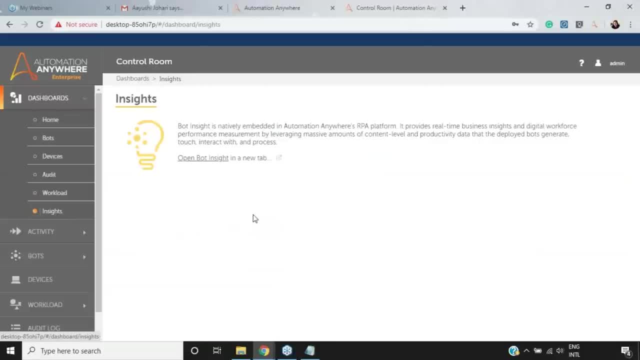 on providing real-time business insights and the digital workforce. So this is something that I'm not going to touch presently over here because this session is on control room. but you can just understand that. you know bought inside is basically embedded in Automation Anywhere's RPA platform. 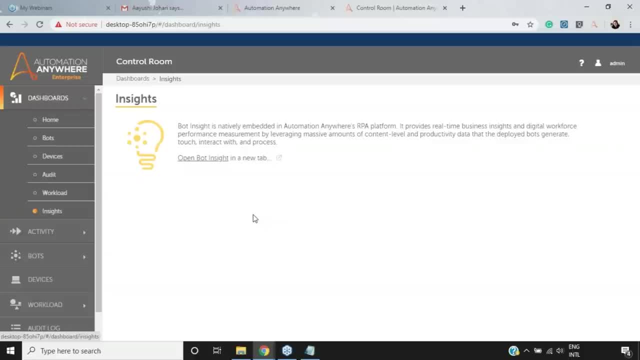 and it aims to provide real-time business units and digital workforce performance to make sure that you know the user understands what is happening in the box and then what kind of data has been read, and then the deployed bots can work in a better way. So that was about the dashboards tab guys. 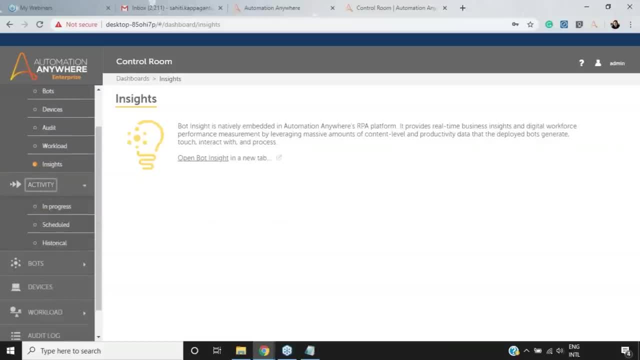 Now let's move forward with the next one, the activity step. Well, the activity feature of the control room dashboard is mainly used to check the history and the progress of the scheduled activities, So it basically again has three tabs. that is the in progress scheduled. 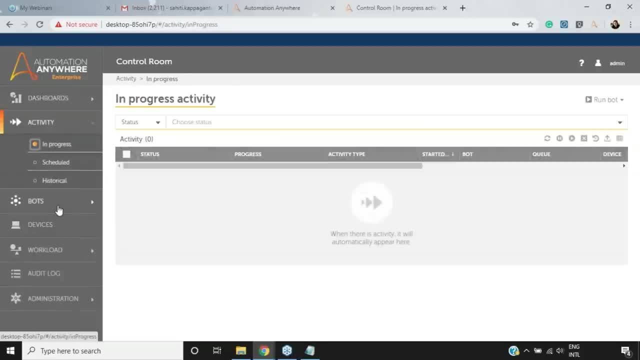 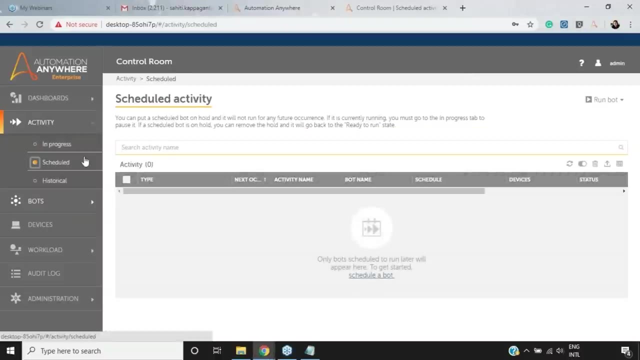 and the historical. coming to the in progress one: the in progress activity tab is used to check the status of the activity which is currently executing, so it gives all the details related to the activity, such as the username, the bot name, the item name and the progress. coming to schedule tab: the schedule activity. 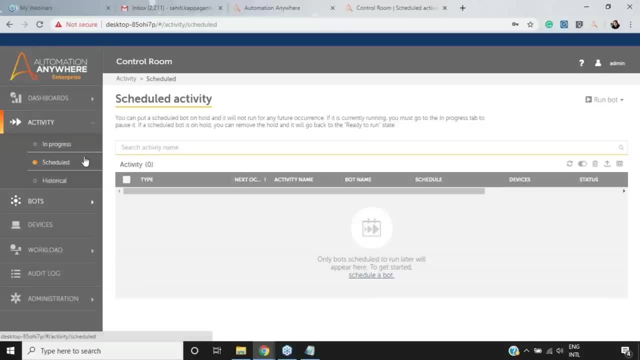 tab is used to check all the details of the activity which is scheduled to execute sometime later. So it basically gives all the details related to the activity, such as username, bot name, item and so on. now, similarly, coming to historical, the historical activity tab is used to check the details of the activity. 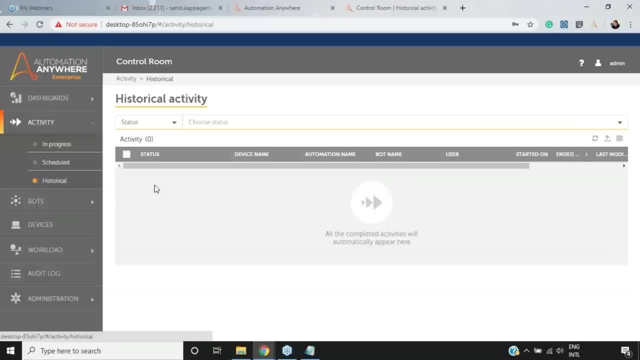 which might have been completed, finished, stopped or timed out. It basically gives details related to the device name, automation name, bot name, user and so on. so basically, guys, the activity tab is used to check the history and the progress of the scheduled activities. Now let's move forward with the next feature, that is, the bots. 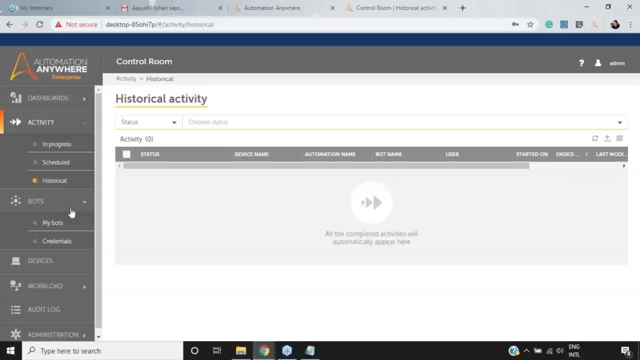 So the bots feature of the control room dashboard is used to see the details of the task created and uploaded. So it gives the details such as the task name, credentials, client name and so on. So it again has two options under it, That is, the my bot section and the credentials section. 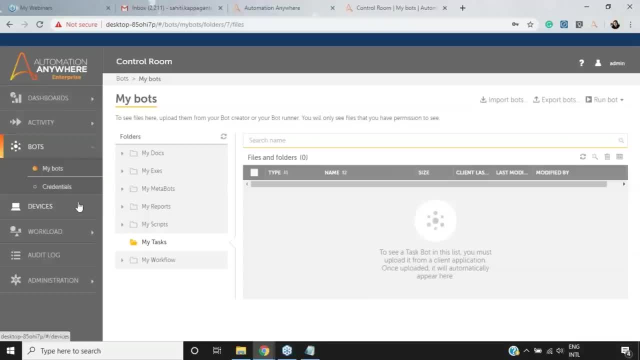 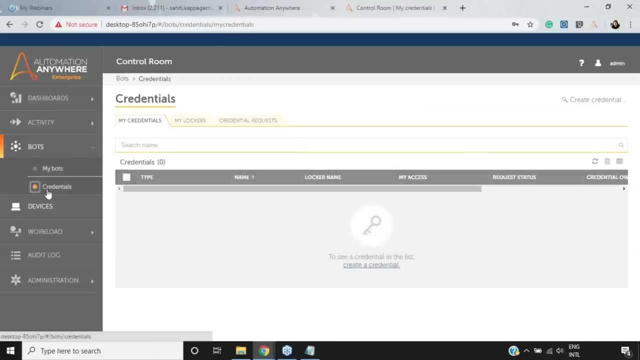 So the my bot section basically has all the tasks and its details, such as unit name, client size and so on. coming to credentials, the credential tab basically displays the credentials, the lockers and the credentials request. So basically all the credentials that are used or maybe, if you want to set a credential into the list. 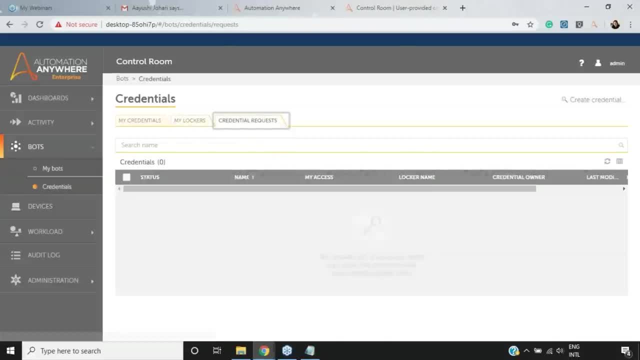 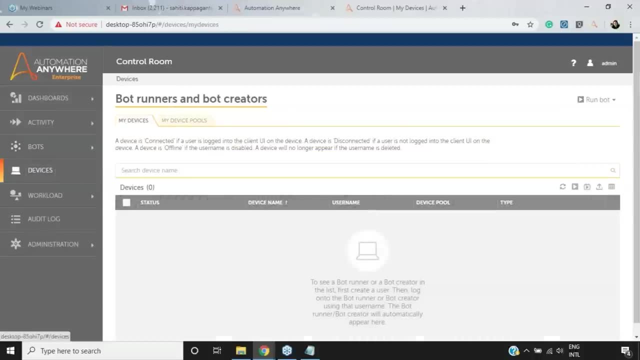 and maybe, if you want to, you know, create a locker and then you want to put on a credential request. You can go forward and do it over here. moving on to the next feature, that is, devices, for the device feature basically displays whether a user is logged. 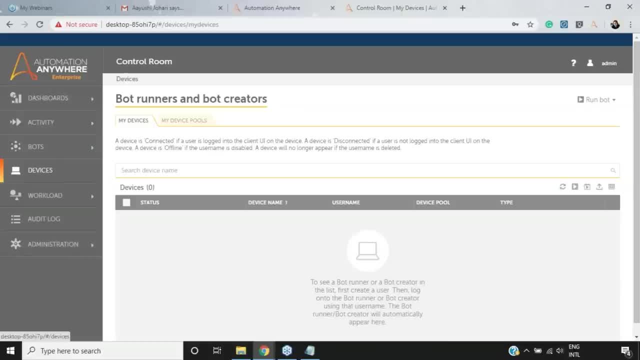 into the client UI on the device or not. So if the username is disabled in, the device is offline, and if the user is deleted, then the device name will no longer appear. so don't worry about it. I'm going to show you when I do the hands-on part. 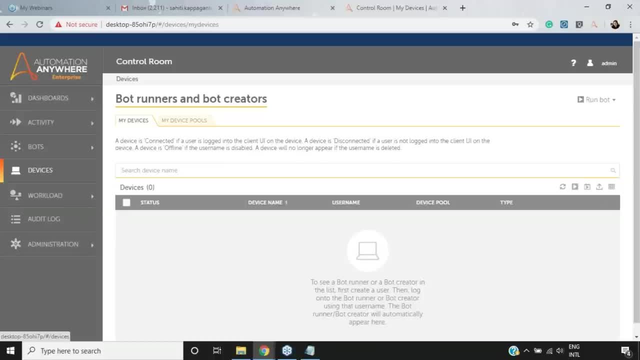 So when we log into the client you are, you'll automatically see that the username is enabled and then you know, the user will be shown online. else, you know, the username will be disabled and the device will be shown offline. apart from this, the devices tab also has the my device pool section. 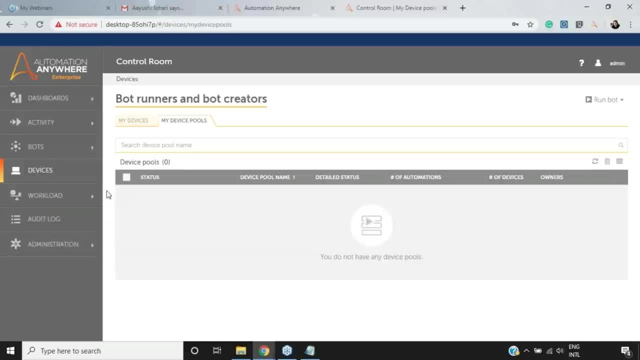 where you can have a set of- you know- device pools to perform any kind of tasks. now coming to the next feature, that is, workload. Well, the workload feature of the control room dashboard displays the load of queues by displaying details such as queue name, automation name, automation status. 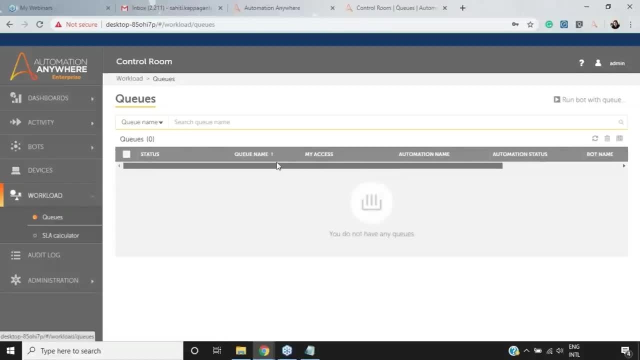 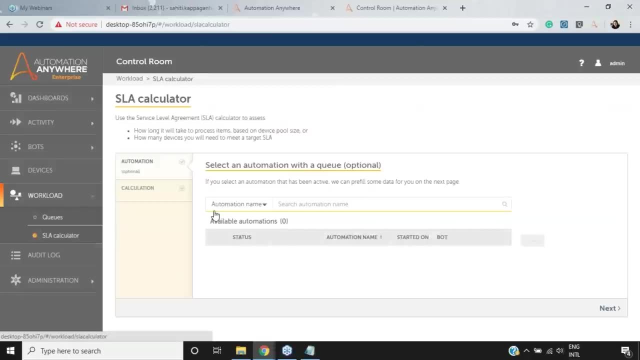 what name and so on. So if I click on Q, you'll see various parameters that can be mentioned for queues, like you know: Q name, my access, automation name, automation status and so on. and coming to SLA calculated, This is basically used to SS. 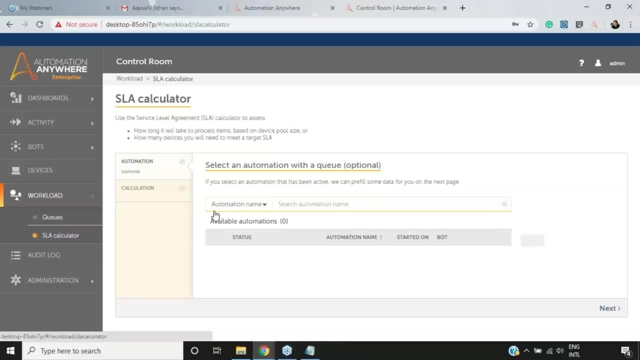 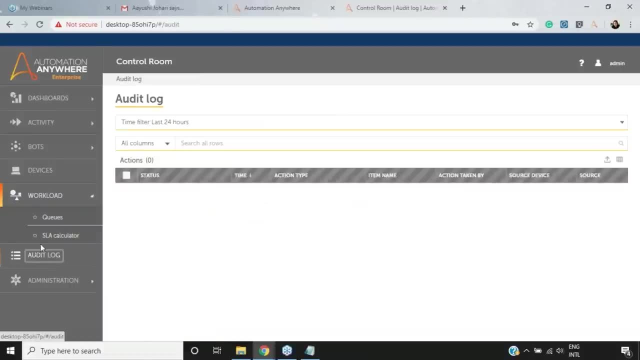 How long will it take to process items based on the device pool size or how many devices are required to meet the target SLA right? So this is basically used to calculate that, and after that we have audit log. Well, the audit log feature is again used to keep a track. 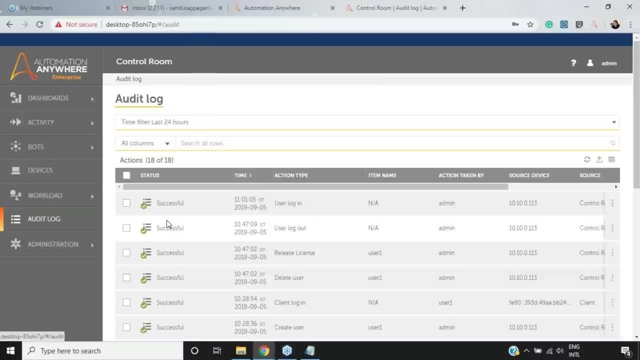 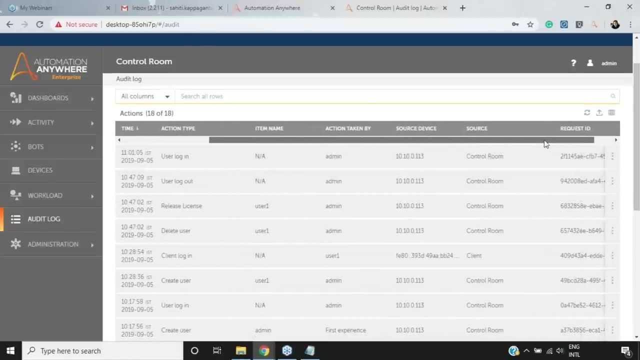 of all the actions performed by various users. So basically, you know over here, you see that, you know the user has logged in, the logged out, and then you see action taken by which user on which device and what is the request ID and then what was the status, right? 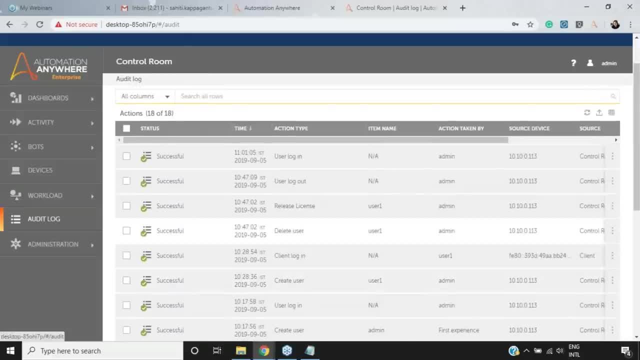 So in the audit tab of the home dashboard you saw that. you know, basically all these actions were shown in a pictorial format, or maybe all were visualize, and over here you see it in a table format. Now, after that comes the last option, that is, the administration tab and our administration tab. 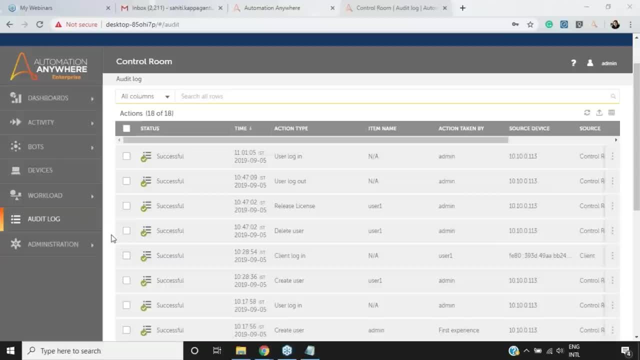 is only seen when you have installed your control room using the Enterprise Edition. So since I've installed using Enterprise Edition, I've got this administration tab. So if I click on this administration tab, you see ways, options, like you know: settings, users, roles. 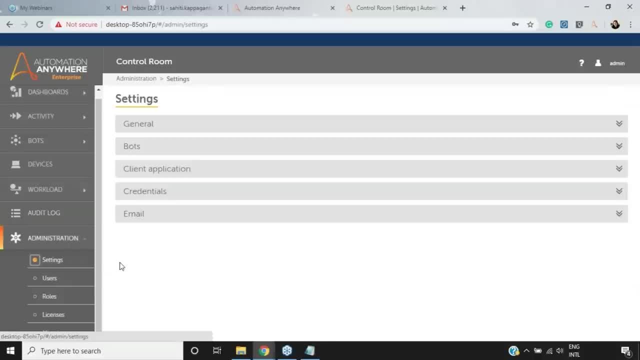 licenses and migration. So talking about each one of them one by one, Well, the settings tab basically provides the configuration settings of control rooms, such as the database configurations, the board configurations, the client application settings, credentials and the email notifications. So if I just click over here, 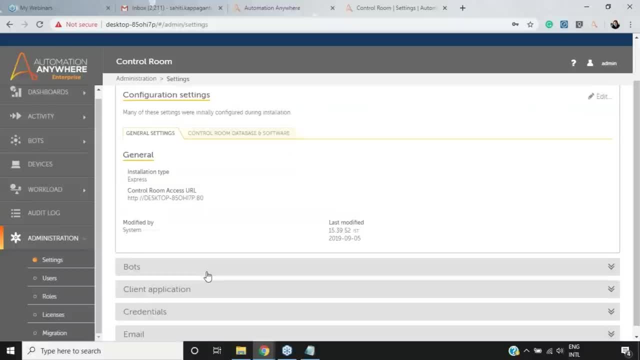 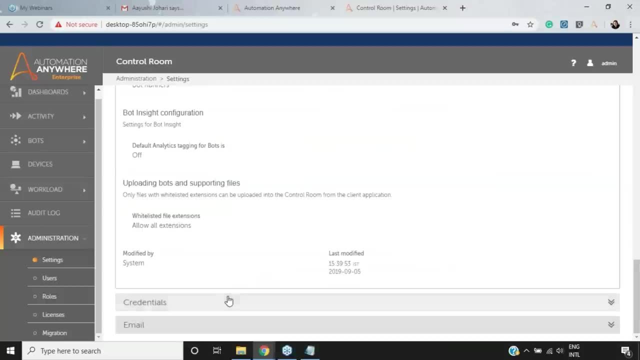 you can see that my general installation type is Express. This is my URL. the bots are nothing at present. The client application has been installed and then you know all the URLs are present over here. Similarly, coming to credentials, I've mentioned the master key, that installation type. 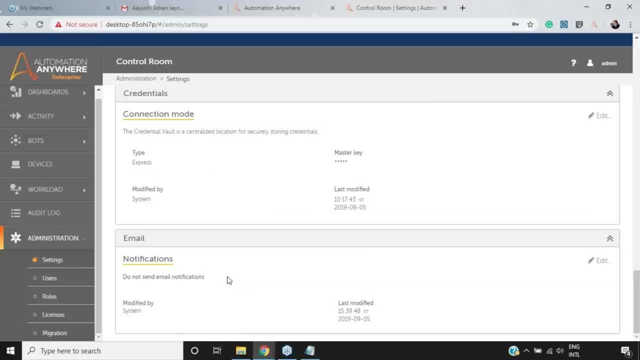 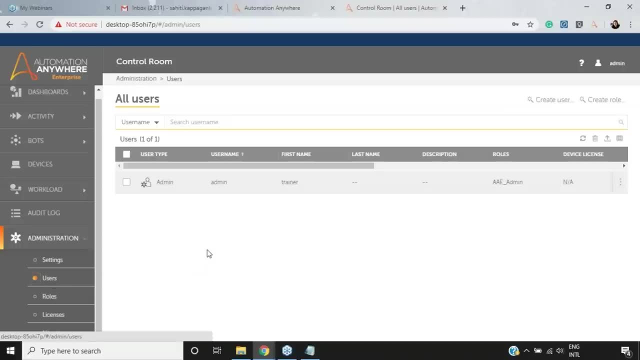 to express and the email IDs to send any notifications if this something happening. now, coming to users, Well, users tab is basically used to create users with various roles. I'm going to do that in the hands-on part, Don't worry. moving on to roles, roles tab again shows a list. 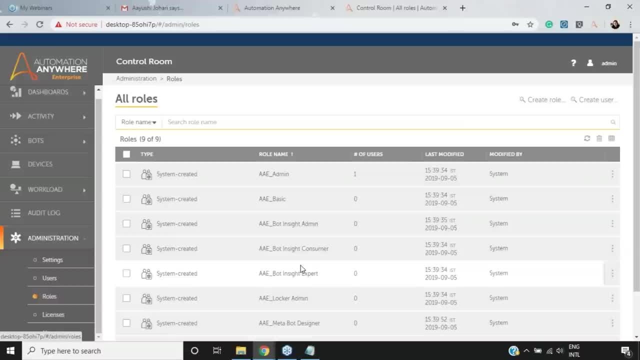 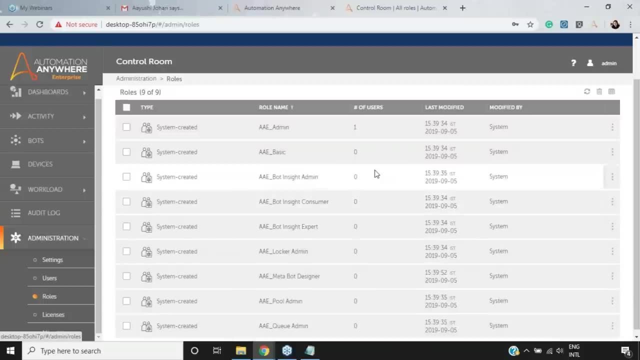 of all the predefined roles or you can also create a role for yourself, right? So you can either create a role or you can use the predefined roles and then shows you know what role name can be used and how many users are using that particular role. 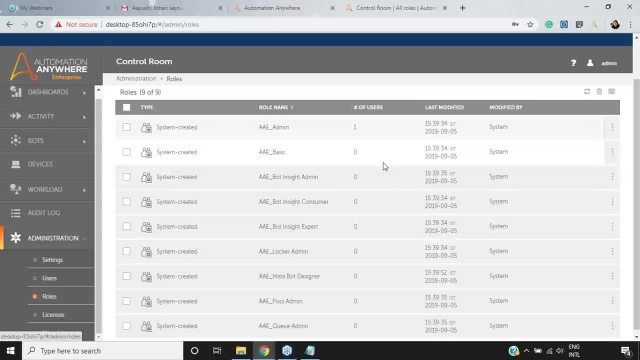 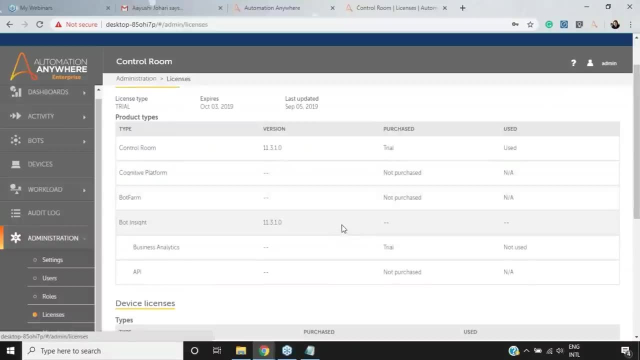 For example, let's say, a admin is used by one of the users, that is the admin itself. now coming to licenses: licenses basically shows a list of product and device licenses. It also shows which licenses are purchased and whether they used to not, for example, let's say, over here. 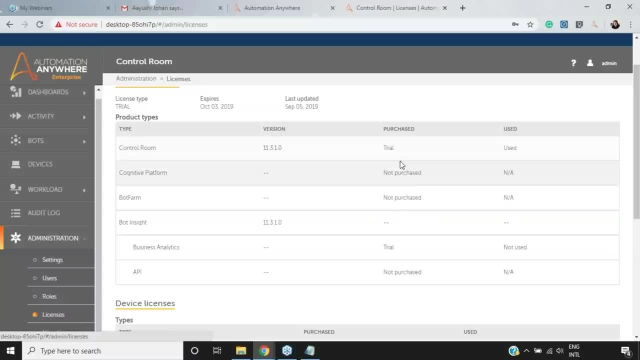 You can see that in a control room, version 11.3.. One is being purchased for trial version and is being used. cognitive is not purchased. What farm is not purchased? bottom side is present for 11.3.. One version- business analytics- is purchased. 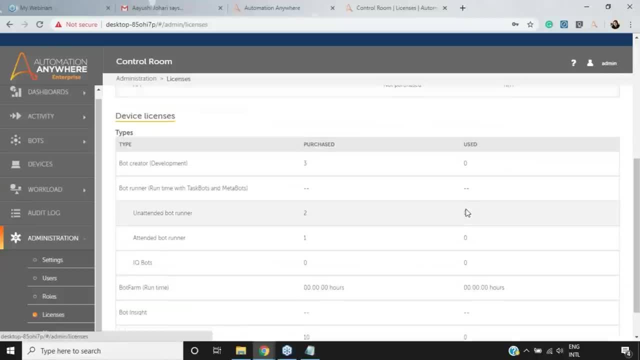 and then you know I've not used it yet. Api is not purchased. similarly, coming to device licenses, You can see that you know the bot creator, the unattended bot runner, attended bot runner, and so on. licenses have been purchased, But yet have not used them yet. now moving on. 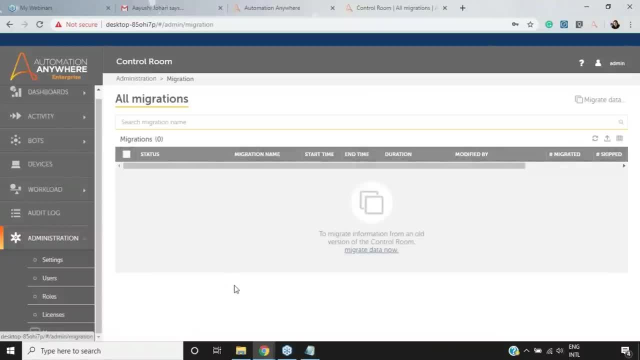 to the last section, that is, migration, with the migration tab is basically used to migrate information from an old version of the control room to the new version. So, guys, that was about various features and functionalities of control room. I hope you've understood. What are the different features offered by control room? 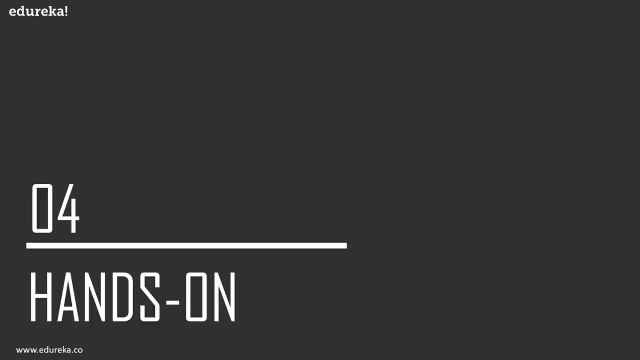 and how you can use it. Now let's move on to the hands-on part, where I'll show you how you can upload a bot on the control room. So to do that, what you have to do is you have to create a user. you have to assign the user with the roles. 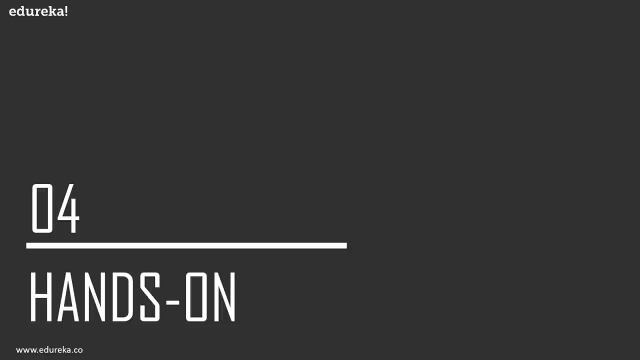 and then you have to allocate a license to the user. after that, you have to log into Automation Anywhere client with the user details, and then you have to choose a task which has to be uploaded. So that's what I'm going to do. So now let's get started with the hands-on part. 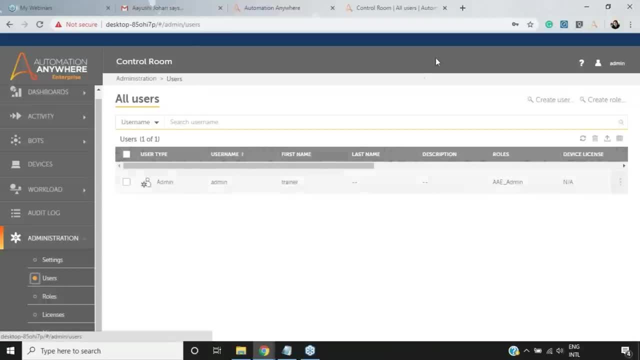 So, to start with the hands-on part, what I'm going to do is I'm going to first create a user, So I'll go to the users tab, and then what I'll do is I'll choose this option of create a user after that. 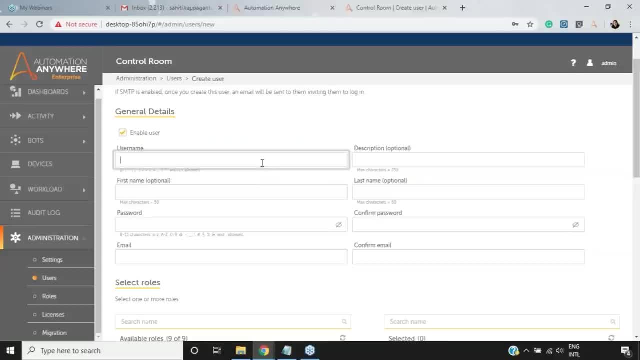 I'll just mention the username, description and so on. Let's say I mentioned username to be user, one description to be sample user. first name: Let's say I mentioned my name, Let me mention my last name, also password, And then I'll confirm my password. 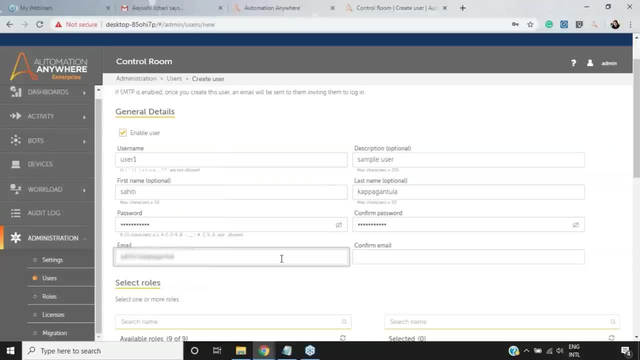 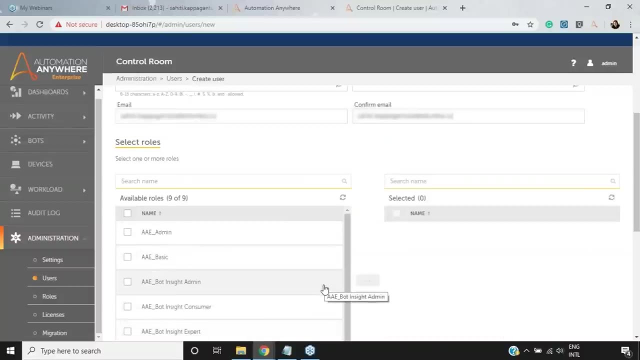 Then I'll mention my email ID Right and then again I'll just confirm my email ID Right. after that I'll just select the rule. So over here you have various roles, like you know: admin, basic, bottom side, bottom side, consumer, and so on. 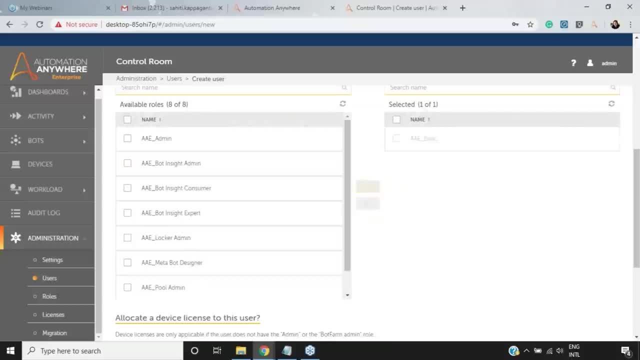 Right. So what I'm going to do is I'm going to just choose this a basic role, and then I'll just click on this arrow. Once I click on this arrow, you'll see that you know this particular role has been selected for this particular user. 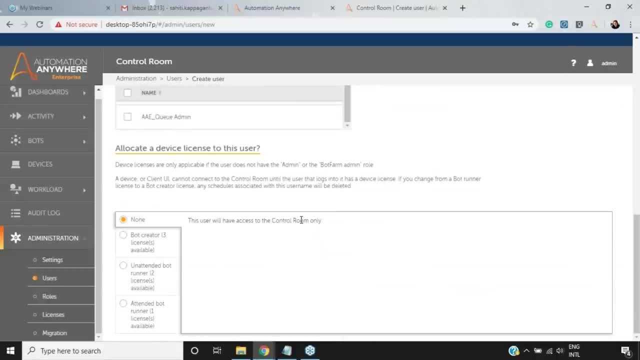 Now what I'll do is I'll scroll down and then I'll allocate a device license to this particular user. So, since you want to upload a bot, what I'll do is I'll just choose this option of pod creator. We basically have three bots. 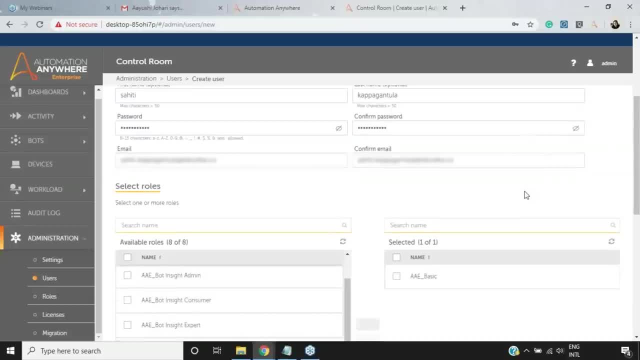 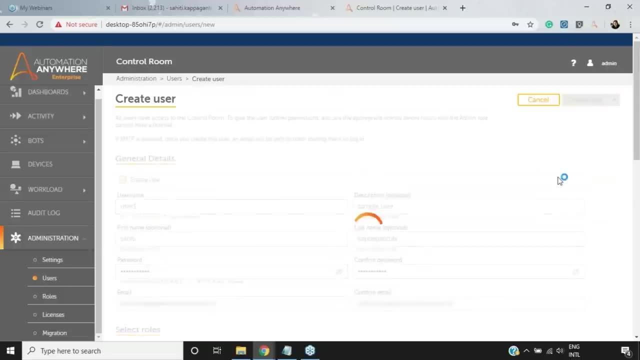 and then we can upload one of them right now, once all the details are mentioned. so you can just go forward and just check the details, and once you think all the details of mine, I'll go forward and click on create user Now. once the user has been created, you automatically see. 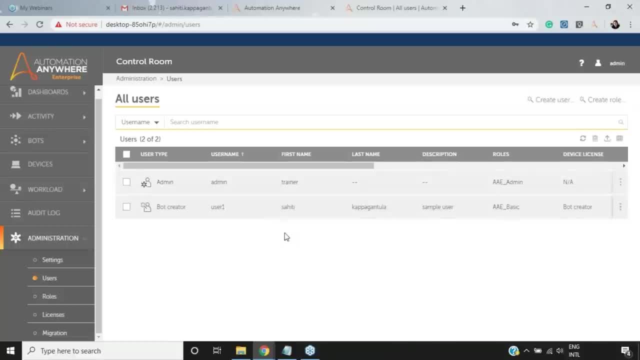 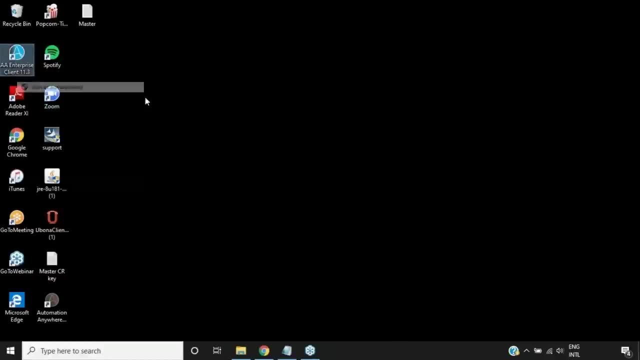 that you know, the user, one with username- first name, last name and so on- has come into the users list. Now, after that, what I'm going to do is I'm going to log into my automation anywhere- Enterprise client, So I'll run as administrator. 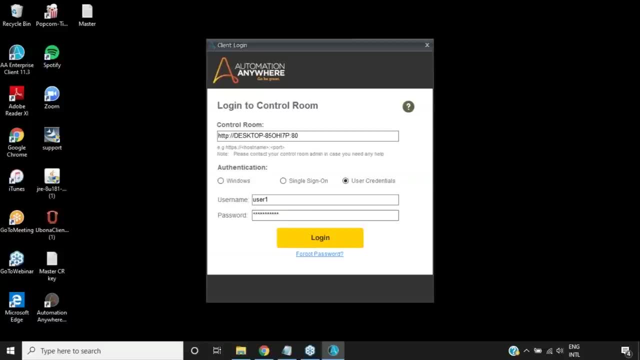 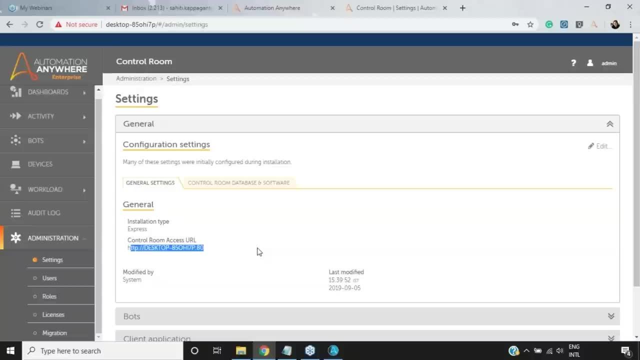 And then I'll mention the username and the password. So let me just mention the username and the password and then you can just check the control room URL from the settings tab of the administration tab. So we are. this is basically a control room URL. 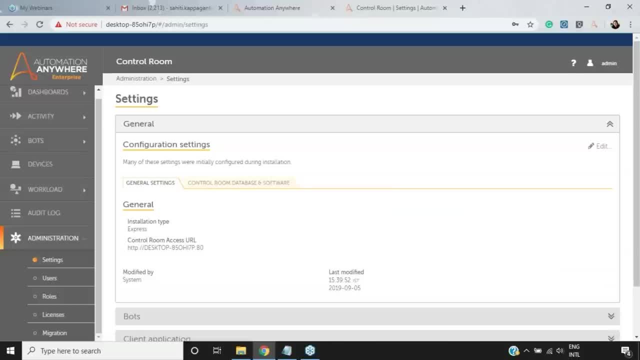 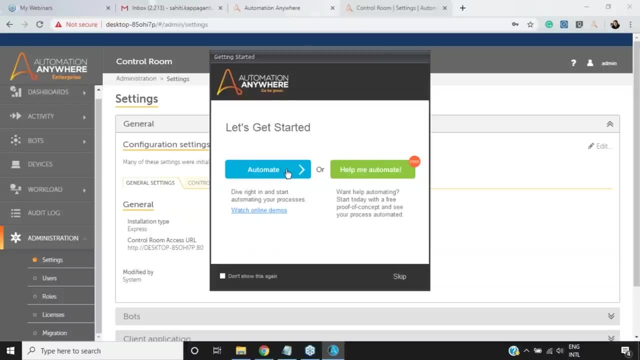 So you can just check that and then you can click on login Now, once the user logs in. what we can just do is we can just click on this option of let's get started and then we can choose this option of automate. now, once the Enterprise client opens up. what we can do is we can 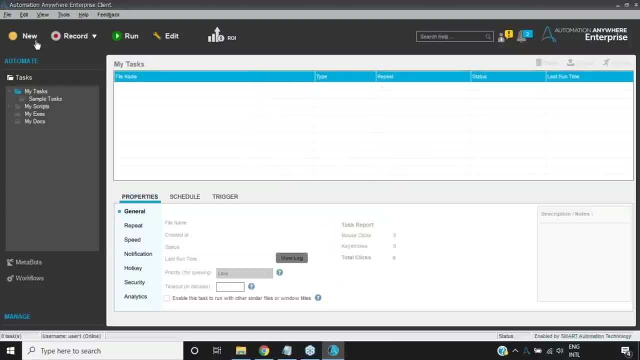 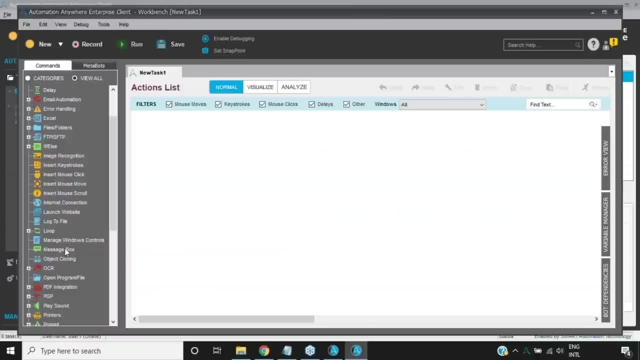 just create a task and then we can upload the task. So, to create a task, what we can do is I'll just click on new and let's say I'll choose workbench, And then let's say: you know, I create a task. 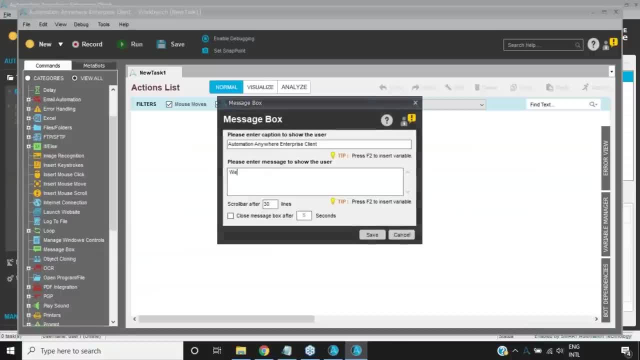 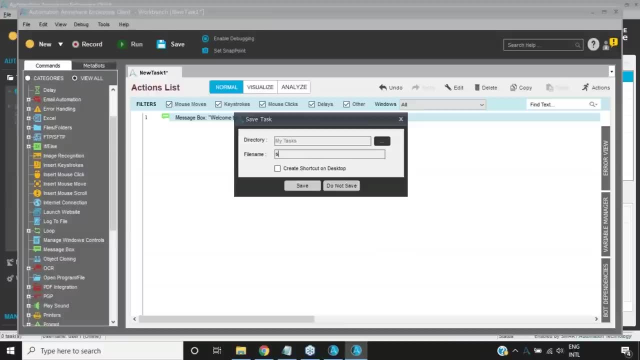 So for that I'll drag and drop a message box And let's say I mentioned welcome to Edureka and then I'll click on save. once I click on save, I'll just mention my task, Let's say sample task. click on save again. 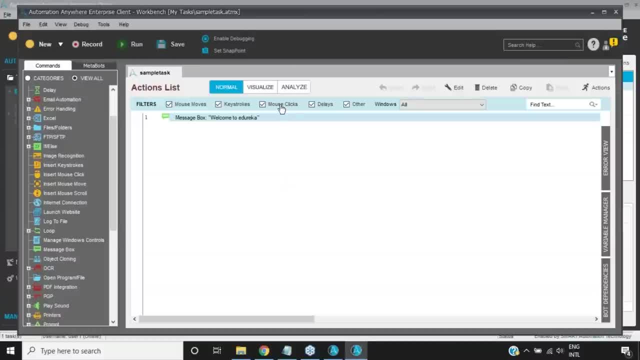 And then what I'll do is I'll just execute once to check if it's working or not. So once I click on execute, you see the output that you know. welcome to Edureka. now I'll just click on ok- close this particular. 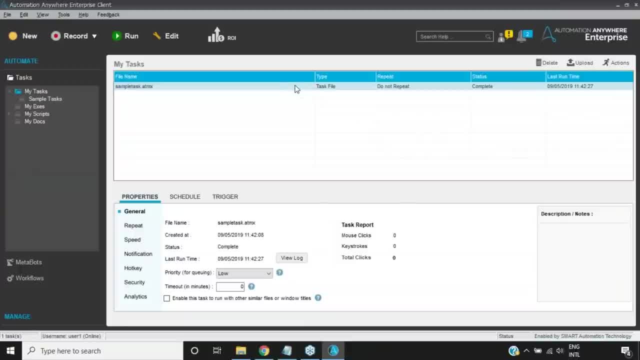 workbench, and now what I'm going to do is I'm going to upload this task. So for that, what I'll do is I'll choose this option of upload And then, when I choose this option of upload, you see that you know, upload a successful, that means this particular task. 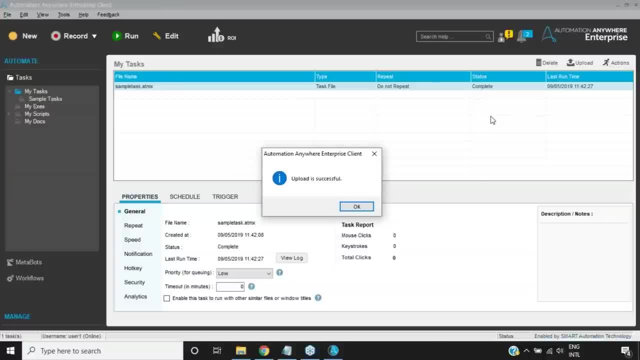 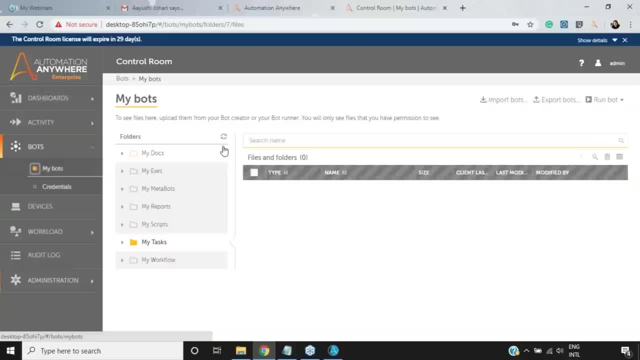 has been uploaded successfully. So that is how, basically, guys, you can upload a task. So now what we can do is we can go back to our control room, right, and then we can go to bots. We can go to my boss and then in my bots. 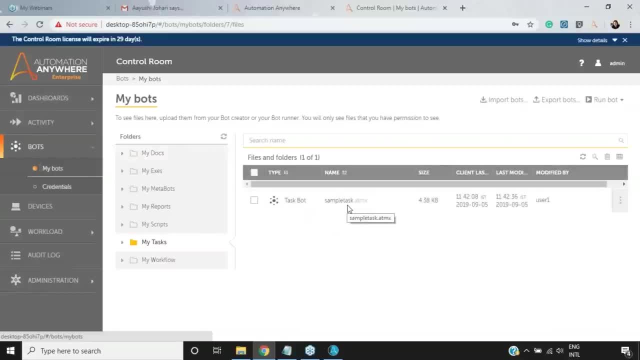 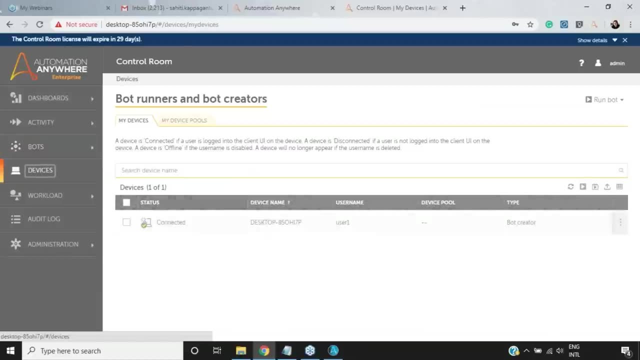 you see a task bot with the name sample task. That was basically a task name and that has been uploaded by the user with the username user one and its size has been mentioned. apart from that, also if you go back to devices over here, you see that you know device with the device name. 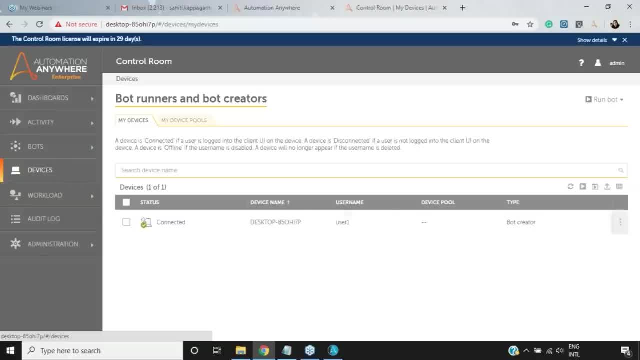 and it's just top and 850 HI 7 P, with username, user one and the license type to be bought- creator has been connected. Now, this is connected because you know our client has been logged in with that particular user and our client is running if our client is logged out. 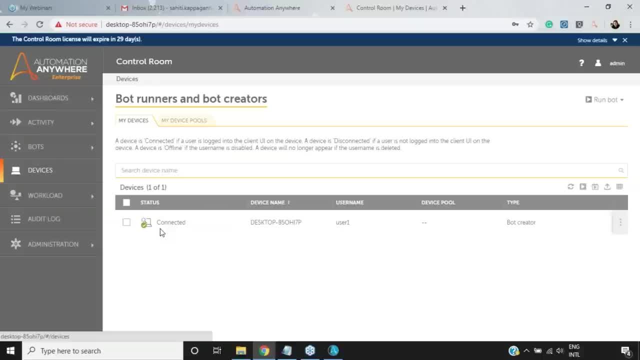 and the client is not running, You'll see that you know the connection is disabled. So that's how, guys, you can use automation anywhere, control room and its features for various kinds of tasks, from simple to complex, and then you can upload tasks as bots and deploy them. 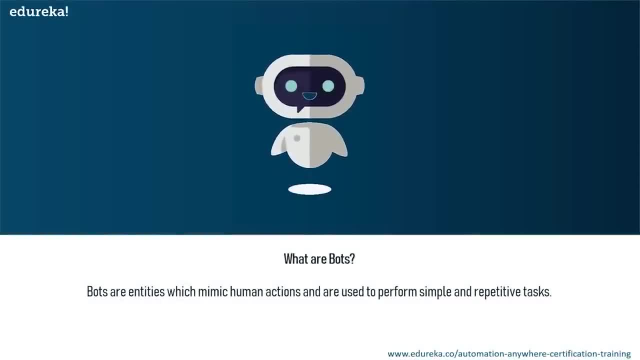 Bots are basically any entities which mimic human actions and are used to perform simple and complex tasks So that the requirement of human employee to perform any task is reduced. So in such way a human's brain can be used in many other intelligent ways to benefit the organization. 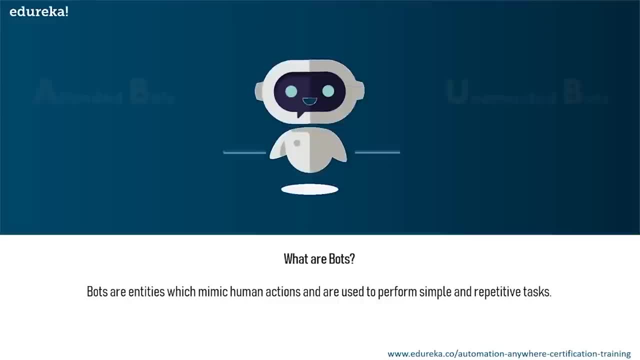 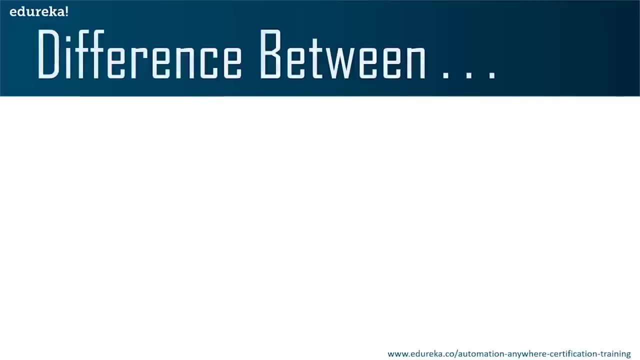 rather than just sitting and doing the repetitive, mundane task. right? So mainly there are two type of boards, that is, the attended boards and the unattended boards. So next in the session, let's understand the difference between the attended boards and the unattended boards. 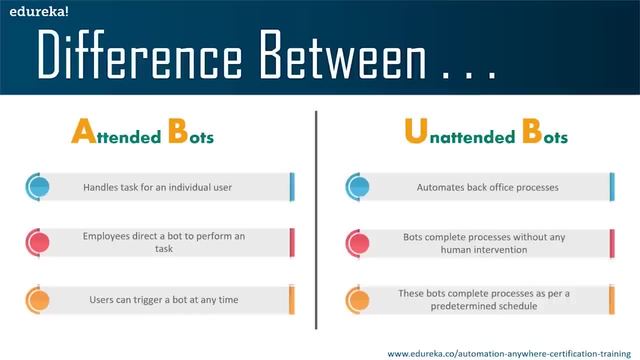 So talking about the attended boards first. So the attended boards handle the task for an individual user. the employees have to direct the board to perform the task and the users can trigger a bot at any time. So attended boards, As the name suggests, basically depend on a user. 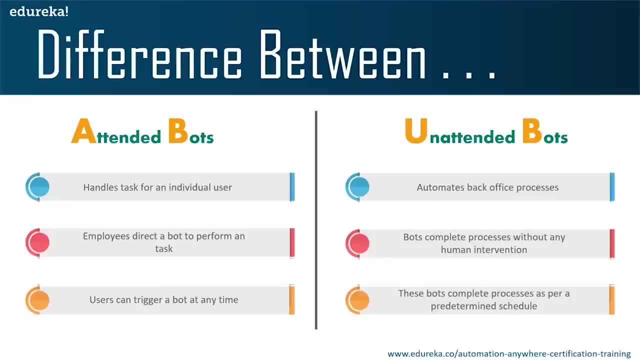 who directs a board to perform a task and it is handled by an individual user and that particular user can also trigger a bot at any time. coming to unattended boards: The unattended boards automate the back-office processes at scale, So boards complete processes without any human intervention. 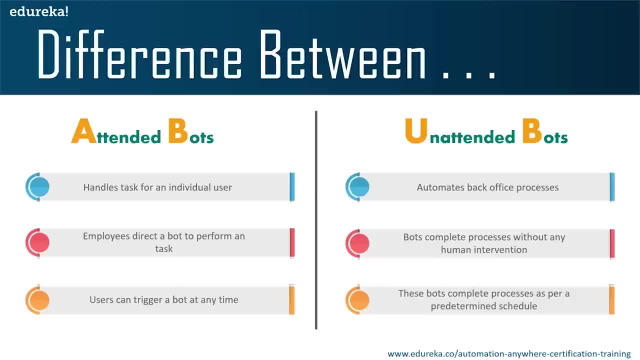 So basically, the boards complete processes for predetermined schedules. So when I say predetermined schedules, I mean that you know when the boards are created. these boards are scheduled at a specific time to perform a specific task. So whenever the specific time occurs, the boards execute the mentioned. 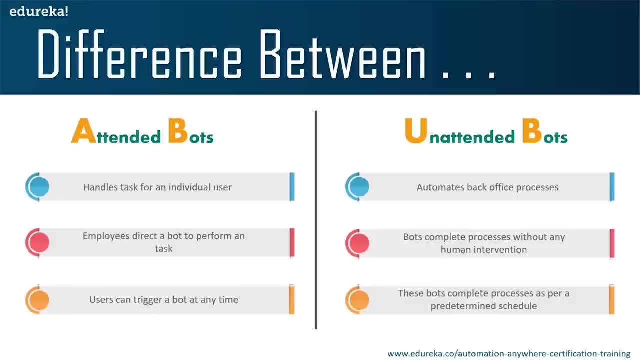 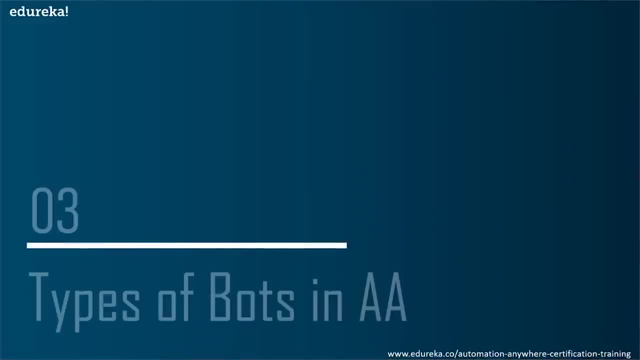 task and then they generate the output so you can see the meaningful results, right? So, guys, these were the difference between the attended boards and the unattended boards. So now that you know what is automation anywhere and what are boards, Let's next look into the different types of boards in automation. 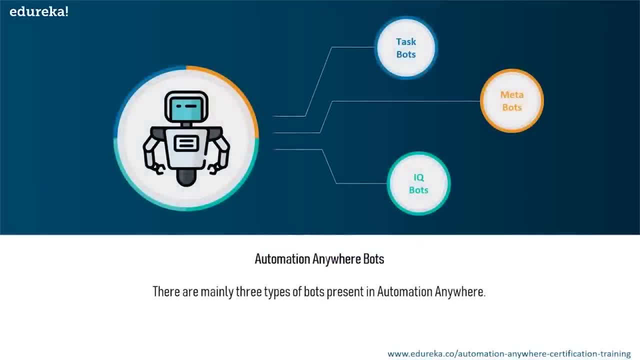 anywhere. well, in automation anywhere, There are mainly three type of boards, that is, the task boards, meta boards and the IQ boards. So we're going to look at each one of them one by one. So, starting with the task boards. the task boards are mainly the core of the automation. 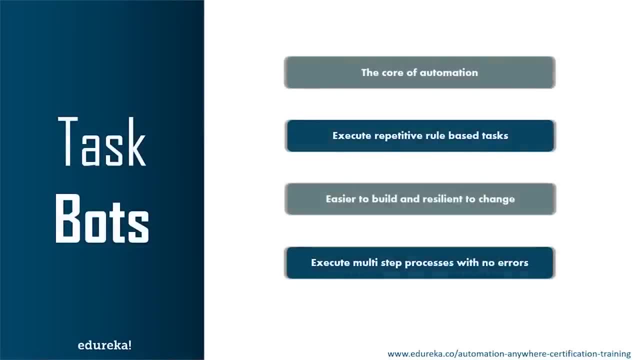 and execute repetitive, rule-based tasks, So these are basically really easy to build and then these can execute multi-step processes with no errors, right? So if you have to understand task boards, guys, the task boards are basically the core of automation and execute repetitive tasks so that the manual intervention is reduced. 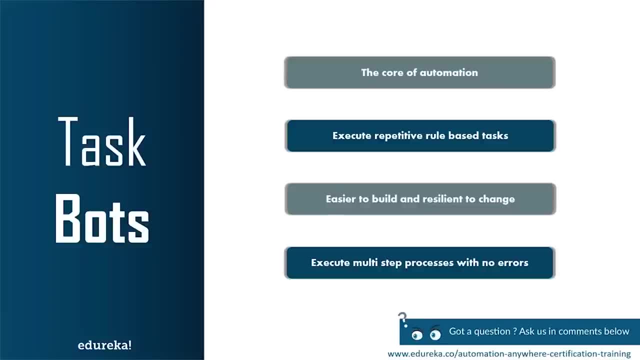 and these boards are really simple to build and can execute multi-step processes, or you can even understand that you know these can execute complex processes with no errors, right? So this was about task boards, So let me just shift back to my automation anywhere workbench. 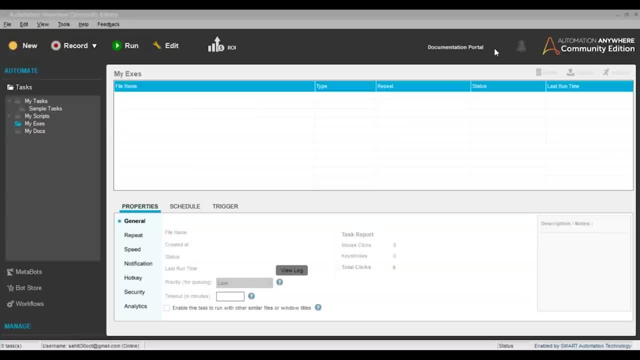 and show you how you can create a task board right. So, as you can see on my screen, this is my automation anywhere workbench. now to create a task board, you can either go through two options, That is, the new option or the record option. 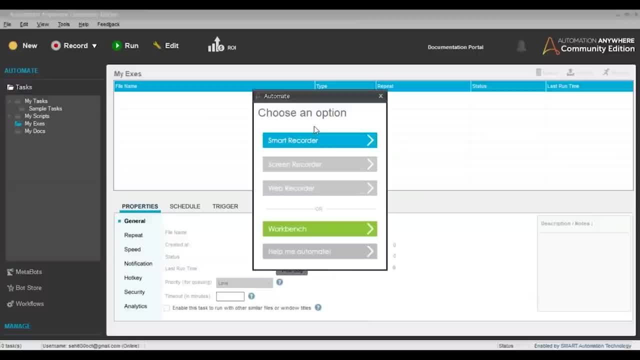 but I'll go to the new option. So when I click on the new option, you can see that, you know, we get a dialog box which opens up and offers various options for us to automate tasks. Right, Well, I'm going to simply go to the workbench option so that I get all the options. 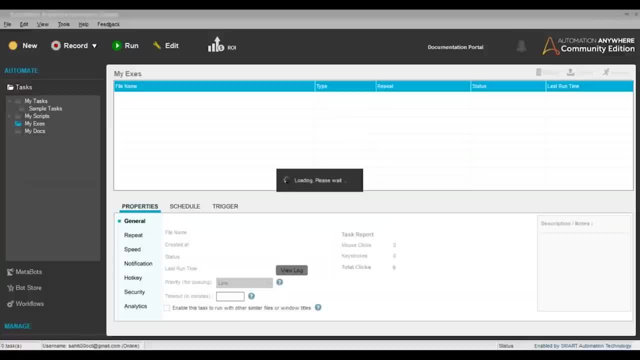 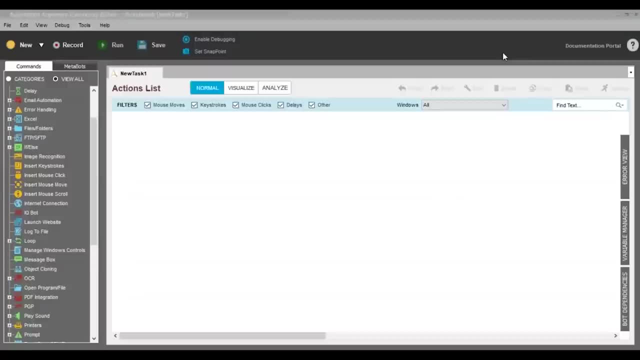 of the activity so that I can just create a simple task and show you how the task board is created. So let's wait for it to open. All right, So as you can see on my screen, my workbench has opened. So now let's say: 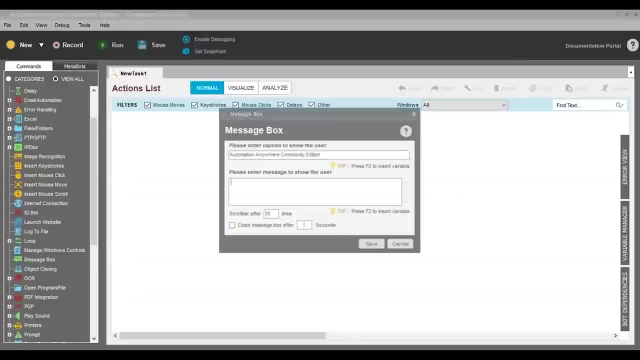 you know we want to display a message right, So I'll just drag and drop the message box command And let's say we write a message that you know, hi from Edureka. and then I click on save right And let's say, if I 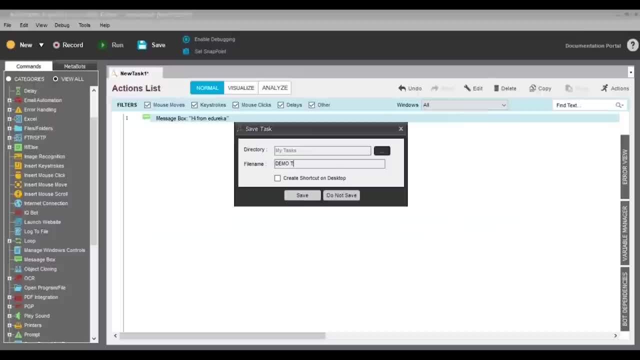 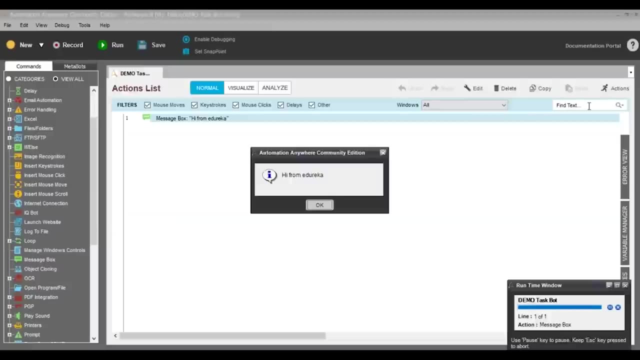 I save this task and let's say we mention it to be demo task board, I'll click on save again and then I'll execute this task. So when I execute this task you can clearly see that you know I've got an output which displays hi from Edureka. 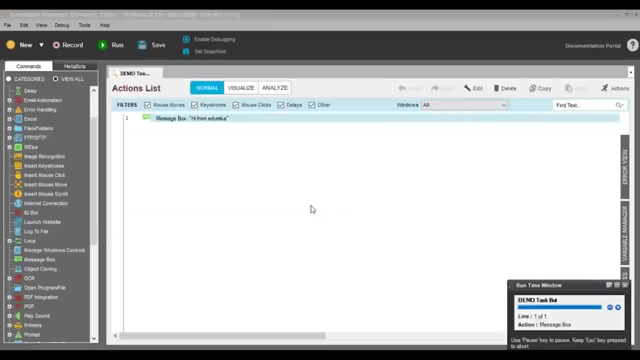 That was there in my message box, right? So once you've created a task and once the task executes, then that is set to be a task board, right? So in my previous session on the Automation Anywhere examples, I've created n number of automation. 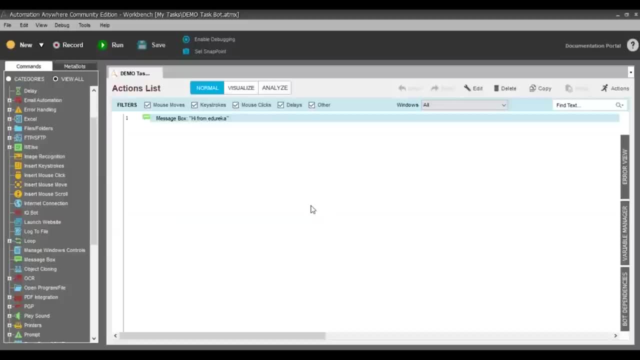 as based on the different commands present in Automation Anywhere, and also specifically on Excel automation and PDF automation. So all the tasks that I created over there with basically the task for, so basically task for, if you just have to understand, is a simple task that you create either to automate a simple. 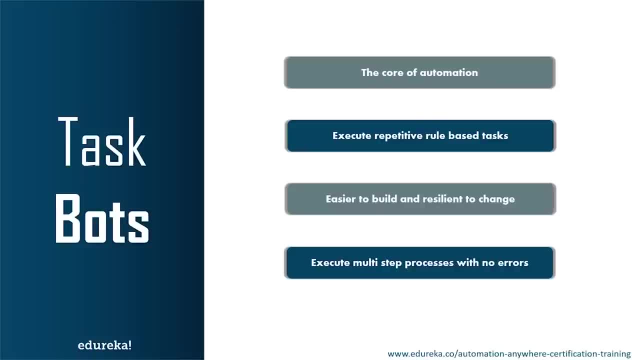 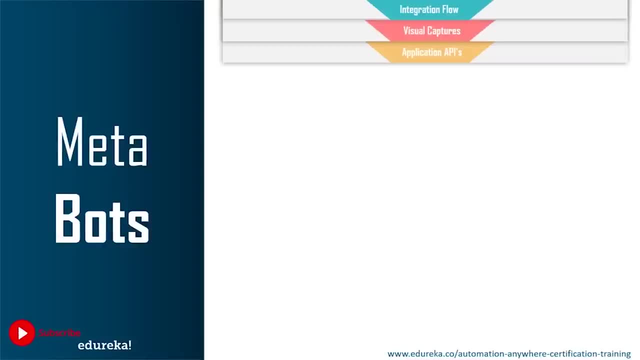 or a complex automation right? So, guys, this was about the task force, So now let's move back to the next type of box in Automation Anywhere, That is, the meta box. So you can understand the meta box to be an advancement. 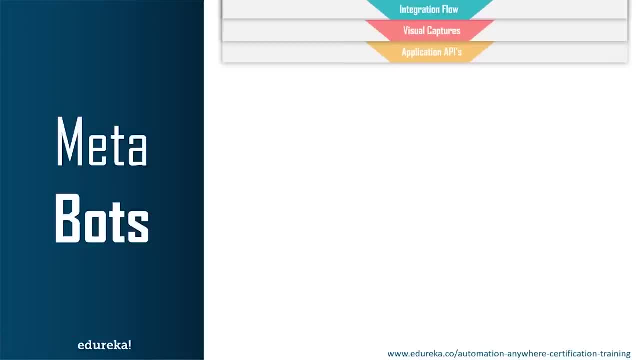 Of the task box. So, as you just saw, task box are created in a really simple way where you know it's not any application specific. You can just drag and drop few commands from the workbench and then you can define rules to perform automation. 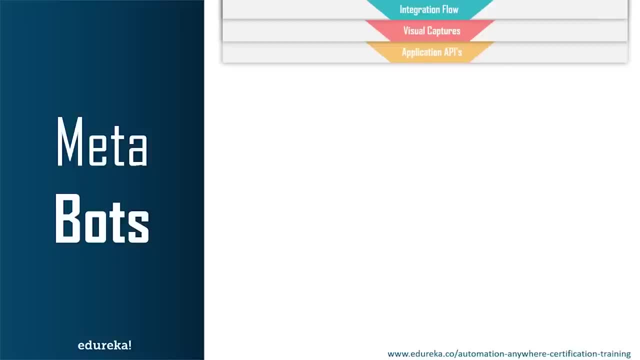 But when it comes to the meta box, you can either create meta box application specific or you can also create for all applications. So I'm going to show you how you can create that, But before that, let me just tell you that you know. 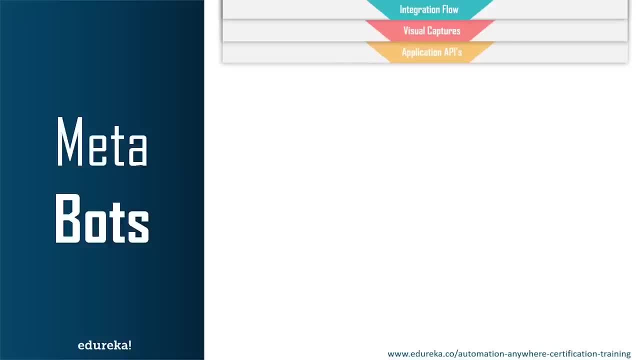 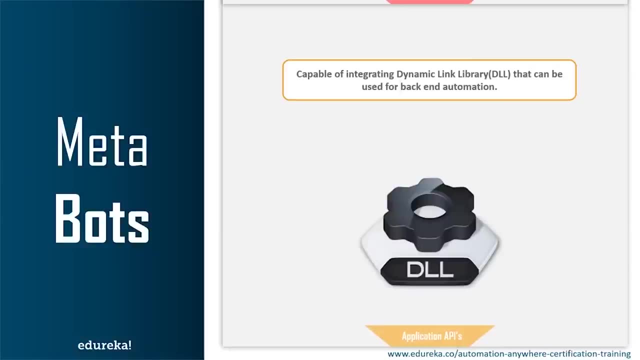 meta box are created based on the application API is visual captures and integration flows. Coming to application Api's. application Api's are basically capable of integrating dynamic link libraries that can be used for the back-end automations. So when you create a meta board and then you go to the meta 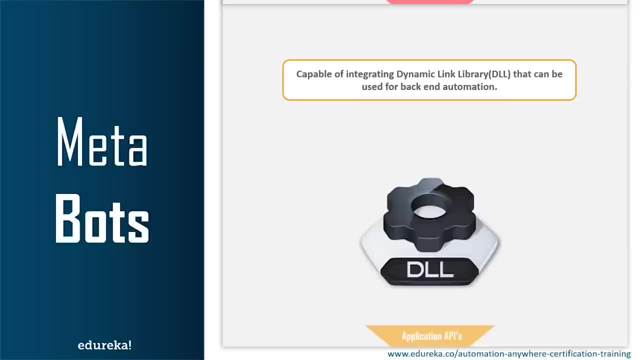 board designer, you get an option of add DLL. So basically, through that option you are capable of integrating dynamic link libraries. So these libraries can be then further used to automate tasks at the back-end automation right. So that was about application Api's. moving on to the next feature, that is, visual captures. 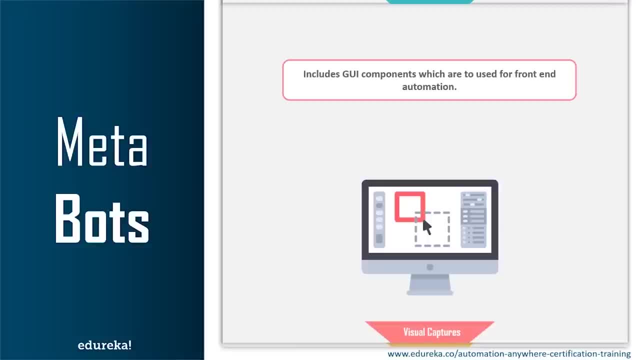 So when I say visual captures, I mean that you need to includes the GUI components which are used for the front-end automation. So, for example, you have an application and then you know you want to enter some text into some part of the application. 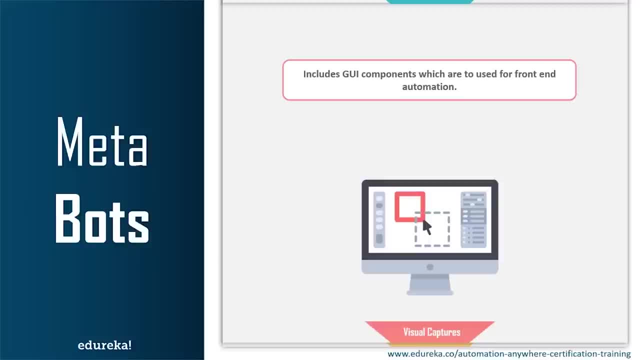 then automatically, meta boards are created based on the GUI components to identify that particular area where you know you want to mention the text, and then you can just enter the text that you want. So don't worry, I'm going to show you how that's going to be done very soon. 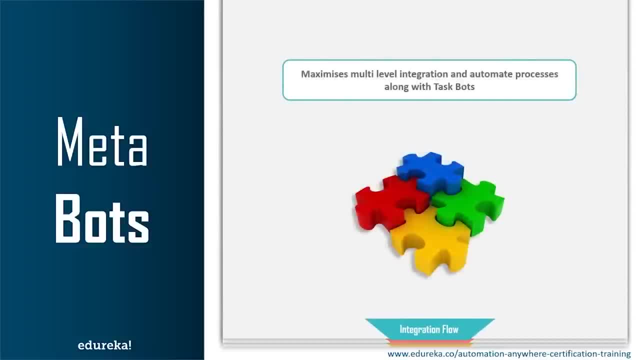 moving on to the third point, that is, integration flow. So basically, when I say integration flow, I mean that you know meta boards, maximizes multilevel integration and automates process with the task boards, For example, if you have a meta board created and then you know. 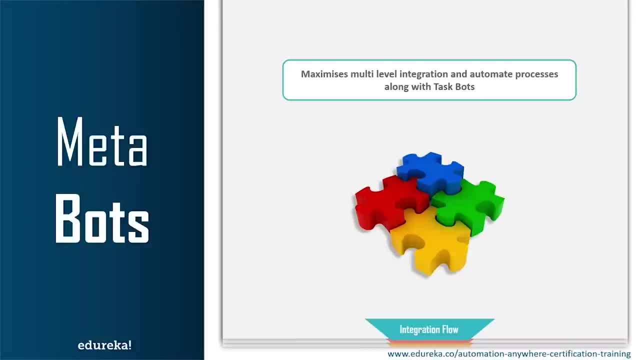 you want to execute or maybe you want to automate some specific task in that particular meta board, then you can obviously integrate both these boards together through a workbench and create a proper logic flow for all the meta boards to execute specific tasks so that the automation 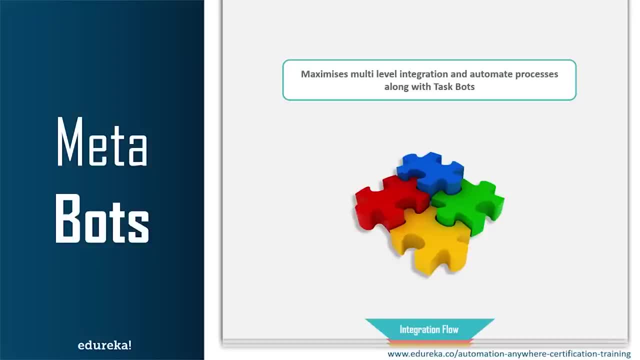 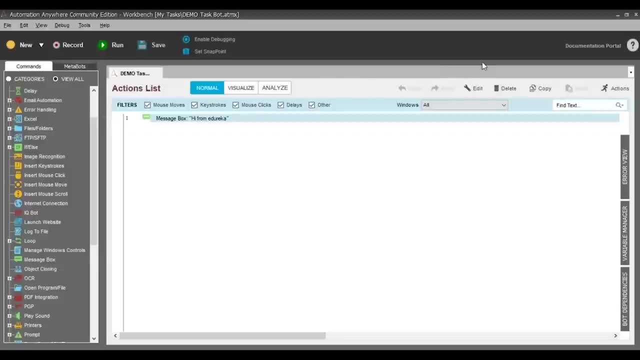 is occurred. So that was about meta boards, guys. So let me just quickly shift back to my automation in your workbench and show you how that's done. So, as you can see, this is my workbench. So what I'll do is I'll go to my client and then, when you go to 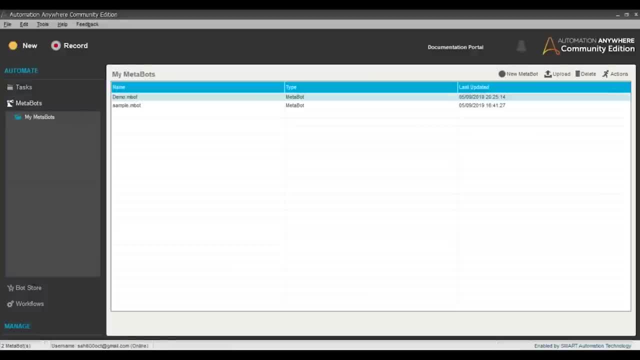 the client, you see an option for meta boards, So I'll just click on the meta boards option. So, as you can see, when I click on the meta boards option, your redirected to this particular page, which shows you know where you can create a meta board. 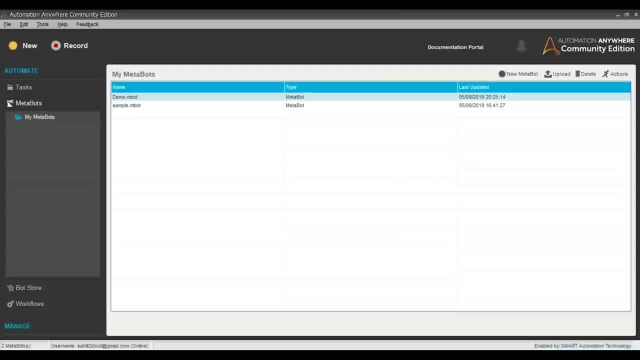 right. So before I start creating a meta board, I just want to tell you one thing over here: You have to be an administrator to create a meta board. So basically, if you're not the administrator of your account, then you cannot create a meta board. 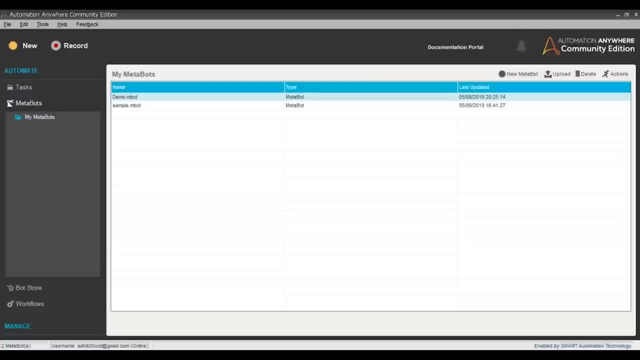 You won't get an option To create a meta board. So to run as an administrator you can just, you know, right click on the automation anywhere icon and then choose the option of run as administrator. So with that, you know, you get this option of creating a meta board. 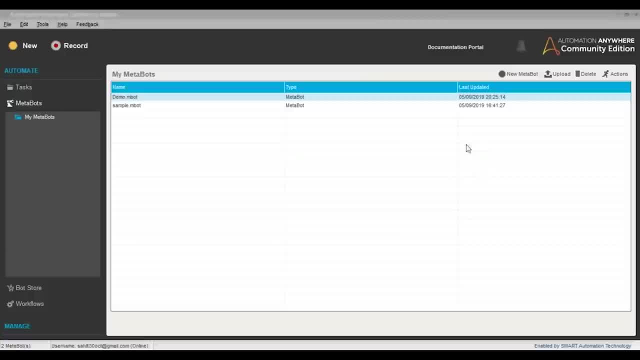 So now moving forward to how to create a meta boards. So, as you can see, on my right hand side there's an option for new meta board, right? So I'll just click over here. When I click over here, you can see that. 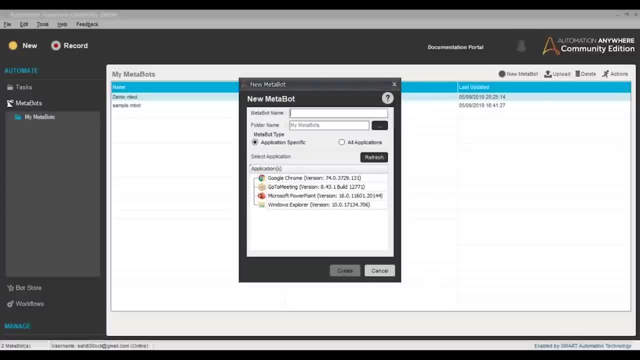 you know we have various options of you know meta board name, folder name and the application type and the meta board type. So you just have to mention the name. or maybe if you want to store the meta board in a folder, then you can mention the folder name. 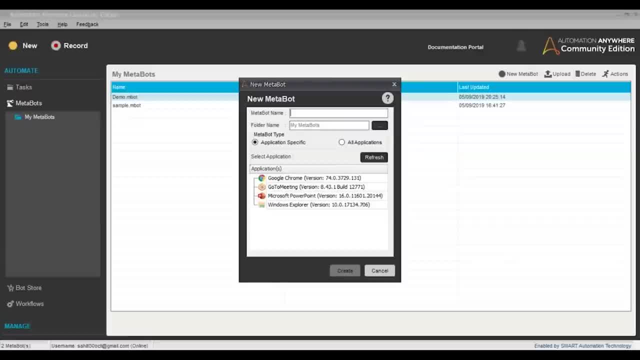 and you have to choose the meta board type, that is, application specific or all applications. So when I say application specific, you'll have to choose any specific application from the list that is shown to you And then, if you choose all applications, then the meta board that you create will basically apply to. 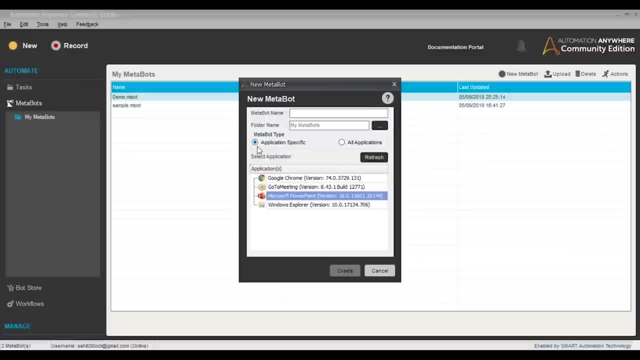 all the applications that are open in your system, right? So what I'm going to do for this particular demo is that I'm going to open an Amazon website and then I'm going to show you how you can sign up for the Amazon website. 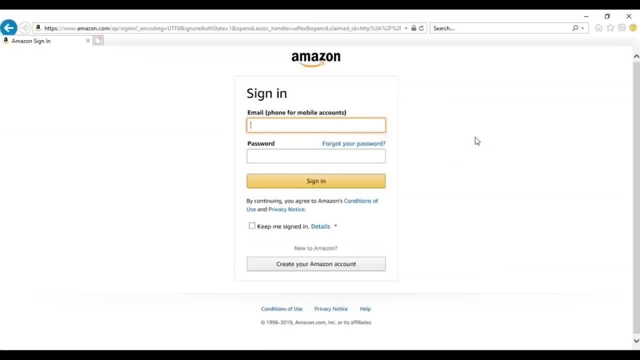 Right. So basically, this is the Amazon sign-in page. Now what I do is I'll go back over here, I'll close this dialog box, then I'll open again. So when I open again, you can clearly see that. 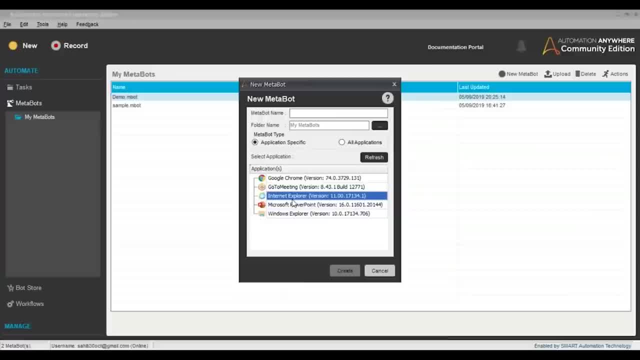 you know, I've got my internet Explorer, in which I've opened the Amazon sign-in page, right, So I'm going to select that particular application, choose application specific And let's say we mentioned the meta board name to be demo meta board. 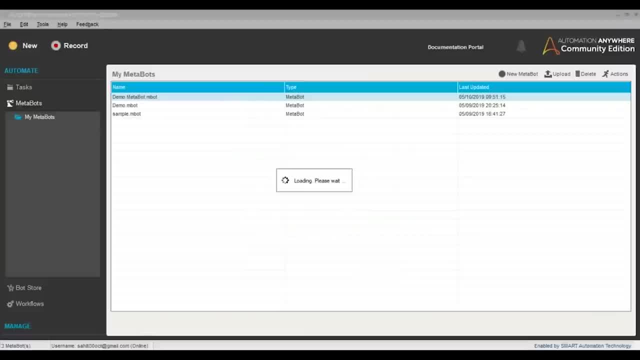 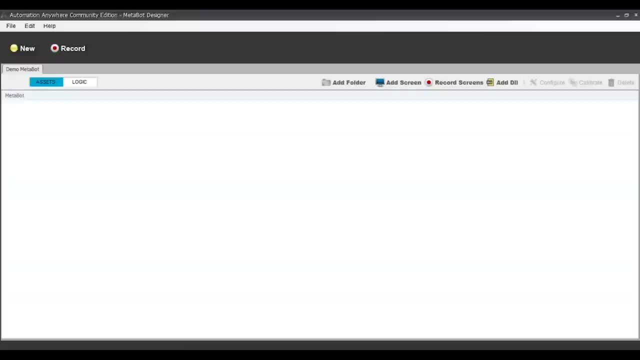 And then I'll click on create. So once I click on create, you can clearly see that you know my meta board is getting created, But the specific application that I chose, that was basically my internet Explorer with the Amazon sign-in page right now. 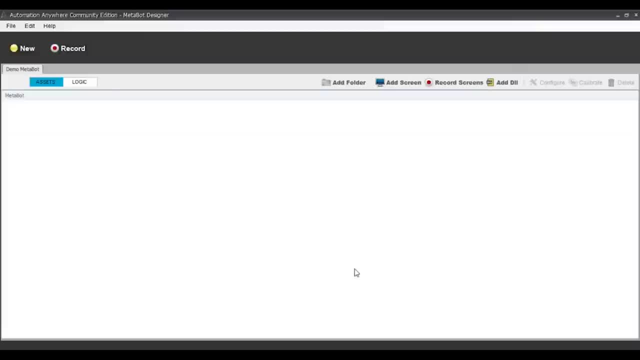 once the meta board designer opens, you basically observe two options over here, That is, the assets and the logic tab. So basically, the assets tab has few options and the logic tab also has few options. So first, what I'll do is I'll talk about the assets tab and 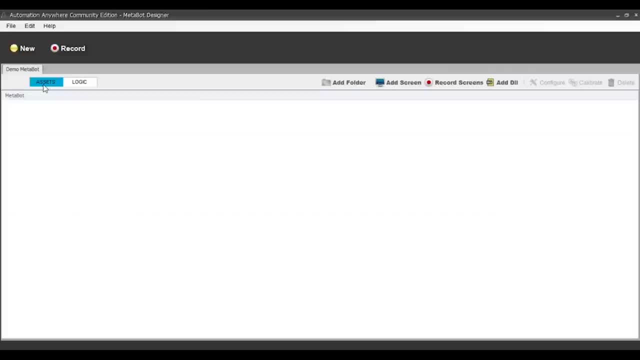 then I'll talk about the logic tab, right? So what we'll do is we'll go to the assets tab. So, as you can see on my screen, this is the assets tab. So in the assets tab there are mainly four options. 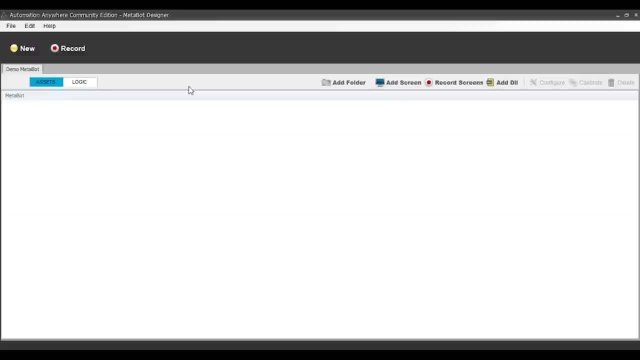 That is the add folder, add screen, record screens and add DLL. So you can just consider the assets tab to be basically, you know when you can add n number of screens as you want. So for example, let's say in my internet Explorer: 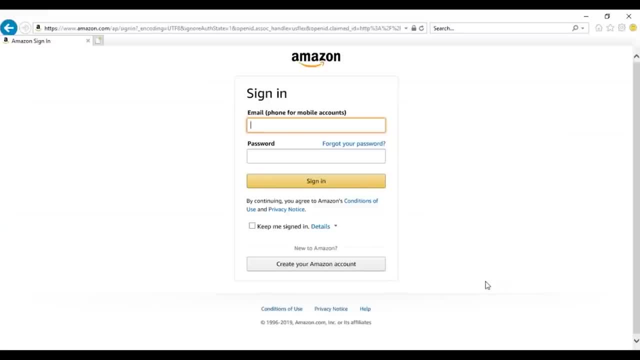 I just opened a single screen. right, That was basically a single tab. So let's imagine if we had around 20 tabs open in the internet Explorer, then all those particular screens can be added to the assets tab So as to ensure on which screen what automation has to be occurred. 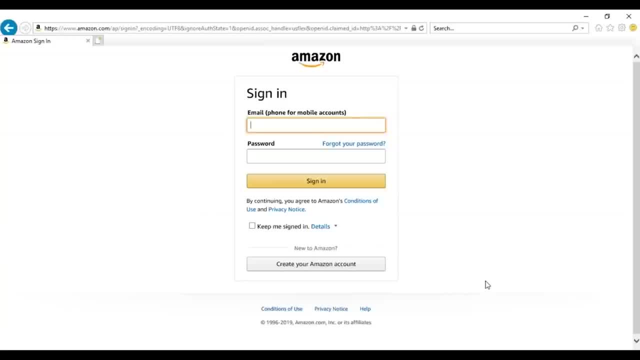 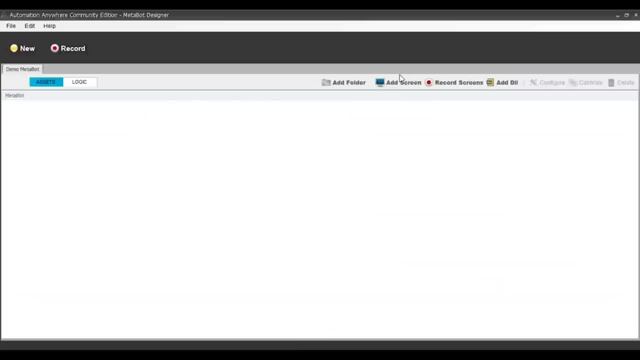 right. So for your better understanding, I'm just going to consider one screen over here, so that you understand how we can do that. So I'll just shift back to my metabot designer over here And what I'll do is I'll first add the screen. 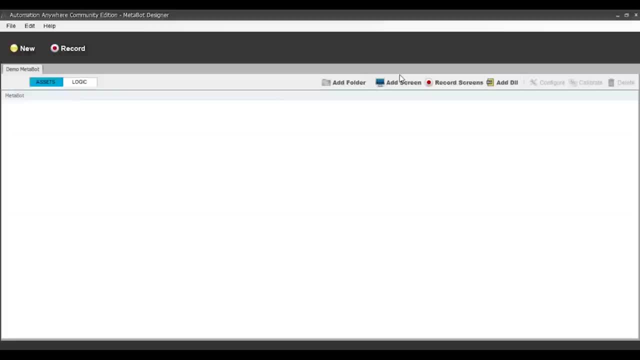 So when I say add screen, I mean that you know, since you've already created a metabot for a specific application, that particular screen will be automatically open, right? So I'll just click on add screen and then you'll see that. 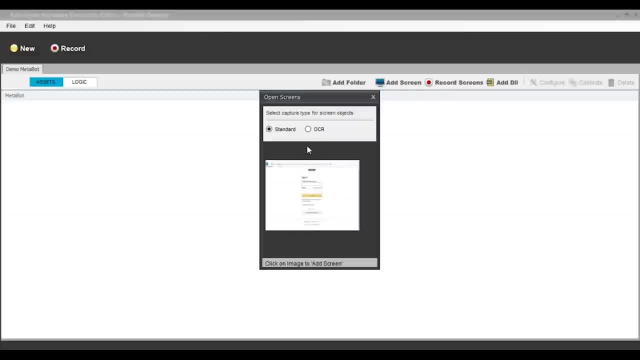 you know you get an option for standard and OCR. So I'm going to choose by default standard. But if you choose OCR then you'll have to choose the OCR engines also. So by default it is Tesseract, But yes. 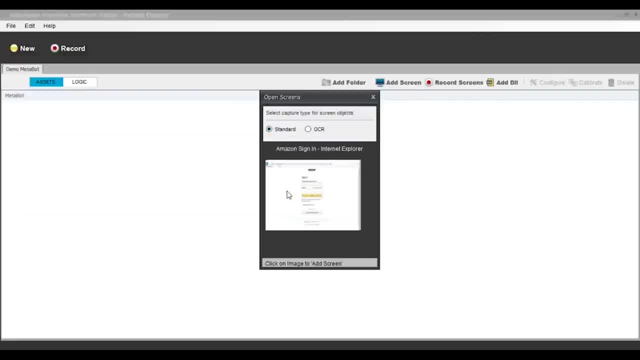 over here for our particular demo. I'm going to choose the standard one, So what I'll do is I'll just choose this particular screen, That is, the Amazon sign-in page. So that will be one screen of mine. So, as you can see, 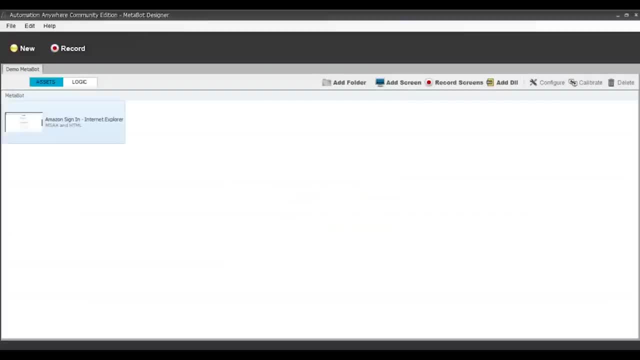 the screen is getting created, So let's wait for it to happen. So, as you can see, my screen has got created right, So now, like this, you can add n number of screens that you want. So if you had a different tab open, 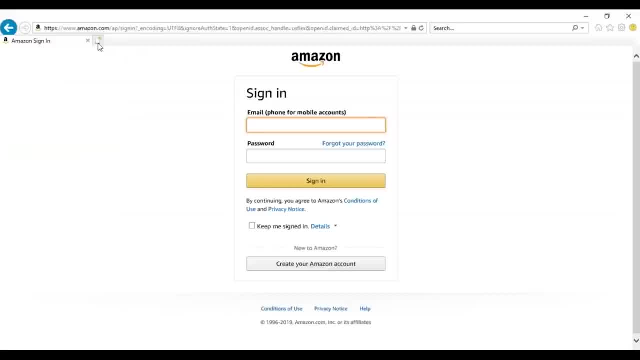 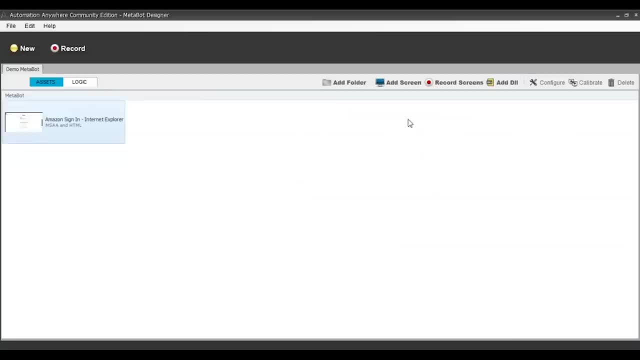 let's say, you know, if you had a Facebook tab open, right? So let's say I add facebookcom. Let's say this particular tab was open, Now I'll shift back, go to add screen and then choose Facebook. 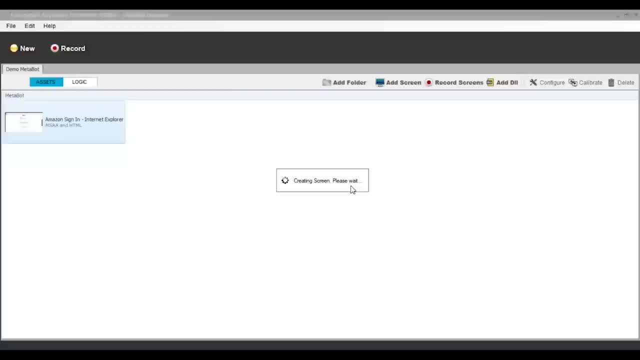 right. So basically, this will be the second screen that is created right. So now, if you clearly observe over here, there are two things that you need to understand. The first is that you know, whenever you add a screen, your previous screen should be open. 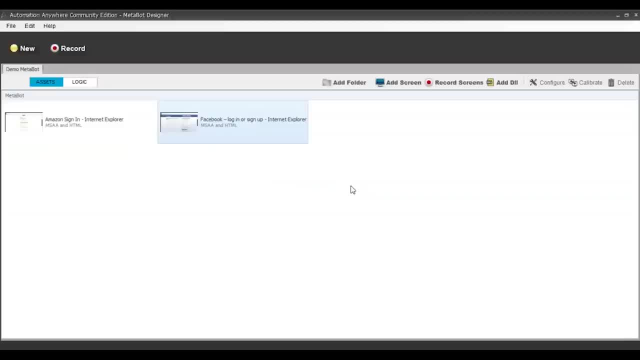 So, for example, if you wanted the Amazon sign-in page to be added as a screen, then the Amazon sign-in page should be open in the selected application. Similarly, if you wanted Facebook screen to be added, then the Facebook screen had to be open. 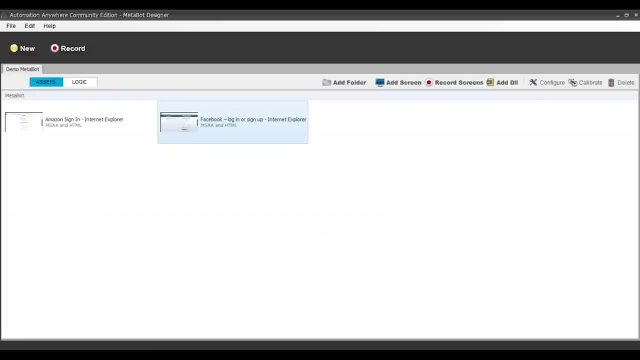 The second point is that you know it's not restricted that there should be only two screens. There are multiple screens that you can add in a single asset and then you can play around with your automations. So that was about add screen guys. 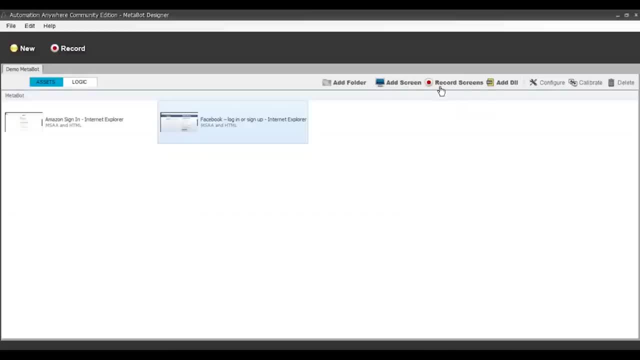 Now, if you move forward to the record screens option, so when I click on record screen, so it will basically record all the actions that I do on the screen. So let's say, you know I choose the screen of Facebook, right? 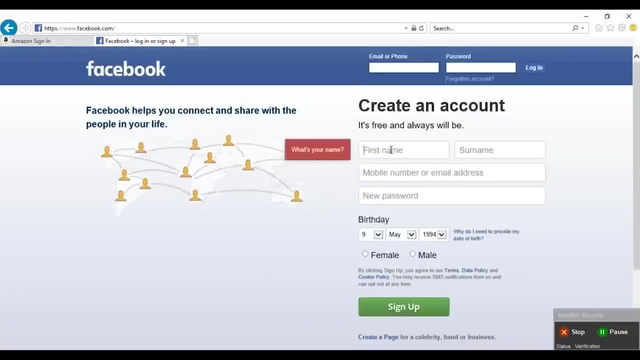 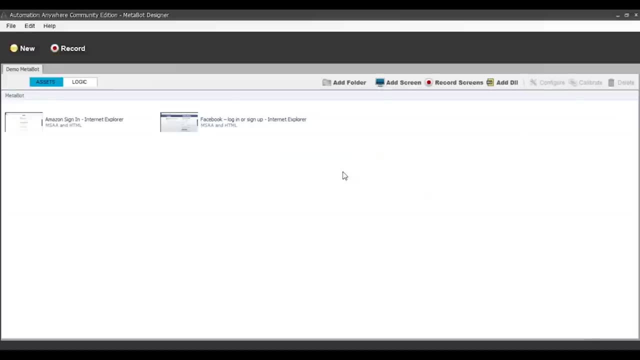 So that is the open screen and let's say, you know we mentioned something, Let's say we mentioned name, And then you know we click on stop. So basically that particular action of me writing my name is been recorded and then it will be stored. moving on to add folder: guys. 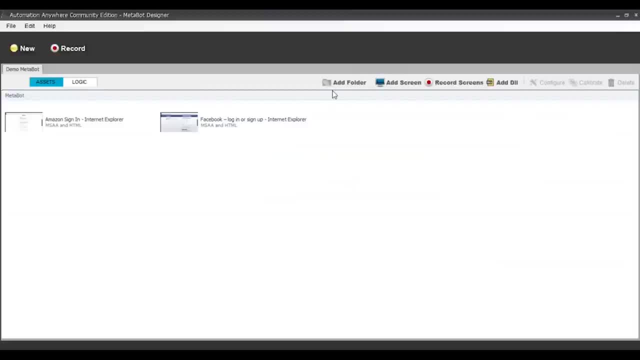 So add folder is basically to put all the screens in a specific folder. So if you just click on add folder and let's say we give the folder name to be example, and click on create and let's say we put the Facebook one inside this, 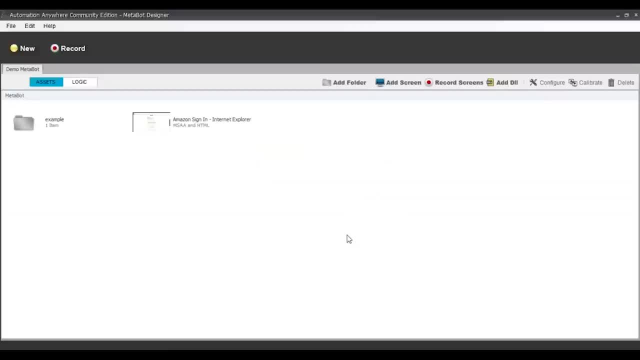 right. So basically inside a folder you can have n number of screens again. and moving on to the final option, that is, add DLL. So, as I previously mentioned, the add DLL option is to basically integrate the dynamic link libraries for the back-end automation. 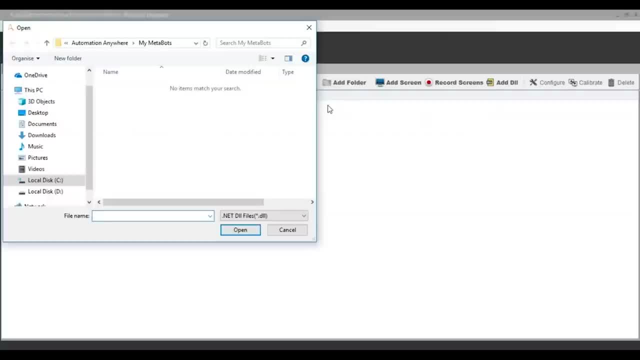 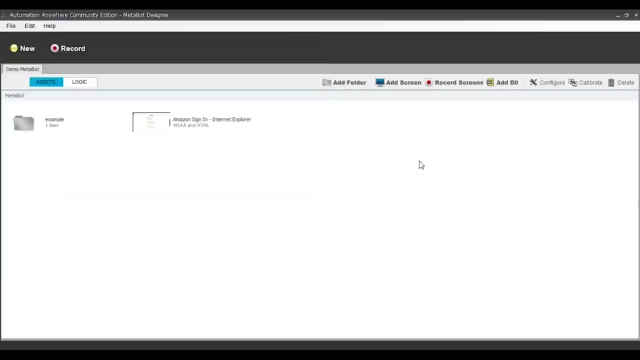 So to do that, you can just click on add DLL and then choose what all dynamic link libraries that you want to open, right? So, guys, that was about the different options available in assets. Now, apart from these, there are ways, other options, that is, the configure, calibrate and delete. 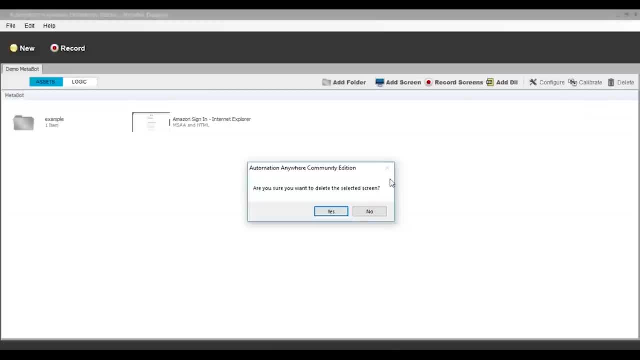 So, coming to delete, when I say delete, you can just delete any particular folder or screen over here. I'm not going to delete any particular screen over here presently, but whatever is the selected screen, that particular screen will get deleted. coming to configure. So when I say configure, 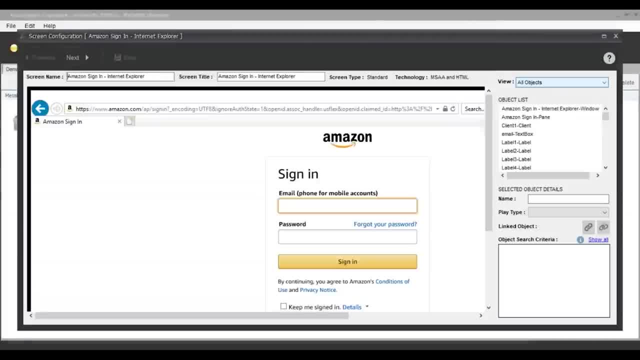 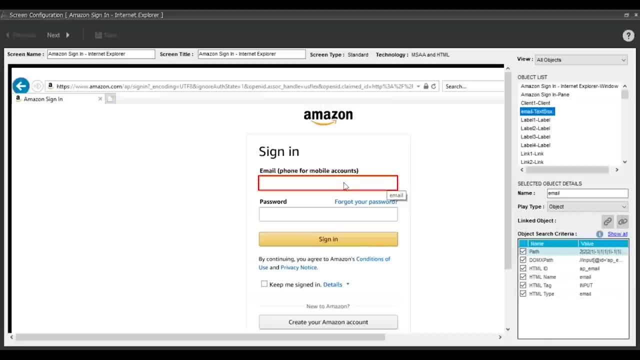 let's say we choose the screen and then we click on configure. So basically it will show you all the options through which you can configure your particular screens. So, for example, let's say: you know, I want to type some text over here. 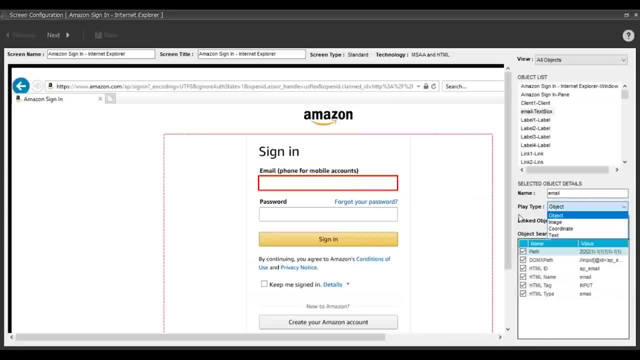 right? So our name is email and play type is identified as object, right? So for example, if you want to type any text so we can identify that particular play type to be text, so that you know text is mentioned over here. 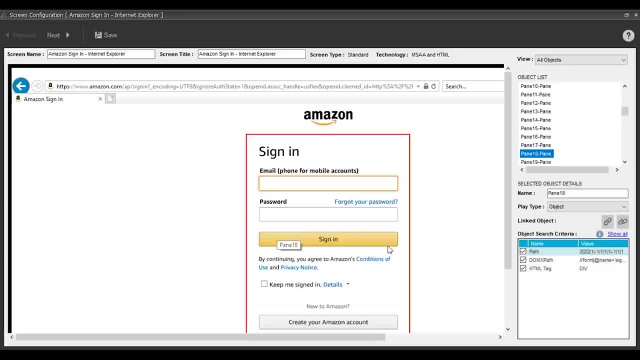 Apart from that, it also gives you all the GUI components search criteria. As you can see, I've selected this particular object, So according to that, in the object search criteria you can see what all HTML tags or, you know, path or the other back-end stuff are there. 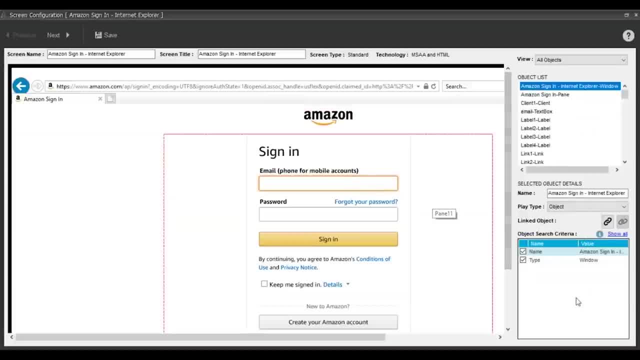 Similarly, if you want to say Amazon sign-in, that is considered, then you can see that you know the name and type of the window is considered, Let's say if we consider the sign-in button. So when I say sign-in button, you can clearly see that. 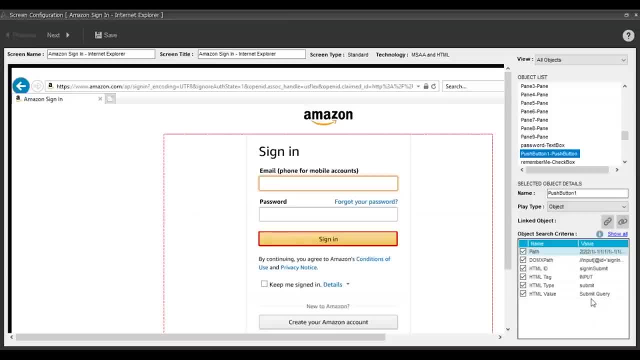 you know, the HTML ID for sign-in- submit is there, where you have an HTML tag and then you have a submit query and so on. So that's how you can identify all the GUI components for the selected application. Apart from that, you also have a view option, from which you know. 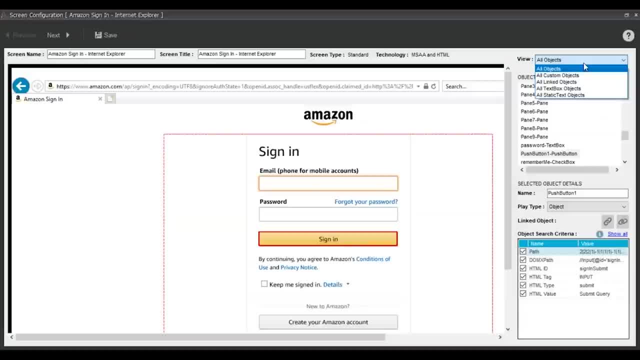 you can either view all the objects or maybe the custom objects in which you want to specifically identify an object. For example, let's say you know this particular part is not identified. I can just drag and drop and then I can identify that particular object and then that will be the custom object. 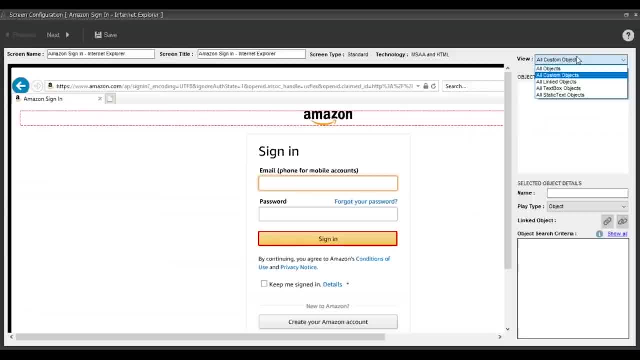 Similarly, we can identify the link text box and the static text object moving forward with the screen types to screen type of standard. that was because previously I had chosen standard instead of OCR- and then we can also edit the screen title and the screen name, and then what I can do is I can just click on save to save my configuration. 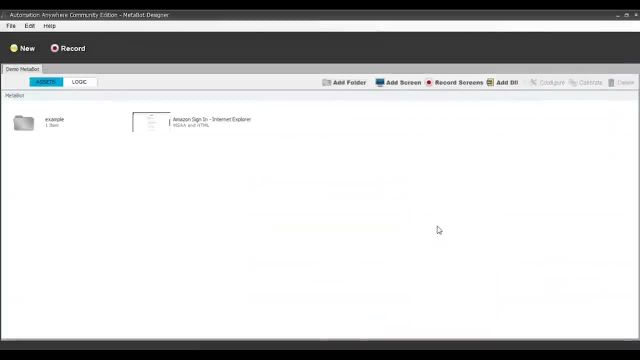 So, as you can see, my screen has been saved. now. I'll just close this part right now, coming to the next option, That is, the calibrate option. So the calibrate option is basically used to Compared to screens. So this is basically used in real life, as a particular web page is never static. 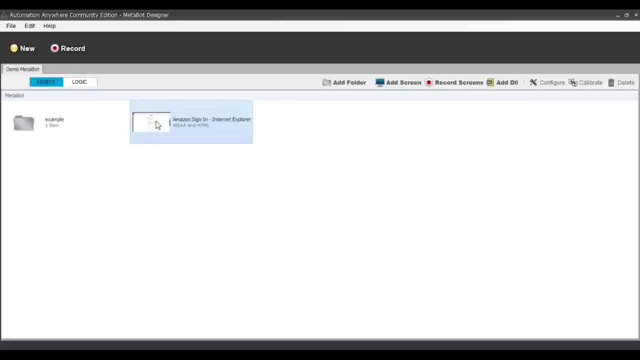 right, It always keeps on changing. Maybe there are a few additions, few deletions. Maybe, you know, some components are shifted from right side to left side, or maybe they're just deleted, and so on. Right, So a web page can definitely change its complete look. 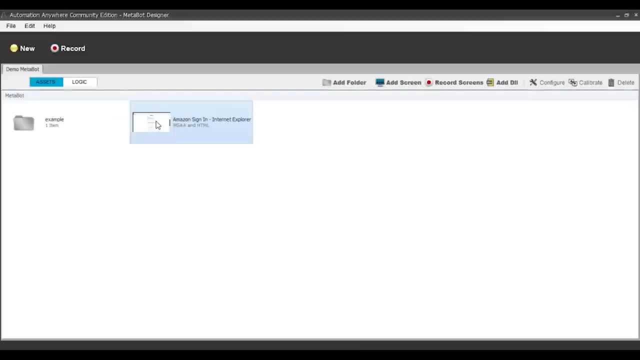 right. So to keep a track on you know what are the changes from the updated view to the past view. you can use this option of calibrate. So to show you how to use the calibrate option, first I'll add a screen of Facebook. 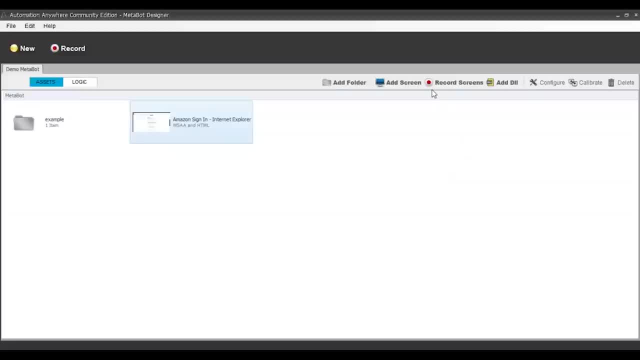 And then what I'm going to do is I'm going to add a different screen of Facebook, right? So let me just add the screen of Facebook. So my Facebook screen has been added right? So let's just wait for it to create. 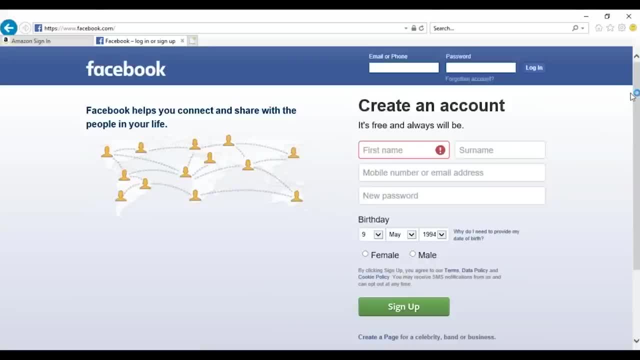 Right now. Remember one thing over here. So whatever is captured on your full-size window is basically considered for the calibrate option. So when I scroll down you'll see that you know these particular elements will not be visible in the full-size window. 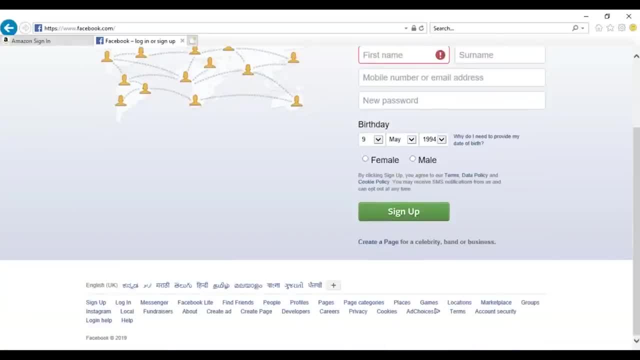 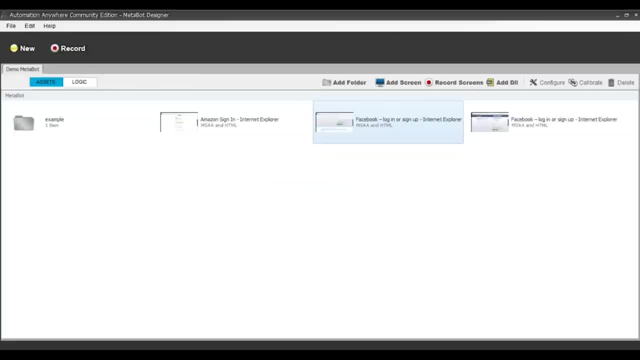 right. So for the calibrate option, this will make it a different screen, So for that I'll just Add a different screen over here. So I'll click on add screen again and choose this particular screen, Right? So basically, as you can see on my screen, 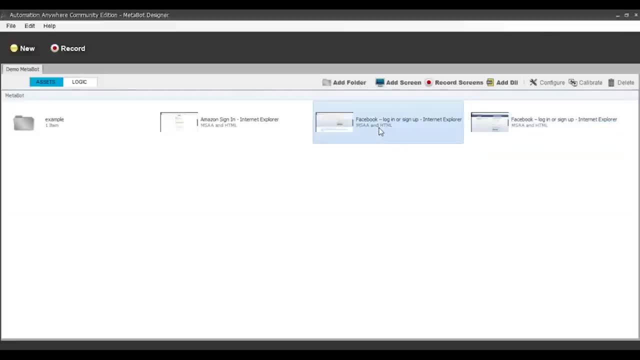 I have two different screens that are present. that is Facebook original page And the other one is Facebook, just scrolled up. So what I'll do is I'll use the calibrate option. So initially I just select this particular screen, click on calibrate, and then what I'll do is I'll compare these screen. 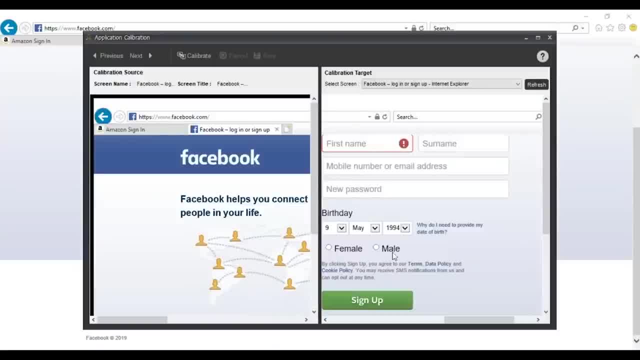 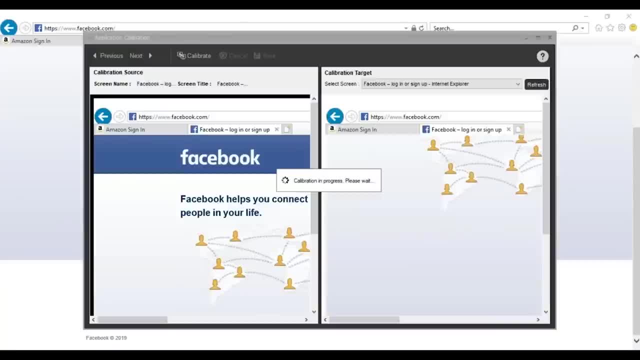 So, as you can see on my screen, both the screens are available. as you can see, the left side screen shows the Facebook icon, but the right side screen doesn't show the Facebook icon, Right? So what I'll do is I'll just click on calibrate and you'll see that. 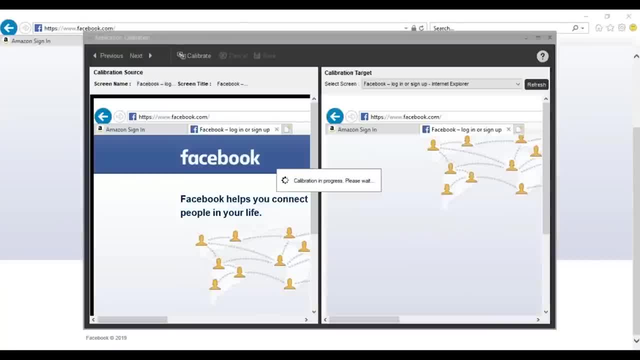 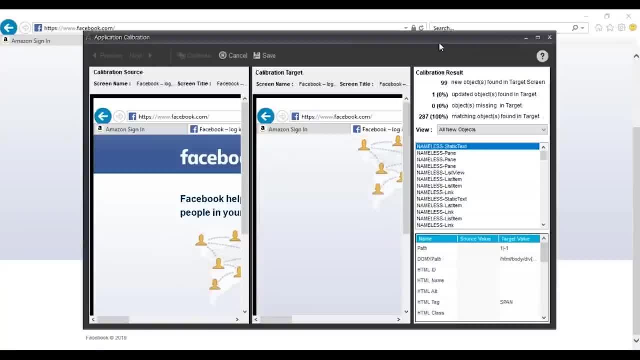 you know there are a few changes in both the screens, So let's just wait for the output to come. All right. So as you can see on my screen, the calibration is successful. So when I click on okay, you get the results that 99 new objects are found in the target screen. 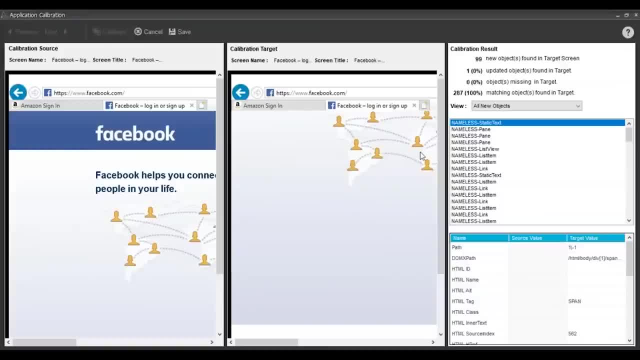 One object is updated found and there are 287 matching objects found in the target screen. So that's how, basically, you can use the calibrate option to compare both These screens. So this was about the calibrate option, guys. Now you can either save this calibrate screen or you can just cancel this. 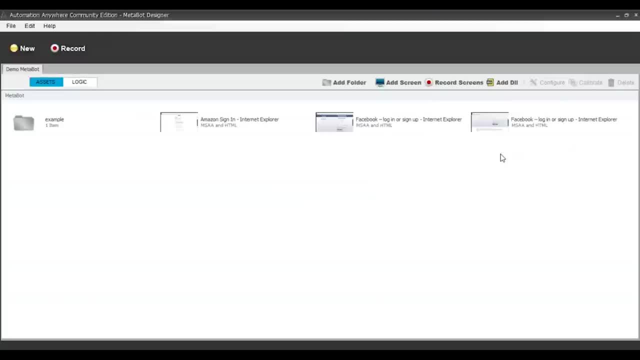 I'm just going to cancel and then I'm just going to close, Right, So now let's move forward with the next tab, That is, the logic tab. So the logic tab is basically used to add logic to your metabots. So when I say add logic, 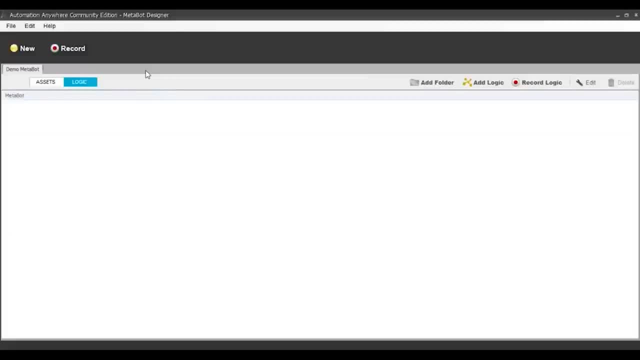 I mean that, basically, you have to define the rules or the steps through which you can perform your automation. So, before I choose the option of add logic, what I'll do is I'll go back to my assets tab and then let me just remove these screens, so that you know. 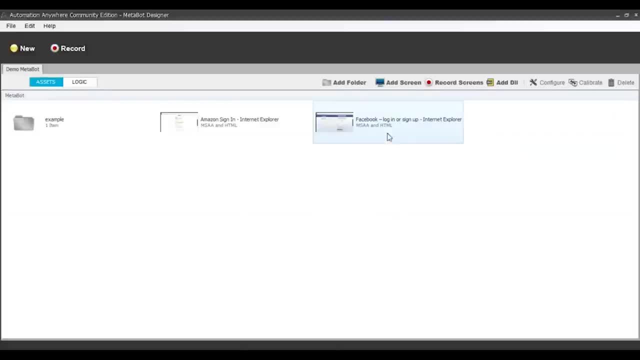 there's no confusion. So click on delete. I'll click on delete again. I choose this particular screen. go to logic. go to add logic. So when you click on the add logic option, you can clearly see that you know the Amazon screen will come right now. 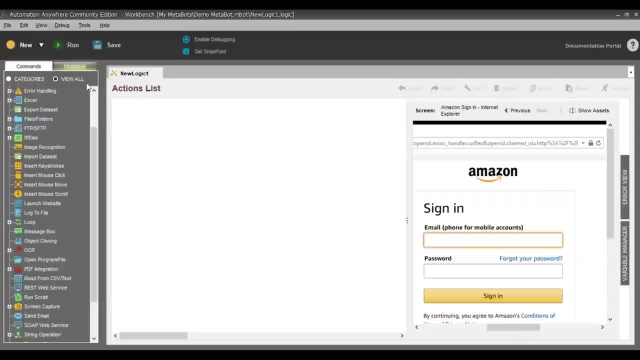 as you can see, the workbench has opened up with all the activities or the commands on the left hand side, as it is simply in the simple workbench, and on the right hand side you have a view to your application, right? So before I start with, 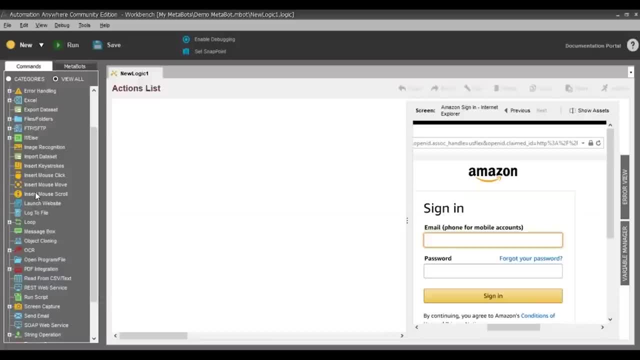 you know executing anything over here. I just want to tell you one thing over here: that two more commands are added to the list of the commands over here. That is the export and the import data set when you choose the option of add logic. 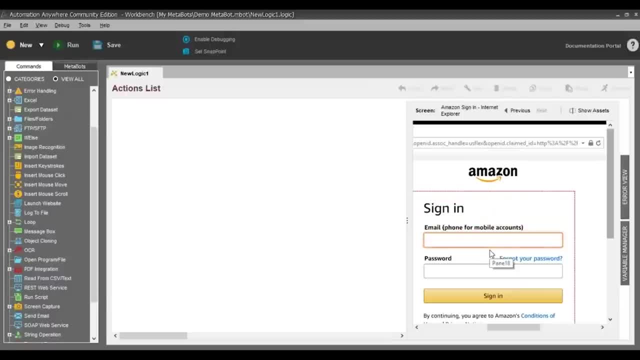 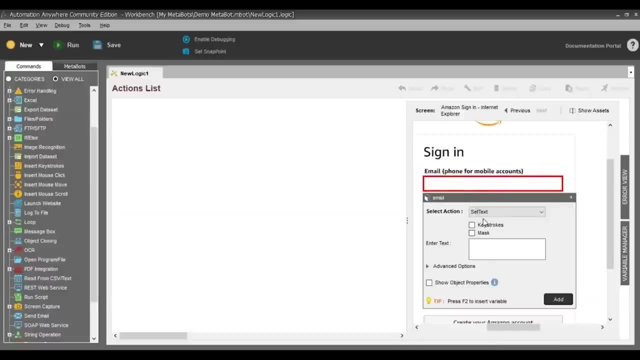 right. So now let's go forward to just enter the email ID and password over here. So to do that I'll just double click over here. So when I double click over there you can clearly see that you know you get an option of set text. 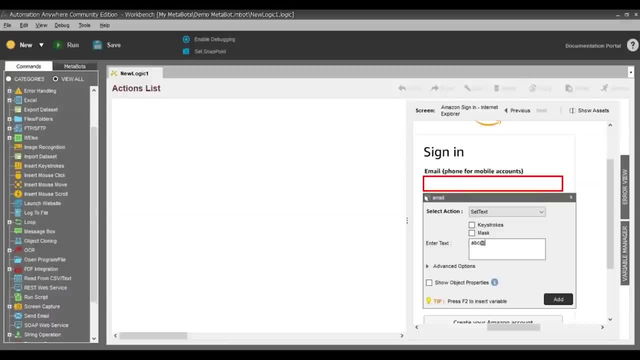 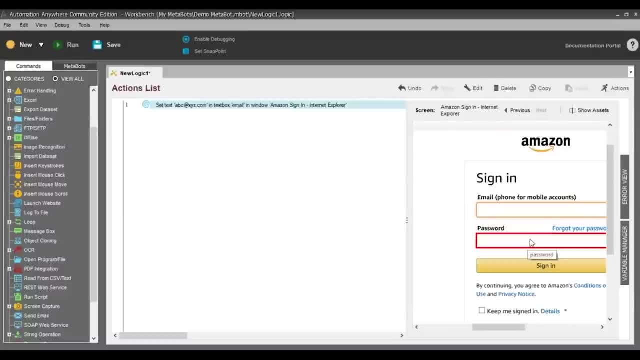 right. So over here I'm just going to mention the email ID, Let's say abcadretxyzcom, And click on add Now. Similarly, I'll do it for password also, So I'll just double click on password. 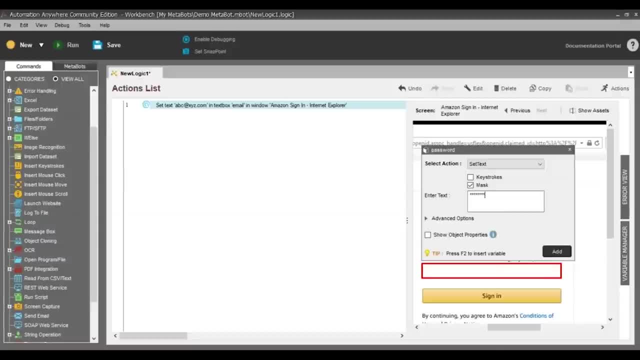 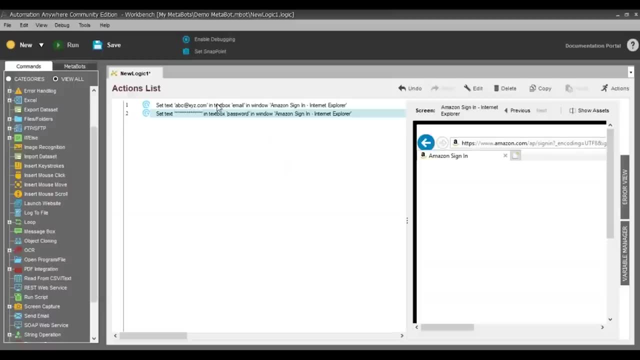 So when I double click on password I can just enter the text again. So let me just enter some random password and click on add right. So, as you can see in the task pane of your workbench you get two commands. that is set text, basically email window of the Amazon sign-in page. 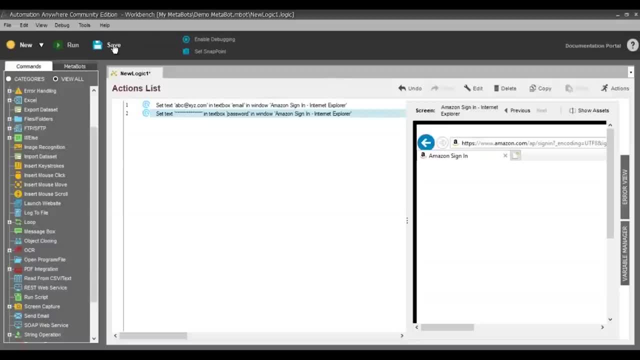 and similarly set password in the password text box in the Amazon sign-in page. Now you can just save your task and let's say we make it demo meta Sign in and click on save. So now, when I execute this task, let's see what the output is. 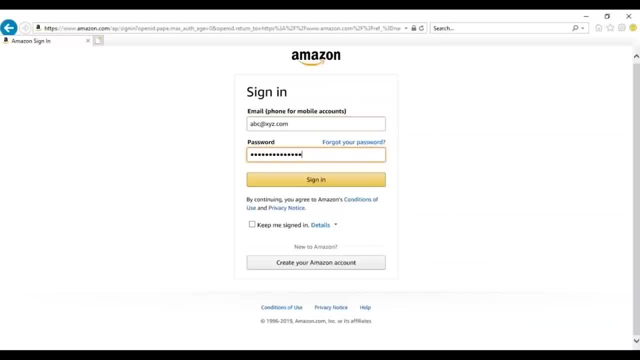 You'll see that you know automatically email ID and the password is entered into the application, right? So that's how, guys, basically you can automate tasks using metabots and taskbots. Basically left to configure a metabot for a specific application and then you have to define the task for it. 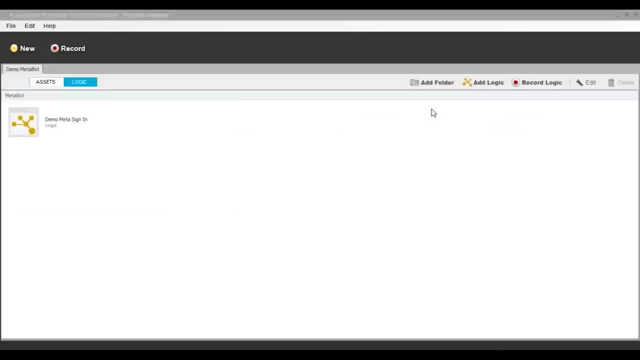 Apart from that, a metabot designer in the logic tab also has other options, like you know: add folder, which was similar to that of this assets tab. Basically, you can add all the logics to the folder and record logic is basically where you can record a specific logic. 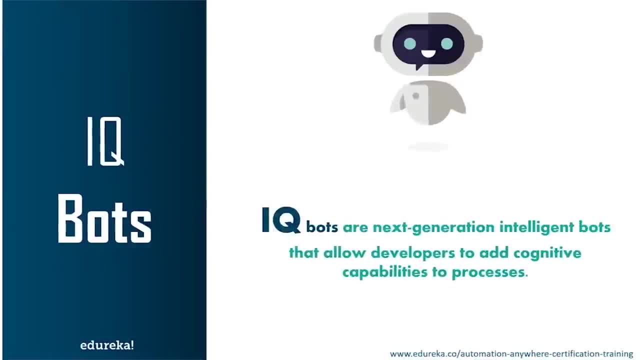 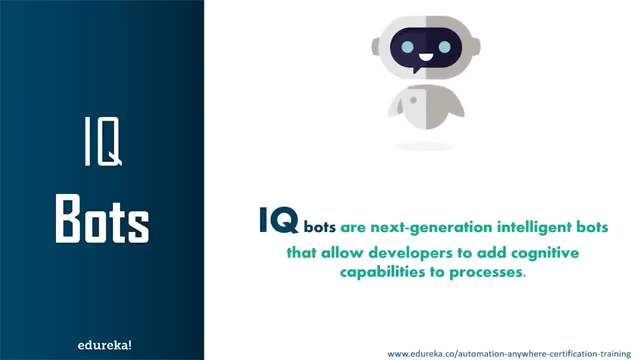 right. So, guys, that was all about metabots. Now let's move forward and see what IQ bots are. So IQ bots are basically the third type of bots provided by Automation Anywhere. So IQ bots are basically the next generation intelligent bots. that allows the developers 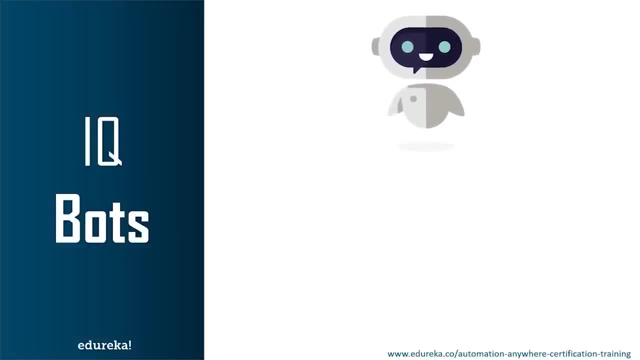 to add cognitive capabilities to processes. IQ bots basically use cognitive capabilities to extract the information from the semi and unstructured data. So it can happen That you know all the data is always not structured right. It can happen that you know. 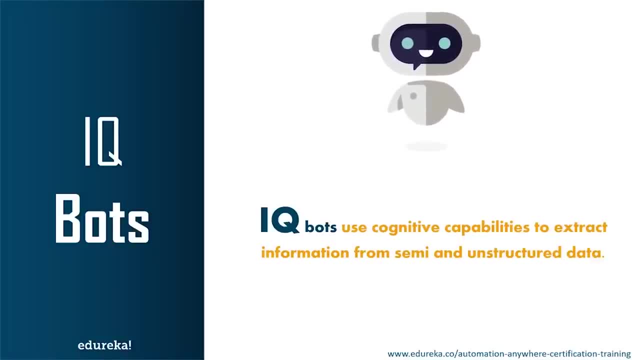 the data collected can be semi or unstructured. So in such scenarios we mainly need IQ bots. So IQ bots also learn to detect patterns, so that the next time the pattern is encountered the bot knows exactly what has to be done. And finally, IQ bots learn and grow smarter with every human validation. 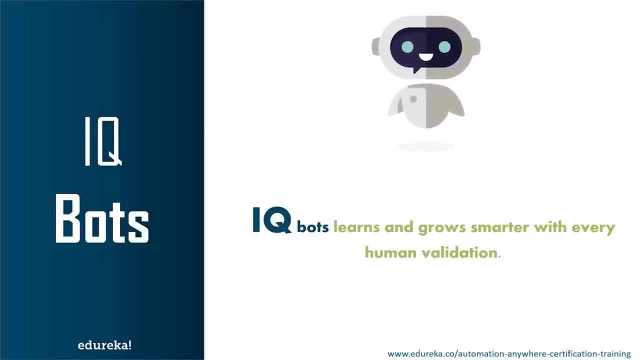 So, basically, IQ bots learn from their learning instances. So, for example, you know if you have to process hundreds of invoices present in a folder and you want to extract the amount, the quantity and the transaction type, Now you don't have to do it for all the invoices yourself. 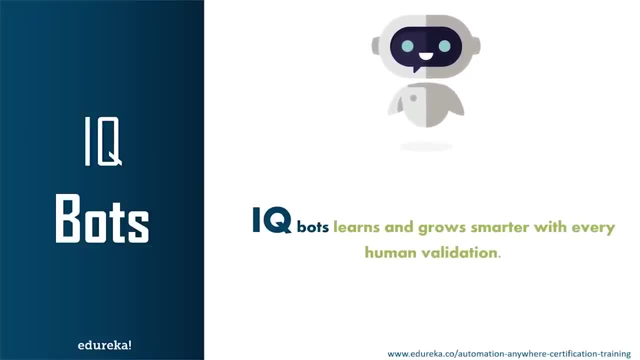 What you simply have to do is you have to do either for one or two, and then IQ bot will learn itself from those particular actions that you do on the one or two invoices- Basically the actions that you repeat- and then it will implement the same actions on the rest of the invoices. 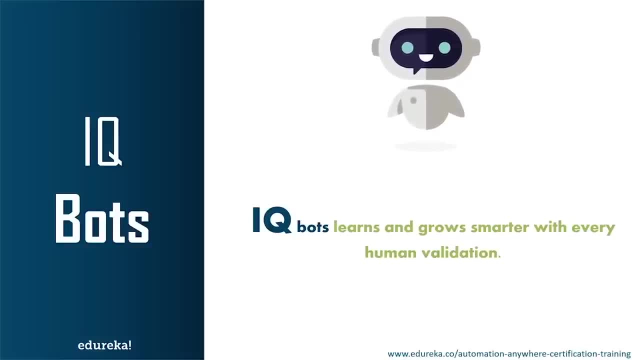 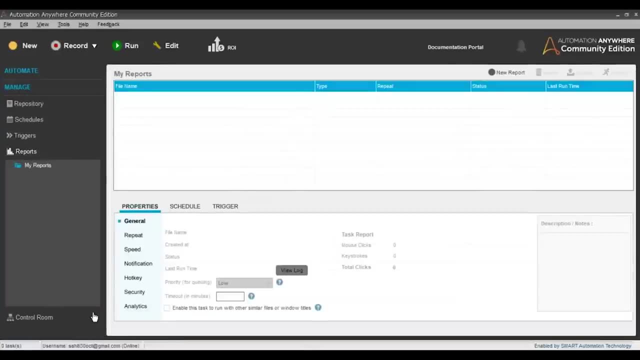 right. So this is a really simple example to understand IQ bots guys. So if you have to launch the IQ bots, what you have to do is you have to go back to your client, go to manage, go to control room, Just log in. 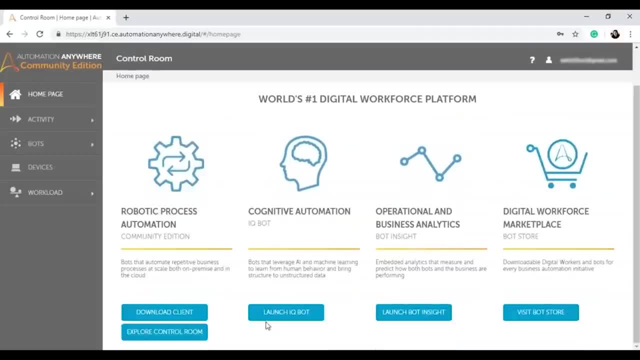 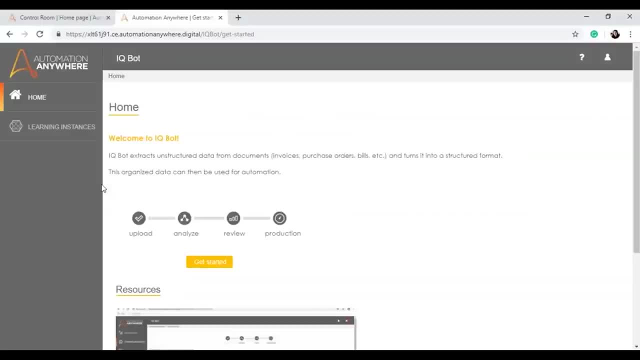 And then, once you log in, what you have to do is you can just go to this option of launch IQ bot, And if you have the license to launch the IQ bot and then create an IQ bot, then you can go forward and get started with it. 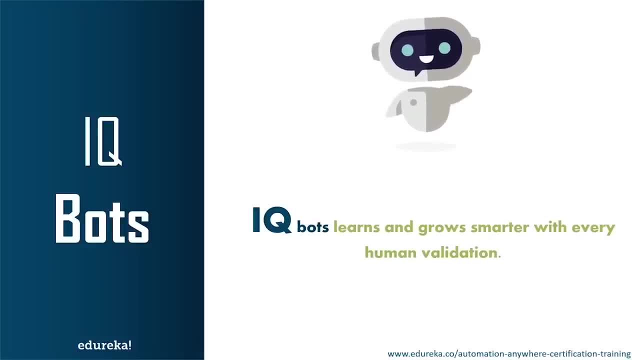 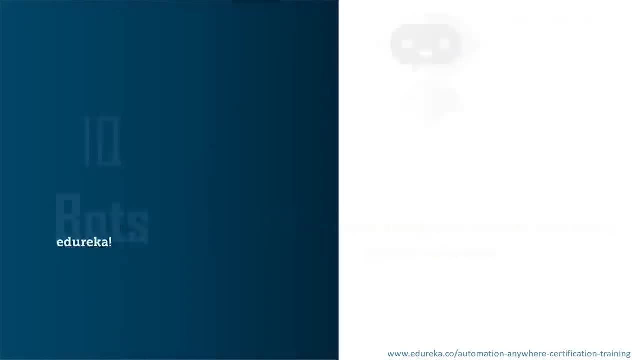 So, guys, these were the different bots in automation anywhere. That is, the task bots, meta bots and the IQ bots. So all of them have their own importance and all of them are really great to learn. Now let's move forward with the final topic. 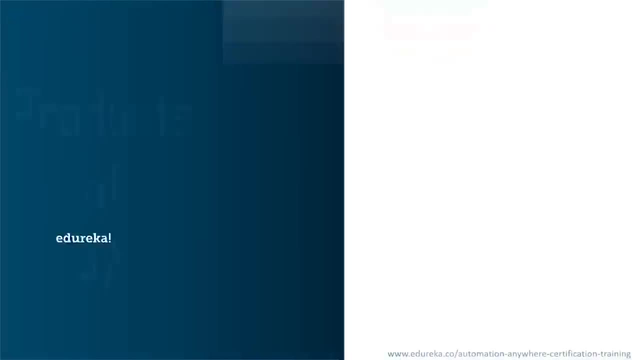 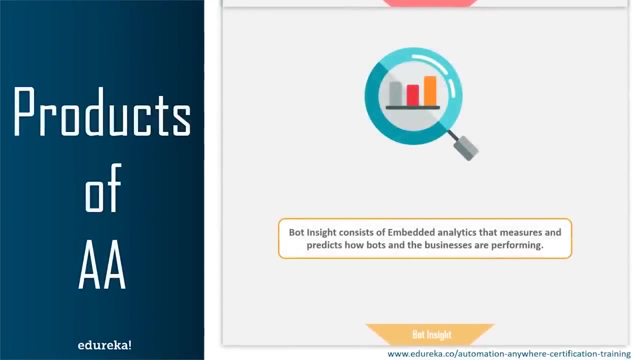 For today's session, That is products of automation anywhere. So the products of automation anywhere are the bot store, the bot farm and the bot inside. So coming to bot inside, the bot inside is basically the analytics part of a bot. So basically in the bot inside you get to understand how your bot is working. 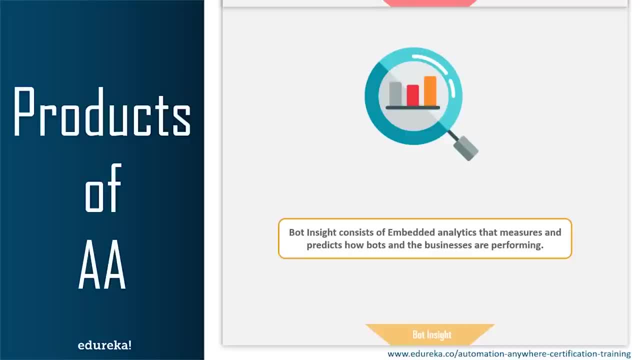 How much GPU is it taking? which bots are running, which bots are failing, Why is it failing? What is the time that it is taking to execute a specific task, Or maybe when is it scheduled, and so on. right, So it's basically the complete analytics part. 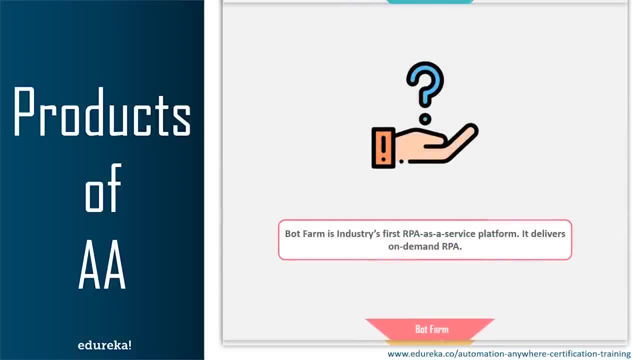 Moving on to bot farm. So basically, bot farm is the industry's first RPS service platform, moving forward with the next one, That is, the bot store. The bot store is the marketplace for bots, So you can shop a variety of ready-to-deploy bots as per your requirement. 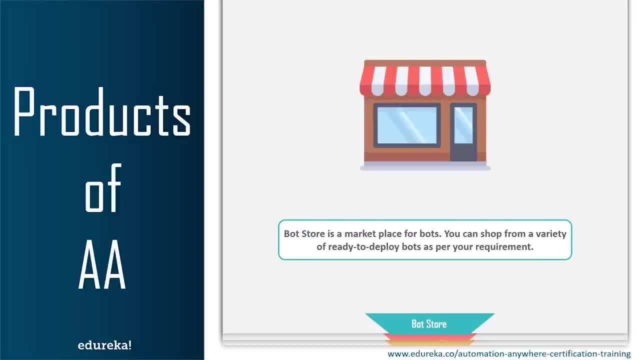 So bot store is where you know where you have hundreds of boards which are ready to deploy. For example, if you want a bot for email automation, so it may happen that you know that is present in the bot store, So you can just search for the email automation bot in the bot store. 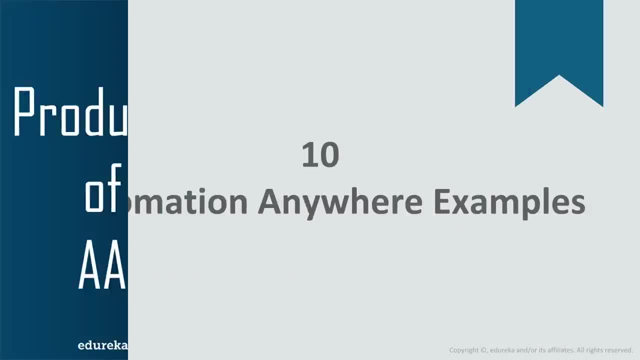 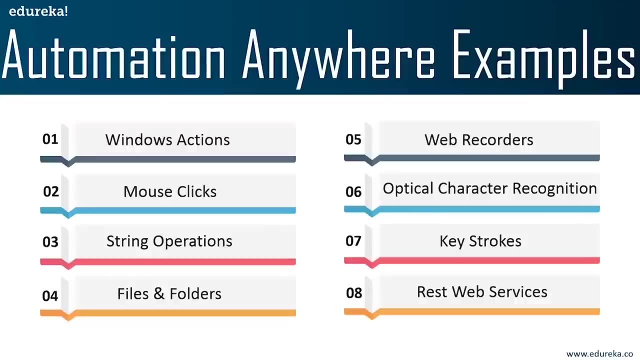 And then you can just deploy that particular bot for your requirement. So in this session mainly I'll be focusing on two subtopics. in the examples In the first part of the section I'll be talking about the different action commands that you can use to automate simple tasks. 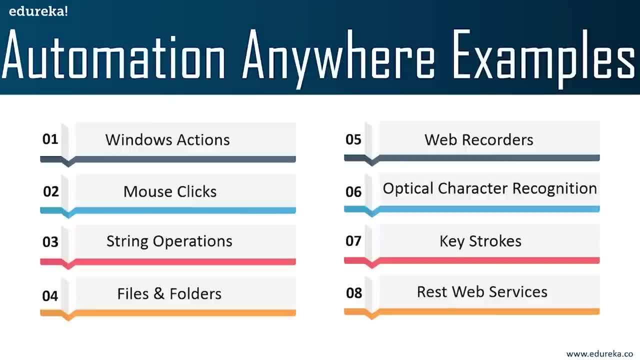 And in the next section I'll show you how you can perform Excel automation and PDF automation. So, starting with the first section, as you can see on my screen, we're going to discuss these few commands and then I'm going to show you how you can use them. 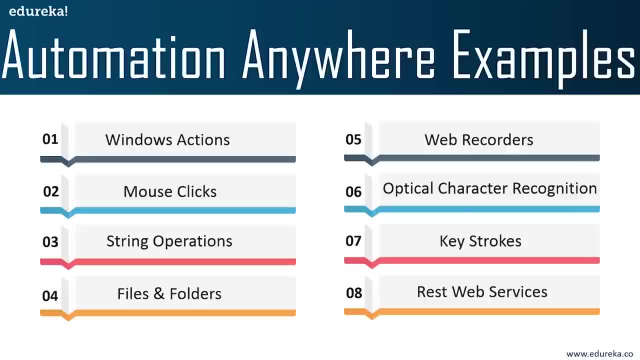 These few commands to automate simple tasks. So we're going to start by discussing the Windows action: the mouse clicks, string operations, files and folders, web recorders, optical character recognition, keystroke and rest web services. So starting with Windows actions first. 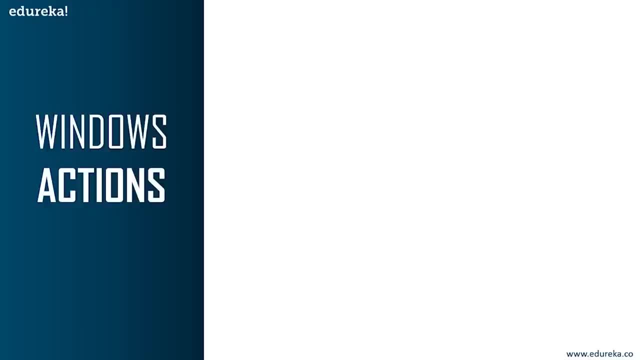 So, basically, when I talk about Windows actions, guys, I mean that you know you have an option in the automation anywhere client where you know you can automate tasks related to your windows, like you know: closing a window, opening a window- Maybe you want to resize a window? 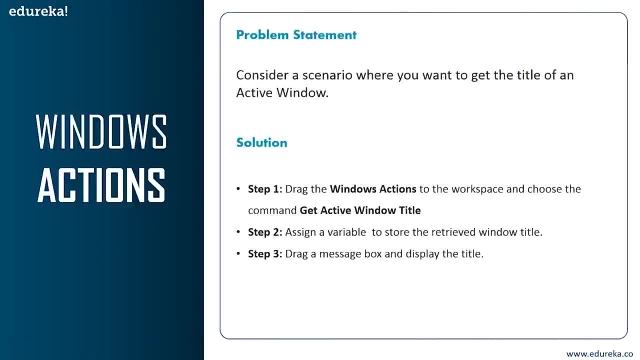 You can also, you know, maximize the window, Minimize the window. So that's what we're going to do. So, in our problem statement, what we're going to do is we're going to get the title of the active window. 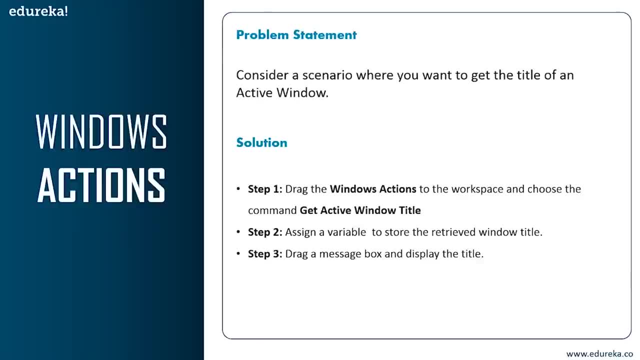 right. So to get that, you're going to follow a few steps, So let me just take you through the steps first and then I'll show you on my automation anywhere. client. So what you have to do is first you have to drag the Windows actions command into your workspace. 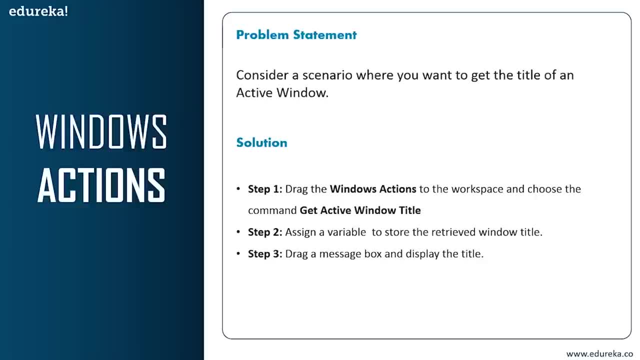 and then you'll have to choose get active window title from there. After that you have to assign a variable to store the retrieve window title and then you can drop a message box into your workspace with the variable inside it so that it displays the output. 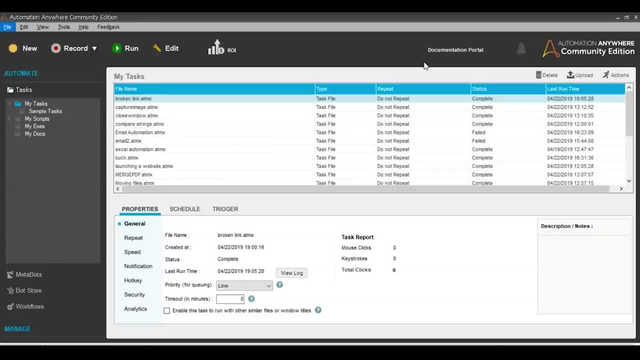 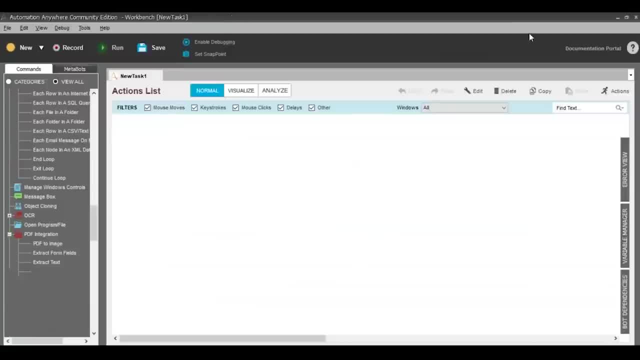 So let's get started. So I just open my automation anywhere client. So this is my automation anywhere client. Now what I'm going to do is I'm going to go to the option new, and then I'm going to choose workbench, and now what we're going to do is we're going to, you know, 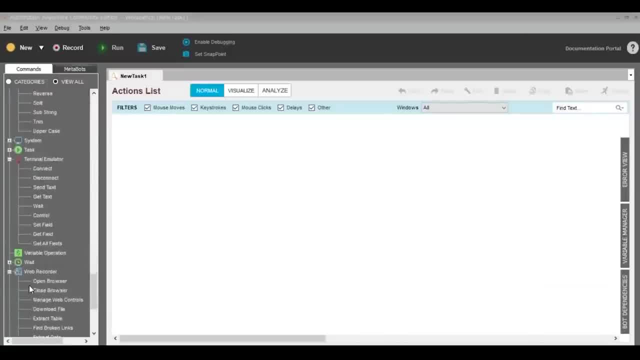 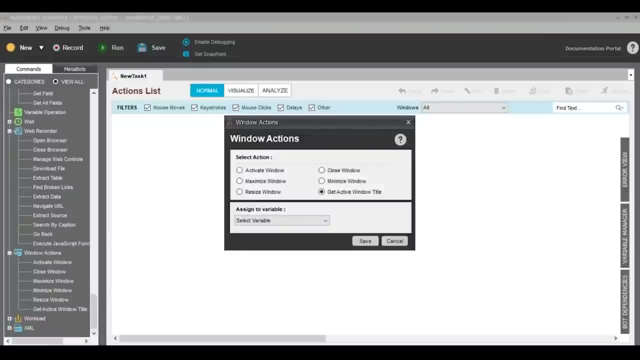 get the active window title. So for that you have to first search for Windows actions, choose the option of, you know, get active window title, drag and drop it over here. All what you can do is you can directly drag and drop the Windows actions and then you can choose an option from there. 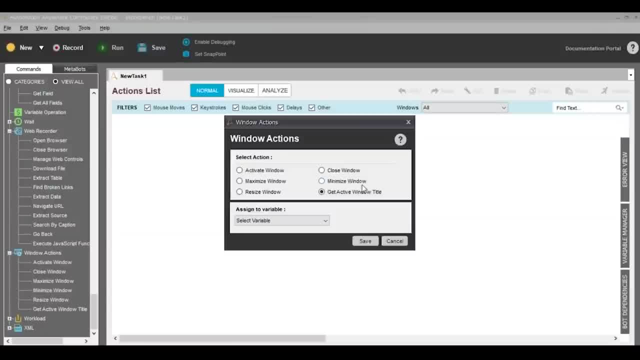 So initially I just dragged and drop the get active window title, So I didn't have to do that. Now what I'm going to do is I'm going to assign a variable, right, So I'm going to select the predefined variables. that is, a system variable. 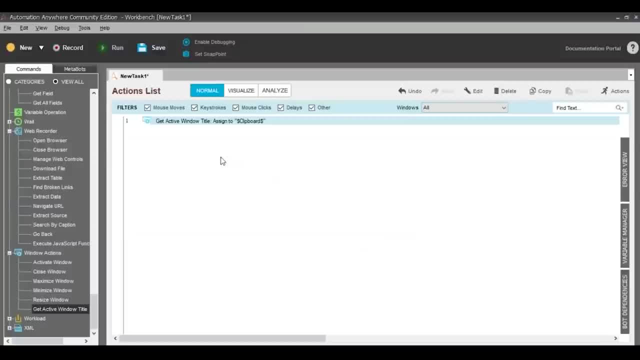 So I'm going to select the clipboard variable and click on save. now, Once I click on save, what I want to do is I want to display the output in the message box, right? So I'm going to search for a message box And then I'm going to drag and drop it over here, over here. 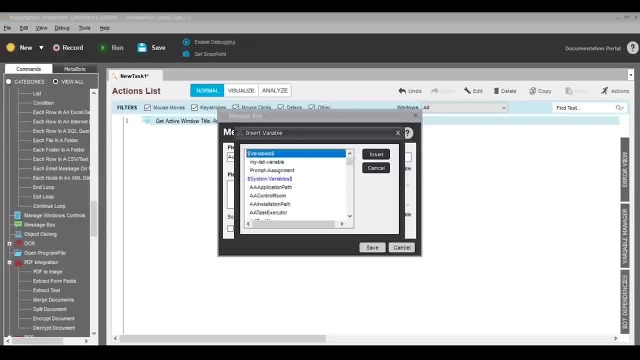 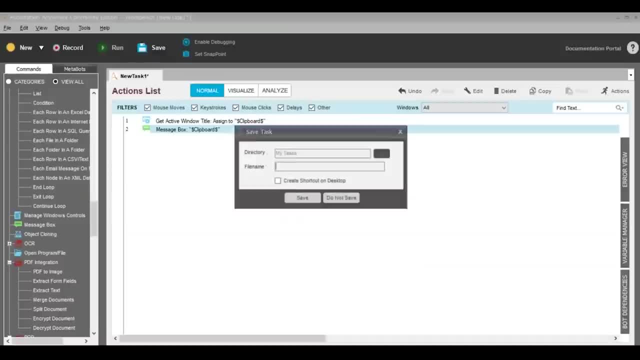 I'm going to press on control F2 and mention my variable. So I had assigned it to the Clipboard variable, right? So I'll search for clipboard variable and click on insert Now. once this is done, I'll save my task. 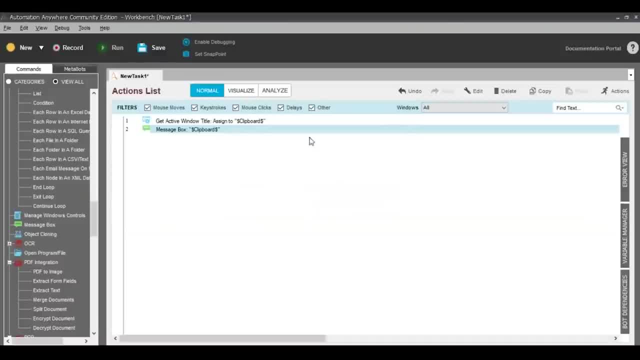 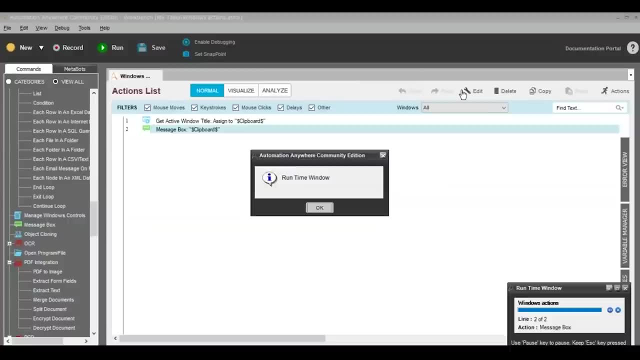 So let's say Windows actions, and then I'll click on save and now I'll run. So, as you can see, my task has been executed and we get the active window title, That is the runtime window, right. That's because you know that particular window is active right now. 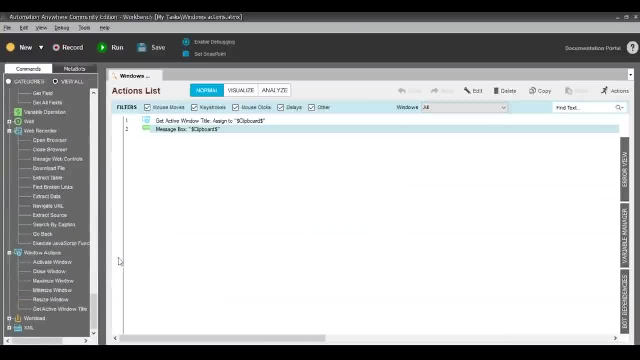 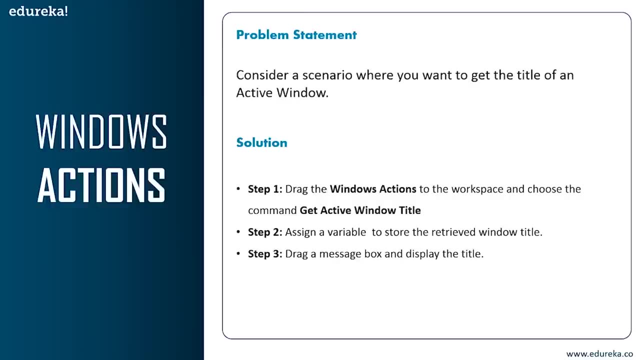 So that's how, guys, you can get your active window title. apart from that, We have also various other options, like you know: activate window, close window, maximize and resize a window. So let's consider the scenario where you know we want to resize a window to any size that 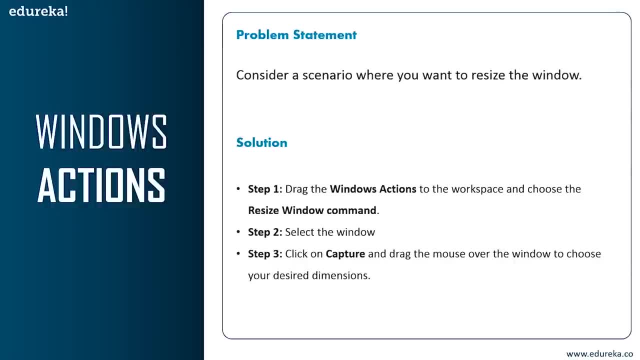 we wish to write, So any dimension that we wish to. so for that, what you have to do is you have to again drag and drop Windows actions command into your workspace and then choose the resize window command. after that You'll have to select the window for which you know you want to resize a window, and 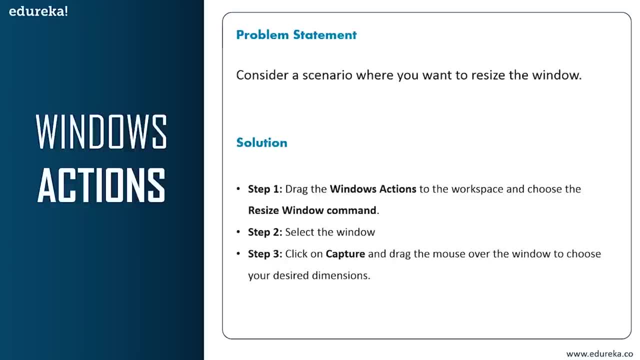 then you have to click on capture and drag your mouse over the dimensions that you know you want the window to be resized, So let's just do that. So for that, what we're going to do is: I'm just going to Remove this part. 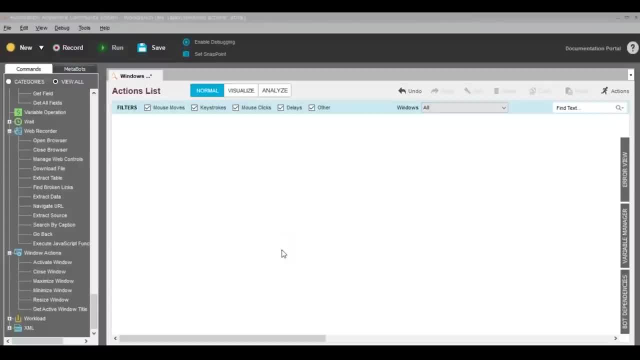 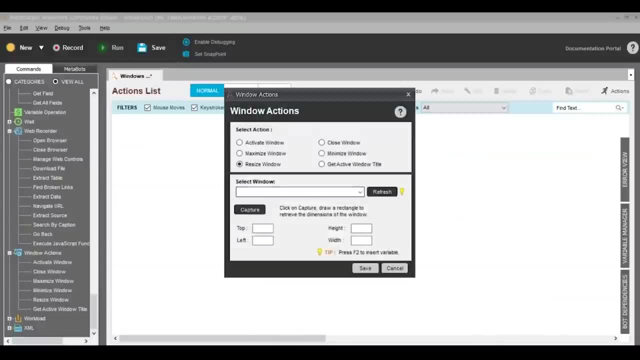 Now what we're going to do is, let's say, you know, we want to resize the window of a notepad file, right? So I've already opened a notepad file. So what I'm going to do is I'm going to drag and drop the resize window command over here. 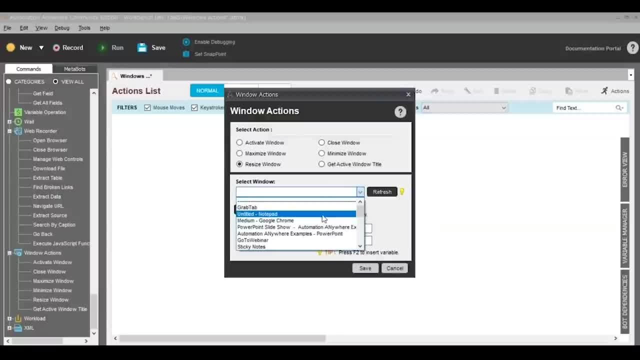 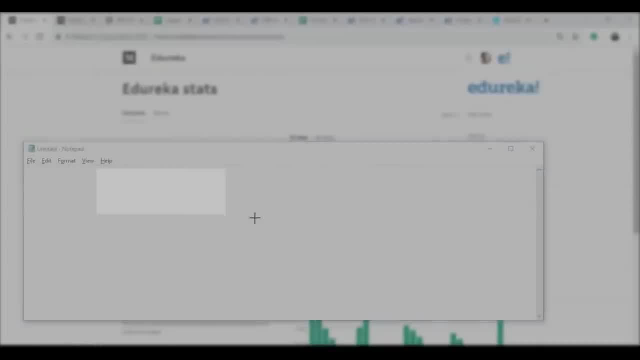 and then I'm going to select the window, right, So I can just select a window. that is my notepad file. Now I'll click on capture and then I'll capture of how much ever size that I want. For example, if you just want from here to here. 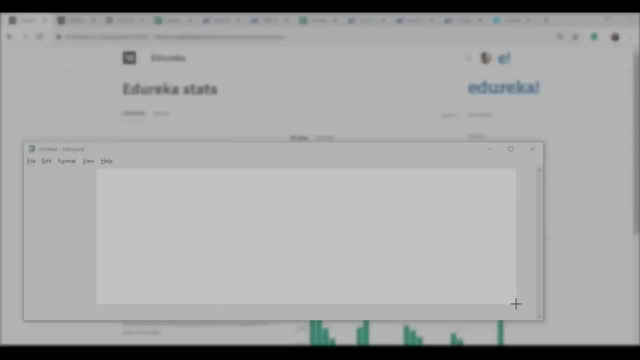 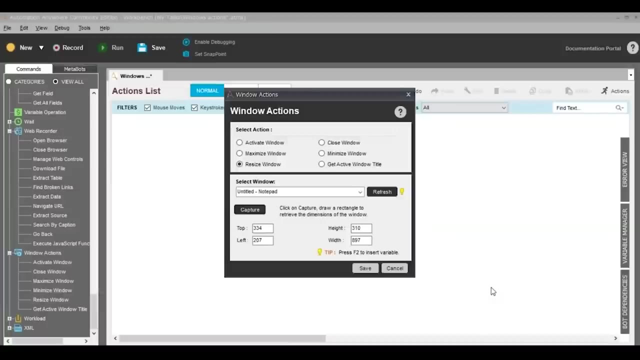 So basically, we want the dimensions of the notepad to be of the selected dimensions, right? So I just want the dimensions to be so small. I'll drag my mouse and then I'll select the dimension. Once you just leave your mouse, click, you'll see that you know automatically dimensions. 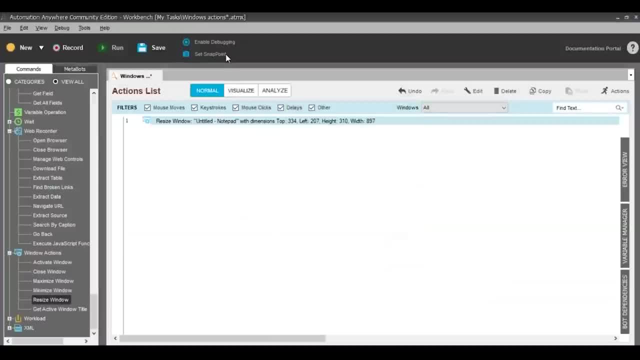 will be there on your dialog box. After that I'll click on save and then I'll again save this task and then I'll click on run. So once I click on run you can see that you know my task has got executed and the 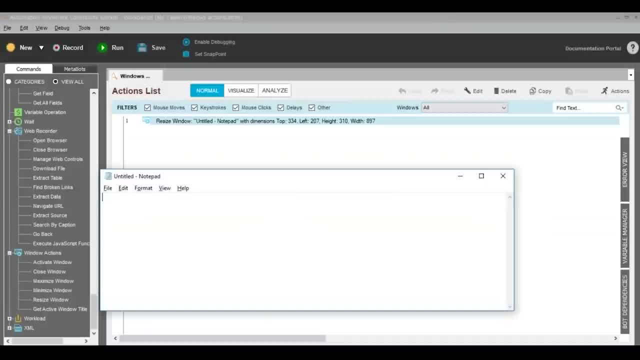 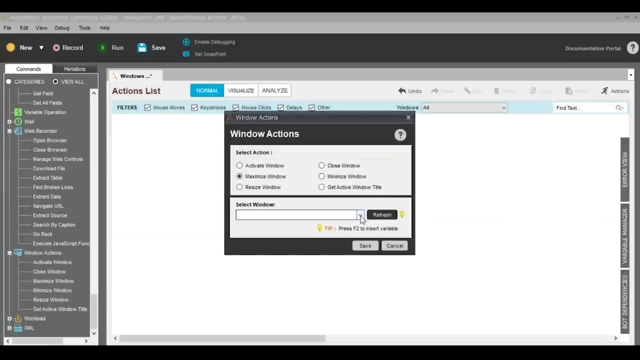 initial notepad file was reduced to this size that we selected. So, guys, this was how you can- just you know- resize a window. Well, obviously, you can Maximize, minimize and close the window. For example, if you want to maximize the window, then you choose the option of. 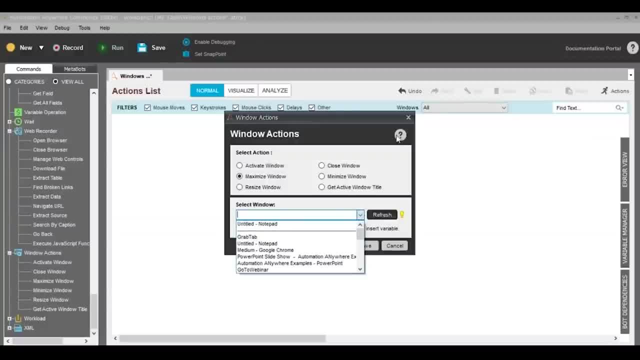 maximizing a window. and then you select the window which you want to maximize and click on save and execute the task. So once you'll execute the task, you'll see that your window has been maximized. So same goes with you know how you want to minimize the window or close a window. 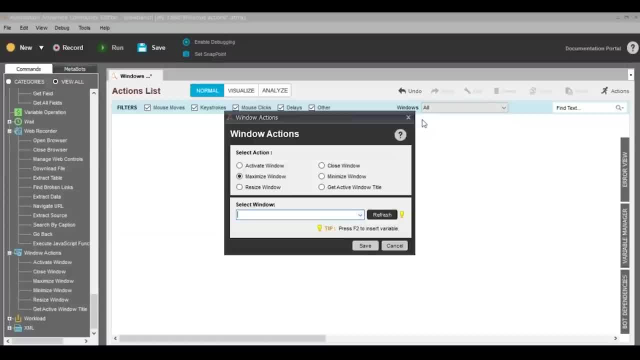 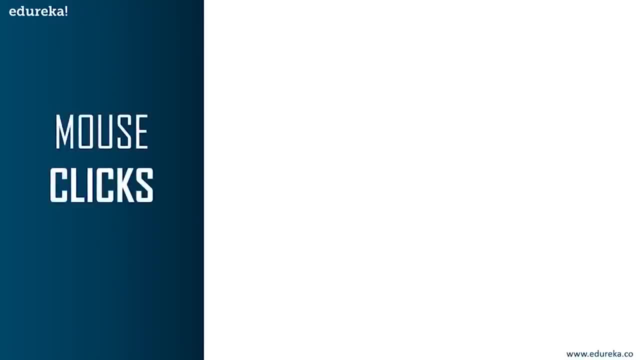 or even activate a window. So that was about windows actions, guys. Now let's move forward with the next topic, That is, mouse clicks. So when I talk about mouse clicks, I mean that you know you can automate the task of where do you want to click on an application, or you know where do you want to click on. 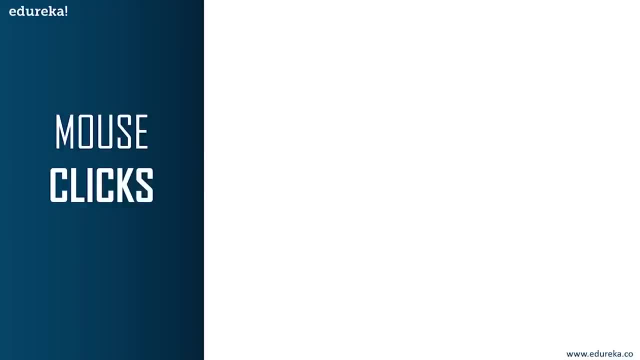 a window. So, for example, if you want to just close a file, or, for example, if you want to minimize a file, you can just automate this task by, you know, choosing the option of insert mouse clicks. So what I'm going to do is I'm going to automate the task of, you know, clicking at a specific. 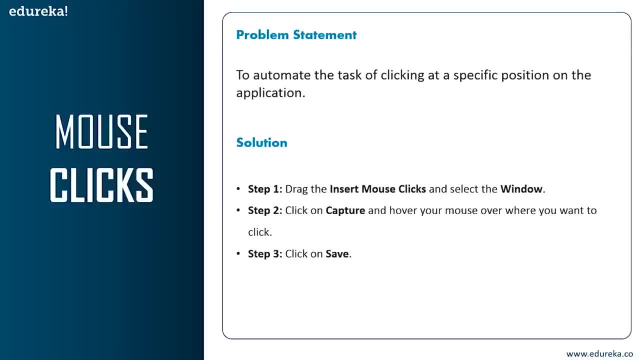 position of the window. Let's say, you know we're going to do it for notepad file, So to do that you'll have to follow a few steps. So basically you'll have to drag the insert Mouse clicks command into the workspace and then select the window. 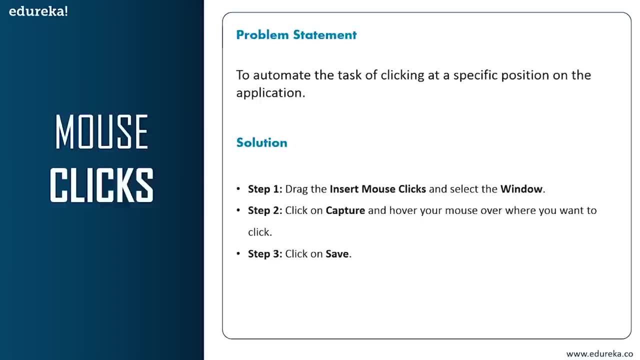 So we are. I'm going to show you for notepad, So I'm going to select the notepad and then I'll click on capture. So basically, I'll have to click on capture and then hover my mouse over the closed symbol or minimize the maximize symbol, according to what I want to do, and then I'll click on. 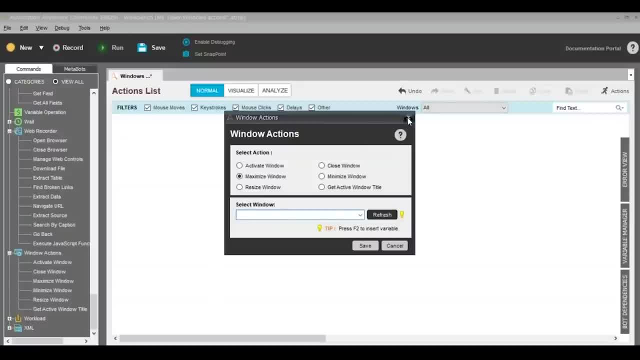 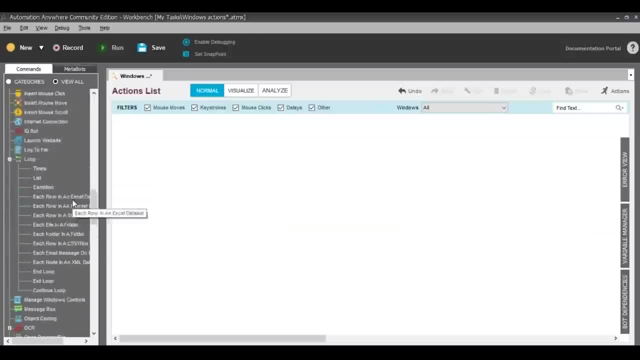 save. So let's just do the same for that. What I'm going to do is I'm just going to close this part over here and then in the same task file. What I'm going to do is I'm going to go for insert mouse clicks. 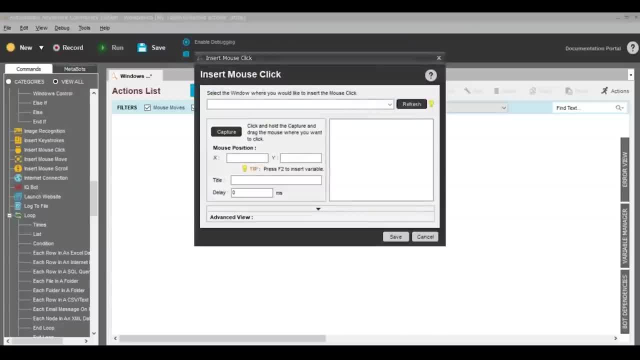 I'm going to search for insert mouse clicks over here. I drag and drop it over here. next I'll just refresh it so that you know all my active windows are visible in the drop-down list and then you can see. you know, I have a notepad file, right? 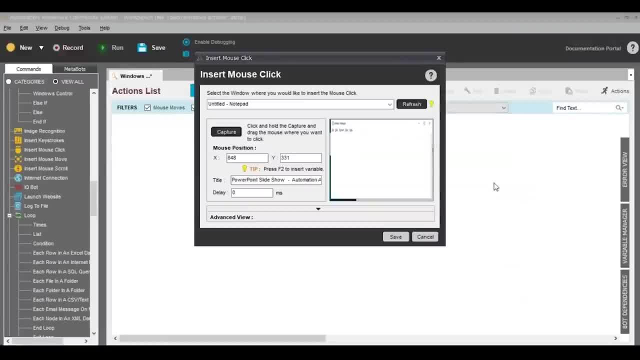 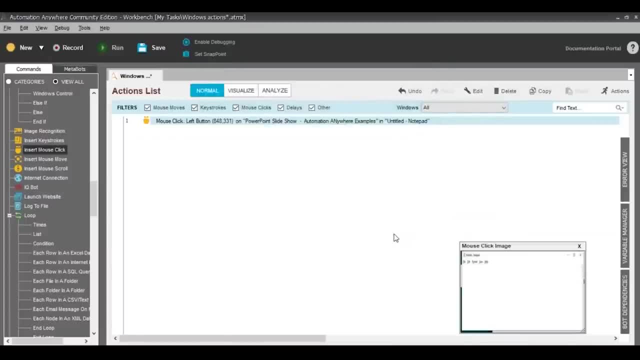 So I'll select that notepad file, I'll click on capture and drag my mouse over the close button right- So you saw how that's happening- and then I'll click on save right. So basically that's how you can see in your preview that you know this particular file. 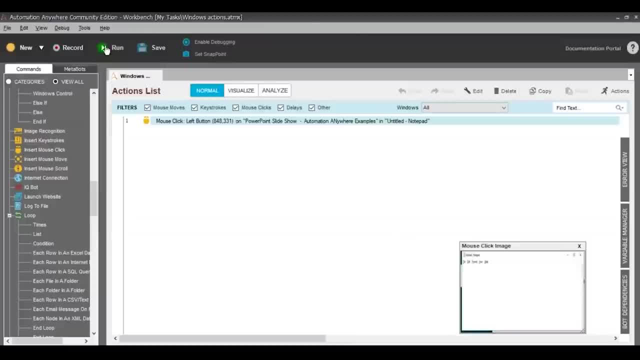 would be safe. Now I'll just save this task again and click on run. So as I click on run, you can see that you know my task got executed And my notepad file got closed. So, guys, that's how you can use the insert mouse clicks. 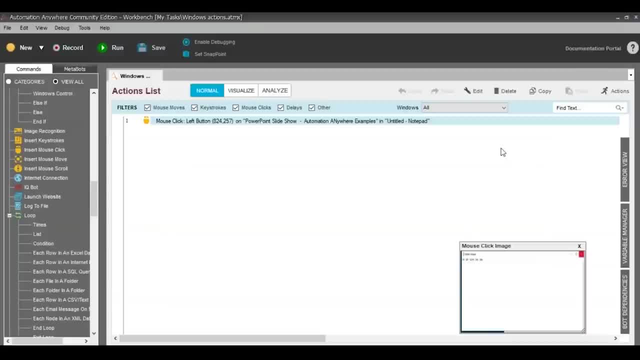 It's really simple to use these mouse clicks I just showed you for a notepad file, For example. you can also, you know, define it for an application, where you want to click on a specific application and then you want to click to go somewhere else, right? 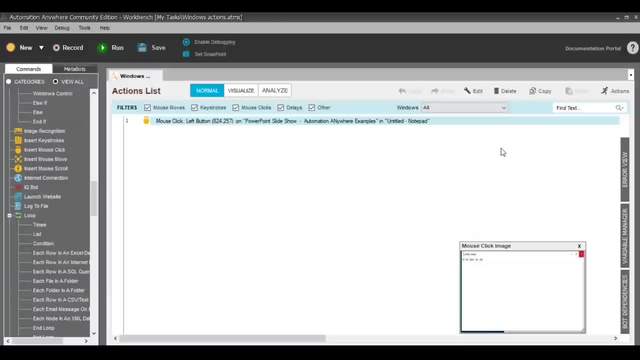 So you can use all these kinds of simple actions in loop actually. So, for example, if you're searching for something on Stack Overflow, right, And then you want to search something based on your tags, So what you can do is you can just, you know, go to the launch website. 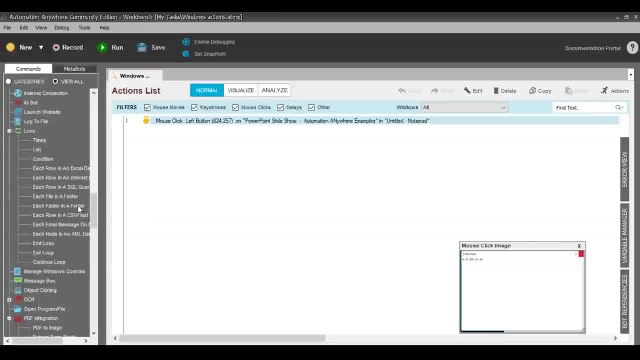 Activity, or you can also go to the web recorder where you got to record something for that. What you can do is you can just use the web recorder, then mention the URL. The URL will open. Now what you want to do is: you want to specify your search according to tags, right, 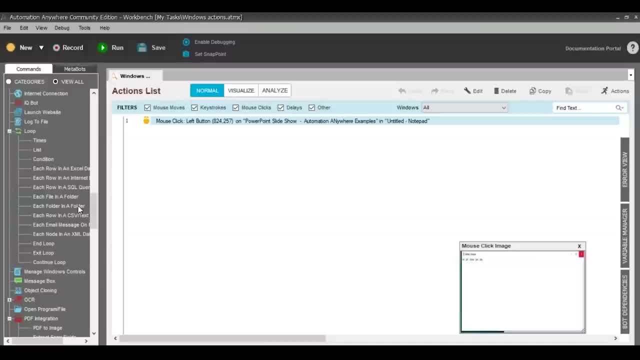 So for that again you can mention that you know in the search bar. So you basically will have to click on the search bar right. So for that you can use the insert mouse activity and then you can make sure what you want to. 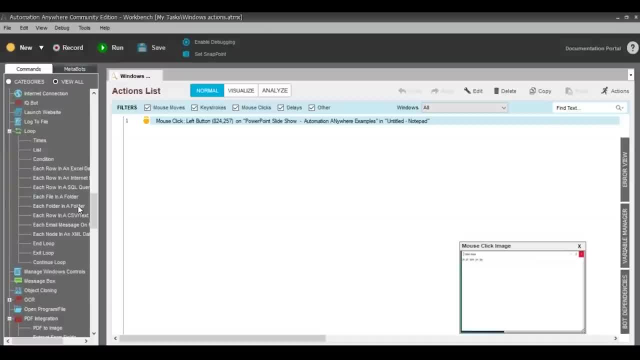 type again, You'll have to press on enter right. So for that either you can use the keystroke or you can use the insert mouse click to click on the arrow On the right side. So that's how you can use a combination of, you know, different actions or commands together. 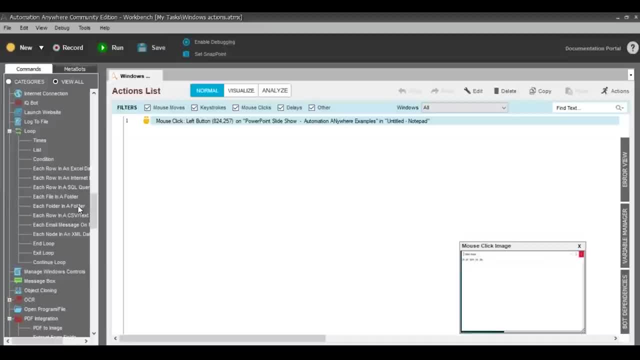 to automate a large, humongous task. Well, in this session I'm going to focus on, you know, simple, simple tasks, so that you understand how to use this task mainly, and then we'll combine all these actions and look into the Excel and the PDF automation on that node. 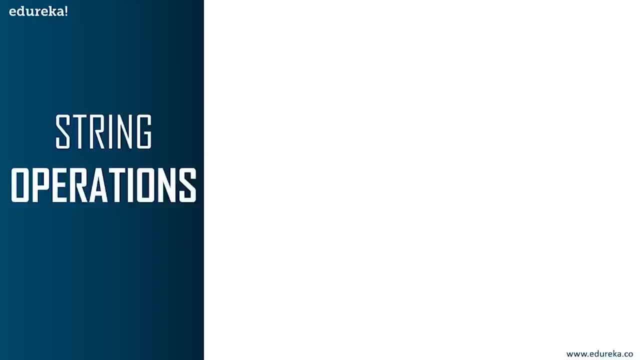 Let's move forward with the next operation, That is, the string operations. So, as we all know, string operations are really important in today's Market because all programming languages or all automation tools, Everything is related to, you know, string operations. So in such scenarios, string operations are really important to use in automation anywhere. 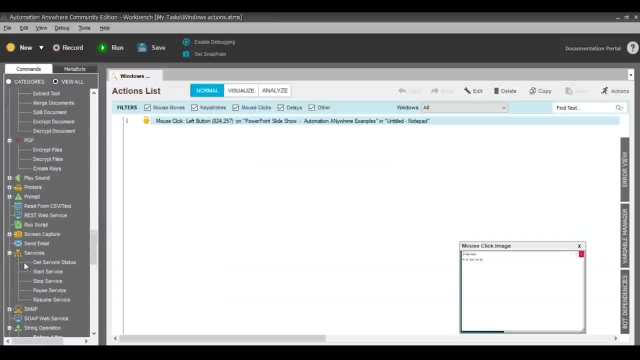 If you look at the client, I'll just open and show you that you know when you search for string operations, you can see that you know you have various operations on the left hand side. That is basically the before, after: compare, find, join, length, lowercase, replace, reverse. 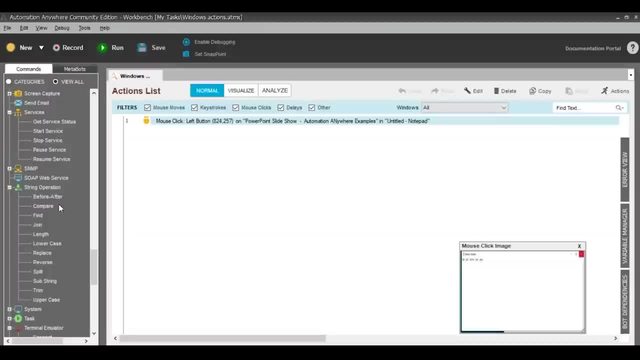 split substring, trim, uppercase it. So basically by that what I mean is: you know you can either compare two strings, or you can find a specific string, or you can convert String from lowercase to uppercase. Maybe you know you want to just find the substring from a string and replace some values. 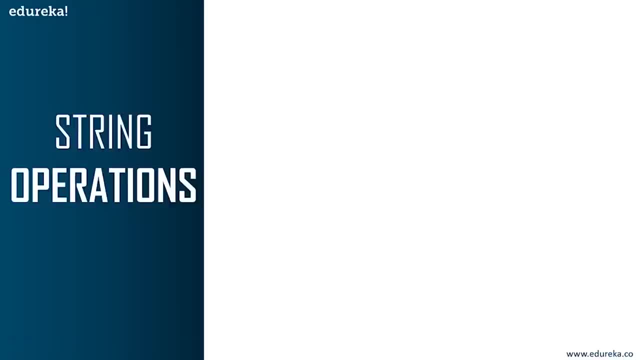 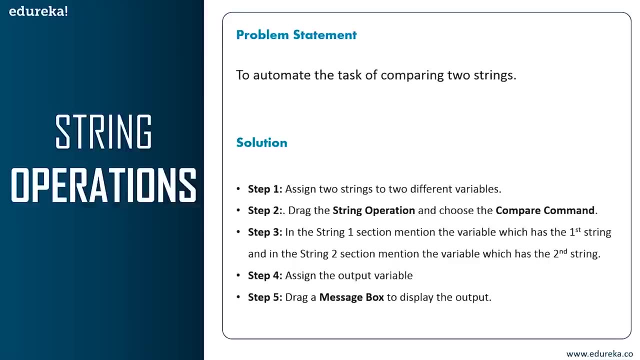 from the specific strings and so on, So you can do different kinds of operations. today in this session will focus on how you can automate the task of comparing two strings. So the steps are really simple. to compare two strings, You first have to assign two strings to two different variables. 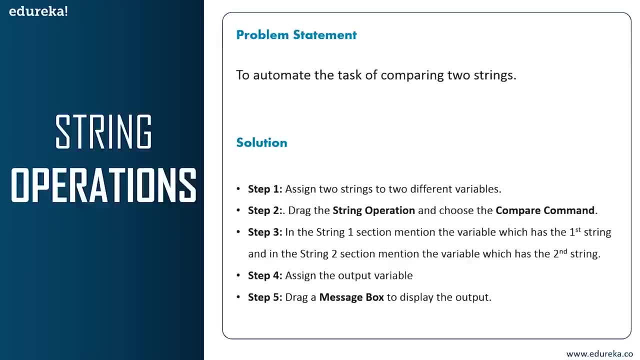 Then you have to drag the string operation command and then you have to choose the compare command. after that, in the string one section You have to mention the variable for the string one and in the string two section you have to mention the variable for string two. 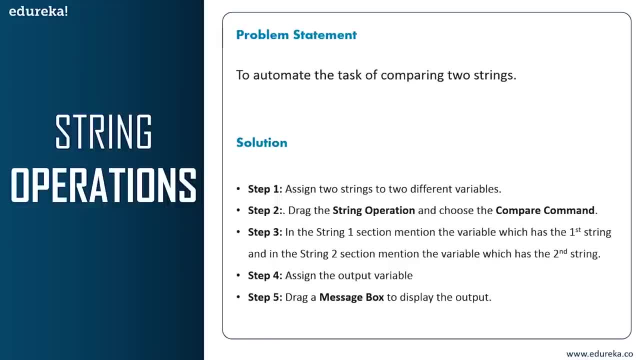 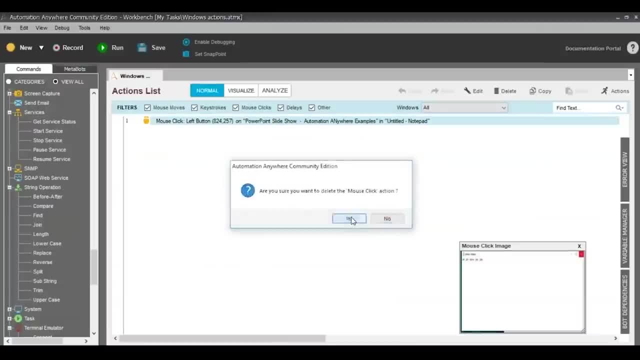 Then you'll have to assign a variable for the output, and then you can use the message box to display the output. So what I'm going to do is I'm just going to shift back to my workbench over here, and then what I'll do is I just leave this part. 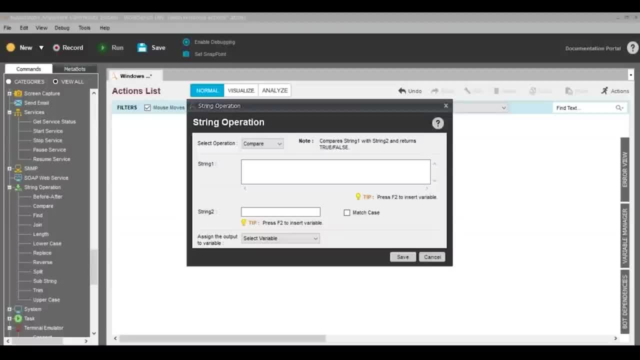 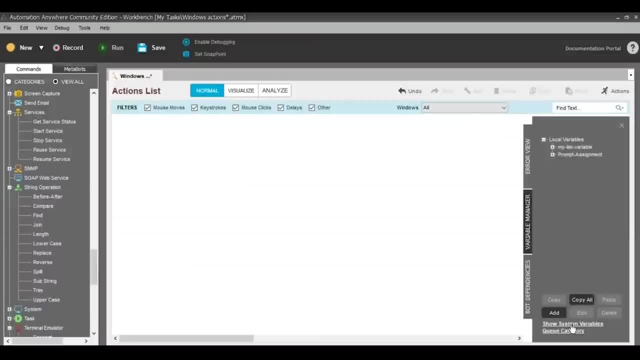 Now what I'll do is I'll, you know, drag and drop the string operation for compare. but before that what we have to do is we'll have to assign two variables, right. So for that, what I'll do is I'll go to the variable manager, add two variables, right. 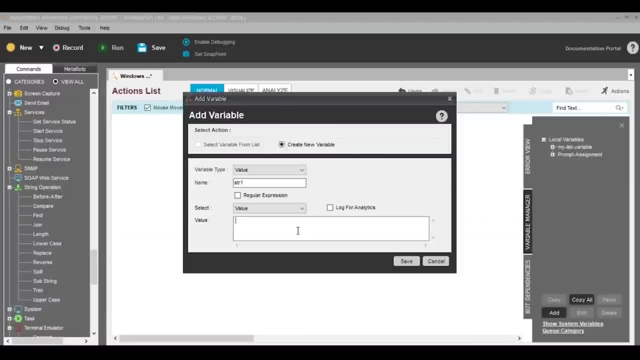 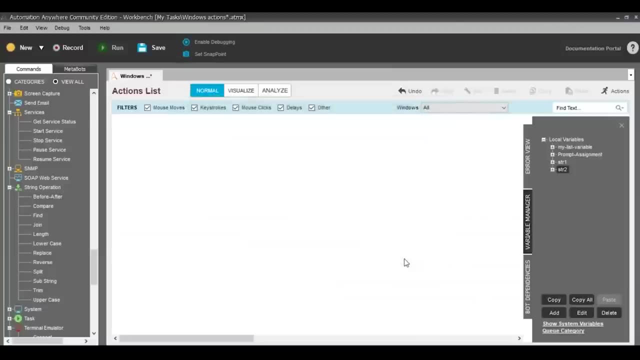 So let's say I add a variable str1.. And let's say value will be high from edureka, and then I'll click on save. then I'll again add a variable str2.. Let's say welcome to edureka, and then I'll click on save now. 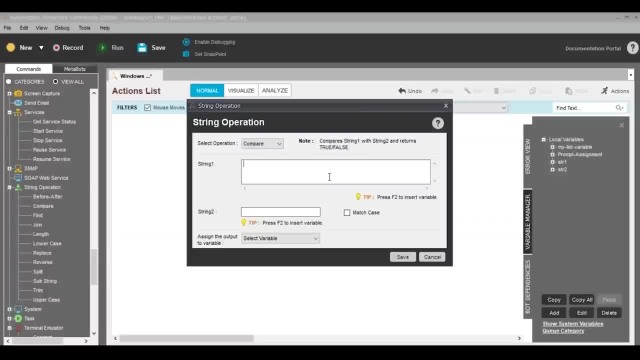 What I'll do is I'll drag and drop the compare command and then in the string one section I'll mention str1 right. So for that I'll press on control f2, mention str1 and click on insert similarly in the string to my section. 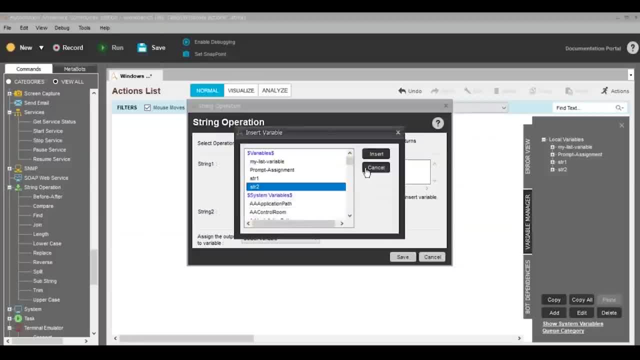 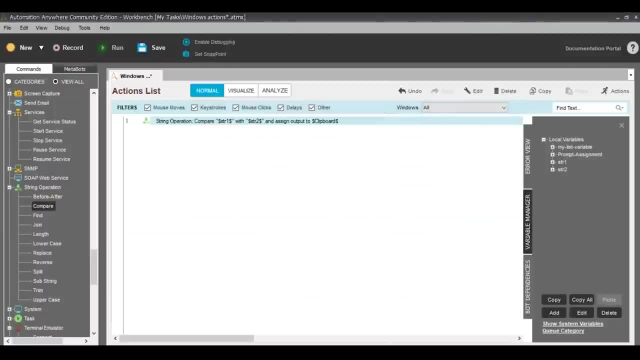 I'll mention str2.. So I'll press On control f2.. I'll choose str2 and click on insert. after that I'll select the variable to assign the output. Let's say, you know we choose clipboard and then I'll click on save now. 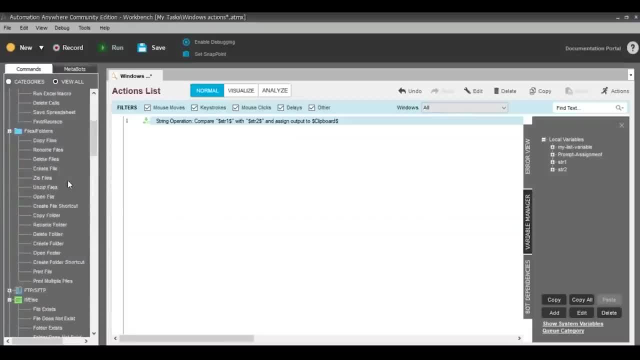 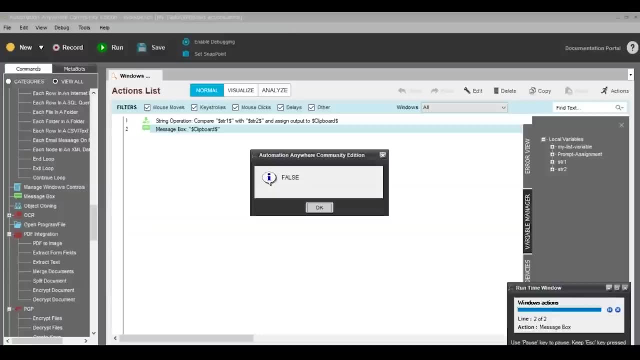 What I'm going to do is I'm going to search for a message box And then I'll mention the output variable. that was clipboard. I'll click on save. once I'm done, I'll save this task and then I'll execute So you can see the output as false. right, that was because you know both are strings with. 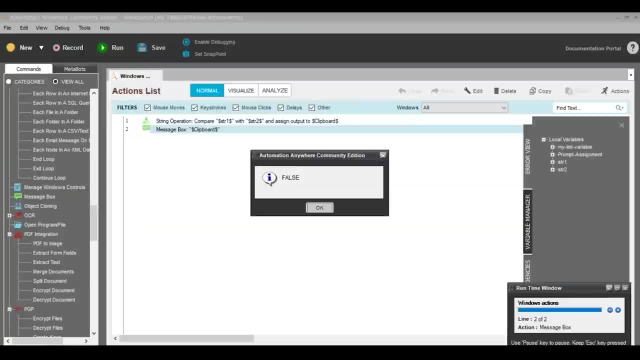 different. the string one was high from Edureka and string two was welcome to Edureka, right? So since I both the strings were different, our output was false. else, if a string was same, then you know the output would be true. So let me just show you that scenario also. 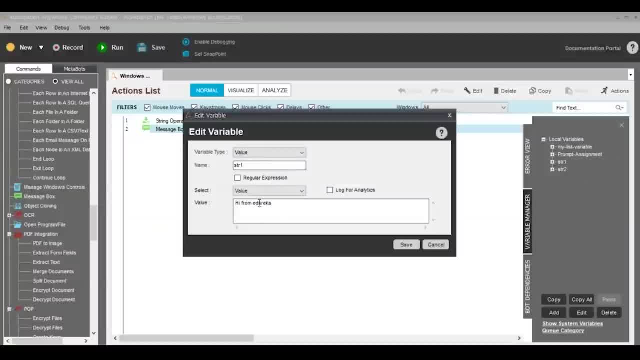 So what I'm going to do is I'm going to edit this variable- Let's say, you know, we just mentioned Edureka- and click on save over here Also. I'm going to just mention Edureka and then I'll click on save then again. 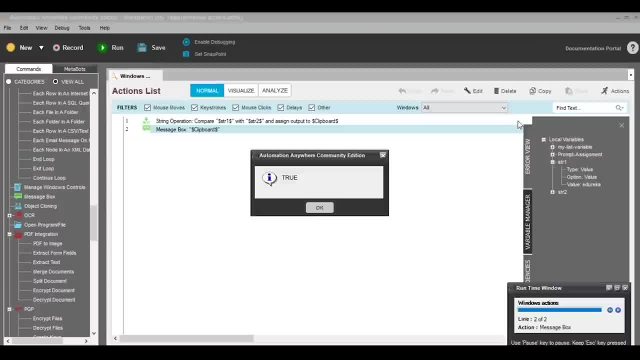 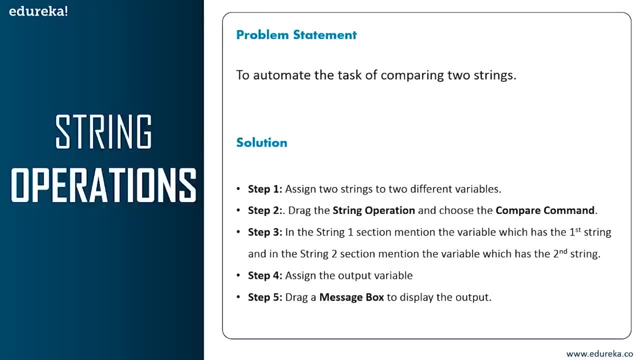 I'll save this task And then I'll execute, So, as you can see the output, the output is true. that was because you know both the strings had the same string, that was Edureka. So that's how, guys, you can use the string operation to compare two strings. 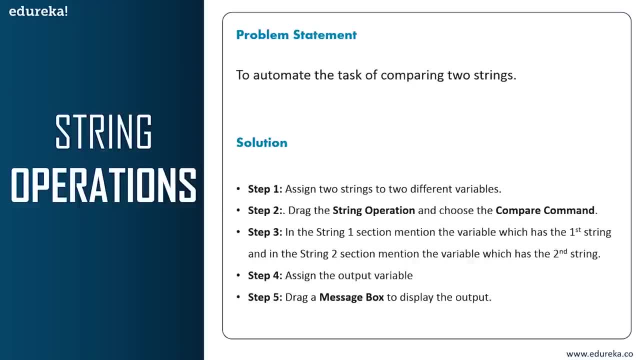 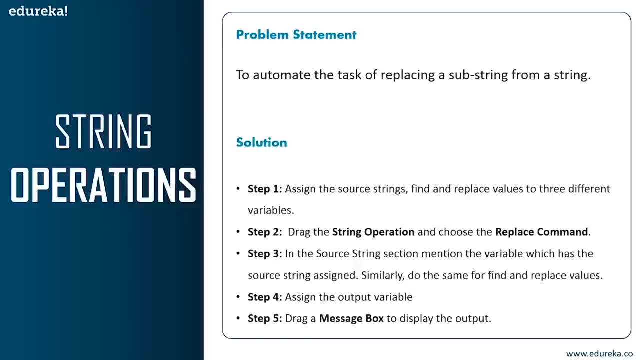 Now let's look into one more scenario of the string operations. That is how, you know, we can automate the task of replacing the substring from a string. So, for example, in the string of, you know, Edureka, let's say we want to replace, you know. 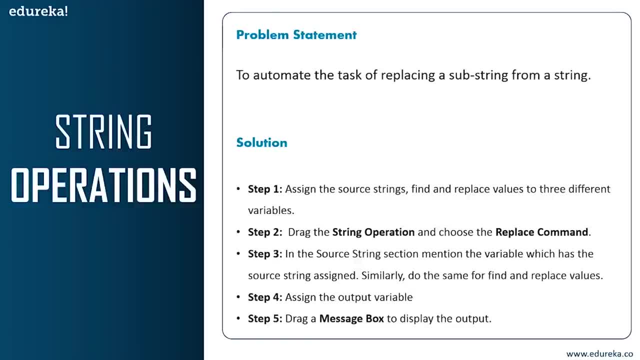 Edu to something else like, say, tick right. So how do you replace that? So for that, it's really simple. Again, you have to follow the steps that you can see on my screen, that is, you first have to assign the source strings, find and replace values to three different variables. 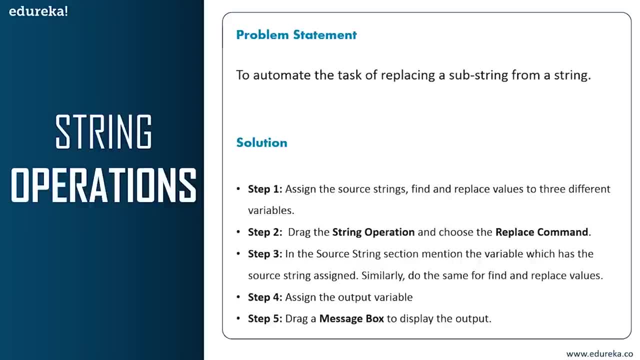 After that you have to drive the string operation command and choose the replace command. in the source section You have to mention the source variable and then in the find and replace section you'll have to mention the find and the replace variables. where you know you basically find from a 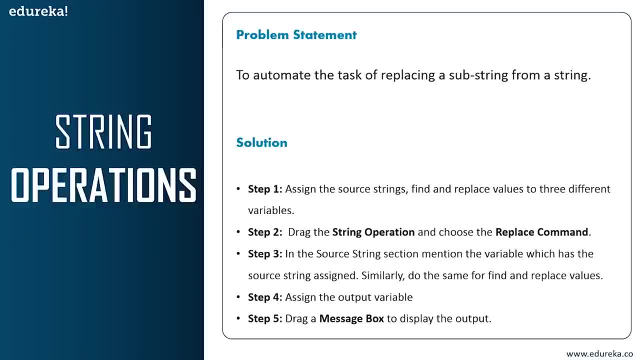 specific string, that is basically Edu, that we're going to find and then we're going to replace it with tick. after that will assign the output to the variable and then drag a message box To display the output. So let's just do the same. 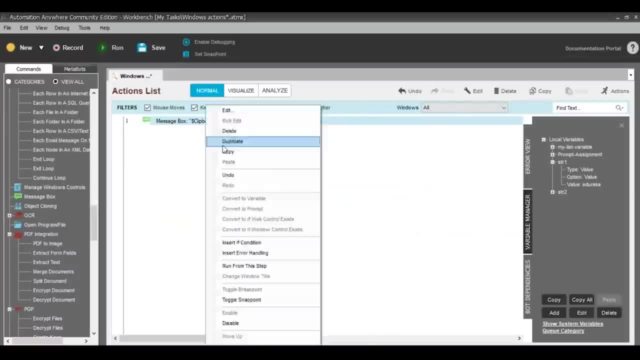 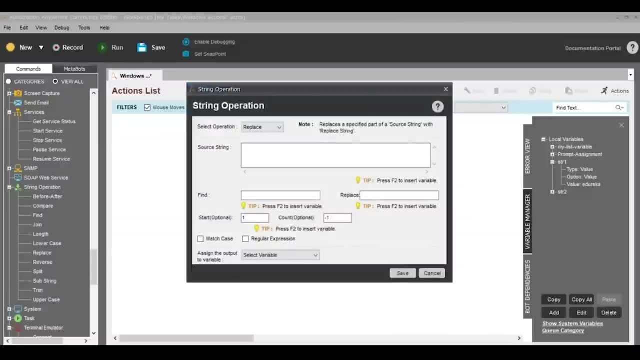 So for that, what we'll do is I'll just remove this part And then I'll again search for string operations and then drag and drop replace. when I drag and drop replace, you can clearly see that you know we need three variables, that is. 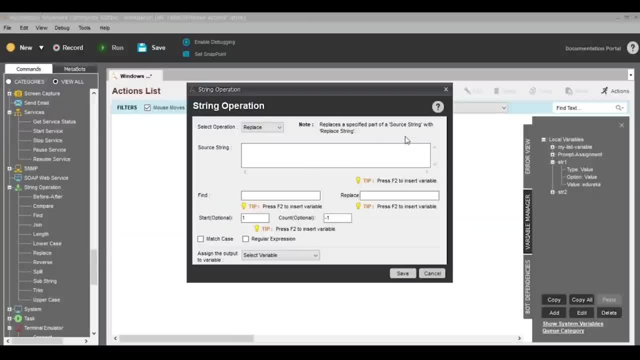 the source string find and replace. So initially, if you do not want to use variables, then you can also just mention the text. Let's say you know I want to mention the text Edureka and then I'll mention Edu in the find section. 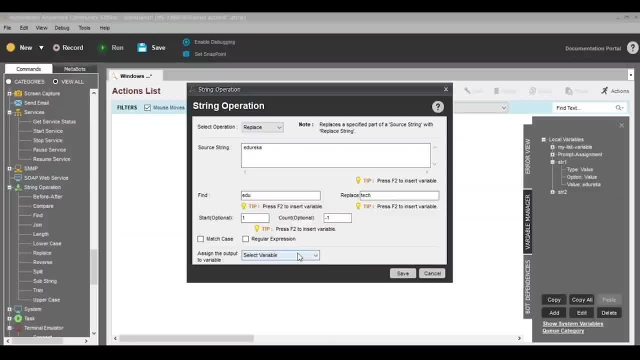 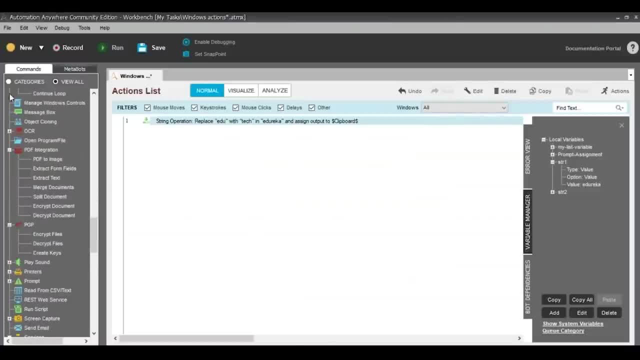 I'll replace it with tech, and then what I'll do is I'm going to assign the output to a variable. Let's say we assign the output to clipboard variable, and then I'll click on save. after that I'll drag a message box. 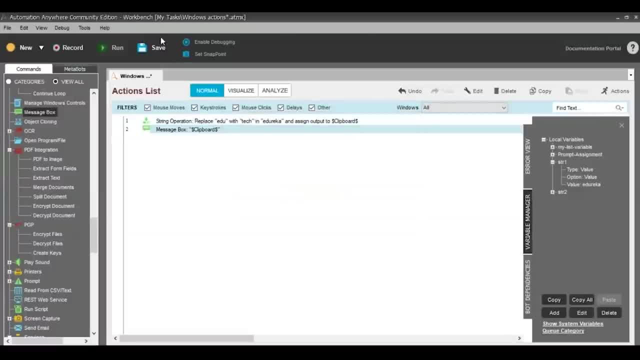 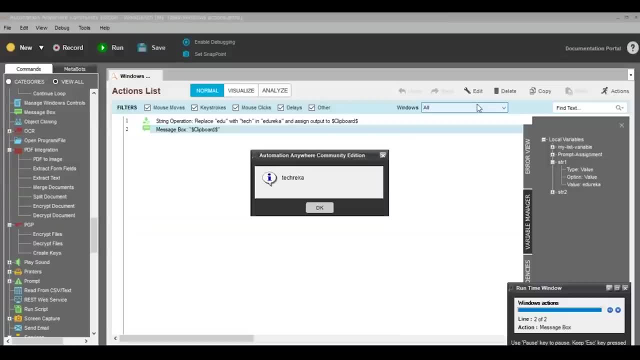 Mention the output variable and click on save again. after that I'll save this task and click on run. So basically, for my spring Edureka we had to find Edu, and then that had to be replaced with tech. That's what got replaced: the output. 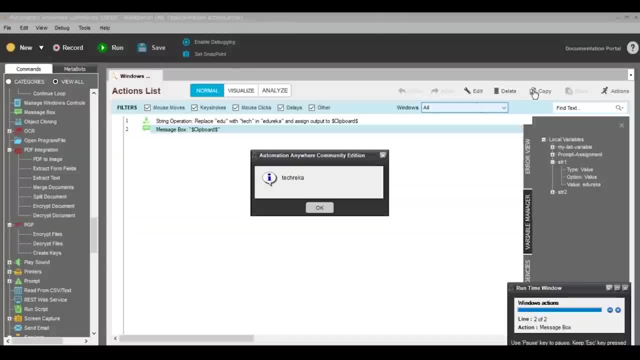 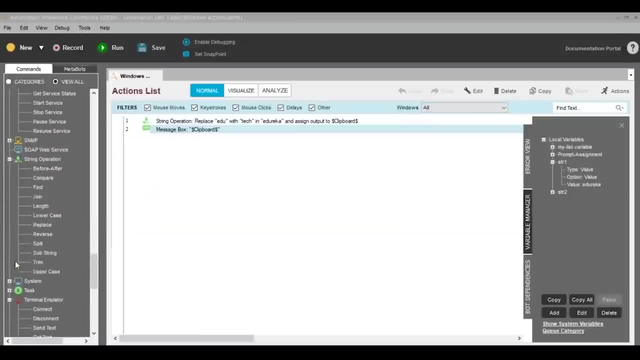 This tech record. that is basically. you know, I just replaced Edu to tech. So that's how, guys, you can replace strings. Well, guys, these are only two operations that I showed you with strings. Well, you can explore more and then you can play around with a lot of string operations. 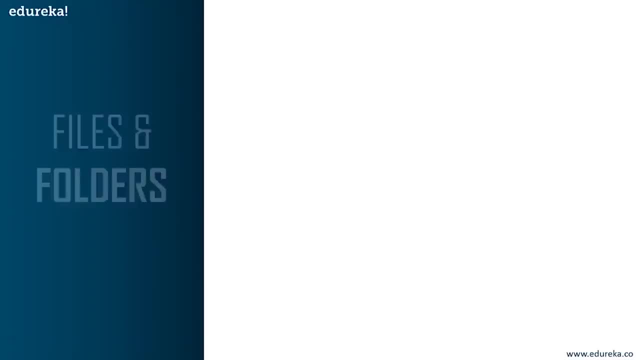 even in the complex automations. Now let's move forward with the next command. that is basically files and folders. So files and folders are also one of the most important topics that need to be covered in any automation tool. So, as all of us deals with, you know any n number of files every day. 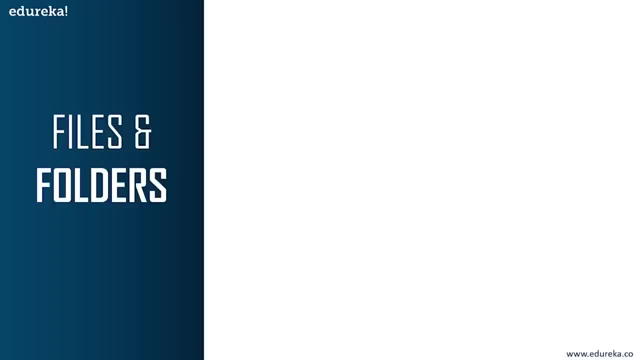 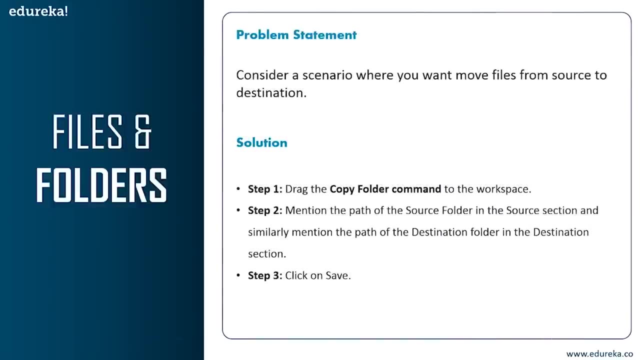 We have so many files and folders stored in our local system and maybe even on the cloud, and so on, Right? So how do you think we can automate this task of you know, transferring files and folders automatically from one folder to another folder and maybe, if you just want to zip a folder, 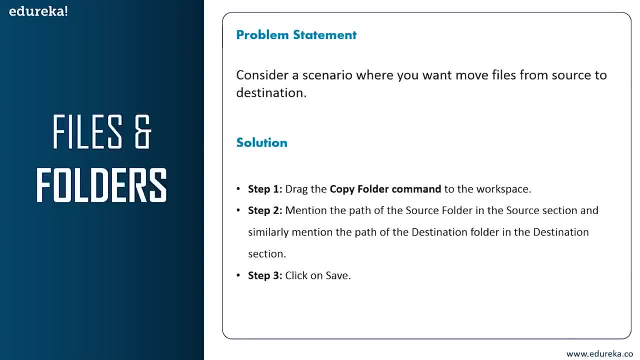 or unzip a folder and so on. So I'm going to do the same. So what I'm going to do is, initially, I'm going to show you how you can move files from the source to destination. So basically what I'm going to do is I'm going to choose two folders, basically the source. 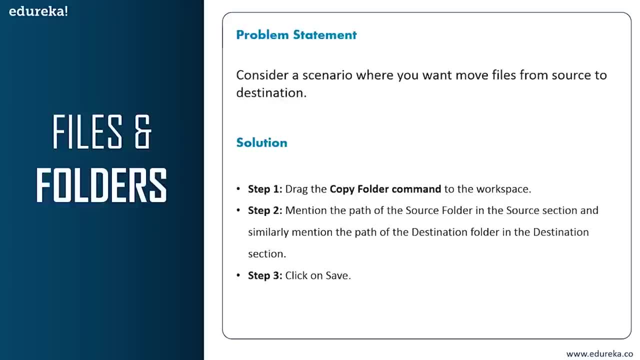 folder and the destination folder. Now the source folder will have n number of files, Basically those files we want to move from source folder to destination folder. So I'm going to drag the copy folder command to the workspace and mention the directory of the source folder in the source section and the destination folder in the destination. 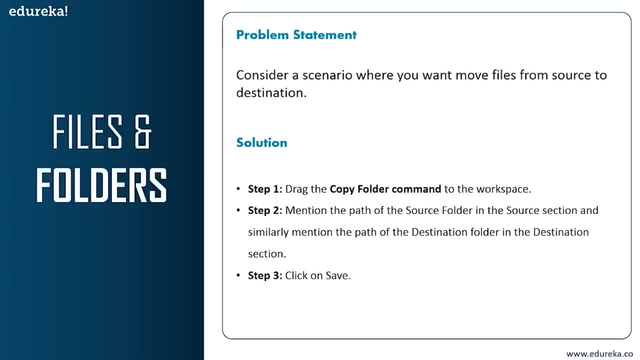 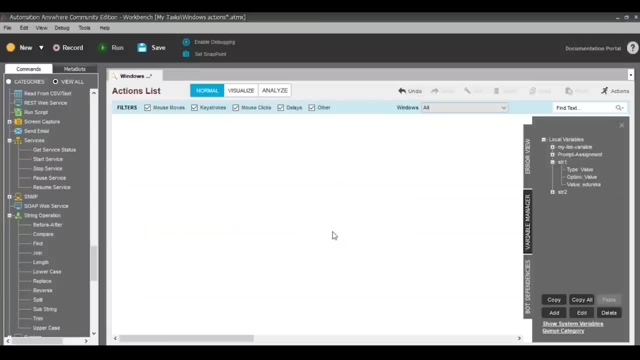 section and then I'll click on save. So let's just do that. So what I'm going to do is I'm just going to delete this part. Now, what I'm going to do is let me just open and show you the folders, basically, 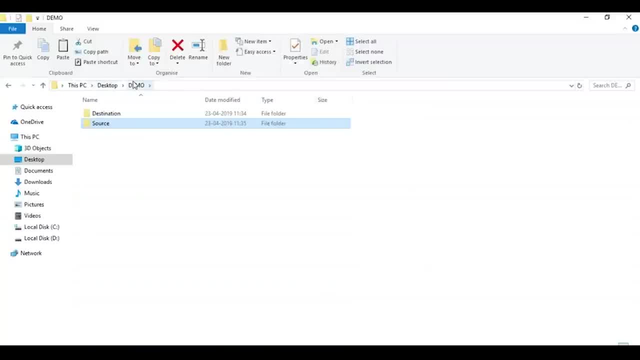 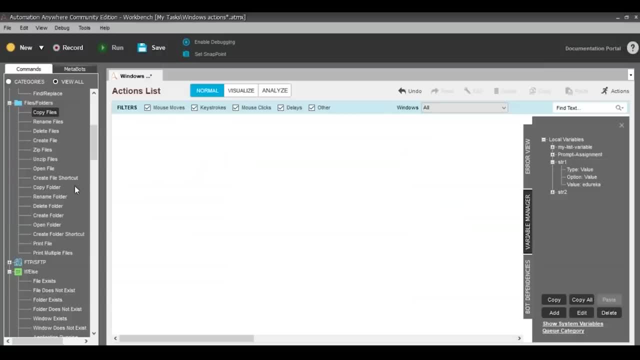 So, guys, this is my source folder. Now what I want to do is I want all the files to be moved from The source folder to the destination folder. Basically, I want to copy all the files from source to destination. So for that, what I'll do is I'll drag and drop the copy folder section and then I'll mention the 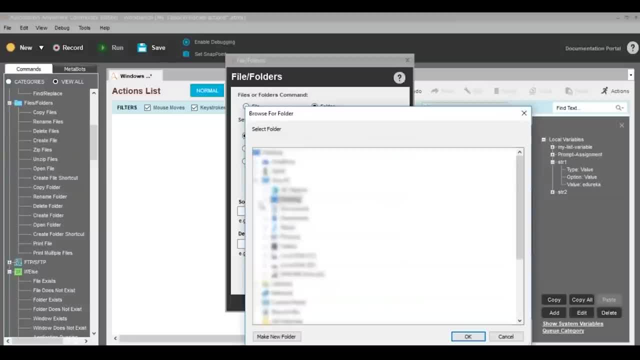 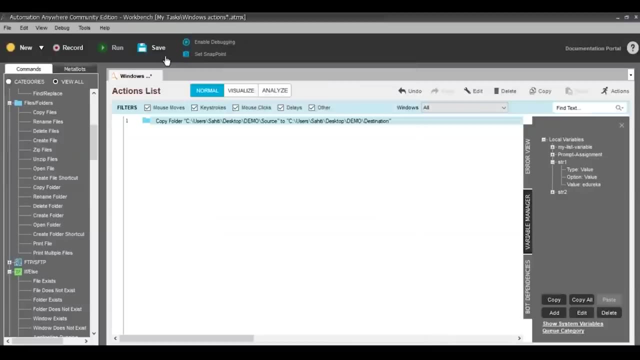 path of the source folder and the destination folder. right, I'm going to browse, mention desktop, and then in demo I'm going to choose for source And again in desktop I'll go for demo and choose destination. After that I'll click on save and then I'll just execute this task. 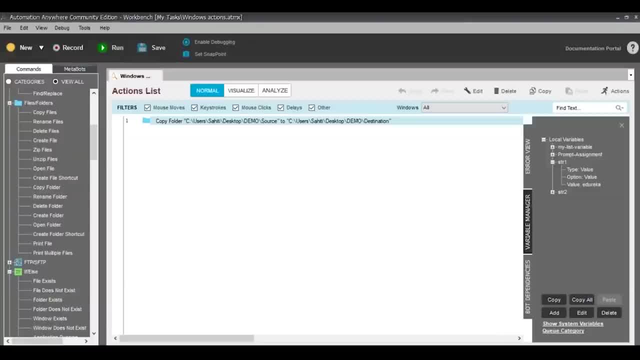 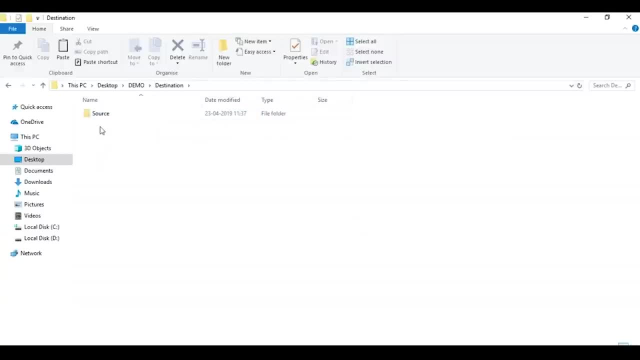 So, as you can see, my task is got executed, So I'll just go back to my destination folder and then you can see that. you know, in the destination folder we have the source folder in which all the files are present. So that's how, guys, you can copy files from a specific folder to another folder. 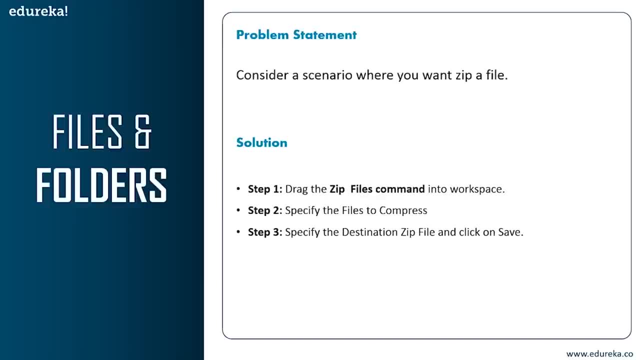 Now, apart from this, I'm also going to show you a scenario where you know we want to zip a file. So to zip a file, it's really simple. Again, you have to drag and drop the zip files command into your workspace, then specify the files. 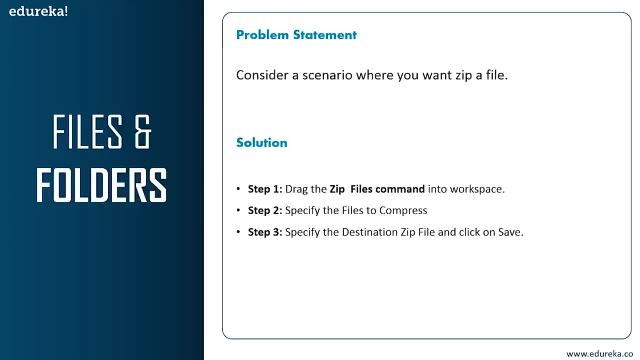 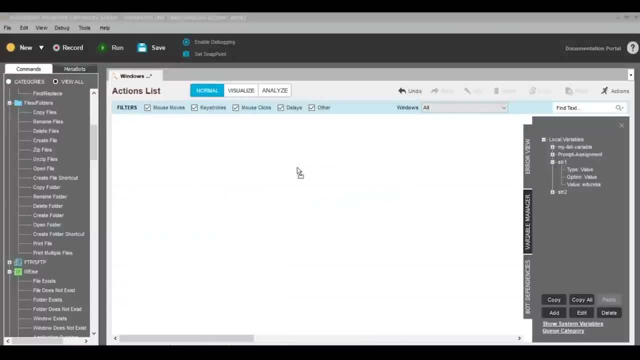 You want to compress and then specify the destination zip file And click on save. So let's just do that. So you know, I'll just delete this part. I'll drag and drop the zip file section. Now what I'm going to do is I'm going to specify what I want to zip. 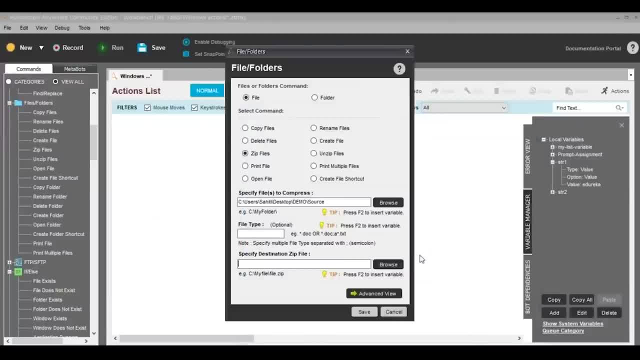 For example, let's say, you know, I want to zip the source folder itself. Now what I'm going to do is I'm going to specify the destination zip file, So I'm going to go for browse, and then let's say, we mentioned sample, and then open. 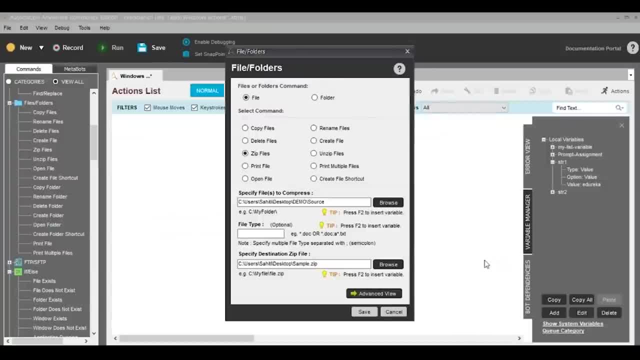 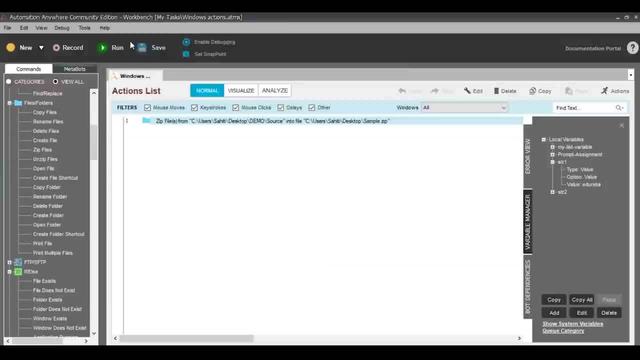 So basically, all our files will be compressed from the source folder and will be stored into the destination zip folder. that is the sample zip file. Now click on save and then I'll save the task, and then I'll click on run And my task is got executed. 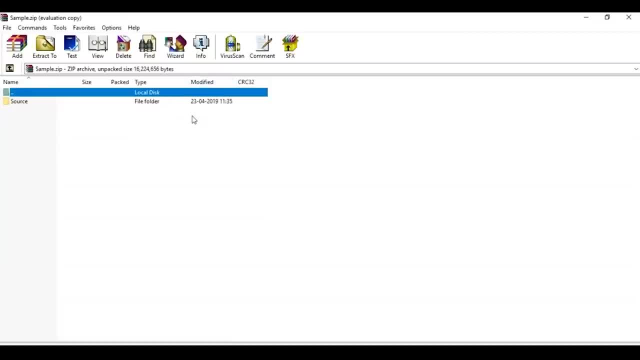 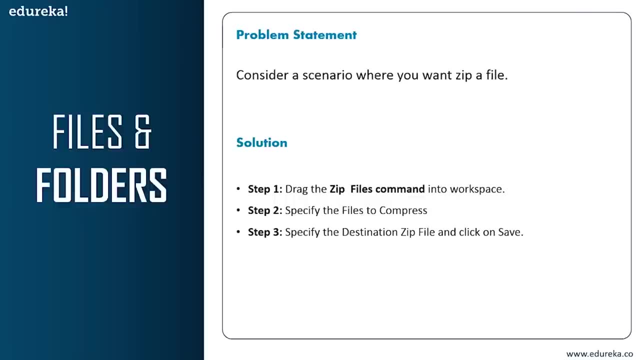 Now, when I open my sample zip file, you can clearly see that you know this particular source folder has been zipped into the sample zip file. That is basically a destination zip file. So, guys, that's how you know you can use the files and folders command. 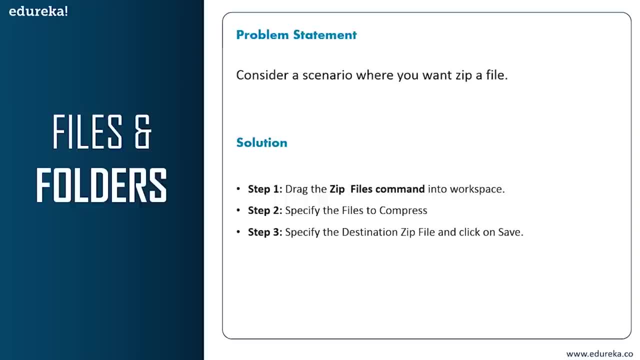 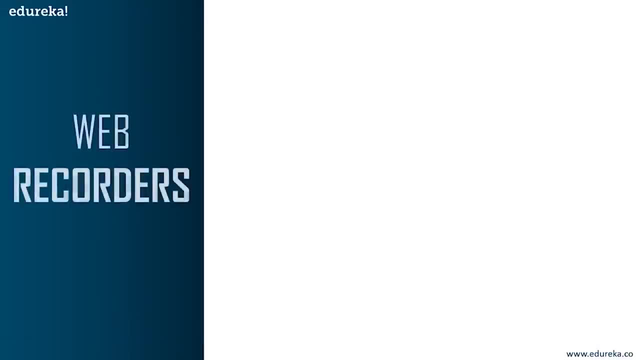 Well, over here, I just showed you two commands related to files and folders. Well, there are n number of other commands that you can use, and then you can play around with it. Now let's move forward with the next command, that is, the web recorders. 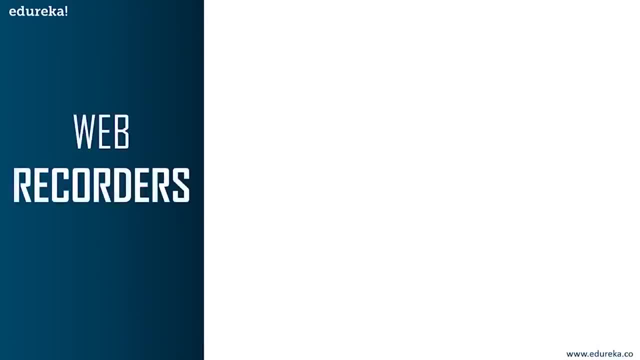 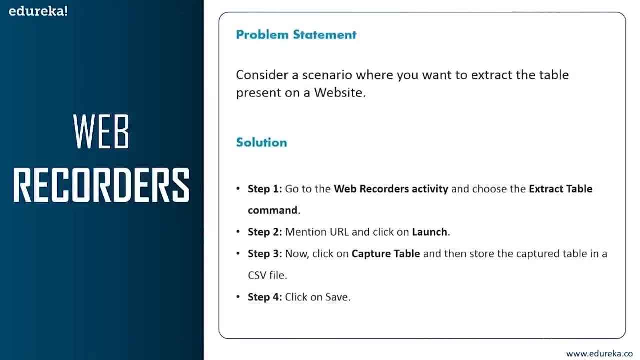 So web recorders, as the name suggests, mainly, you know, deal with how you can record data from websites, or maybe how you can store and extract data from websites. So I'm going to do the same. what I'm going to do is I'm going to consider a table which is on a website. 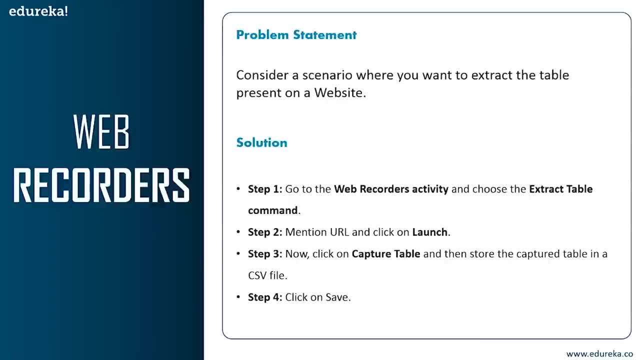 basically on a URL, and then I'm going to save that particular table to a CSV file. So to do that, what you have to do is you have to go to the web recorders activity, choose the extract table command, and then you'll have to mention the URL and click on launch. 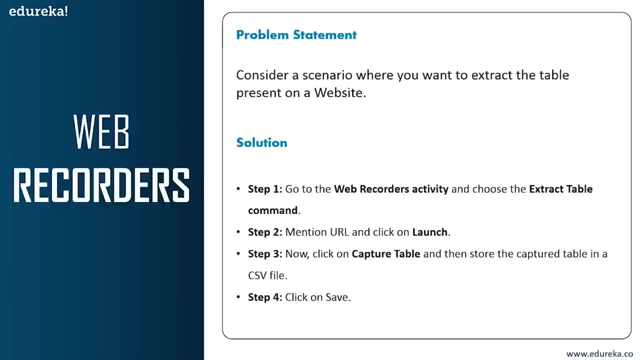 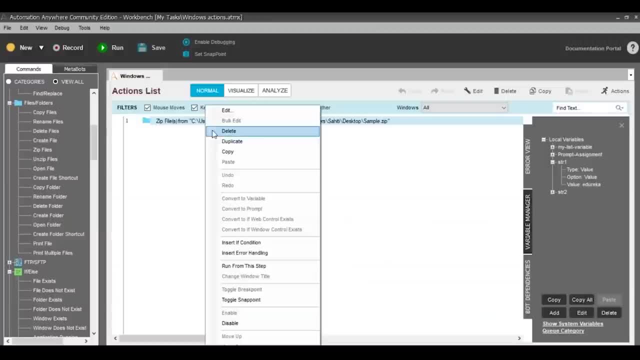 After that, you'll have to click on the capture tables and store the captured table in a CSV file and click on save. So that's what I'm going to do. So let me just shift back to my automation. anywhere to workbench, I'll remove this part. 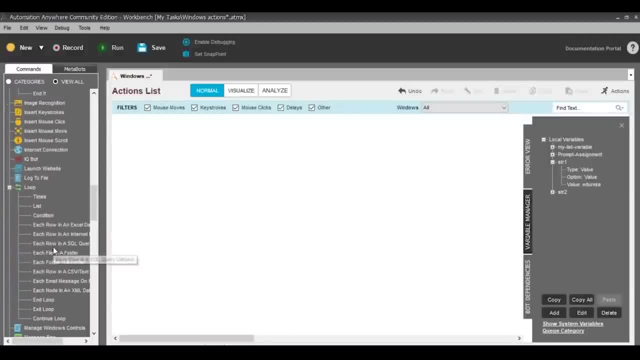 Now what I'll do is I'll search for the web recorders activity over here. So let me just go to W and then, as you can see, we have various options, like you know: opening a browser, closing a browser, maybe managing web controls. downloading, extracting tables. finding broken links, extracting data. navigating URL. 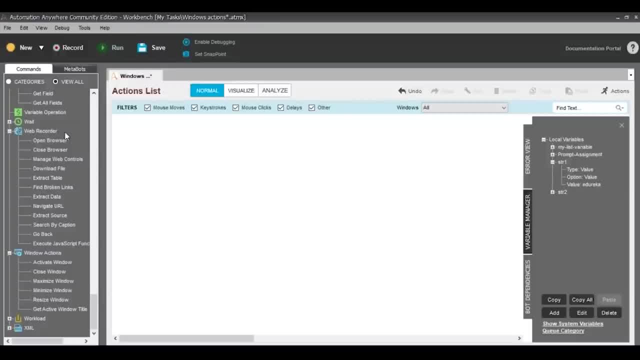 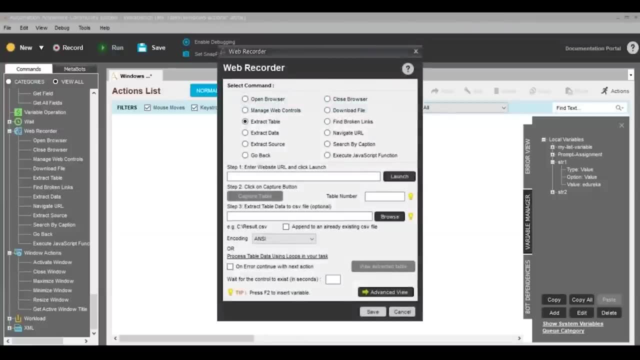 Extracting data, Extracting source, search by caption, go back and execute JavaScript functions. So what I'm going to do is I'm going to extract a table, right. So for that, I'll drag and drop the extract table command and then I'll mention the URL. 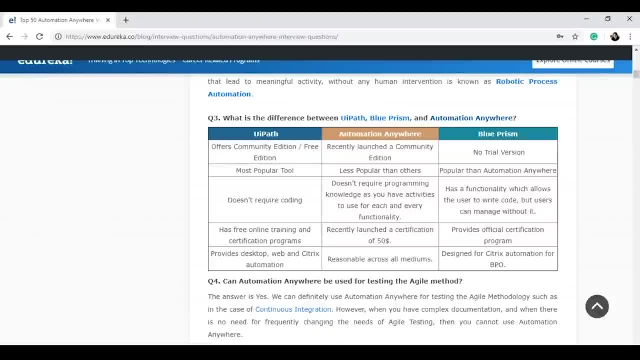 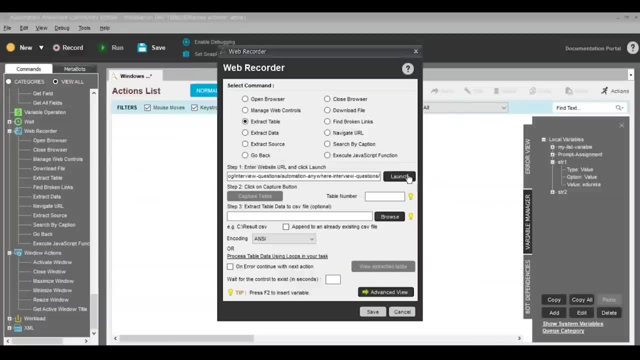 So let's say, you know we want to extract this table. So for that, what we'll do is I'll mention this particular URL. So I'll copy this URL from here and mention it over here. I'll click on launch. So when I click on launch it will automatically open in an Internet Explorer by default. 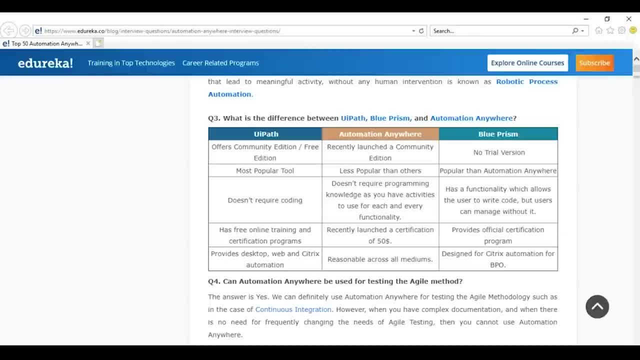 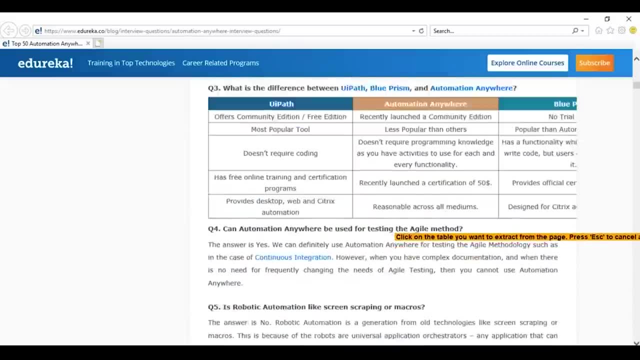 So, as you can see, my website Launched on my Internet Explorer. Now what you have to do is you'll have to click on capture table and then you'll have to search for the tables that you want to capture. So, for example, I want to capture this particular table. 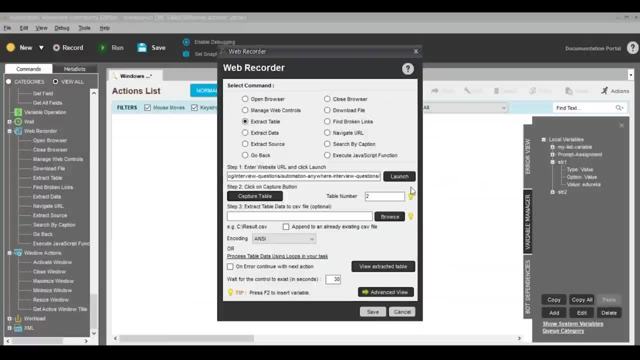 So I'll click over here and then you'll see that you know, automatically the table would be captured. So what I want to do is that I want the extracted data, that is basically the extracted table, to be stored in a CSV file. So for that, I'll click on browse and choose my CSV file. 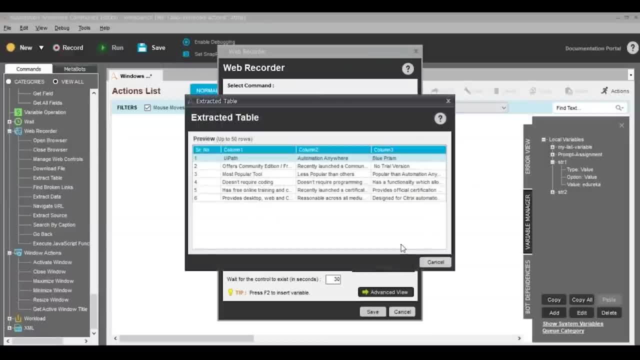 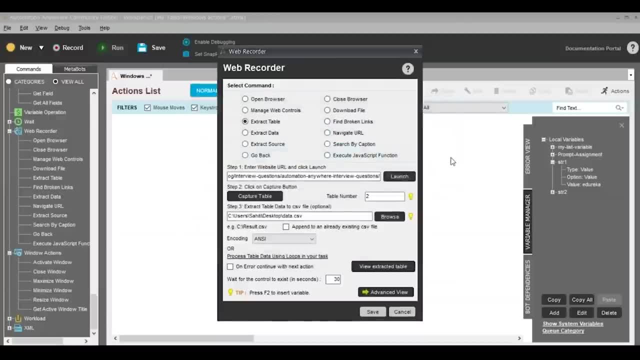 And then I'll just choose the option of You extracted table. that is basically second table that was chosen. That is the differences between UiPath- automation anywhere- and blue prism. since I just view this table, I'll just click on save and then what I'll do is I'll save this task and then I'll click on run. 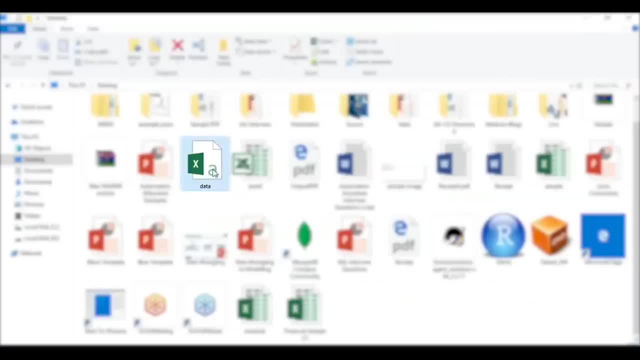 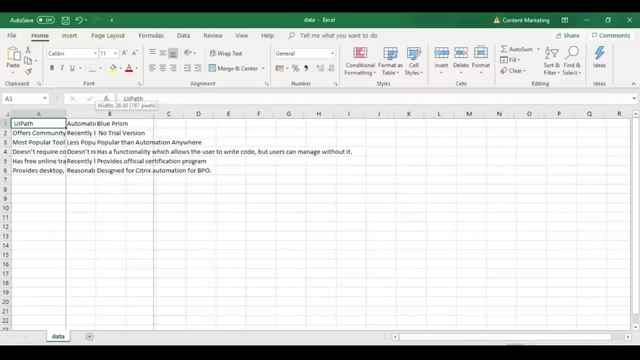 So, as you can see, my task has got executed. So let me just open my data dot CSV file. So, as you can see that you know our table has been extracted. So that was the difference between UiPath, blue prism and automation anywhere and you can see how the 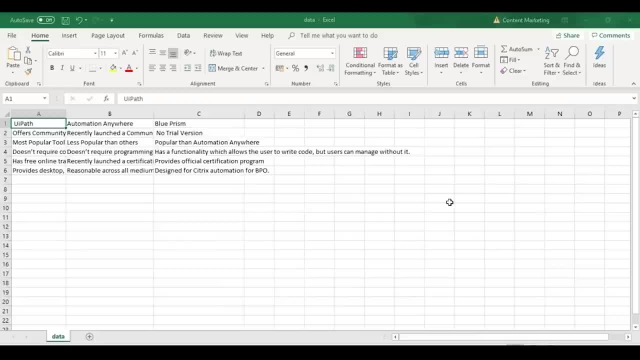 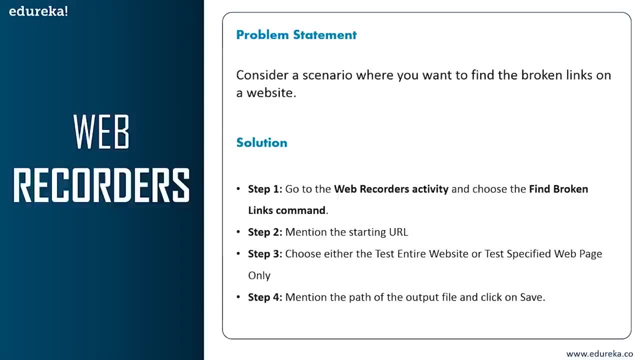 It has been extracted to a CSV file. So that's how, guys, you can use the web recorders to extract the table data into a CSV file. Now, Also, what I'm going to do is I'm going to show you another scenario where we're going to find the broken link on a website. 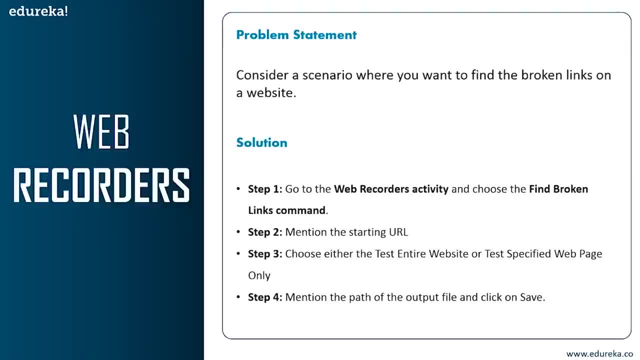 So to find the broken links on a website, what you simply have to do is you have to again drag and drop the web recorder activity and choose the find broken links command. After that you have to mention the URL, choose the option of you know, either testing the entire website or testing the specified web page only, and then you have to mention the path of the output file. 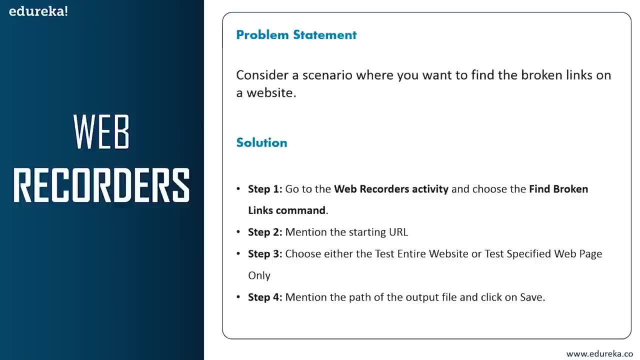 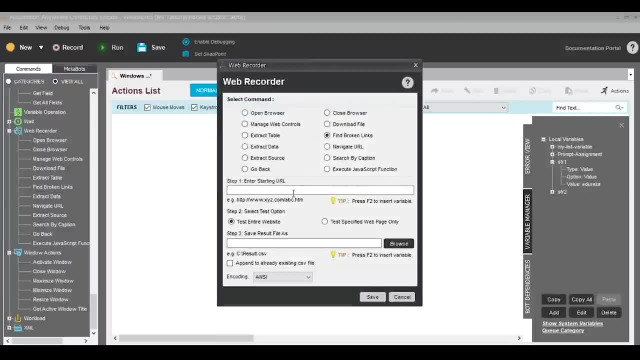 And click on save. So we'll do the same. So what I'm going to do is I'll go back to my automation anywhere workbench, I'll delete this part and then I'll drag and drop the find broken links. So let's say, you know, we want to mention the URL. 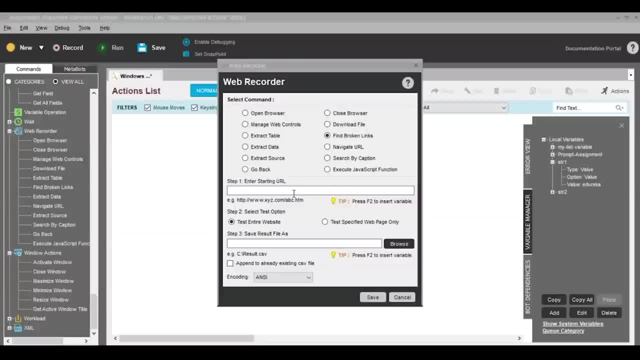 Let's say we check for our interview questions, right? So I'm going to search for interview questions of the Edureka domain and then I'm going to search for test entire website. After that I'm going to save the output data in a CSV file. 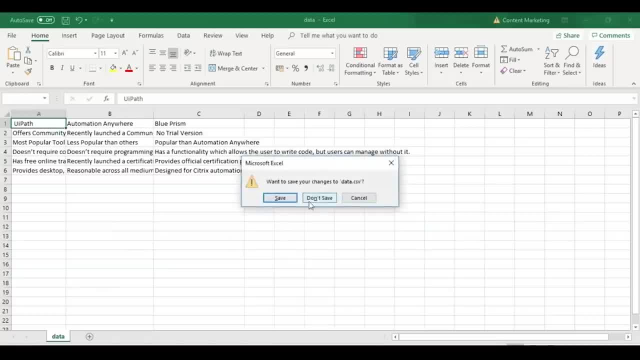 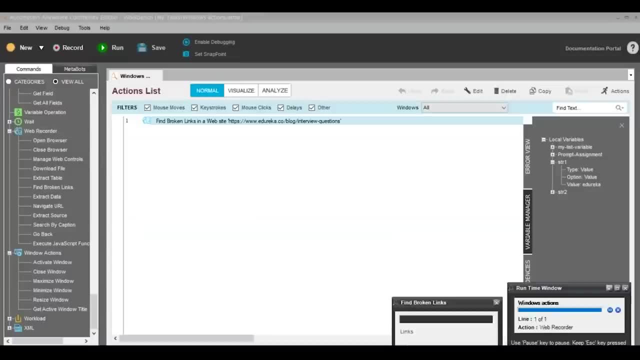 Let's say we save it in data and click on save. So initially I'll Just close this file and then I'll click on save and then, finally, I'll execute this task. So, as you can see, my task is getting executed and all the broken links will be found out and will be collected. 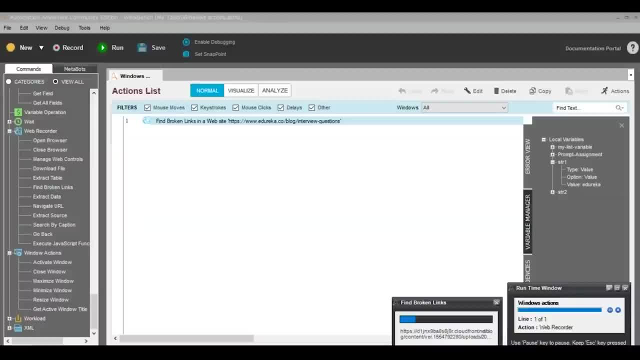 So, as you can see, it is happening on my screen, So let's just wait for it to complete. All right. So, as you can see, a lot of links have been tested, So I'm just going to stop this automation at this moment and I'm going to show you the output for how many of the links that have been tested. 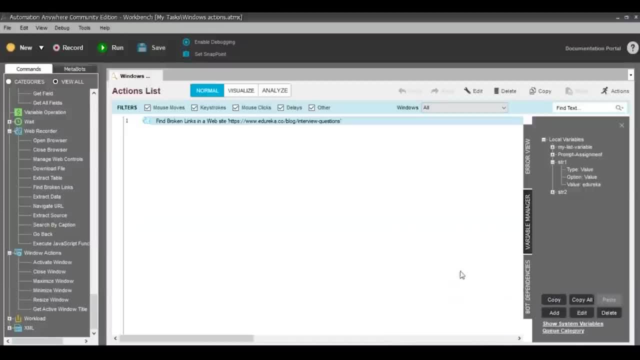 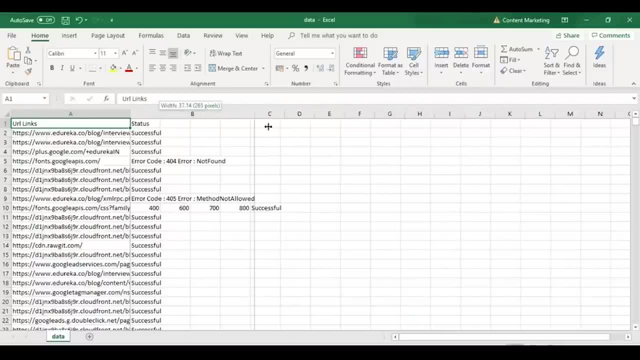 So let me just close this automation over here, Right, and then I'll open my CSV file. So, as you can see that, you know, basically there are two columns, that is, the URL link and the status. So basically the URLs that have been checked are around in hundreds and then few are successful. 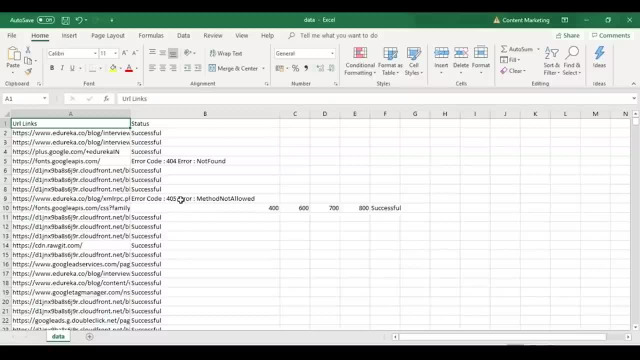 Few have an error. that is basically method is not allowed- 404 error, and the others are successful. So that's how, guys, you can find the broken links through the web recorders. So these are two commands that I talked about. Well, you can explore the rest. 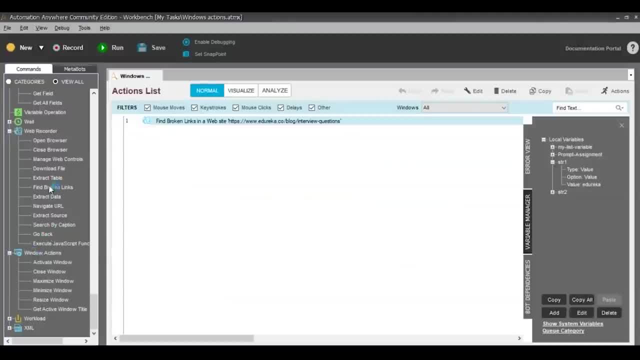 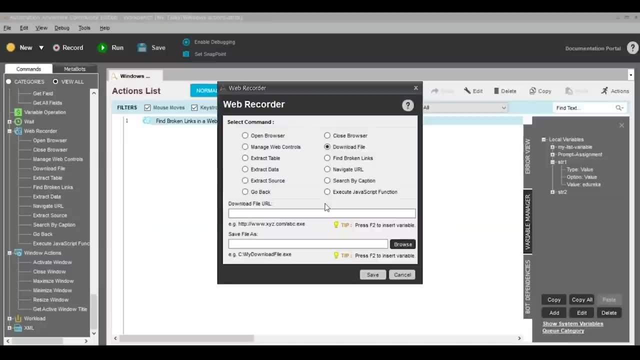 Almost all the other commands are really same. So, for example, if you just want to download a file, you drag and drop this option of downloading a file, then you choose the download file URL and then you save the file as whatever file type that you want. 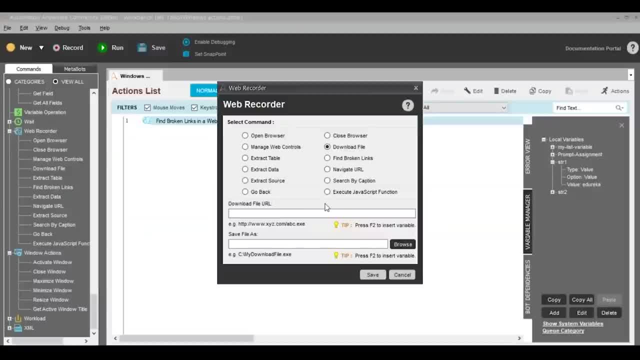 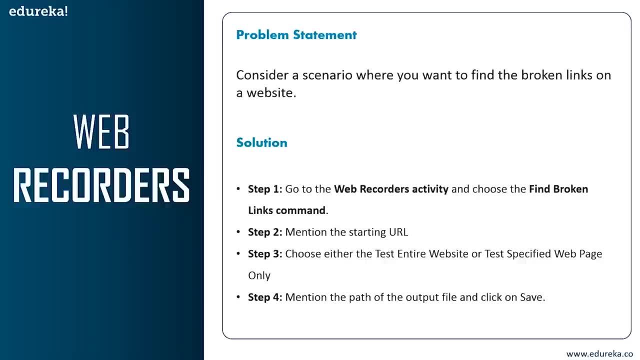 You can use a navigate URL to navigate to a specific URL, You can use the go back command to go back to a specific URL, and you can use the manage web controls to manage the other web controls, and so on. So, guys, that was about web recorders. now moving on to our next command, that is, OCR. 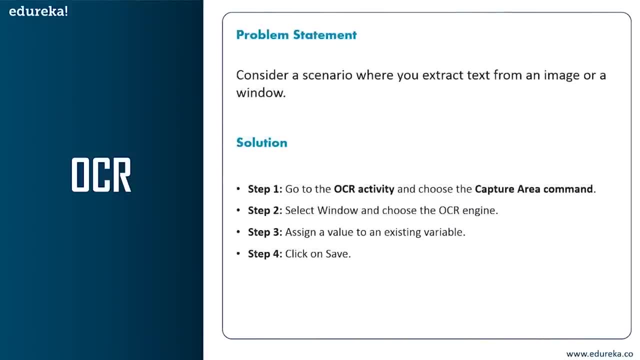 So OCR is nothing but The optical character recognition, which is mainly used when you want to extract text from an image or a window, and then you know you can capture either a specific area or a window itself. So we're going to do the same. 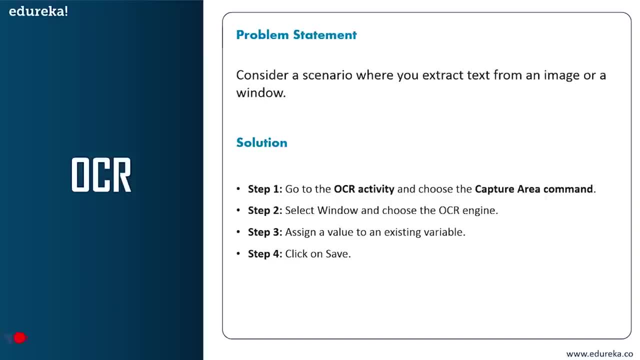 So to do that, what you have to do is you have to go to the OCR activity capture, the capture area command, because we want to capture the specific area, and then you choose the window. So, basically, you can either choose an image or, maybe you know, you can choose a notepad file or any other application that you wish to. after that, you have to choose the OCR engine, and Tesseract is chosen by the OCR engine. 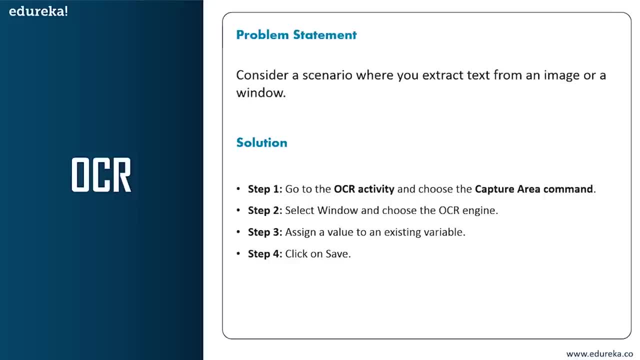 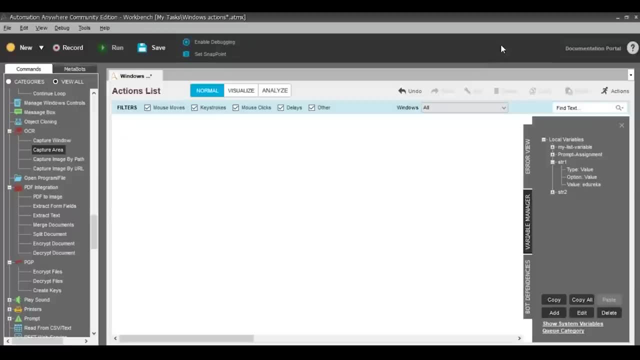 And Tesseract is chosen by the OCR engine, And then you have to assign a value to an existing variable and then click on save. So we'll do the same. what I'm going to do is I'm going to go back to my automation anywhere- workbench. 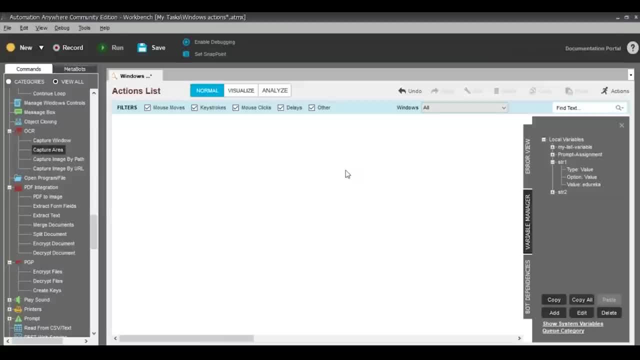 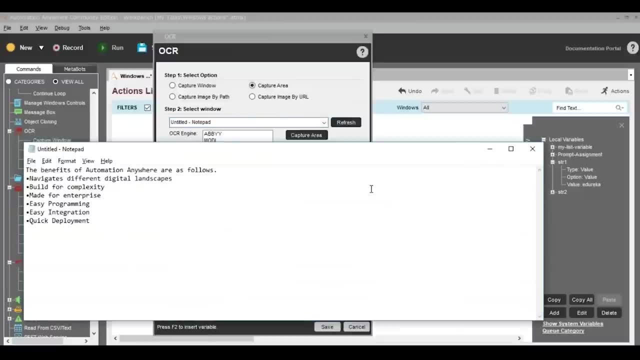 And then what I'm going to do is I'm going to drag and drop the capture area command. After that I'll just, you know, choose the window. Let's say we choose the notepad windows. So in the notepad you can see that. you know, I have few text available. 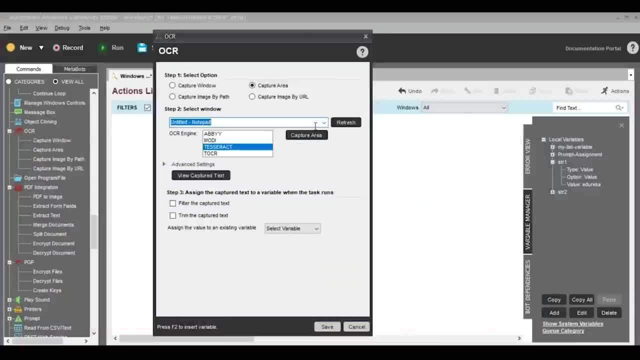 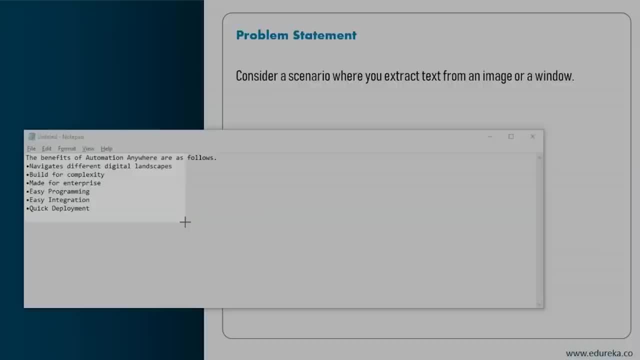 So we're going to extract the specific text. So after that I'll choose capture area. I'll capture the area. Let's say you know I want to capture from here to here. So basically, if you observe I'm not capturing the text after follows right. 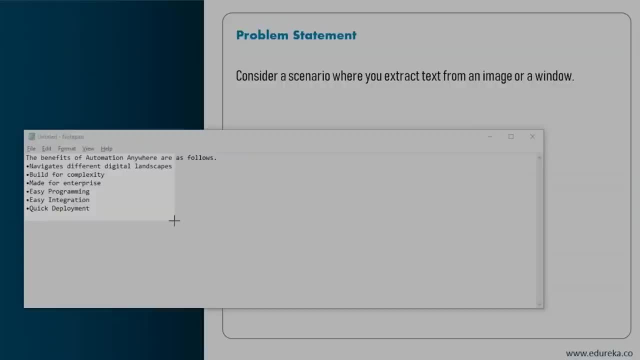 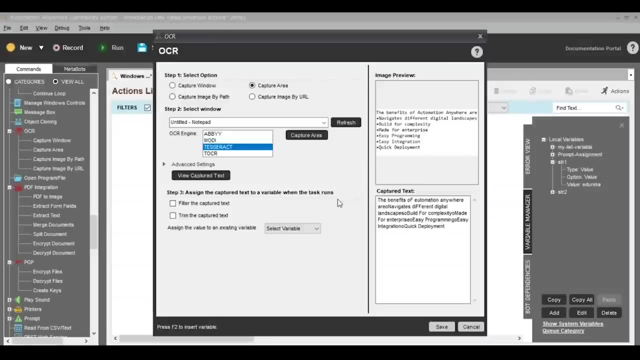 So basically, I'm going to capture the benefits of automation are and after that we're going to mention all the benefits. So I'm going to capture this particular area. then I'm going to view to capture text. So, as you can see, it's loading and you can see that you know. the captured text is: the benefits of automation anywhere are basically XYZ benefits, right? 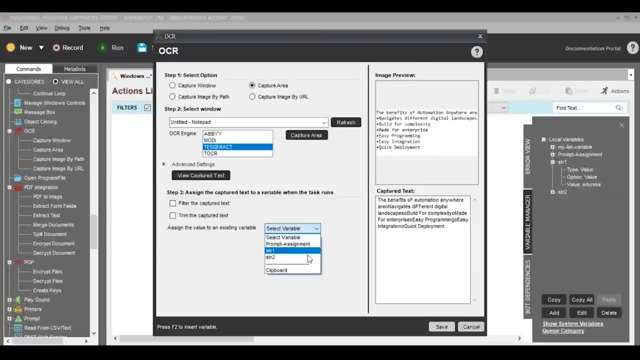 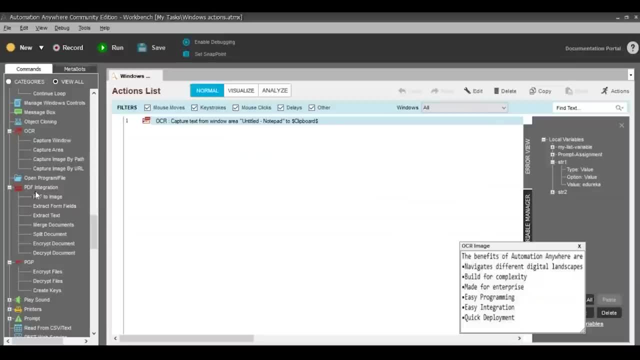 Now, after this, what I'll do is I'll assign a variable to store the value. So let's see, you know, I assign the variable to be clipboard and click on save. right after that I'll click on save and then let's say: you know, we use a message box to display an output. 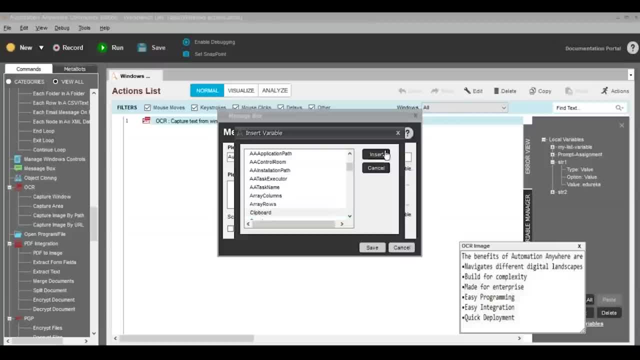 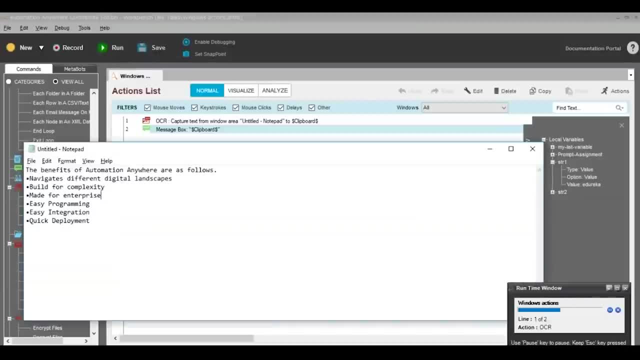 So I'll drag and drop a message box and then I'll mention the variable and click on save. after that I'll save this task and click on run So you can see that you know my task is getting executed and you can see that you know the text has been extracted. 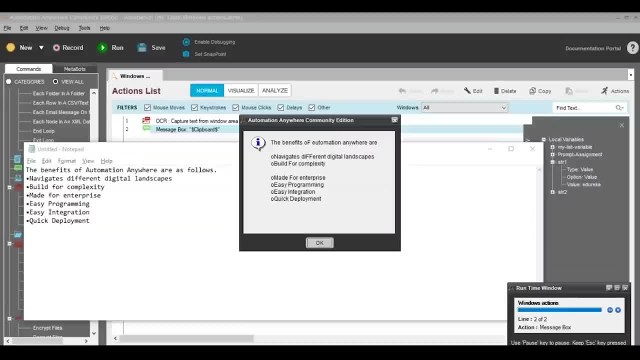 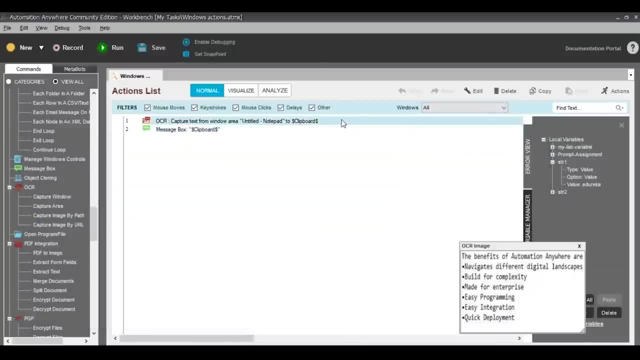 So obviously this is not in proper format because you know we had bullet points there and we captured only a specific text Area, right? So it completely depends on what area that you want to capture. And even if you want to capture the complete window, which window do you want to capture? 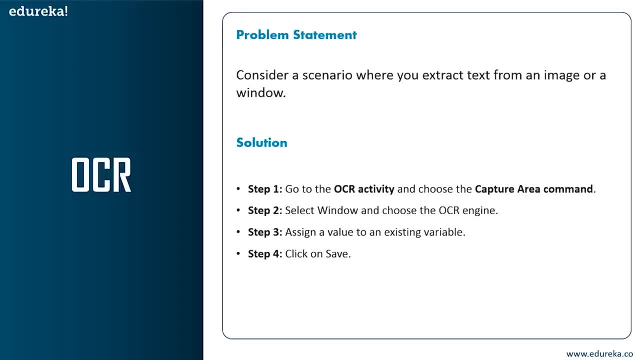 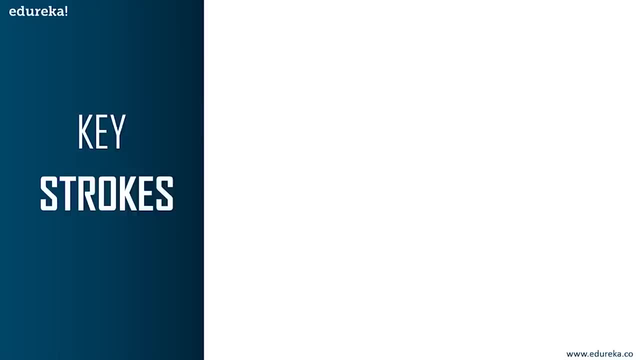 What would give you the most app extracted values, and so on. So that was about OCR guys. So now let's move forward with our next command, that is the keystrokes command. So the keystrokes are basically those commands which deal with your keyboard. 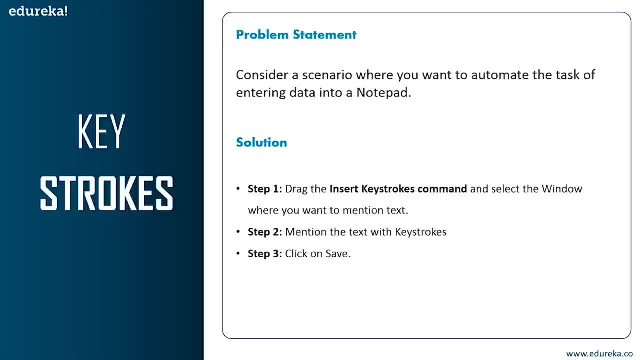 So, for example, when you're mentioning a text, you want some text characters to be maybe uppercase, and maybe you want two sentences in two different lines. right, So you can automate this completely. It does using the keystrokes. So what we have to do is you'll have to drag and drop the insert keystrokes command and select the window where you want to mention the text. 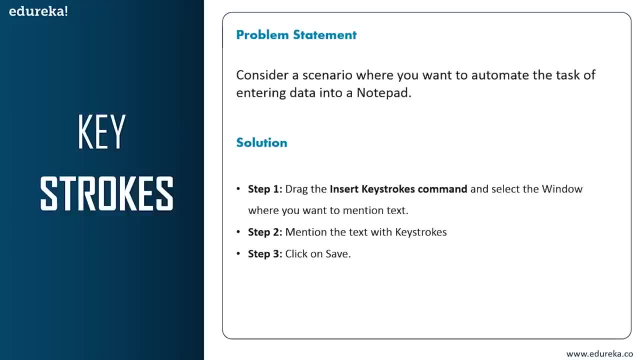 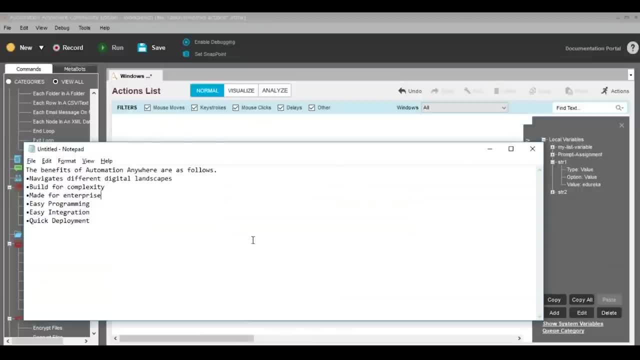 After that, you can mention the text with keystrokes and click on save. So that's what I'm going to do. I'm going to go back to my automation anywhere workbench. I'm going to delete these steps. I'm going to remove text from over here. 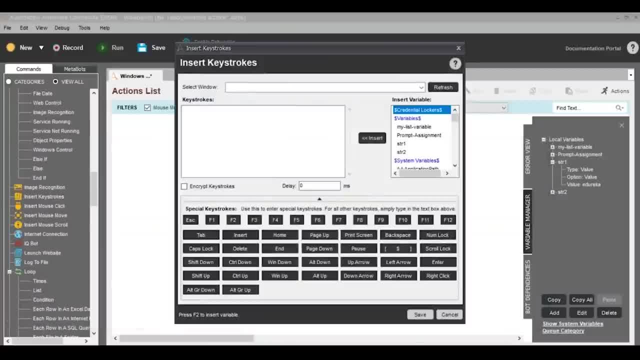 So what I'm going to do is I'm going to drag and drop the insert keystrokes command and over here I'll select a window, Let's say notepad. Now, Let's say we mentioned hi from Edureka and then we mentioned caps lock over here, and then we mentioned enter. 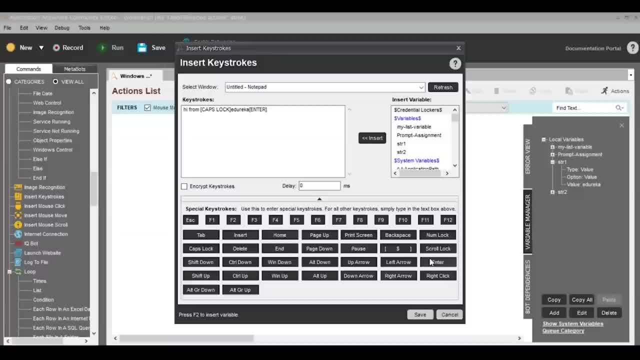 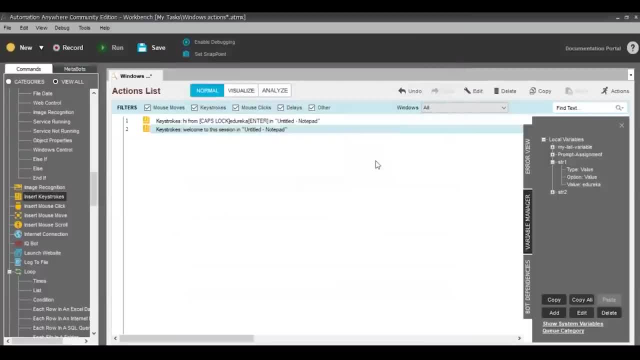 So basically we want to go to the next line. So we'll mention enter over here Now. after that we'll mention welcome to this session, right, And then I'll click on save and then I'll save this task again and then I'll execute this task. 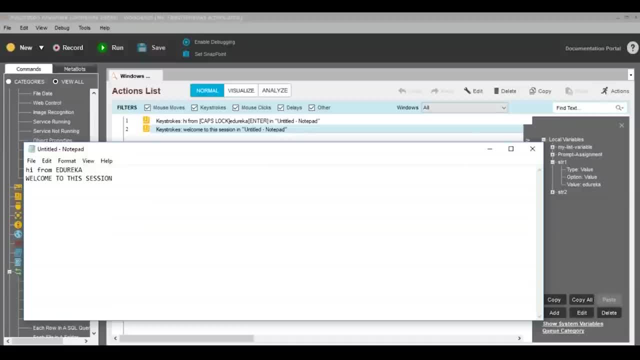 So you can see that you know hi from Edureka. So Edureka came in caps and after that everything Also came in caps, because you know we mentioned caps lock before. Edureka, right. So welcome to the session is also in caps. 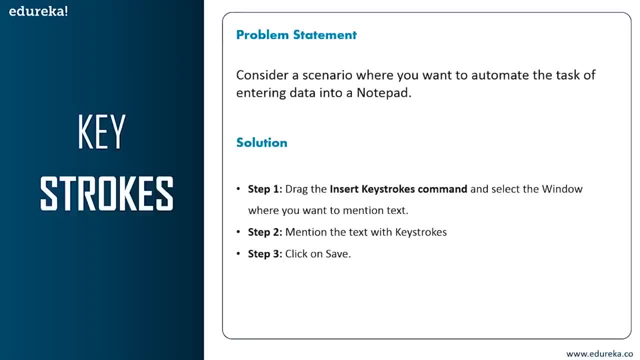 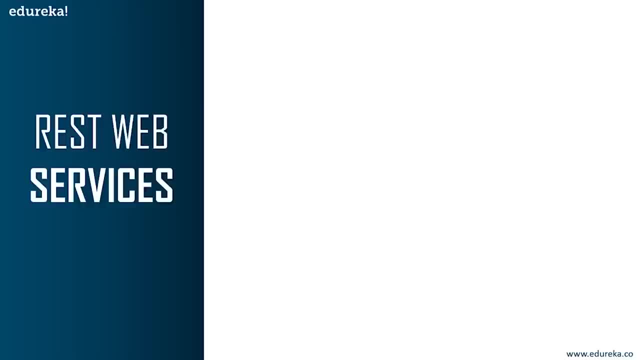 So that's how, guys, you can use the keystrokes command and automate the task. Now let's move forward with our final automation for this particular section, That is, the rest web services. So the rest web services basically deal with websites and basically deal with JSON files. 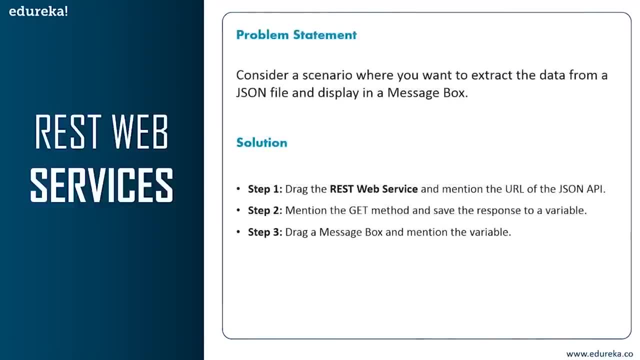 So what you can do is you can, you know, extract the data from a JSON file and also displayed in a message box. So for that, what I'm going to do is I'm going to drag the rest web service and mention the URL of the JSON API after that. 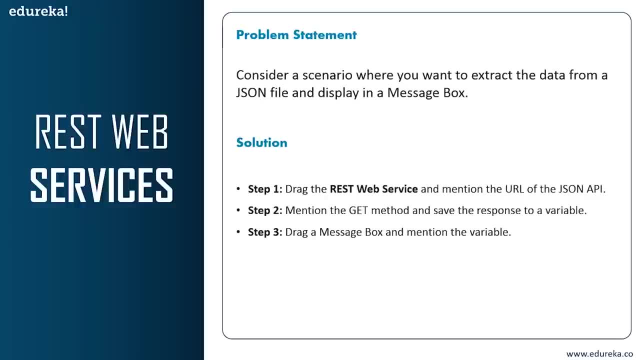 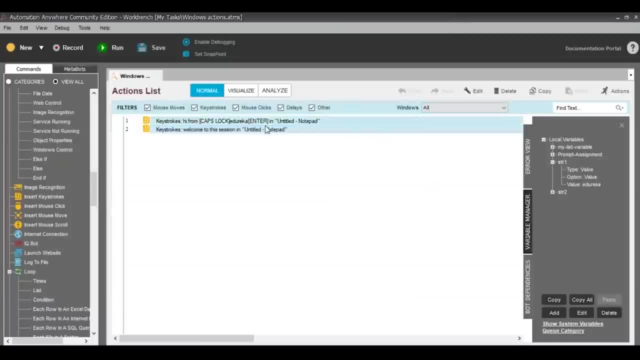 I'm going to mention the get method, so that we get the data and then we assign the data to a variable. after that We're going to drop a message box to display the output. So let's just shift back to my automation. Anyway, workbench, and what I'll do is I'll just open the URL and show you first. 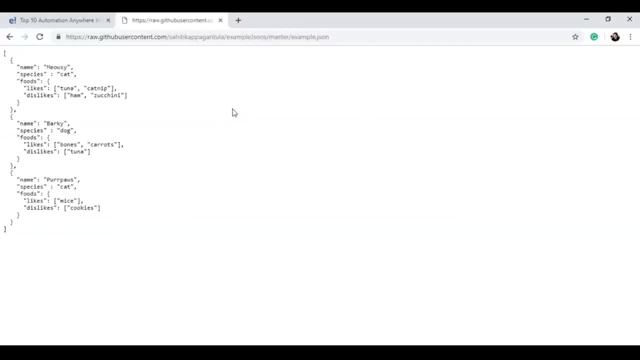 So, as you can see, this is my JSON API. Basically, I have stored it on my GitHub account, So this is a JSON file that I have, So I'm going to use this particular URL, and then what I'm going to do. 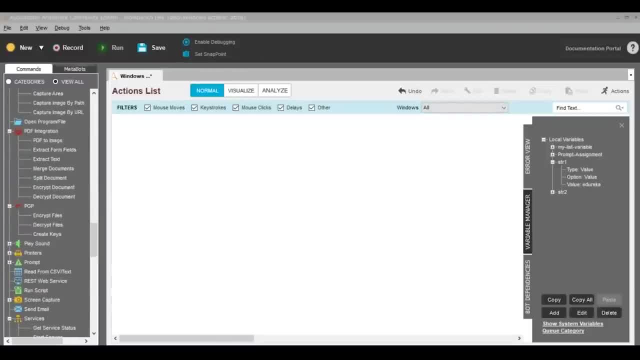 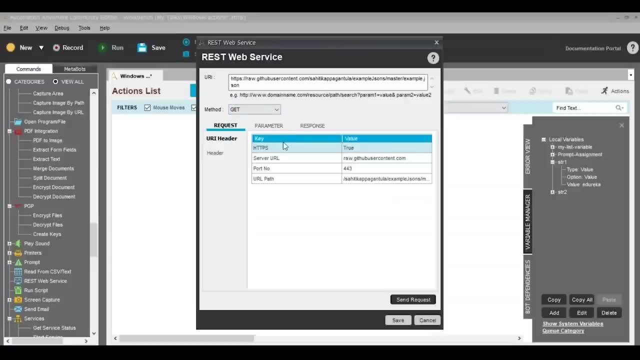 Is I'm going to drag and drop the rest web services over here, Then I'm going to mention the URL and over here I'll have to mention the method- get- so that we get the data. after we mentioned the get method, What you have to do is you'll have to mention the response variable. 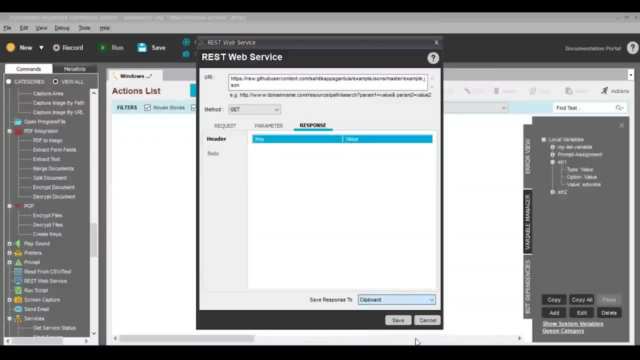 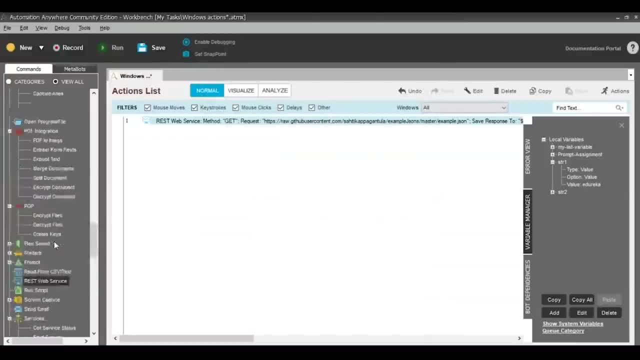 So basically go to the response section, mention the variable. Let's say we choose the predefined variable to be clipboard and click on save. after that We can use a message box to display the output. So I'll just use the message box, press on control F2 and then mention. 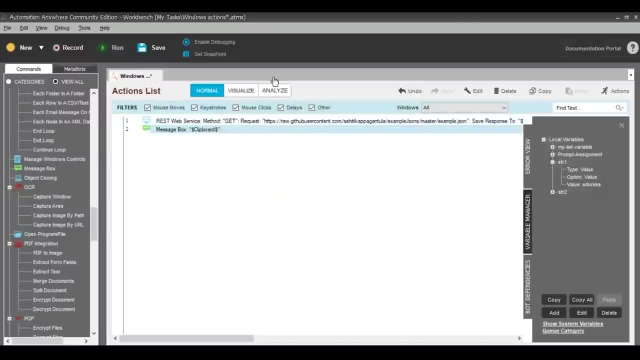 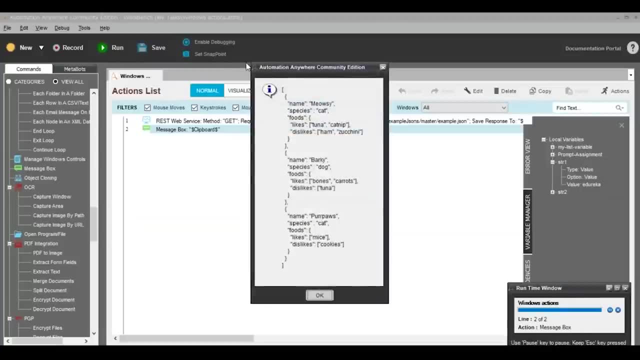 Clipboard, click on insert and click on save. after that I'll save this task and then click on run. So once I click on run, you can see that you know my JSON data has been extracted and stored into the message box, right? 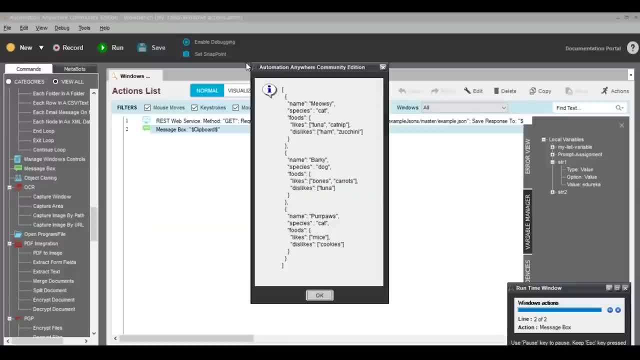 So this was that. you know I stored it into a message box. Basically I just want to do a display, the output. Well, you can definitely store the JSON file into any other files, like you know: text document, or maybe you know you want to store it in any other kind of documents, like PDF document. 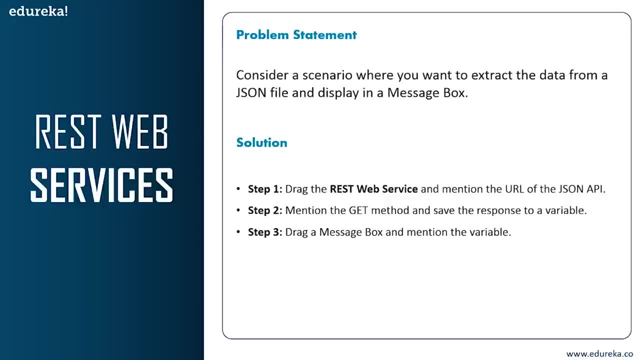 Also. you can definitely do that. So that's how guys, you can Use this rest web services. So I hope all of you have understood this basic examples and understood how you can use this. different commands to you know to do different kinds of automation. 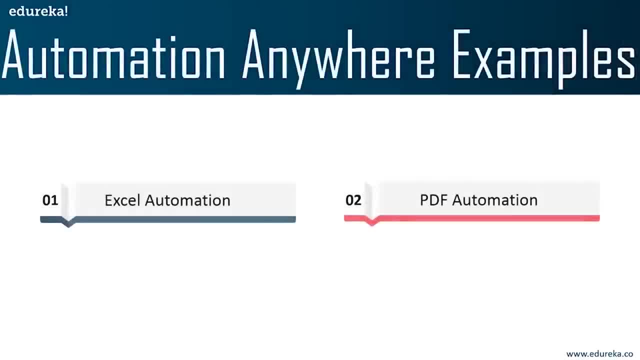 Now let's just look into something more interesting, That is, the Excel automation and PDF automation. Well, I was stressing about Excel automation and PDF automation because, you know, in many companies manual Workforce is employed to do simple, simple tasks that can be automated in Excel or PDF. 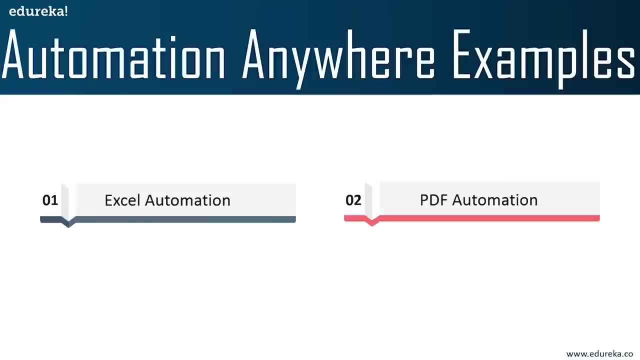 So to use manual Workforce in a better way and use their intelligence so that you know they can benefit Their organization in a better way. We can definitely automate the redundant task in both Excel and PDFs, So we'll start with Excel automation first. 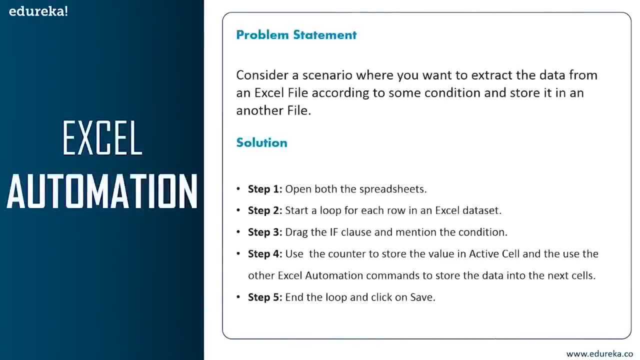 So the problem statement for our Excel automation is basically that you know we want to extract the data from an Excel file according to some specific condition that I'm going to talk about, and after that we're going to store the extracted data into another Excel file. 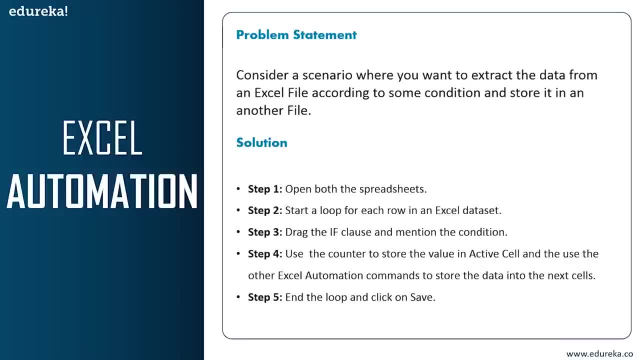 So, for example, if you see, if you have two Excel files, let's say a and B- now a is our source file and let's say it has 10 columns. Now what we want to do is we want To consider a specific column and then we'll mention some conditions. 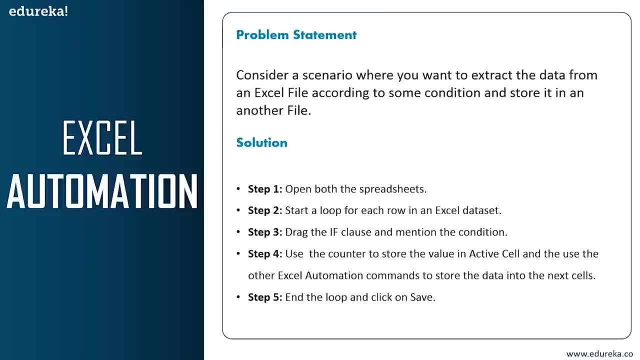 So let's say, you know we want to consider the second column and let's see note: in the second column We got to specify a condition that you know. let's say the value should be less than hundred. So all the data present according to values in the second column which are less than hundred should be stored in the second spreadsheet, right? 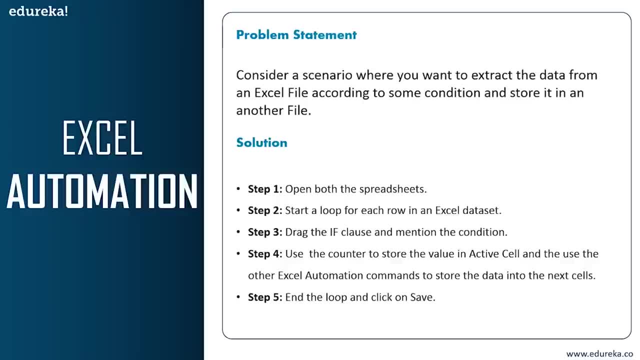 So that's what we're going to do. So to do that, what you have to do is you have to first open both the spreadsheets. after that you have to start to look for each row in Excel, data set and then drag and if cross where you mentioned the condition. 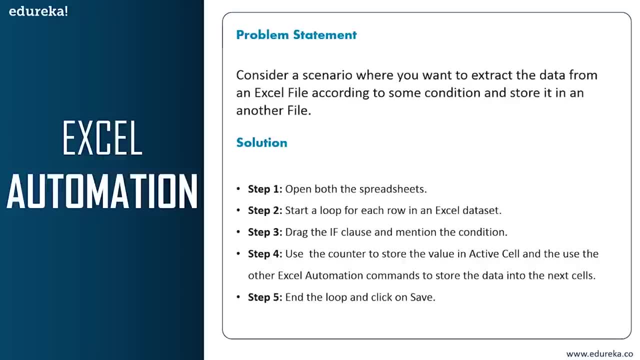 After that you have to use the counter variable to store the value in active cell and use the other Excel automation commands to store the data into the next cell, and then you'll have to end the loop and click on save. So we're going to do the same. 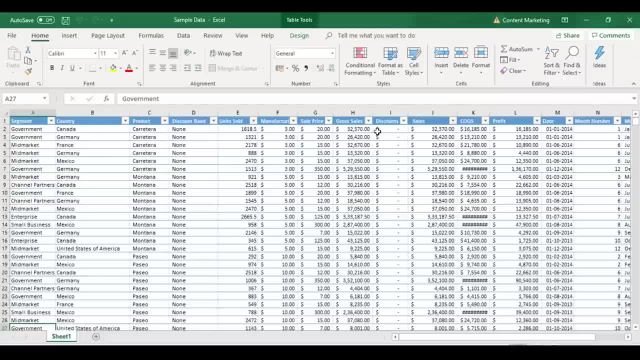 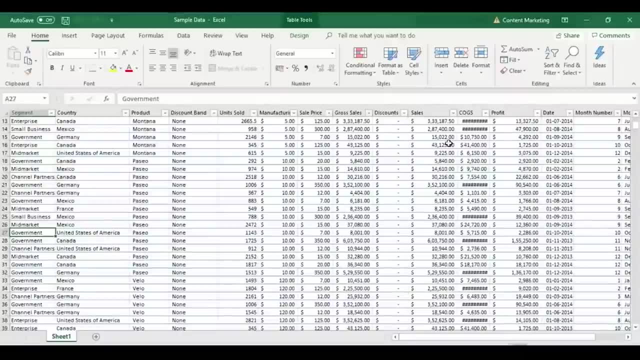 So, initially, let me just show you the Excel sheets. So, as you can see in my screen, this is the sample data that I'm going to consider. So, based on some column, let's say you know we're going to consider the sales column and let's say our condition will be: you know, all the data of all the rows whose sales values greater than 10,000 should be stored in our output. 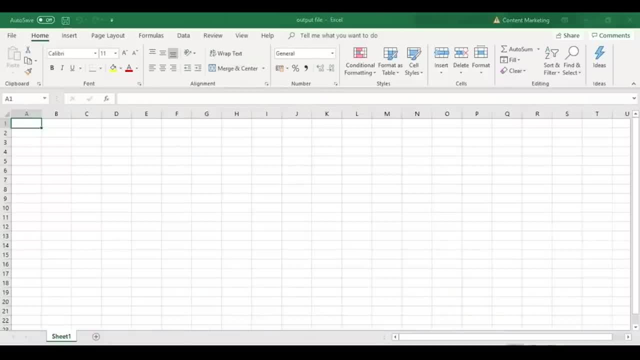 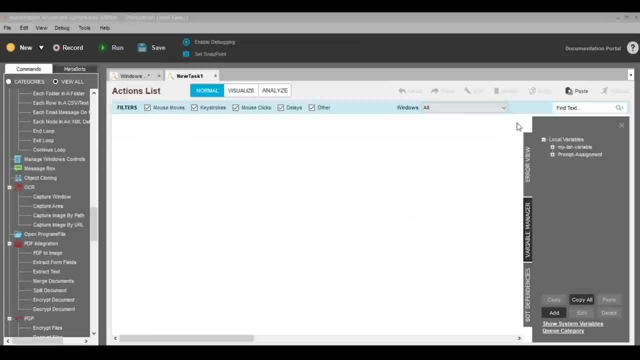 So that's what we're going to do. So to do that, let me shift back to my automation anywhere workbench, and then I'll delete this section. So what I've done is I'm going to open a new task. Now what we have to do is our first step is to open both the spreadsheets. 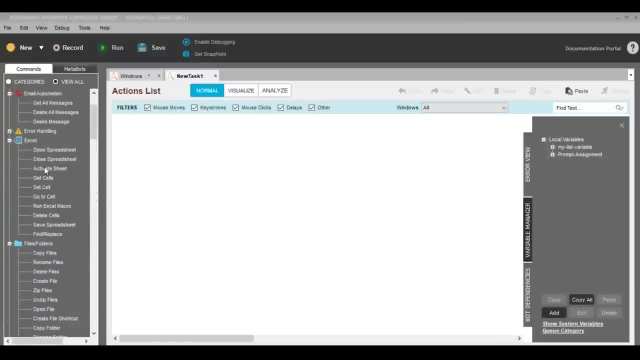 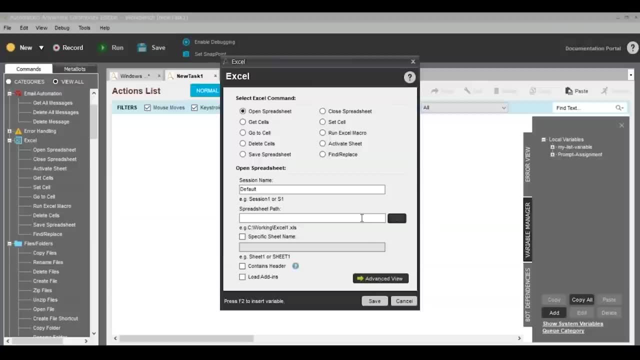 So for that, we'll go to open file. So for that, what we'll do is we'll go to the Excel commands and choose the option of open spreadsheet and drag and drop it over here. Now, in the open spreadsheet, I have chosen default. 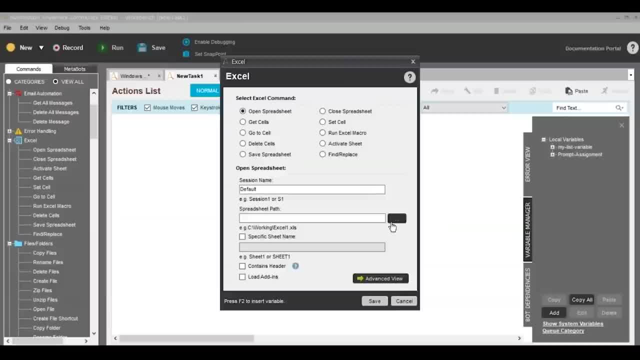 That is basically the session name for our first spreadsheet And then I'll mention it. I'll mention the spreadsheet path, So sample data will be a first spreadsheet And since our spreadsheet contains header, I'll check on contains header and click on save. 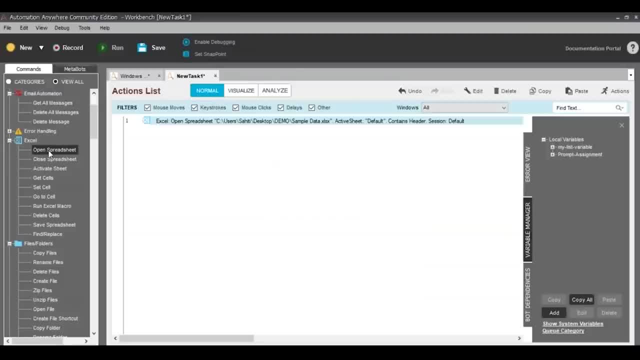 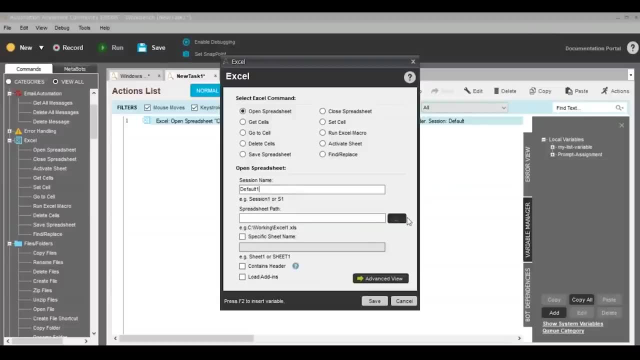 Now what I'll do is I'll open the second spreadsheet, So again I'll drag and drop it over here. Now I'll mention the default session name, to be default one, And then I'll mention the spreadsheet part, Let's say output file, and click on save. 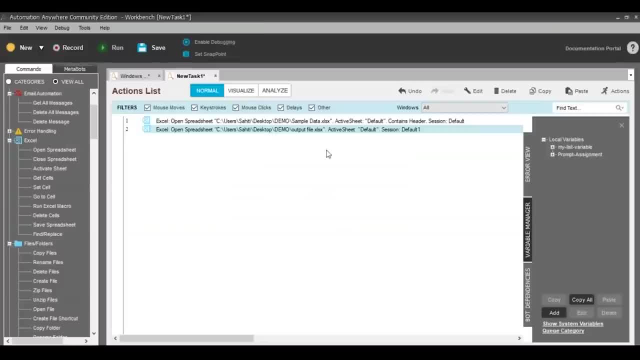 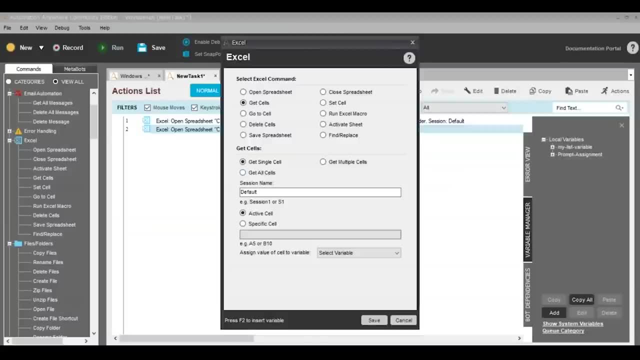 Now what you have to do is you have to drag and drop the get cells command and get all the cells. For that You'll drag and drop get cells command from the Excel command and then mention the session name: default. That is from the first spreadsheet. 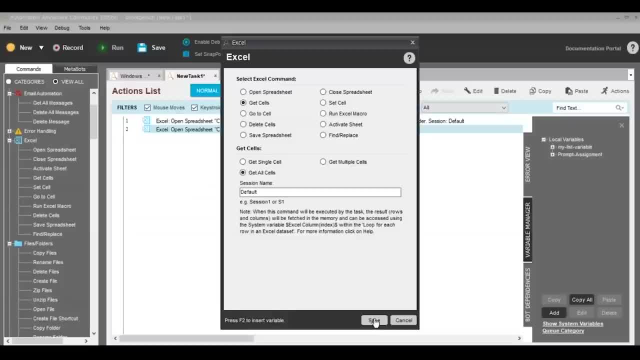 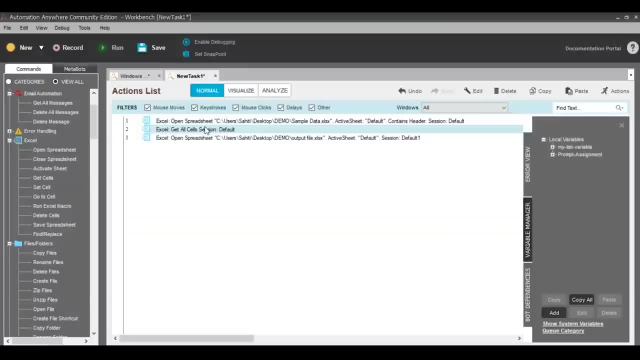 We want all the cells right, So for that we'll mention default and choose get all cells and click on save. After that, this step has to come between opening both spreadsheets. Now what you have to do is you have to start a loop to find out for each row in the Excel, data set right. 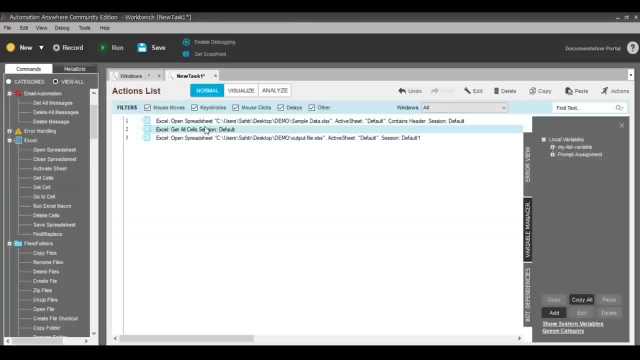 So, for each row in the Excel data set, what we want to check is, in the sales column, If the value is more than 10,000 or less than 10,000.. If it's more than 10,000, then we want the data to be extracted and stored into the output file. 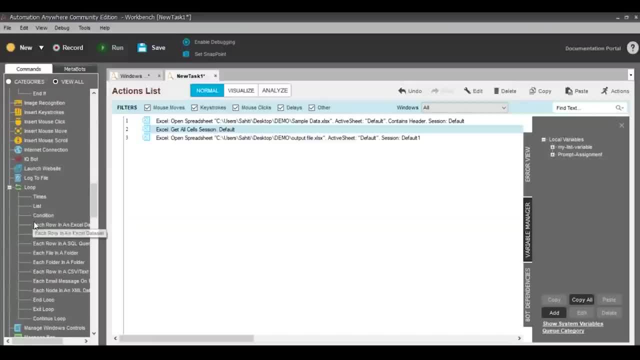 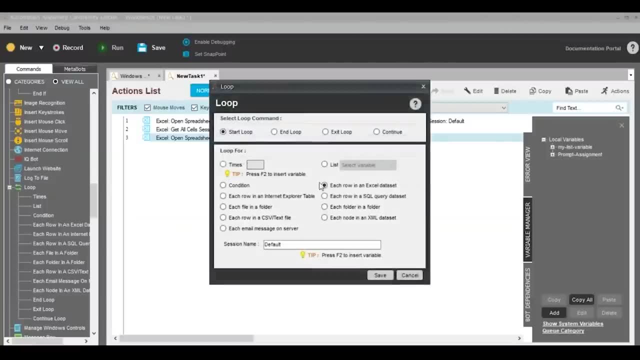 So for that, we're going to search for loop And then choose for each row in an Excel data set, And then what we're going to do is we're going to choose start loop, And then what we have to do is we have to mention that session name to be default. 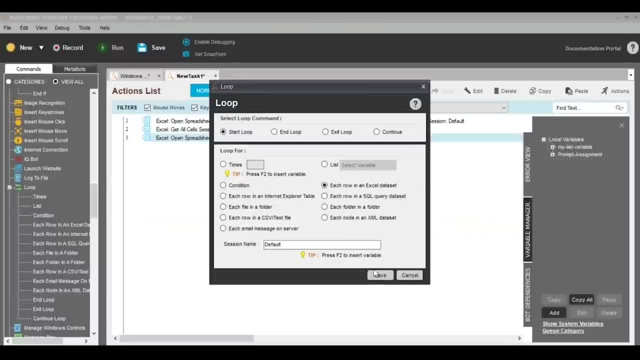 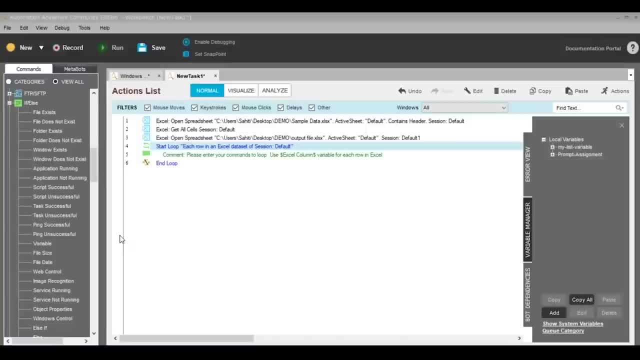 That is because you know we are dealing with the first spreadsheet now And then we're going to click on save. Now what you have to do is you have to drag and drop the if-else clause. So in the if-else clause, if you see, you have various options, right. 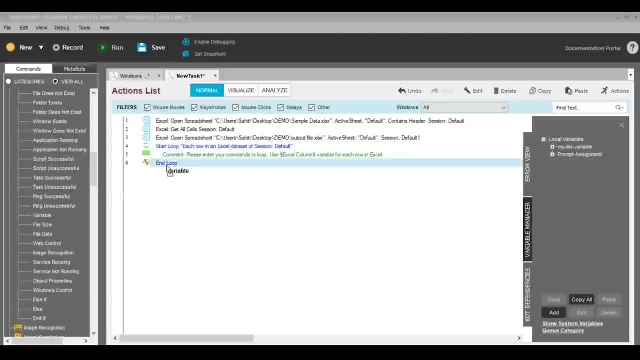 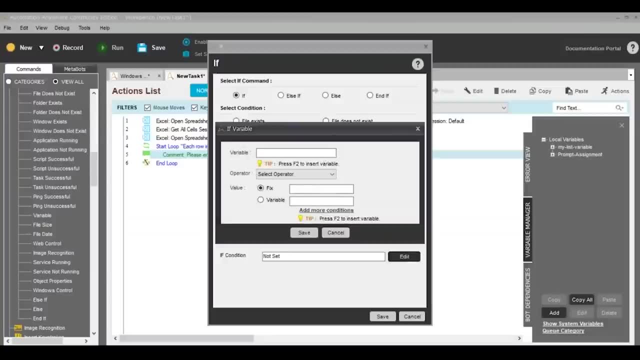 So I'm going to choose the variable set, So that you know we've mentioned a variable, and then I drag and drop it over here. So we are. what we have to do is, in the if condition, you'll have to click on edit and then mention the variable. 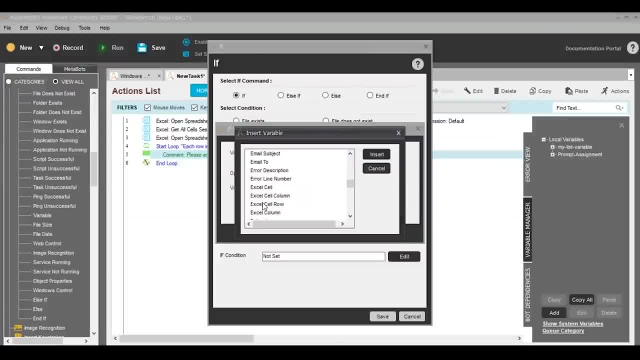 So over here we'll have to press on control F2 and search for Excel column, So insert, And then what you have to do is you'll have to mention the value or the variable. So we have to consider it for the sales column, right? 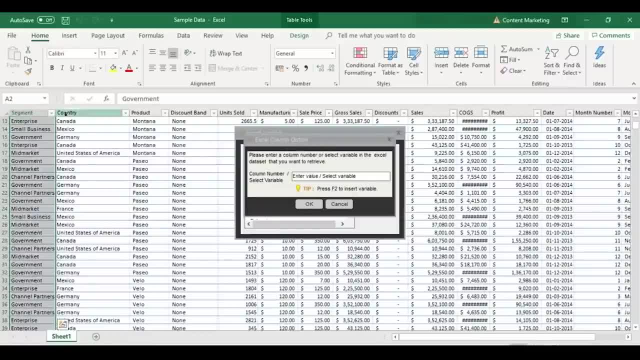 So let's just count the column number of sales. So that is 1,, 2,, 3,, 4,, 5,, 6,, 7,, 8,, 9,, 10.. So we're going to search for 10.. 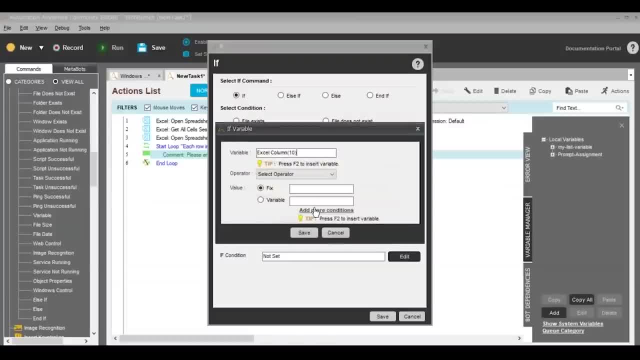 So we're going to mention 10 over here and then press on OK. Now what we have to do is we have to choose an operator. So I want to consider: all the rows whose values are greater than 10,000 should be stored, right. 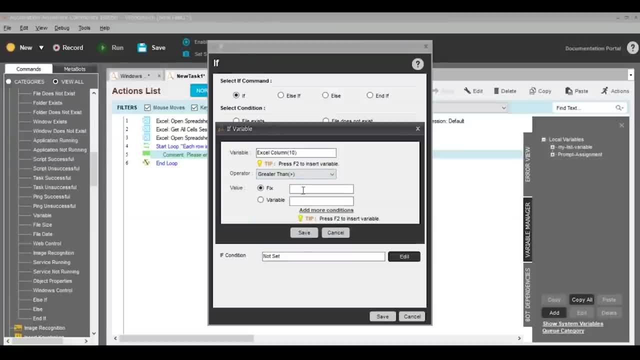 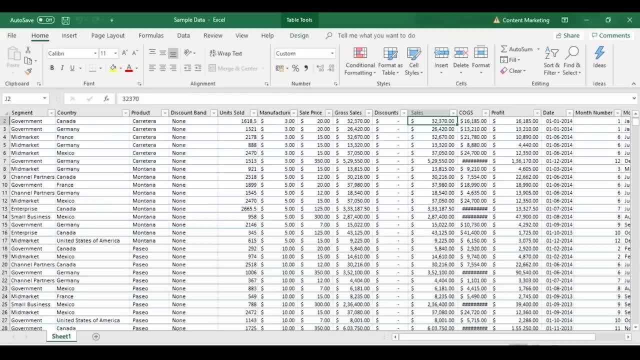 So for that, we're going to search for the greater than operator and then mention the value to be 10,000. And then what I'm going to do is I'm going to press on save. Now what I have to do is for each column in the data set: 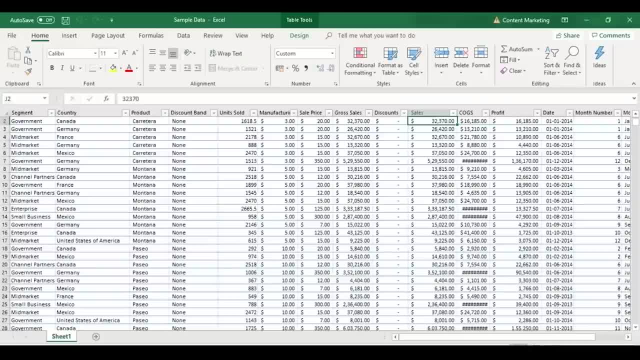 what I want to do is I want to extract the data and store it into a specific position in the output Excel file. Okay, So for that we have to count the number of columns that we have. So it's 1,, 2,, 3,, 4,, 5,, 6,, 7,, 8,, 9,, 10,, 11,, 12,, 13,, 14,, 15,, 16, right. 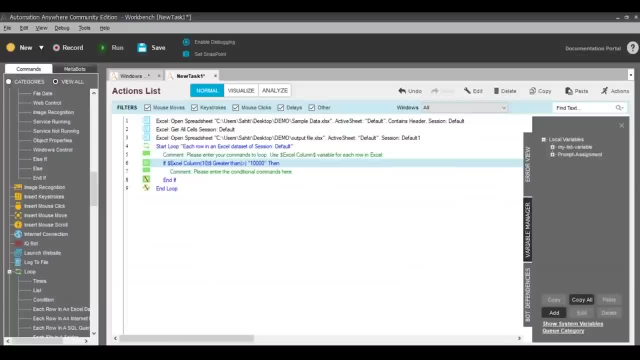 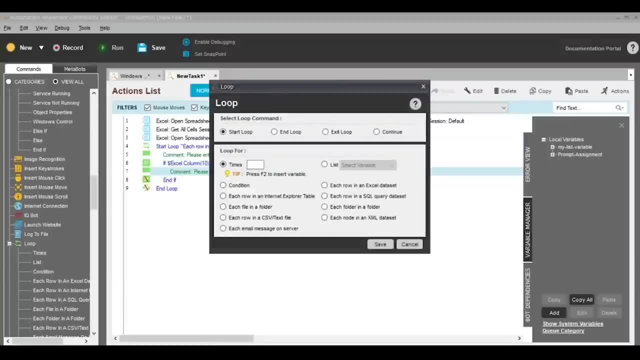 So we have 16 columns. So what I'm going to do is I'm going to search for loop and then I'm going to drag and drop the times command in the loop. Now, in the times command you have to mention basically how many times that you want the loop to be iterated. 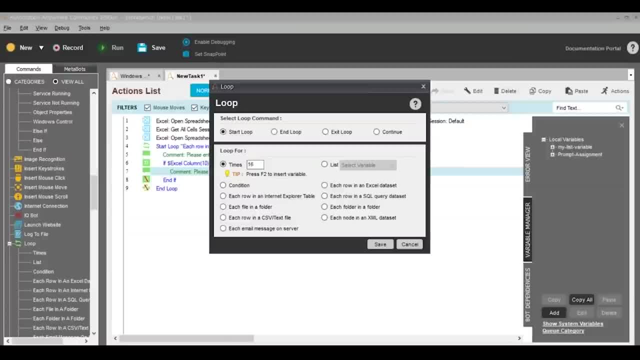 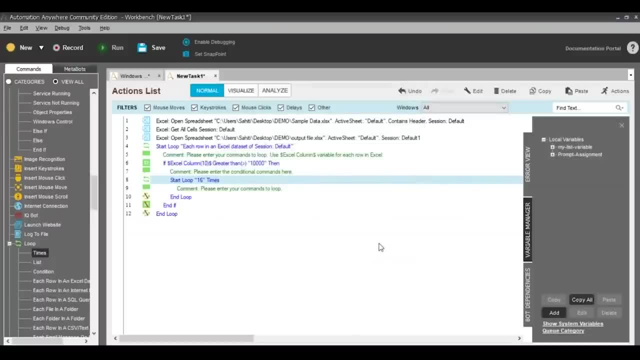 So I wanted to iterate 16 times, So I'm going to choose 16 times, And then what I'm going to do is I'm going to click on save Now for each time the loop is iterating. what we have to do is we have to extract the data from the first spreadsheet. 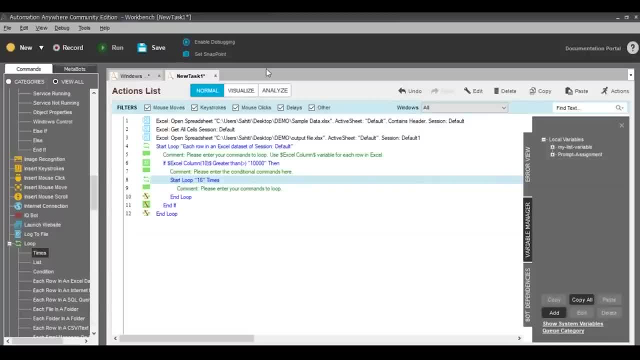 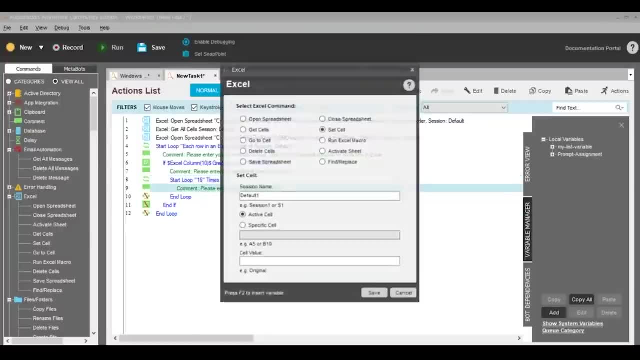 and then store the data into a specific cell in the second spreadsheet. So for that what you have to do is you'll have to go to the Excel command again, and then you'll have to drag and drop the set cell command, And then what you have to do is you have to set the value of the active cell. 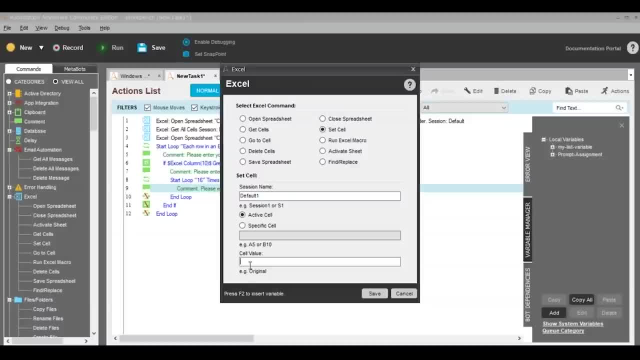 and then mention the cell value, to be our Excel column value, and then the counter value. Basically, the counter will run 16 times, right, When the counter is 1, then it goes 16 times. So the first column gets the active cell. 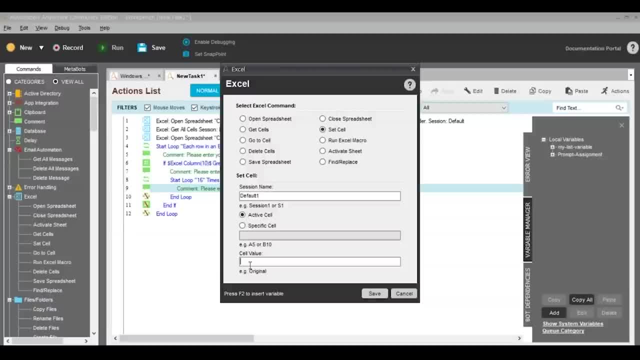 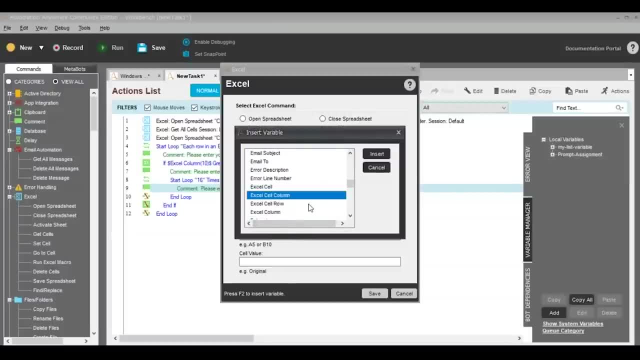 That is basically our value from the first row, first column and then stores it into the first row, first column of our output file, right? So for that we'll mention control F2.. We'll mention Excel column And then what we'll mention is: we'll mention the counter variable, right? 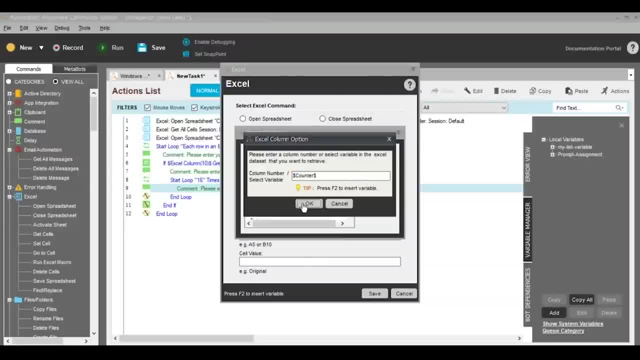 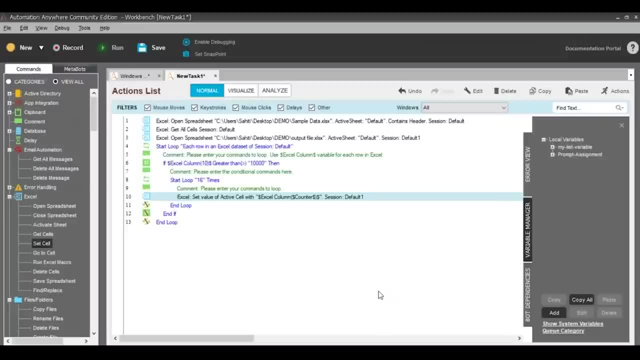 So that's again: control F2,, counter and press on OK, And then I'll click on save. Now what you have to do is, once the value has been stored in the cell of row 1,, column 1,, the next value has to be stored. 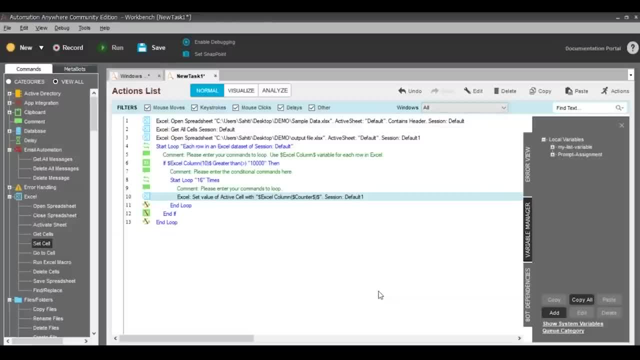 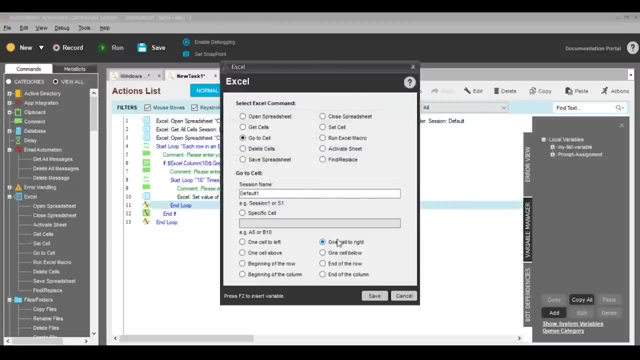 in the next column, but the same row right. So for that you'll have to move one cell towards the right. So for that you just choose the option of go to cell, drag and drop it over here and choose the option of one cell towards the right. 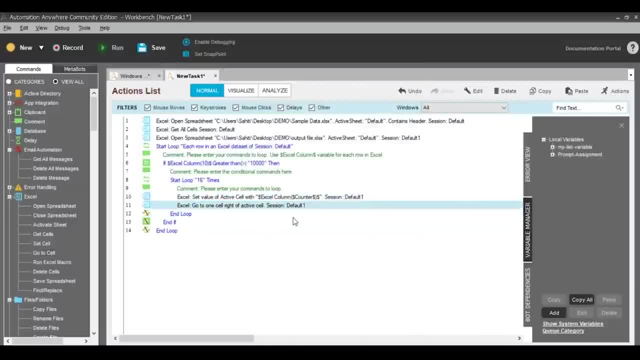 and click on save right, So I'll push it before this loop. Now what I want to do is, once you know one complete row data has been stored, it has to again come back to the beginning of the row. So for that, what you have to do is: 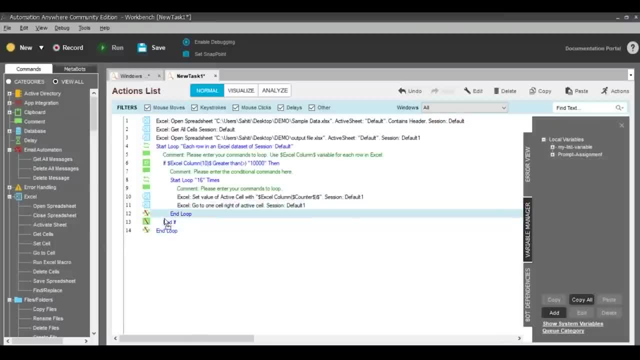 you'll have to choose the option of beginning of the row from the go to cell option. So I'll push it after this loop and then choose beginning of the row and click on save Now. once you go to the beginning of the row, the active cell will be the cell from the first row, first column. 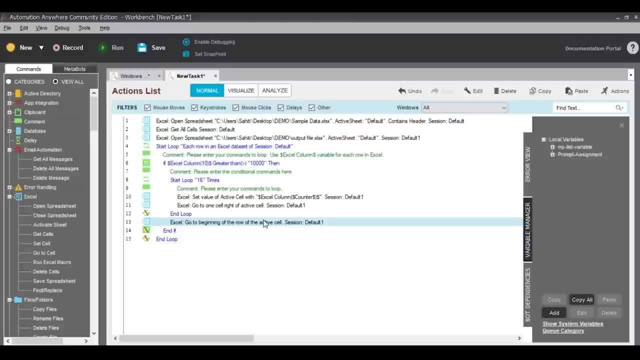 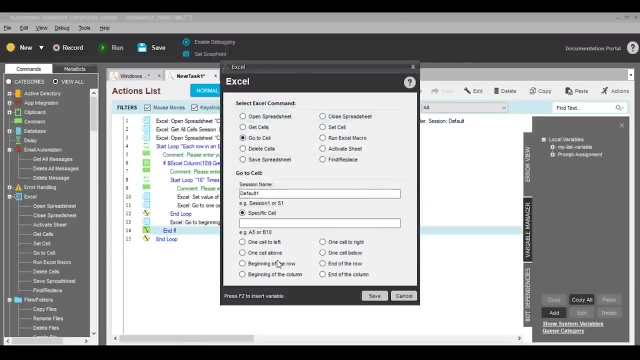 where the data has been already stored. So to store the new data what you have to do is you have to go one cell below. So for that you again go to the go to cell option, drag and drop it over here and choose one cell below. 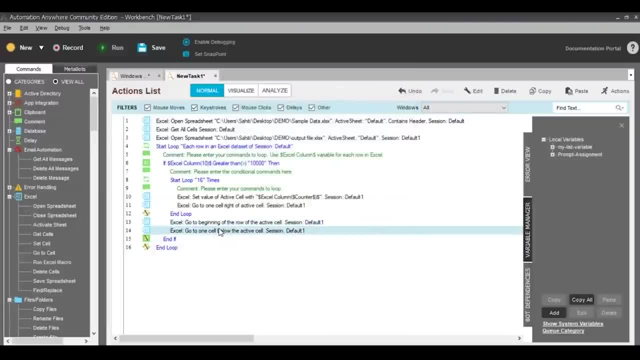 and click on save. So basically what's happening over here, if you see the loop, is that you know you first open both the spreadsheet and then what you do is you get all the cell values from the first spreadsheet. After that you start a loop for each row in the Excel data set. 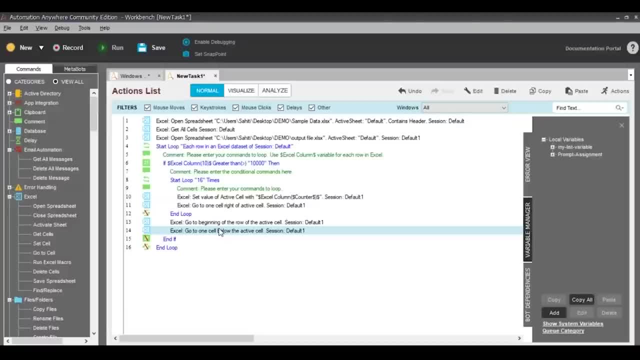 and then you mention the spreadsheet session name and underneath that loop you'll have to mention an if condition where you know if the Excel columns value, basically the sales columns value, that is, the column number 10- has greater than 10,000, then what you want to do is: 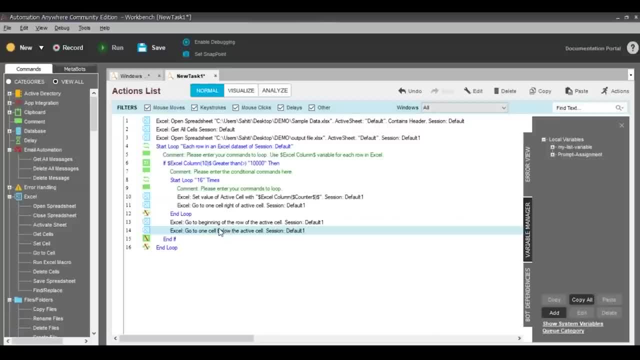 you want the loop to iterate 16 times, because we have 16 columns and for each active cell you'll have to retrieve the data from the cell and then store it in the output file. So what you want to do is you want to store it in a proper format, right? 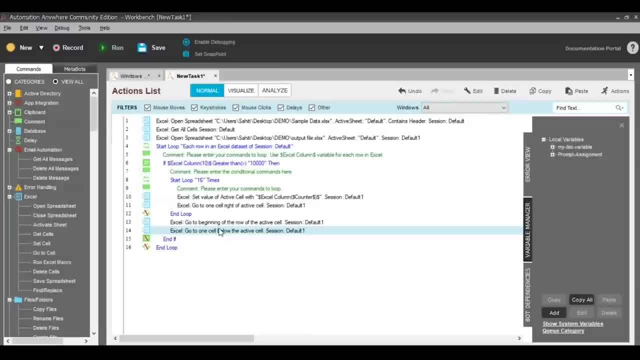 So, like the first value has been stored into the first row, first column, the second value will be stored into the first row, second column, and so on, for 16 times. After that, what you want to do is you want to come back to the beginning of the row. 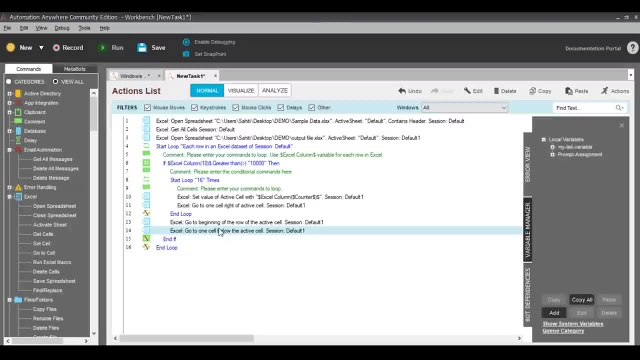 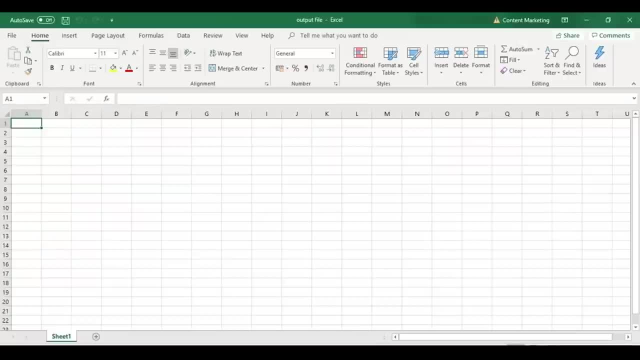 but the next row, right. So for that you choose the command: go to the beginning of the row of the active cell and then go to one cell below the active cell. Now let's just, you know, close this particular spreadsheets so that we get the output. 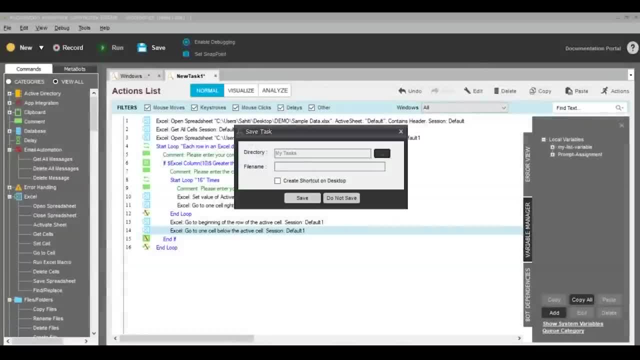 So I'm just going to close this particular spreadsheets, I'm going to save this task. Let's say, you know, we save the task here. it has to be Excel- and then I click on run. So once I click on run, 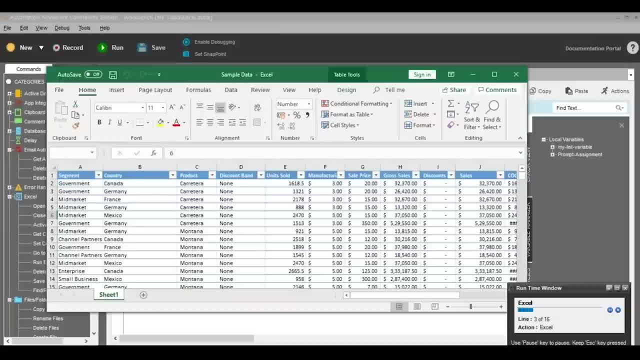 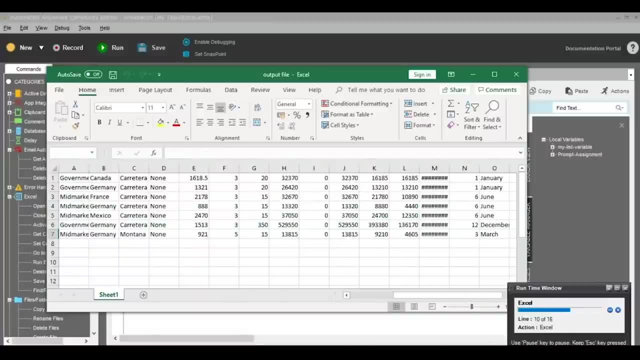 you can see that. you know my task is getting executed, So all the data has been extracted from the first spreadsheet and then it has been getting stored in the second spreadsheet, right? So you can see that happening. So let's just wait for it to complete. 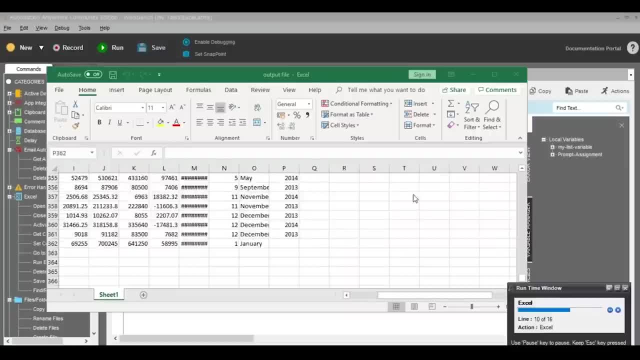 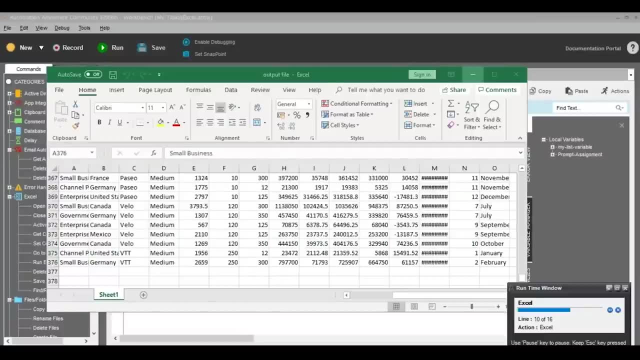 All right, guys. So, as you can see, it is automatically extracting the data from the first spreadsheet and storing the data into the second spreadsheet. So that's how guys you can do Excel automation. Well, I'm going to improve this automation at this moment. 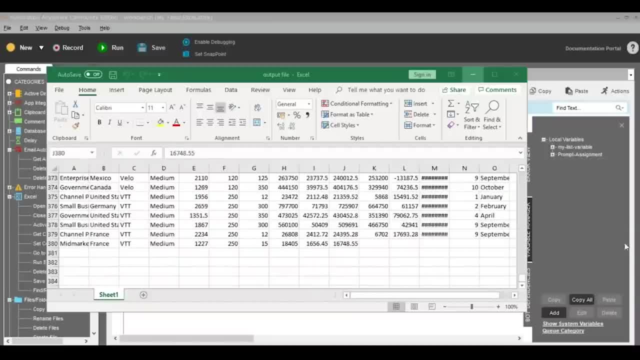 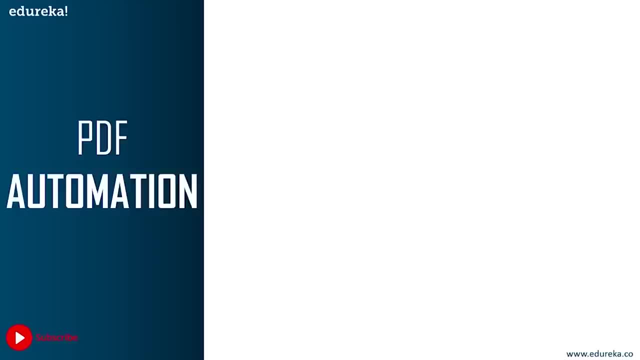 and I'm going to continue with the session, So let me just close this automation Now. next in this session, what we're going to learn is PDF automation. Now, PDF automation. It's also one of the most popular automations in the industry, as I was talking about before. 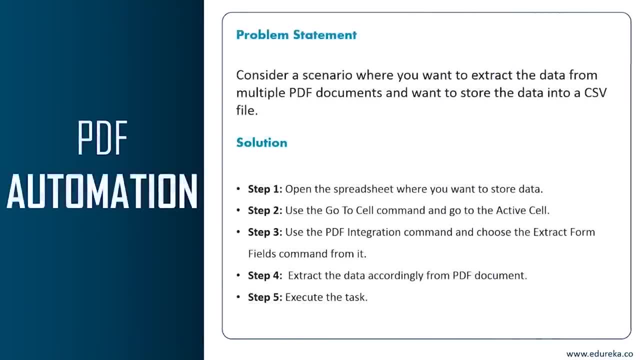 So PDF automation is generally used. you know where you want to merge multiple documents into a single document. or maybe you want to extract data from multiple documents and then store it into a specific file. or maybe you know you just want to extract data until a specific page in a document. 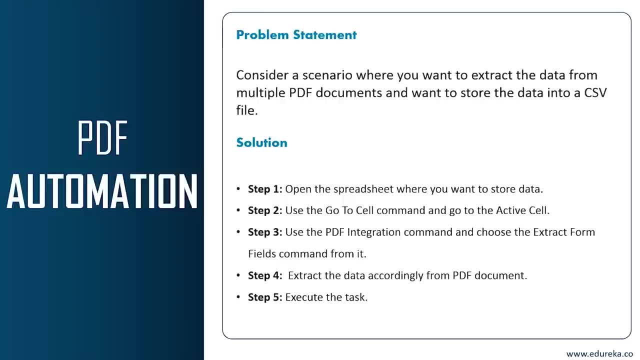 and so on. So what we're going to do is we're going to extract the data from multiple PDF documents and then we're going to store it in a CSV file. So to do that, you'll have to follow a few steps. So first, 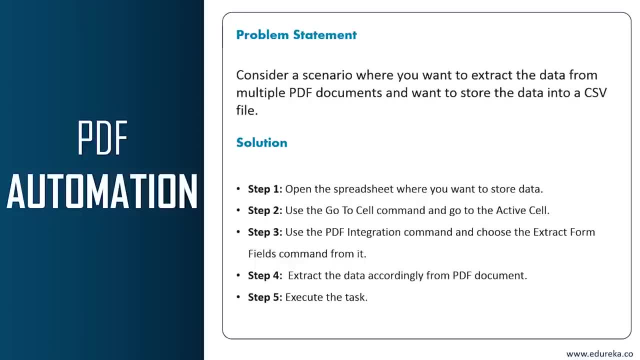 you'll have to open the spreadsheet where you want to store the data, and then you have to use the go to cell command and go to the active cell. After that you have to use the PDF integration command, choose the extract form fields and then you'll have to extract the specific data. 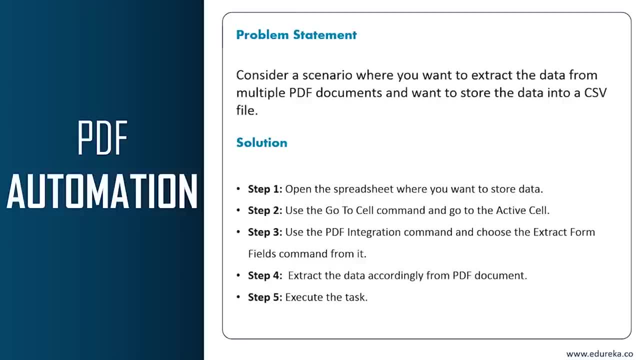 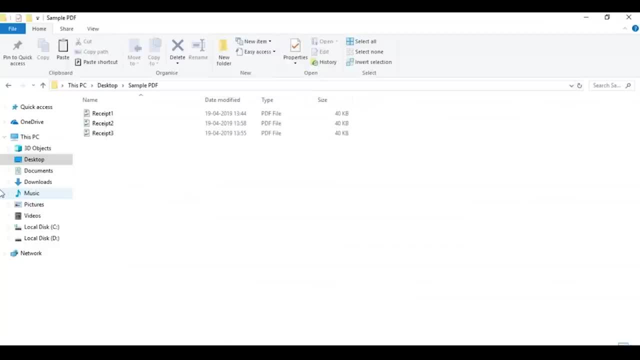 that you want to extract and then use the other Excel commands to decide where you want to store the data. So let's just do that. So, before I do that, let me just open my- you know- PDF documents and show you the documents. 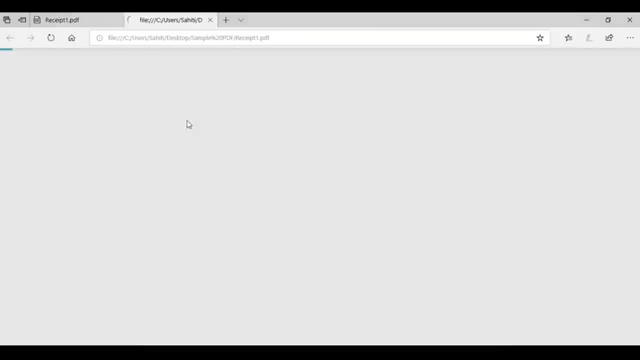 that I'm going to consider. So, as you can see on my screen, these are the documents that I'm going to consider. So, basically, these are the receipts of few students who are studying in a school. So what I'm going to do is. 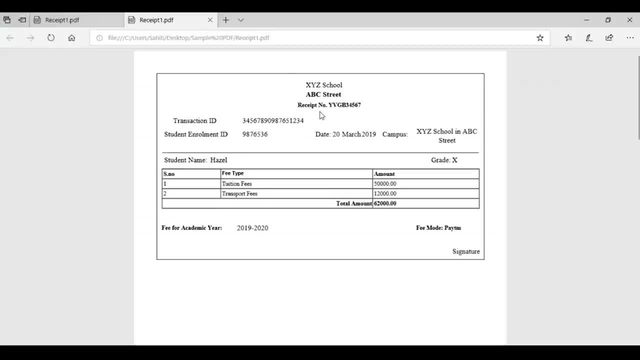 I'm going to extract data, like you know: the receipt number, the transaction ID, the student enrollment number, date, campus, student name, and then total amount and then fee mode. So let's just extract data and extract this data So to do that. 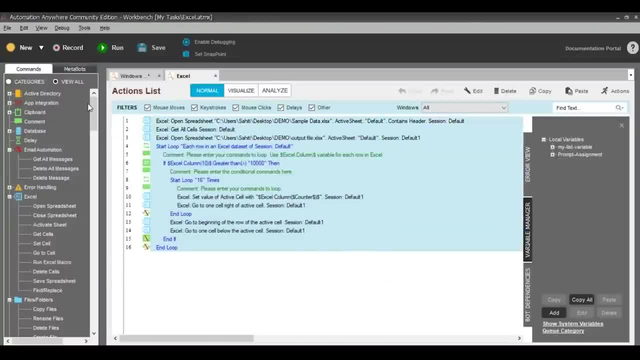 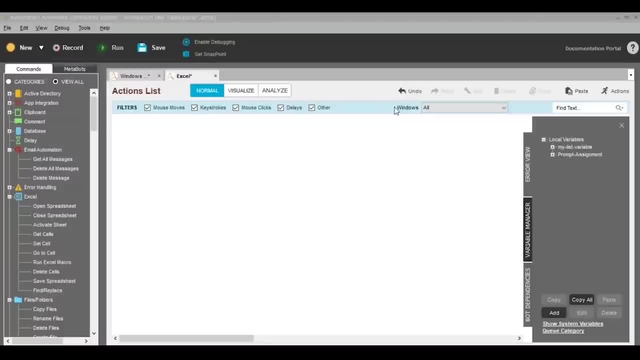 what you have to do is first you have to go back to your Automation Anywhere Workbench. Let's just, you know, remove all this part. So our first step is to open the spreadsheet. So we're going to open the spreadsheet where we're going to store our data. 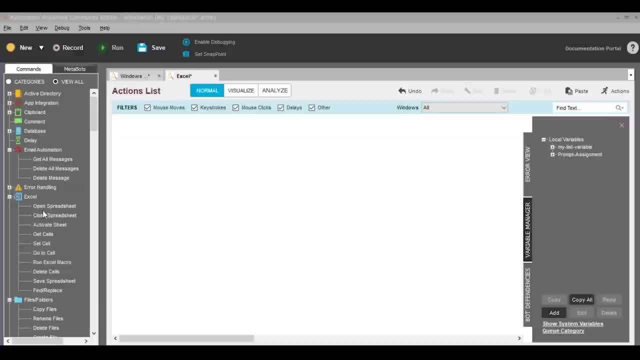 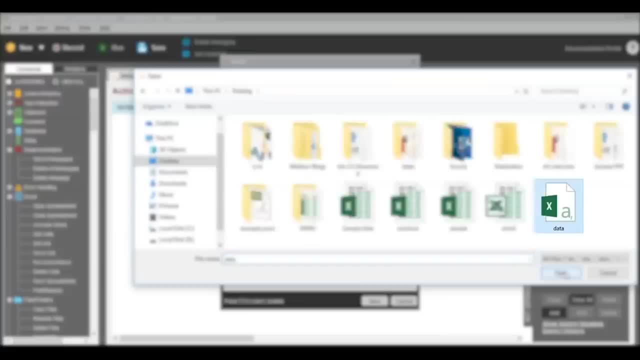 So to do that, what I'm going to do is I'm going to go to the Excel command, drag and drop the open spreadsheet, and then I'm going to mention the part of the spreadsheet. Let's say, you know, we mentioned the part of data. 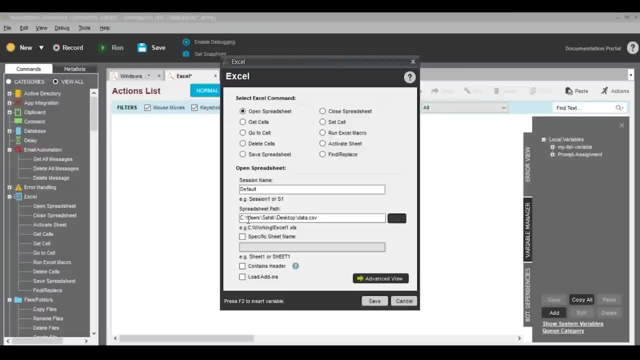 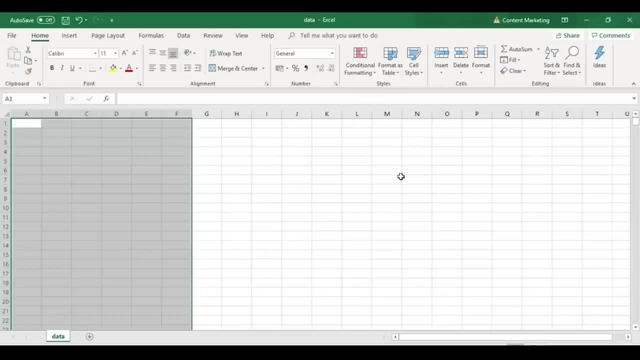 So basically, we're going to store the file into our CSV file. Now what we're going to do is we have to go to our first cell, right, That is basically our A2 cell. So let me just open that spreadsheet and show you. 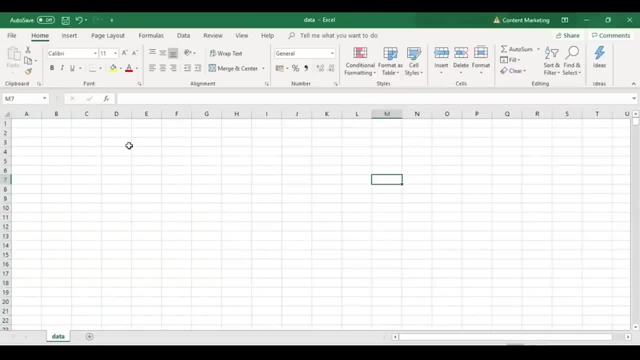 why we're going to the A2 cell. So, as you can see, this is our spreadsheet. Now, why we're going to A2 cell is because you know that is the first cell where we want our data to be stored. That's the reason. 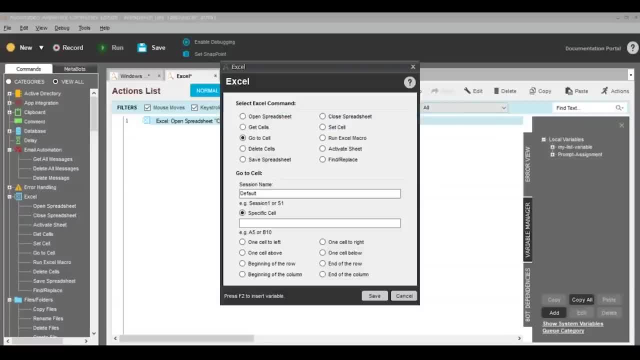 we're going to go to the A2 cell. So to do that, what you can do is you have to drag the go to cell option and then you'll have to mention the specific cell. So we're going to mention the specific cell to be A2. 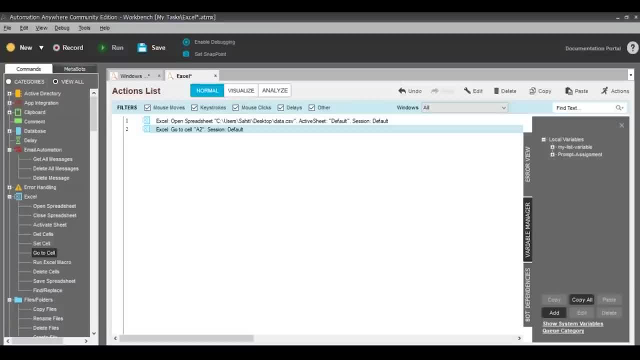 and then we're going to click on save. So basically, what you have designed in your automation pane is that you know it has to open the spreadsheet and then it has to go to the A2 cell. Now what you have to do is: 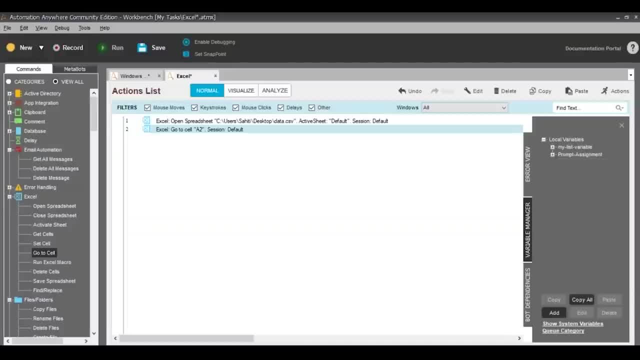 you have to extract some data from the PDF document and then you'll have to store it into the spreadsheet. So, before you know, we start extracting the data. let's create variables to do that. So we go to the variable manager and then we'll add variables. 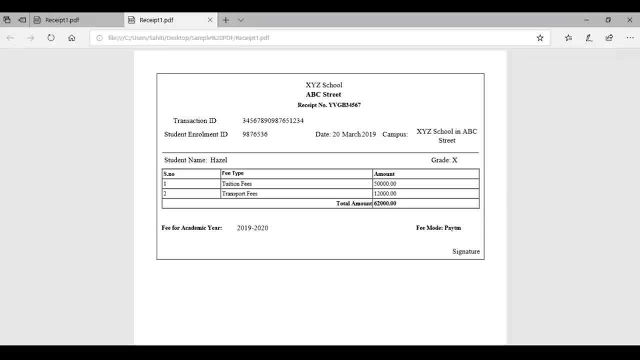 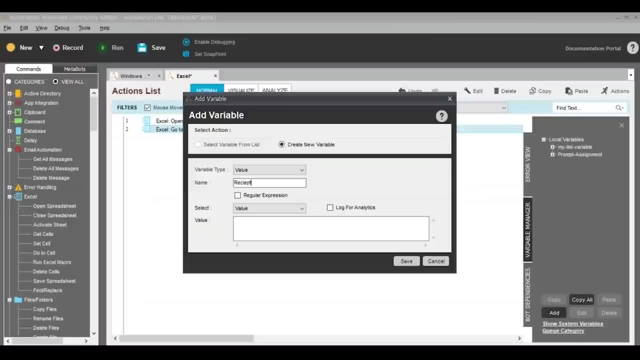 So what I want to extract is the receipt number, transaction ID, student enrollment ID and so on. So for that let's just create the variables. So first I'm going to create a variable for receipt number and then I'll click on save. 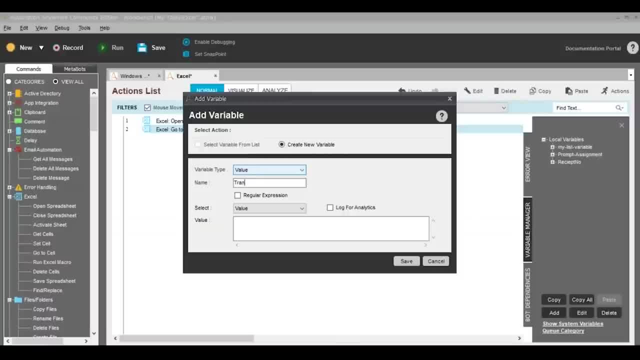 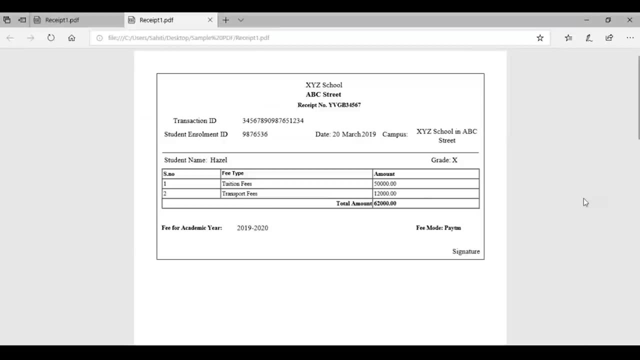 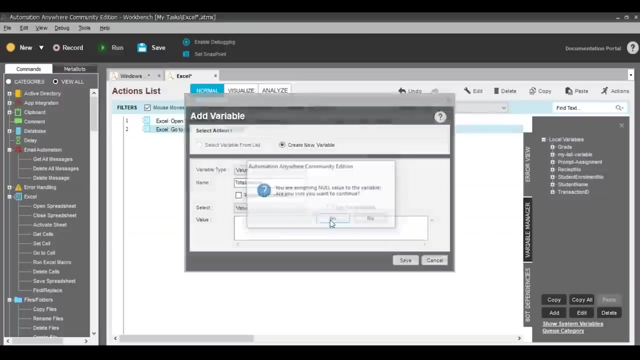 Similarly, I'm going to create variables for the other, like you know, transaction ID, student enrollment number, then student name. Then let's also create variables for you know grade, total amount, fee mode, payment, And let's also create a variable. 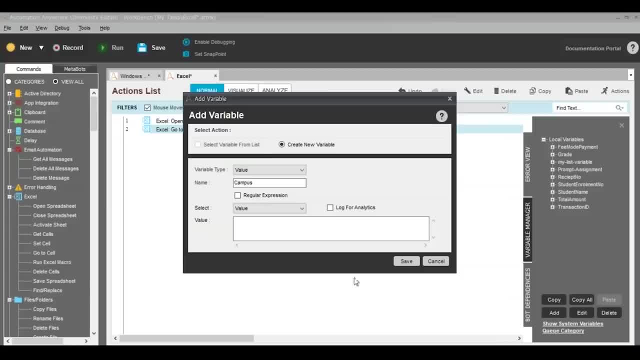 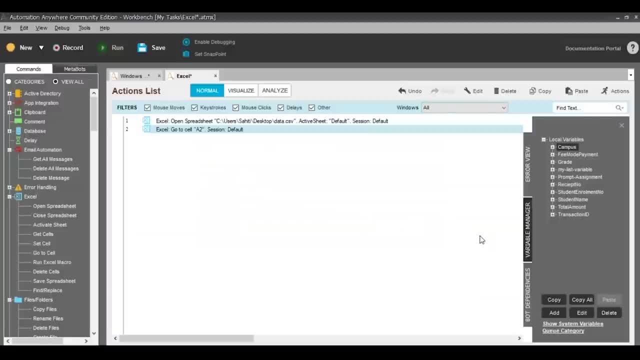 for the campus, right? So I'm just going to create a variable for campus and click on save. So these are the various stuff that we want to extract from our PDFs. Now, to start extracting data from our PDF, what we have to do is: 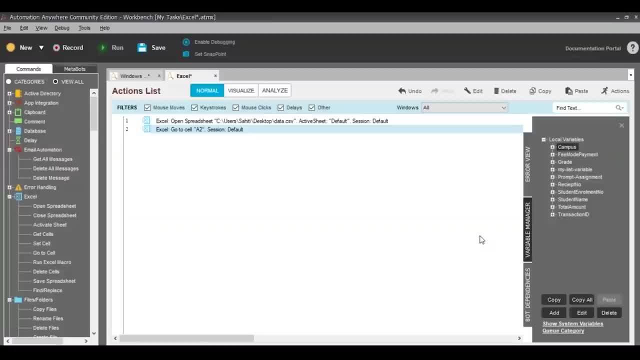 we have to design a loop, So we have to choose the loop of each file in a folder, because all our PDFs are present in the folder. So for that we'll go to loop option, then choose each file in a folder, drag and drop it over here. 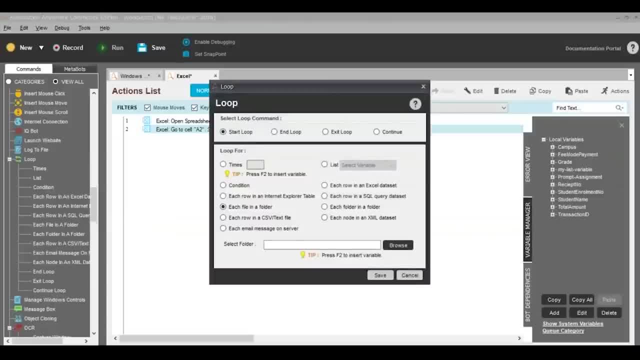 and then what we'll do is we'll mention the folder's name. So I'll mention sample PDF, and then we'll choose each file in a folder, drag and drop it over here, and then what we'll do is we'll mention the PDF name and click on OK. 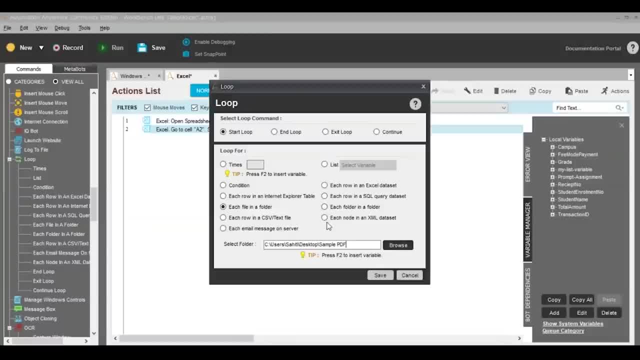 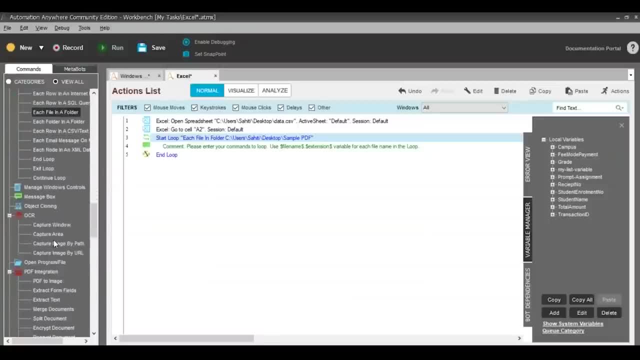 So for all the PDFs present in this particular folder, the data would be extracted and it would be stored into the CSV file. So we're going to do that and then we'll click on save. Now what we'll do is we'll use the PDF integration command. 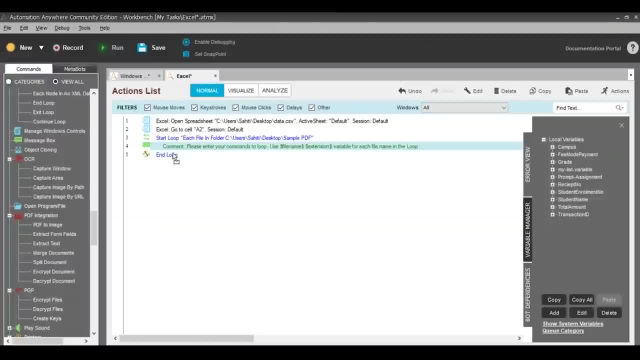 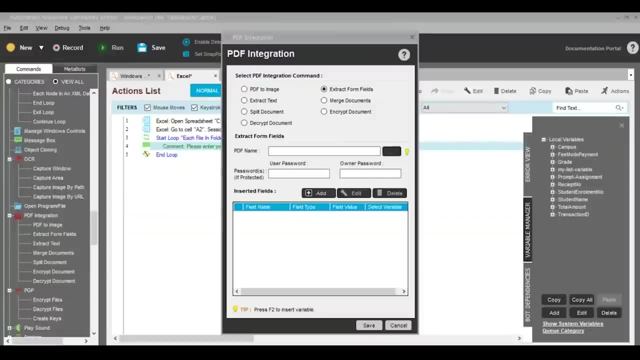 and then we'll choose extract form fields. This is because you know we want to extract specific values from the PDFs, right? So that's the reason we'll choose extract form fields and then over here we'll mention the PDF name. 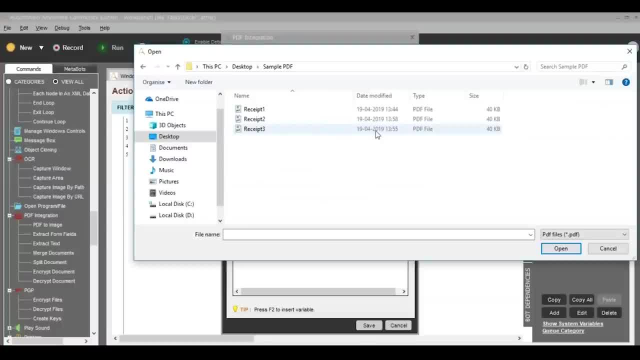 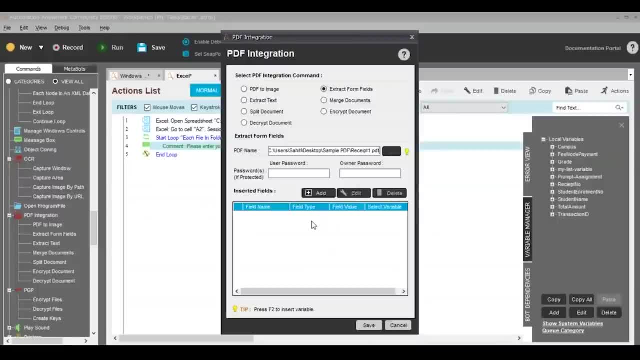 So, for example, let's say we mentioned the first PDF name, So for that we'll choose the first one open, And then you know if your PDF is encrypted and you can mention the user password and the owner password. So for example, 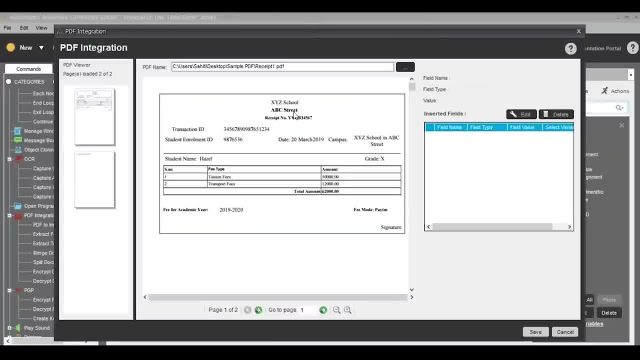 if I want to extract the received number. what I'm going to do is I'm going to go to add, I'm going to drag my mouse over the received number and then I'm going to right click over here, choose add field and mention the fields name. 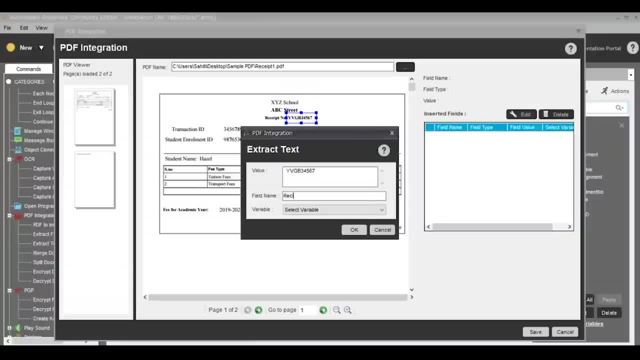 So let's say you mentioned the fields name to be received number and choose the variable where it has to be stored. So it is basically received number, and then we'll click on OK Now. similarly, I'll click on save over here and then I'll again click on add. 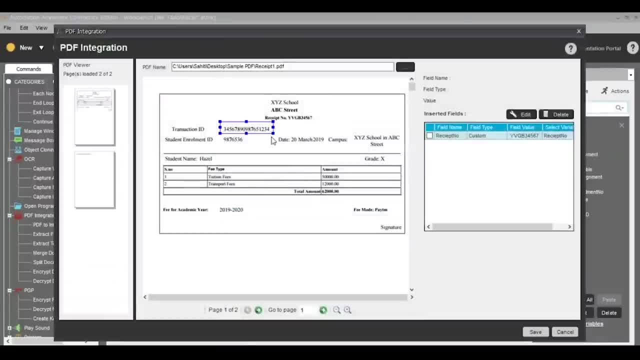 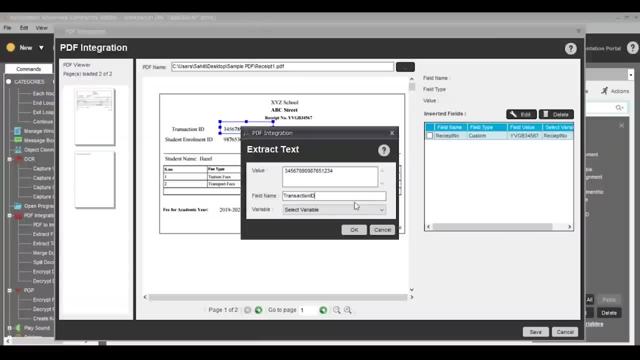 and choose the transaction ID. I'll right click over here again, go to add field and then mention the field name. that is transaction ID, and then I'll choose the variable. So our variable is transaction ID. for this I'll click on OK and save. 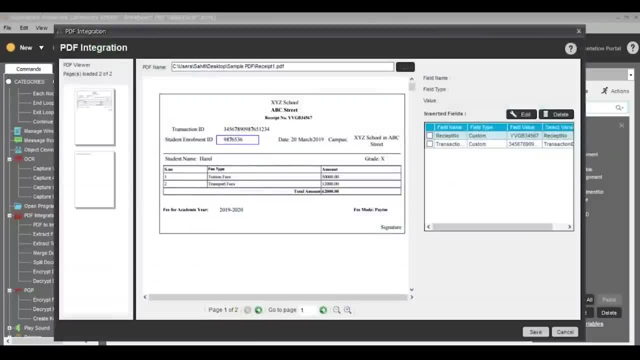 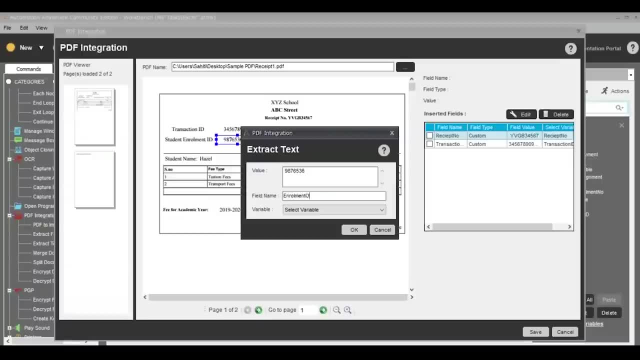 Similarly, what I'm going to do is I'm going to drag my mouse over the student enrollment ID. I'll right click over here, choose add, mention the fields name, let's say enrollment ID, select the variable of student enrollment number and click on OK and save. 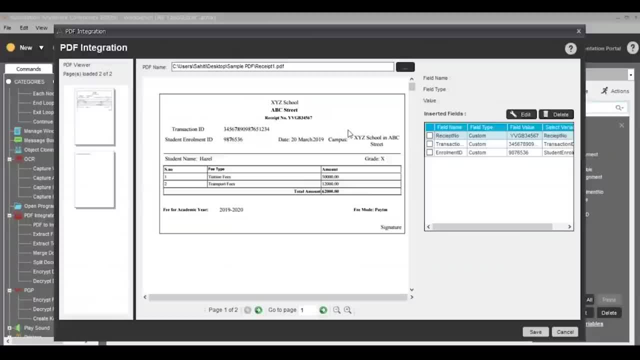 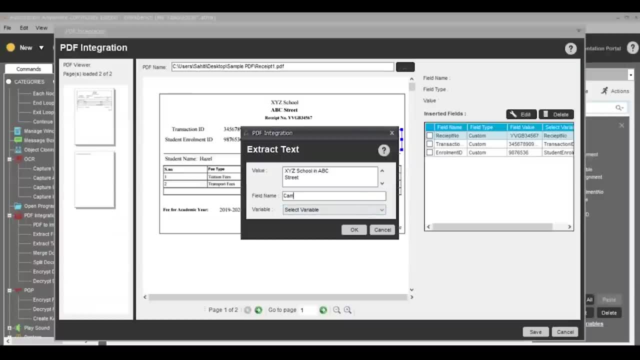 Similarly, I'm going to add again for the others, like you know, campus. So I'm going to choose drag and drop this campus right click over here, mention the field name to be campus, select the variable for campus, click on OK, save. 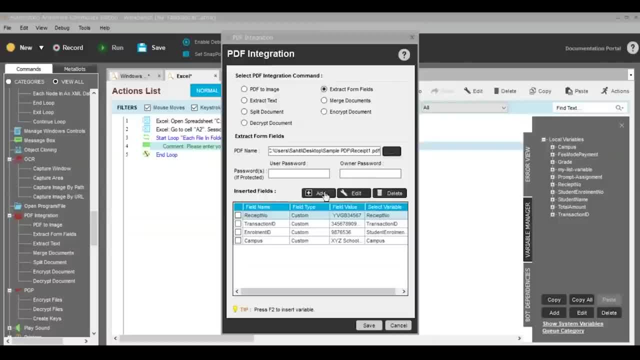 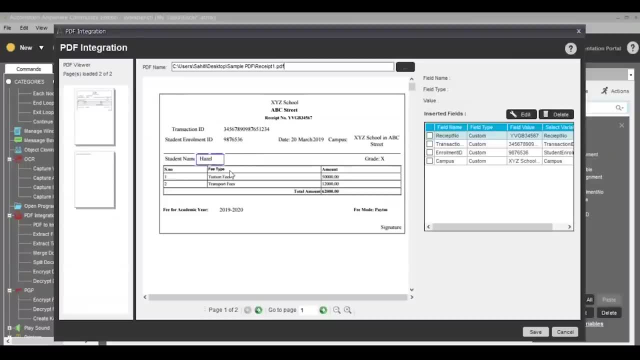 Now, guys, this step is going to repeat until we cover all our variables. So let's just keep covering all our variables, one after the other. Now I'm going to extract my student name, So that is, I'm going to drag my mouse. 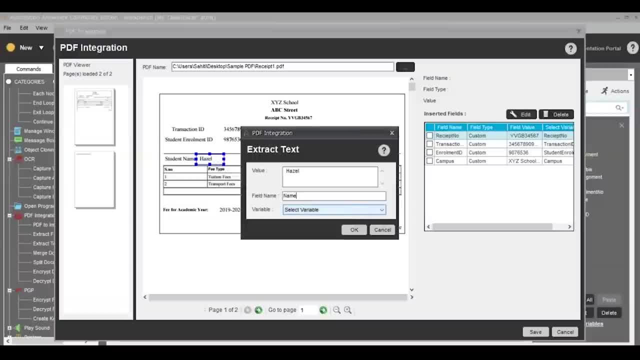 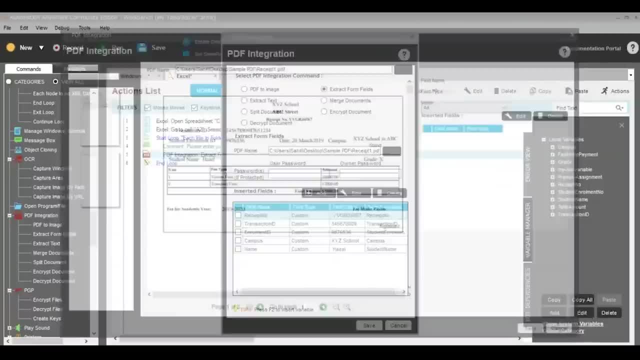 over here right click, choose add field. mention name as my field name, mention student name as the variable. click on OK and save. Now again I have to click on add and then I have to choose total amount, right? So I'm going to drag my mouse. 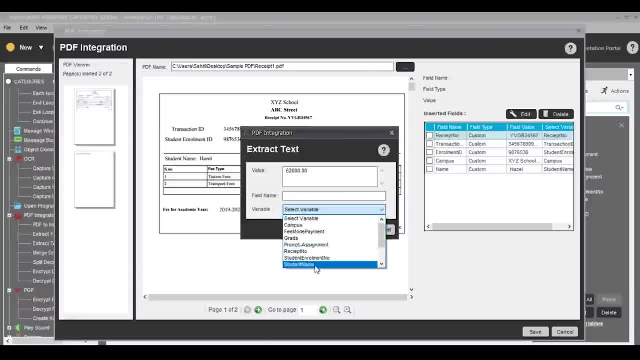 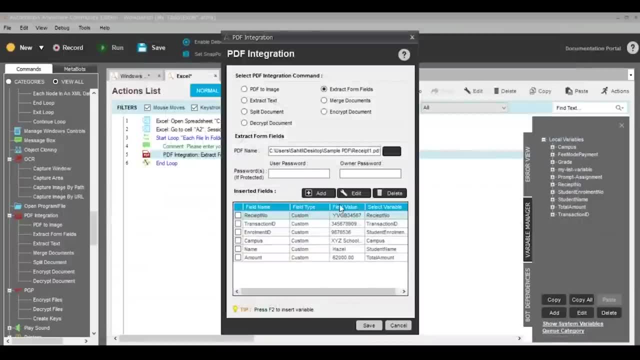 over here, right click over here. mention the variable name to be total amount. mention amount as field name and click on OK and click on save. Similarly, I'm going to do that for my fee mode, So I'm going to mention: 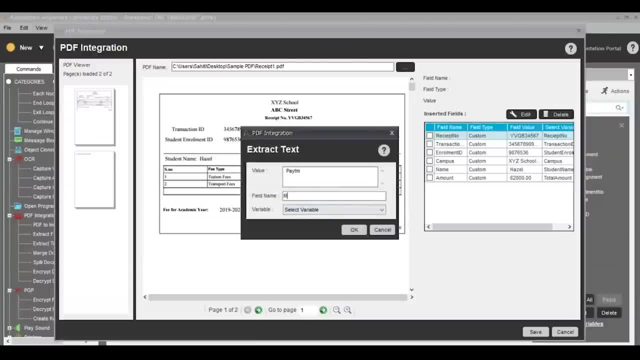 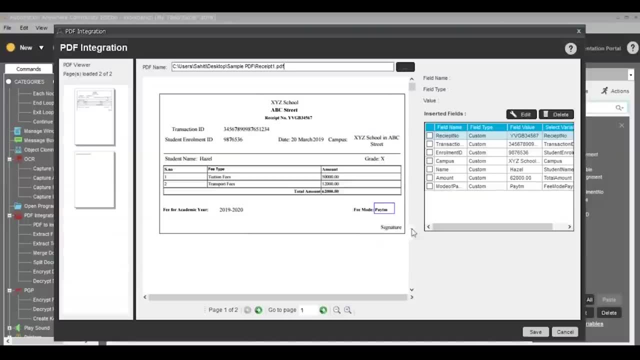 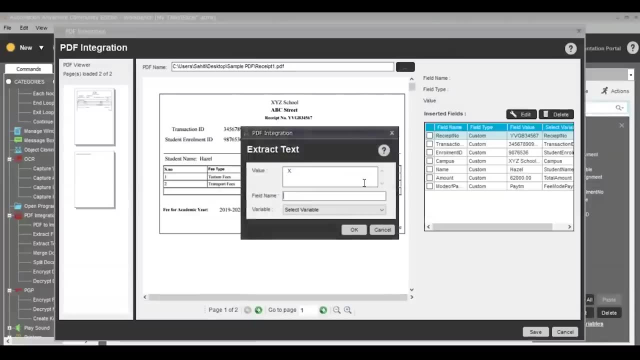 my fee mode right. click over here again. mention mode of payment. select variable, that's fee mode payment. click on OK, click on save again. Now again, I'm going to do the same for grade add field again, and then I'll just say: 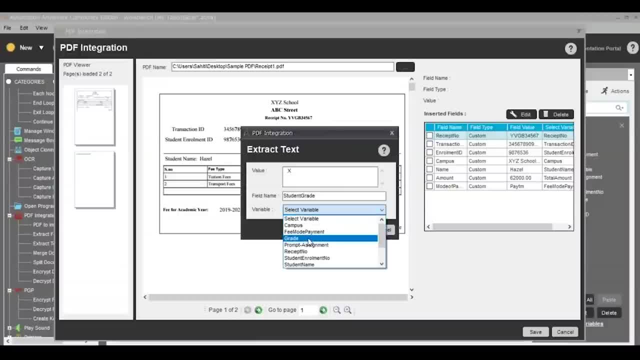 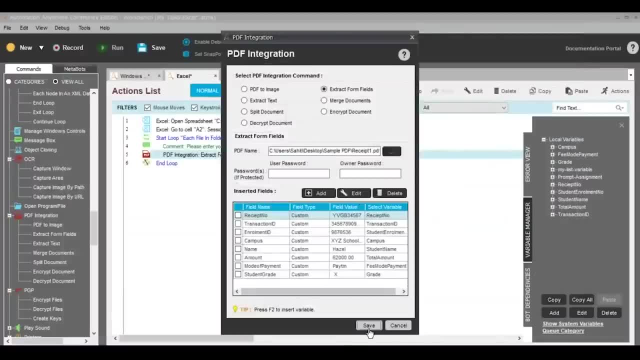 student grade, select variable grade, click on OK and save. And now, since all our variables have been covered, I'll just click on save. and this is done. Now, once all the data has been extracted, what has to be done is 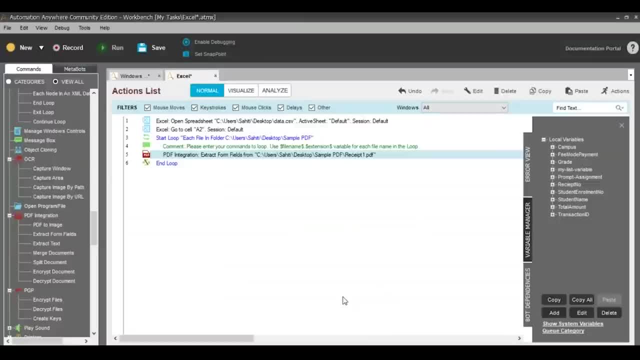 it has to be stored in specific values, right in specific cells of the Excel sheet, right? So to do that, what you have to do is you'll have to go to the Excel command, And then what you have to do is you'll have to set values. 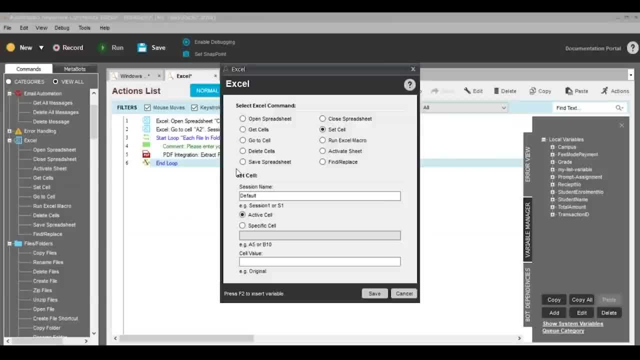 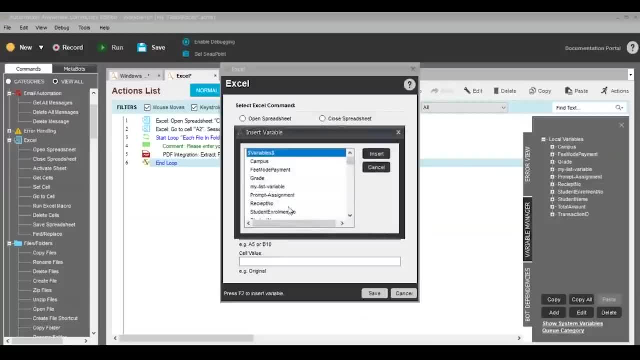 and then move your active cells to the next cells, right? So you'll have to set values. let's say you know we've set our specific active cell to be of received number, So we'll just press on control F2, choose first value. 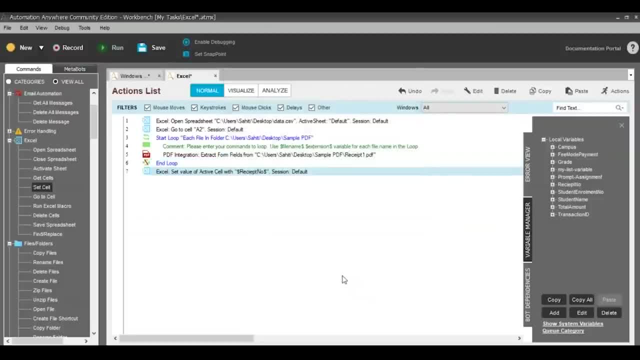 to be stored. that is received number. click on insert and save. Now what I'll do is I'll go one cell towards the right so that I store the next value of the same PDF. So I'll just drag before the loop ends. 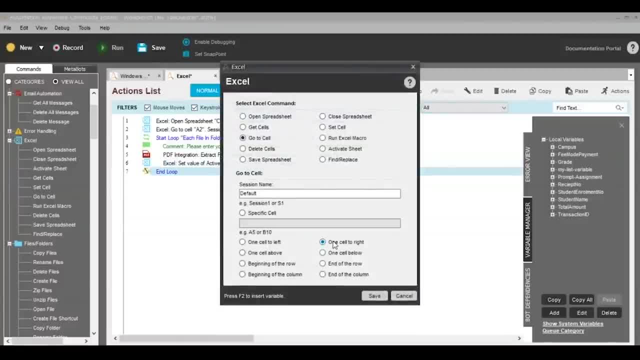 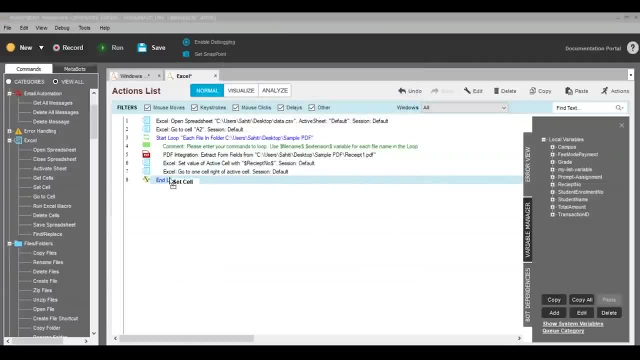 And now I'll just drag and drop, go to cell over here and choose one cell towards the right and click on save Now. similarly, I'll have to do this to save all the variables. So let's just drag and drop the set cell. 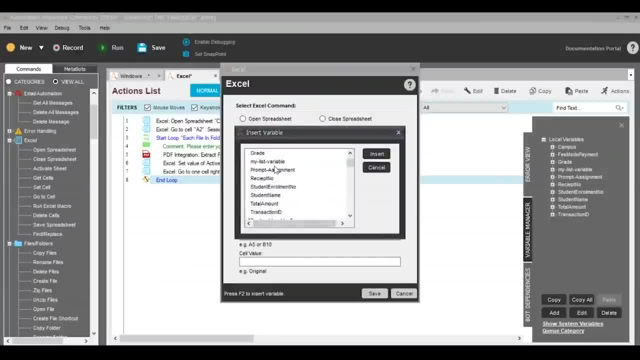 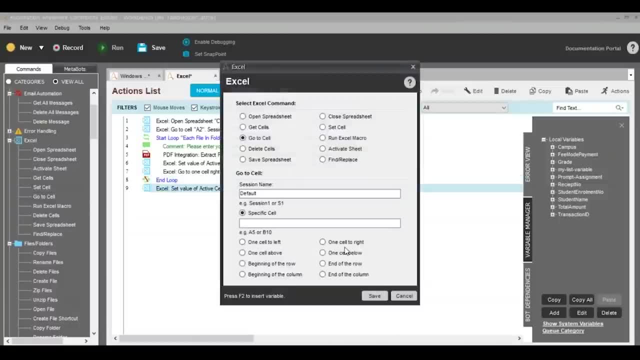 action again Now over here after the received number. I want the transaction ID to be saved, So I'll choose a transaction ID variable, I'll click on save and then I'll choose go to cell and then one cell towards the right. 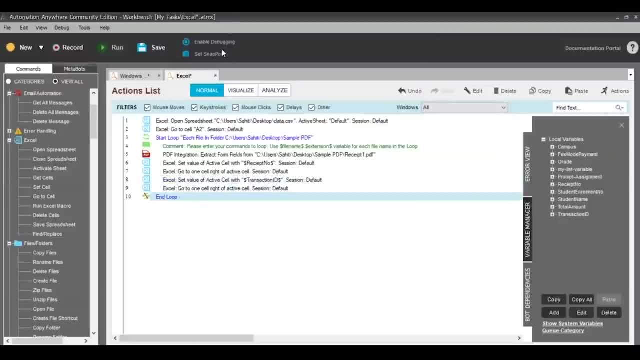 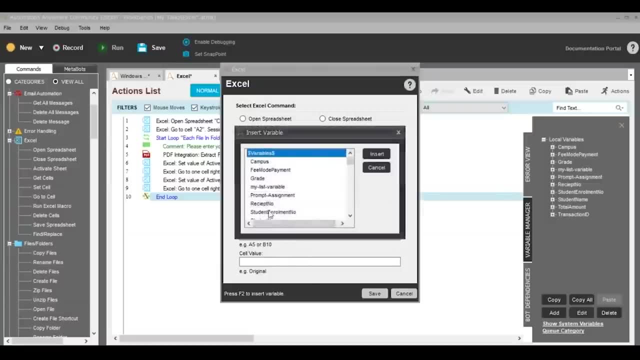 So these two have to come before the loop ends. Similarly, all the actions have to come before the loop ends. So I'm going to do it quick now. So I'll drag set to cell again and then I want student enrollment number to be saved. 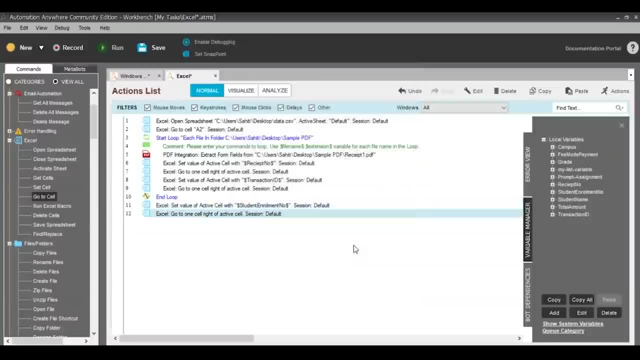 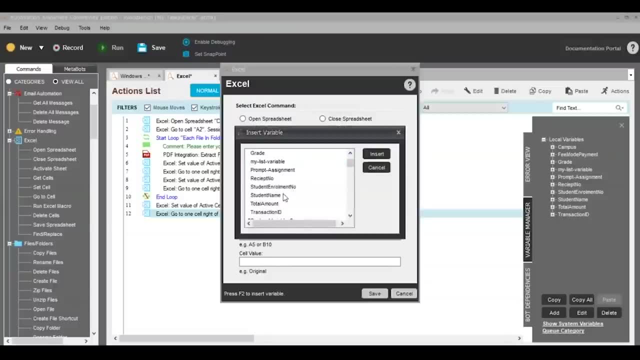 All right. Now you'll have to again go one cell towards the right and click on save Right. Similarly, you'll have to again drag the set cell option and let's say we want to choose the student name. So I'll mention student name. 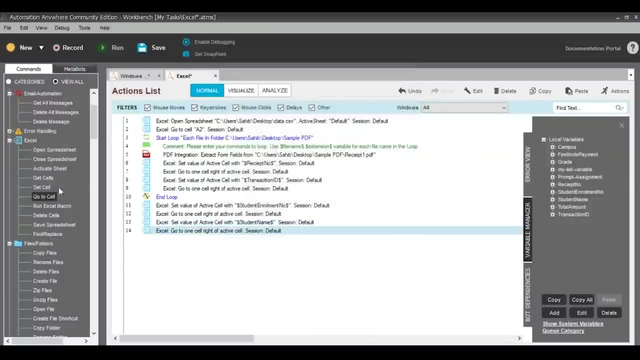 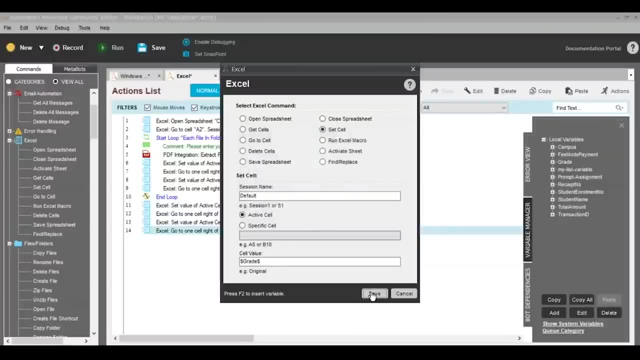 click on save and then again drag the go to cell option and choose one cell towards the right. Similarly, I'll drag the set cell option and let's say we want to choose the grade Right, So we'll choose grade and then click on save. 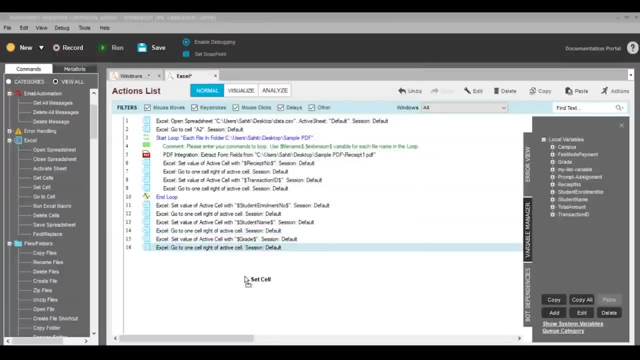 and again drag the set cell option and click on save. Similarly, I'll drag the set cell command again. and now let's say you know we want to save the campus, I'll click on insert, I'll save, I'll again go to. 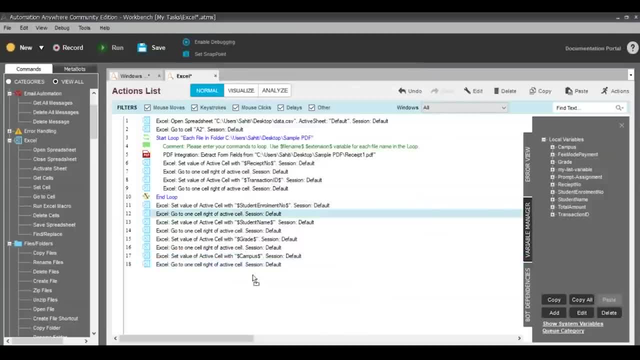 go to cell and then I'll choose one cell towards the right and click on save. Now I'll again drag the set cell option and let's say we want to save the total amount, So I'll search for total amount. click on insert. 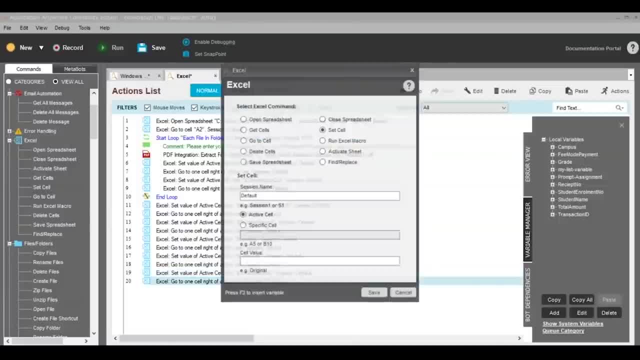 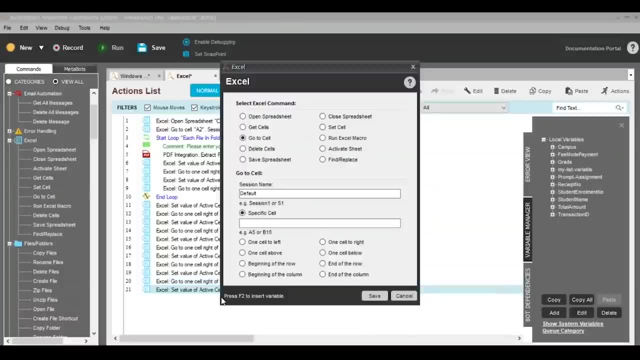 save, then go to cell and one cell towards the right option and then I'll finally save the fee payment, Basically the fee more payment. I'll click on save and then choose, go to cell and choose one cell to the below. This is because 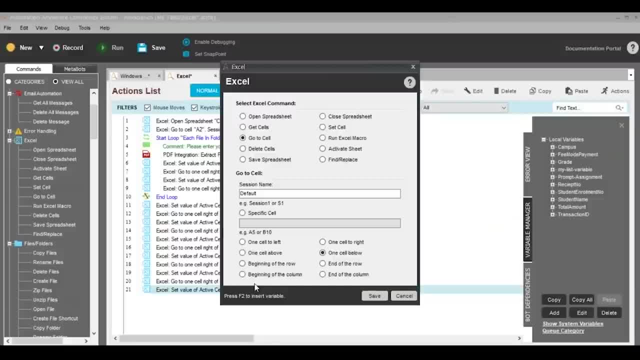 you know, this is the final value that will be stored for one PDF. After that, to iterate the same thing for other PDFs, what you have to do is you have to go to the next cell and then go to the beginning of the row. 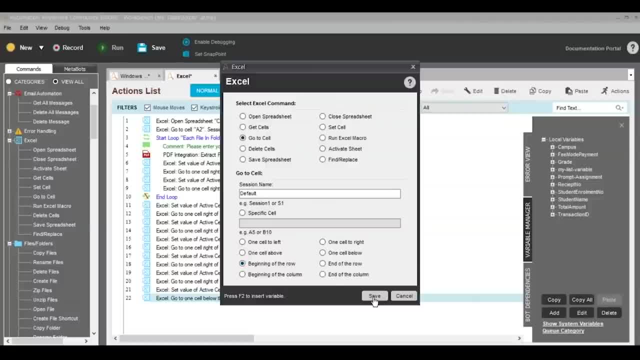 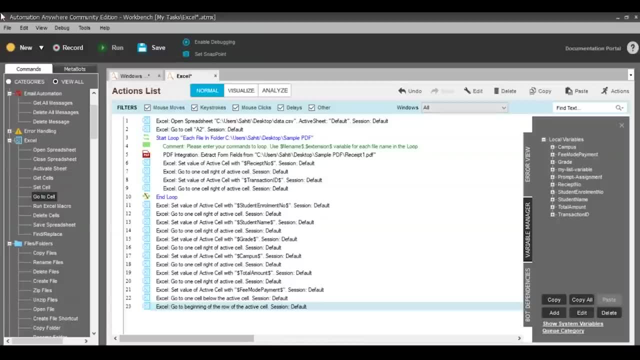 Right, So we'll go to one cell below and then what I'll do is I'll again drag, go to cell and choose different data of different PDF documents into a single CSV file, into different different rows. Right, This has to basically come at the end. 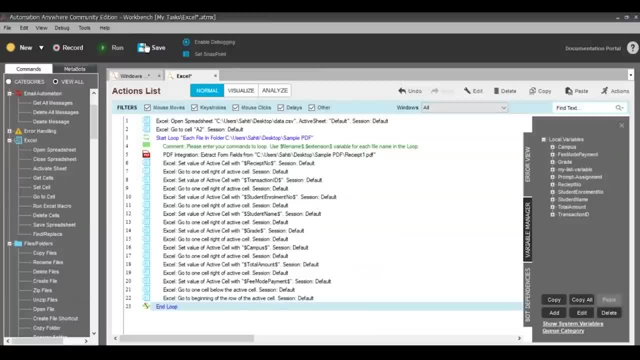 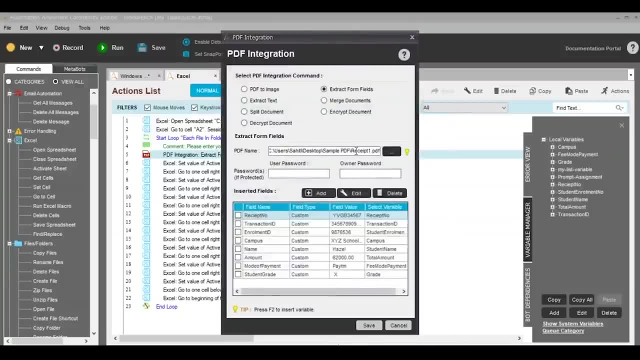 so that you know we finished a loop, and then I'll just click on save Now, once the task has been saved. one more thing that you have to change is in the PDF integration command, If you just observe, you've just mentioned. 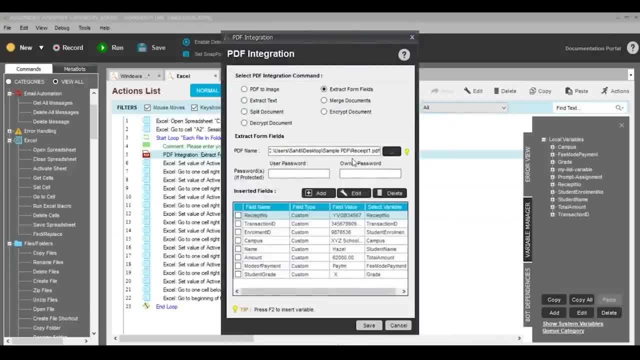 the PDF name to be of a single PDF. But yes, we want all the PDFs in a specific folder to be taken into account and from there all the data has to be extracted and stored into a CSV file. Right, So for that. 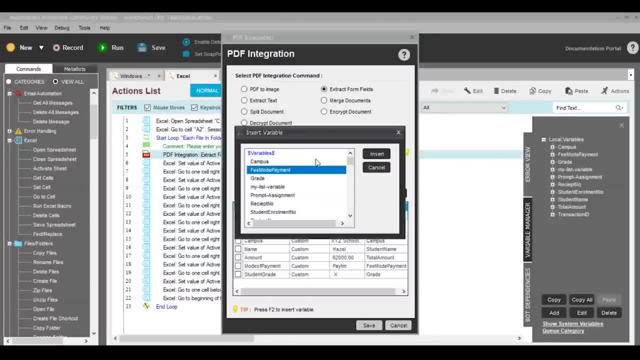 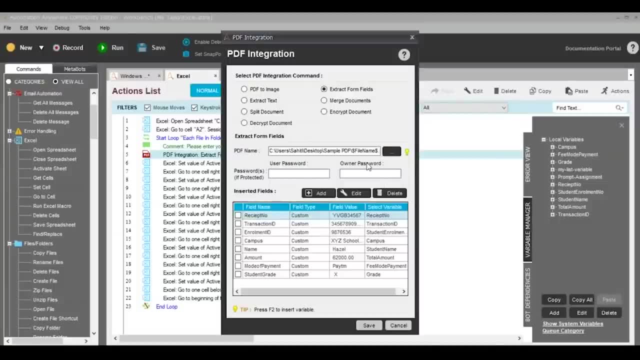 we'll remove the file name and you'll use the variable of file name, that is, control F2.. If you press, if you search for file name, you'll get the variable file name. You can click on insert and then, if you just save your task. 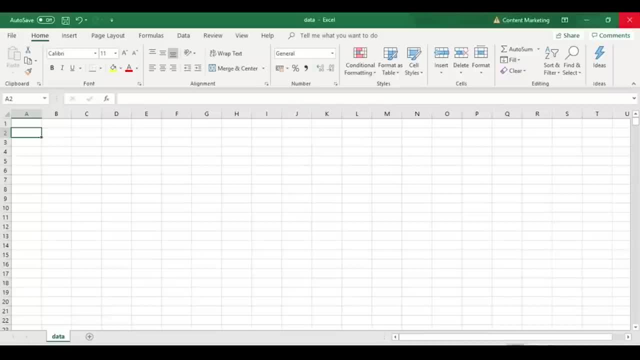 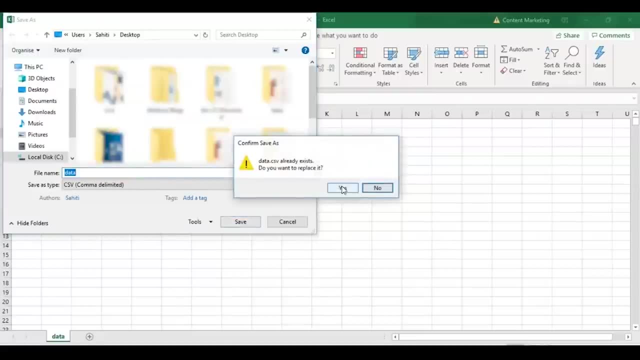 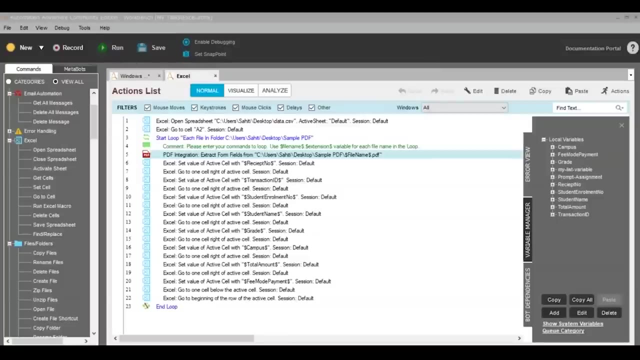 you're good to go to execute this task, Right? So let me just close this datacsv file. I'm just going to run, I'm just going to execute this task and once the task is getting executed, you'll see that you know. 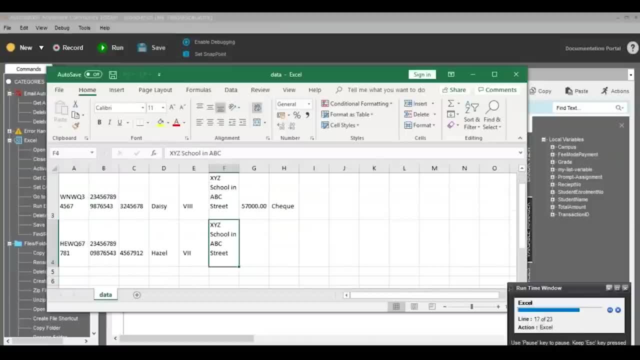 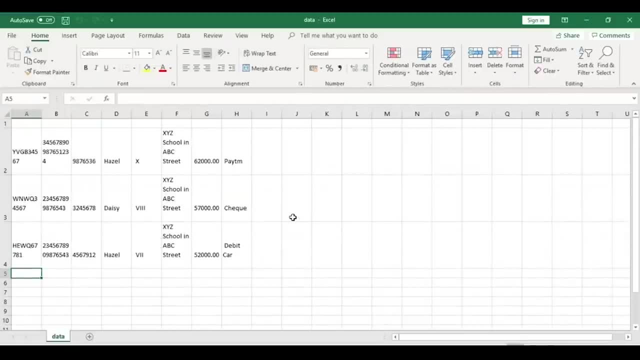 automatically, data will be filled into the Excel file. So you can see that you know. automatically the data from the three PDF documents that were present in that particular folder, that is, the sample PDF folder, are filled into our CSV file. So that's how, guys. 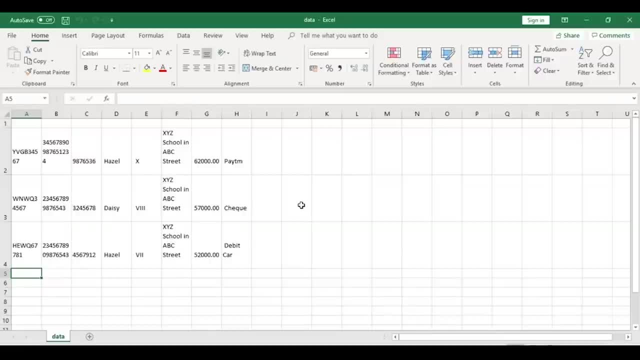 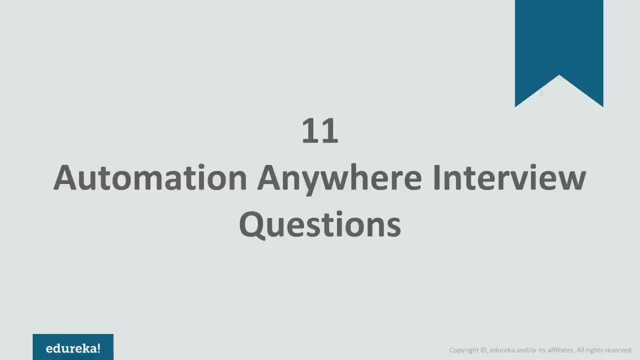 you can automate task on PDF documents and also integrate the Excel commands with the PDF commands. Welcome to this session on automation anywhere- interview questions. So without any further do let's look into the topics for today's session. So we'll start today's session. 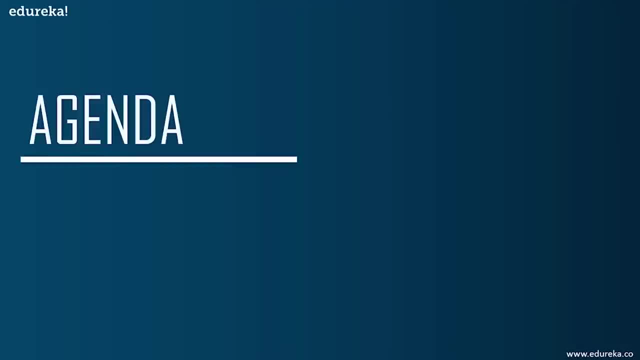 by looking into the market demand of automation anywhere, and then I'll take you to the different types of interview questions. So, for your better understanding, I have divided this interview questions into three sections, That is, the basic interview questions, the tool based interview questions and the scenario based interview questions. 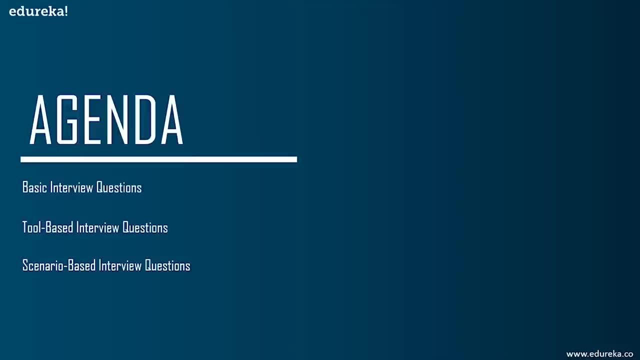 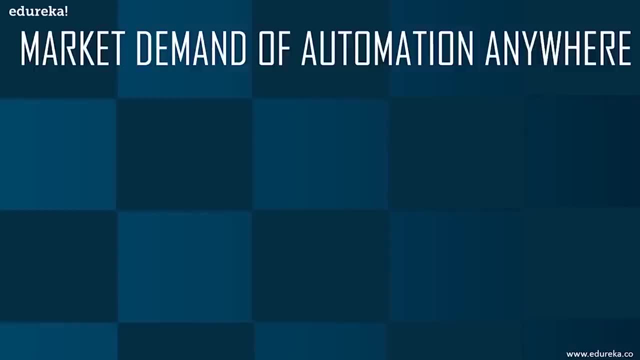 So in each section we're going to discuss different types of interview questions. So, guys, I hope I'm clear about what we're going to discuss today. So let's get started with the market demand of automation anywhere. So, as you can see on my screen, 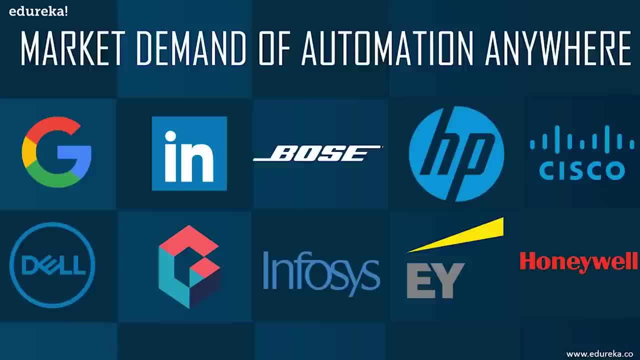 multinational companies such as Google, LinkedIn, Cisco, Dell, Genpak, Honeywell, IBM, HP, Infosys and many other companies use automation anywhere in their day-to-day tasks to automate simple to complex tasks. But the problem is not everybody has the knowledge of automation anywhere in depth. 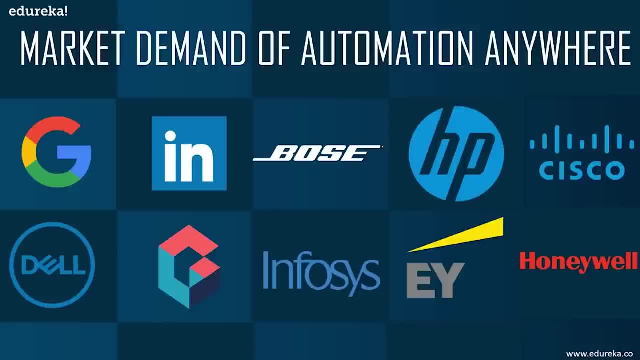 So if you're working for a company and if you want to scale your career as an RPA developer, then you need to have an understanding of different tools used in the RPA industry, such as UiPath, Blue Prism and automation anywhere. So, guys, I hope you know. 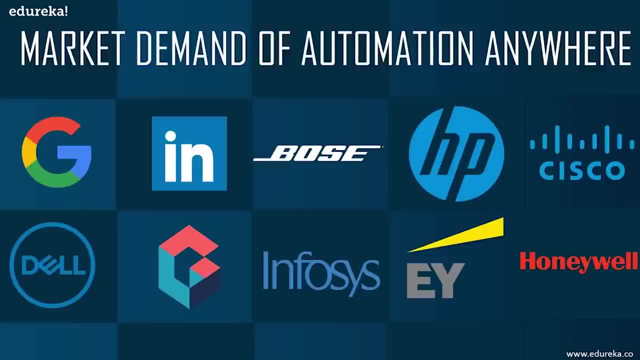 you have understood what is the importance of RPA developers in today's market. So, in that note, obviously anybody who wants to scale their career as an RPA developer needs to have an understanding of various tools, as I said before. right, So this session will focus. 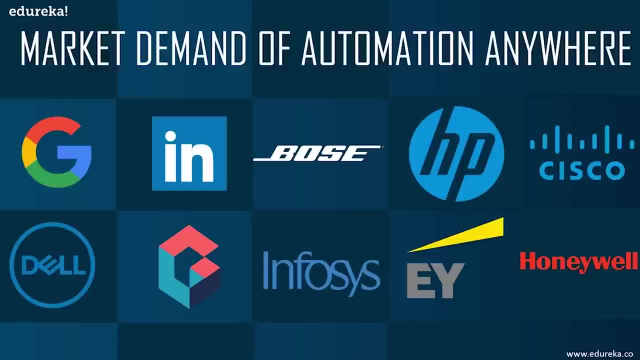 on automation anywhere. So in this session on automation anywhere, as I previously told you, I'll be discussing the top questions that are asked in your interviews related to automation anywhere. So we'll start with the basic questions first. Well, this section of questions will consist: 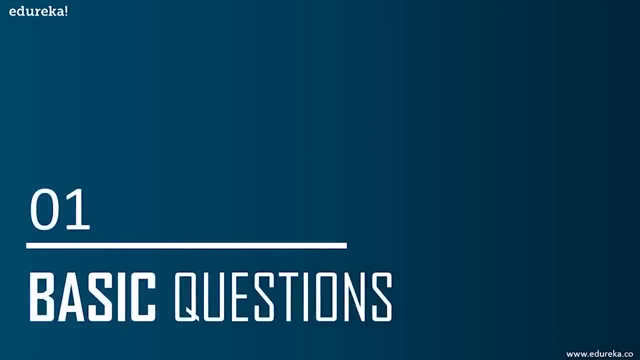 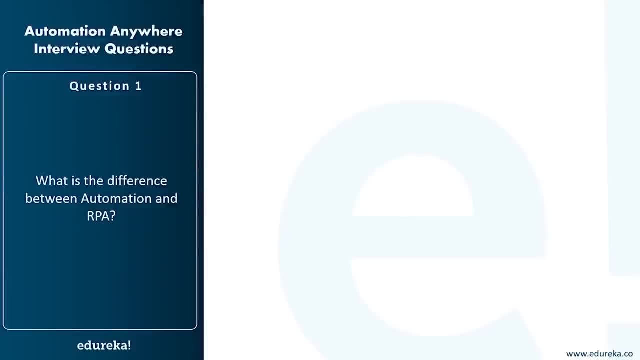 of those basic questions that you need to understand, related to robotic forces, automation and also the tool automation anywhere. So, starting with the first question, the first question is: what is the difference between automation and RPA? Now, if you have to differentiate automation and RPA, 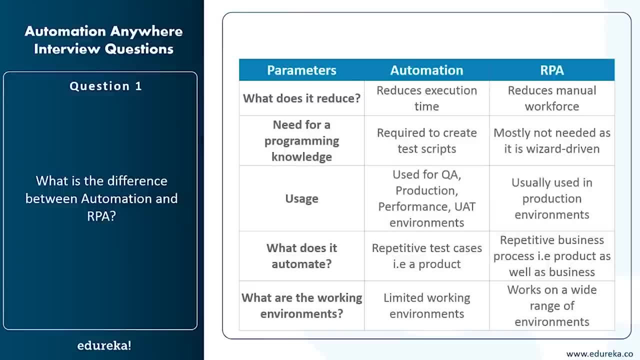 well, you can differentiate automation and RPA on various parameters. The parameters could be: what does it reduce the need for automation, for programming, knowledge usage? What does it automate and what are the working environments? Talking about the first parameter, that is, what does it reduce? 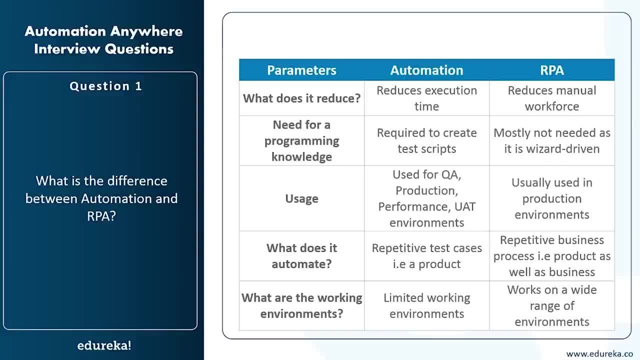 Well, automation reduces the execution time and robotic forces automation, or RPA, reduces the manual workforce. Coming to the need for programming knowledge: for automation, you do need programming knowledge to create test scripts, but coming to RPA, you do not actually need programming knowledge, as it's mostly. 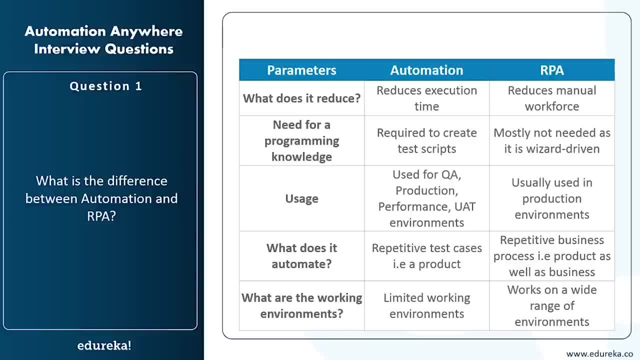 wizard-driven. So basically, you'll have a tool and then you'll have various functionalities and tools to you know, automate different tasks, So you do not actually need programming knowledge. coming to usage parameters, on comparing automation and RPA, on usage parameters, Let me tell you: 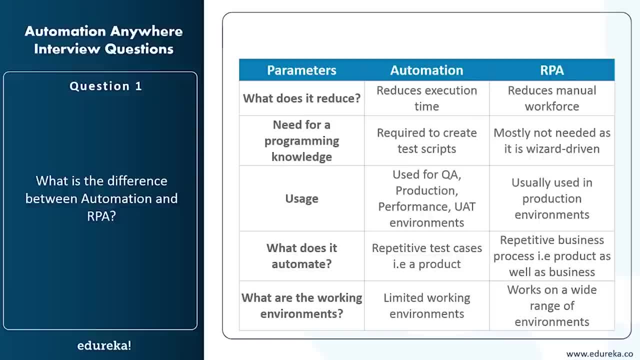 that automation is used for quality analysis, production performance, user acceptance, test environments and so on. and coming to RPA, RPA is mainly used in the production environments. coming to the next parameter, that is, what does it automate? So automation basically automates the repetitive test cases. 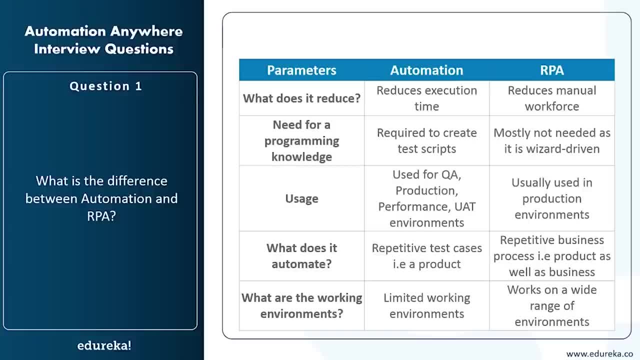 that is a product and RPA automates repetitive test cases. that is a product. automates repetitive business processes. that is, products as well as business. Now coming to the final parameter, that is, what are the working environments for automation and RPA? So, for automation, 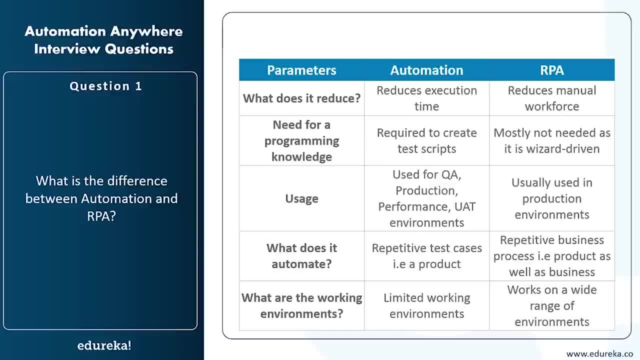 there are limited working environments and for RPA there are a wide range of environments. So, on comparing automation and RPA, automation basically reduces execution time. programming knowledge is required to create test scripts. It's mainly used for quality analysis, production performance, user acceptance, test environments. 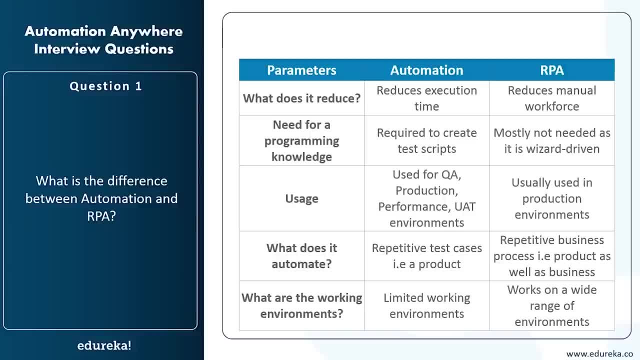 and automates repetitive test cases. that is basically a product and is also mainly used in limited working environments. coming to RPA, RPA reduces manual workforce. the programming knowledge is not much needed as it's, you know, wizard driven. it's mostly used in production environments. it automates 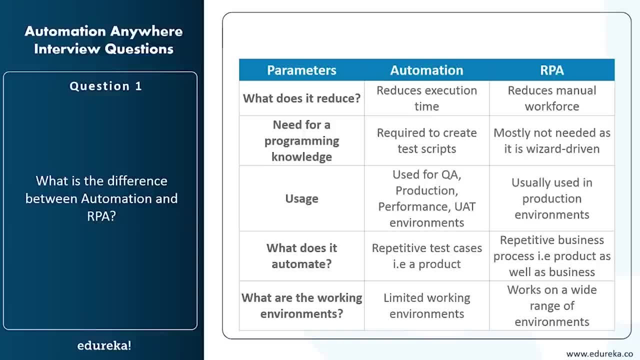 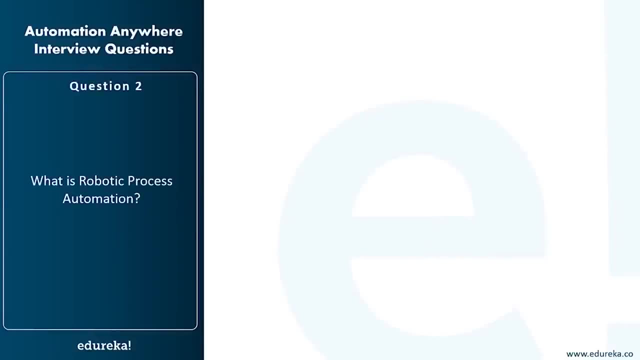 repetitive business processes. that is basically the products as well as business, and works on wide range of environments. So, guys, these were the differences between automation and RPA. now, moving on to the next question, that is, what is robotic process automation? So, if you have to understand, 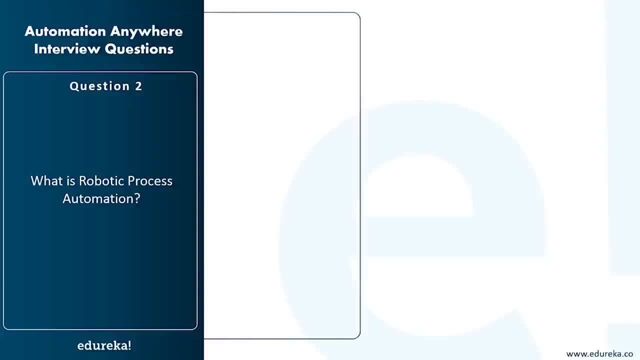 what is robotic process automation then? it's really simple. robotic process automation is basically the process of automating tasks with the help of software's or tools to deploy boats which reduce the involvement of humans to perform any task. So over here, if you look at the term, 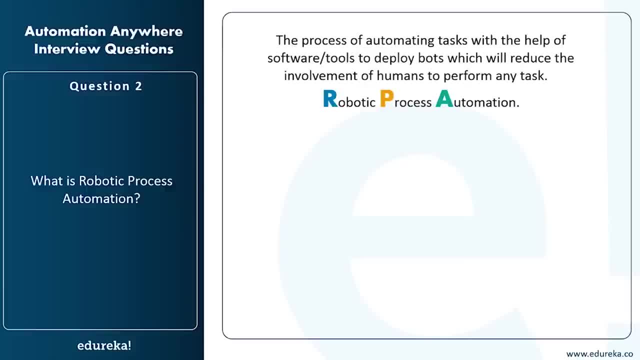 robotic process, automation, then there are mainly three terms that you need to understand, that is, robotic, process and automation. So let me just explain you each one of them one by one. So, starting with robotic: robotic are basically any entities which mimic human actions, So any entities. 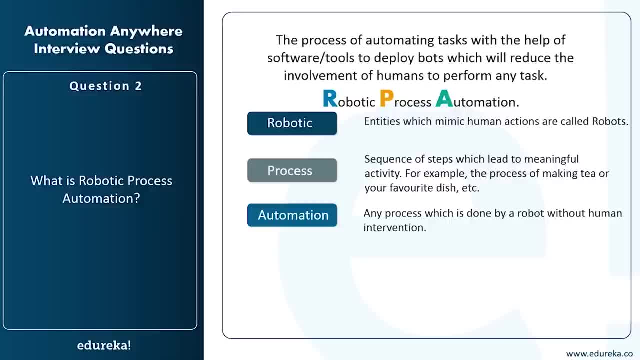 which mimic human actions- basically are known as robots- and with the help of these boards, you can automate any task coming to process. process is basically a sequence of steps which lead to a meaningful activity. So, for example, if you want to make copied, then you follow. 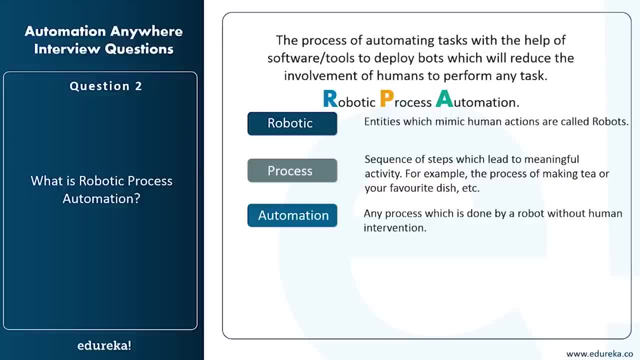 proper process, right? So that is what basically processes. So basically, robots follow this process to automate a task and finally coming to automation, as the term suggests, automation is basically any process which is done by a robot without any human intervention. Now, if you summarize, 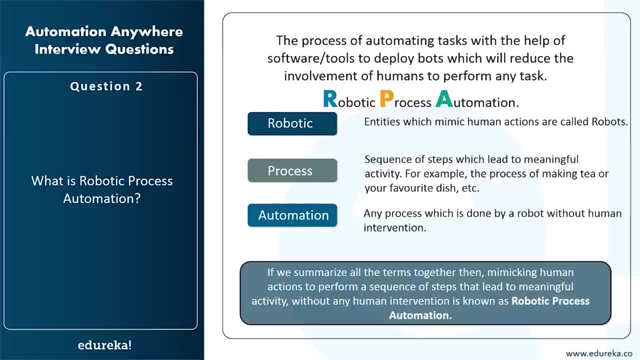 all these three terms together. then, mimicking human actions to perform a sequence of steps that lead to a meaningful activity without any human intervention is said to be robotic process automation. Now, moving on to the next question, that is, what is the difference between UiPath? 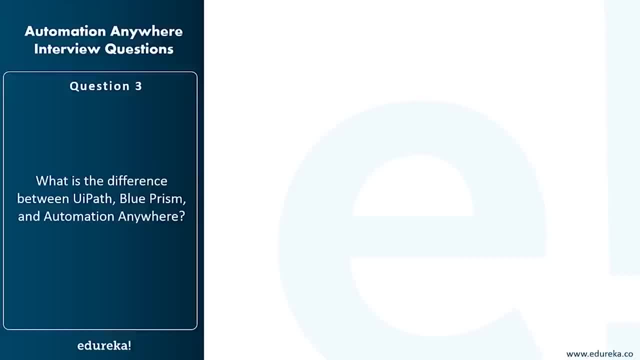 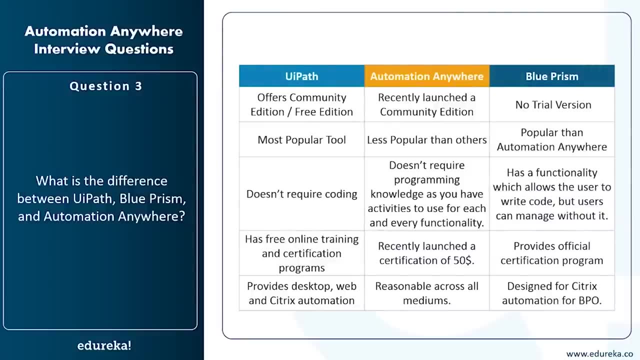 blue prism and automation anywhere. So basically, these three tools are the most popular tools in the RPA industry. Now, if we have two tools based on various parameters, then let me start with UiPath first. UiPath basically offers a community edition or a free edition. 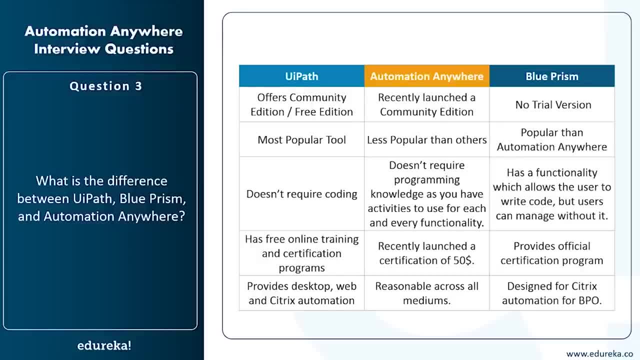 which you can use for lifetime, So you can keep using that addition until you know you get a good experience in the tool. coming to automation anywhere, automation anywhere has recently launched a community edition. Now, apart from the community edition, it also has an enterprise edition. 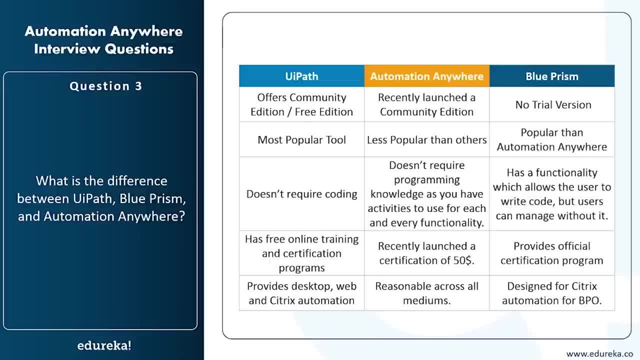 with a 30-day trial right, So you can go for the community edition, which is again free for the lifetime, and then there's also Enterprise Edition, UiPath and finally, coming to blue prism, blue prism has no free edition. Basically, it offers no trial version. 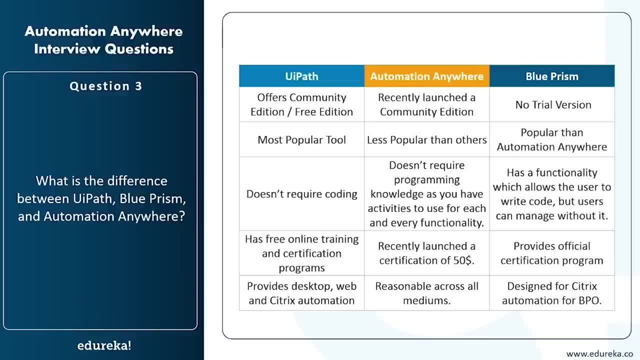 So you'll have to pay money, get the license version and then you can start automating tasks in blue prism. coming to the Google Trends popularity, basically, which tool is popular more? So I'll say that you know, UiPath is the most popular tool. So on the popularity. 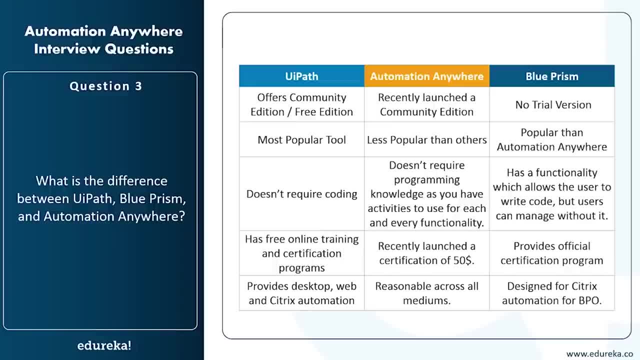 basis. it's clear that you know UiPath wins the competition, but it's never a do. as you know, automation anywhere has also recently launched a community edition, So you never know the return, and automation anywhere can also become one of the most popular tools coming. 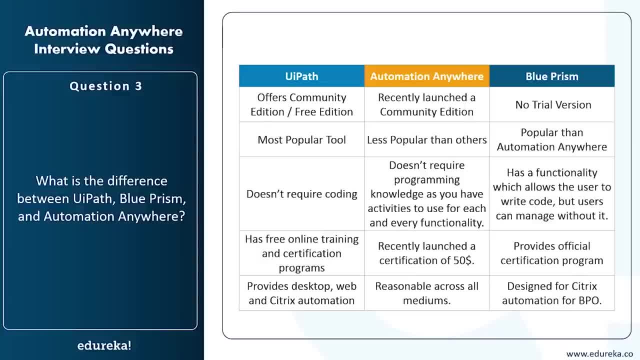 to the programming knowledge. UiPath doesn't require much coding. as you know, it's always an activity. So, for example, if you want to use a for loop, then you have a for activity. You just have to drag and drop it in your sequence and then you. 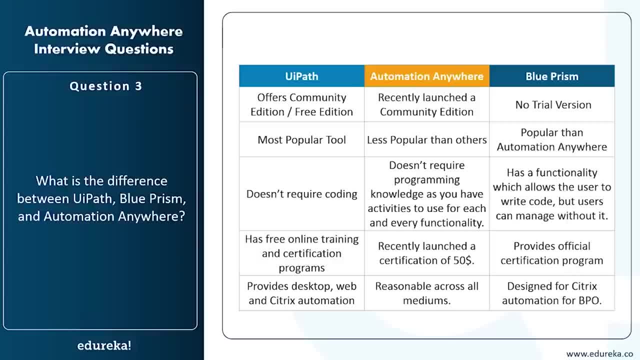 can start using it, coming to automation anywhere. automation anywhere also doesn't require programming knowledge, as you have activities to use for each and every functionality. So when I say activities over here, I basically mean commands that I'll show you later in the session how you can just. 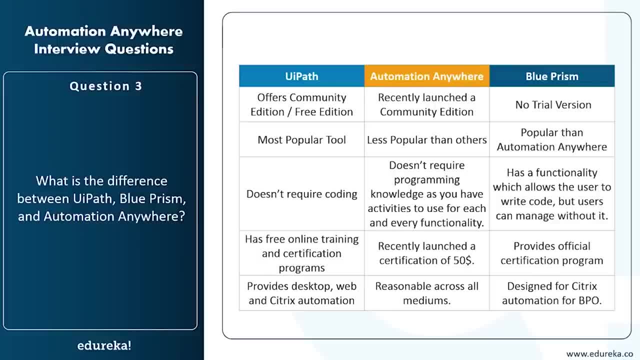 drag and drop the commands into your sequence and automate us. and finally, coming to blue prism, blue prism basically has a functionality which allows the user to write code, But, yes, users can also manage without it. So, coming to programming knowledge, all the three tools, almost not. 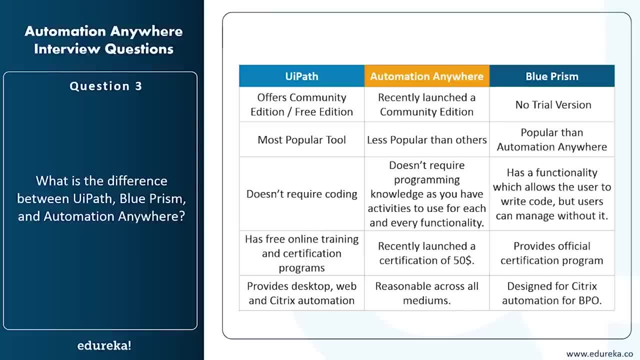 require programming knowledge, as each and every tool has its own functionality to cater the needs. coming to the training programs, UiPath has free online training and certification programs and automation anywhere. has also recently launched a certification for $50 and it's free. online training and certification programs and blue. 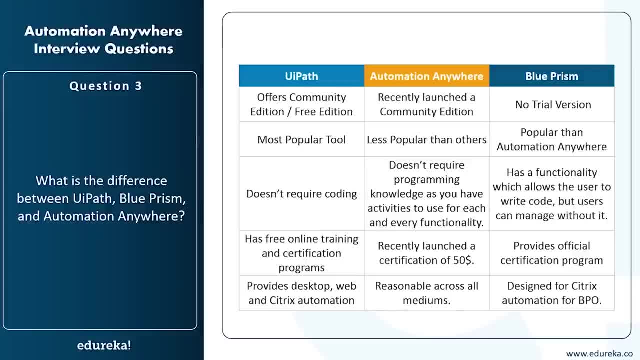 prism also offers his official certification program. So all the three tools make sure that you know the users can learn, get certified in it and upscale their careers. and finally, coming to the usage of these tools, UiPath is basically used to provide desktop web and Citrix automation. 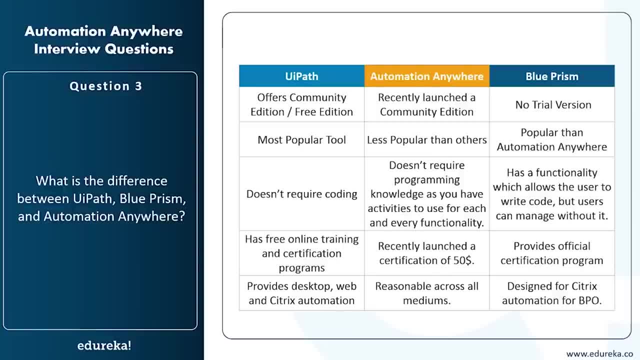 automation anywhere is reasonable across all the mediums and blue prism is mainly designed for Citrix automation for business process outsourcing. So, guys, these were the differences between UiPath, blue prism and automation anywhere. Now moving on to the next tool, which is blue prism. Moving on to the next, 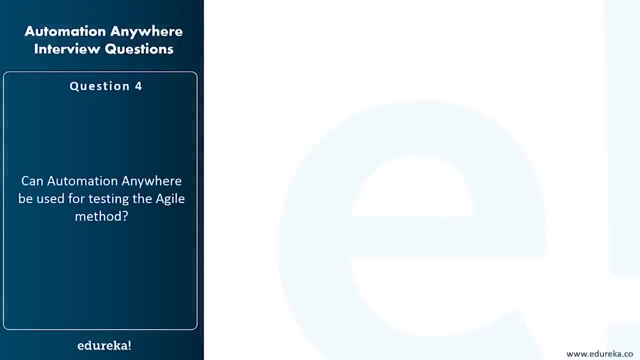 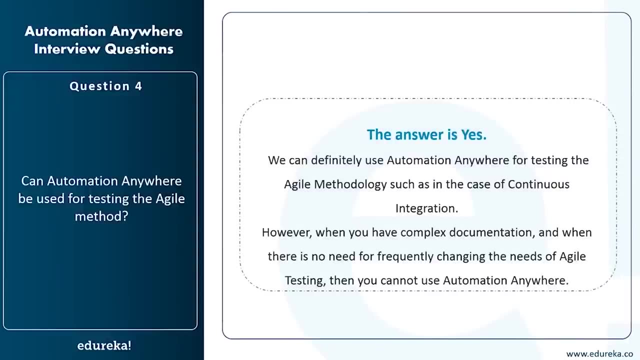 question that is: can automation anywhere be used for testing the agile method? Well, the answer is yes, We can definitely use automation anywhere for testing the agile methodology, such as in the case of continuous integration. So, if you don't have an idea of continuous 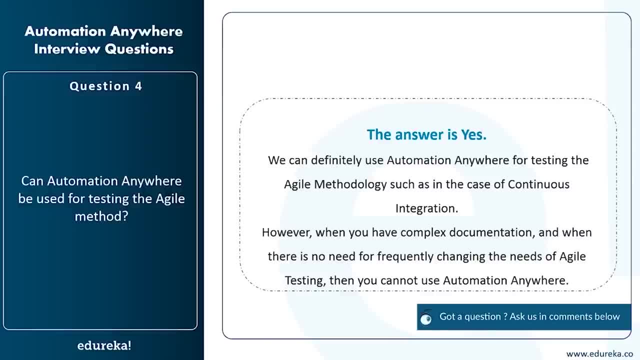 integration. I'll leave the link of the video in the description box and then you can understand what continuous integration is. However, you cannot use automation anywhere when you have a complex documentation and when there's no need for frequently changing the needs of agile testing right. 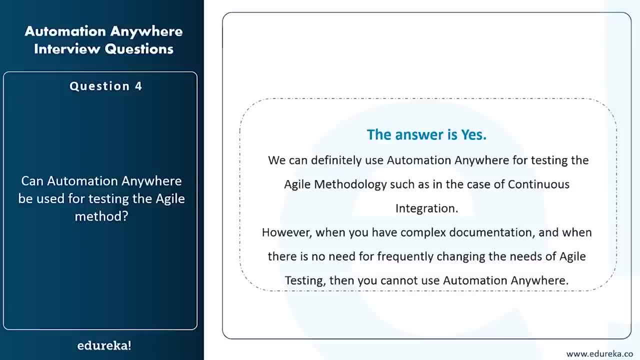 So you can use automation anywhere. definitely for testing the agile methodology, but in the case of continuous integration- but yes, if you come to the case when you have complex documentations and then there is no need of frequent changing- It's not advisable that. 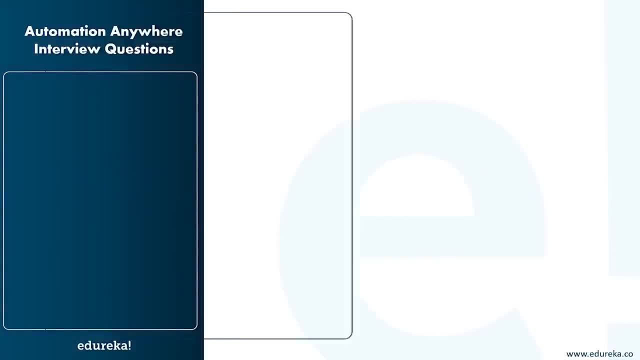 you know you use automation anywhere over there. Now, moving on to the next question, that is, is robotic process automation like screen scraping or macros? Now, this is one of the most popular confusions that people all the time have. that, you know, is robotic process automation only. 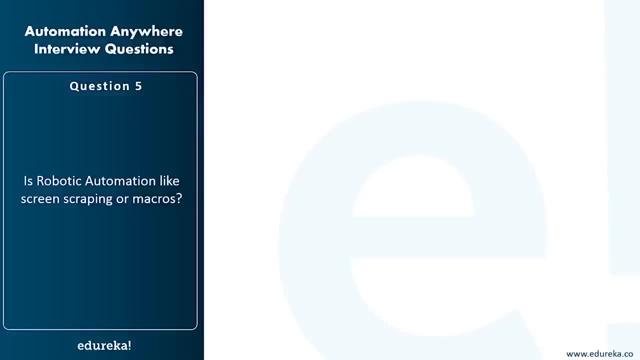 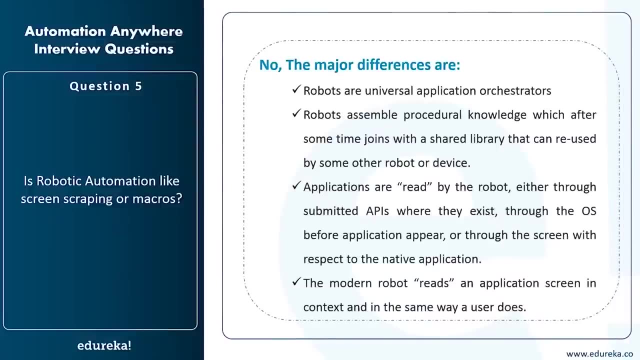 respective to screen scraping or, you know, doing simple tasks. Well, let me clear your confusion and tell you that you know the answer is no. So robotic process automation is basically a generation from all technologies like screen scraping or macros. So the major differences between the robotic 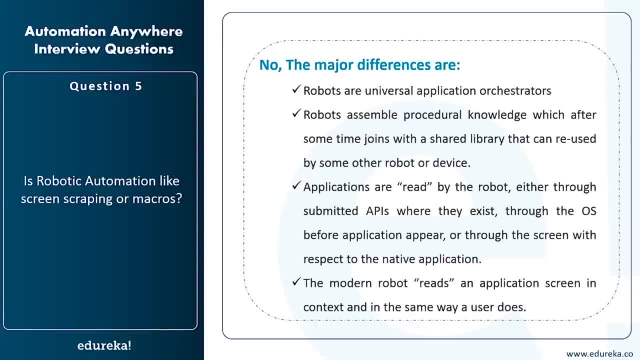 automation and the screen scraping or macros, is basically that the robots are universal application orchestrators and any application that can be used by a man can be used by present-day robot, whether you know it's a mainframe application or a desktop application or a legacy application. 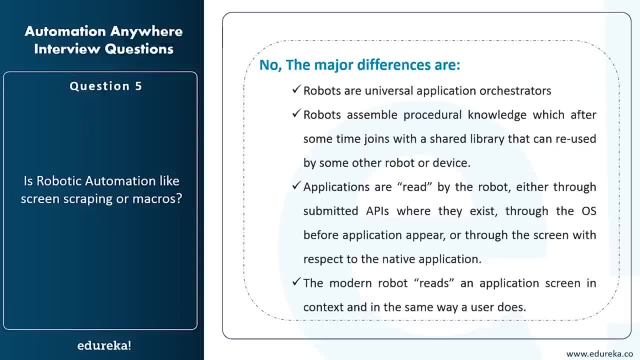 or even web service enabled, or even if it is a closed-source application. This is a third-party API hosted service. robots basically assemble procedural knowledge which after some time joins with a shared library that can be reused by some other robots or devices, So applications are read. 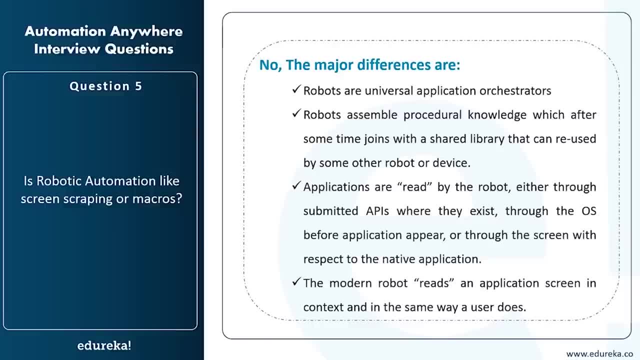 by the robots, either through submitted APIs, where they exist, through the operating systems before the application appears, or through the screen with respect to the native application. in this last case, the modern robot reads an application screen in context, as the same with the user does, right? So as part of the 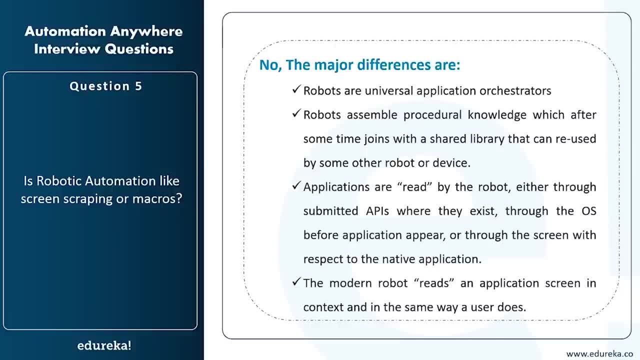 robot training. it is shown how to read the application screen in context, as the same way the robot reads an application display, much like a user is shown. So basically, robotic automation is not like screen scraping or macros, as robots are intelligent enough and they can see the 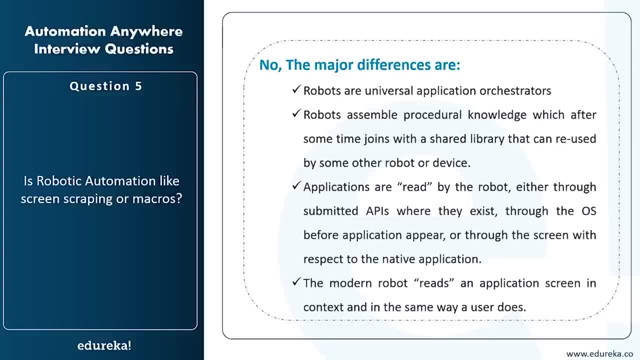 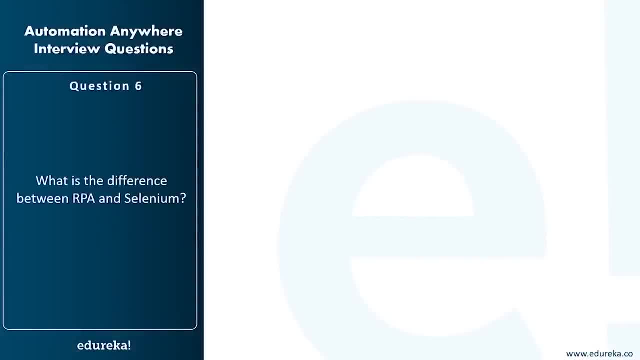 data as a user can see, and obviously they can be reused for any other applications or services. now moving on to the next question, that is, what is the difference between RPA and selenium? that this is also one of the most popular confusions that mostly arises between RPA and. 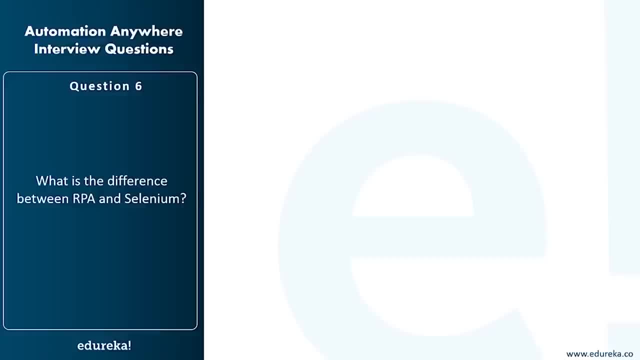 selenium, as both of them automate tasks. Well, let me just clear the confusion, for the first thing is clear the confusion for you guys. So we'll compare RPA and selenium based on various parameters. So, starting with automation, RPA basically automates business. 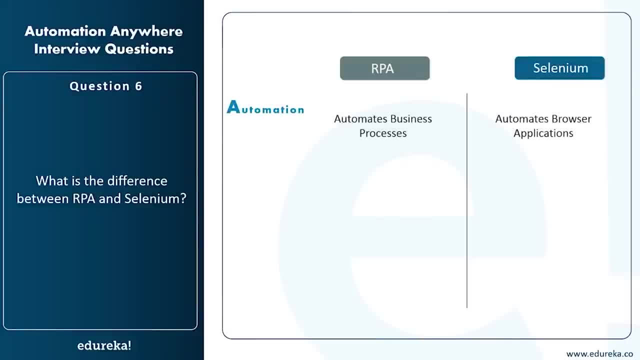 processes, whereas selenium automates browser applications. So you can't automate everything with selenium. Basically, you can't automate different kinds of applications. like you know, if it's not a browser application, then you cannot automate with the help of selenium. But yes, you can. 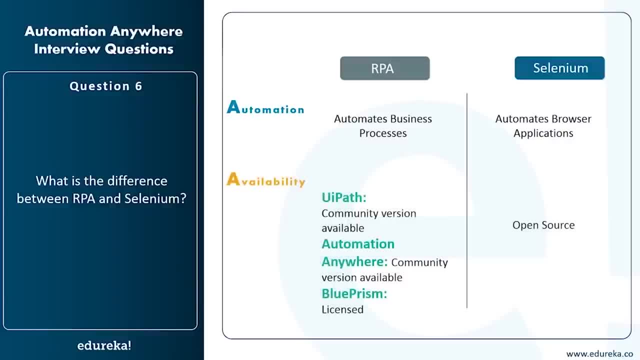 automate with the help of RPA. moving on to the next parameter, that is, availability, RPA has various tools- and it's also available industry- with the help of which you can automate tasks. So the most popular tools, as I said before, are UiPath, Blue Prism. 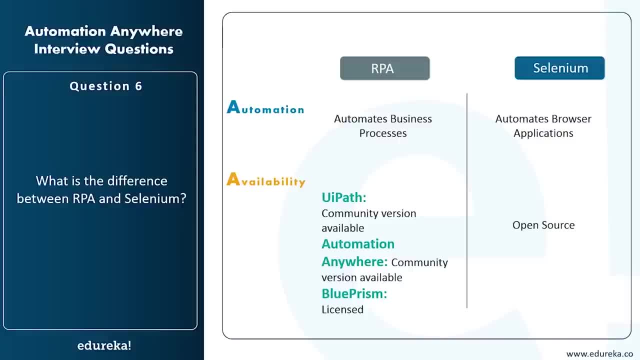 and automation anywhere, and UiPath and automation anywhere have free trial versions, whereas Blue Prism has licensed versions. coming to selenium, then selenium is open source. moving on to the next parameter, that is, where is the task performed? well, in RPA, the task is performed at the back end of the 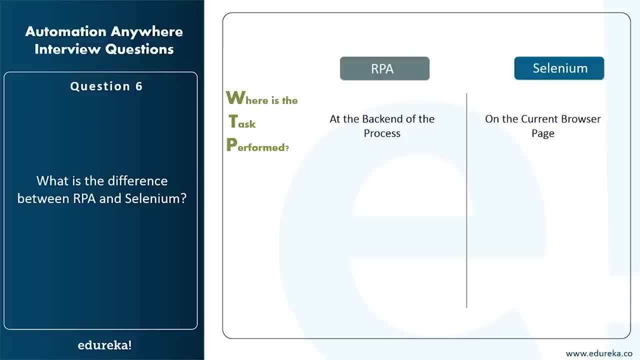 process and in selenium, it is performed on the on current browser page. coming to the next parameter, that is, the major components used: RPA mainly uses the RPA boards and, in the case of selenium, the selenium web drivers are used. coming to the next parameter, that is, the level. 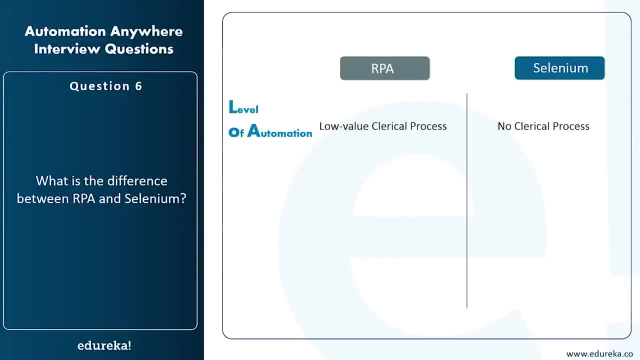 of automation: RPA basically automates the low-value clerical processes and selenium automates no clerical processes. coming to life cycle, then the life cycle of RPA is simple and easy and selenium is relatively difficult when compared to RPA. coming to platform dependency, then RPA is. 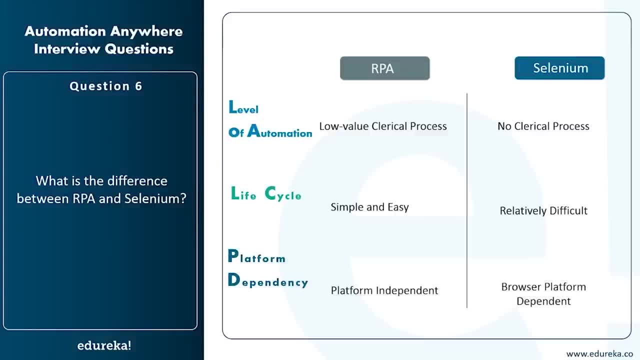 platform independent and selenium is basically a platform dependent and selenium is basically a browser platform dependent. next, coming to programming knowledge. so for RPA you do not actually need programming knowledge, but for selenium you do need programming knowledge. and finally, coming to the skills required, then the skills required in: 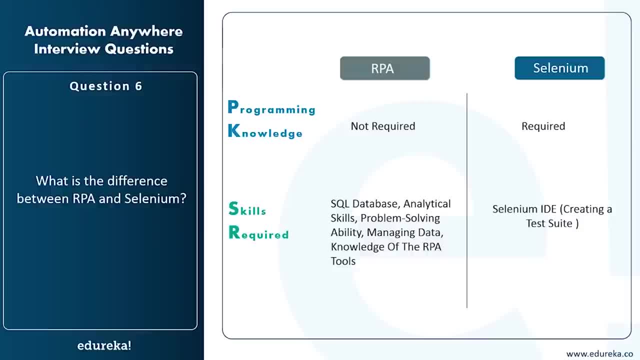 RPA are sequel databases, analytical skills, problem solving ability, managing data and the knowledge of RPA tools. and coming to selenium, then the knowledge of selenium ID is required to create a test suit. now, moving on to the next question, that is, what do you know about automation anywhere? 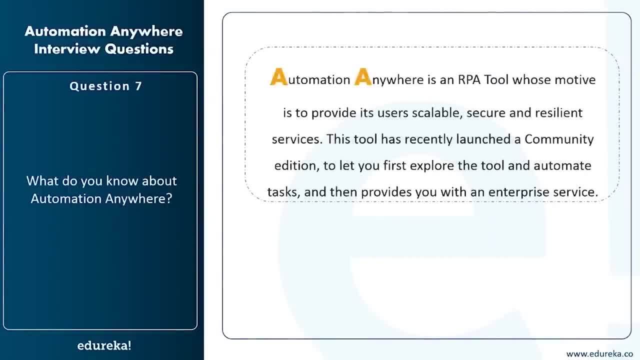 so, basically, as I said before, automation anywhere is an RPA tool whose motive is to provide its users with scalable, secure and resilient services. this tool has recently launched a community edition to let you first explore the tool and automate tasks, and then it also provides with an enterprise. 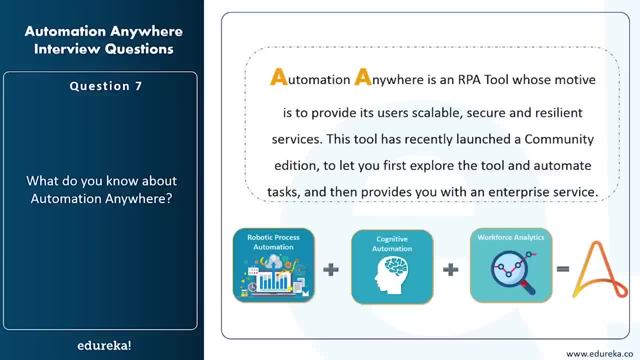 version with which you can automate tasks at an enterprise level. so automation anywhere also offers better performance, as it has the ability to integrate with different platforms and also scale simultaneously. so this tool is meant to be used for an enterprise level, I would say- and it's mainly designed. 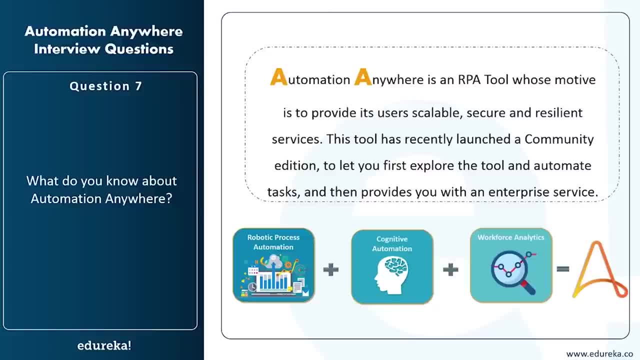 for solving complex issues. so if you have to summarize automation anywhere, then you can just say it's a summation of robotic process automation plus cognitive automation plus workforce analytics, which is nothing but automation anywhere. so you can just summarize automation anywhere in this way. now let's move. 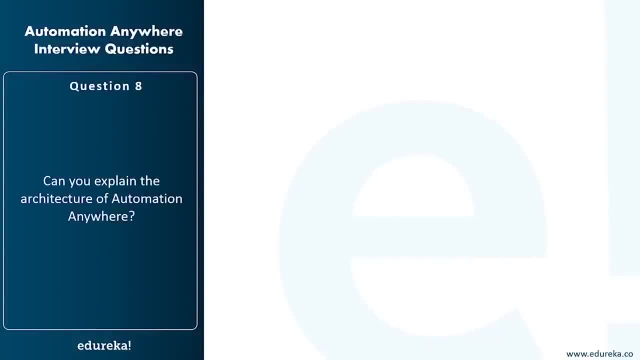 forward with the next question, that is, can you explain about the architecture of automation anywhere? coming to the architecture of automation anywhere, automation anywhere, for automation anywhere, follows a distributed architecture. so through this architecture, automation anywhere makes sure that you know it has centralized management, which is accomplished through: 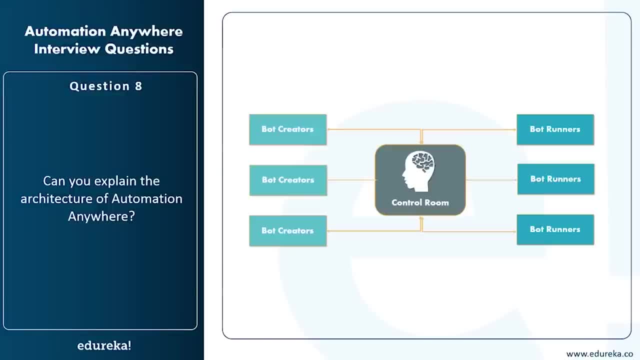 the automation anywhere control room. so the architecture of tool is mainly segregated into three components, that is, the bot creators, the bot runners and the control room. so, as you can see on my screen, the bot creators and the bot runners are basically connected to the control room, and control room is 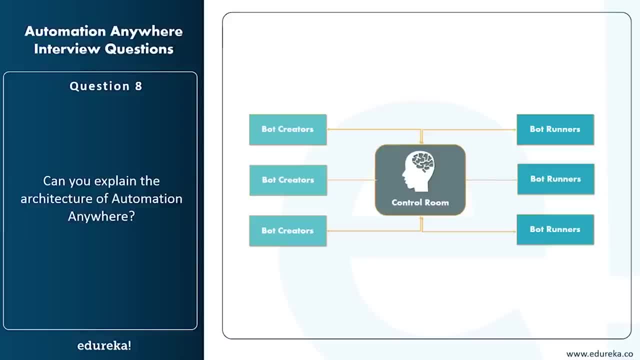 the brain of automation anywhere. so let's just discuss each of these components one by one, starting with bot creators. so bot creators, as the name suggests, are used to create bots. these are basically desktop based applications which authenticate against an active control room and only have an access. 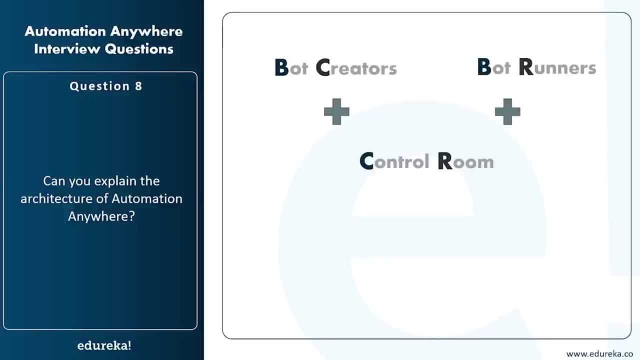 to upload or download the boards on configuring these boards for the control room. multiple developers can also create individual tasks of both and can execute all of them at once. coming to control room: control room is the most important component of this architecture. it's a web server that basically controls. 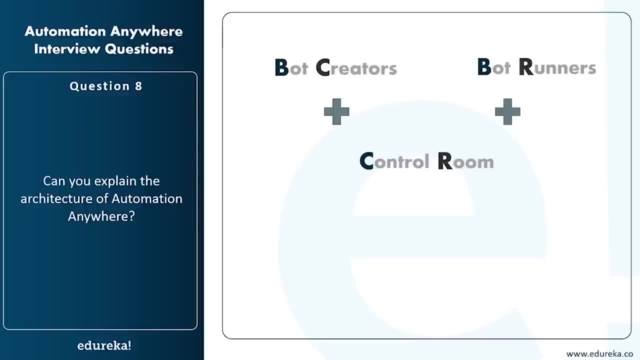 the boards created by the bot creators and, as automation anyway, focuses on the centralized management with the help of control room. the control room offers features such as centralized user management, automation, deployment, source control and also provides a dashboard. coming to bot runners: the bot runners are used to execute the 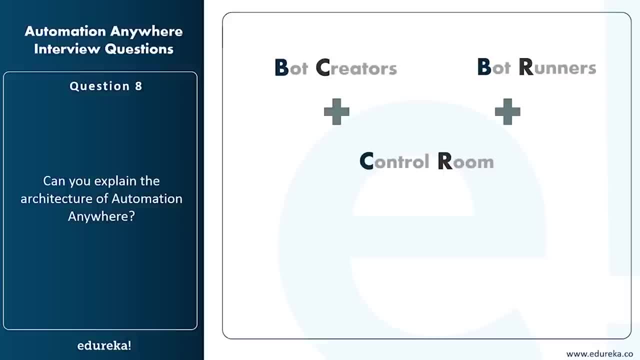 bots. so multiple bots can be executed in parallel and cannot update or create an automation. so they basically runtime clients which are installed on the Windows machines and can report back the execution log status to the control room. so if you somehow remember the control room, so if you summarize all these, 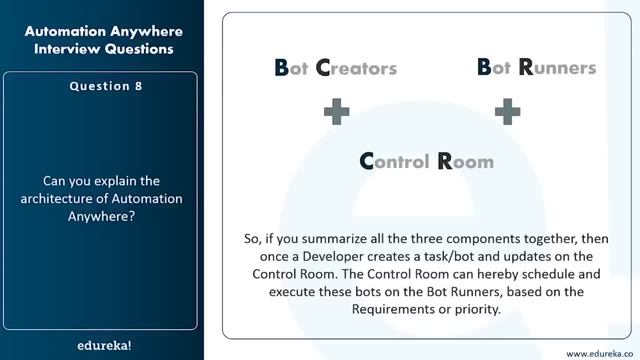 three components together. then, once a developer creates a task or a board and updates on the control room, the control room can hereby schedule and execute these boats on the bot runners based on the requirements of priority. so, guys, that was about the architecture of automation anywhere. now let's move forward. 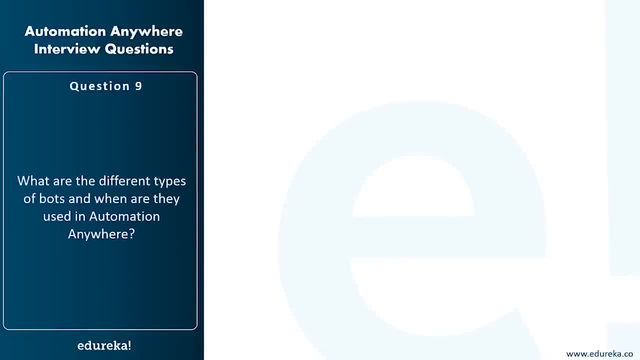 with our next question, that is, what are the different types of boards and when are they used in automation anywhere? so there are mainly three different types of boards in automation anywhere. that is, the IQ boards, the task boards and the meta boards. so, talking about the IQ boards, first the IQ. 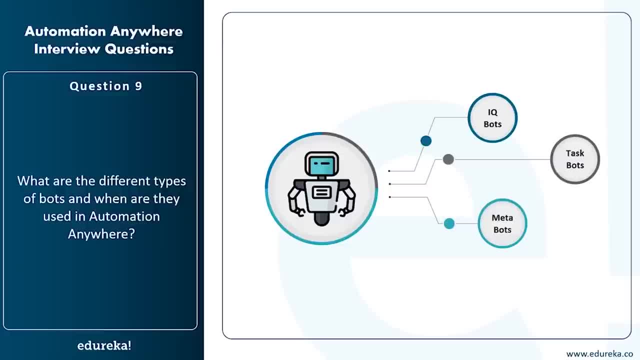 boards allow the developers to add cognitive capabilities to the process. so it uses cognitive capabilities to extract information from semi and unstructured data and also detects patterns, so that the next time the pattern is encountered, the bot already knows what exactly has to be done. coming to taskbots: the task. 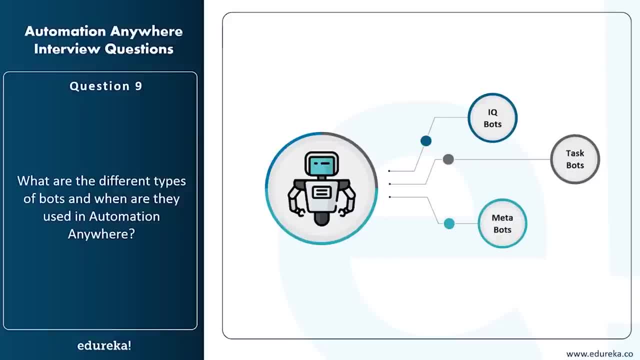 bots are the core of automation, so these bots execute repetitive, rule-based tasks that rely on structured data and are easy to build. they can be used for a variety of tasks and they can be used for different tasks. and they can be used for a variety of tasks and they can. 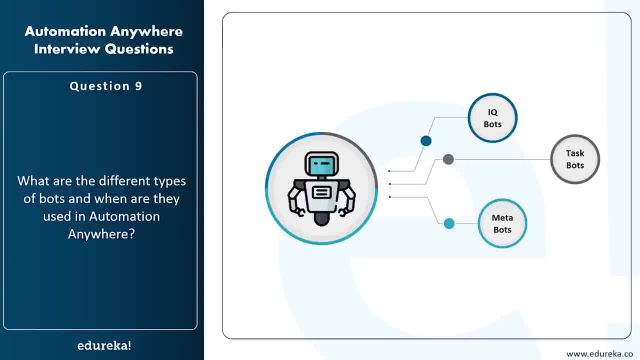 execute multi-step processes around the clock with no errors. coming to the final part, that is, the meta bots, the meta boards have the capability of integrating dynamic link library. that is the DLL that can be used for back-end automation. it includes UI components which are used for the 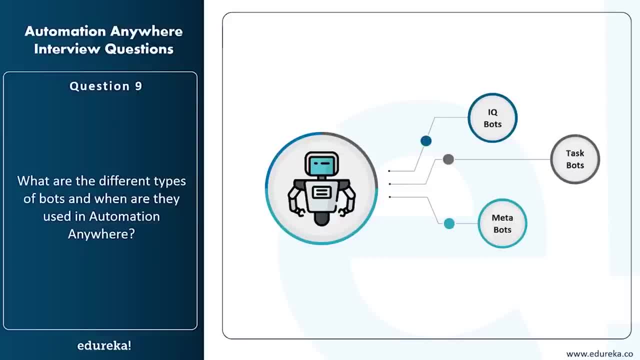 front-end automation and maximizes multi-level integration to automate business processes, along with the task boards. so this was about the different bots in automation anywhere. there are mainly three types of bots in automation anywhere. that is, the IQ boards, task boards and meta boards. so the IQ 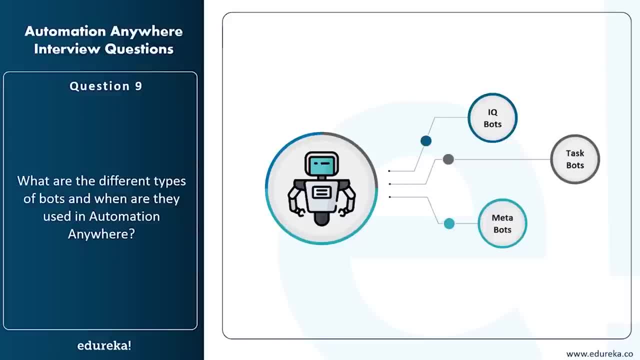 boards allow the developers to add cognitive capabilities. task boards are basically the core of automation. and coming to the meta boards, the meta boards have the capability of integrating dynamic link library that can be used for the back-end automation. now coming to the next question, that is, what are the 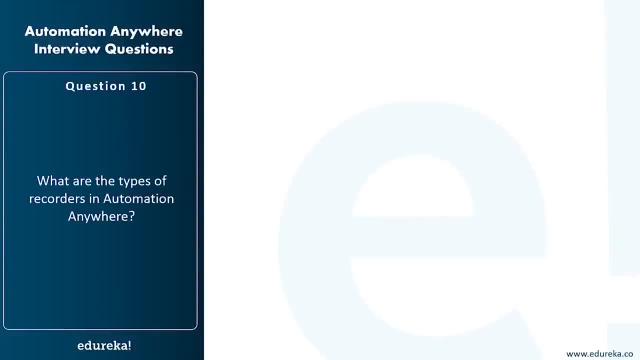 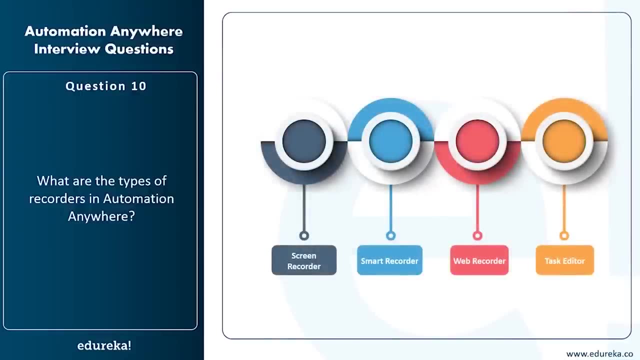 different types of recorders in automation anywhere. so there are mainly four recorders in automation anywhere. that is, the screen recorder, the smart recorder, the web recorder and the task editor. coming to the screen recorder first, the screen recorder first. is the task editor, the screen recorder or the other? 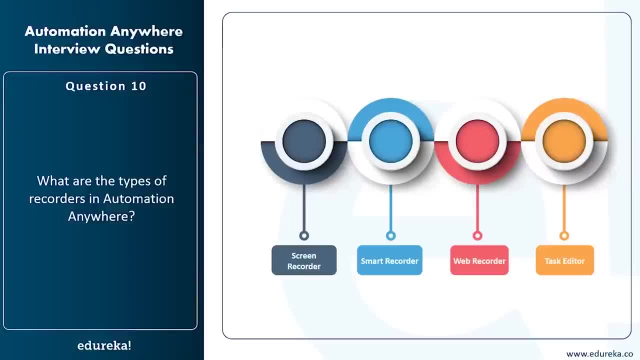 standard recorder provides the easiest way to create a simple automation process. it is usually used when the task involves many mouse click and keyboard operations. coming to the smart recorder: the smart recorder, or the object recorder, is the most feasible method for building tasks. it is ideal for desktop. 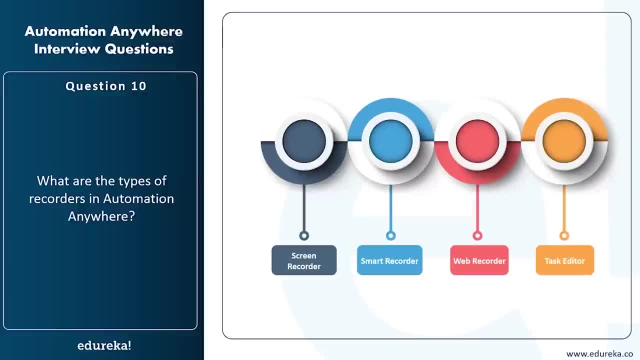 applications and captures objects such as drop-down menus, list boxes, radio buttons, check boxes and mouse clicks. coming to the web recorder, the web recorder is used to perform tasks that require a certain amount of time, so the task editor is usually the one that performs tasks that require repetitive actions. 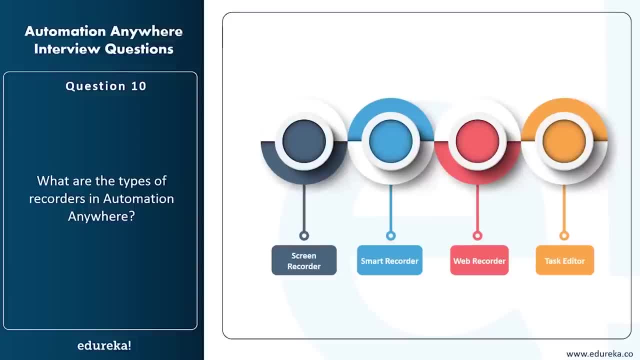 such as extracting data from multiple web pages, extracting data from tables on the web pages and also filling the web forms. coming to the task editor, the task editor is used to process any command with the help of several commands. this editor allows you to open multiple tasks by 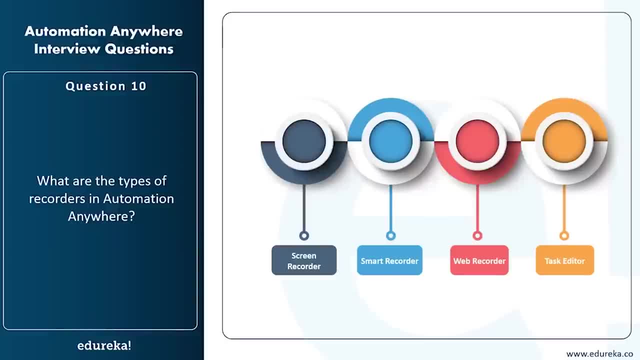 editing them simultaneously, and the task editor has components such as commands panel, task action list, the action buttons, error view and variable manager panel. so, guys, these were the various recorders in automation. anywhere the task editor has components such as commands panel, task action list, the action- that is a screen. 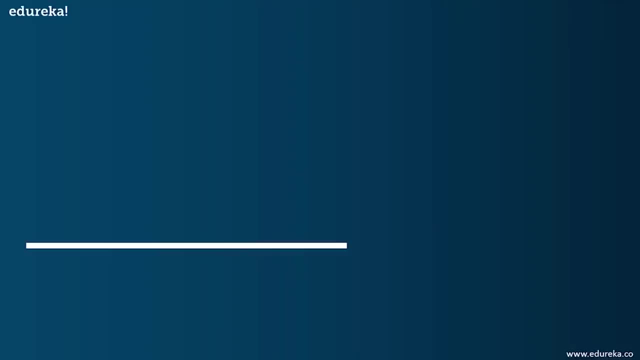 recorder, the smart recorder, the web recorder and the task editor. now moving on to the next set of questions, that is, the tool based questions. now, this section of the session will basically consist of those questions that are mainly related to the tools. so basically, you can understand, you know. 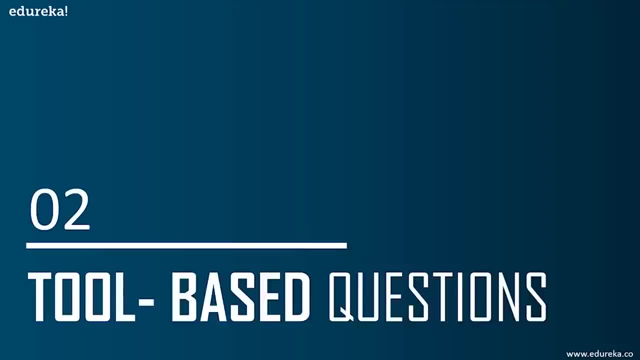 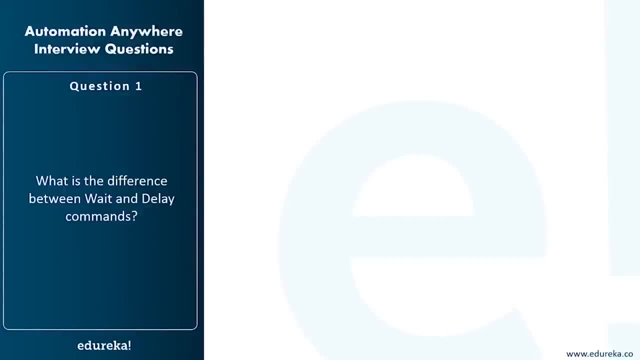 these questions will be related to the working of the tool, so let's just get started with this section of questions. so, starting with the first question in this section, that is, what is the difference between the weight and the delay commands? so the major difference between the weight and the delay. 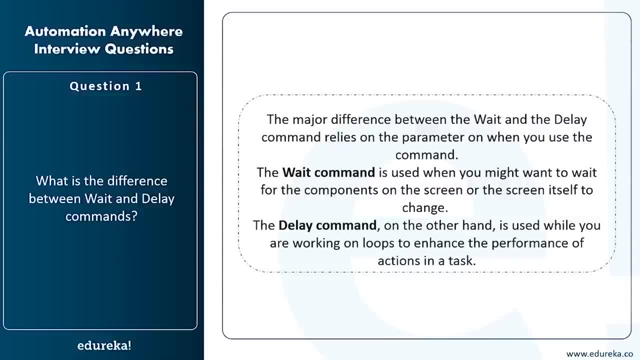 command relies on the performance of the screen and the screen itself, and the weight command relies on the parameter on when you want to use the command. so, basically, the weight command is used when you might want to wait for the components of the screen or the screen itself to change and 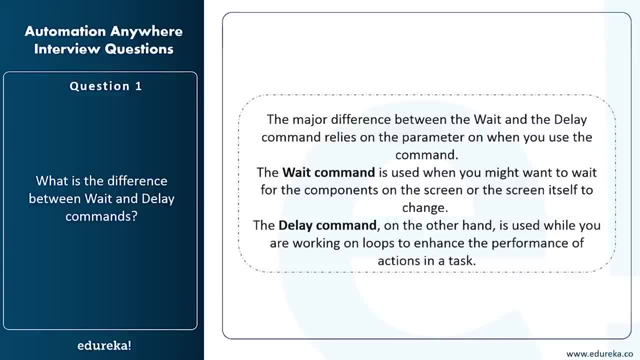 coming to the delay command. delay command, on the other hand, is basically used when you're working on loops to enhance the performance of actions in a task. so this is basically the difference between the weight command and the delay command. the difference mainly relies on when you want to use. 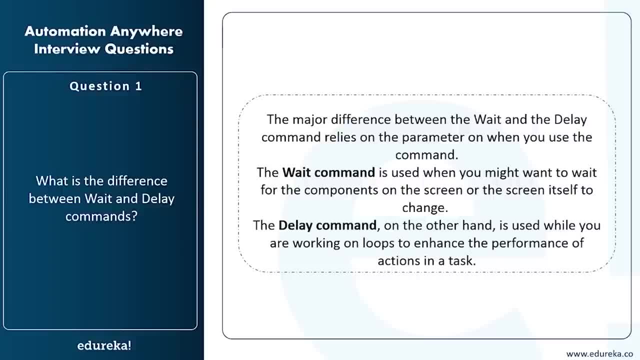 the command. the weight command, as I said before, is used when you want to wait for the components to change in the screen or the screen itself to change, and the delay command is used when you're working on loops. So, guys, this is the main difference between these. 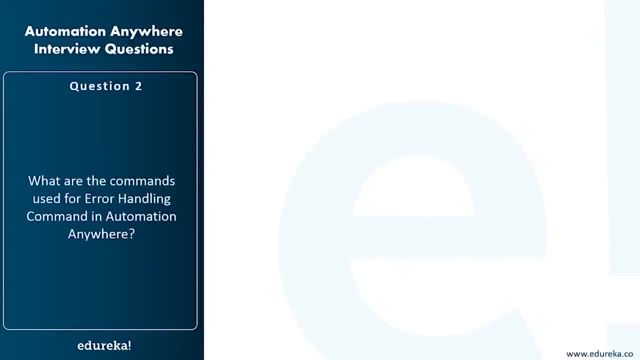 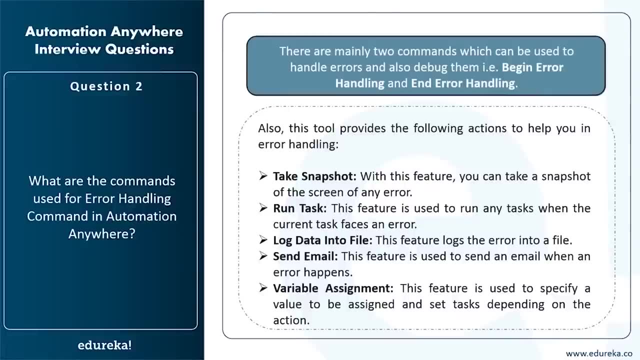 two commands. now moving on to the next question, that is, what are the commands used for error handling in automation anywhere? So there are mainly two commands which can be used to handle errors and also debug them, that is, begin error handling and end error handling. So these are. 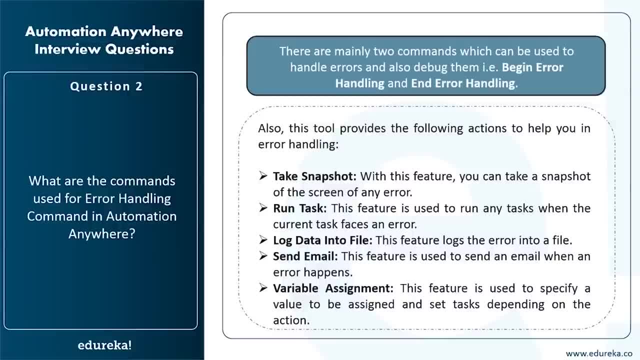 mainly two commands that are used in error handling. well, apart from these two options, that is, the begin error handling and the end error handling commands, There are also various other actions that you can follow to perform with the help of these two commands, that is, take snapshot run tasks. 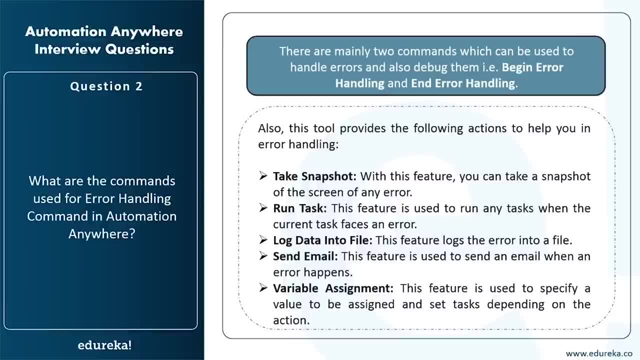 log data into file, send email and variable assignment. talking about taking snapshot, with this feature You can take a snapshot of the screen of any error coming to run task. This feature is used to run any task when the current task faces an error coming to log data. 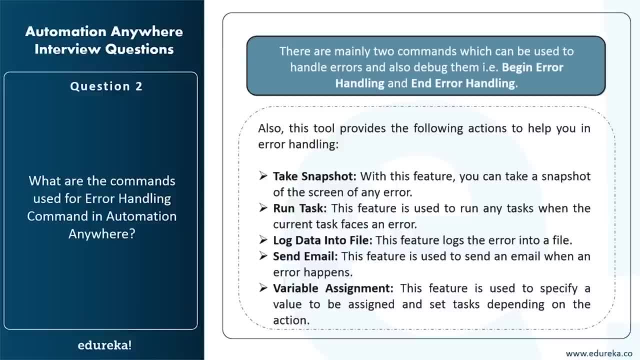 into file: This feature is basically used to log the errors into a file. coming to send an email: This feature is used to send an email when an error happens. and coming to variable assignment: This feature is used to send an email when an error happens. This feature is 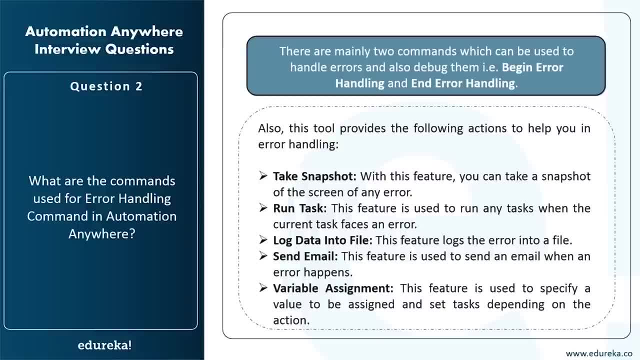 used to specify a value to be assigned and set tasks depending on the action. So, guys, these were the commands used for error handling and automation anywhere. that is the begin error handling and end error handling, with any number of features to let you perform different actions. moving on to the next, 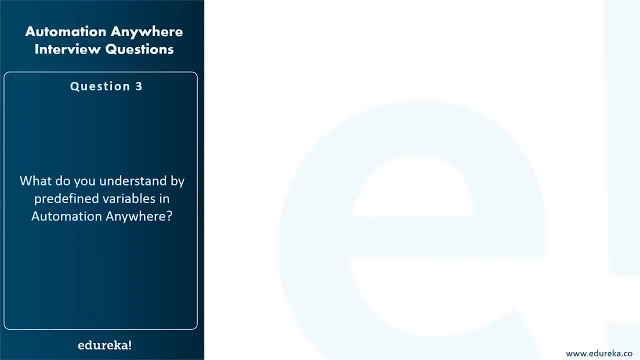 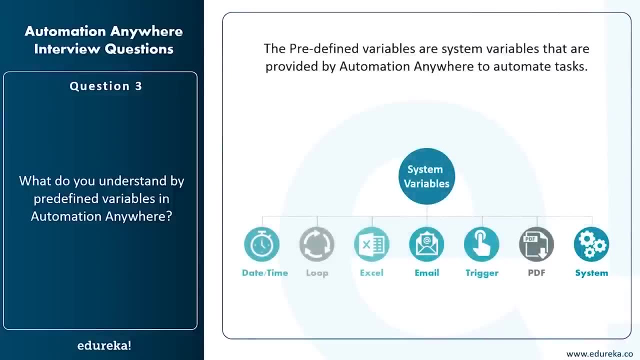 question That is: what do you understand by predefined variables and automation anywhere? So the predefined variables are basically the system variables that are provided by the automation anywhere to automate tasks? The different predefined variables are as you can see on my screen. that is the date. 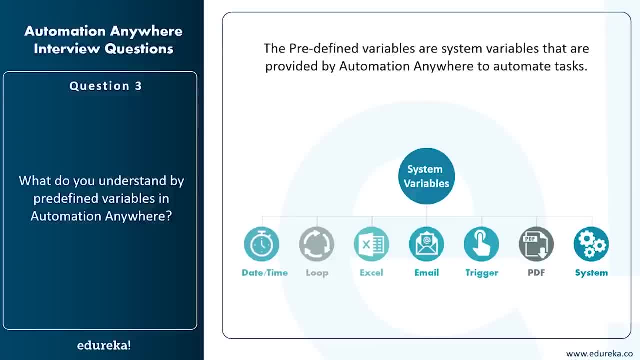 and time loop, Excel, email trigger, PDF and system. So, guys, these are the various system variables that are used in automation. anywhere now to check the predefined variables, What you can do is you just have to go to the variable manager on the right side of the task pane, click on. 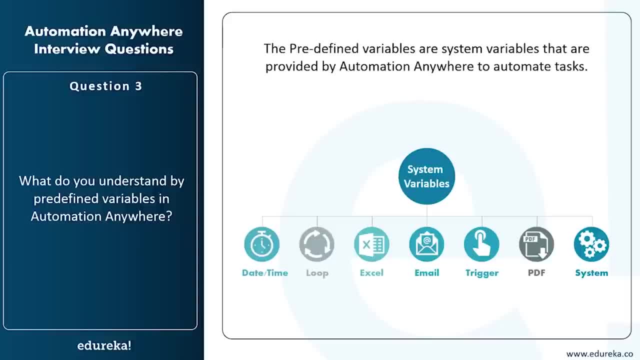 the show system variables and it will open all the system variables for you, for your better understanding. I'm going to show you how you can see the system variables and then I'm also going to show you how you can use those predefined variables. What I'm going 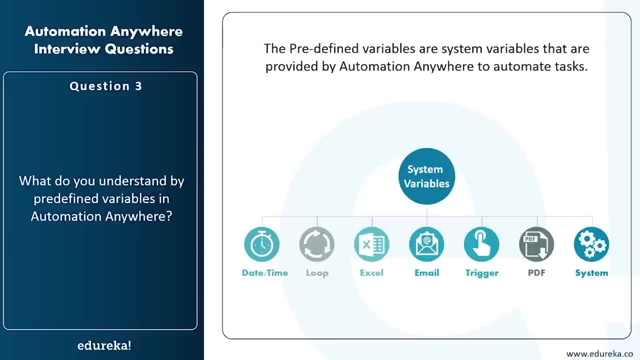 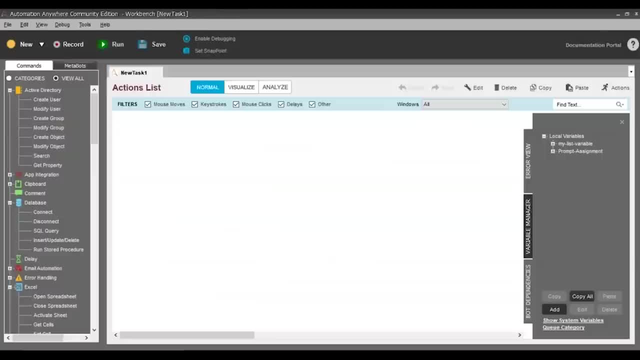 to do is, first of all, I'm going to shift to my automation anywhere client. So this is my automation anywhere client guys. Now what I'm going to do is I'm going to go to new choose workbench. Then this is how my workspace looks. 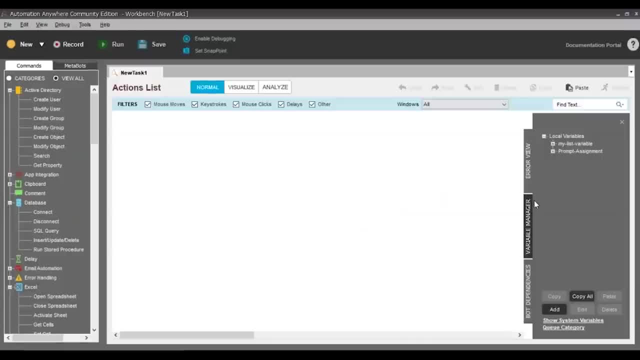 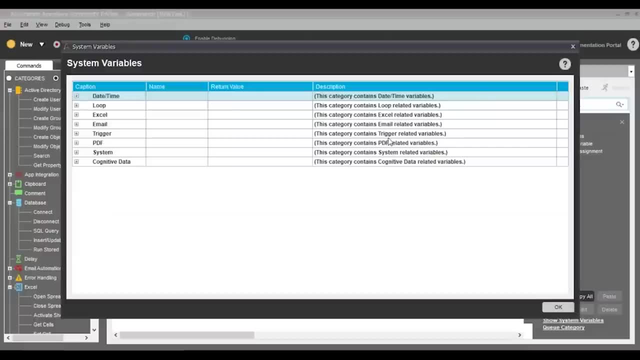 like So, to check the system variables, What you can do is you have to go to the variable manager, So this is the variable manager, and then you can go to show system variables. So as I clicked on show system variables, as you can see on my 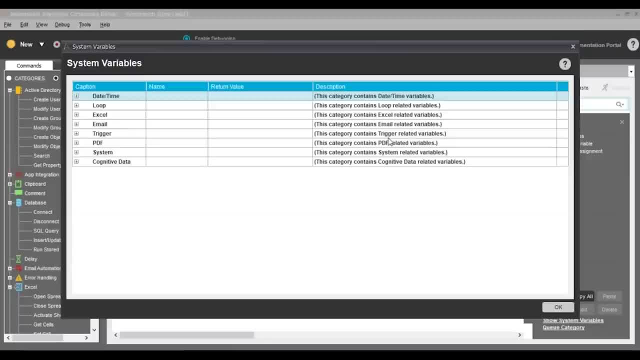 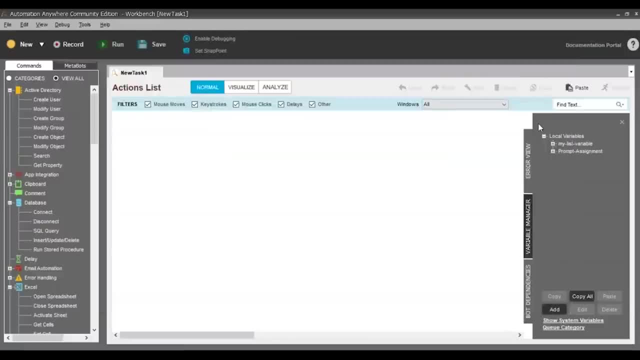 screen. These are the various system variables that are already predefined in your workspace. now to use the system variables, I'm going to automate a simple two-step task and show you how you can use these variables. So what I'm going to do is I'm going 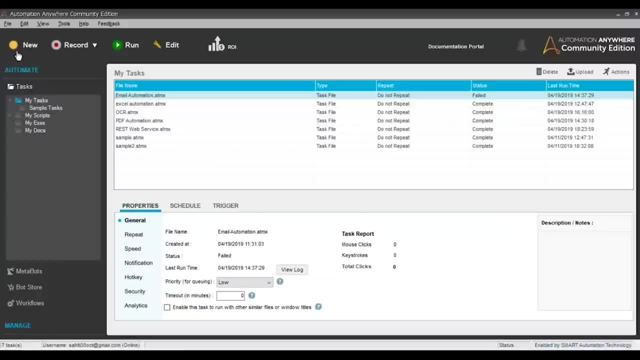 to use the predefined variable clipboard over here, right, All right. So what I'll do is I'll go to new and I'll choose web recorder. Now, what I'm going to do is I'm going to mention my URL, So I'm going to mention. 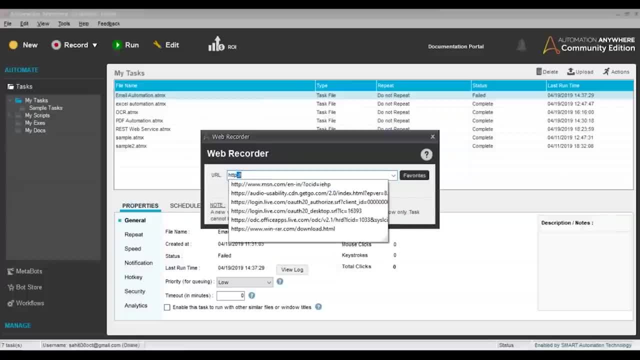 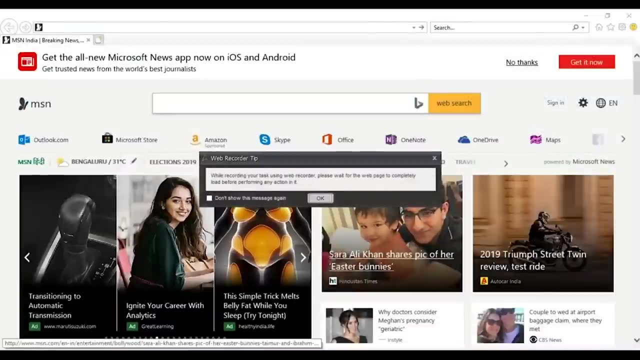 the URL for our blog page. So that's HTTPS colon slash slash. wwwedurekaco slash blog. I'm going to do this and then I'm going to click on start. So basically, this is what I'm going to do. So, basically, when you 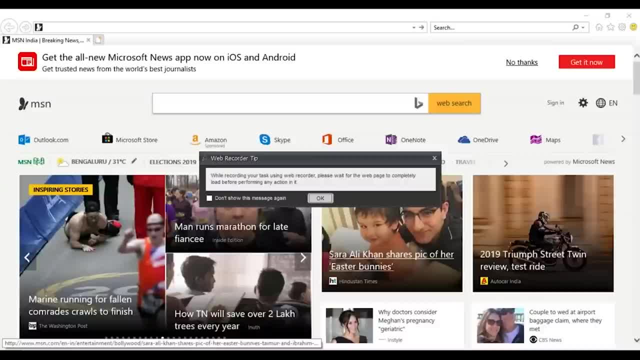 click on start, you'll see that you know the web recorder has started. So while recording your task you have to make sure that you know you wait for the page to load completely. So I'm going to click on OK over here. 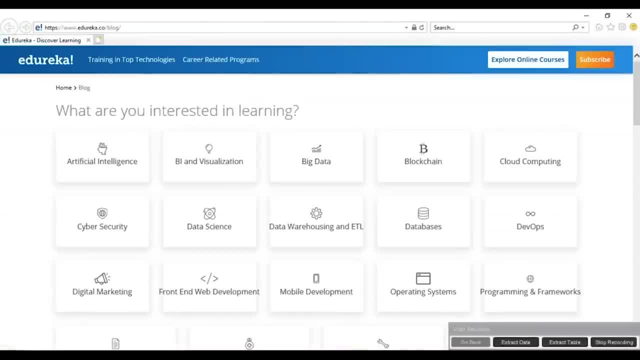 and then you will see that you know our edureka domain has opened. Now what you have to do is you have to choose this option of extract data from the bottom corner that you can see on my screen, and then I'll choose either regular data or pattern. 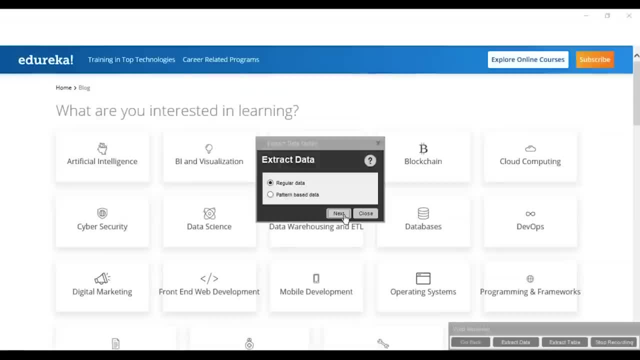 based data. So I'm going to choose regular data. I'll click on next and then I'll choose what data has to be extracted. So I want the BI and Vigilance data to be extracted. So I'll click over here and then you. 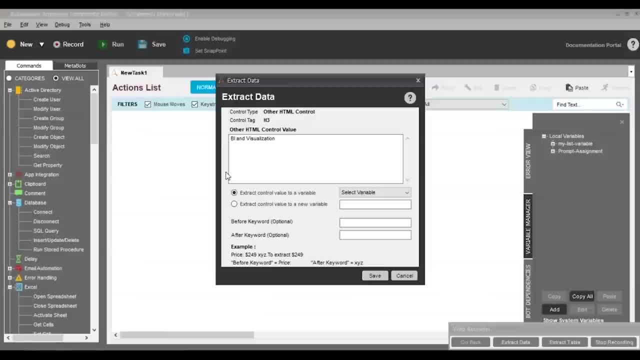 can see that you know behind visualization has been extracted. Now what you can do is you can select the variable so that you know the control value can be stored to a variable. So I'm going to choose the clipboard variable And then I'll click on save. So once I 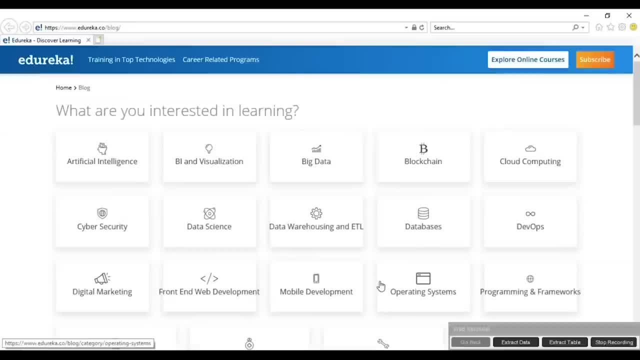 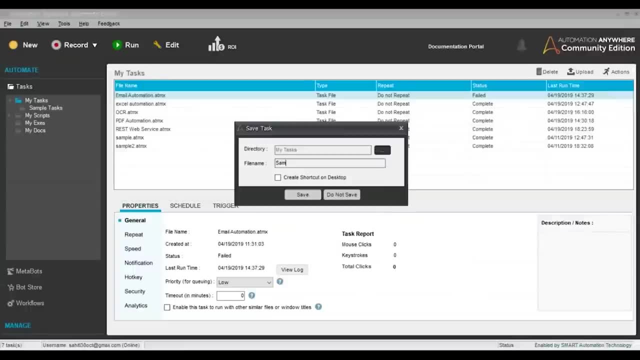 click on save, you can see that you know it has been extracted. Now what can I do is I can just stop the recording and then I can just go back to my task. I'll save this task as, let's say, you know, sample with: 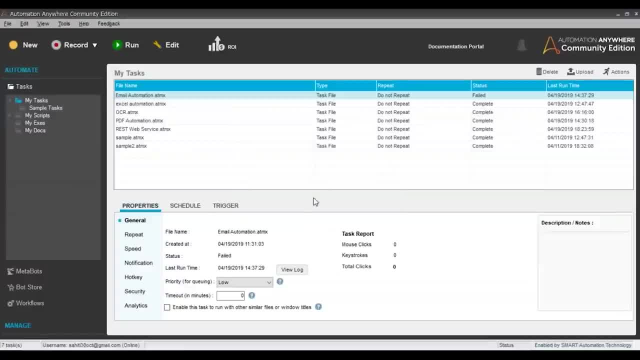 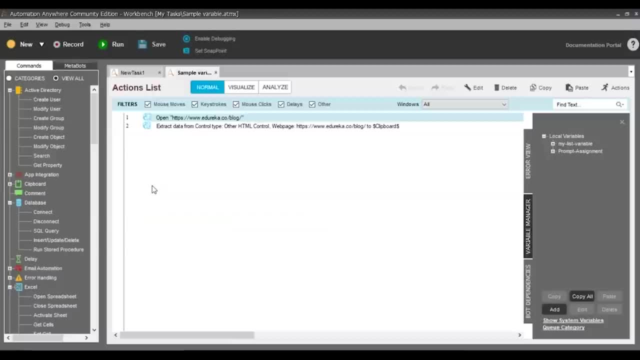 Vigilance data and I variable. I'll click on save. Now I'm just going to edit this task again. And now what I'm going to do is I'm going to display a message box so that you know, you can see the output. So I'm going to search for message box over here. I'm going to drag and drop. 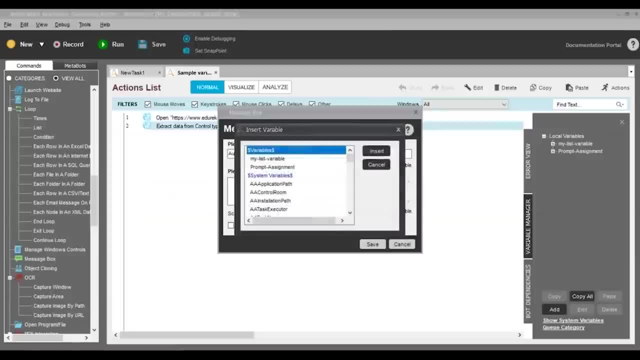 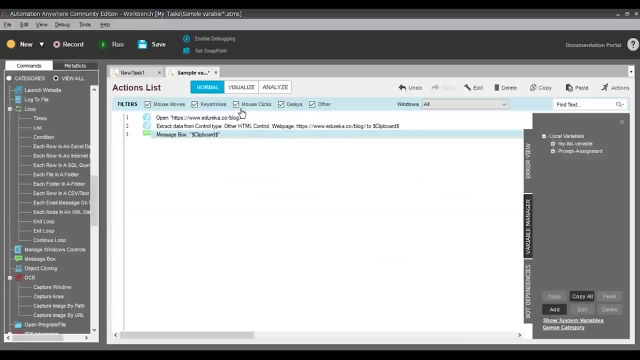 it over here And over here I'll press on control F2 and choose the clipboard variable right, So you can see the clipboard variable is inserted, and then I'll click on save. Now I'll again click on save to save the task and then I'll click on run. So when I click 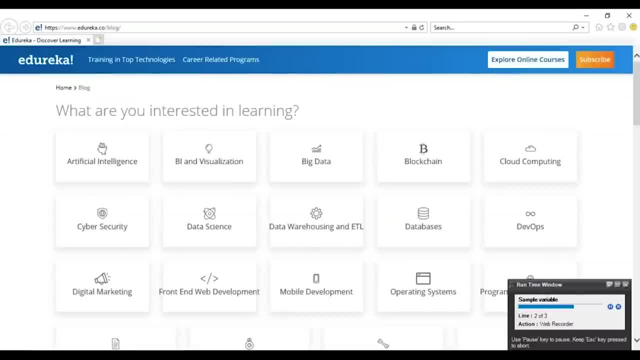 on run. you can see that. you know my task is getting executed, The data is getting extracted And finally, a message box would be displayed right. So we'll wait for that action to happen. And you can see that you know. the message box displays an output of BI and visualization. 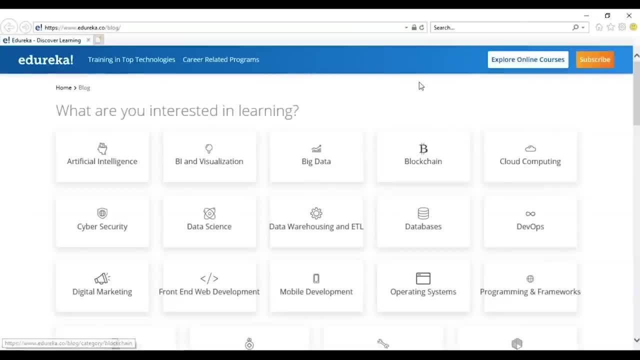 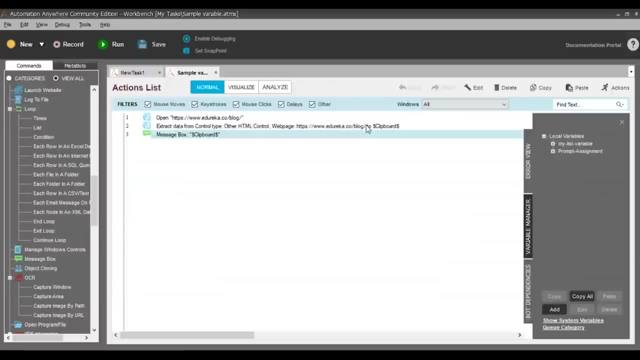 right. So that's how, guys, you can use the predefined variables for any type of automation. Well, when an interviewer asks you what and how the predefined variables are, please don't stick to the theory language. And please don't stick to the predefined variables. Please don't stick to the theory language. 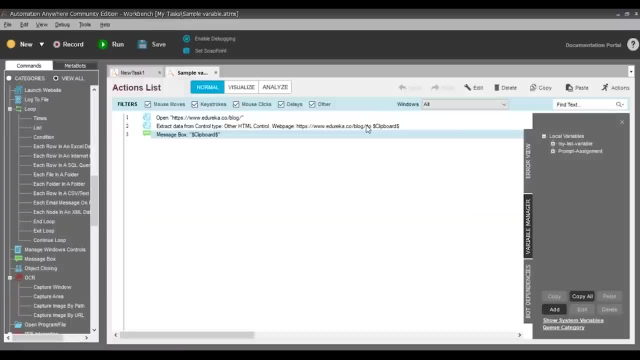 Instead, I would say you can answer by, you know, showing them simple demos or talking about steps through which you can just use these predefined variables in different scenarios of automating a task. So, guys, that was about the predefined variables. Now let's move. 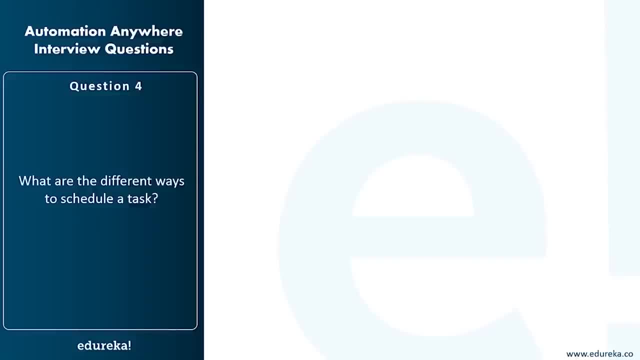 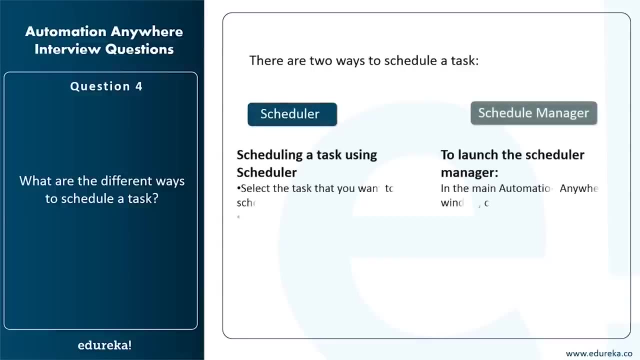 forward with our next question, That is, what are the different ways to schedule a task? So there are mainly two different ways to schedule a task. that is either by using the scheduler or by using the schedule manager. So, starting with, you know the scheduler, so to schedule a task using the scheduler, you 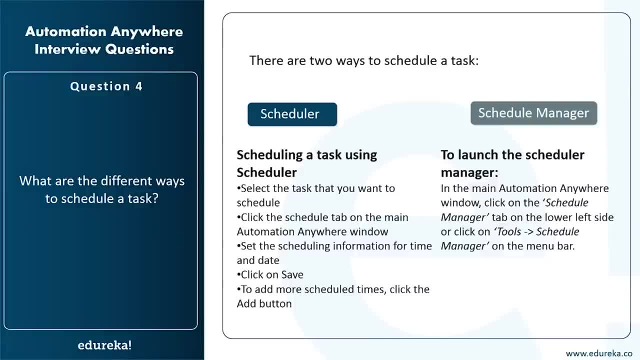 have to select the task that you want to schedule, Click on the schedule tab on the main automation anywhere window and then set the scheduling information for time and date And finally you can click on save. This is how you can schedule a task for a scheduler and coming. 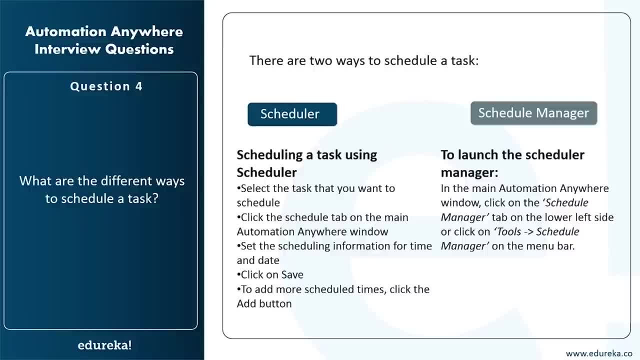 to schedule manager in the main automation anywhere window, Click on the schedule manager tab on the lower left side or, you know, you can also go to tools and go to schedule manager in the menu tab. So let me just show you that if I just want to schedule a task, let's just 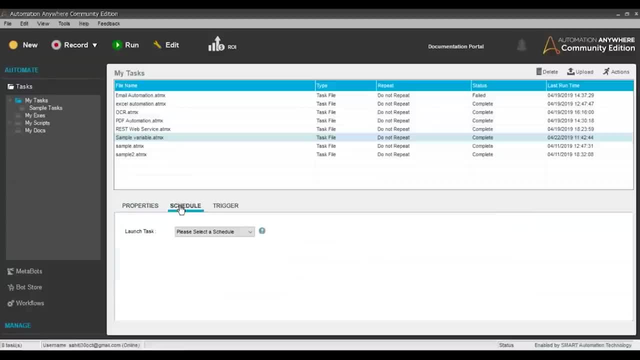 say, if I want to schedule a task to sample variable, what you can do is you can go to schedule over here and then you can select. you know a schedule that is either a one time only or maybe you want it to repeat. I am choosing over here one time only and then you can mention. 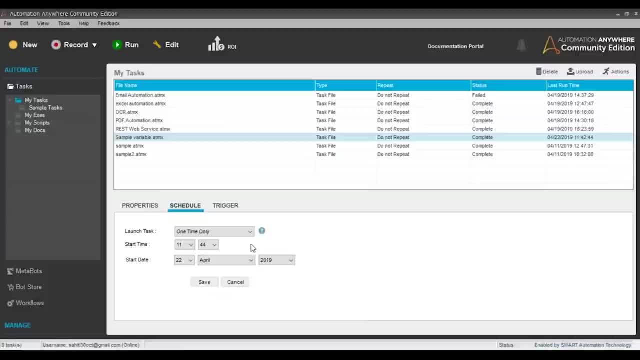 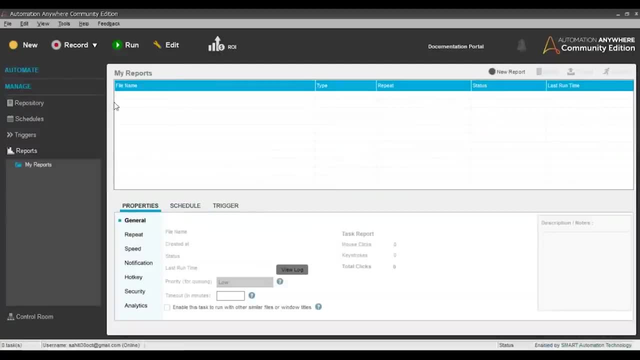 the start time, start date and click on save. So this will basically schedule the task for you and this is how you can use the scheduler. now, coming to schedule manager: now to use the schedule manager, What you can do is you can go to schedules over here and then we'll. 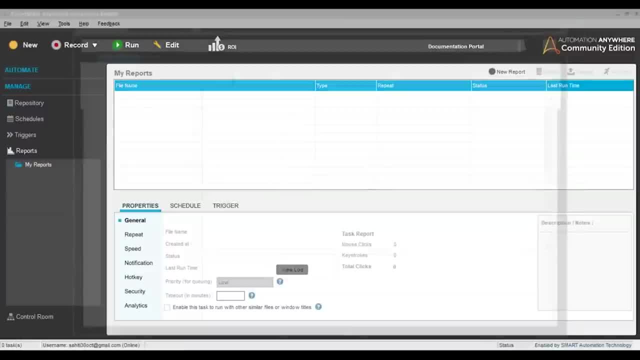 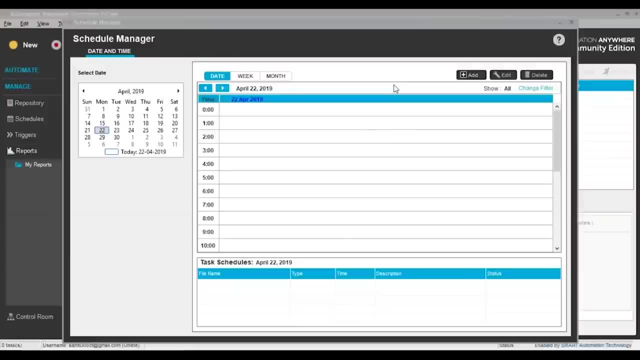 wait for it to load, and once it loads, you can just schedule the task from this point. So, as you can see, this is the schedule manager. So over here You can mention the date, the week, the month, basically when you want to start, how many. 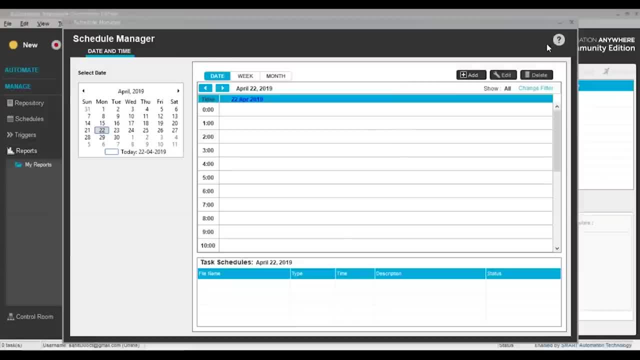 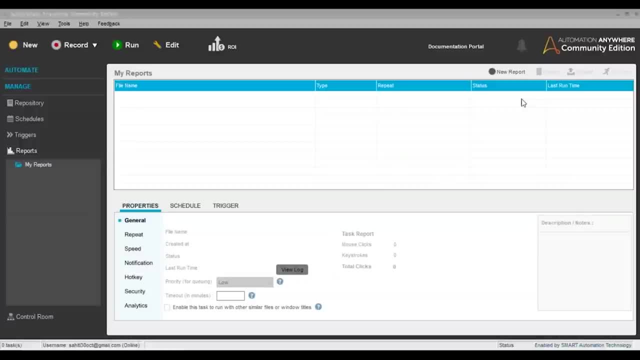 times do you want to repeat? and then you can keep adding the schedules by using the add option. So, guys, that's how you can schedule task in automation anywhere. There are mainly two options, that is, the schedule manager and the schedule. now moving on to the next question. 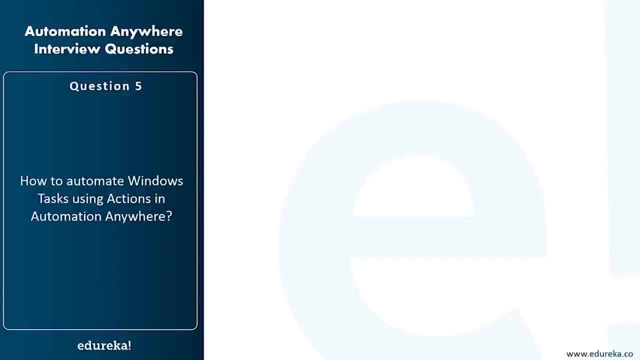 that is how to automate Windows tasks using actions in automation anywhere. So to automate Windows task using actions in automation anywhere, What you can do is you have to choose the Windows actions activity from the activity pane. So there are obviously various actions that you can perform with the window. either you can resize it or you 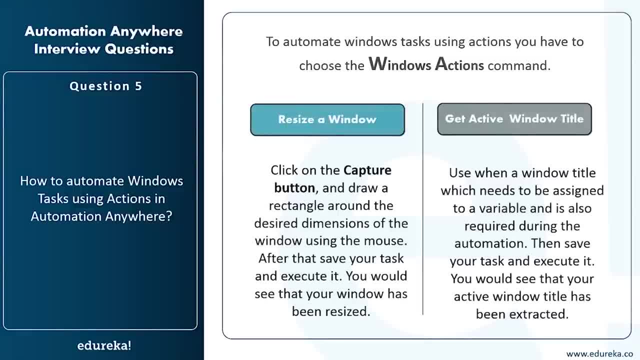 know you can get an active window title, or maybe you can- just you know- maximize the window, minimize the window or close the window, or maybe you can also open a window right. So, for example, if you want to resize a window, what you can do is you have to click on the. 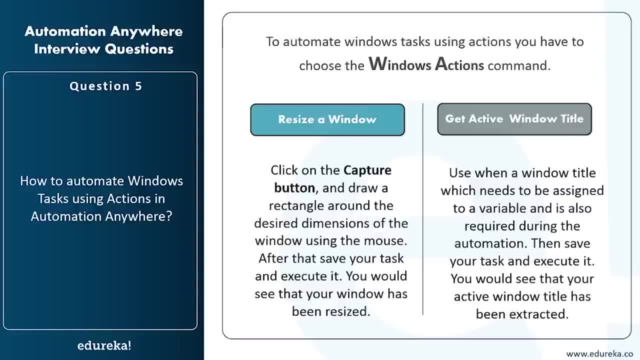 capture button and draw a rectangle around the desired dimensions of the window using the mouse, and after that you can just save the task and execute it. You would see that you know your window has been resized. Similarly, if you want to get the active window title, 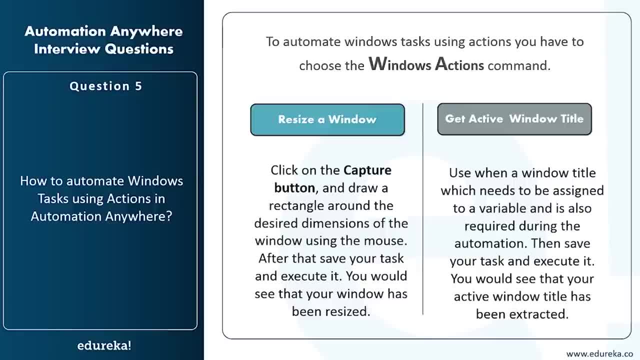 what you can do is you can just get the active window title And then assign it to a variable, and then you can just save your task and execute that task so that you know you can see that the active window title has been extracted. So 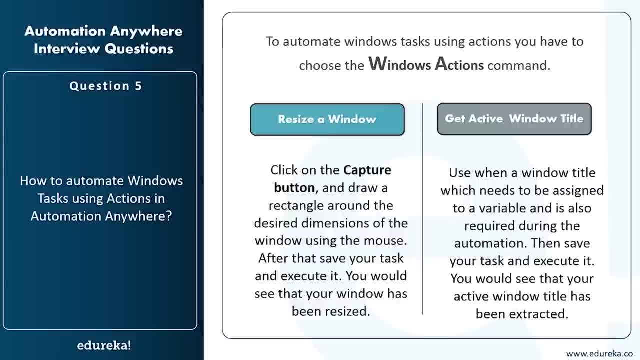 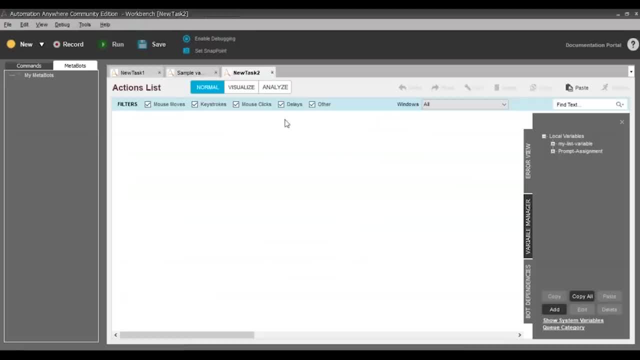 for your better understanding, let me just show you how that is done. So I'll shift back to my automation anyway. And then what I'll do is I'll click on new, I'll choose workbench and let's say, you know, we create a new task to choose the Windows actions You have to. 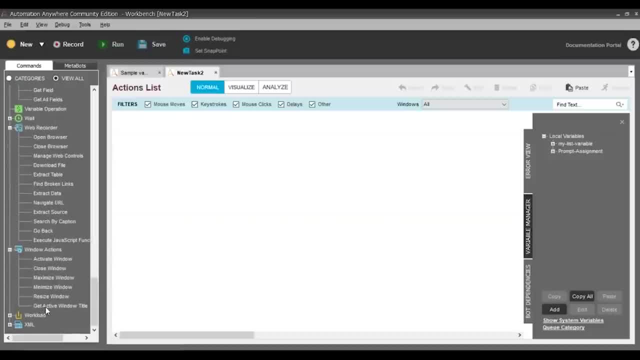 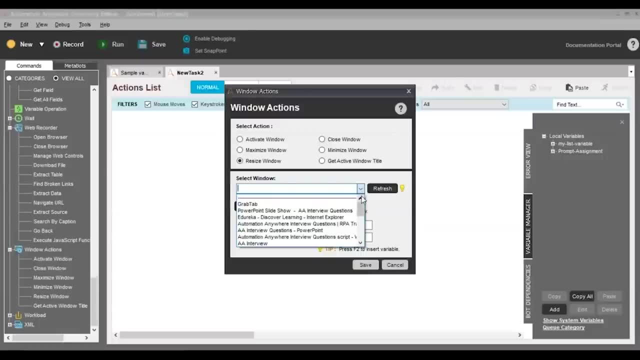 actually search for Windows actions activity on the left side of the pane. So for example, let's say: you know I want to resize the window, So I'll drag and drop it into the workspace and then I'll select the window. So it could be any of them. So let's say: 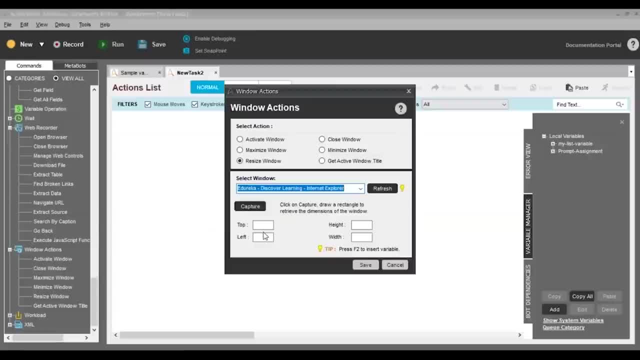 you know, I'm resizing this Internet Explorer window that has been opened, and then you can just click on capture and draw a rectangle to retrieve the dimensions of the window. So I'm going to do that. So let me make sure that is my next step, and then I'm going to 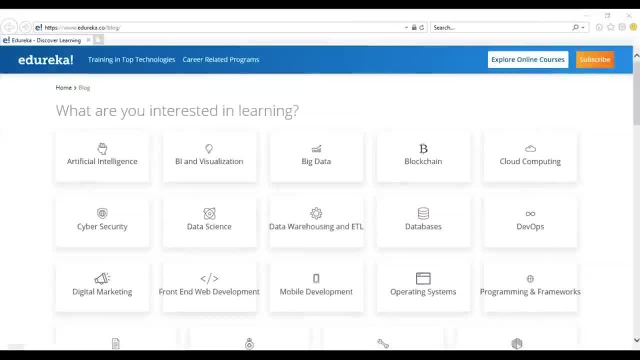 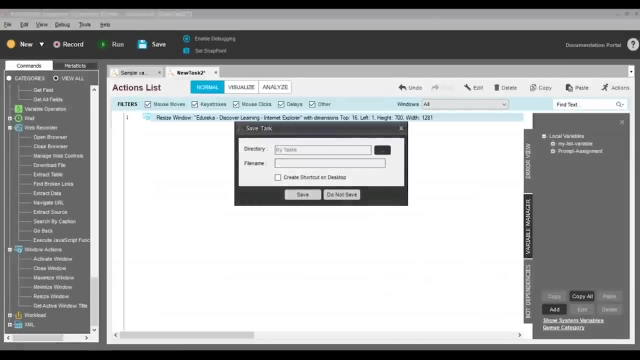 capture. So let's say, you know, we capture till here, And then I'll click on save. Once I click on save, I'll click on save over here, I'll execute the task. So I'll save my task again. So let's say this is resizing window And then I'll click on save and then I'll just 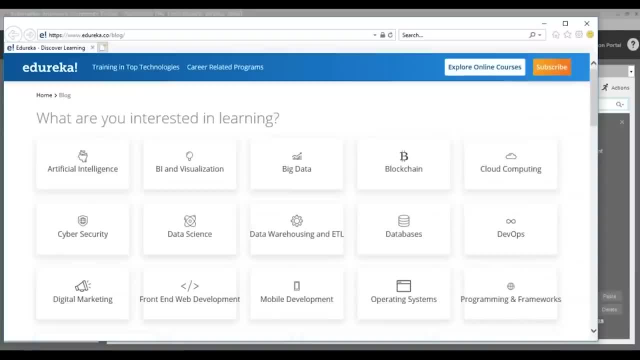 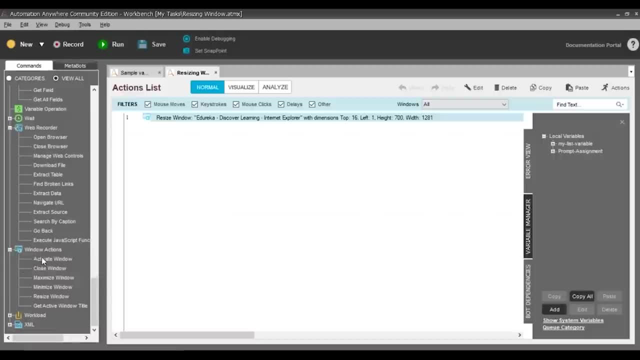 run this task. So when I run this task, you can see that you know the window side has been resized right. So that's how, guys, it's really simple to use this Windows actions where I just showed you for resizing a window. You can use other options, like you know. 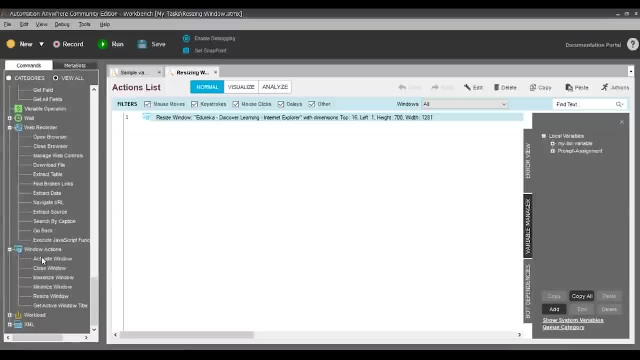 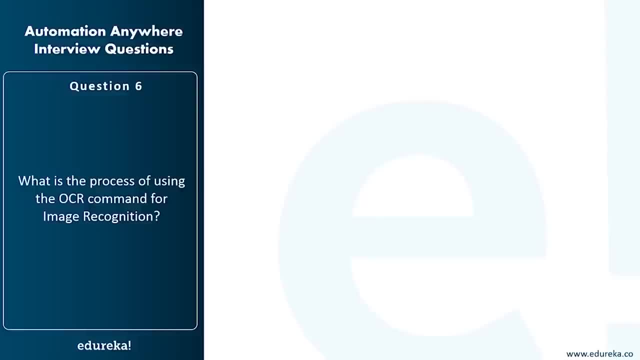 activate, close, maximize, minimize and also get the active window title. So, guys, that was about this question. Now let's move forward with our next question, That is, what is the process of using an OCR command for image recognition? Now, OCR is something really popular. 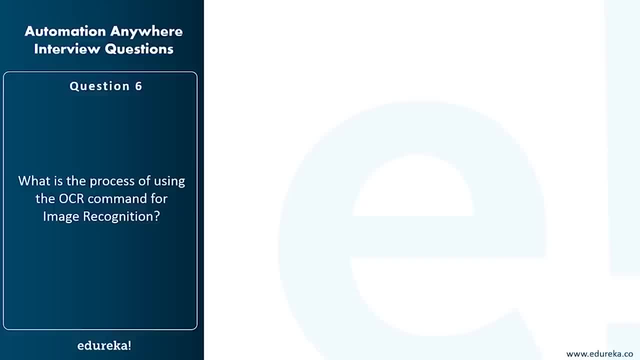 that is used in the industries on day-to-day basis And it's obvious that you know you should know the answer for this question. So, basically, the process for using an OCR command for image recognition is as you can see on my screen. The step one is to specify: 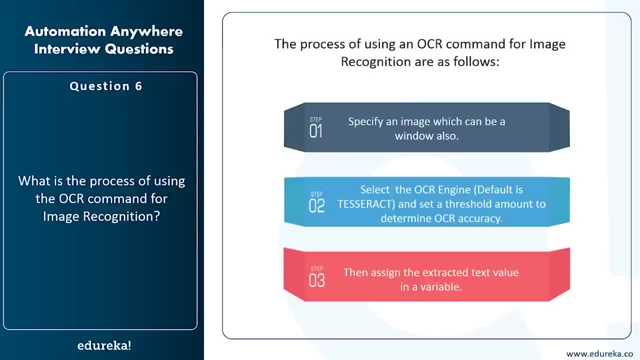 an image, which can be a window Also. the step two is to select the OCR engine. by default It is Tesseract and set the threshold amount to determine the OCR accuracy. And the third step is to assign the extracted text value to a variable, so that you know, you can see. 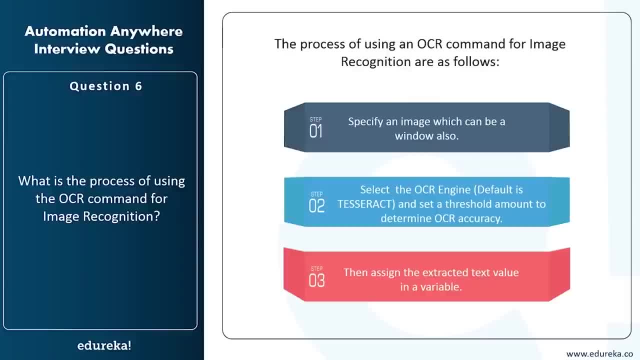 the output either in a message box or you can store it in a file. So, guys, these are the various steps of using the OCR command for image recognition. that starts with specifying an image and then selecting the OCR engines, and then mentioning the threshold amount and. 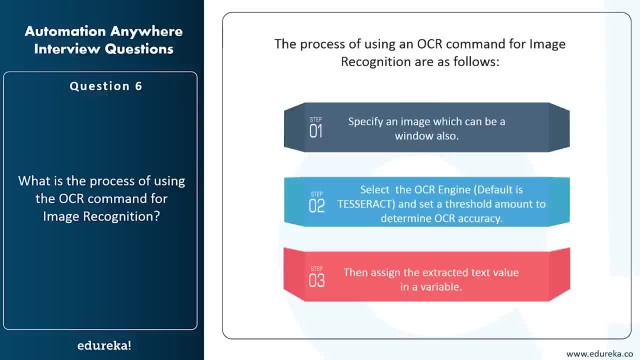 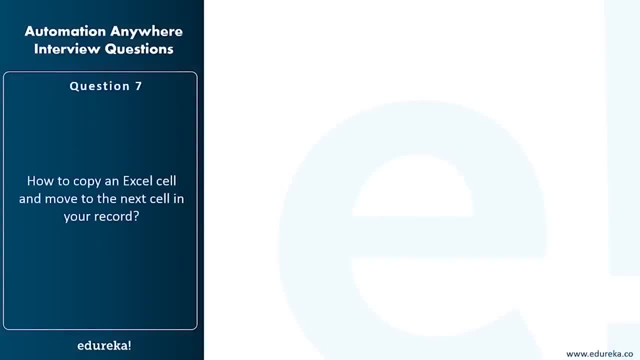 then finally assigning the extracted text value to a variable. So, guys, this was the process of using the OCR command for image recognition. Now let's move forward with our next question, That is, how to copy an Excel cell and move to the next cell in your 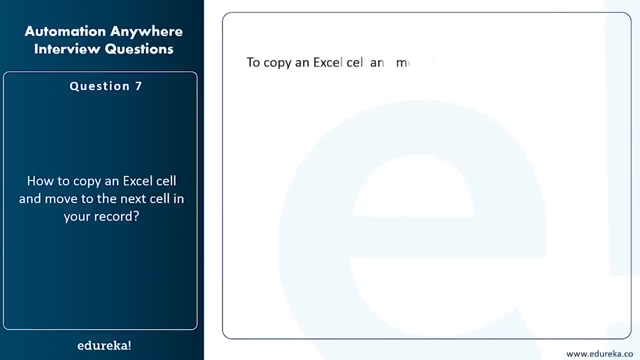 record. So to copy an Excel cell and to move to the next cell in the record, you can first copy the data into the cell using the keystrokes, as you can see on my screen, that is F2,, HOME, SHIFT-DOWN, END, SHIFT-UP, CTRL-DOWN, CTRL-O, and then you can move the cursor to the next. 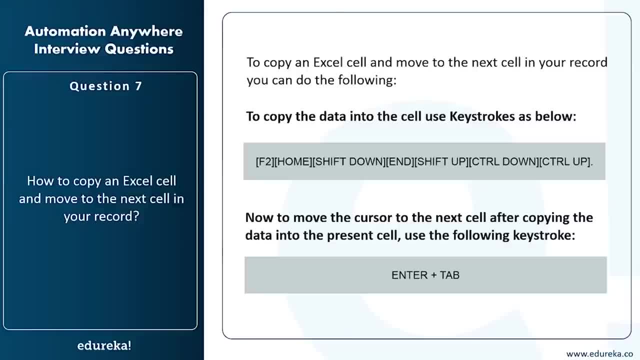 cell after copying the data into the present cell using the keystroke Enter plus Tab. So basically, guys, you can use the keystrokes to copy an Excel cell and move to the next cell in your record after mentioning the data into this present cell. So, guys, that was about. 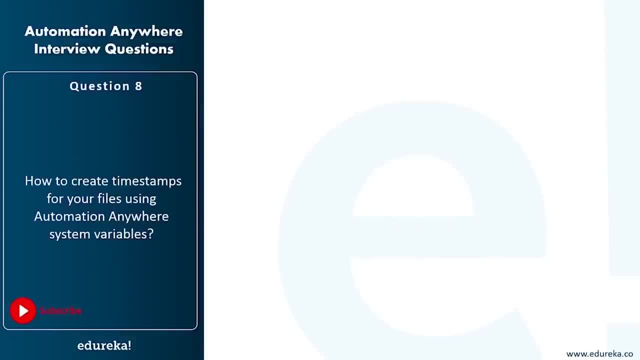 this question. Now let's move forward with our next question, that is, how to create timestamps for your files using Automation Anywhere- system variables. The system variables are basically the predefined variables in Automation Anywhere and under date and the time field, the most popular system. 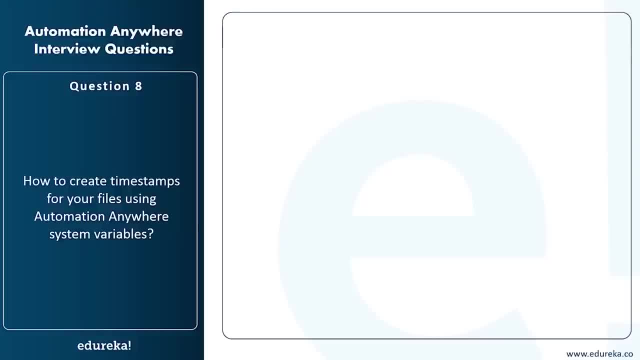 variables are the year, month, day, hour, minute, second and date. Now, basically, you can combine these variables to create a timestamp of your own choice. So, for example, if you want to append the year, month, date at the end of the word example, you can write the: 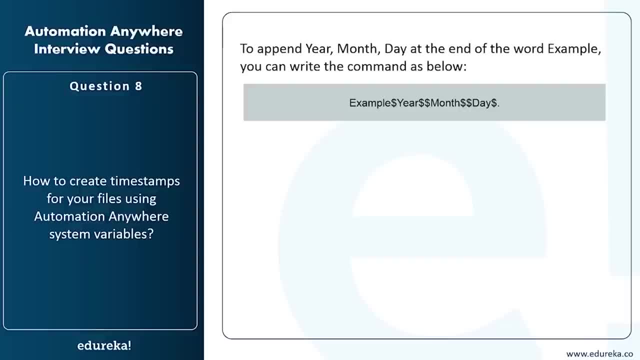 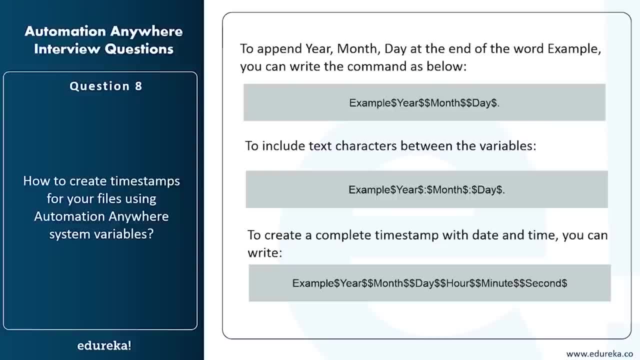 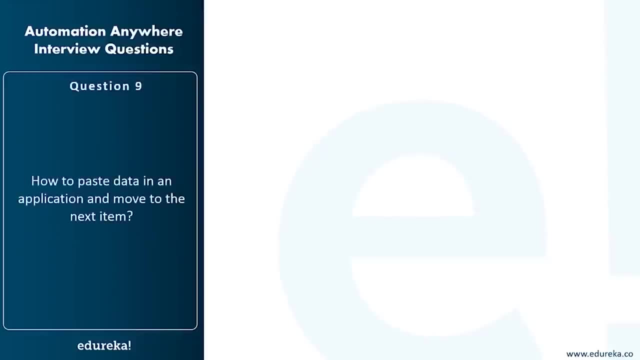 So that's how, guys, you can create timestamps for your files using automation. anyway, system variables, You mainly have to use the year, month, day variable so that you can create them. So, just in case, if you want to configure the format of the date variable, then you can just go to tools, variable manager, system variable and date. Now, moving on to the next question, that is, how to paste data in an application and move to the next item. Well, to paste data in an application and move to the next item, you have to follow the process that is mentioned on the screen. That is first is to identify an element which you wish to copy and use. 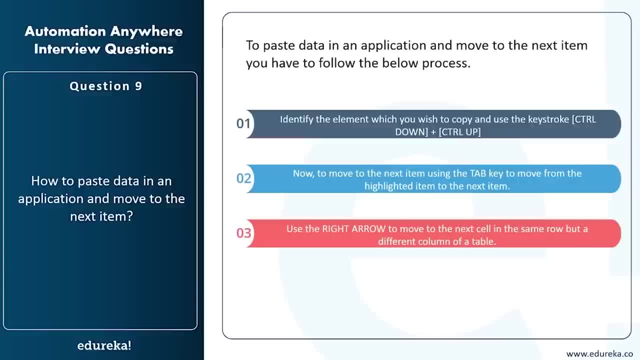 the keystroke, that is, ctrl down plus ctrl up, then after that you have to move to the next item, using the tab key to move from the highlighted item to the next item, and finally, you have to use the right arrow to move to the next cell in the same row but a different column of the table. So, guys, that's how. 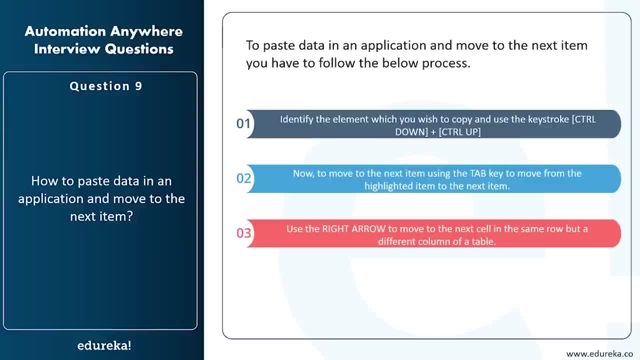 you can paste data in an application and move to the next item. Now, one more thing that i would like to tell over here is that in some applications also support using the space bar to move to the next control or the button. so it's completely based on your application. So that's. 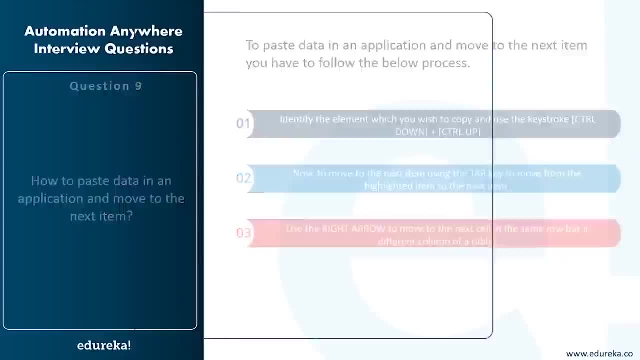 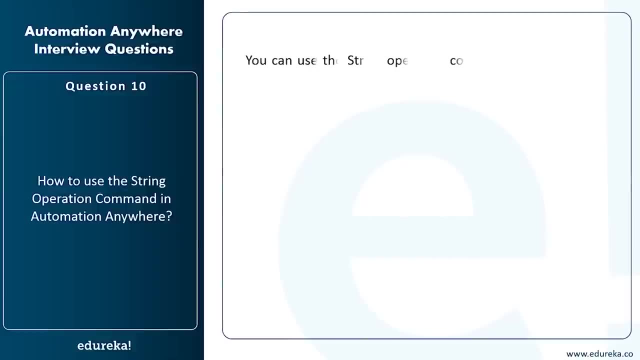 how you can paste the data in an application and move to the next item. now, moving on to the next question, that is, how to use the string operation command in automation anywhere. well, you can use the string operation command in automation anywhere to perform various actions, like you. 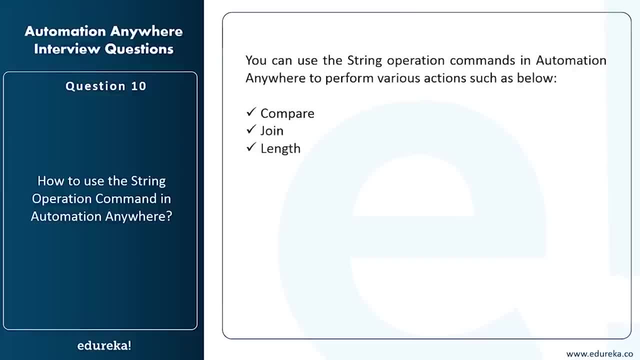 know, comparing two strings, joining two strings, finding the length of a string, reversing a string, either cutting a string- that is basically trimming a string- or finding before and after a string, or you can, you know, make the string to low case or change it to uppercase. you can also replace the. 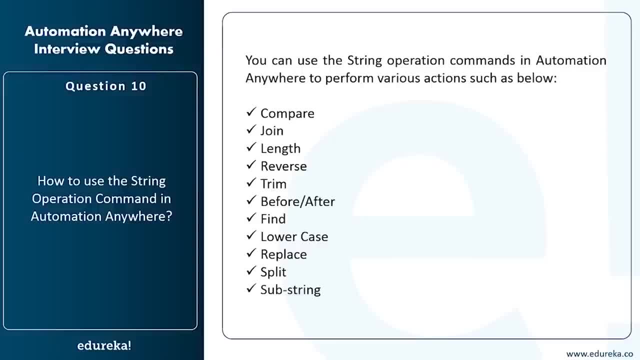 string, split the string and you can also find a substring from a string. basically, guys, these are the various operations that you can perform with the string command. so, for your better understanding, i'm going to shift to my automation anywhere client and i'm going to show you how you can. 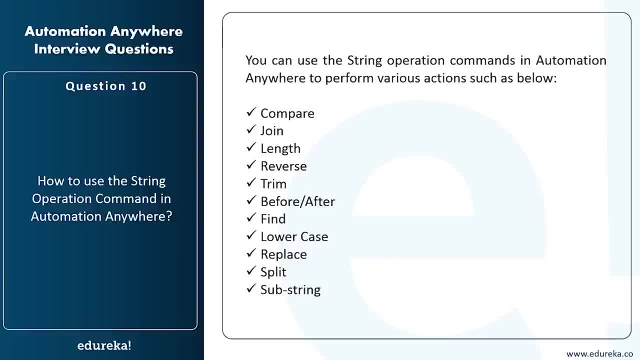 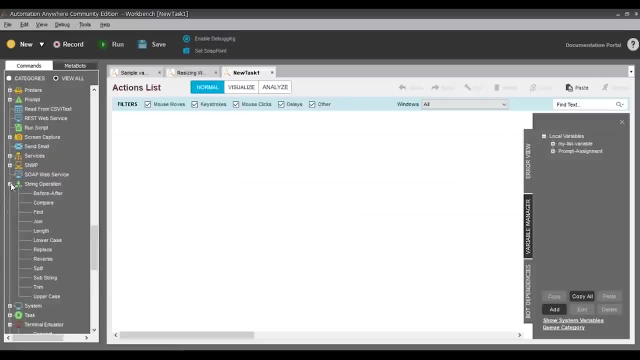 compare two strings. so let me just shift back to my automation anywhere client. now i'll again add a new task. now, in this new task, what i'm going to do is i'm going to search for string operation. so what i'm going to do is i'm going to compare these two strings. so for that i'm going to assign. 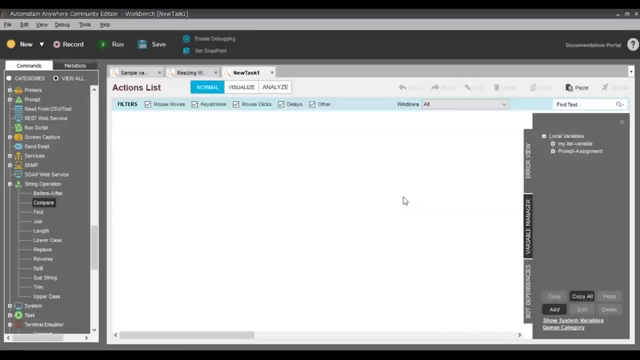 variables with a specific string, so that you know we can use it in a certain way, regardless how you want, for example, a string animation that you��an capable to those variables in the coming up task. So I'm going to go to the variable manager: choose, add. 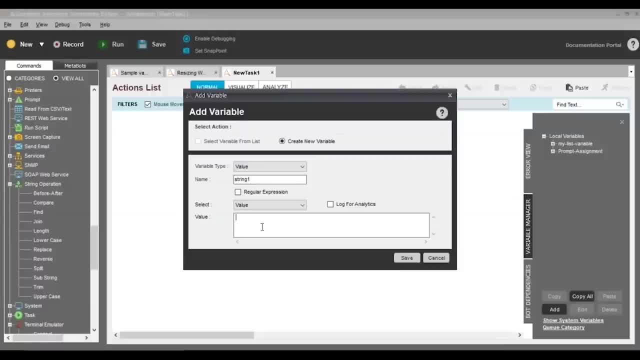 and then I'm going to create a variable, Let's say string one, and let's say we mentioned the value as high from edureka and click on save. Similarly, I'm going to add the second variable, So I'll mention it string- to I'll say welcome from edureka. 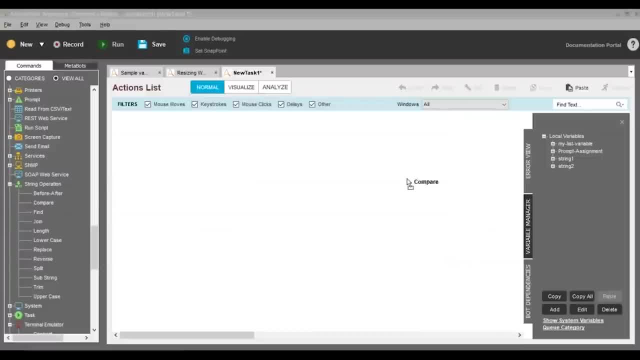 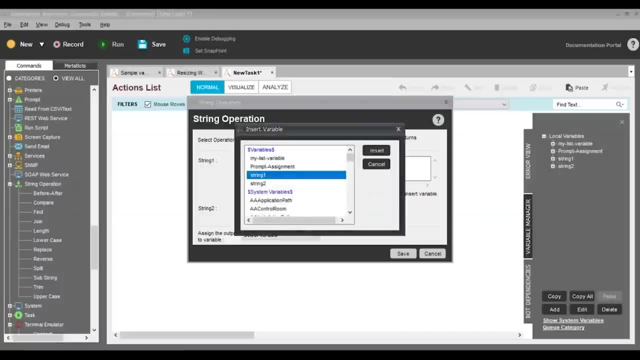 Right, I'll click on save now. What I'm going to do is I'm going to drag and drop the compare string operation into the workspace and then, in the spring one, I'm going to press on control F2 and mention the variable string one, and in the spring two, 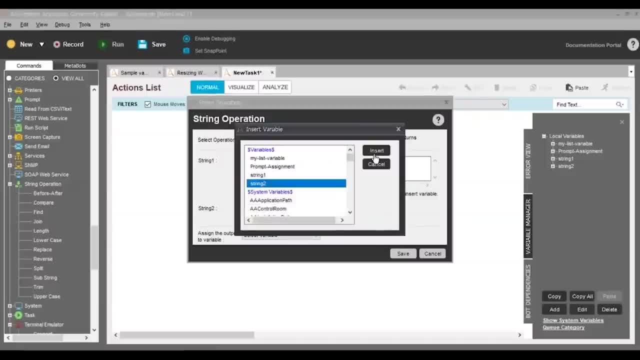 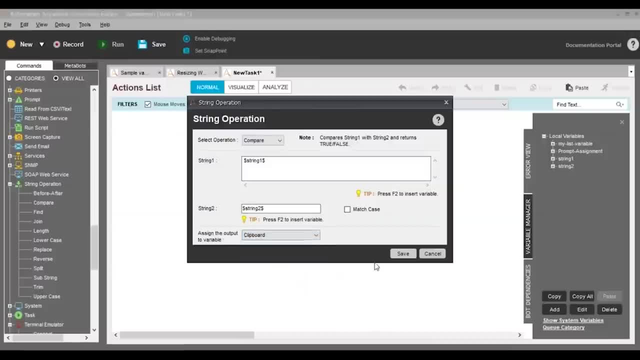 I'm going to again press on control F2 and mention the variable, string two, and then what I'm going to do is I'm going to assign the output to a variable. So I'm going to use a predefined variable over here. So I'm going to use the clipboard variable. 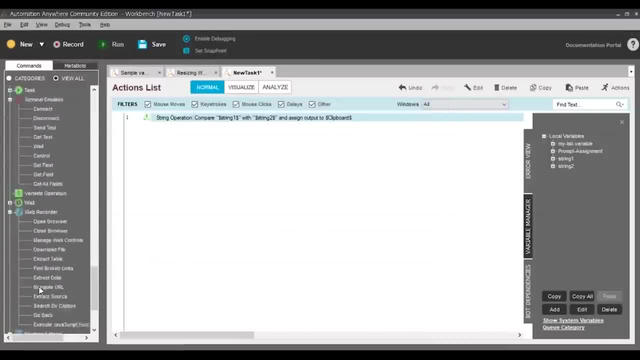 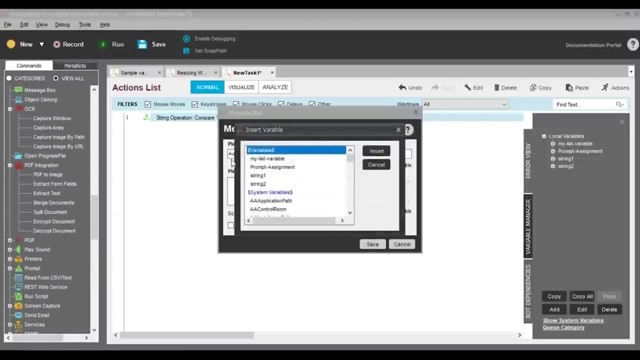 and then I'll click on save. once I click on save, what I'll do is I'll use the message box to display the output. So I'm going to search for message box And then I'll press on control F2 and choose clipboard. 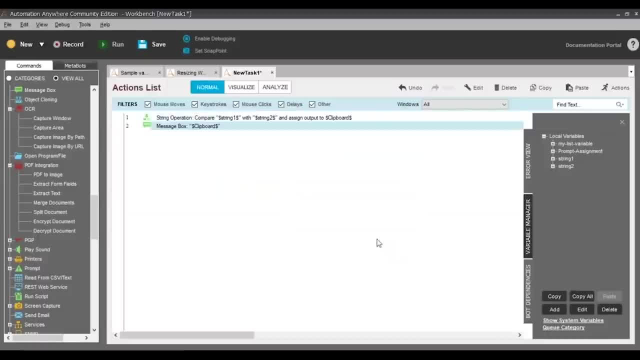 And then I'll click on save. once I click on save, I'll again save my task. So let's say, we mention it, compare strings, And then I'm going to just execute this task. All right, So, as you can see, the output is false. that is because you know. 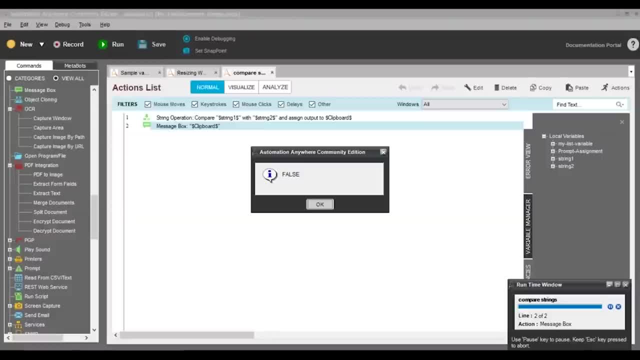 the first string was high from edureka and the second string was welcome from edureka. So these two strings are two different strings. So the output is false. else, if you know the two strings were same, then the output would come as true. So, guys, 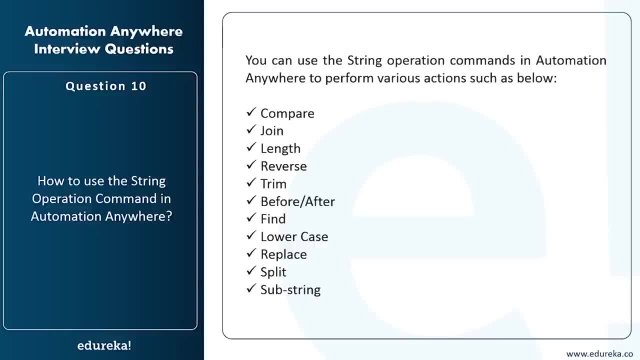 that's how you can use the string operation command and Automation anywhere. So I just explained you with one simple example. you can obviously impress the interviewer with complex examples related to Springs. now, moving on to the next question, That is, what are the system variables? current directory. 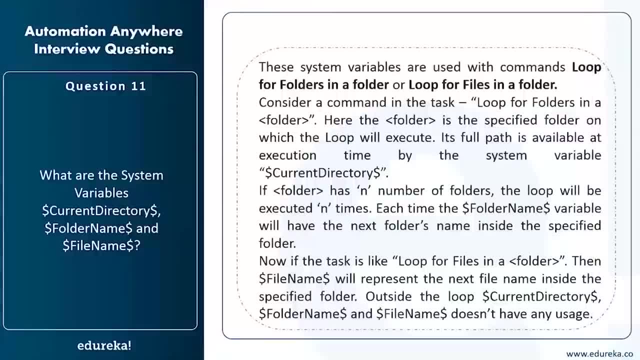 folder name and file name mean well the system variables current directory, folder name and file name basically are used with commands for loop for folders in a folder or loop profiles in a folder. So basically, if you consider a command in the task loop for folders in a folder, here 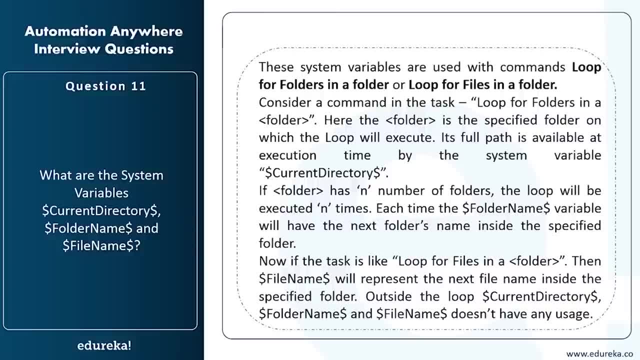 basically, the folder is the specified folder on which the loop will execute, So it basically needs a full part which has to be available for execution time and that you can provide by using the current directory. Similarly, if the folder has n number of folders in the loop will be executed n times. 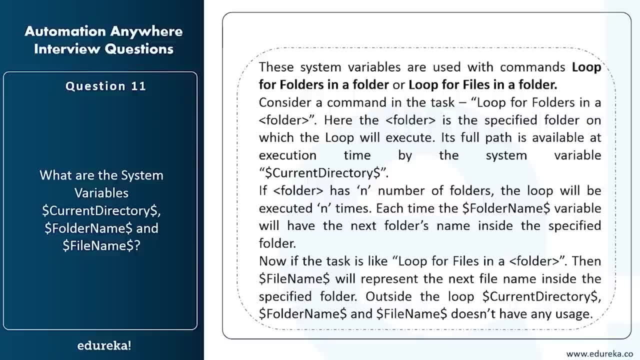 So basically, when you use the folder name variable, each time the folder name variable will have the next folders name inside the specified folder. and now, if the task consists of the command loops for file in a folder, then the file name will represent the next file name inside the specified folder. 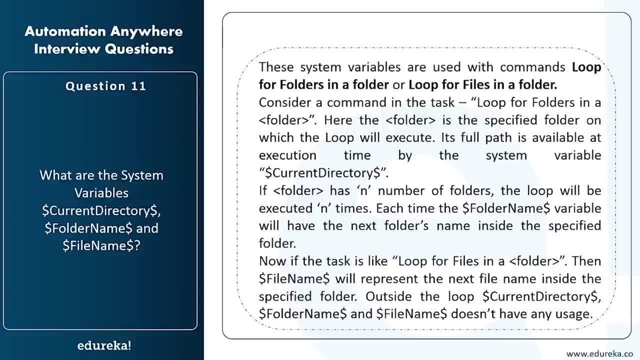 So, outside the loop, the current directory, the folder name and the file name actually do not have much usage, But yes, inside these loops They do have a good amount of usage when you're designing a large, complicated task. So, guys, this was about the system variables- current directory. 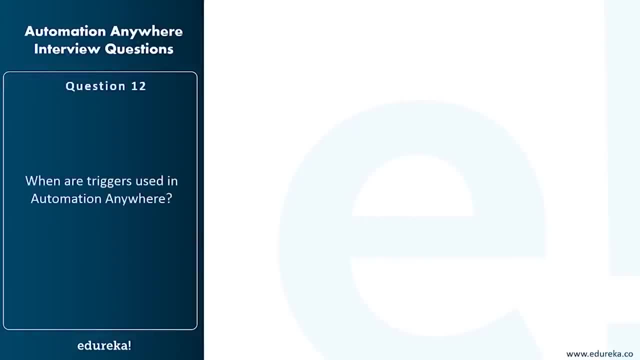 folder name and file name. Now let's move forward with our next question, That is, when our triggers used in Automation anywhere. Well, the triggers are used in Automation anywhere to launch the manager by clicking on the triggers in the main window to add. 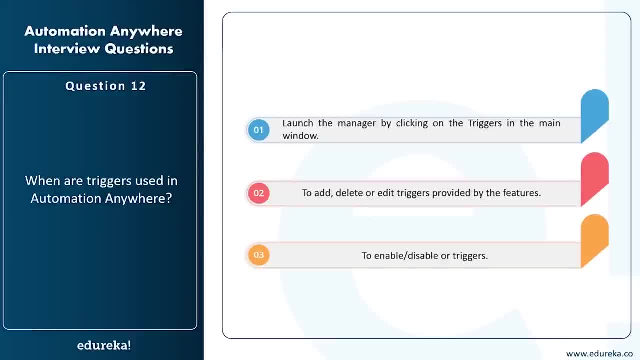 delete or edit the triggers provided by the features and to enable or disable the triggers. So these are mainly the three usages of triggers. that is, to launch the manager by clicking on the triggers in the main window to add, delete or edit triggers provided by the features. 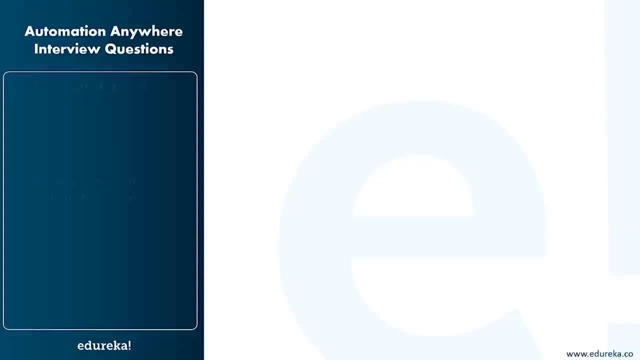 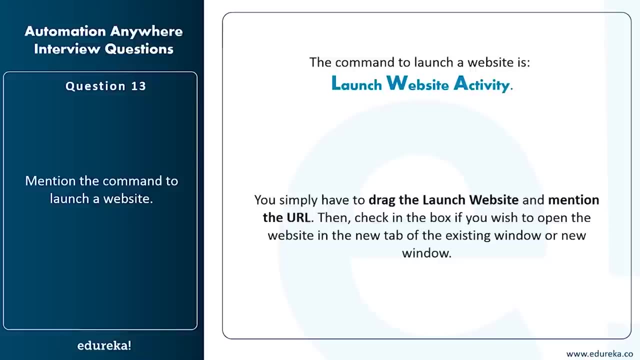 and to enable or disable the triggers. now, moving on to the next question that is mentioned, the command to launch a website. Well, the command to launch a website is to launch website activity. So you simply have to drag the launch website activity and then mention the URL and then you can check in the box. 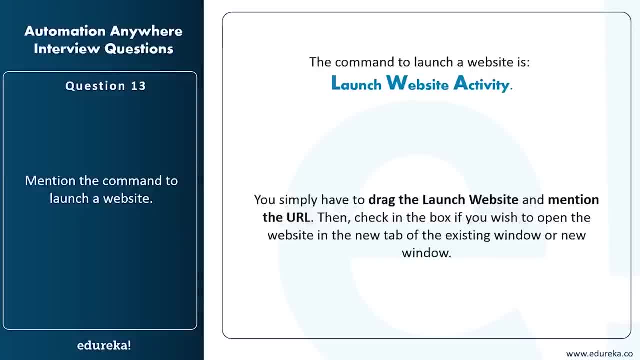 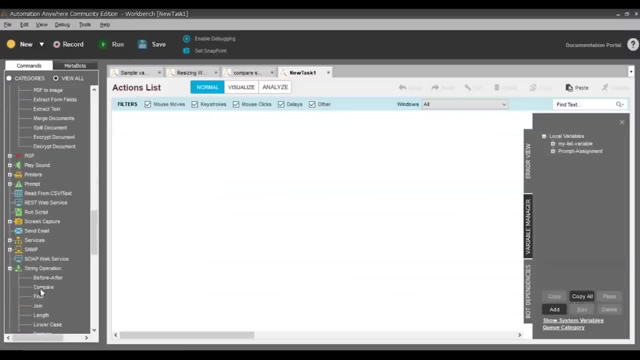 If you wish to open the website in the new tab of the existing window or the new window, So let me just show you the same. So I'll shift again to my Automation anywhere client. I'll click on new- make a new task, and then I'll search for launch. 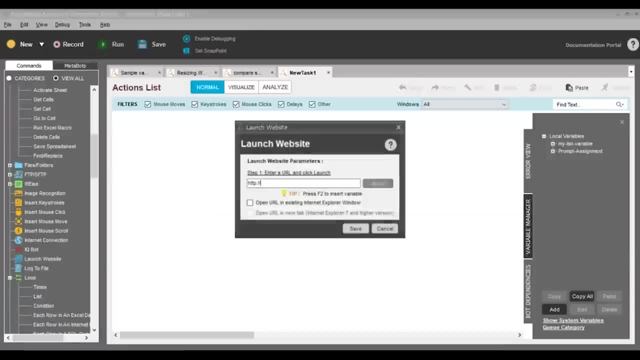 website Right. So this is my launch website activity. I'll drag and drop over here, So I'll just mention my URL over here. Let's say we mentioned Edureka domain, So that's wwwedurekacom, and then over here you can check in. 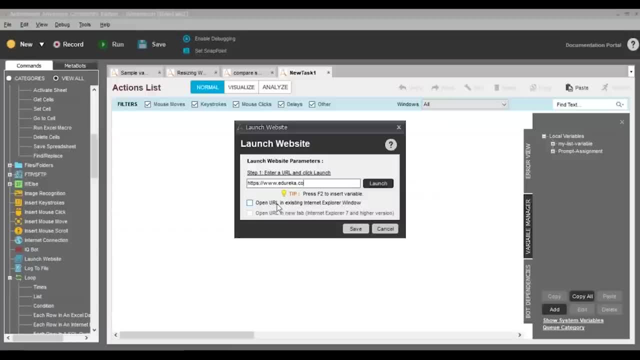 the box. you know, either to open the URL in the existing internet Explorer window or to open the URL in the new tab. So I'm going to choose the option of open the URL in existing internet Explorer window and then I'll click on save. 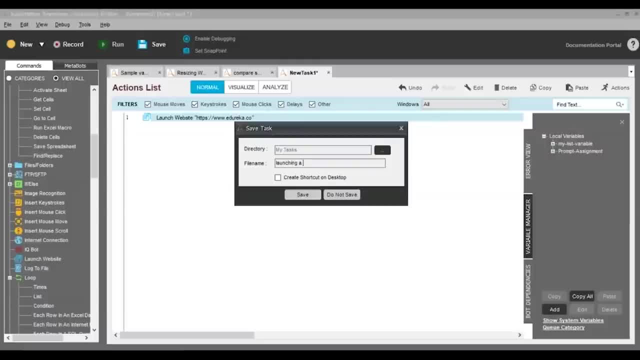 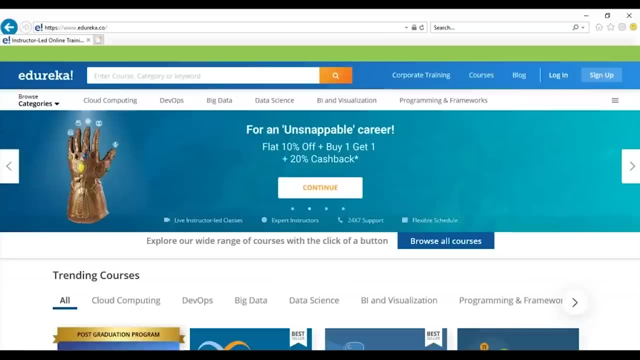 I'll just save the task again. Let's say we mentioned the task name to be launching a website, And then I'll click on run. So the URL that I mentioned in the launch website activity has opened in our internet Explorer. So, guys, this was about you know how you. 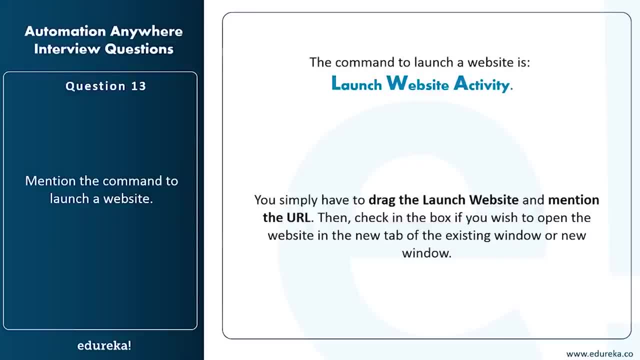 can launch your website. Well, this question was kind of important because you know this type of questions can be used to just to check your knowledge about the tool. So this was just one command that I mentioned about. well, there could be any number of commands that you can be tested about, like 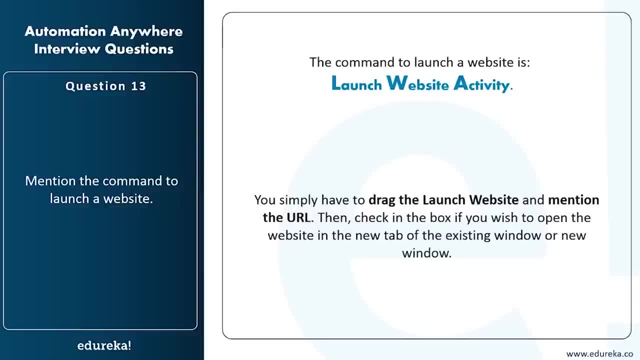 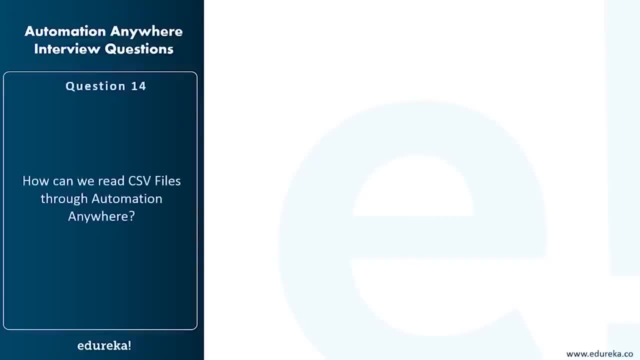 you know how. where do you use the PDF integration? or when do you use the Excel automation commands and what are the different commands inside the Excel automation activity and so on. now moving forward with our next question, that is, how can we read CSV files to automation anywhere? well, to read the CSV file in an automation. 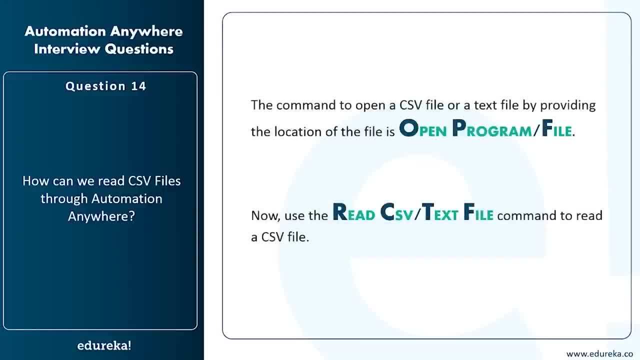 anywhere, You first have to open the file right. So to open a CSV file or a text file you have to provide the file location of the file in the activity open file and then you have to use the read CSV file or the text file command to read the CSV file. 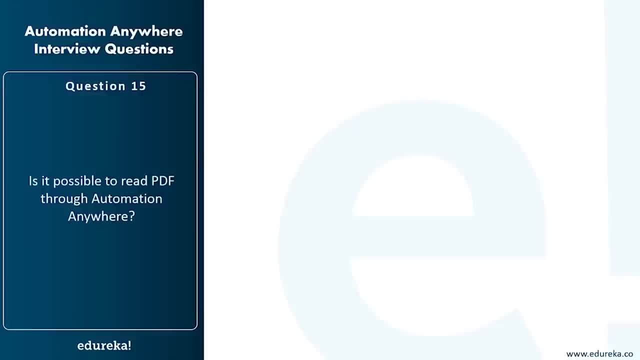 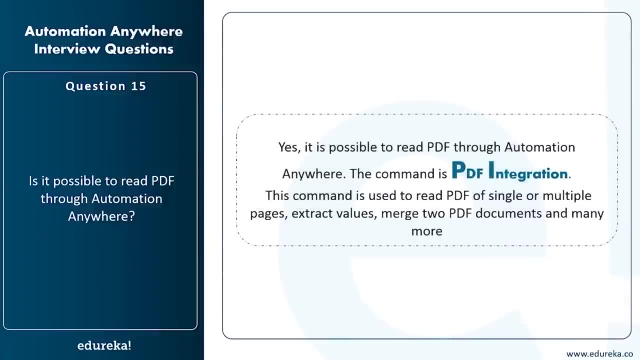 Now moving forward with our next question, that is, is it possible to read PDFs to automation anywhere? Well, this is quite an obvious answer that you know. it is definitely possible to read the PDFs to automation anywhere. The command used is basically the PDF integration command. 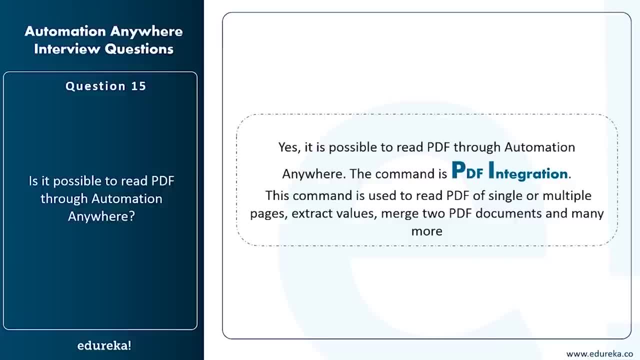 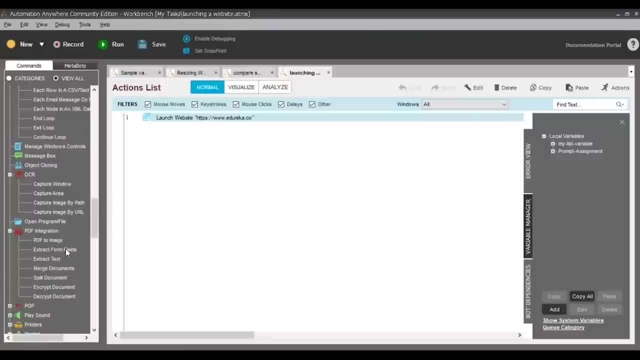 So this command is used to read PDFs Of single or multiple pages, extract values, merge to documents and many more. if you go to the PDF integration command, then you have various commands under it, such as PDF to image, extract form fields, extract text, merge documents, split document, encrypt. 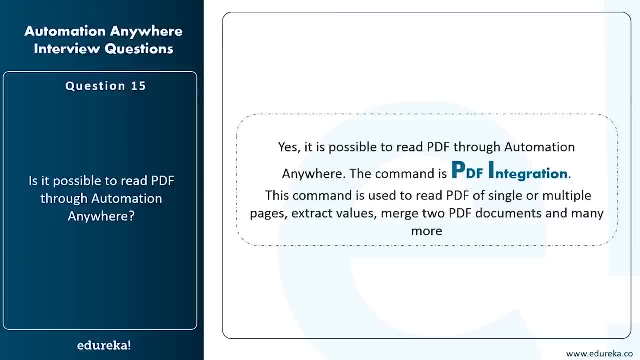 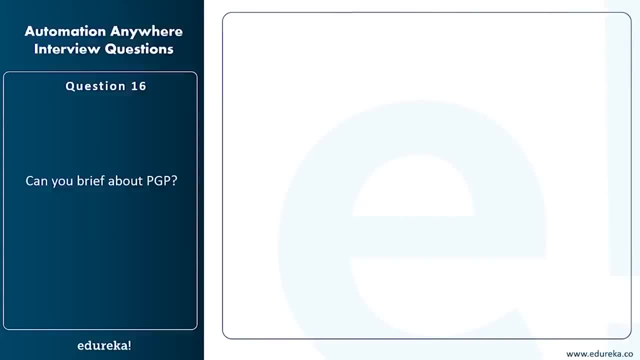 document and decrypt the document. So, guys, that was about this question. Now let's move forward with our next question, That is, can you brief about PGP? Well, PGP is used to encrypt or decrypt the files or create keys by assigning the passphrase. 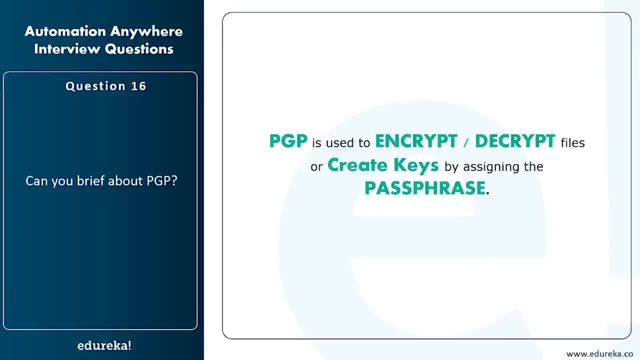 So if someone asks you what is PGP, then PGP is also a command or an activity in automation, Anyway, that is used to encrypt or decrypt the files or create keys by assigning the passphrase. now moving forward to the next question, That is, which commands are not recommended to use if the 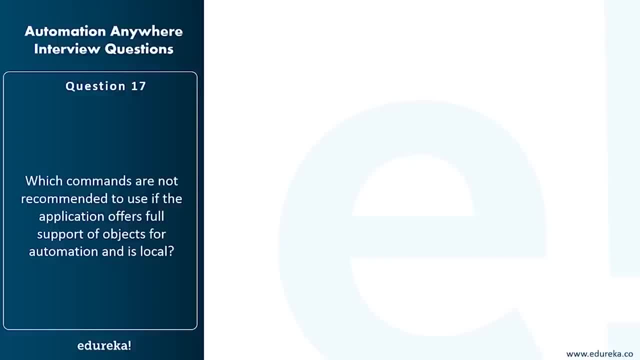 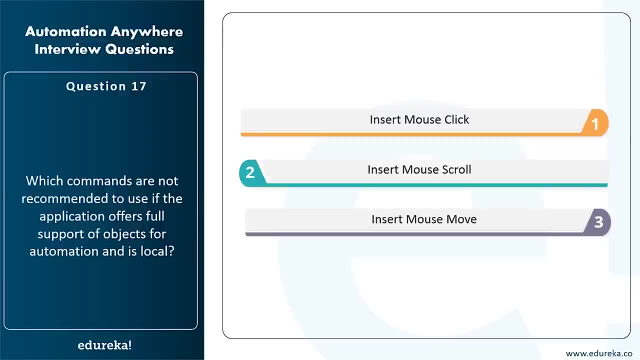 application offers full support of objects for automation and is local. Well, the commands which are not recommended to use are the insert mouse click, the insert mouse scroll and the insert mouse move. This is mainly because you know these commands are related to the mouse click actions. 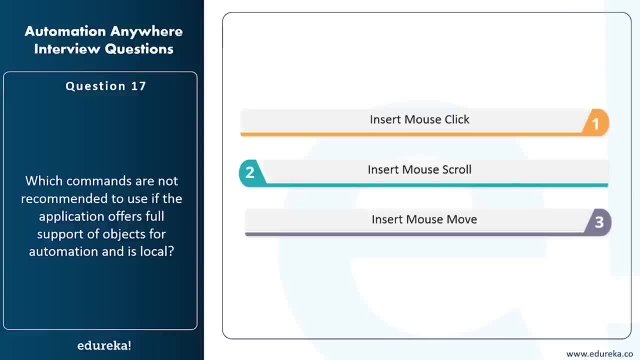 And if an application offers full support for objects for automation and is local, then it can obviously happen that you know the objects can change. so it's not recommended to use these actions of insert, mouse click, mouse scroll and mouse move. Now let's move forward with our next question. 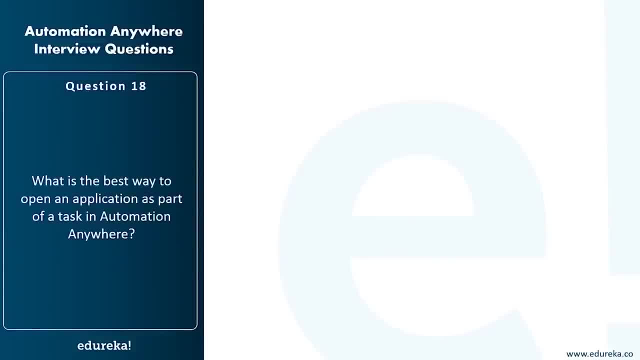 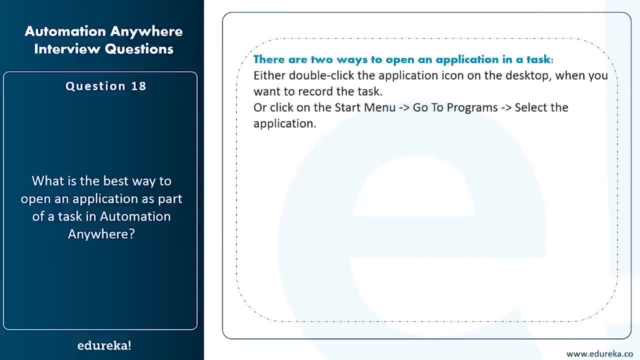 That is what is the best way to open an application as part of a task in automation anywhere. Well, there are mainly two ways to open an application as a part of task in automation anywhere. that is either by double-clicking the application icon on the desktop where you 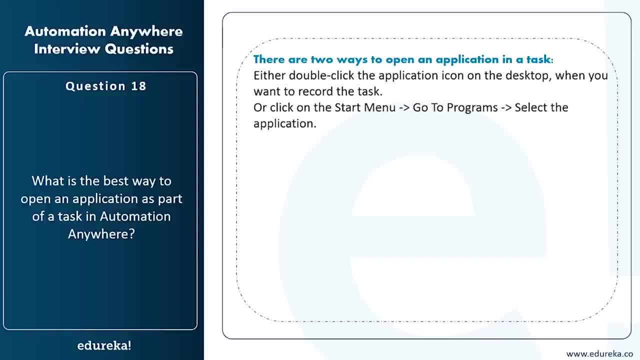 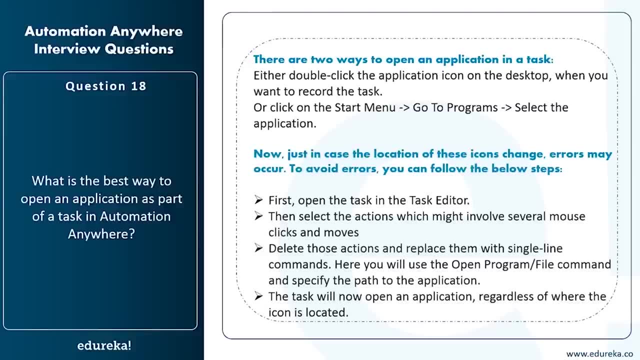 want to record the task, or by clicking on the start menu, Then go to programs and then selecting the application. Now, just in case, if the location of these icons change, then it will definitely result in an error when you're trying to execute the task. 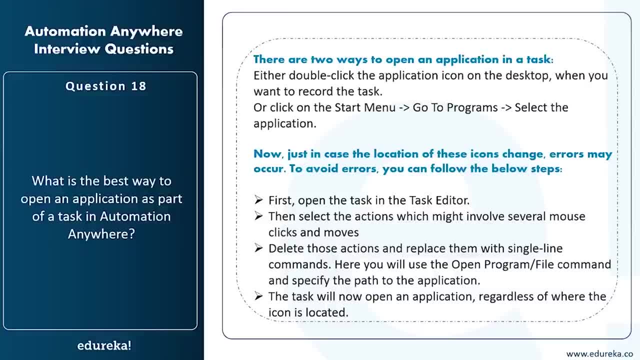 So to avoid errors, you can follow the steps that you can see on my screen, That is, firstly you open the task in the task editor and then select the actions which might involve several mouse clicks and moves, then delete those actions and replace them with single line commands. 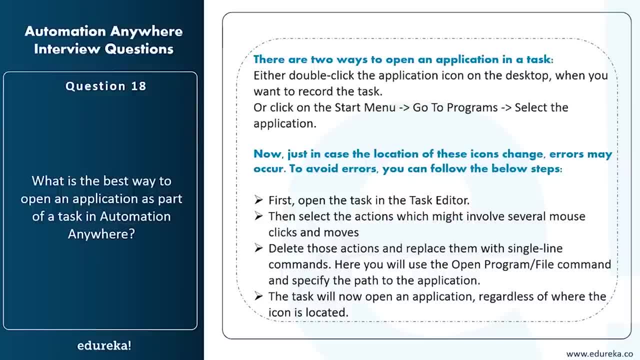 So here you'll basically use to open file command and specify the path of the application, and then the task will now open an application, Regardless of where the icon is located. So that's how you can avoid the error, guys. Now moving forward with our next question. 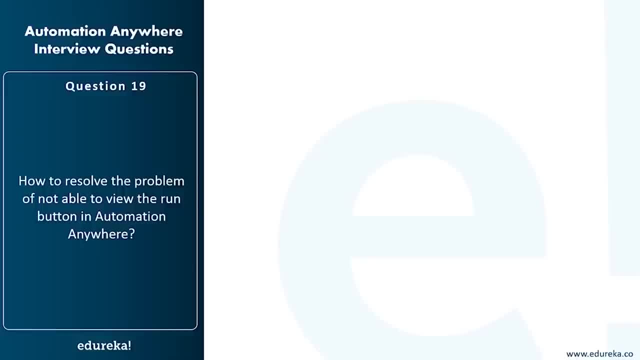 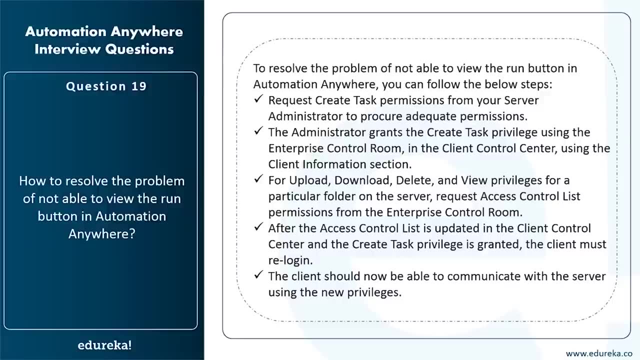 That is how to resolve the problem of not able to view the run button in automation anywhere. Well, to resolve the problem of not able to view the run button in automation anywhere, You can follow the steps that you can see on my screen. You can request the create task permissions from your server. 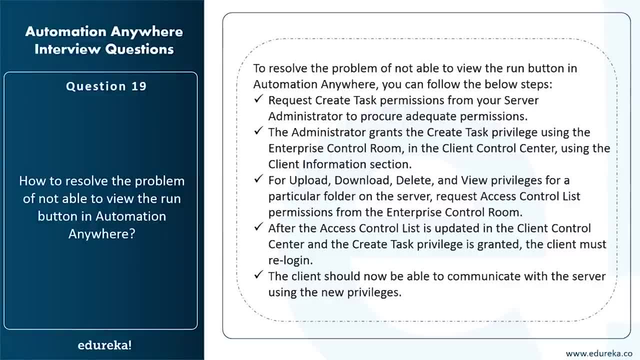 administrator to procure adequate permissions. Then the administrator will grant the create task privilege using the enterprise control room in the client control center, using the client control room Information section and for upload, download, delete and view privileges for a particular folder on the server. You can request the access control list permissions from: 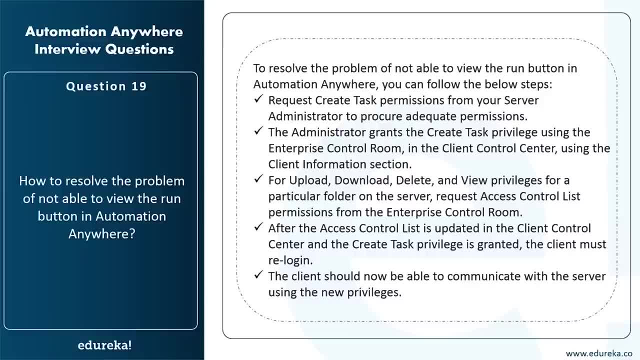 an enterprise control room. after that, the access control list is updated in the client control center and the create task privilege is granted and the client must re-login. So, with the steps that I just explained you, the client should be now able to communicate with the server using the new 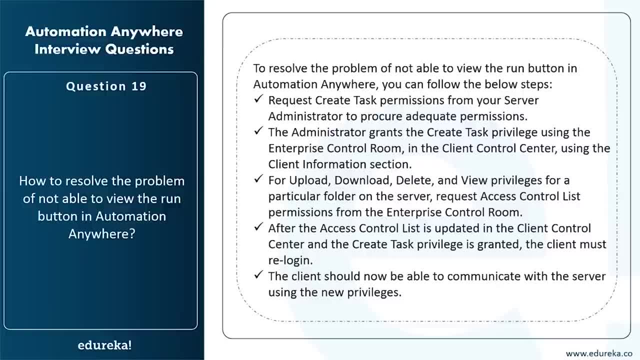 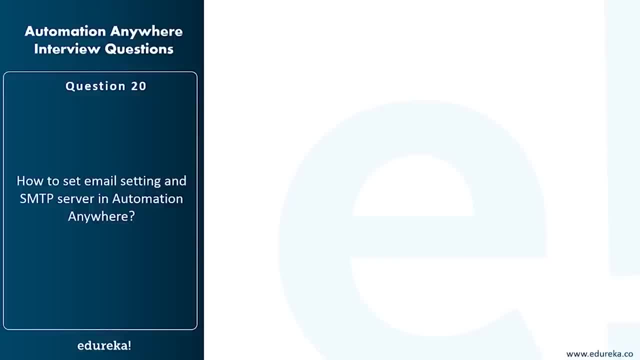 privileges. That's how you can resolve the problem of not able to view the run button in the automation anywhere. Now moving forward with our next question. That is how to set an email setting and SMTP server in automation anywhere. Well, to set the email and SMTP server in automation anywhere. 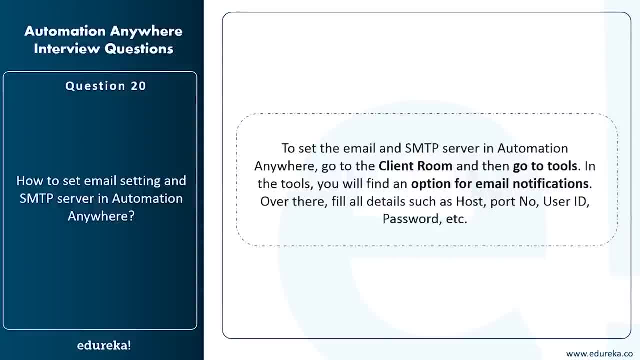 You have to go to the client room- that is basically your client server- and then go to tools. in the tools You will find an option of email notifications over there. You'll have to fill in the details, such as the host name, port number, user ID, password, and then you'll be all good to do. 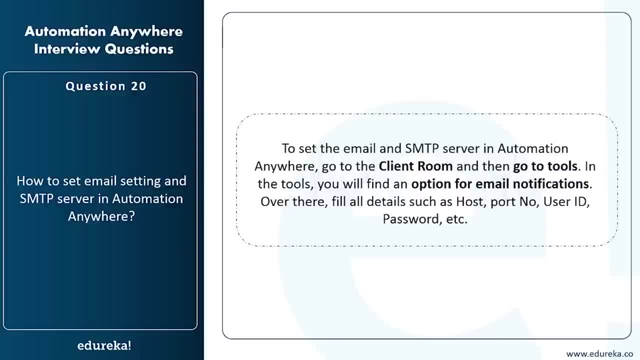 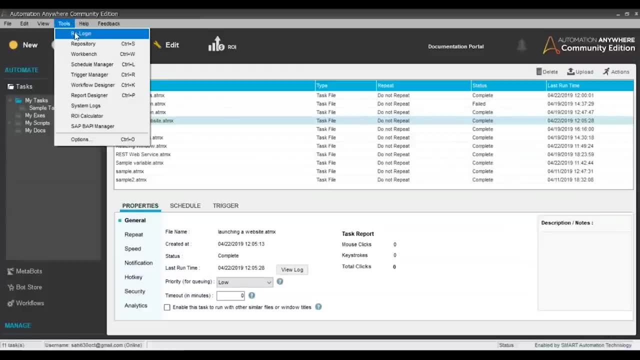 email automation, right. So that's how you can set your details for emails and SMTP server. So let me just show you in my automation anywhere client. So I'll just go back, go to tools over here And then what I'll do is I'll go to options over here and in the 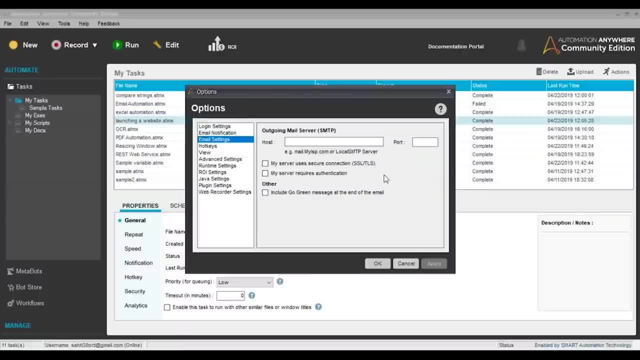 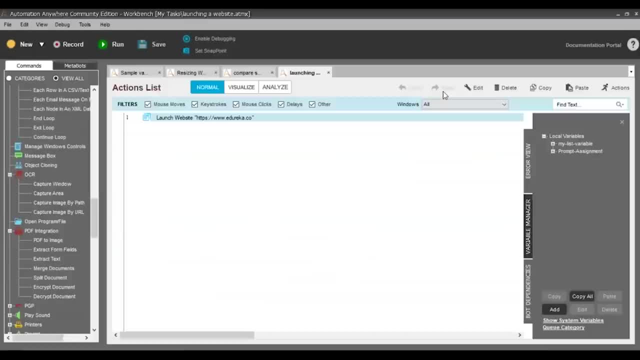 options you'll find an option for email setting. So in the email settings you'll have to mention the host and the port number and then you can click on Okay, and that's how you're good to go for email automation. So, guys, with this we come to an end of our tool based questions. 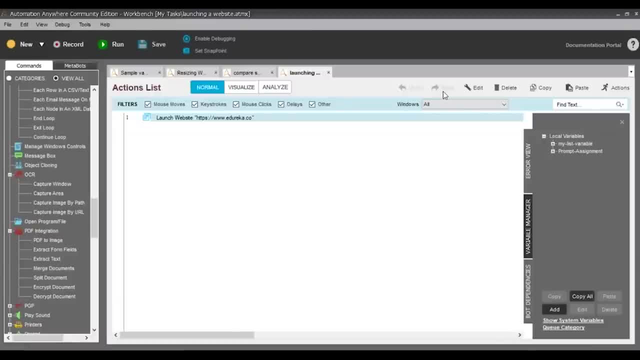 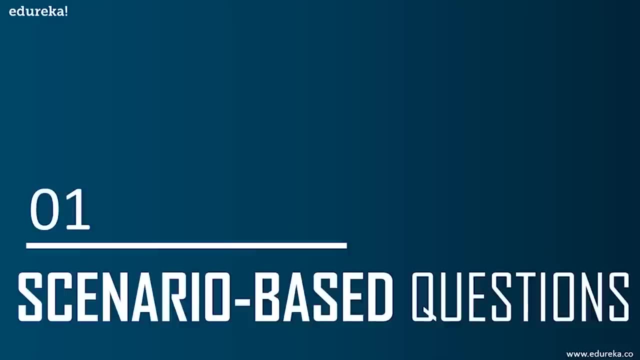 So I hope you have understood all the questions and I hope it was clear to you guys till now. Now, next in this session, We'll move forward with our scenario based questions. So the scenario based questions will basically consists of different scenarios where you can use automation anywhere and 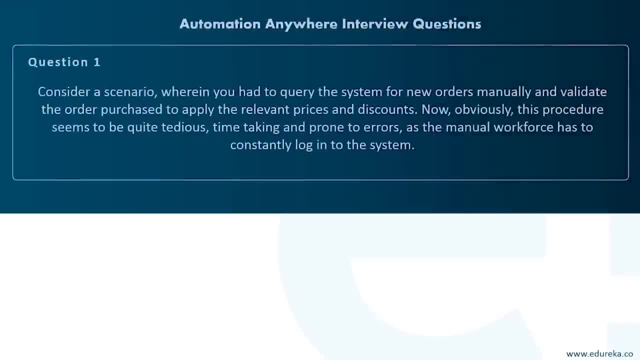 how you can automate different tasks. All right, So let's start with the first question now. consider a scenario wherein you had to query the system for new orders manually and validate the order purchase to apply the relevant prices and discount. Now, obviously, this procedure seems to be quite tedious and 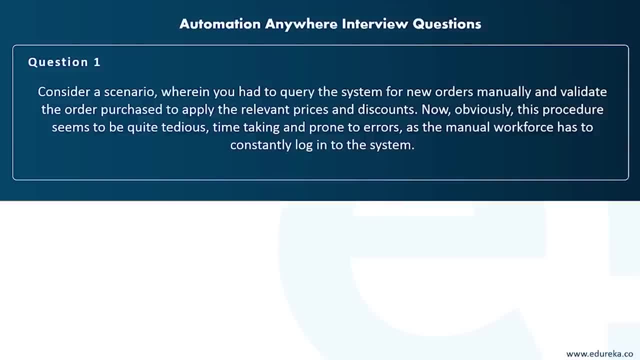 time-taking and prone to errors. right as you know, manual workforce has to constantly log into the system, and then they have to validate the process, enter the data Again, and then they also have to apply the discounts. right now, What do you think will be the process workflow to resolve this? 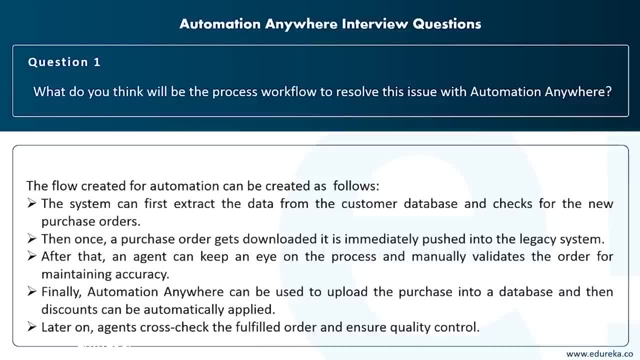 issue with automation anywhere. Well, you can answer this question by just imagine just drawing a workflow in your mind and then you know, you can explain the interviewer your workflow. So the flow that can be created for automation can be, as you can see on my screen. 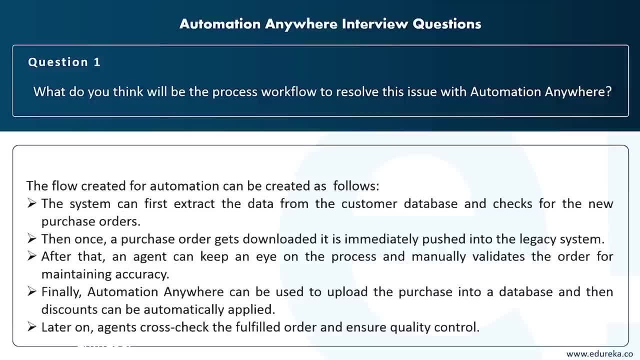 The system can first extract the data from the customer database and then check for the new purchase order. Then, once a purchase order gets downloaded, it is immediately pushed into the legacy systems. After that, an agent can keep an eye on the process and manually validate the order for maintaining accuracy. and finally, 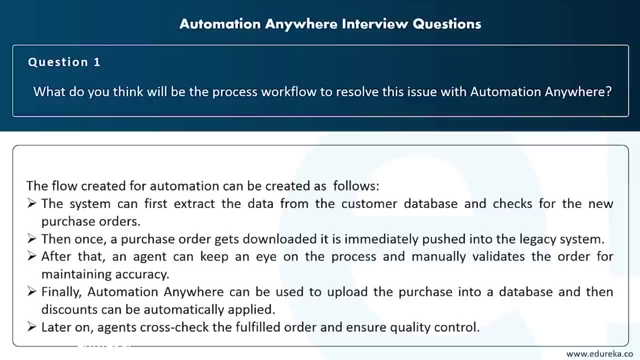 automation anywhere can be used to upload the purchase into a database and then the discounts can be automatically applied. later on, the agents can cross check the fulfilled order and ensure quality control. So, guys, this was the workflow that can be used to resolve this issue with automation anywhere. 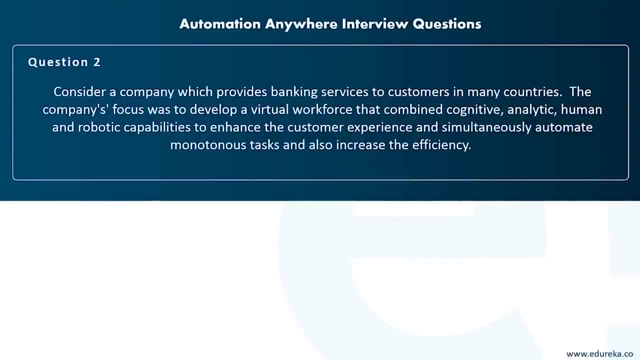 Now, moving on to the next scenario. Let's consider a scenario of a company which provides banking services to customers in many countries. Now, the company's main focus is to develop virtual workforce that combines cognitive, analytic, human and robotic capabilities to enhance the customer experience and simultaneously, 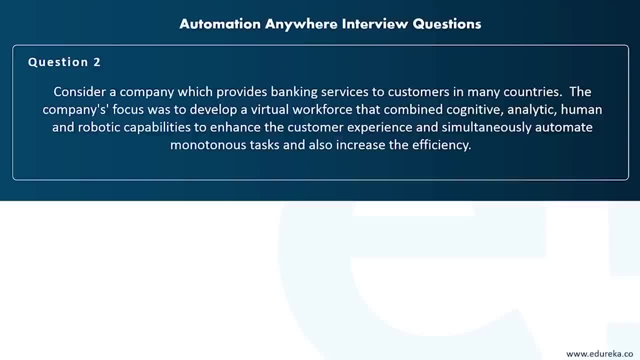 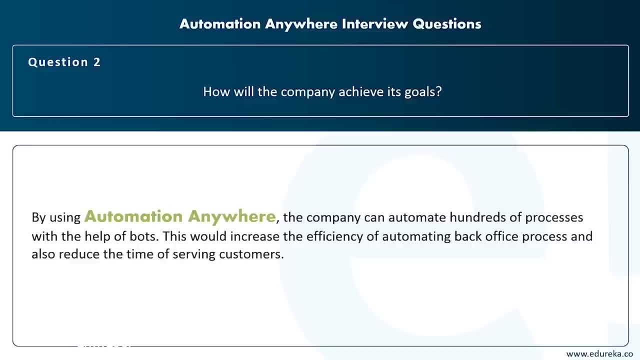 automate monitoring starts and also increase the efficiency. Now, how do you think will the company achieve its goals? Well, the answer to this question is obviously by using an RPA tool and I would say, by using automation anywhere. So, by using automation anywhere the company can automate. 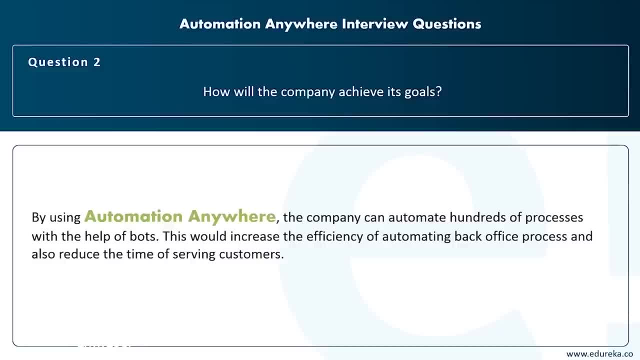 hundreds of processes with the help of both. this would increase the efficiency of automation, Automating back-office processes and also reduce the time for serving customers. This is how the company can achieve its goal. It's just that you know they have to use an RPA tool. 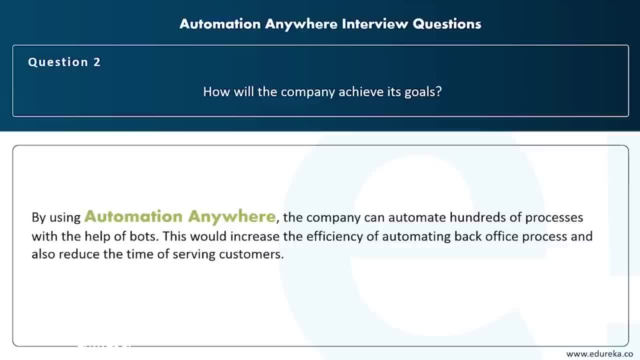 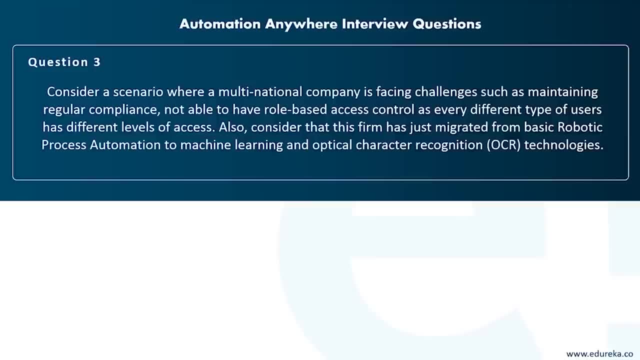 So here I would say: they can use automation anywhere, and then they can automate hundreds of tasks with the help of both. Now, moving on to the next question, consider the scenario where a multinational company is facing challenges such as maintaining regular compliance. as you know, they do not have. 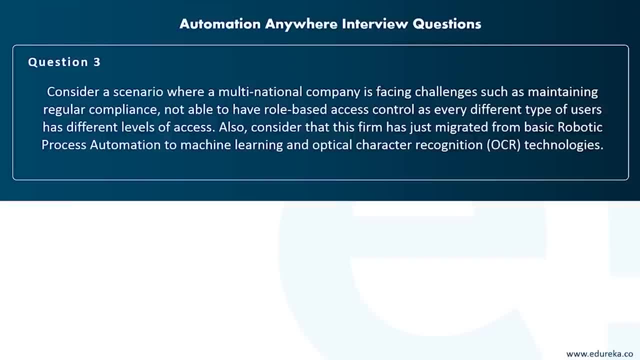 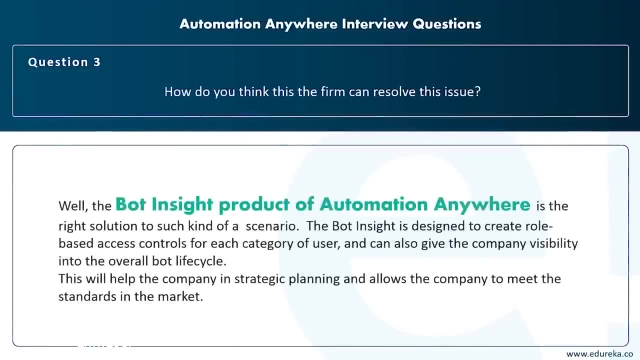 the ability to maintain the role based access control, as every different type of users have different levels of access. Now also consider the fact that you know the firm has just migrated from basic robotic process automation to machine learning and optical character recognition technologies. Now how do you think the firm can resolve this issue of 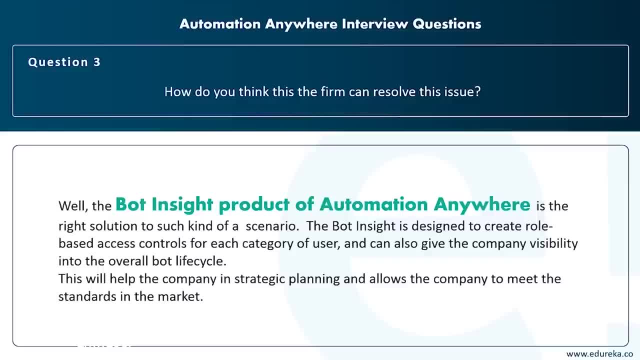 maintaining the regular compliance. Well, to resolve such issue, the company can use the bot inside product of automation anywhere. as you know, the bot inside is desired to create role based access controls for each category of user and can also give the company the visibility into overall bot life cycle. 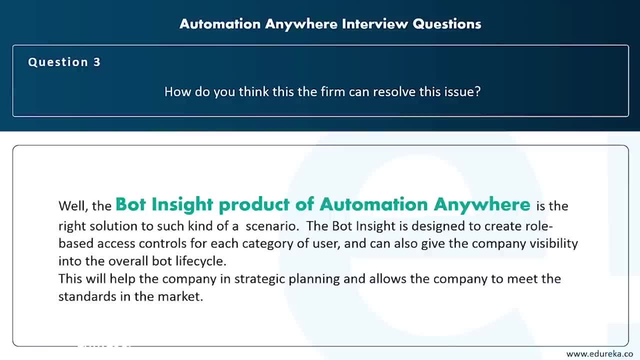 So with the help of this, the company can have strategic planning and also allow the company to meet standards in the market. So basically, the company can resolve this issue by using the bot inside from automation anywhere. Now moving on to the next scenario with this question. 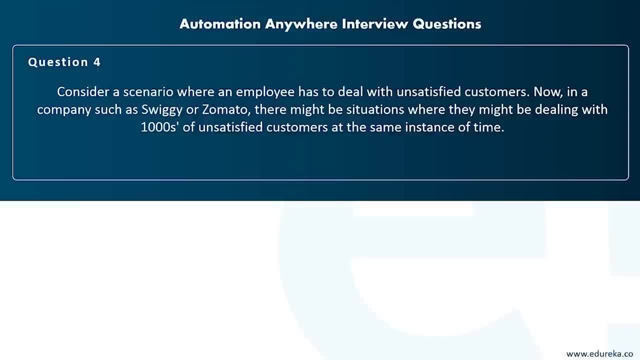 consider a scenario where an employee has to deal with unsatisfied customers. Now, in a company like you know, Swiggy or Zomato- there might be situations, you know, where the team of Swiggy and Zomato have to deal with hundreds of unsatisfied customers all over. 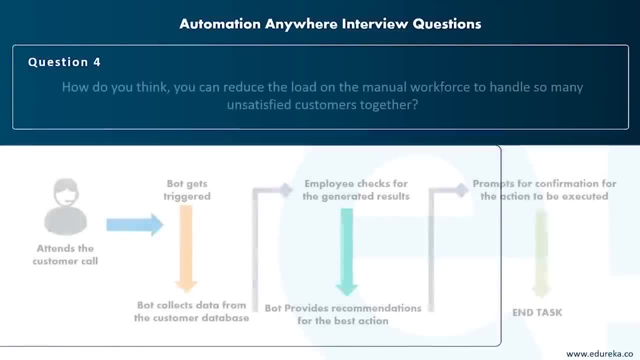 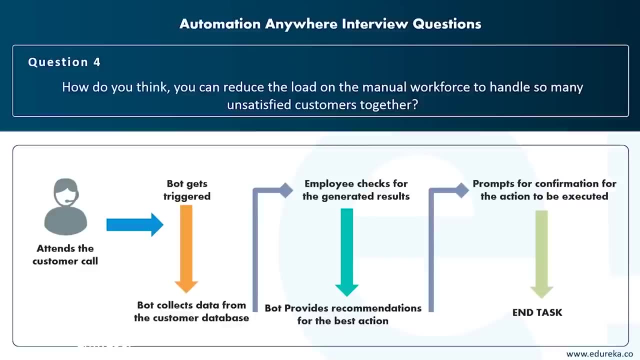 the world at same instance of time. Now how do you think the company can reduce the load of manual workforce to handle so many unsatisfied customers together? Well, to reduce the load of manual workforce you have to design bots in automation. anywhere to suggest questions. 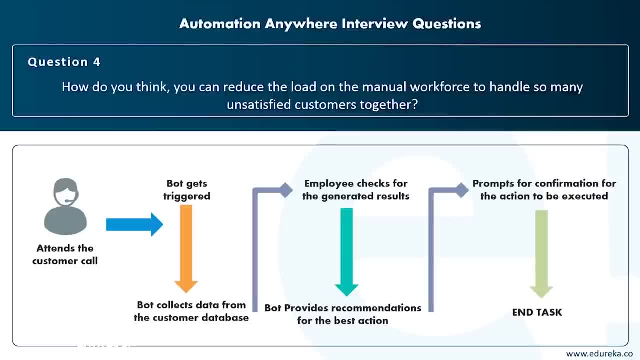 for an agent which can be asked to the customer and also gather information simultaneously. So with the help of cognitive capabilities, the bot can then further give recommendations for the next best actions to be taken. So in such a way, the bot can make sure that you know the. 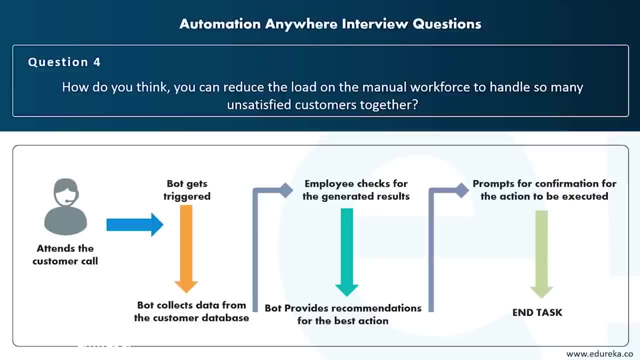 employee provides a better service and can also keep the interaction with the customer aligned To the guidelines of the company. So it's really simple, guys. What they have to simply do is so they have to design bots and automation anyway in such a way that you know the bot can. 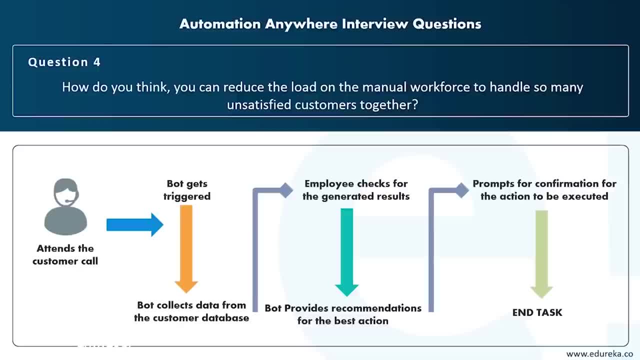 suggest questions for the agent and also gather the information from the customer right. So, for example, the delivery is getting too late. So the reasons could be either the delivery boy is not getting allotted or you know it's raining outside and the network 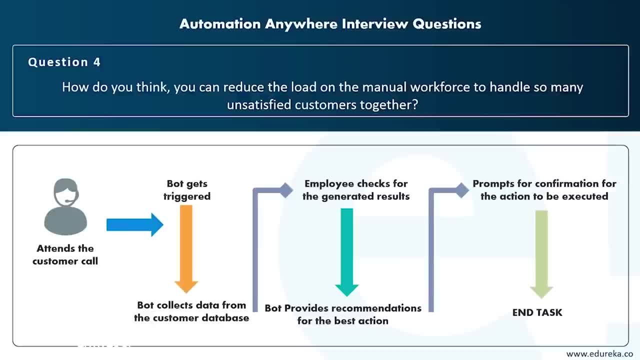 is a problem, or the reason could be that you know the customer cannot contact the delivery boy, and so on, right, So in such a scenario the bot should be intelligent enough in such a way that you know it can suggest the apt questions to. 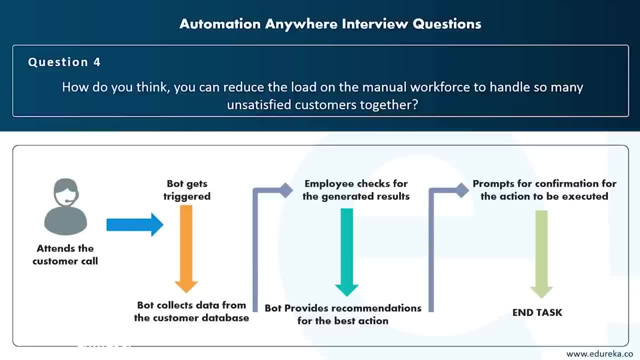 the agent. So you can refer to the flow chart that you can see in my screen so that you understand how, with the help of automation anyway, you can reduce the load of manual work post. So basically, as the customer attends to call, the bots gets. 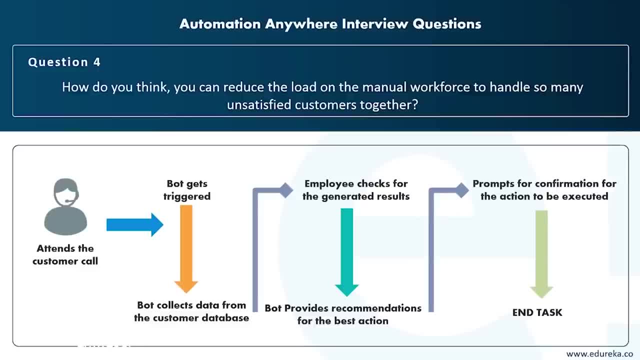 triggered and then the bot collects data from the customer database. Once the data is collected from the previous customer database, the employee checks for the generated results and then the board provides recommendations for the best actions. So, basically, based on the previous customer data and the 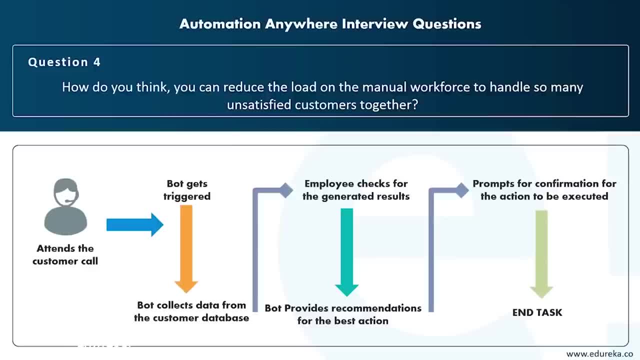 what the customer is saying presently. the board provides recommendations for the best actions and then prompts for a confirmation for the action to be executed or not. If the action is to be executed, then the agent takes over that question and passes on to the customer. and then that's how. 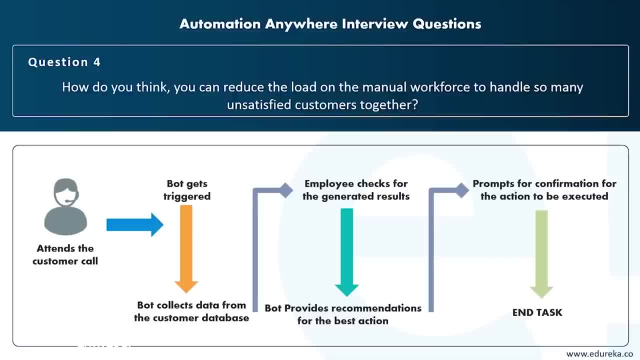 the conversation keeps on going. So that's how the task ends, also, guys. So guys. this is how you know you can reduce the load on manual workforce to handle many unsatisfied customers together. Now let's move forward with our next question. 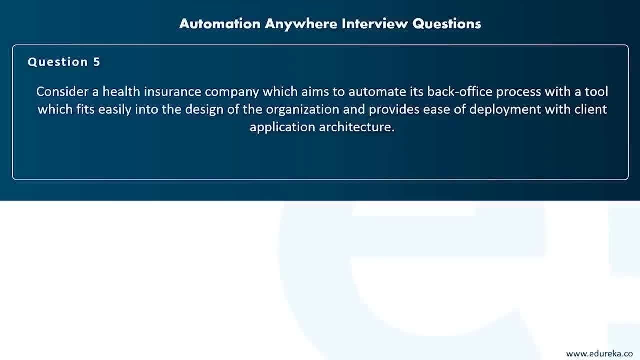 Now consider a health insurance company which aims to automate its back-office processes with a tool which fits easily into the design of organization and provides an ease of deployment with the client application architecture. Now, how do you think the company can automate its back office process with the help of the tool? 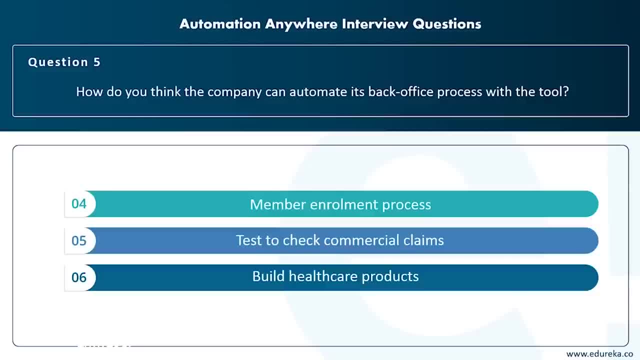 Well, according to me, a health insurance company must focus on automating mainly three tasks, that is, the member enrollment process, the test to check commercial claims and build healthcare products. coming to the member enrollment process, If previously you know, if you do not automate this task. 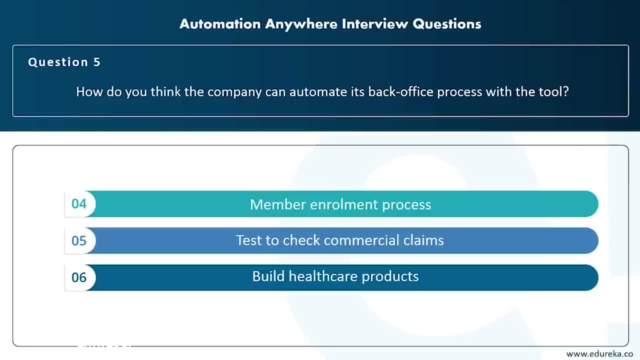 then 90% of the member enrollment data had to be manually entered into n different product lines, toggling between various number of applications. Now this could be obviously simplified with the help of automation anywhere by implementing a two-step solution, that is, converting the XML data into an electronic application. 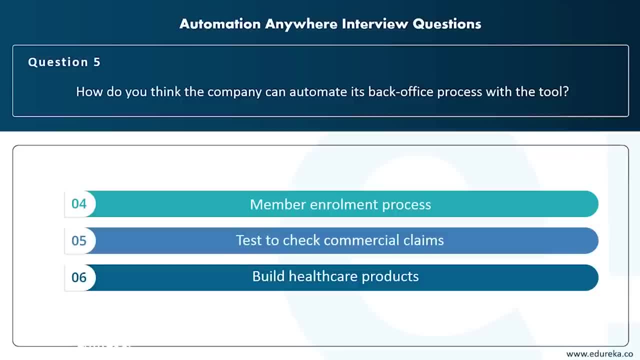 and then enabling the data entry from the electronic enrollment applications into the system. Coming to the test to check commercial claims. the test to check commercial claims can be a very tedious task If, obviously, if it doesn't get automated. so it can be basically. 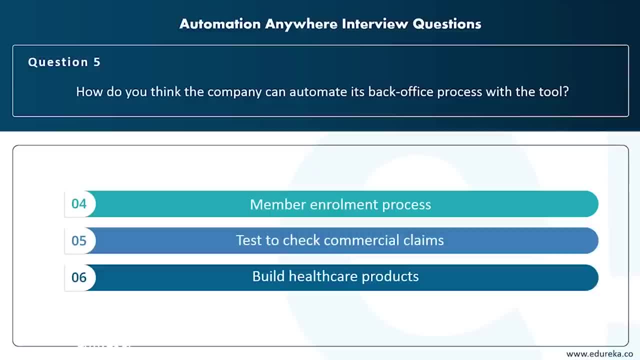 automated in two phases, that is, the first phase is to automate the screen capture process and the second phase is to automate the testing process of the claim. and finally, coming to the build healthcare products. The process of building a package under a predefined insurance plan can be highly time-consuming, taking up to 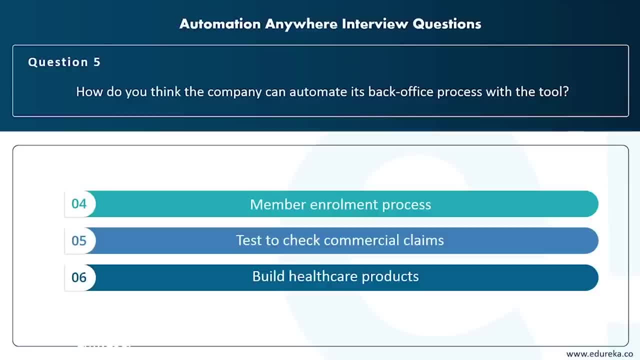 the maximum time for building an individual package. Now, automation anywhere can automate this process by collecting all the required information from various spreadsheets and then to validate the collected informations. The bots can match the extracted information to the business rules and once if it is validated, then they can. 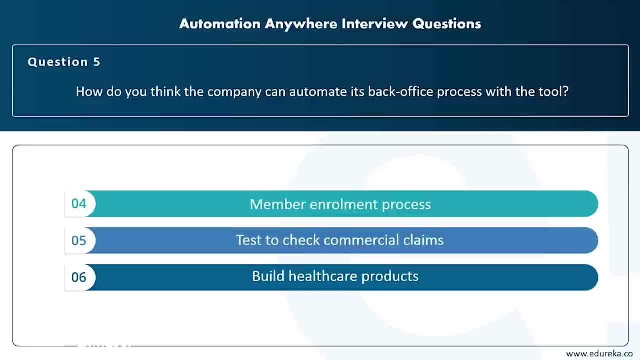 enter the details into the application and, finally, the application can be updated, right? So, guys, these are the mainly three processes that can be automated in the health insurance company and thus reduce the manual workforce and also, you know, automate maximum of its back-office processes. 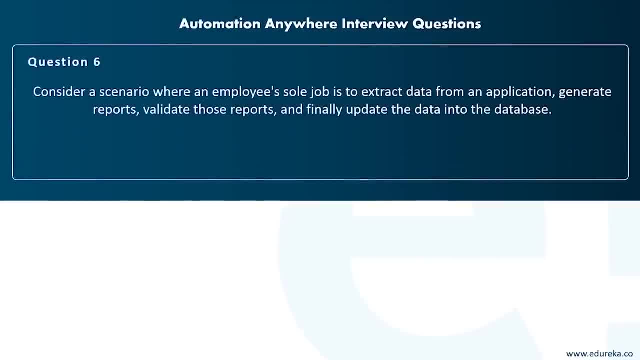 Now moving on to the next question, that is, consider a scenario where an employee's sole job is to extract data from an application, generate reports, validate this report and finally update the data into the database. Now the question is: can you elaborate on the process of 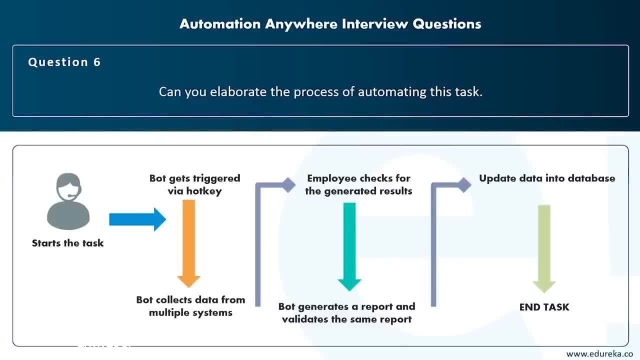 automating this task. Well, the process of automating this task is really simple. as you can see on my screen, an employee can trigger a board via hotkey to collect data from multiple systems, Then the employee can check for the generated results and then 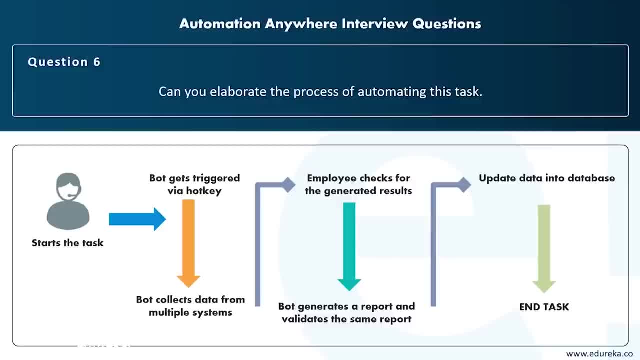 finally generate a report. after validating the report, you can update the data into the database and this will end your task right. So this is a basic process of how you can automate this task. that is basically, an employee can just start the task and then trigger a board. 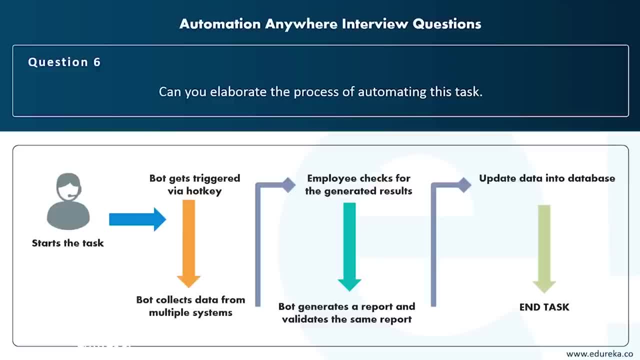 By a hotkey. after that, the board can collect information from multiple systems, check for the generated results and then bot will finally generate a report and validate the same report and then finally update the data into the database. right? So this is how you know you can automate simple to complex. 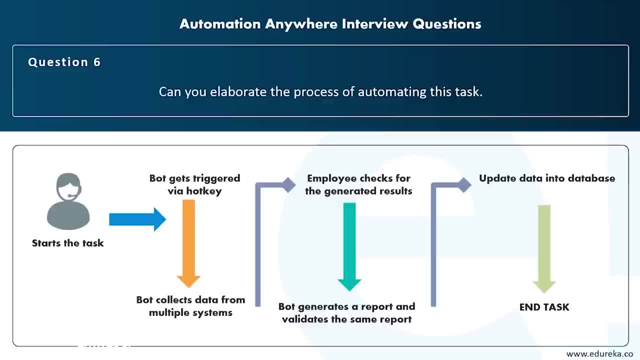 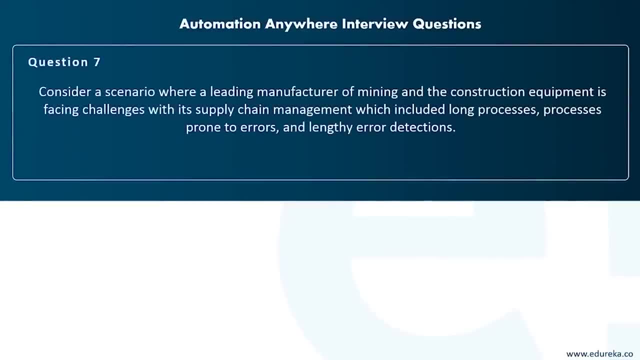 tasks and make sure that you know employees can use their mind in a better way for a company. Now moving forward with our next question, that is, consider a scenario where a leading manufacturer of the mining and the construction equipment is facing challenges with its supply chain management. 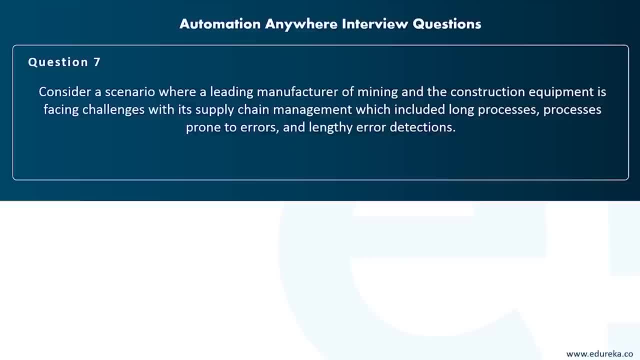 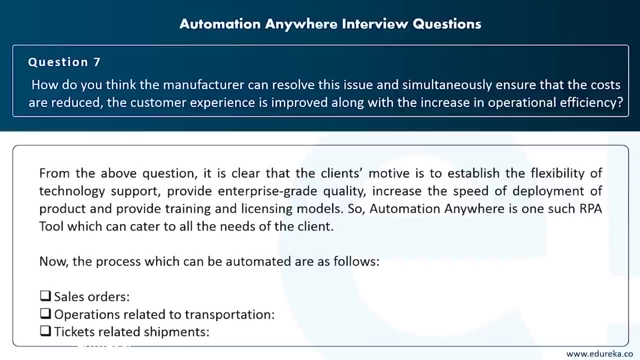 which includes long processes, processes prone to errors, and also lend the error detections. Now, how do you think the manufacturer can resolve this issue and simultaneously ensure that the costs are reduced, the customer experience is improved, along with the operational efficiency to increase? well, from the question. 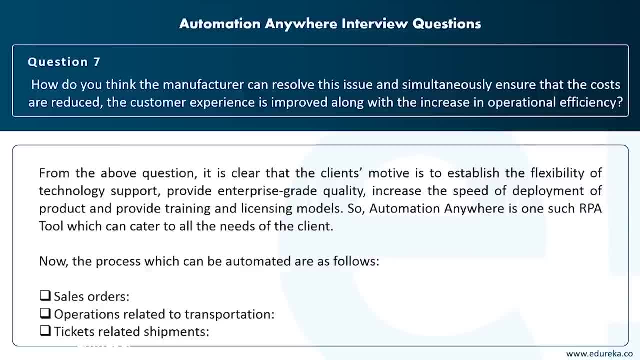 It's clear that you know the client's motive is to establish the flexibility of technology support, provide Enterprise great quality, increase the speed of deployment of product and also provide training and licensing models. So automation anywhere is One such RPA tool which can cater all the needs of the client. 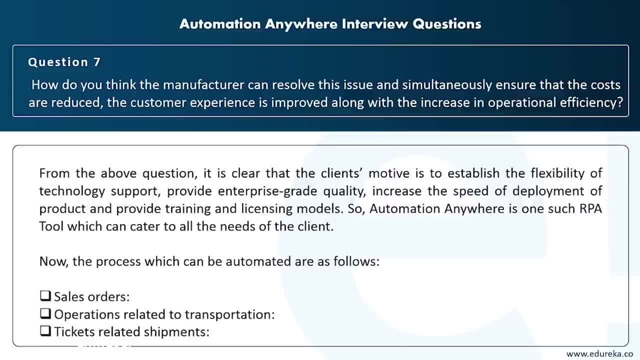 So the process which can be automated is basically the sales order process, the operations related to the transportation and also tickets related to shipments. So, talking about the sales orders, the boards can automate the process of searching the sales order and system check all the details related to the orders, updated data into the 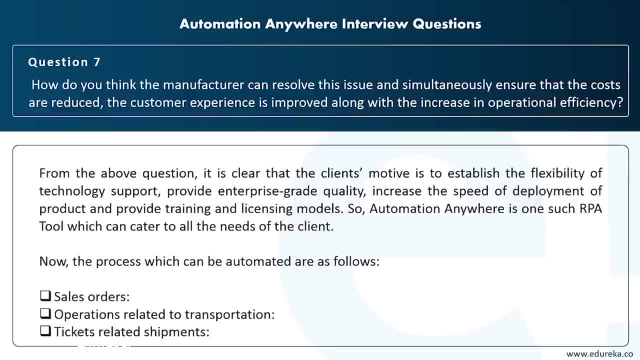 application and also notify the user that whether the task is completed or not. Similarly, operations related to the transportations, the activities such as identifying recent failures, extracting the reason for failure and finally notifying the related teams via emails to resolve- can be automated using various activities in. 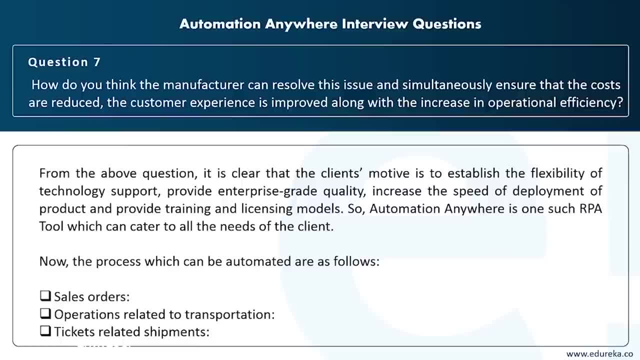 automation anywhere. and finally, coming to the tickets related to shipments, The parts can automatically create a ticket related to the customer query and, once the ticket has been resolved and email, can be sent to the respective client, right? So, guys, these are the processes which can be automated, that is. 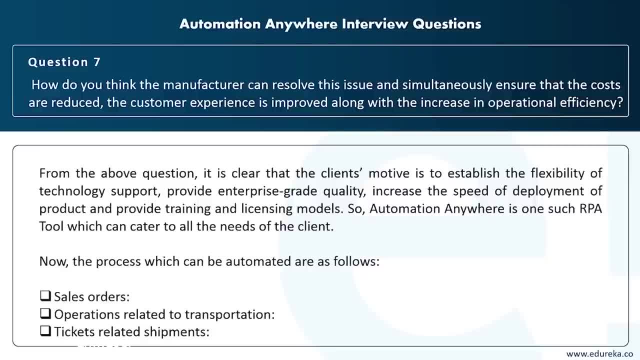 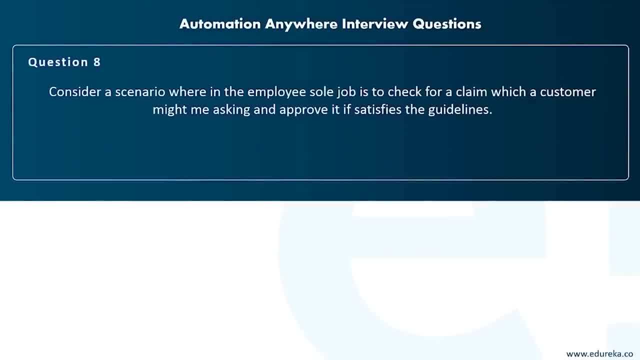 the sales order, the operations related to transportation and tickets related to shipments. Now, moving on to the next question, that is considered a scenario wherein the employee's sole job is to check for a claim which a customer might be asking, and approve it if it satisfies the guidelines. 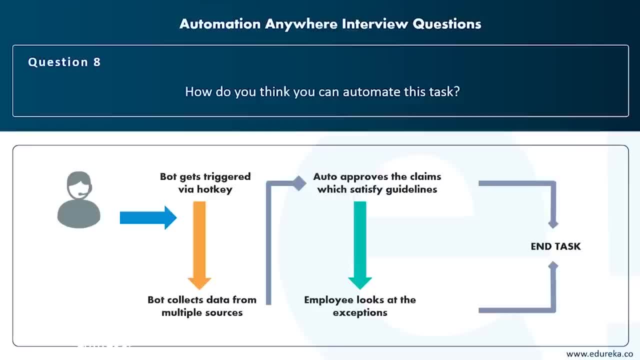 Now, how do you think this task can be automated? Well, you can definitely automate this task by using the automation anywhere client, so you can create a workflow. as you can see on my screen, an employee can trigger a boat via hotkey to collect data from multiple sources. after that, the system 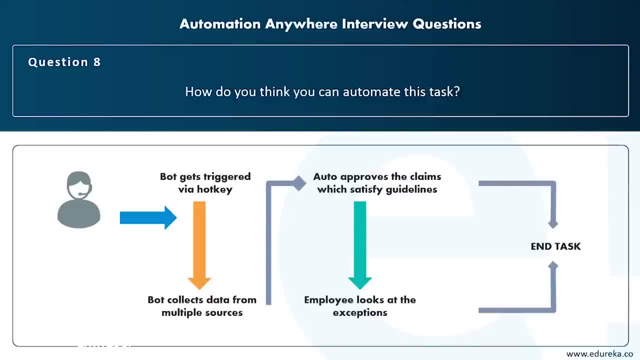 will auto approve the claims which satisfy the guidelines and later on the employee can look for an exceptions found and resolve the same. So if there are no exceptions found, then the task end or, you know, if all the claims are approved and also the task would. 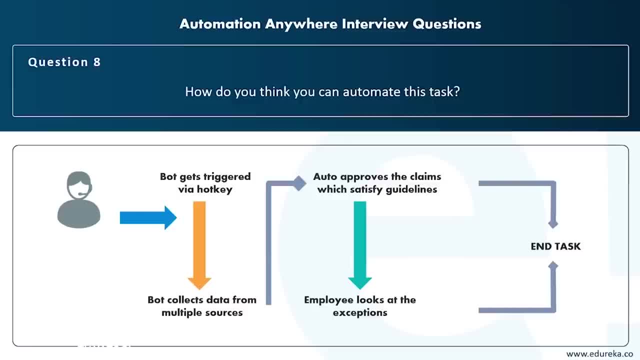 end right. So basically the workflow is, you know the employee has to trigger a boat via hotkey and then the bot collects the information from multiple sources. after that the bot basically make sure that you know the claims are auto approved which satisfy the guidelines, and then the claims. 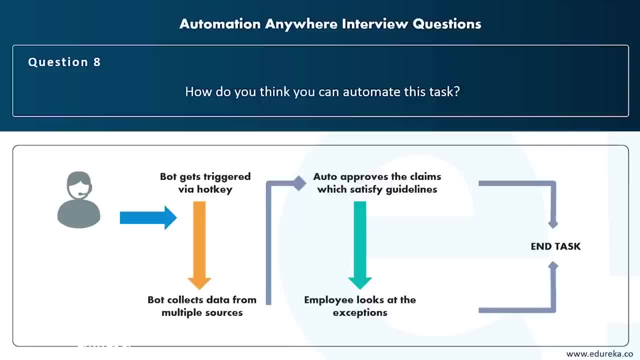 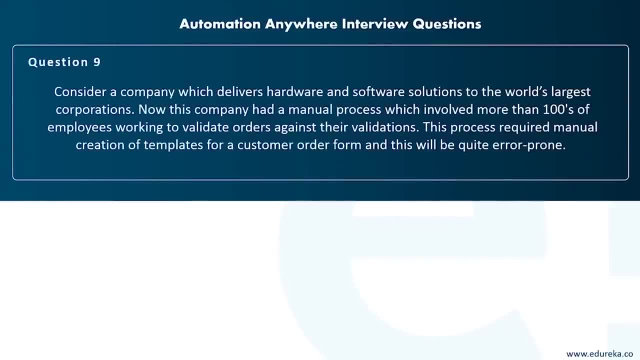 which have an exceptions. the employee would look into those exceptions and resolve the same. So that's how you can just automate this task. Now, moving on to the next scenario, that is considered a scenario where a company delivers hardware and software solutions to the world's largest corporations. 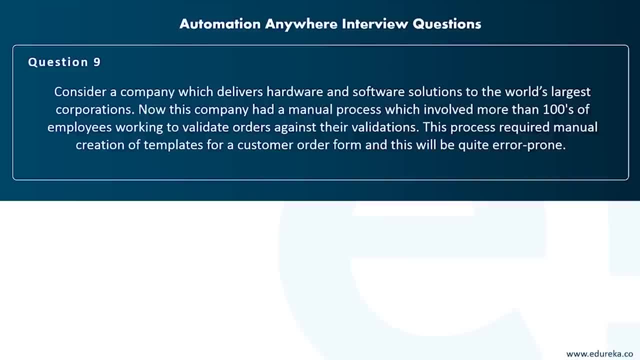 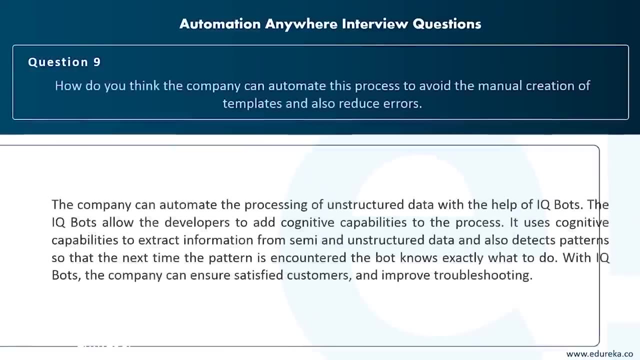 Now this company had a manual process which involved more than hundreds of employees to validate orders against their validations. This process obviously required manual creation of templates for a customer order form and obviously creation of templates manually is obviously quite error-prone right Now. how do you think the company can automate this? 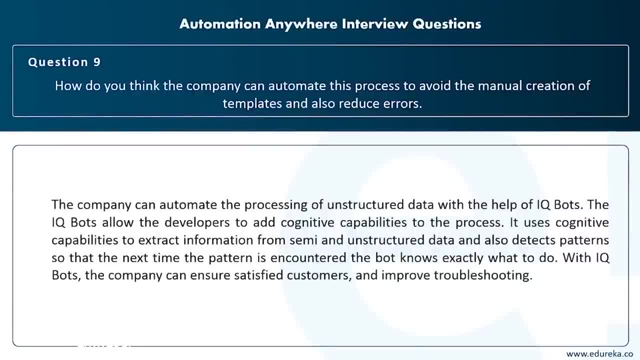 process, to avoid the manual creation of templates and all the also reduce errors. Well, the solution to this question is basically that you know the company can automate the processing of unstructured data with the help of IQ boards. So the IQ boards can allow the developers to add cognitive 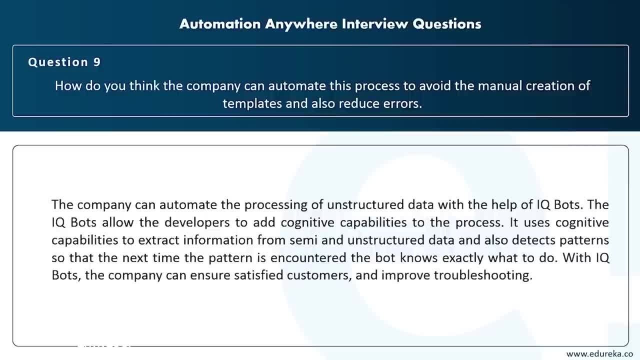 capabilities to the process, and then it uses the cognitive capabilities to extract information from semi and unstructured data and also detects patterns, so that the next time the pattern is encountered, the bot knows what exactly has to be done. So, with the help of IQ boards, the company can ensure that. 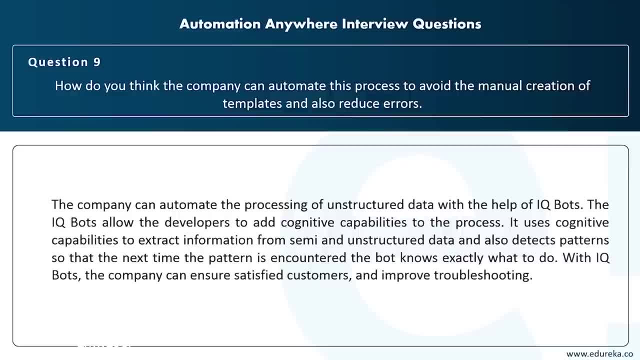 you know, it satisfies its customers and also improves the troubleshooting and reduces the manual creation of templates. So that's how a company can automate this process to avoid the manual creation of templates and reduce errors. Now moving on to the next scenario. Now consider a scenario where an organization offers a wide 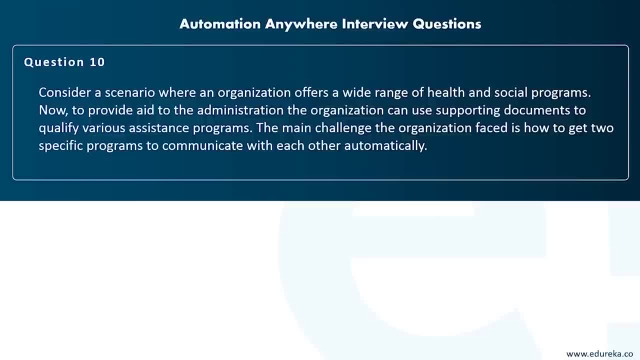 range of health and social programs. now, to provide aid to the administration, The organization can use supporting documents to qualify various assistance programs. Now the main challenge the organization faces is how to get to specific programs to communicate with each of the automatic. Now, obviously, if you think this has to be done without, 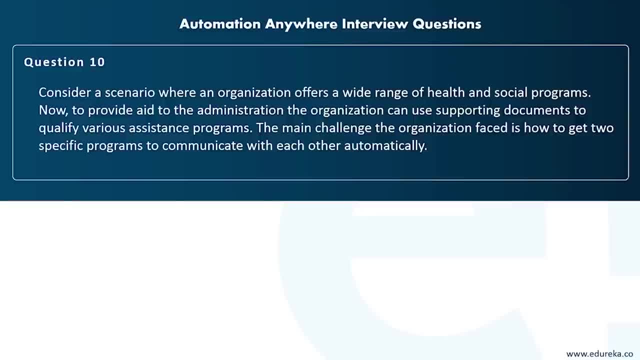 automation. then what would you do? An employee would take an information from relevant forms, look for the supporting documents in different system. after that, the employee would verify the information and provided to the applying individual. Now, obviously this task for hundreds of documents and for 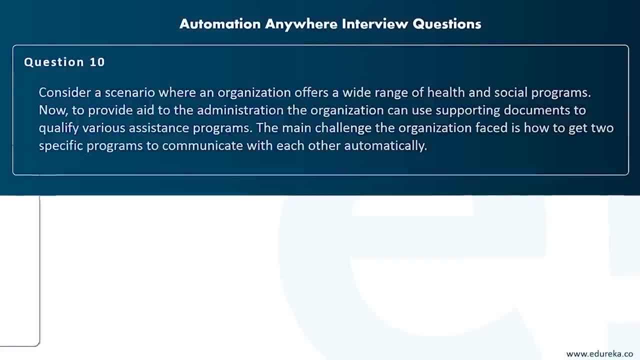 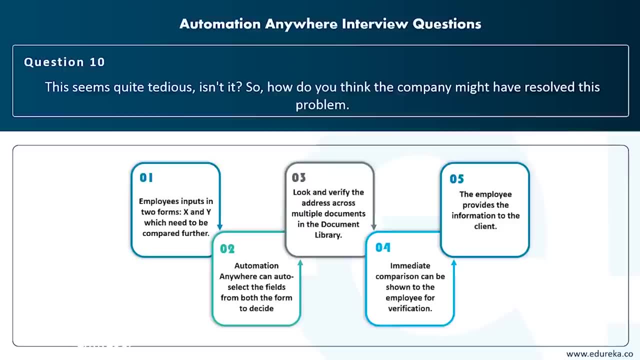 hundreds of customers seems tedious and time-taking also right. So how do you think the company might have resolved this issue? Well, with the help of automation, anywhere again, you can build up a solution to bridge the gap between the employees and the customers. 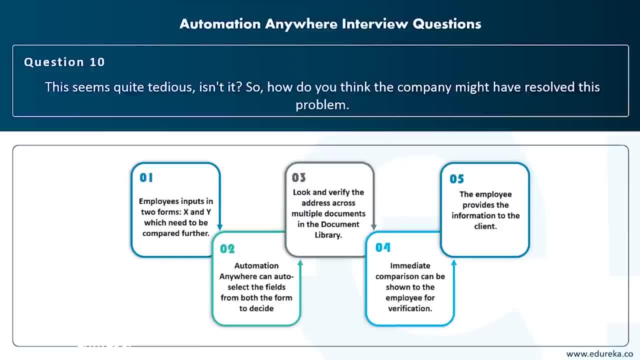 So an employee can get all the required information from the documents library and then launch the verification process with the help of hotkeys in automation anywhere After that. you can also design a workflow to open forms on the employee screen and identify the relevant documents gather. 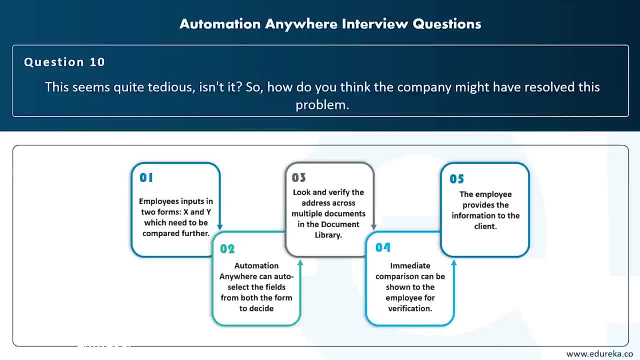 those documents from the document library for the employee, and then the employee can use this documents to provide the information to the clients. So, as you can see on my screen, this is basically the process workflow that you can use. So, for example, if an employee input 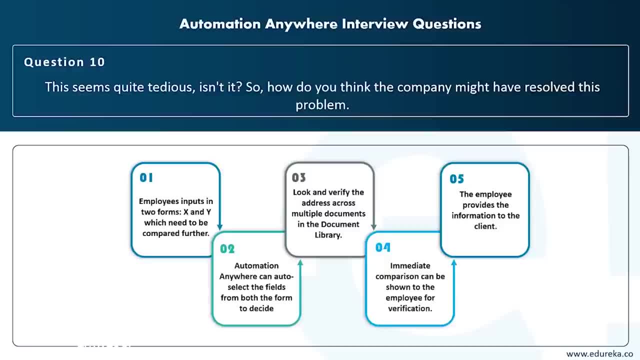 It's two forms, that is, X and Y, which needs to be compared. further automation anywhere can Auto select the fields from both the forms to decide and then look and verify the address across multiple documents in the document library. after the immediate comparison has been done, The immediate comparison can be shown to the employee for 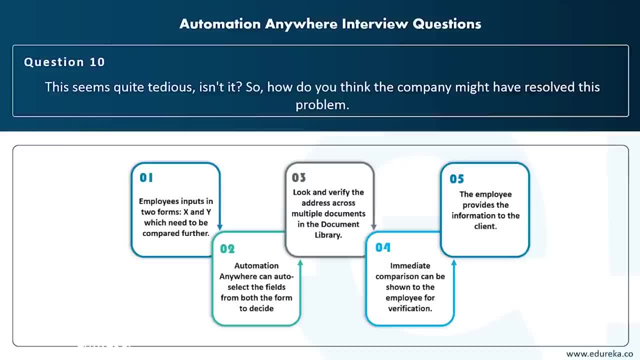 verification and then the employee can provide the information to the client. So, guys, this is the basic workflow of automating this particular task. So, guys, these were a few questions that were completely scenario based. Now, the next five questions in the section will basically: 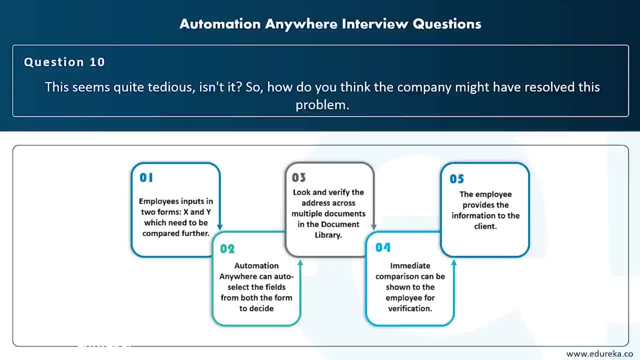 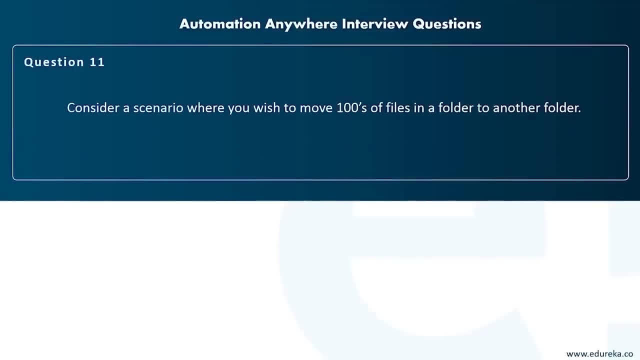 consider of scenarios where you know you can actually automate the task on the tool and show to the interviewer. So let's start with the first question over here, that is, consider the scenario in which you want to move hundred files in a folder to another folder. 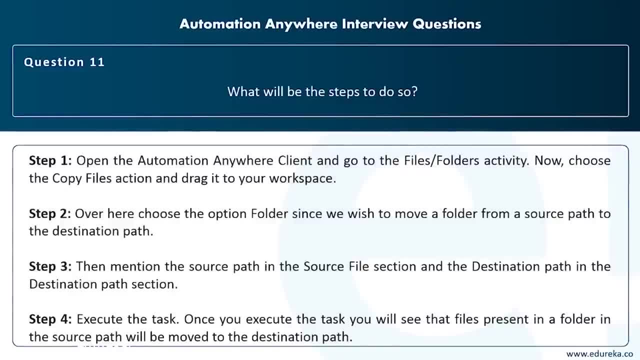 Now, what do you think the steps will be? Well, the steps will be basically to open an automation anywhere- client and then go to the files and folders activity. after that you have to choose the copy files action and drag it to your workspace. after that you have to choose the option. 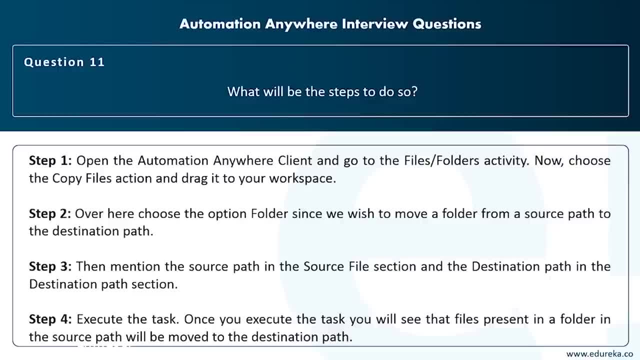 folder, since we want to move a folder from source part to the destination part. After that, you have to mention the source part in the source section and the destination part in the destination section. after that, what you simply have to do is you have to save your. 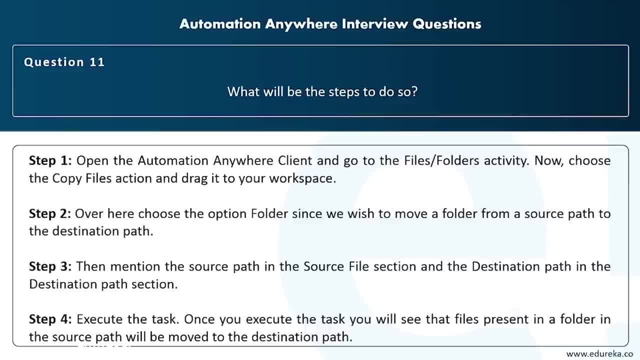 task and execute your task and you'll see that you know all the files present in the folder in the source destination will move to the destination folder. So let me just show you how that can be done. All right, so I'm going to open my automation anywhere. client. 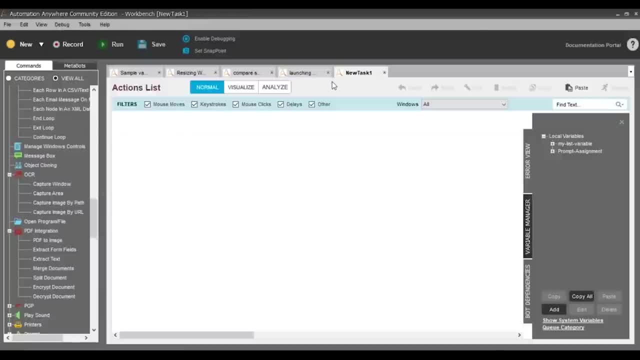 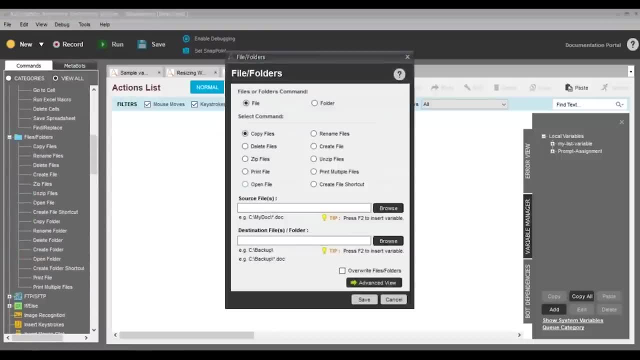 Now what I'm going to do is I'm going to open a new task. So let's open a new task. and now let's say: you know, we go to the files and folders section. Now I'm going to choose the option of copy files. 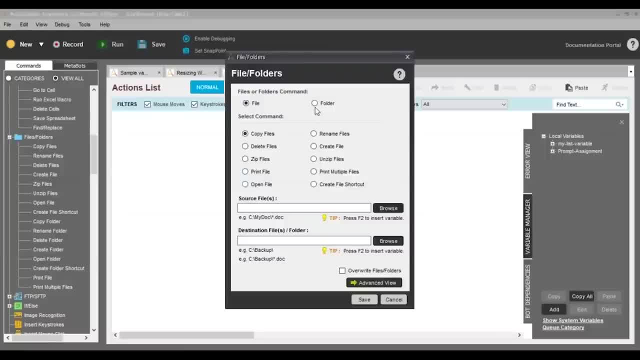 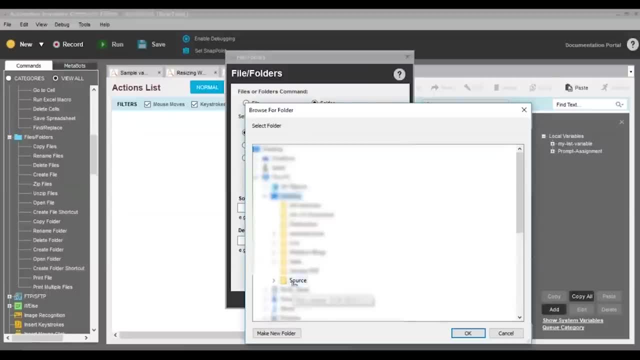 And then what I'm going to do is, in the files and folders command, I'm going to choose folder. So what I'm going to do is I want my complete source folder to move to the destination folder, right? So I'm going to browse for the source folder. 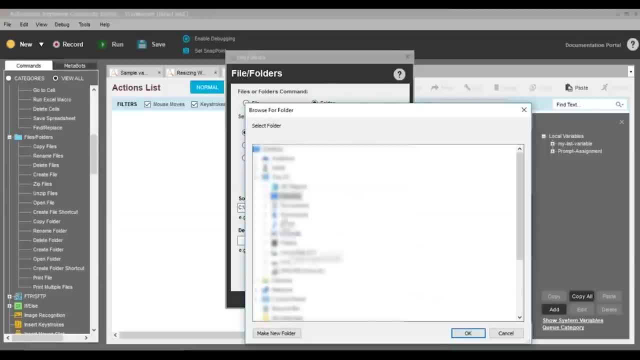 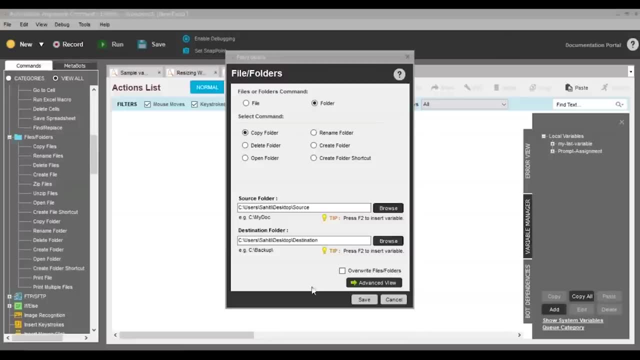 Similarly, I'm going to mention that the path of the destination folder. So let's just mention the path of the destination folder. So, as you can see on my screen, guys, this is the path to the source folder and the destination folder, and now I'll click on save. 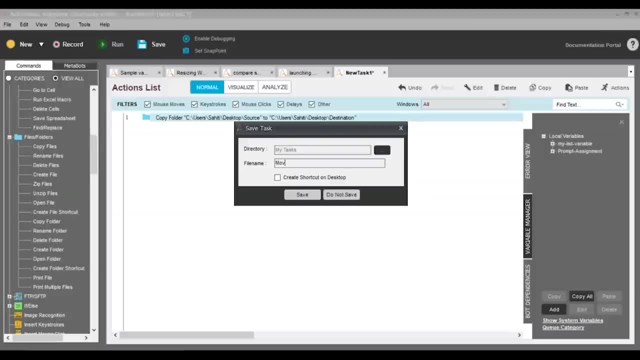 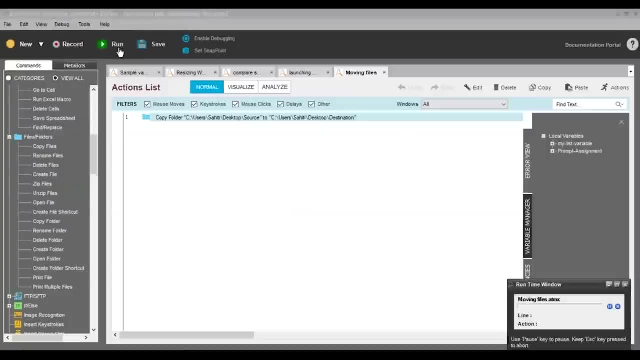 Once I click on save and I save my task- Let's say you know moving files- I just execute this particular task. So you can see that you know my task has been executed. now I'll just go to the destination folder and you can see that you. 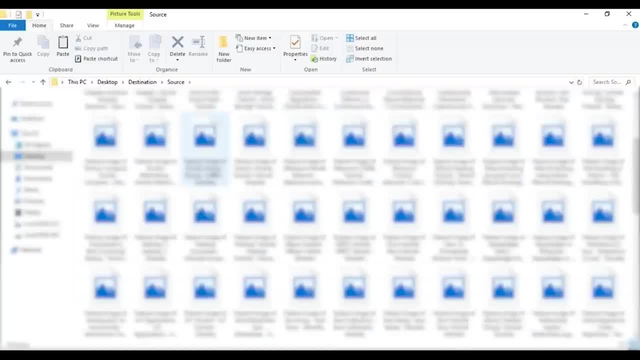 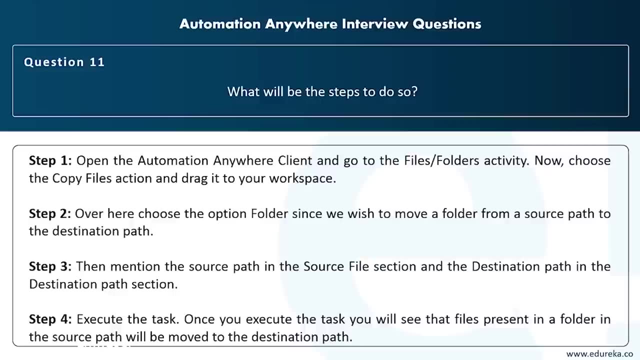 know you have a folder inside the destination folder- That is the source folder, and it has hundred files in it. So that's how, guys, you can move files from source folder to the destination folder. Well, these kind of questions are mainly asked to just check. 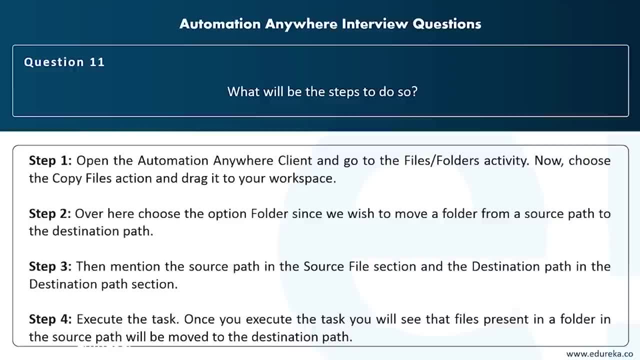 your experience with the tool. They can be either simple, Well, or they can be complex. It's completely based on how good you're with the tool and how many activities or commands that you have an understanding with right now. consider the scenario wherein you wish to automate. 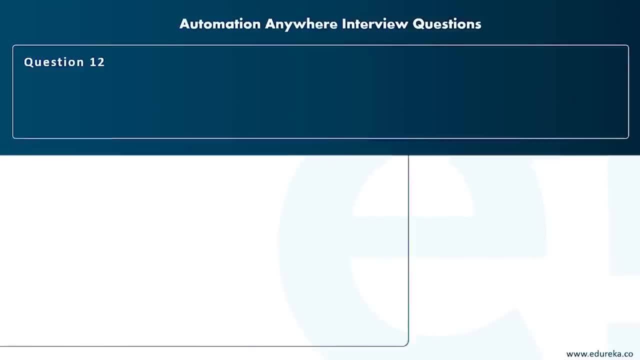 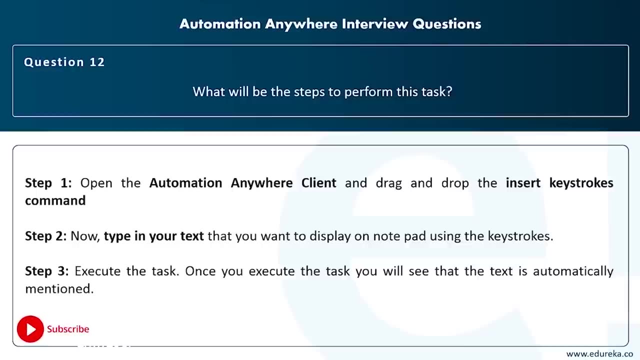 the task of writing text into a notepad file. Now, what do you think will be the steps to automate this task? Well, the steps are really simple. You first have to open the notepad window and then you have to drag and drop the insert keystrokes command into your 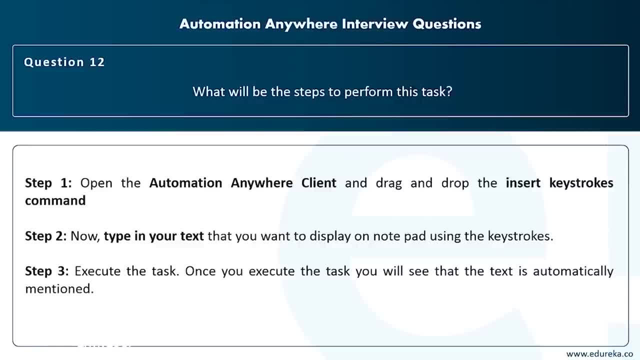 workspace. after that, What you have to do is you'll have to just select the window- that is basically a notepad window- and then you'll have to mention what text you want to mention With which keystrokes. right, So what I'm going to do is I'm going to just open my automation. 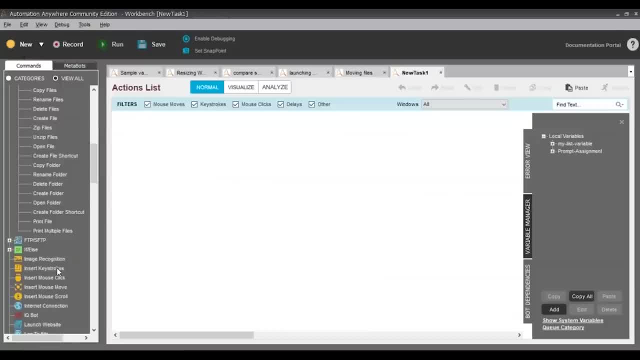 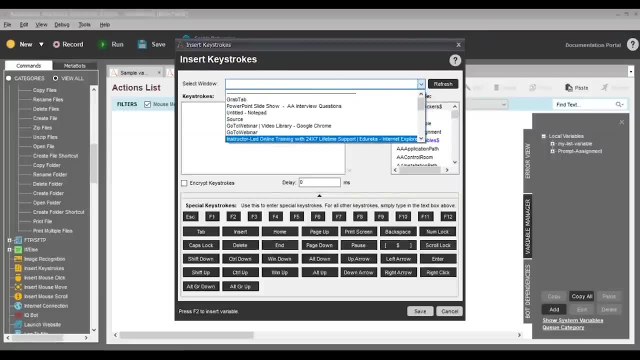 anywhere. client again, and let's go for a new task now over here. I'm just going to drag and drop and insert keystrokes command now over here. I have to select a window, right, So I already I have opened a notepad file over here. 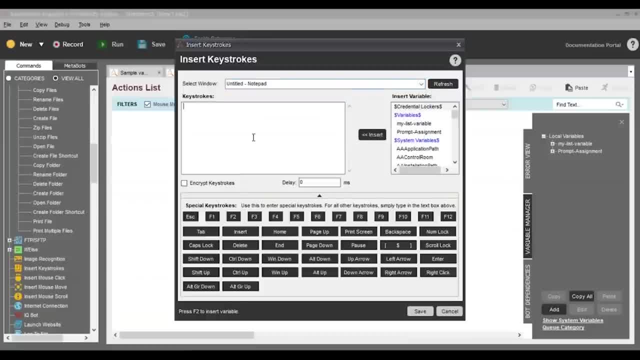 So I'm just going to, you know, select that particular window, and then I'm going to mention the text that I want to mention with you know, maybe two lines, you know, with some letters in caps lock, right. So for that let's say, you know we mentioned hello all, and then 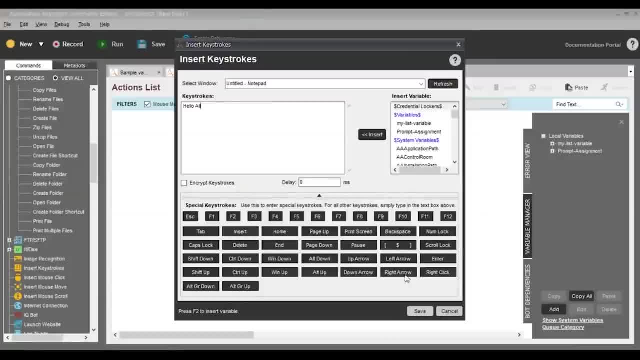 we want the next sentence to come in the next line, So for that we'll mention enter, So I'll type in enter over here. after that What I'll do is I'll say welcome to, and then I want Edureka to be in caps lock. 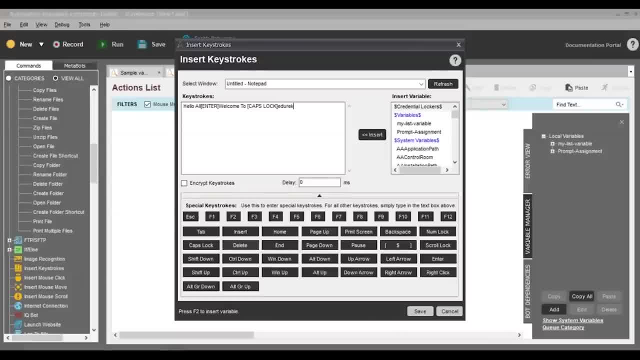 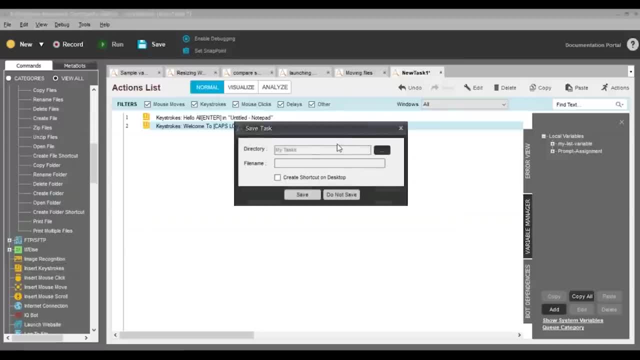 So I'll just mention caps lock and then I'll mention Edureka, right, And then what I'll do is I'll click on save. now, Once I click on save, I'll just save my task again. Let's say, you know writing text, click on save and then I'll click. 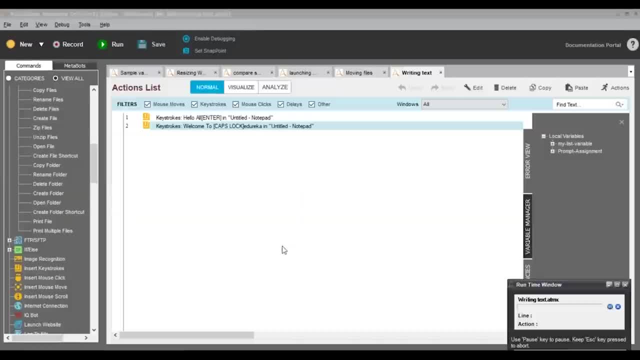 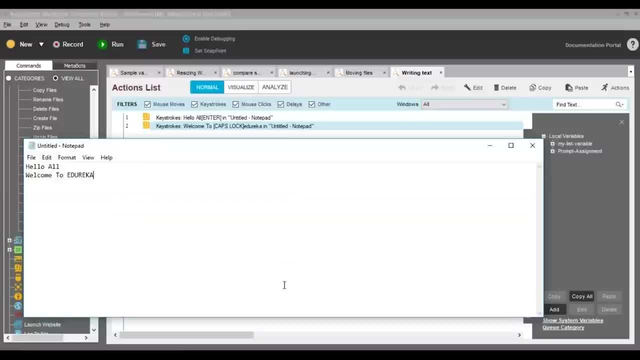 on run. Now, once I click on run, you can clearly see that you know automatically. hello all and welcome to Edureka. have come in two different lines and Edureka has come in caps lock right. So that's how you can automate the task of writing into a notepad. 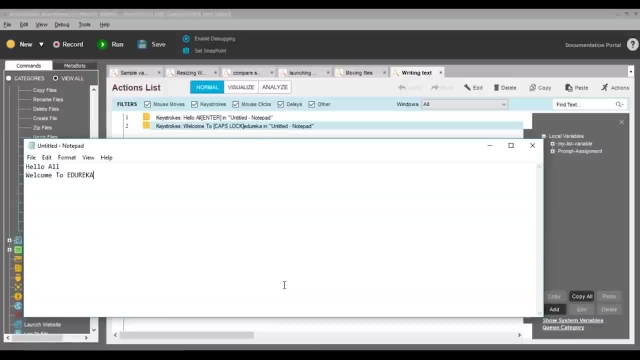 file. Well, this was really a two-line demo that I had showed you, but in industry level, This automation is really used to automate the task of writing text into different files, and the text could be humongous, right. So that's how it is used in Industries. 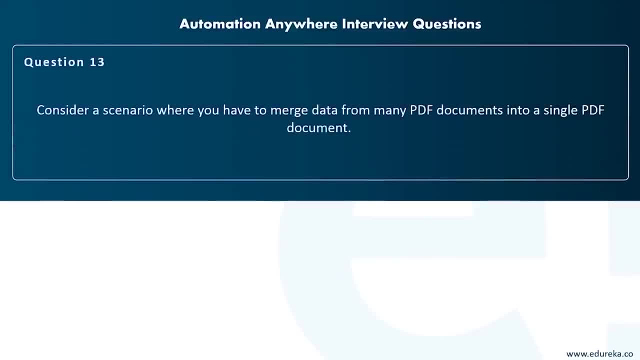 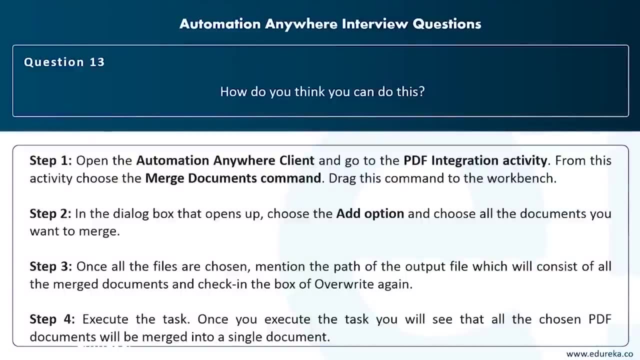 Now let's move forward with our next scenario. That is considered a scenario where you have to merge the data from many PDF documents into a single PDF document. Now, how do you think you can do this? Well, to merge the data from many PDF documents into a single. 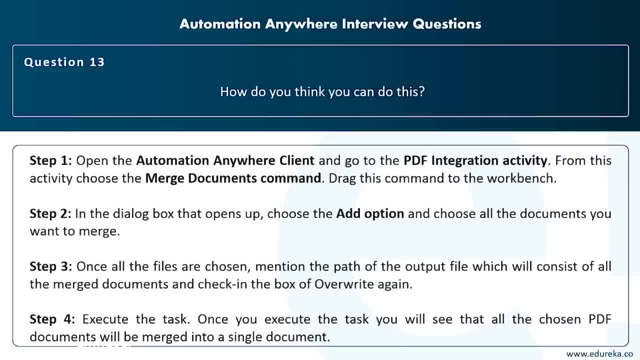 PDF document. what you can simply use is you have to use the PDF integration activity and from this activity you have to use the merge documents command. So, basically, you have to drag the merge documents command and in the dialog box that opens up you have to choose the add. 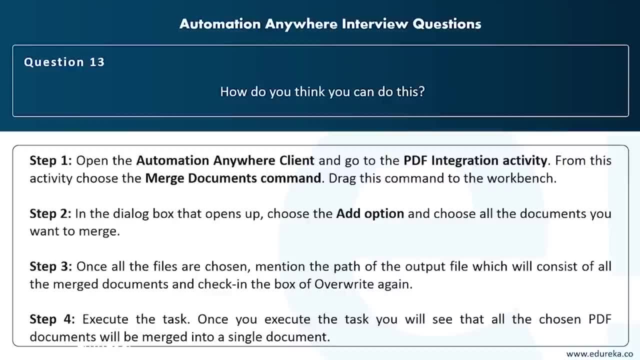 option and choose all the documents that you want to merge. Now, once all the files are chosen, you have to mention the date of the output file, which will consist of all the merge documents, and then you can just check in the box if you. 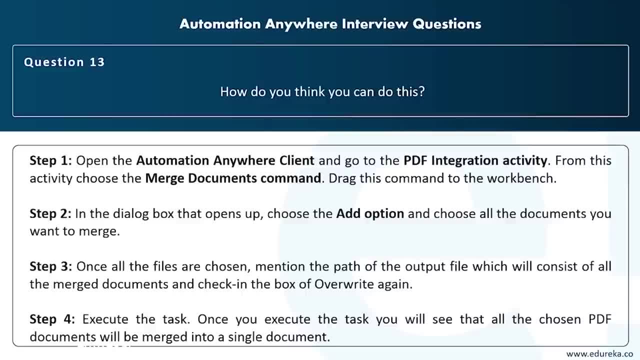 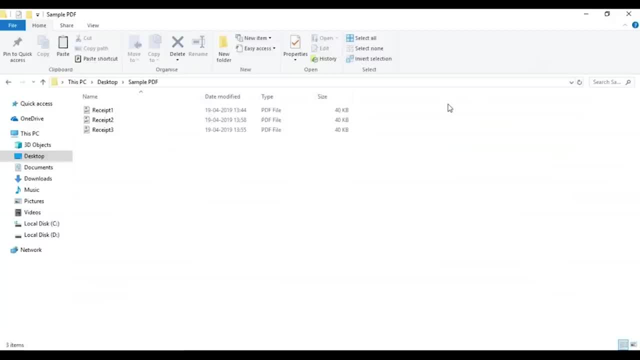 want to just overwrite the file again. So let's just do that. So I'm going to shift back to my Automation Anywhere client and then I'm going to create a new task Now over here. what I'm going to do is: let me just show you which 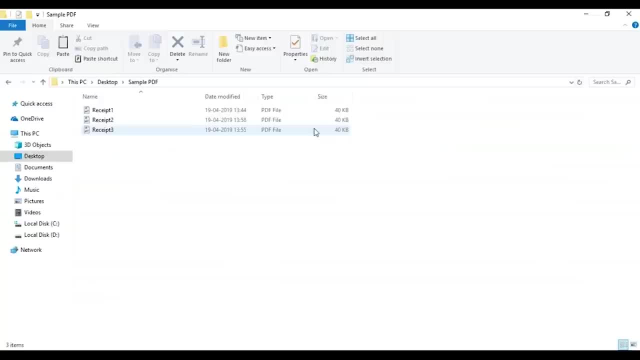 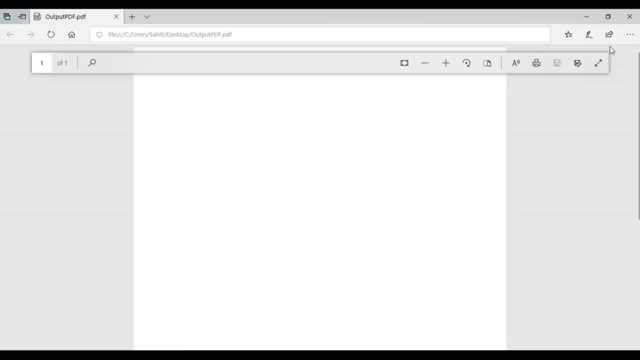 PDF files I'm going to merge. So, as you can see, in my sample PDF folder I have three PDFs, right, That is, receive one, receive two and receive three. So I'm going to merge all these three documents and then put it. 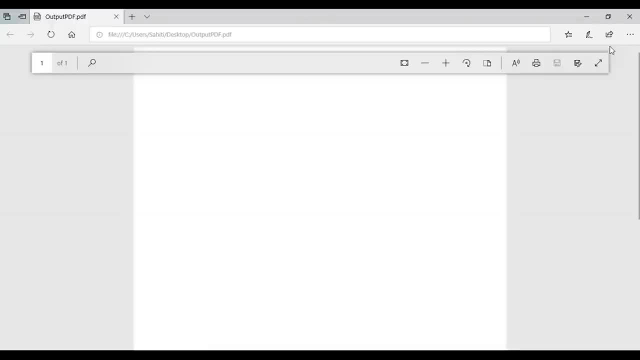 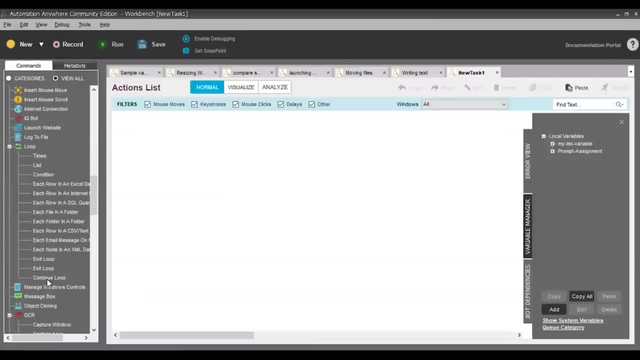 into the output PDF file. So this is basically my sample output PDF file in which I'm going to merge all the documents into right. So I'm going to shift back to my Automation Anywhere client. Now I'm going to drag and drop the PDF integration command. 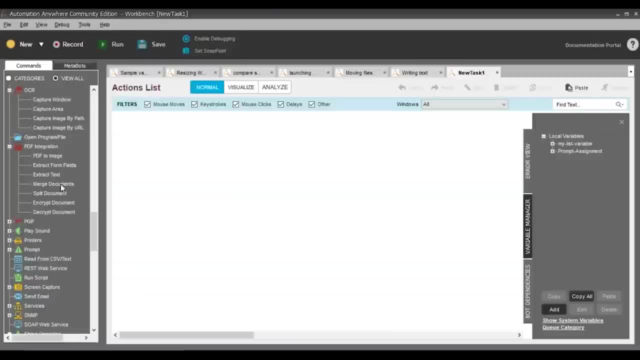 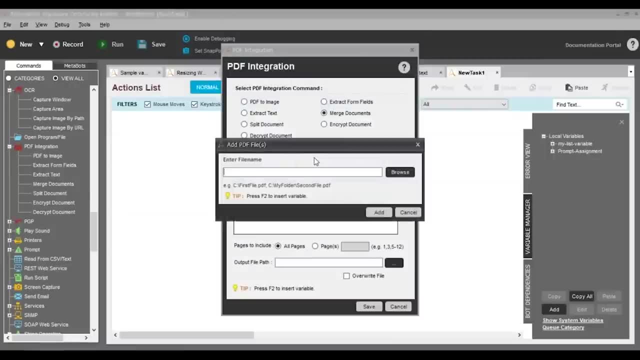 So let me just search for PDF integration command and over here I'm going to drag and drop the merge documents command. Now in the merge documents command I'm going to choose the merge documents and then I'm going to choose for add. So when I say add, so basically over here I have to mention all. 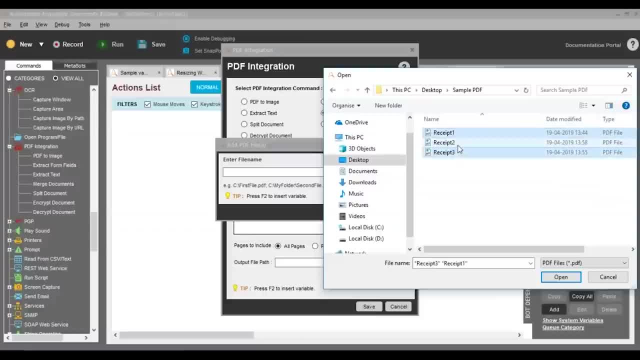 the files that I want to be merged. So in the sample PDF file I'm going to merge all these three files, right? So we'll have to select in an order to get it in an order and then I'll click on add. 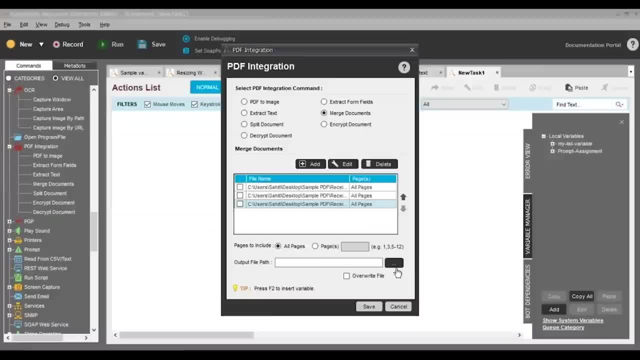 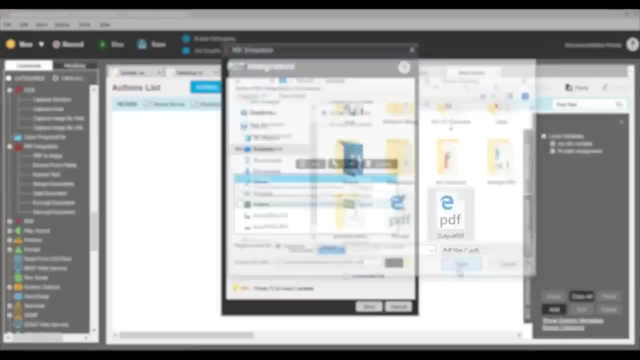 So you can see that you know my all the three PDFs have been added and in the output file path I'll mention the output file. So basically I'll go for browse again, go for desktop and then mention output PDF and then I'll check in, overwrite file, right? 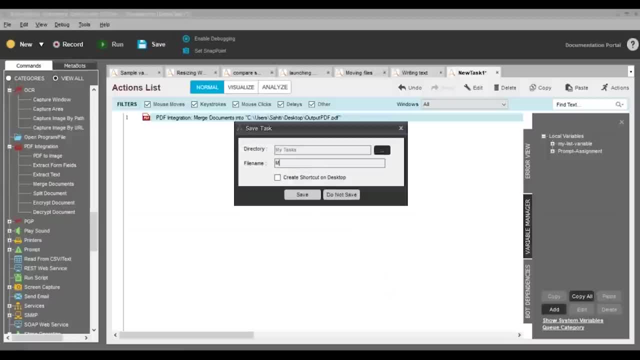 I'll then click on save the save the stars. Let's say you know, merge PDF. I'll click on save over here again and then click on run So you can see that you know my task is getting automated right. 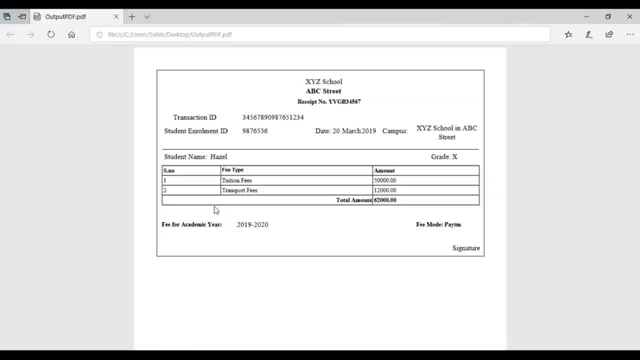 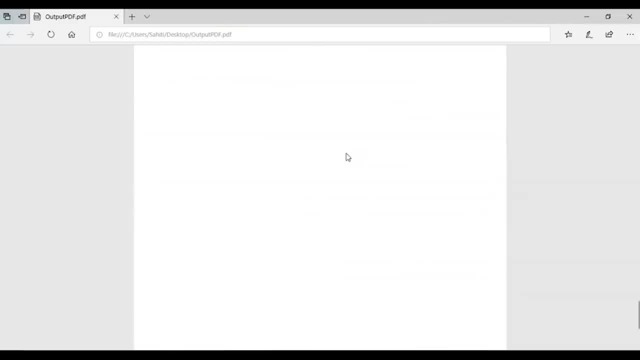 So you can see that in our task has been executed. Now Let's just open that PDF file so that you understand how our documents have been merged. So, as you can see, these are my different PDFs that have been merged together. So that's how, guys, you can merge PDF documents. 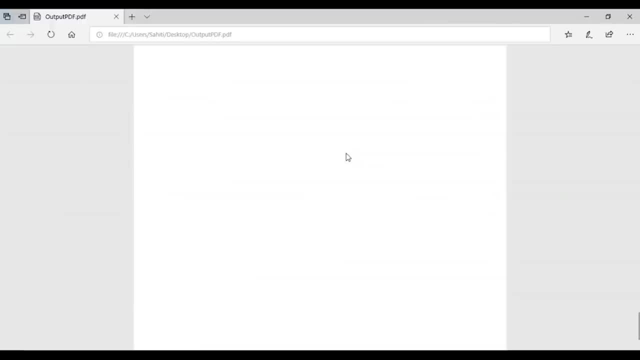 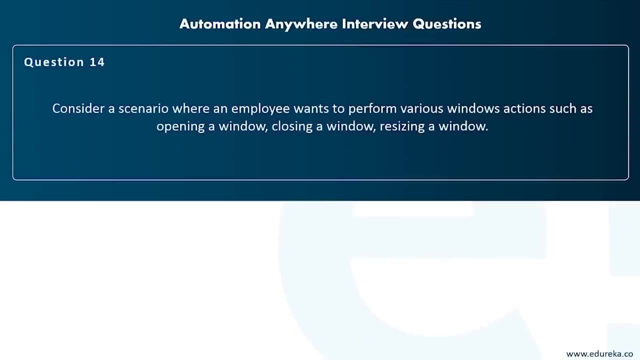 So this was just for three PDF documents, where you can merge any number of PDF documents that you wish to. now, moving on to the next question, that is considered a scenario where an employee wants to perform various window actions, such as opening a window, closing a window or resizing a window. well, to do that, you know. 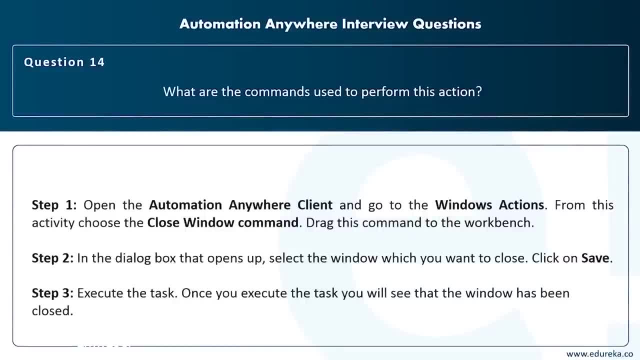 as I've told you previously in the session, we have a windows actions command that has to be used. So under the windows actions command we have various commands, like you know: the closing a window, opening a window or resizing a window. So I'm just going to show you to either, you know, close a window. 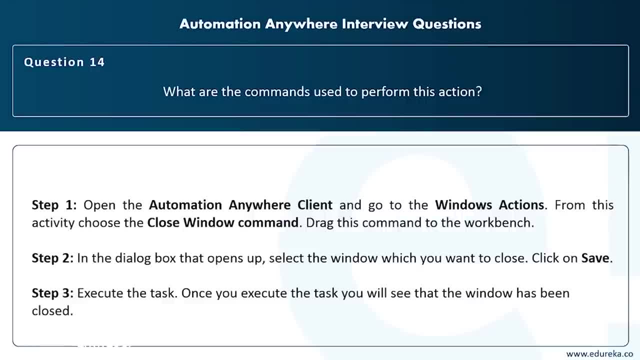 or open a window, because I've already shown you how you can resize a window. So the steps are really simple. You again have to just go to the windows action command, choose the command and then drag and drop it to your workspace. after that You have to choose the window, click on save and then execute. 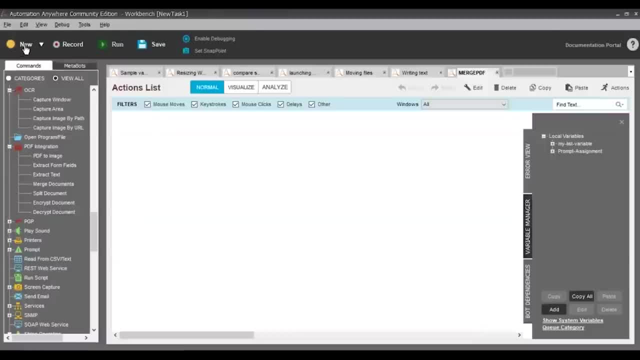 your task right, So let's just do that. So I'm going to go to a new task again, And then what I'm going to do is I'm going to search for windows action. So over here I have various options, right? 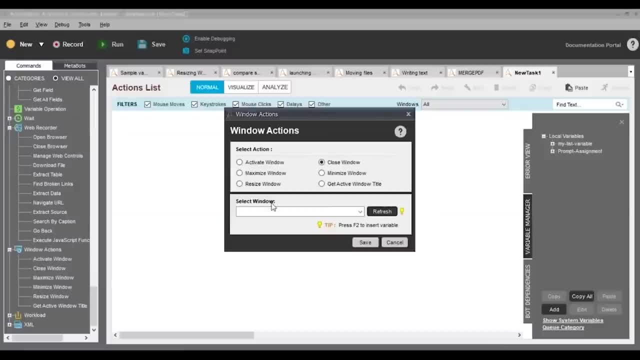 So, for example, let's say I want to close a window, So I'll just choose the option of close a window. I'll select a window. Let's say, you know, I want to close the window of output PDF that we just took. 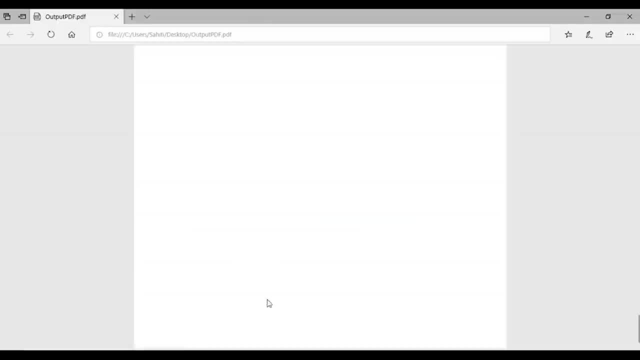 I just want to close this window. So initially you'll see that you know this window is open in my system. If I just want to close this window, I'll just select That particular window, click on save and then save this particular. 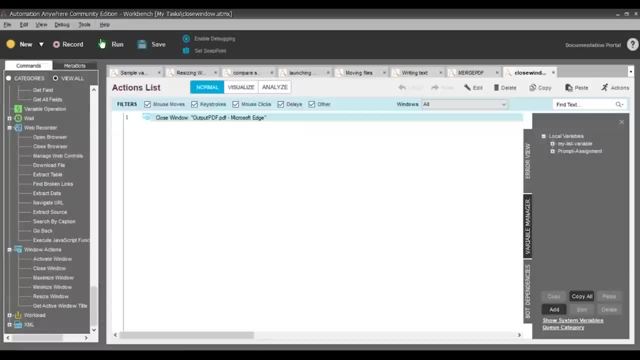 task. Let's say, close window and then execute this task So you can see that you know my window has been closed. So that's how, guys, you can just use this simple window actions to perform different automation tasks related to the windows. 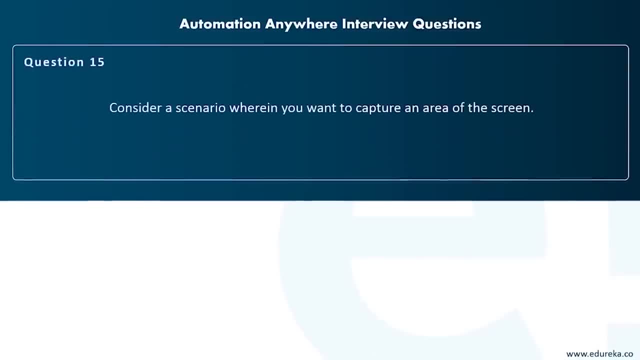 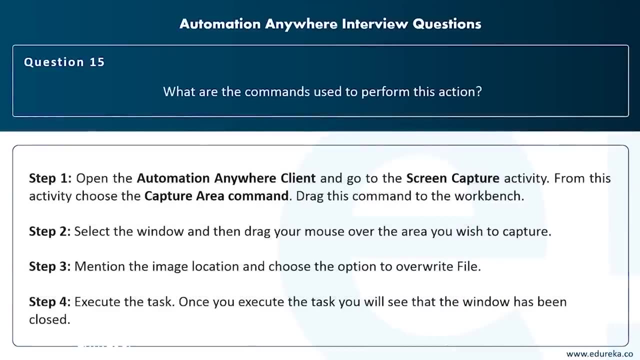 Now, moving on to the final question for the session, that is, consider the scenario wherein you want to capture an area of the screen. Now, what are the commands that you think you need to use to perform this action? Well, the commands Used to perform this action are basically the capture area. 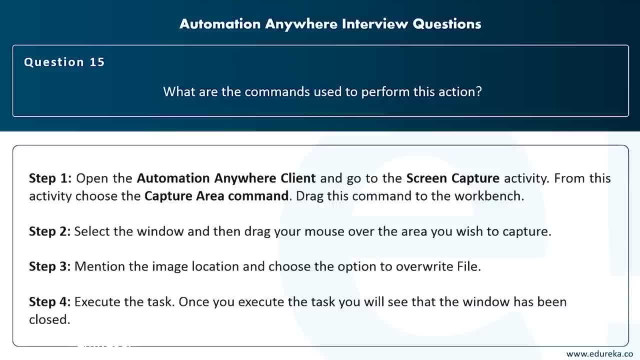 command. So this basically comes under the screen capture activity. What you have to do is you have to select the window, drag your mouse to your area You wish to capture and then mention the image location. So you can just mention an image location and then override the. 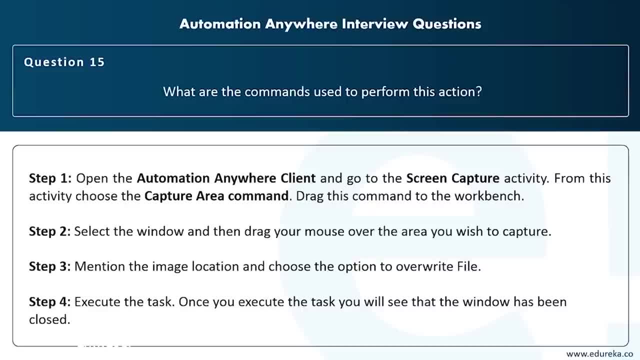 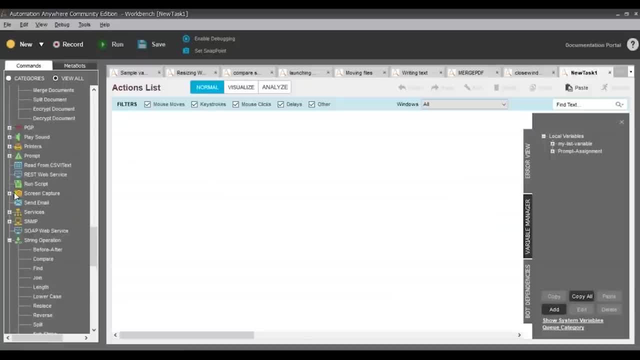 file simply right. So let's just do that. So for that I'll go back to my automation anywhere. client again choose a new task. And now what I'm going to do is I'm going to search for screen capture under the screen capture activity. 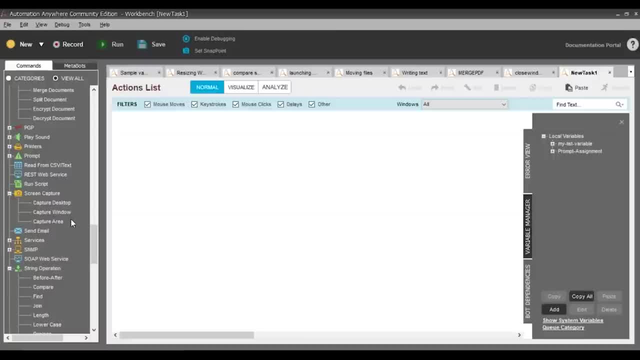 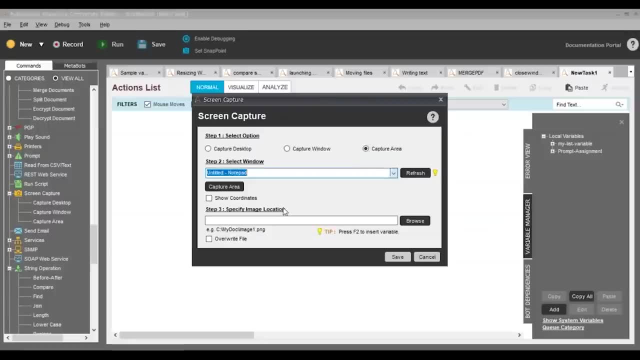 You have options, Like you know: capture desktop, capture window, capture area. So I'm going to choose the option of capture area And then what I'm going to do is I'm going to select a window. Let's say, you know, I want to select notepad, right. 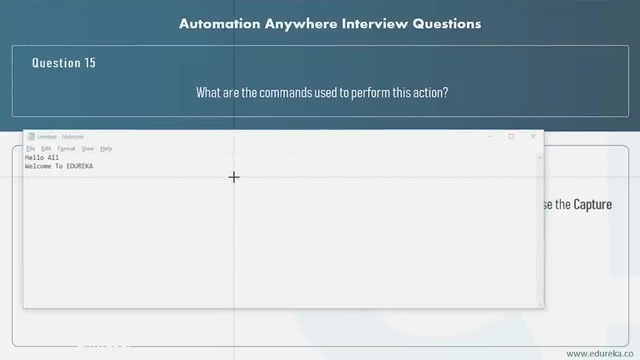 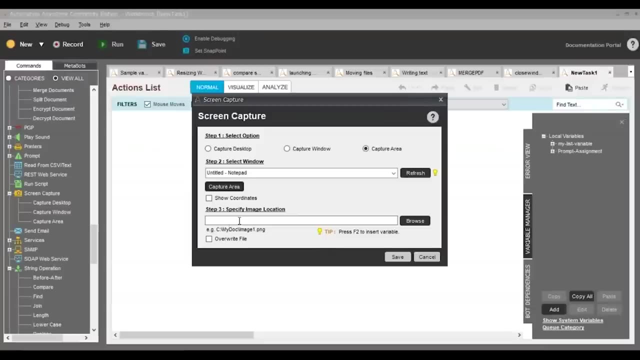 So I'm going to select this notepad and then I'm going to click on capture area. Now let's say, you know, I just want to capture only this amount of area, So I'll just choose that, and then I'll have to mention my image. 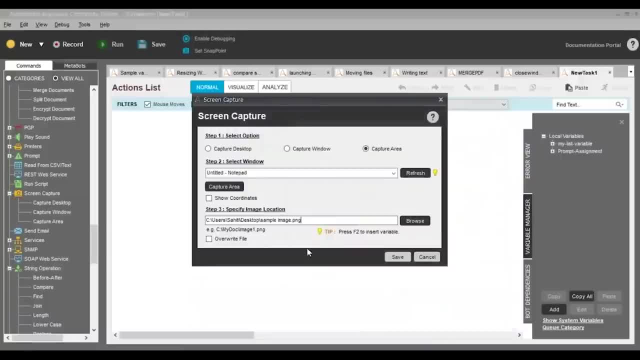 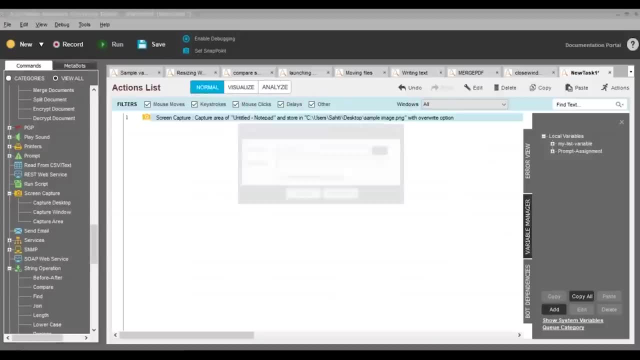 location. So I'll just browse and let's just say I replace the sample image and then I click on overwrite file, right. So that's how you can do. You just have to click on save now save your task again. So let's just put capture image and then execute this task. 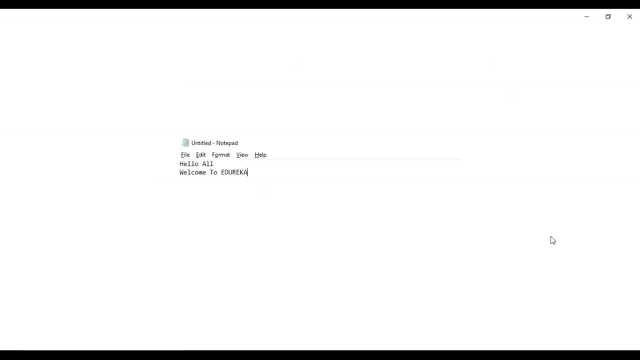 The task has been executed, So let's shift back to our desktop and then choose the sample image. So in the sample image you can clearly see that you know our notepad file has been extracted, basically on the dimensions of what we had mentioned. 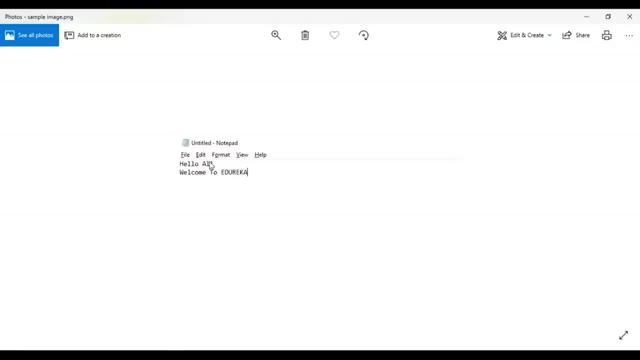 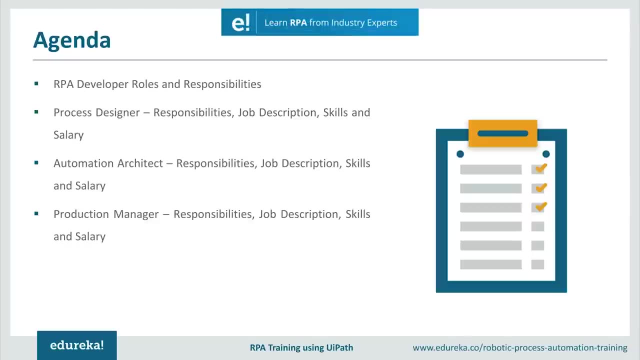 So, guys, that's how you can capture an area in automation anywhere. Well, we'll start today's session by looking into what are the roles and responsibilities for RPA developer and then look into the intricacies of each role. So now let's look into the roles and responsibilities of an RPA. 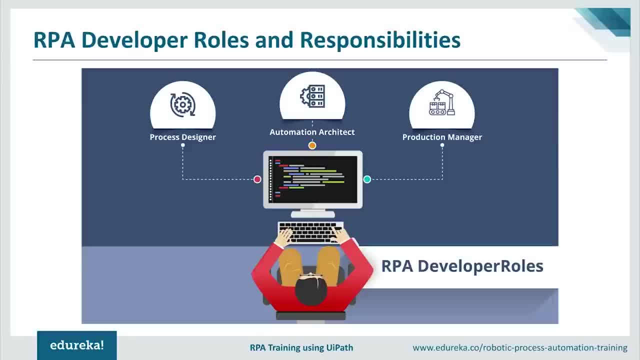 developer. So, when you talk about the roles and responsibilities of an RPA developer, the developer has mainly three roles: the process designer, the automation architect and the production manager, right? So let's move on by looking into the roles and responsibilities of a process designer. 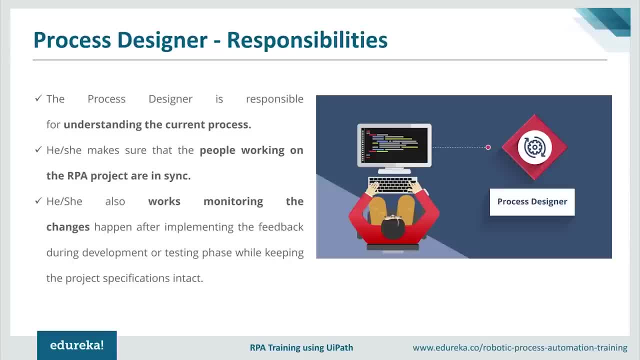 The process designer is usually a business user who understands the existing process, the rules and the vision for the desired process. while this role should be ultimately handled by one person, for accountability purposes, It is important that the process designer works closely with all those who perform the current process in order to accurately 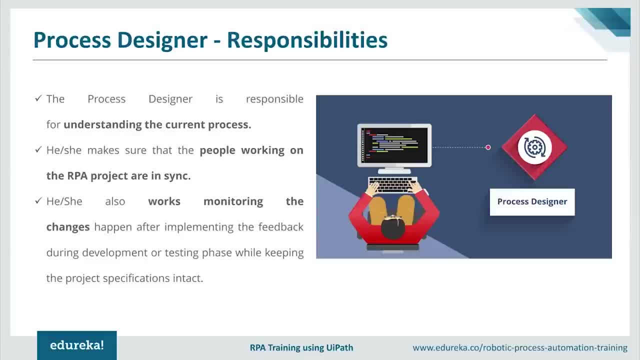 capture the nuances of the process. understanding or incorporating this nuances can make or break the project. ultimately, the process designer needs to learn About and understand this nuances and then either institutionalize or consolidate them. So, basically, the process designer is the keeper of the specification of the RPA project and should be responsible for looping back. 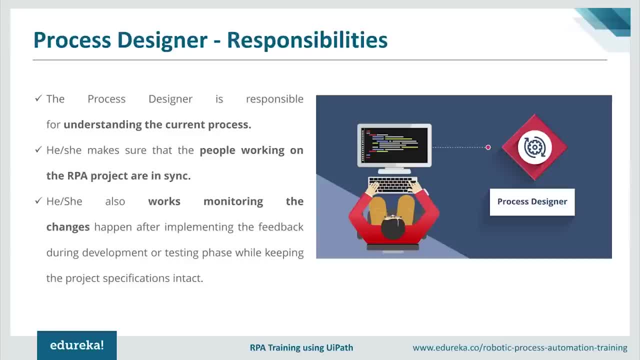 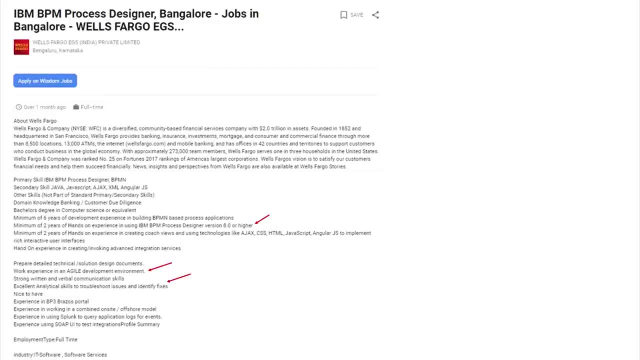 into the specification, feedback and changes made during the development and testing phase. as you can see on the screen, This is a sample job description for a process designer. the skills to become the process designer all stand same for all the companies, but the job description varies from company to company. 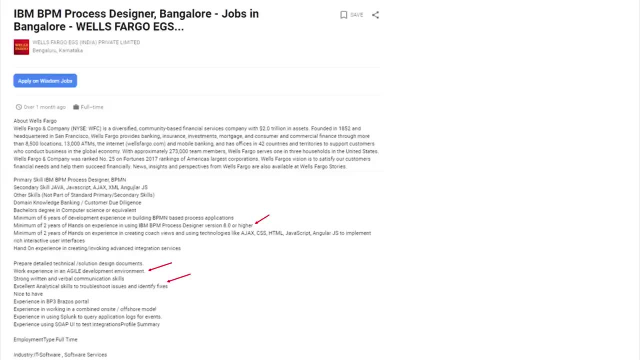 Right, So basically a process designers job description could be like something that he should be able to handle projects in any of the tools such as uipad, blue prism, automation anywhere, etc. that person should have good analytical and problem-solving skills so that he or she can communicate well and handle. 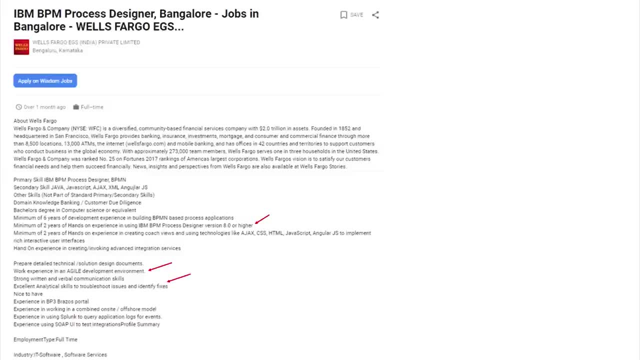 the clients in such a way that the company scales forward. Also, he should have good knowledge of programming languages such as dotnet, Java, and also the knowledge of product architecture, implementation and infrastructure requirements. So this was a sample job description of a process designer. 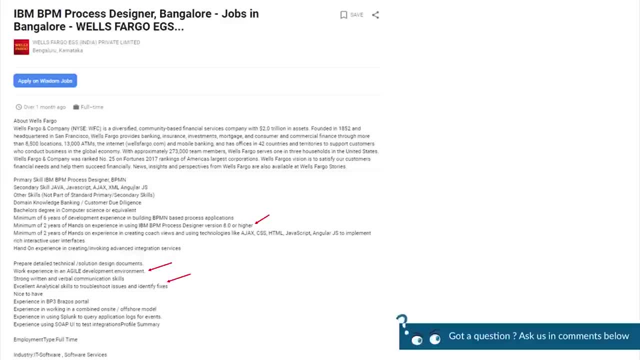 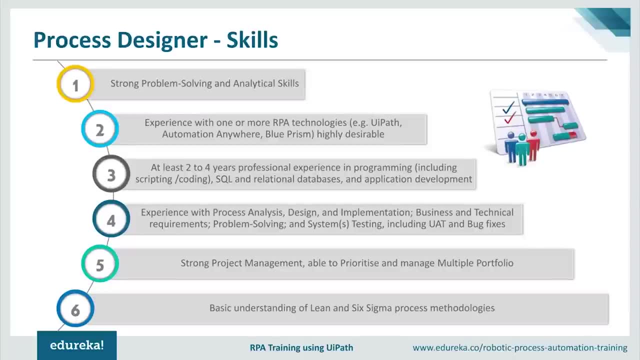 Now, if you want to become a process designer, then you need to have some skills. So what are those skills? So let me just show you those skills. Well, to become a process designer, you should have strong problem-solving and analytical skills. 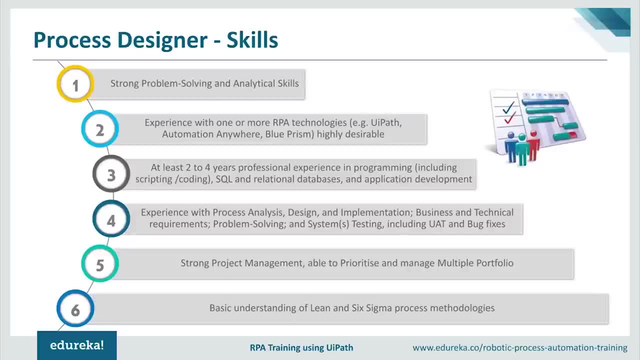 You should have experience with one or more RPA technologies like uipad, automation anywhere, blue prism, Etc. as these three tools at the top trending tools in the market right now. you should have an average of two years of professional experience in programming languages and also SQL and relational databases. 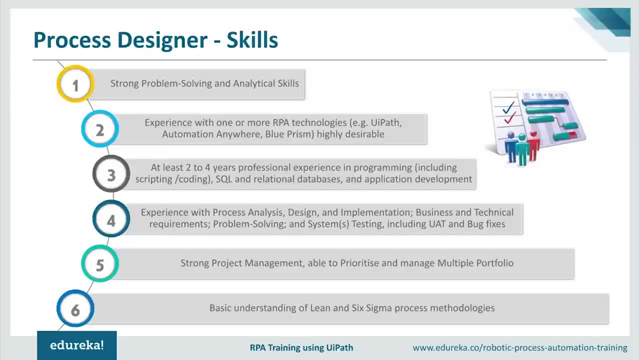 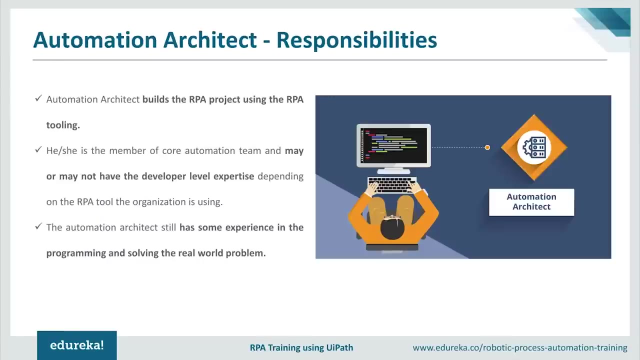 You should have good expertise with process analysis, design and implementation. strong project management skills will also put you one step forward, away from the crowd, right. So these are some basic skills that a process designer requires. now, moving on to a next role, That is, the automation architect. 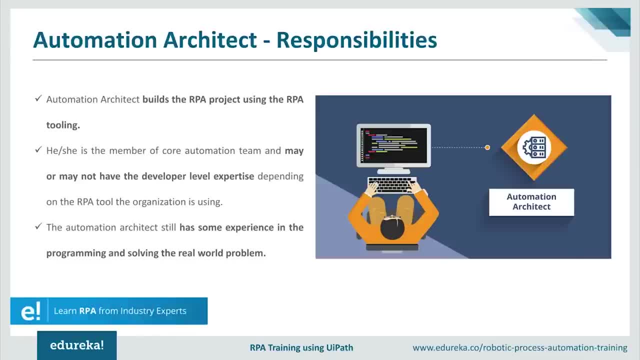 The automation architect is the person who actually builds the automation using the RPA tooling. depending upon the tool, This role may or may not require developer level expertise, while many RPA vendors vouch to the fact that their automation Studios do not require programming expertise. 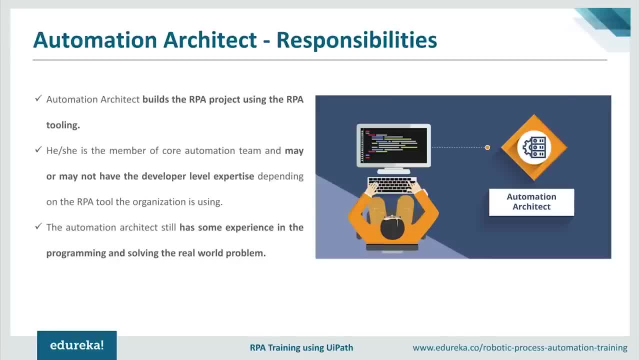 I would say to not believe it, as if you're looking to automate a process that involves rules and logic, which most of the worthwhile automations do, then it definitely requires programming. So whether one is writing syntax or configuring loops and branching it in a case tool, its programming. 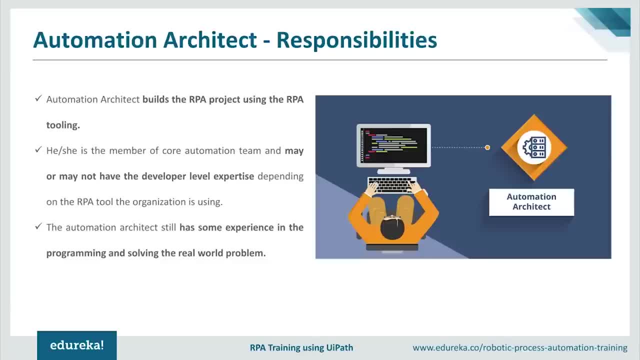 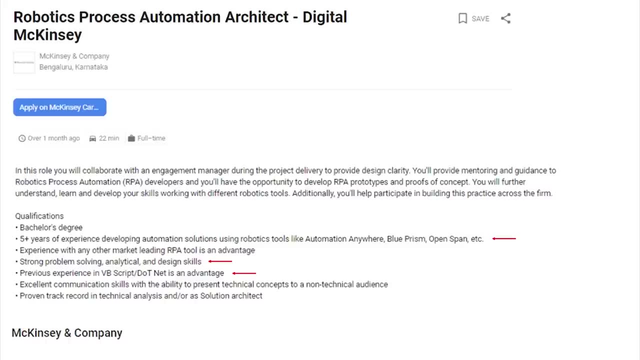 and the automation architect should have some experience for it, right? So let's look at a sample job description of a company for an automation architect. So, as you can see in the screen, this is a sample job description for an automation architect. The qualifications required are basically a bachelor degree. 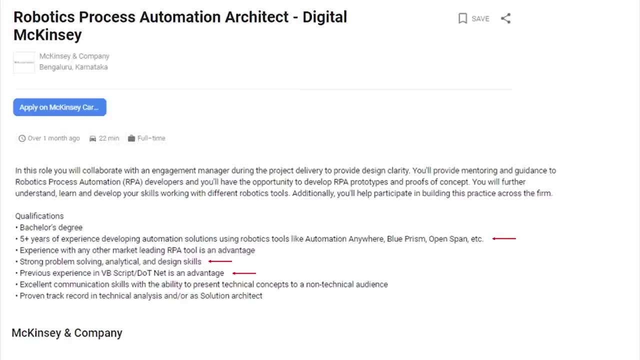 a few years of experience developing automation solutions using robotic tools, like automation anywhere, blue prism, openspan, Etc. experience with any other market leading tools is also an advantage and will also put you out of the crowd right. So if you have good expertise with Ui part tool, 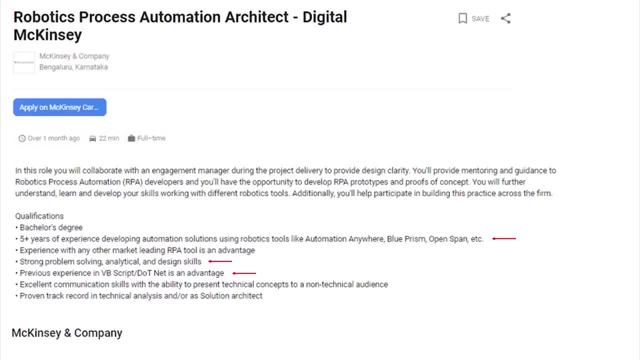 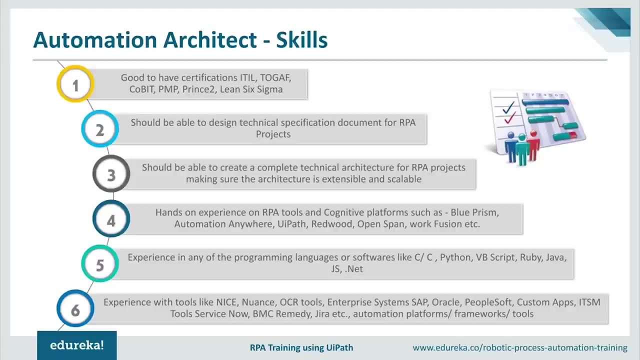 and also have good expertise in blue prism, then that will obviously make you stand out. strong problem solving analytical skills, design skills, experience with coding, languages and communication skills will put you into a whole package of acquiring this job of automation architect right Now. what are the skills that you require? 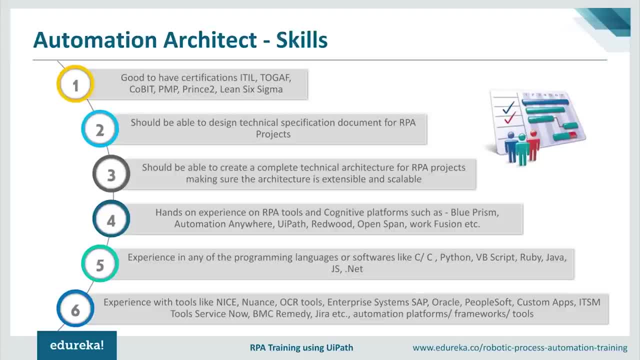 to become an automation architect. Well, the skills required to become an automation architect is that you should be able to design technical specification documents for RPA project. You should be able to create a complete technical architecture for RPA project, making sure that the architecture is extensible and scalable. 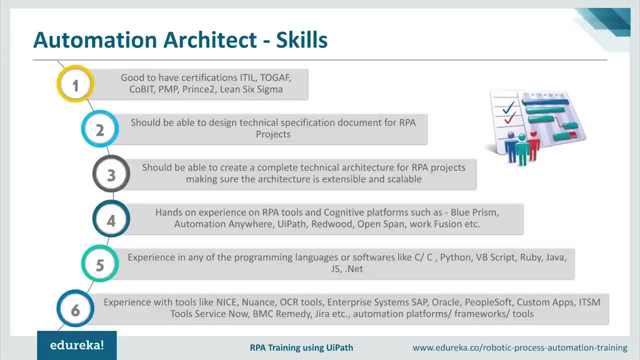 You should have good hands-on experience on RPA tools and cognitive platforms like blue prism, automation. Anyway, Ui, path, Redwood, openspan, work, fusion, Etc. Also, experience in any of the programming languages like C, C++, Python, VB, script, Ruby, Etc will also help you, not only. 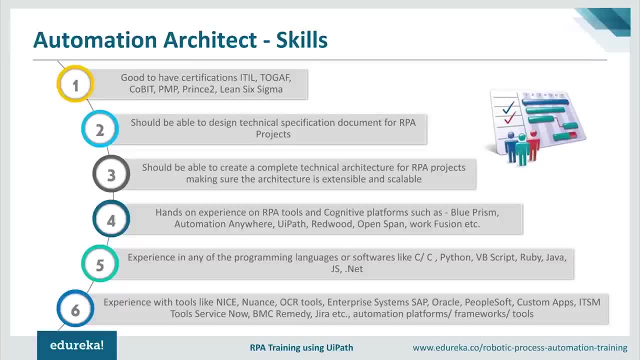 need these skills, but it is always good to have certifications like togap, sobit, PMP, Prince, to lean Six Sigma, so that it will teach you how to handle different projects and also will give you a good high pay. now coming to the last role of an RPA developer. 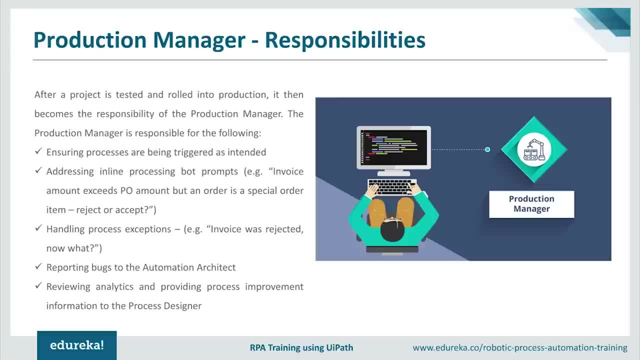 The last role is production manager. So when you talk about a production manager, after a project is tested and rolled into production, it becomes the responsibility of the production manager. So the other two roles, that is, the process designer and the automation architect, come before to that of the role of a production manager. 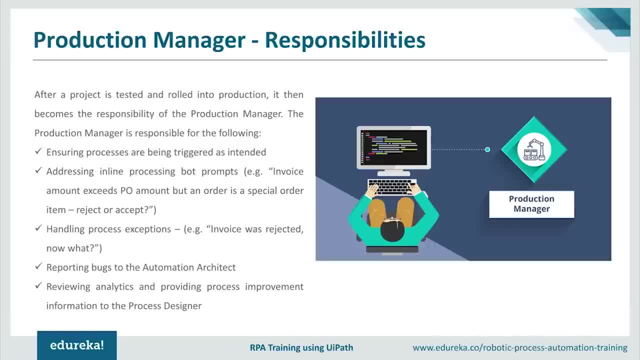 The production manager is responsible to ensure that the processes are being triggered. he or she addresses the inline processing board prompts. a production manager is also responsible for handling process exceptions, reporting bugs to the automation architect and also reviewing analytics and providing process improvement information to the process designer. 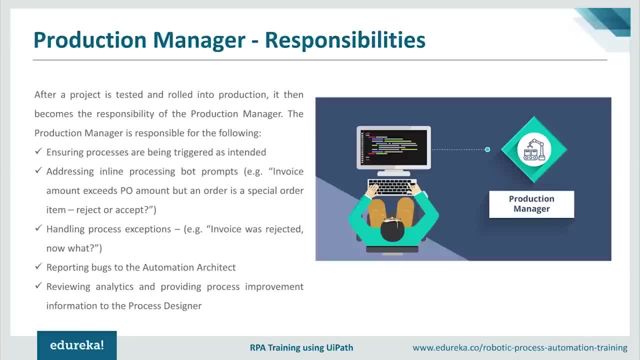 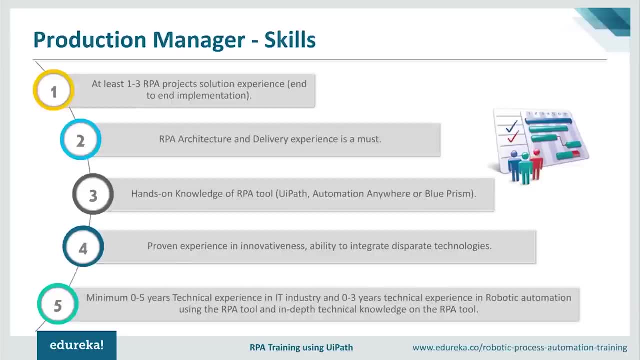 So, as it's very much clear, to become a production manager, You have to understand the roles of process designer and automation architect. So the skills required to become a production manager are somewhat like this: he or she should have at least one to three years of project solution experience. 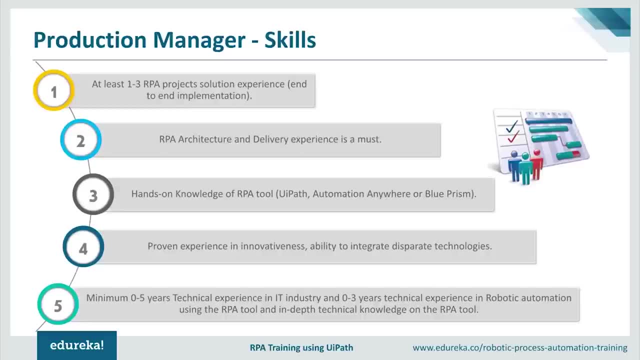 The production manager should be able to understand the RPA architecture. He or she should have the hands-on knowledge of RPA tools such as uipath, automation anywhere or blue prism. He should prove experience in innovativeness and ability to integrate this great technology. 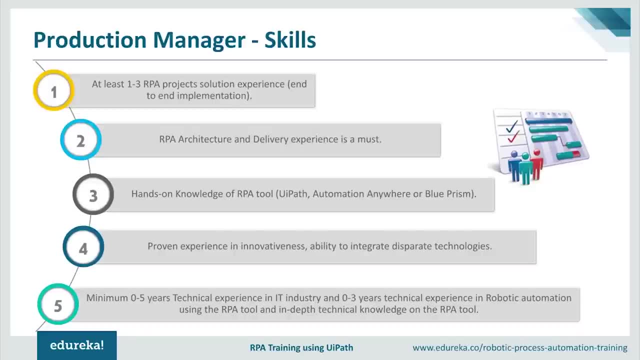 And obviously, if you talk in terms of experience, he or she requires minimum of 0 to 5 years of technical experience in the IT industry and 0 to 3 years of technical experience in robotic process automation using the RPA tool. and then last, I could just say: 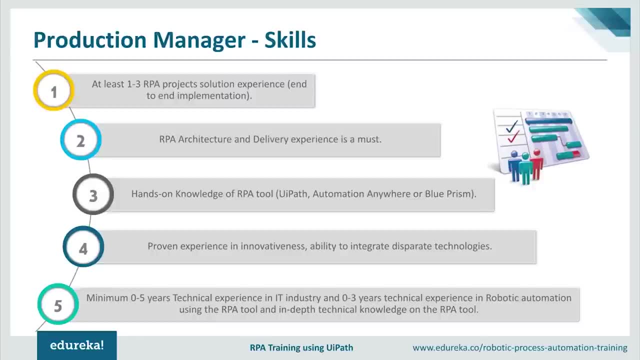 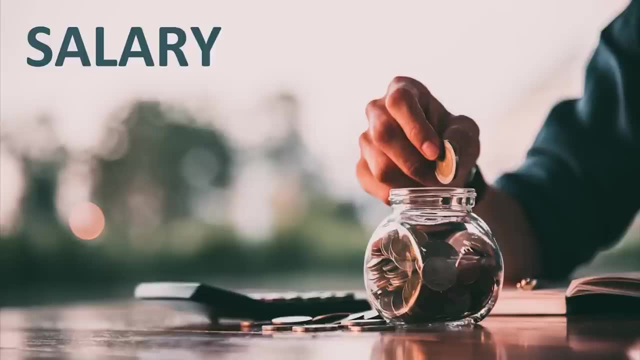 that the production manager requires in-depth technical knowledge of the RPA tools. So, guys, these with the roles and responsibilities of an RPA developer. So let me show you some salary Trends in the market right now. So, for the role of process designer, 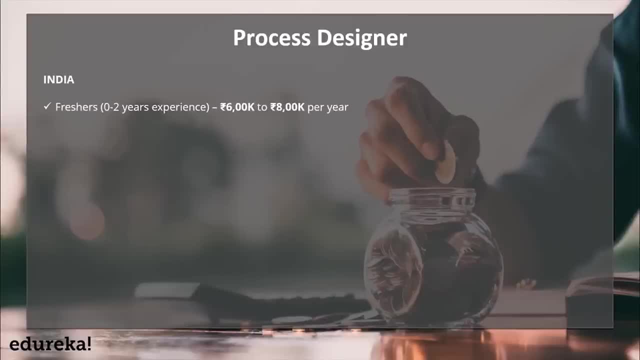 if you talk in terms of countries, then in India, for a fresher with 0 to 2 years of experience, that person would earn around 6 to 8 lakhs per year, and for a senior role with 2 to 6 years of experience. 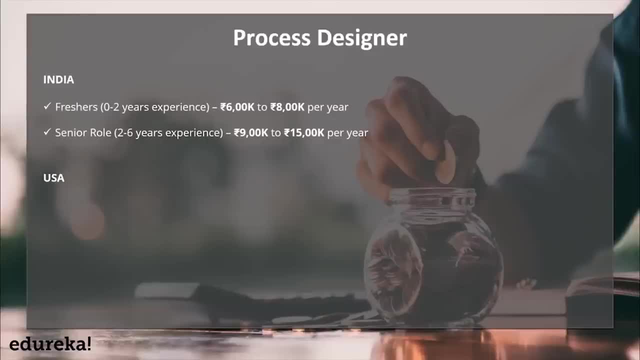 he would earn around 9 to 15 lakhs per year, And then, if you compare it to us, the average salary ranges for around eighty-four thousand dollars to 132 thousand dollars per year for a process designer. Similarly, if you consider it, for a automation architect. 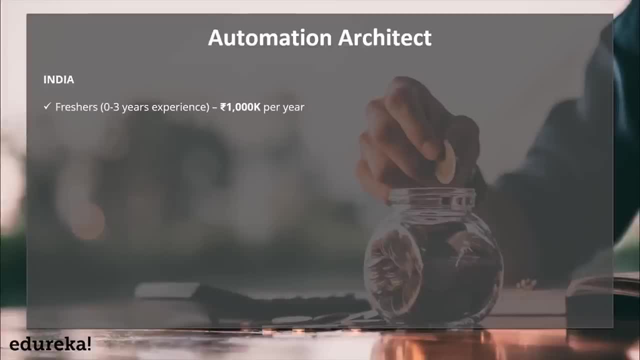 in a freshers role in India with 0 to 3 years of experience, that person would earn around 10 lakhs per year, and for a senior role with 3 to 9 years of experience, then that person would earn around 20 lakhs per year. comparing, 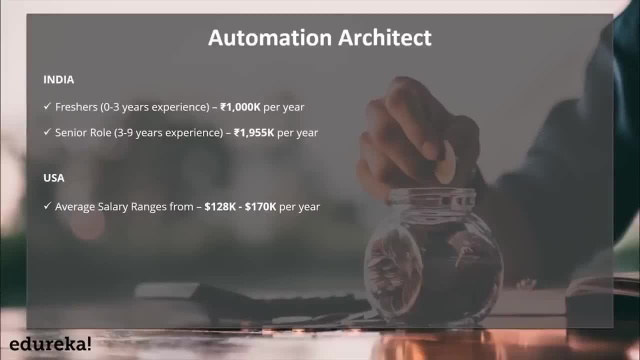 it with the salary Trend in United States. The average salary ranges from around 128 thousand dollars to 170 thousand dollars per year. And finally, as I told you, the production manager is the one who passes the stages of being a process designer and automation architect. 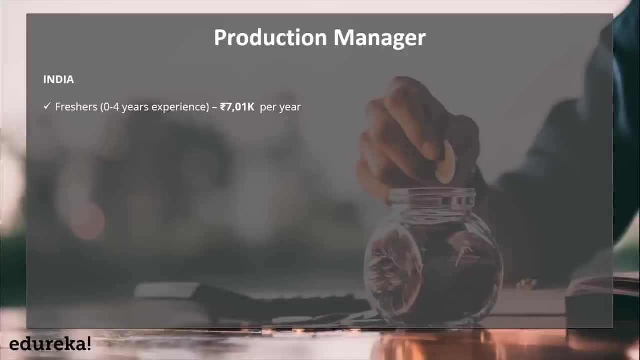 So for a freshers with 0 to 4 years of experience, that person would earn around 7 lakhs per year. when I'm talking about a fresher, then I mean that the person understands RPA technology in depth and has hands-on experience with RPA tooling coming. 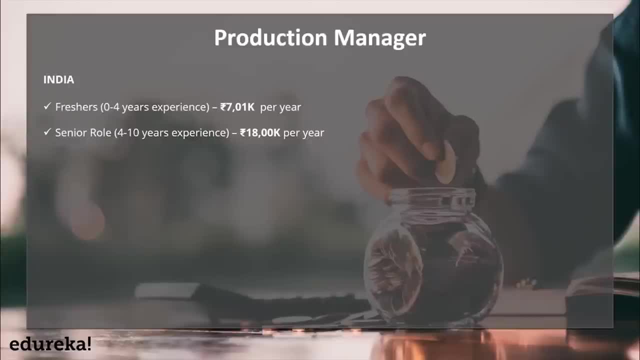 to the senior role in India with 4 to 10 years of experience, Then that person would earn around 18 lakhs per year right. Similarly, comparing it with US average salary Trend, that person would earn around 68 thousand dollars to 125 thousand dollars. 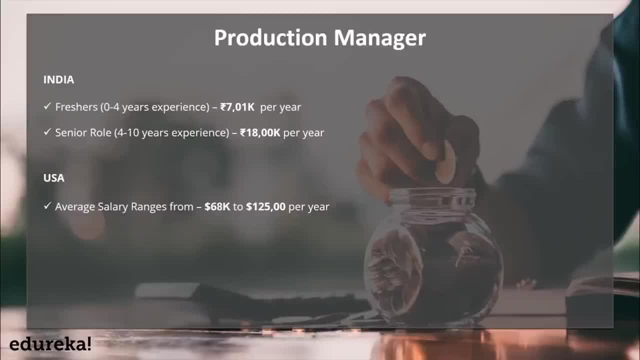 Per year, isn't it a huge amount? So, as you can see that the trend for RPA is increasing day by day, and then there is no end to this technology. So, now that you've seen what are the roles and responsibilities and the salary Trends for an RPA developer, 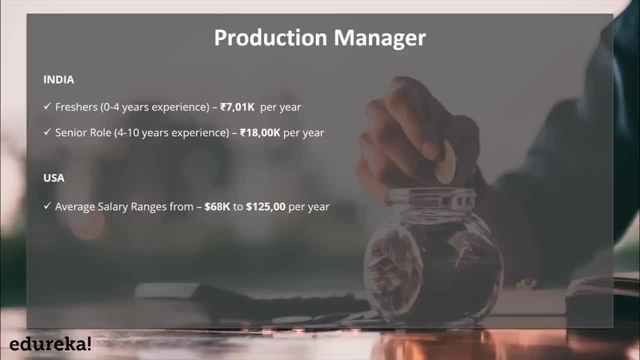 with three different roles. It's a clear fact that if you have to become a production manager, then you have to go through the stages of becoming a process designer and automation architect. So we at Edureka offer RPA training using UiPath, which will enable you. 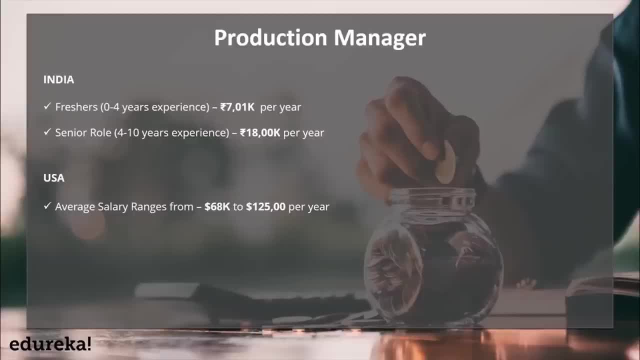 to take up the roles of process designer and automation architect. Once you gain expertise with the tool in UiPath and you have a lot of experience with RPA technology, then that will give you a push to become a production manager in the RPA world.